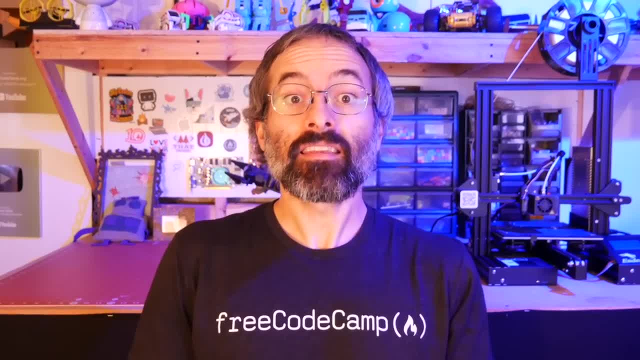 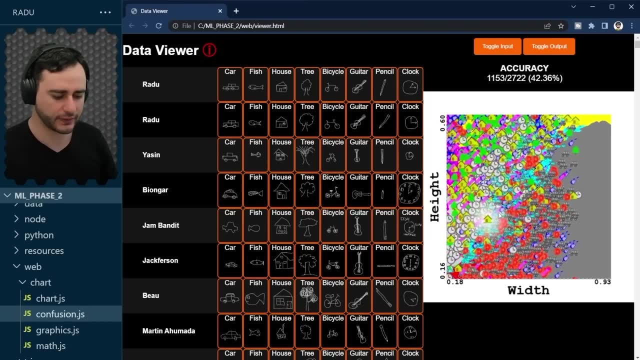 released his No Black Box Phase 1 course. This is Phase 2, but you can still follow along even if you didn't see Phase 1.. In this course, you will learn how to implement classification methods such as neural networks to recognize drawings. You'll also learn about data cleaning. 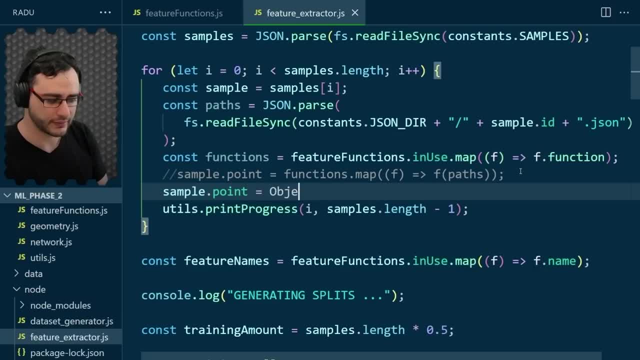 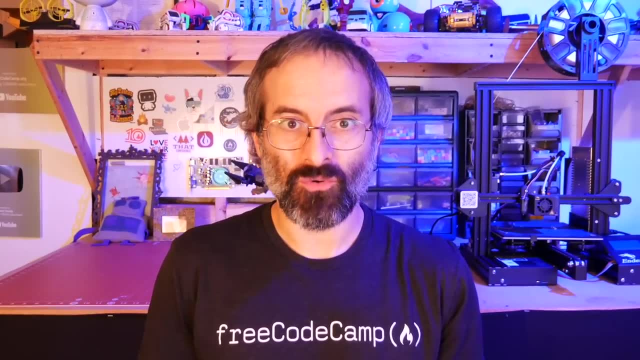 confusion, matrices, geometry and the difference between vector and raster data. If you want to learn how common machine learning algorithms work under the hood, this is the course for you. Hi, and welcome to Phase 2 of the No Black Box machine learning course in JavaScript. 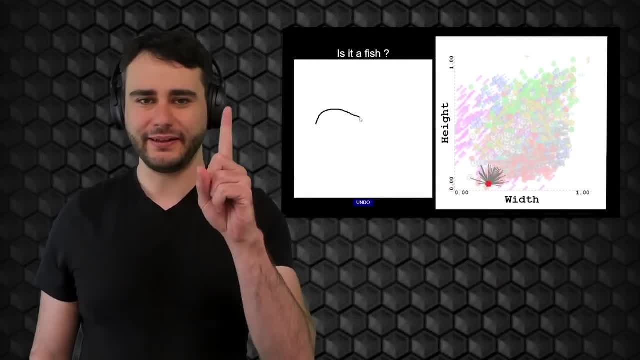 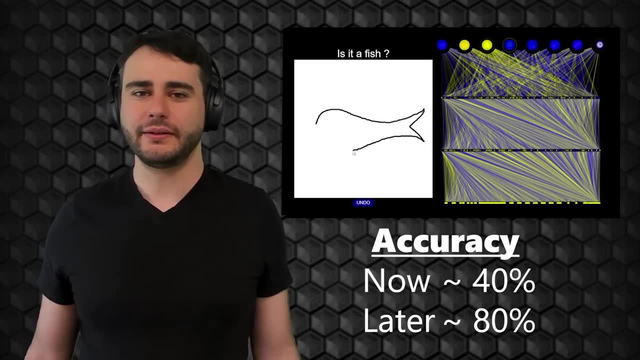 The goal here is to take the drawing recognizer we built in Phase 1 and improve its accuracy by implementing more advanced methods. Now, if you didn't complete Phase 1, you may be okay starting directly with this, especially if you already know some basic machine learning concepts. I will explain our code base briefly. 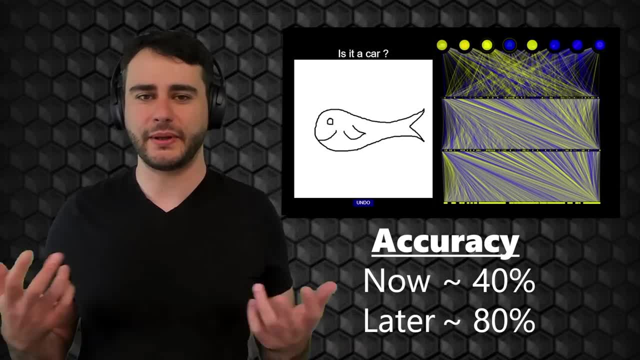 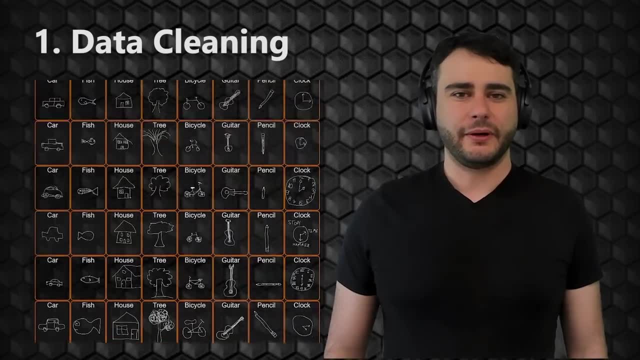 in the beginning. so try to understand, ask questions below or on Discord, and if all else fails, then go to Phase 1.. This time we'll learn about data cleaning. It's a tedious process, but I'll teach you how to build a tool to make the job easier. Then we'll learn. 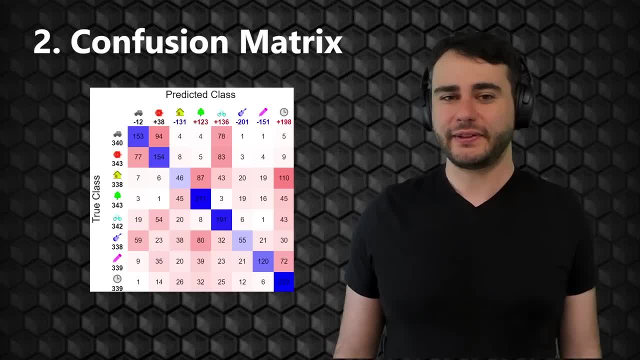 to visualize the data, and then we'll learn how to build a tool to make the job easier. This is a confusion matrix, a special kind of table that helps us understand our model even better than the chart we built last time. It will be especially helpful when working. 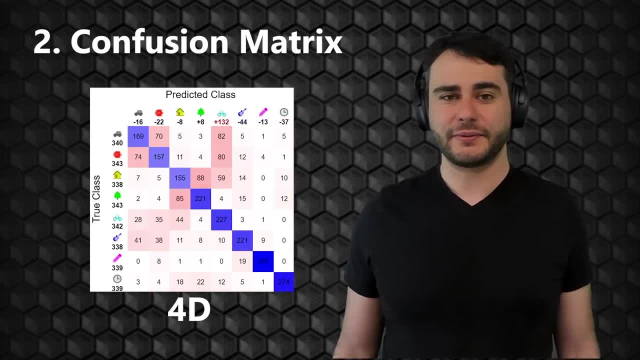 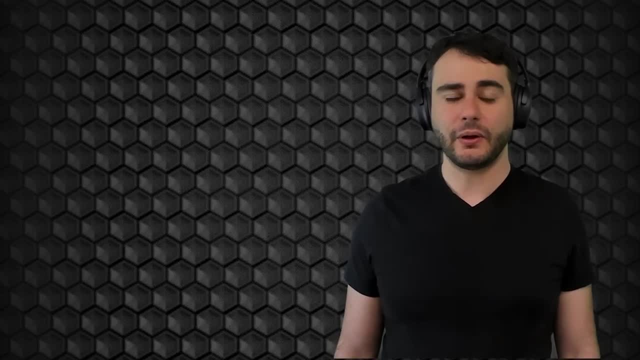 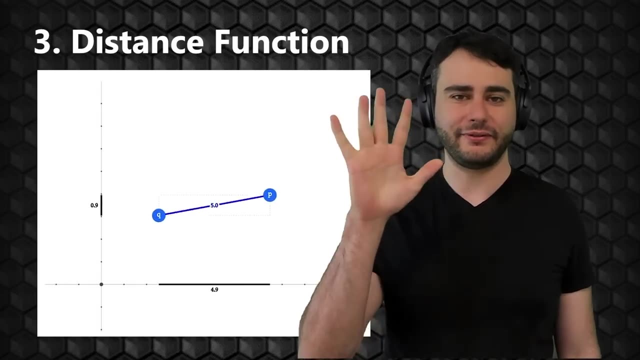 with more than two dimensions, Speaking of which, so far we've only been using two features. but the k-nearest-neighbor algorithm is not limited to that. All it needs is the way to calculate the distance between data points, and I'll teach you how to do that in 3D, 4D. 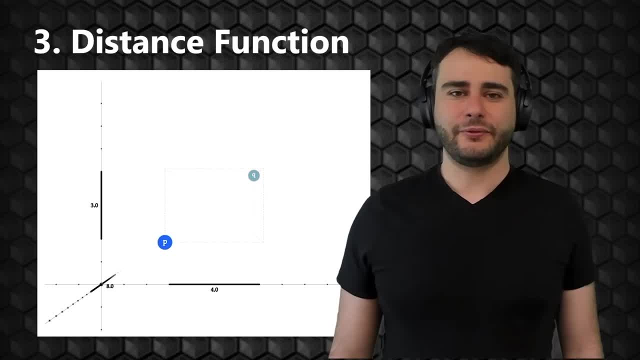 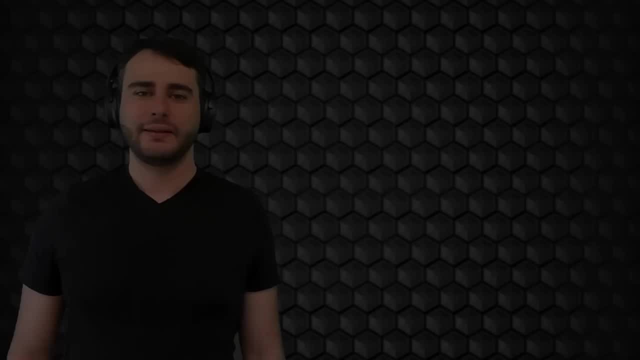 5D- any D, really. I'll show you how to do it, and then I'll show you how to do it in 3D. I'll show you an intuitive way to think about multidimensional spaces and distances, and we'll use up to 400 dimensions. in this course, We also study another classifier, the neural. 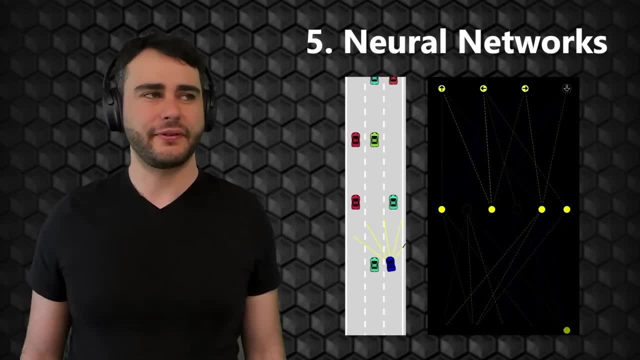 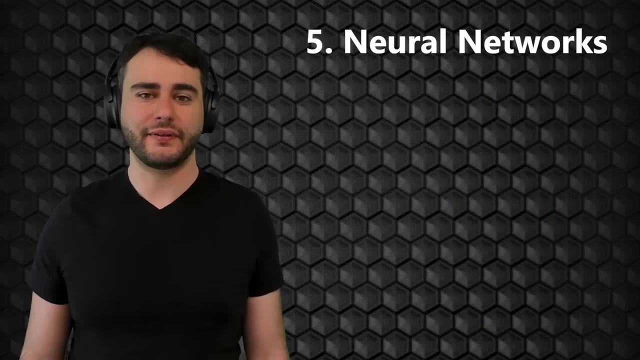 network. We'll use the same code from my self-driving car course because I want you to understand that machine learning methods are general techniques and algorithms we just apply to solve different kinds of problems. Now this is more complex than that self-driving scenario. 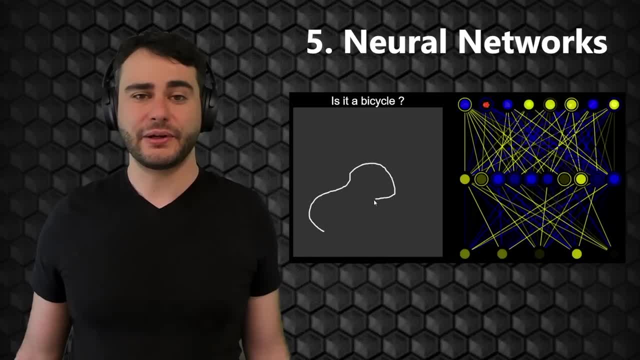 and our optimization strategy there wasn't really good. So I should teach you something better, like backpropagation, but I don't know how I tried to come up with a lesson. I just can't seem to add anything to those out there. So I'll teach you how to train. 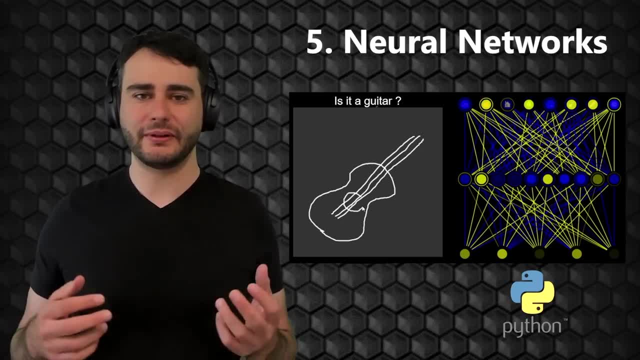 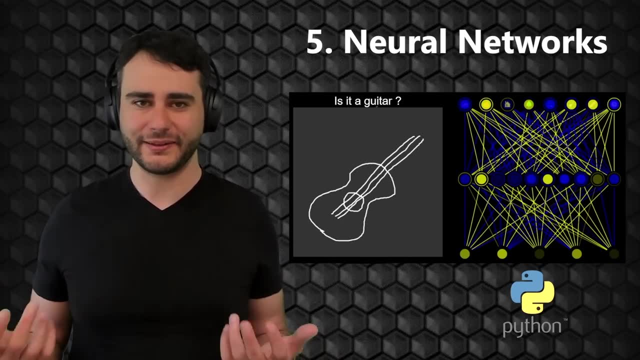 the network in Python and then take the resulting model and just use it in JavaScript. So Python will do the heavy lifting and our JavaScript app just benefits from it. Am I cheating? Maybe a bit, But I think that learning this is possible is a really important lesson here. 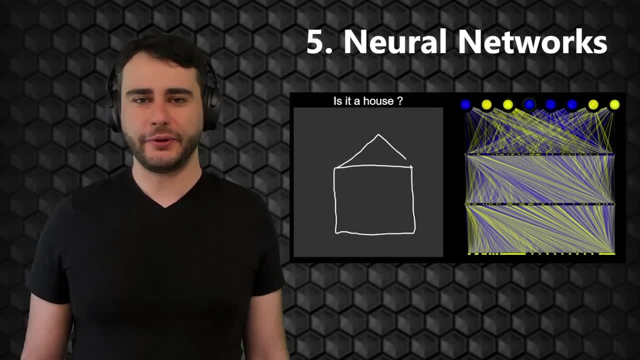 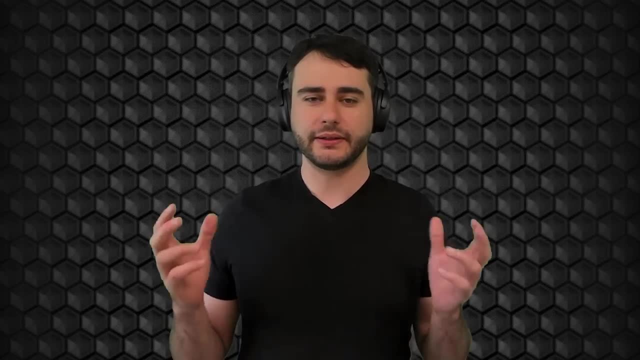 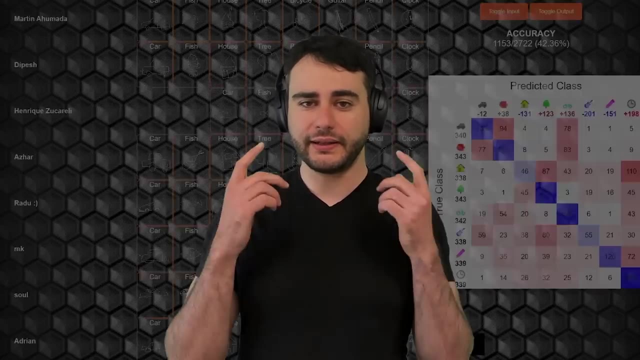 You'll see. Finally, I'll demonstrate deep neural networks as well, so I don't get many comments about it Now. I need to stress: This course is supposed to be a learning experience. I want you to understand how machine learning works and why we do the things we do. We use the data. 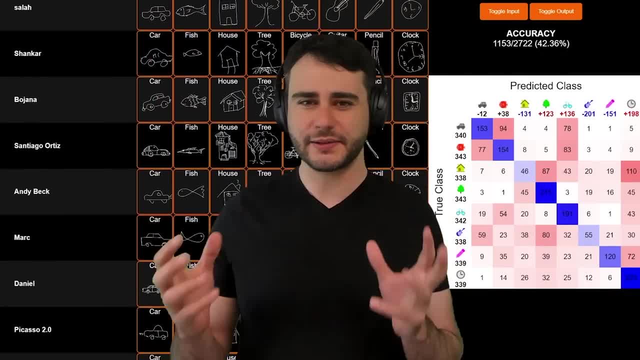 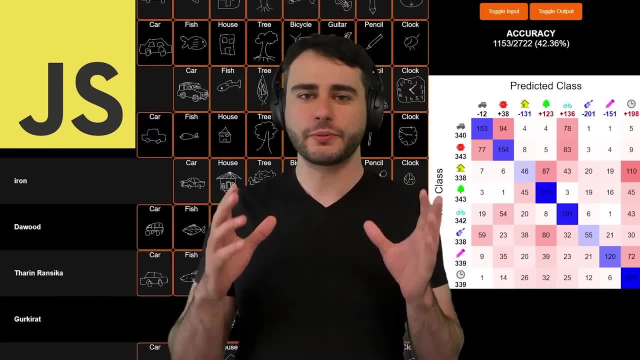 you helped me collect. so we have a real challenge, not some textbook dataset. and we use JavaScript because it's a high-level language where we don't need to worry about the small things, and because we can use it to build nice user interfaces that we can share without the need. 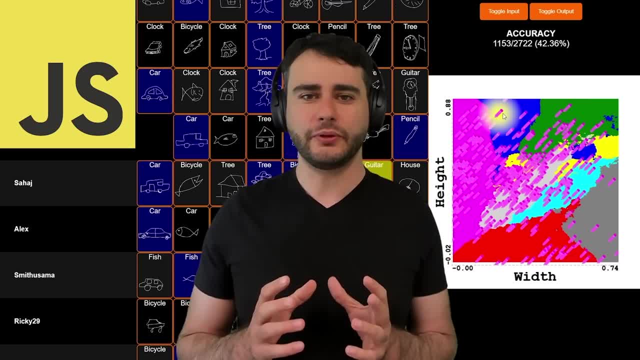 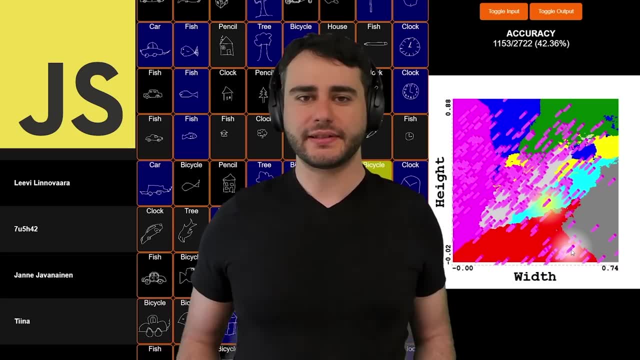 to download, install and so on. I really hope you learn to build real things, not just something that reads from files and writes into the console. Another reason I use JavaScript is because it's not well-known for machine learning, But many people do know JavaScript. 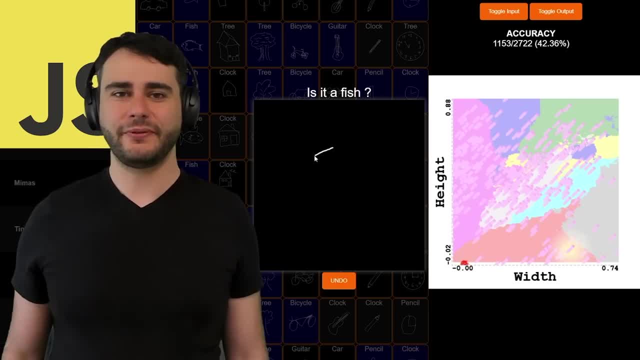 and want to learn machine learning. So if this is you, you've found the perfect course. And if you don't like JavaScript, don't worry, I'll teach you how to do it. So if you don't like JavaScript, take it as a challenge and implement the same things in something. 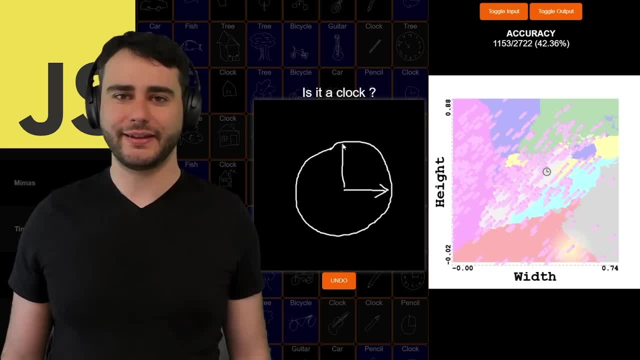 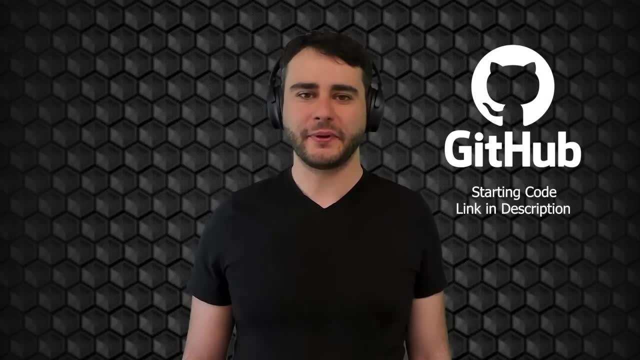 you like. We don't use libraries, so it's really doable, I think Sound good. Okay, then, if you plan to follow along, take the starting code from GitHub. It's similar to the last one from phase one, but a little bit different. I've added your. 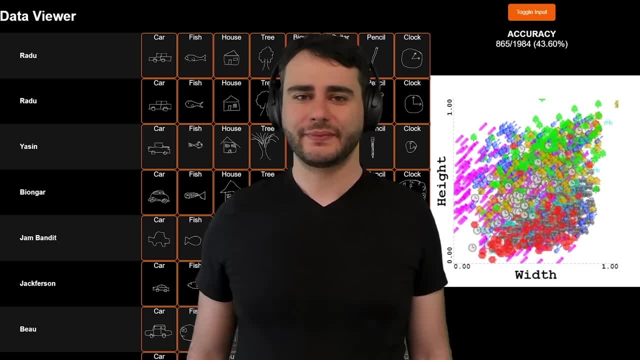 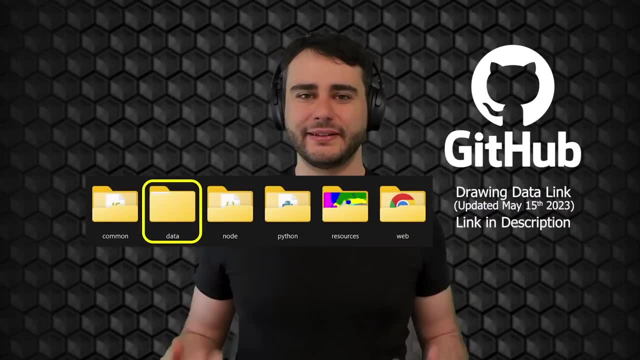 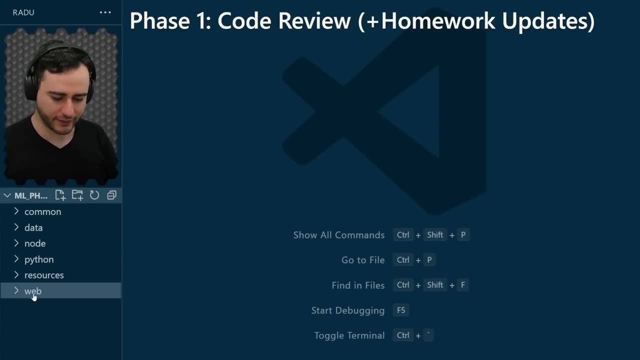 homework submissions and made a few other optimizations as well. Also, remember to get the data from this link. Place it next to the code like this and… you're ready to start. The first thing we'll check out is the drawing app we use to create new data Here inside. 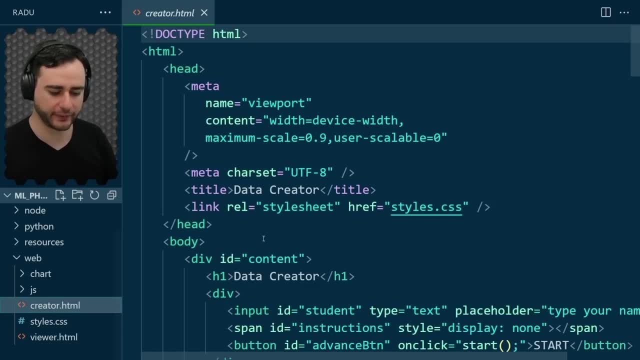 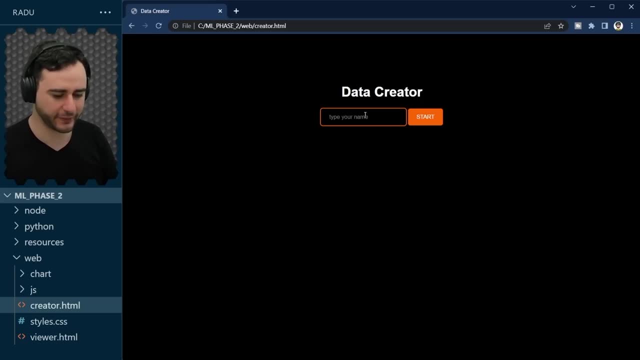 the web folder and create our HTML. If you open this in the web browser, you'll see it looks quite different from before, but the functionality is still the same. It's gonna ask you to enter a name here and then to draw several things, But the style is different. 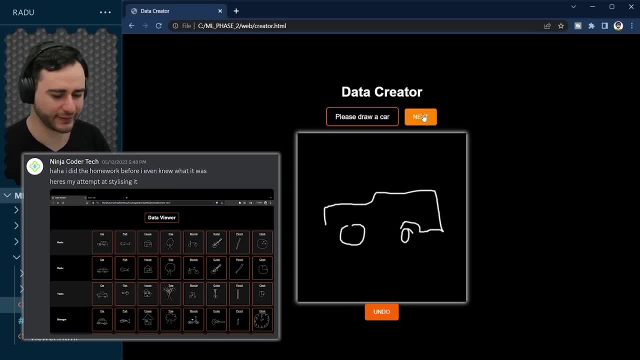 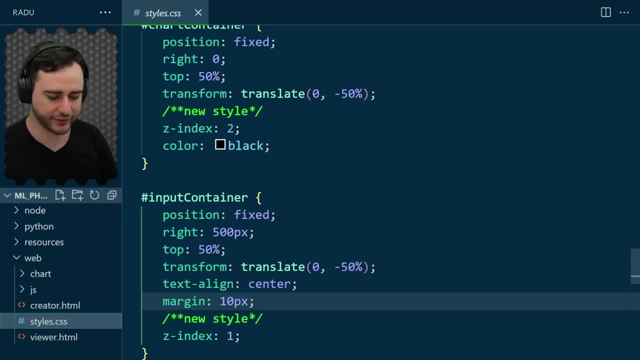 because… I'm not sure if you can see it, but the style is the same as the one I used in Homework 2, and I adopted his style. You can see these changes here in stylescss and everything I've marked as new style. 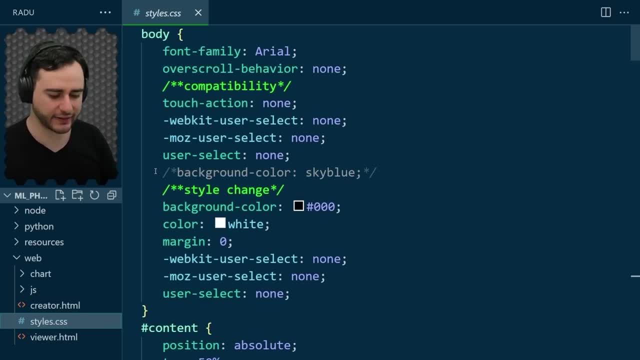 starting from beginning are things that he has added and I commented out previous styles I've used. In case you're curious how to do different styling, I kept both here for reference. Now you'll also notice this compatibility section here at the top, And that's because 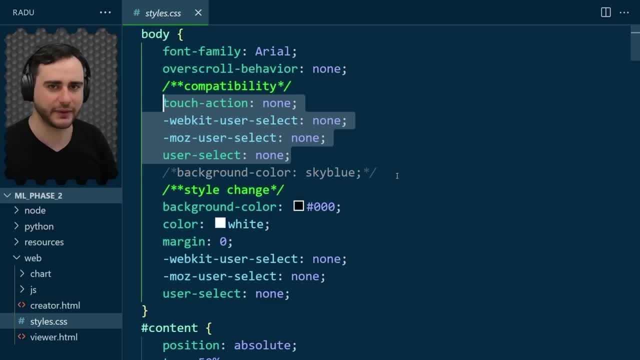 in Homework 1… I've also added a button to the default style that you can use to create some interactions with the app. But here in Homework 2, I've also added a button to the default style to create some interactions with the app. And here you'll notice that in Homework 1… You'll notice that the volume of the app is also the same. I'll set it to 0, and then I ask you to test the app and let me know how it went. 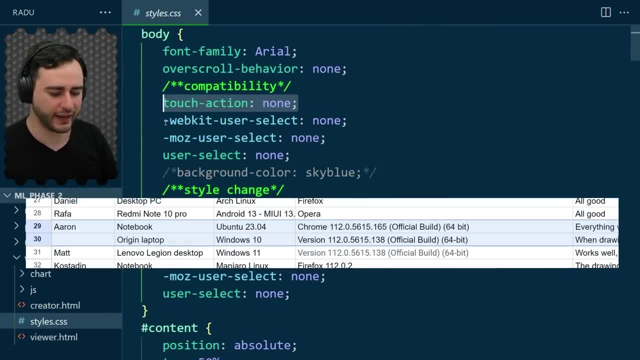 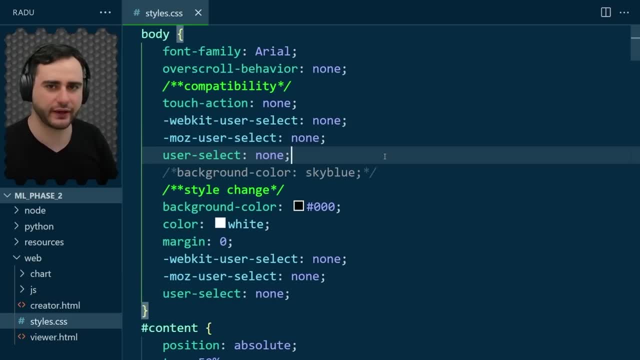 I know there were some problems on iPhones making the screen scroll when you want to draw. I got a suggestion from Meso to set Touch Action to None. Aaron commented that these should be set to None as well for it to work. I'm really not sure if these are enough because I don't have an iPhone to test, but I also 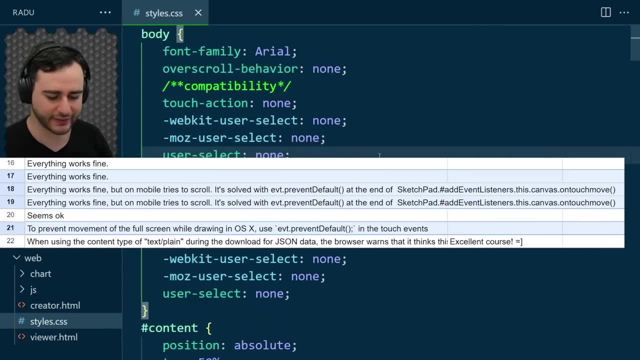 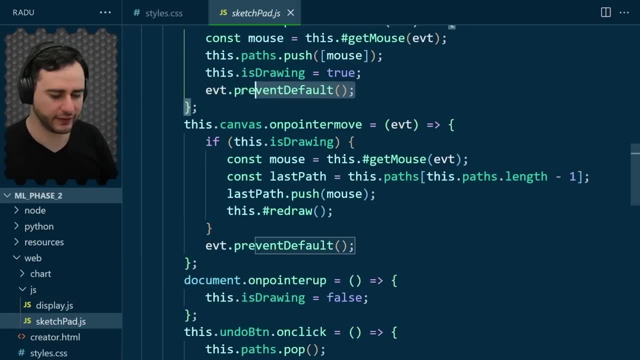 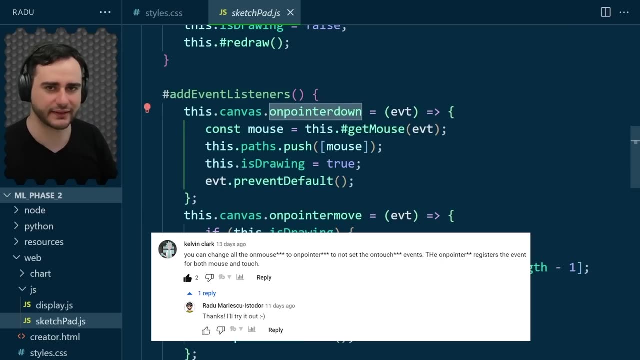 got feedback from MJake and Rick And they said that I should go here in the sketchpad component and add prevent default to the pointer events, which, by the way, kelvin said i use instead of the mouse events and touch events separately. i really don't know if these comments help, because, 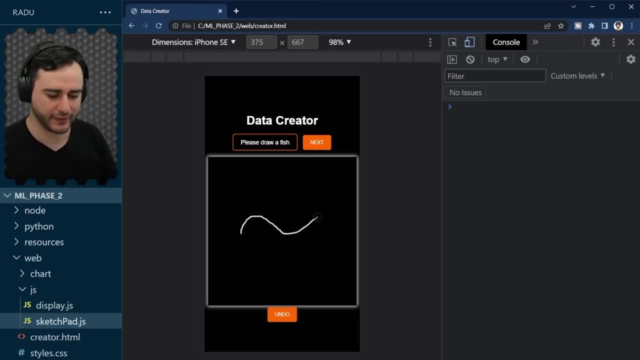 when i test on mobile it works just fine, but please let me know if it works for you. i've added these changes on the version of the app on my website that i still use to collect data if you want to submit, and also in the recognizer that will build by the end of this course. 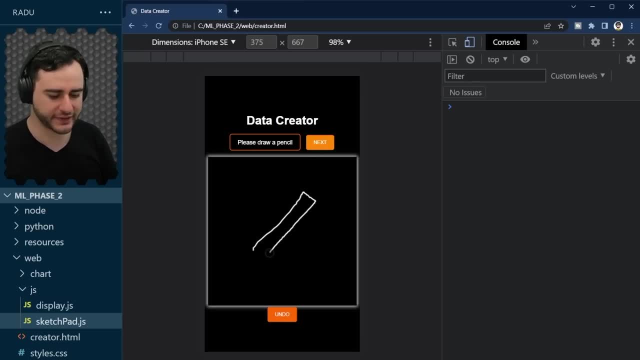 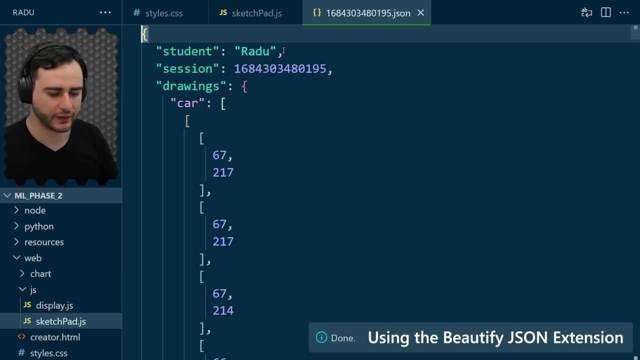 now, after you're done with the drawing and press next, you're gonna get the option to save this and it's gonna create this file that contains all the information about the drawings you just made. it's a JSON file that, if i'm gonna format like so, contains the information about the student. 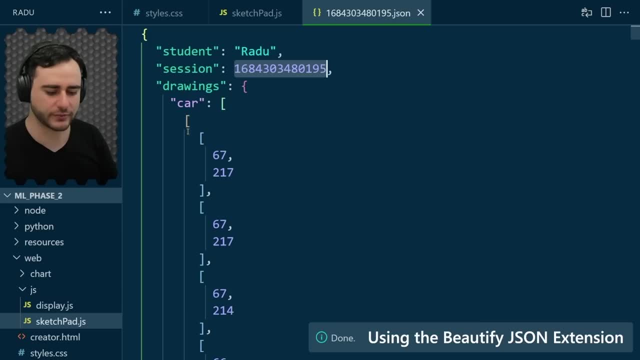 some unique identifier, and then the different drawings. the eight different drawings are going to be displayed on the screen and then, once the user has registered one of them, it's going to say that the interesting component here is that the software doesn't provide any, each of which are made of a collection of paths containing points. 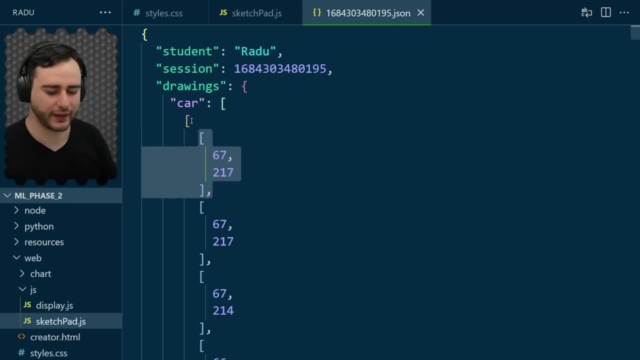 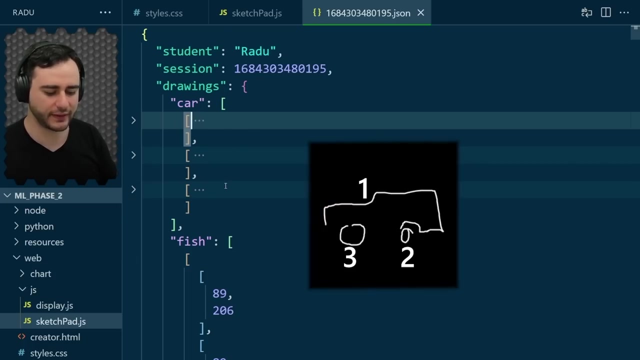 So this is the x- y coordinate of the points, And this here is one path that is used to draw the car, and this is another path of the car and another path of the car. So the car I drew had three different paths, and then the fish and so on. 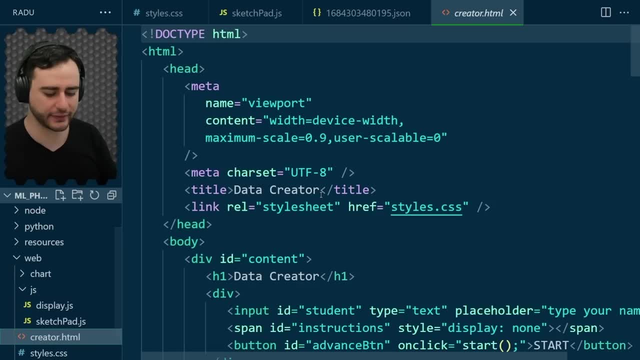 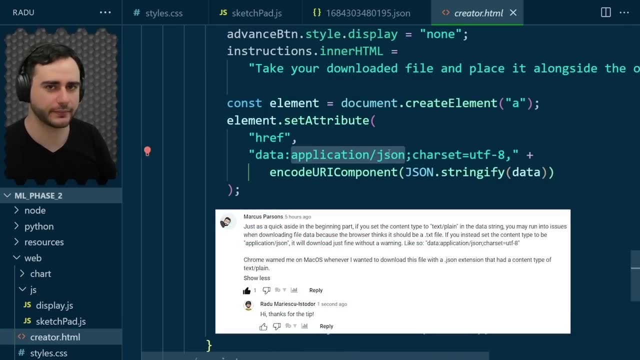 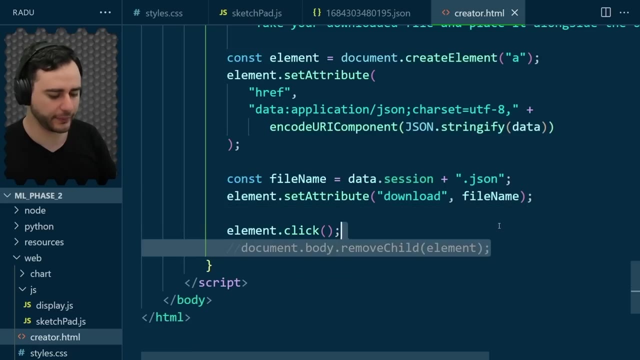 A quick note here about downloading this JSON file. Markus suggested I set here application JSON, otherwise there could be some problems, And godlikemouse pointed out that I don't need to add this anchor here in the body, And it still worked just fine. 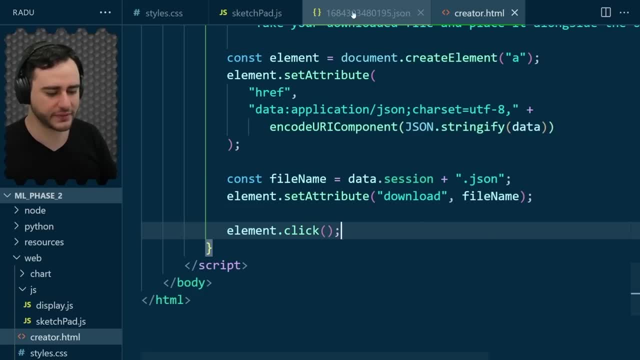 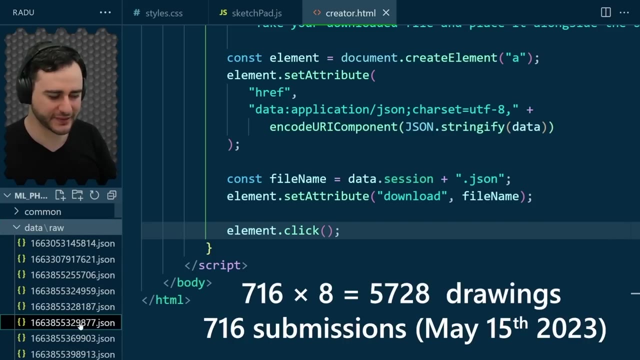 Now, all the data I collected from you has the same structure as this one right here, But it's inside of this data folder and there are a bunch of them. 716 of you made drawings, So that's a total of 5728 drawings. 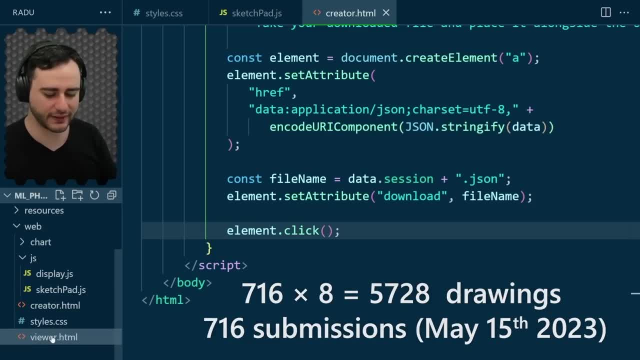 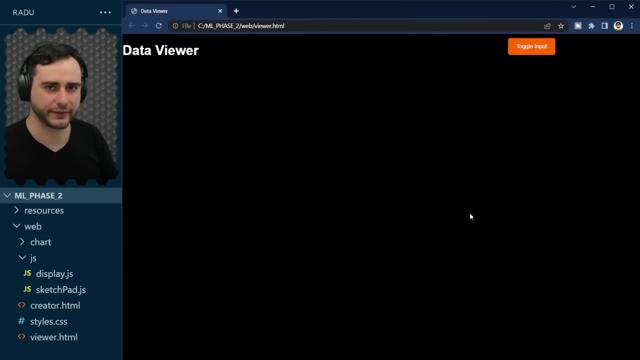 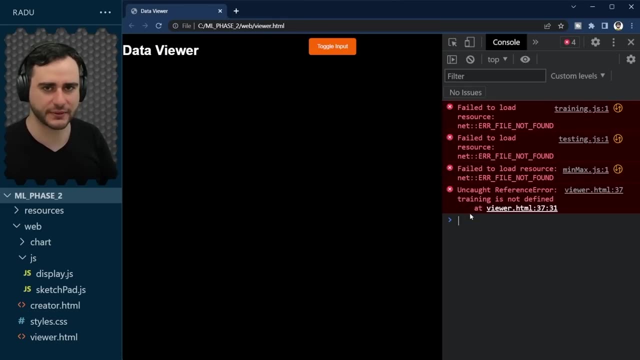 And we can visualize these drawings using this other app that we built. But if we open this viewerhtml in a browser, we see that nothing is there, And if we open the console, there are some errors, And that's because we need to run some scripts to get things started. 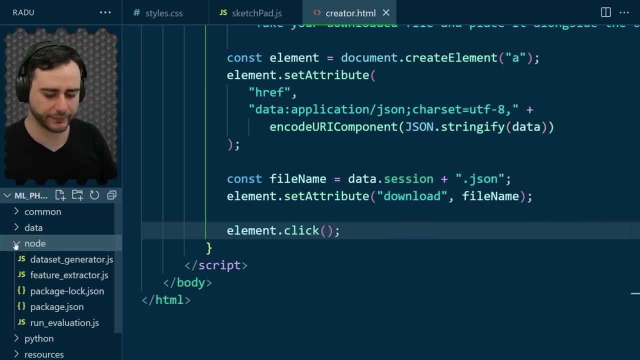 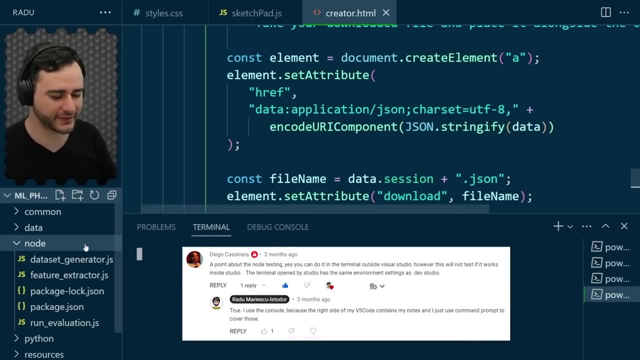 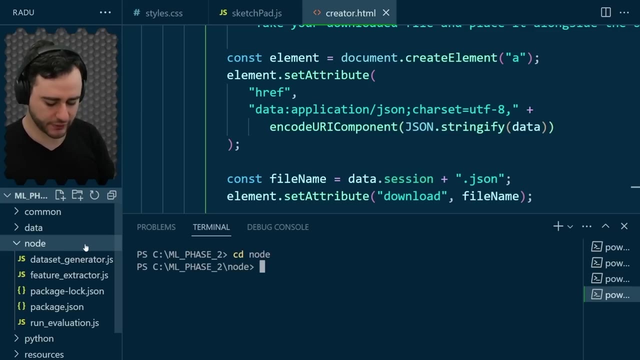 These are here inside of the node folder. We open a text And we have a message that says: I took Diego's advice to use the terminal from here instead of command prompt. Change the directory to be inside of this node folder And let's make sure that we have node installed. 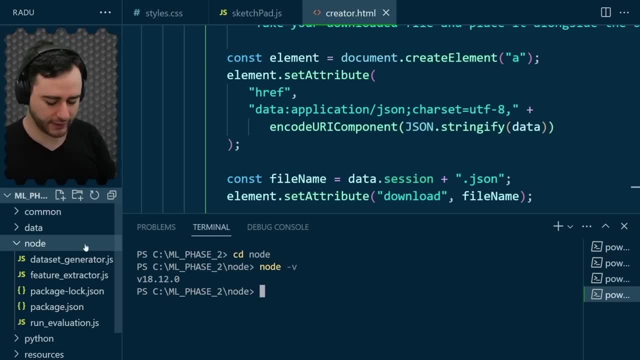 And we do. If not, you're going to have to install it And then you can run npm install inside of this folder And it's going to automatically run all the scripts that we need. It now generates a dataset by running this script. 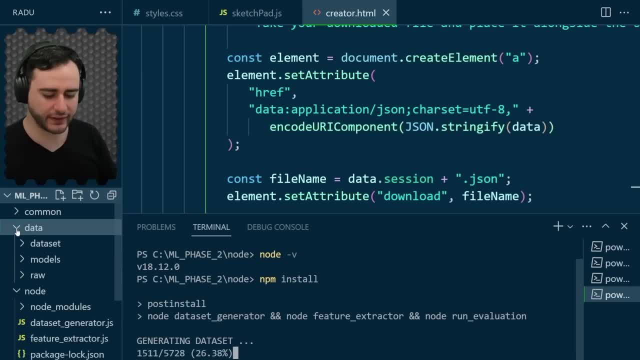 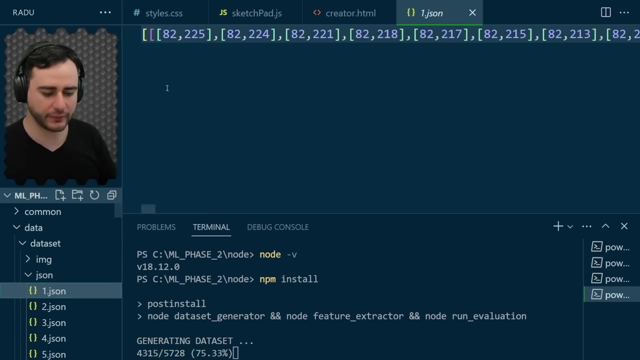 And what that means is that here inside of the data, we don't have just that raw folder anymore. It created a couple of new ones. The dataset folder contains two subfolders. The JSON folder contains one file per sample. So now these paths here are for one drawing. 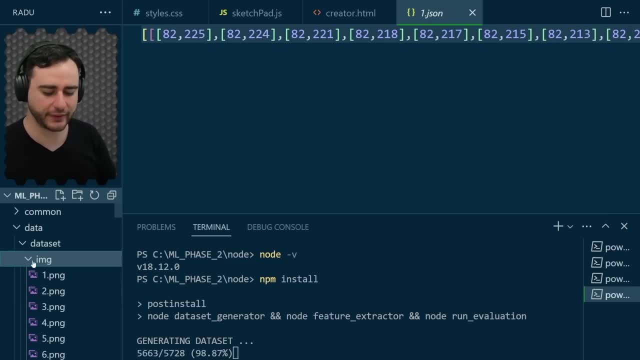 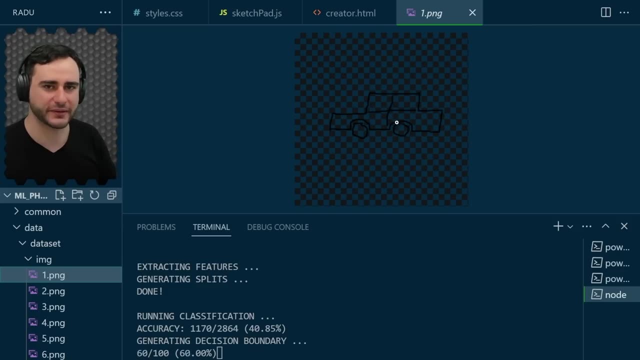 The same drawing that you can actually see here in the image is for the image folder. if you open onepng, There is a car here, but because it's black and with a transparent background doesn't look very nice. But it's okay because all our scripts are finished now. 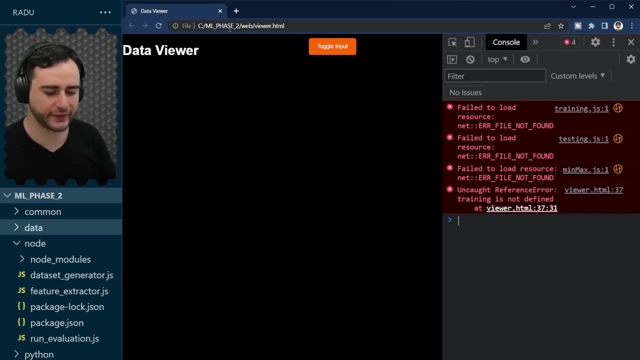 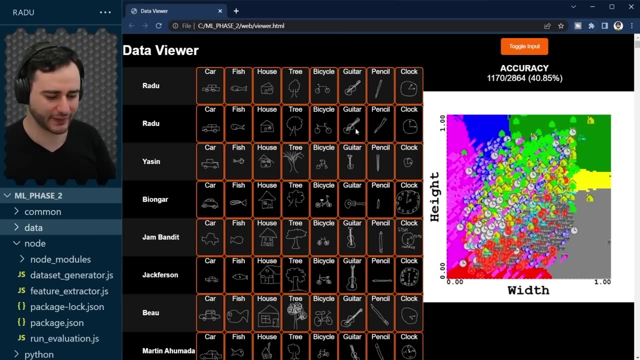 So we can investigate this data in the viewer HTML after we refresh it. You can see how Ninja Coder's style looks here as well. I like this dark mode. I think it's better on the eyes. Now let's see what we can do here. 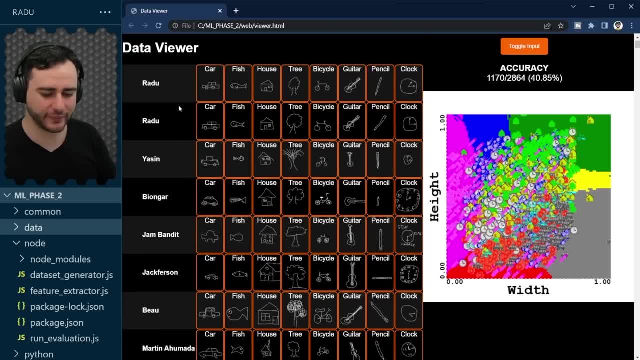 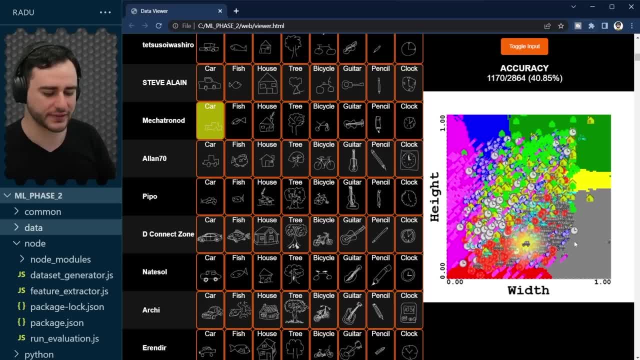 And if you click on one you can see its features on the right highlighted on the chart. Now these features- the width and the height that we extract- are the features of the bounding balls, If I drag this item up here, like so to see it better. 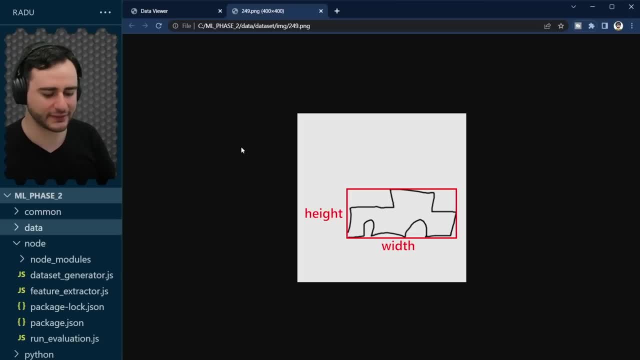 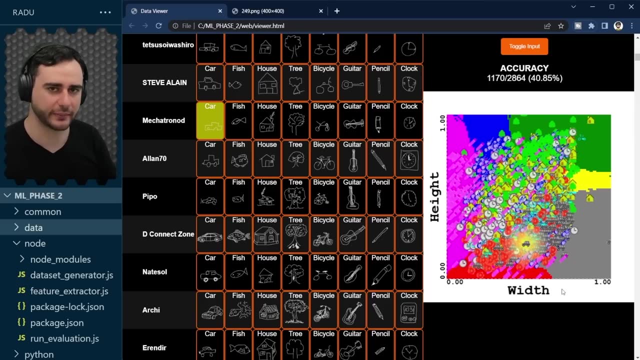 this is what the width means and this is what the height means, and this is what the width means and this is what the height means. So this car has a much larger width than the height. Seems to be about double Now if we scroll down here about halfway. 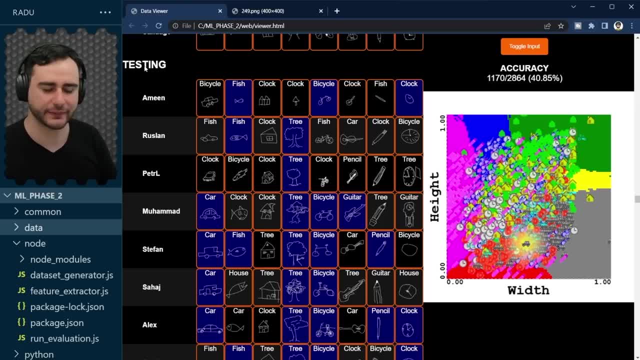 we're going to see a new section starting, called testing, And here the labels that you see written are what our machine learning system thinks that they are. The blue highlights are the correct ones, But the others are wrong. And here, if we are going to click on something, for example this pencil- 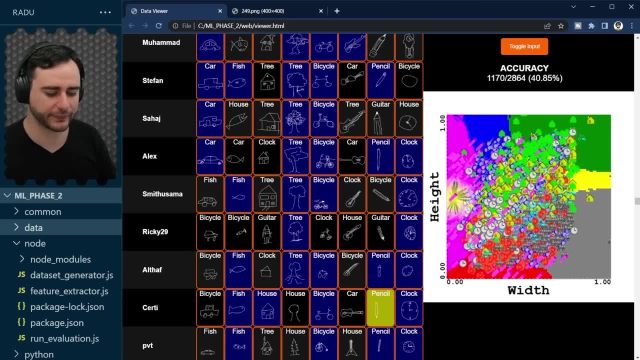 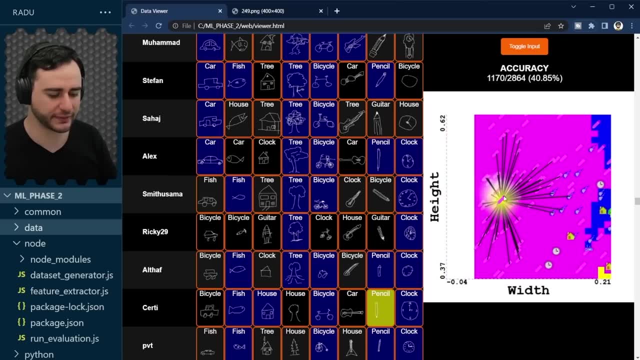 we will see a different kind of highlight here on the chart. Let me zoom in a little bit And, just to make things clear, I'm going to click on this pencil a few more times And notice that it's not originally there. It's a new point that we've added now, and it's categorized as a pencil. 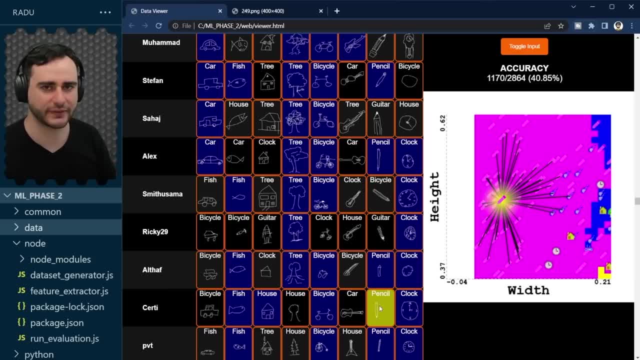 because its nearest neighbors. the majority of them are pencils. Here we use 50 nearest neighbors and I'm drawing a connection to all of them. So, based on the majority, our machine learning system, the k-nearest-neighbor classifier, categorizes this as a pencil. 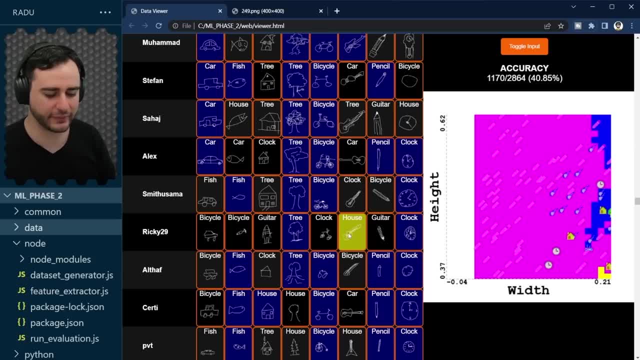 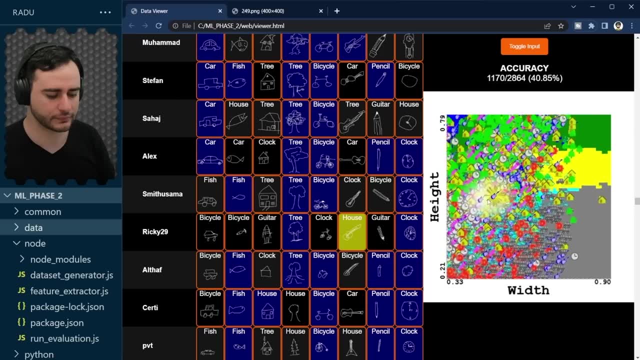 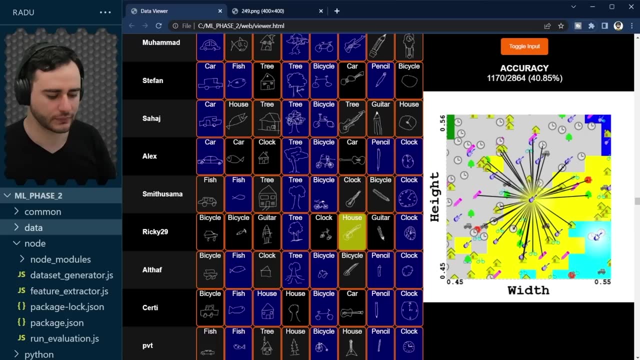 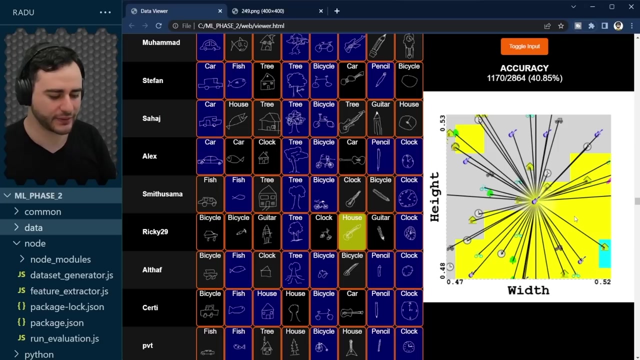 But sometimes, like this guitar, for example, seems to be a house. Let's figure out why. It's quite hard to count, but you can probably see quite many houses here in this area. so it is a house. Our accuracy is not that good at the moment, but I'm going to teach you how to double it by the end of this course. 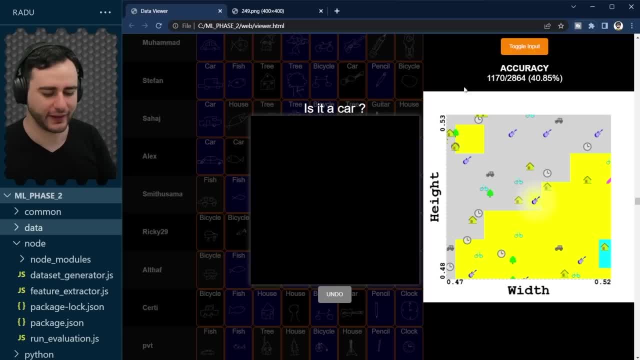 There's also this button here for opening the sketch pad And here you can draw something. And here you can draw something live And in real time. you're going to get the classification. If you zoom out, you're going to see this drawing that we made here and all of its nearest neighbors. 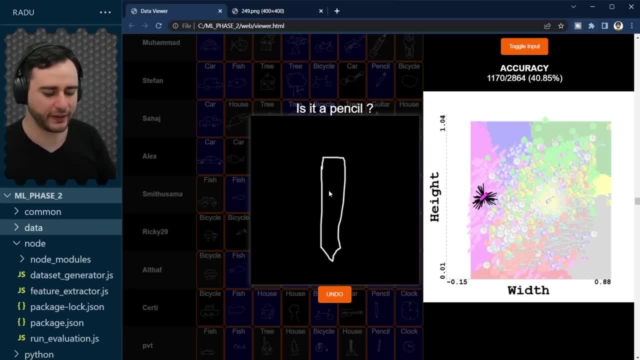 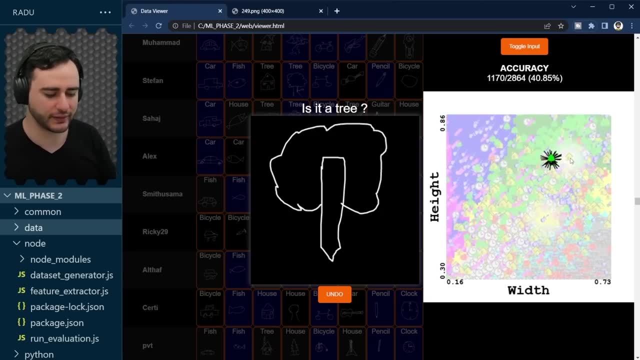 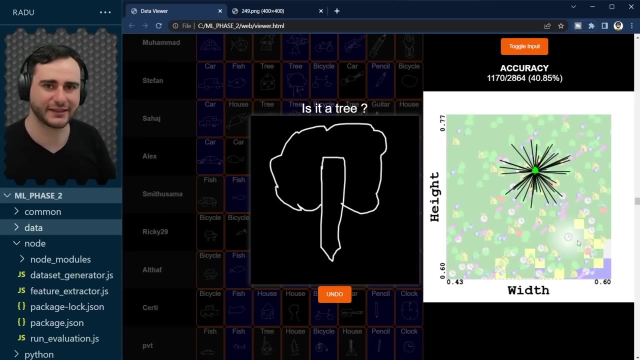 And in this case, the majority are pencils, But maybe if we're going to turn this into a tree, Now, this has changed And the new majority seem to be trees, And the new majority seem to be trees. We built some really nice tools, didn't we? 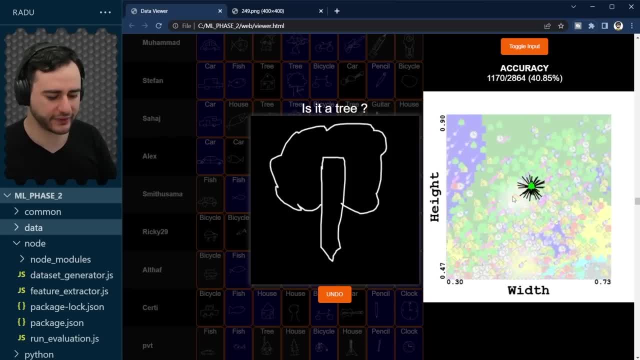 We built some really nice tools, didn't we? One more thing I should remind you of is that we also have this decision boundary plot. One more thing I should remind you of is that we also have this decision boundary plot. One more thing I should remind you of is that we also have this decision boundary plot. 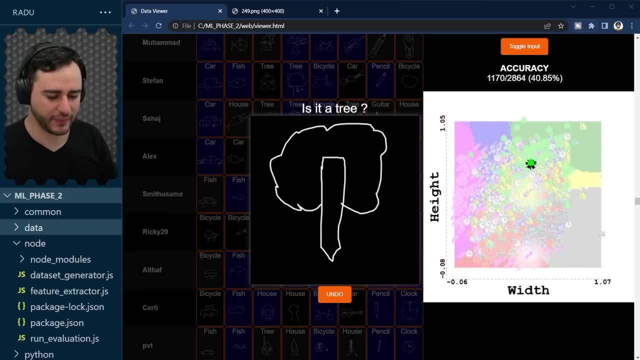 This colored background right here. We can use this decision boundary plot more effectively if we go inside of the viewer here and pass the testing samples instead of the training samples to the chart. We can use this decision boundary plot more effectively if we go inside of the viewer here and pass the testing samples instead of the training samples to the chart. 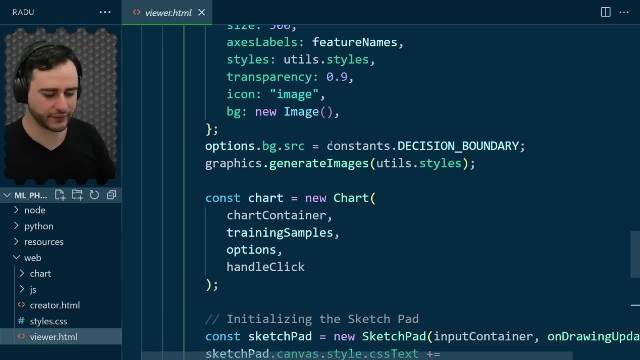 We can use this decision boundary plot more effectively if we go inside of the viewer here and pass the testing samples instead of the training samples to the chart. We can use this decision boundary plot more effectively if we go inside of the viewer here and pass the testing samples instead of the training samples to the chart. 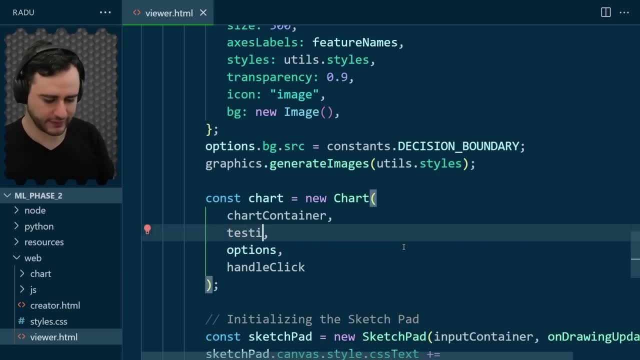 We can use this decision boundary plot more effectively if we go inside of the viewer here and pass the testing samples instead of the training samples to the chart. We can use this decision boundary plot more effectively if we go inside of the viewer here and pass the testing samples instead of the training samples to the chart. 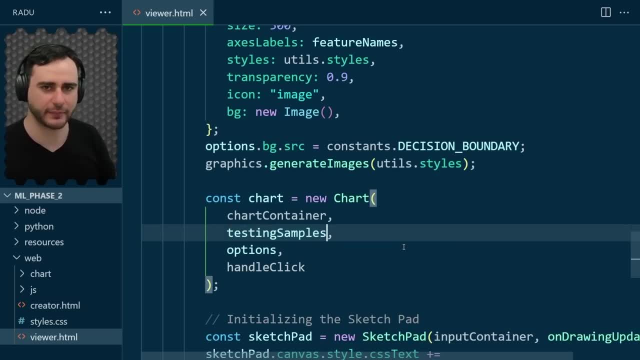 We can use this decision boundary plot more effectively if we go inside of the viewer here and pass the testing samples instead of the training samples to the chart. We can use this decision boundary plot more effectively if we go inside of the viewer here and pass the testing samples instead of the training samples to the chart. 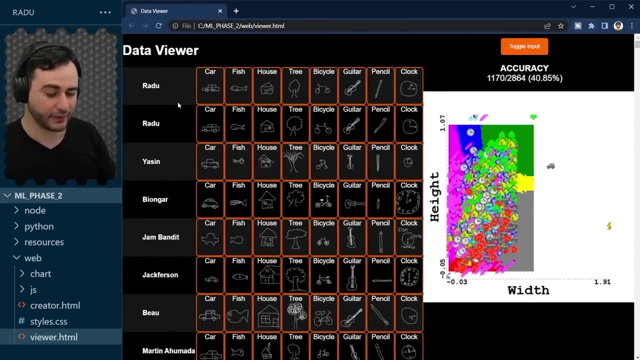 We can use this decision boundary plot more effectively if we go inside of the viewer here and pass the testing samples, instead of the training samples, to the chart. We can use this decision boundary plot more effectively if we go inside of the viewer here and pass the testing samples to the chart. 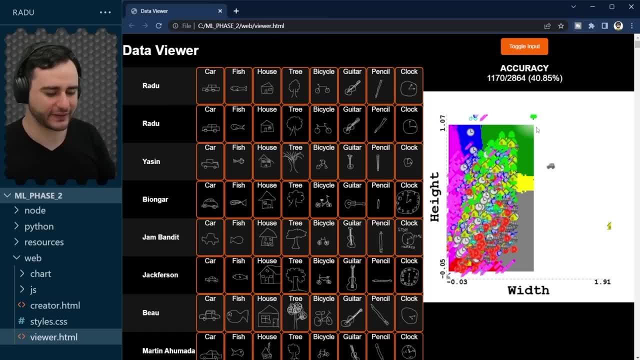 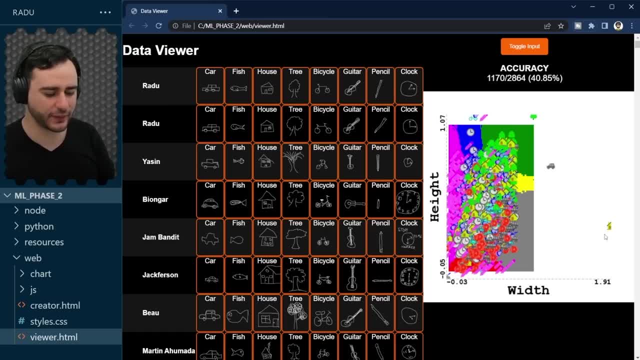 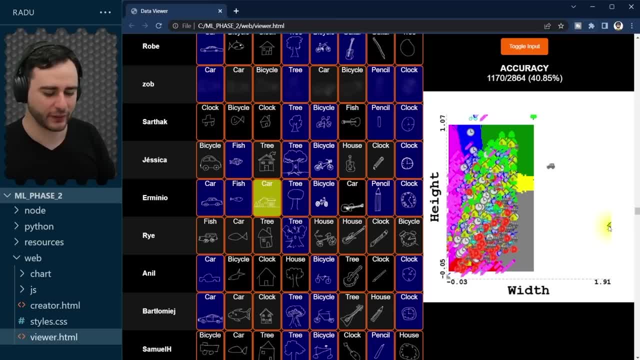 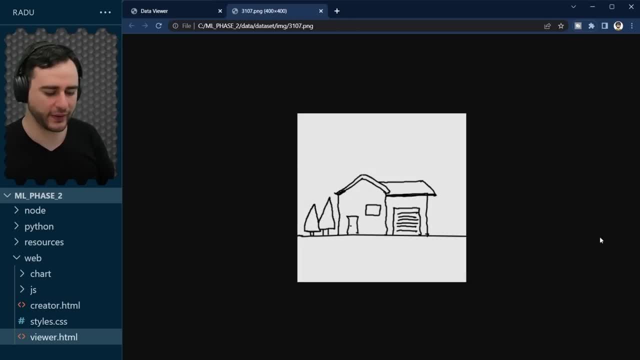 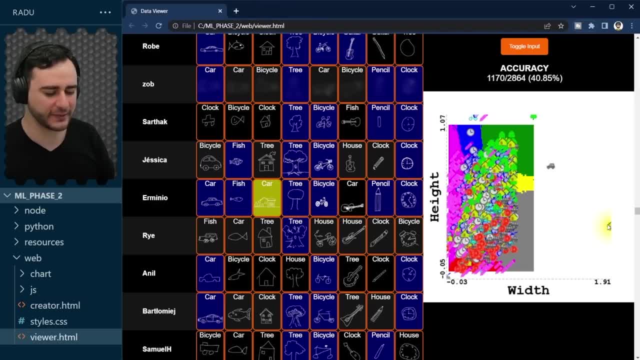 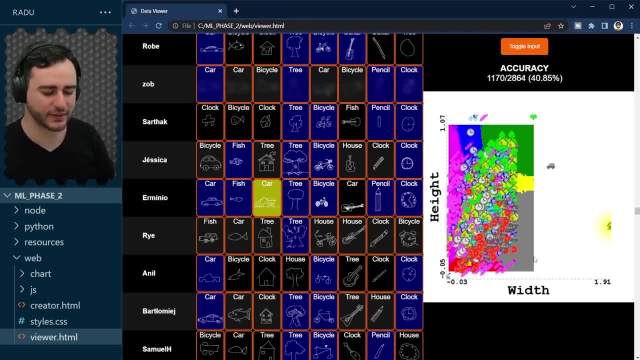 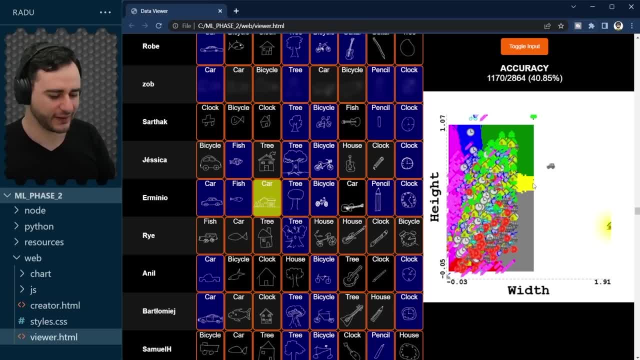 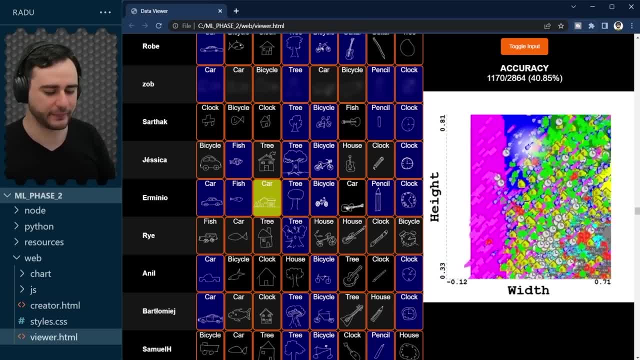 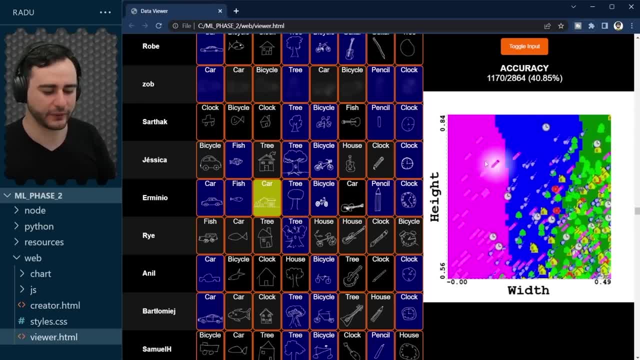 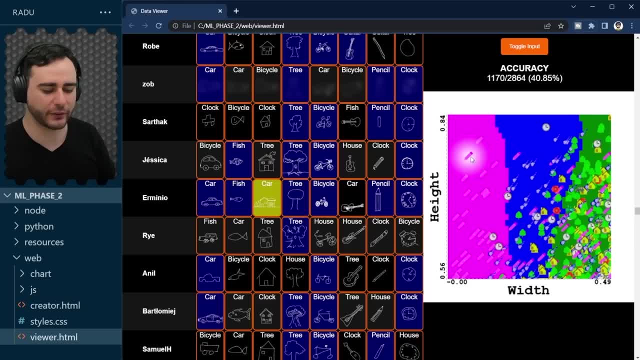 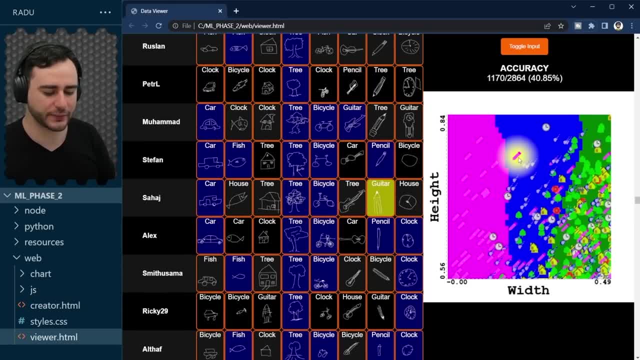 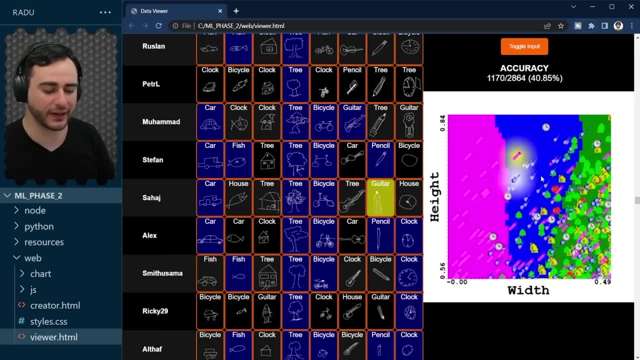 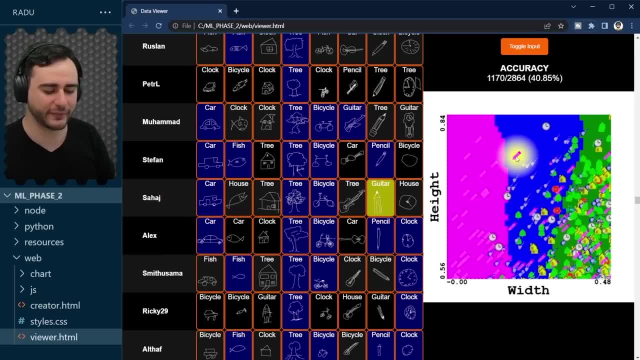 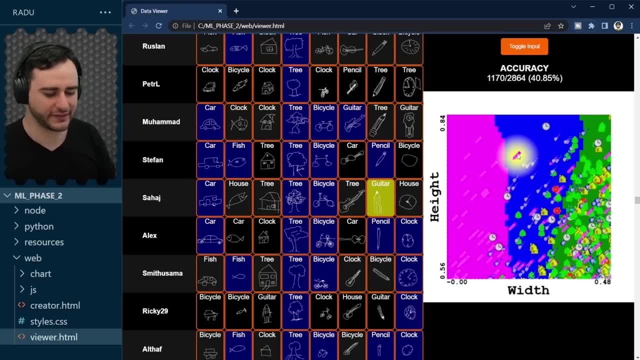 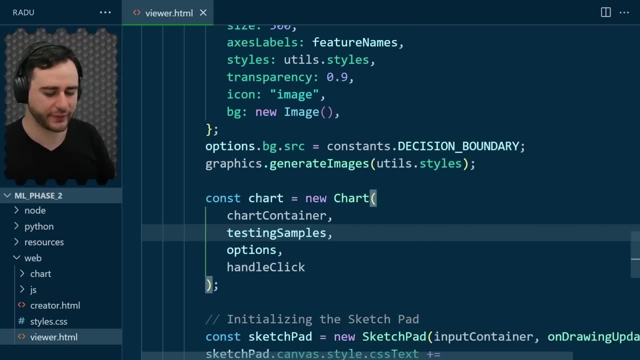 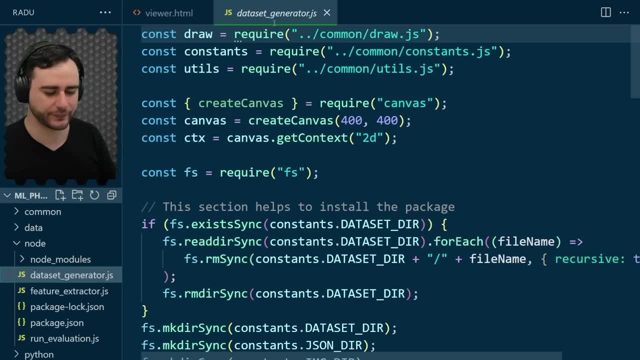 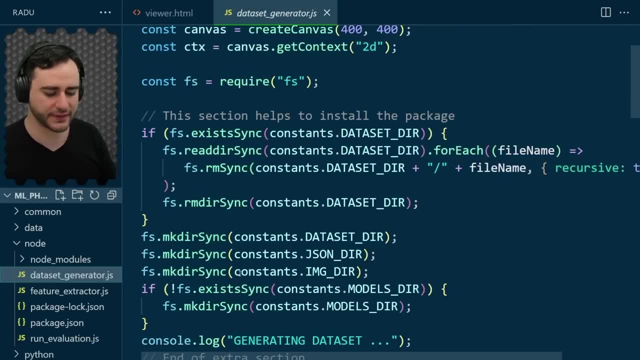 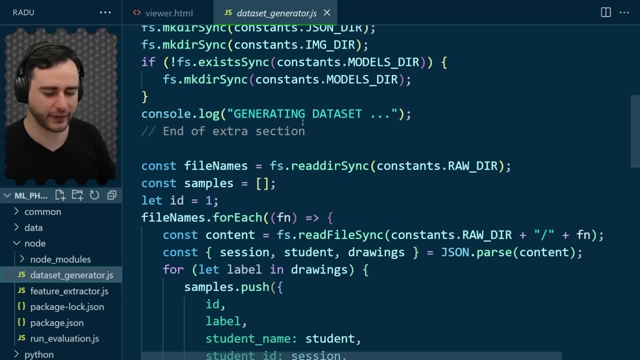 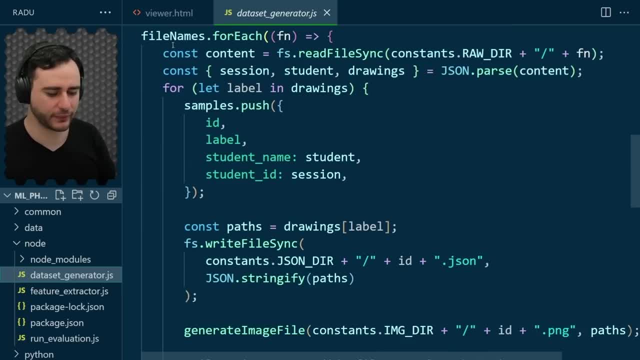 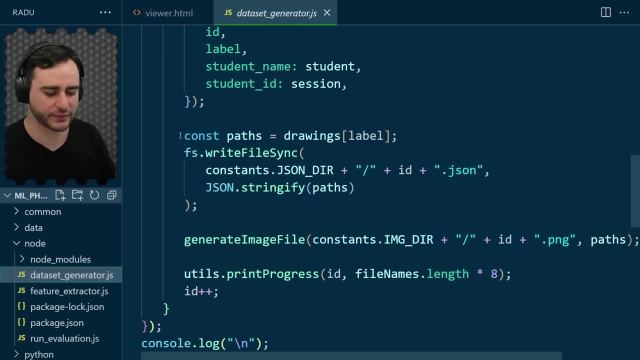 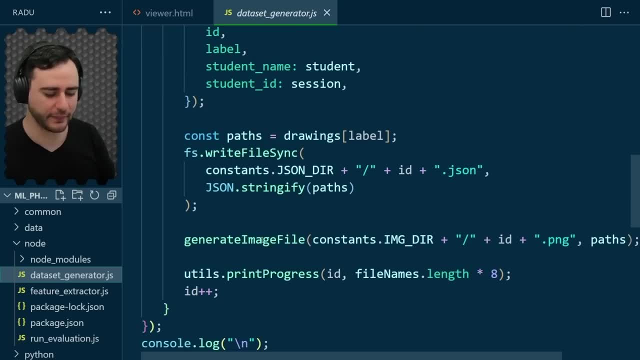 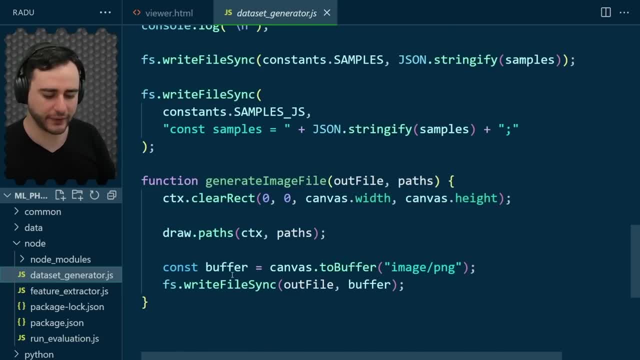 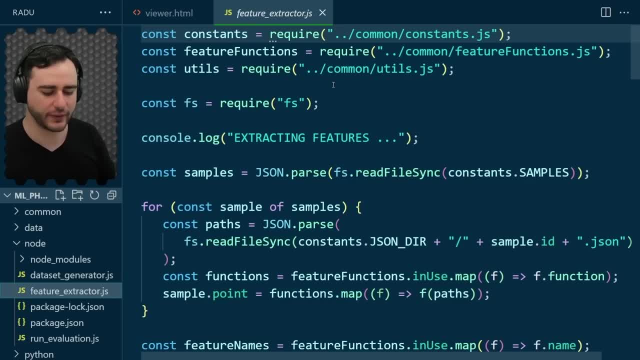 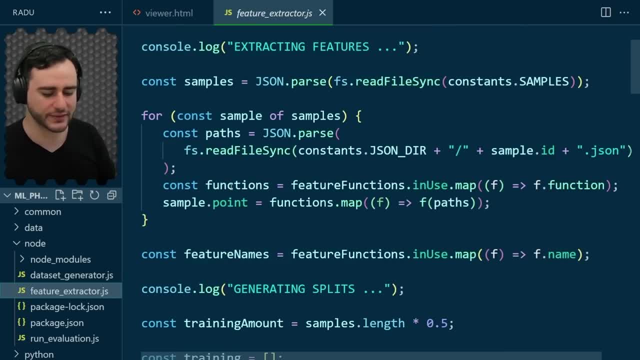 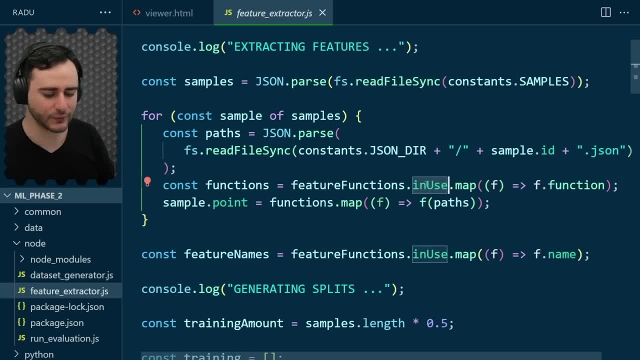 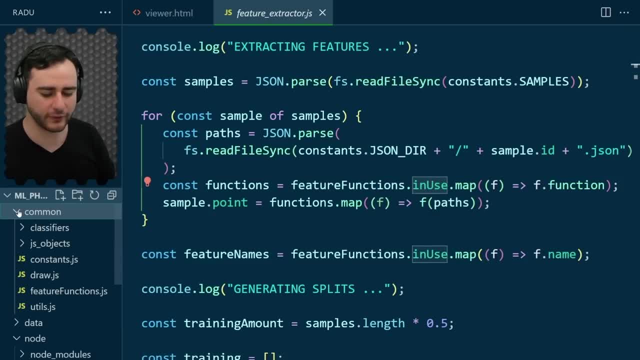 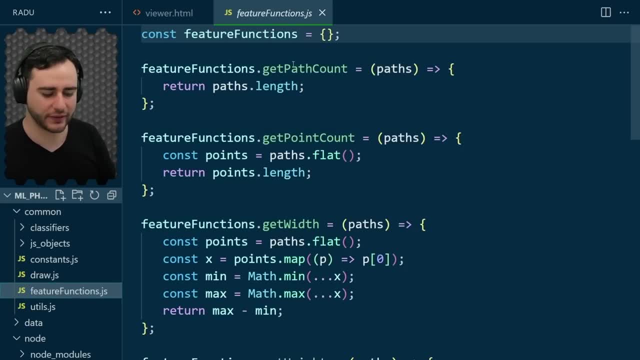 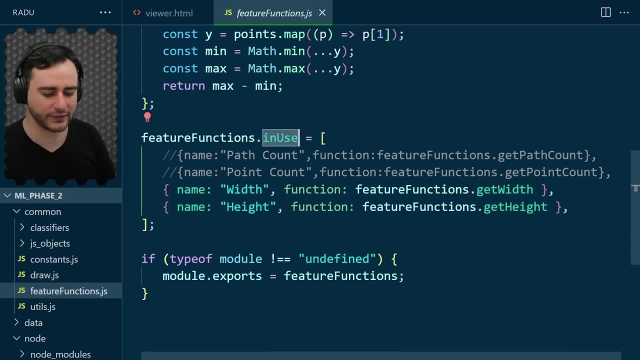 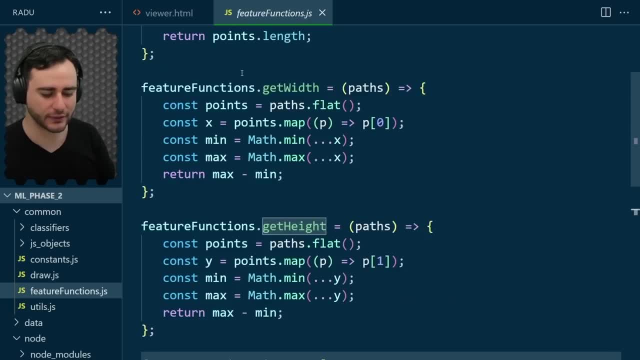 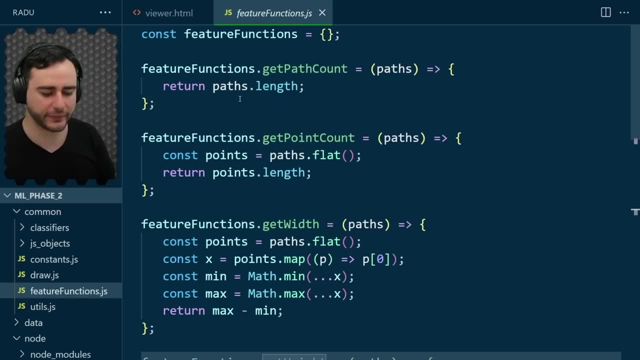 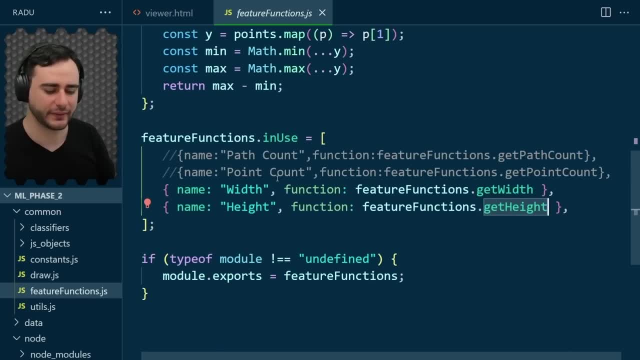 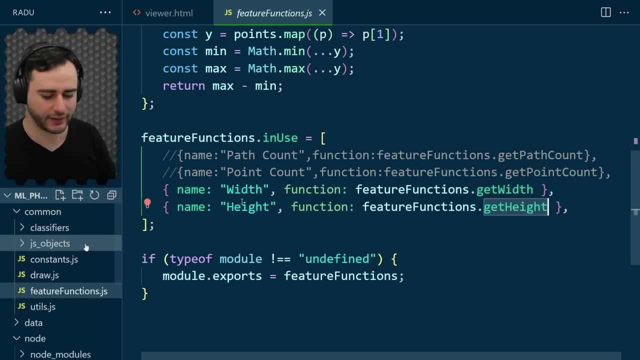 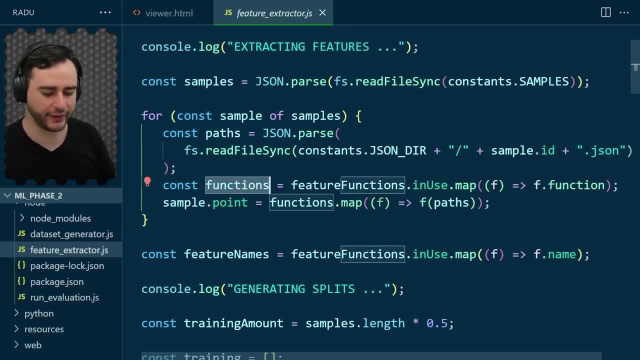 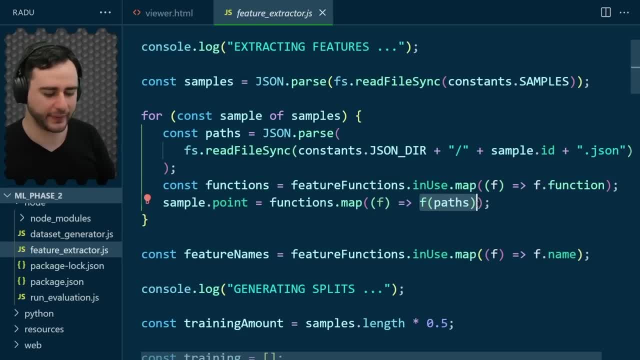 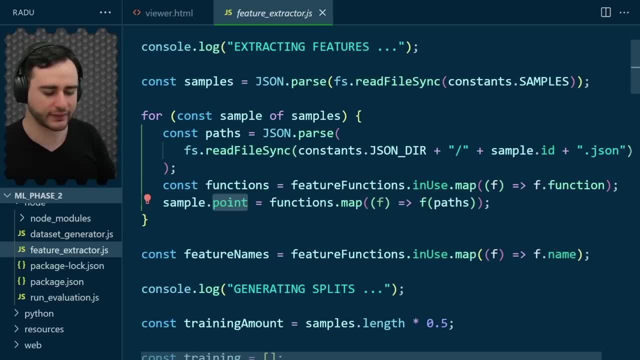 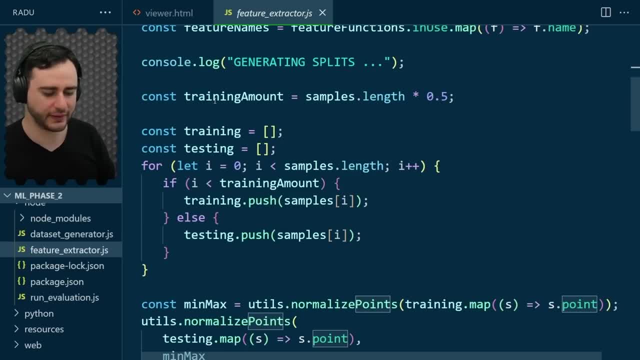 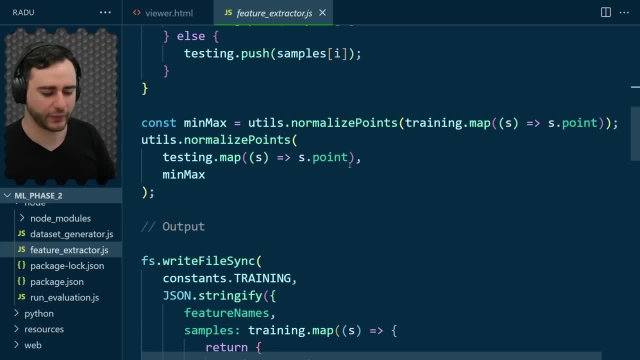 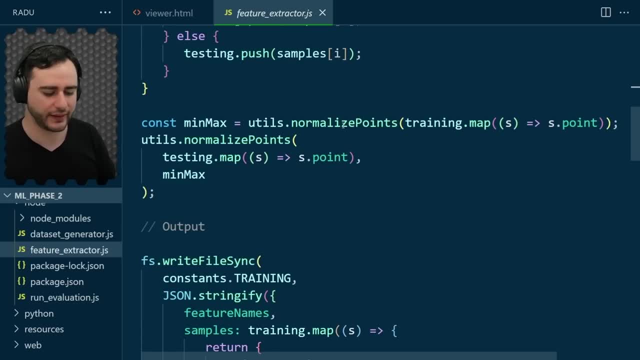 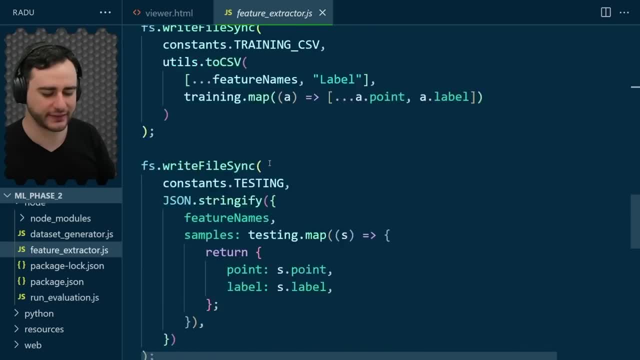 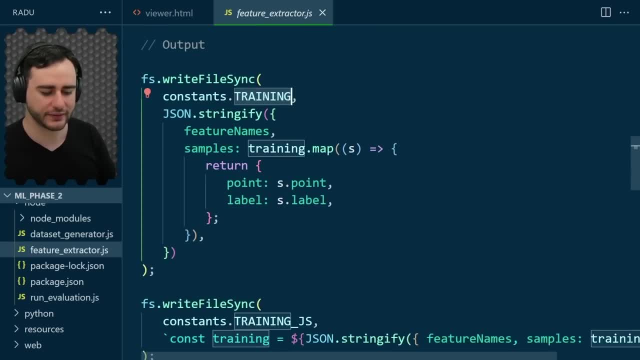 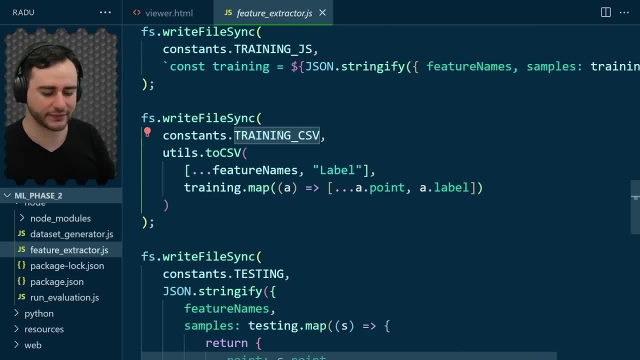 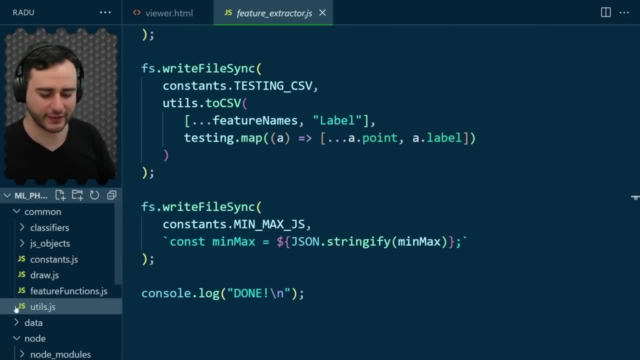 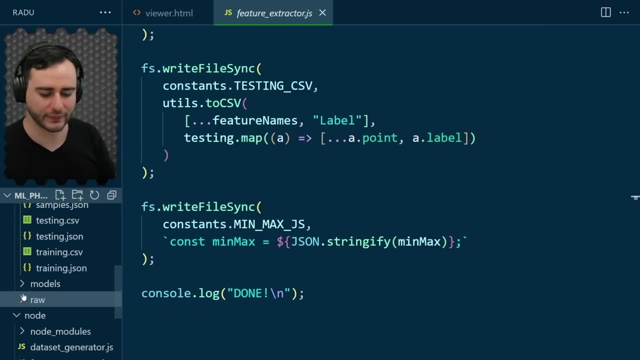 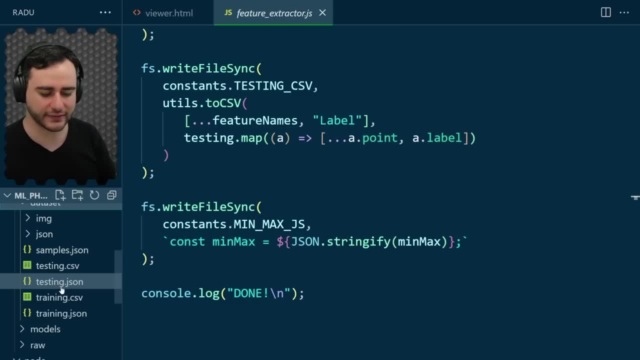 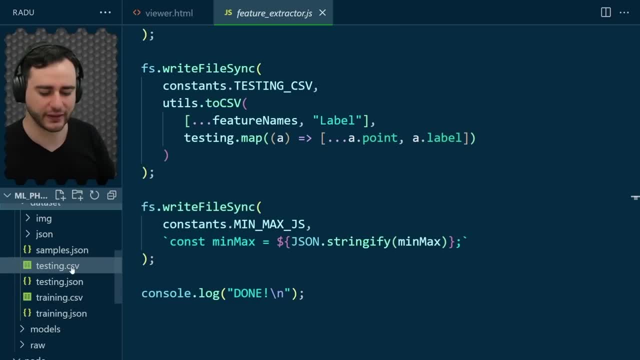 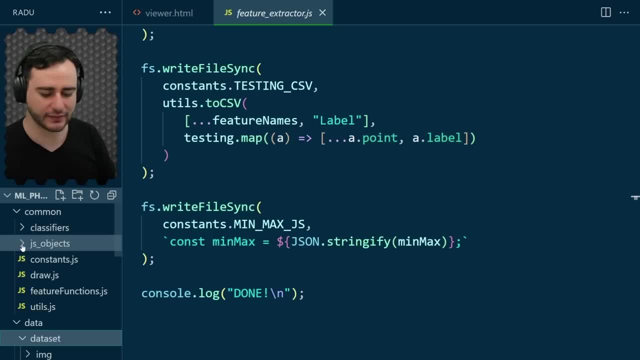 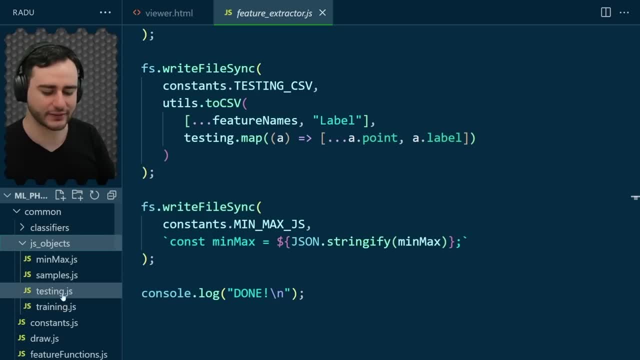 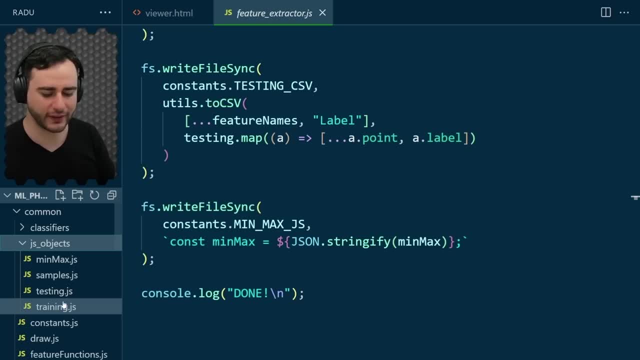 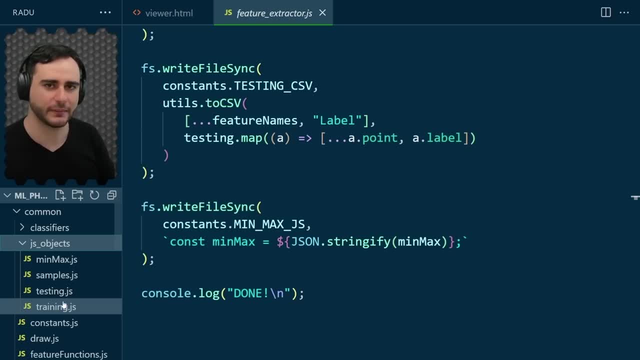 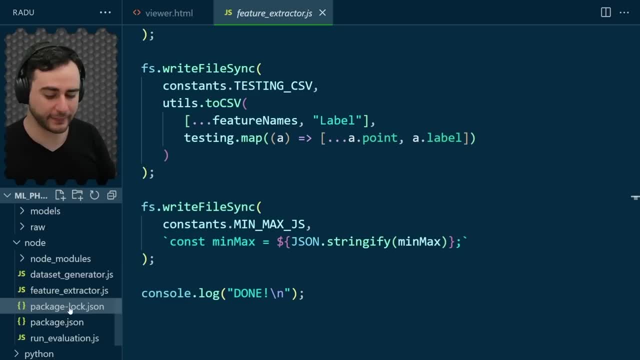 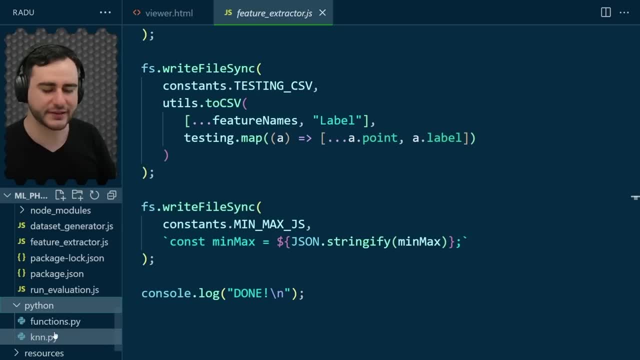 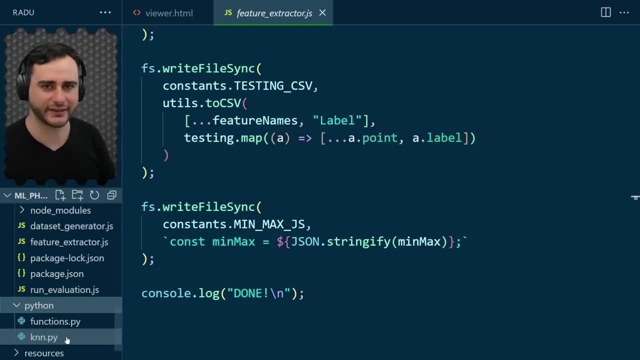 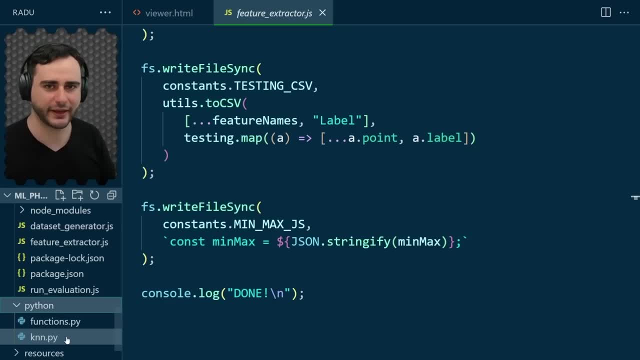 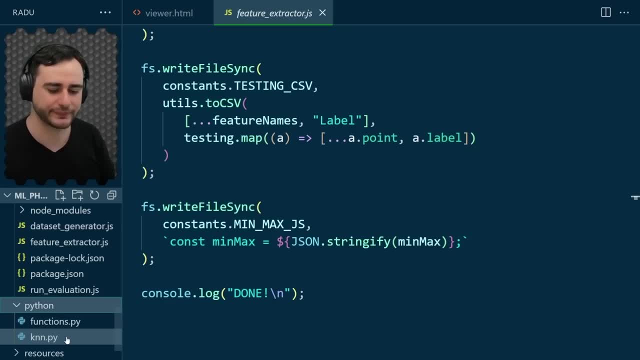 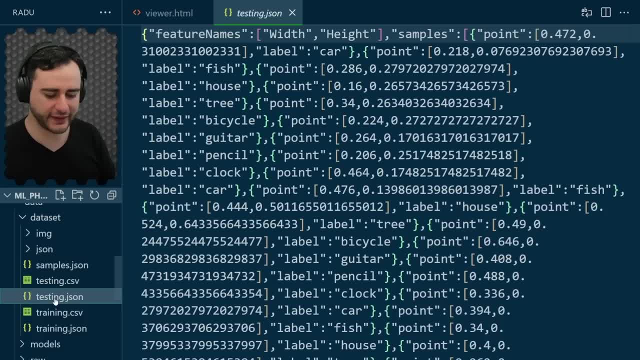 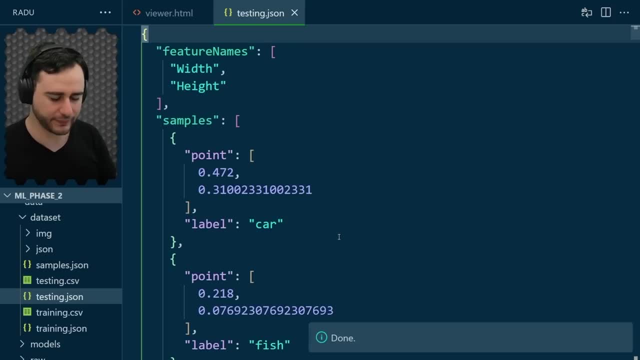 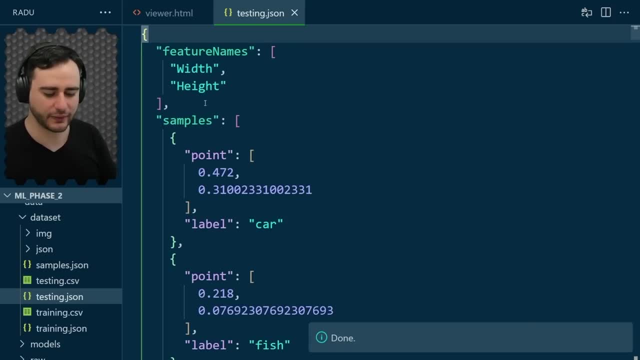 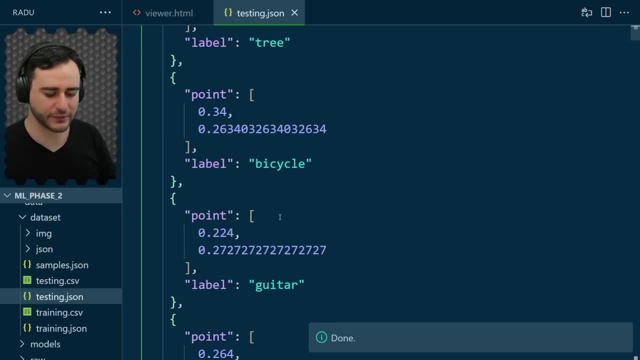 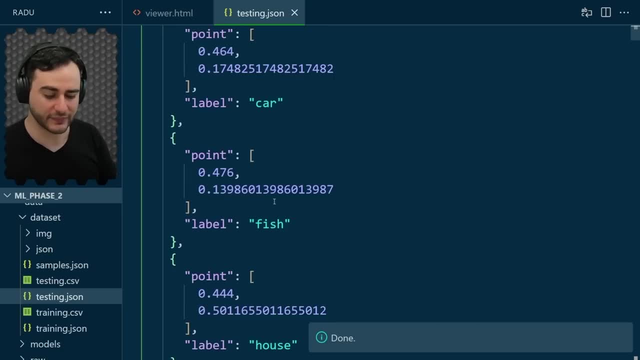 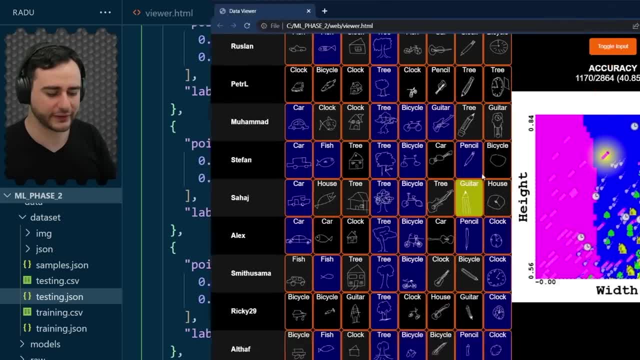 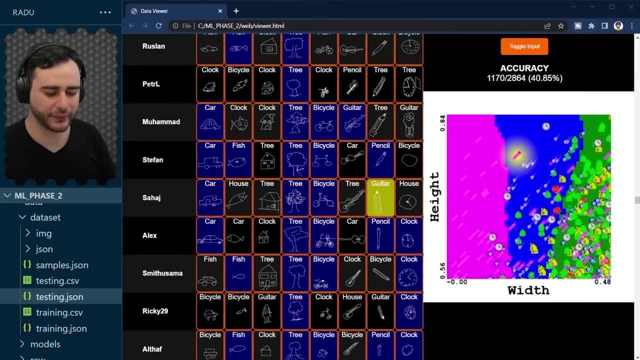 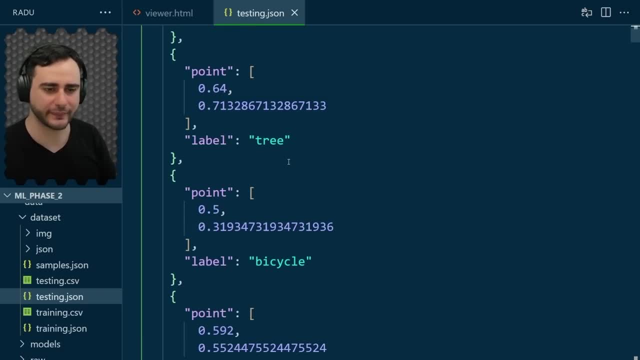 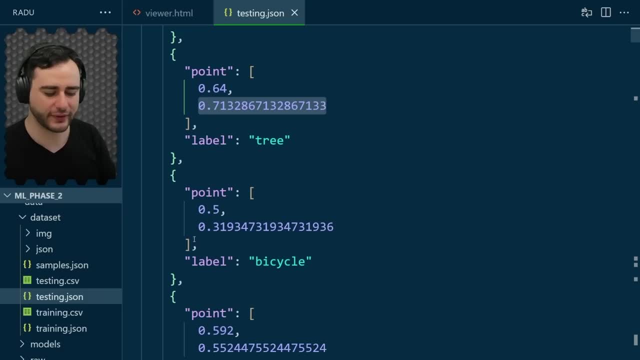 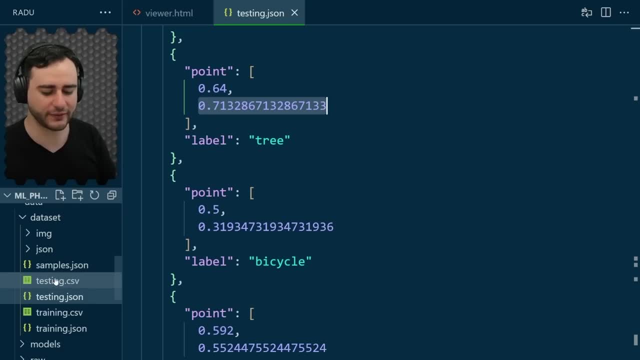 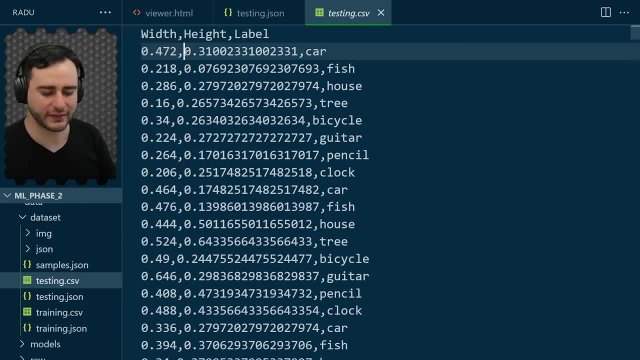 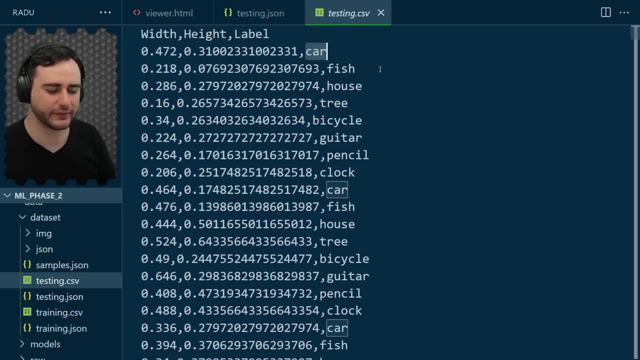 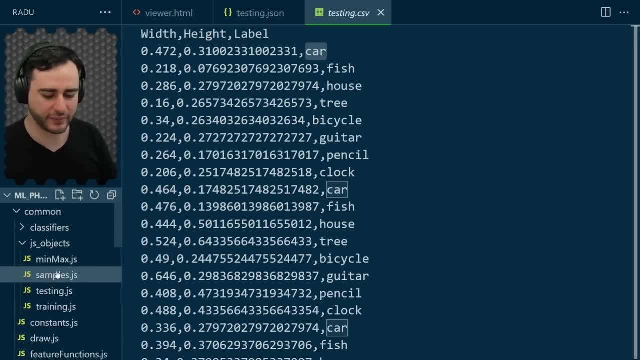 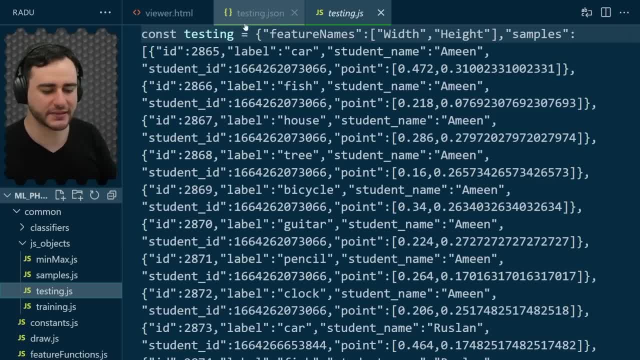 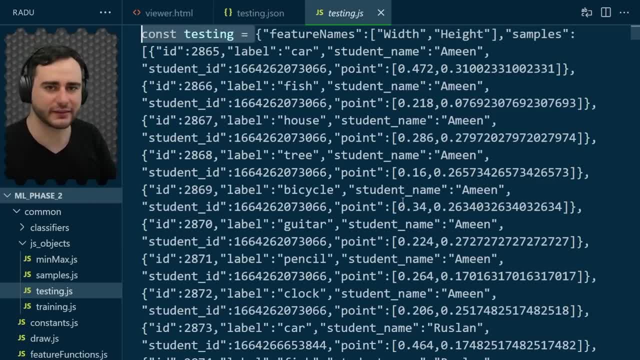 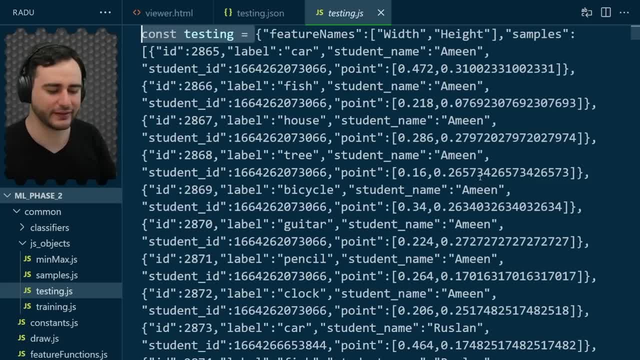 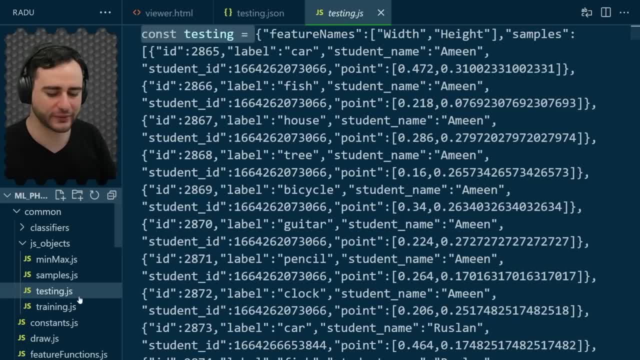 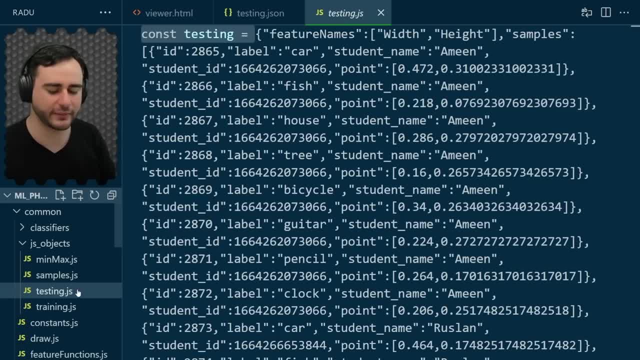 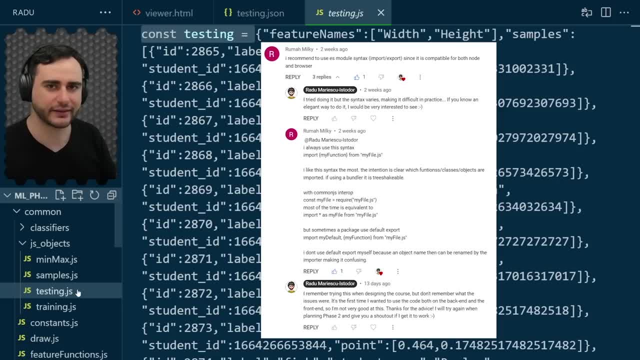 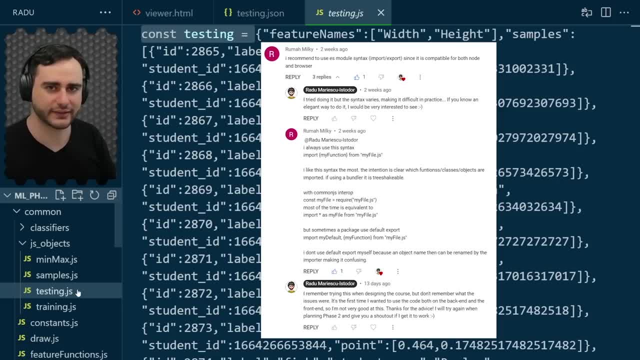 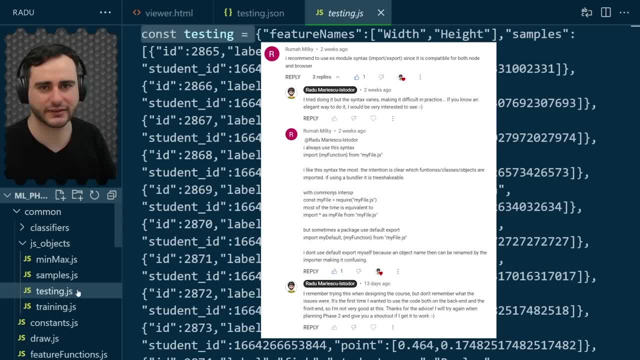 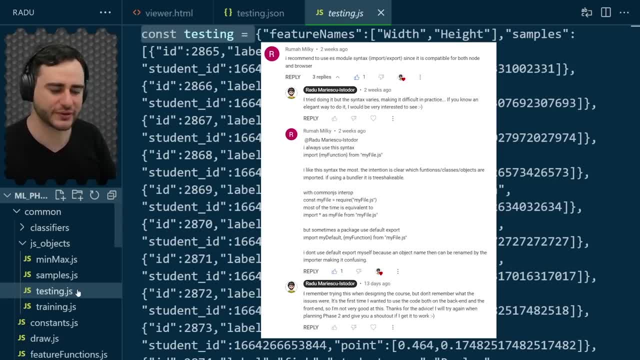 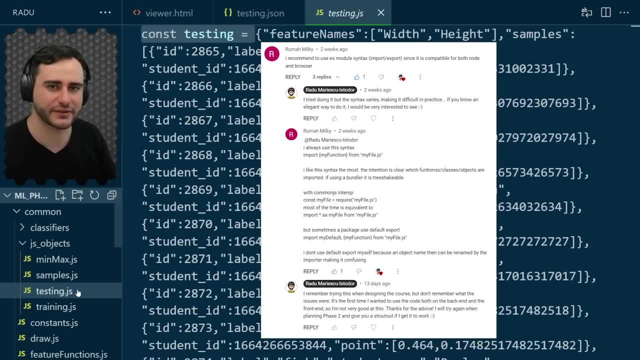 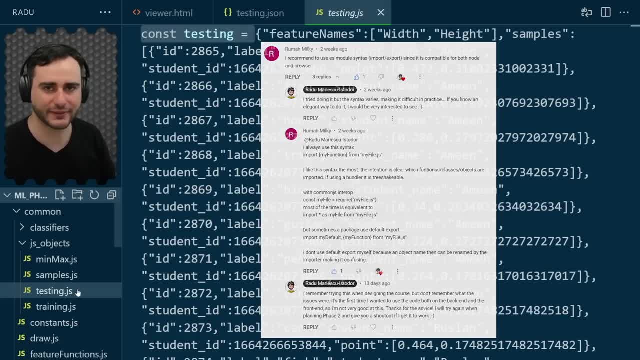 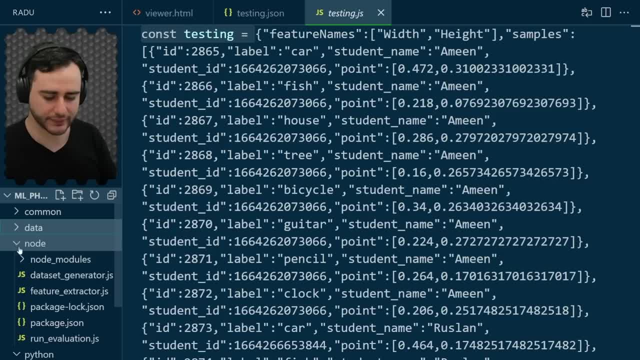 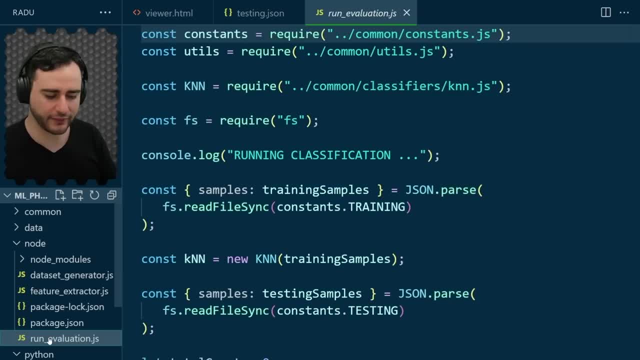 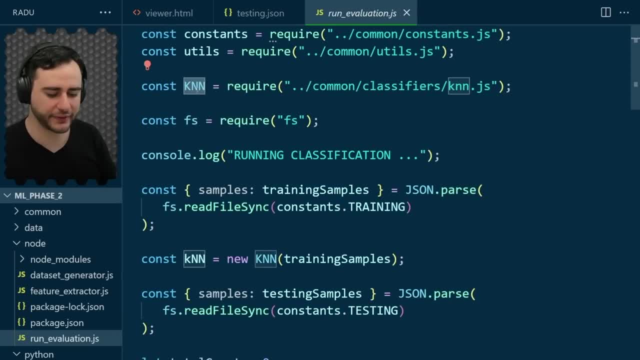 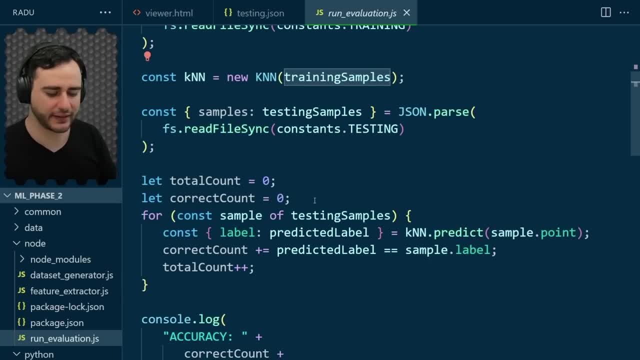 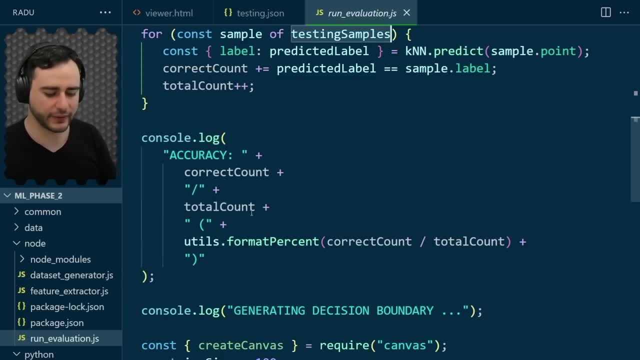 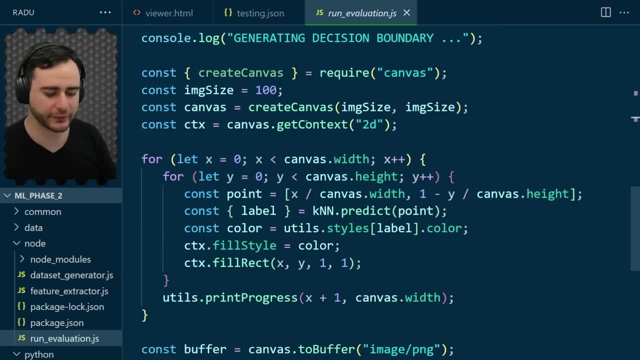 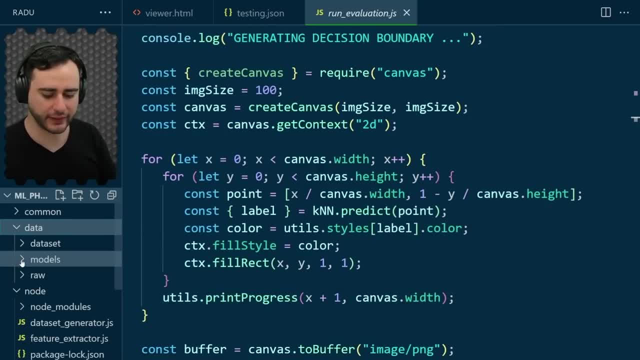 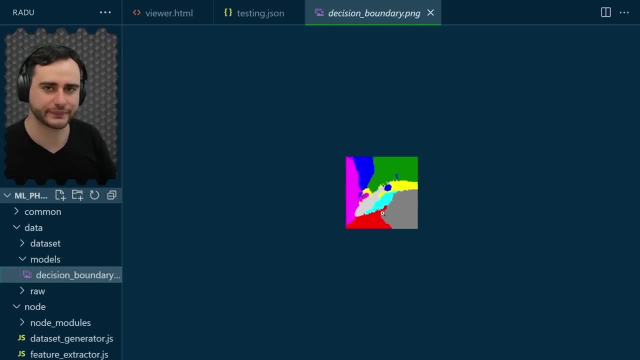 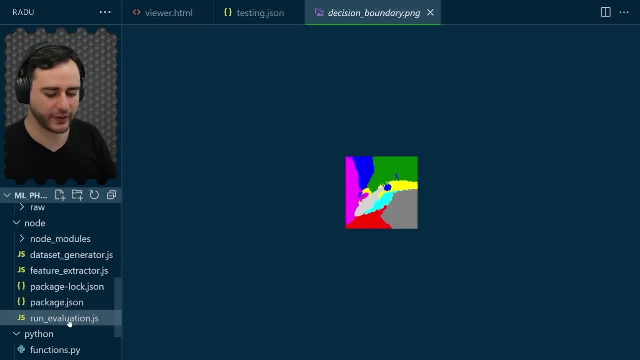 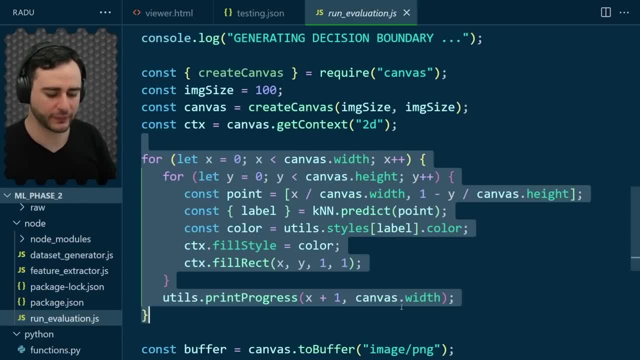 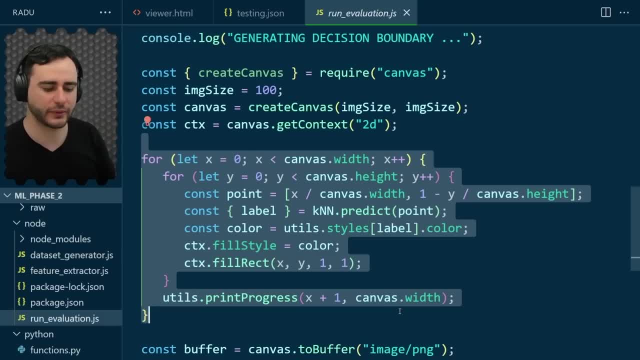 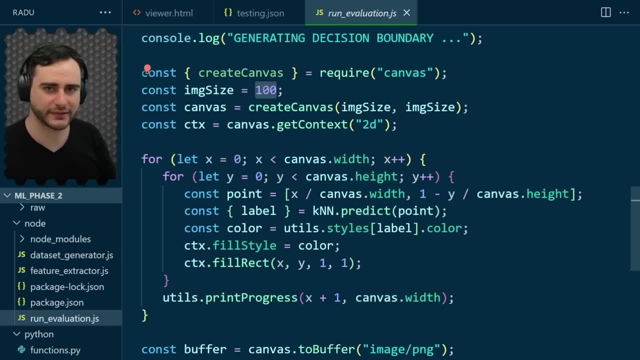 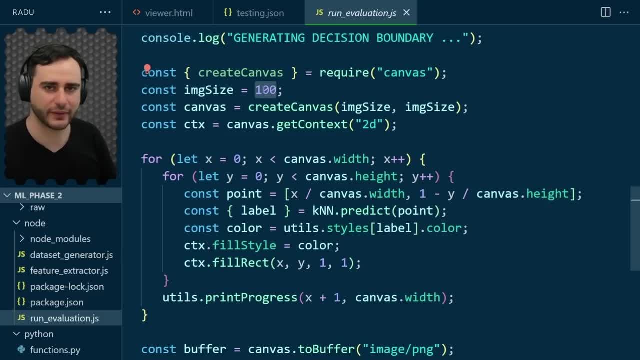 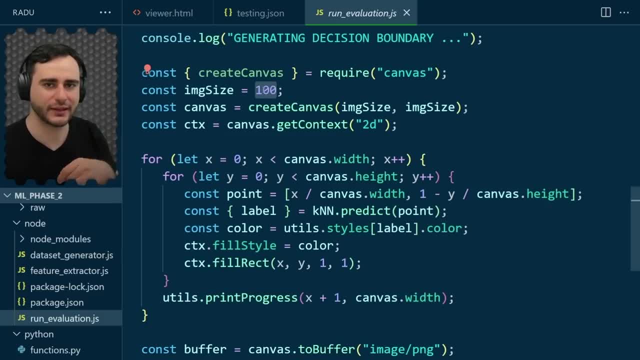 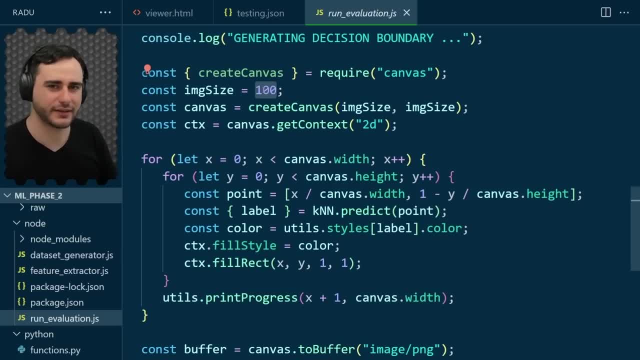 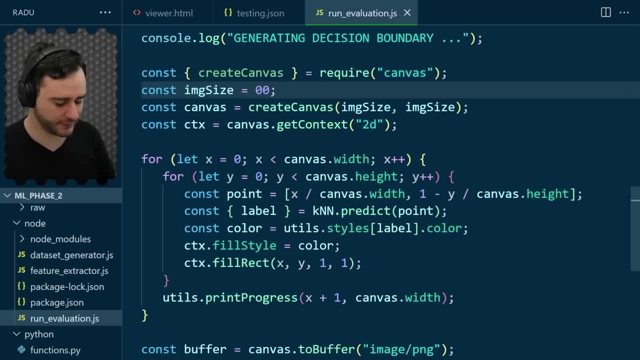 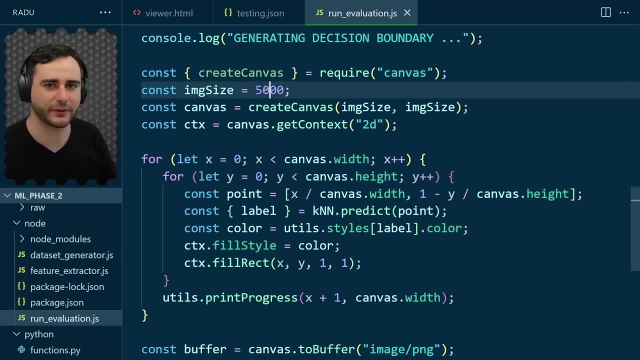 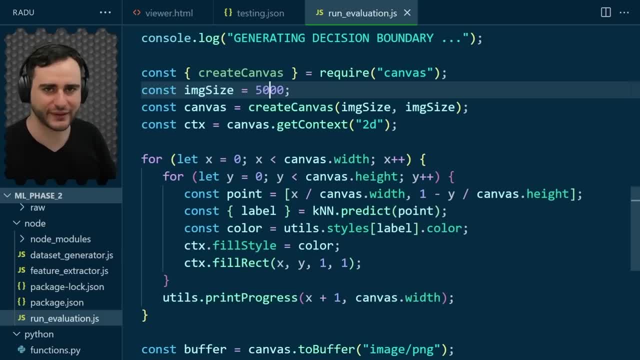 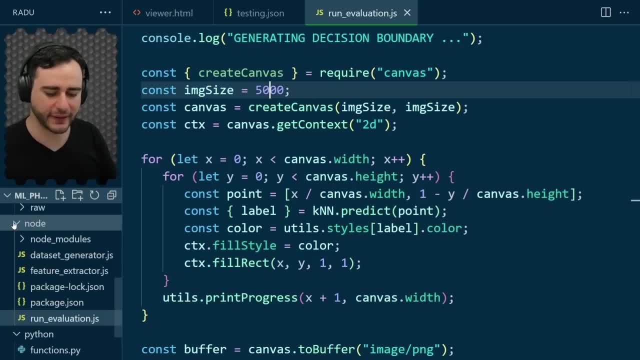 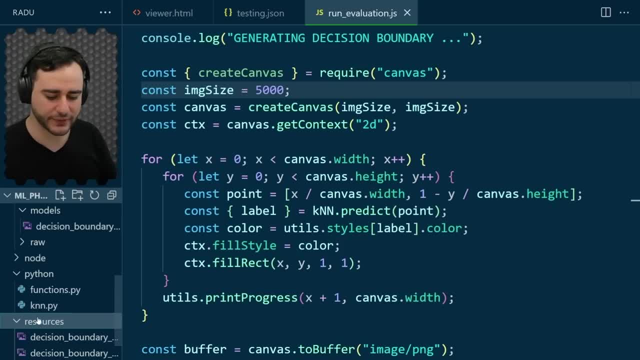 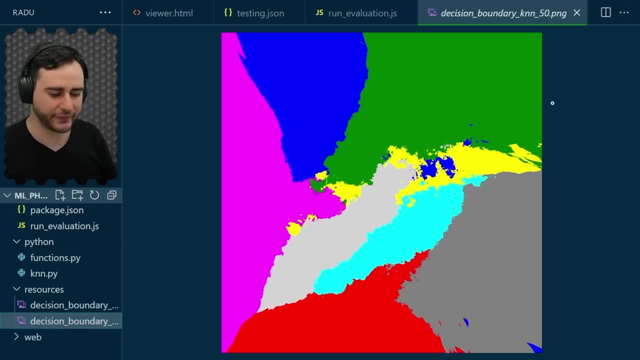 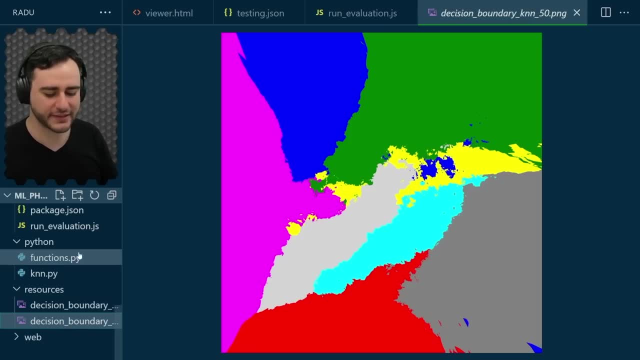 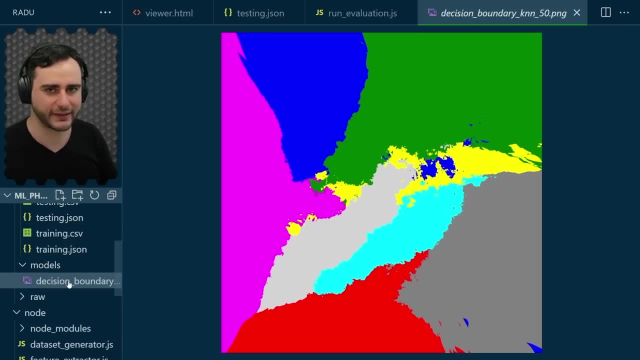 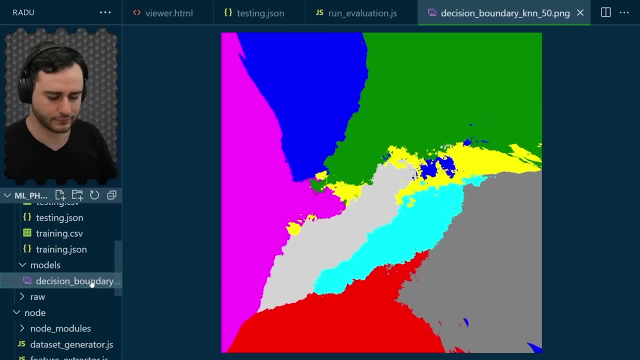 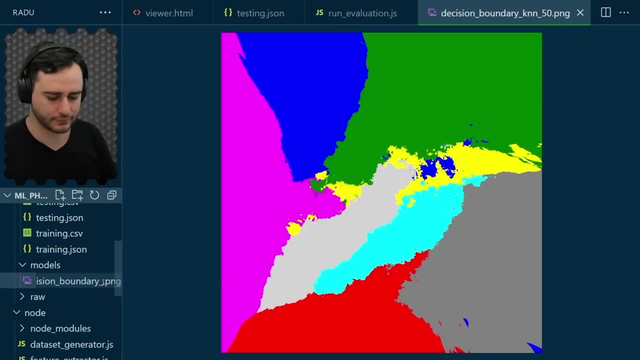 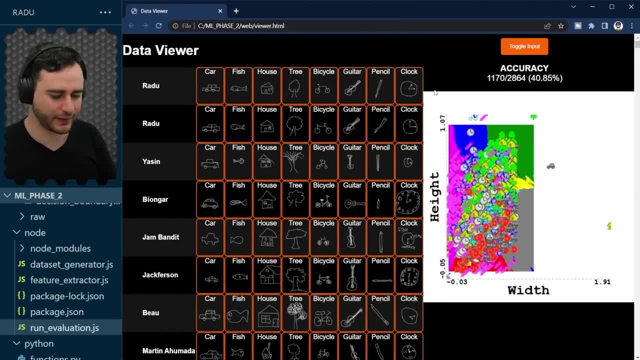 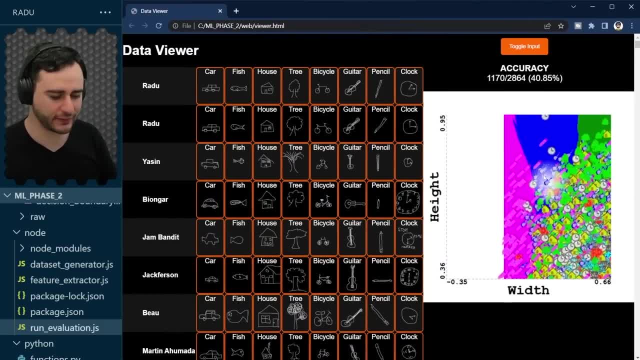 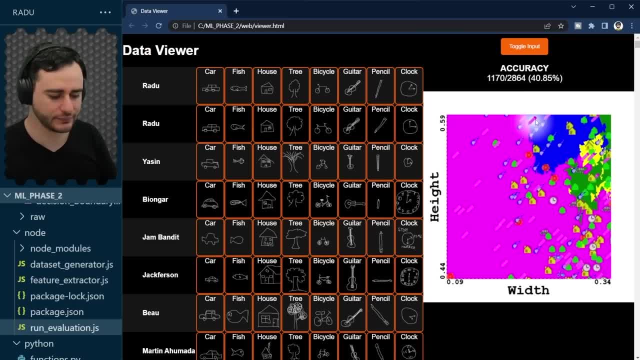 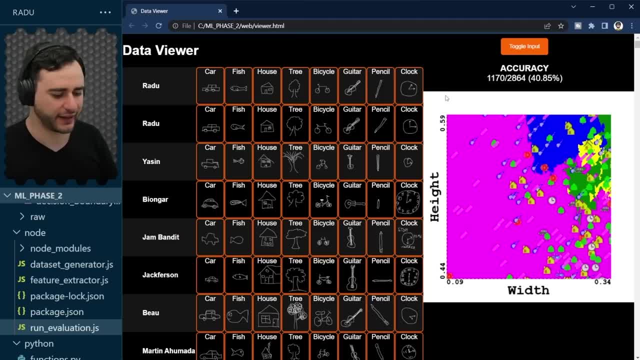 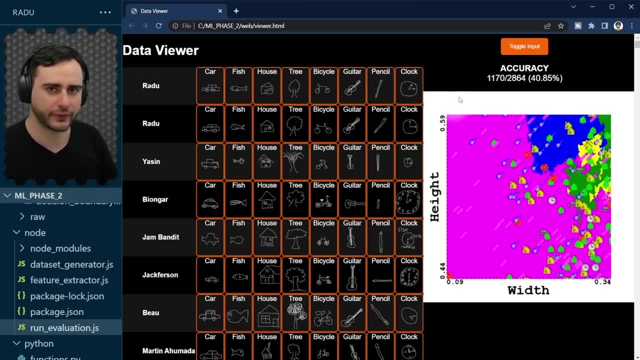 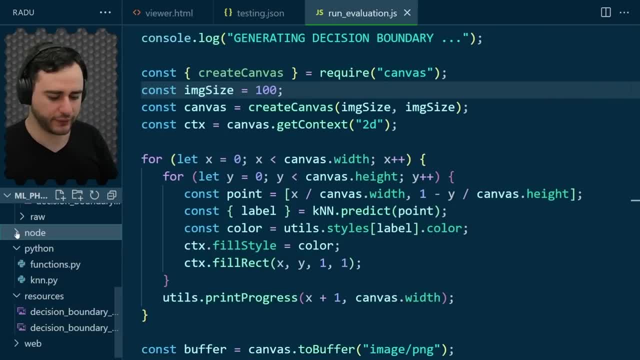 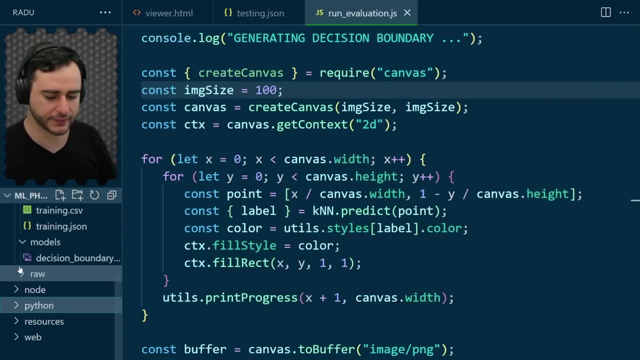 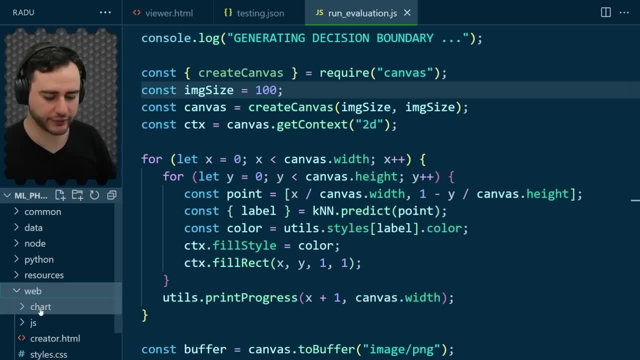 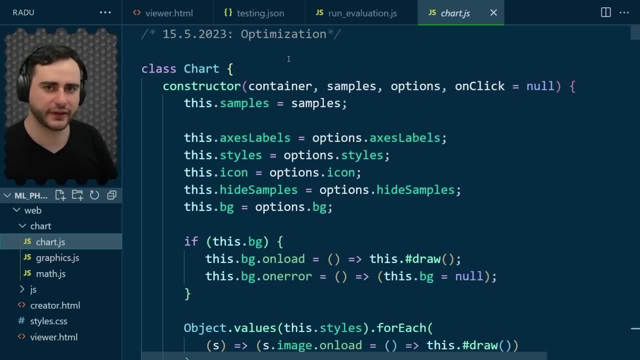 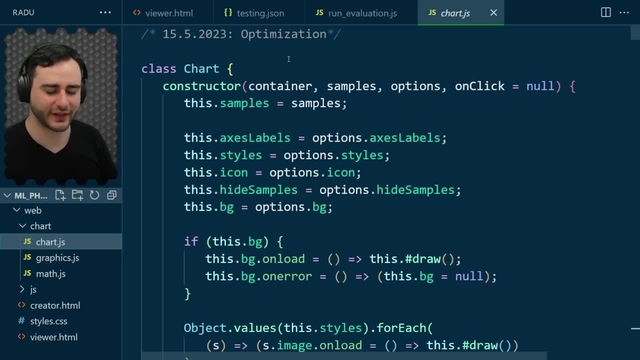 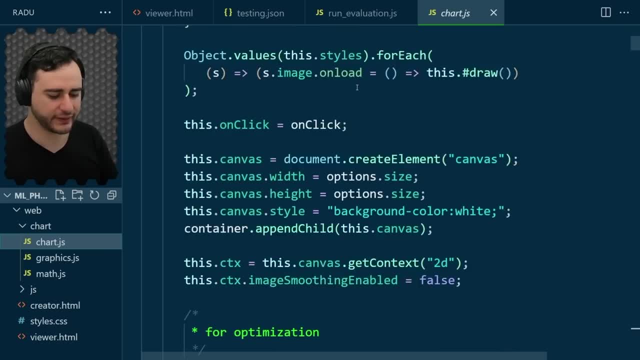 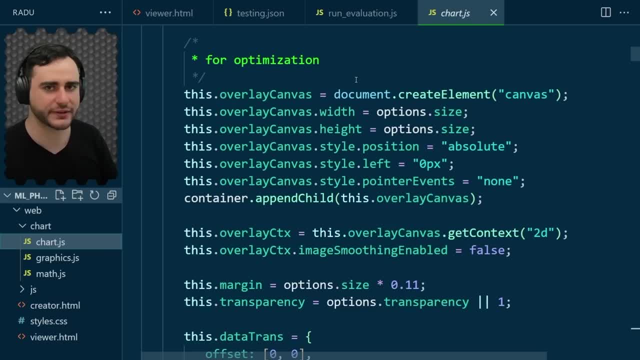 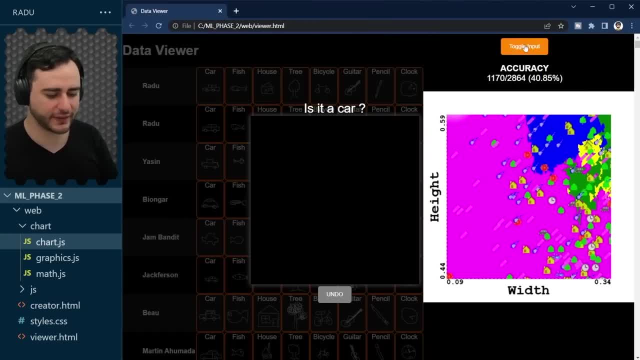 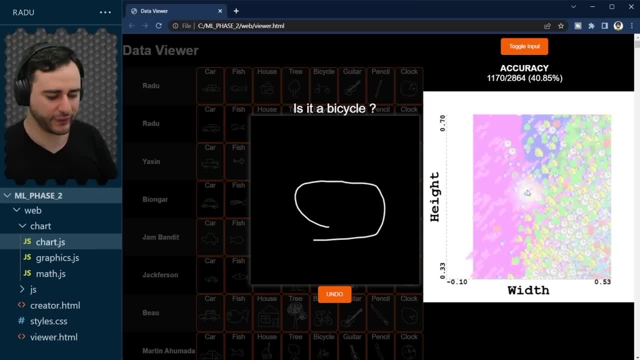 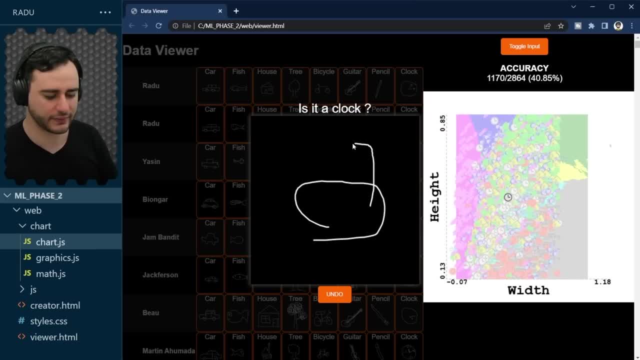 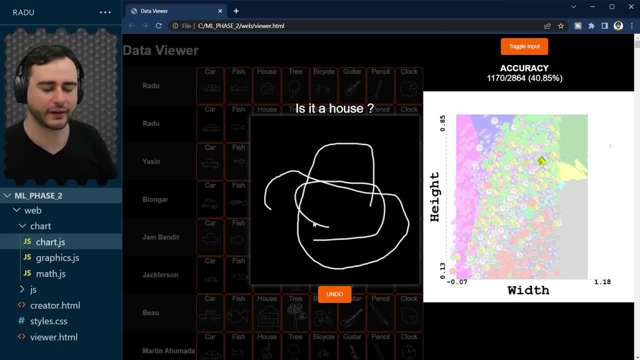 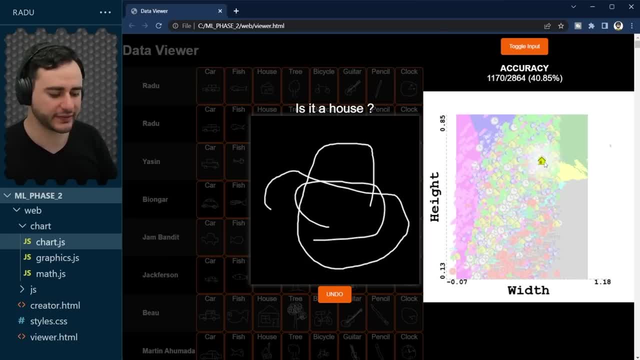 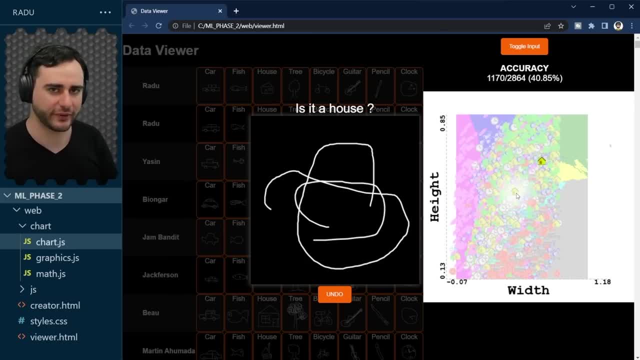 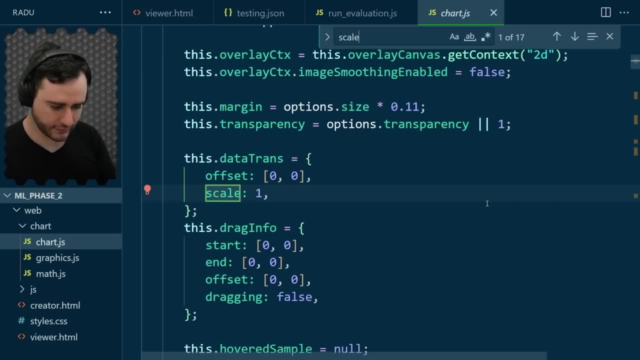 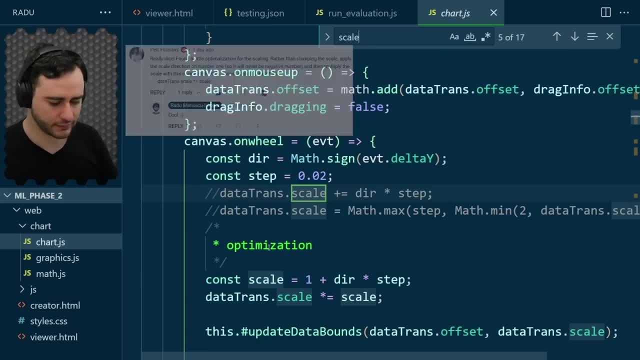 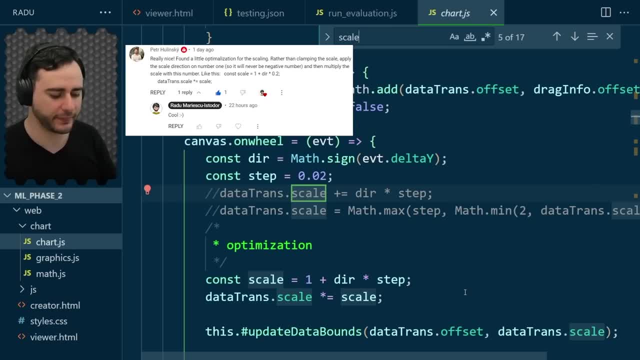 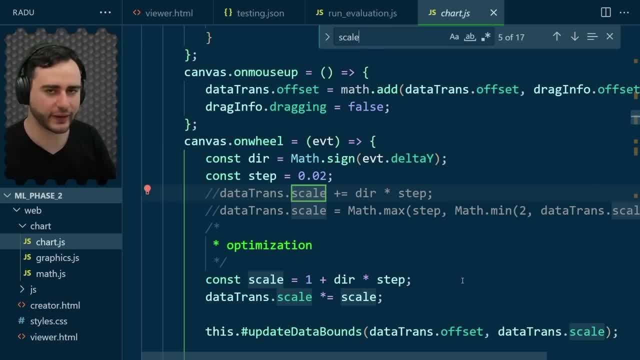 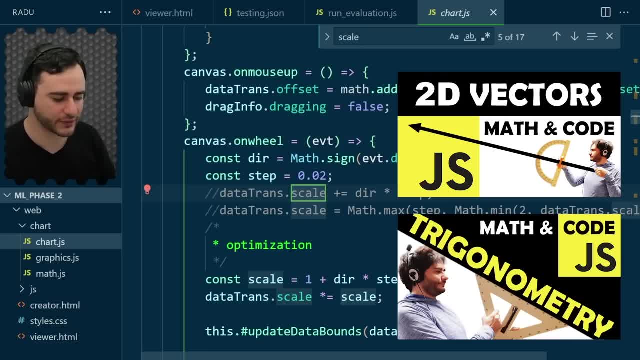 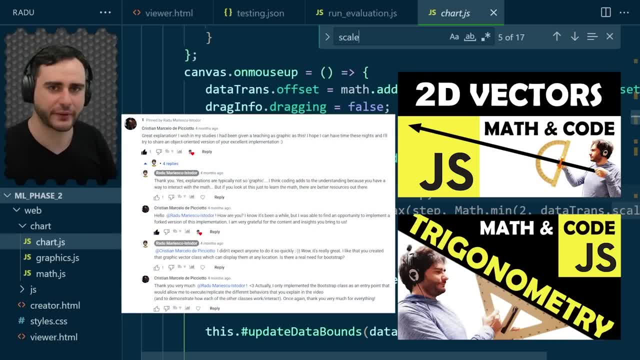 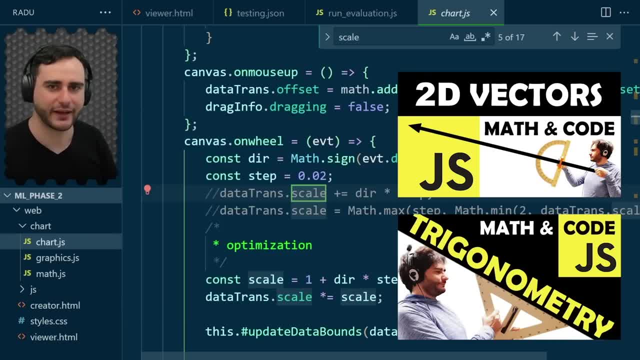 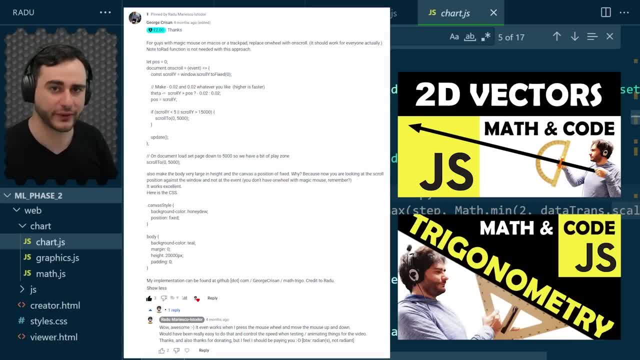 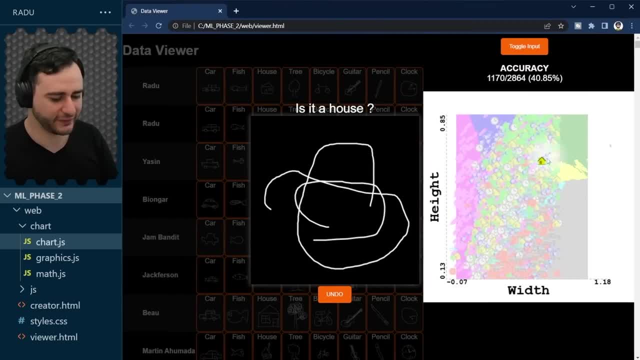 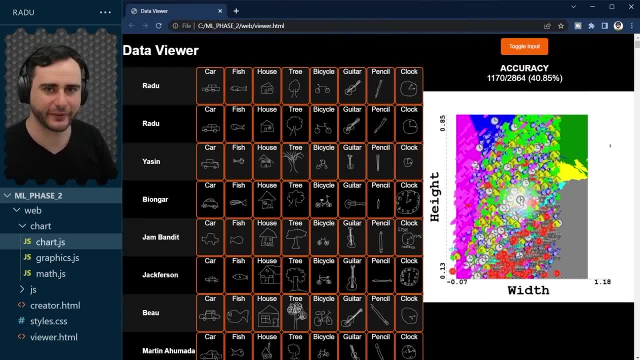 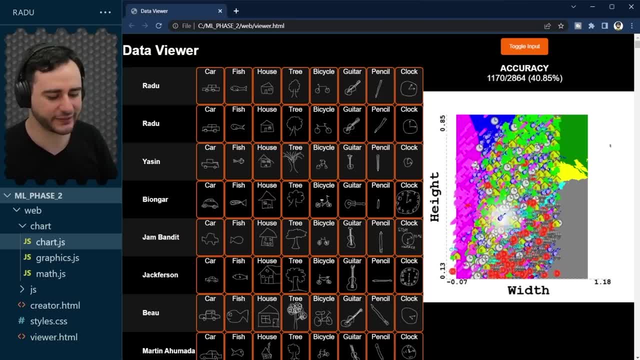 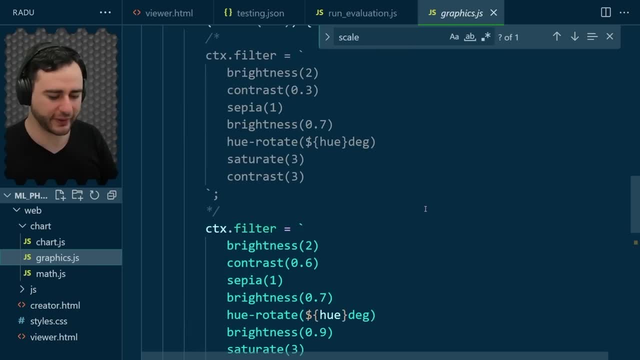 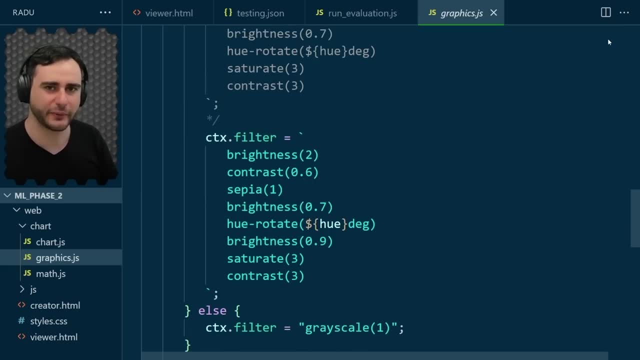 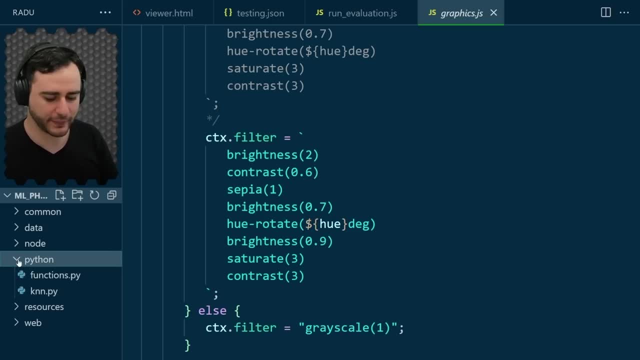 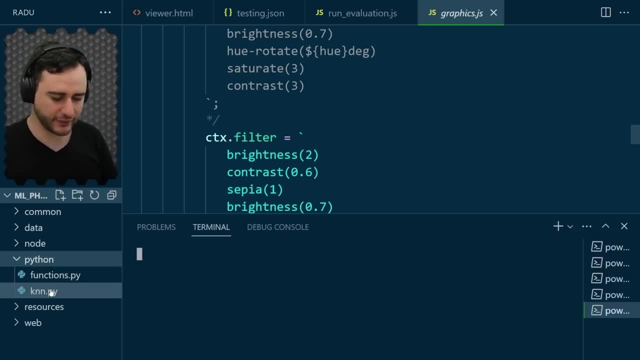 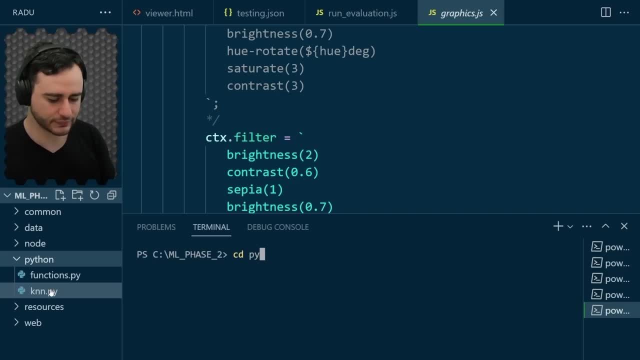 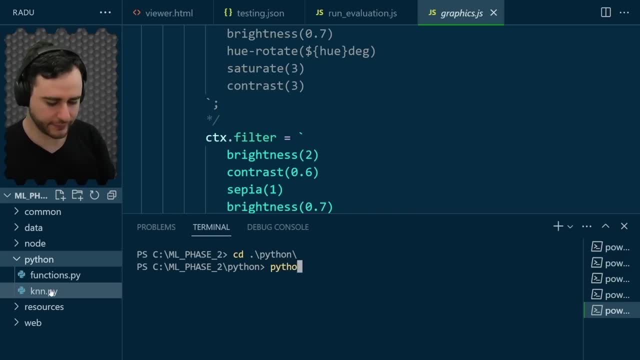 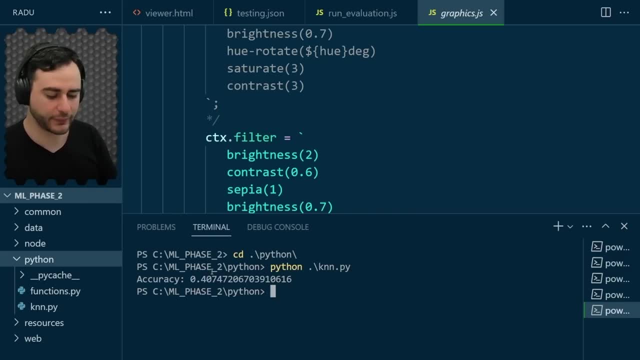 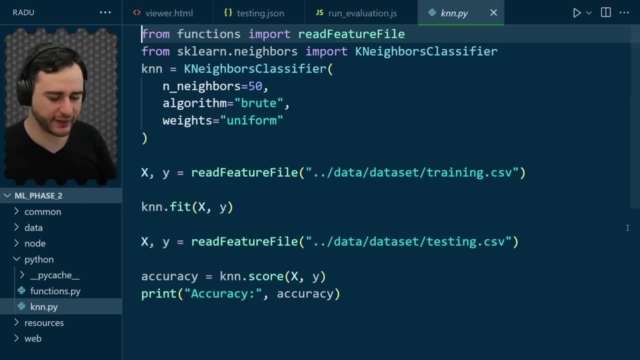 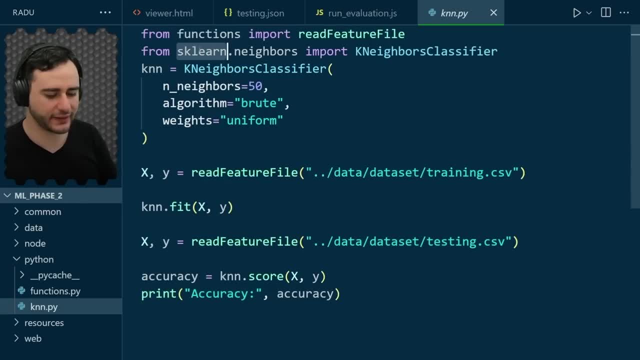 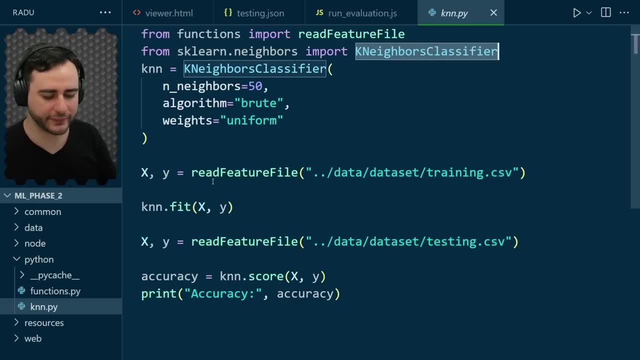 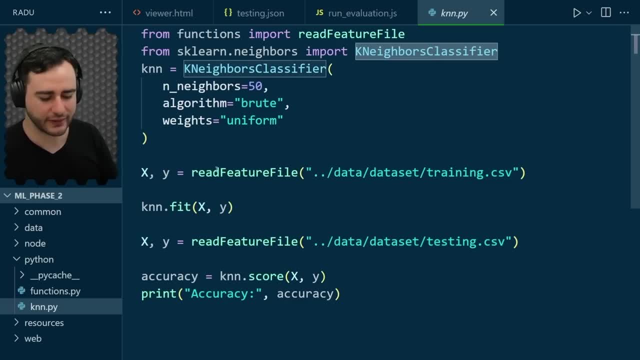 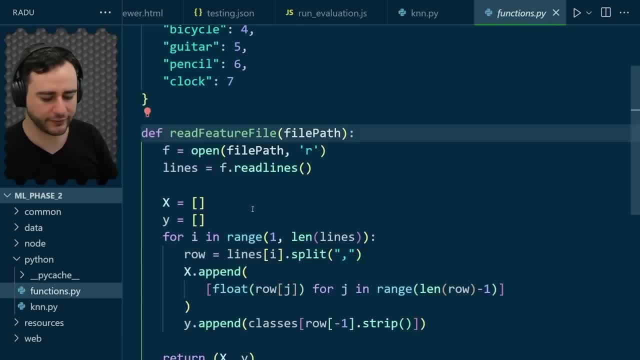 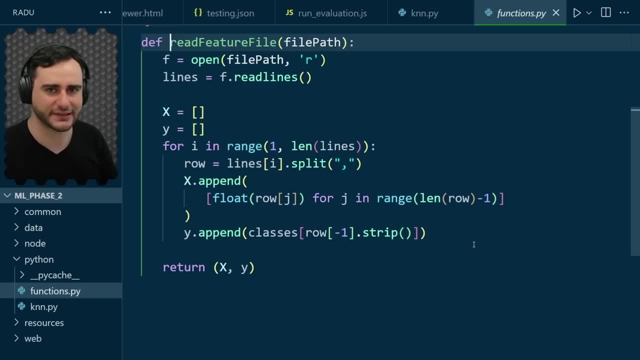 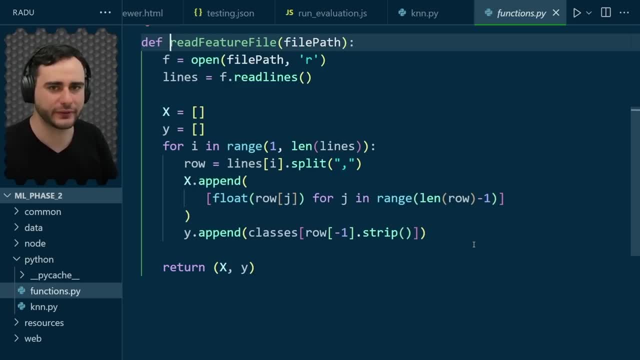 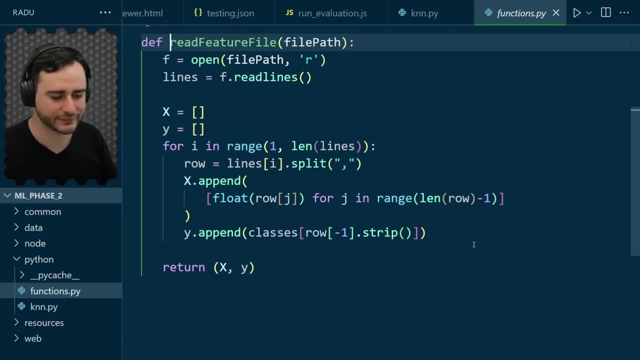 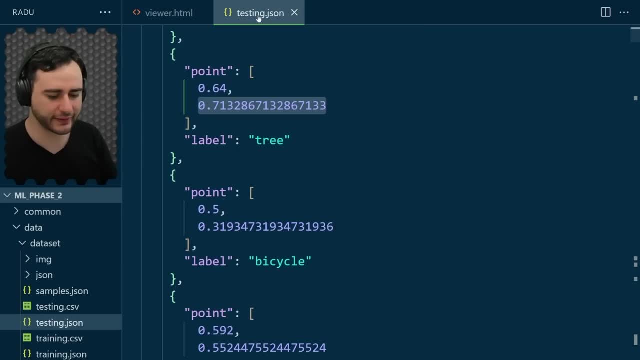 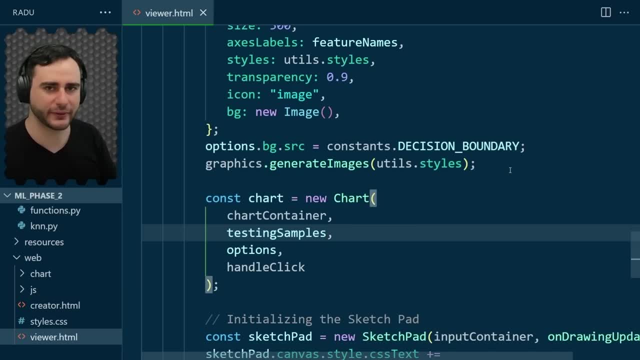 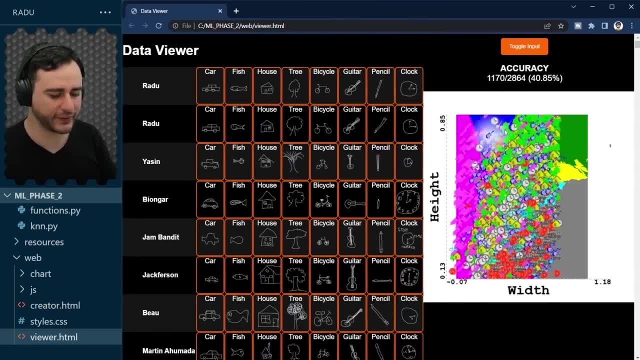 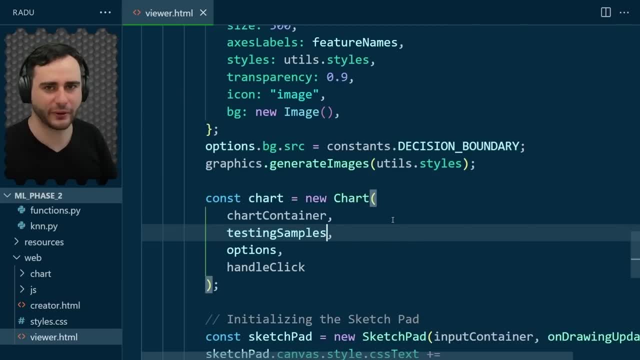 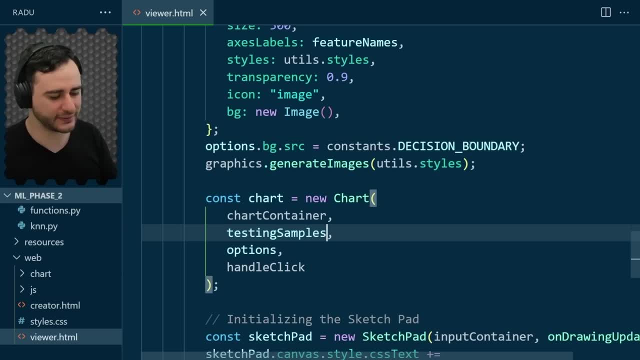 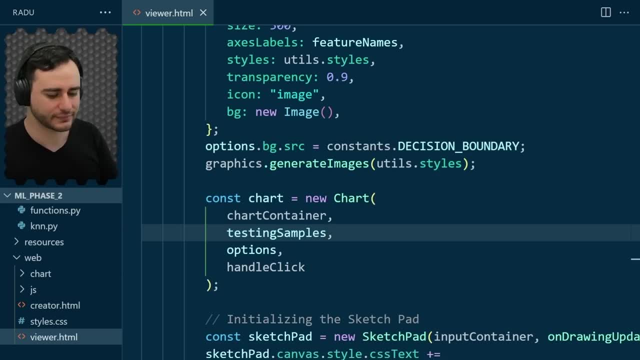 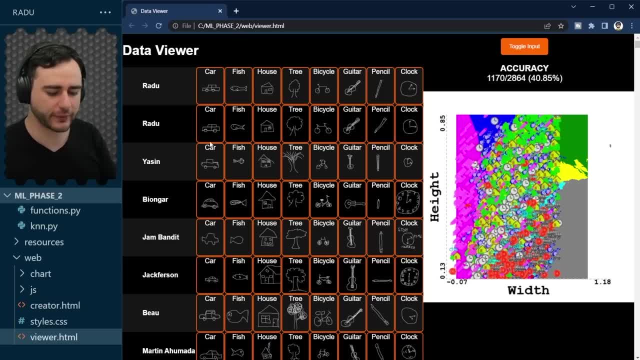 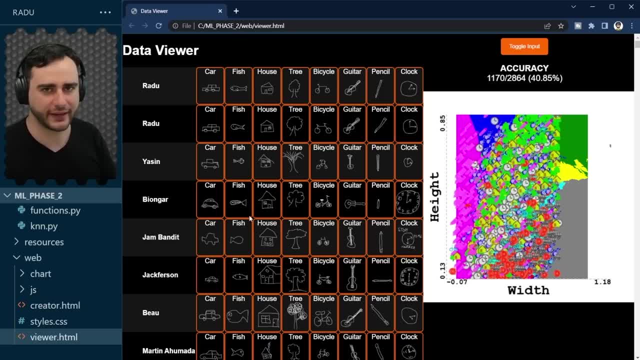 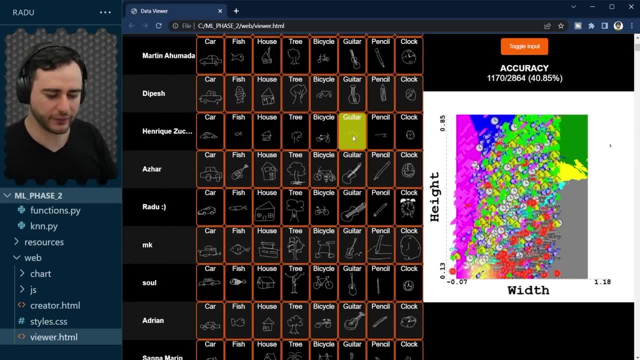 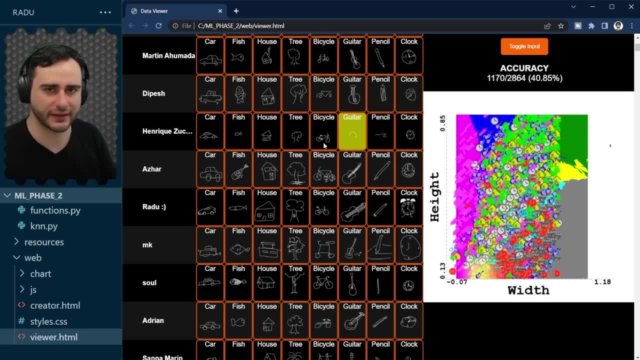 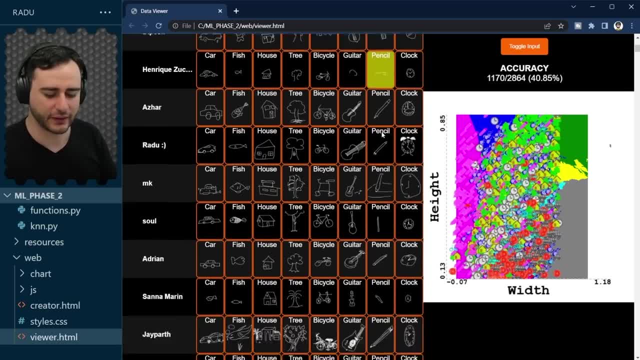 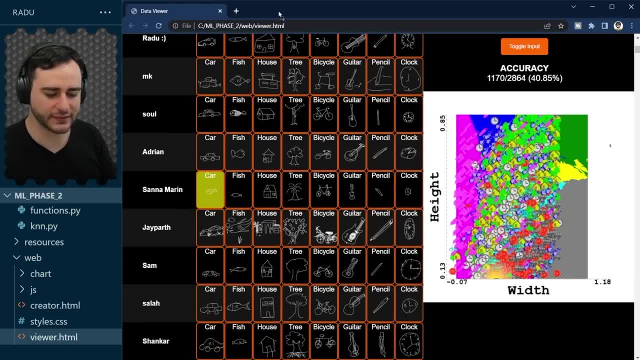 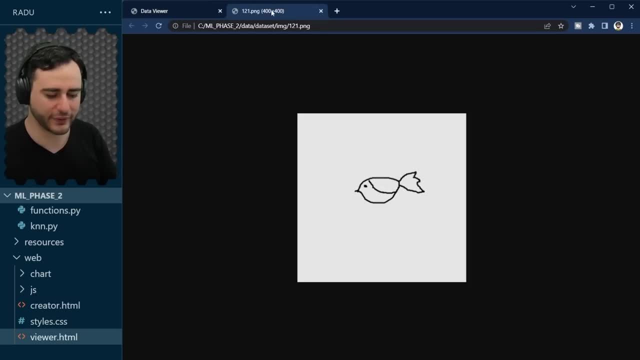 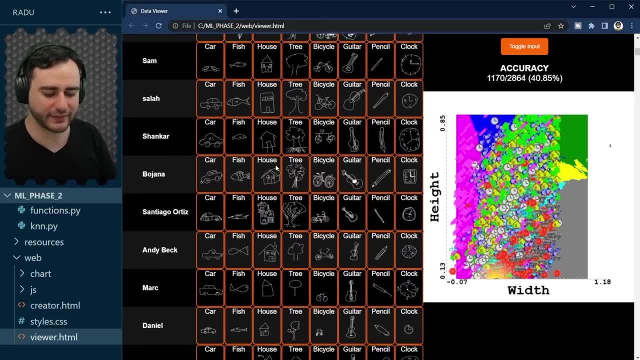 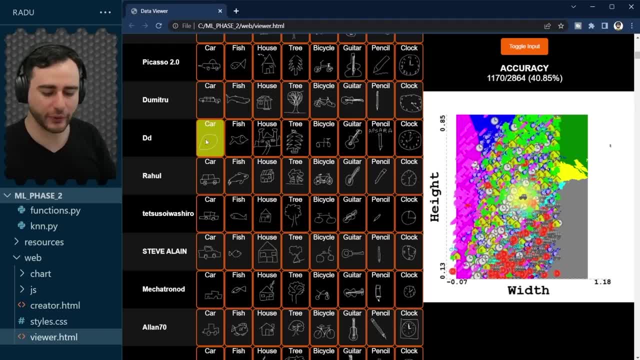 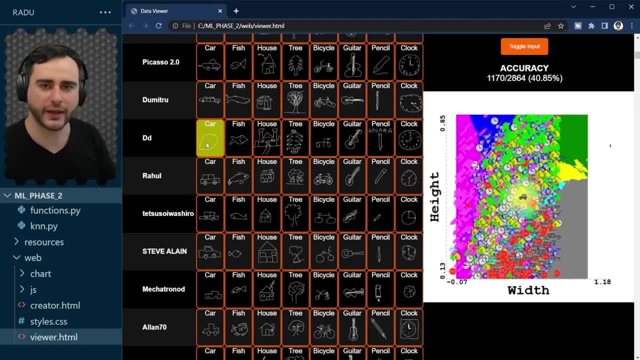 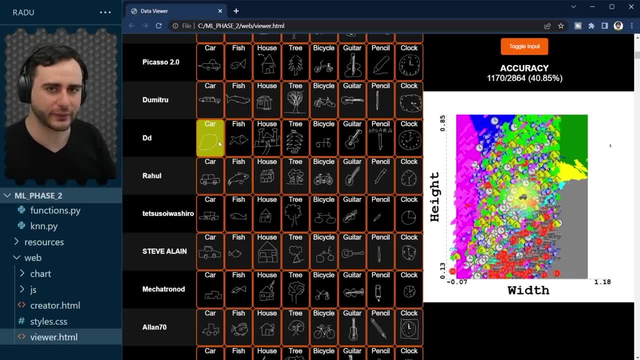 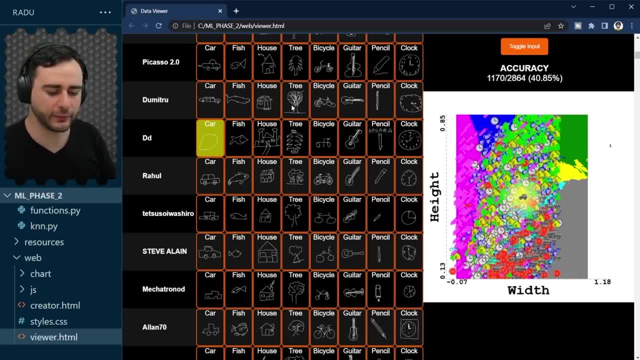 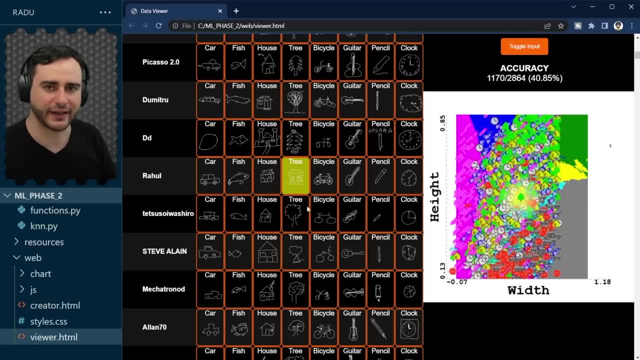 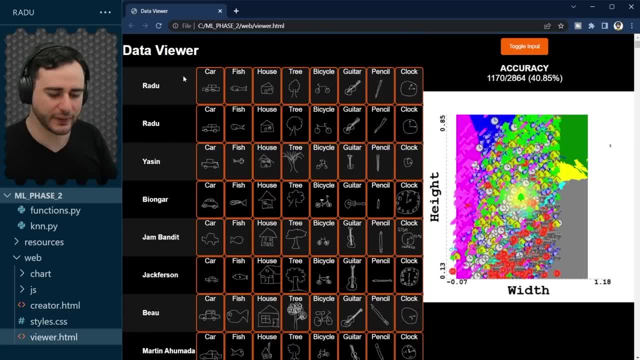 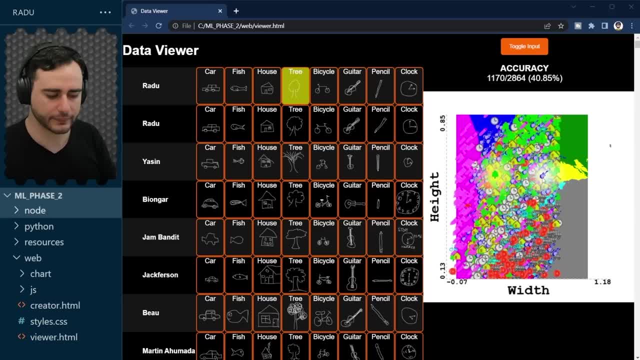 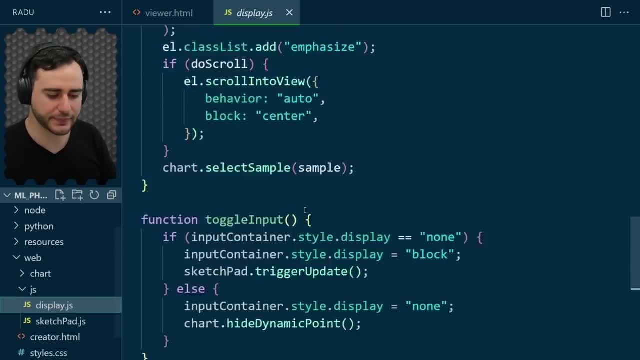 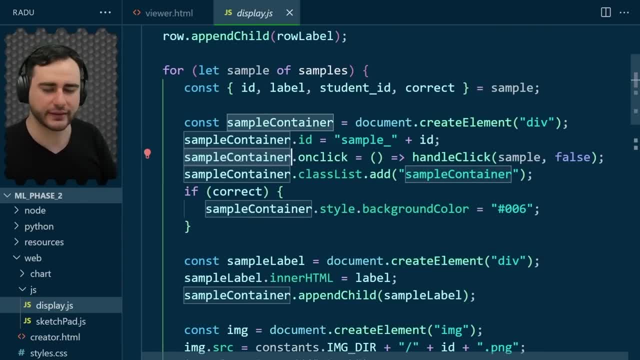 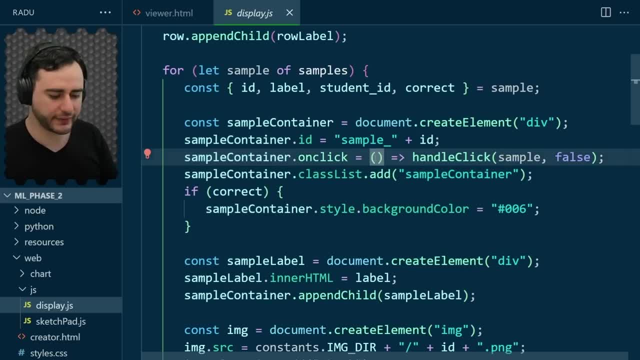 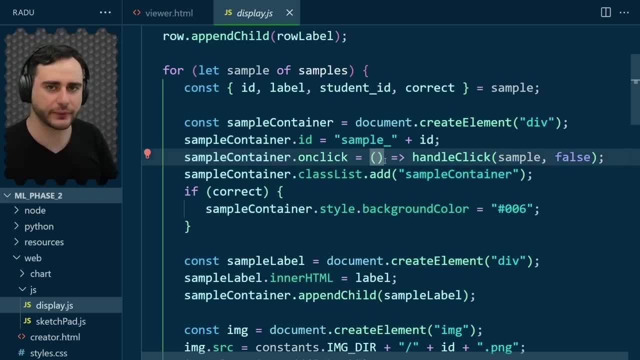 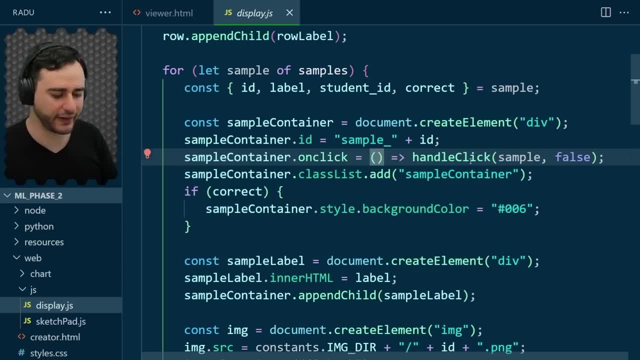 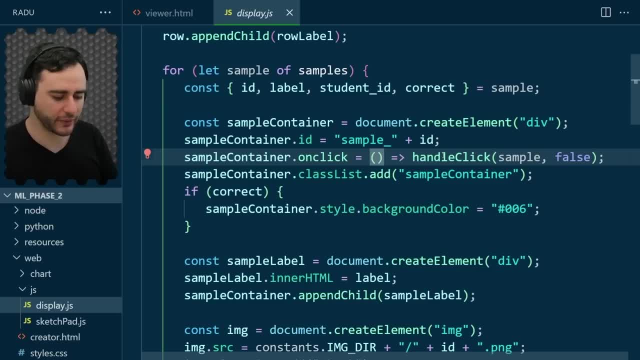 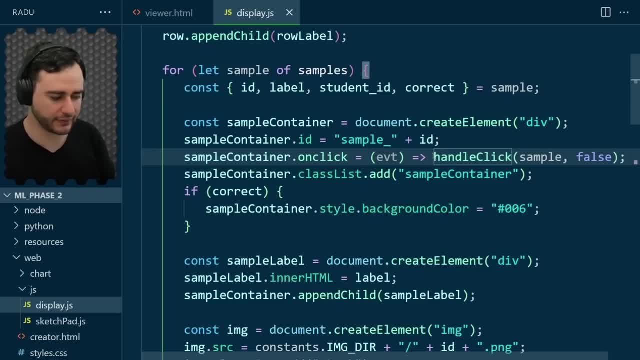 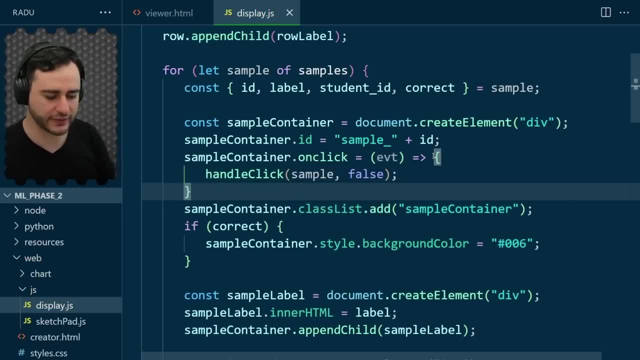 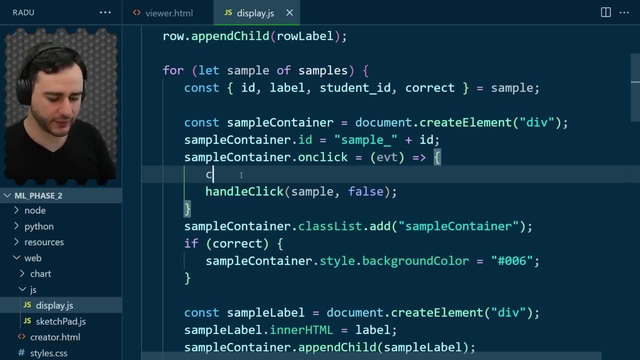 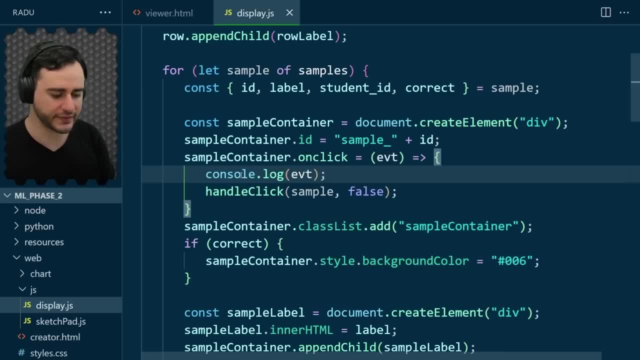 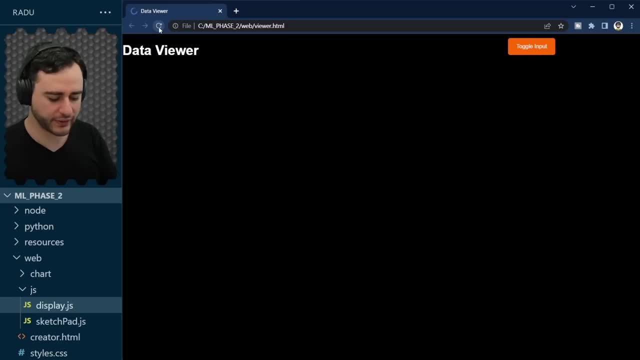 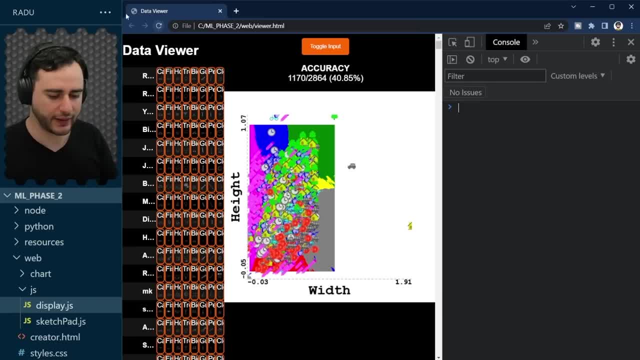 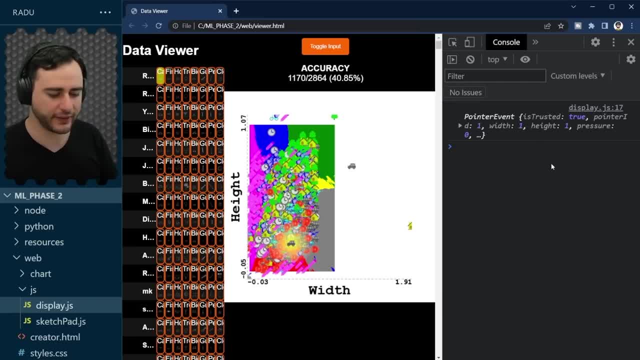 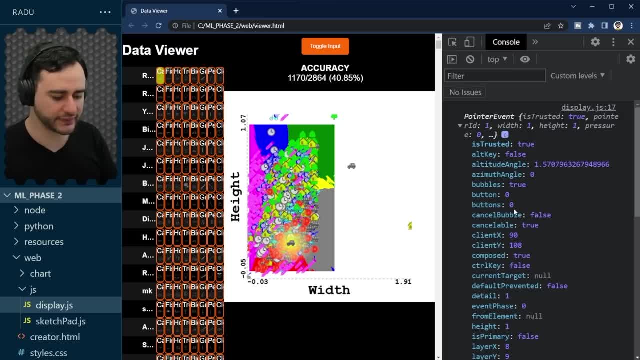 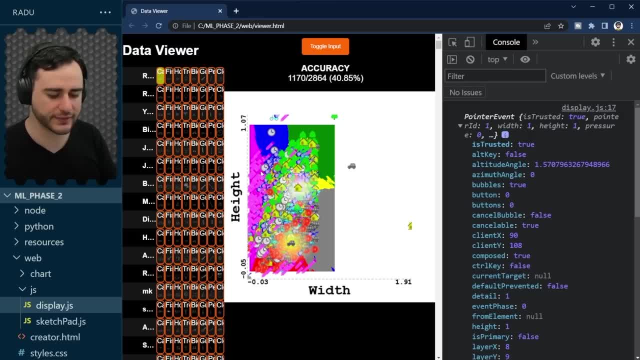 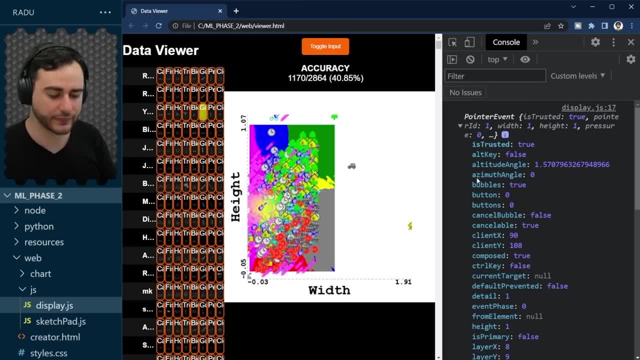 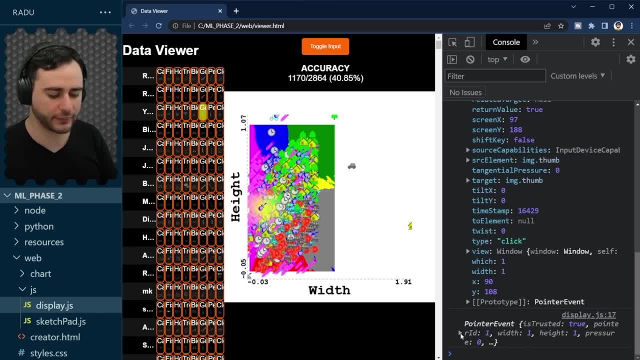 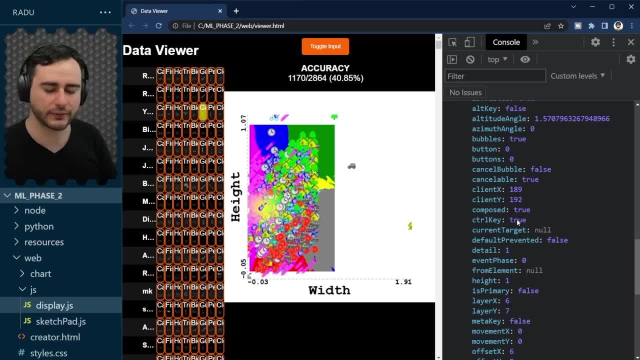 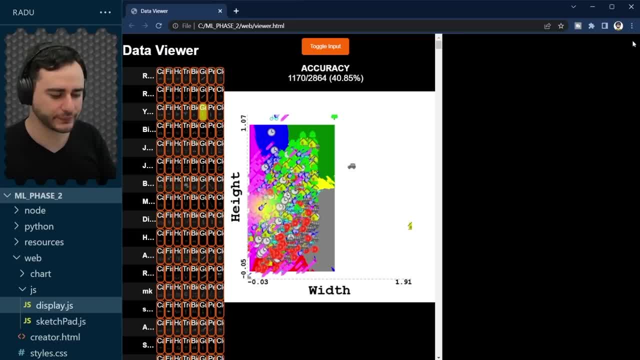 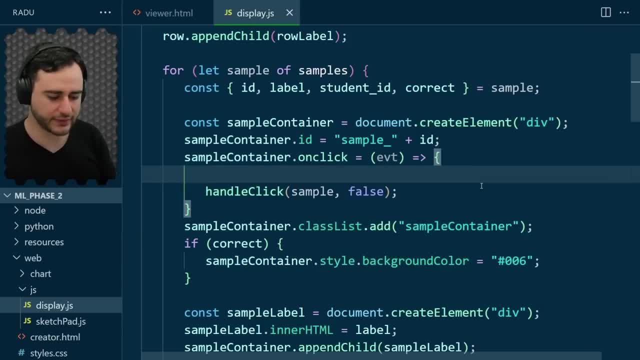 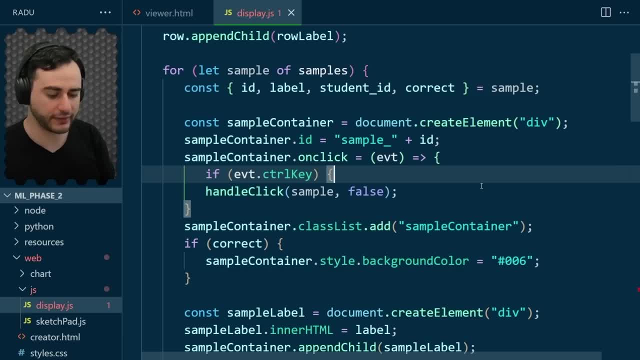 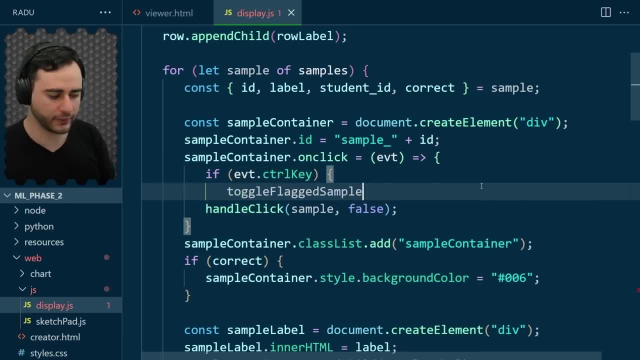 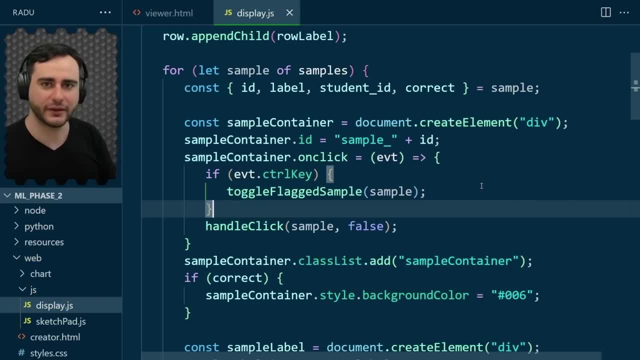 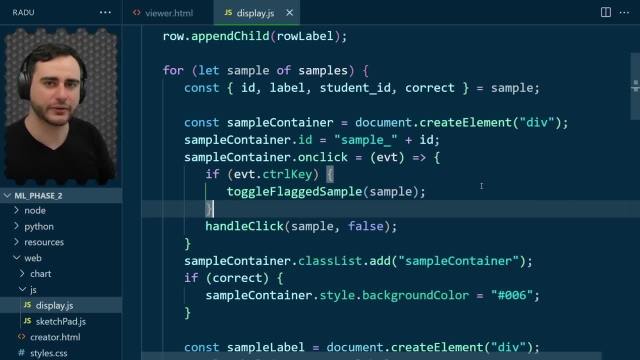 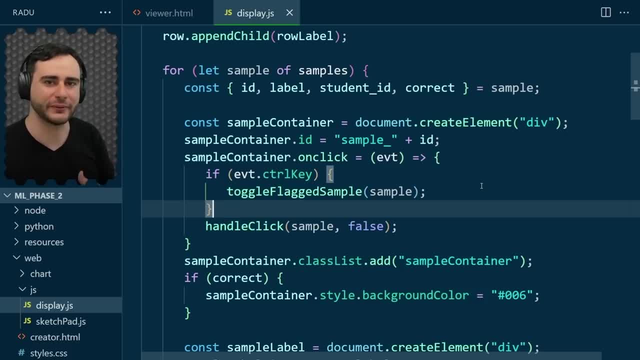 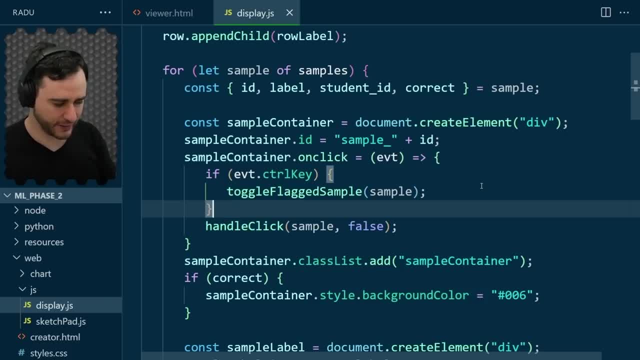 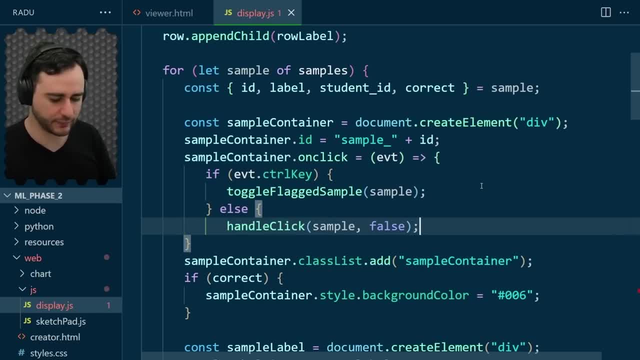 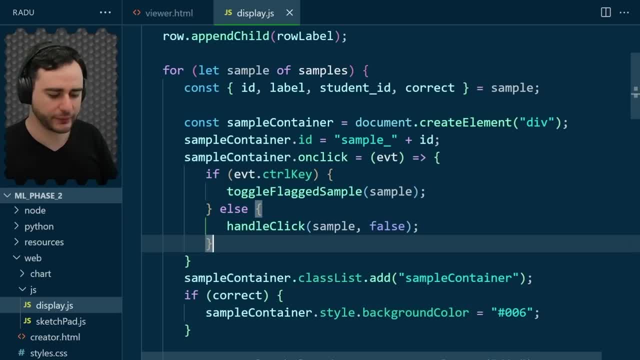 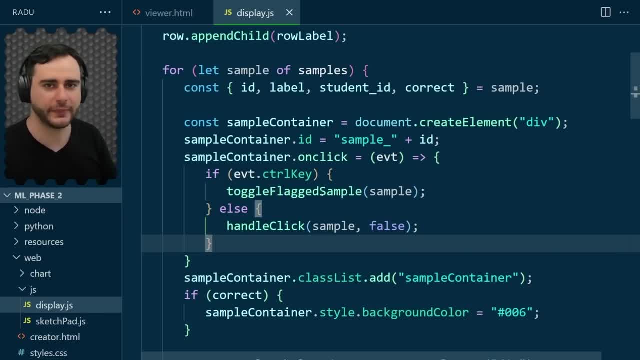 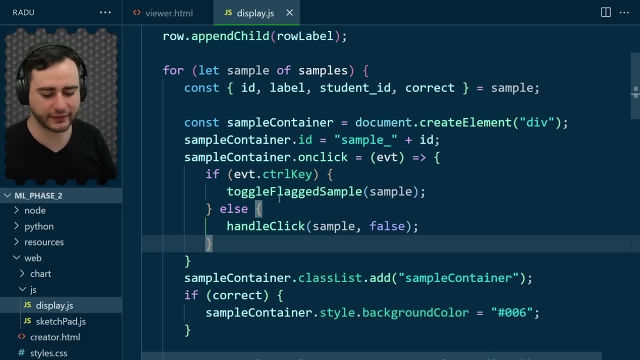 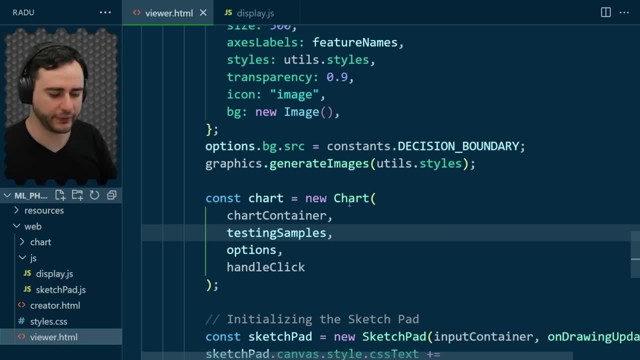 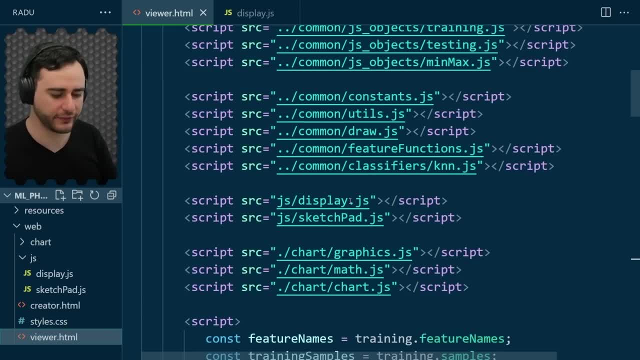 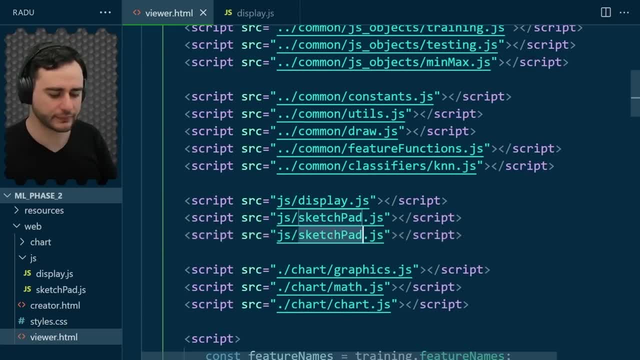 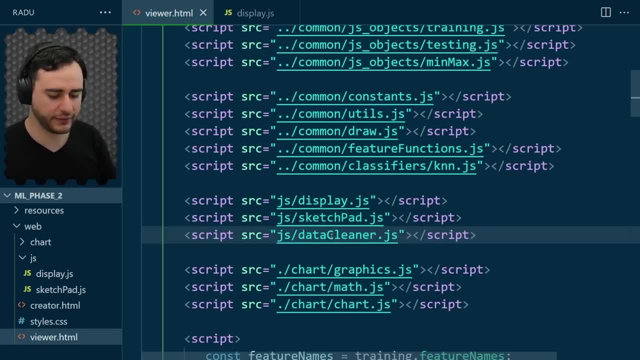 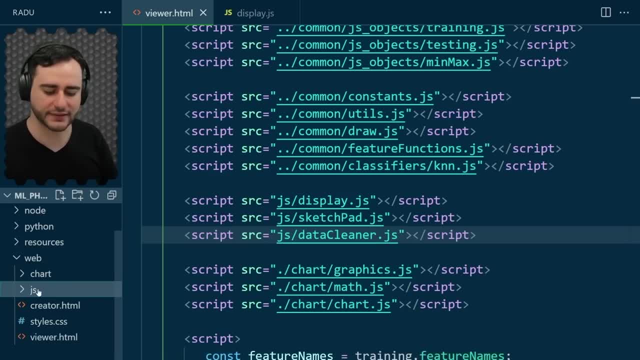 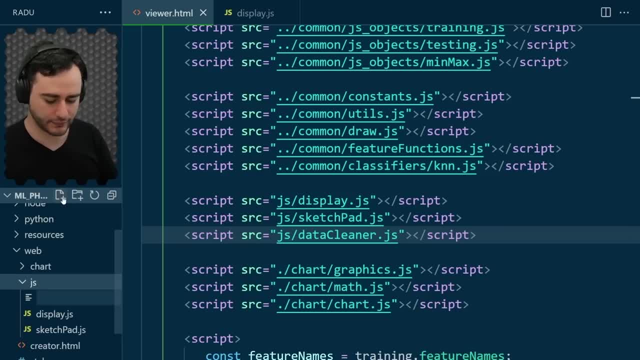 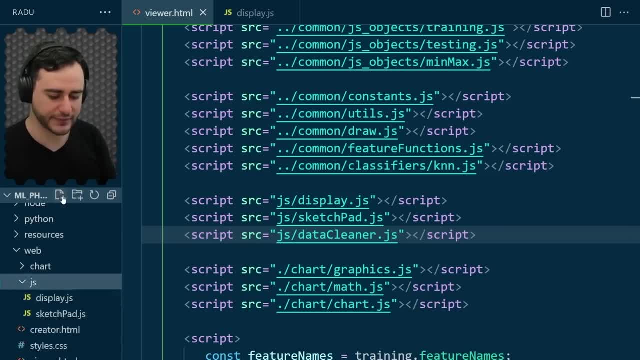 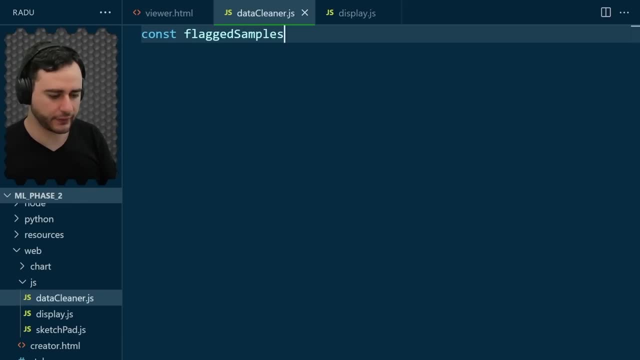 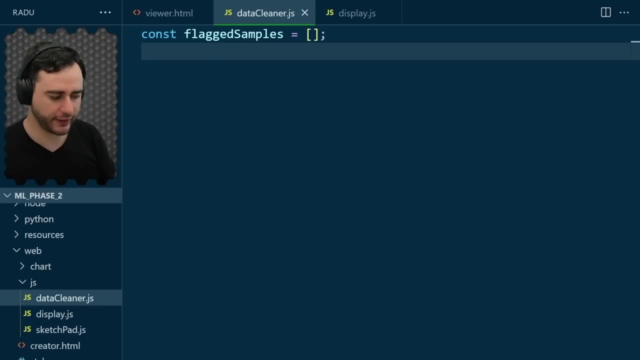 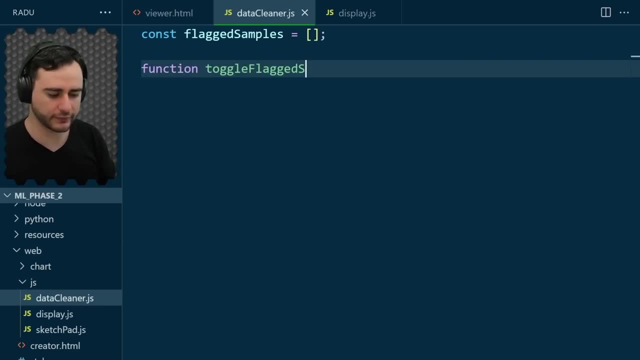 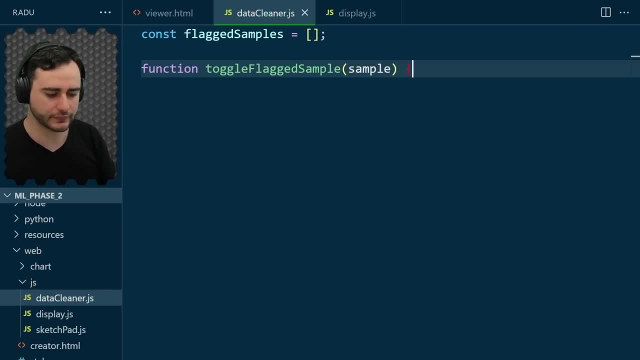 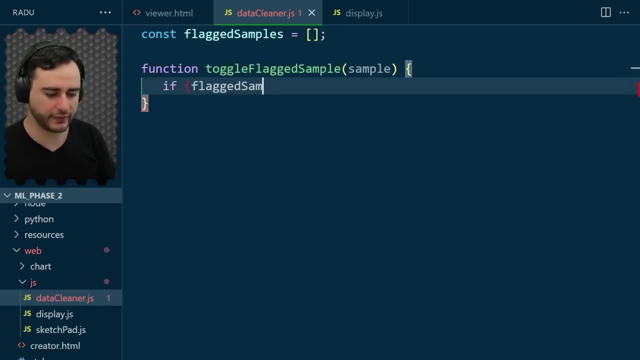 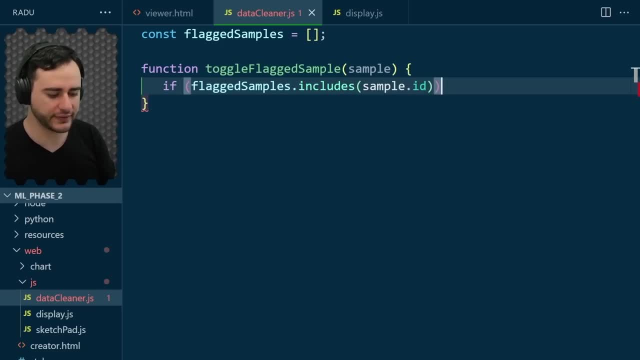 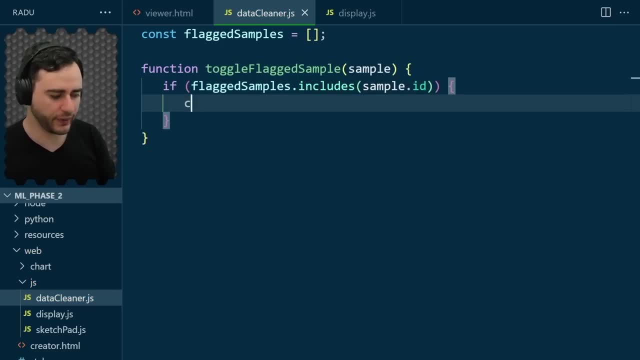 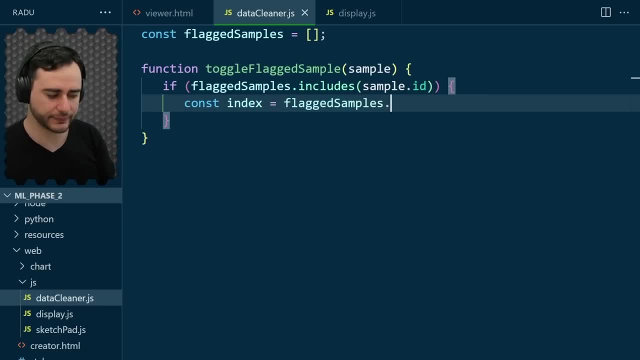 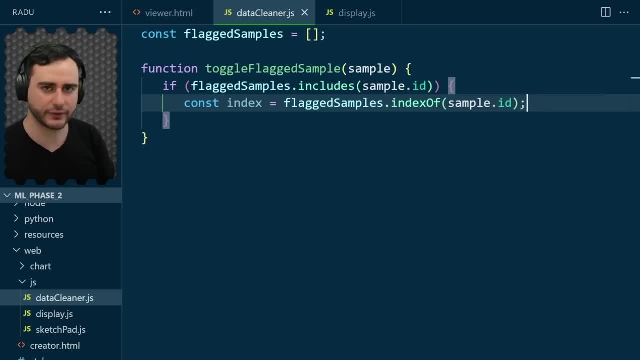 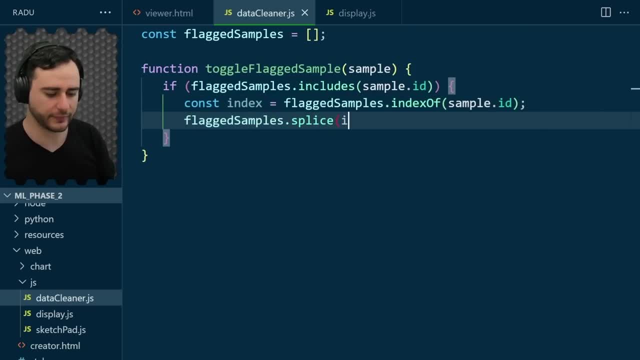 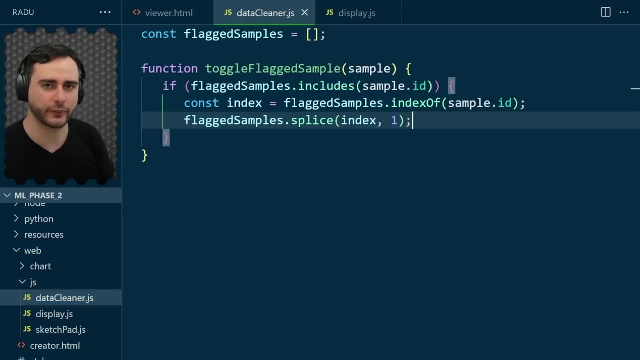 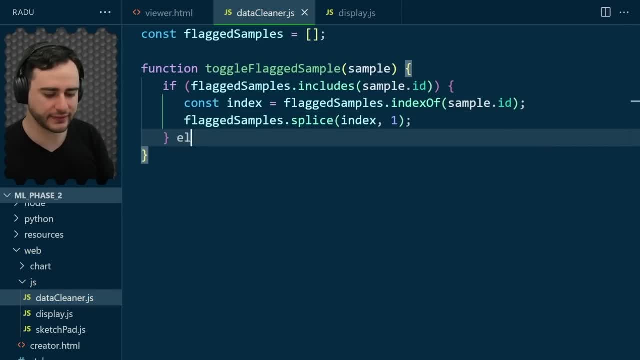 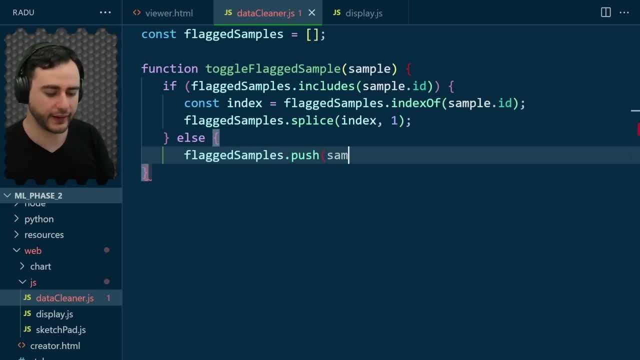 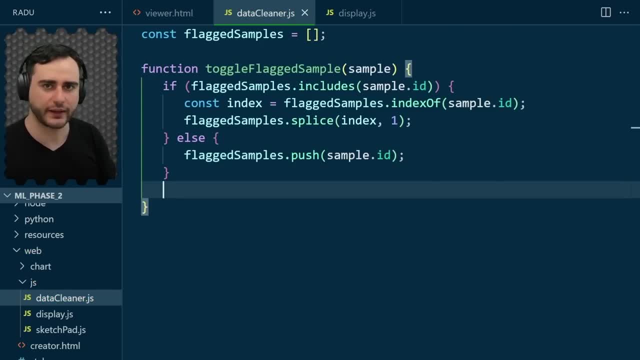 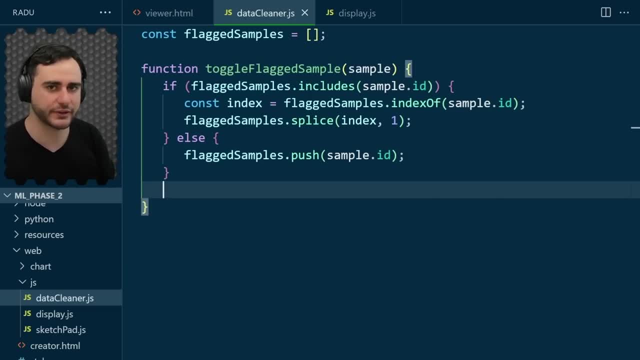 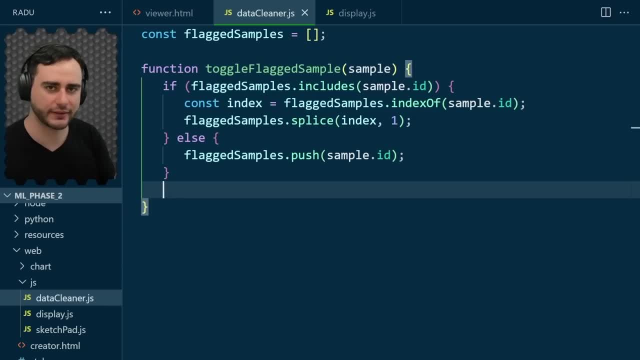 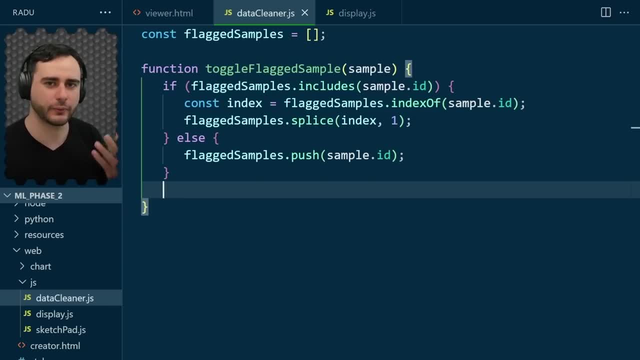 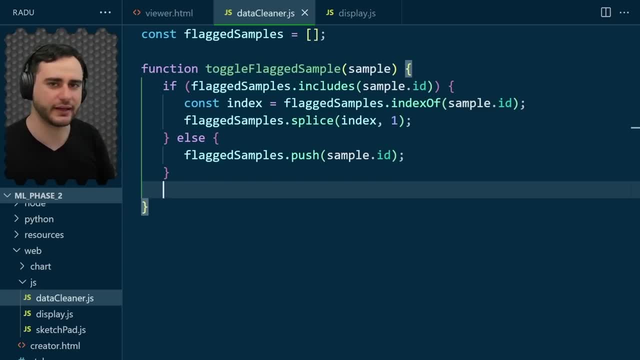 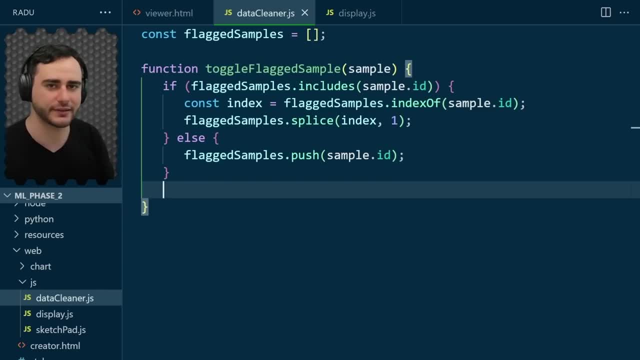 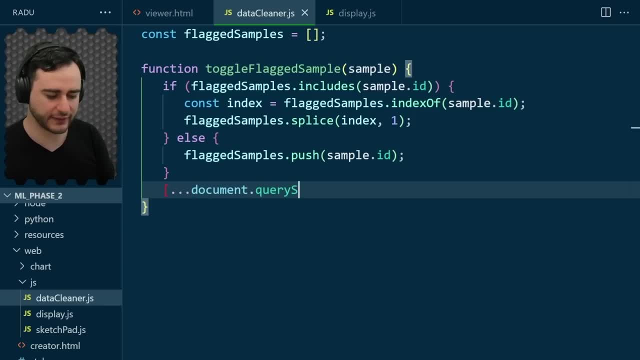 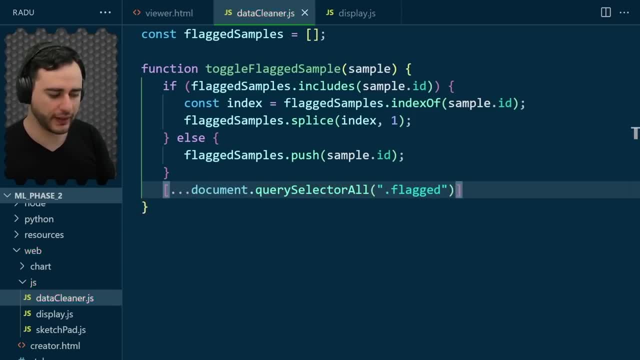 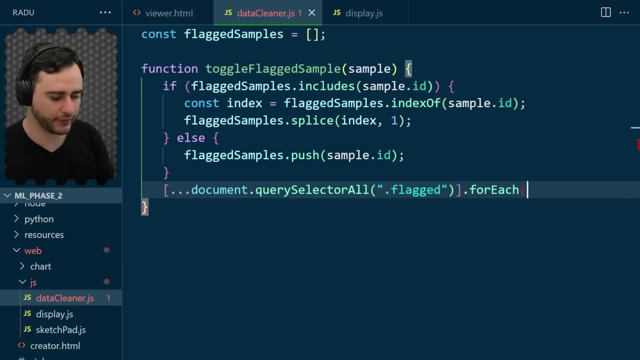 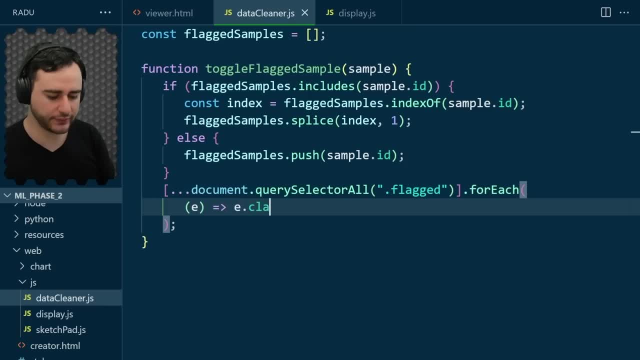 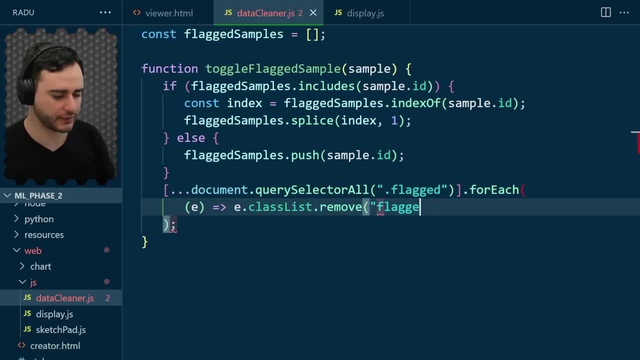 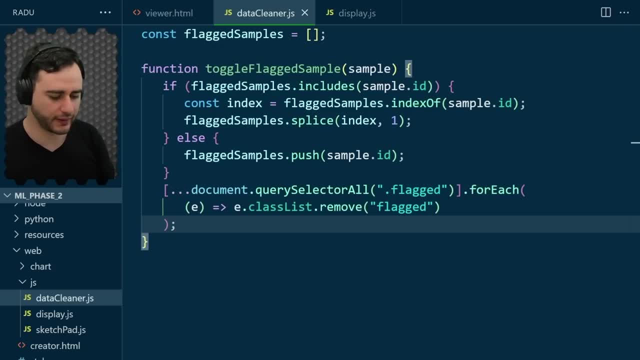 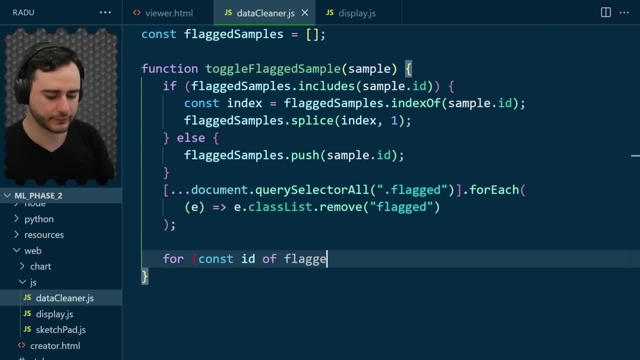 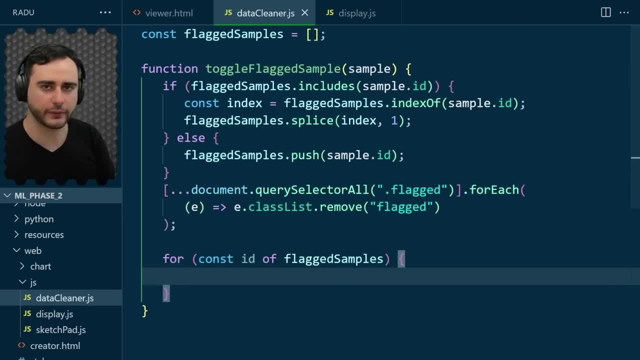 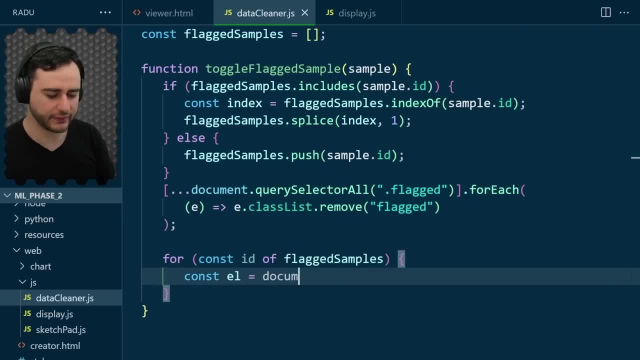 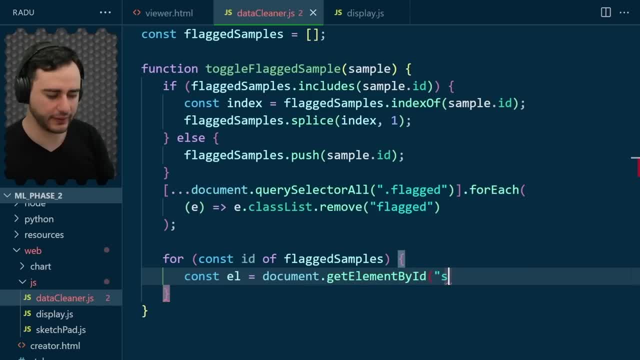 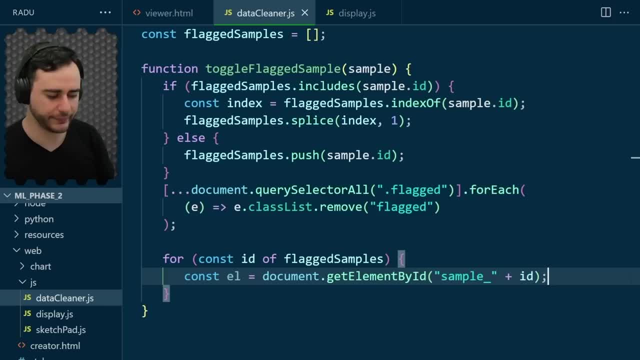 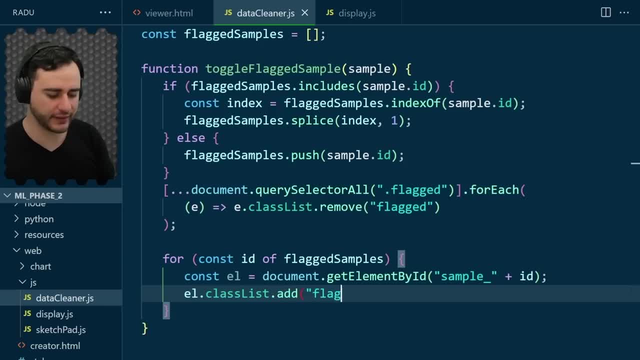 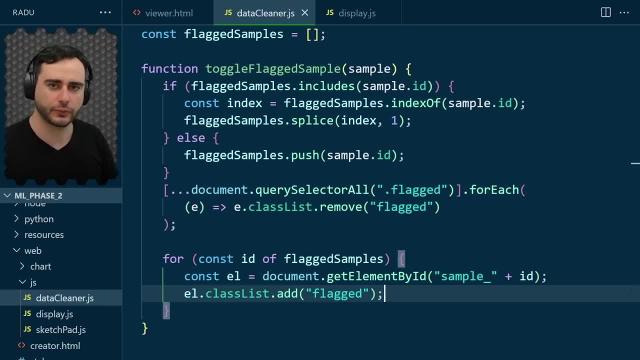 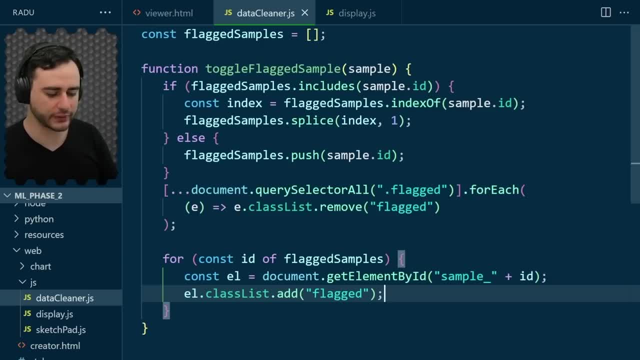 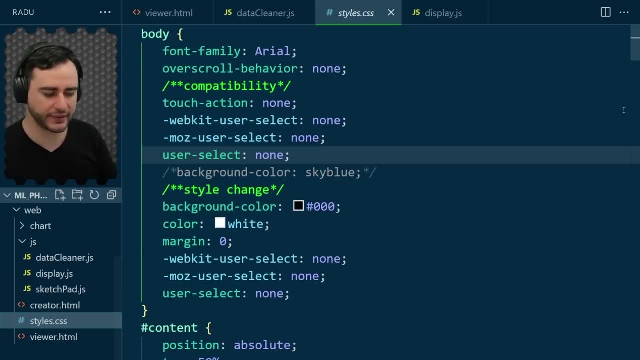 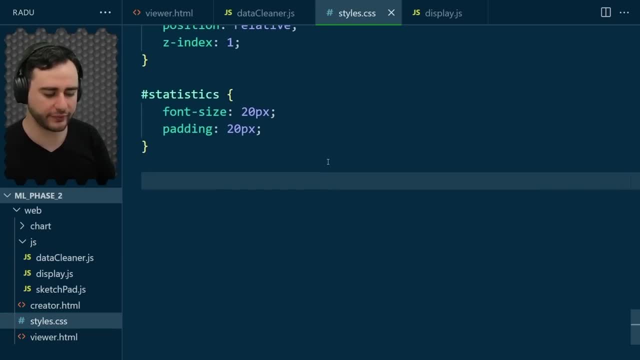 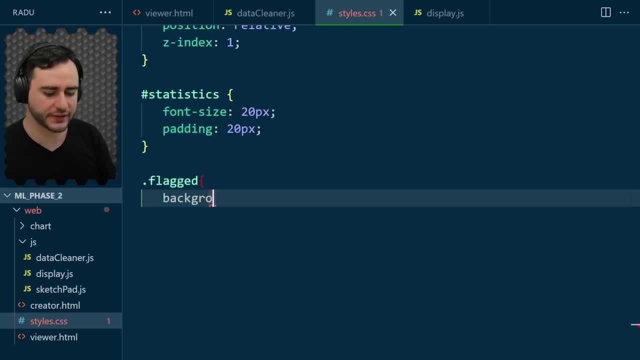 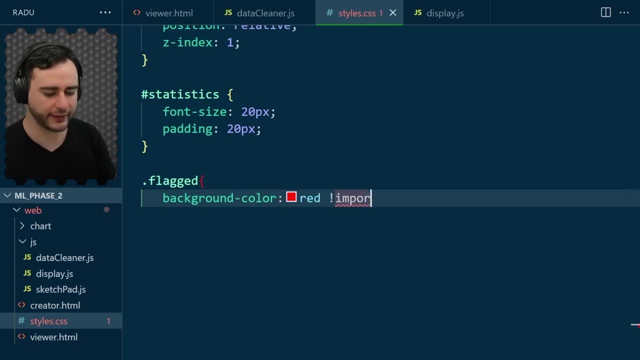 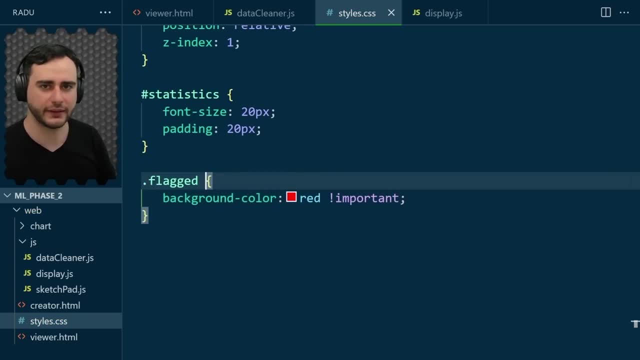 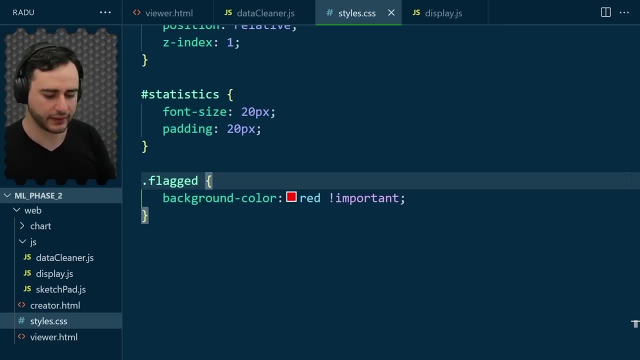 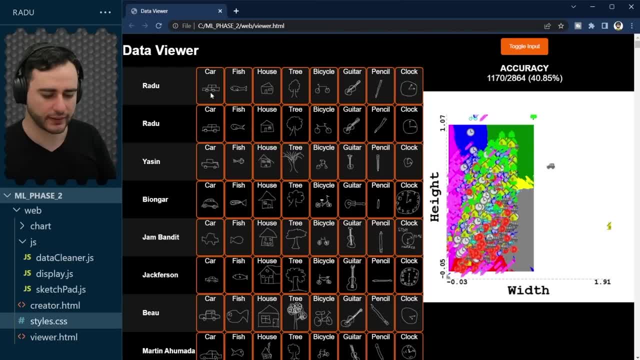 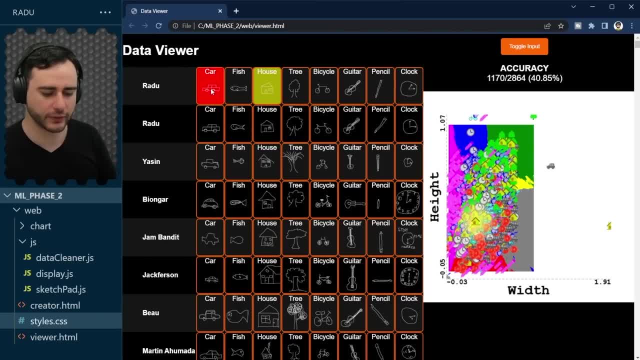 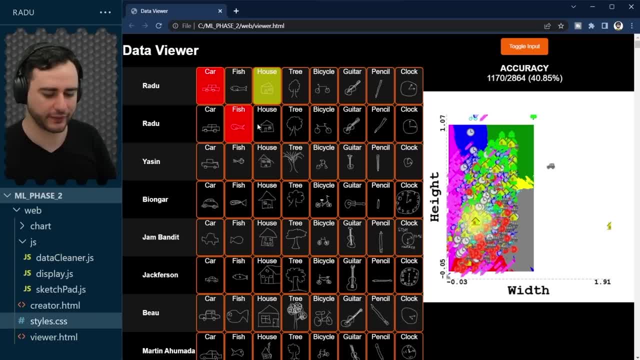 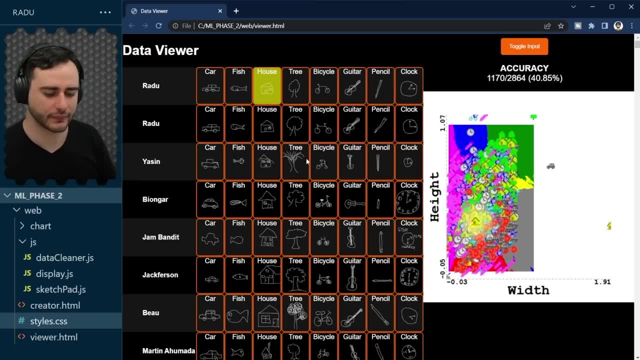 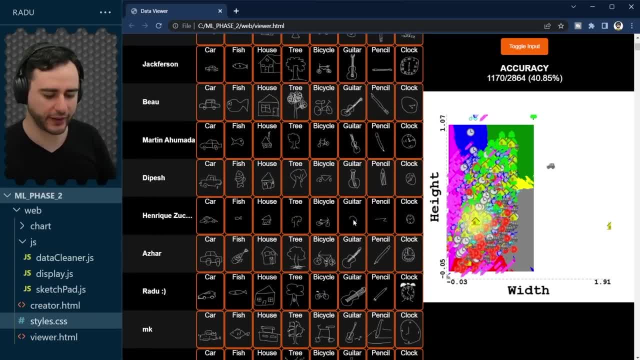 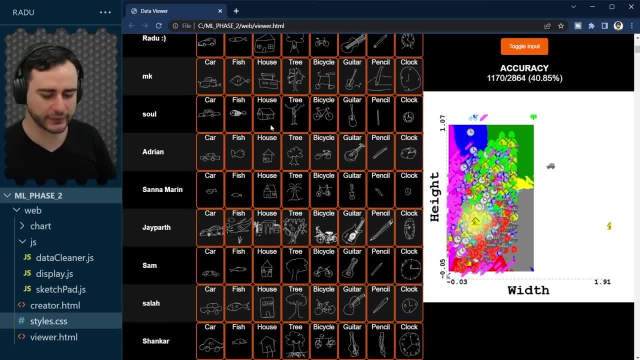 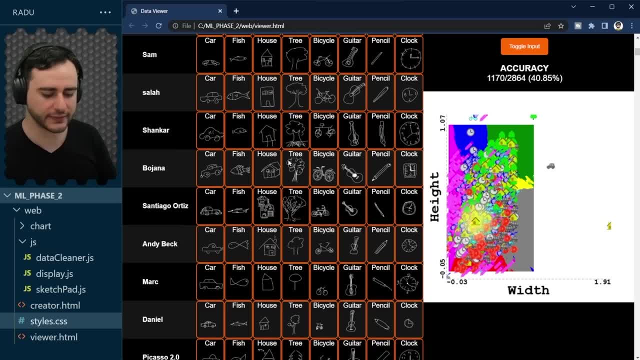 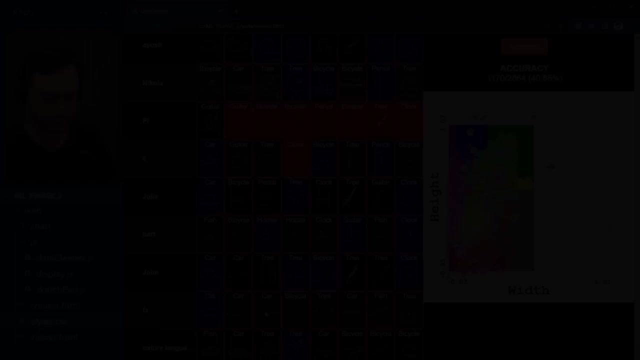 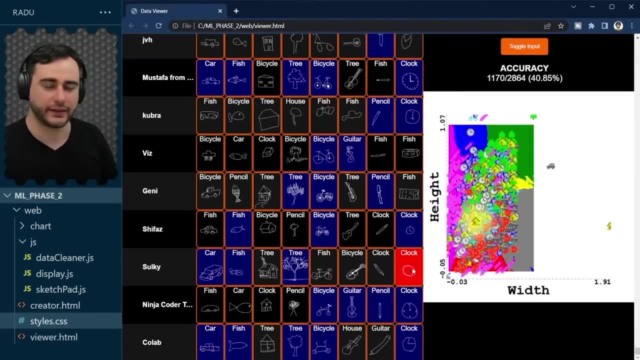 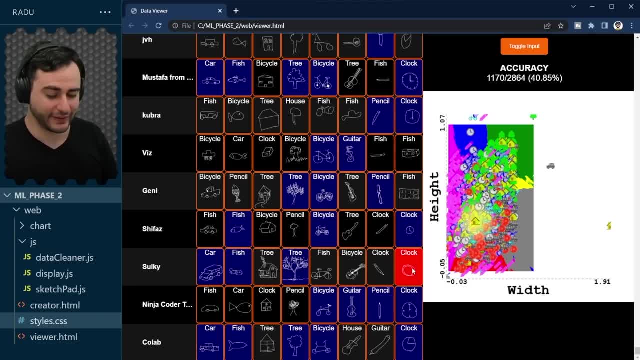 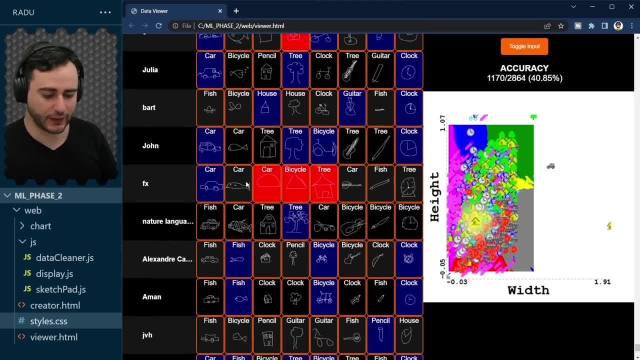 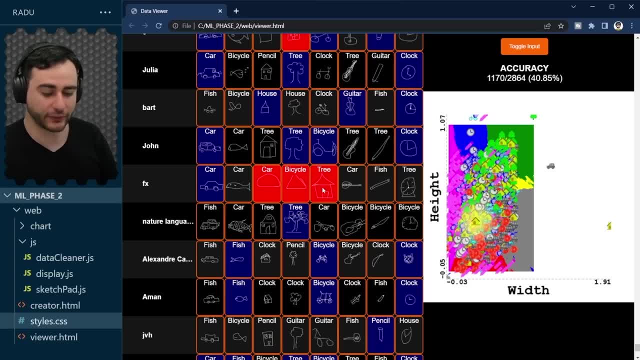 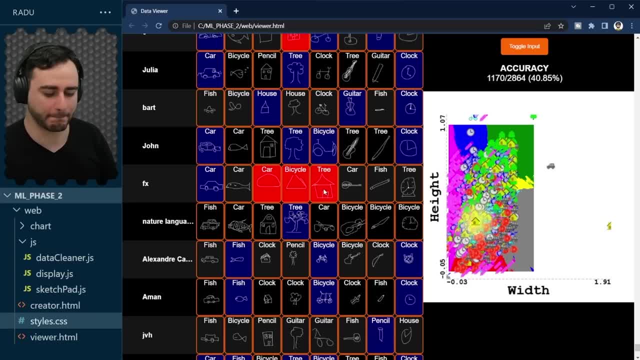 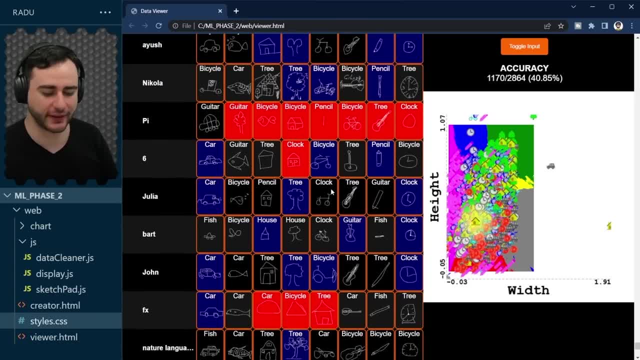 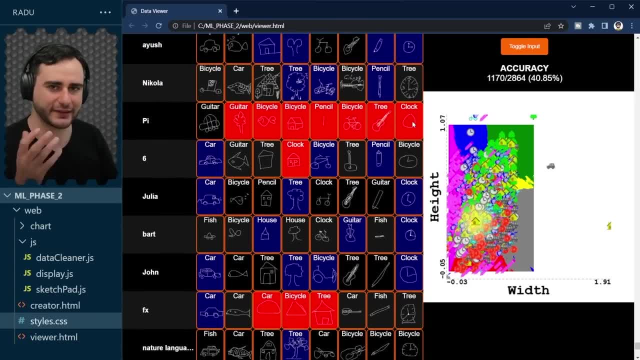 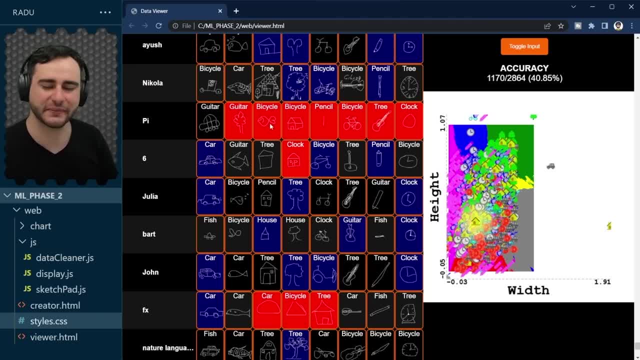 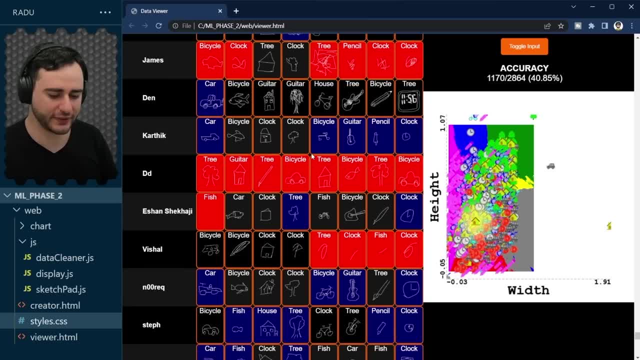 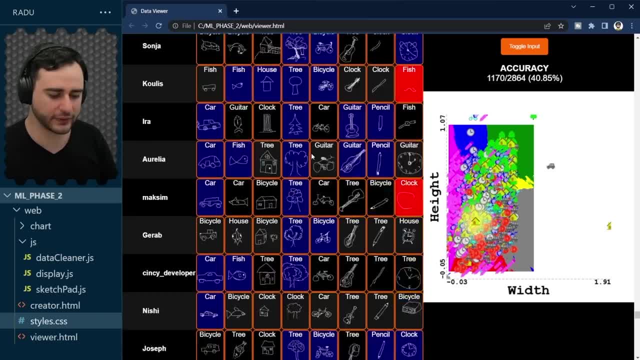 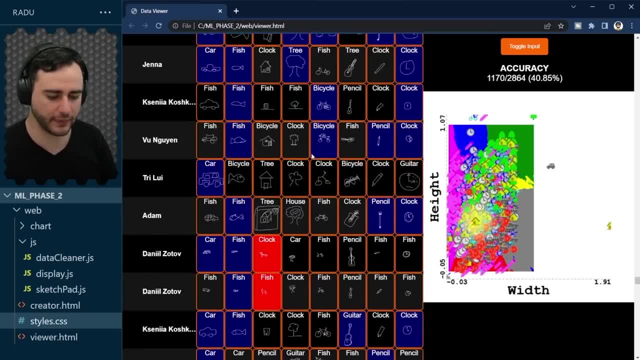 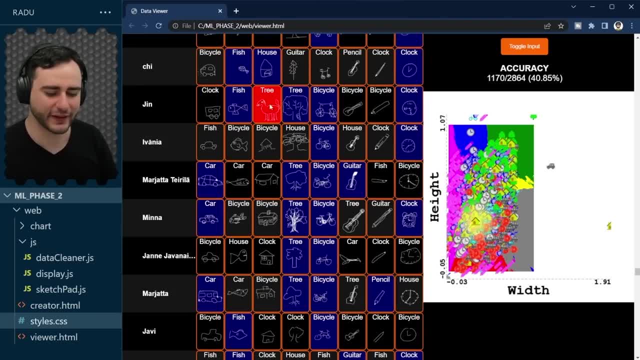 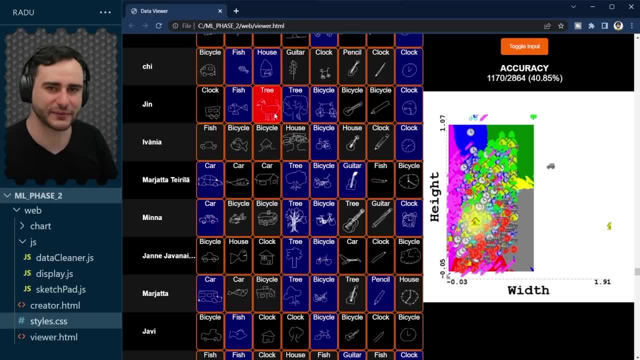 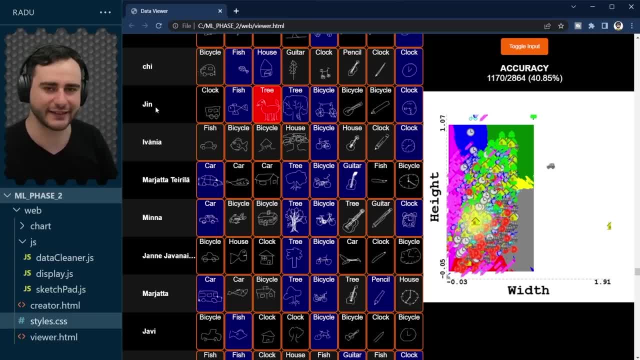 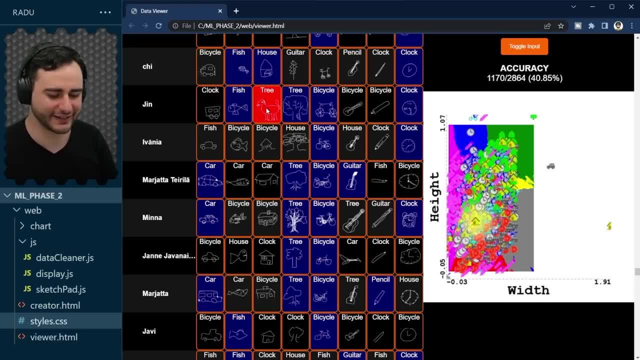 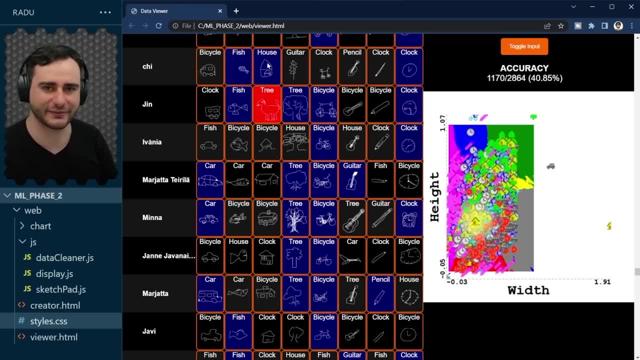 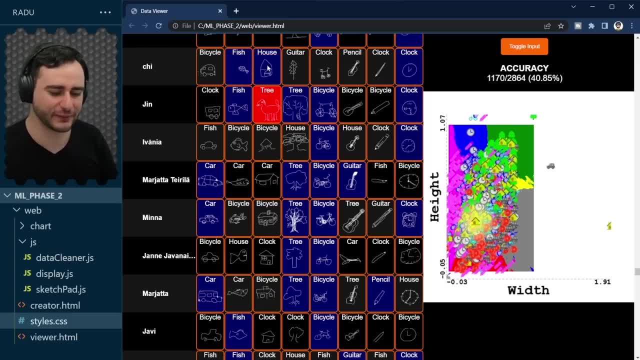 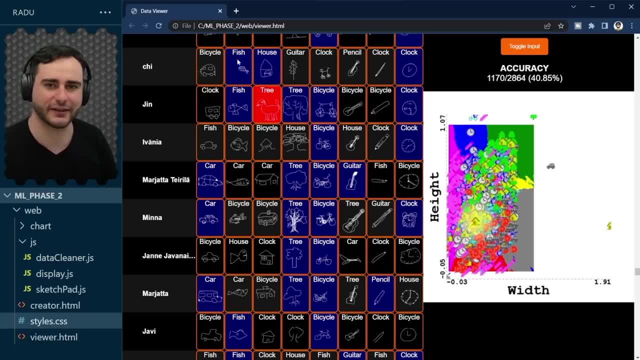 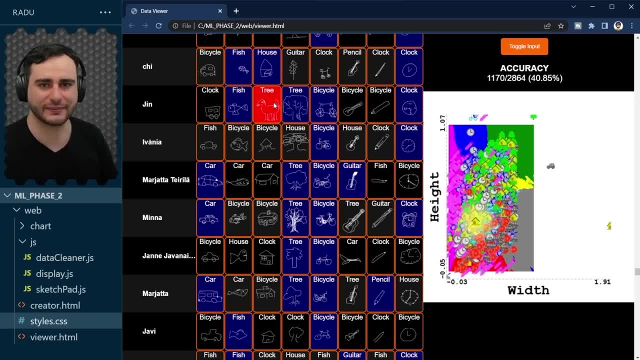 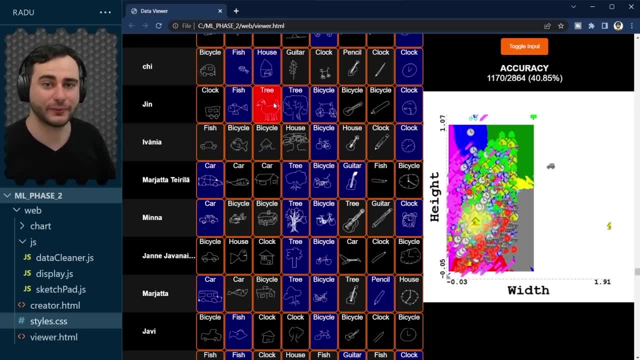 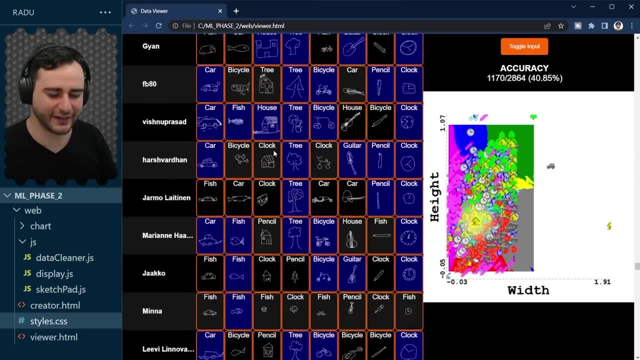 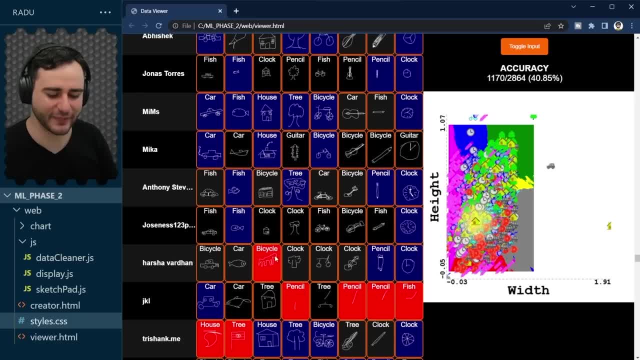 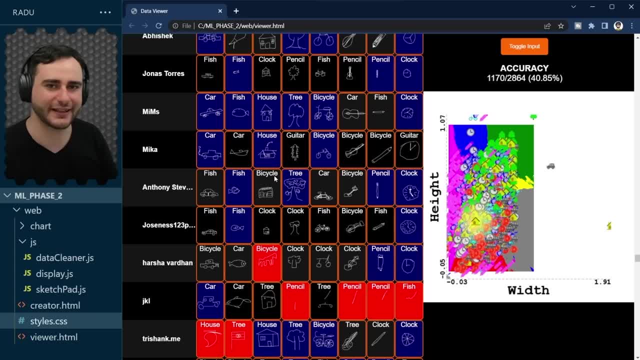 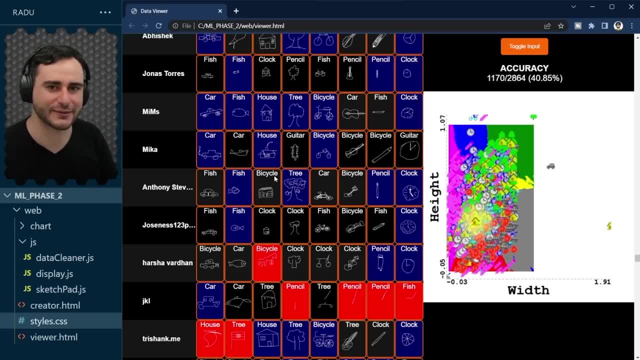 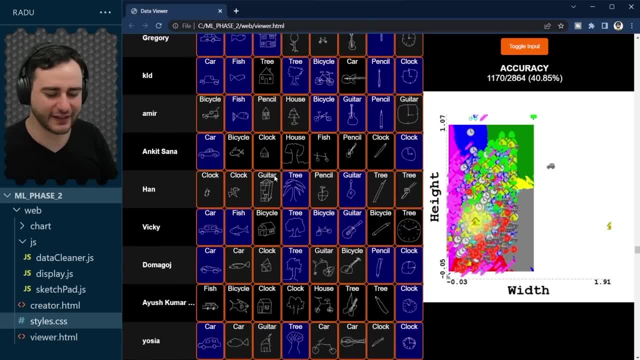 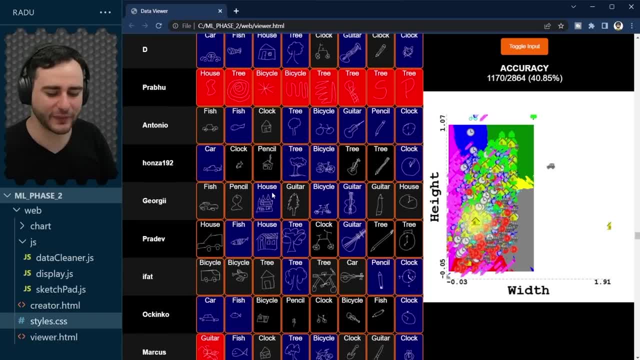 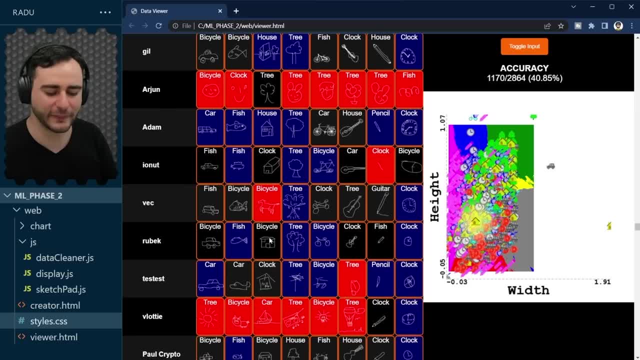 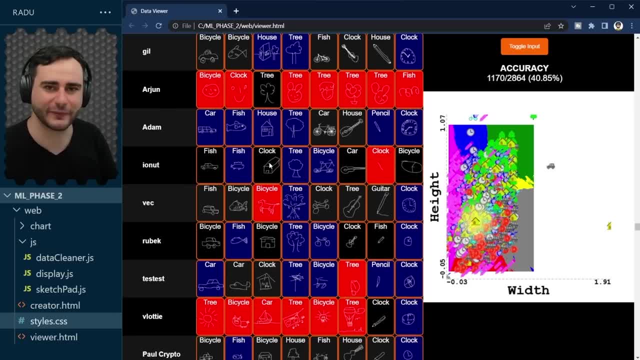 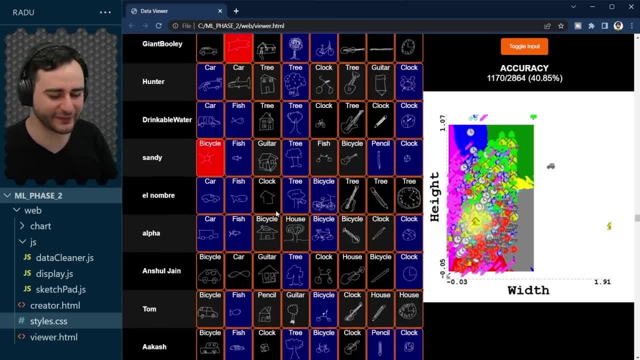 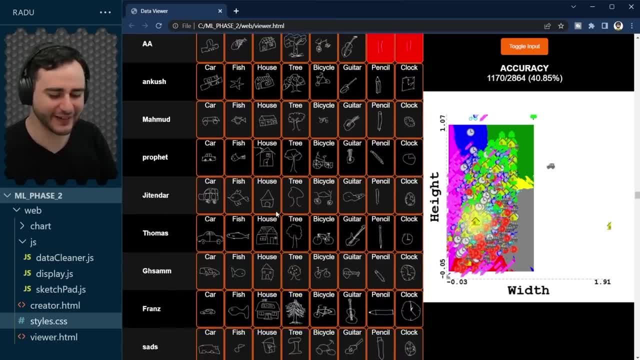 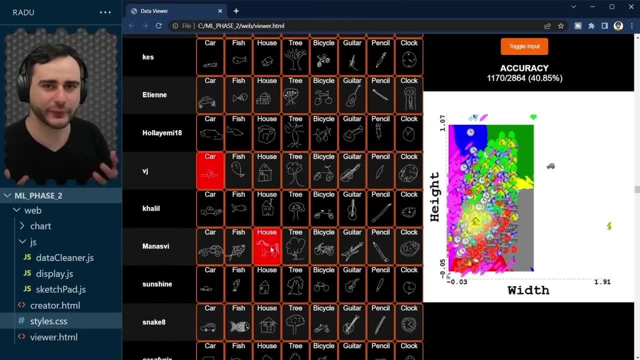 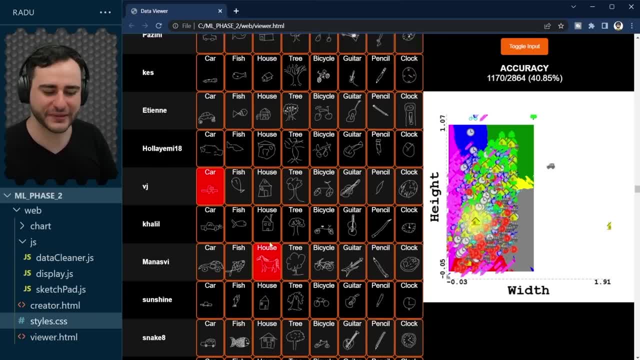 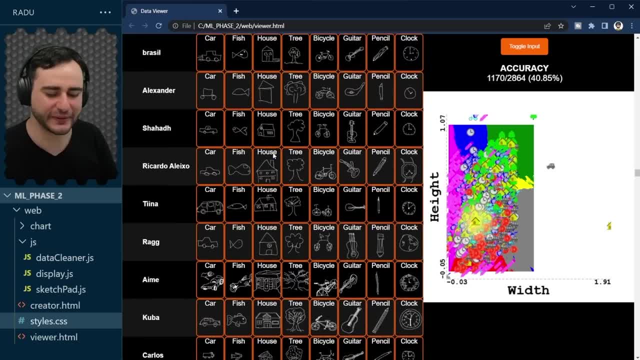 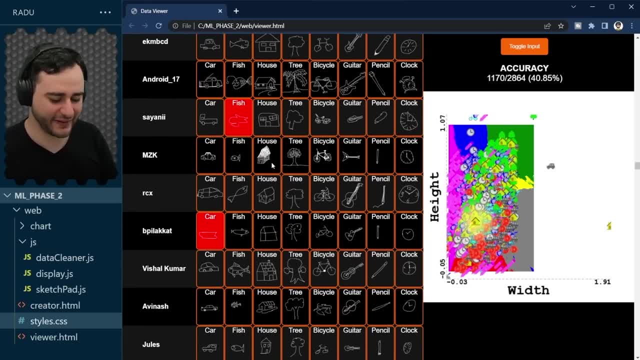 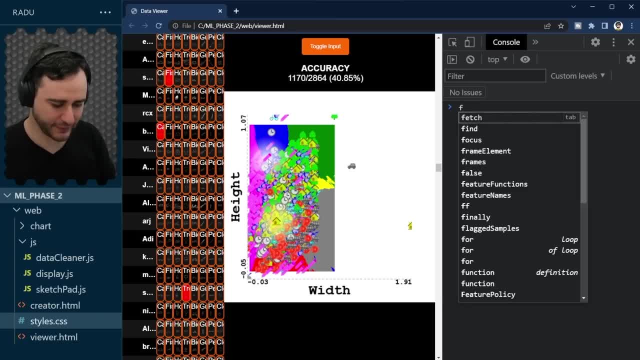 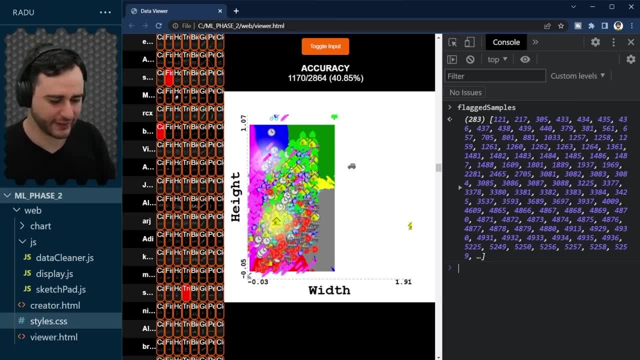 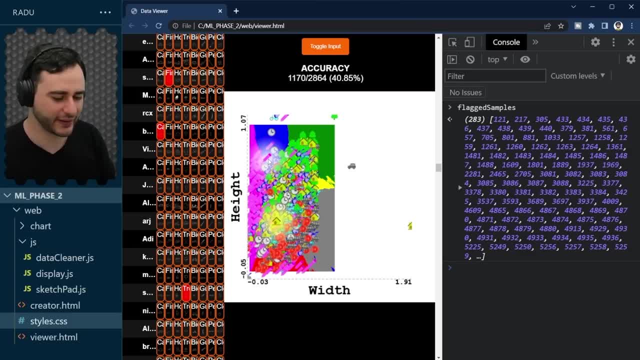 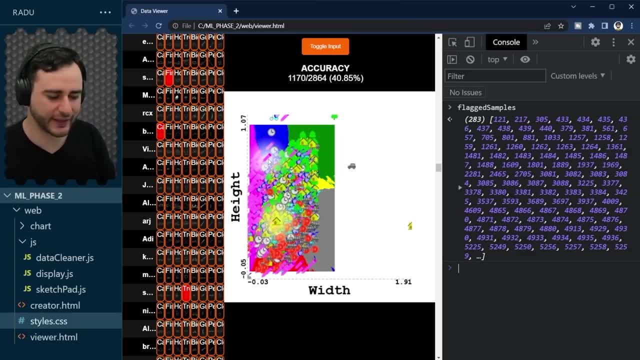 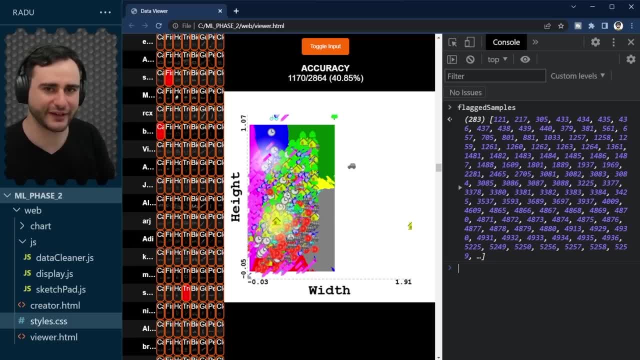 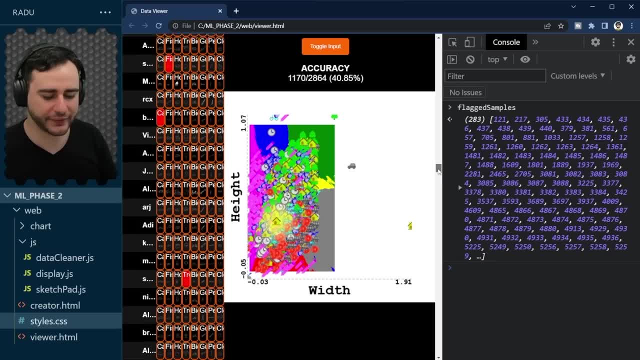 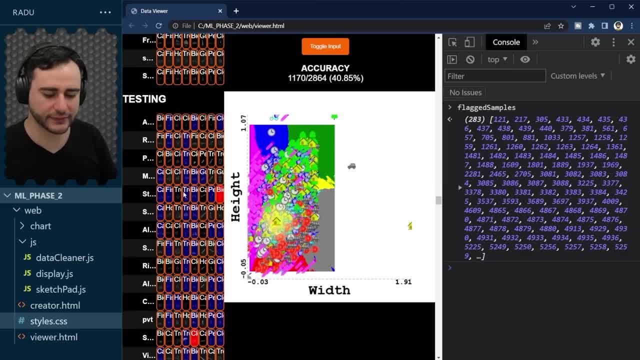 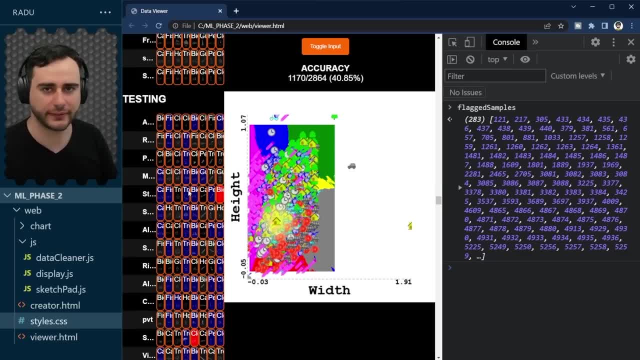 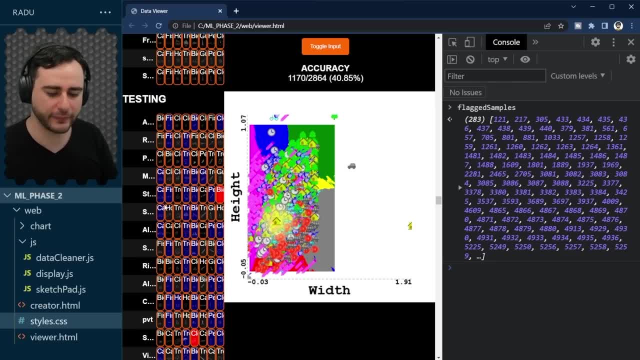 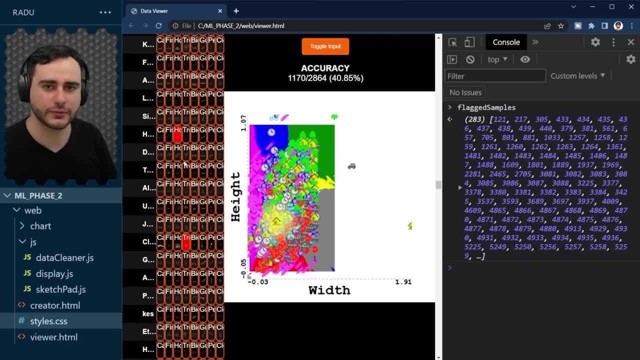 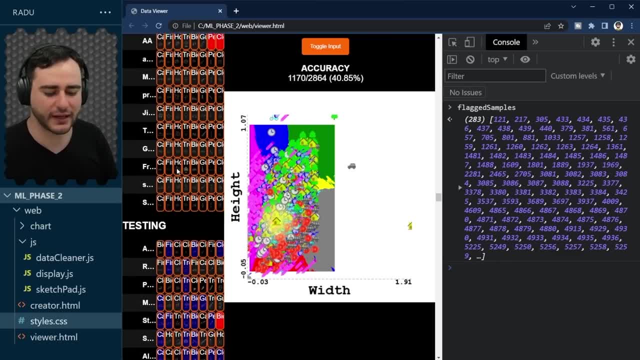 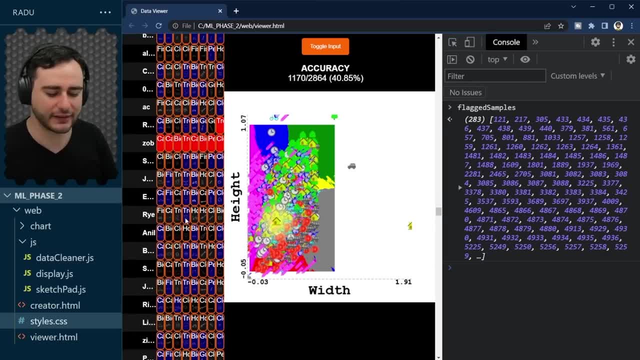 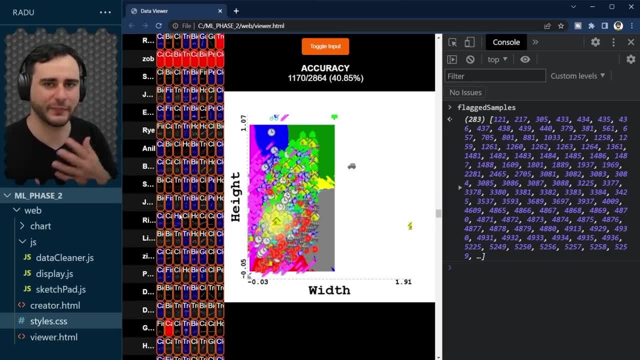 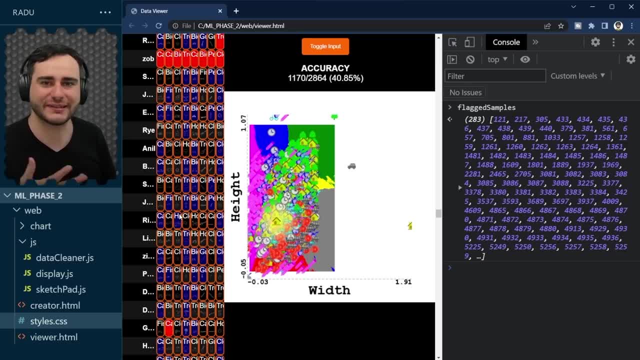 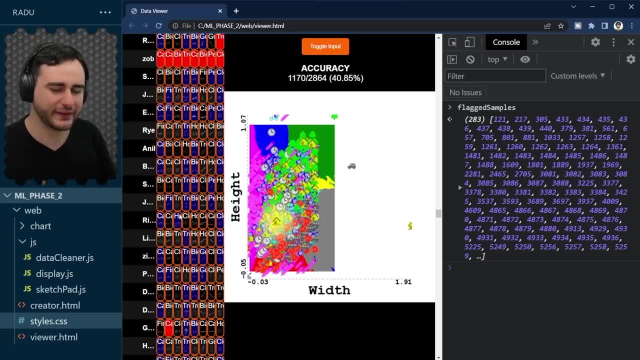 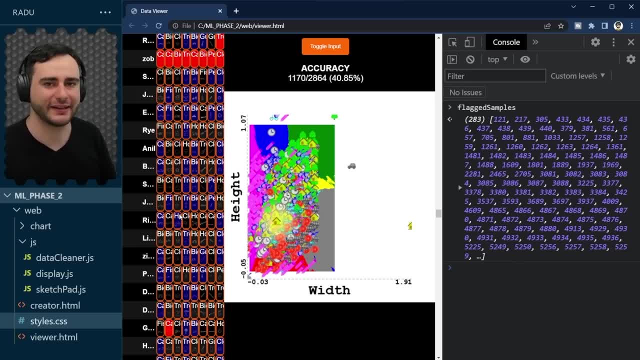 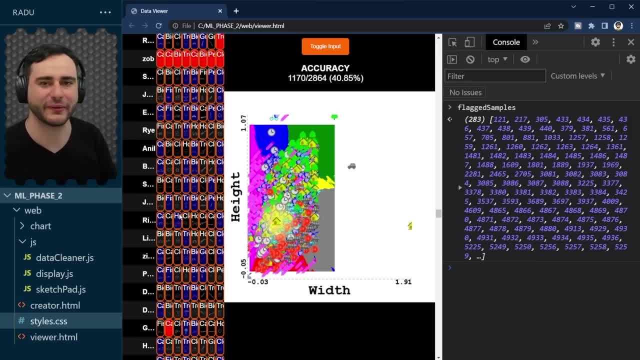 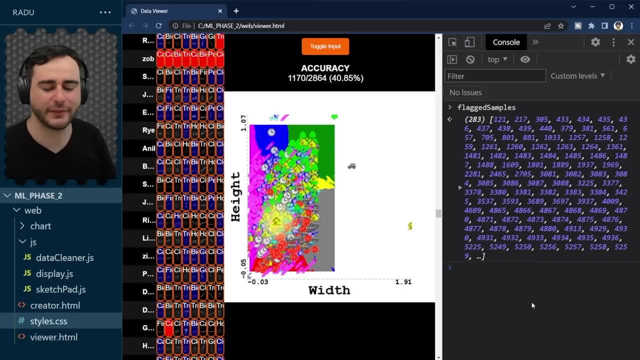 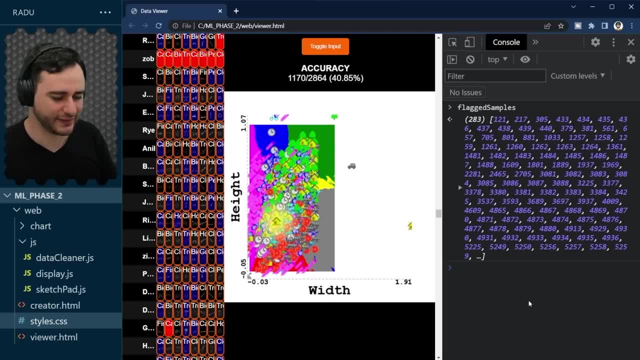 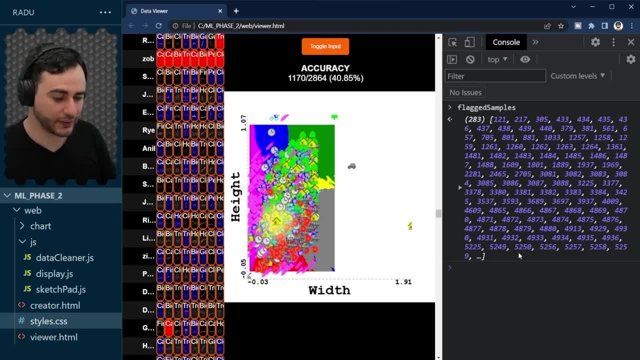 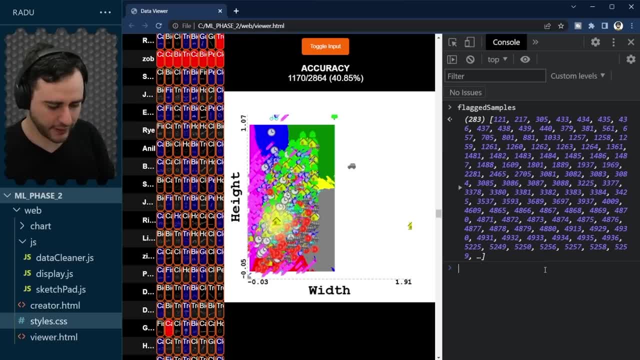 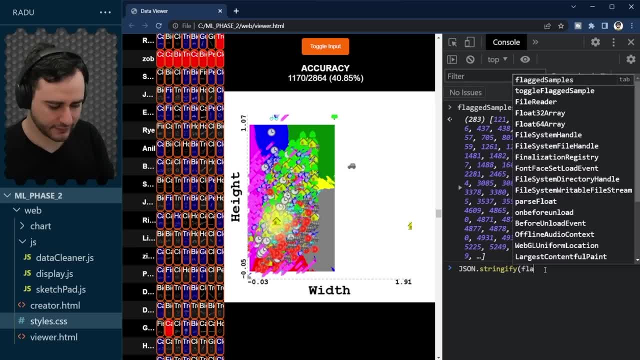 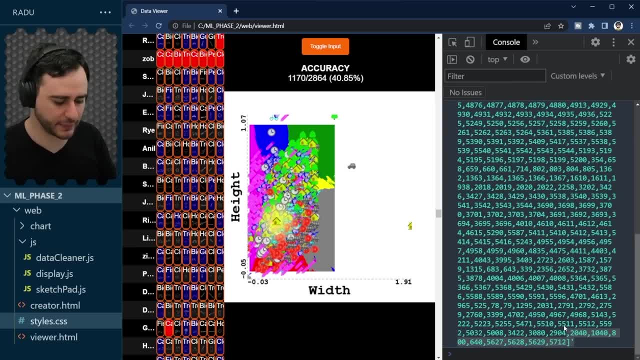 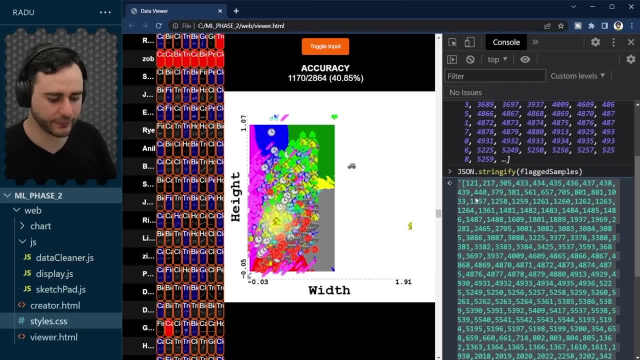 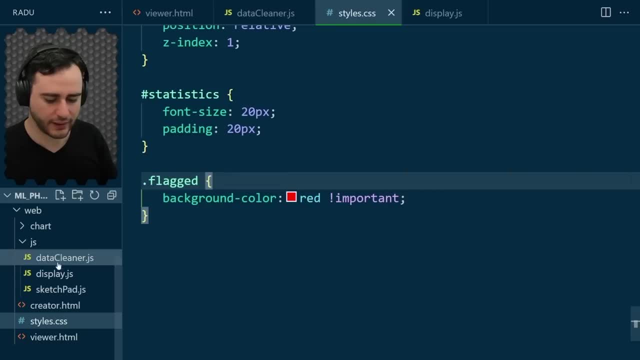 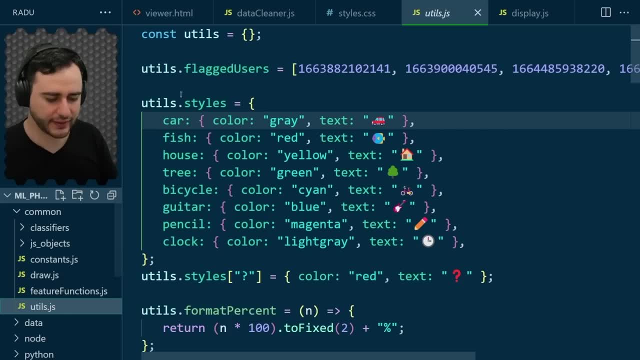 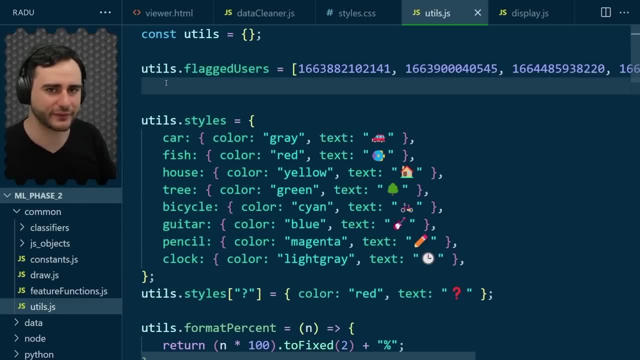 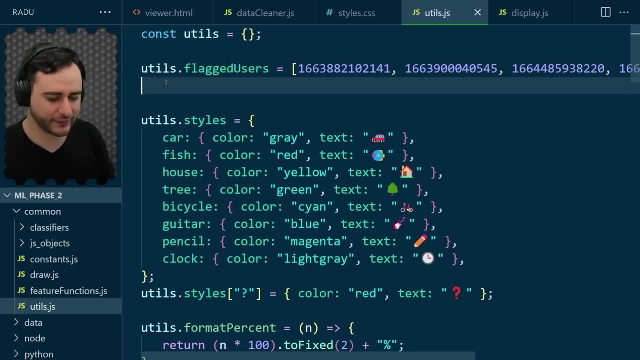 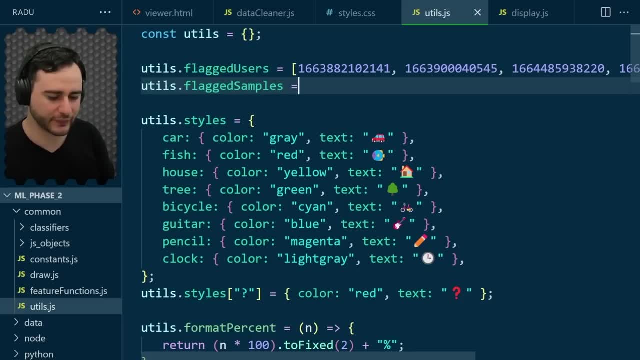 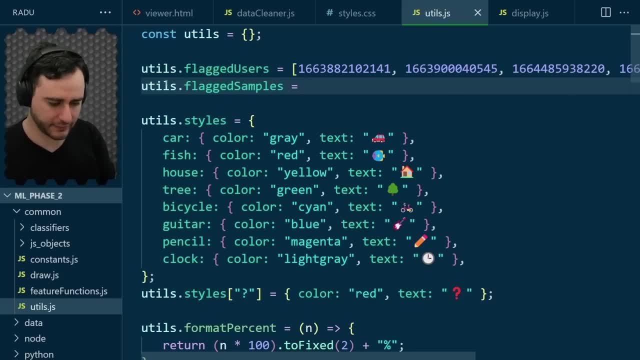 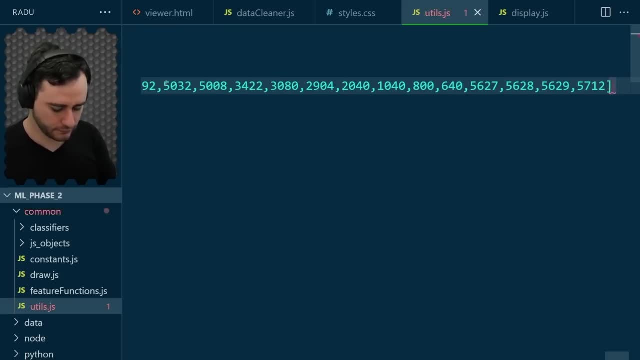 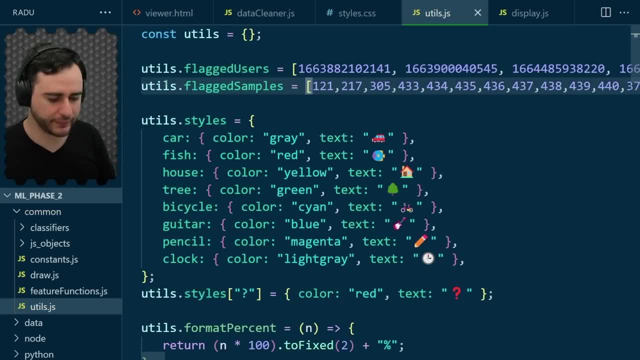 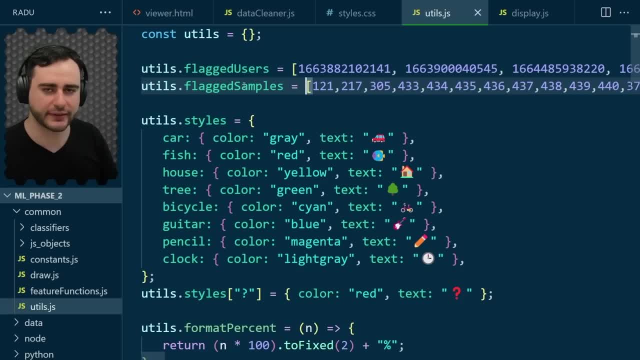 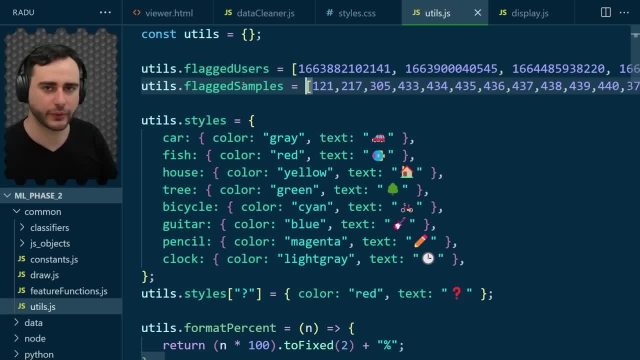 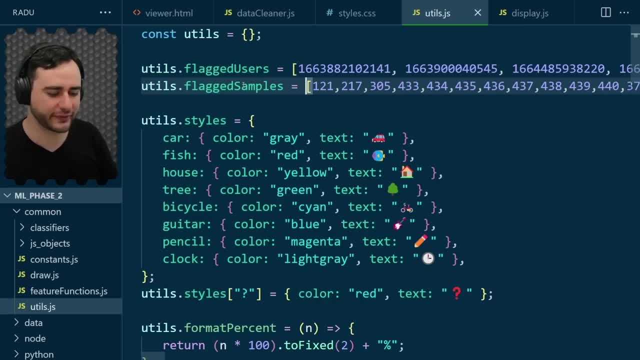 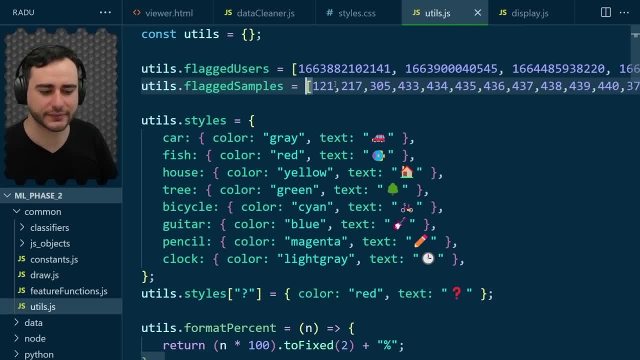 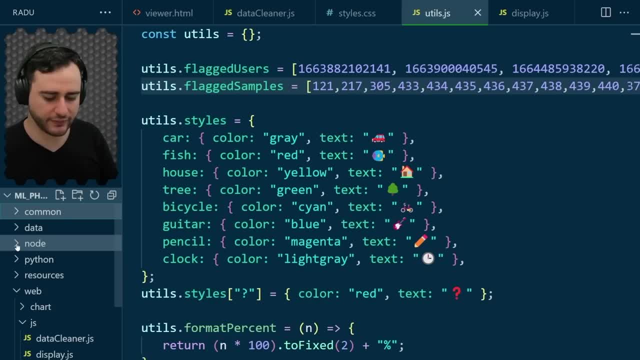 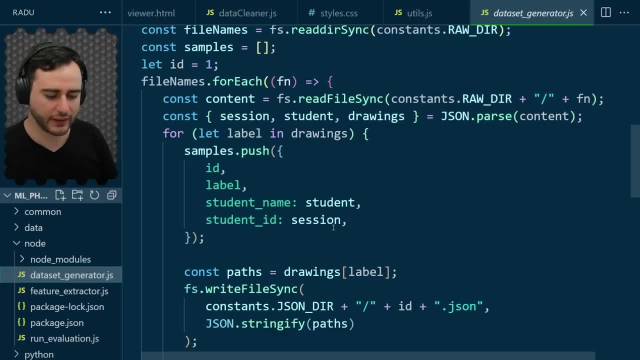 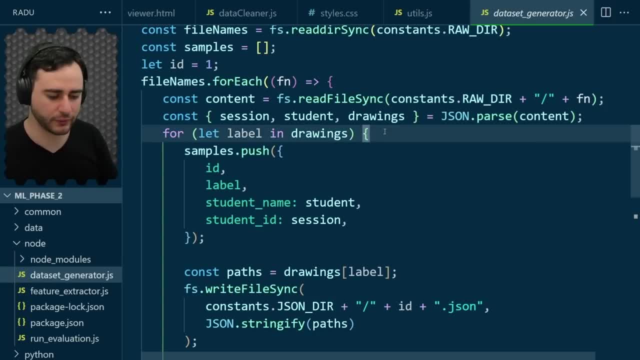 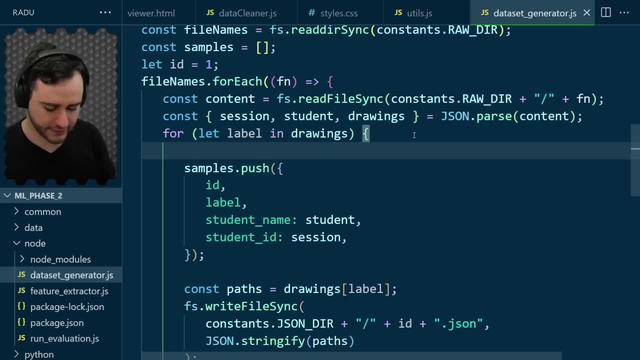 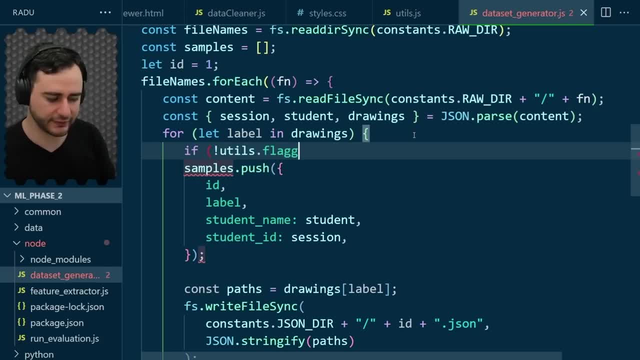 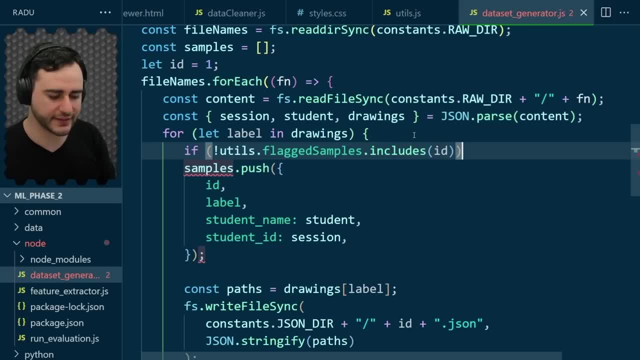 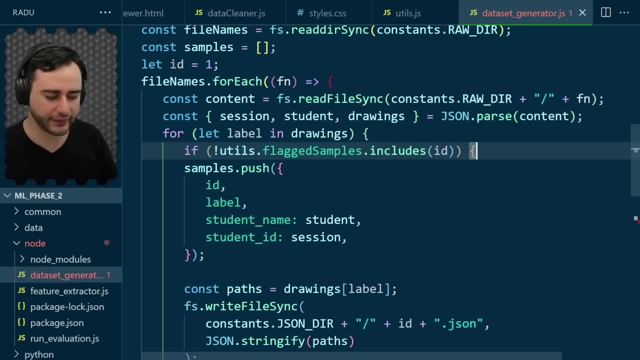 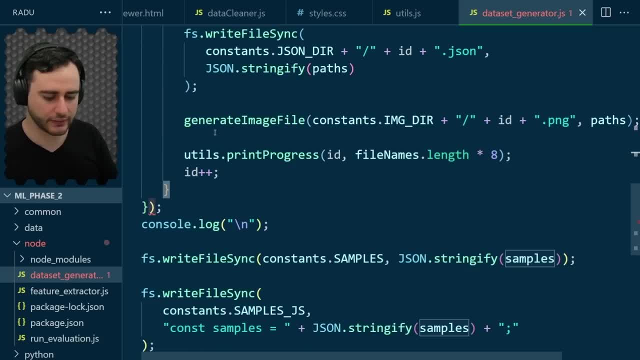 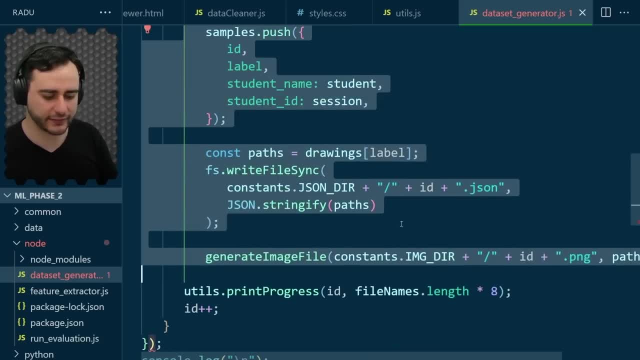 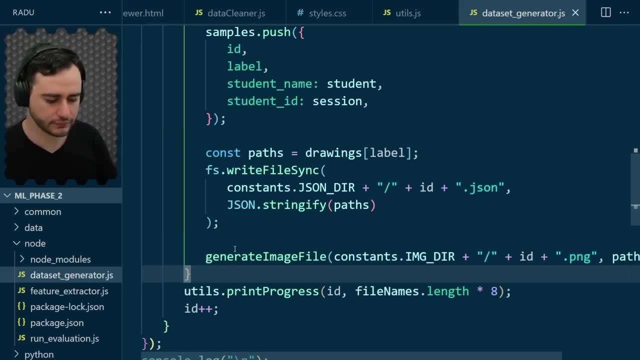 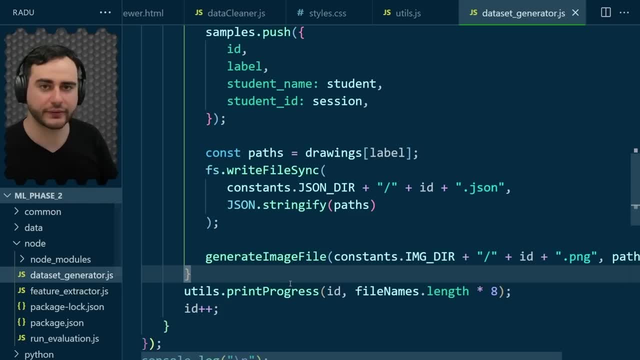 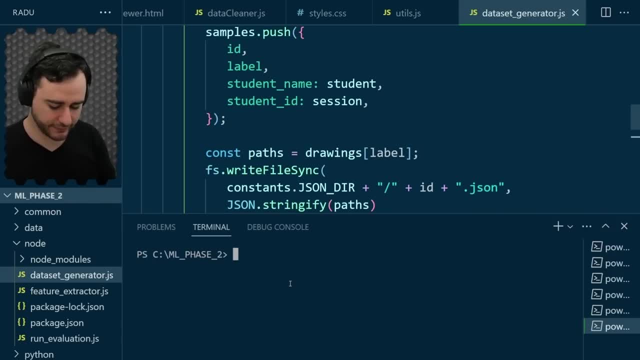 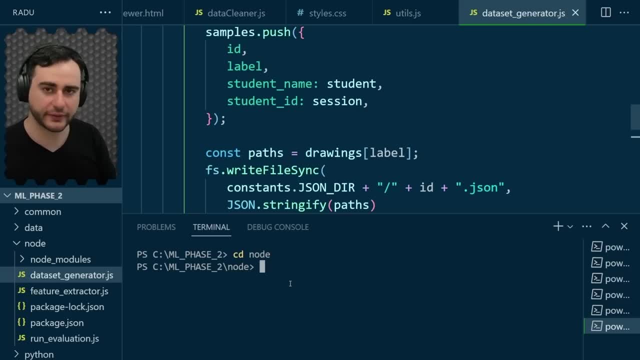 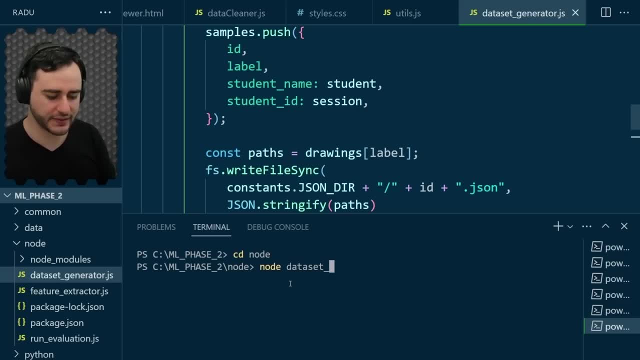 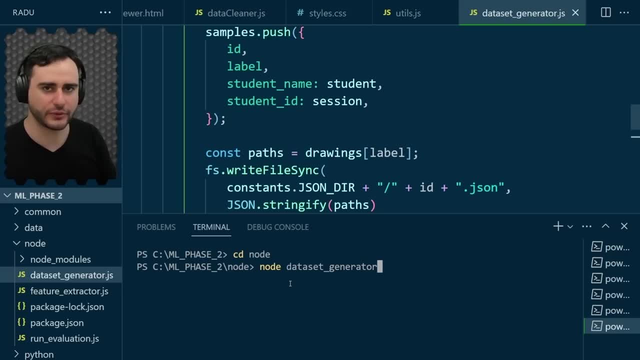 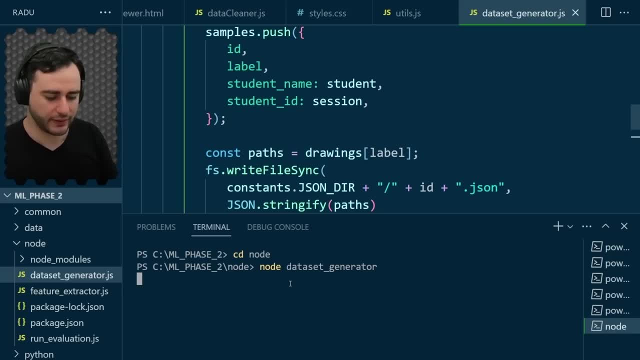 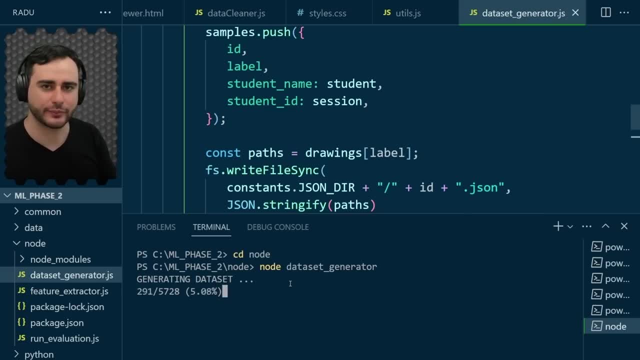 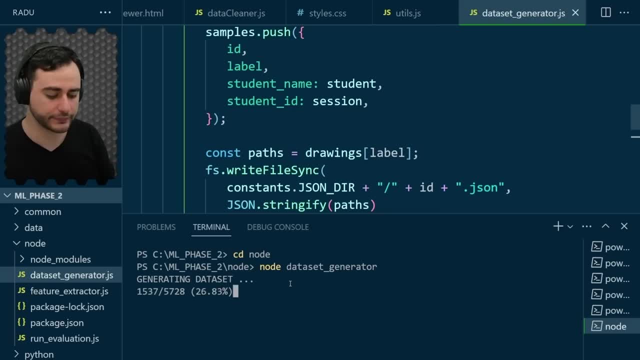 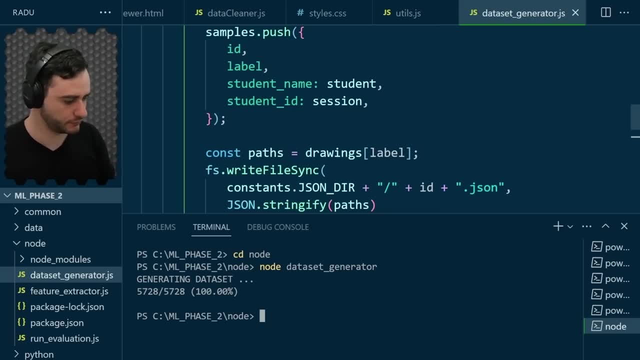 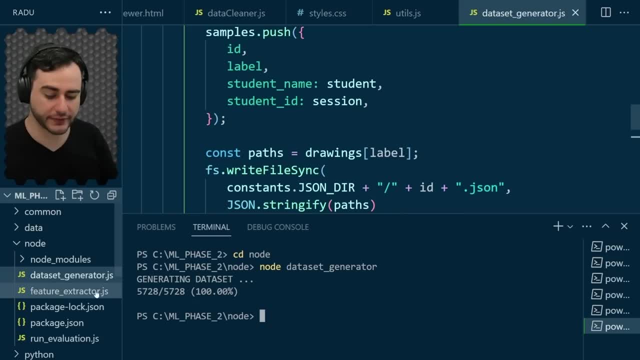 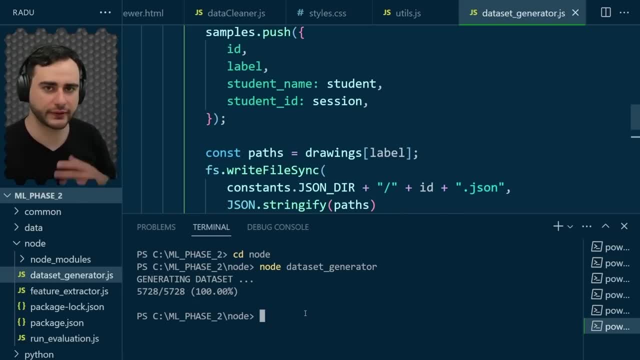 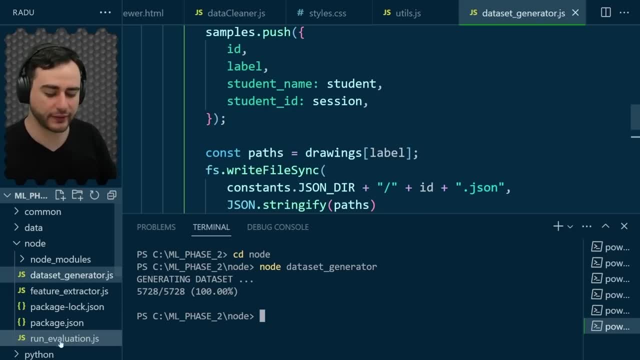 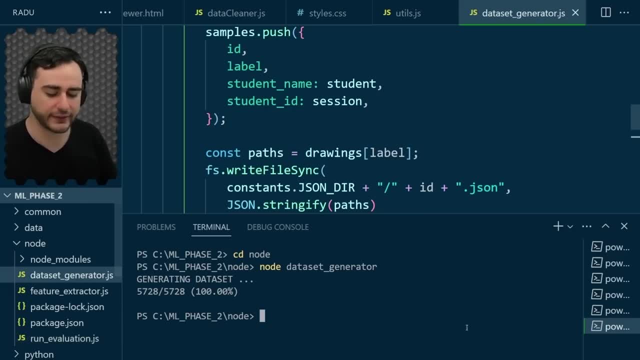 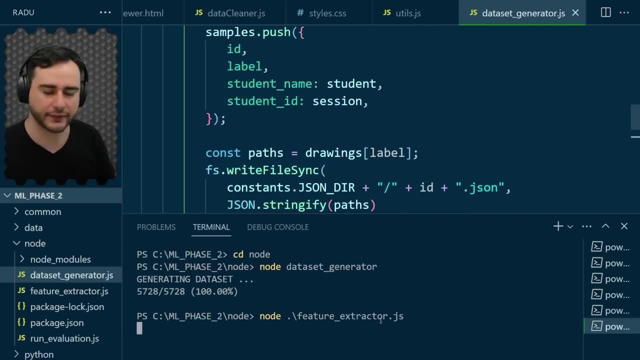 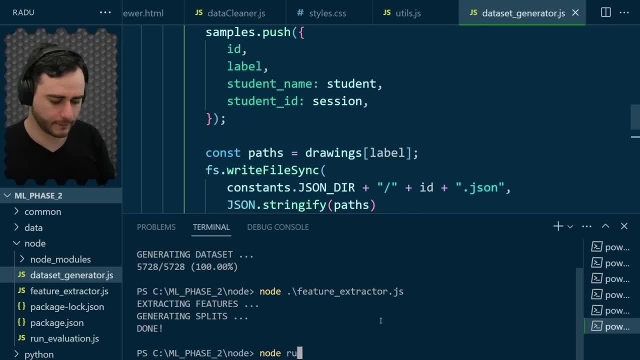 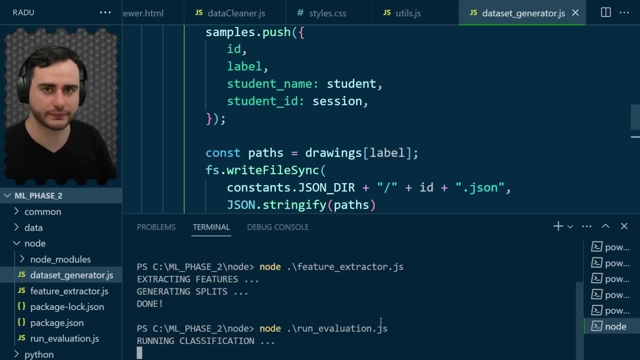 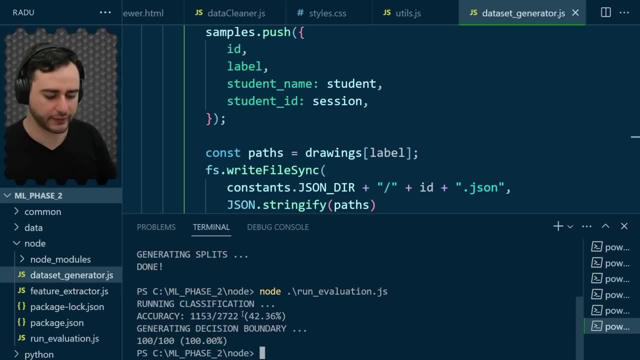 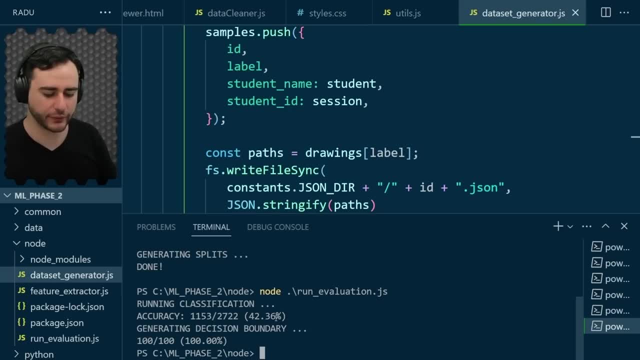 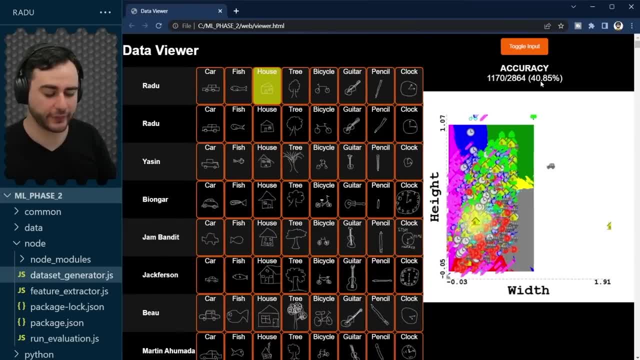 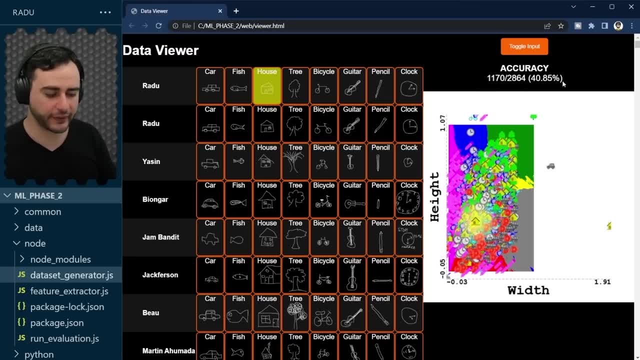 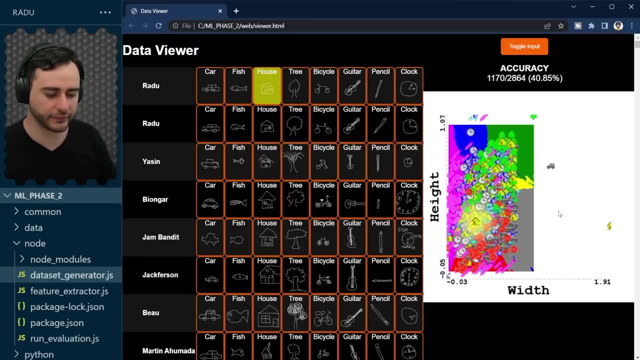 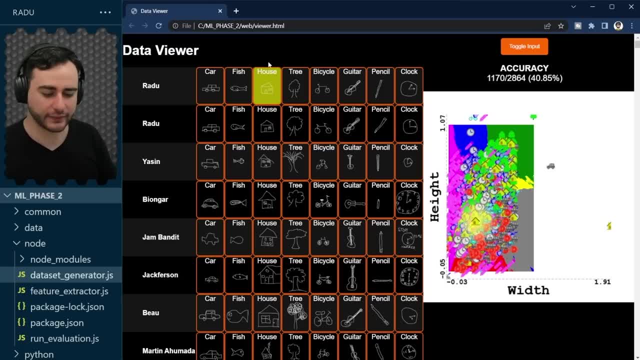 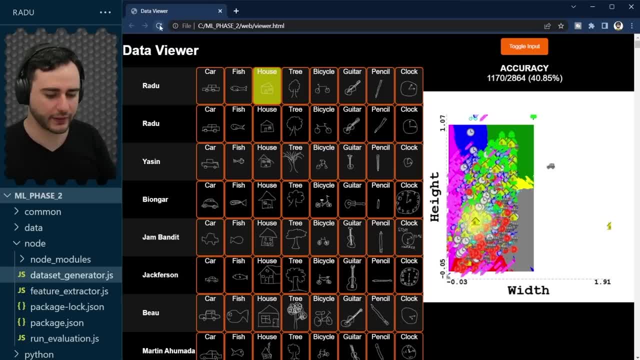 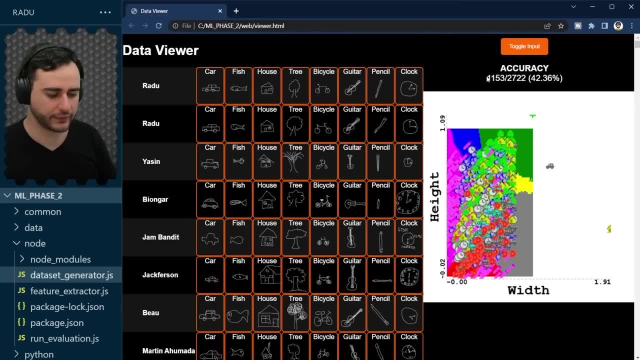 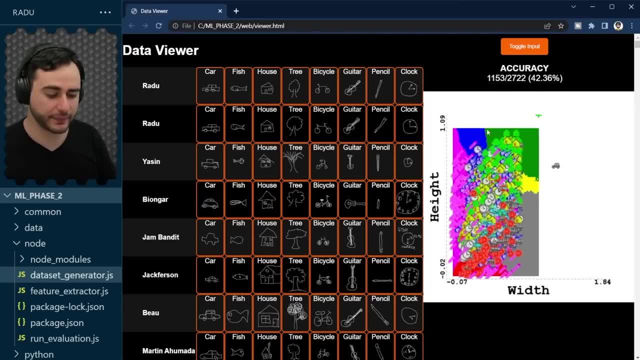 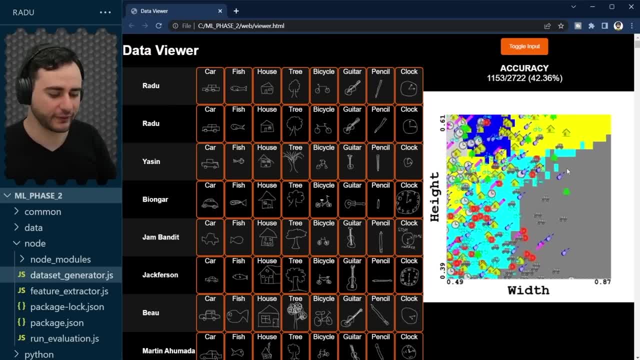 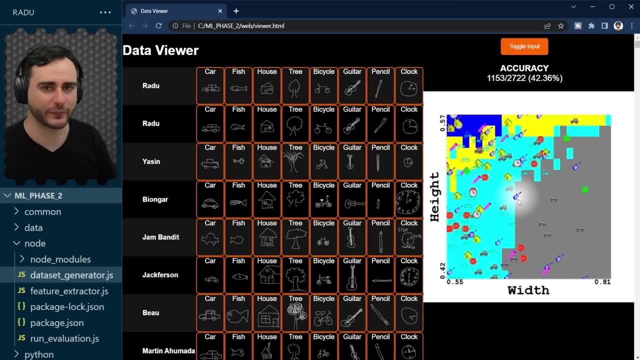 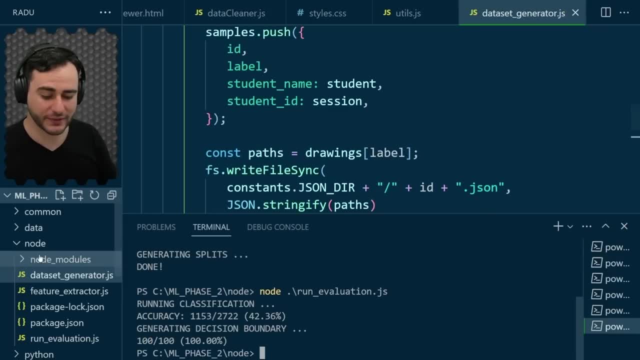 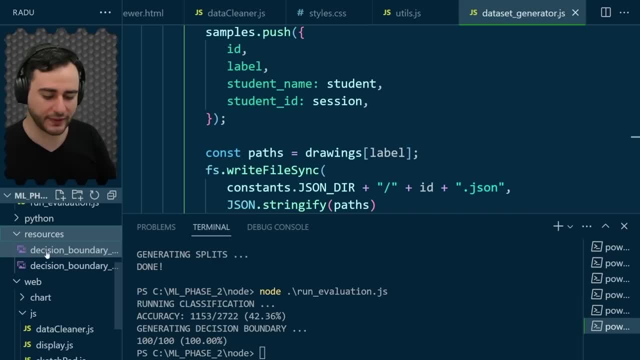 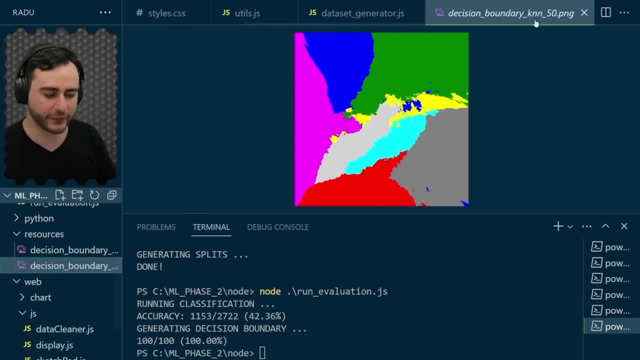 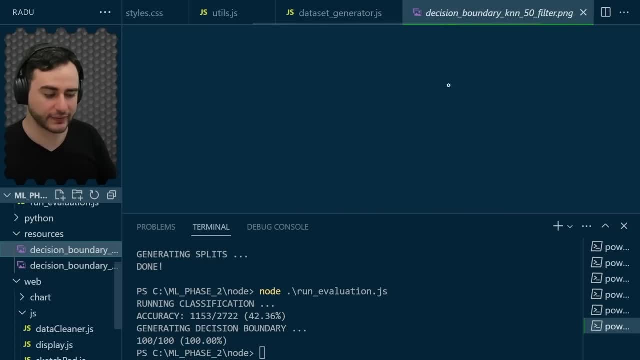 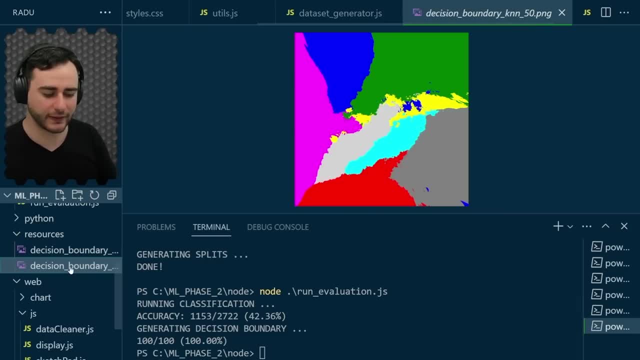 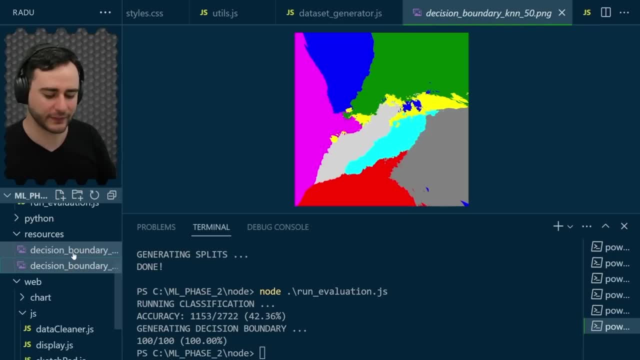 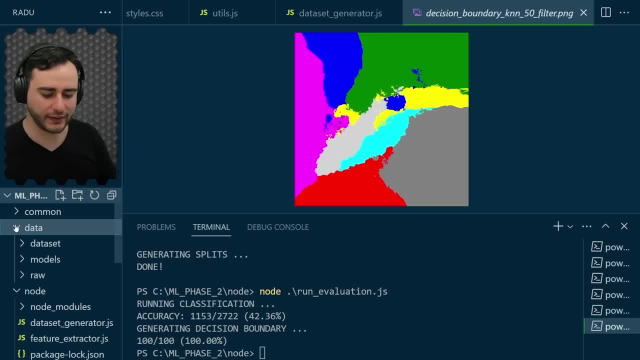 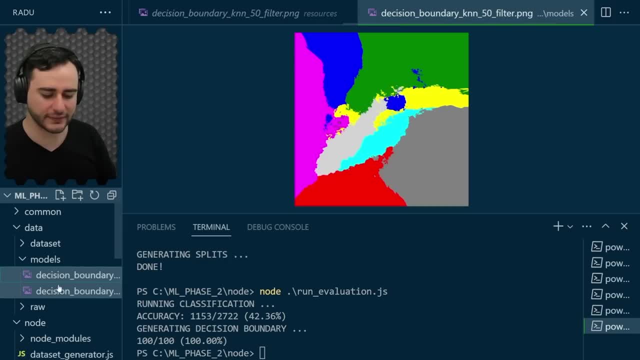 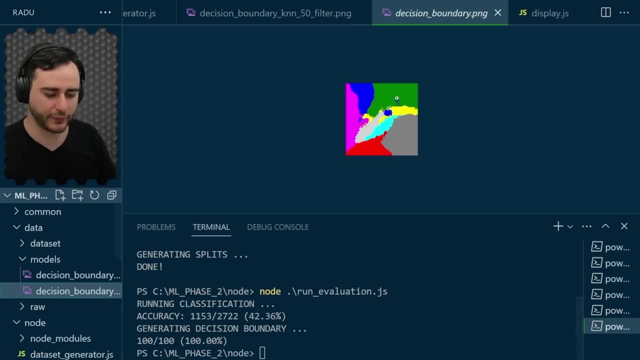 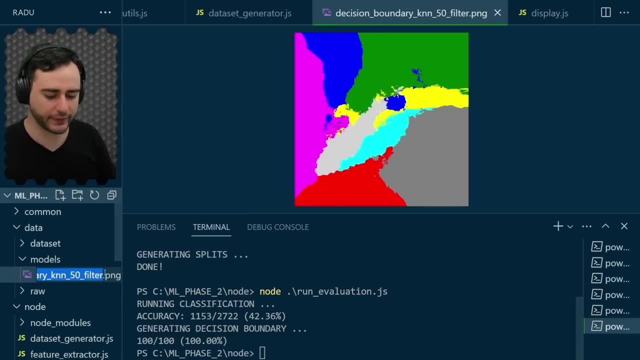 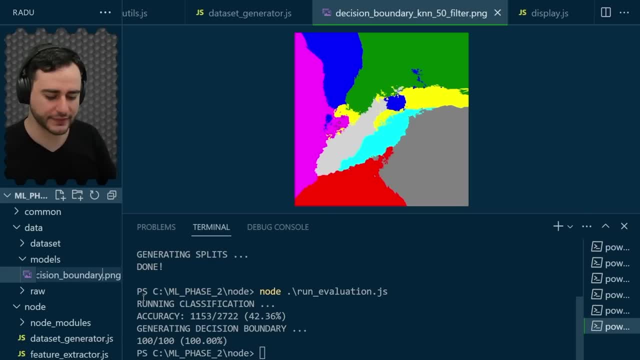 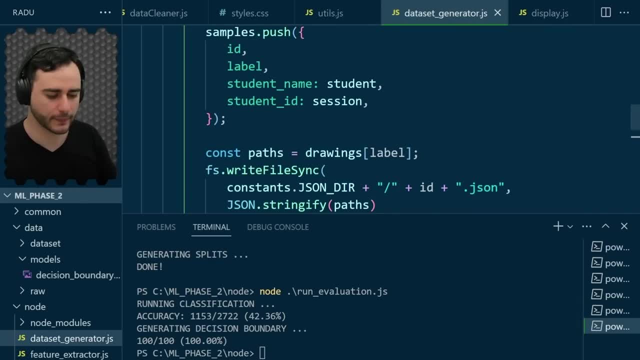 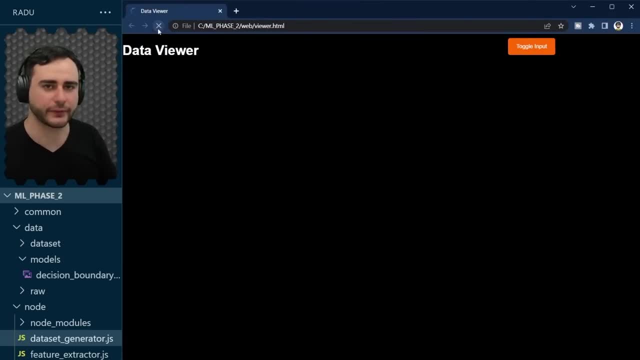 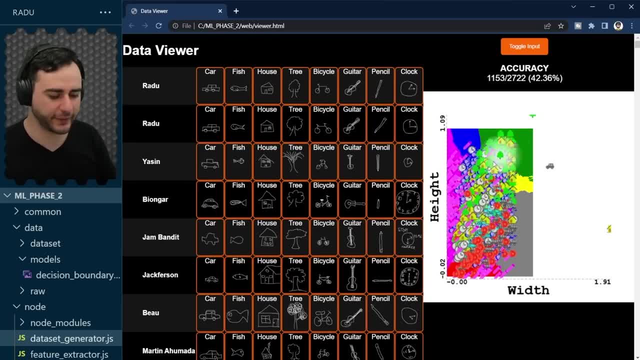 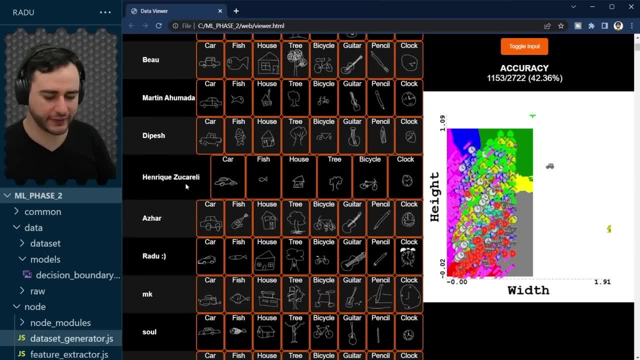 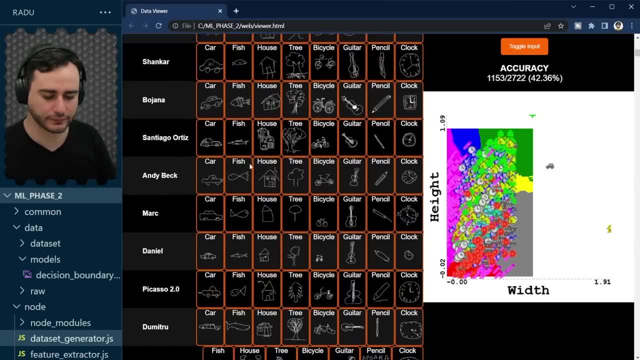 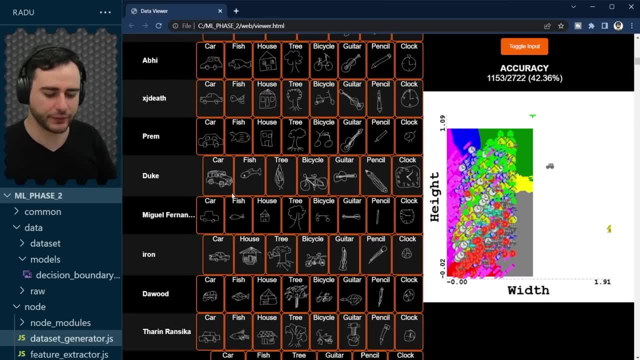 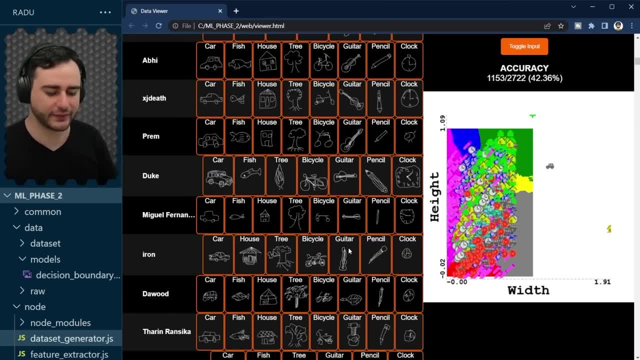 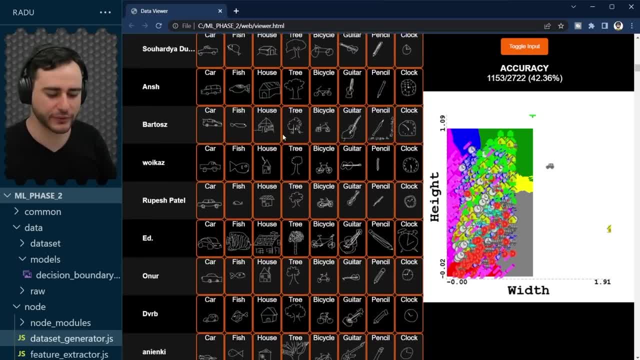 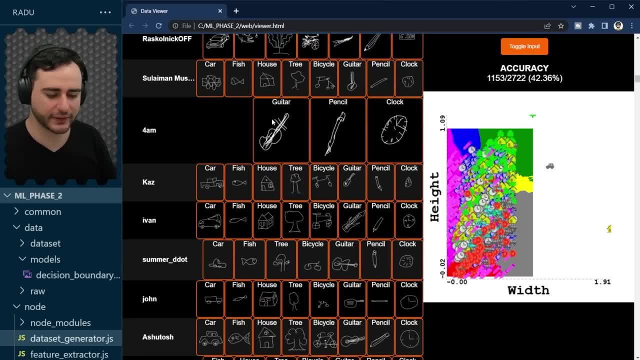 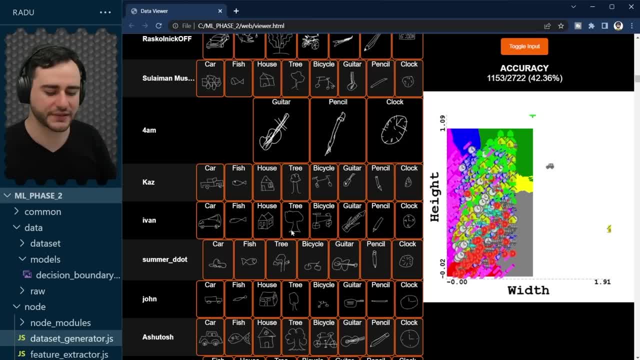 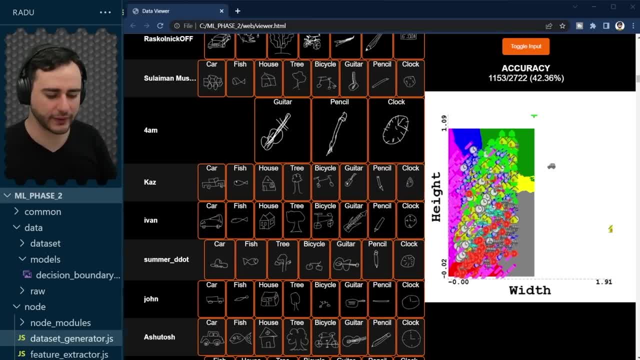 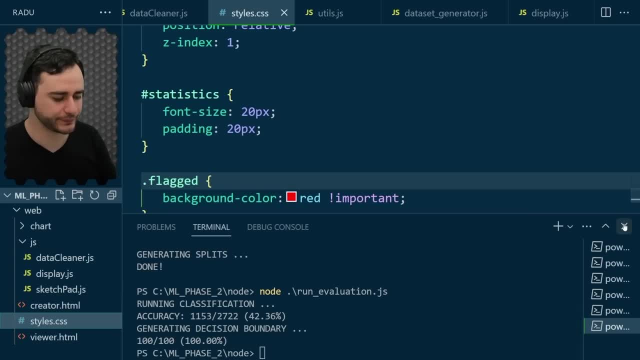 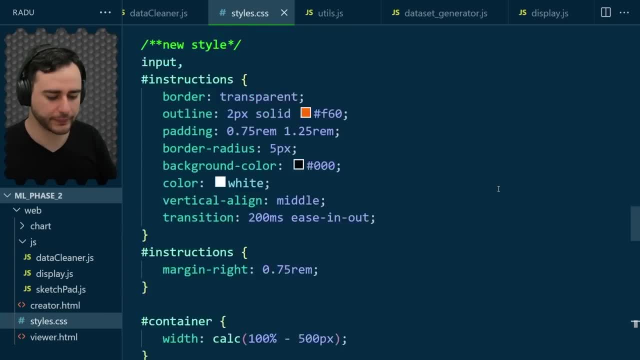 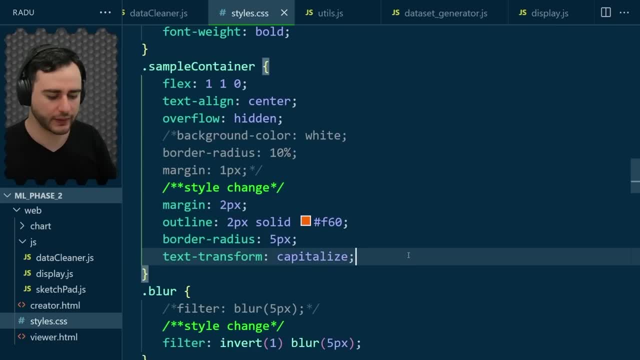 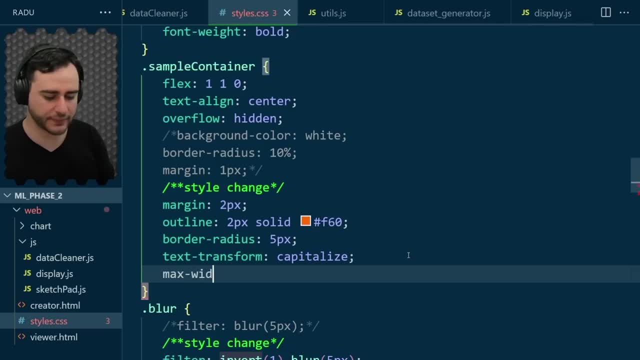 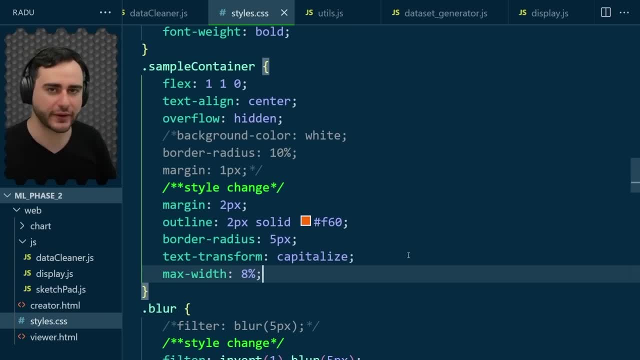 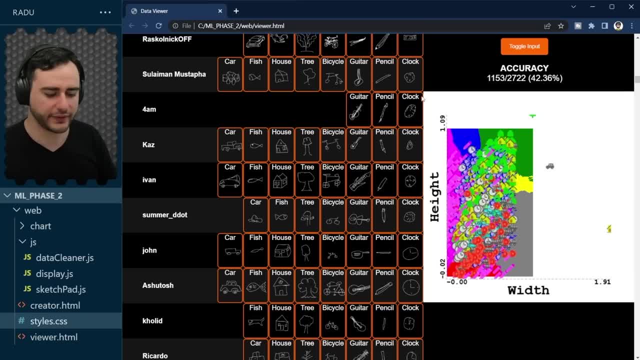 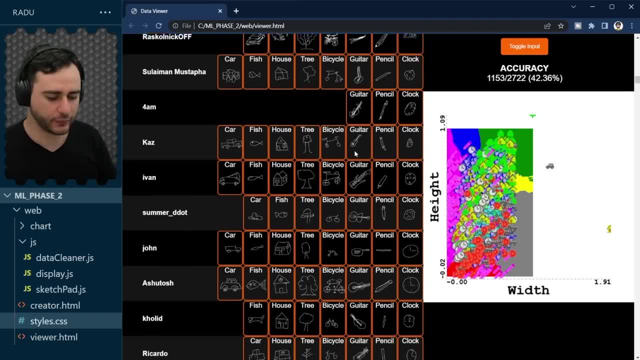 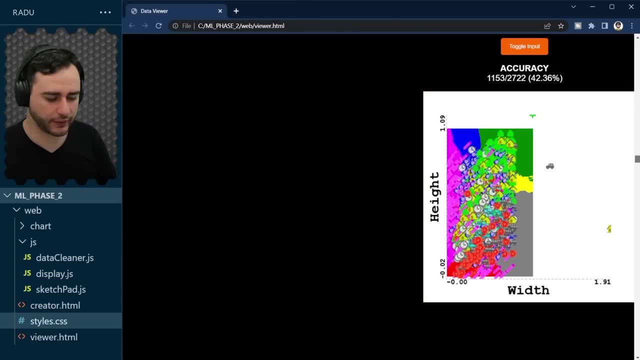 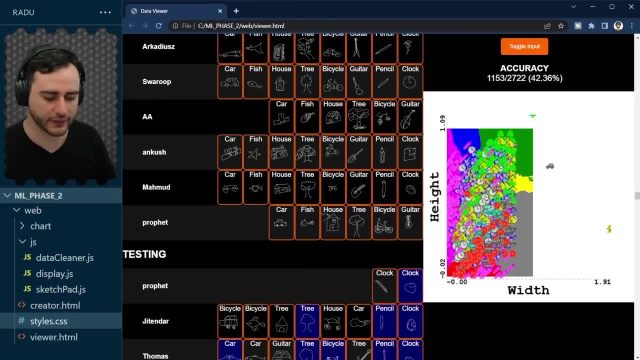 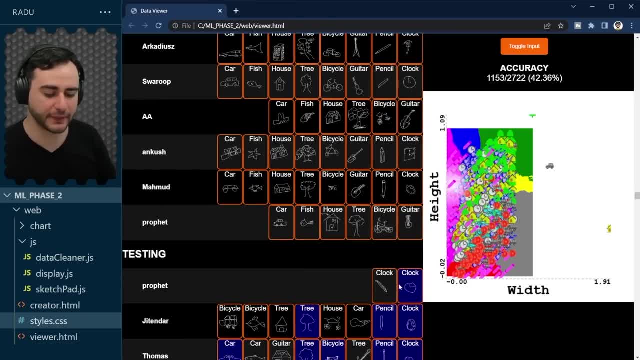 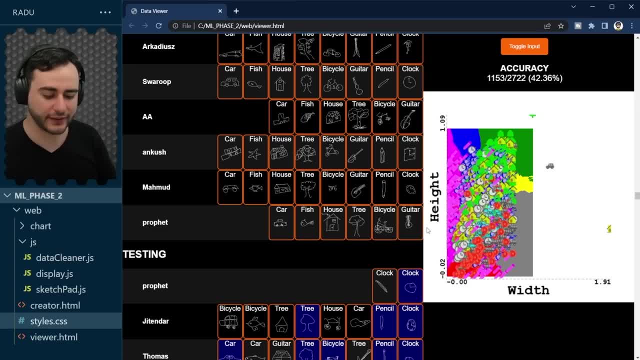 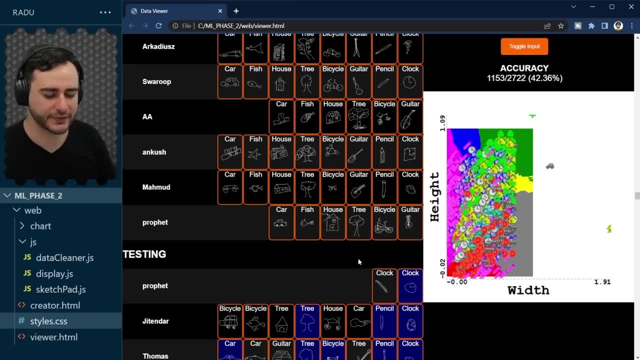 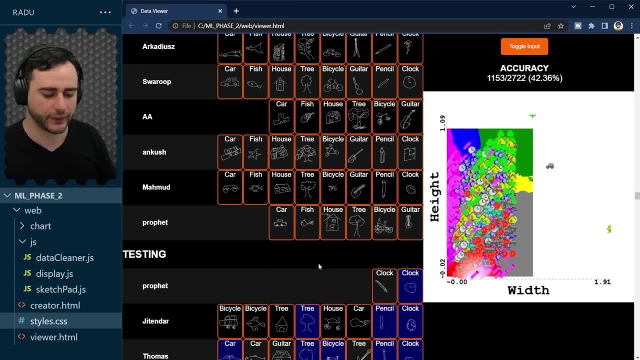 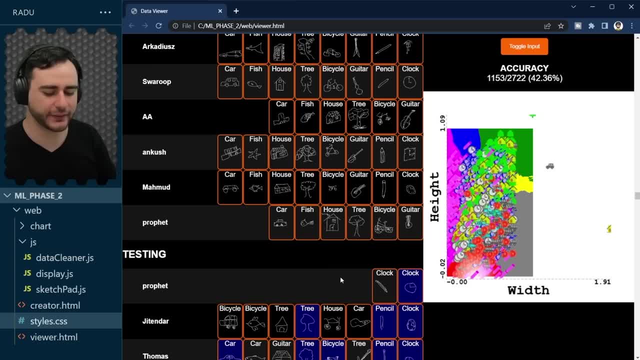 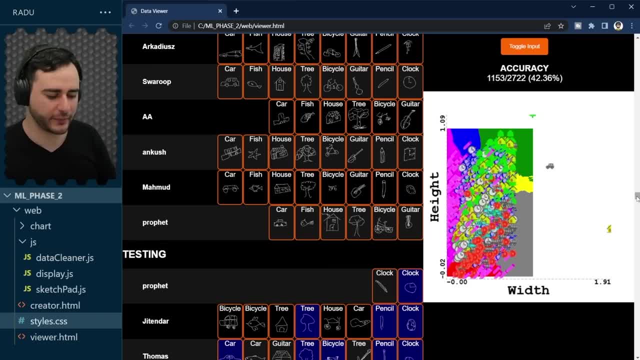 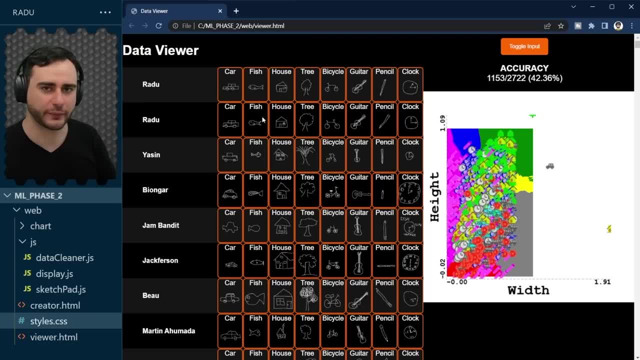 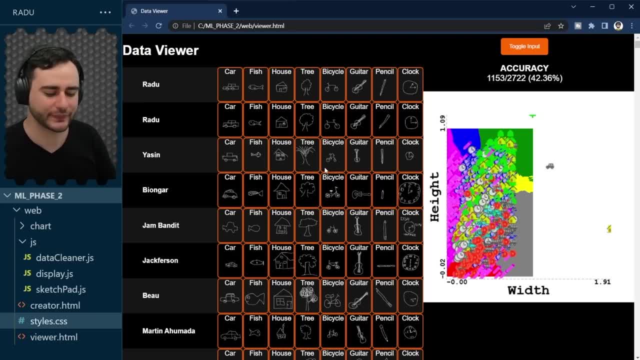 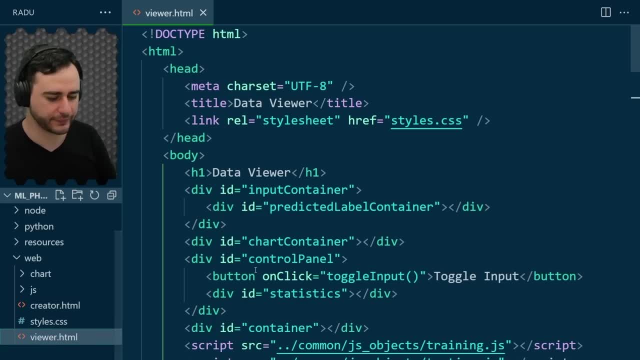 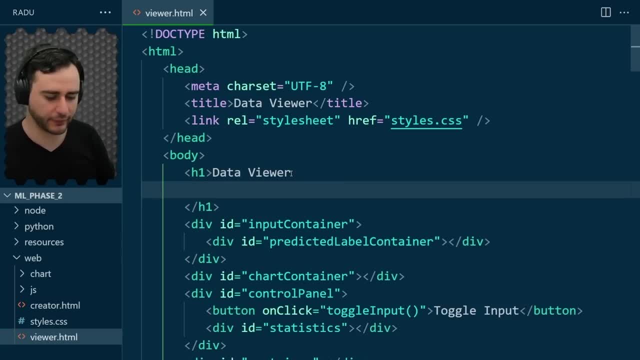 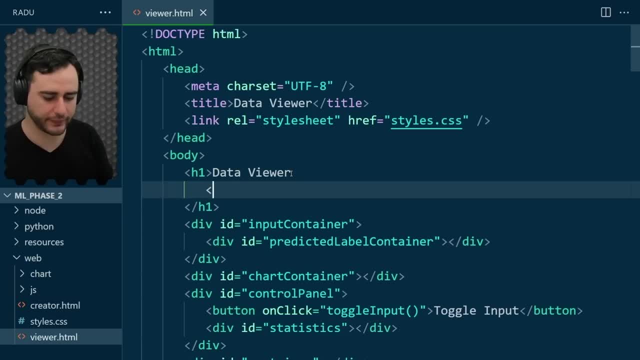 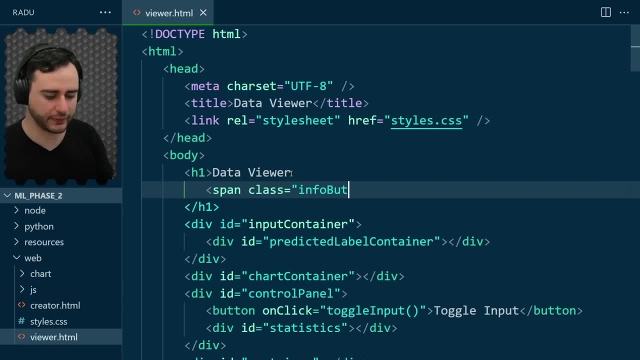 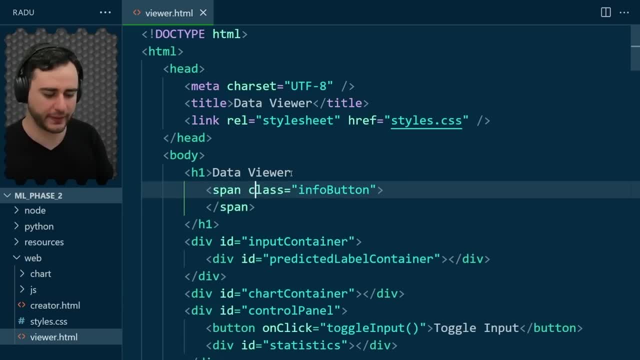 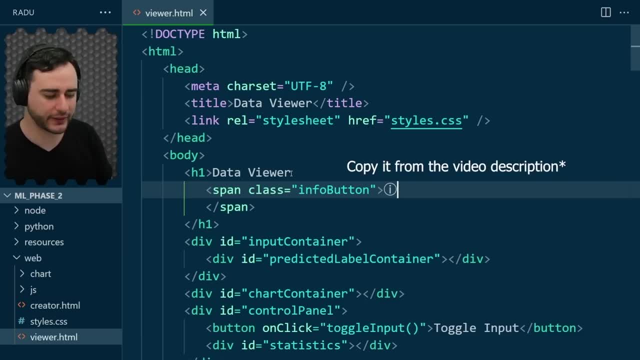 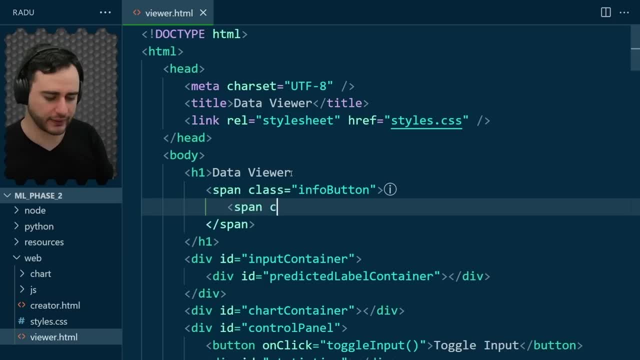 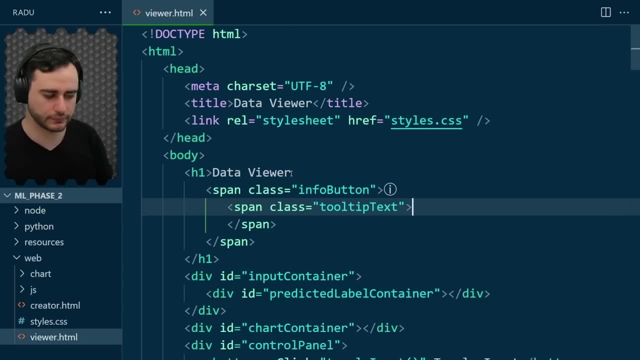 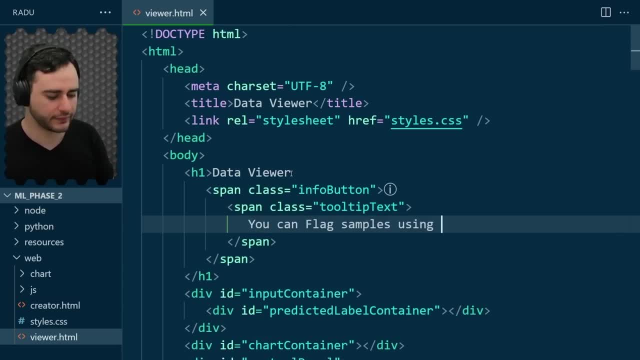 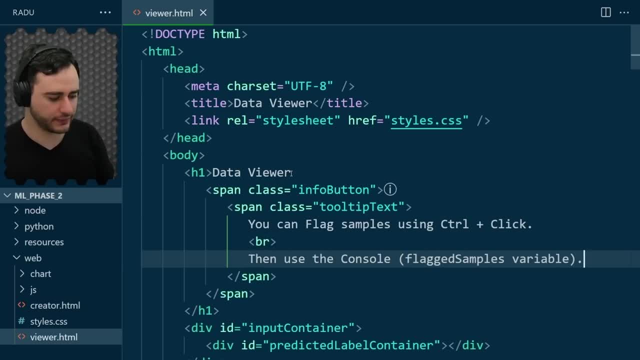 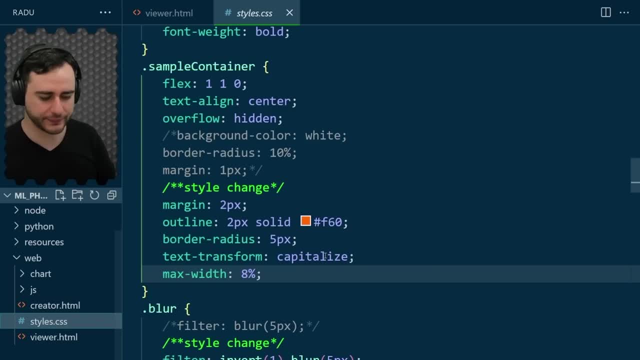 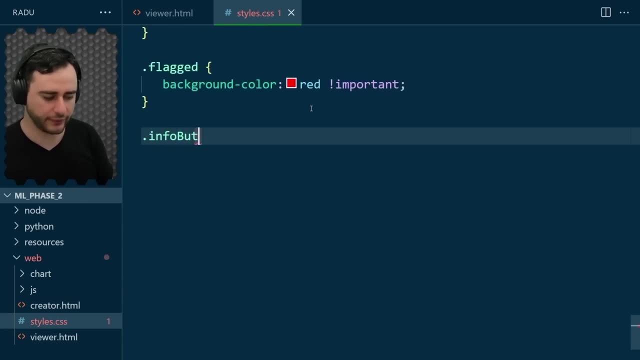 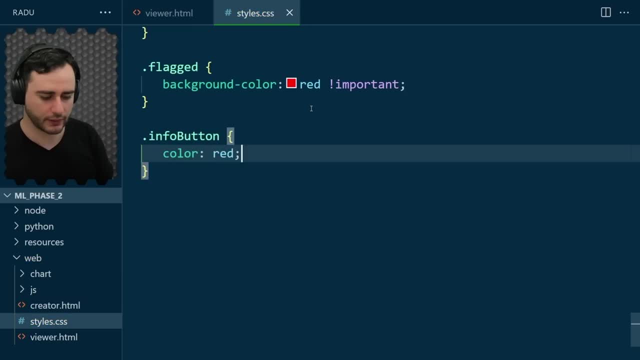 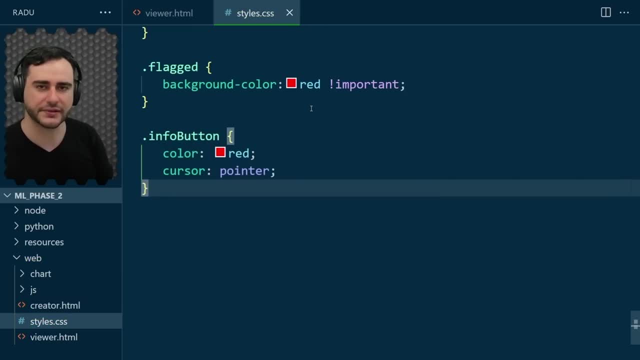 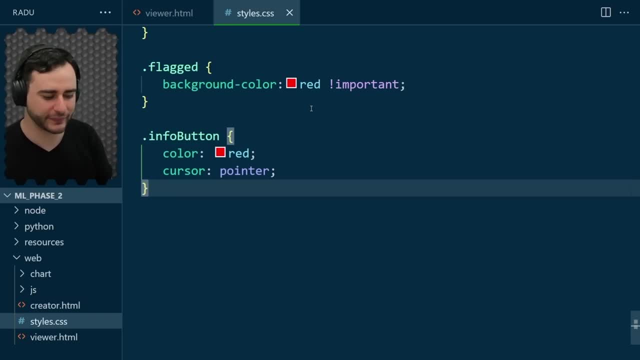 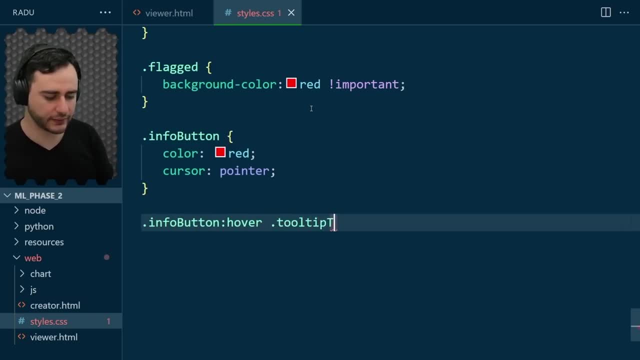 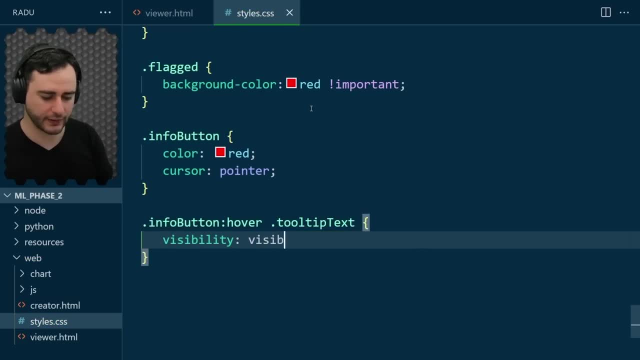 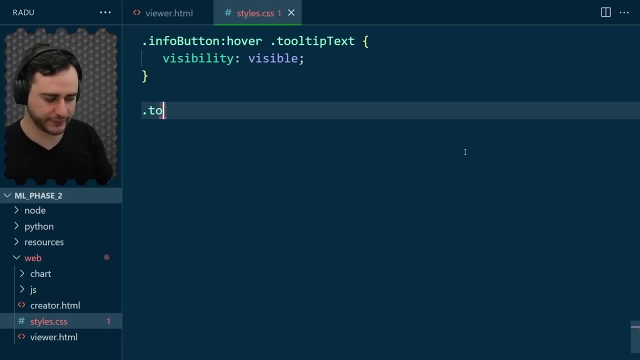 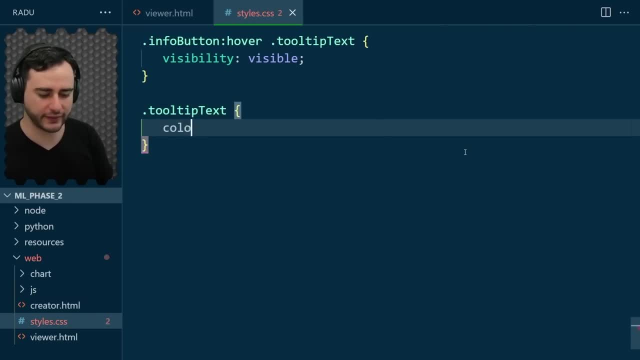 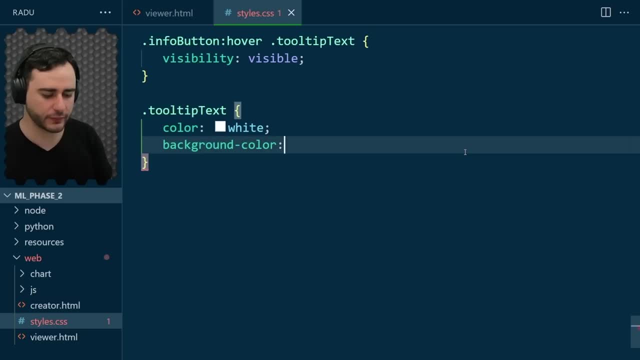 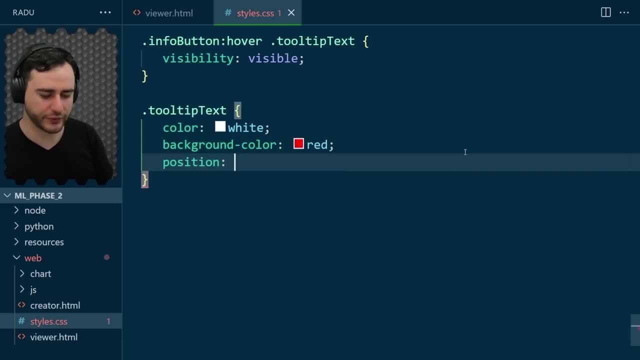 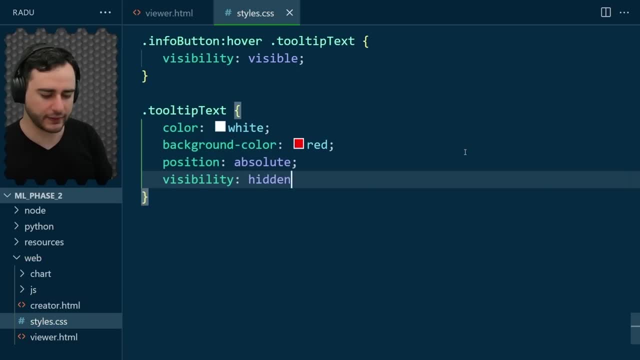 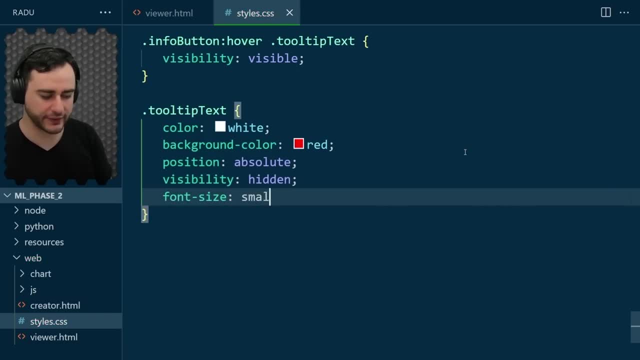 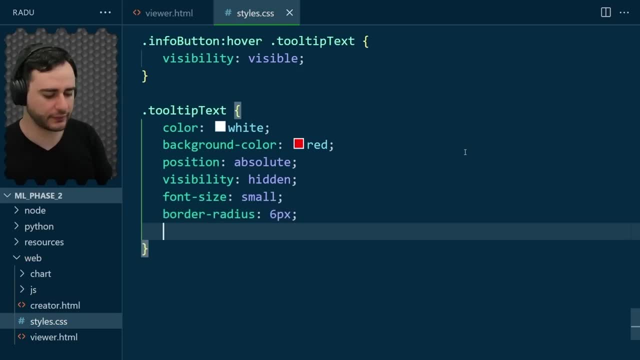 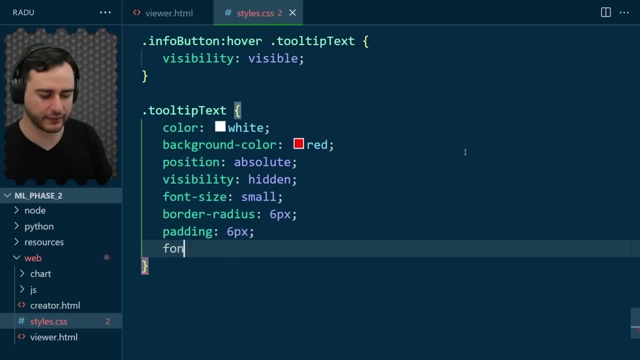 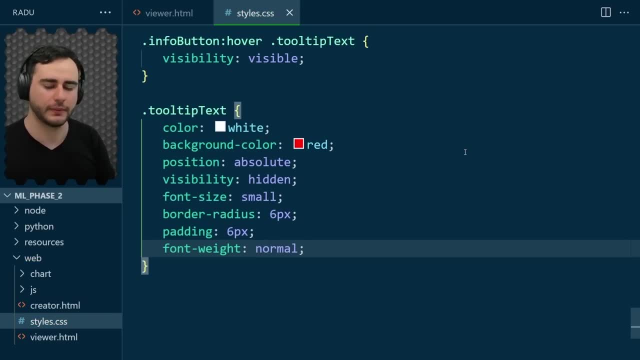 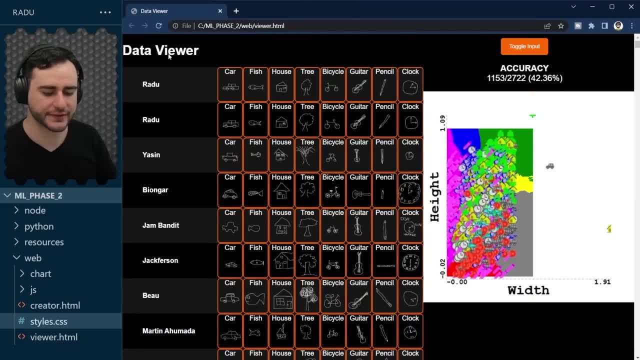 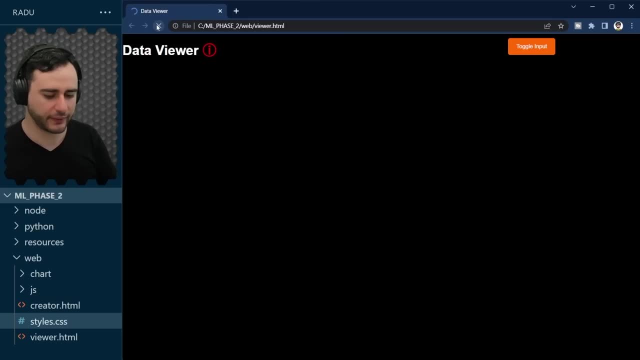 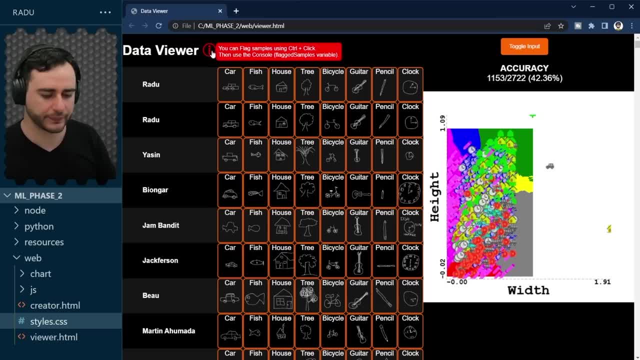 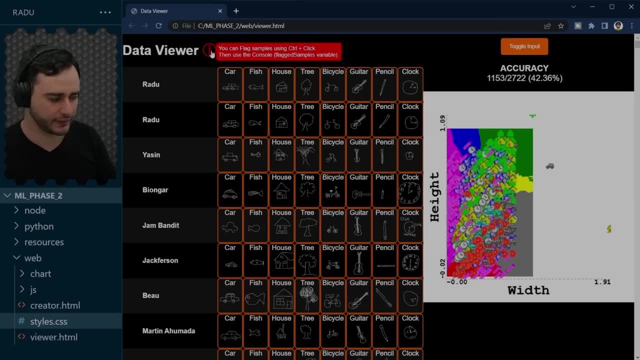 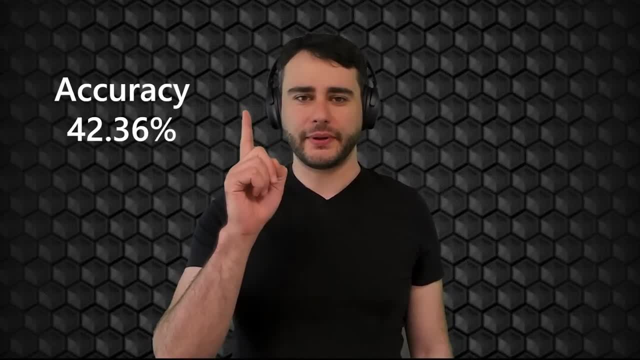 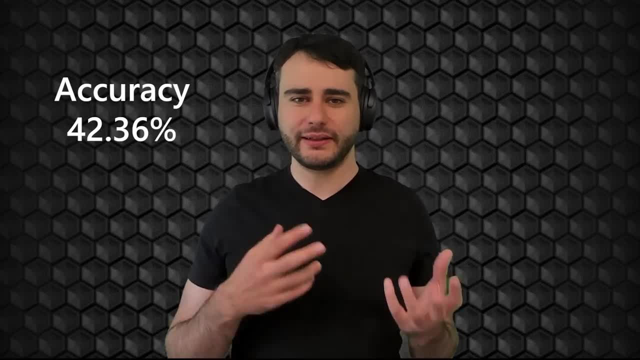 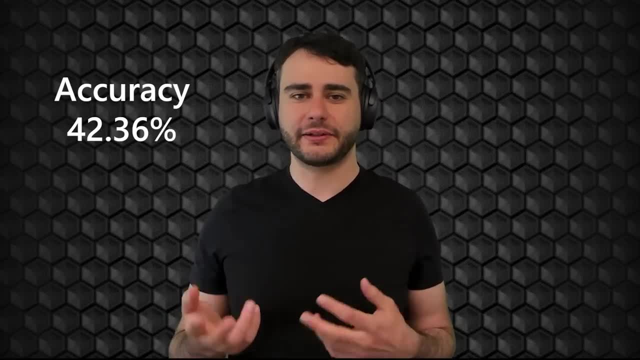 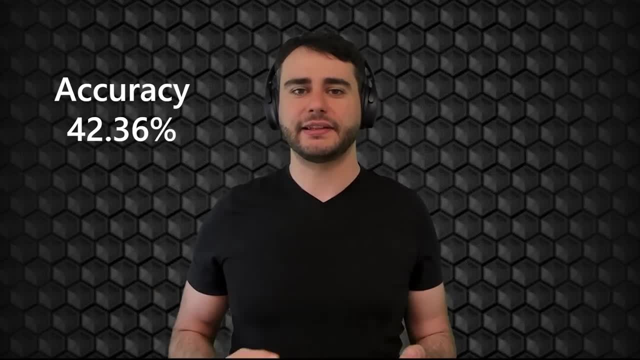 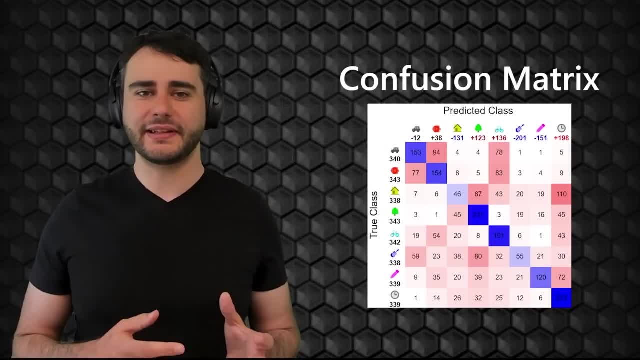 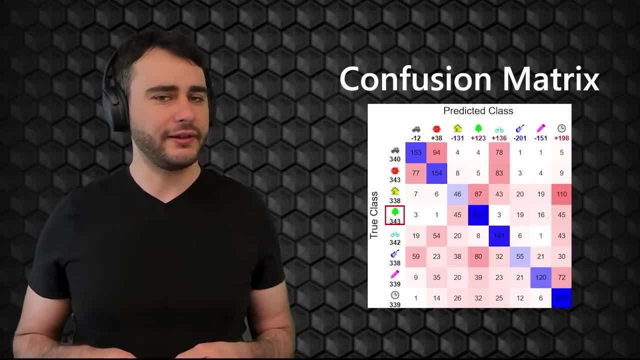 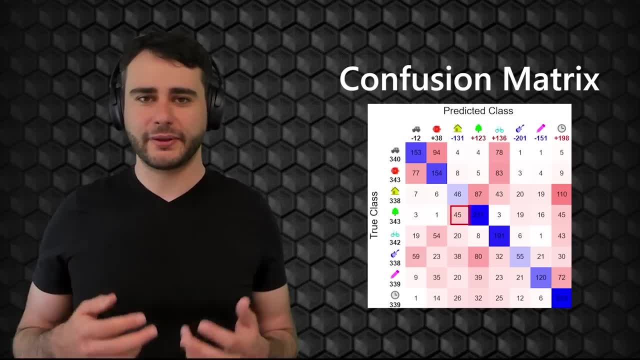 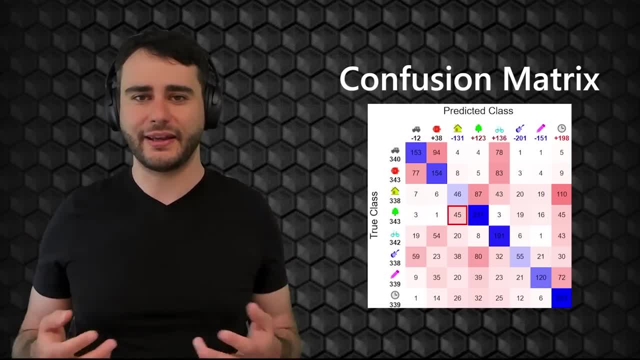 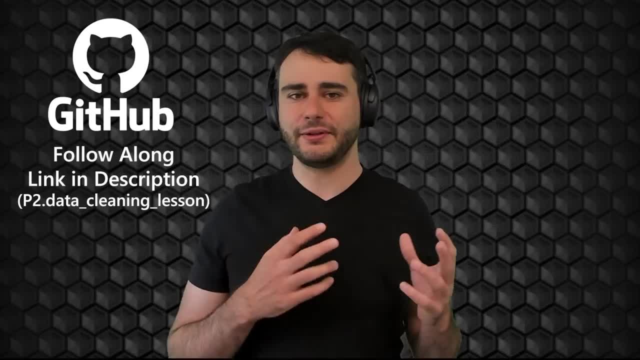 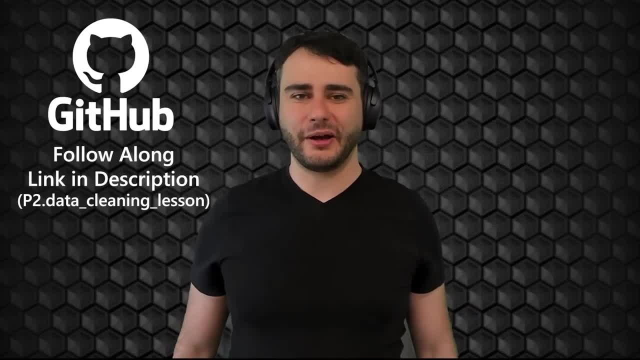 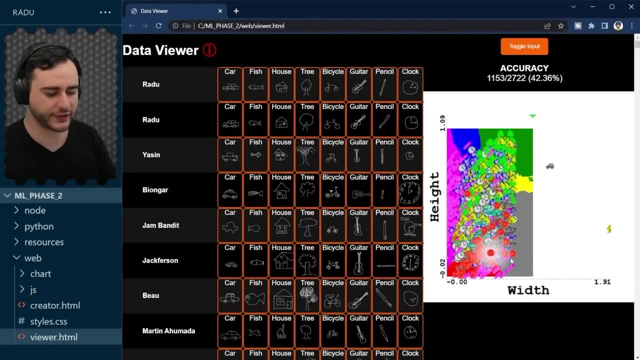 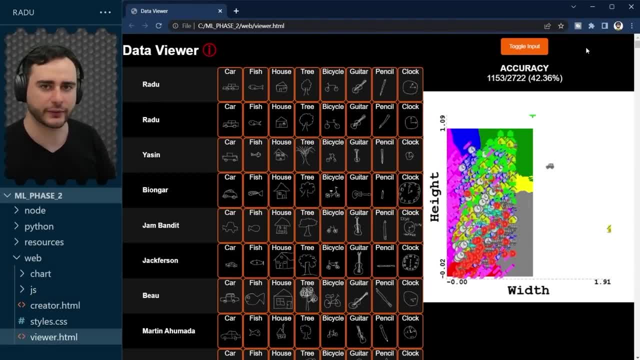 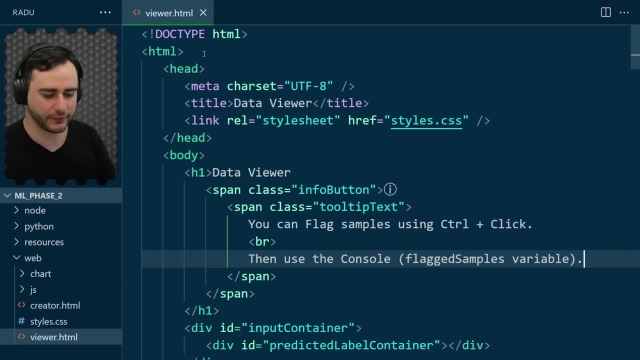 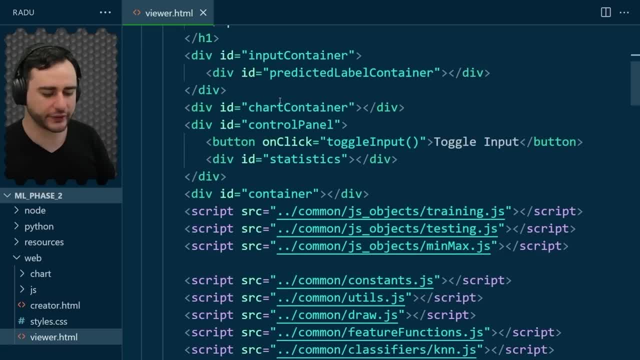 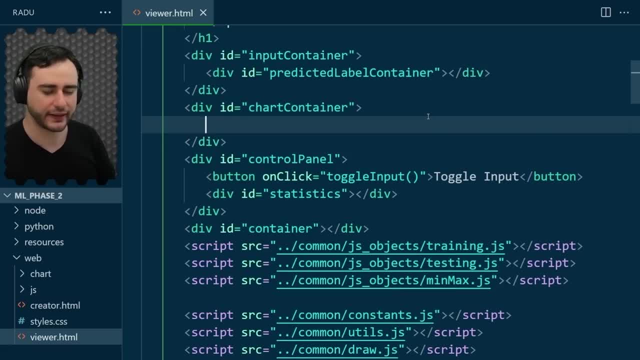 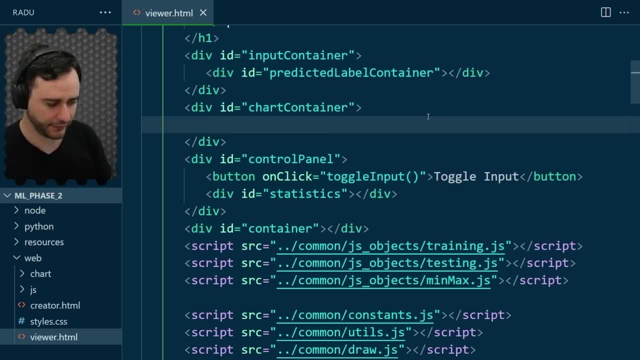 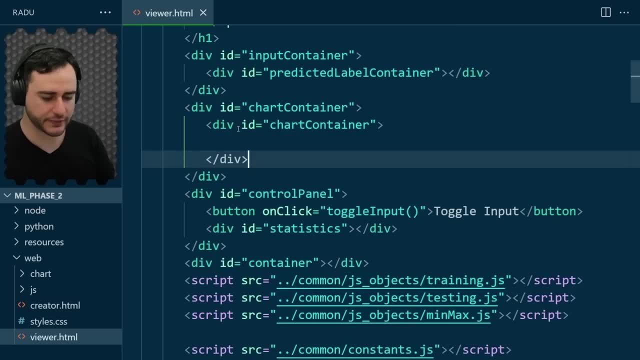 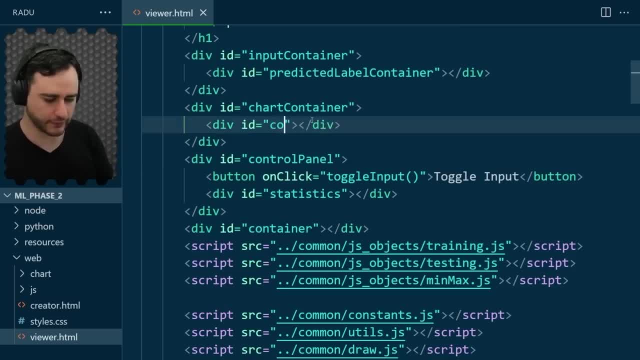 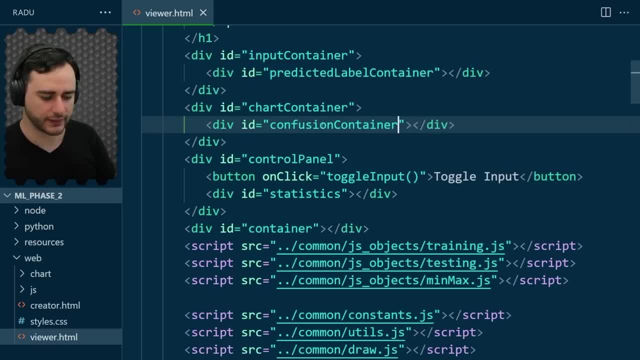 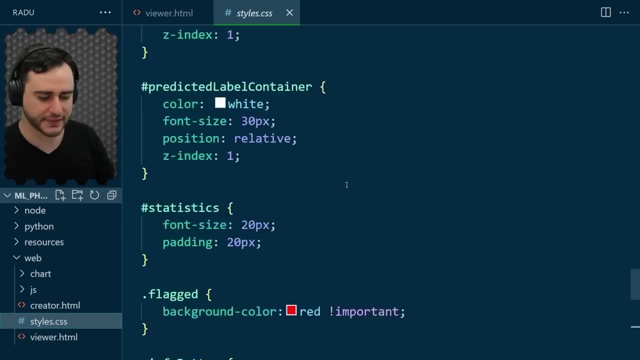 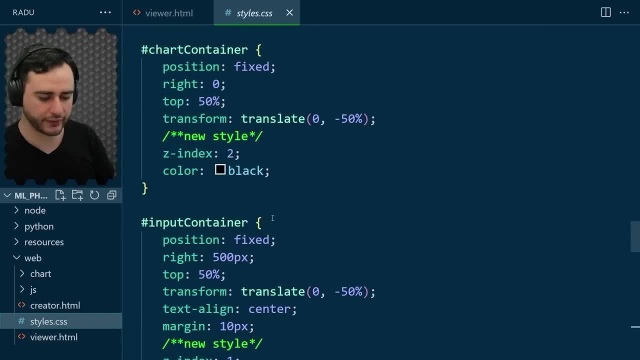 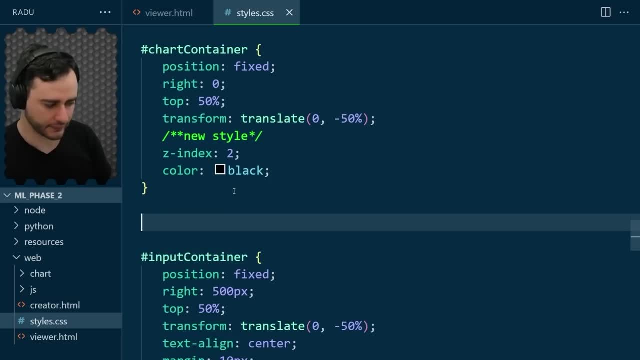 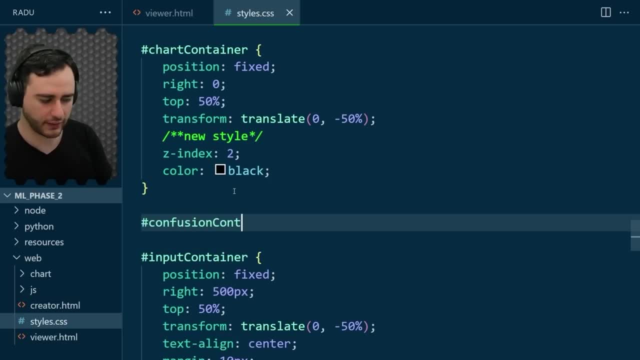 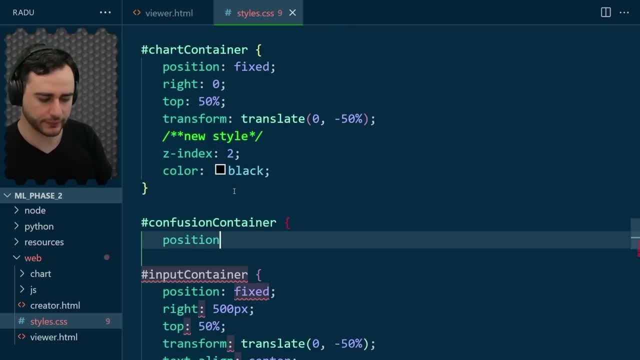 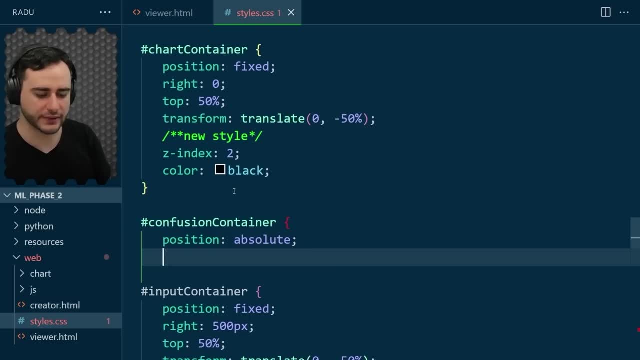 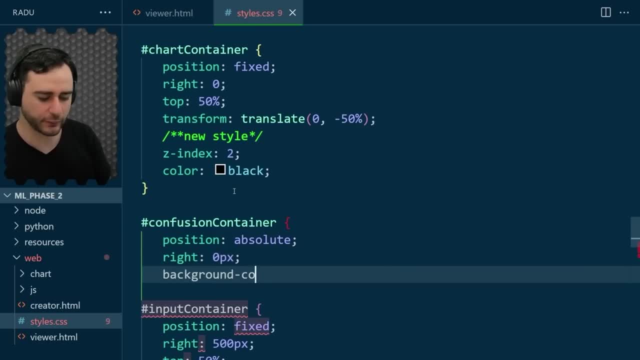 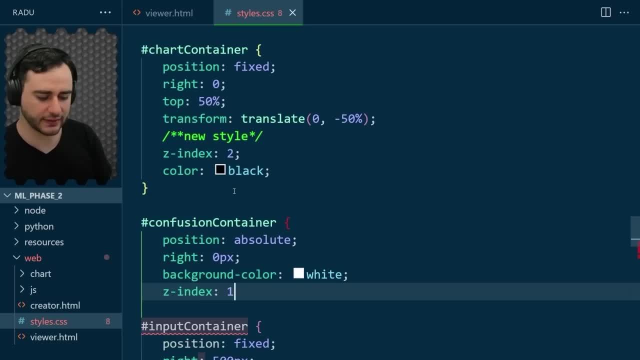 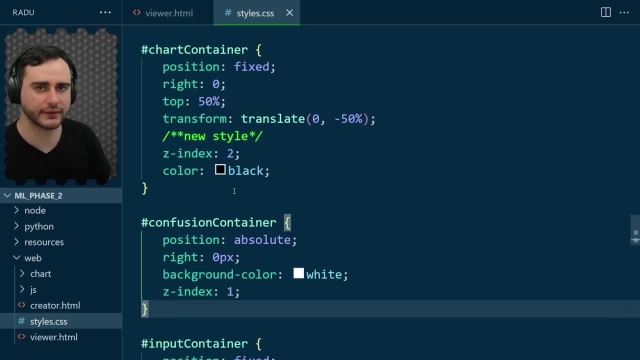 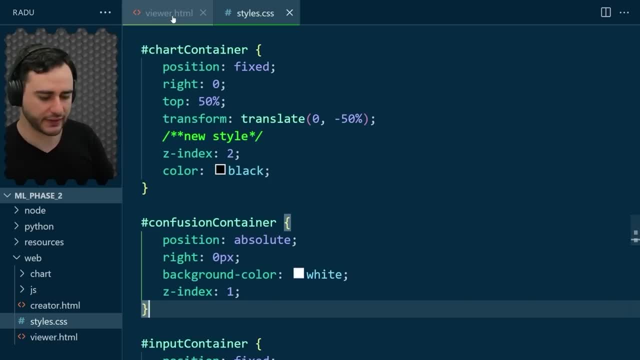 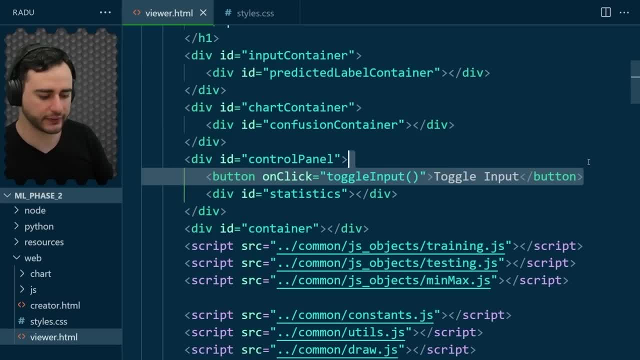 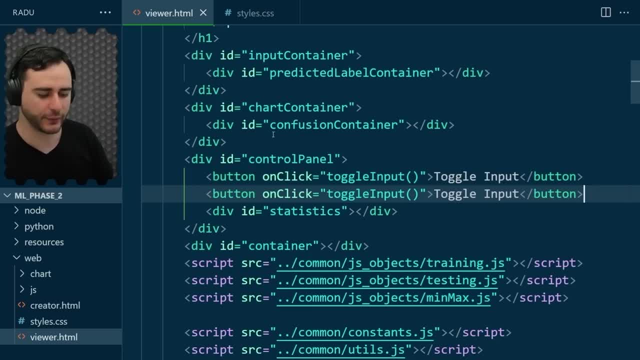 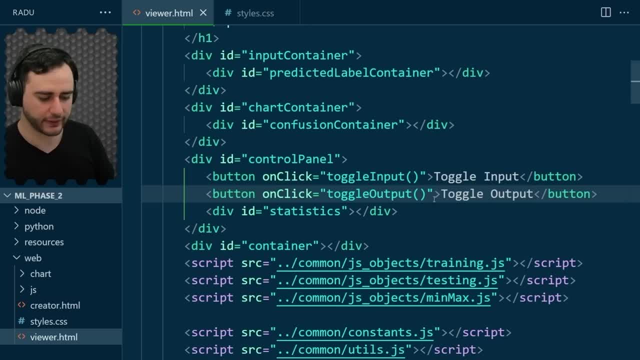 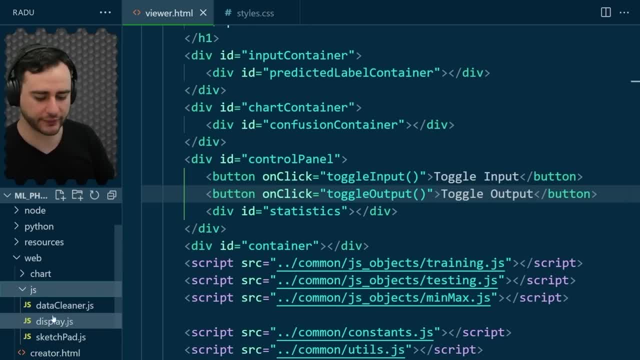 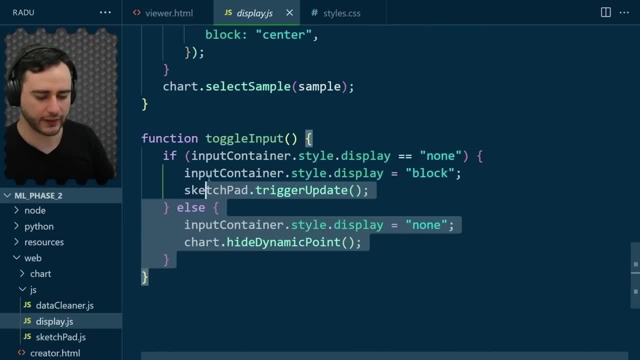 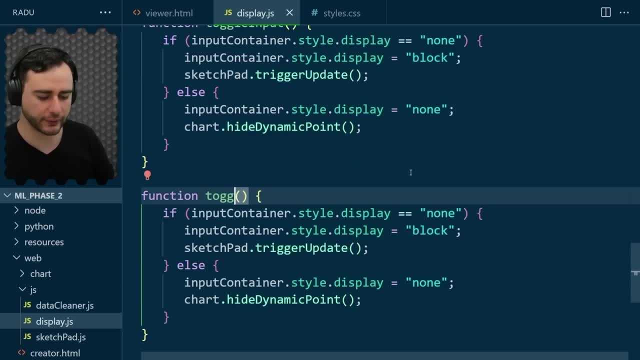 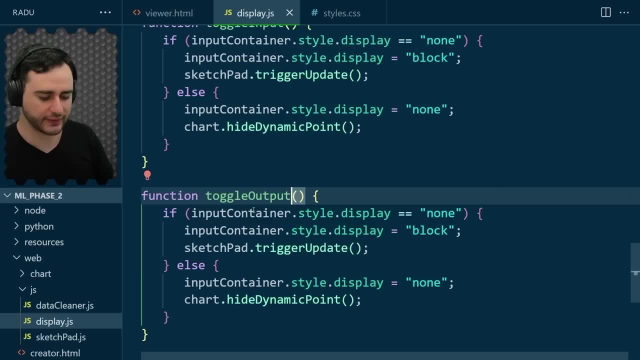 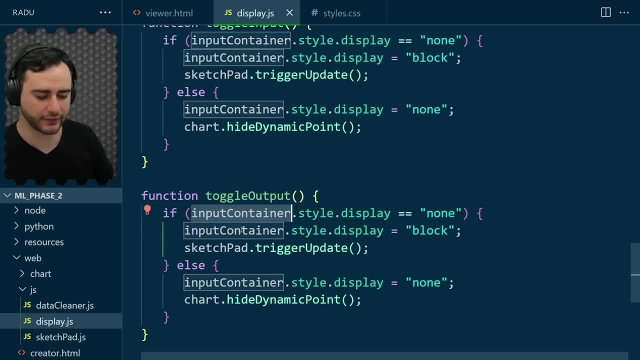 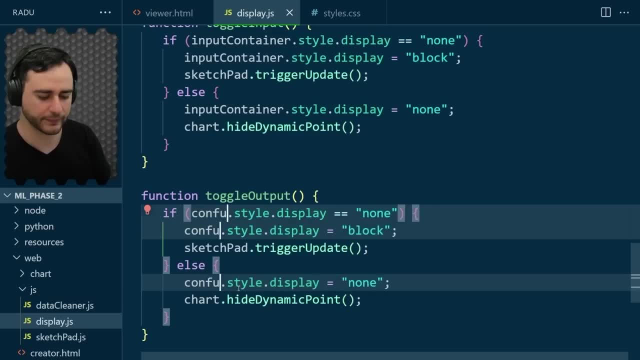 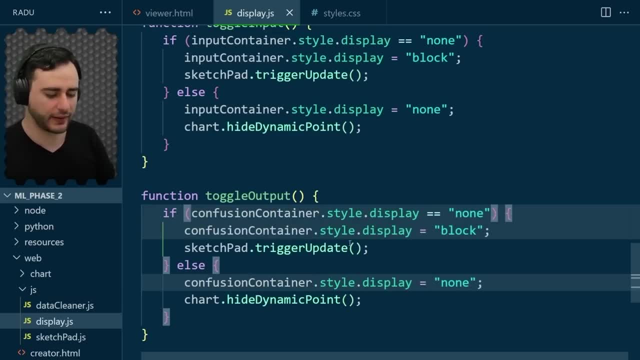 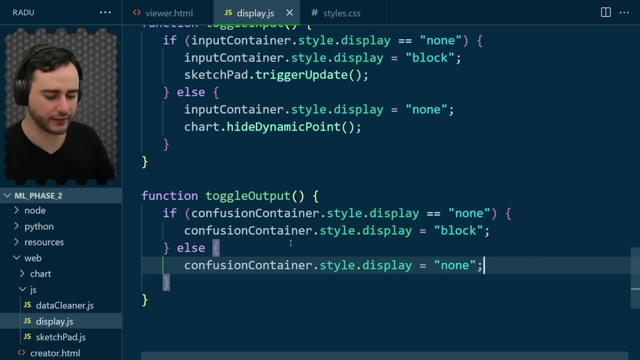 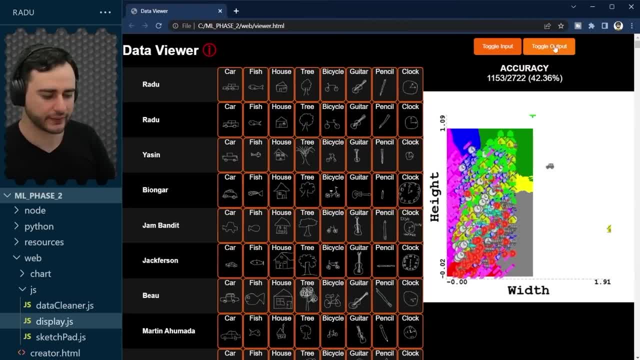 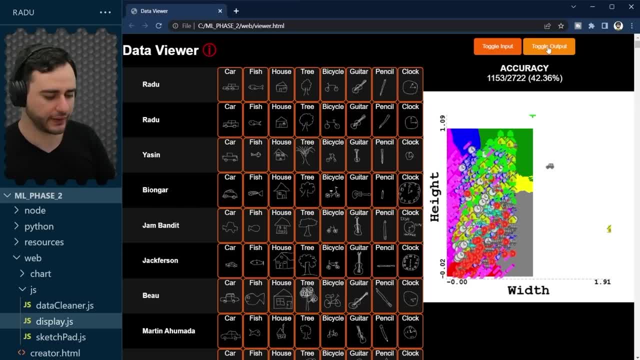 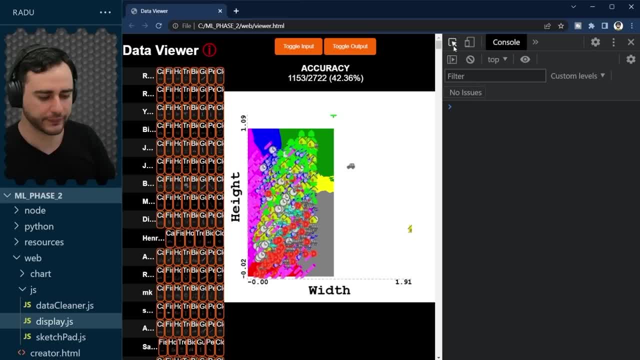 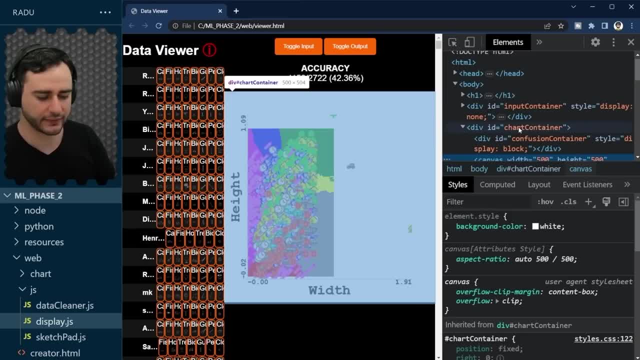 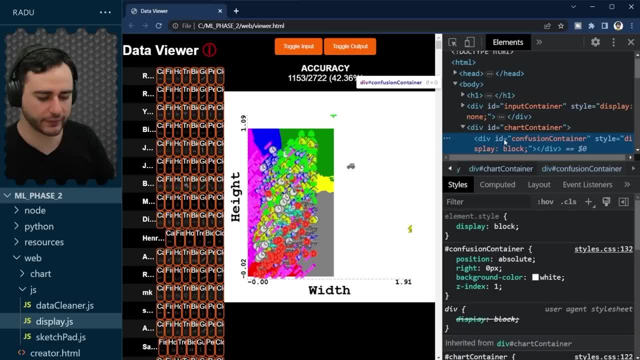 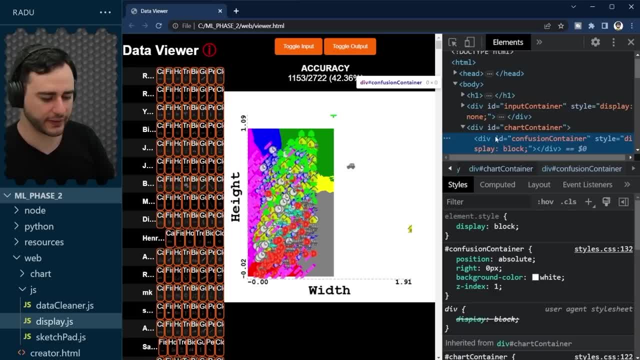 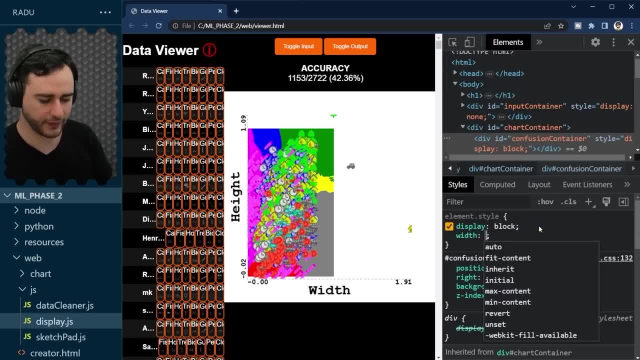 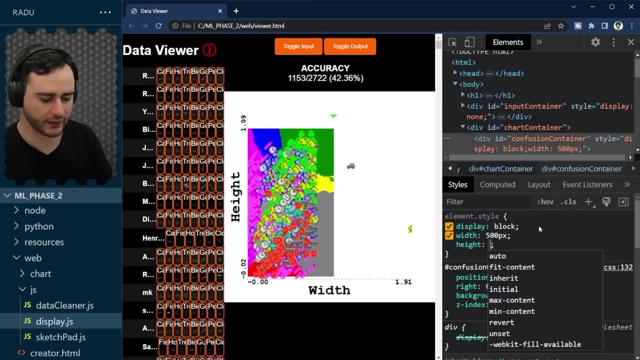 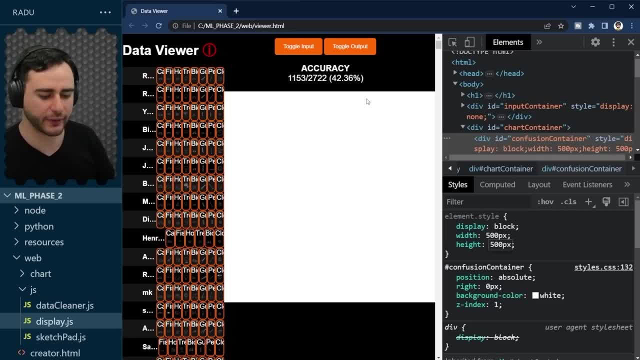 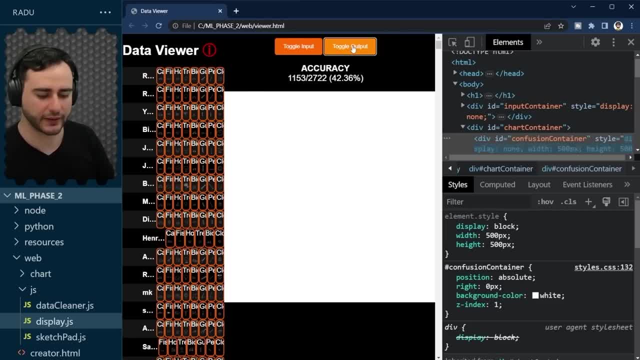 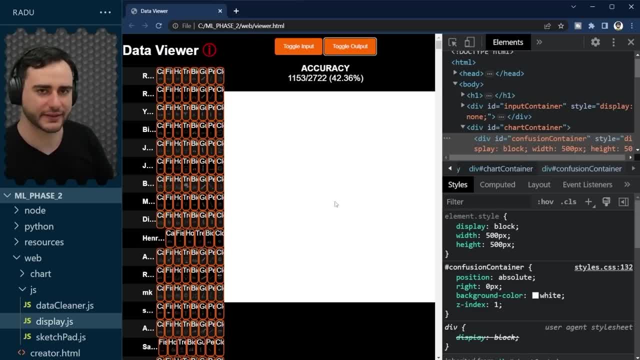 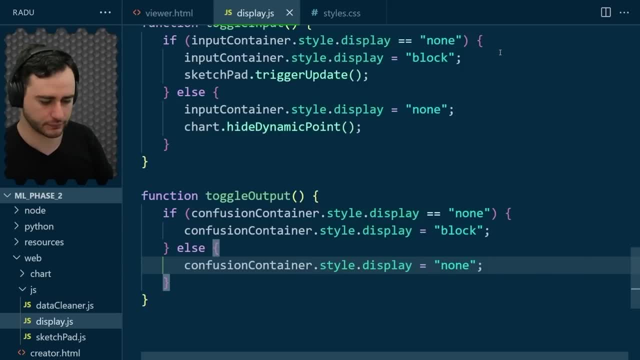 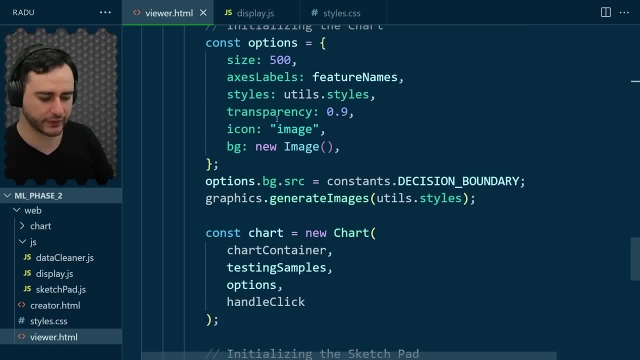 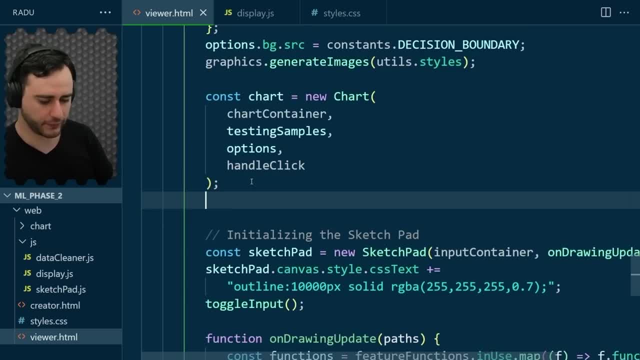 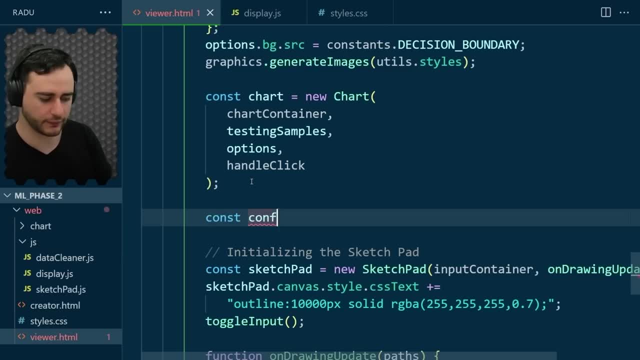 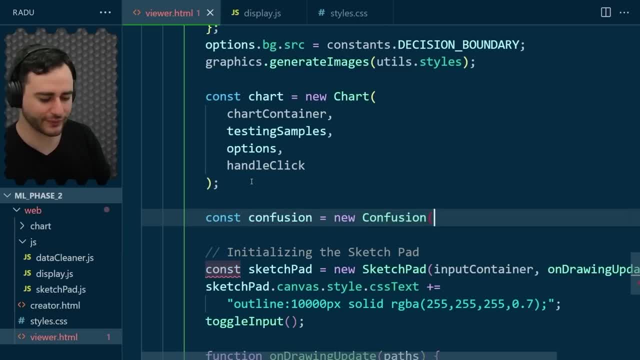 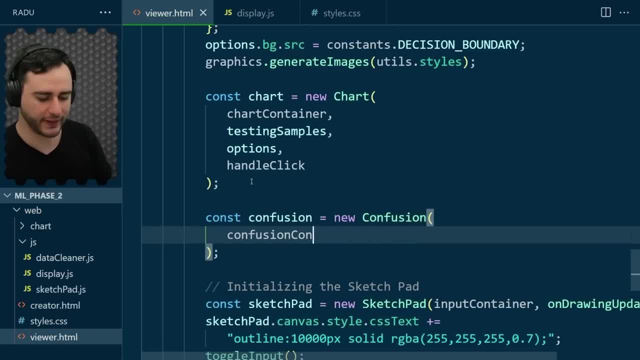 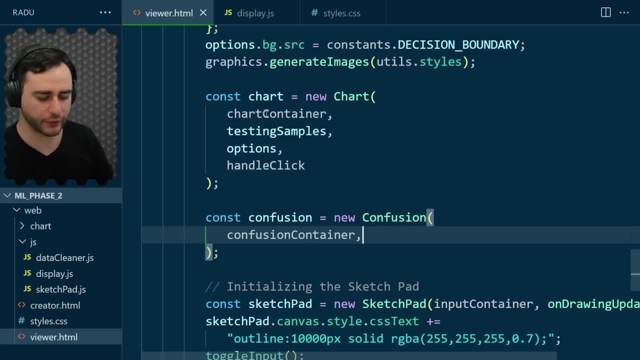 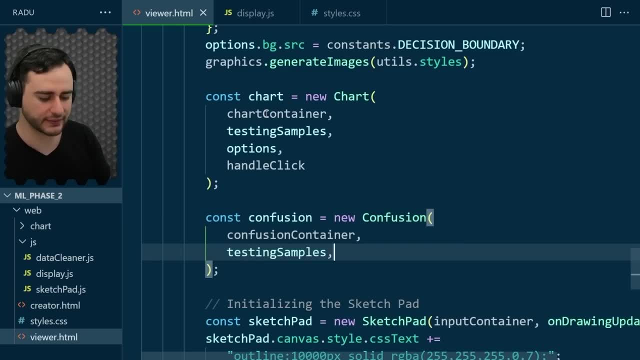 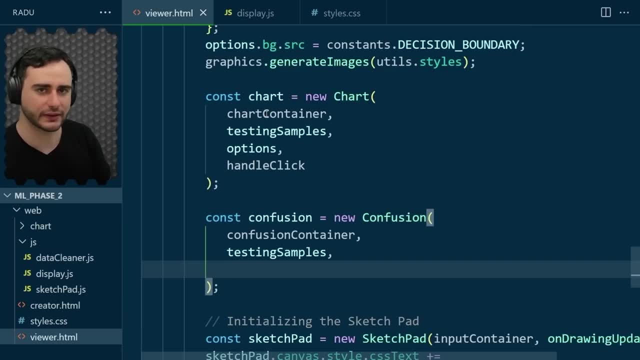 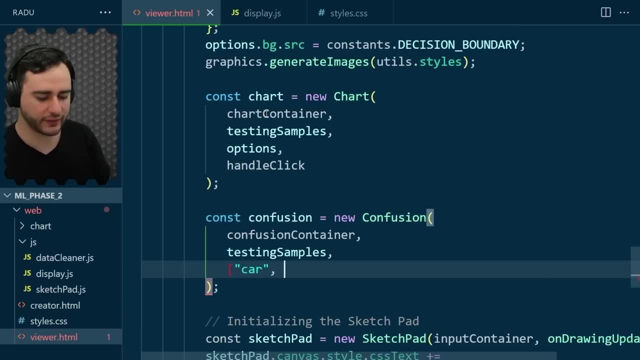 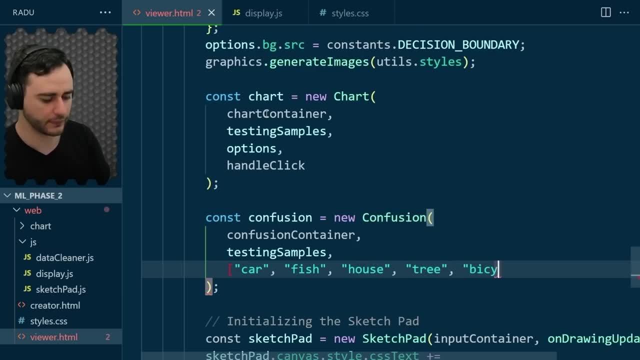 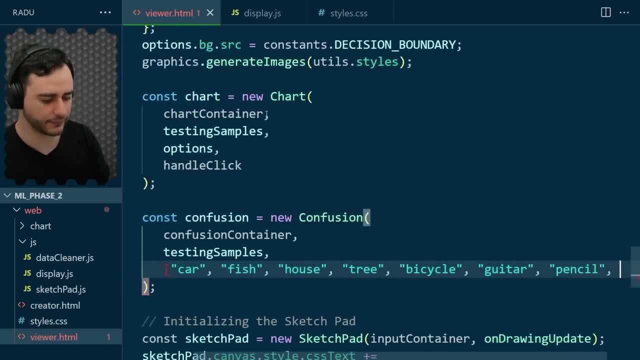 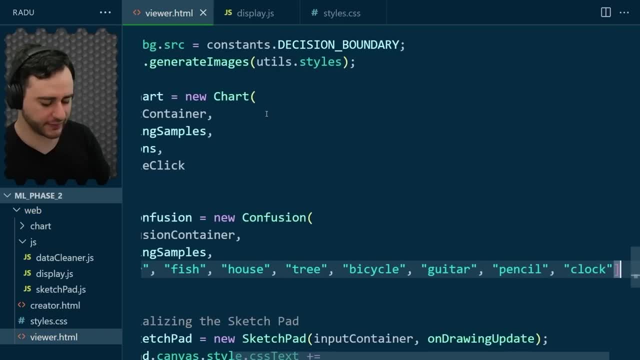 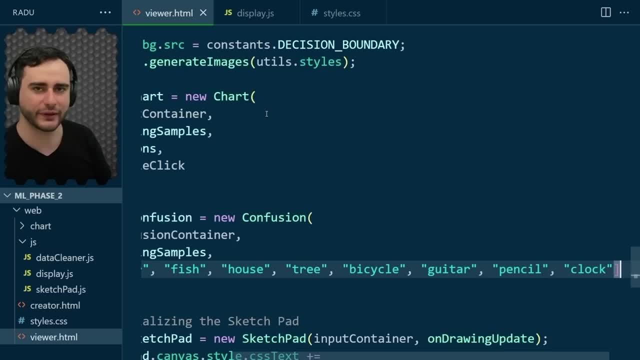 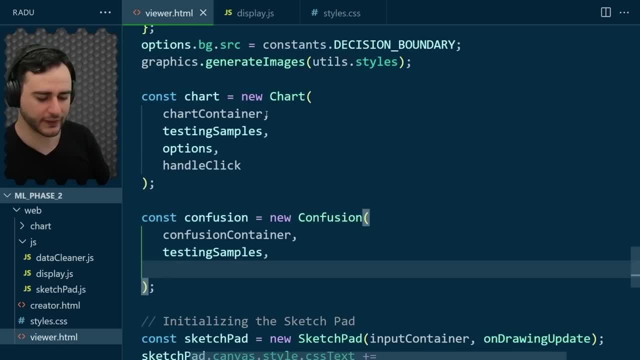 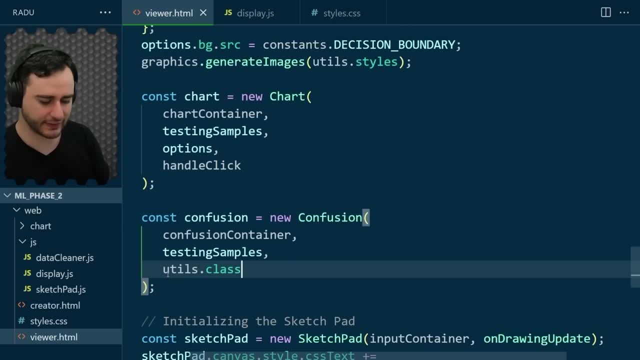 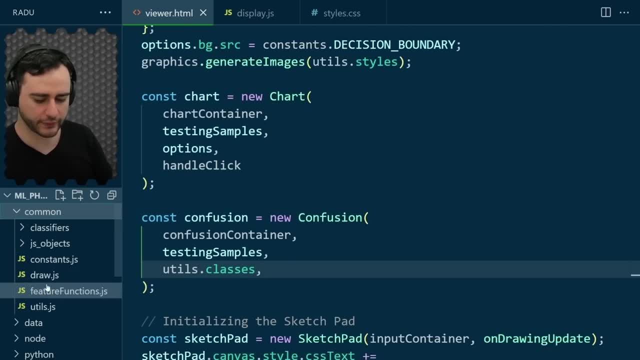 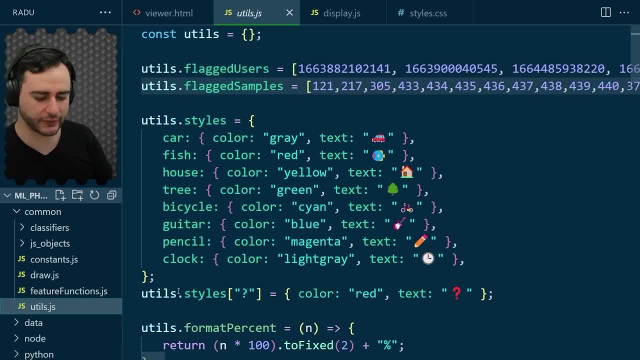 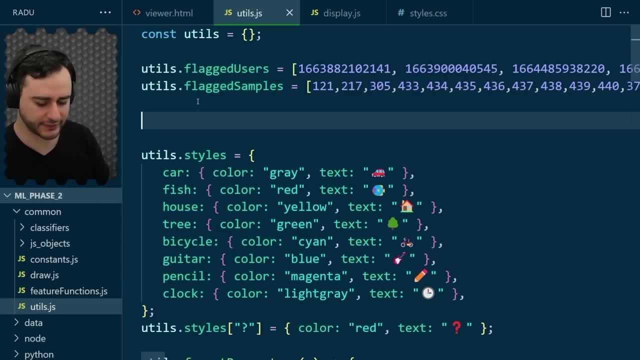 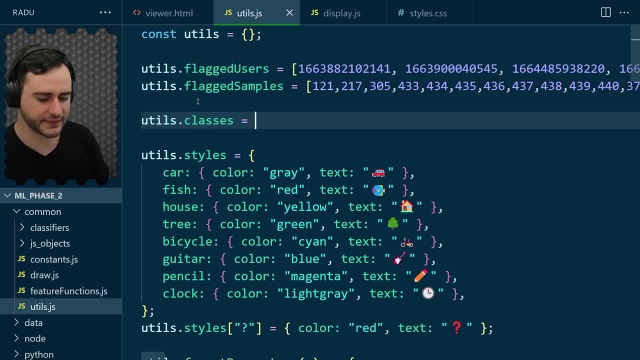 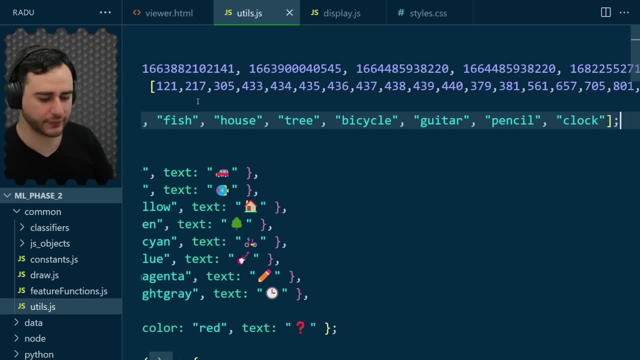 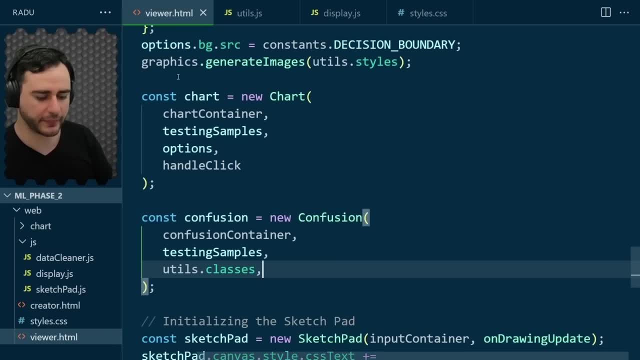 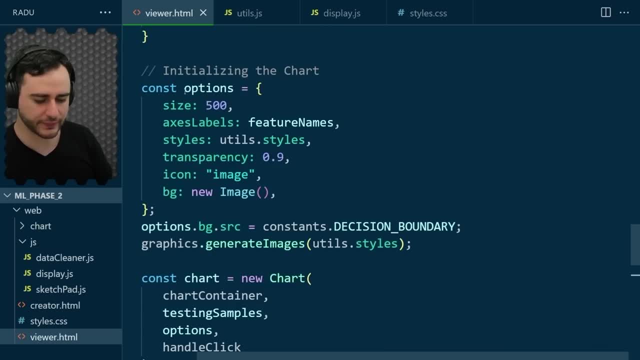 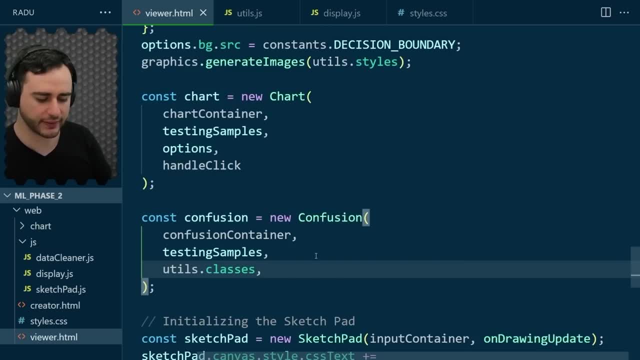 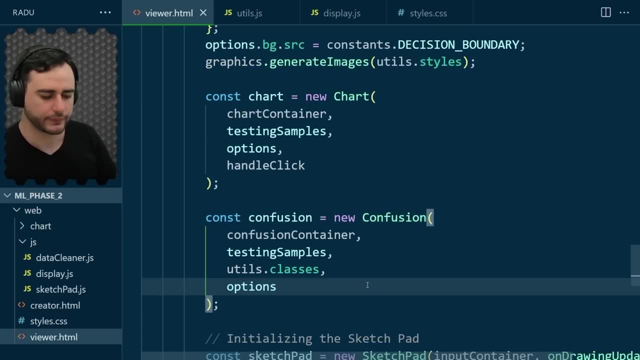 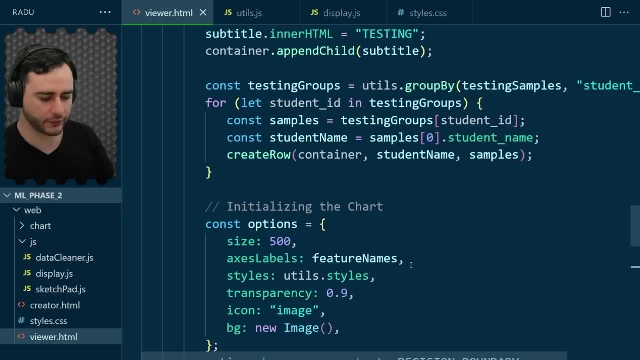 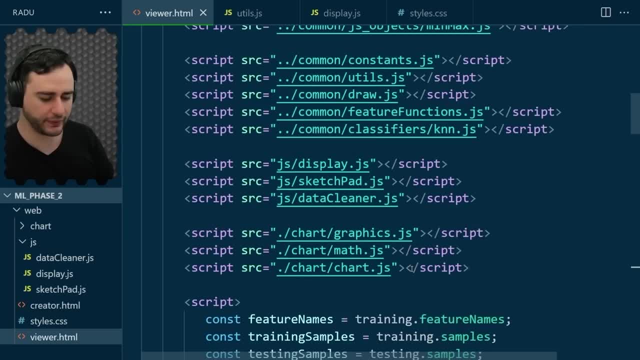 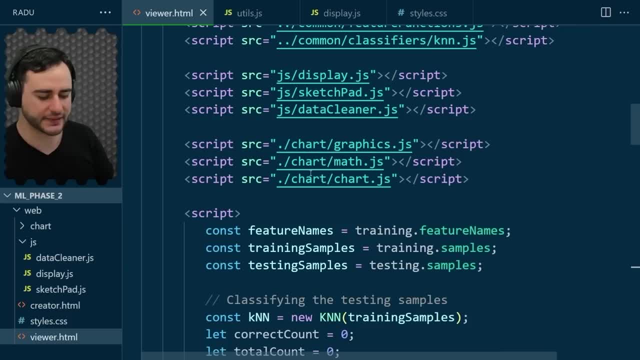 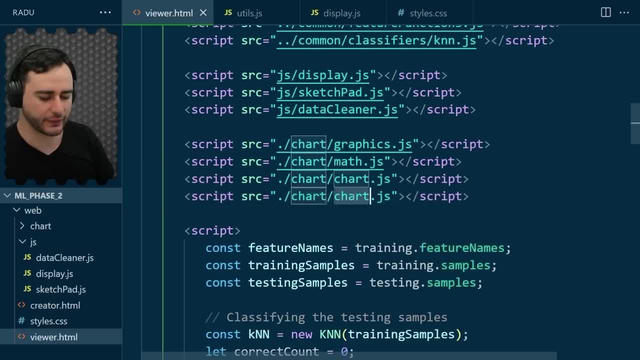 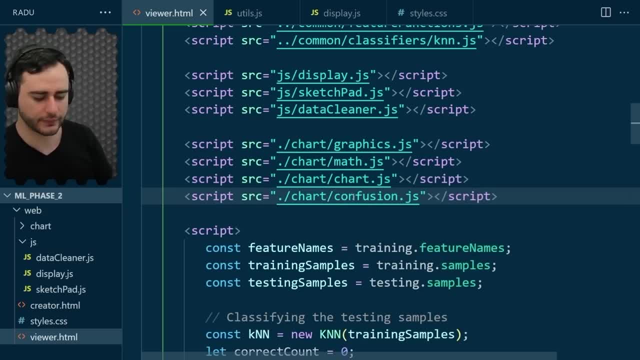 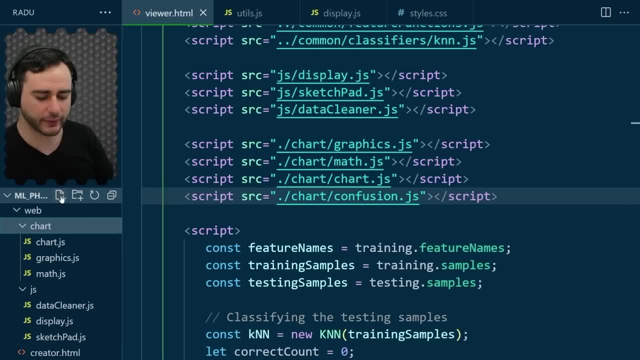 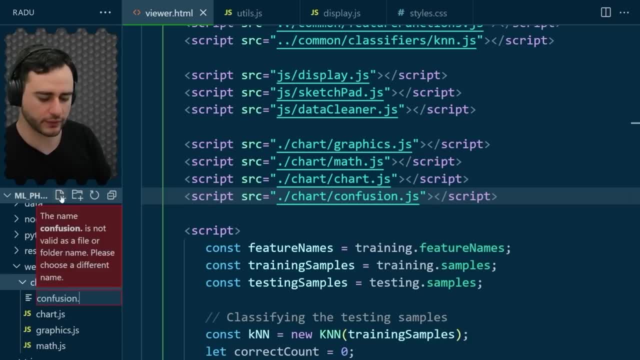 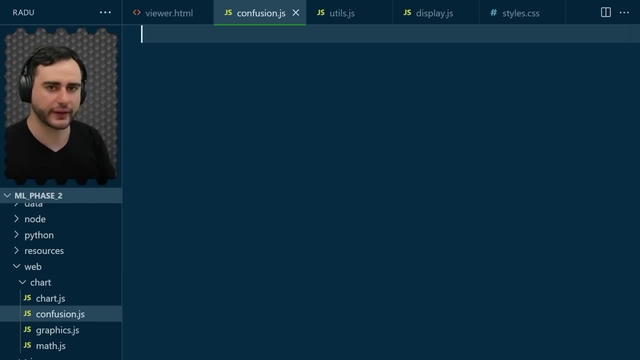 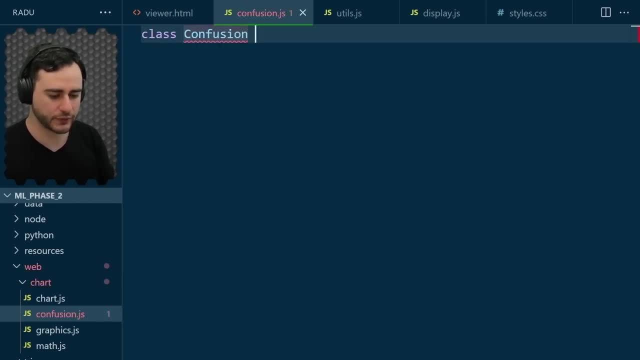 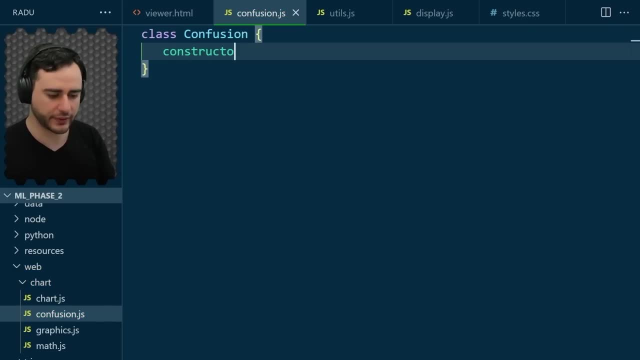 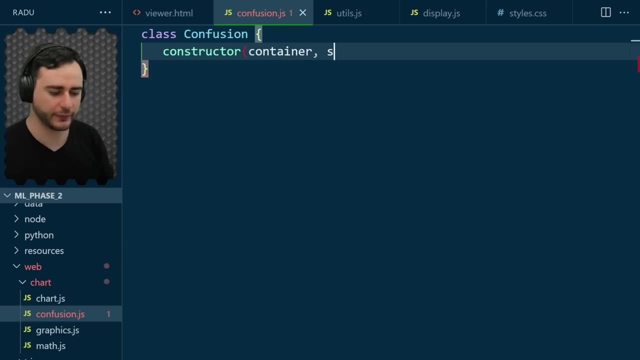 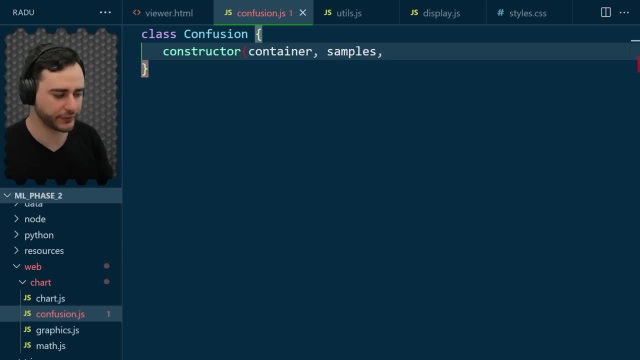 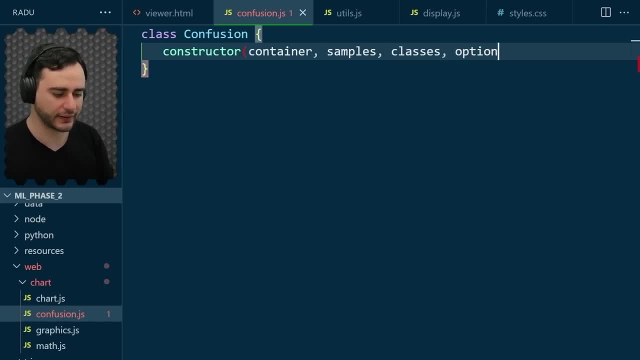 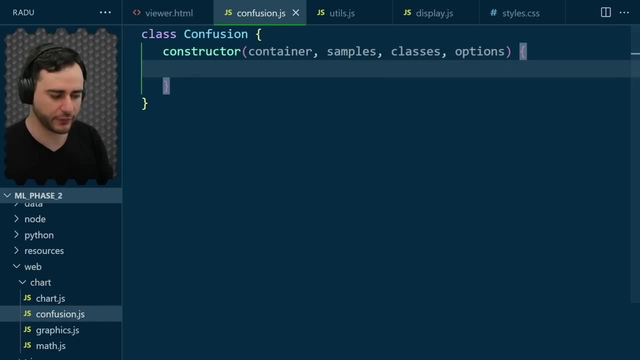 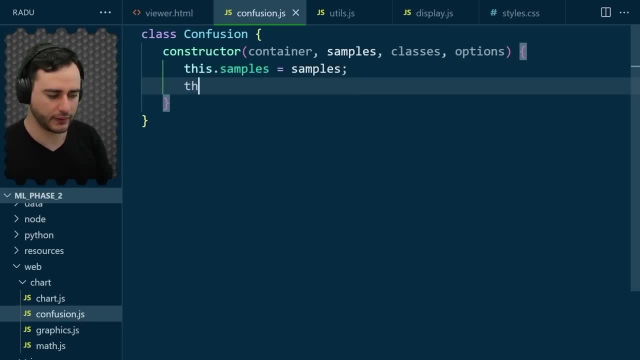 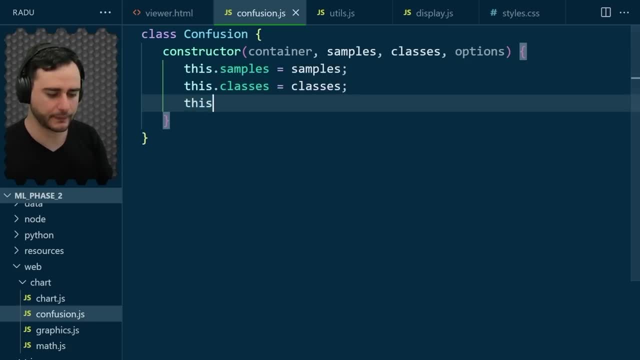 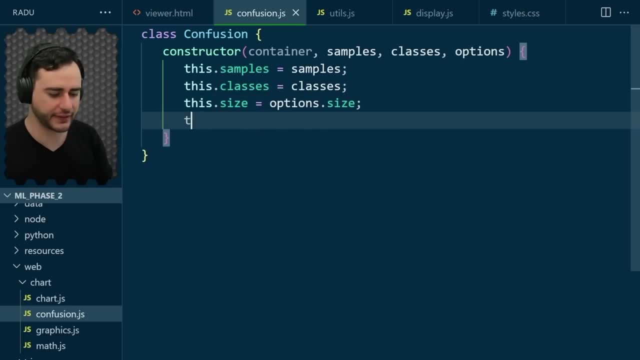 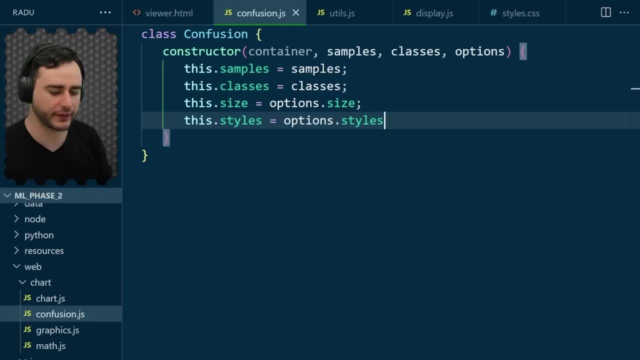 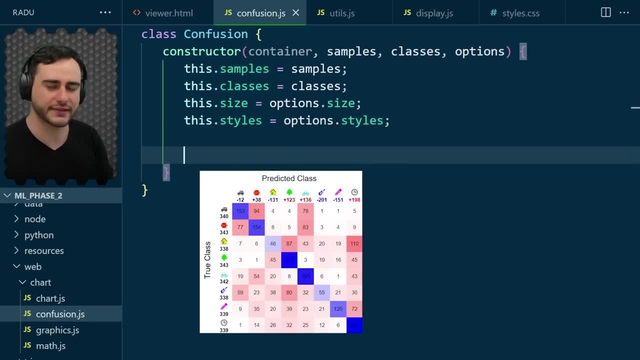 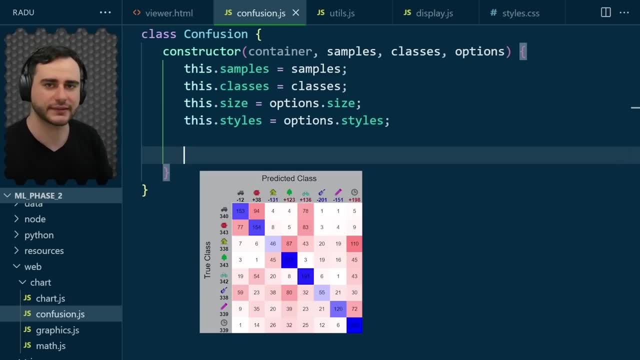 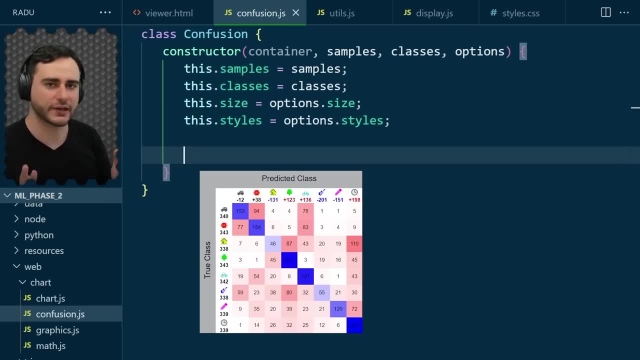 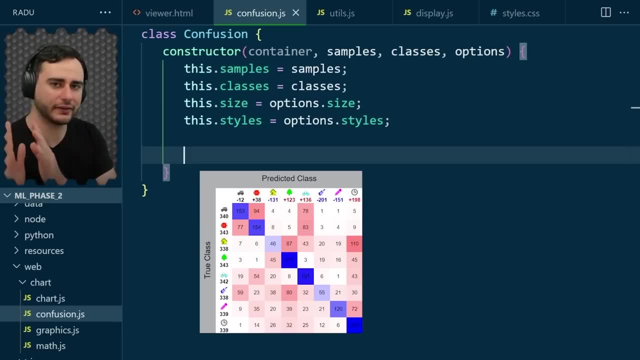 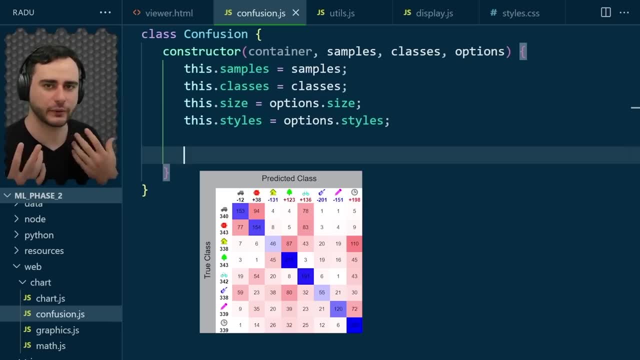 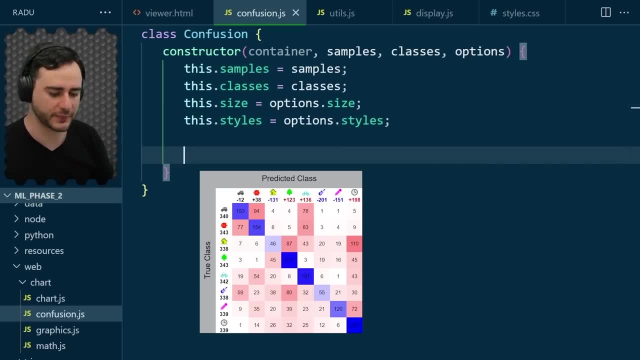 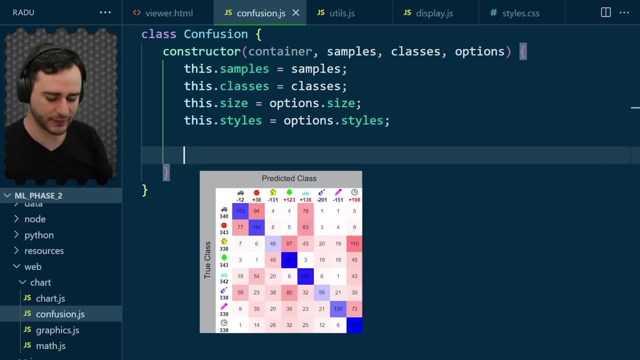 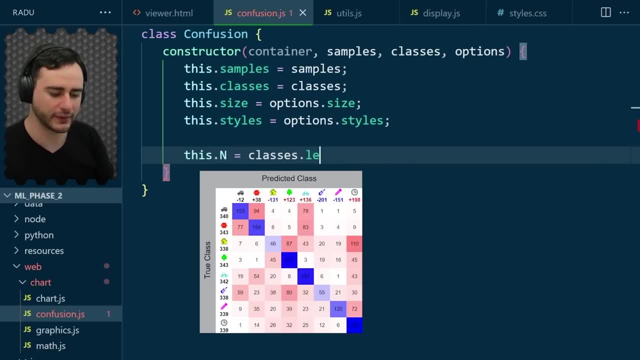 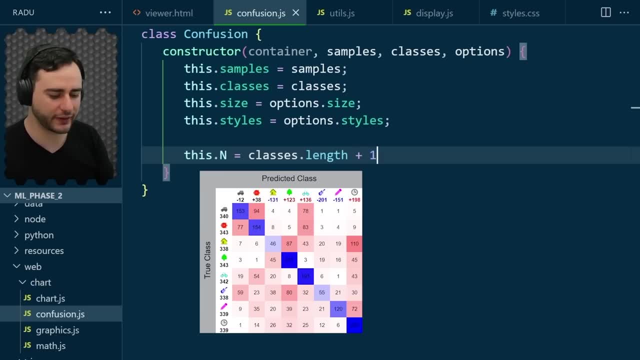 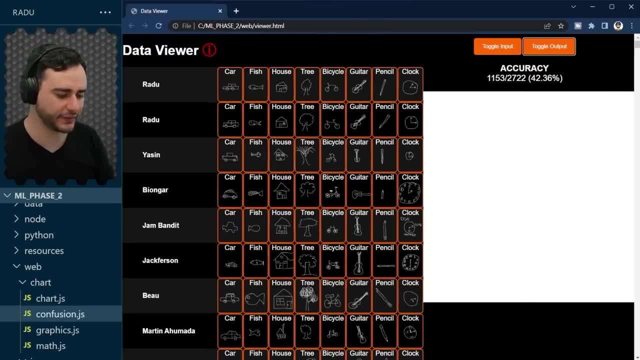 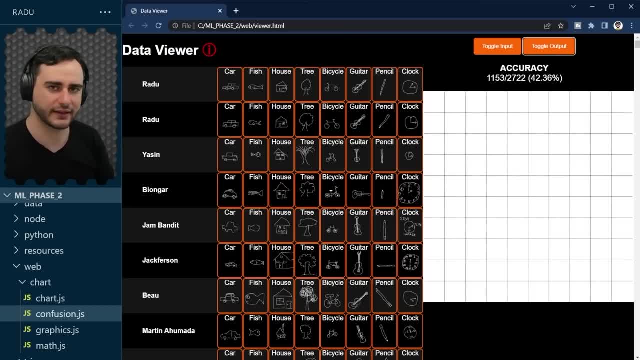 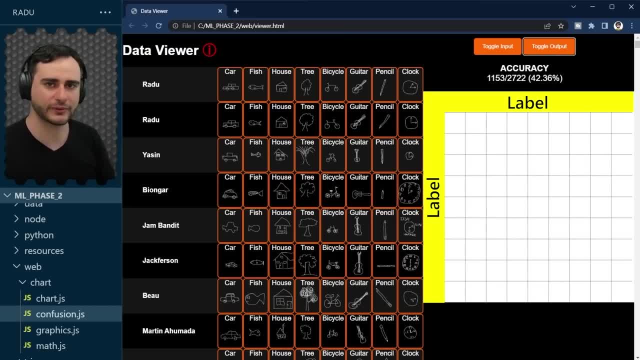 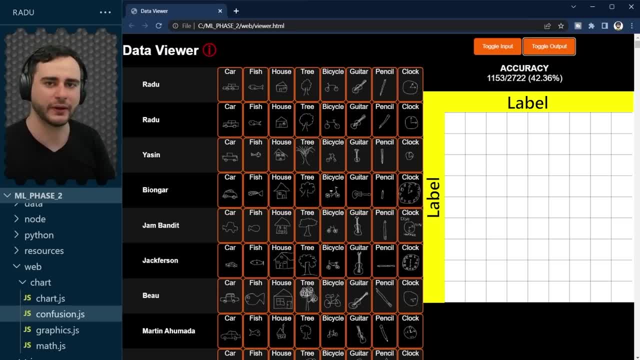 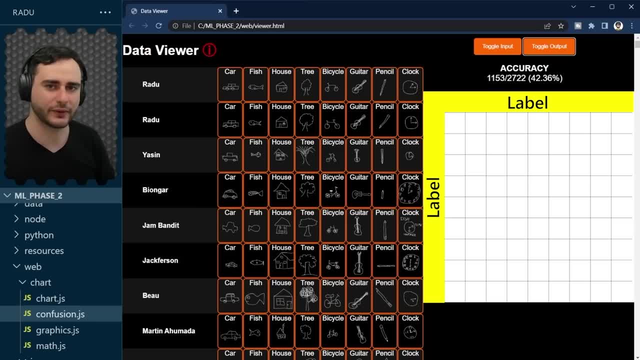 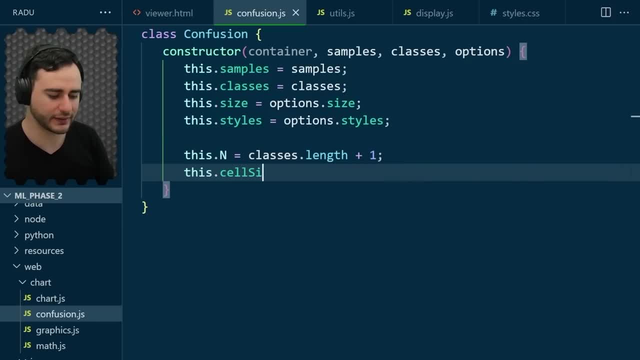 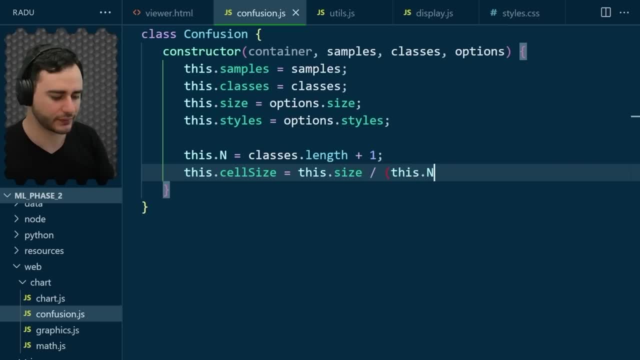 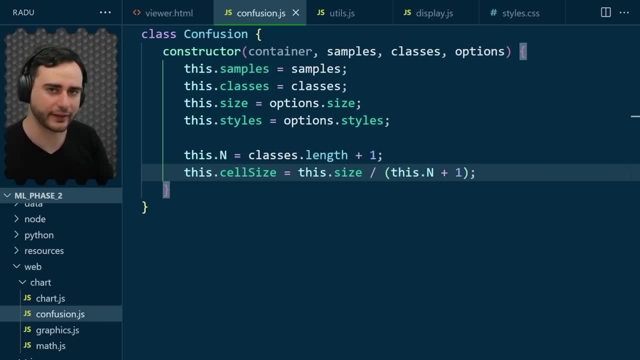 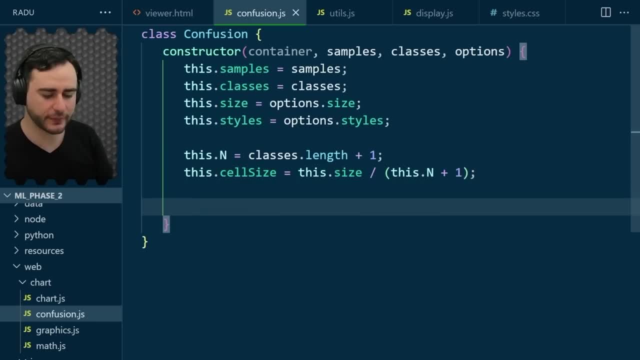 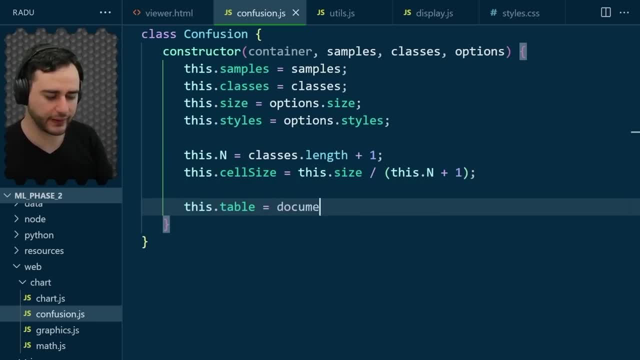 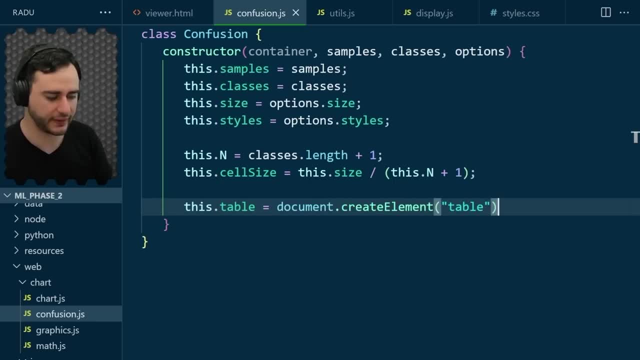 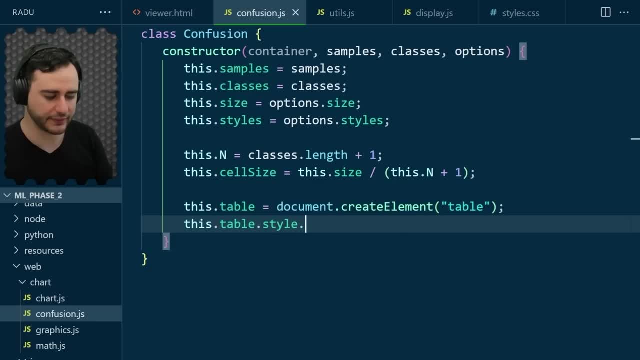 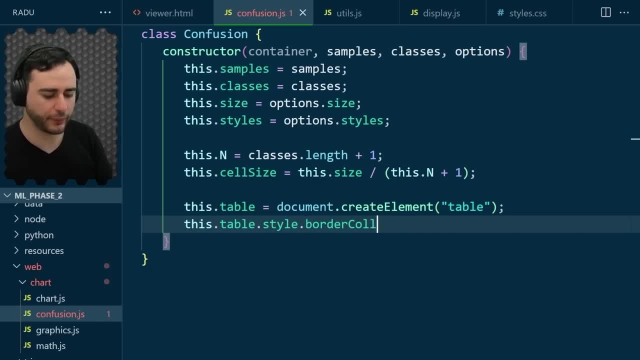 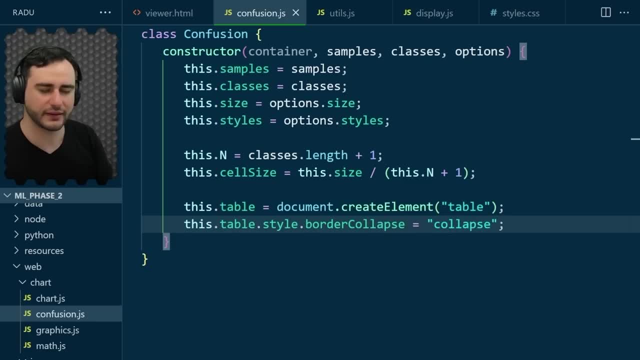 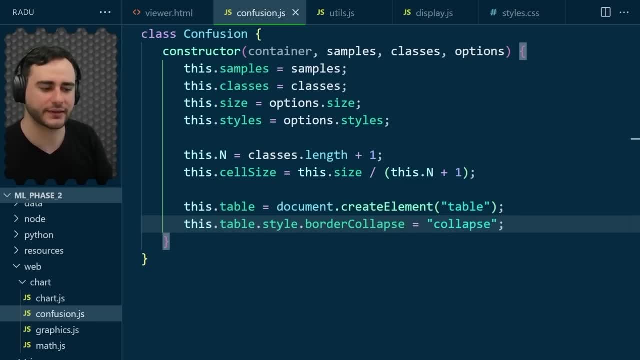 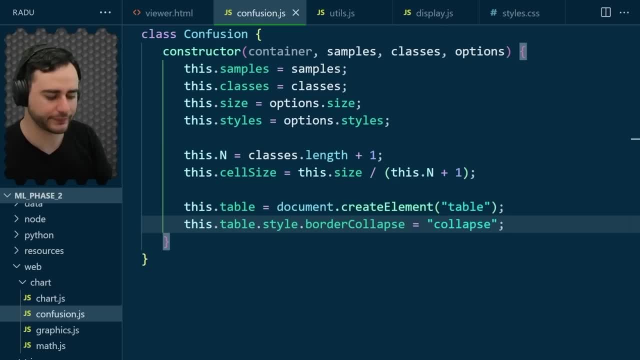 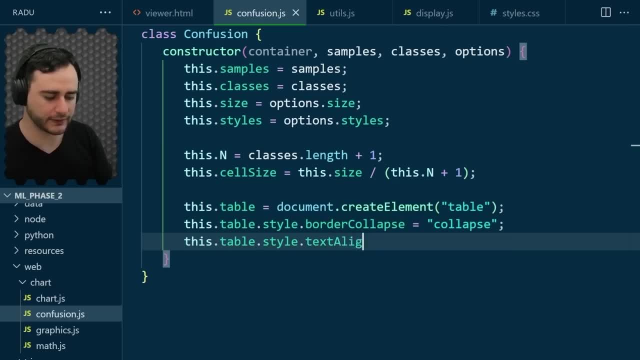 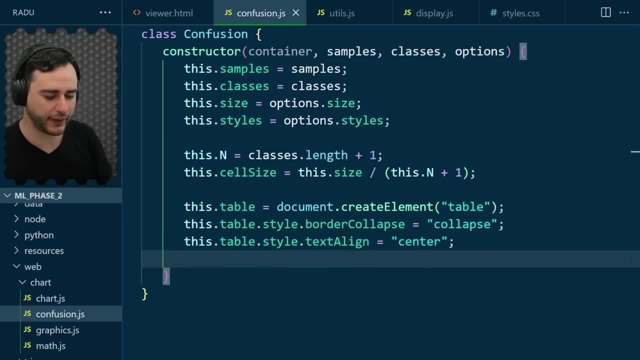 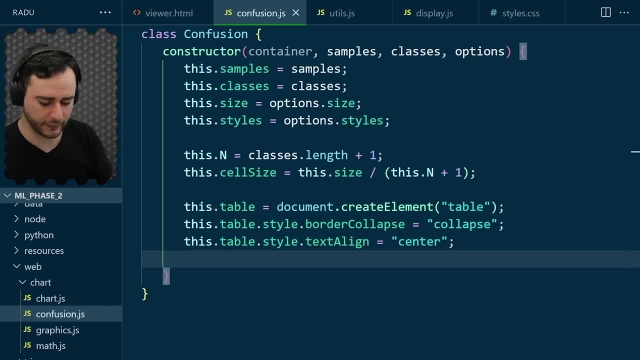 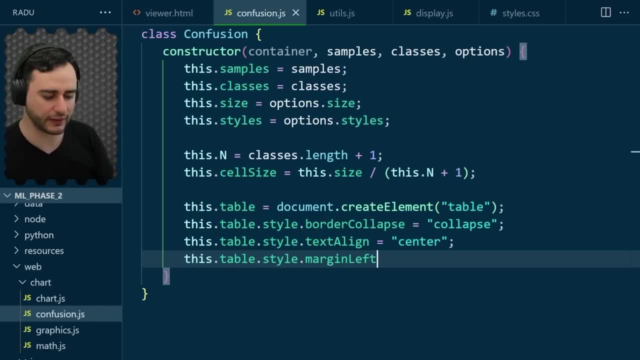 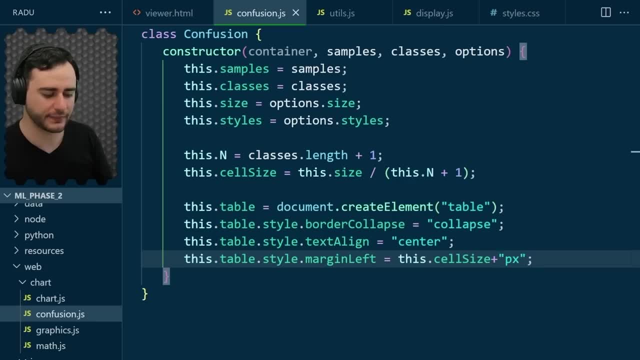 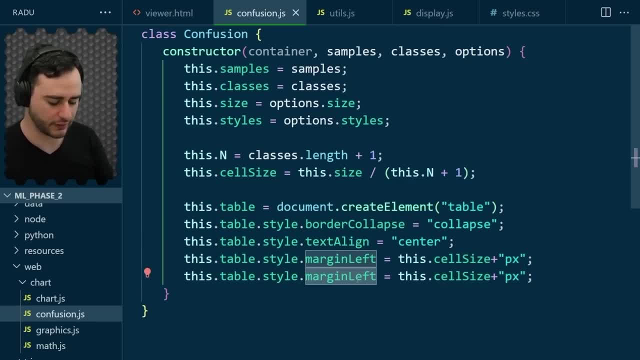 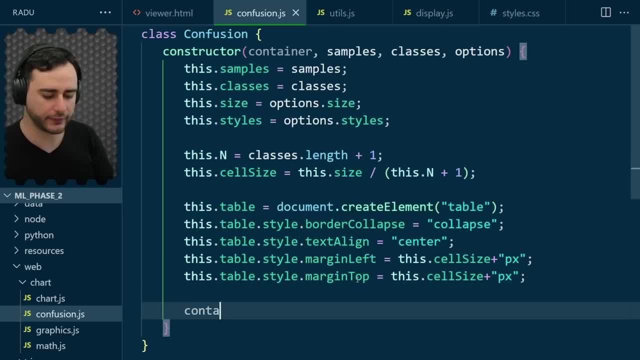 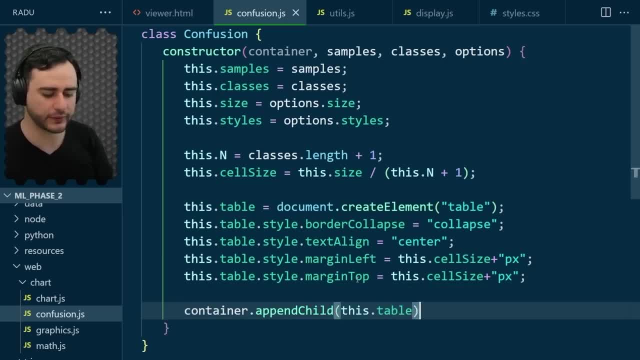 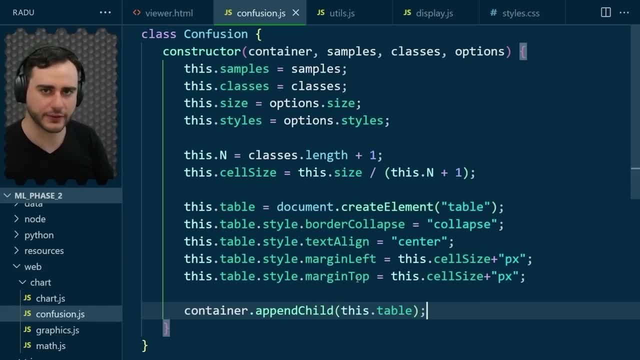 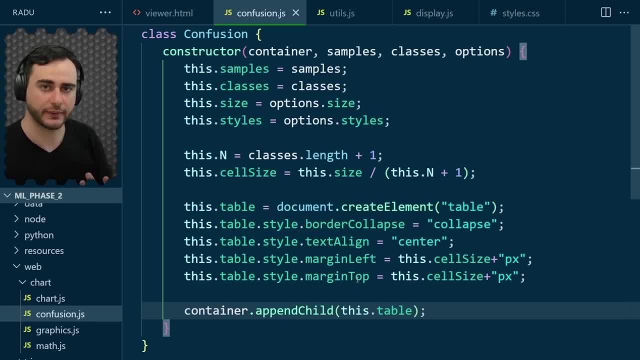 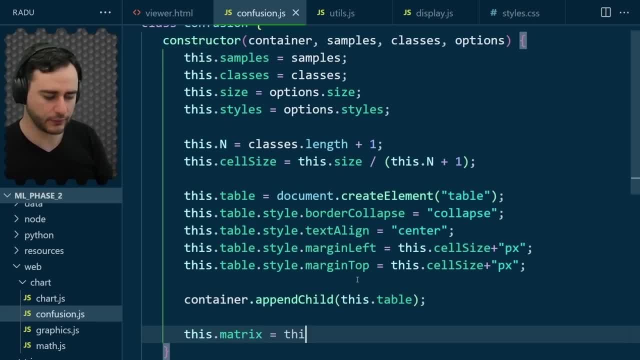 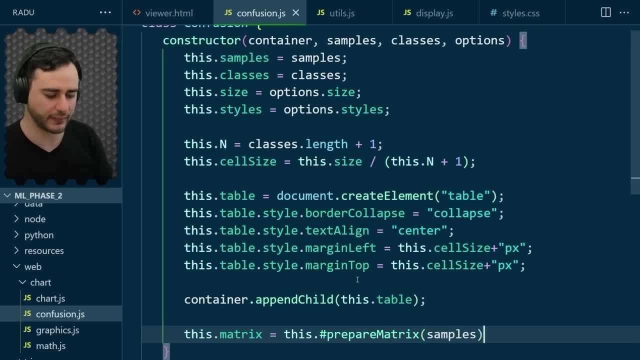 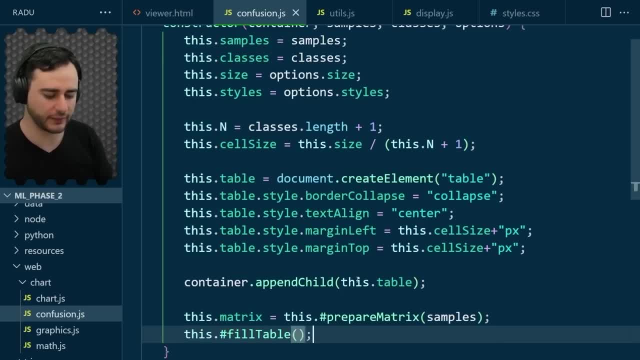 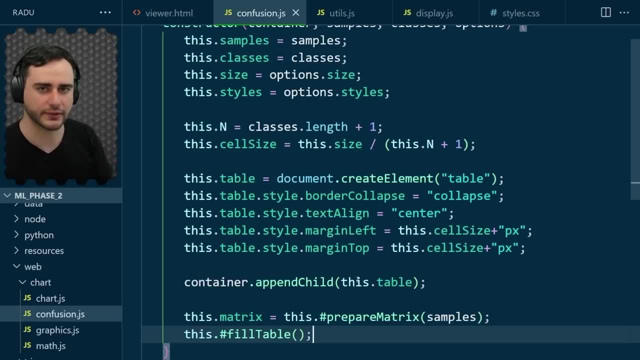 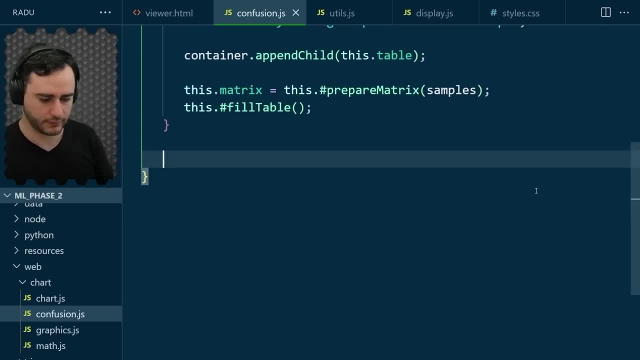 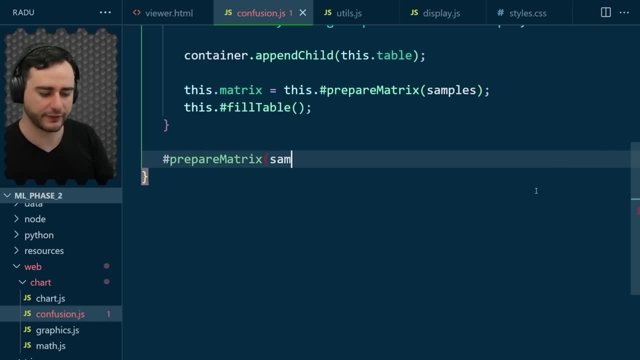 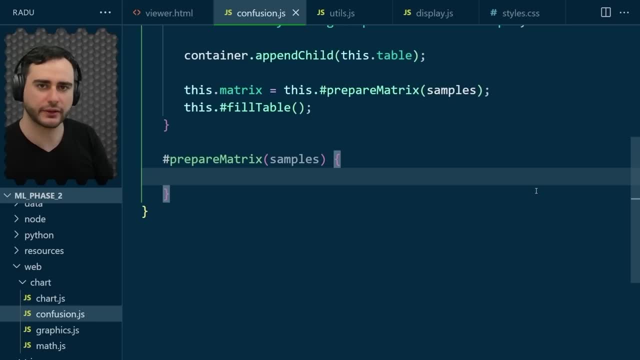 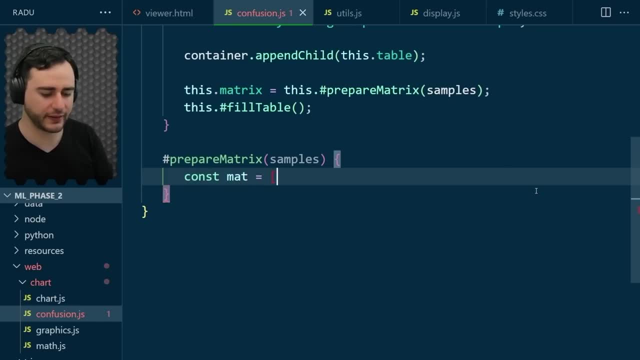 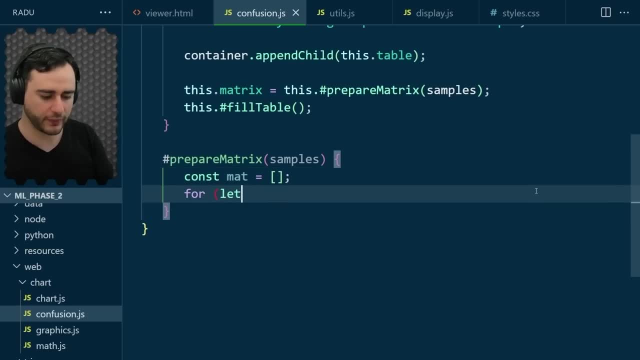 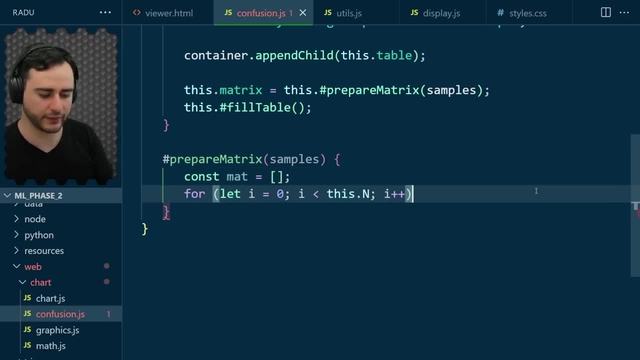 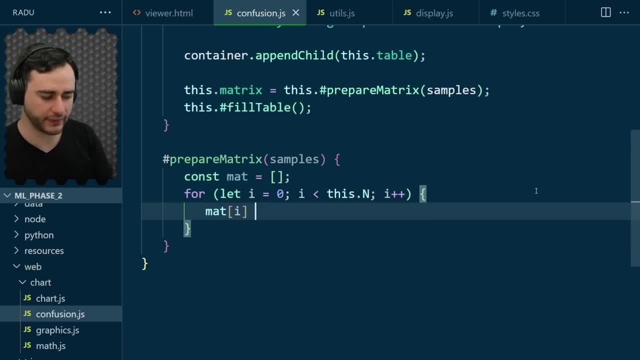 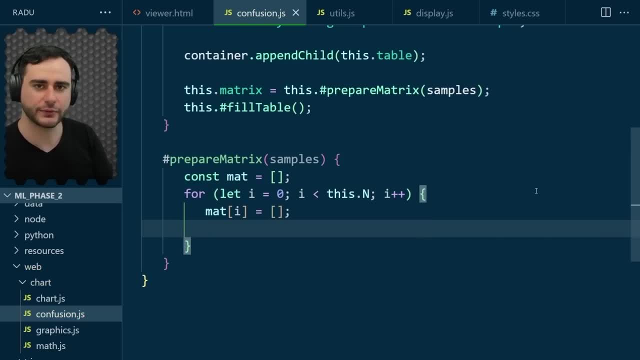 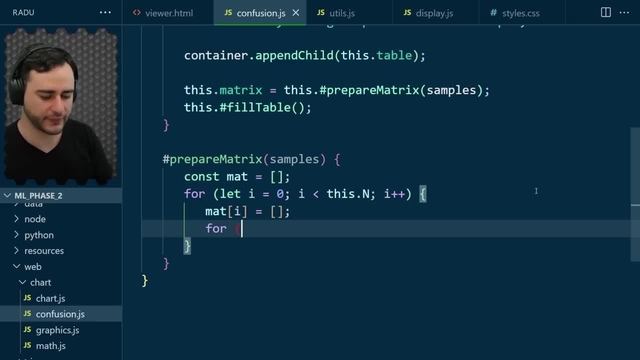 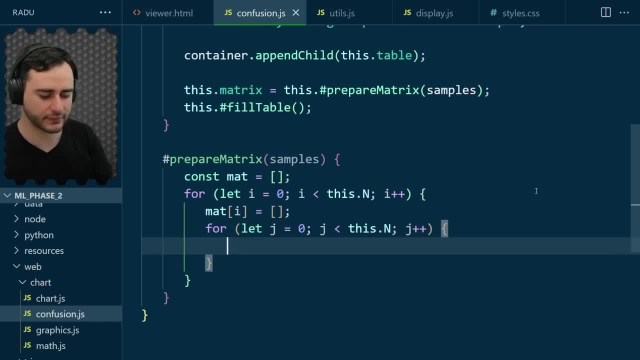 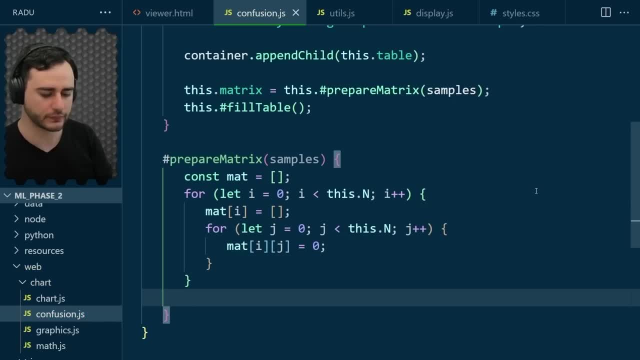 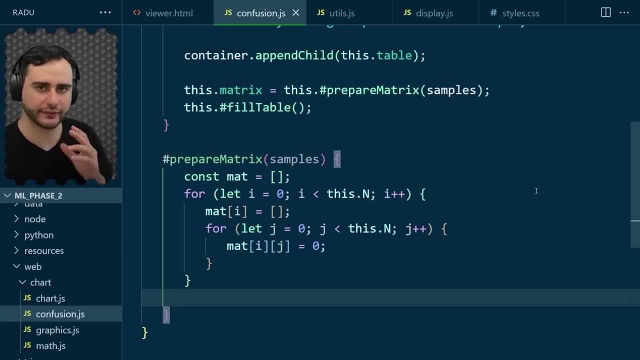 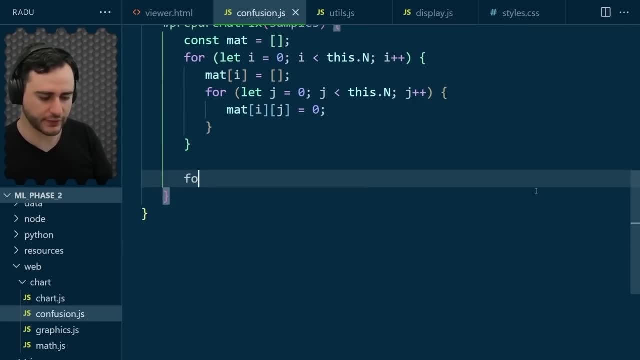 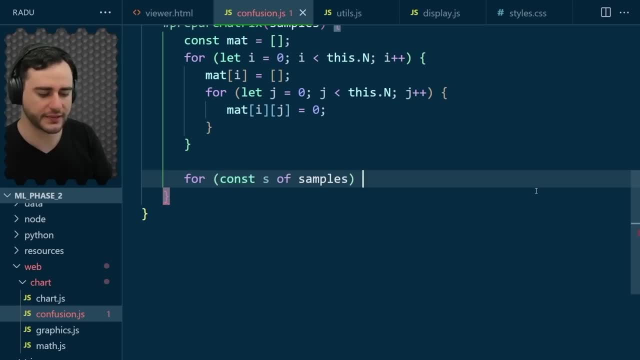 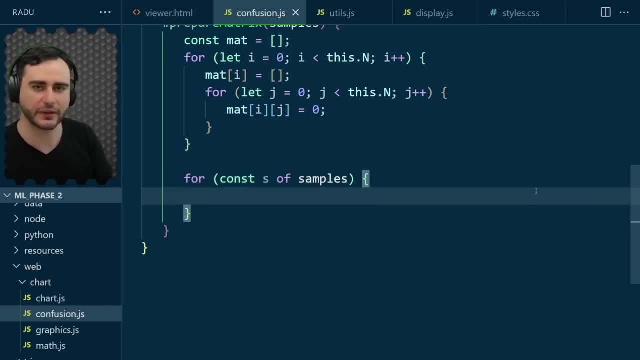 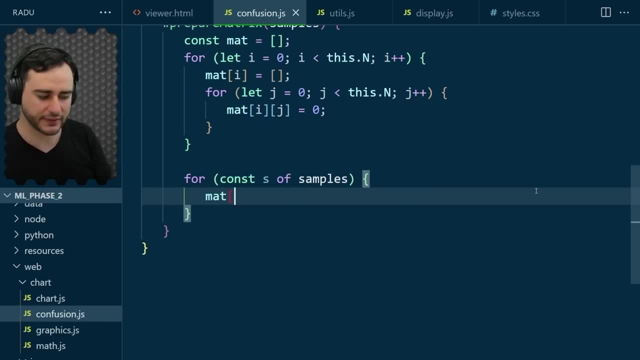 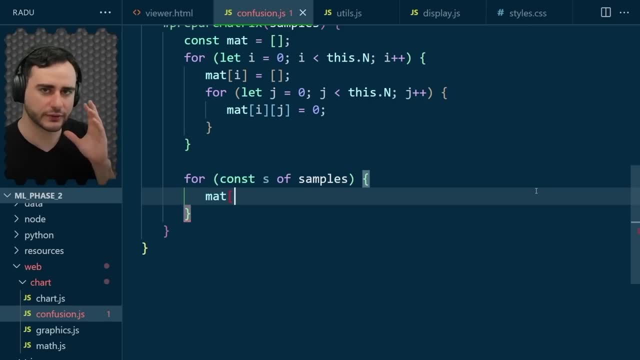 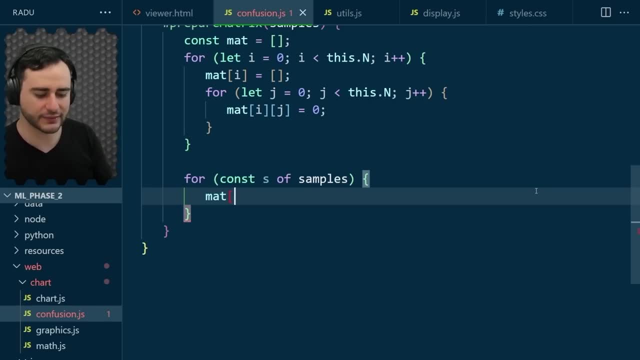 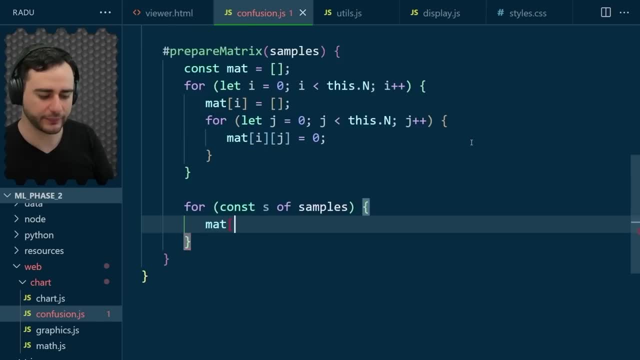 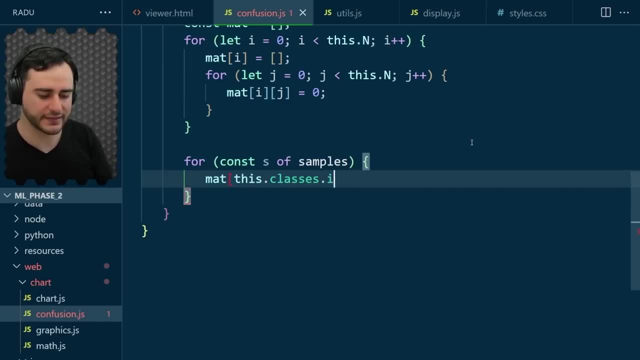 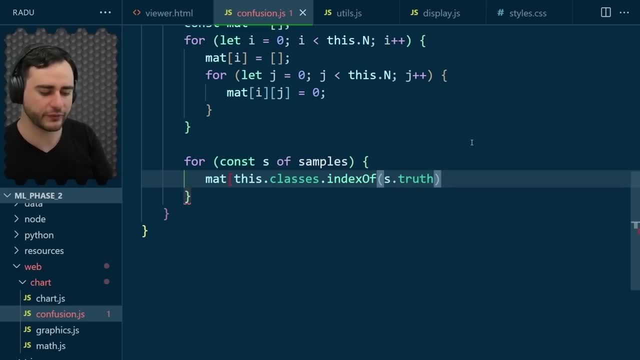 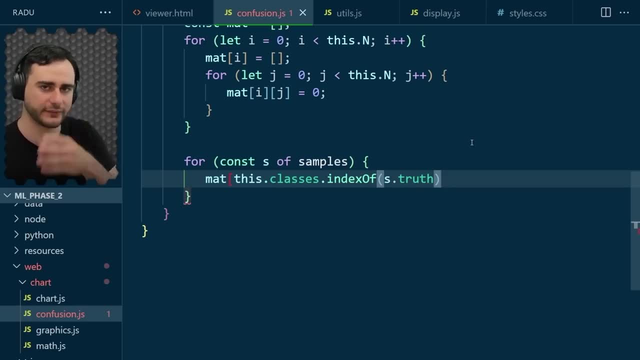 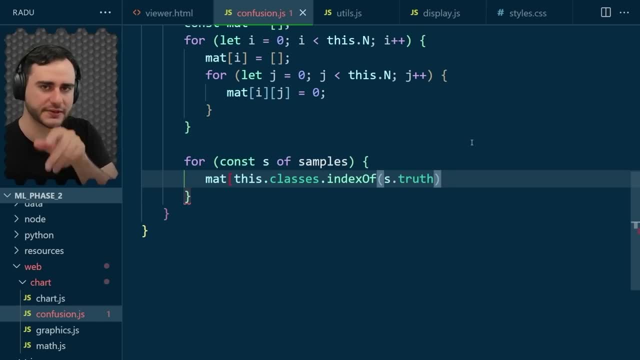 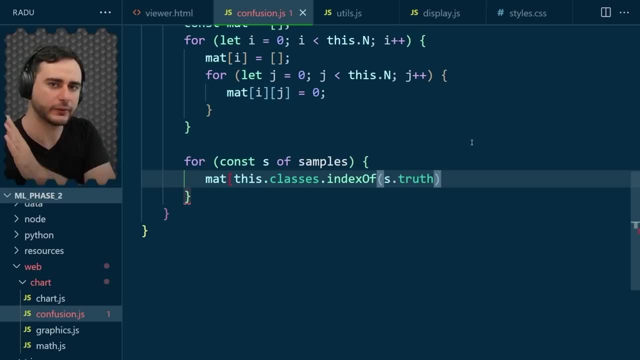 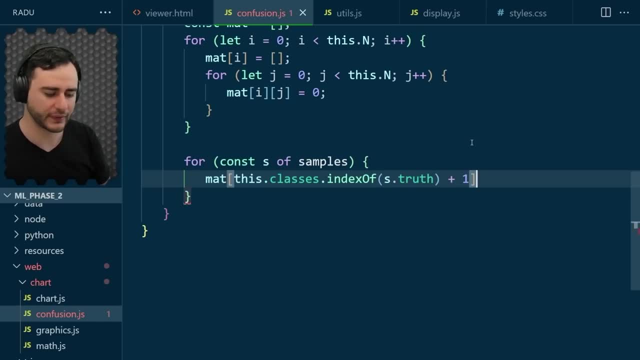 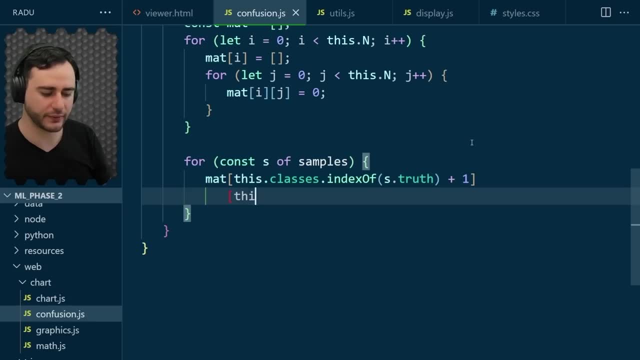 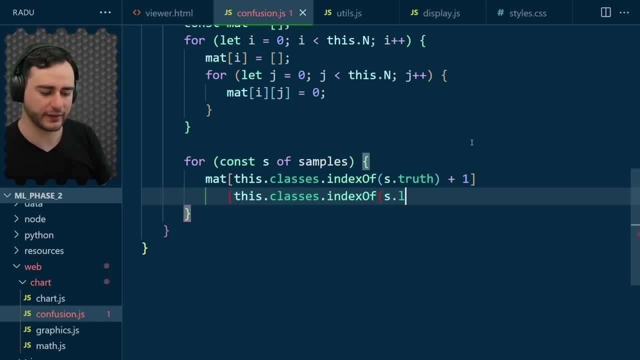 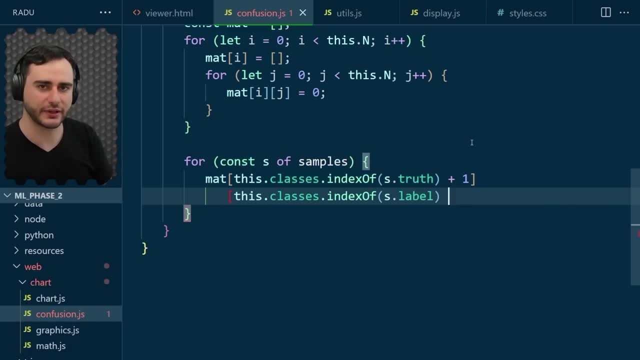 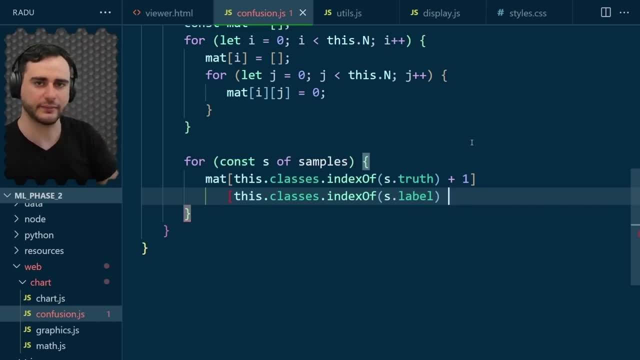 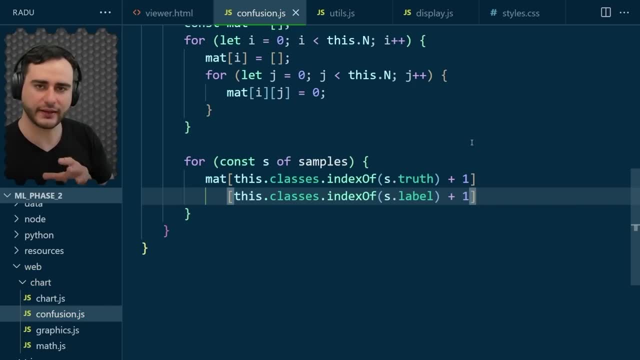 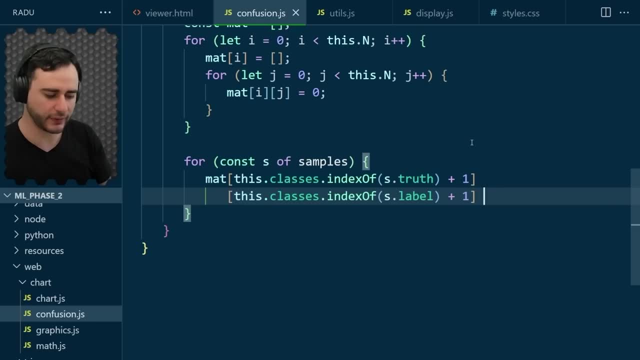 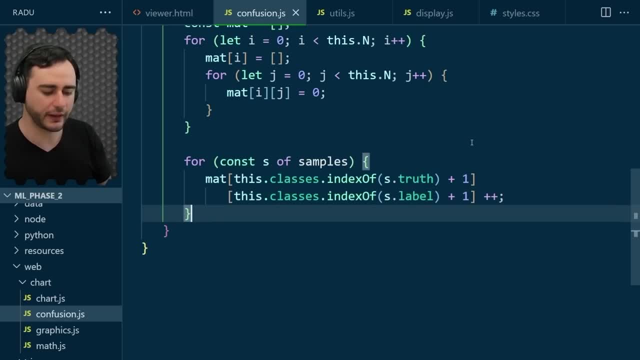 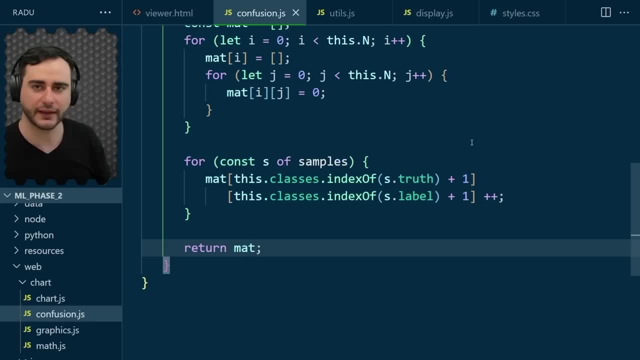 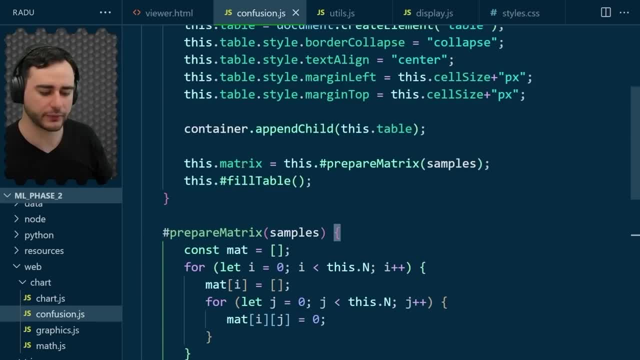 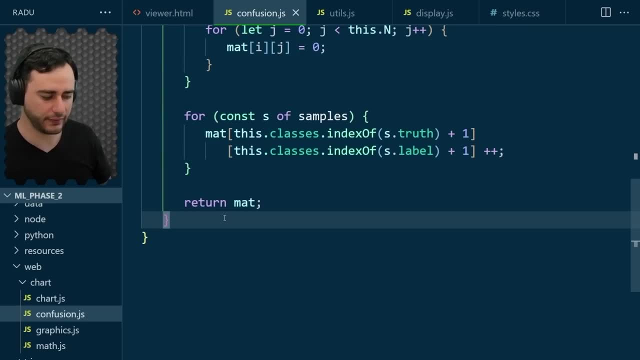 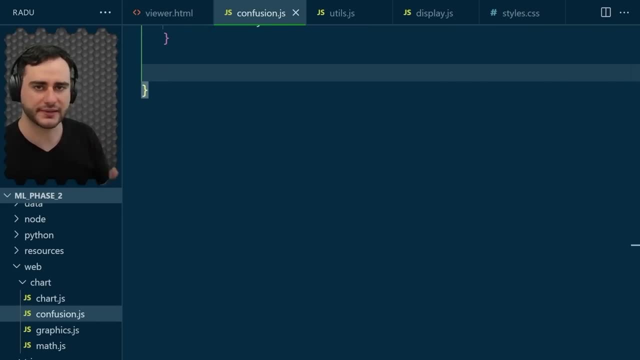 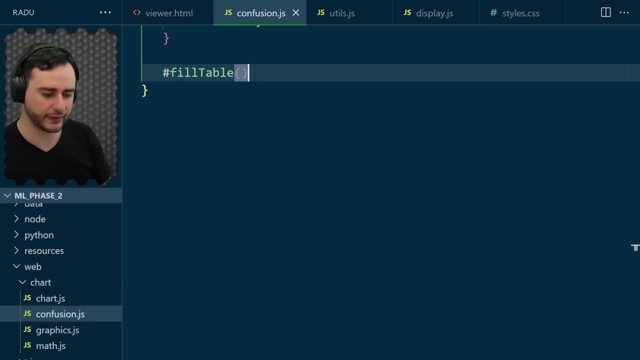 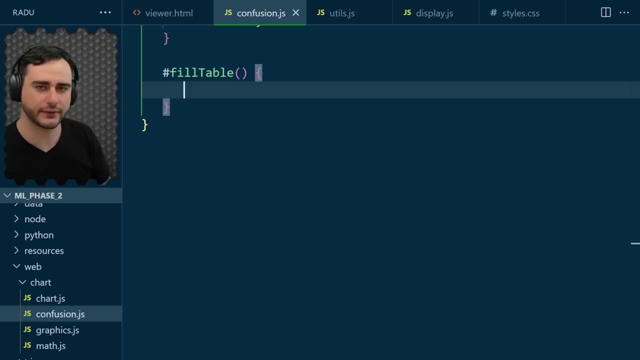 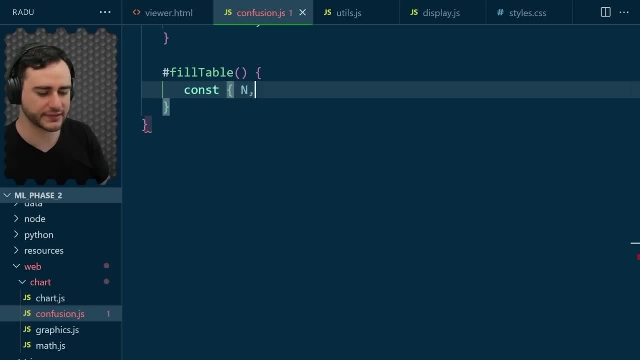 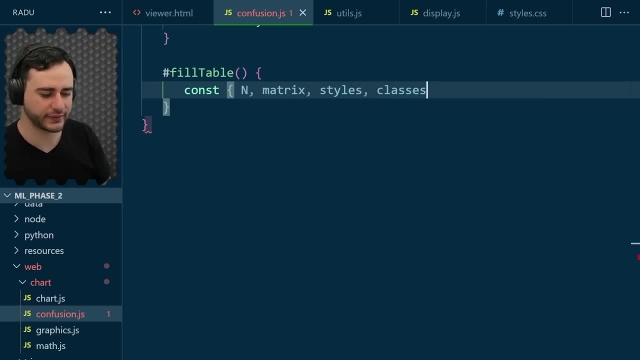 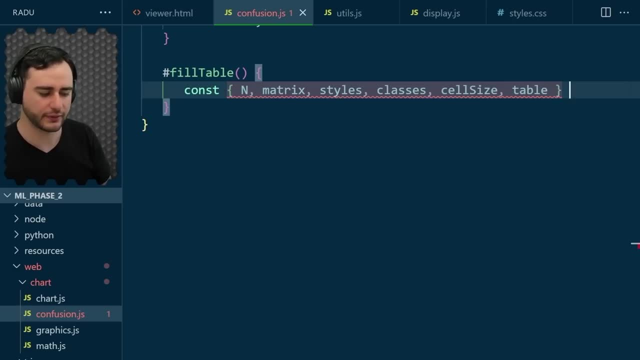 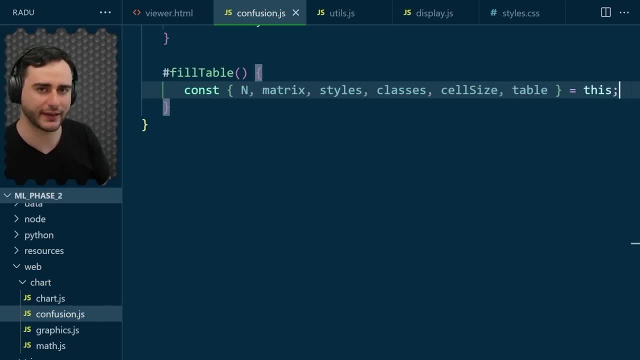 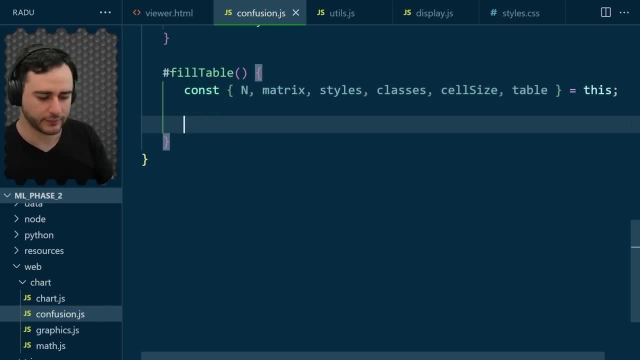 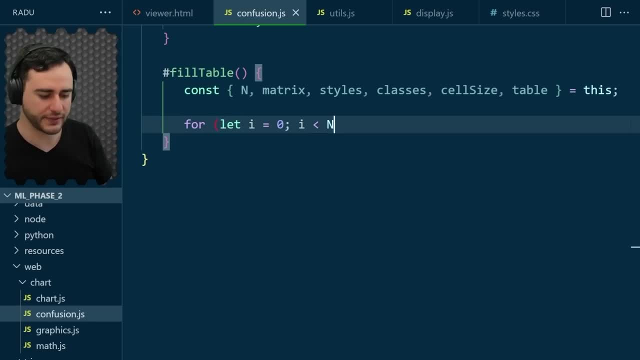 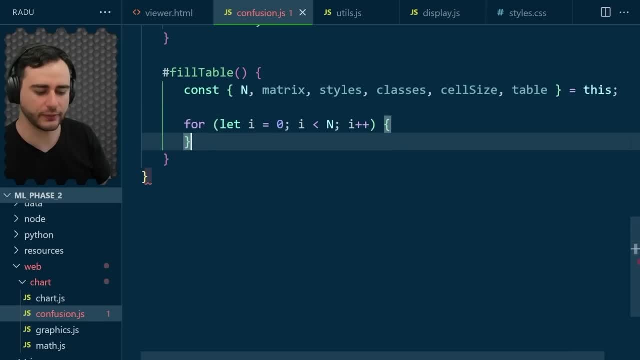 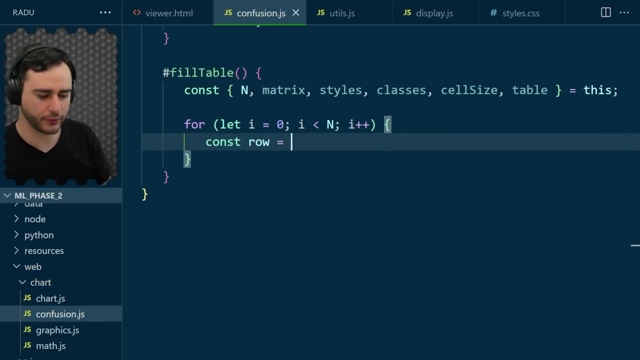 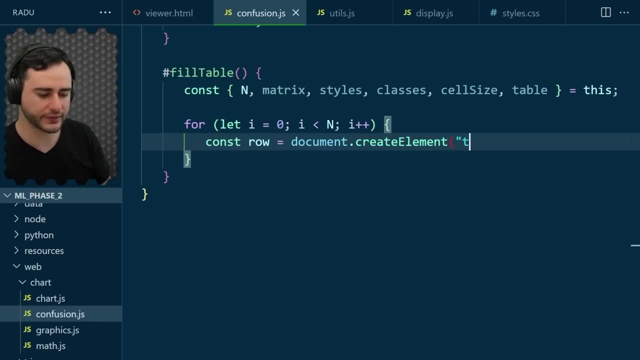 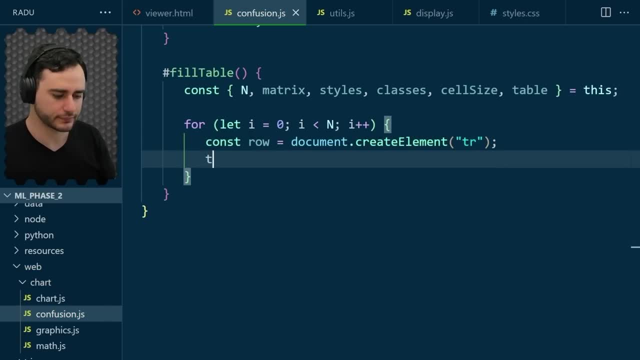 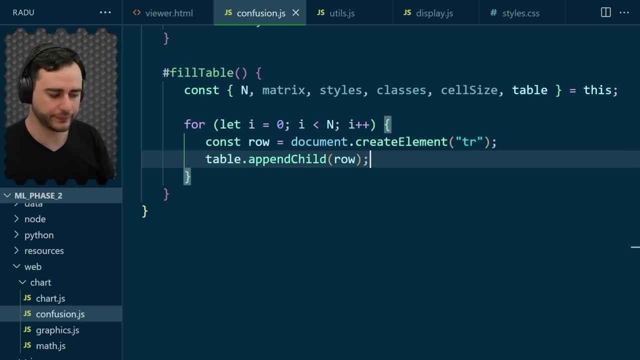 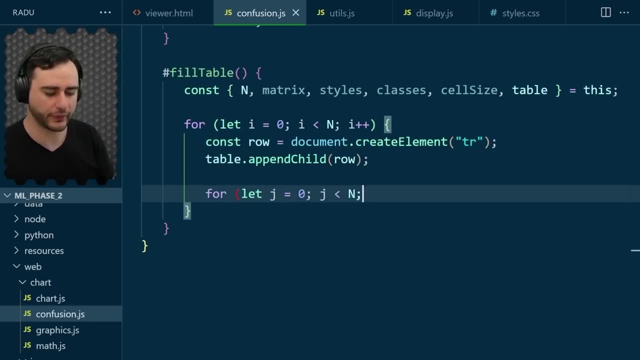 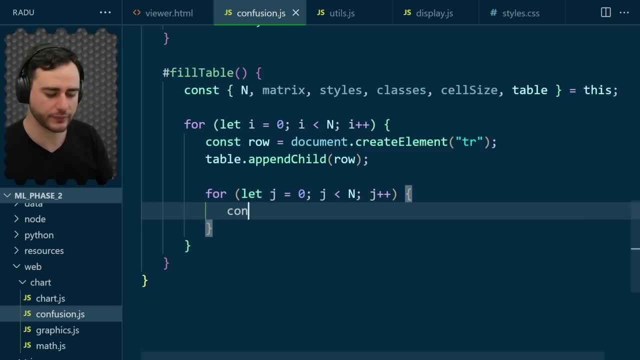 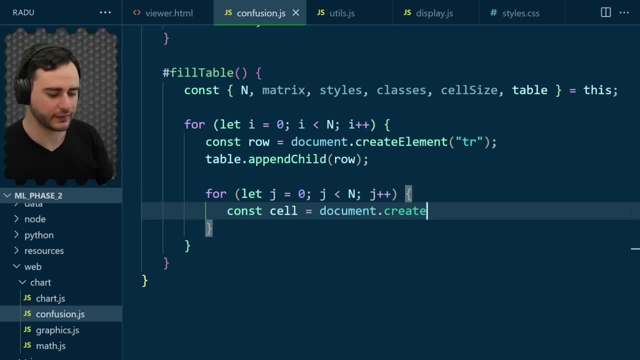 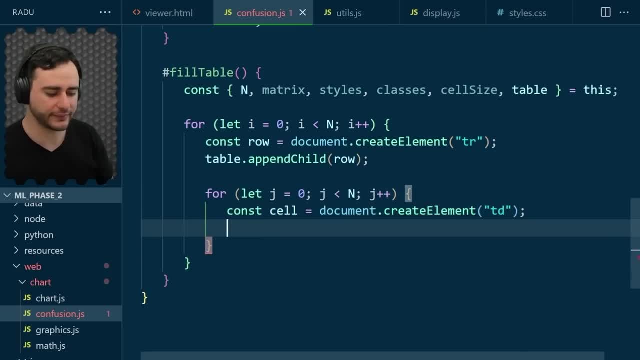 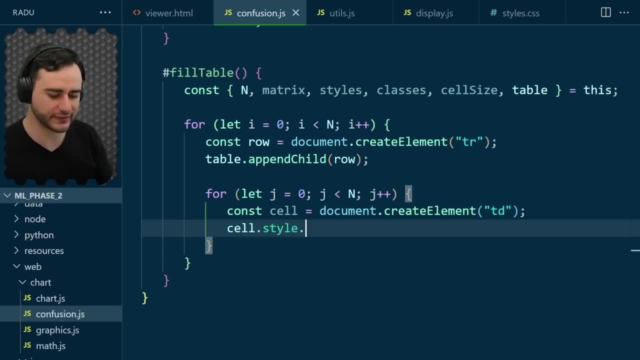 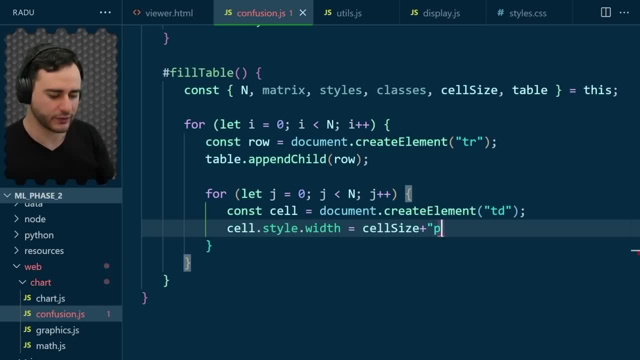 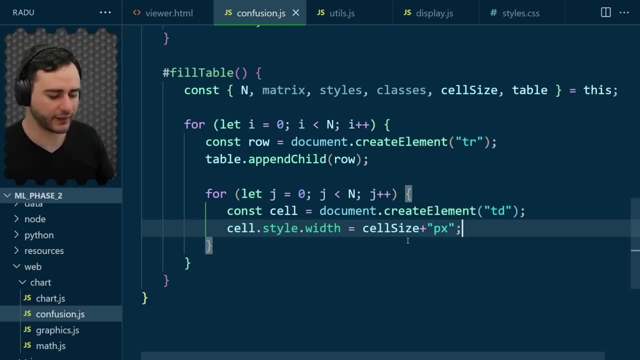 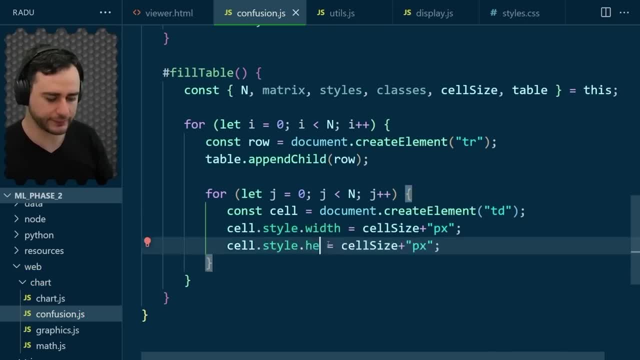 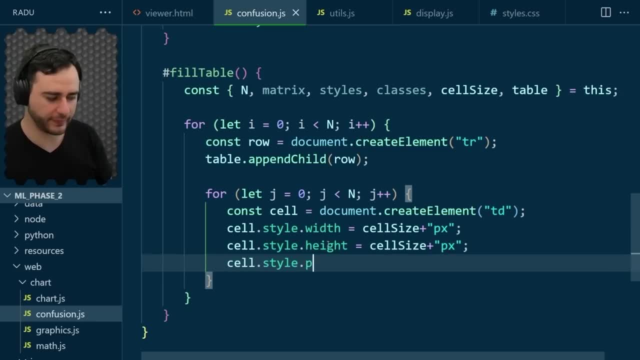 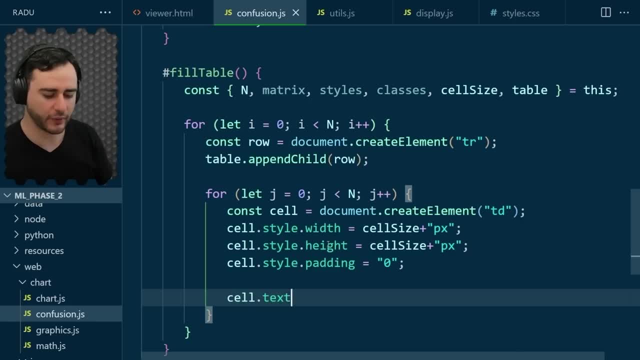 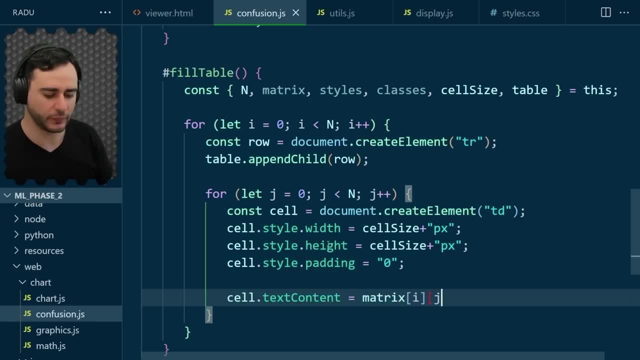 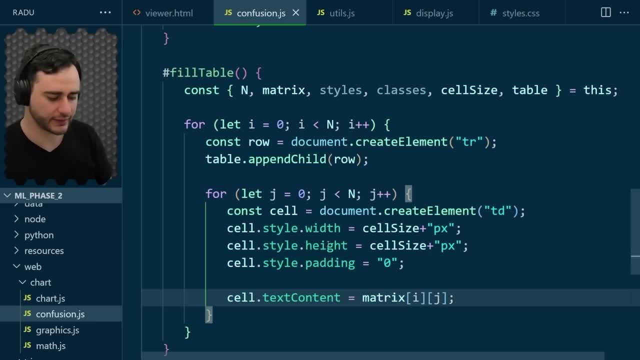 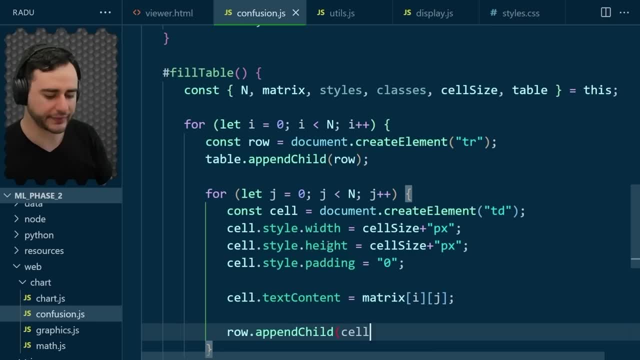 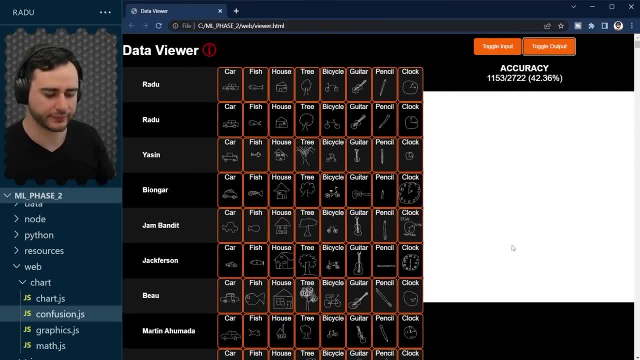 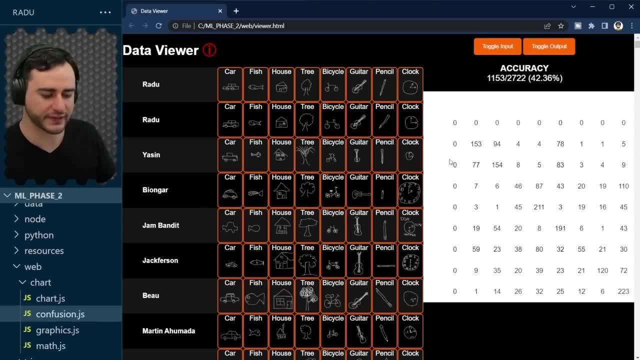 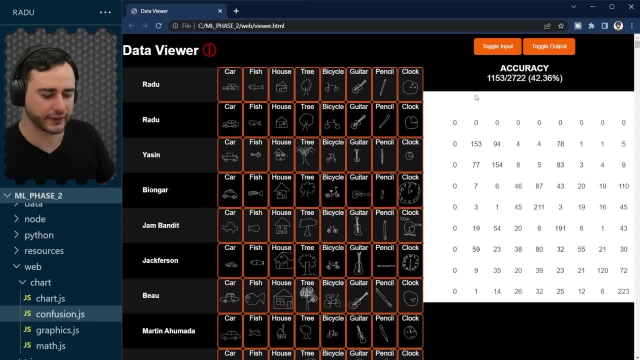 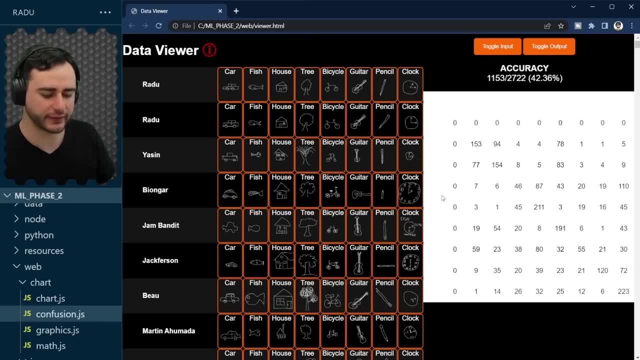 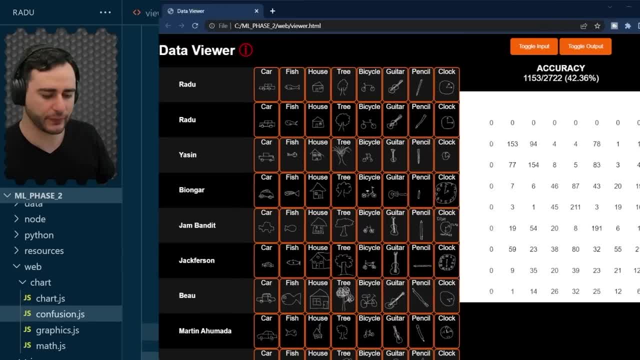 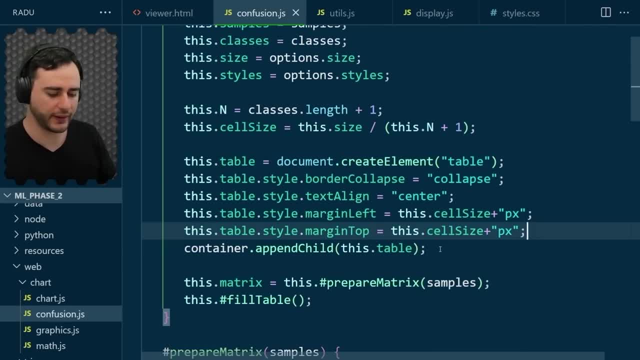 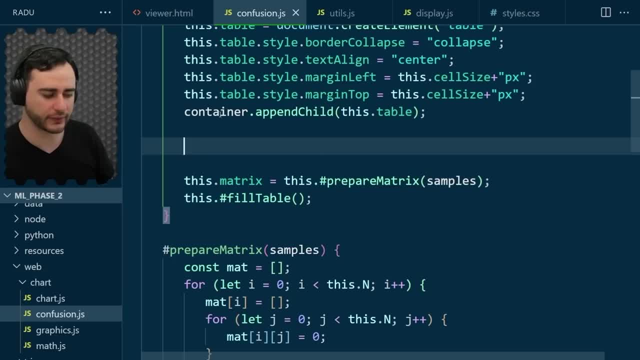 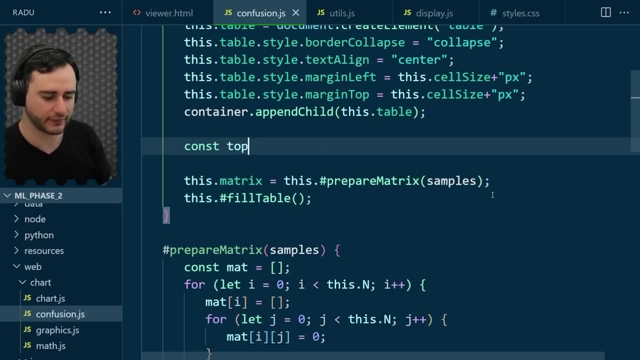 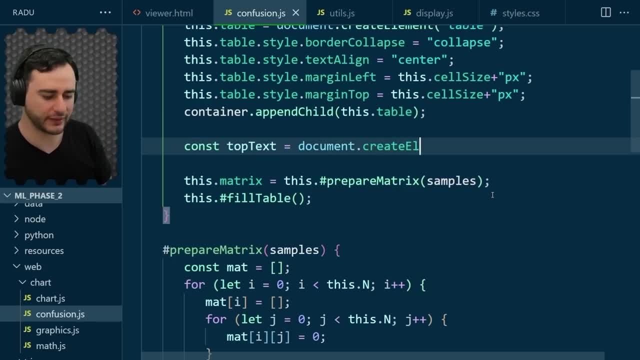 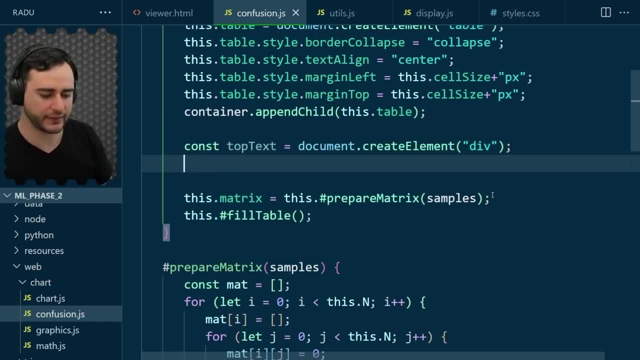 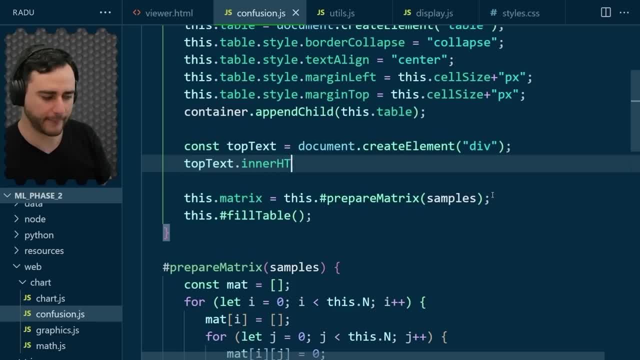 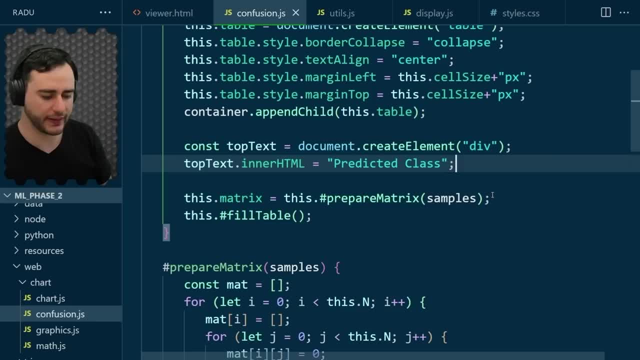 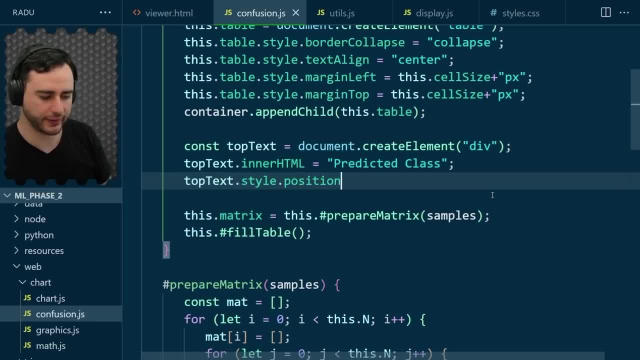 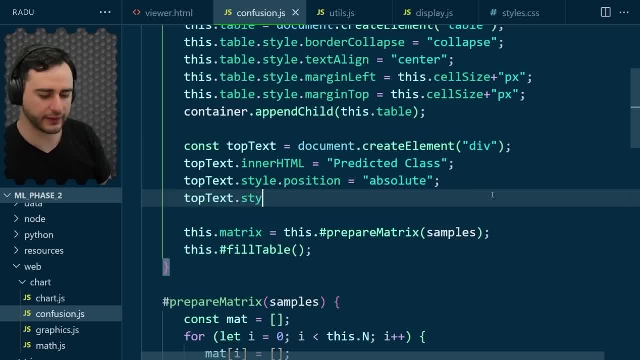 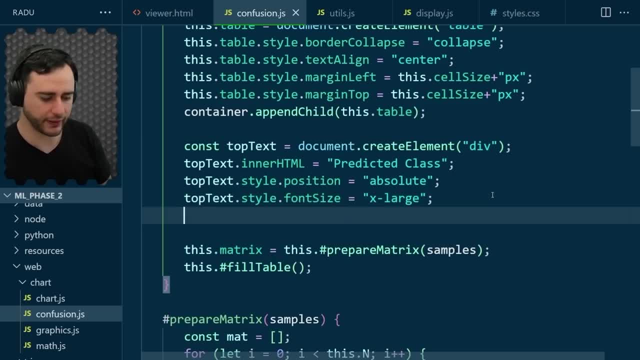 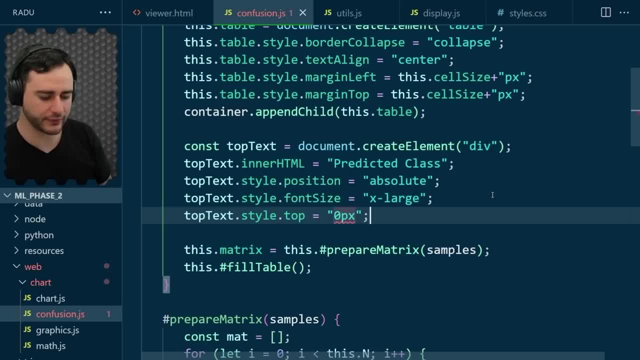 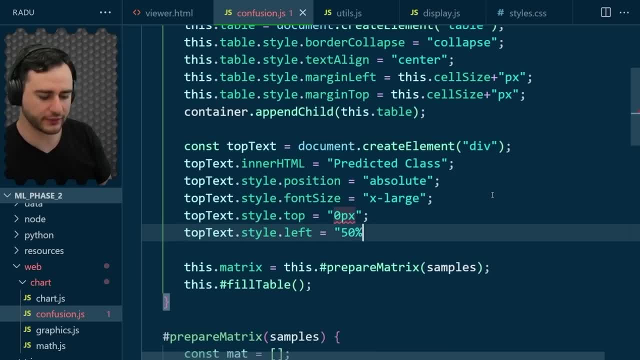 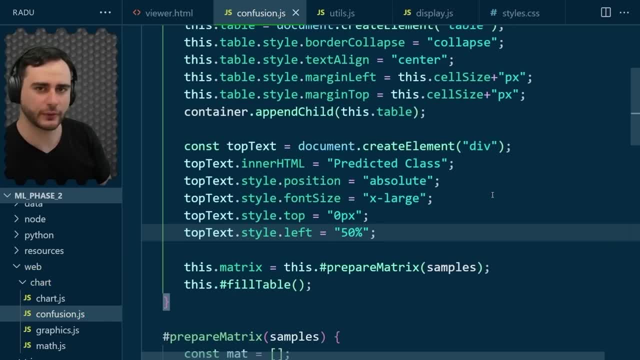 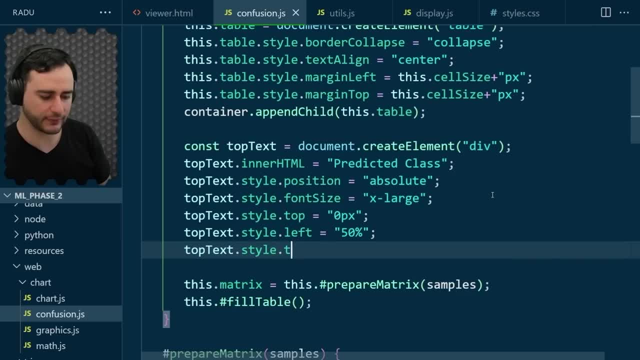 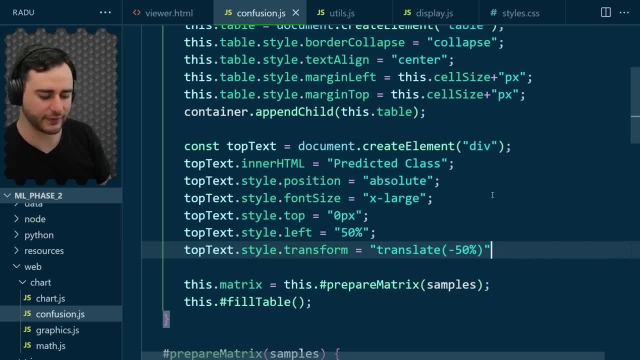 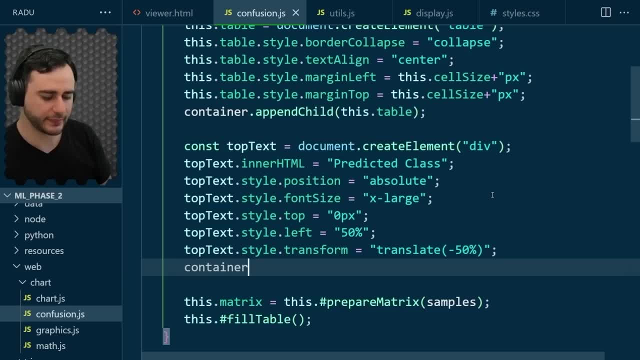 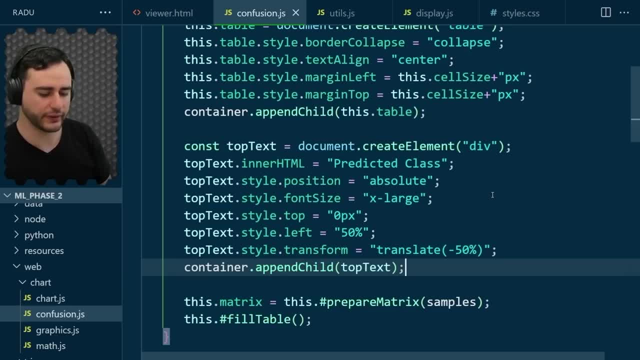 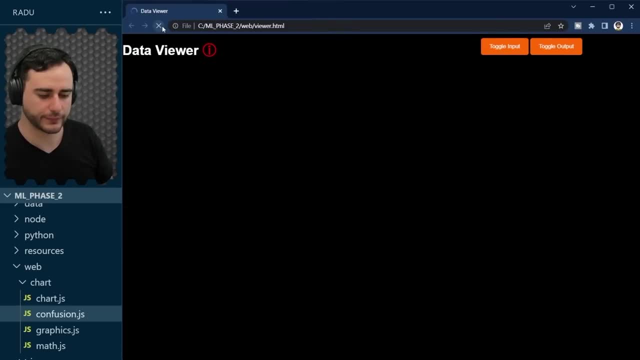 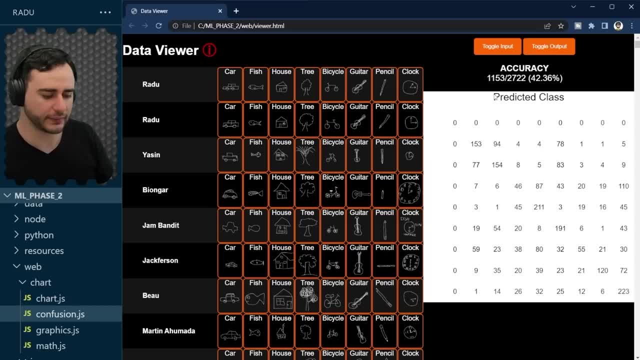 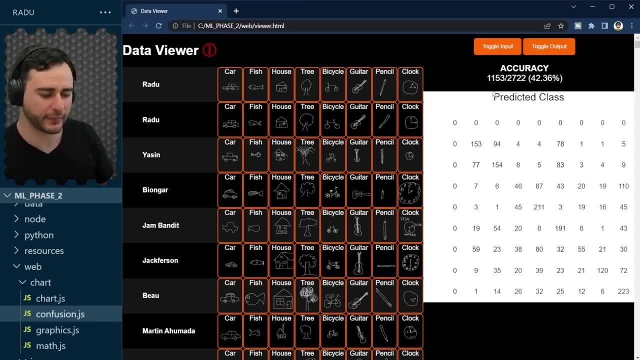 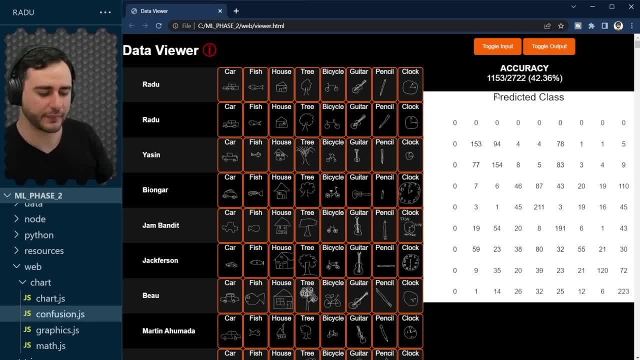 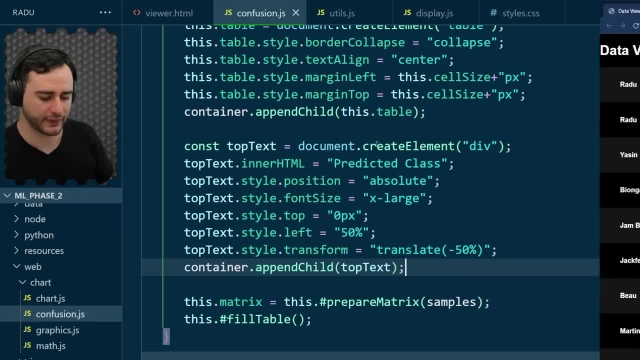 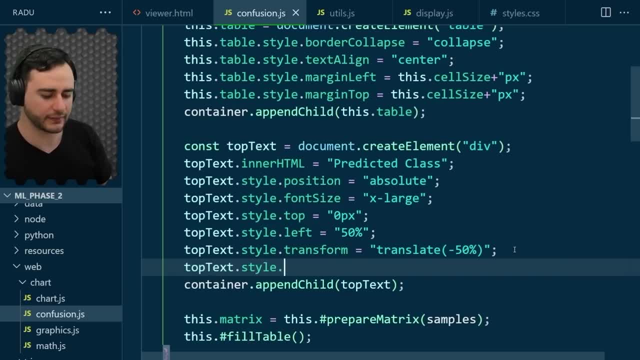 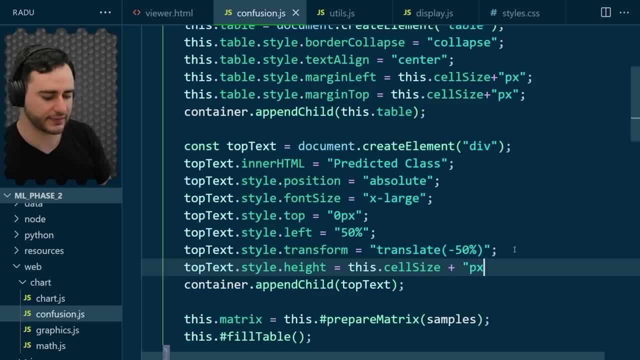 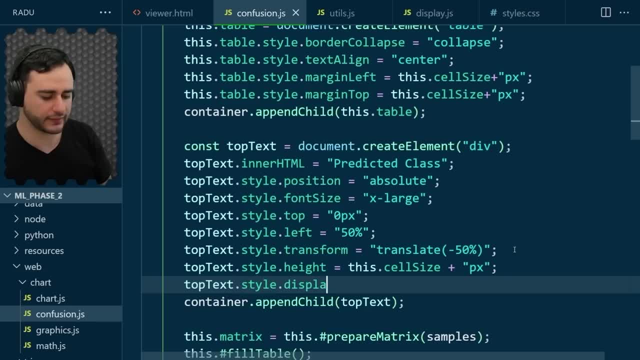 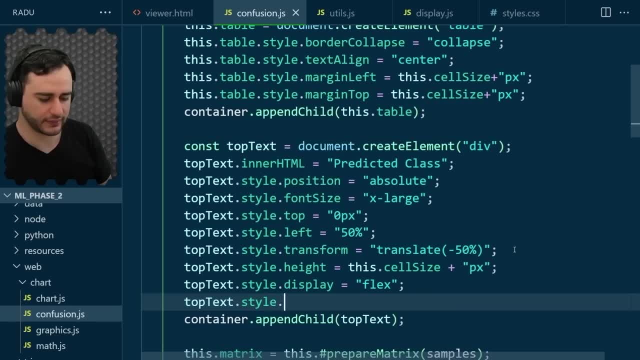 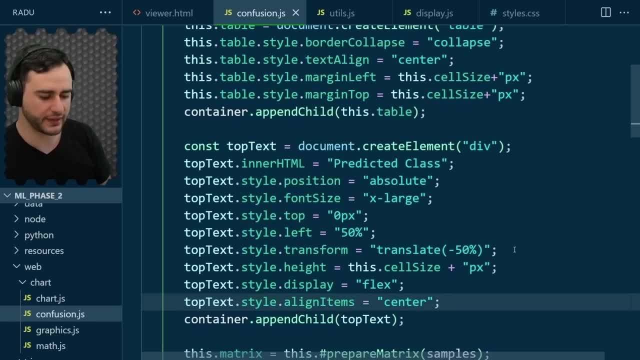 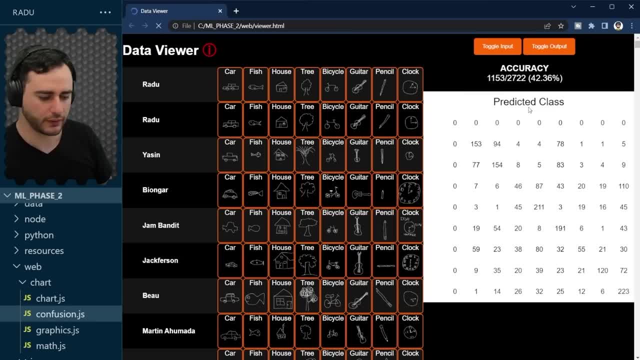 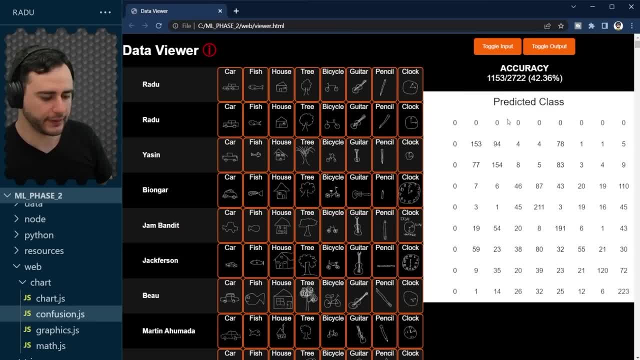 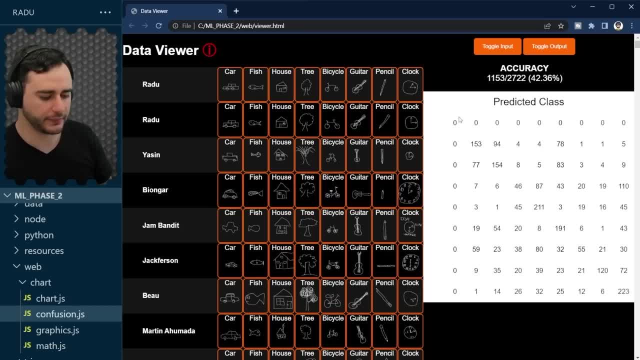 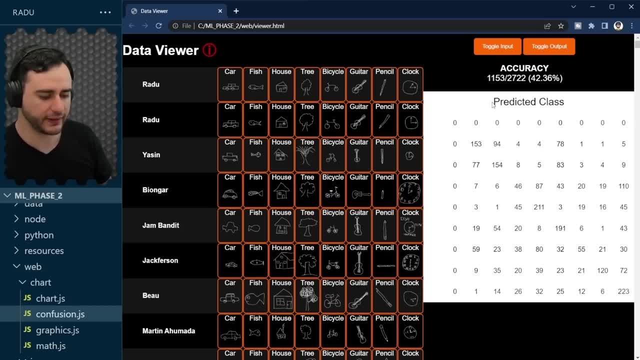 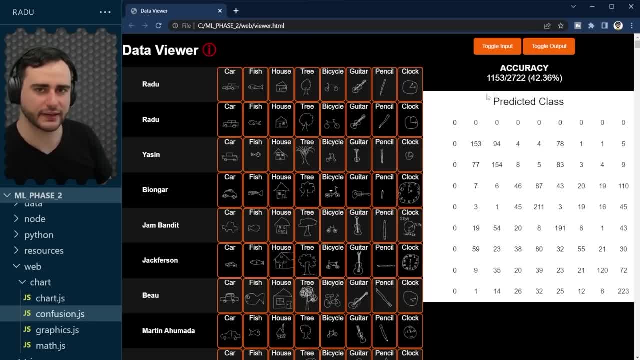 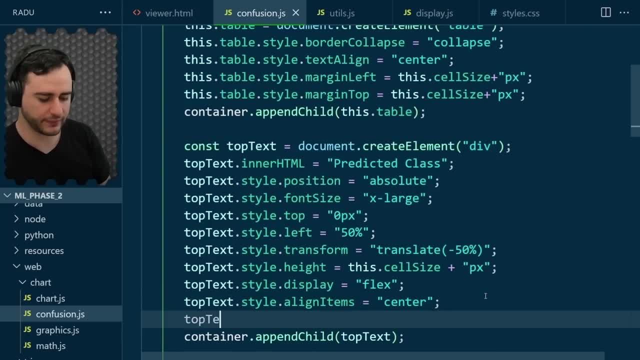 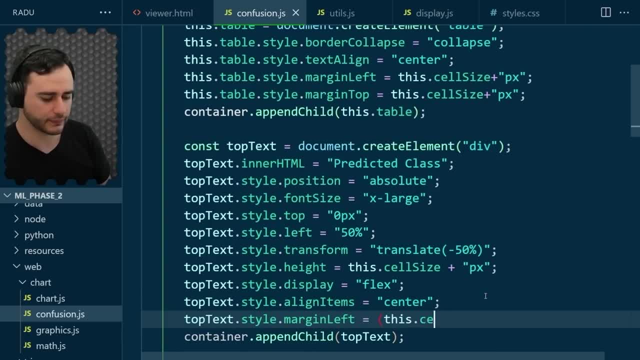 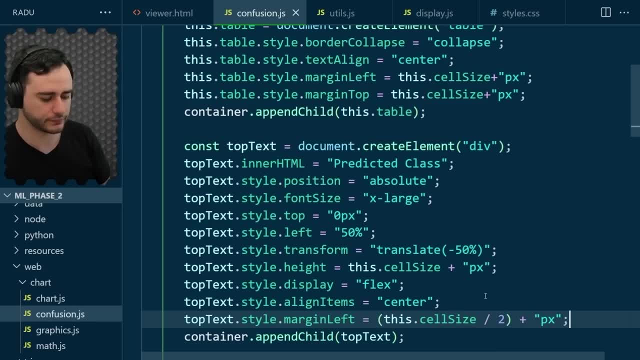 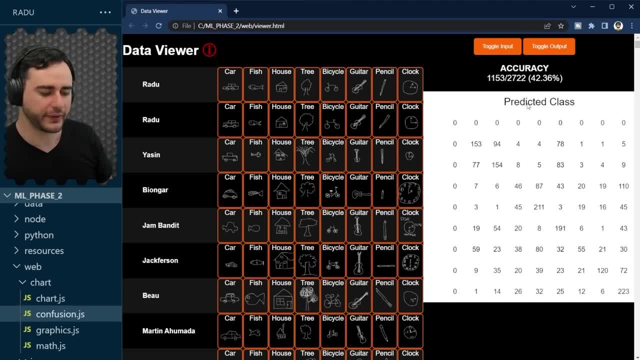 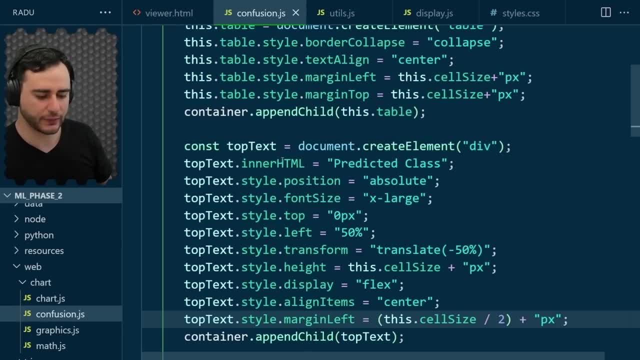 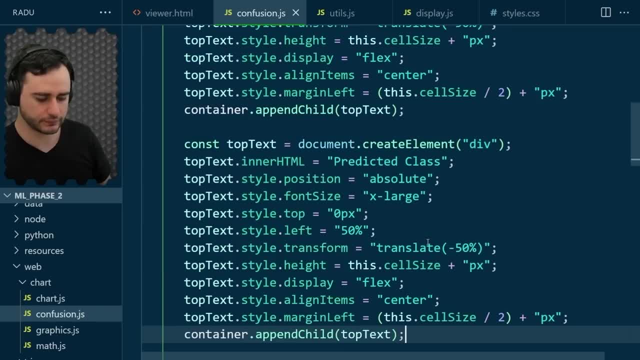 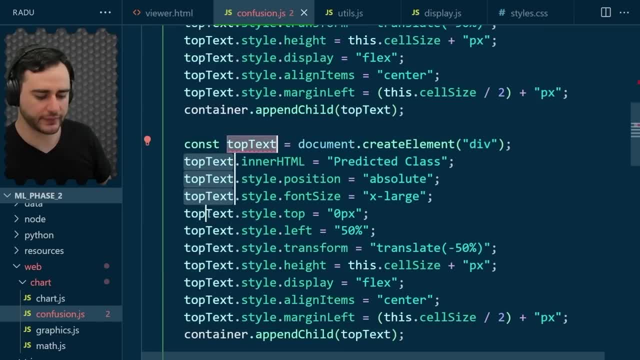 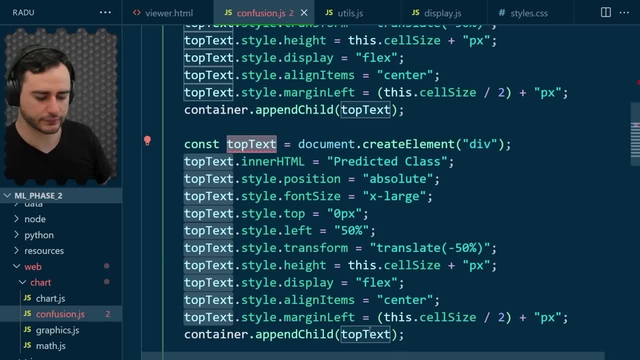 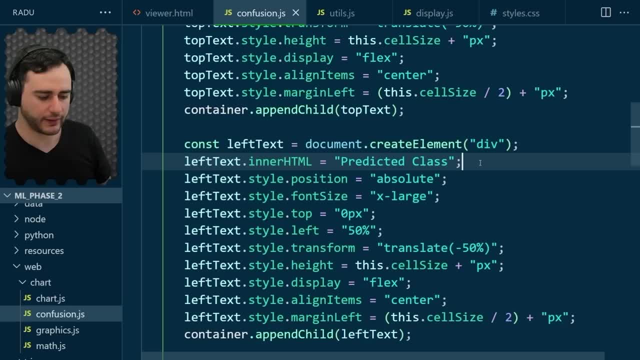 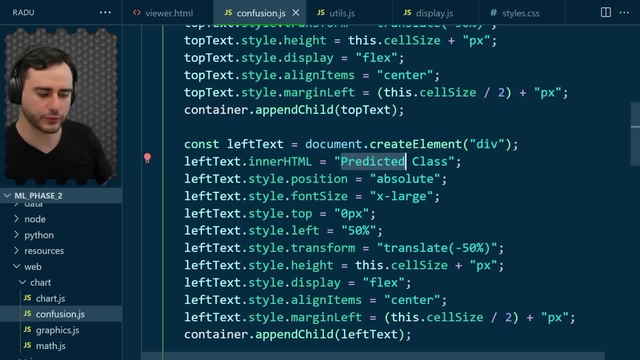 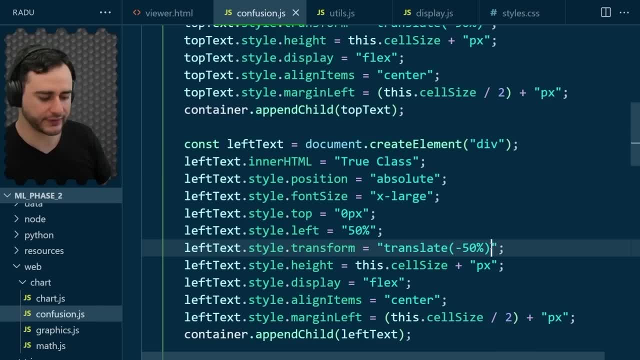 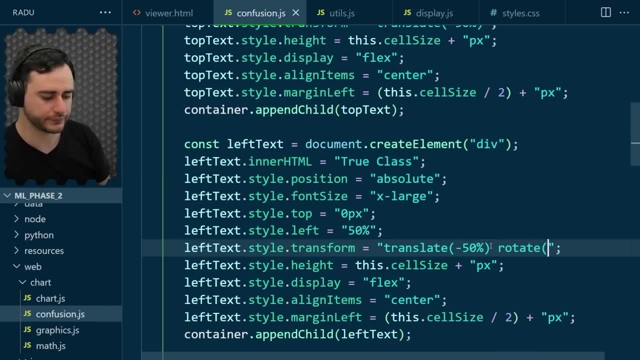 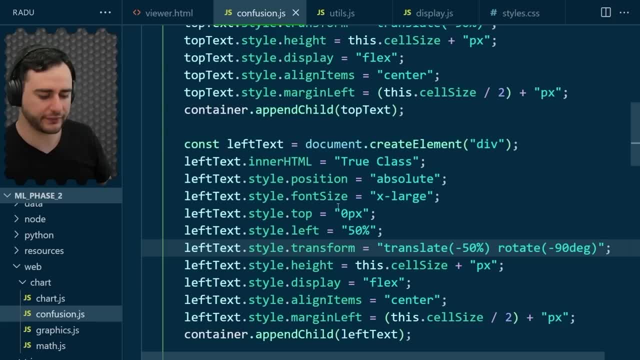 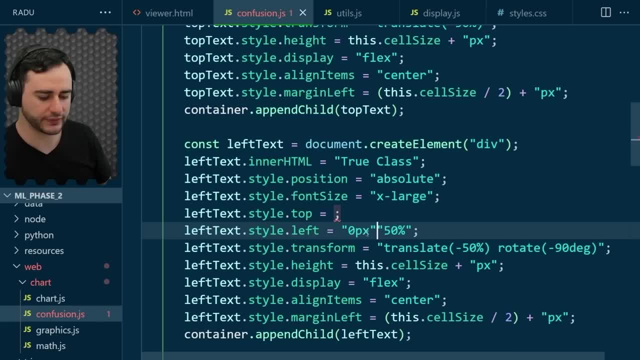 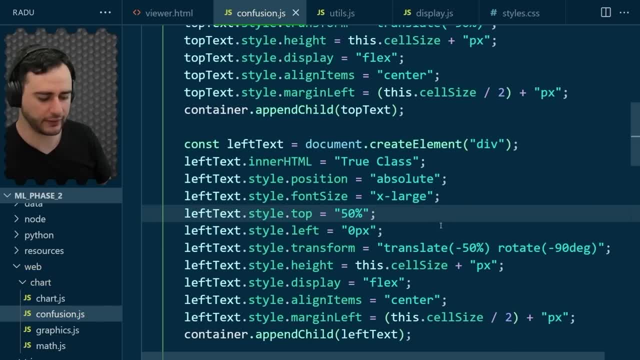 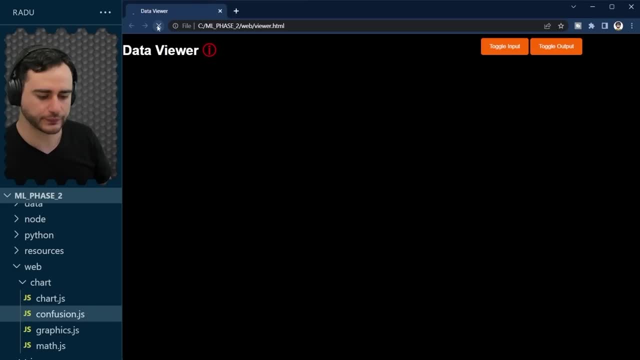 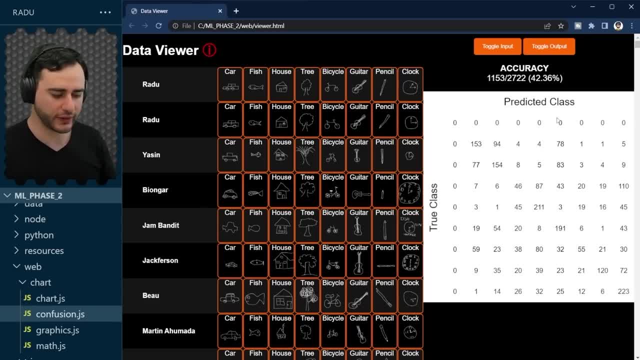 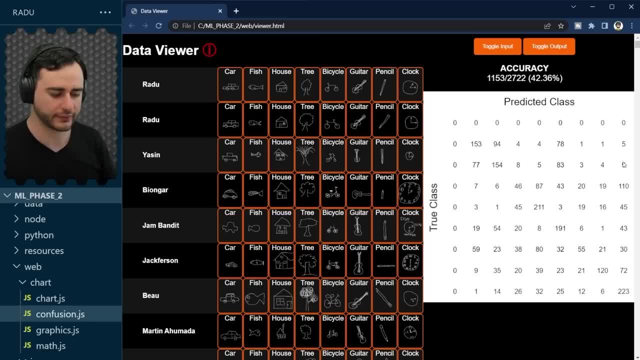 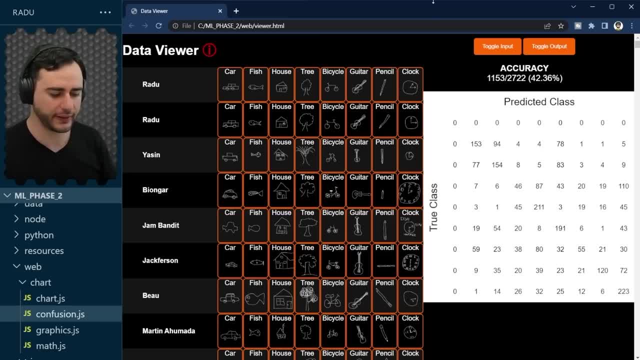 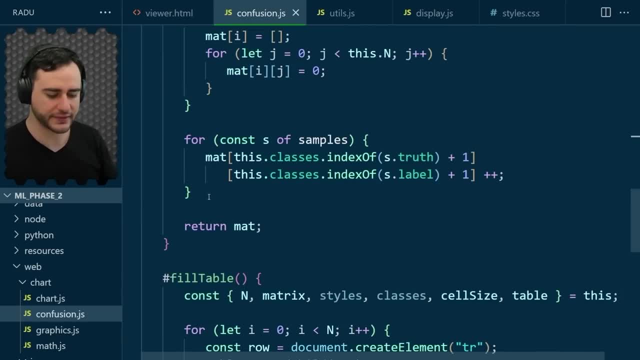 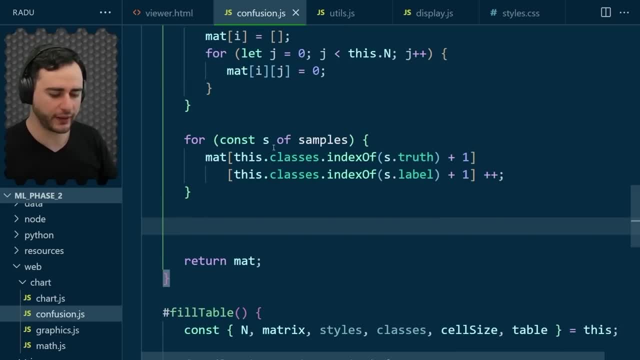 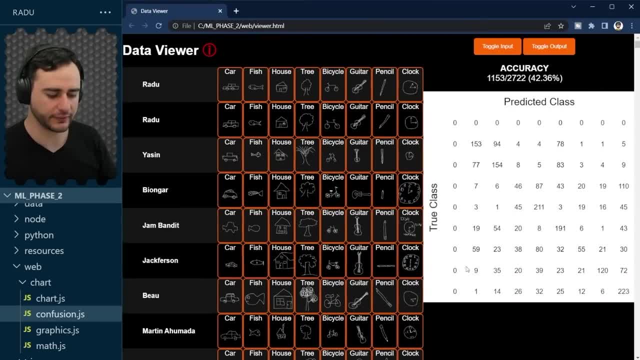 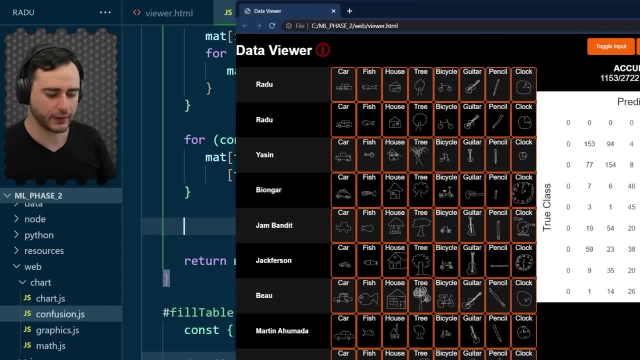 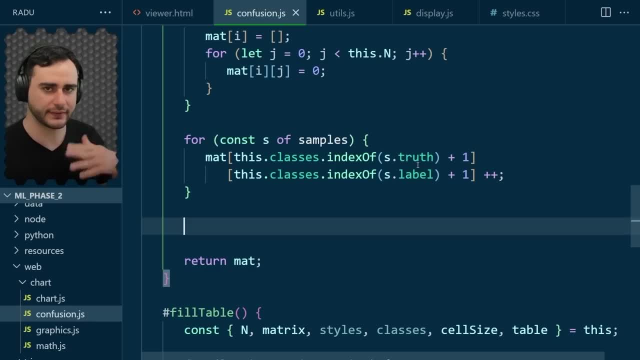 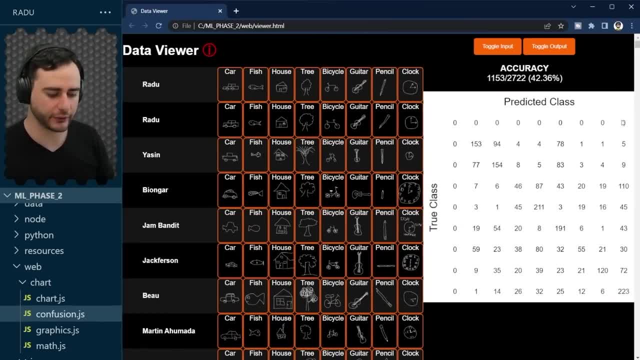 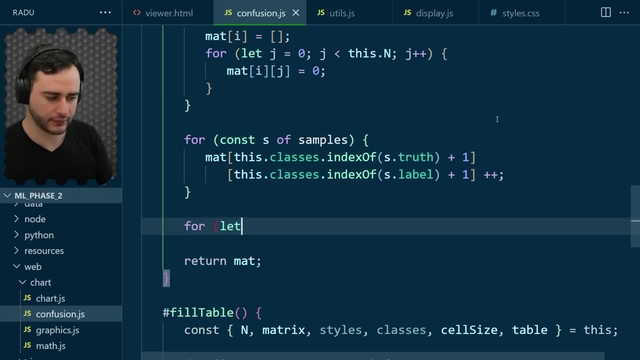 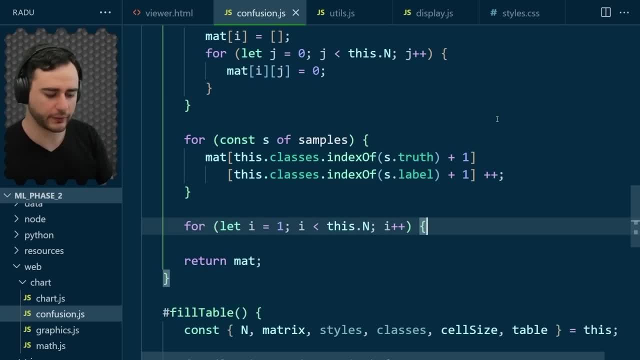 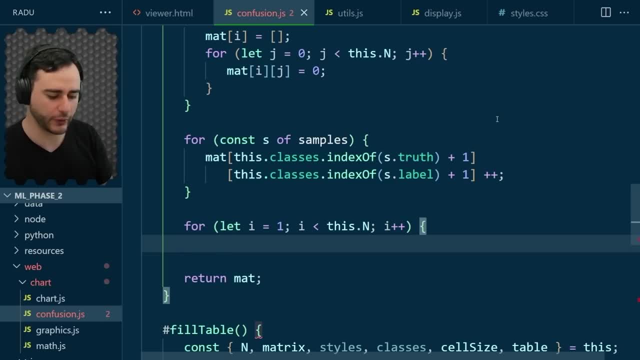 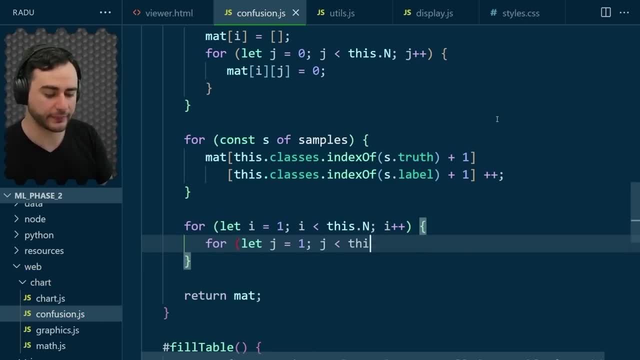 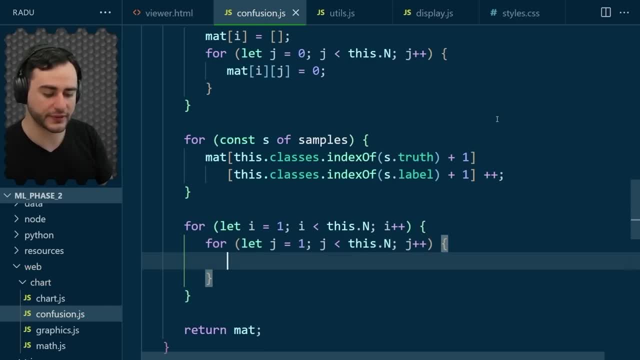 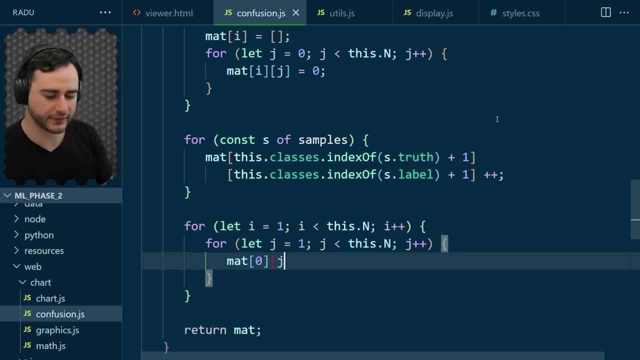 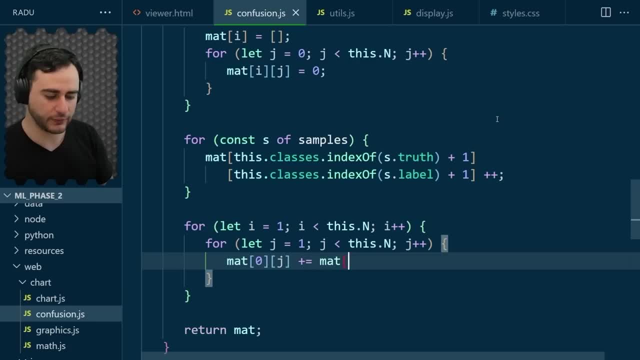 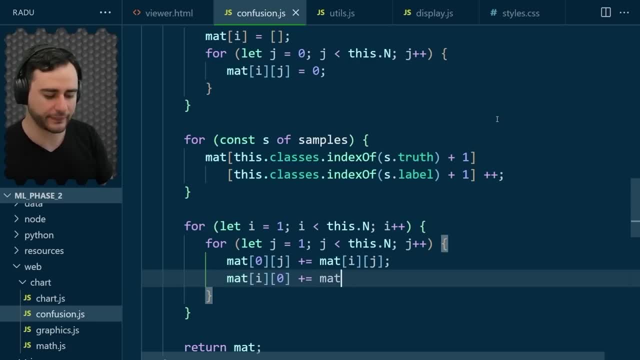 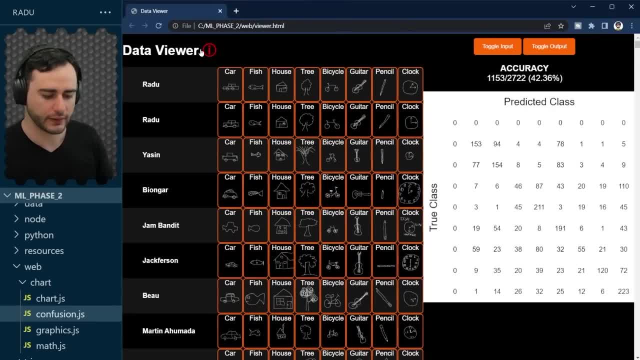 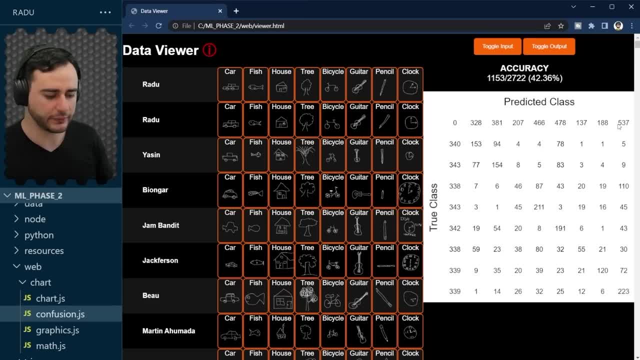 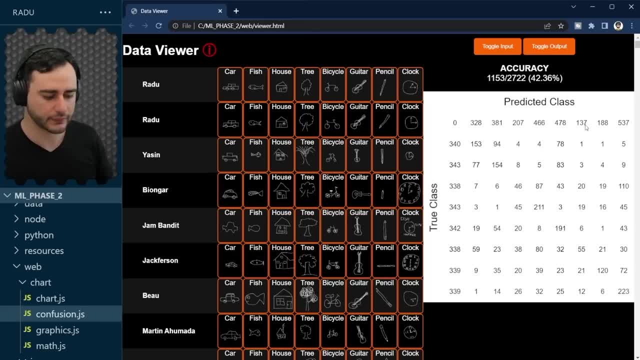 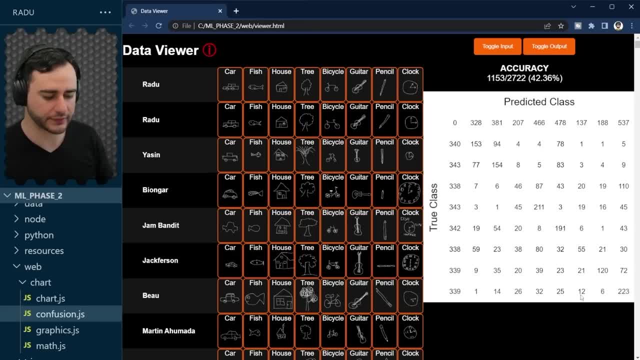 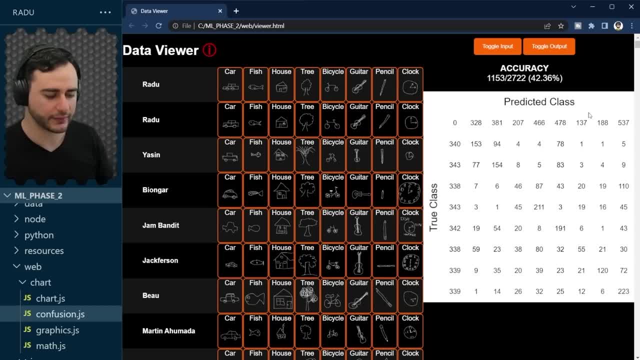 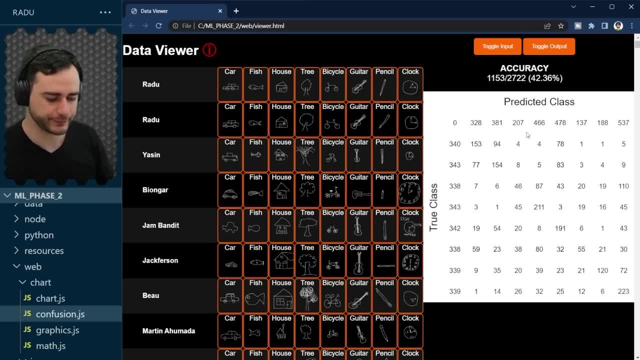 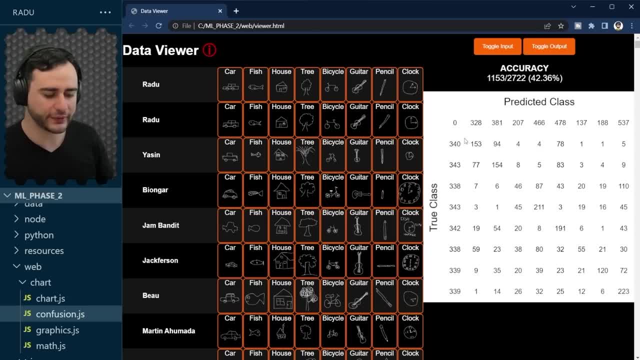 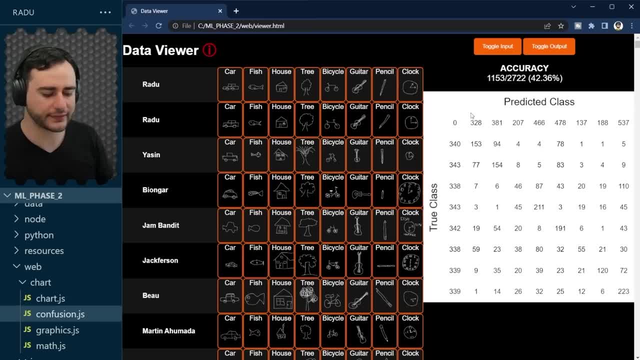 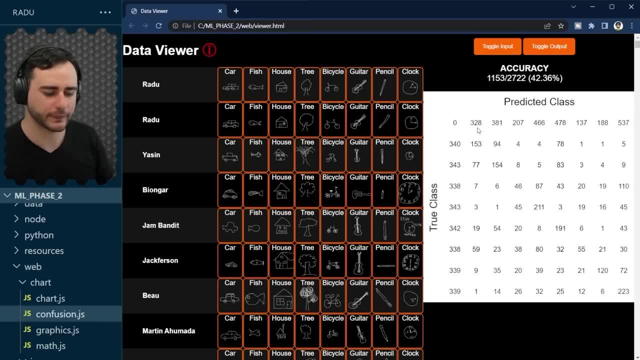 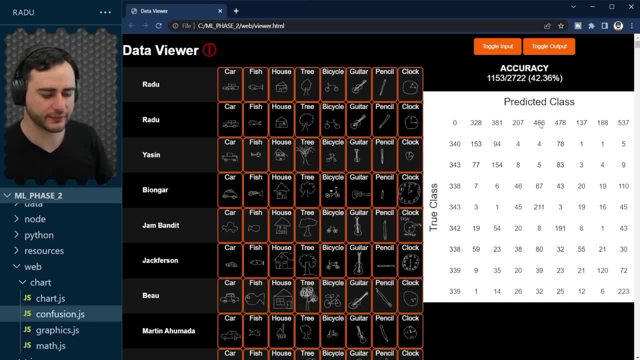 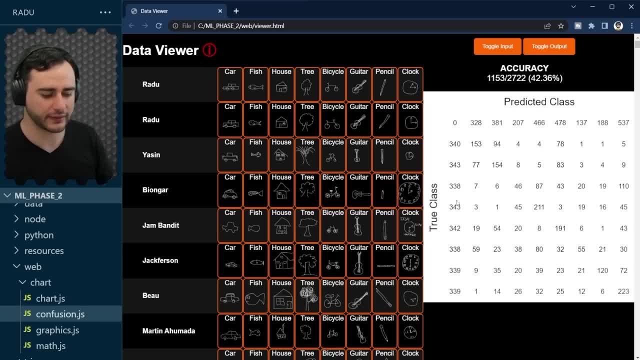 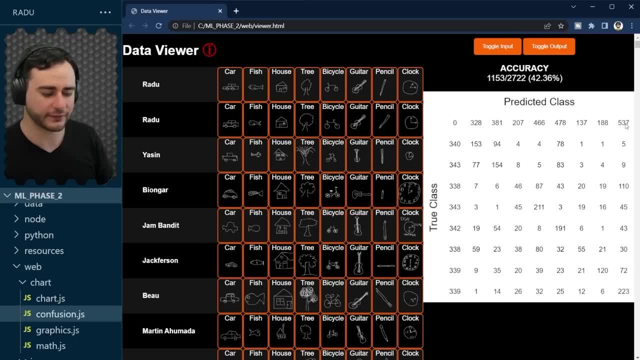 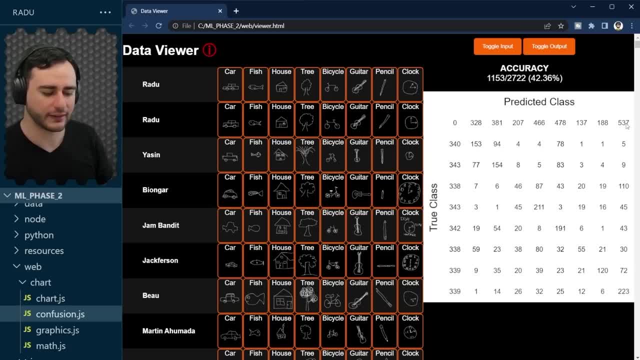 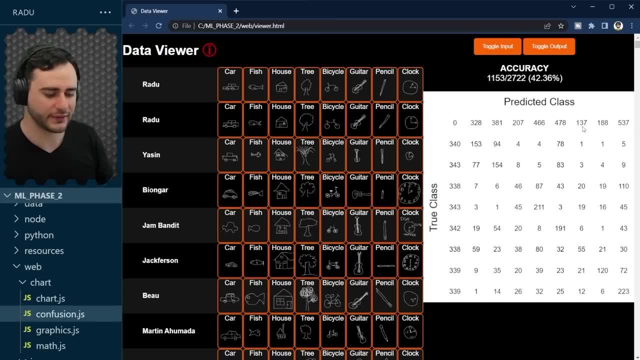 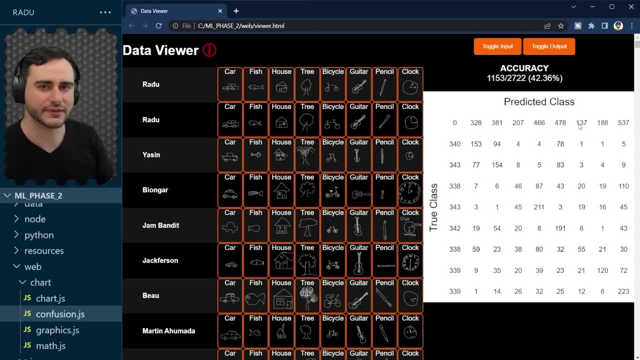 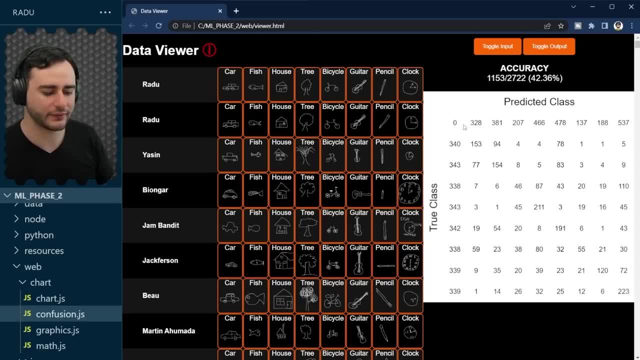 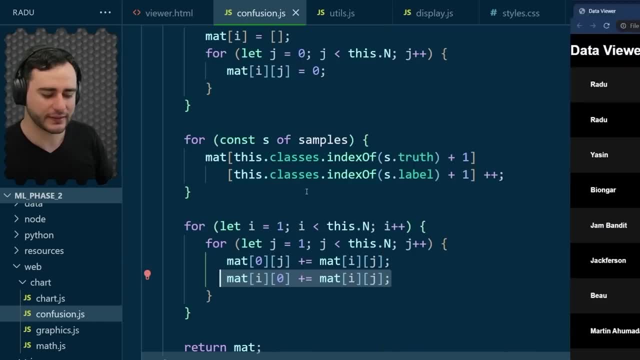 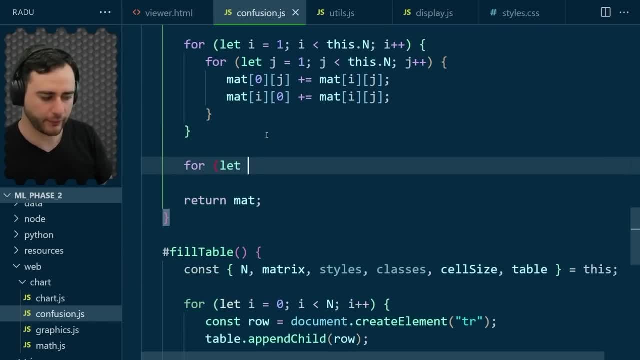 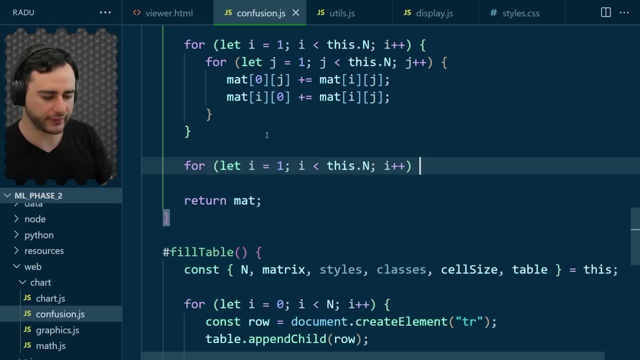 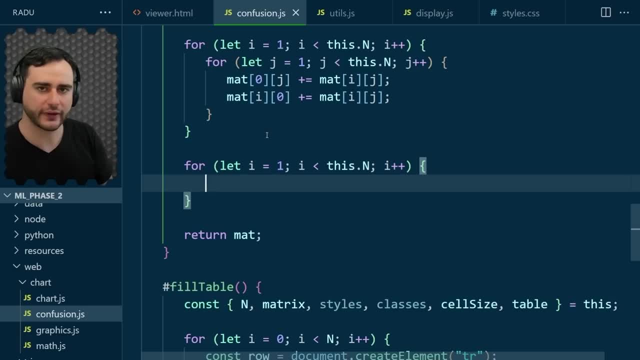 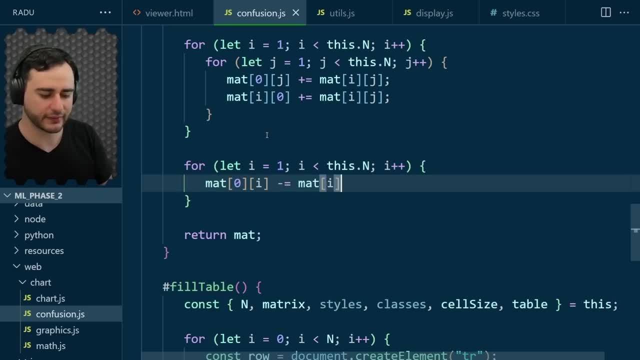 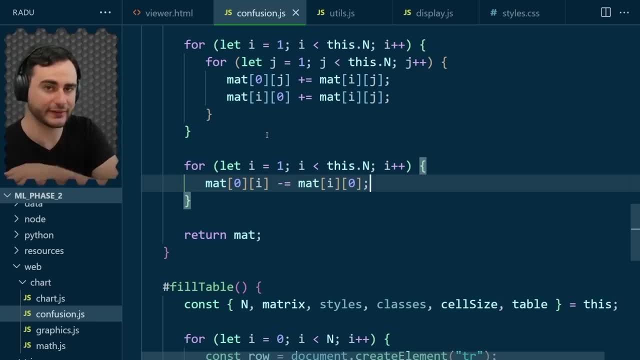 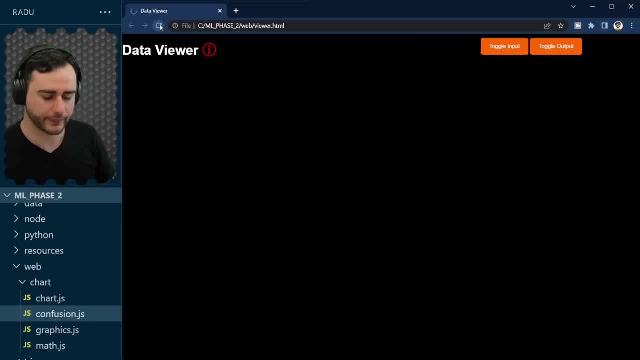 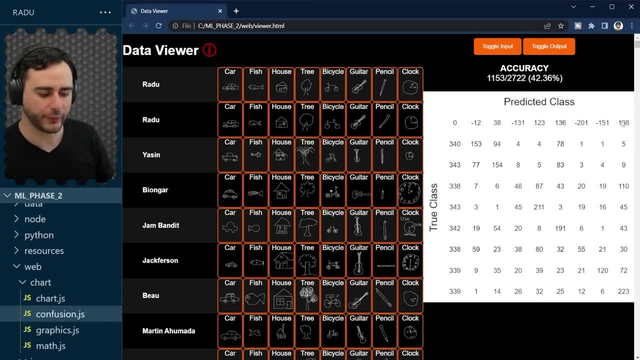 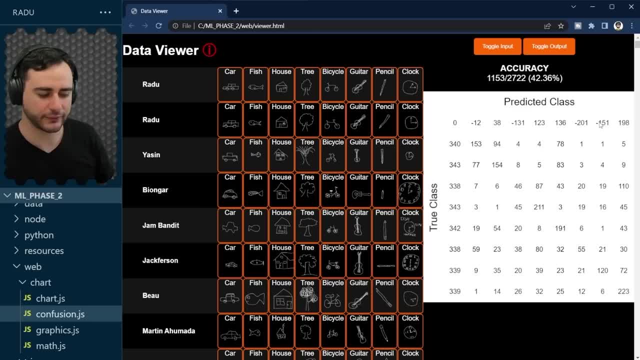 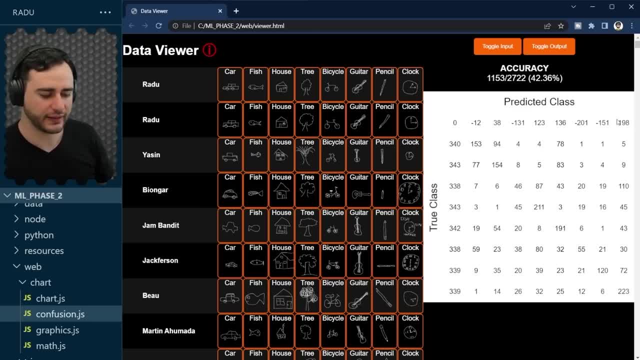 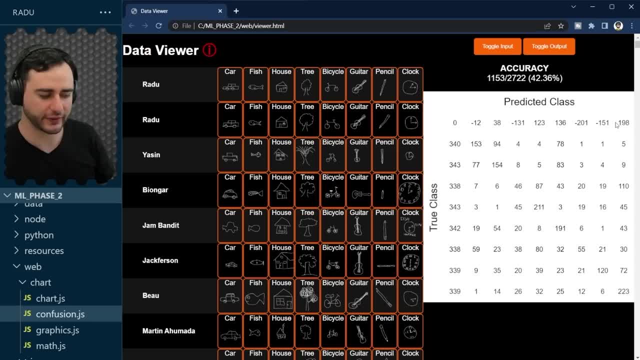 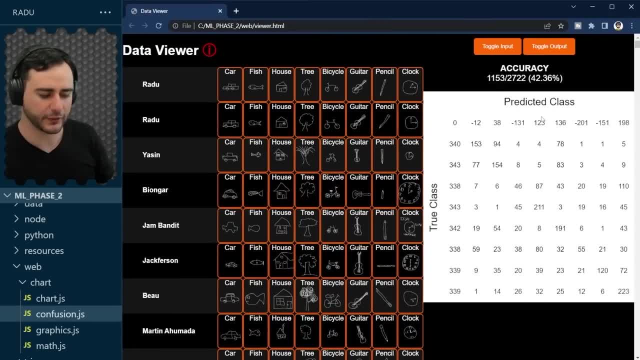 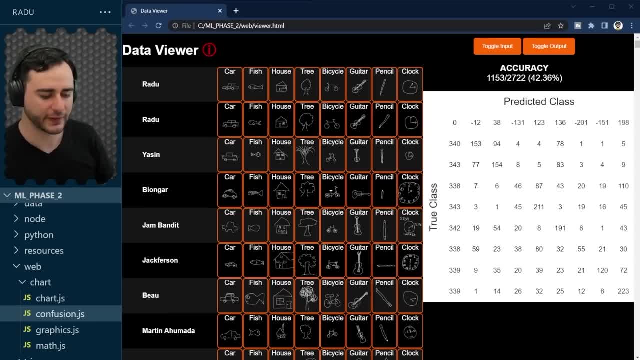 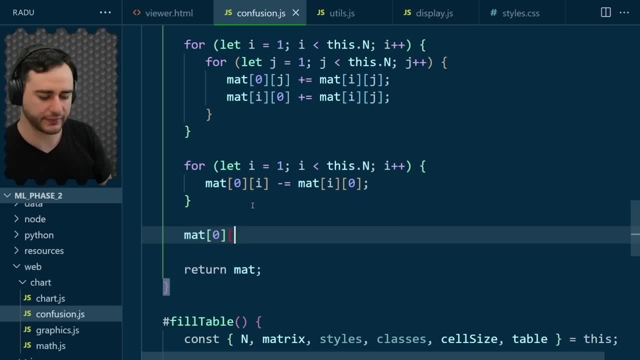 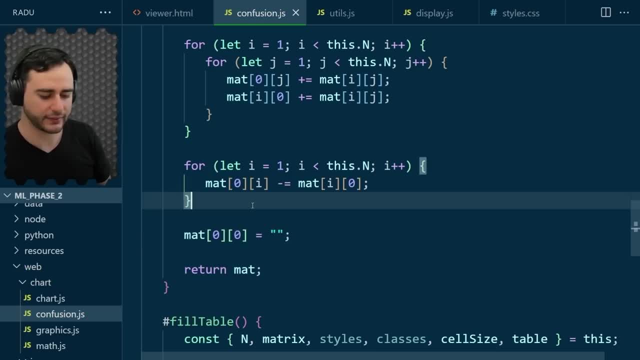 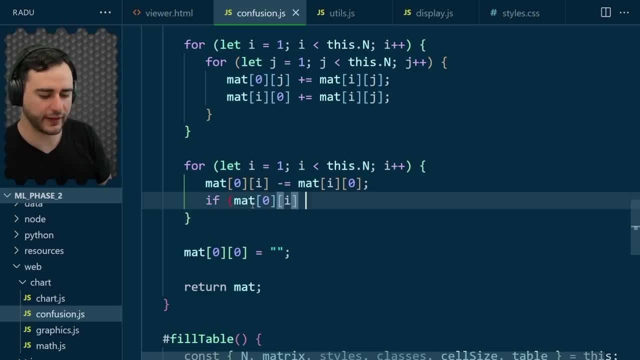 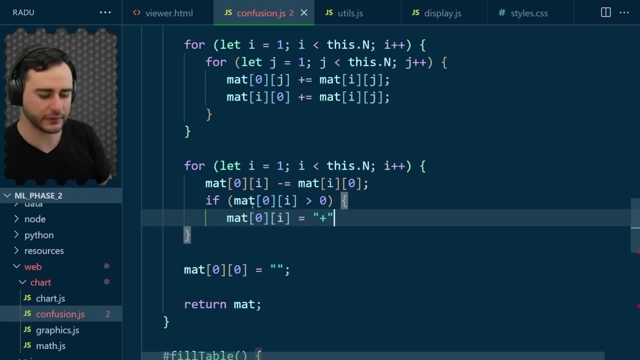 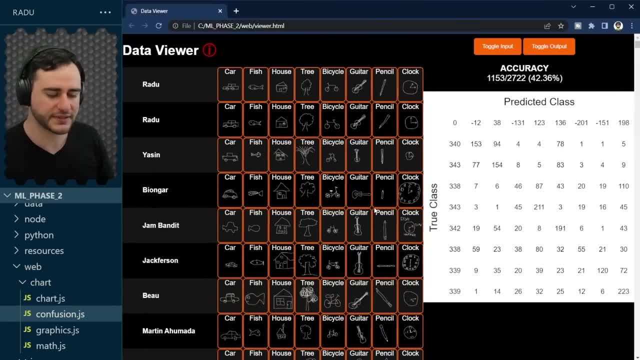 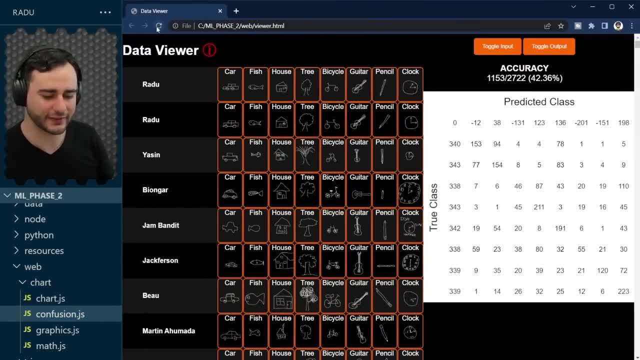 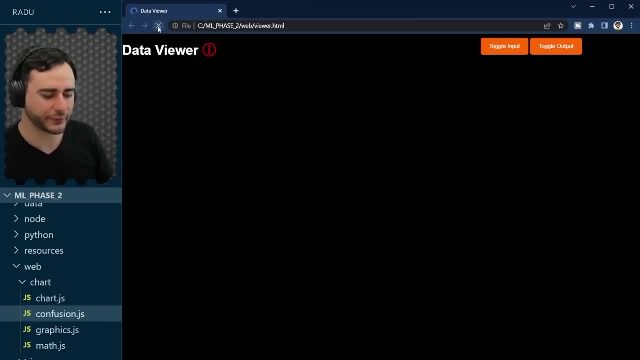 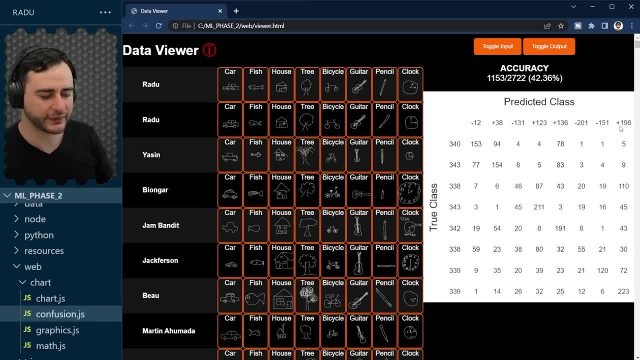 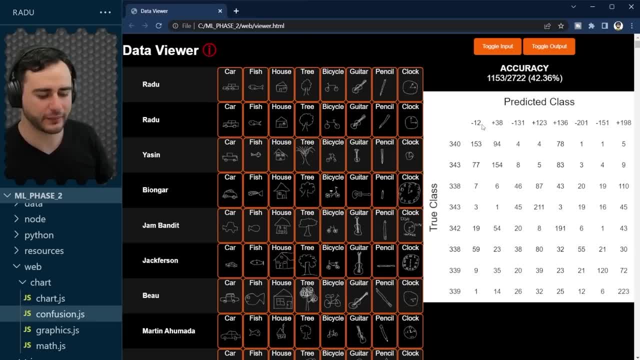 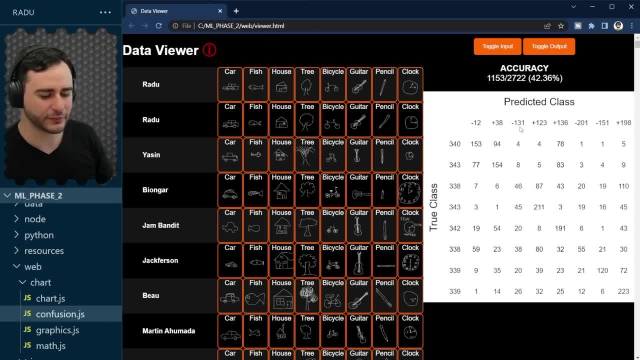 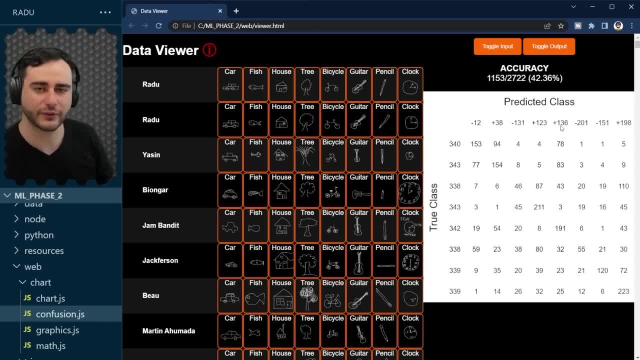 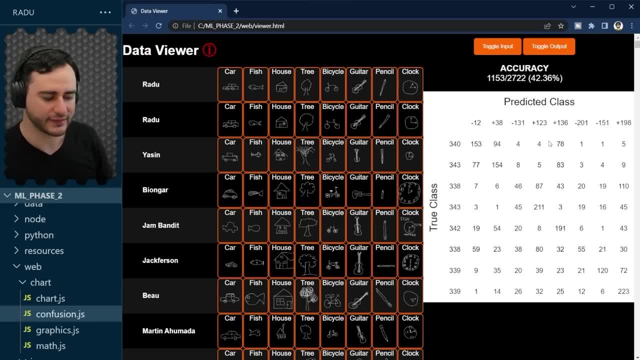 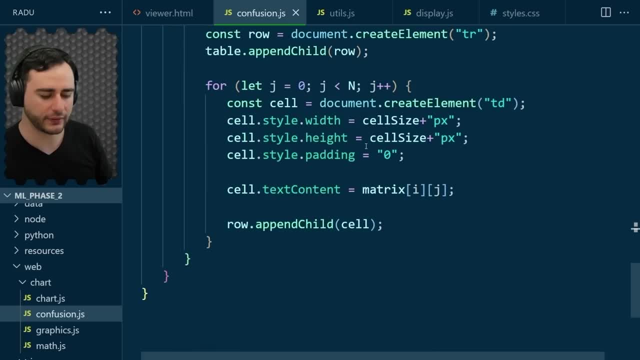 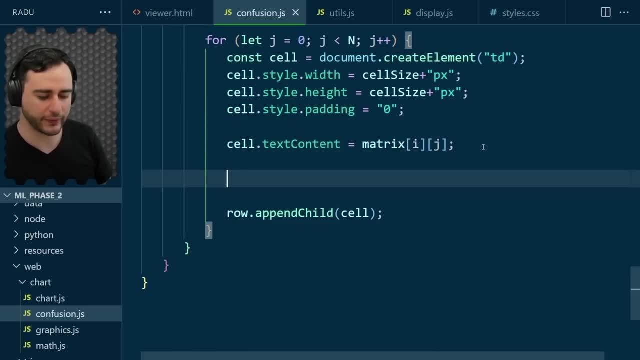 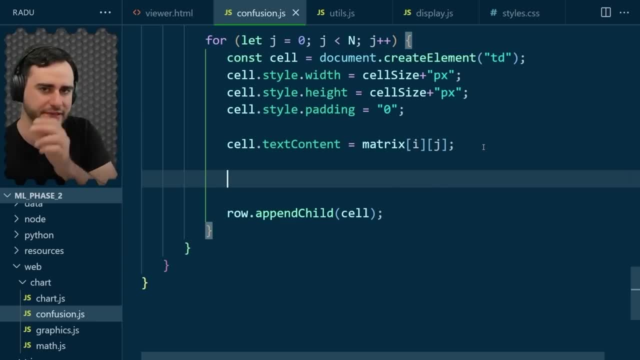 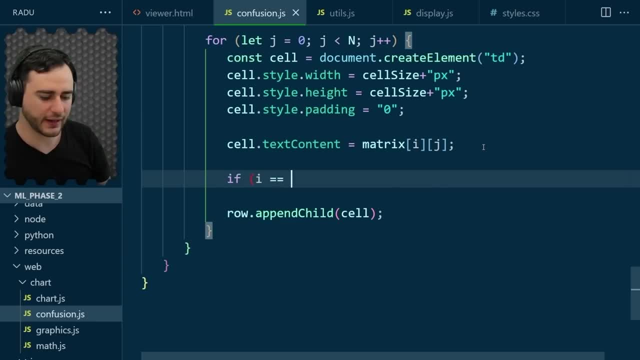 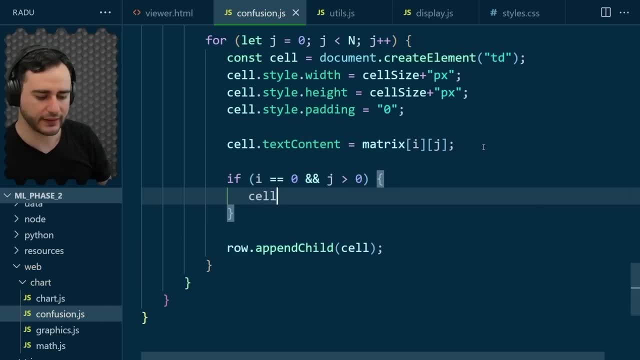 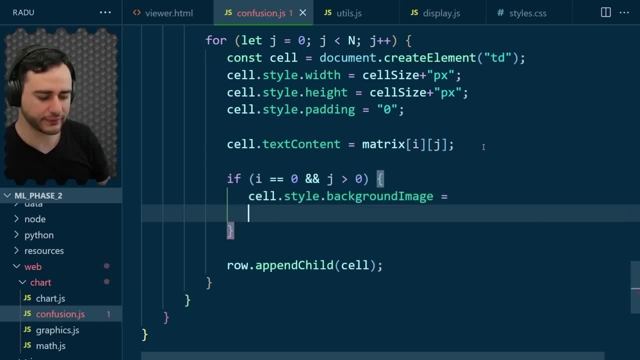 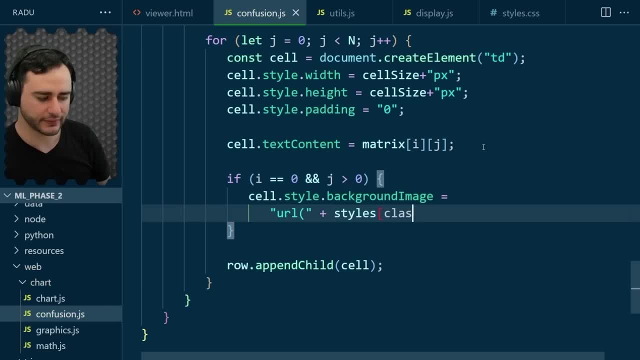 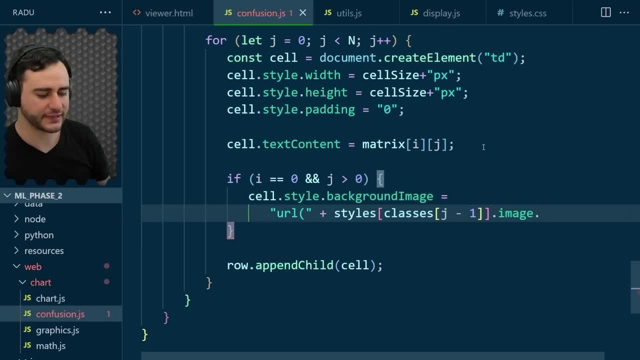 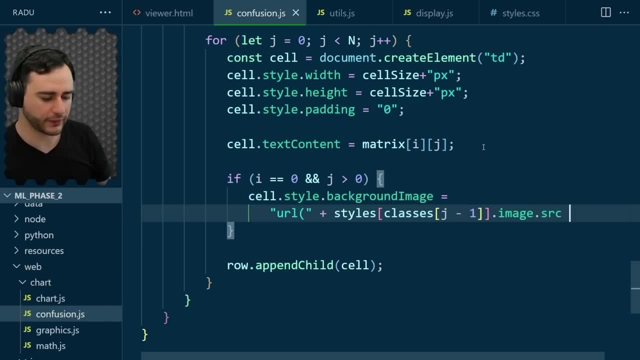 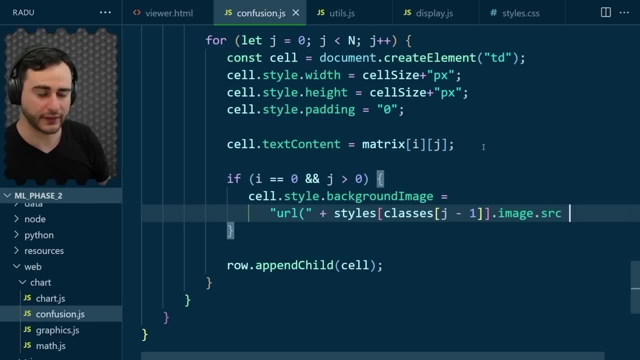 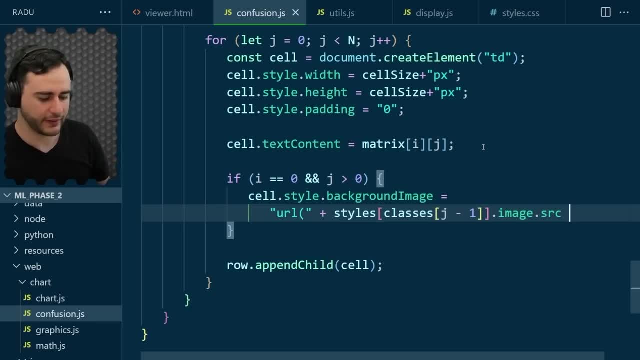 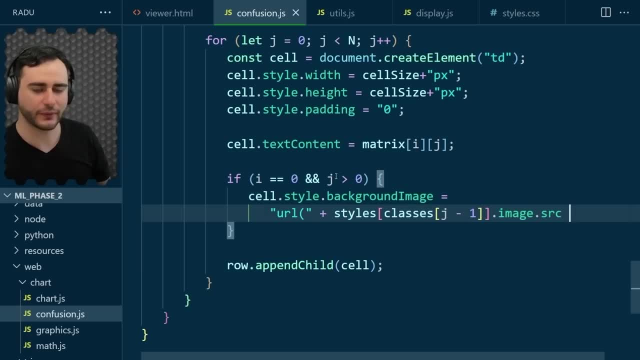 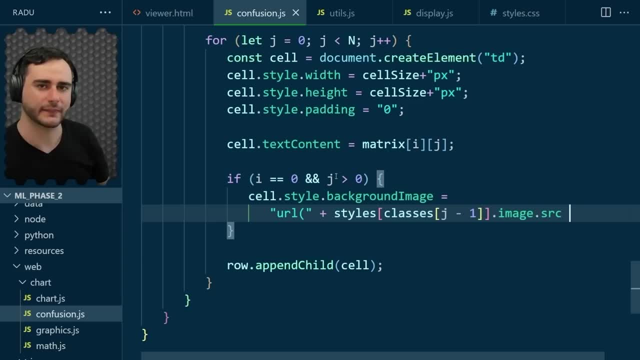 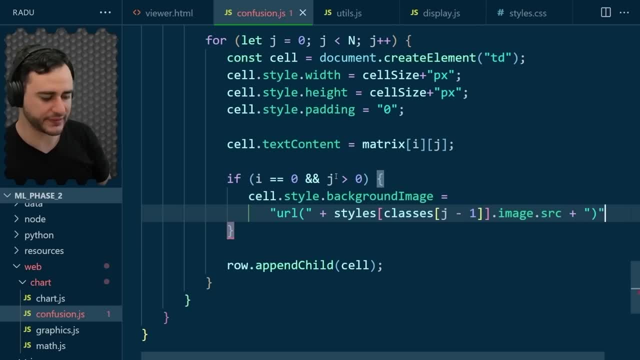 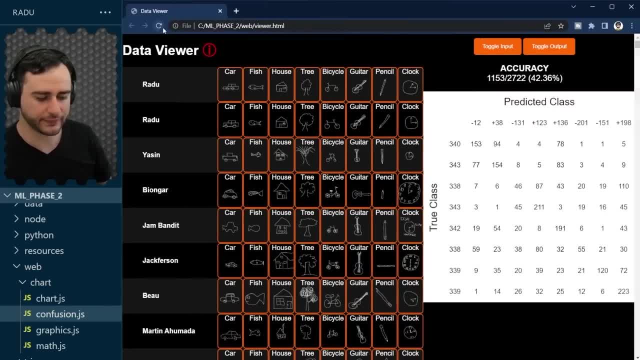 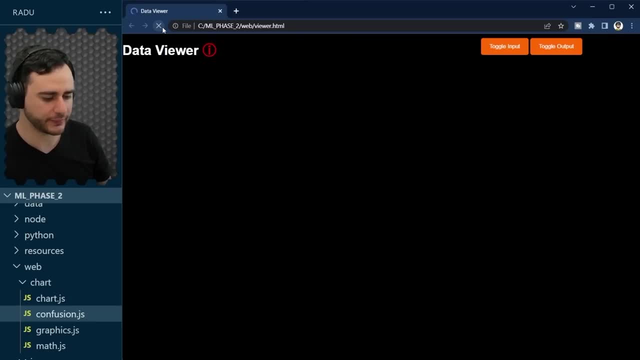 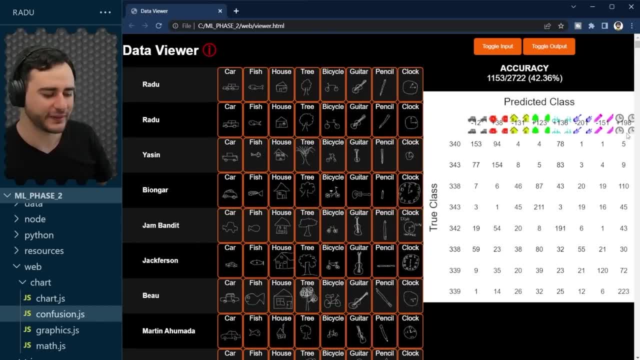 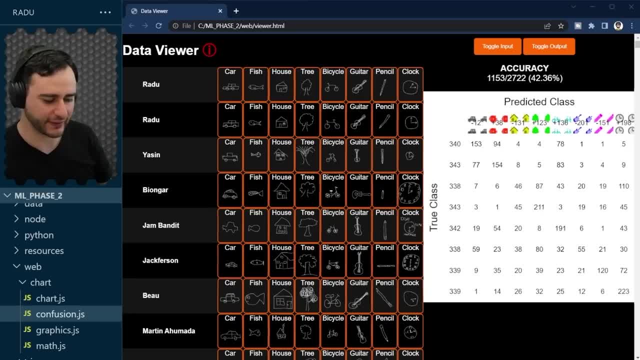 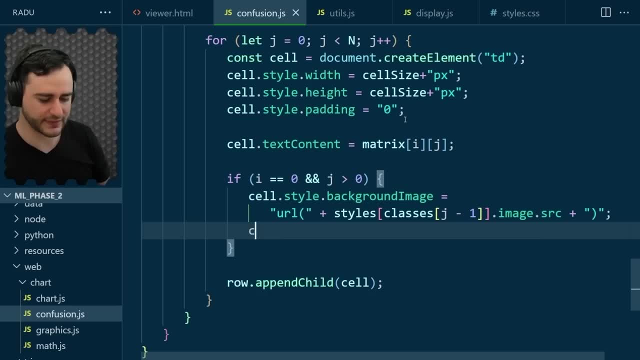 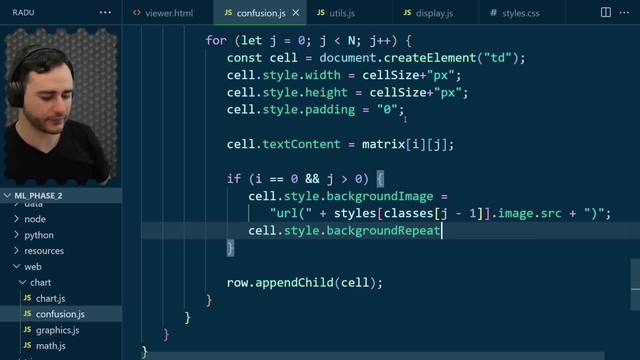 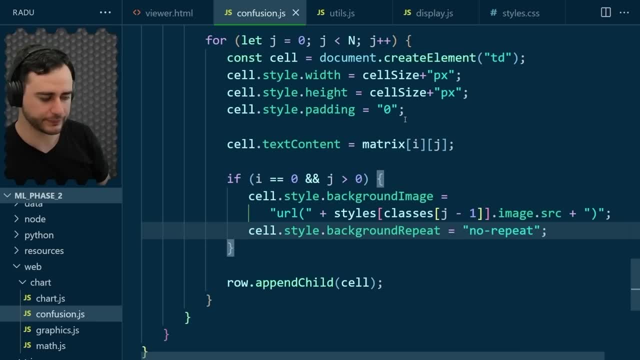 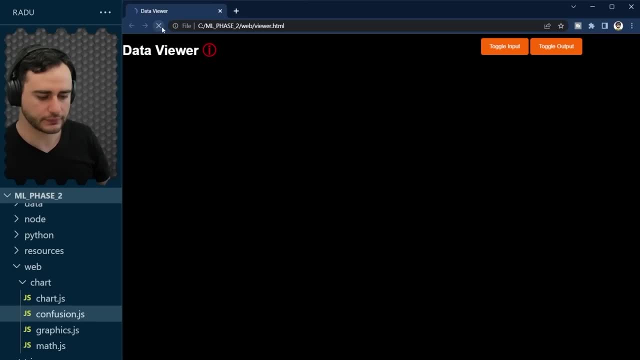 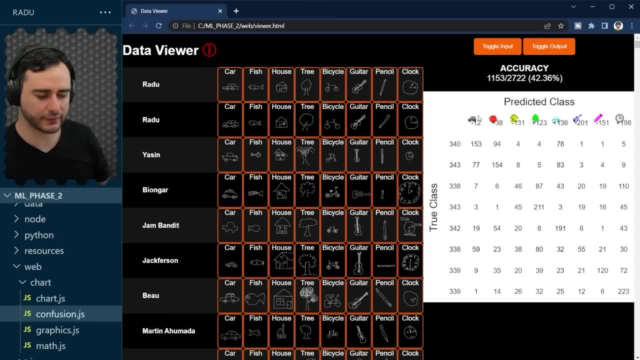 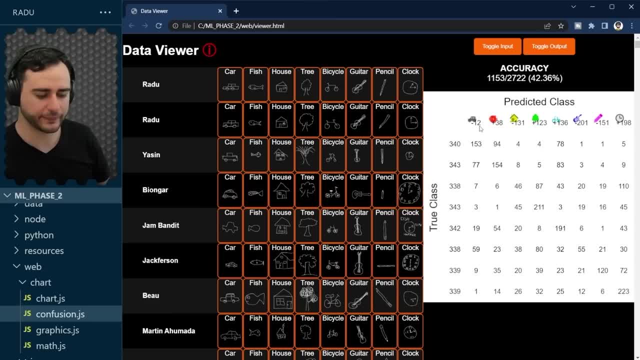 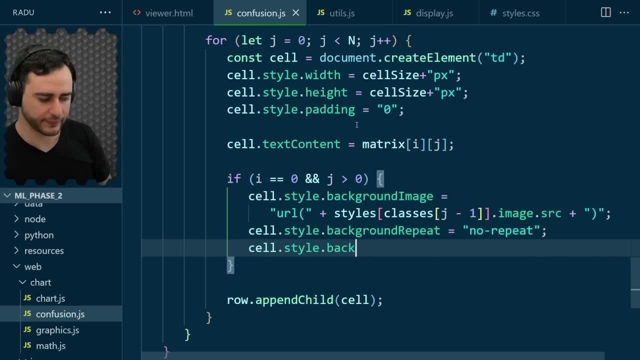 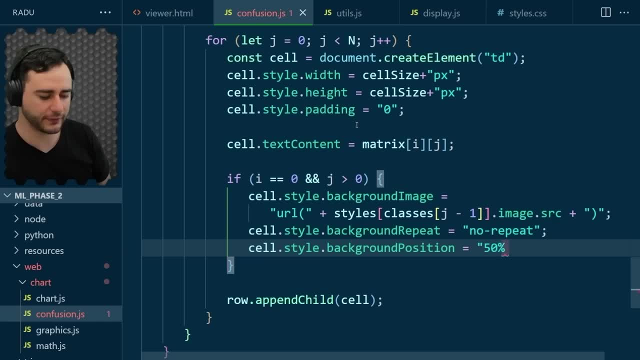 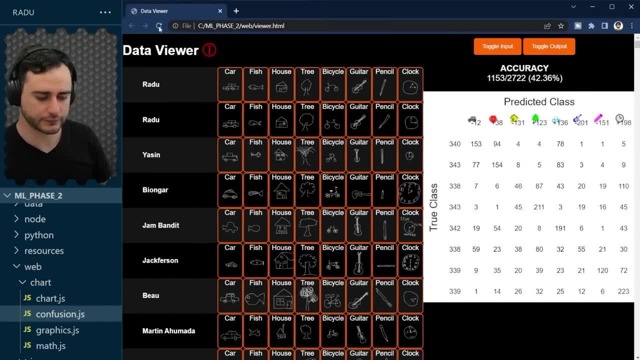 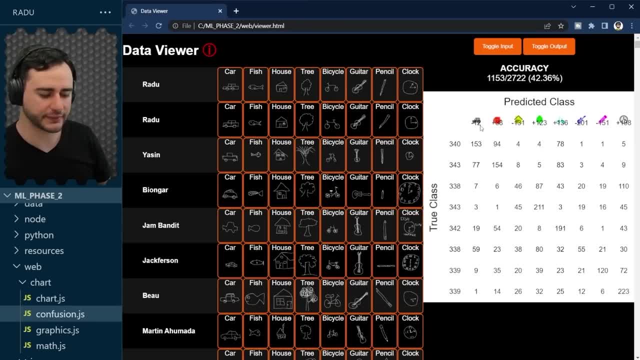 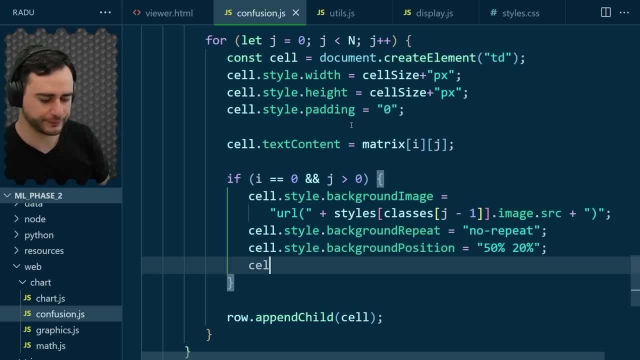 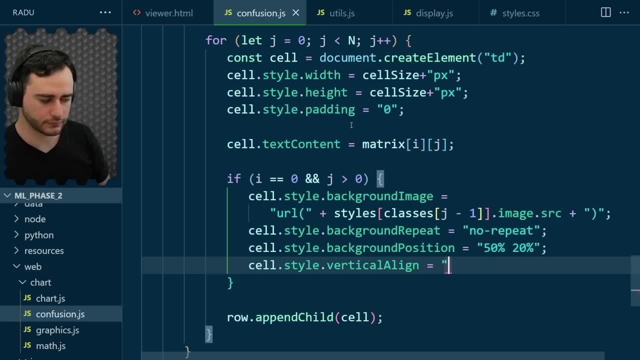 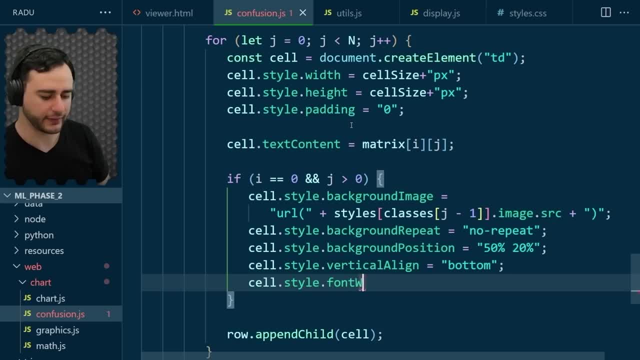 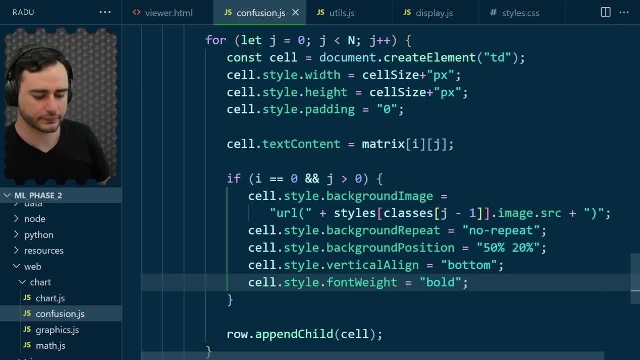 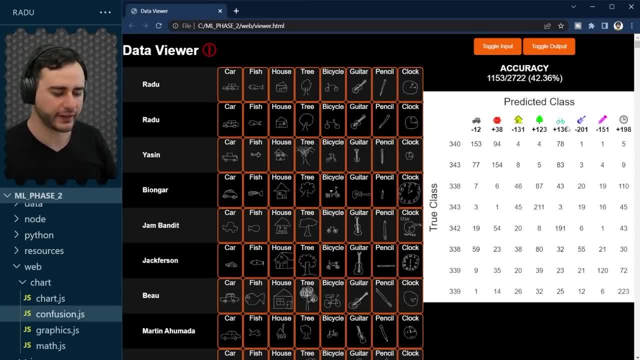 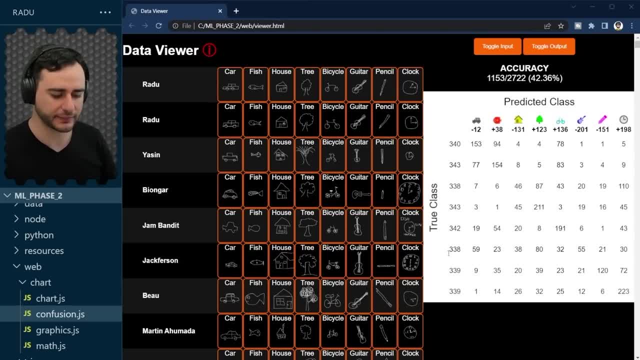 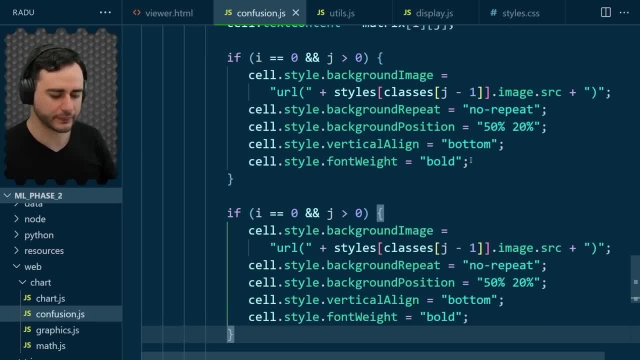 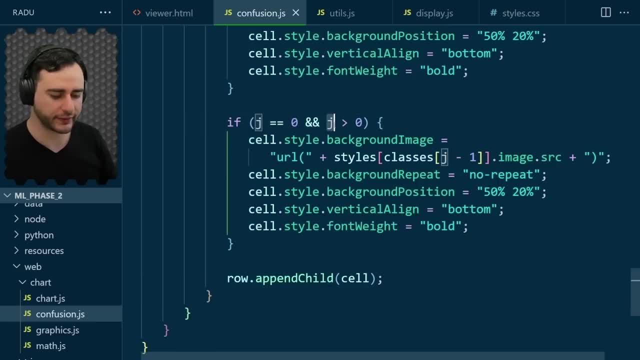 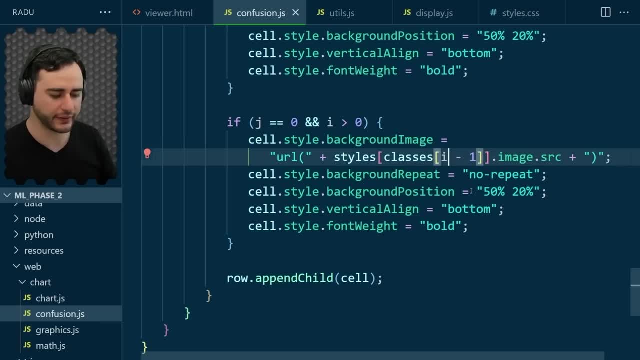 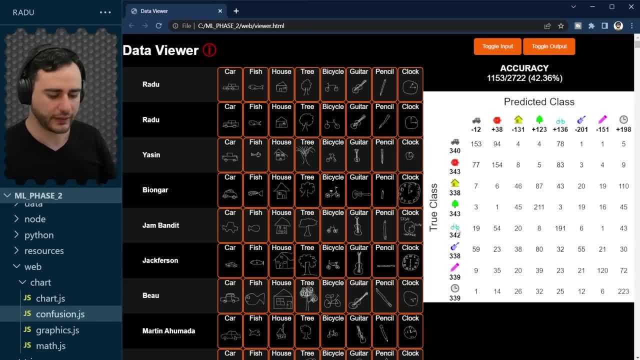 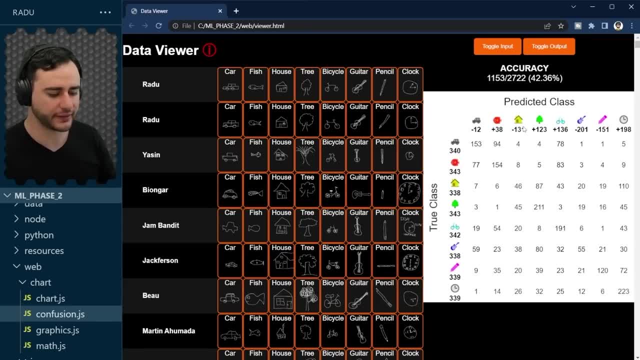 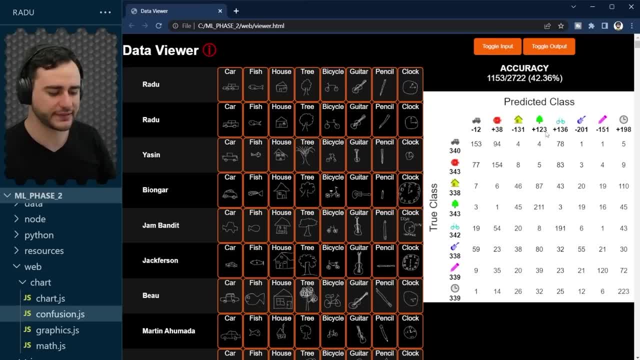 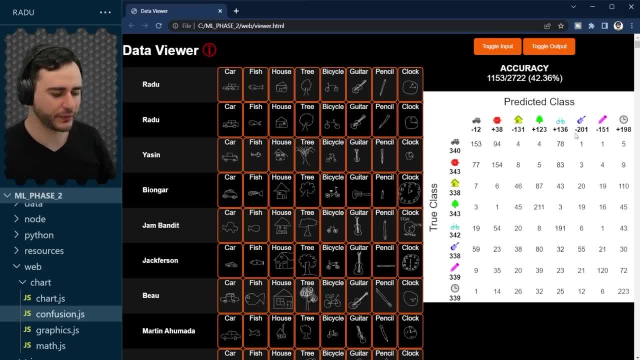 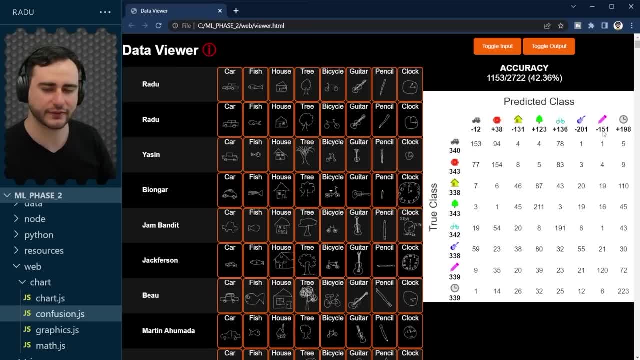 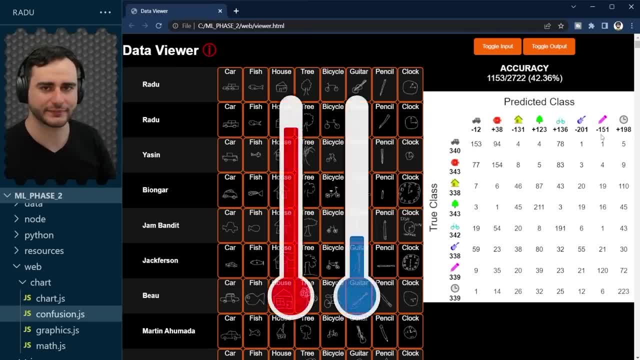 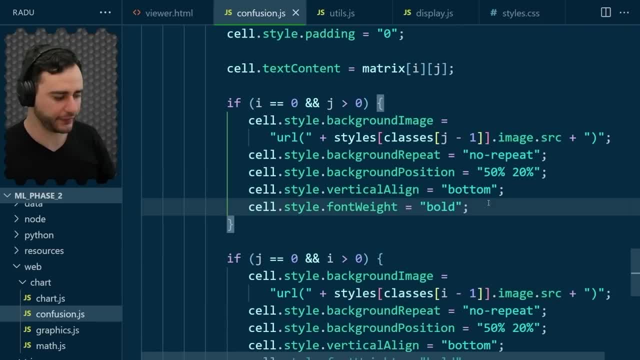 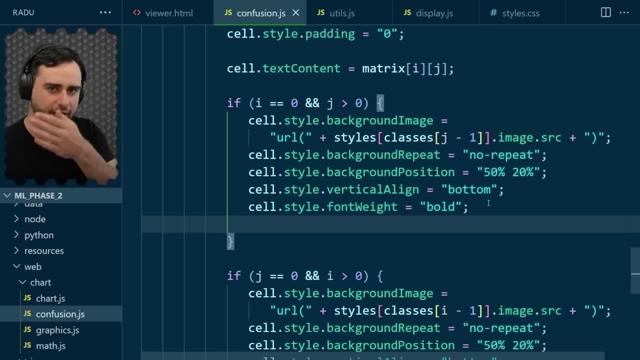 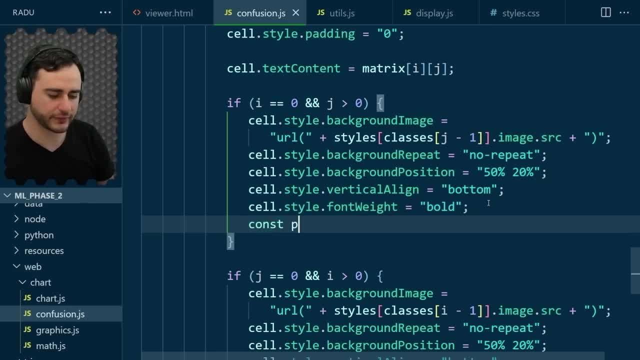 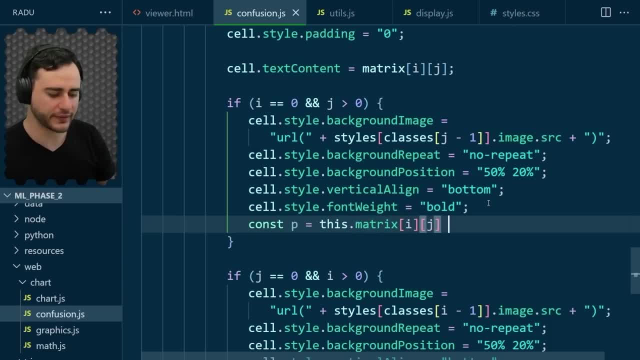 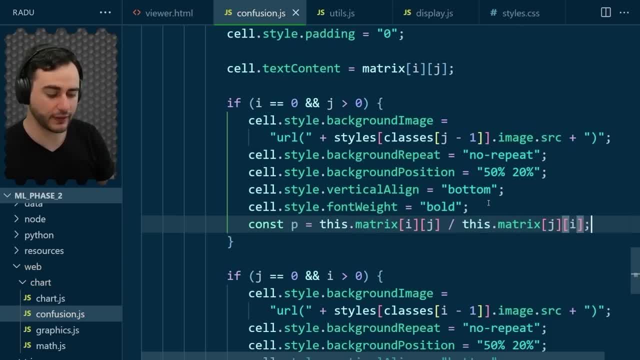 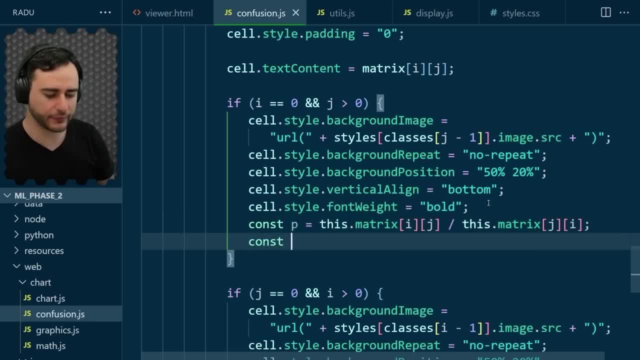 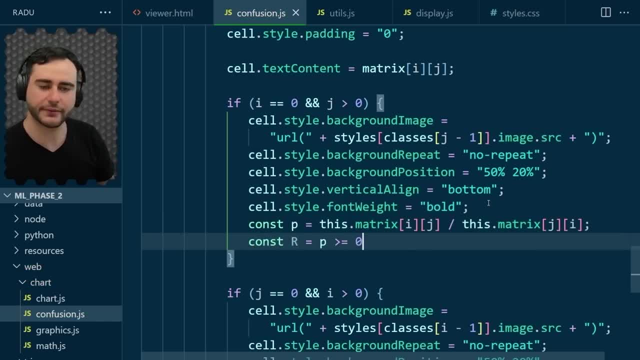 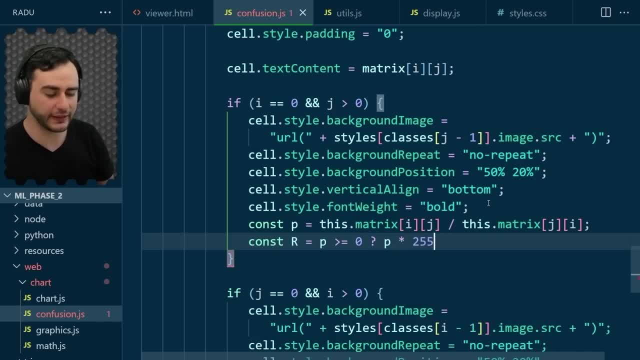 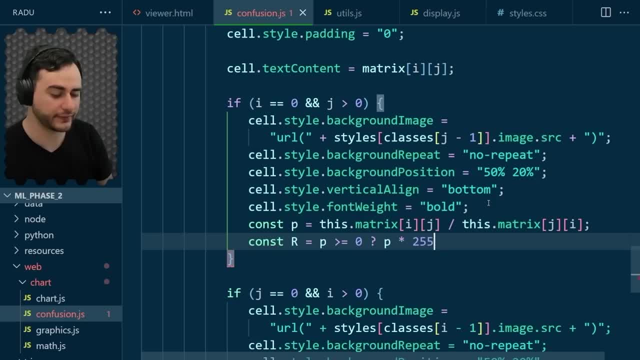 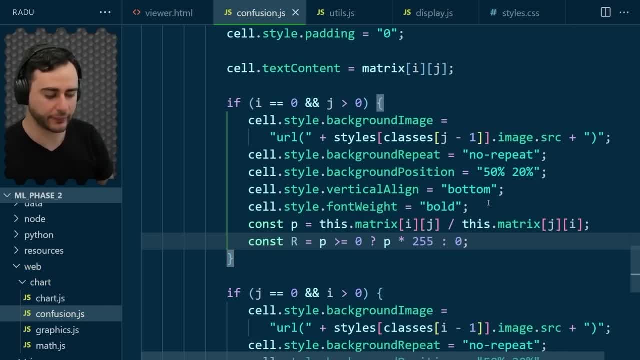 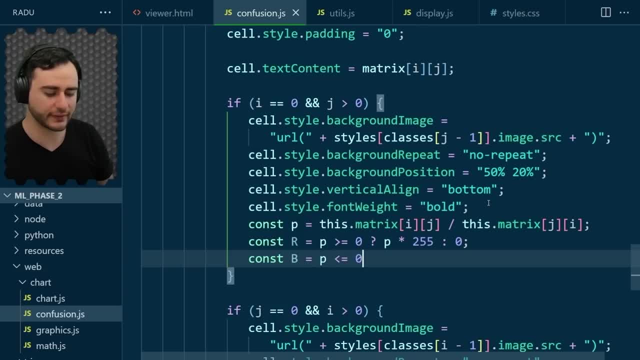 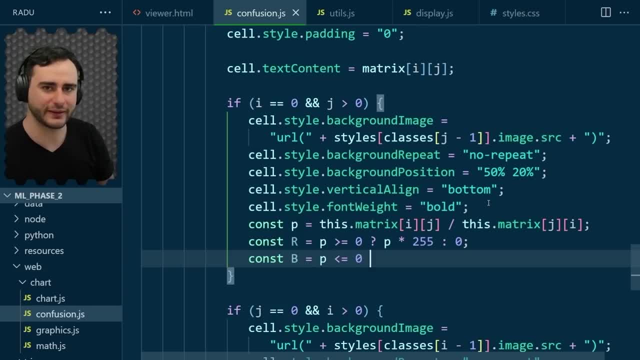 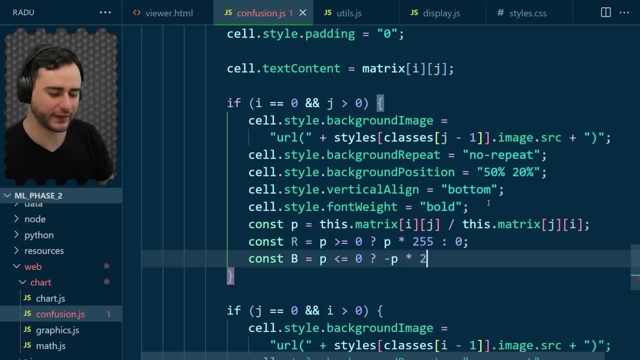 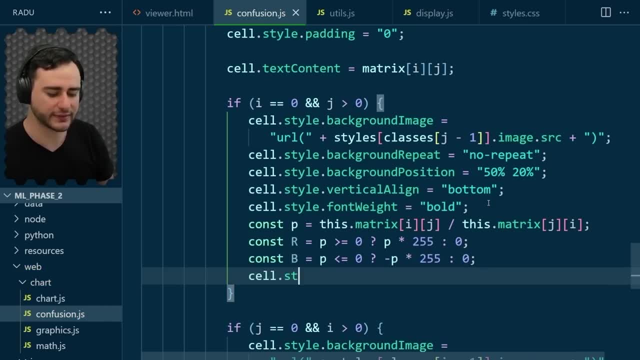 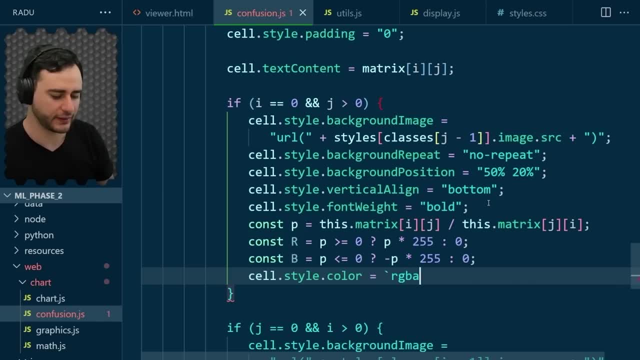 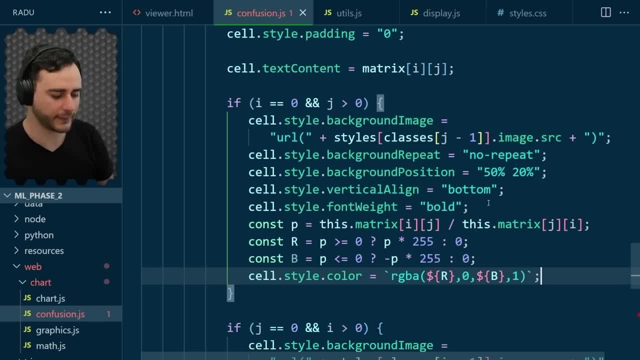 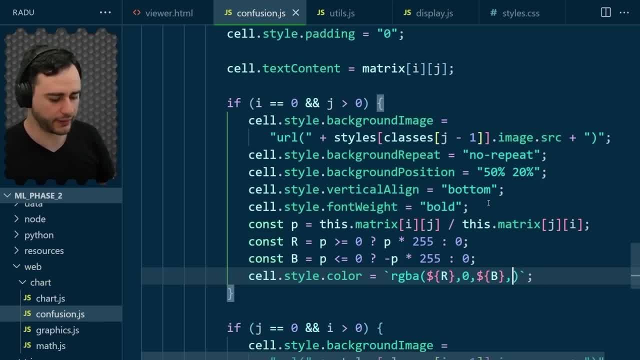 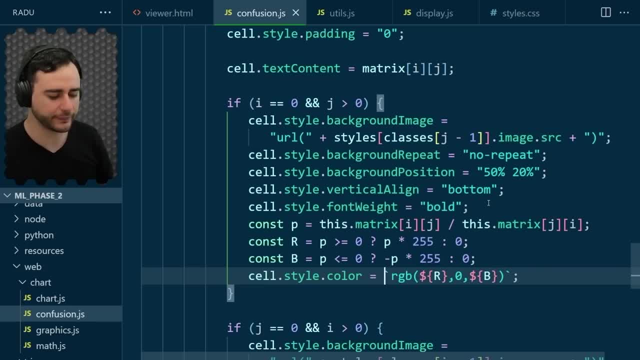 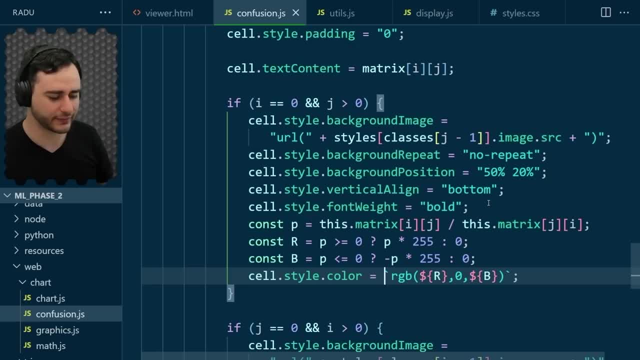 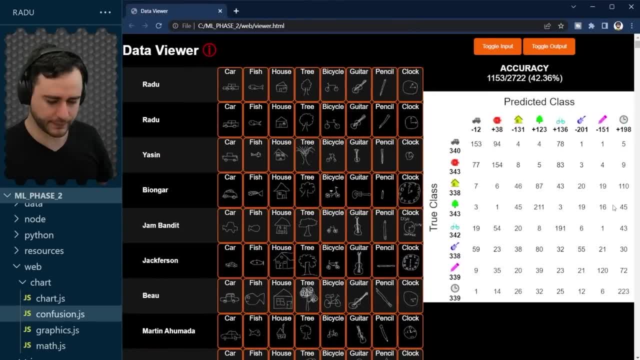 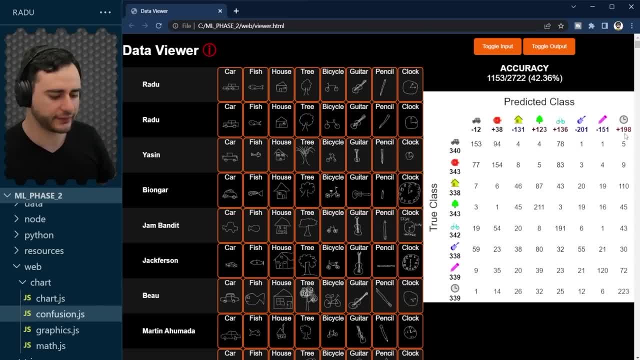 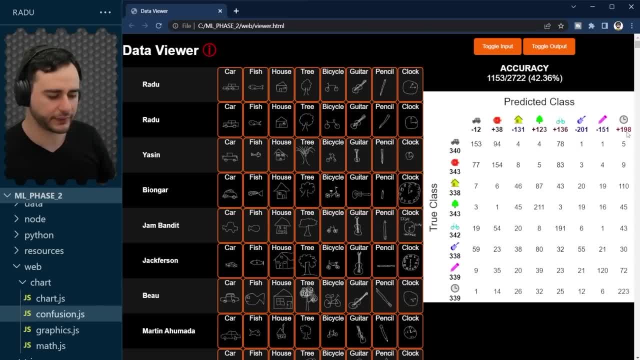 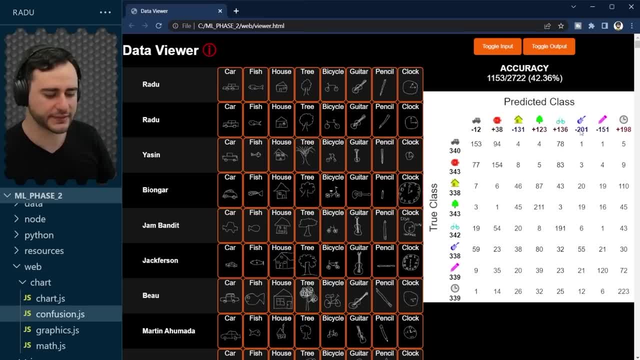 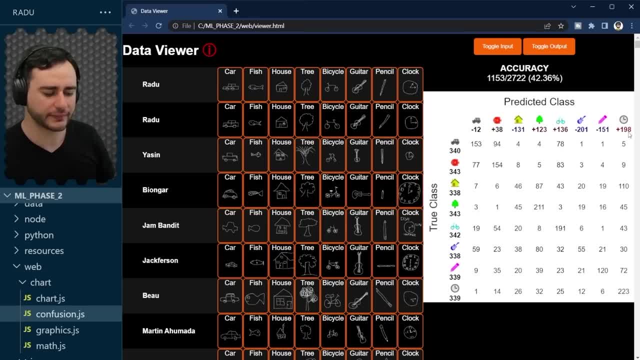 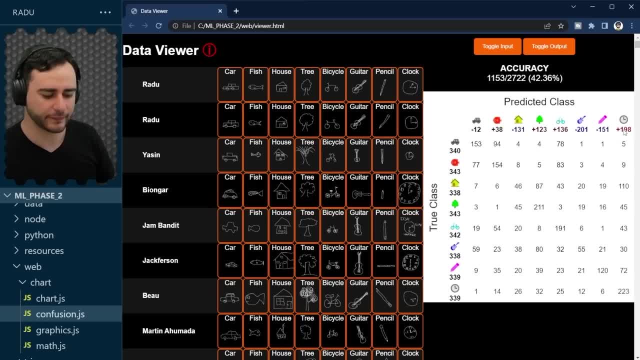 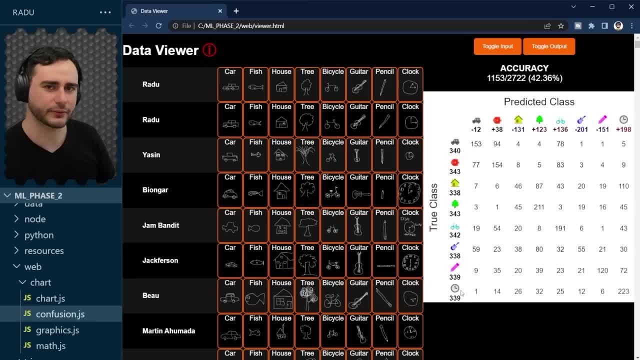 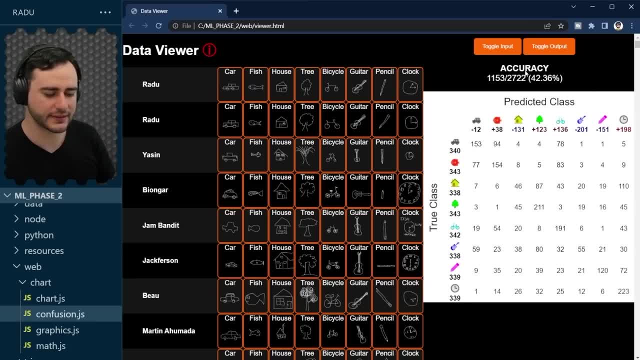 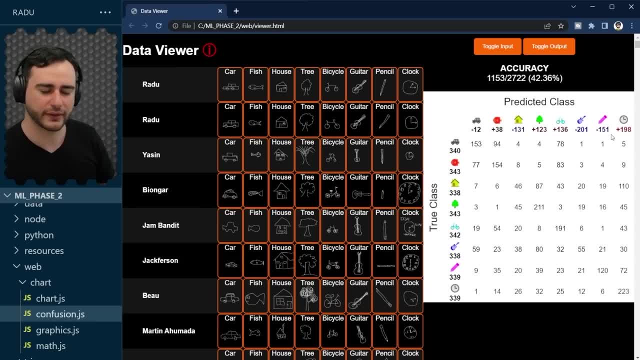 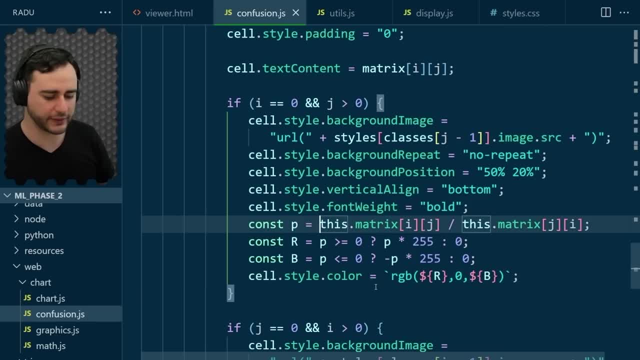 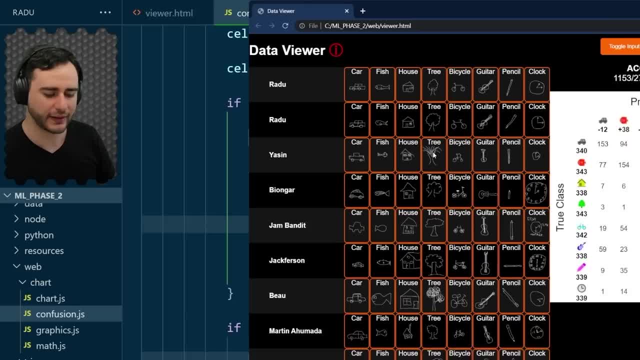 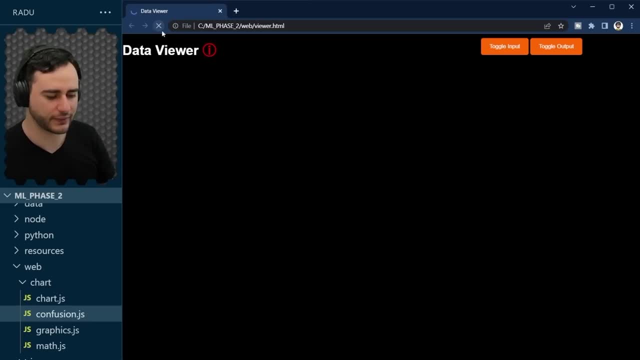 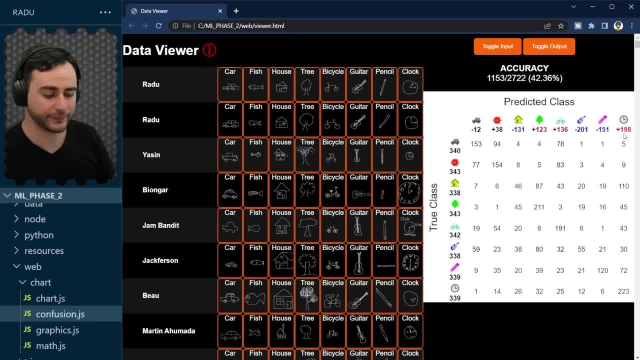 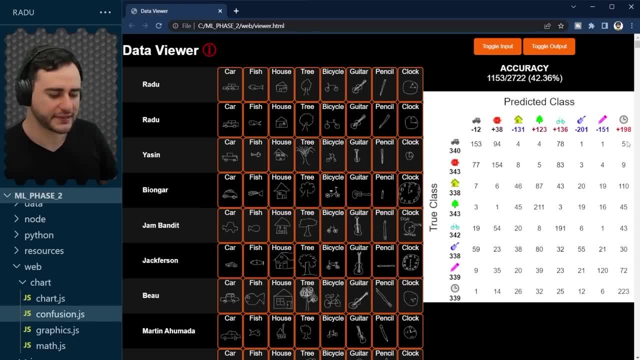 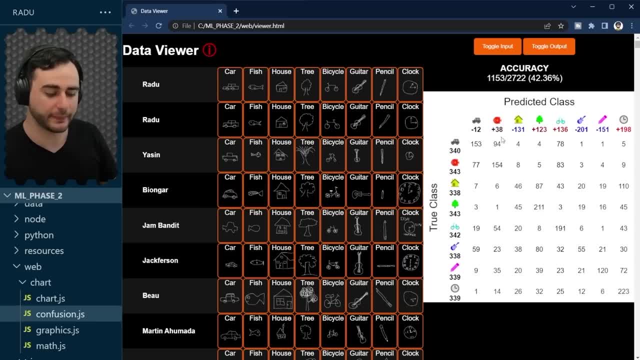 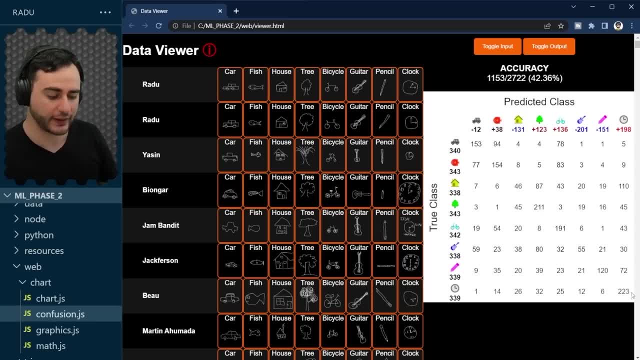 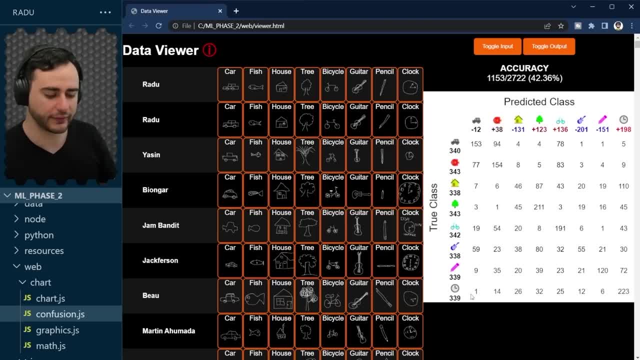 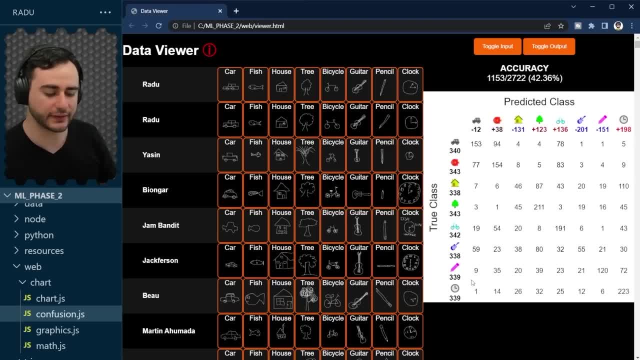 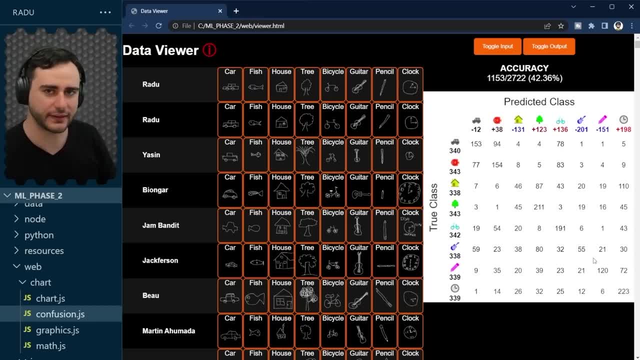 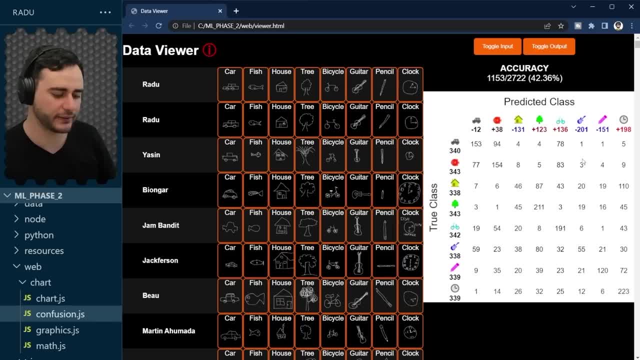 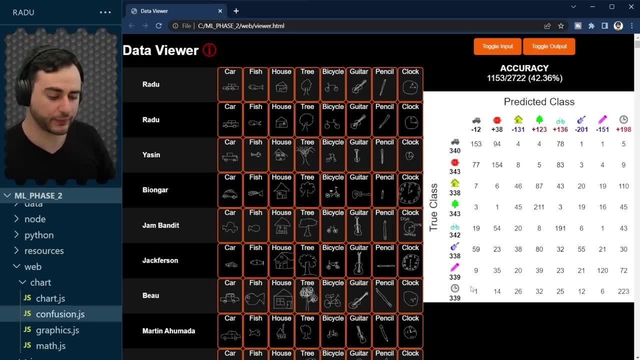 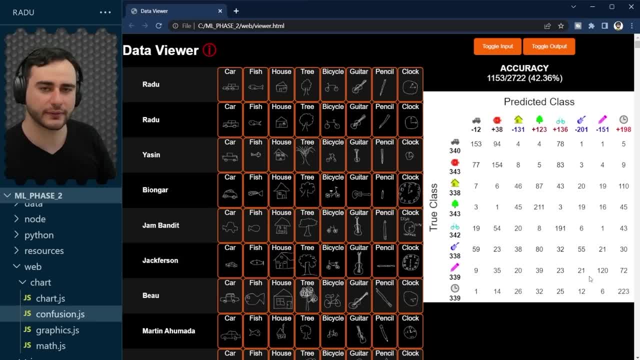 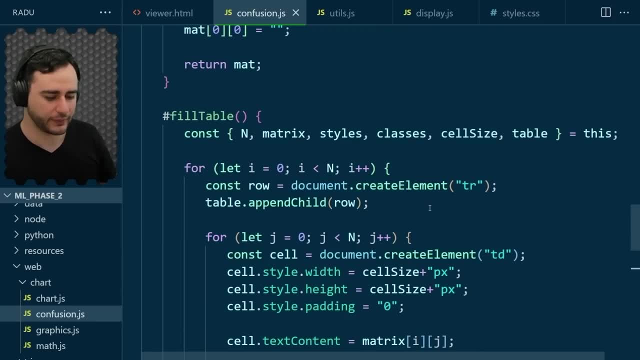 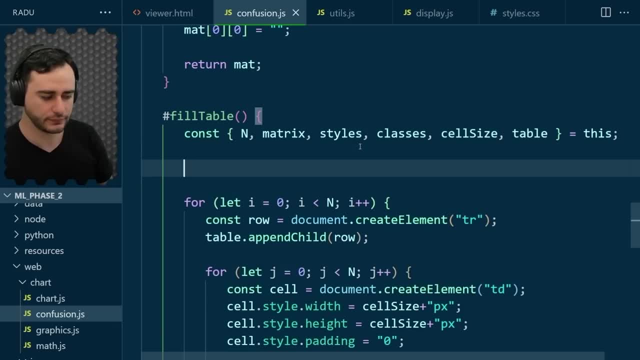 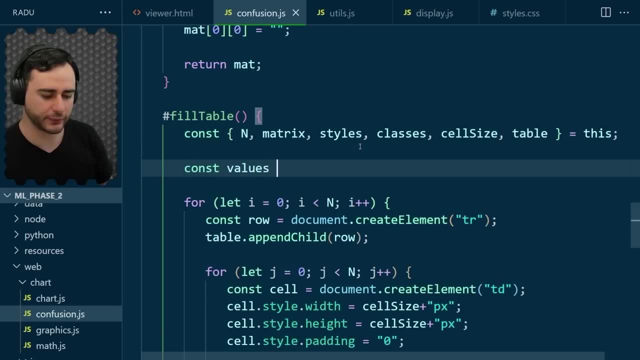 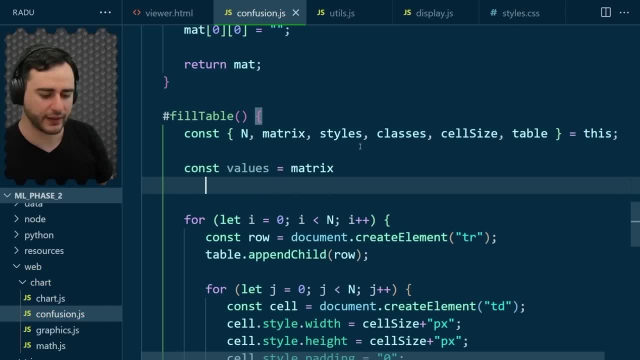 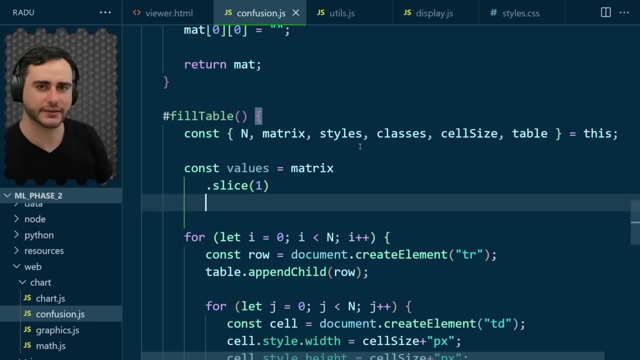 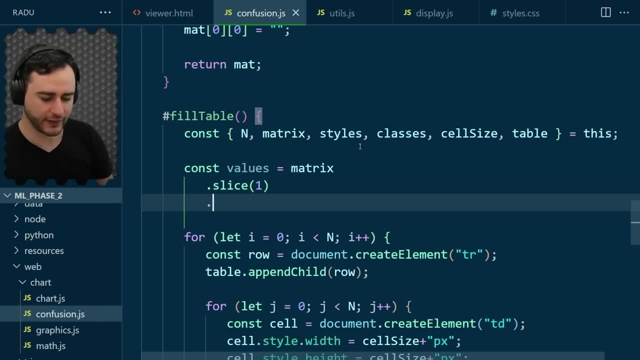 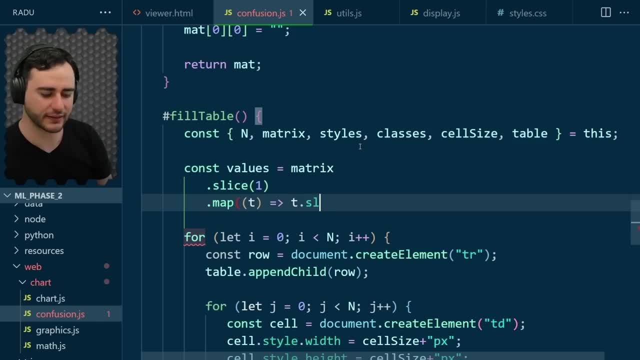 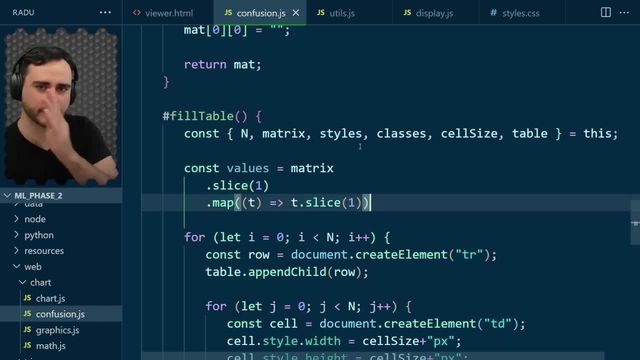 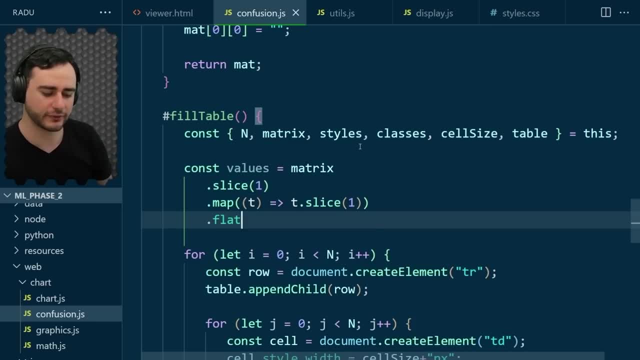 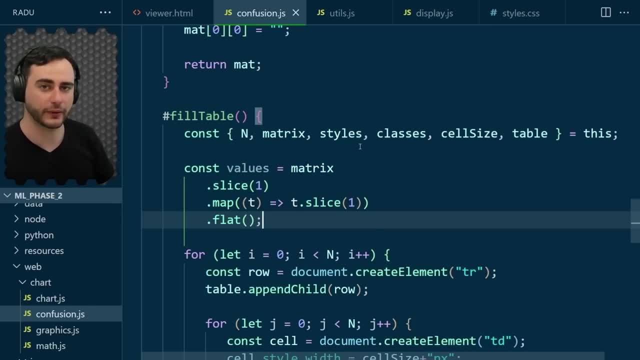 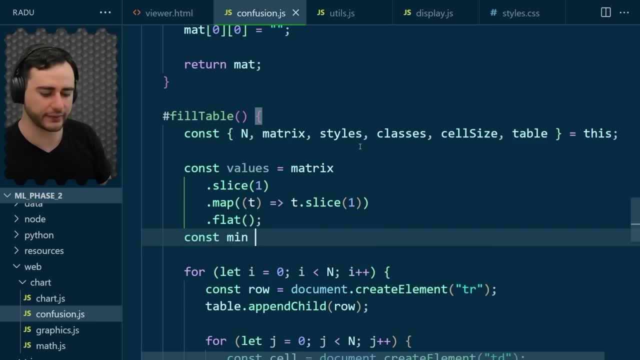 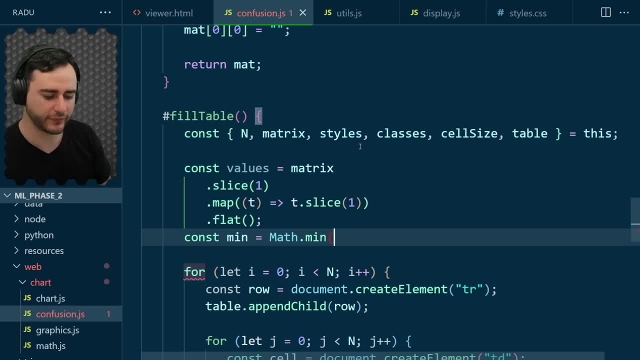 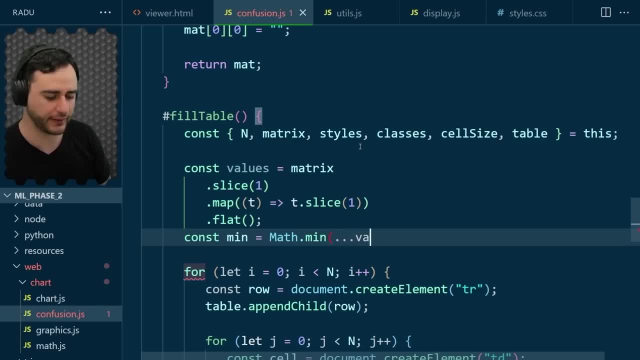 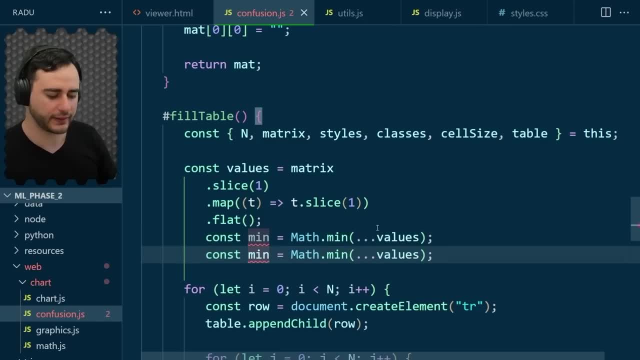 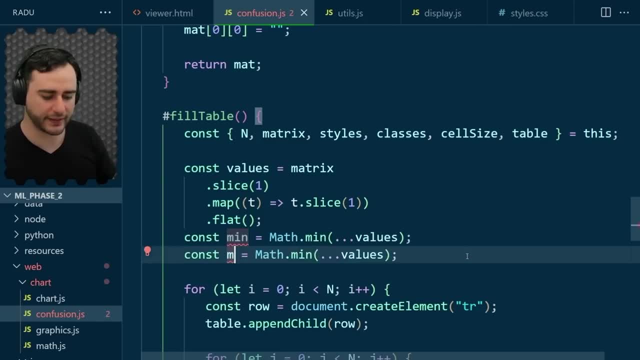 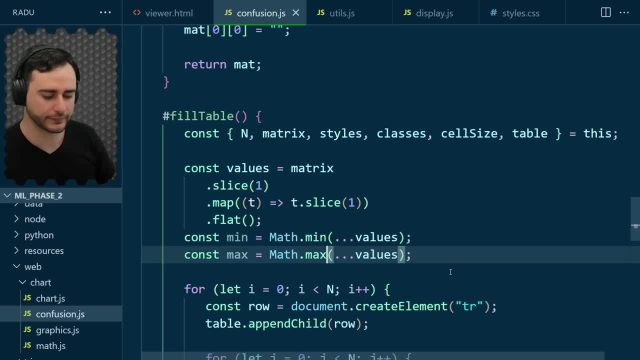 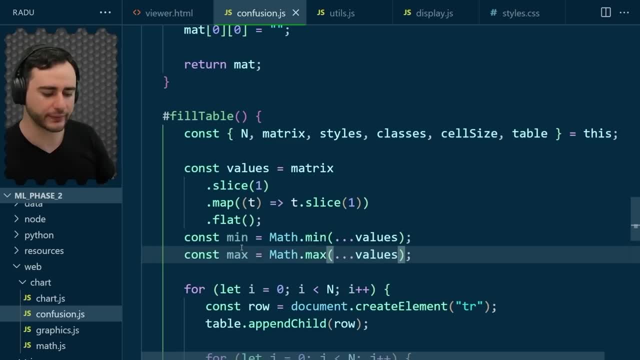 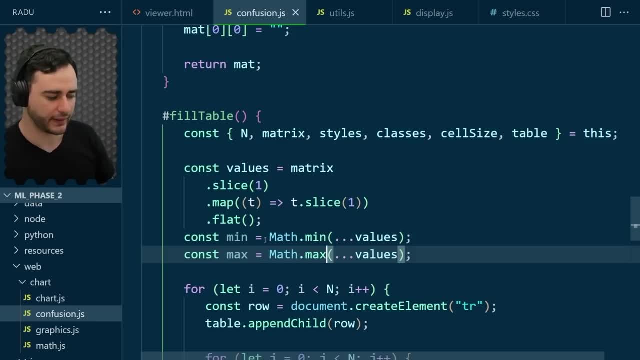 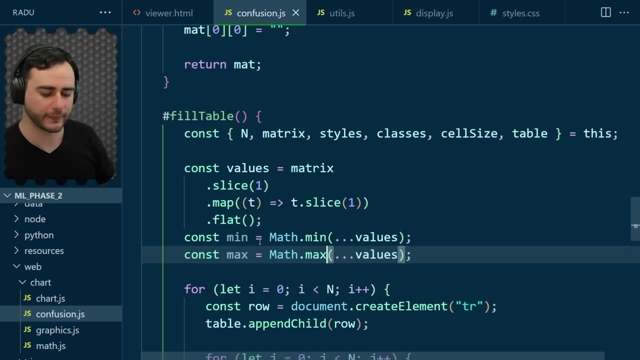 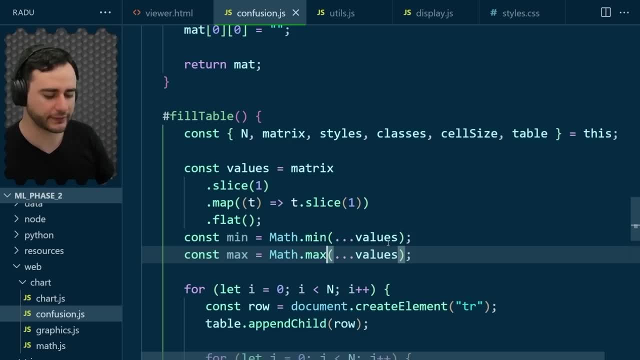 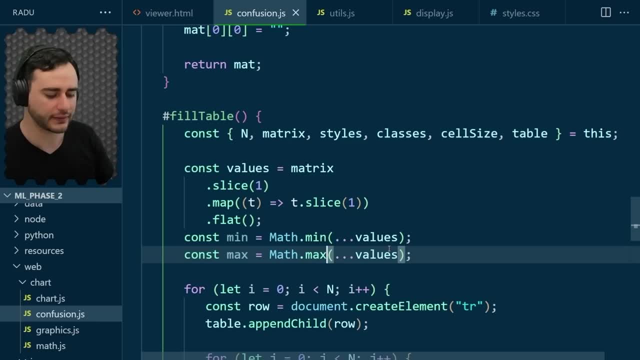 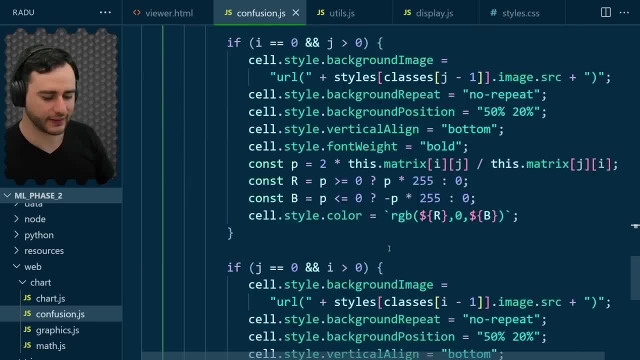 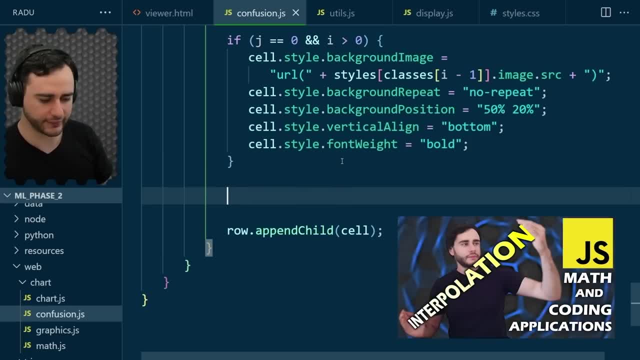 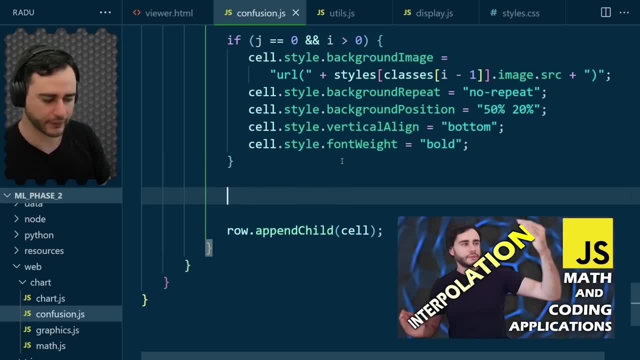 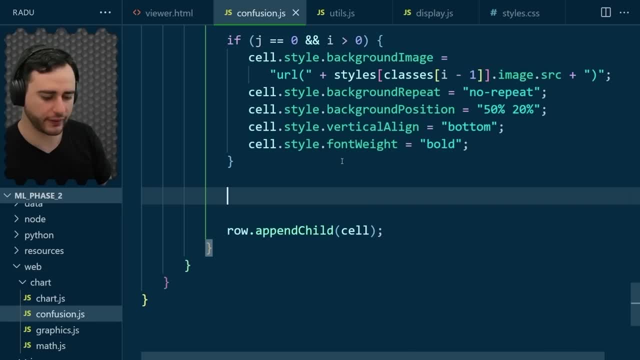 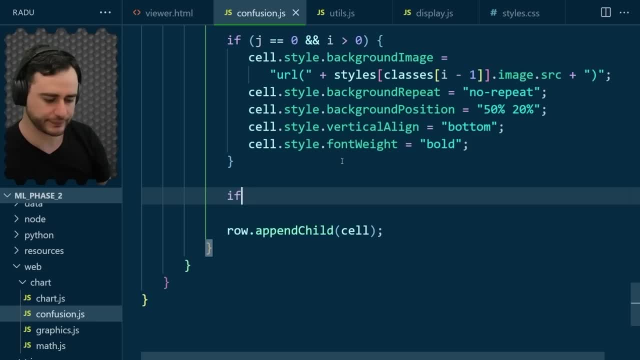 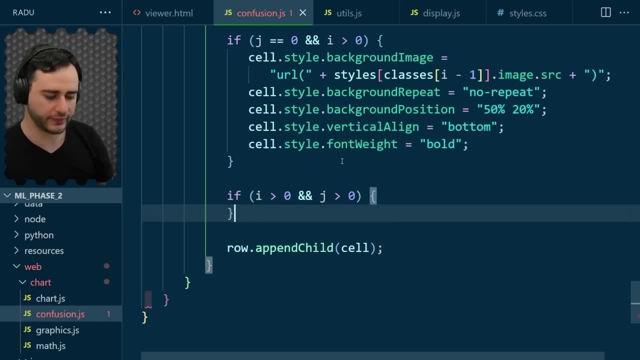 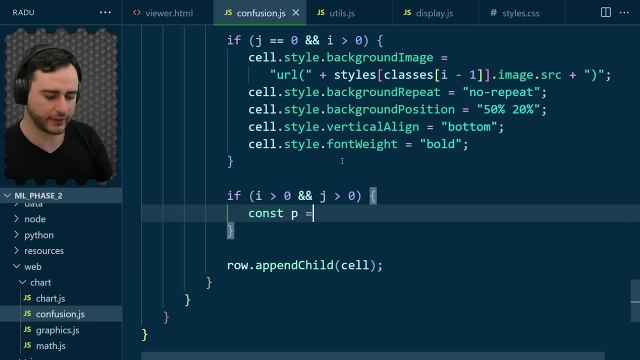 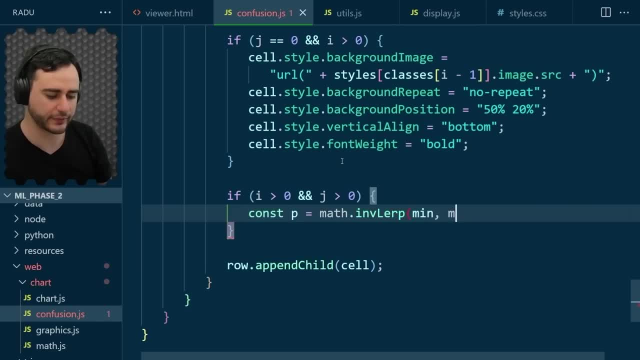 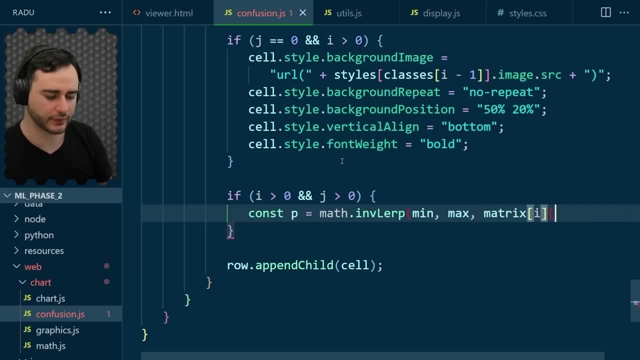 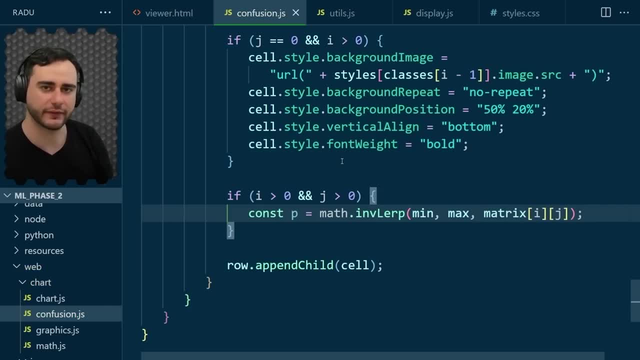 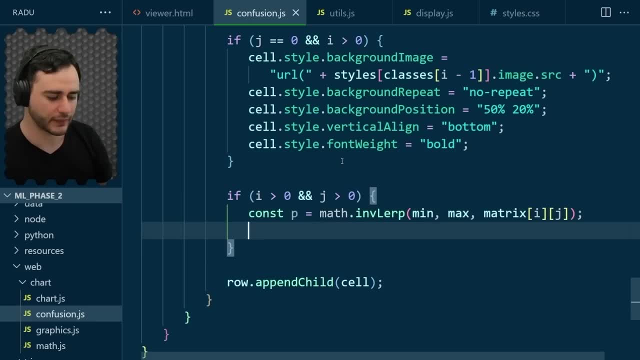 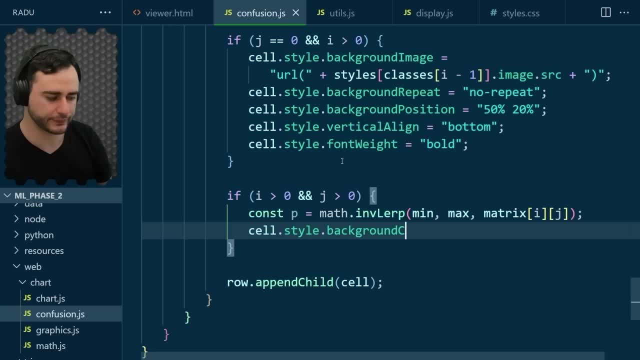 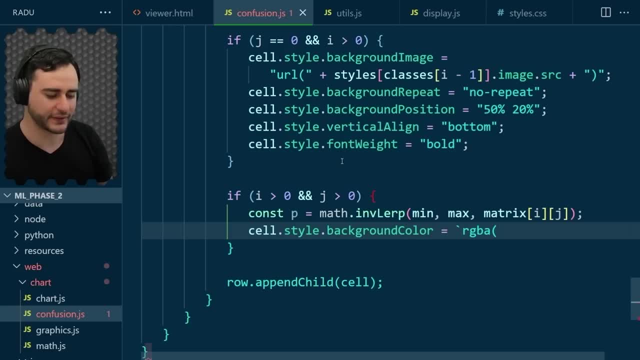 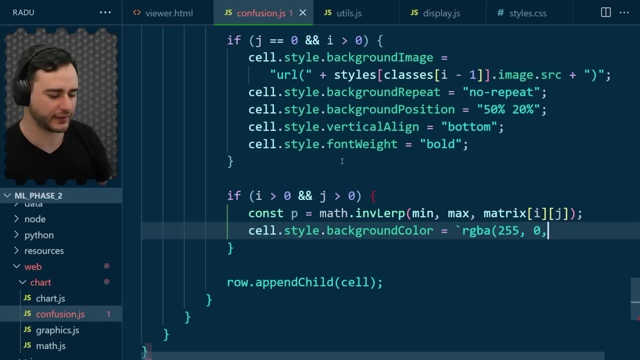 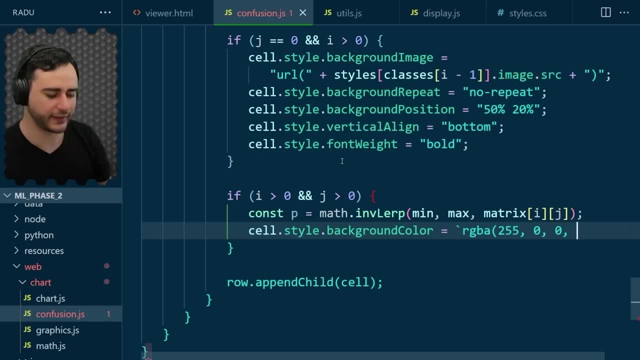 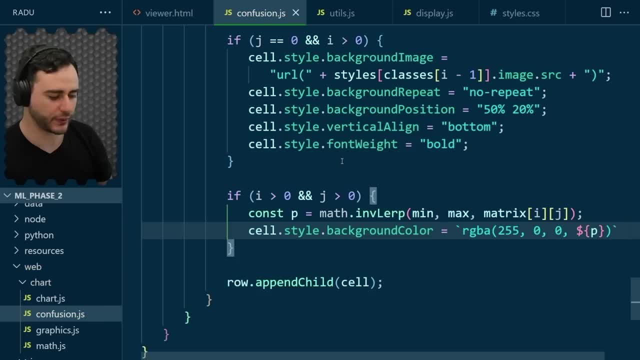 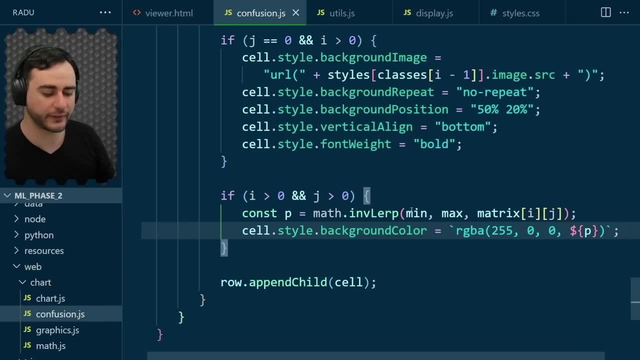 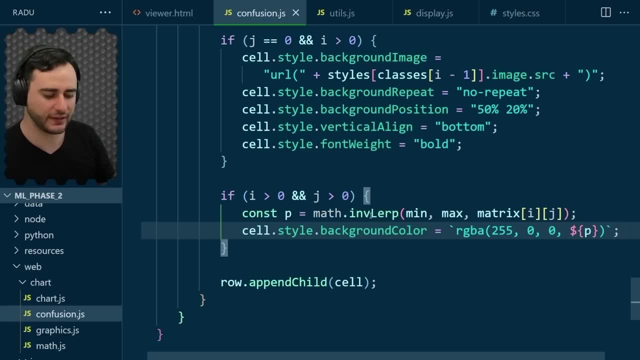 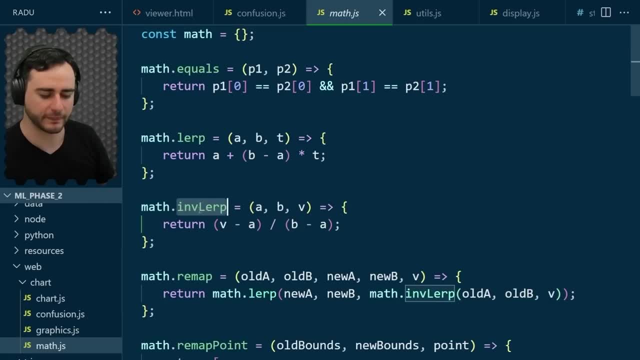 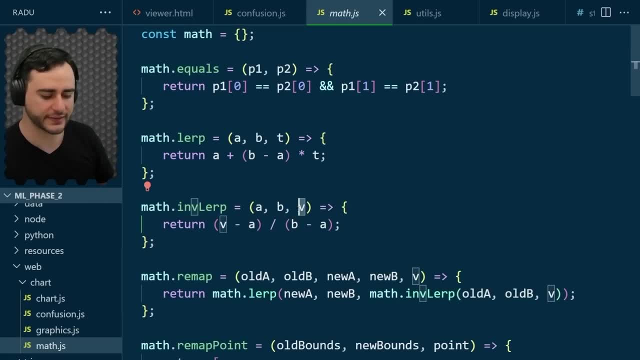 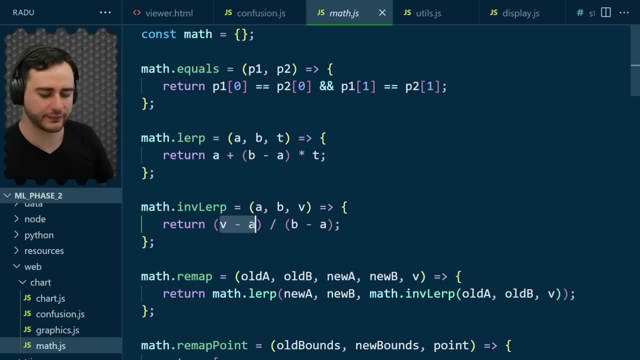 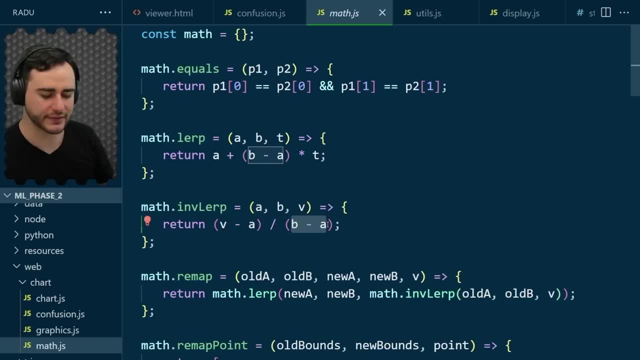 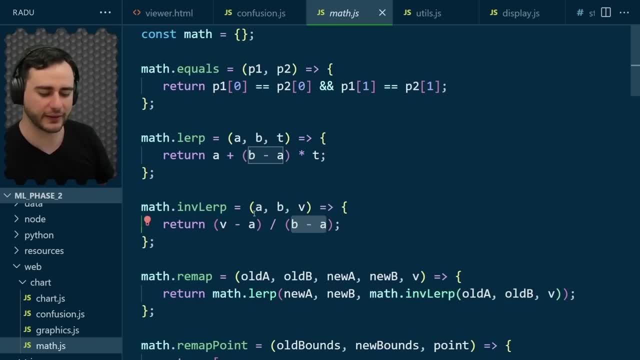 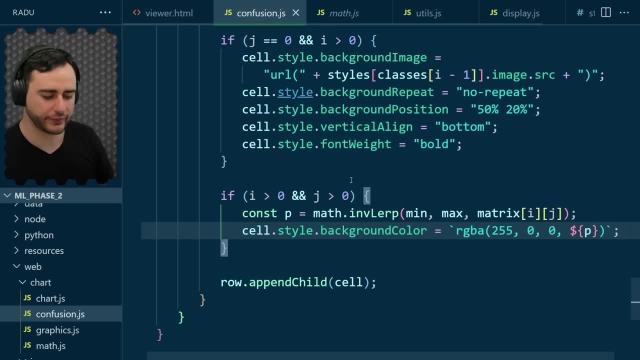 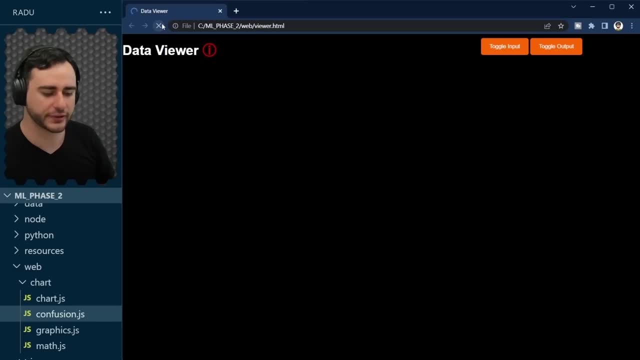 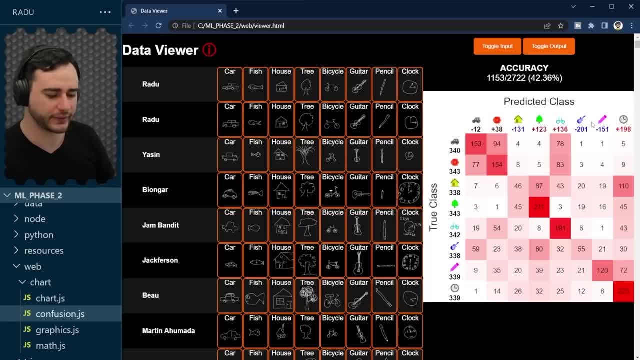 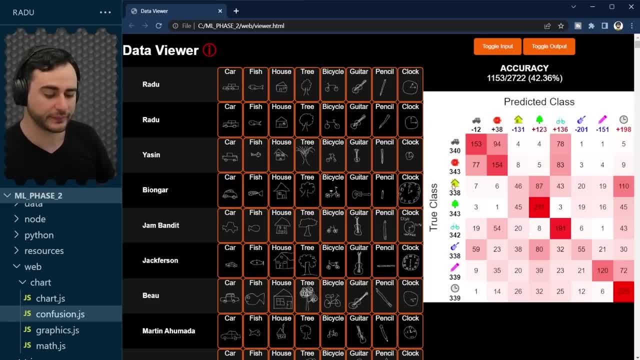 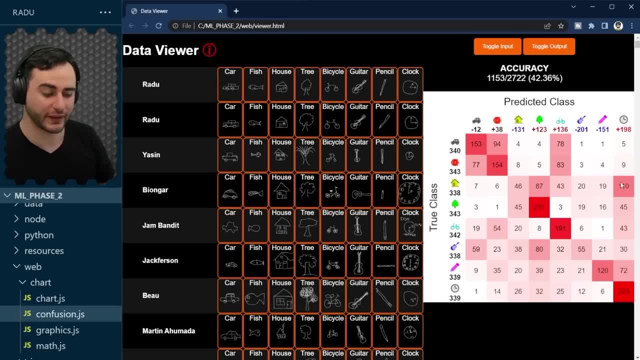 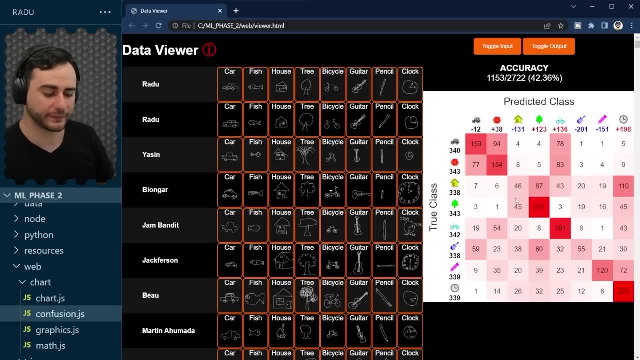 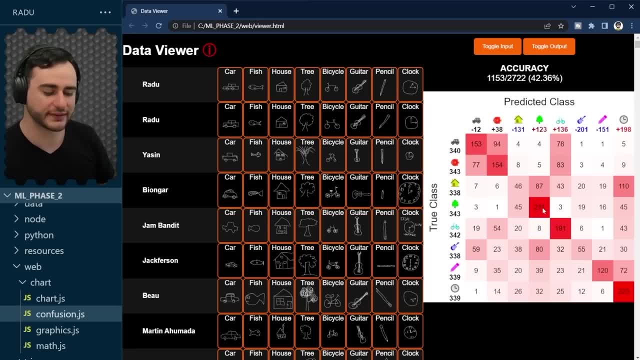 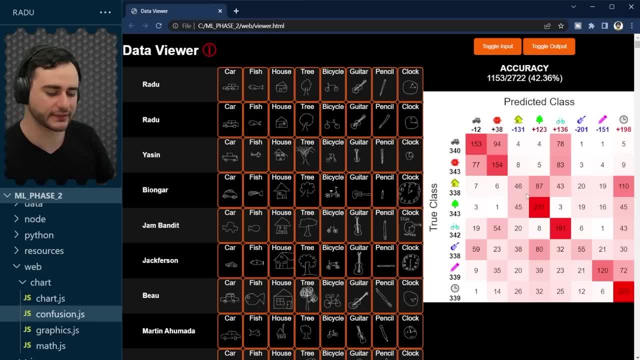 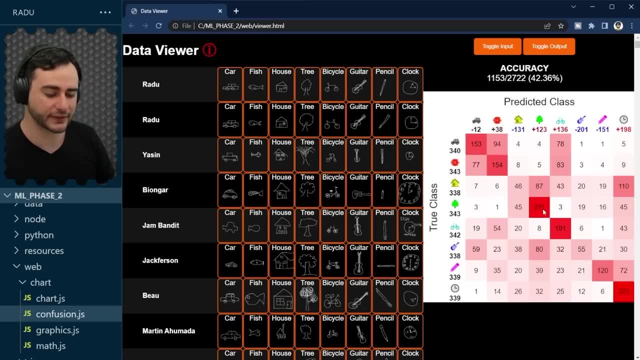 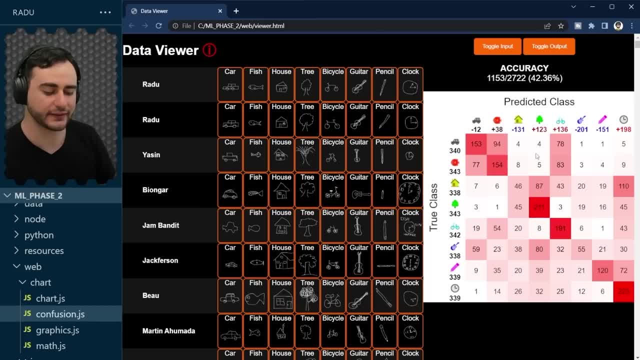 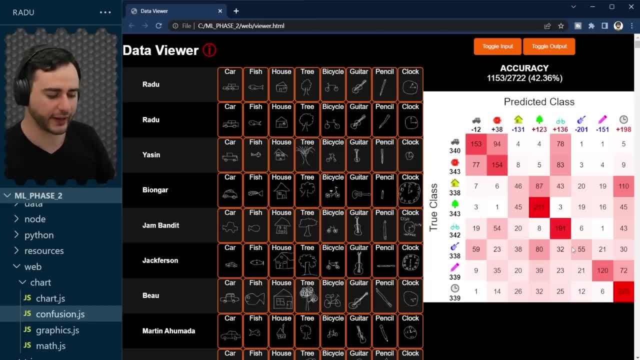 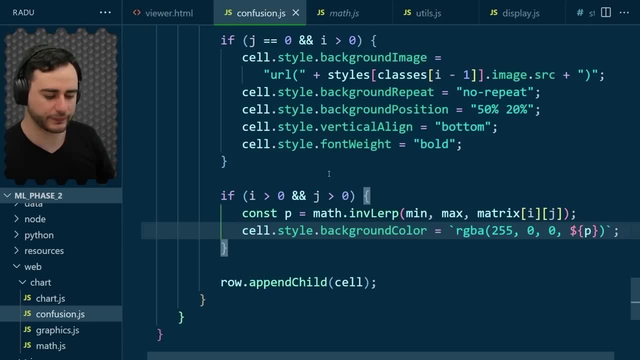 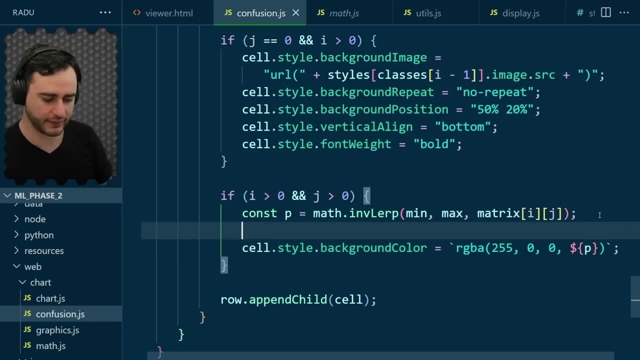 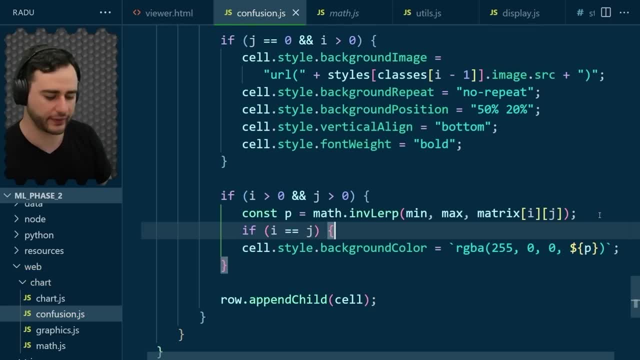 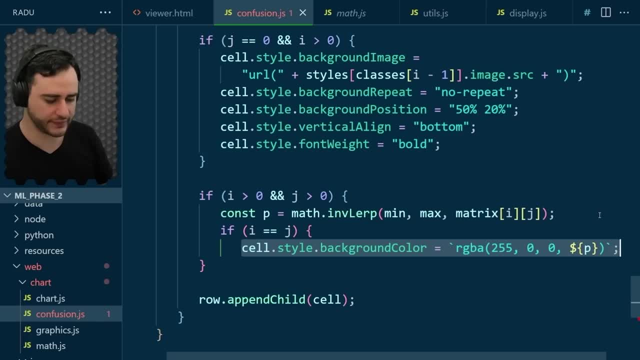 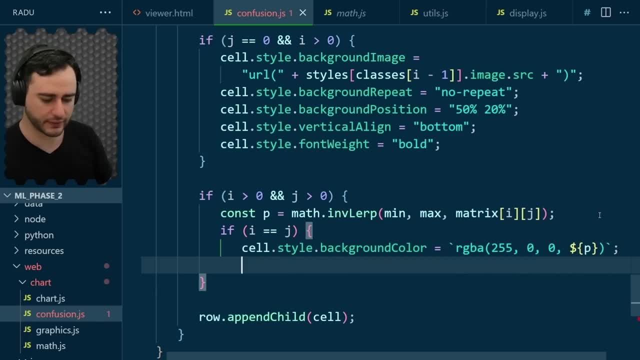 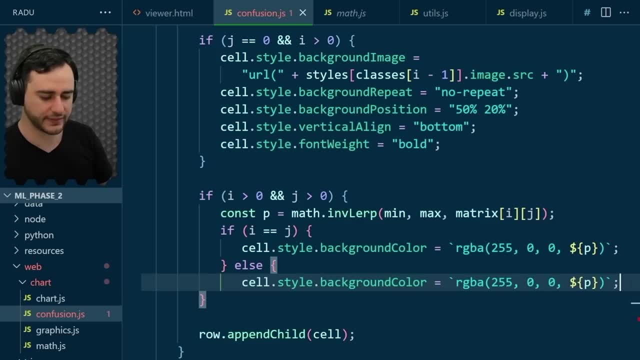 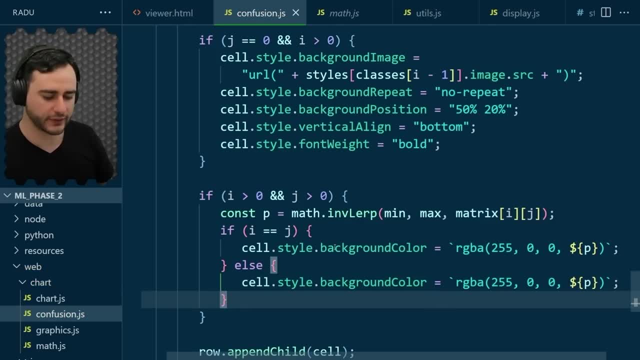 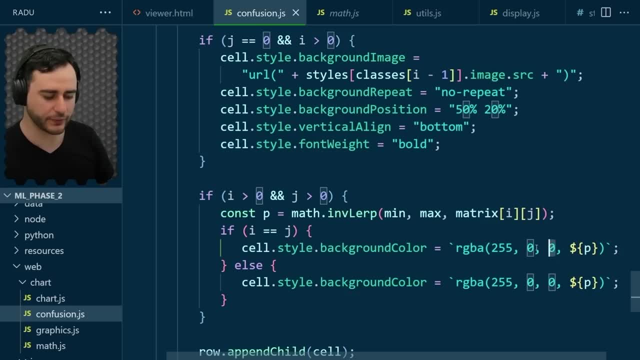 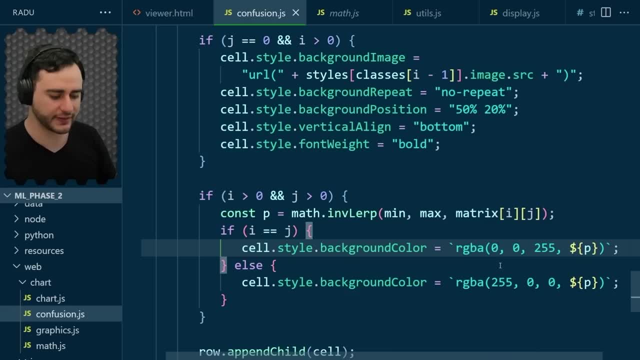 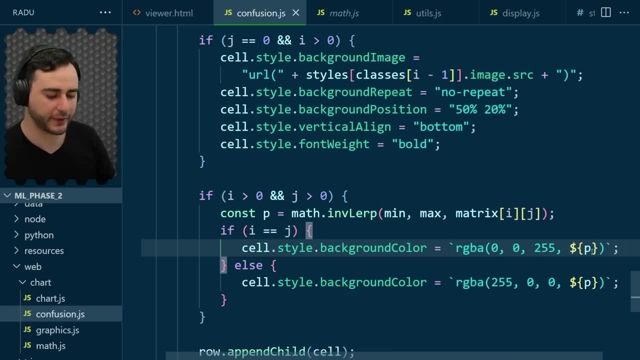 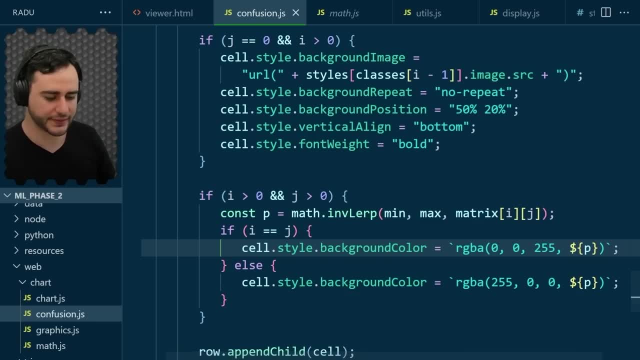 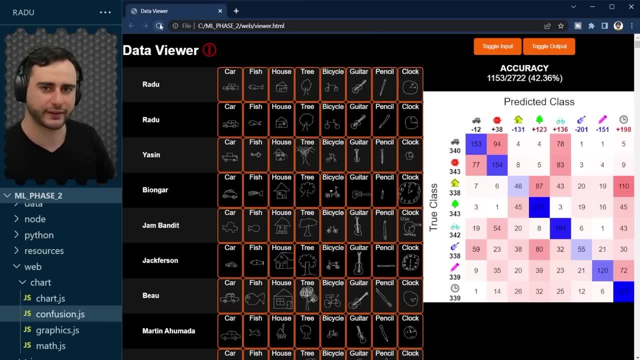 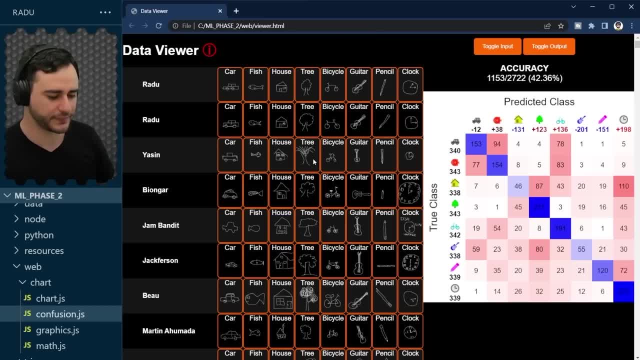 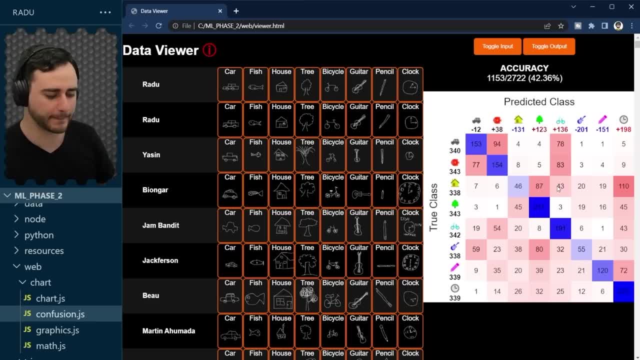 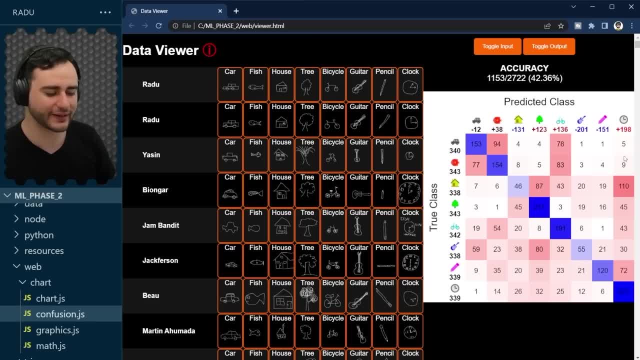 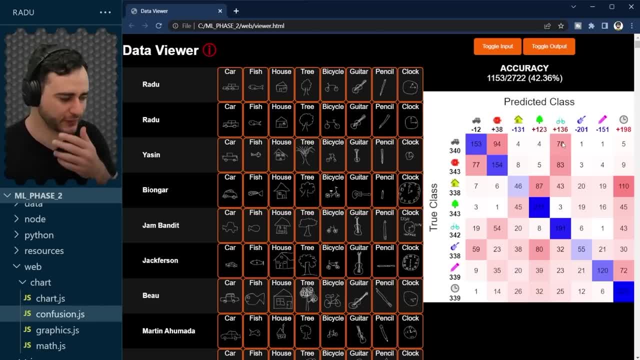 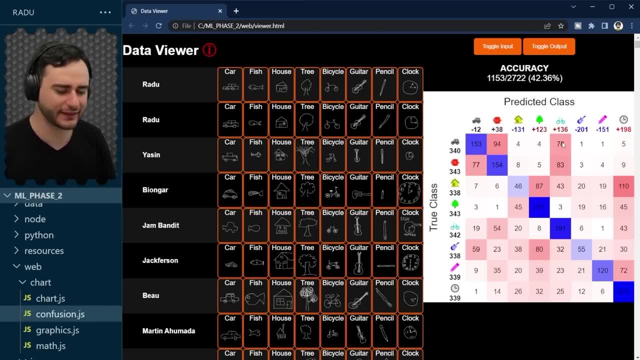 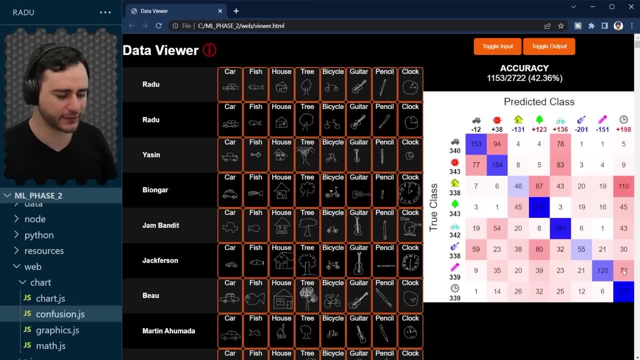 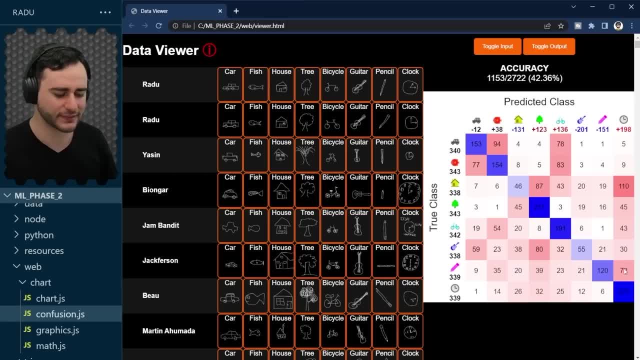 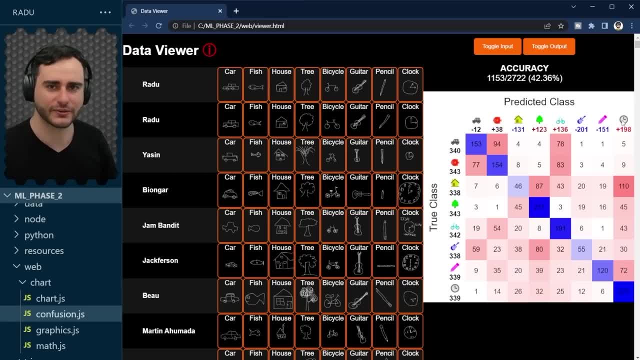 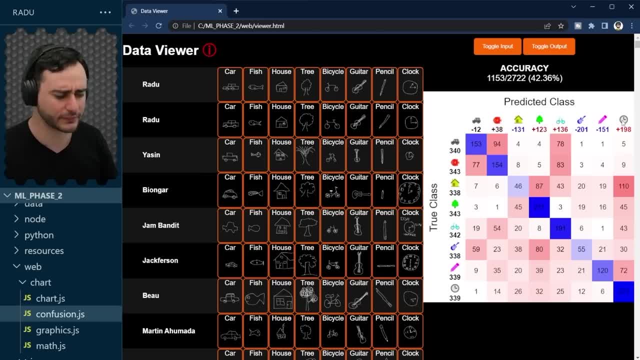 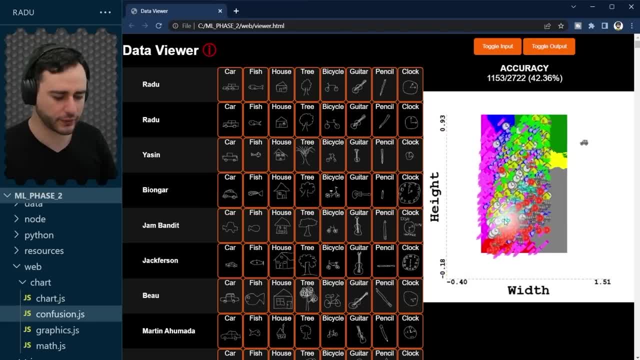 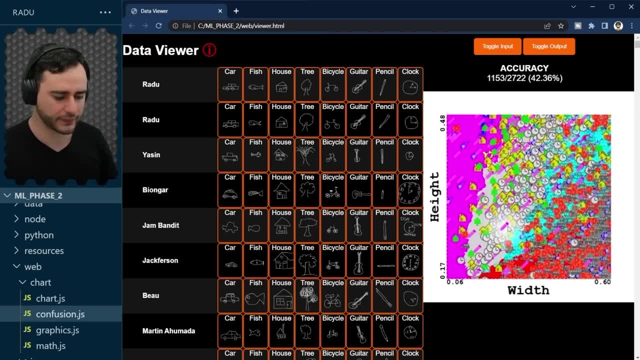 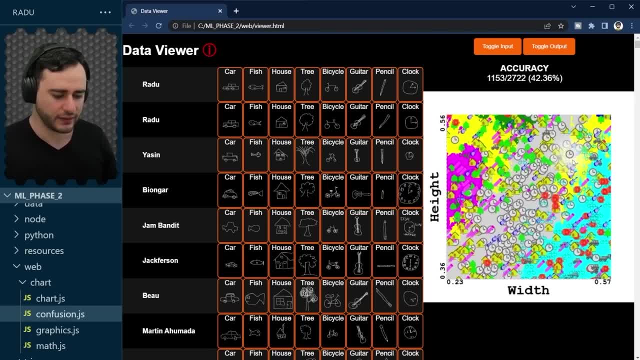 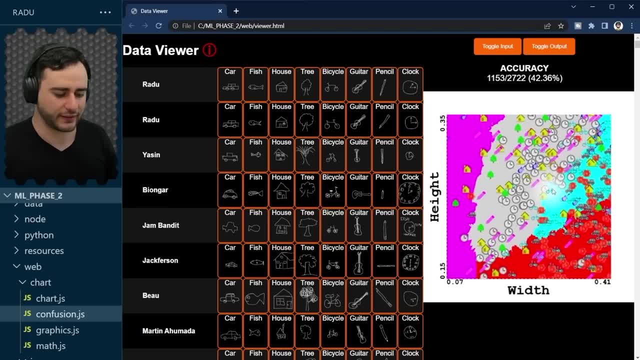 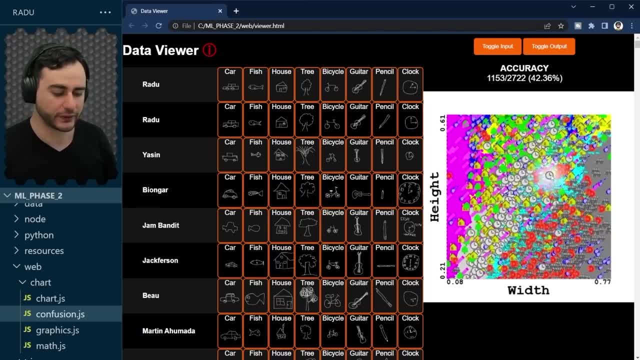 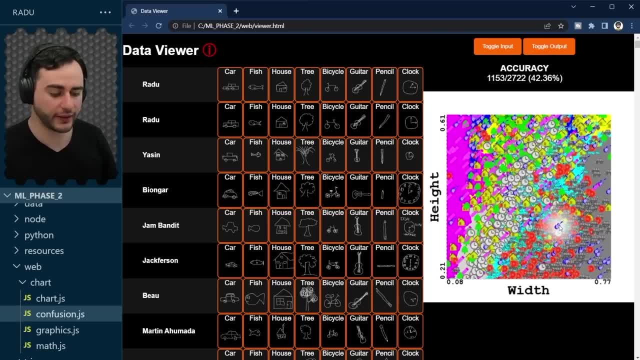 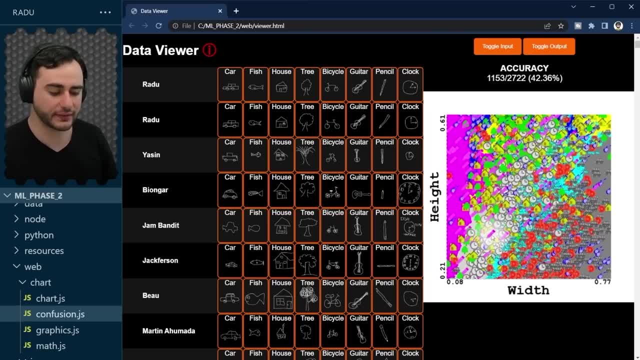 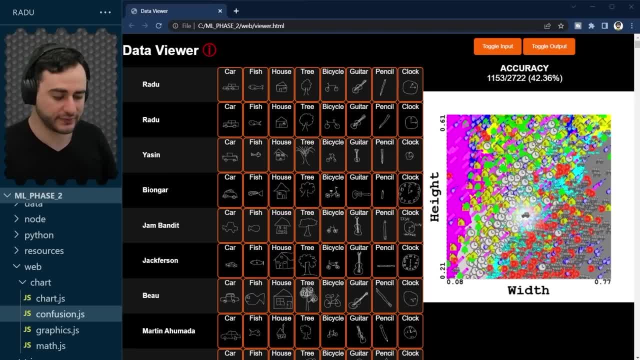 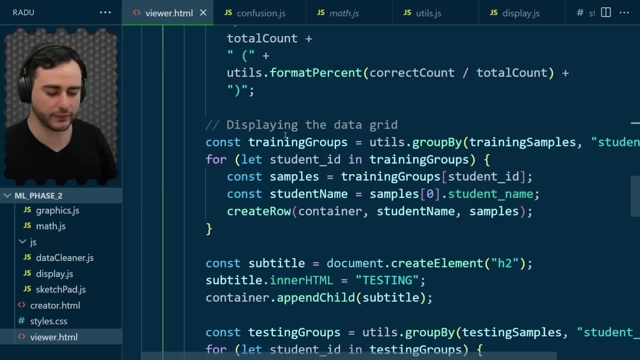 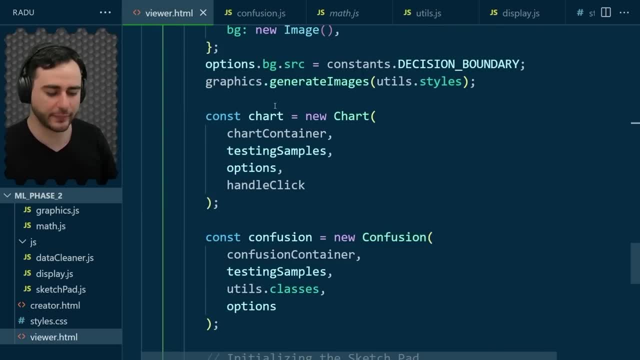 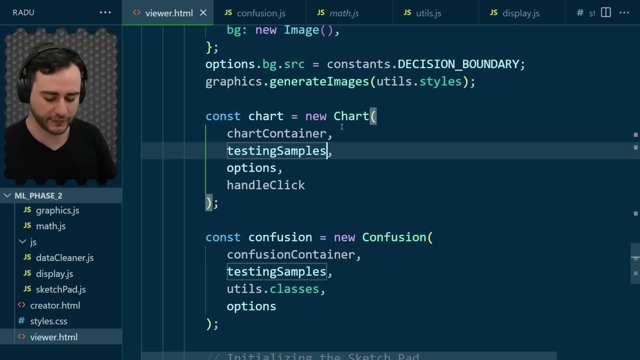 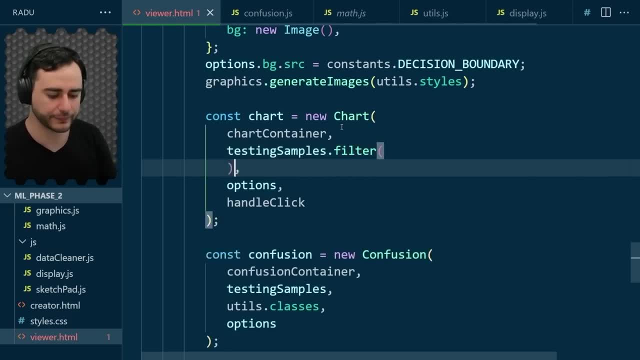 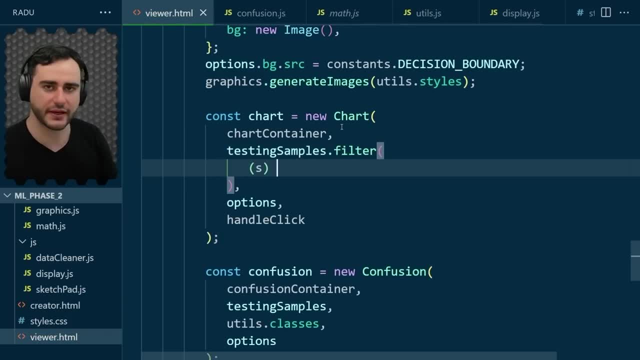 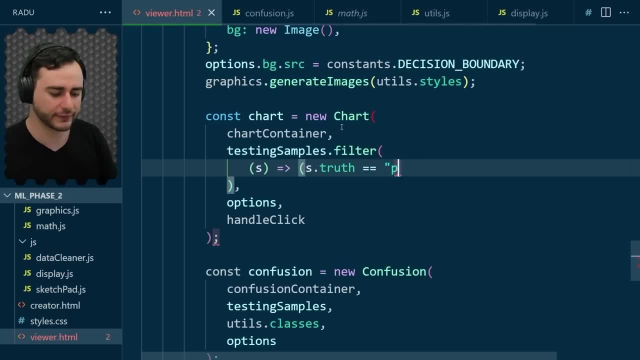 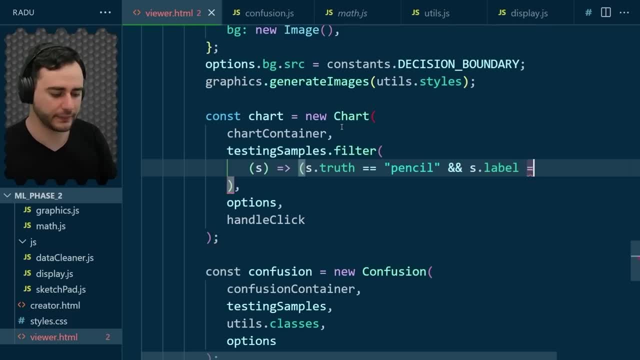 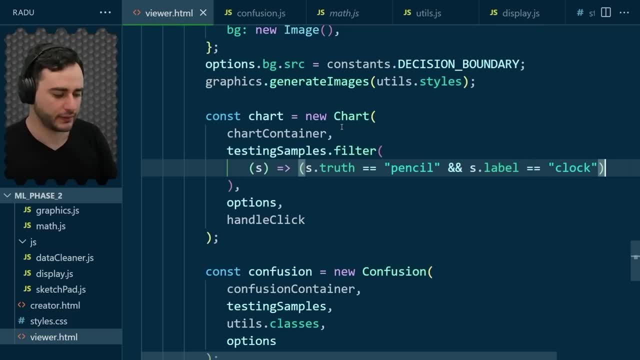 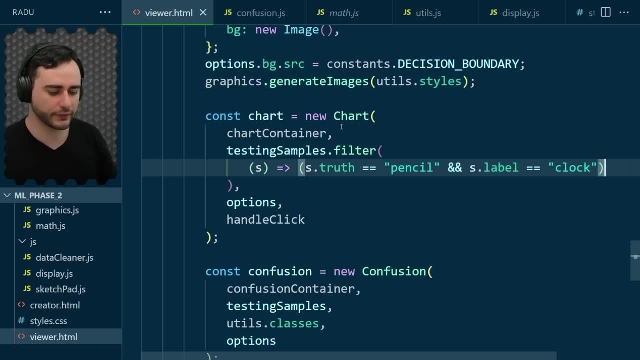 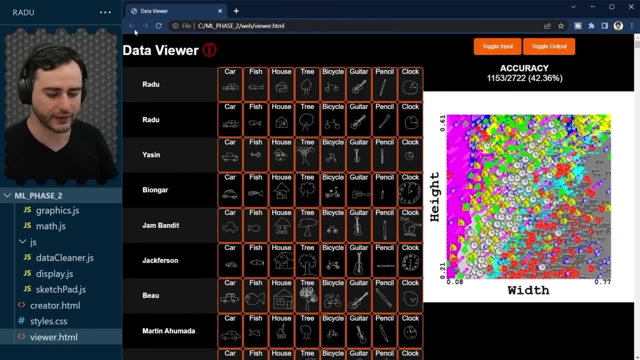 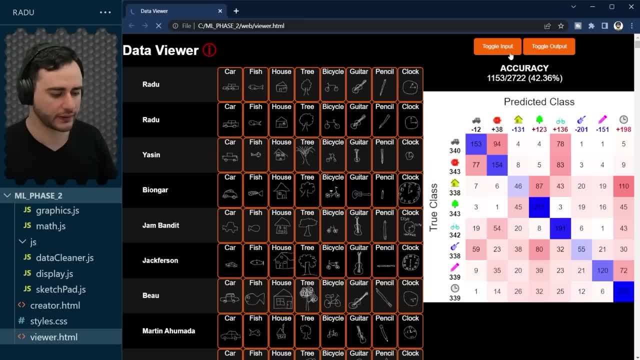 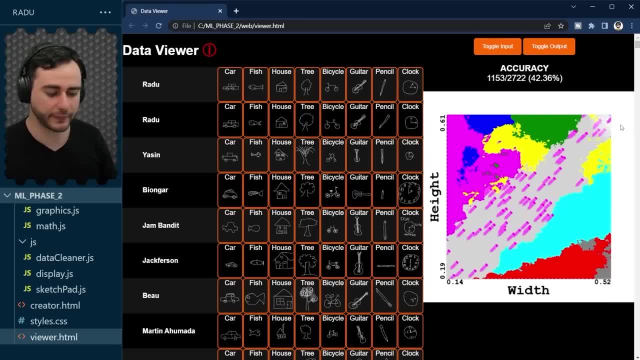 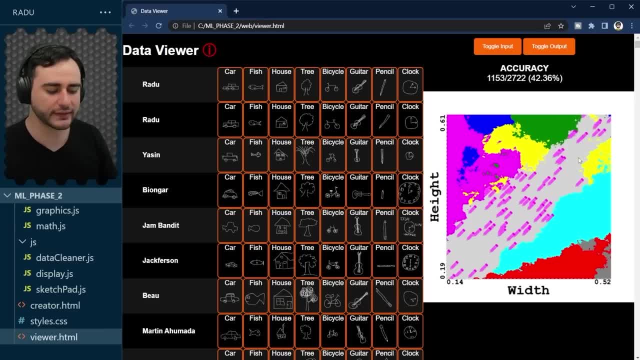 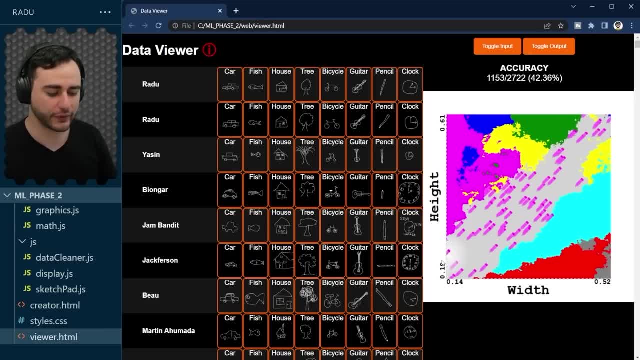 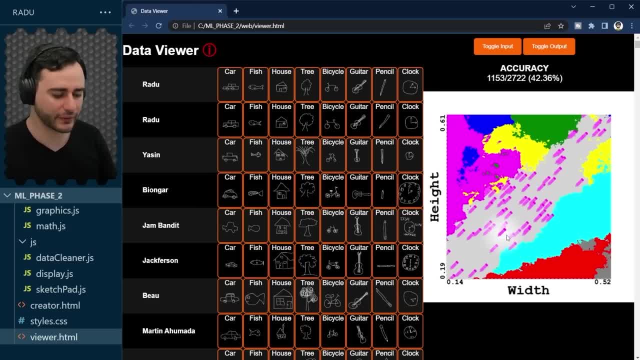 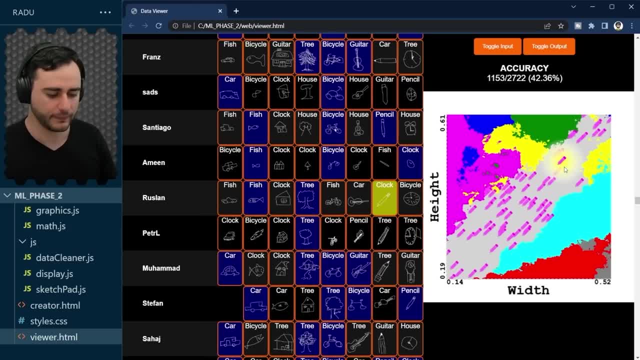 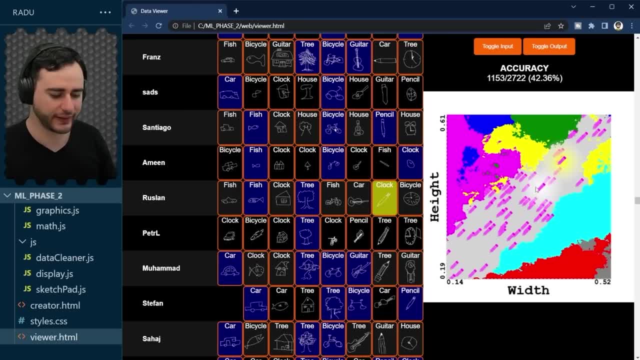 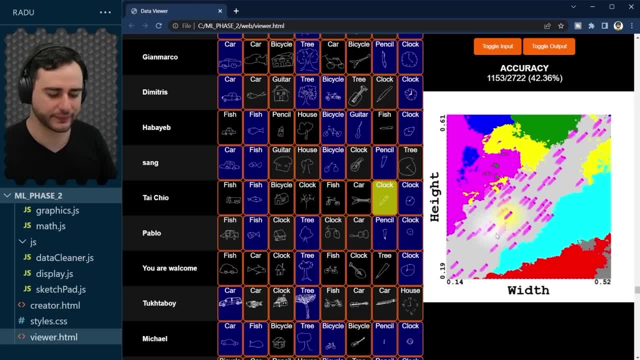 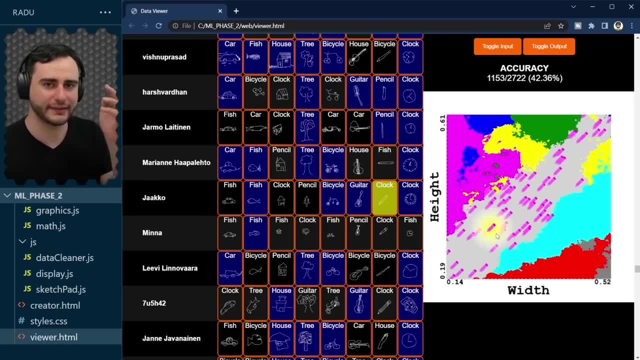 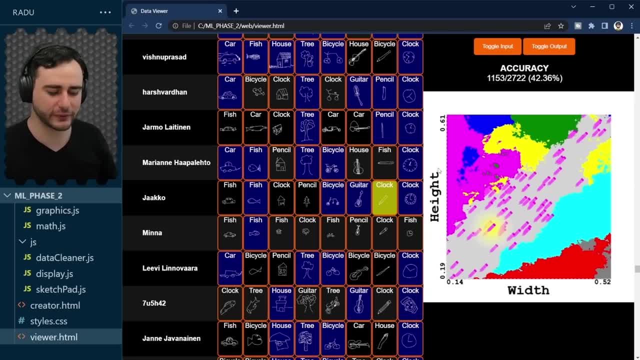 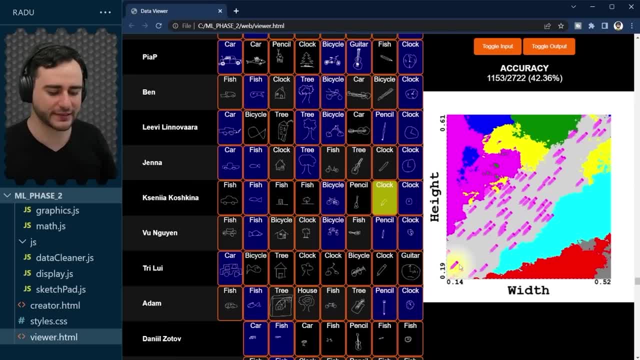 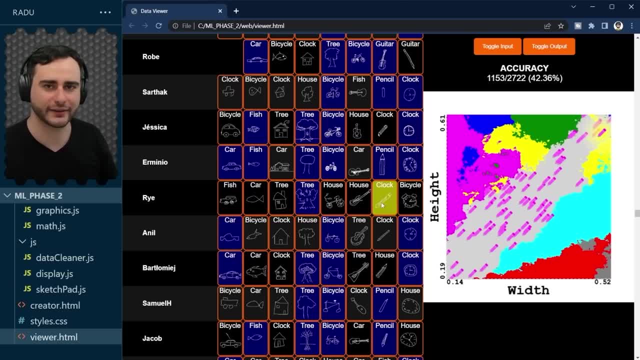 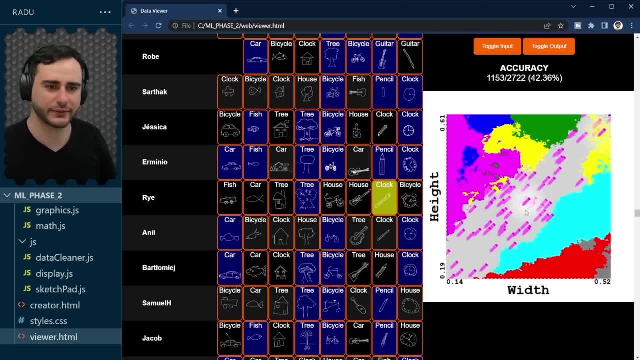 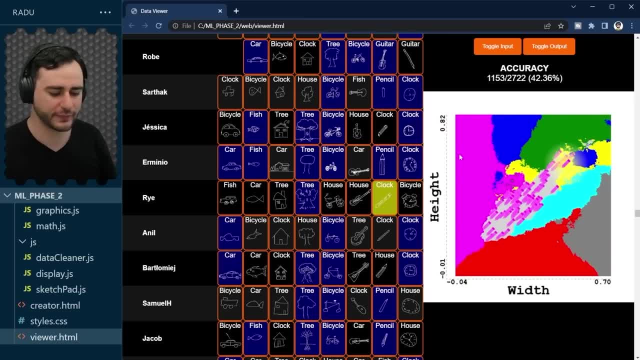 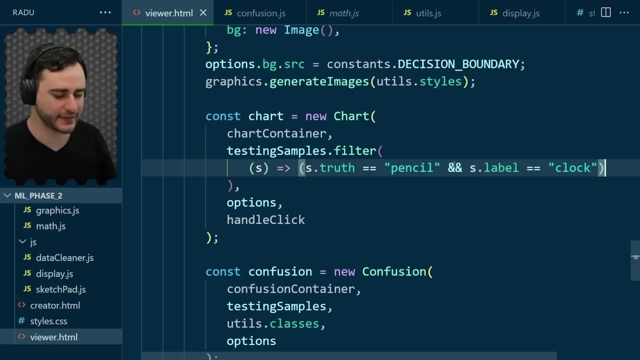 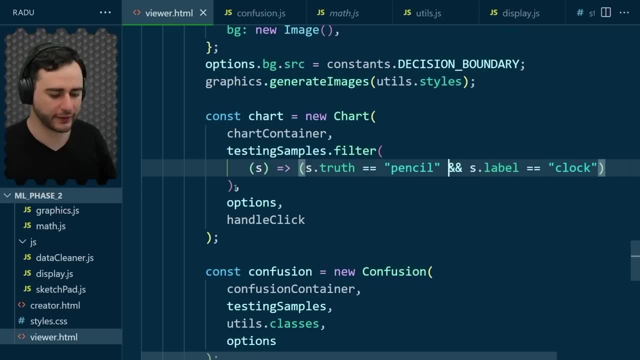 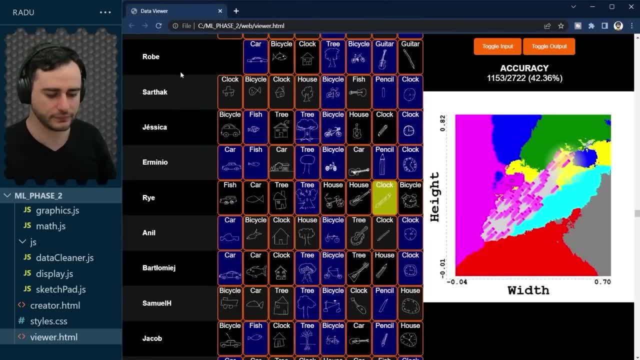 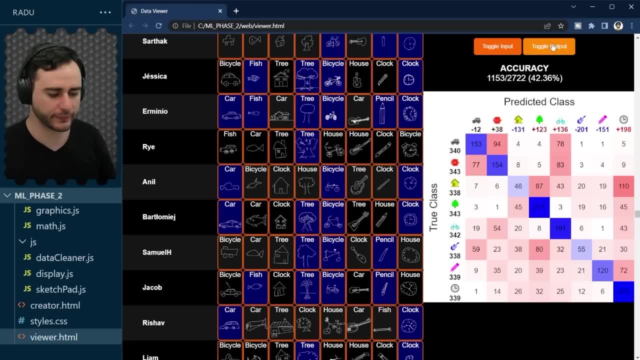 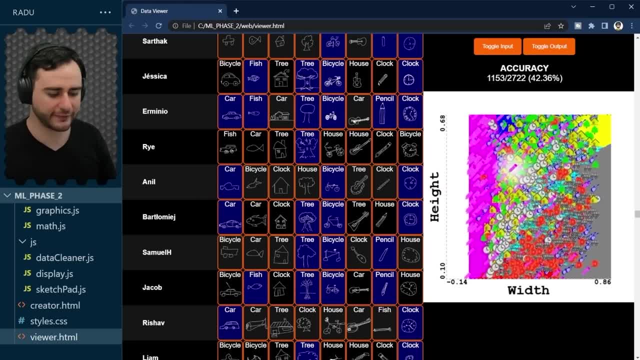 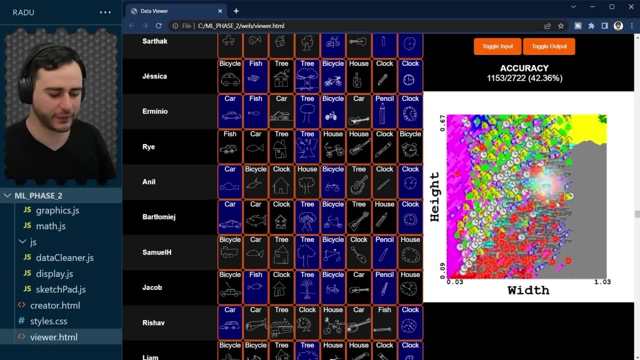 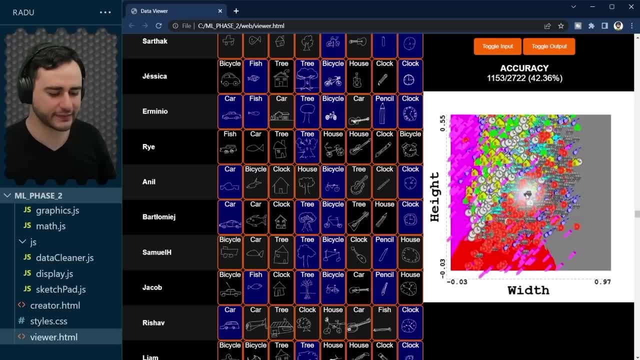 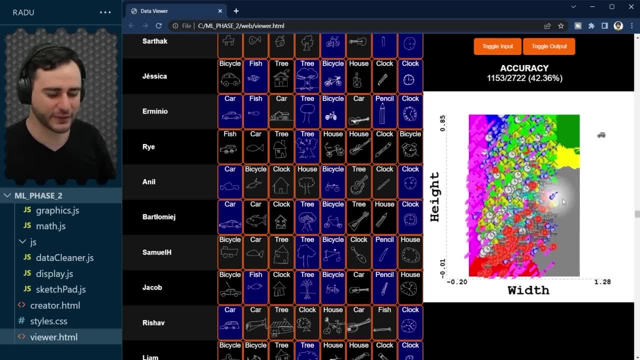 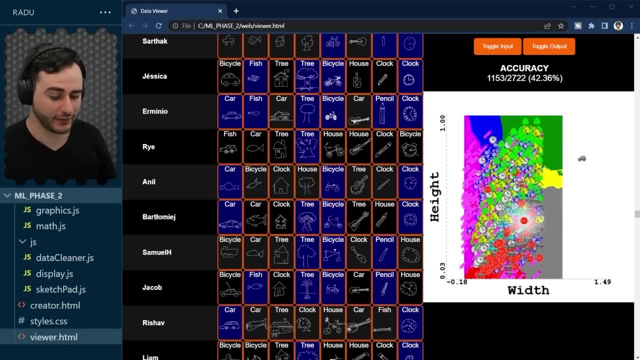 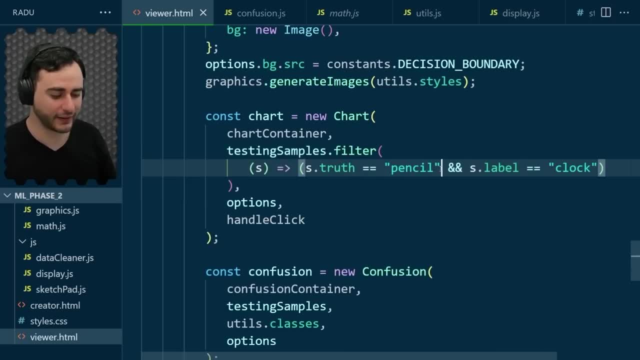 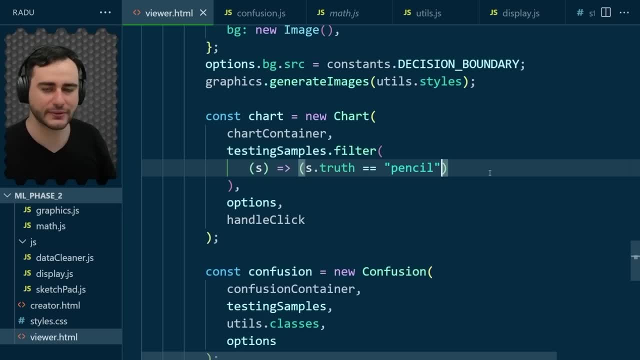 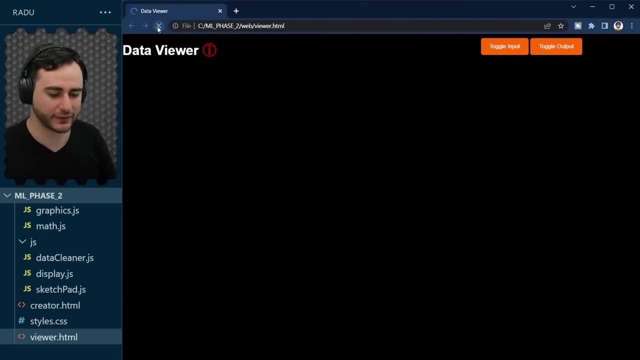 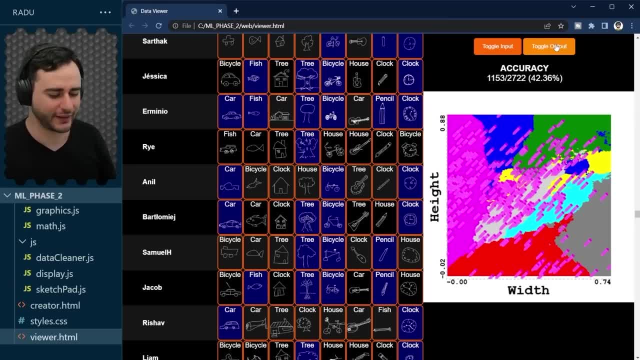 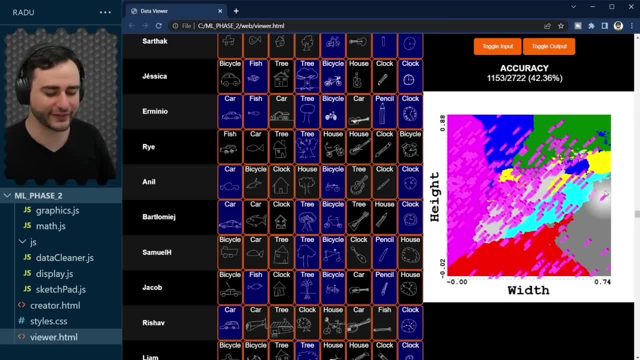 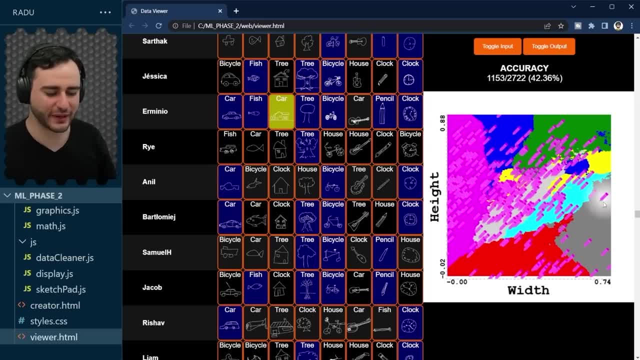 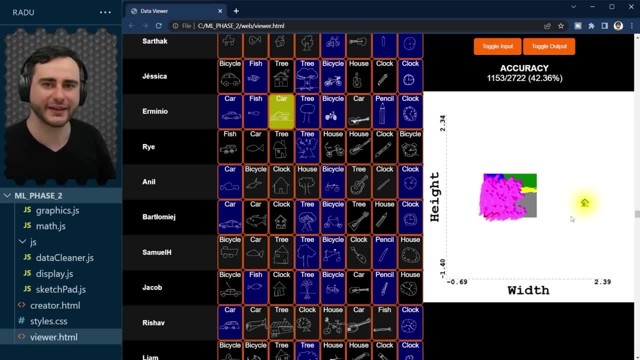 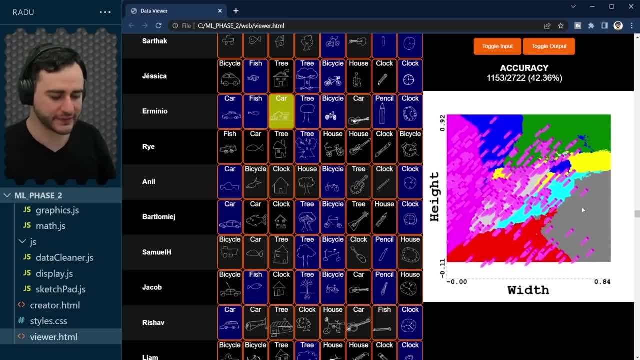 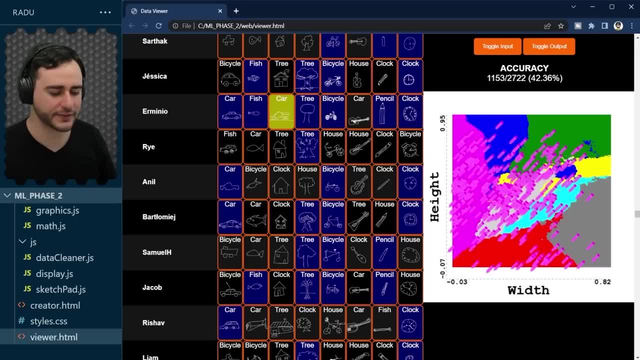 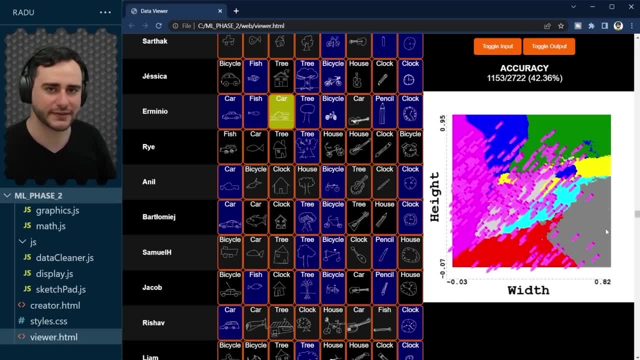 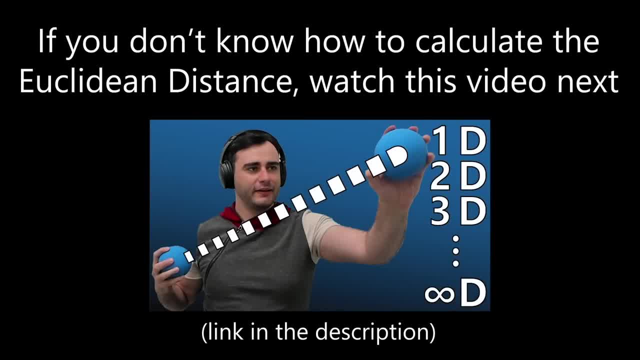 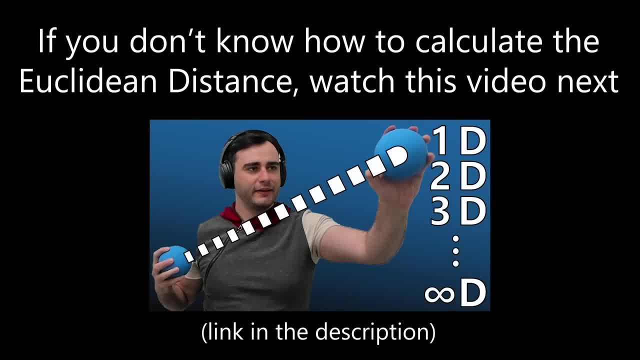 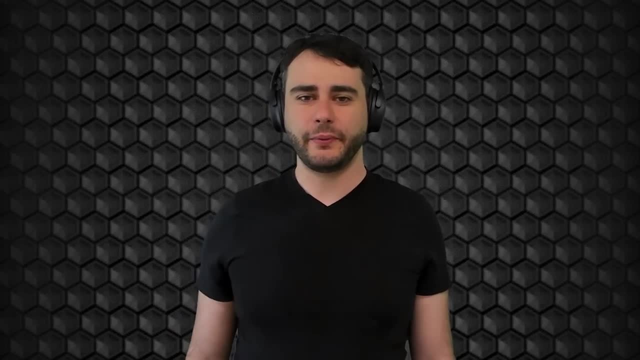 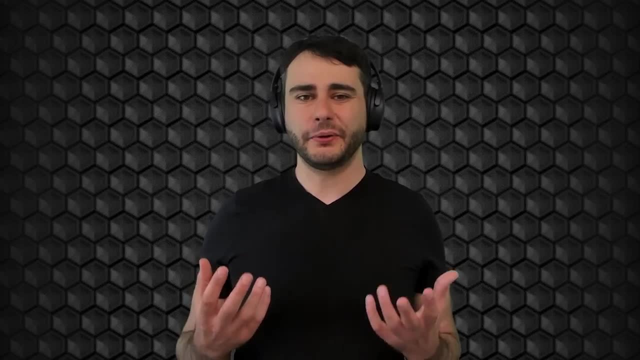 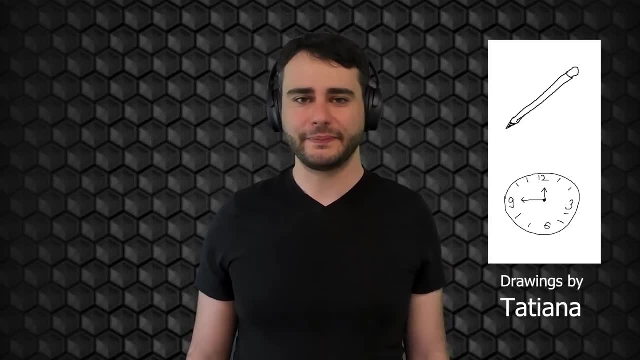 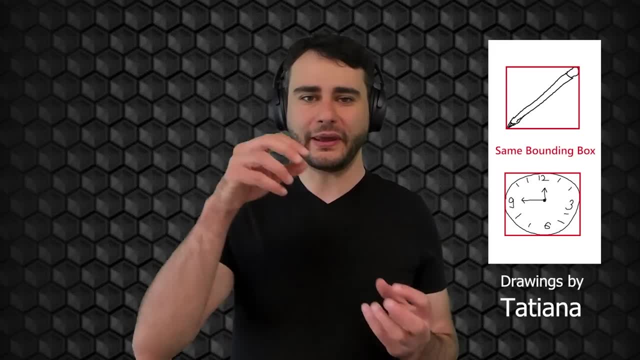 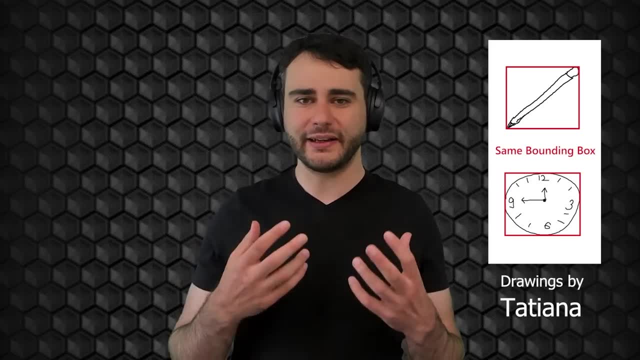 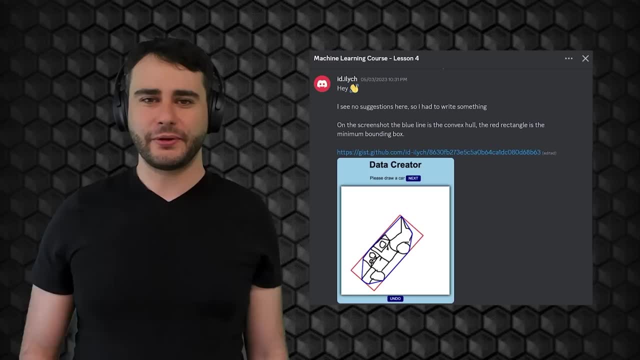 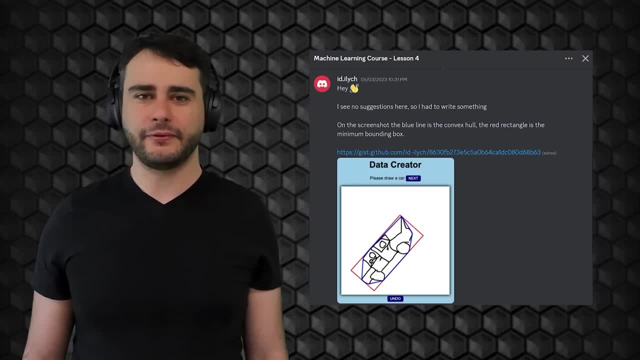 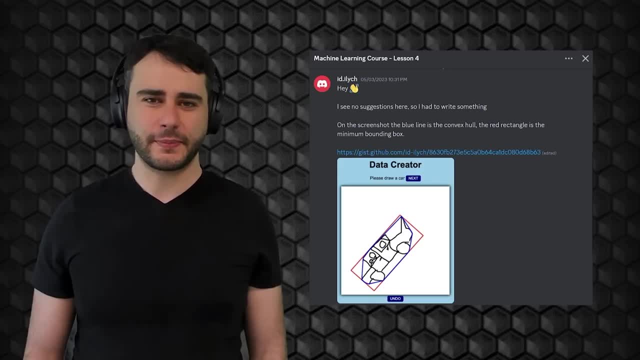 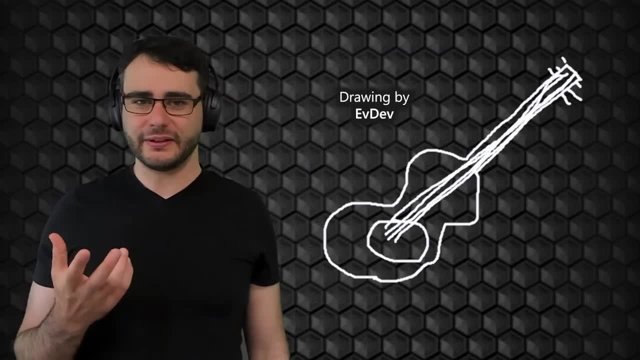 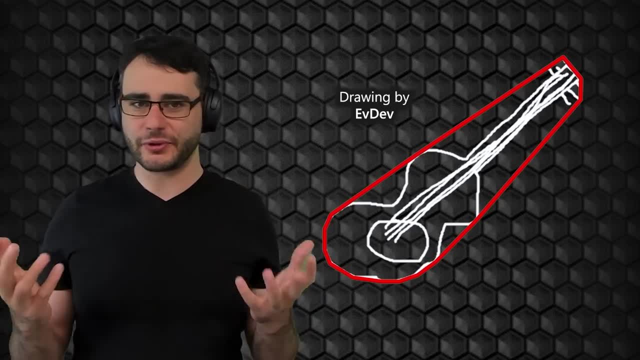 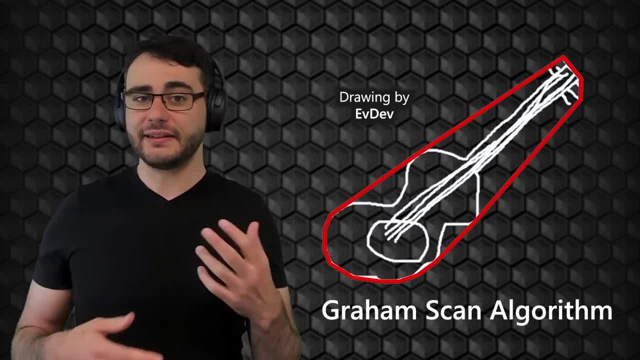 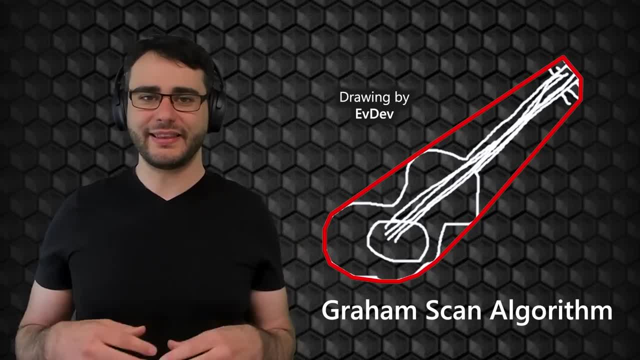 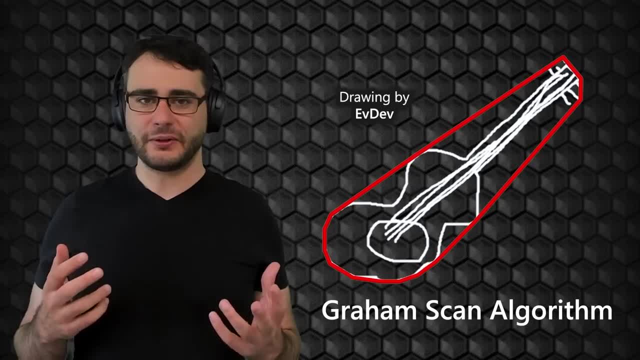 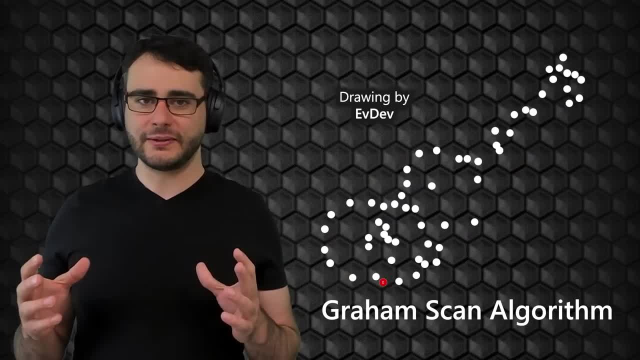 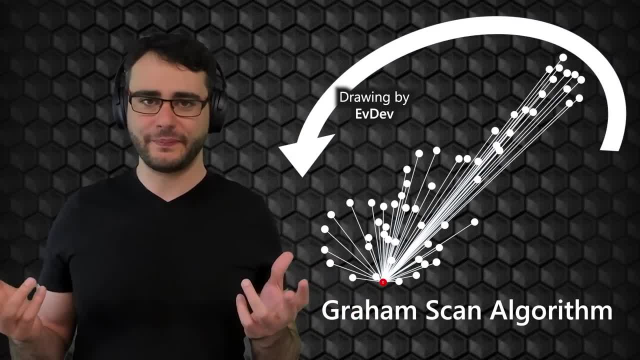 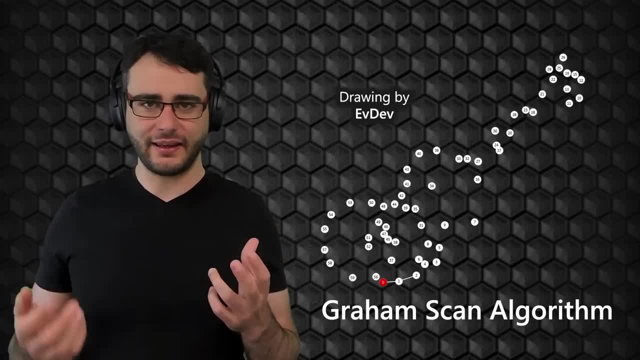 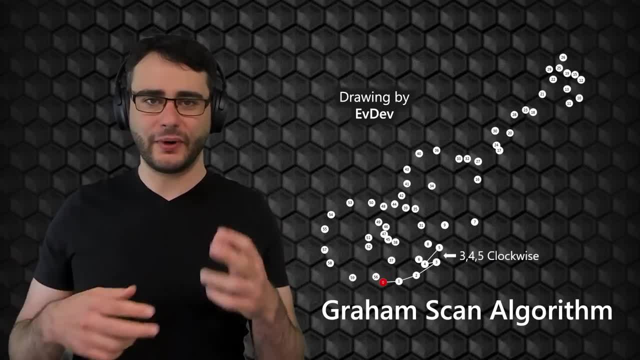 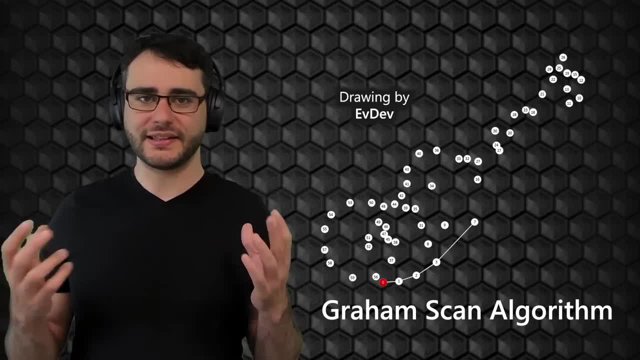 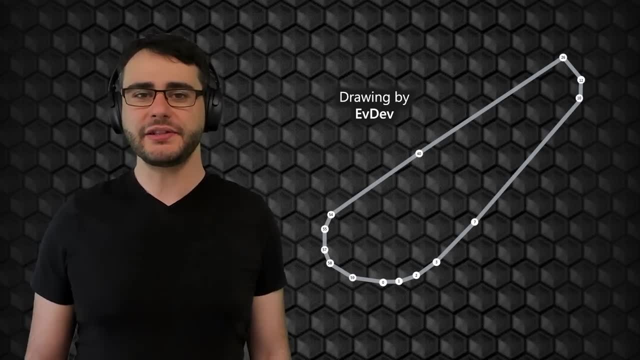 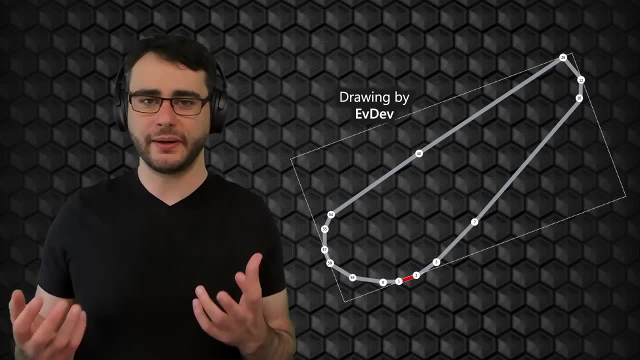 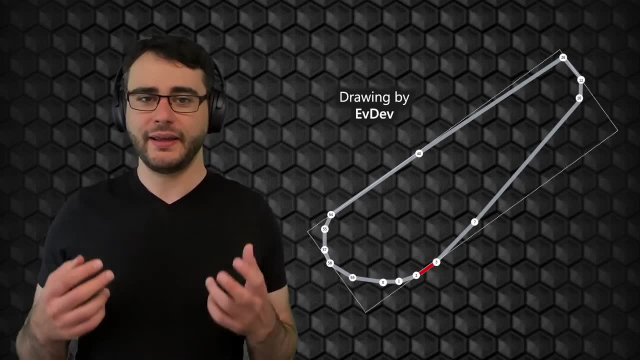 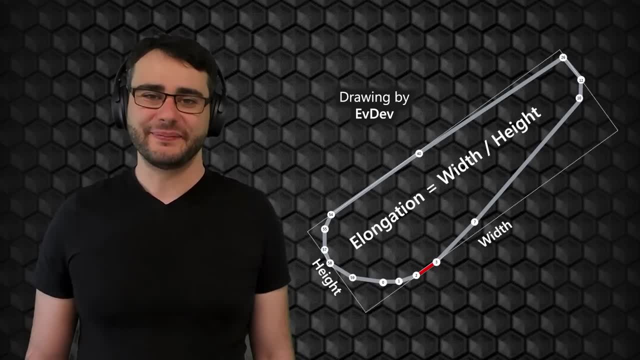 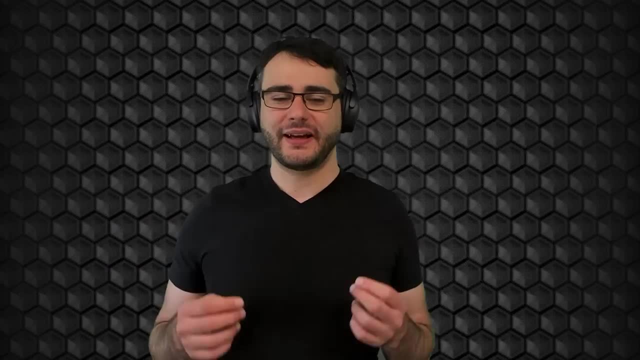 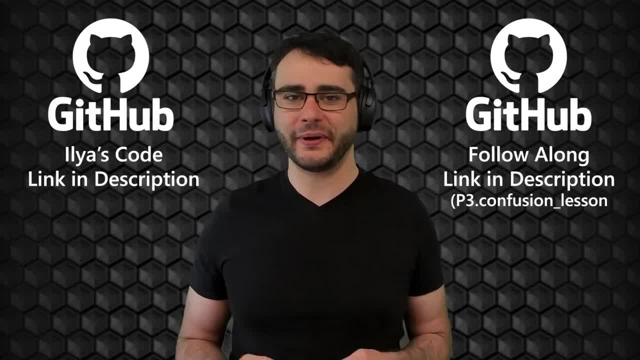 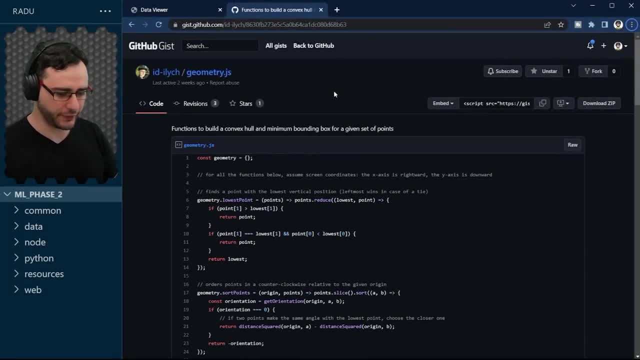 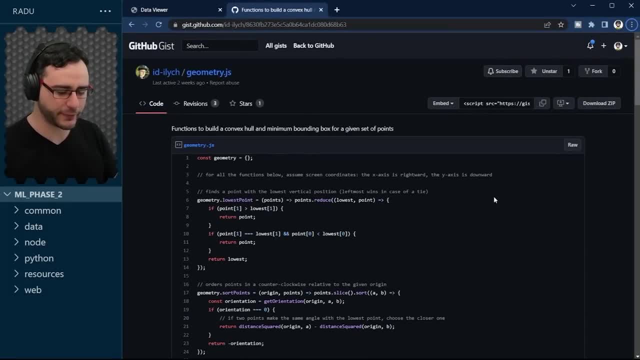 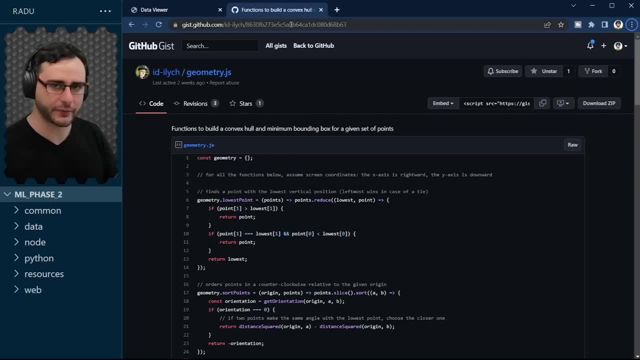 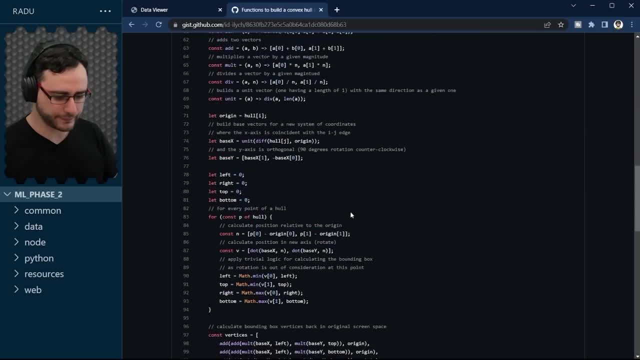 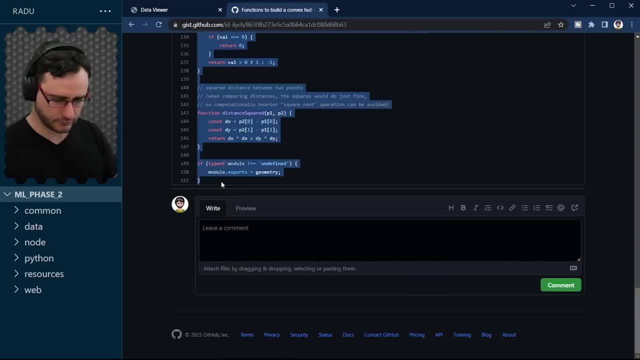 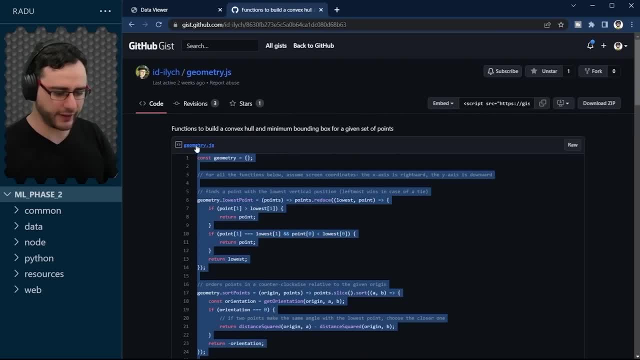 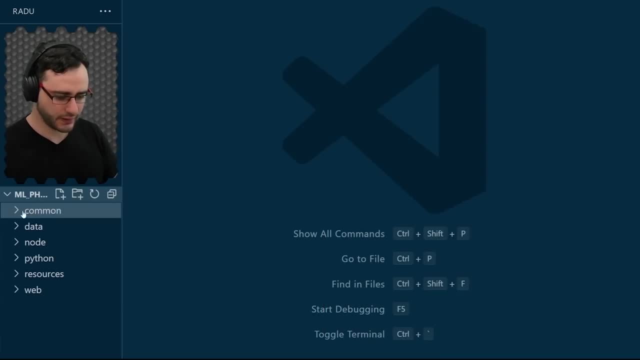 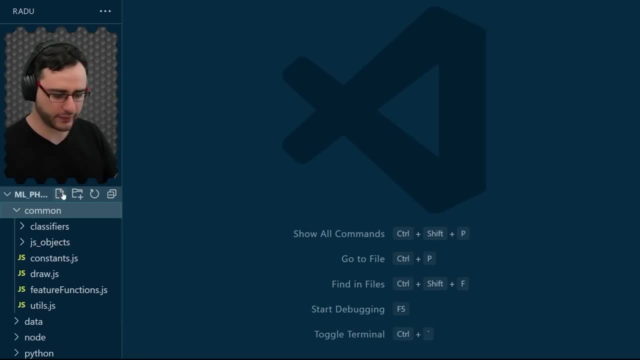 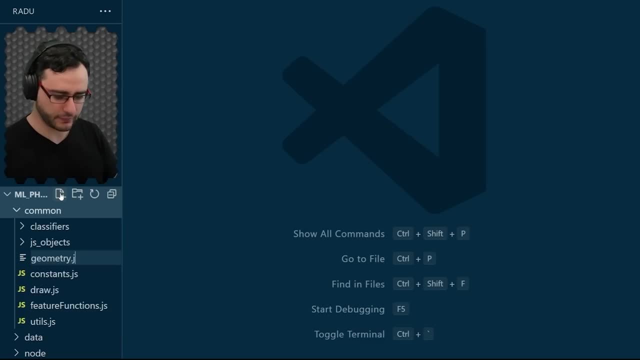 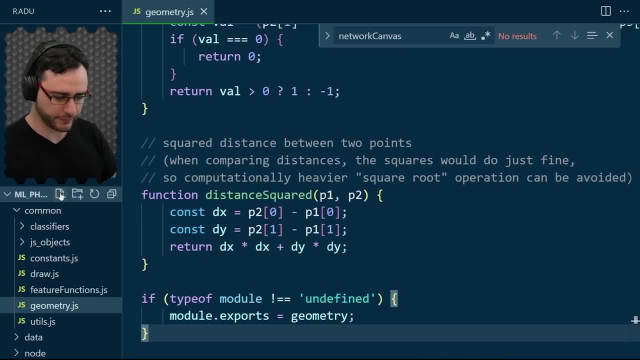 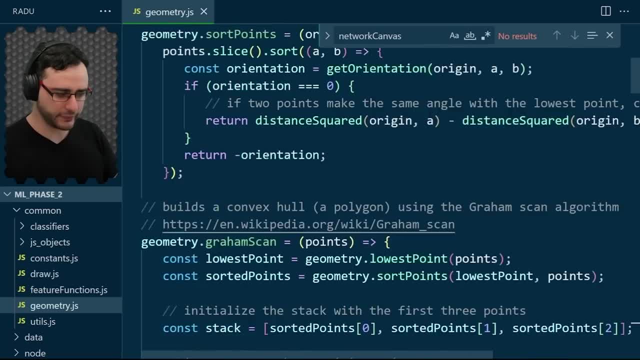 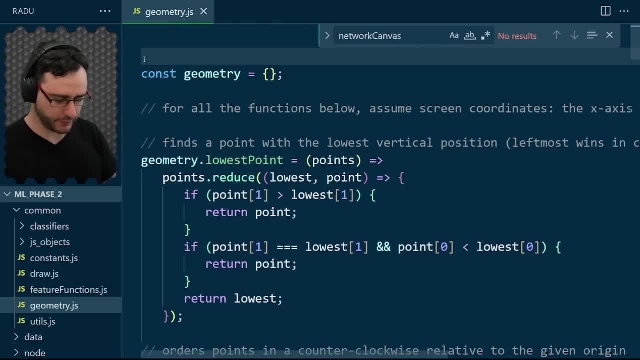 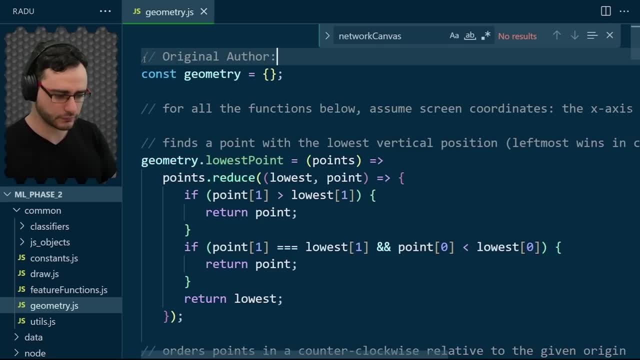 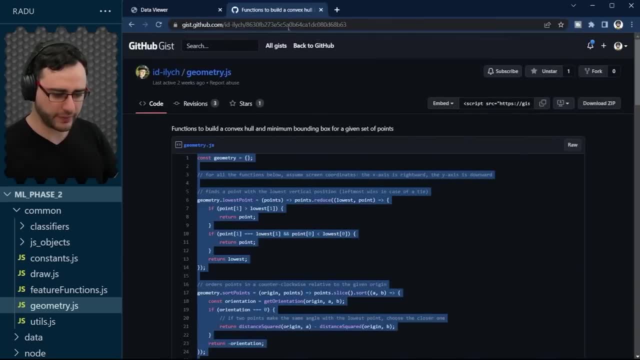 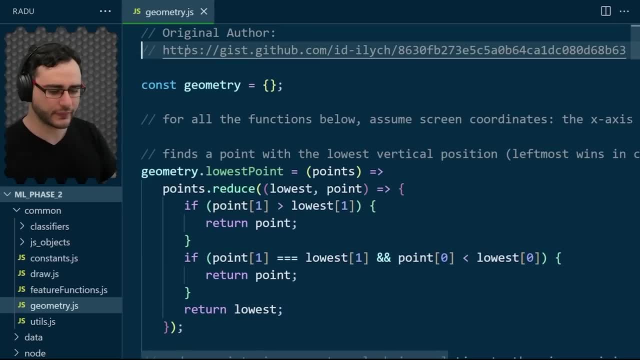 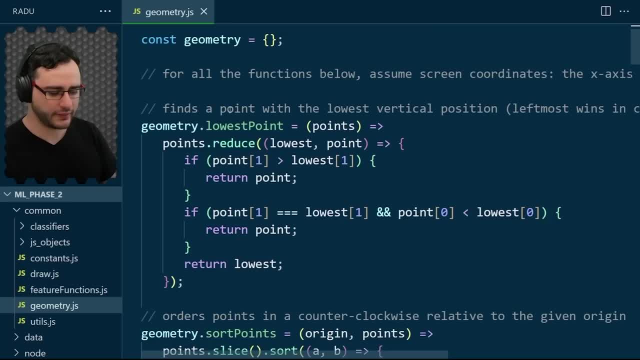 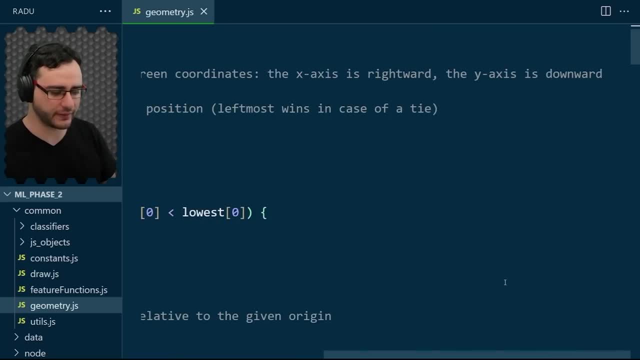 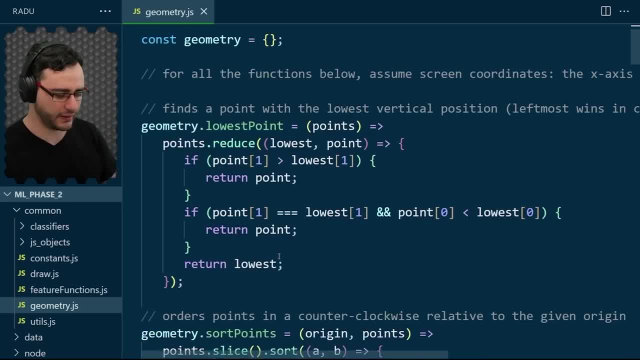 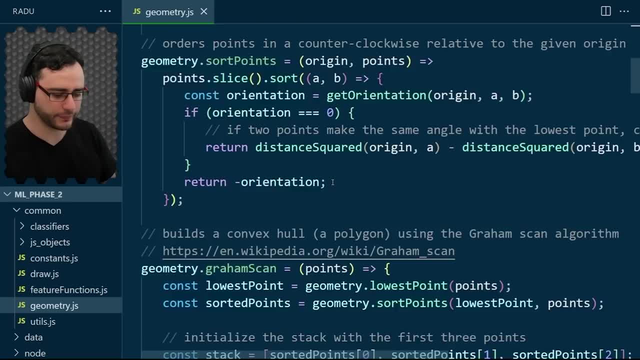 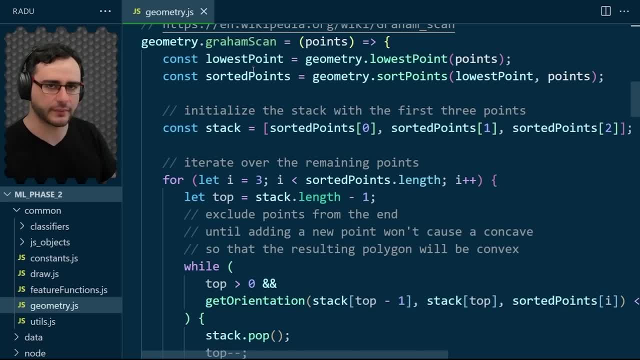 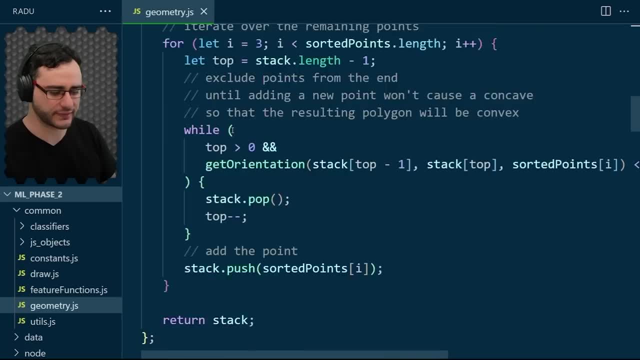 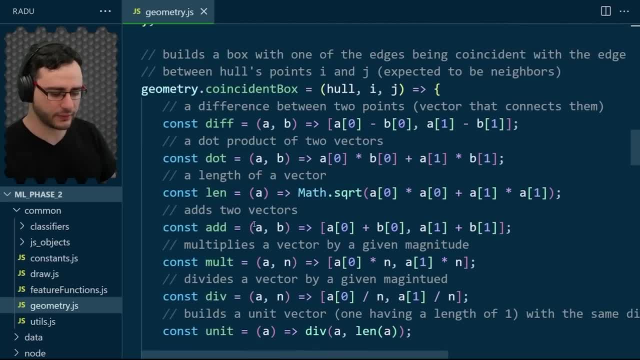 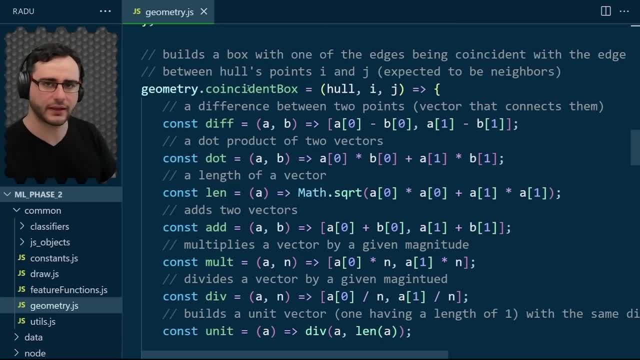 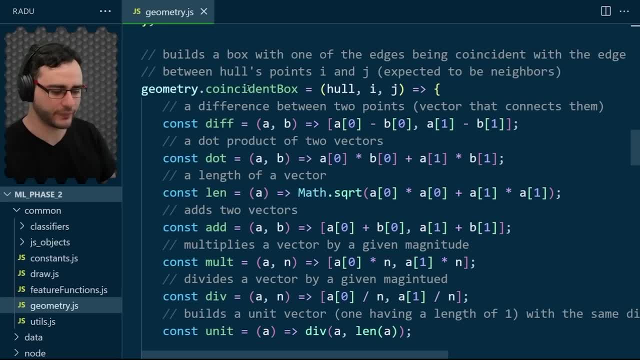 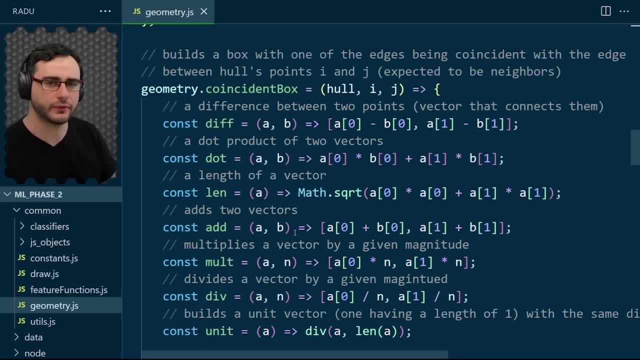 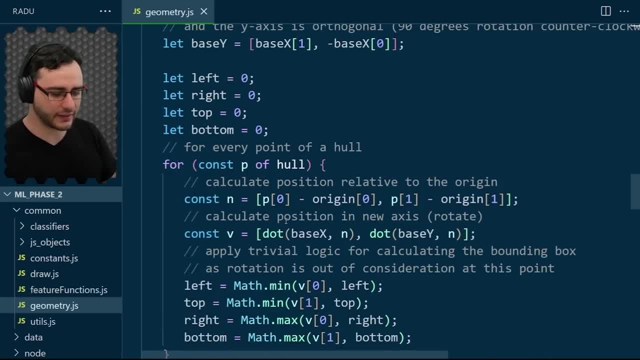 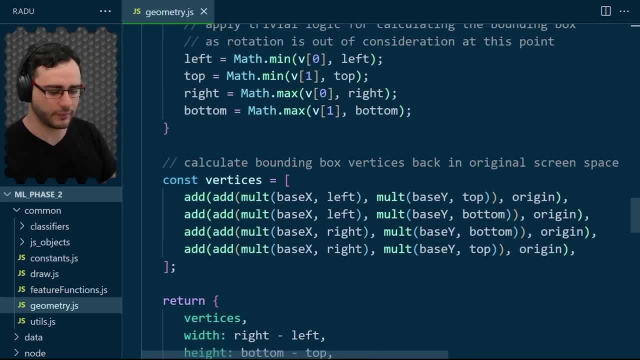 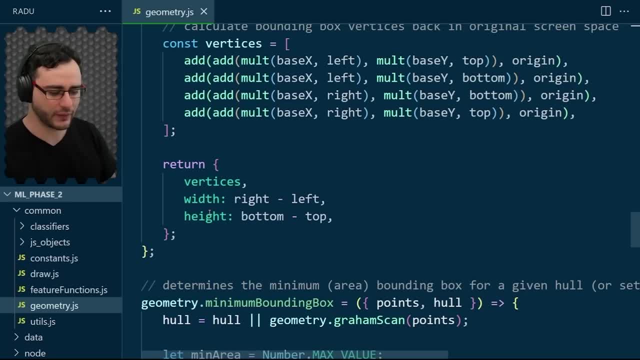 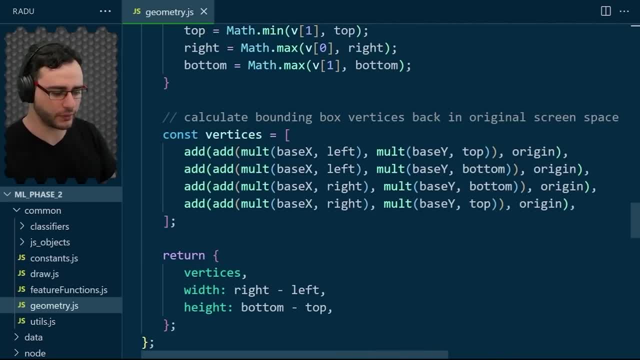 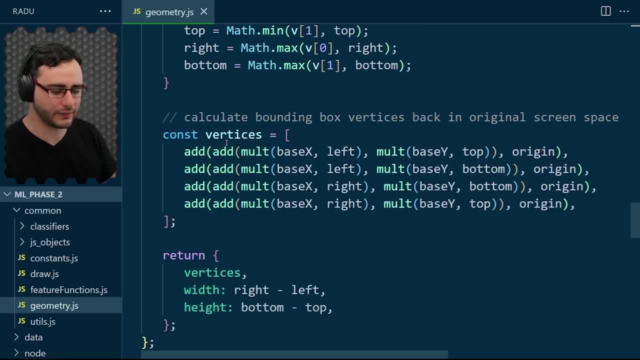 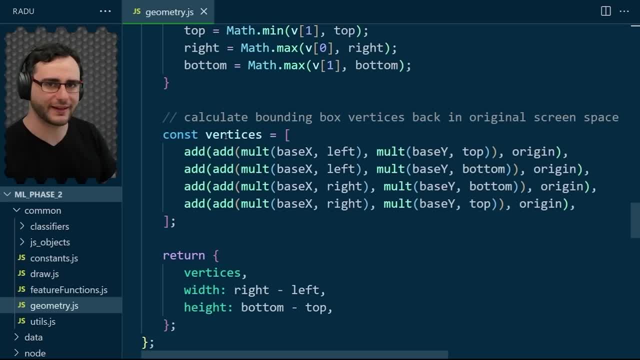 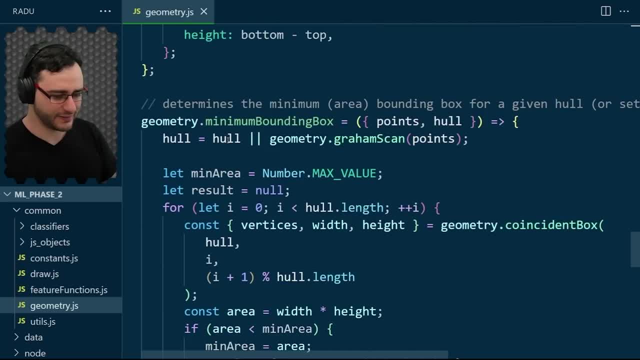 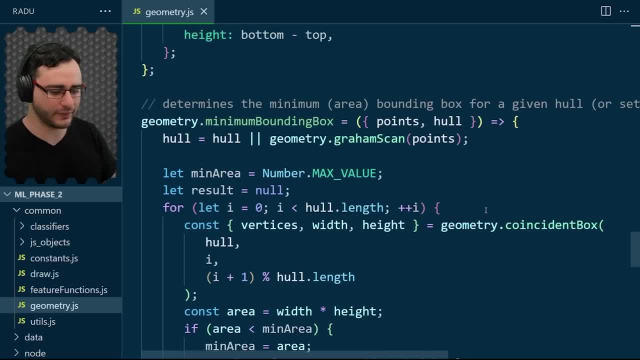 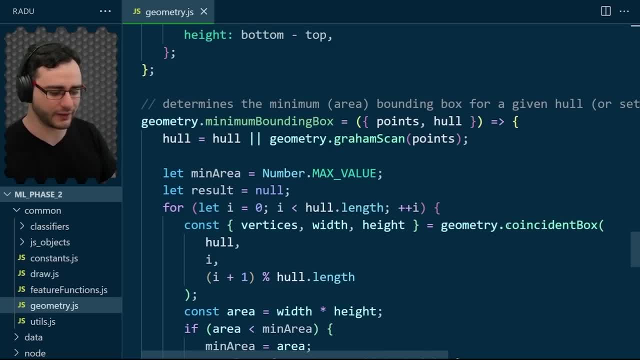 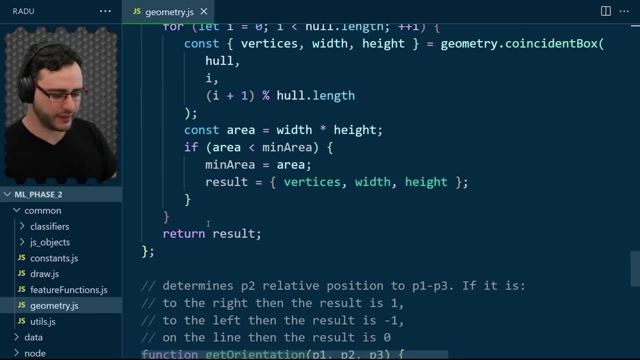 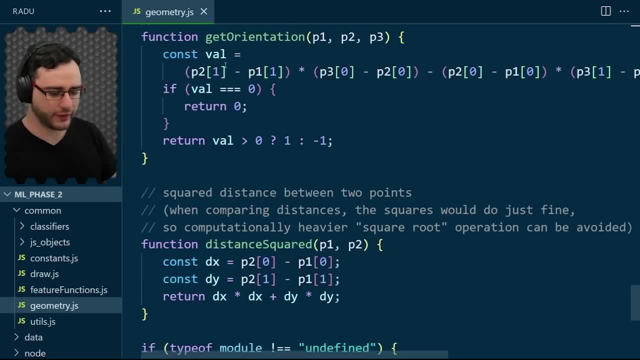 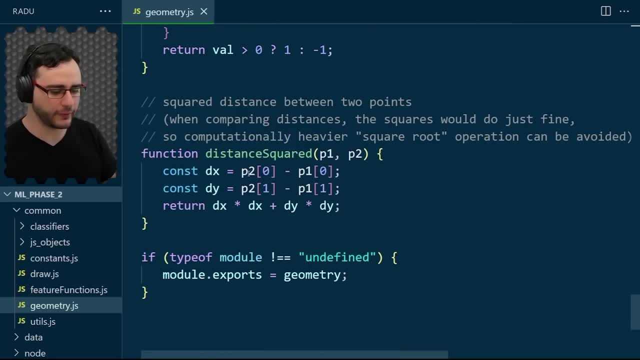 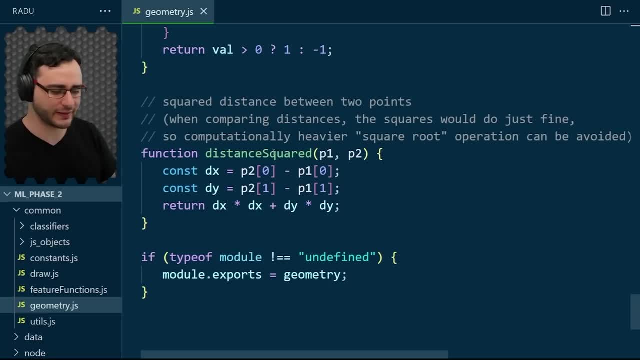 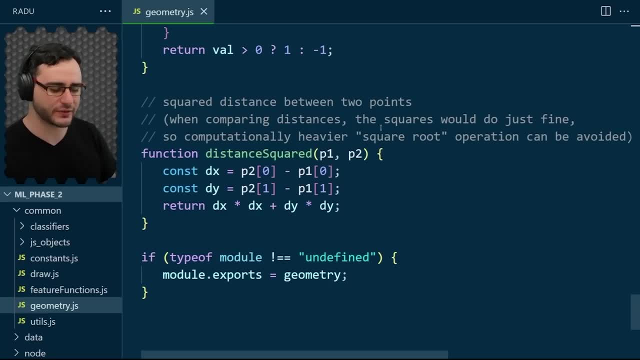 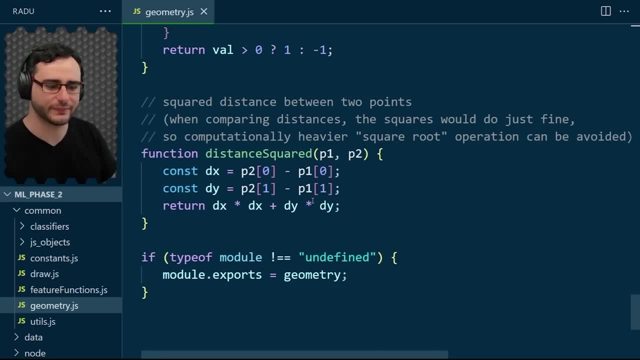 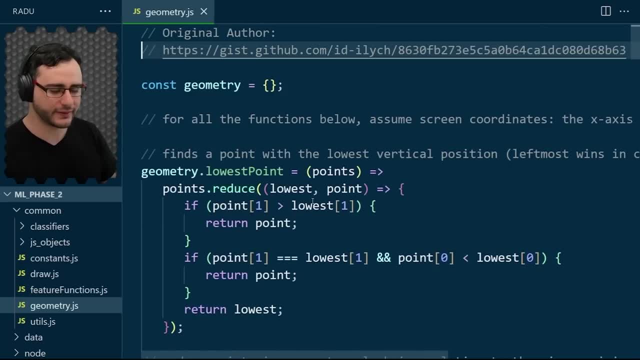 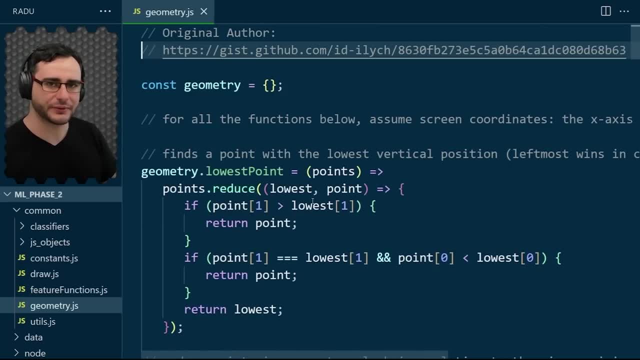 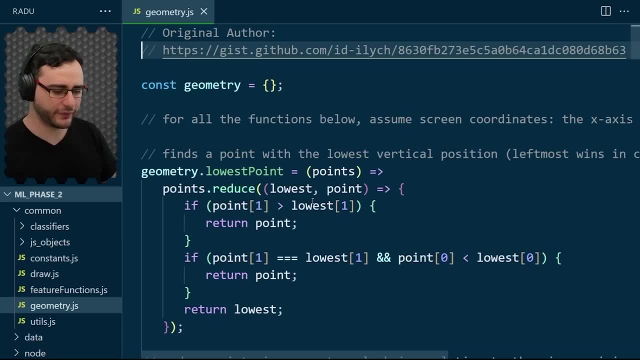 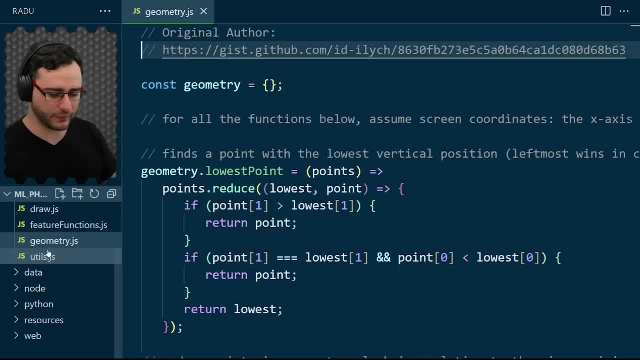 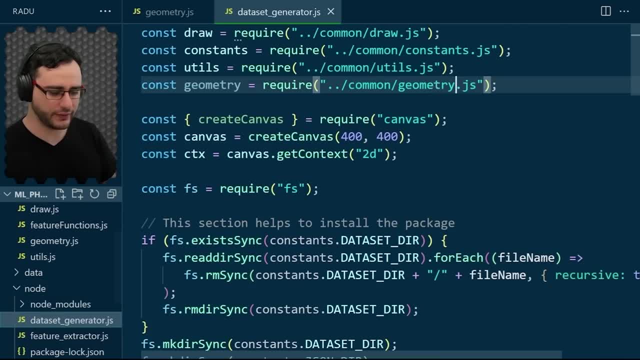 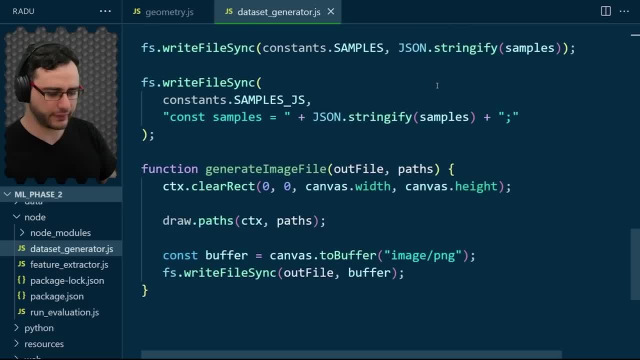 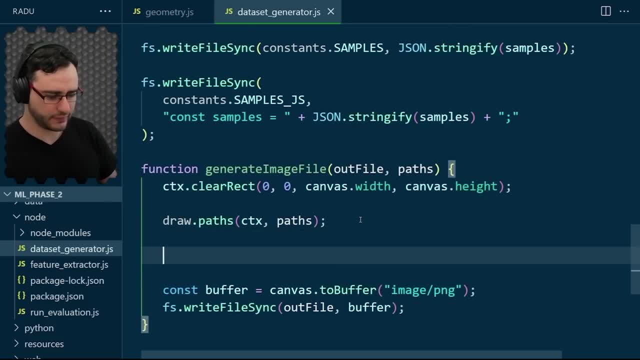 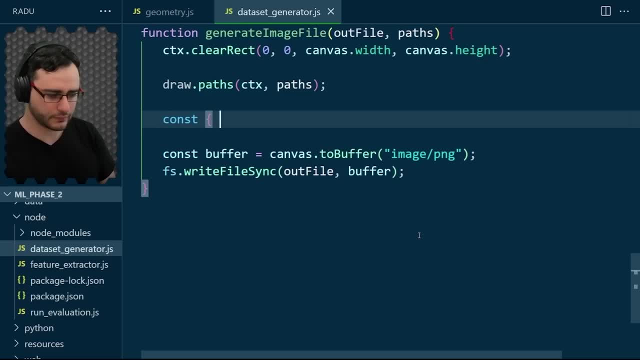 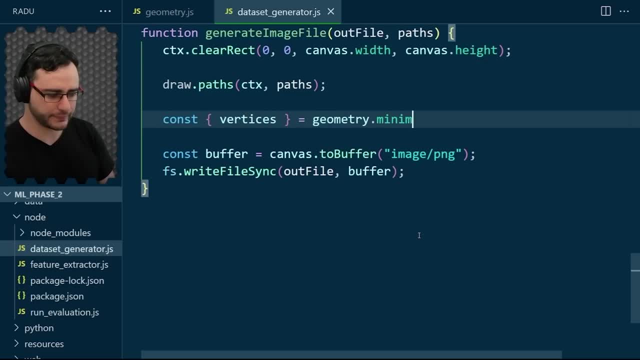 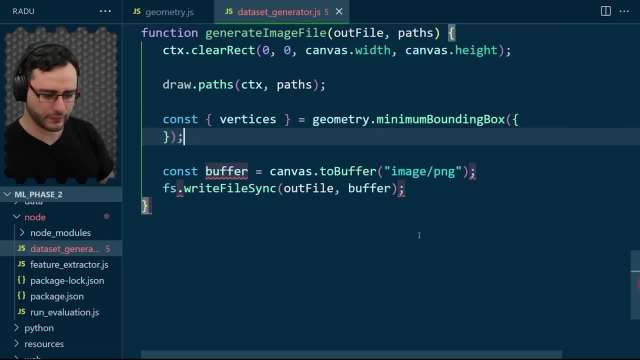 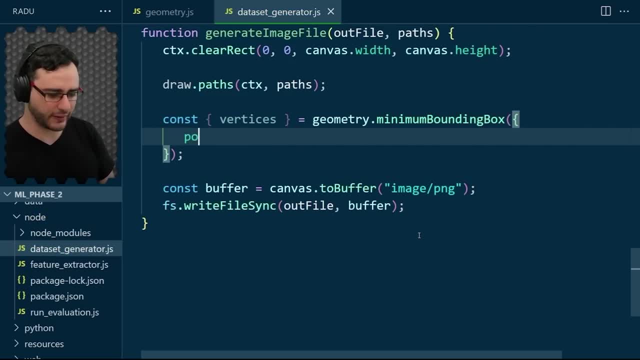 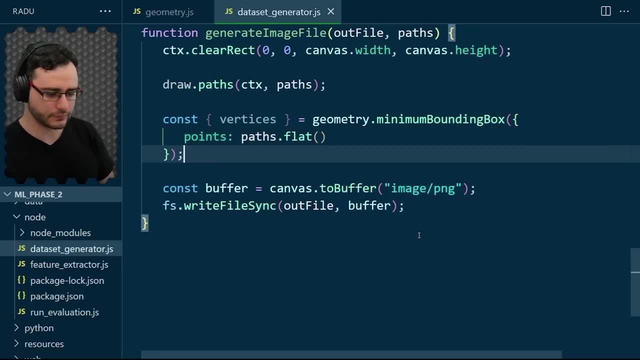 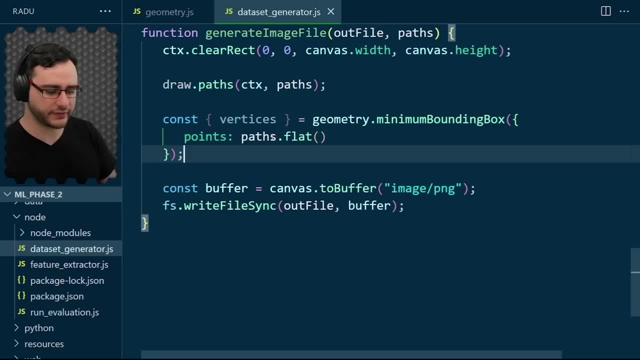 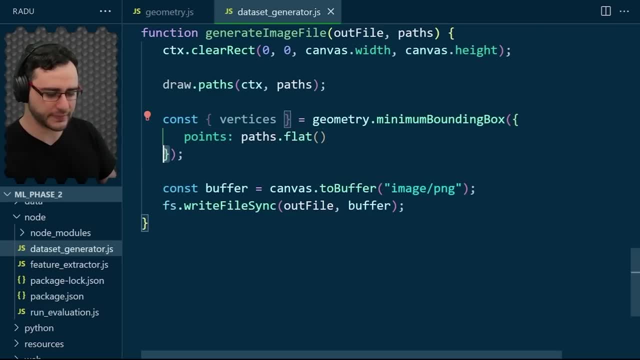 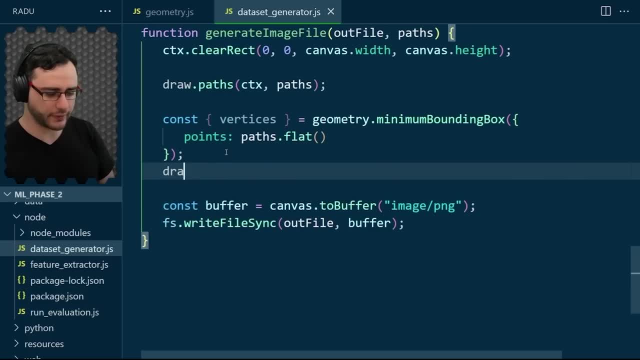 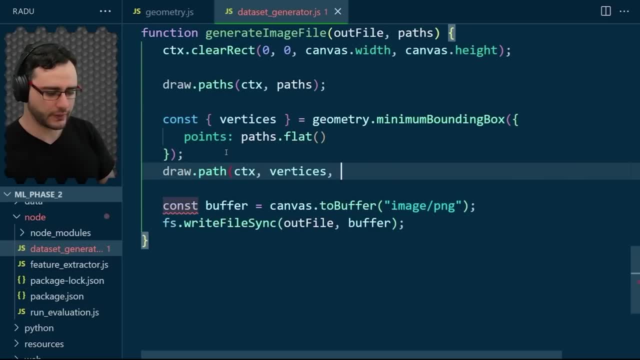 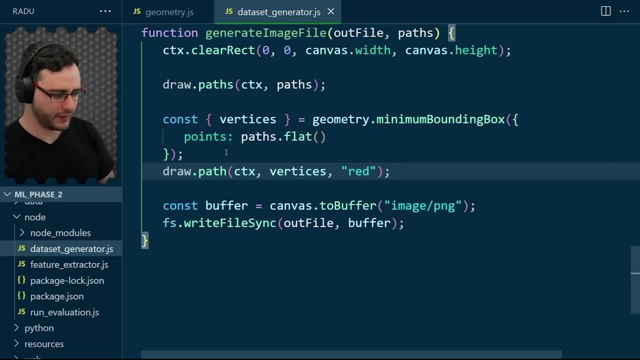 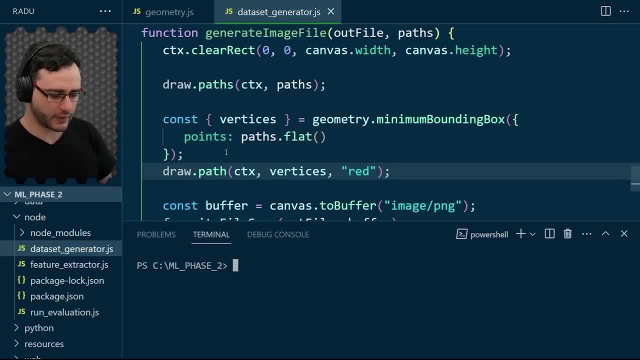 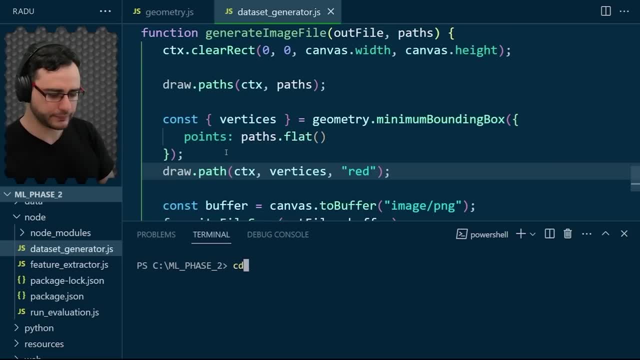 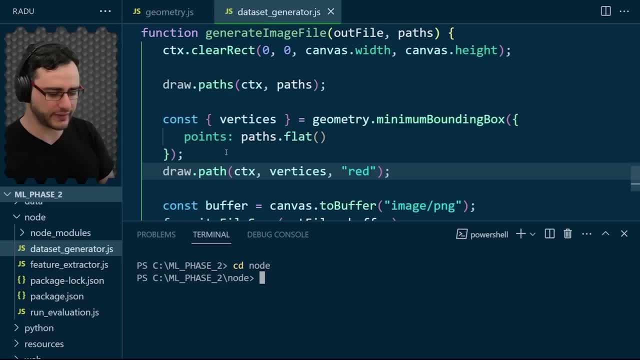 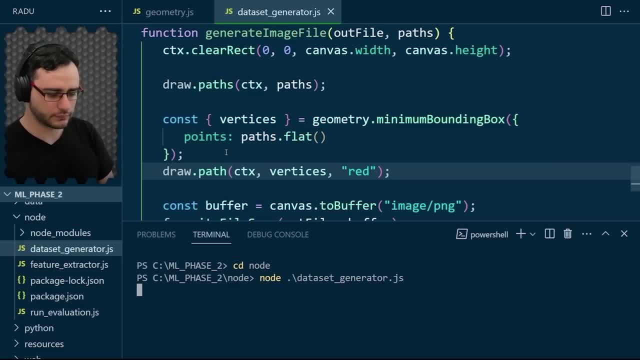 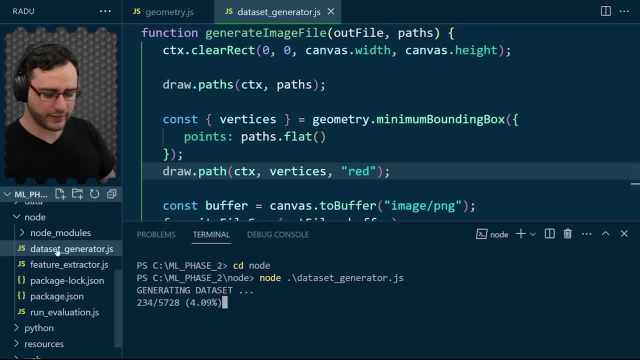 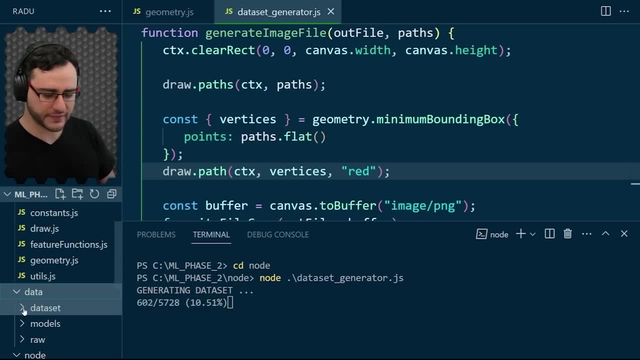 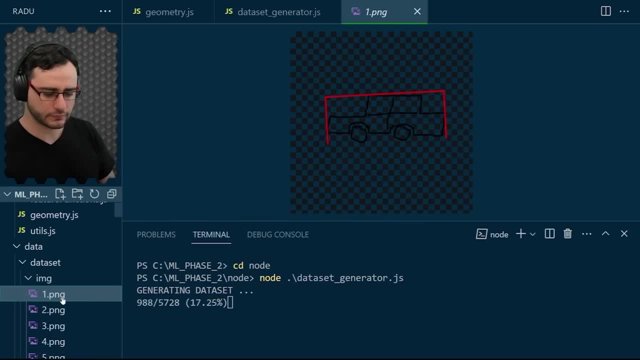 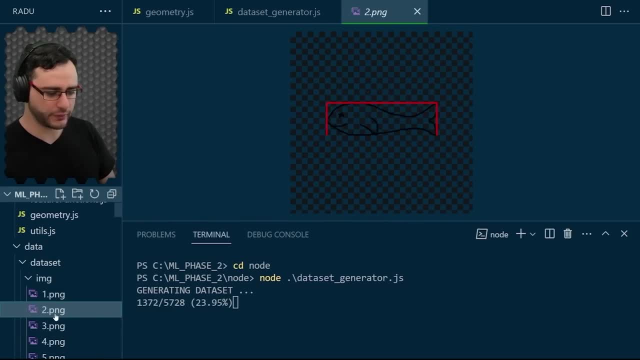 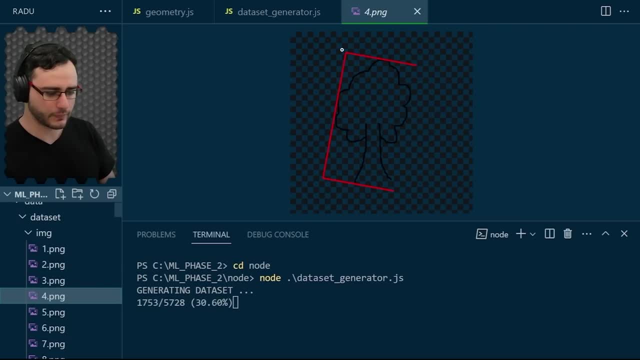 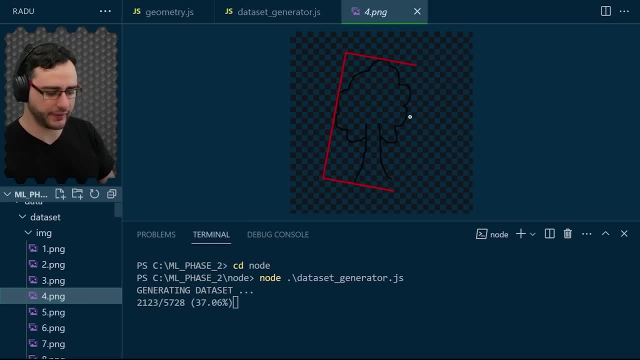 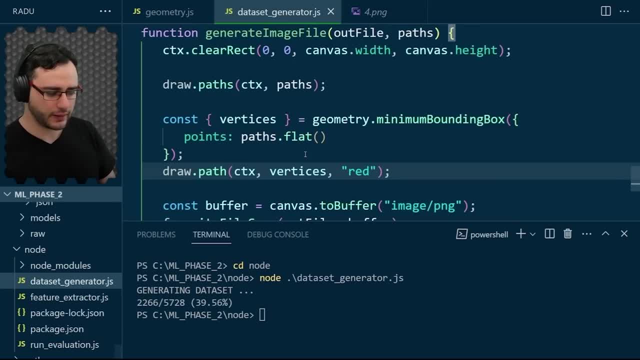 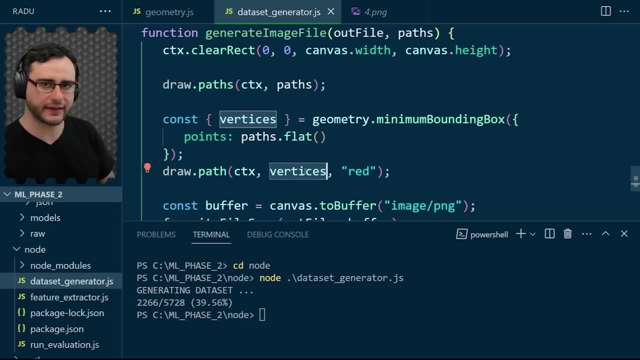 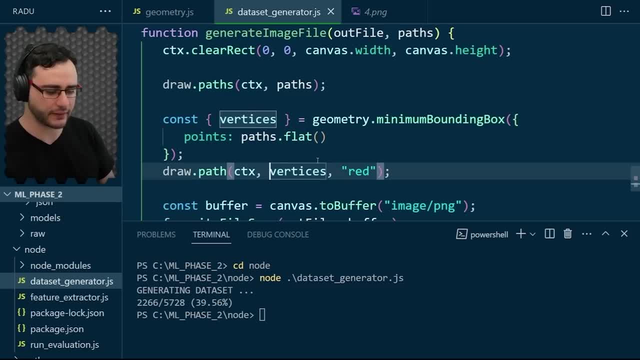 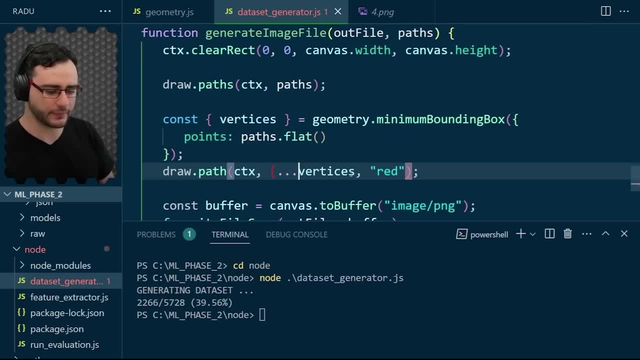 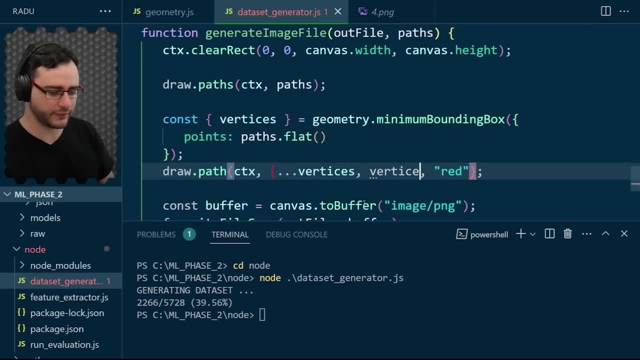 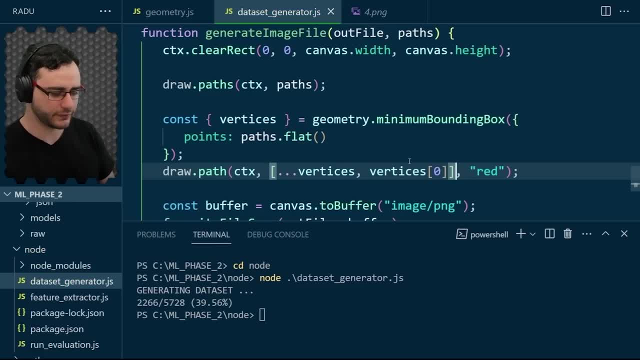 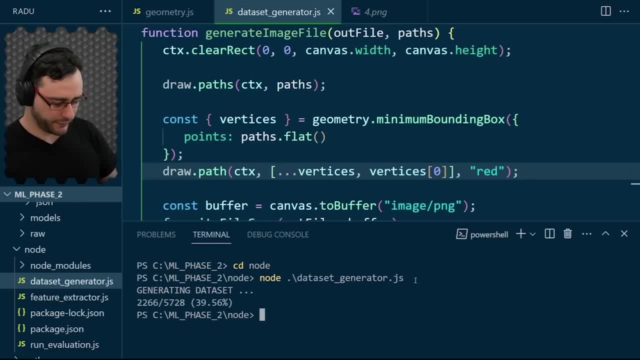 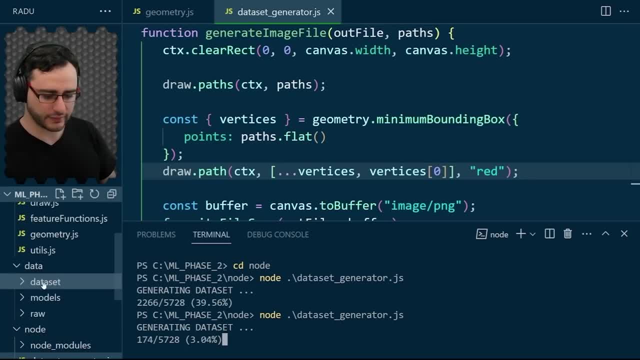 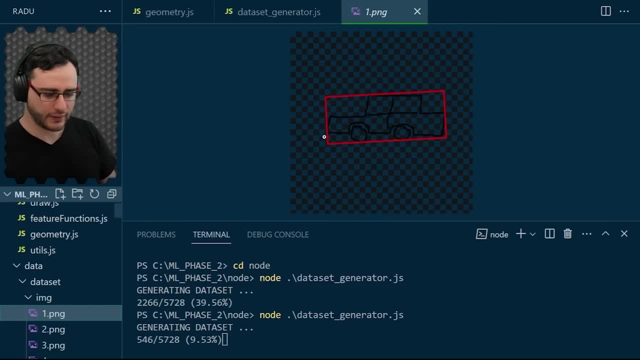 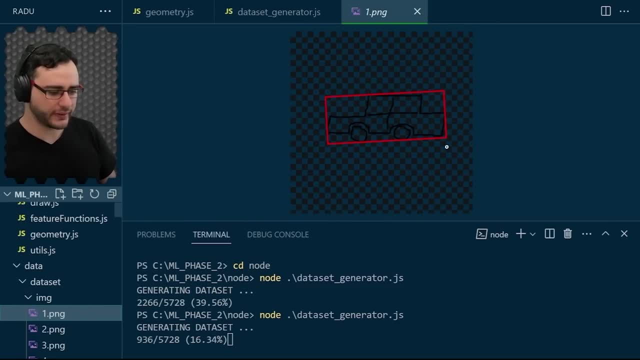 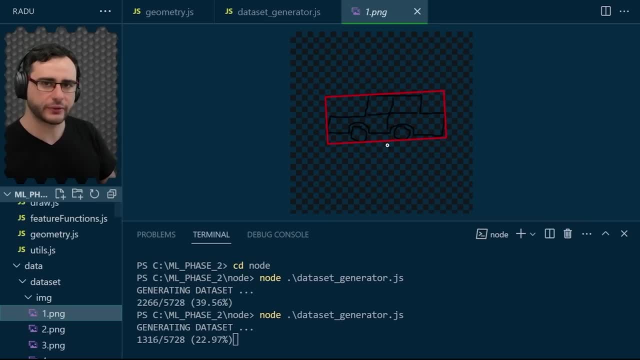 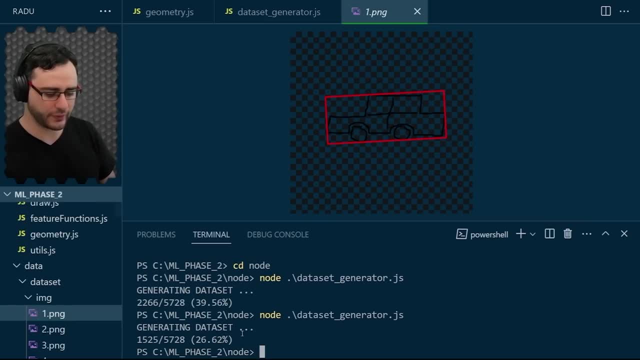 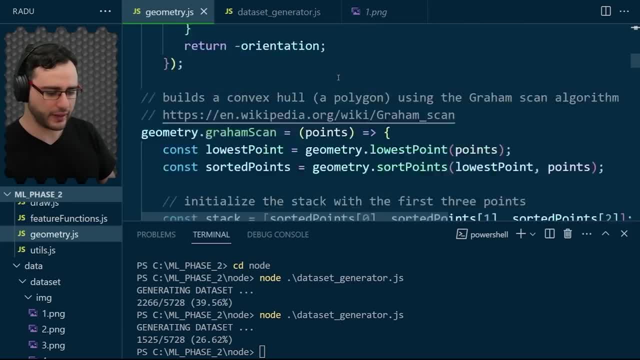 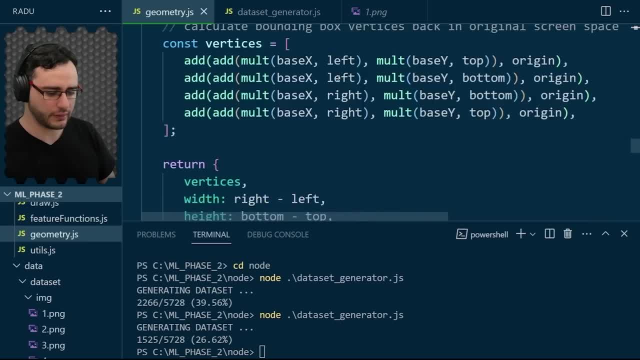 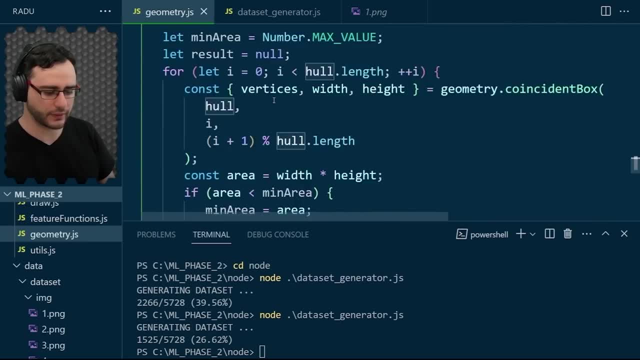 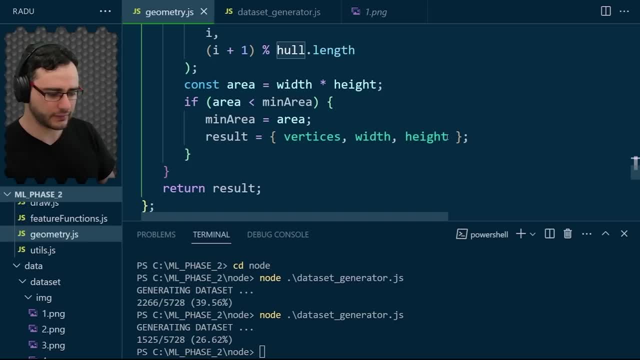 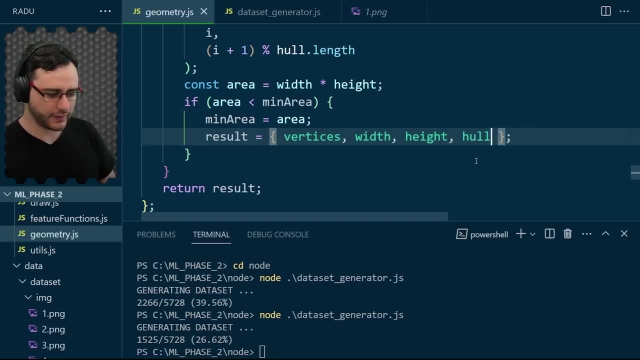 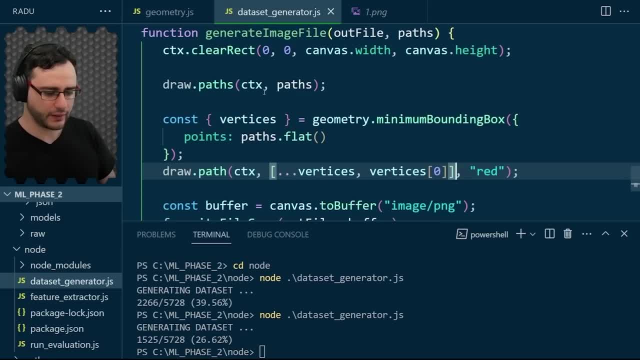 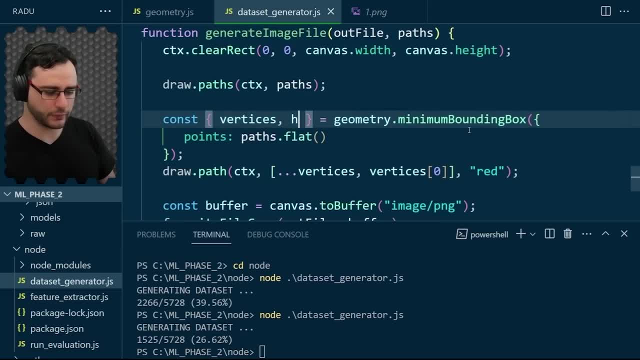 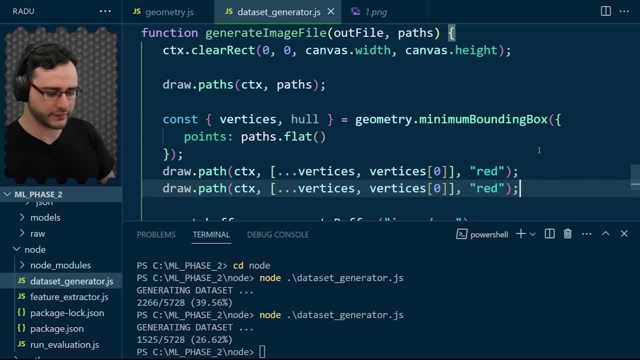 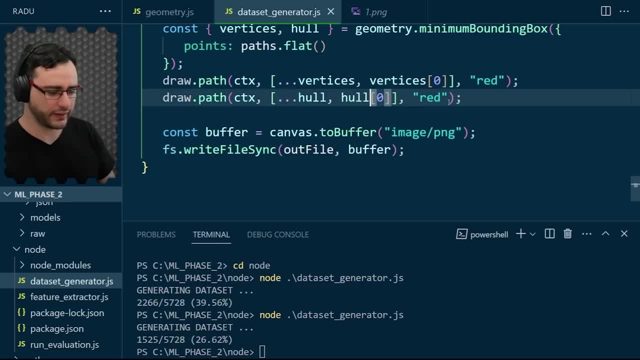 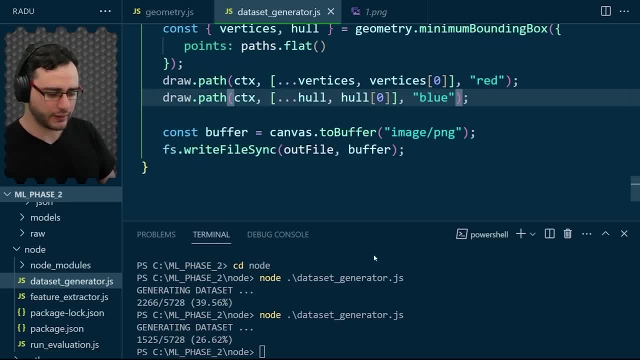 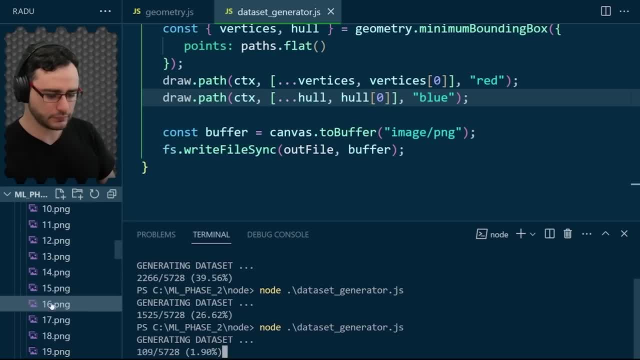 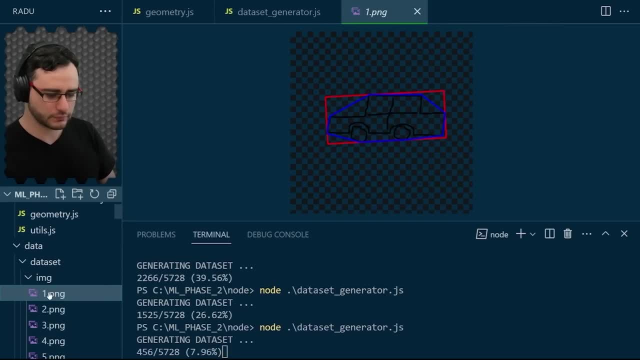 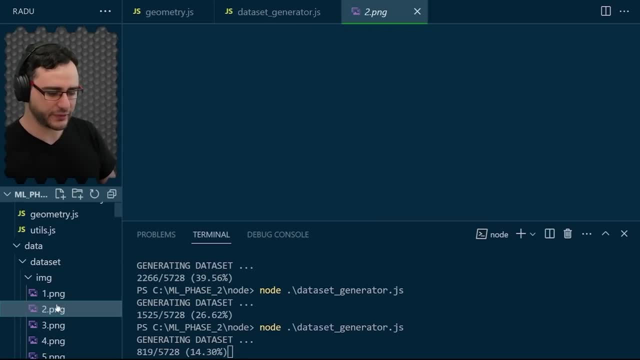 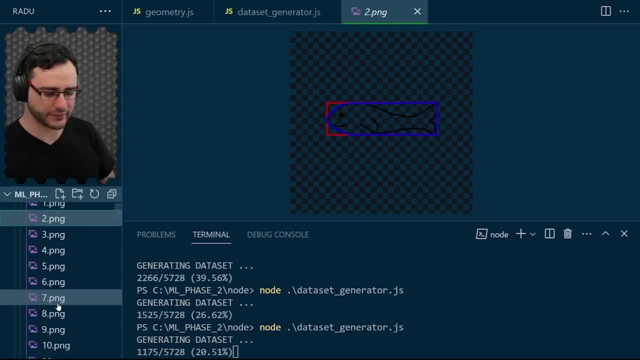 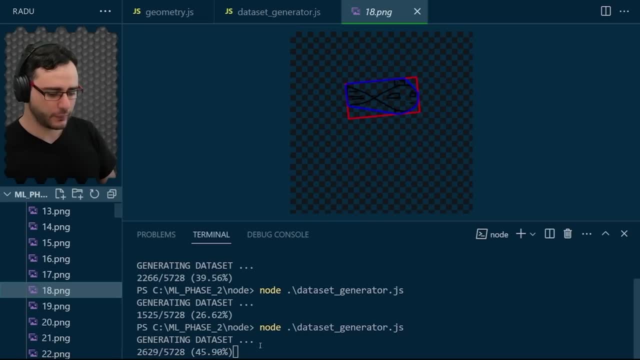 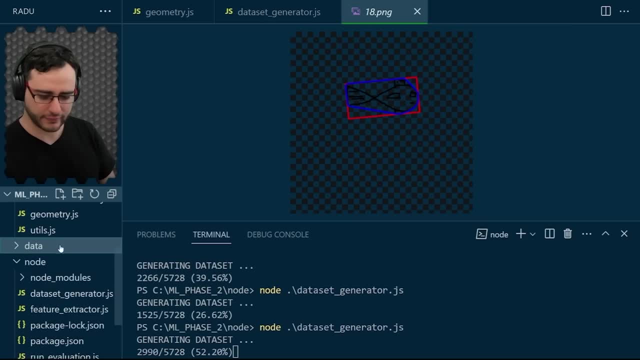 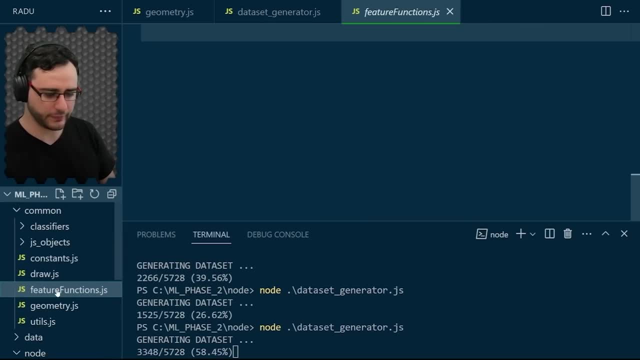 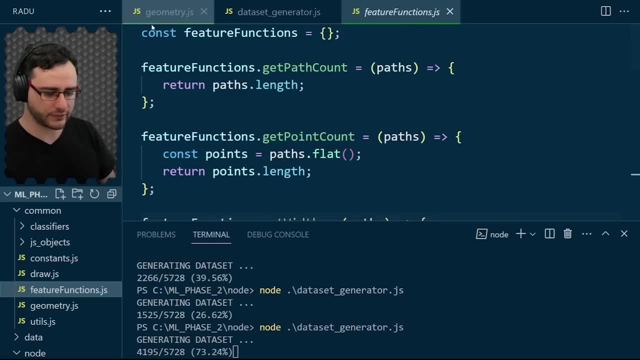 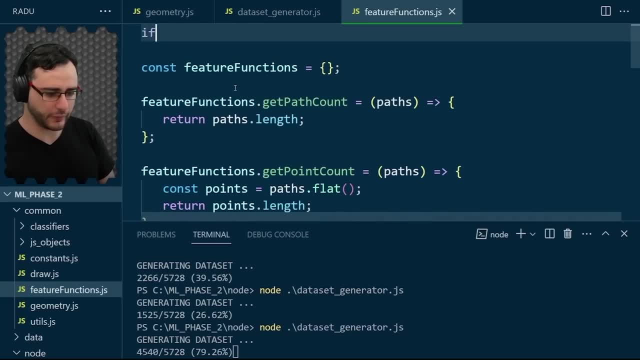 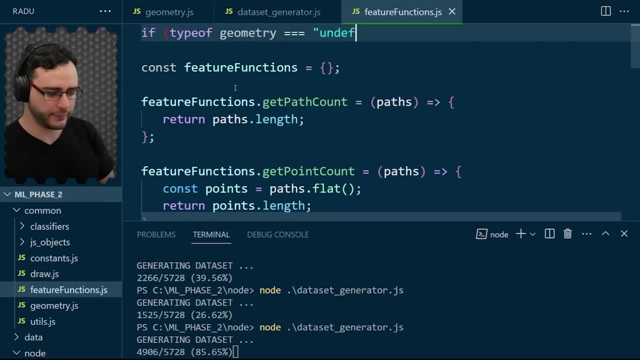 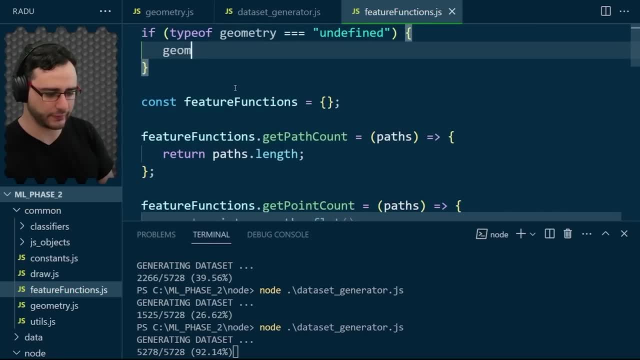 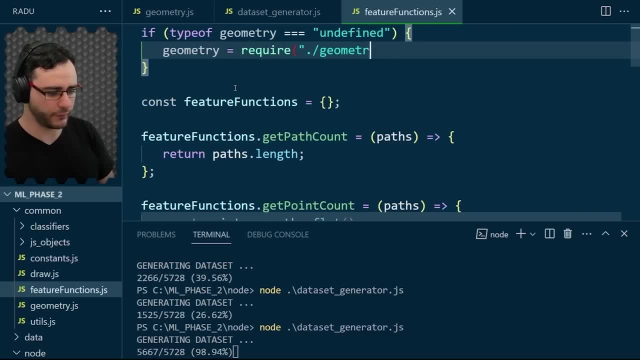 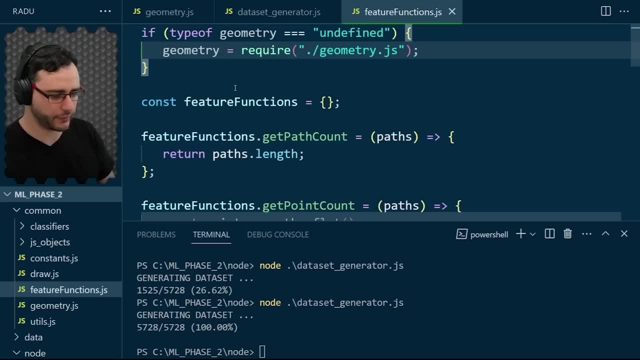 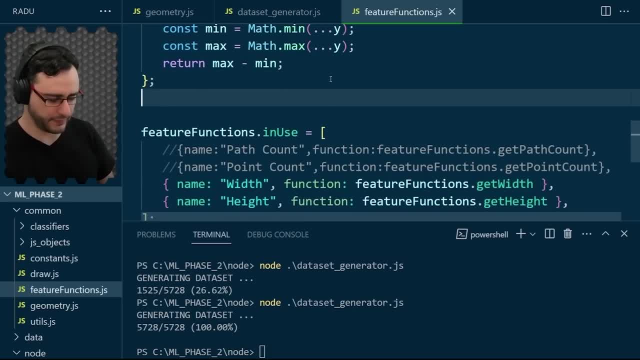 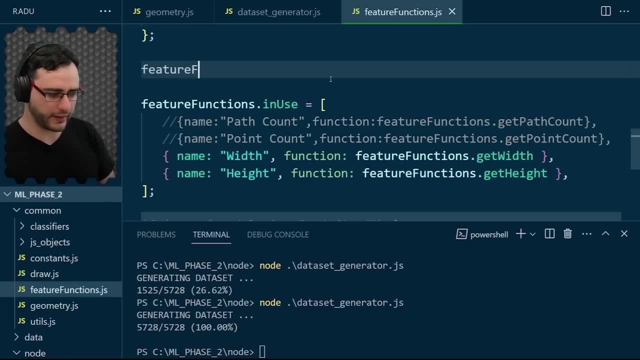 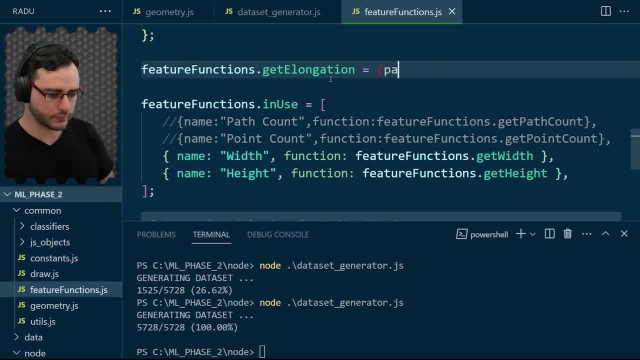 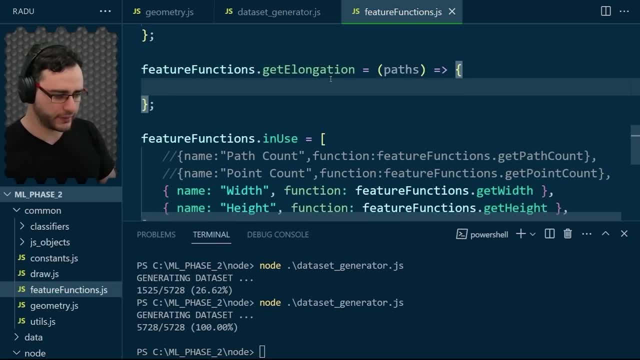 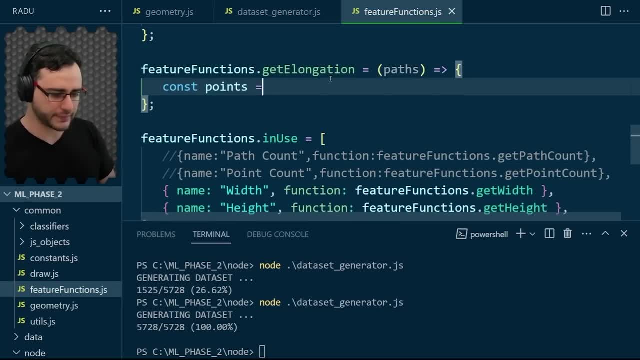 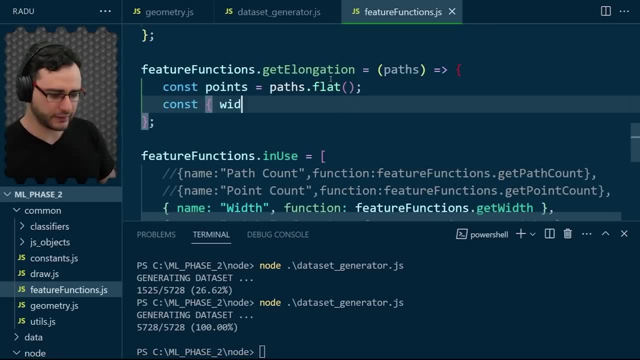 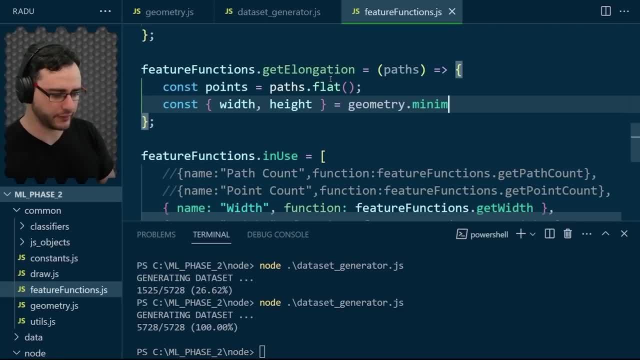 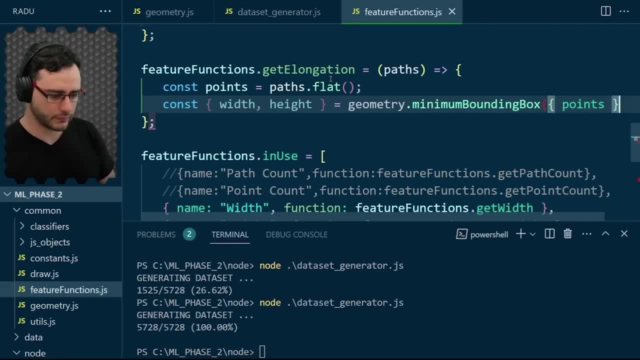 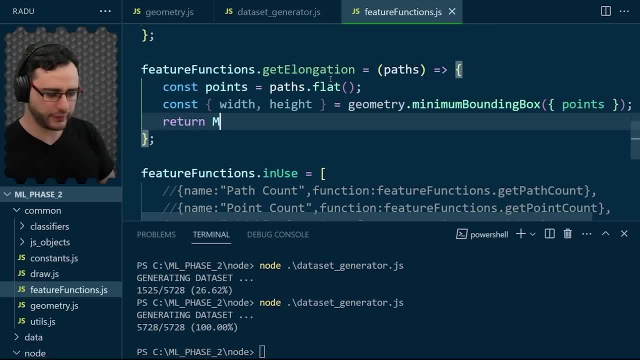 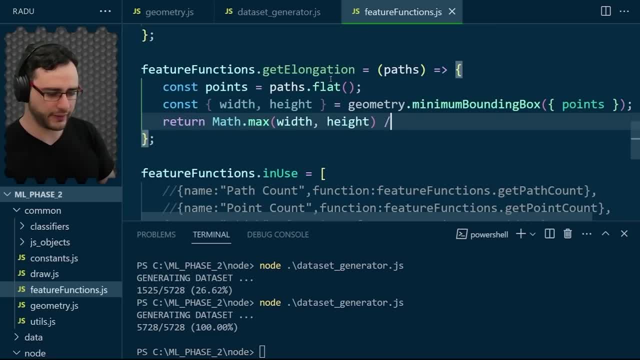 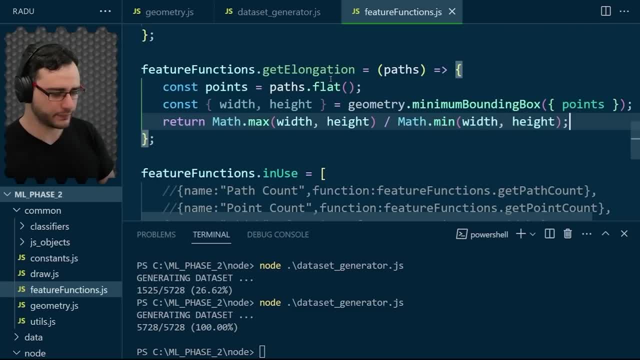 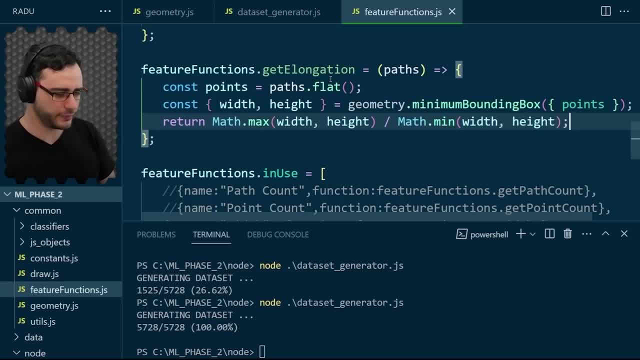 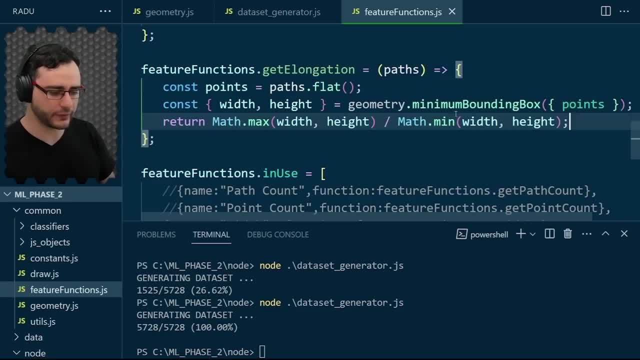 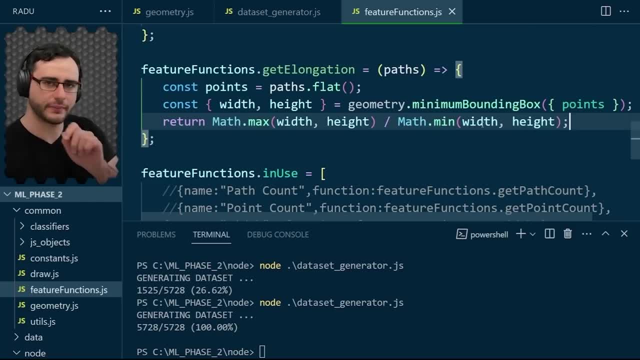 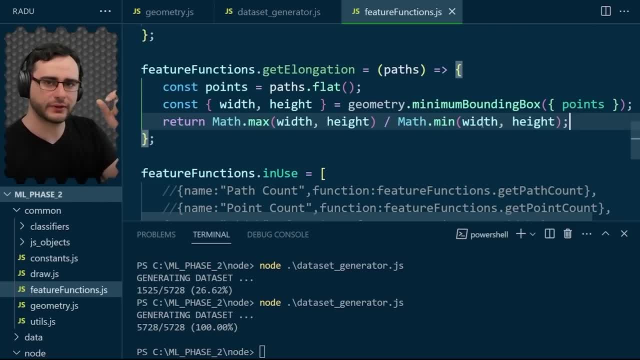 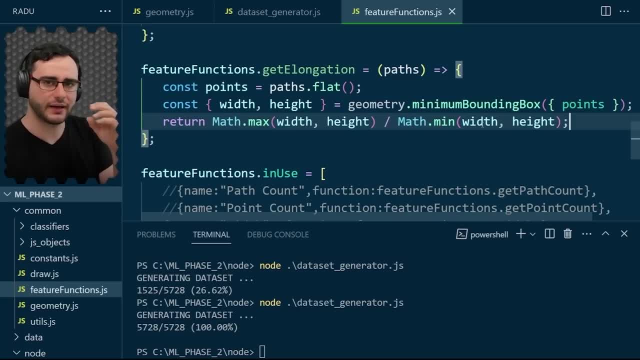 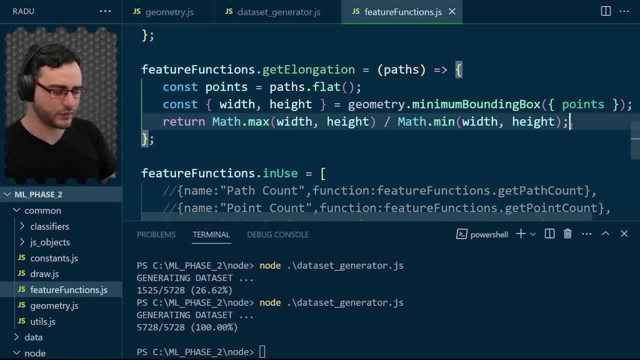 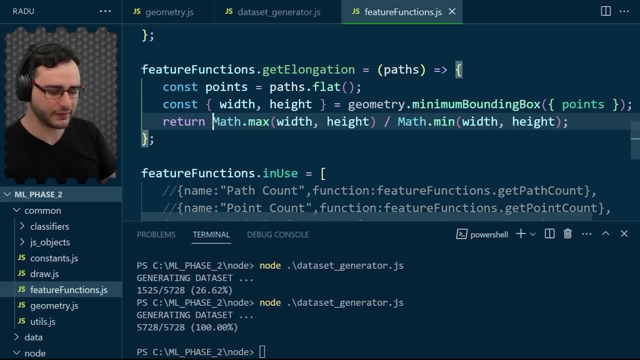 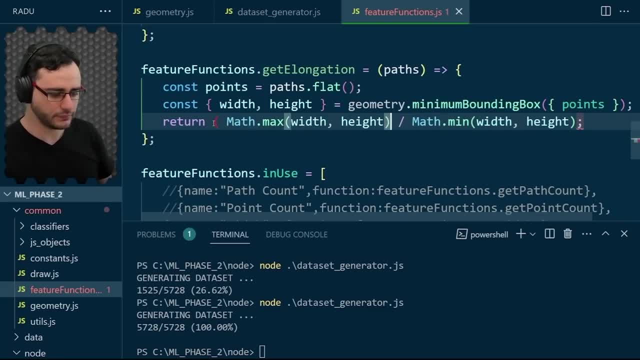 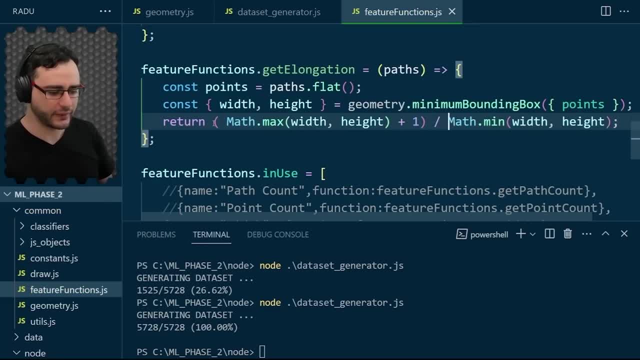 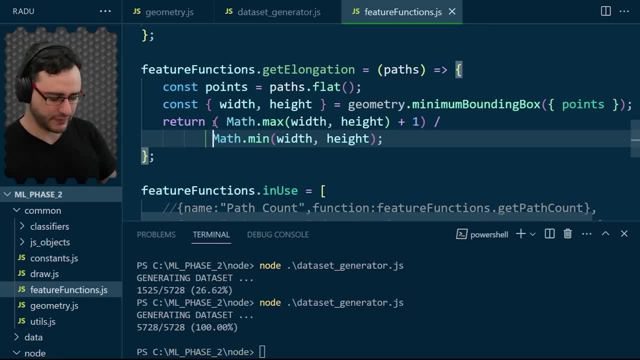 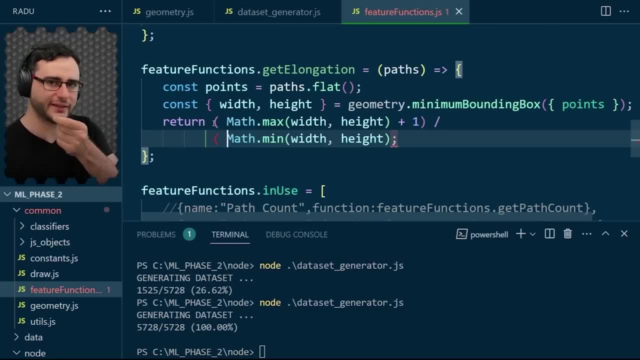 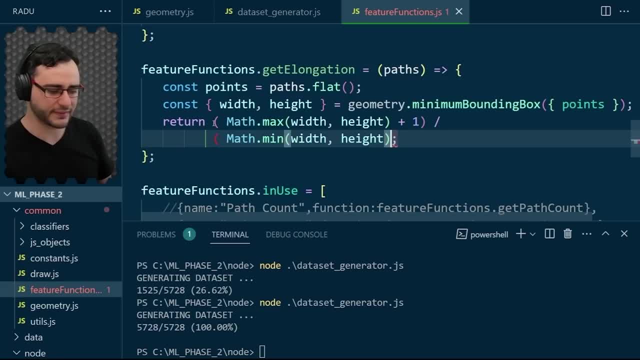 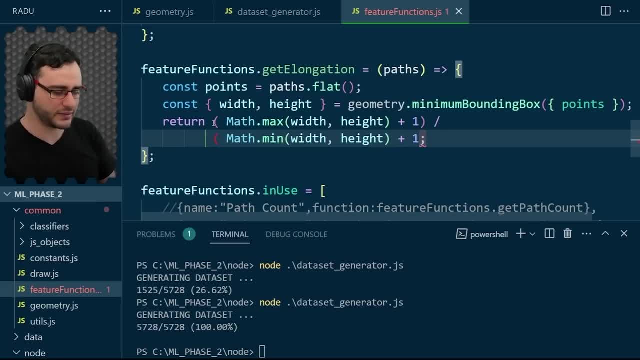 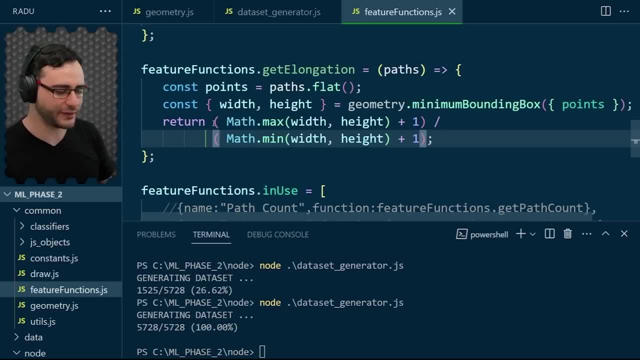 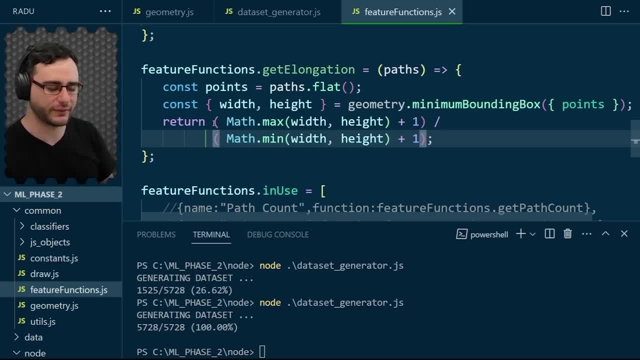 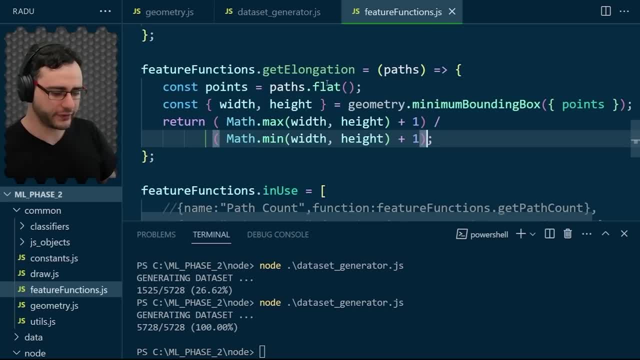 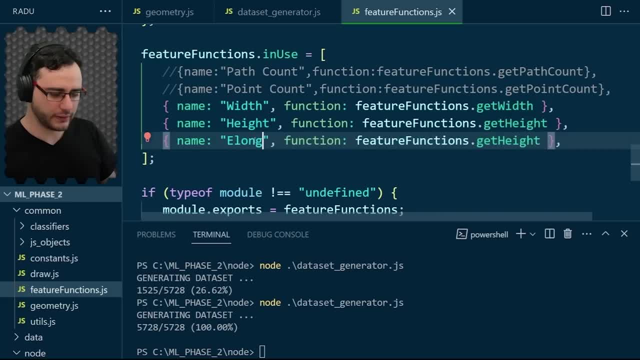 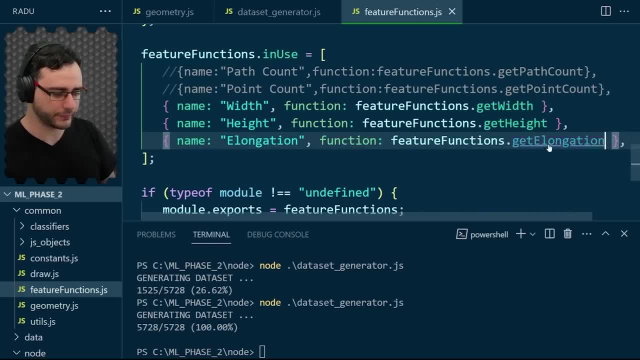 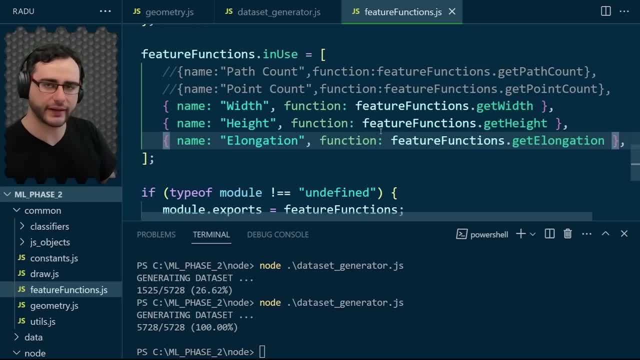 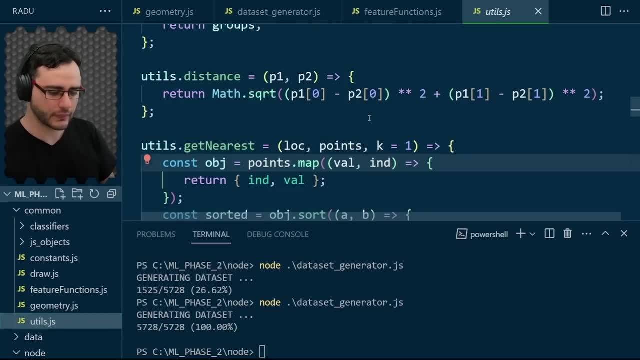 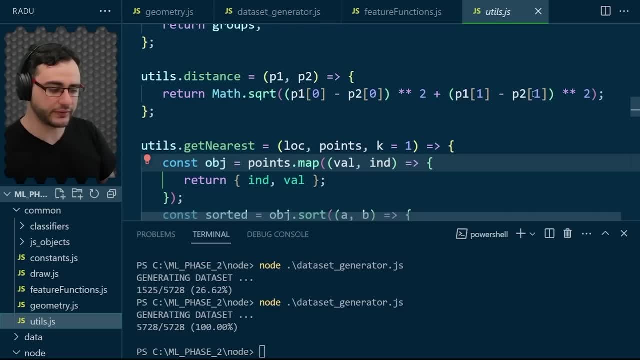 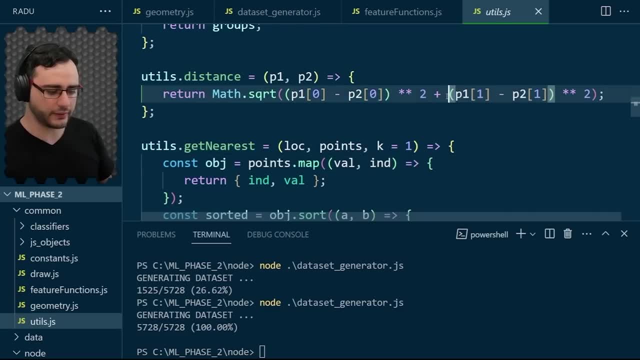 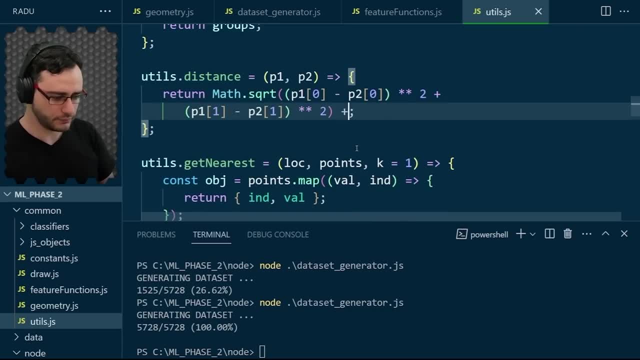 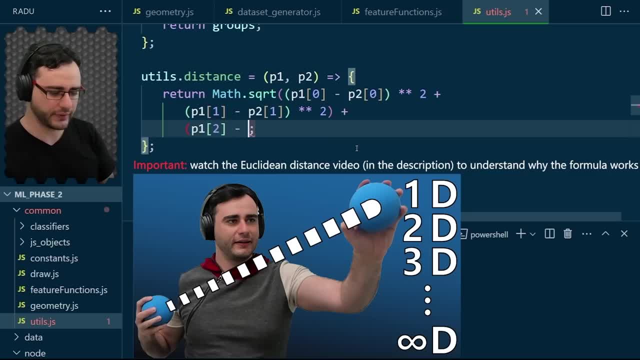 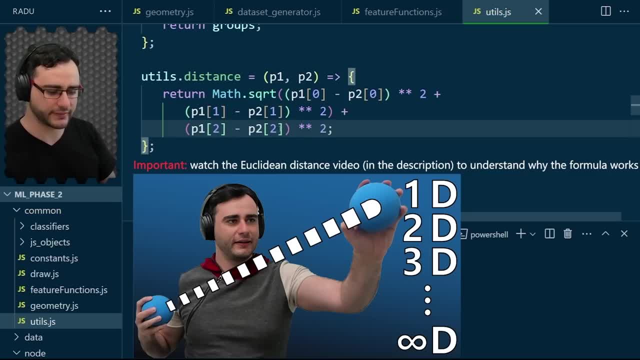 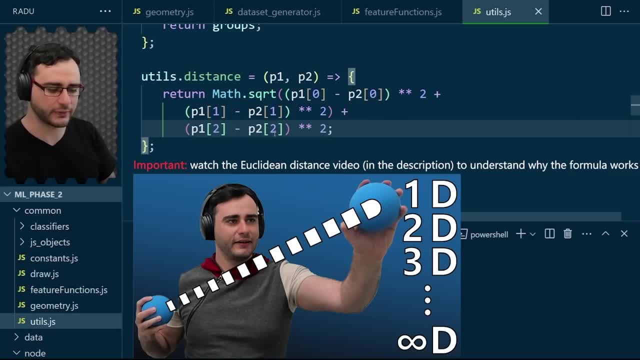 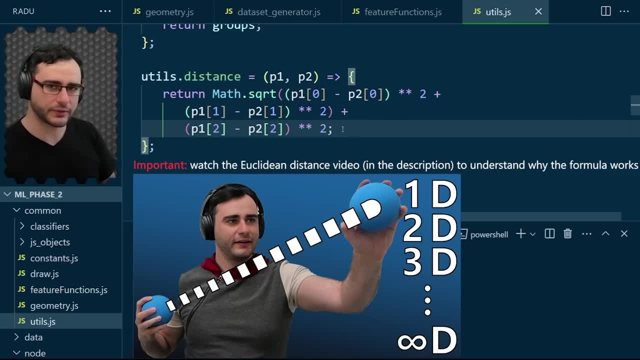 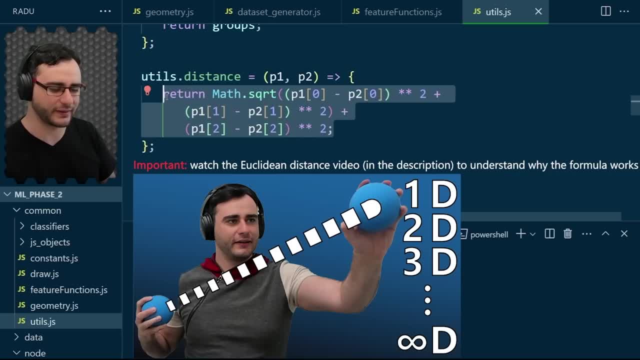 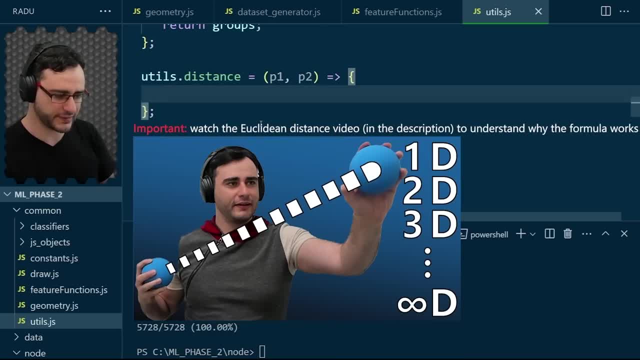 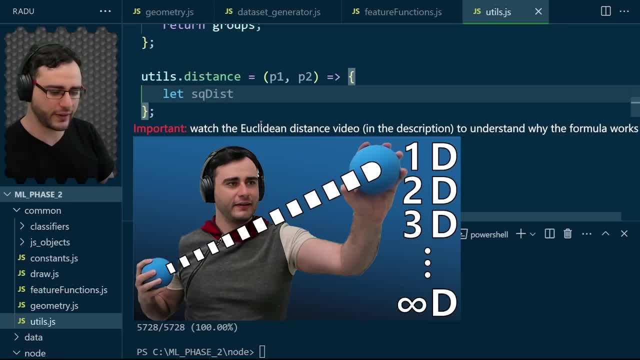 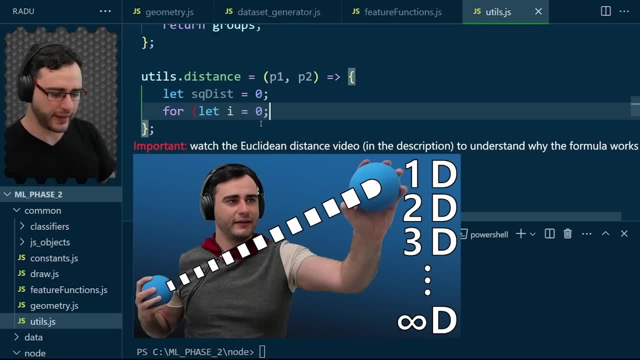 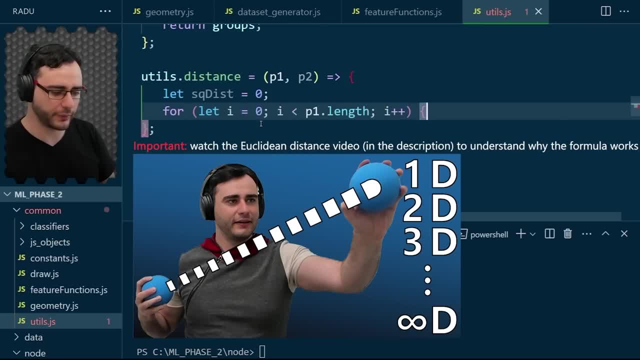 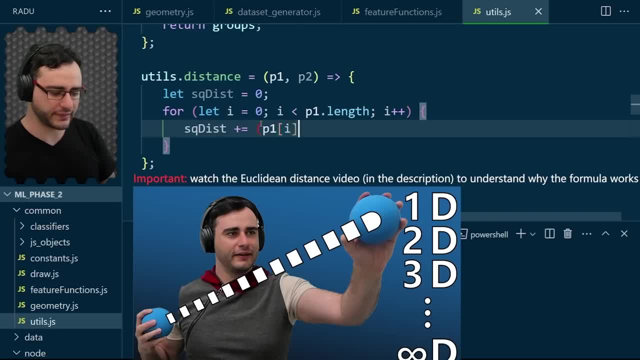 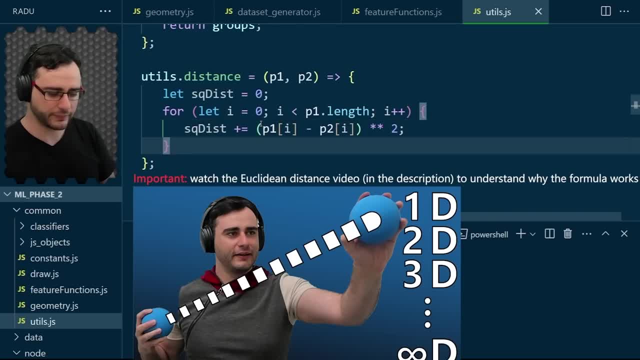 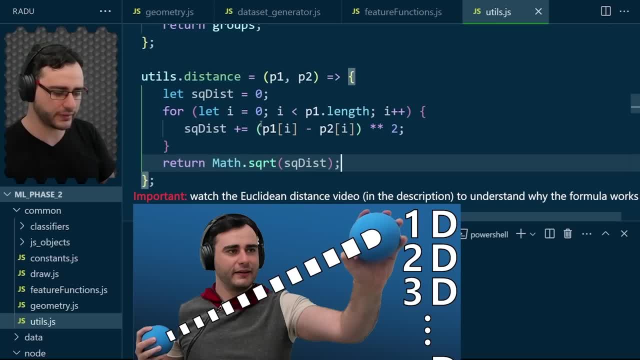 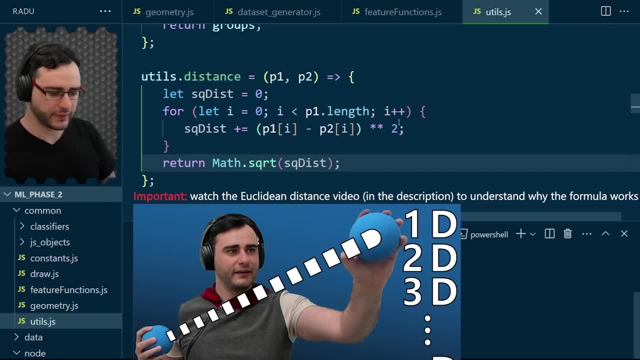 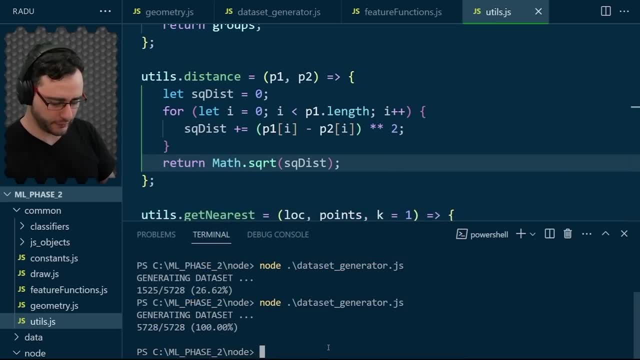 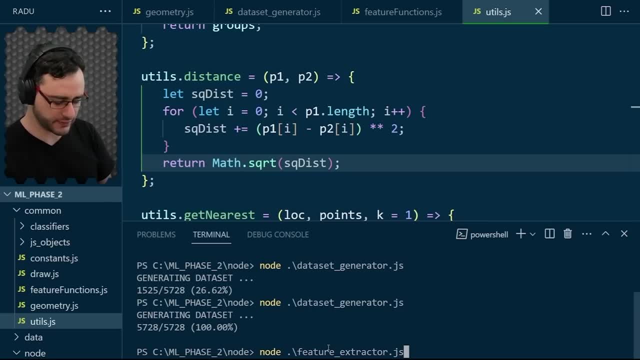 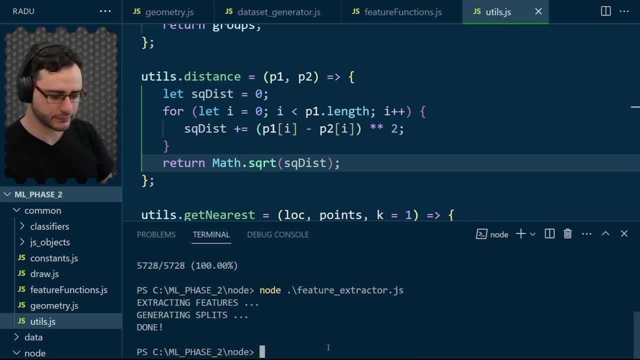 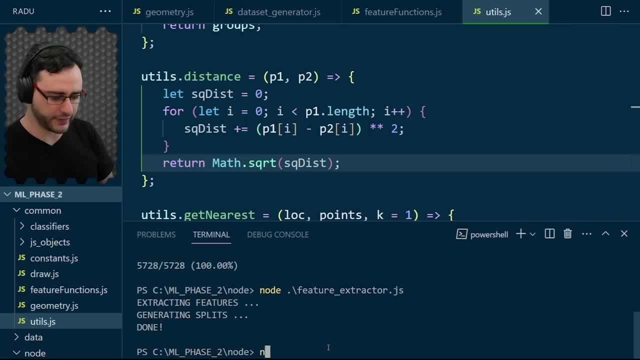 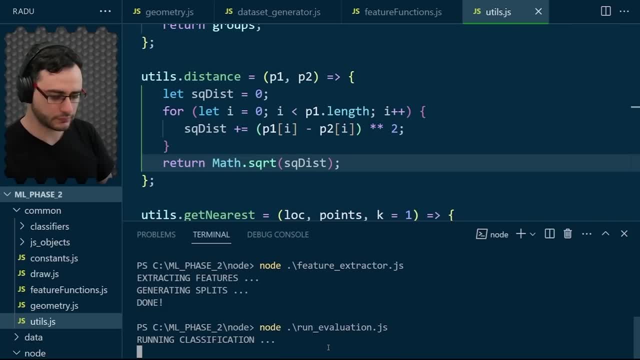 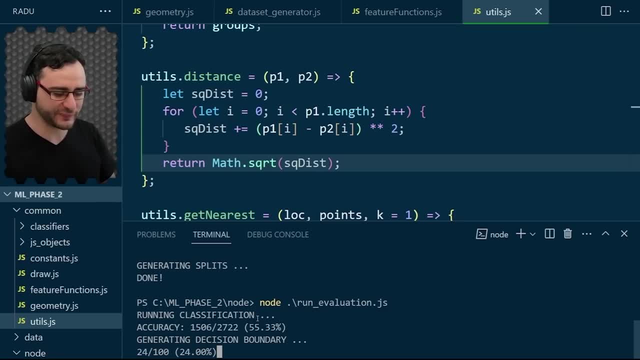 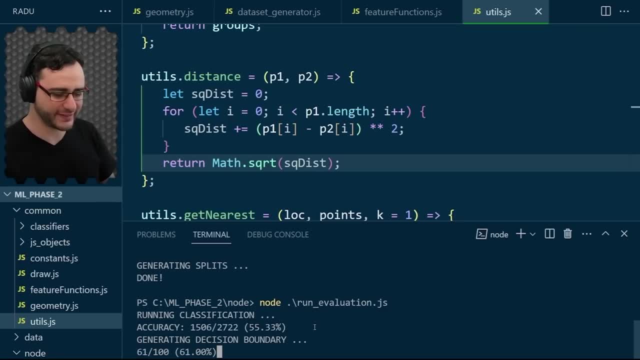 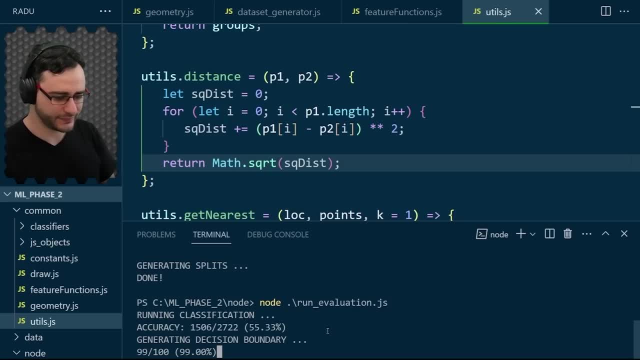 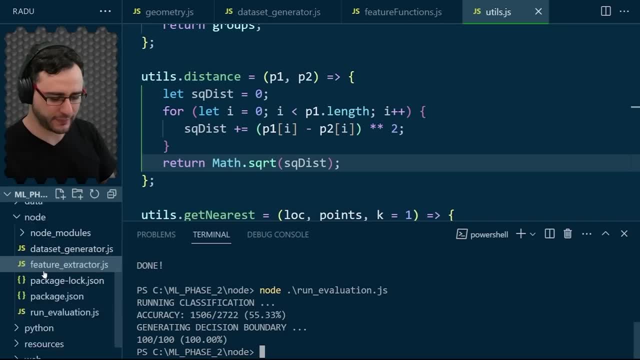 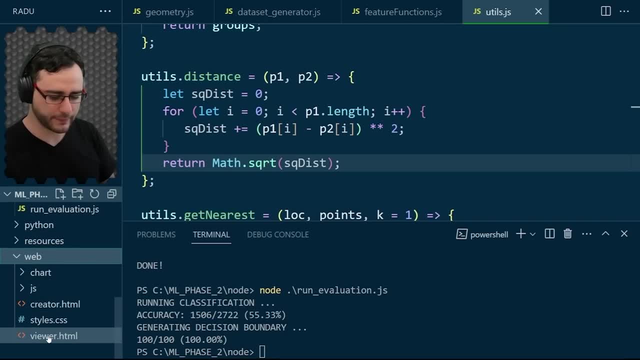 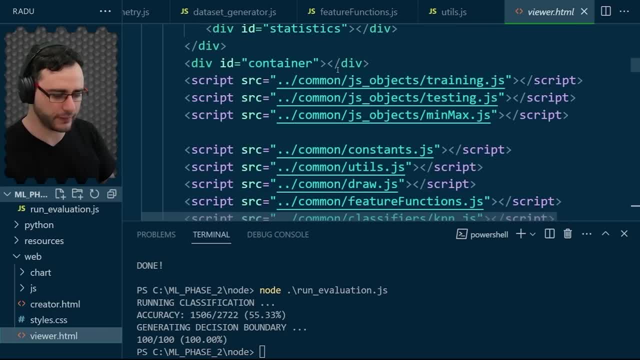 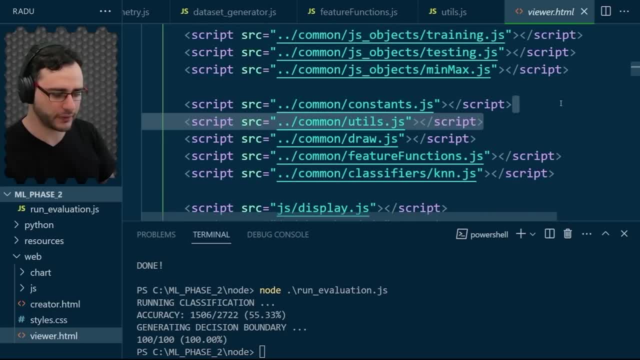 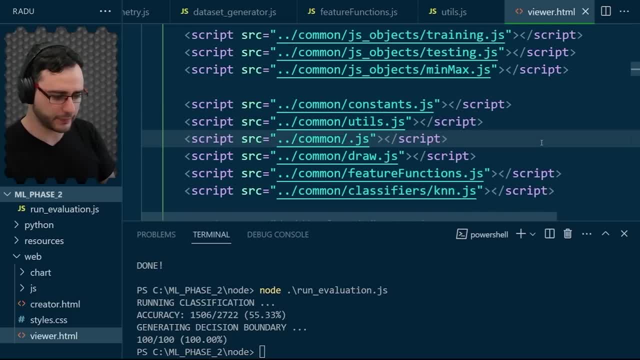 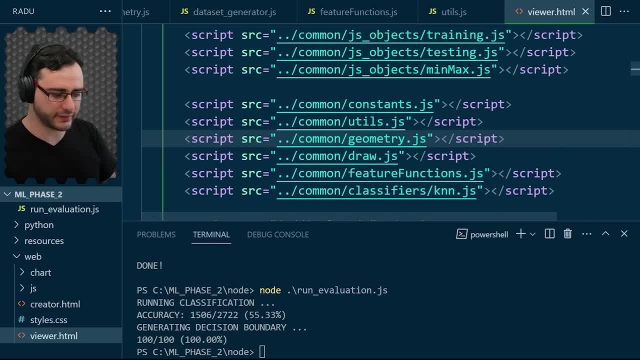 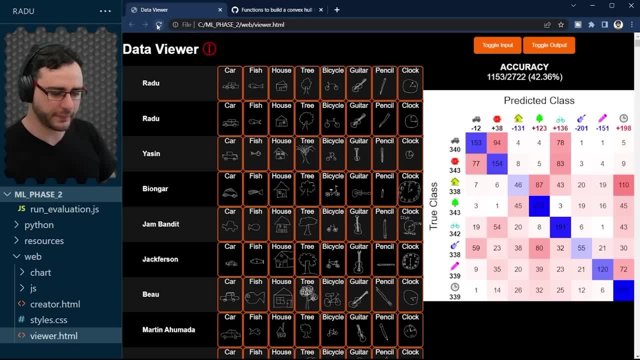 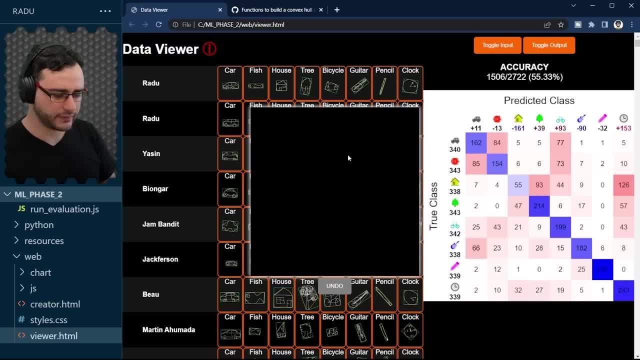 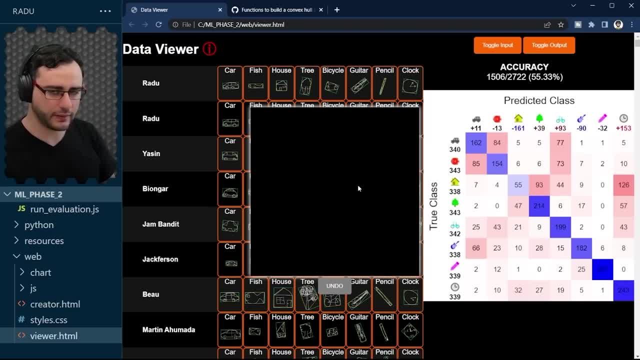 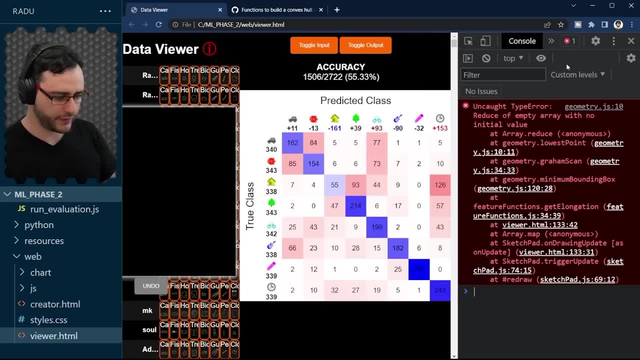 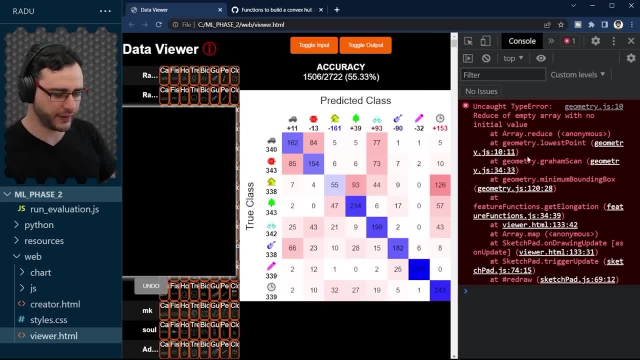 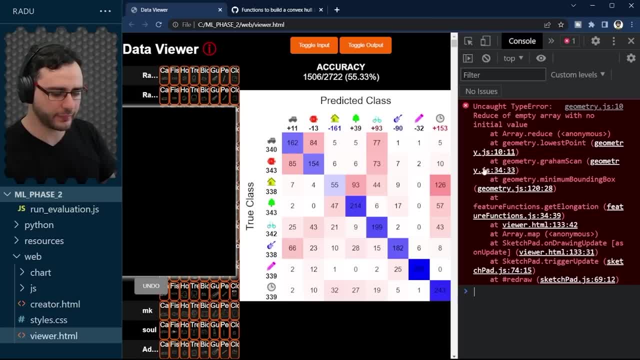 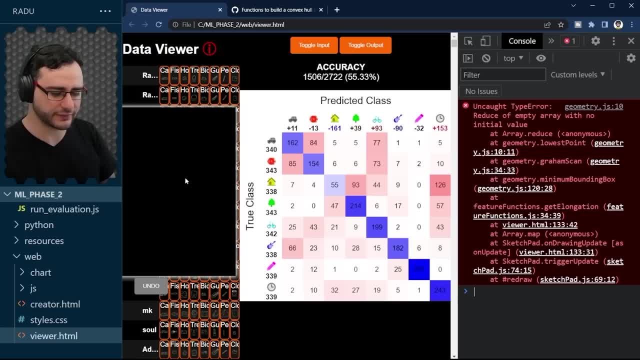 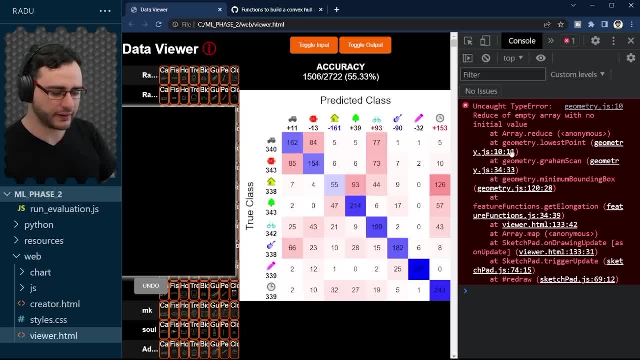 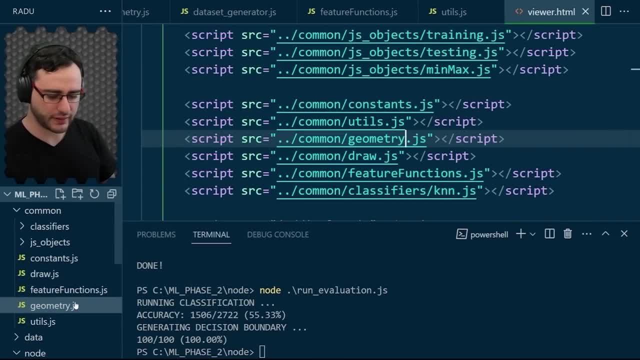 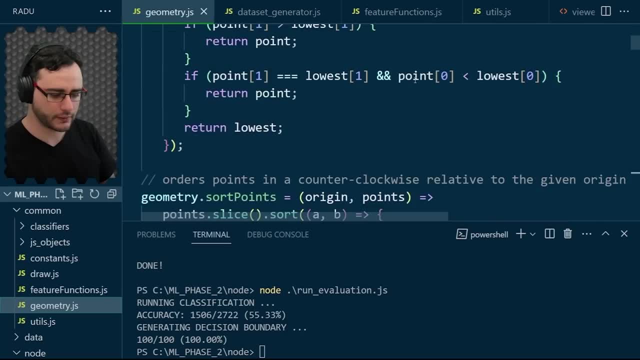 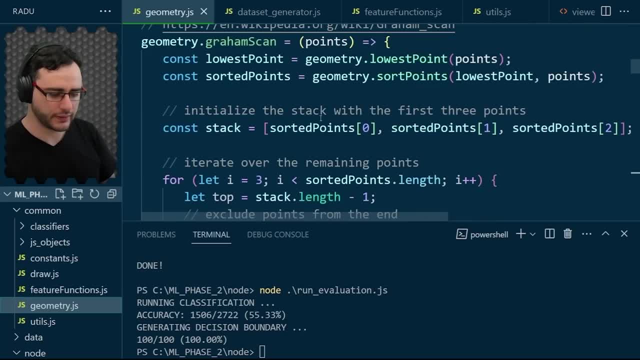 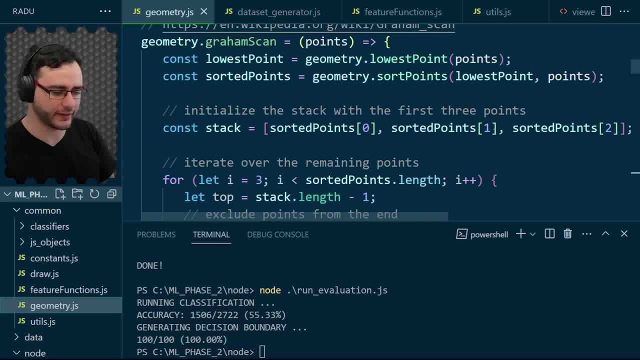 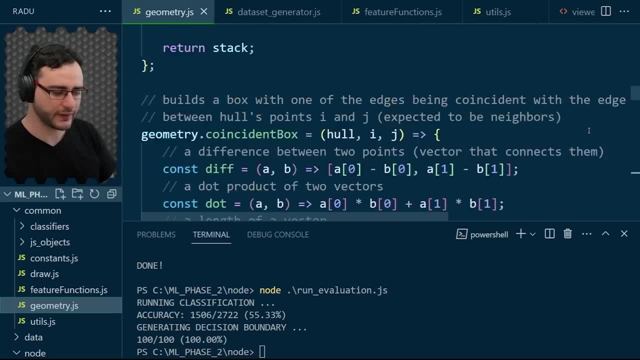 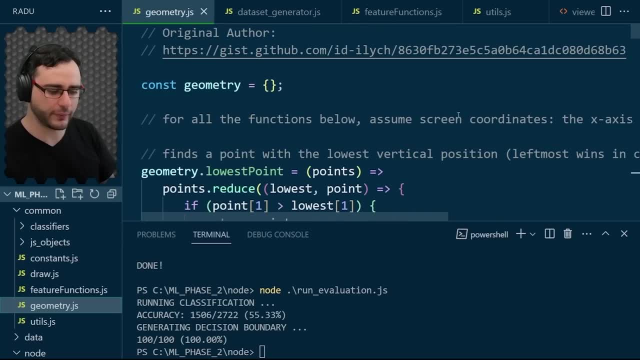 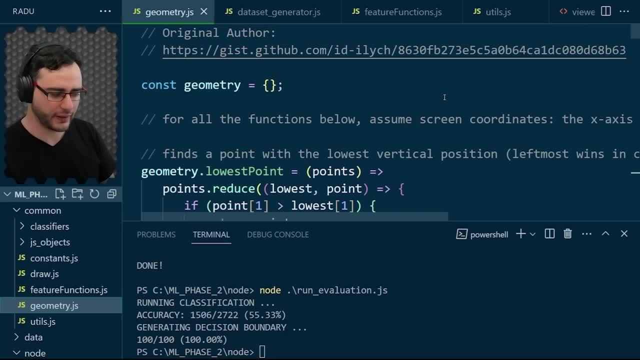 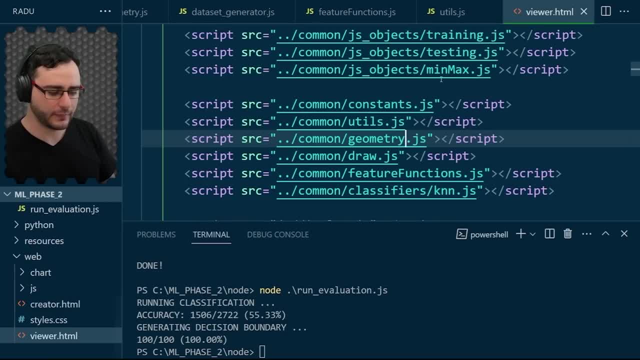 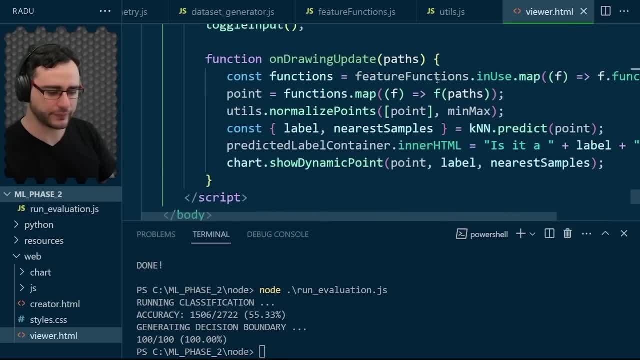 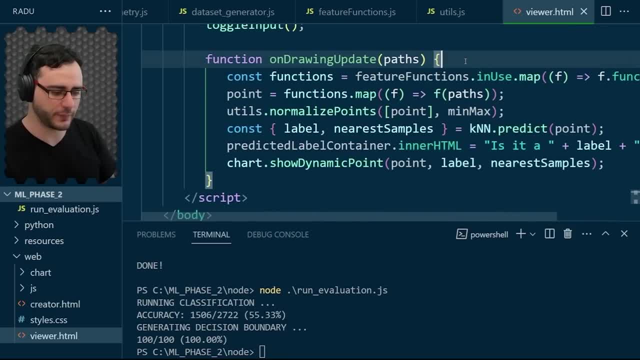 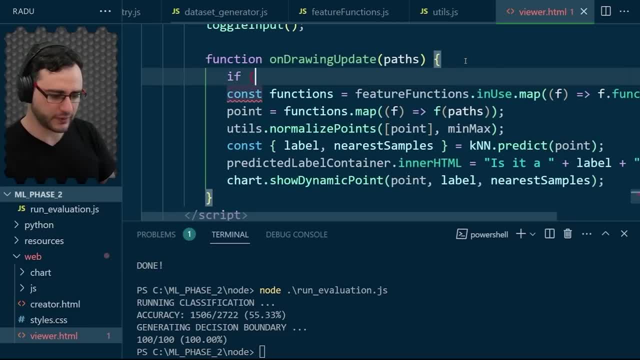 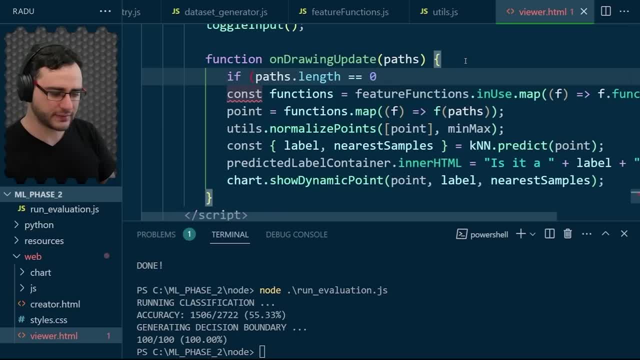 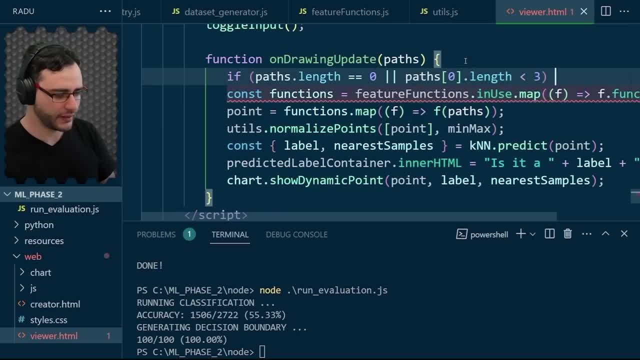 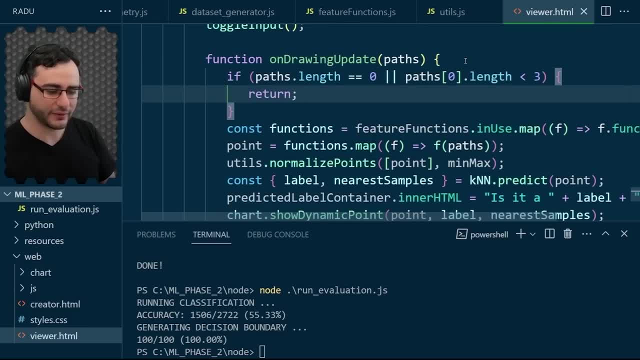 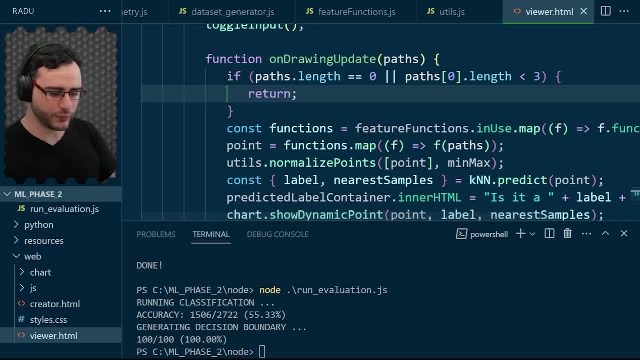 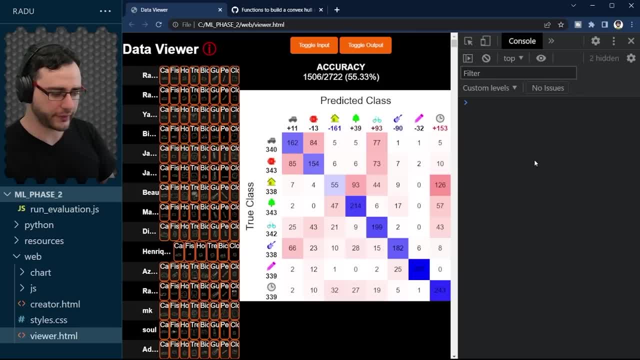 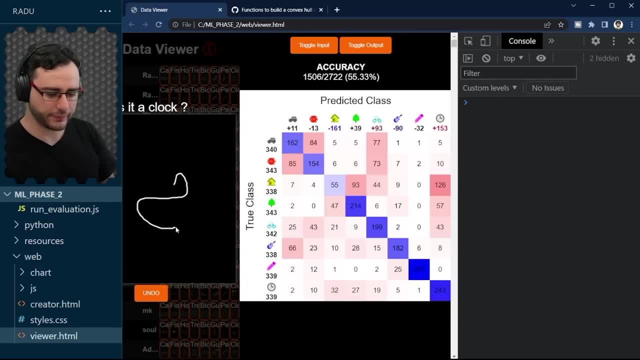 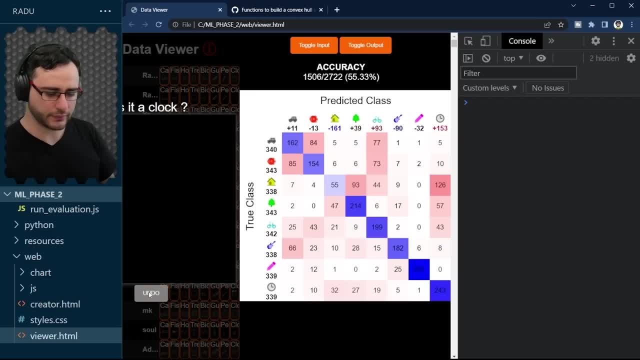 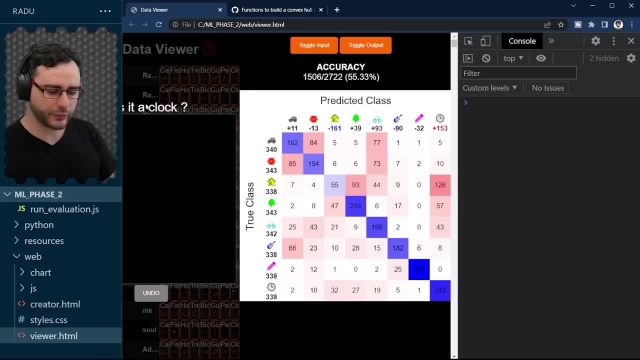 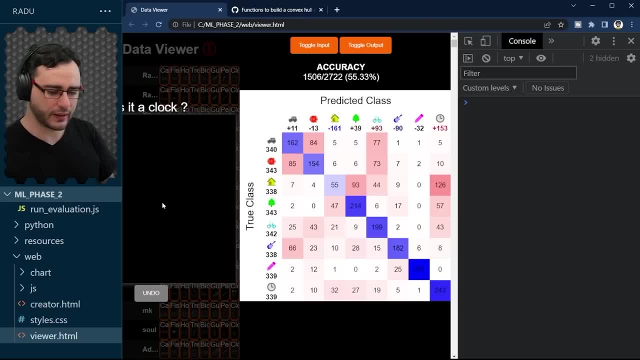 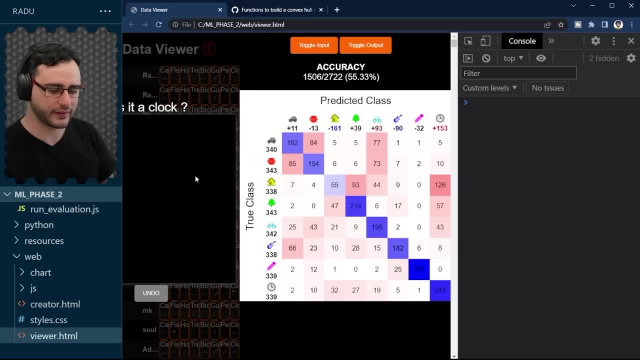 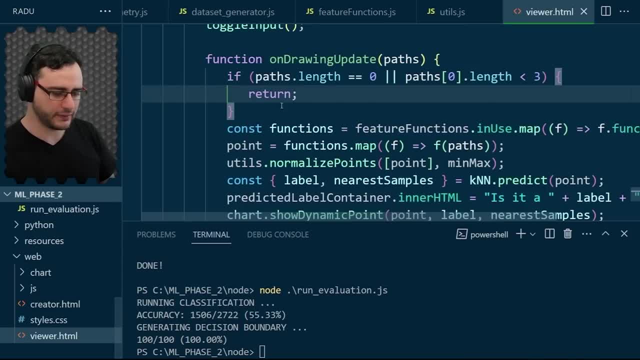 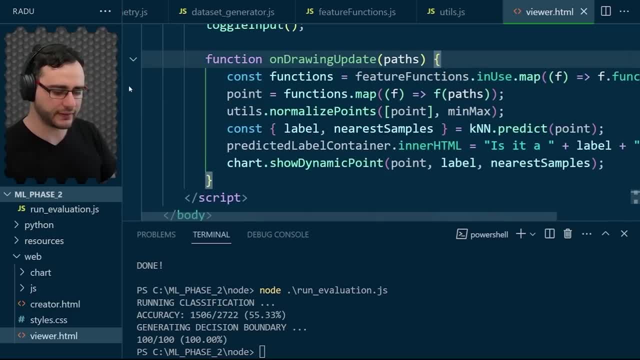 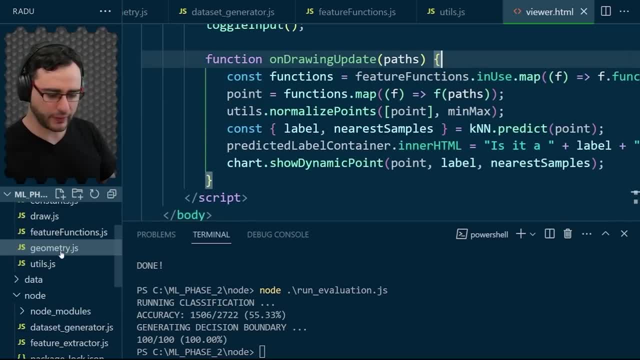 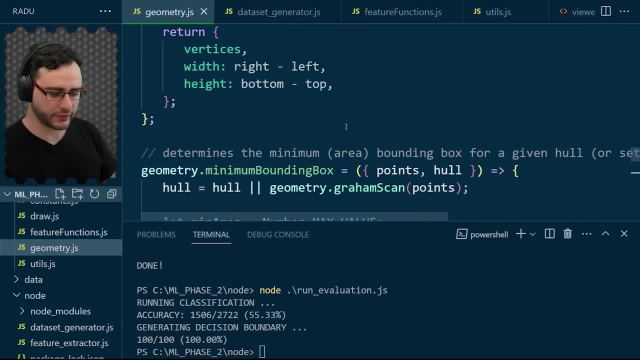 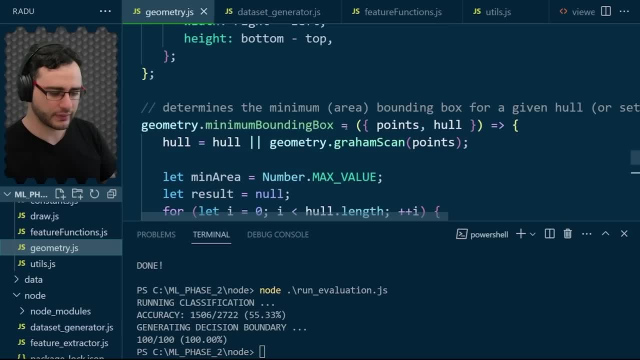 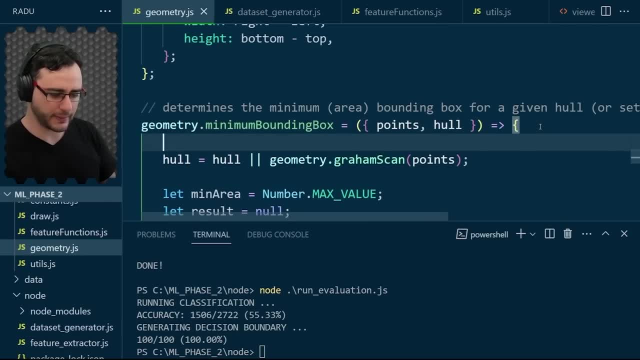 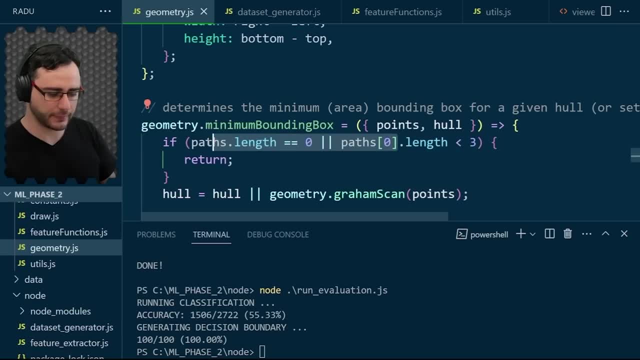 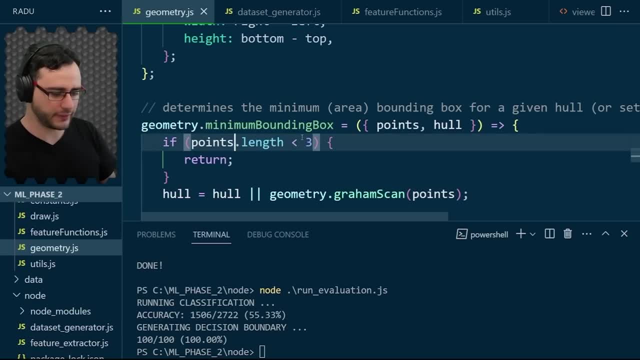 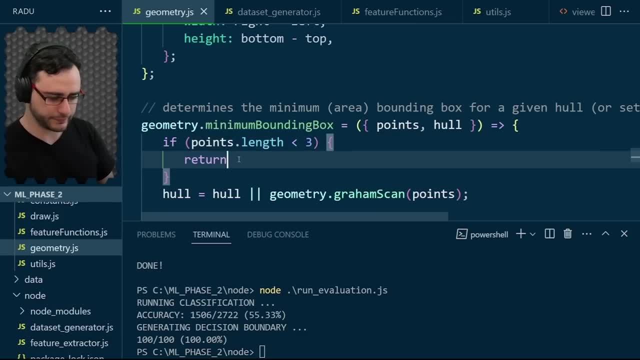 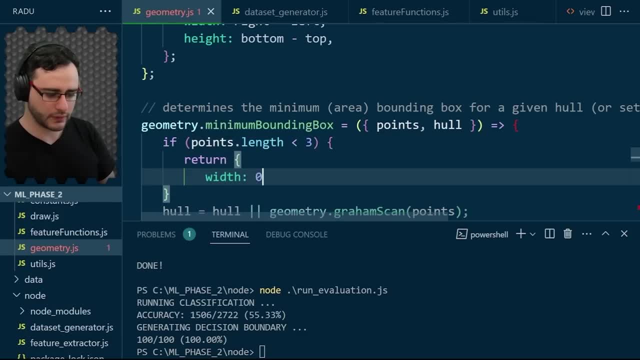 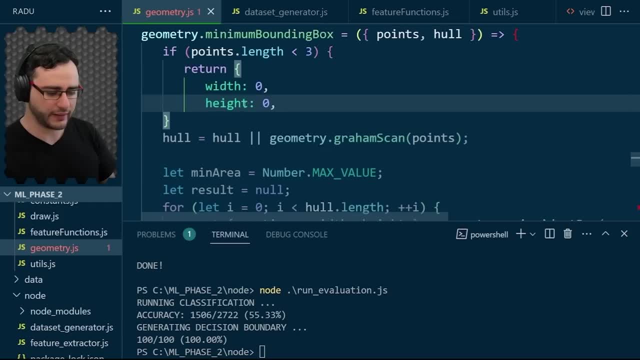 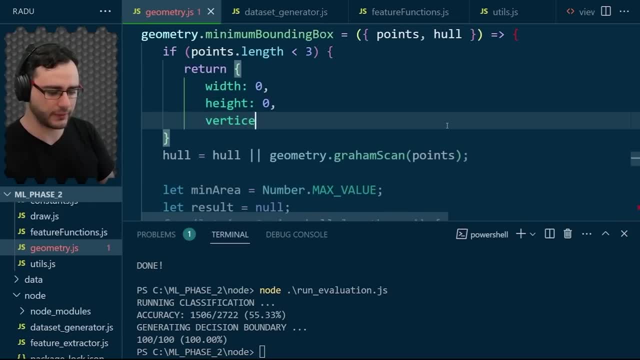 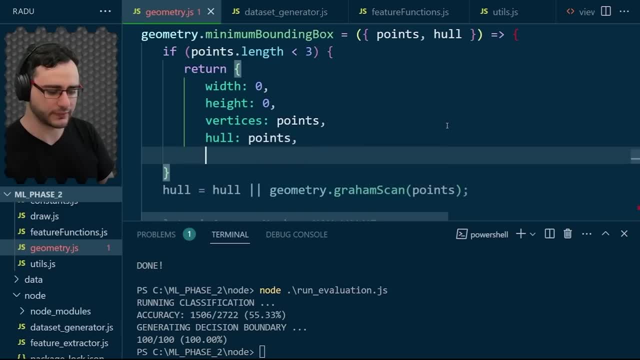 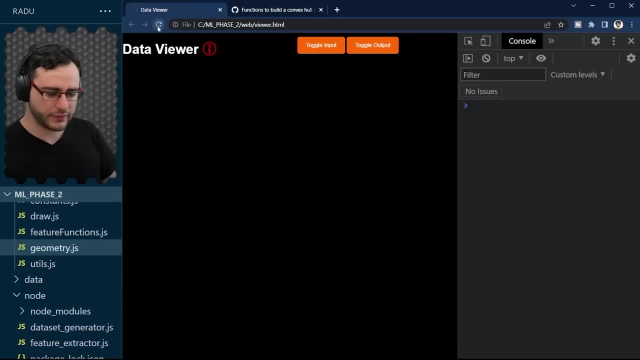 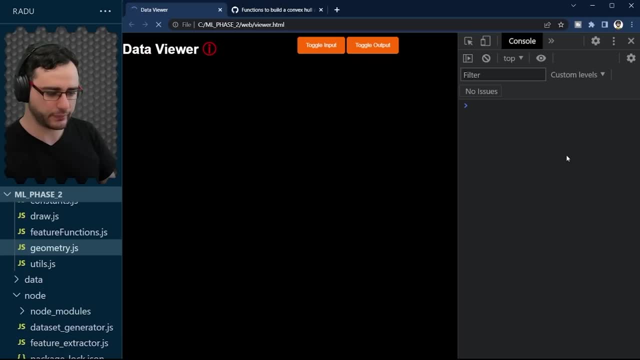 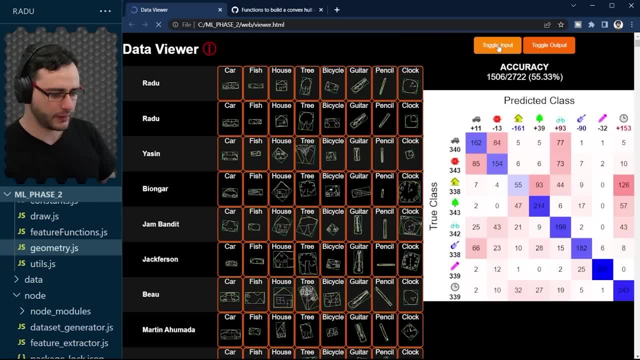 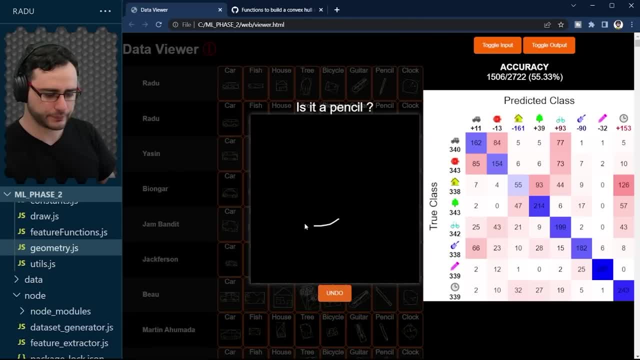 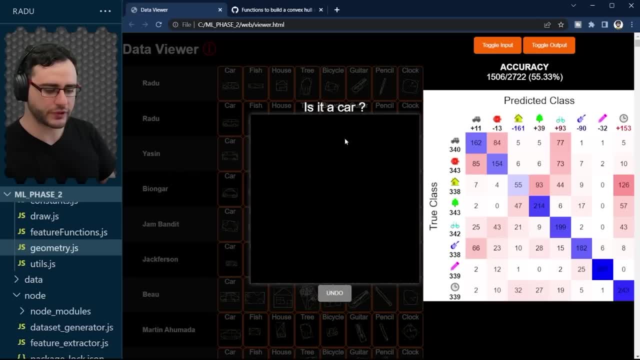 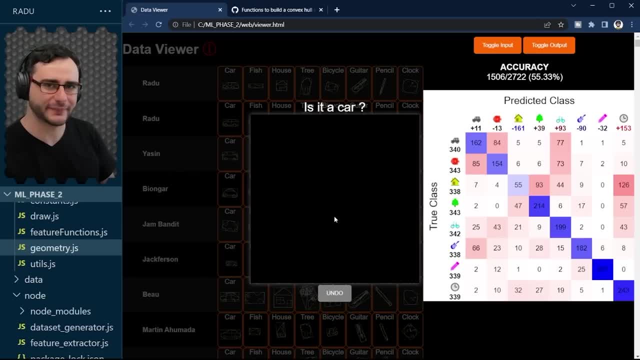 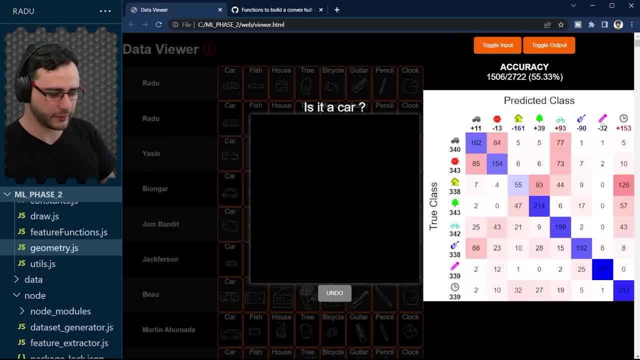 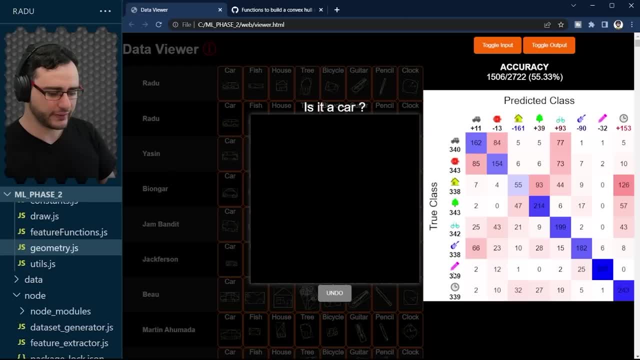 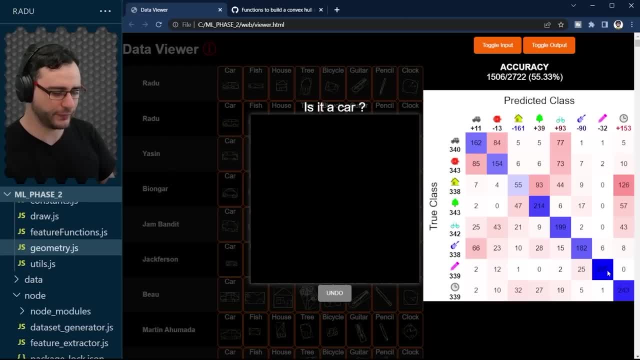 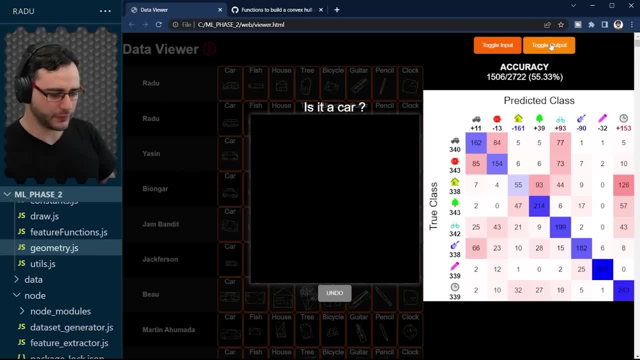 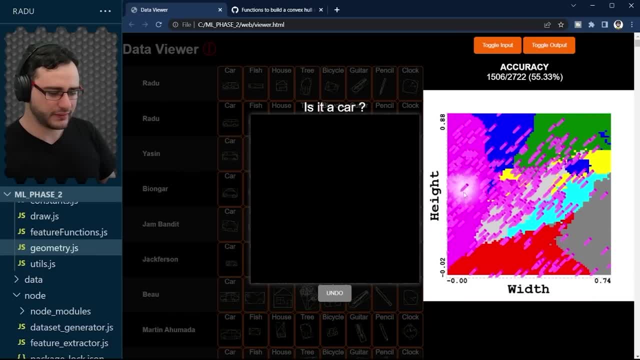 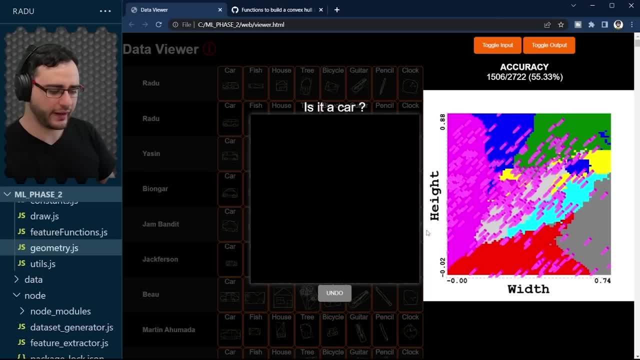 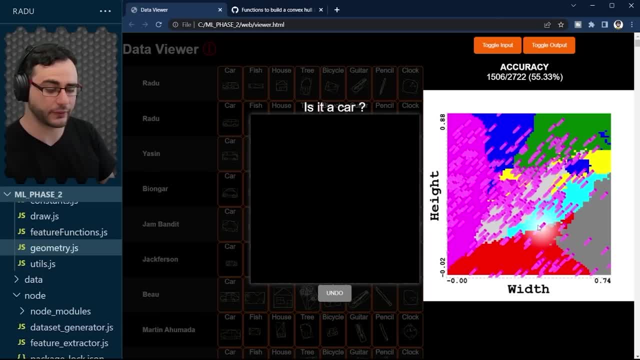 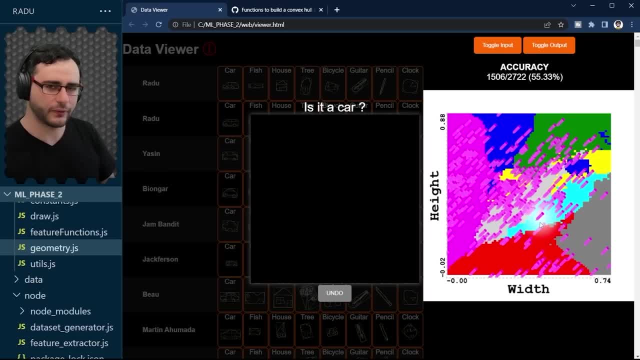 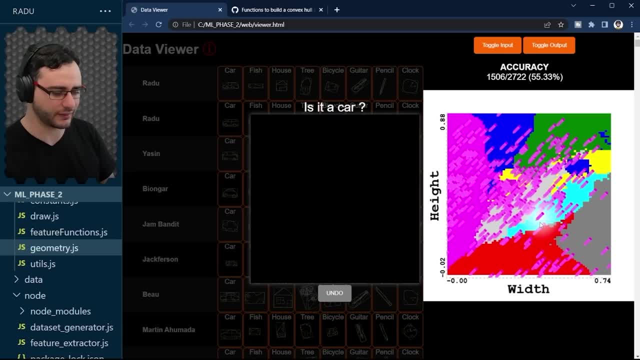 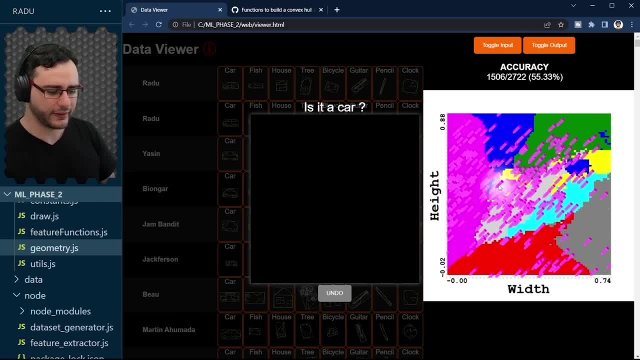 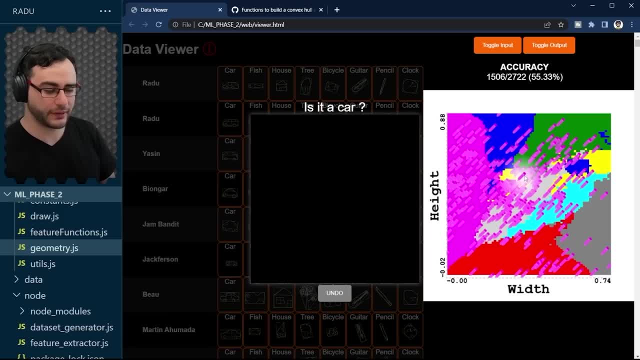 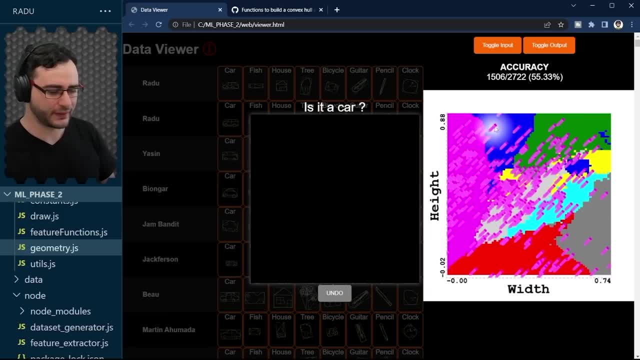 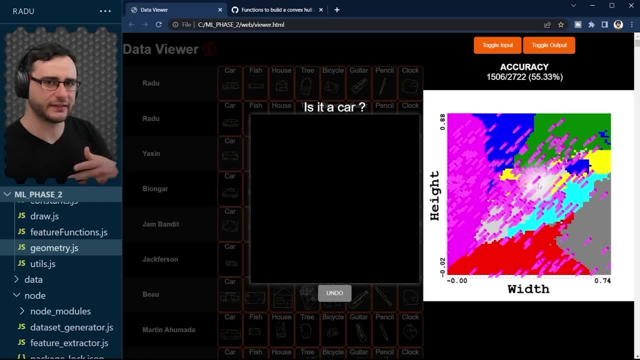 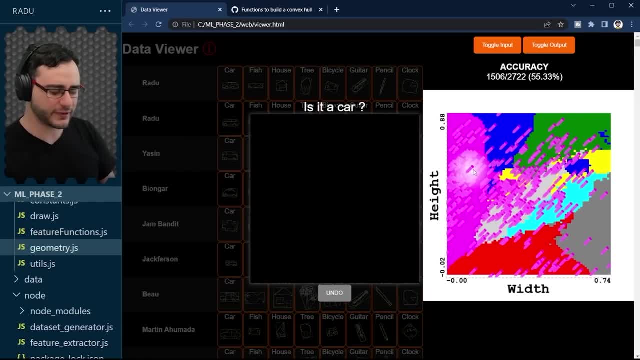 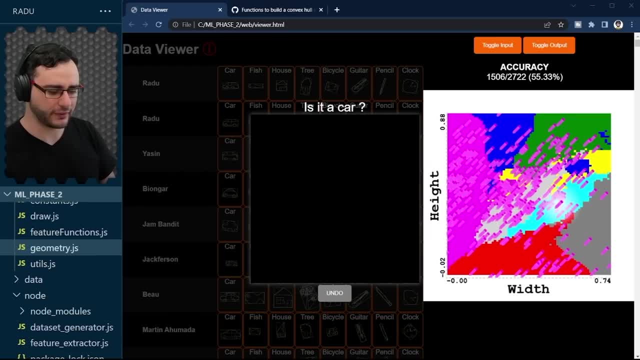 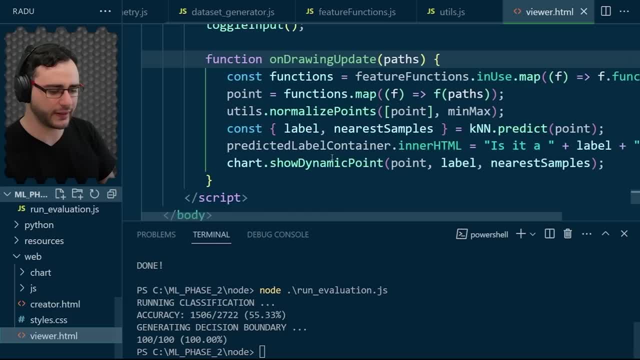 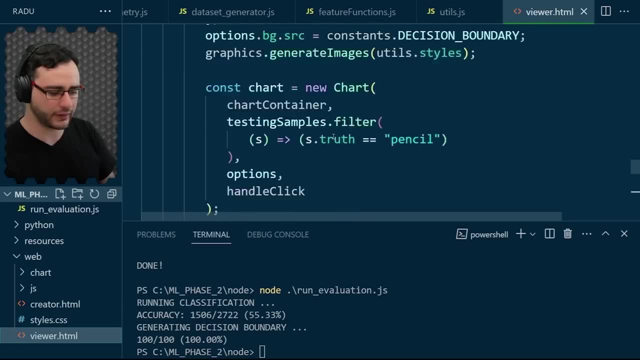 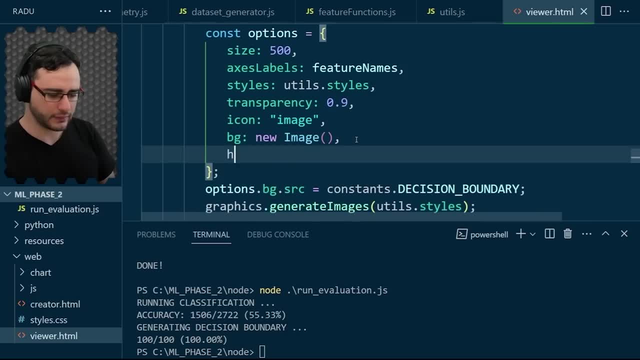 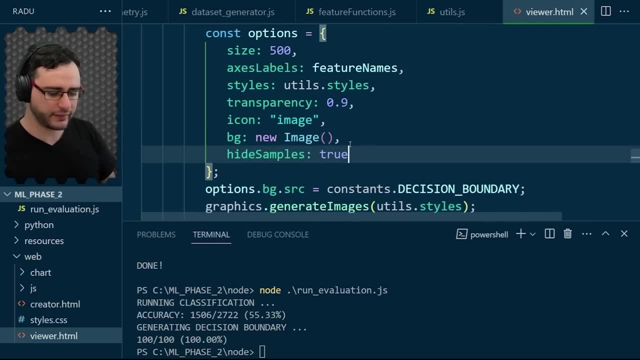 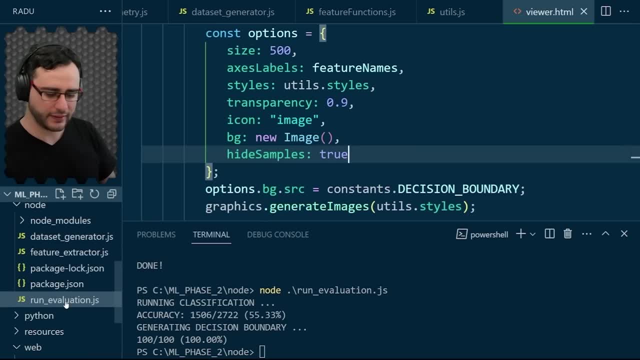 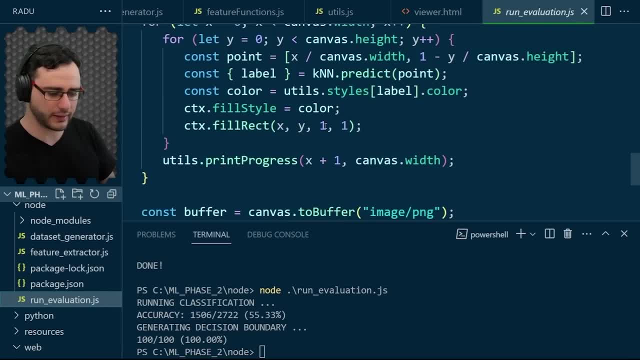 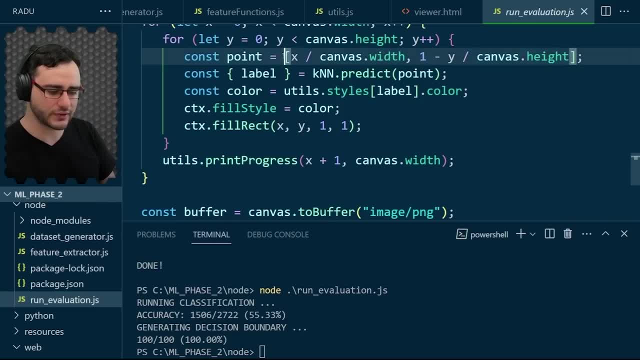 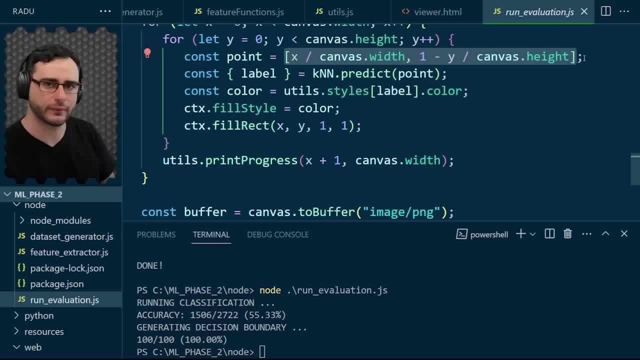 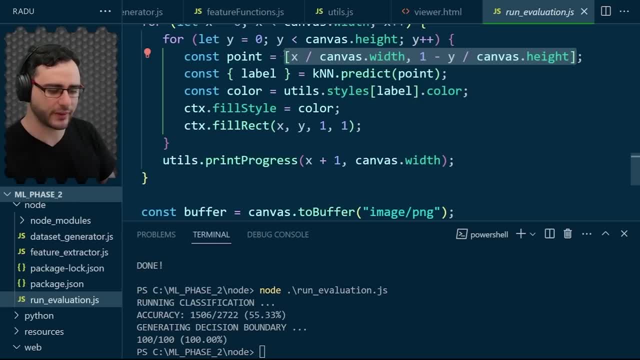 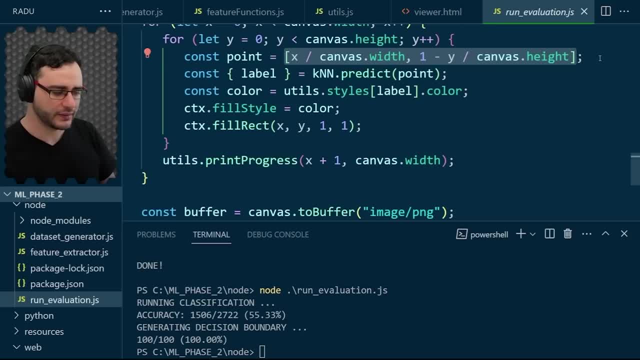 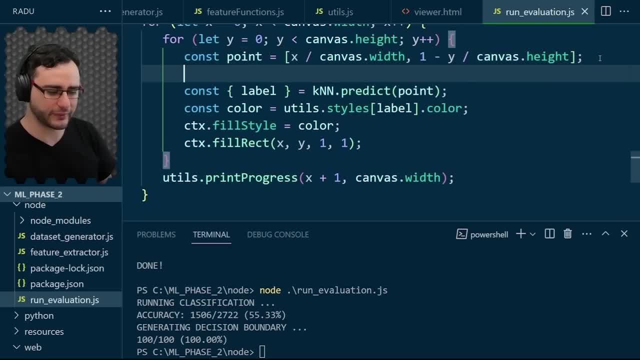 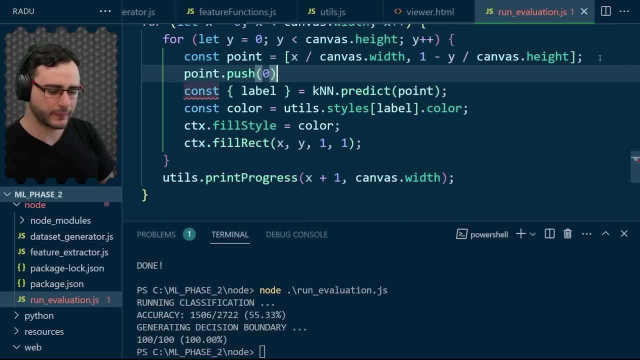 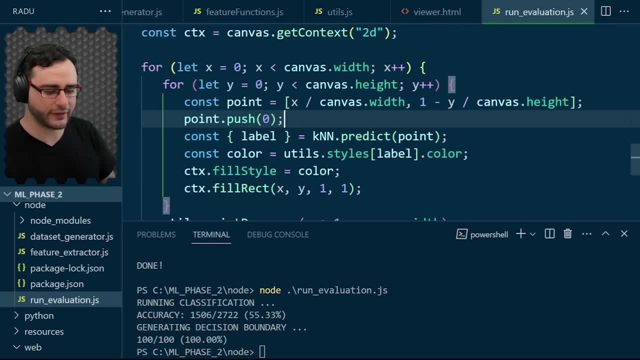 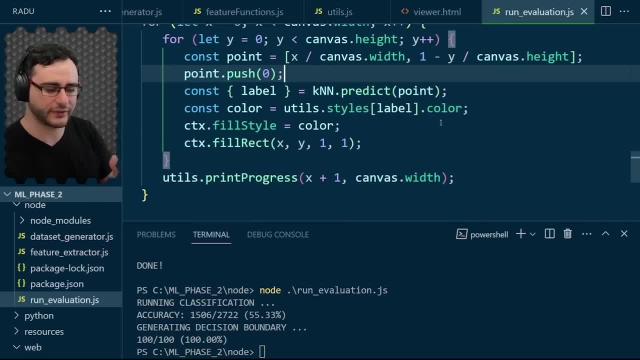 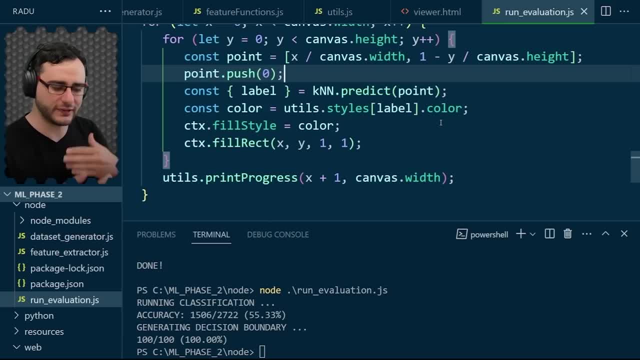 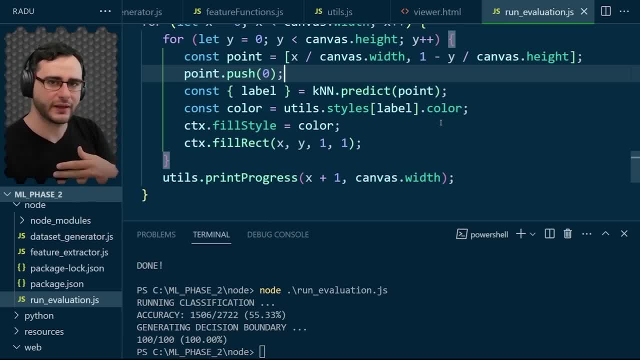 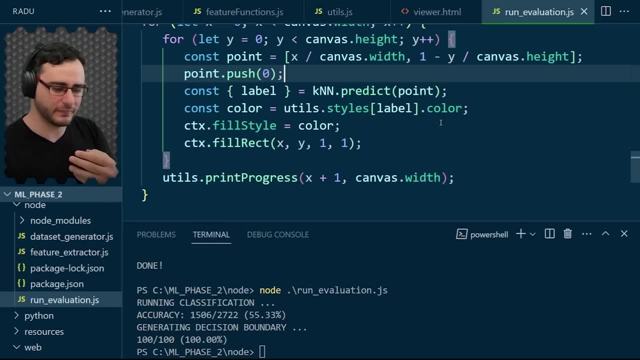 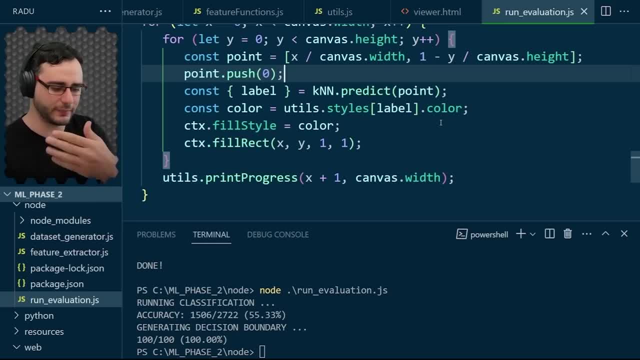 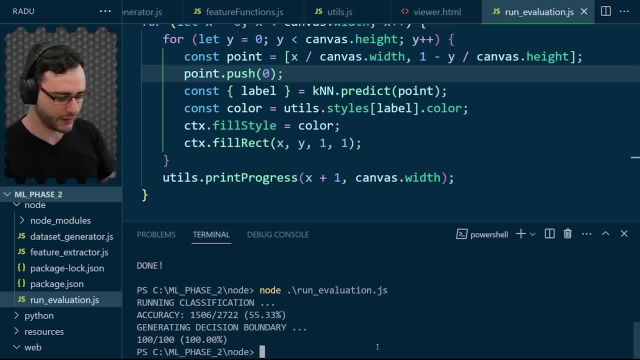 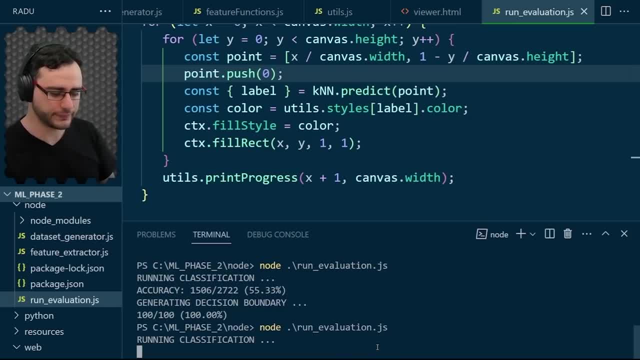 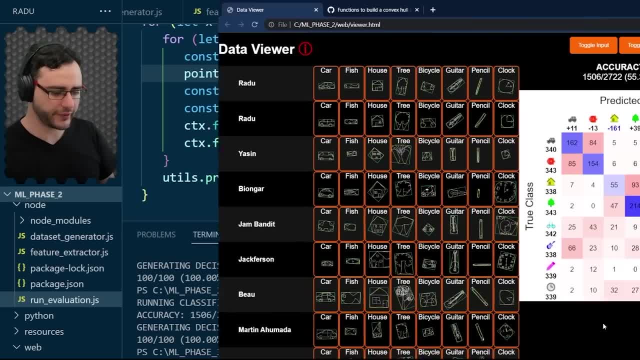 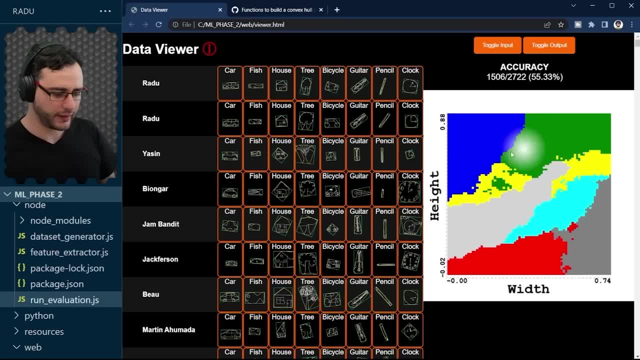 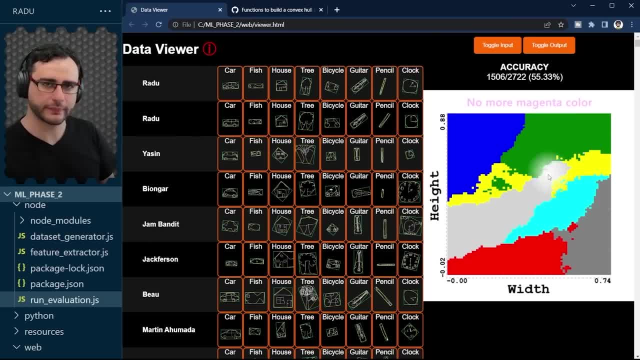 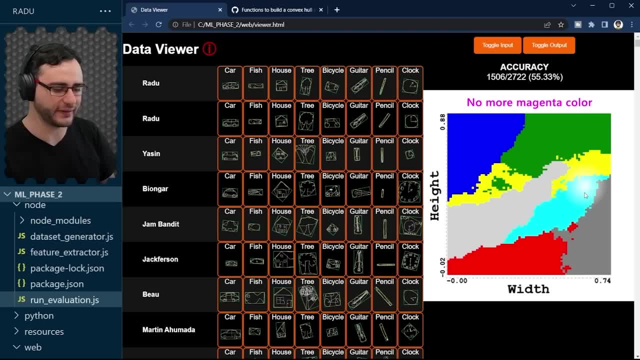 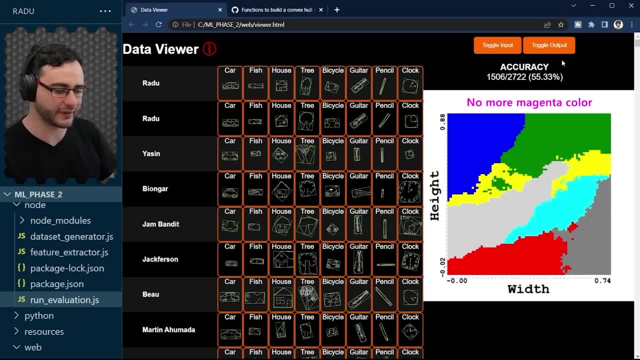 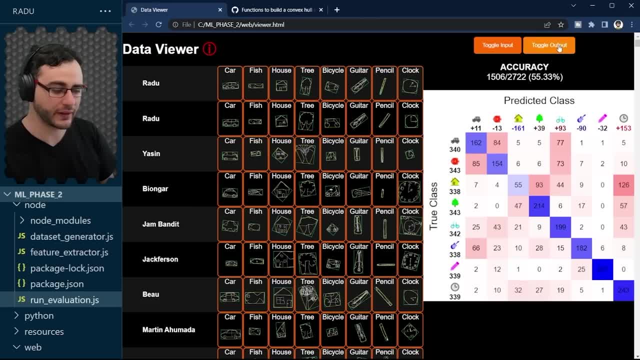 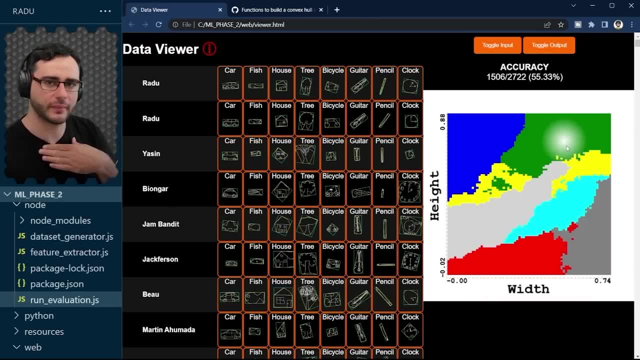 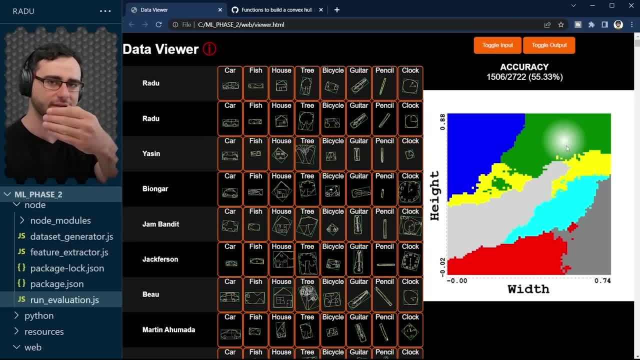 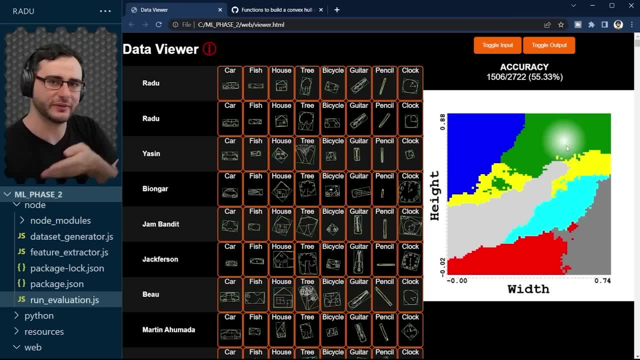 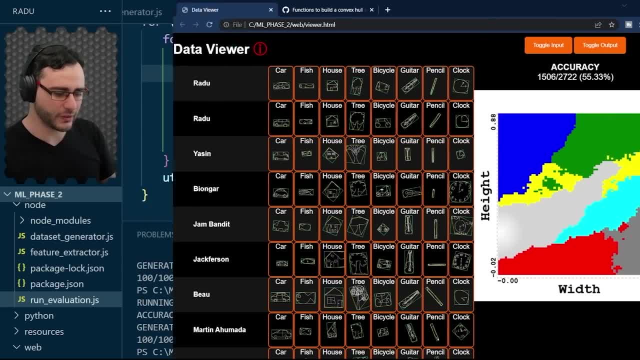 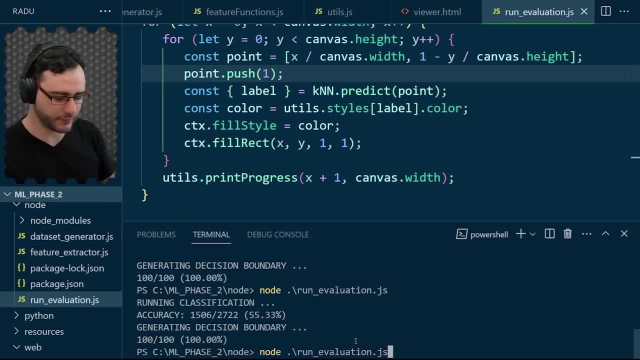 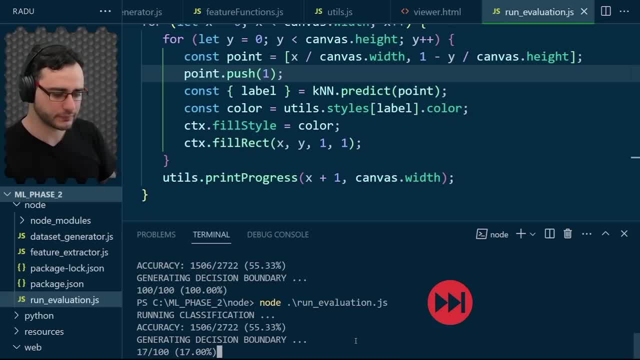 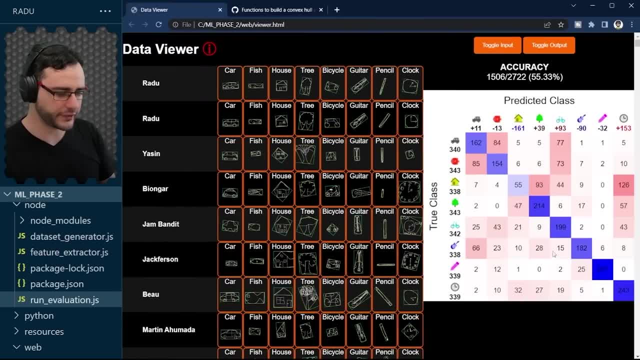 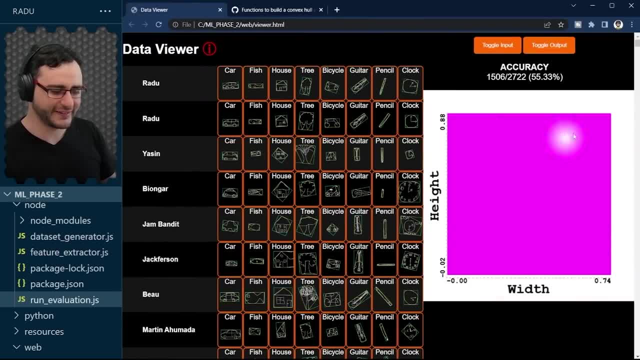 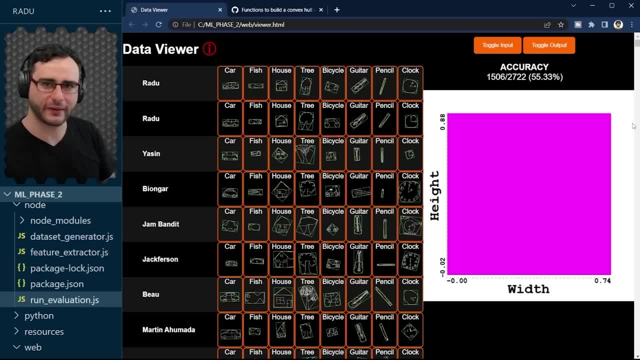 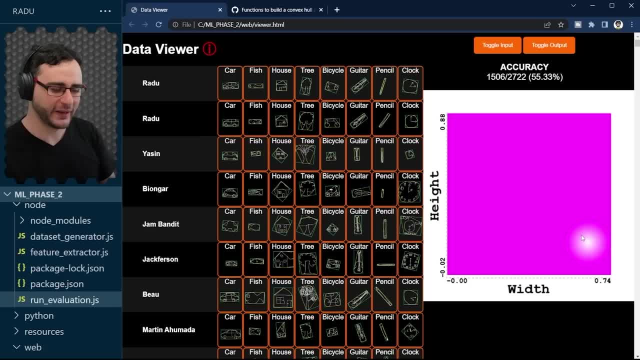 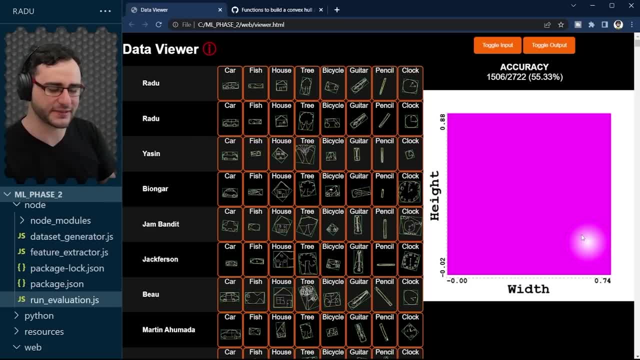 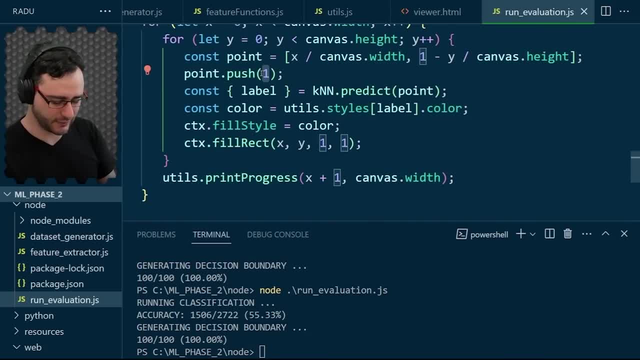 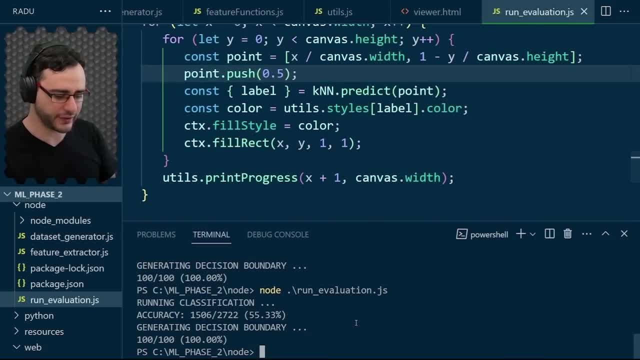 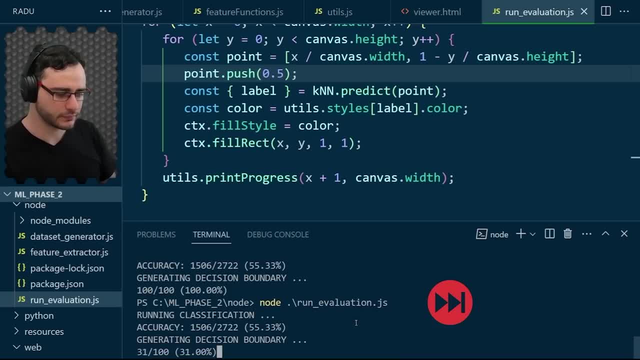 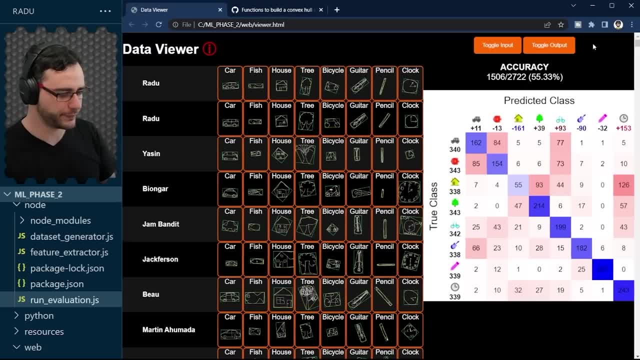 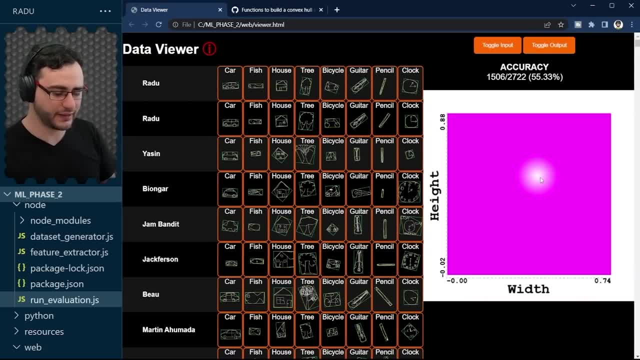 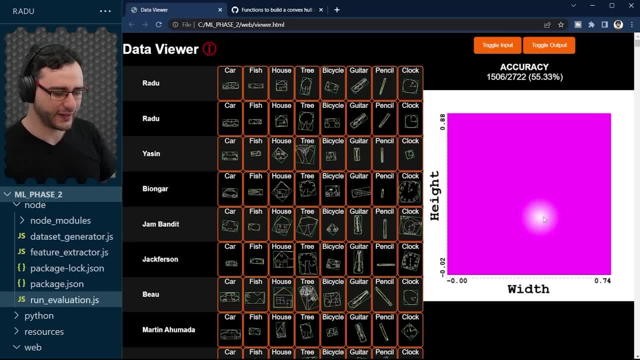 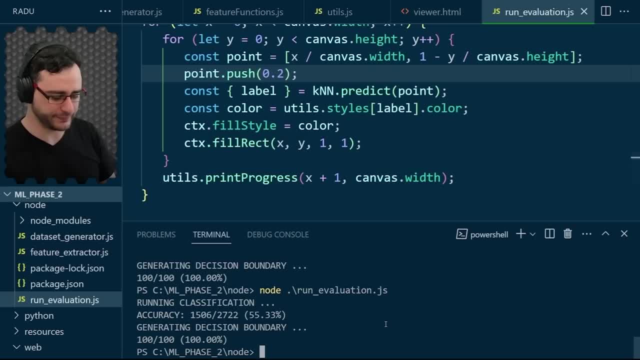 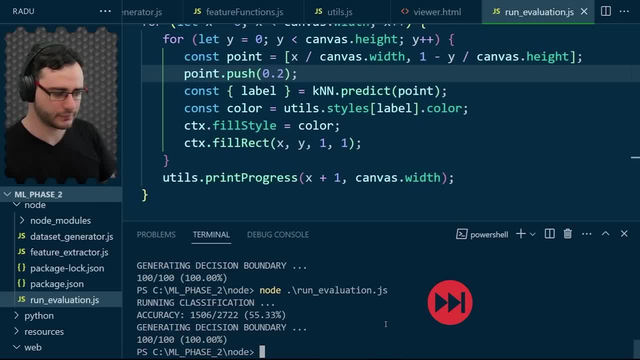 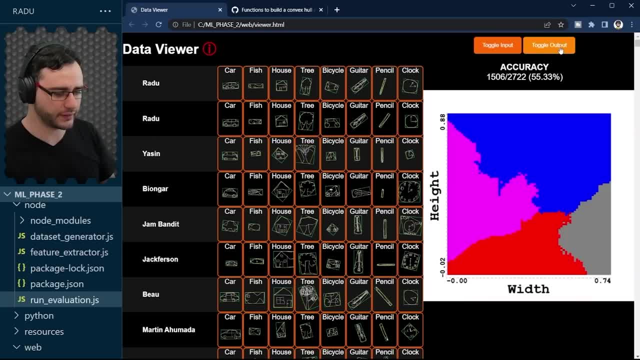 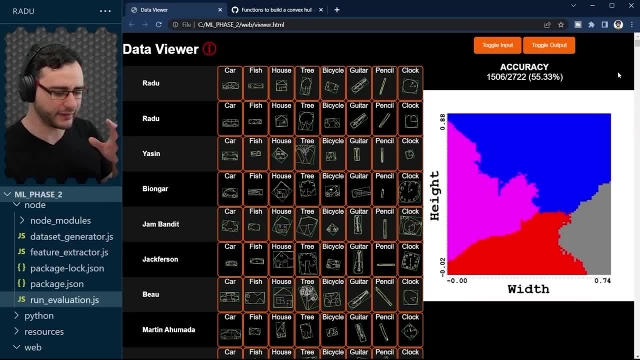 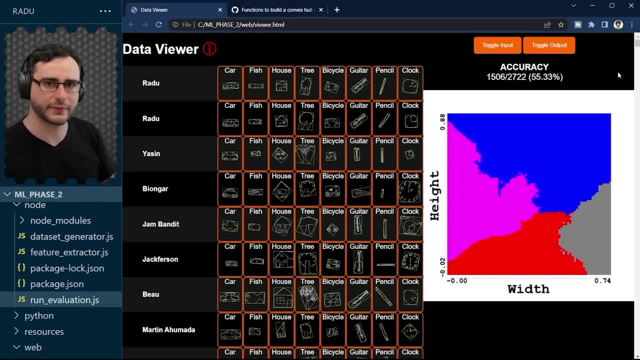 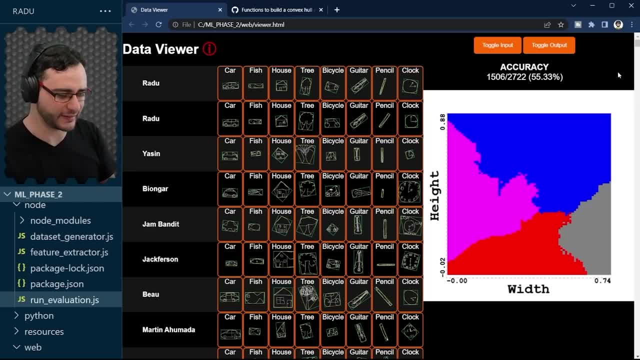 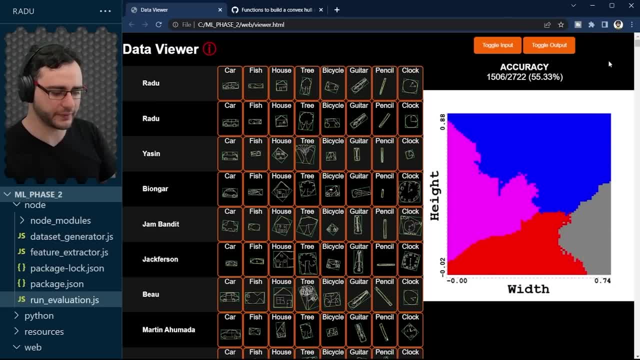 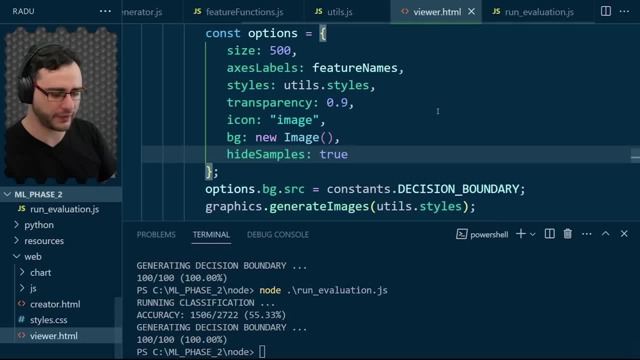 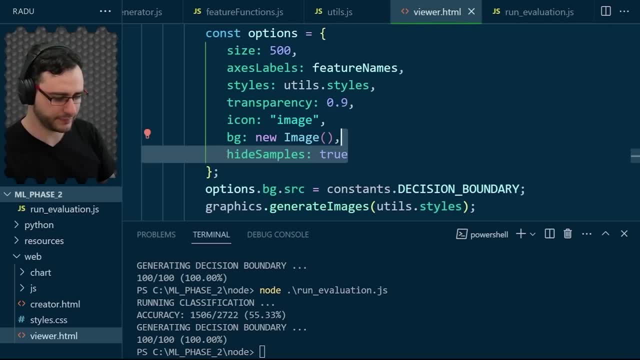 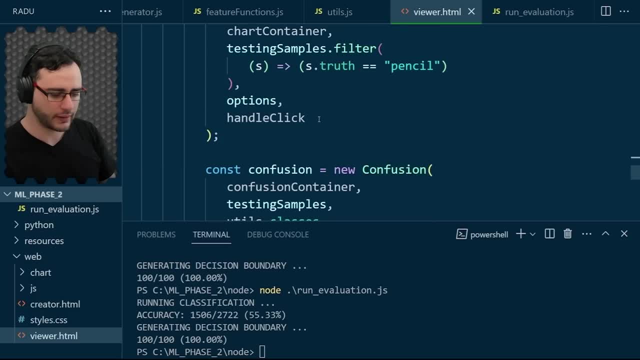 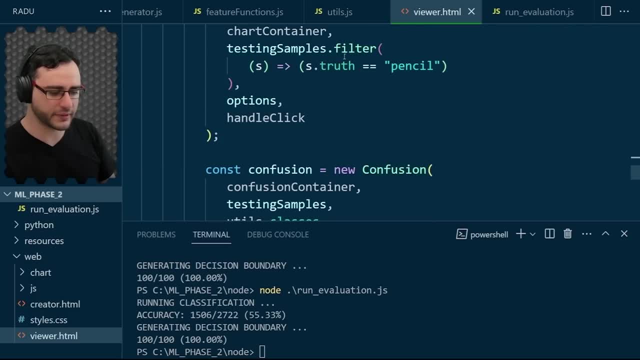 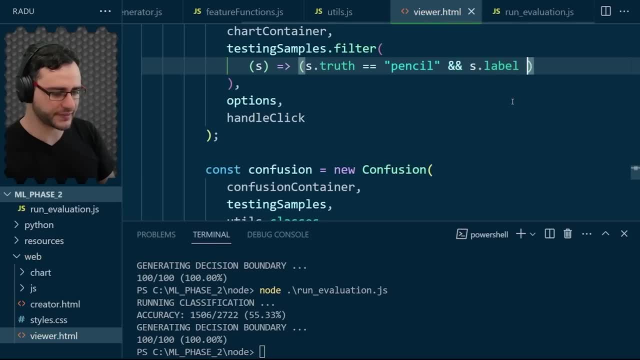 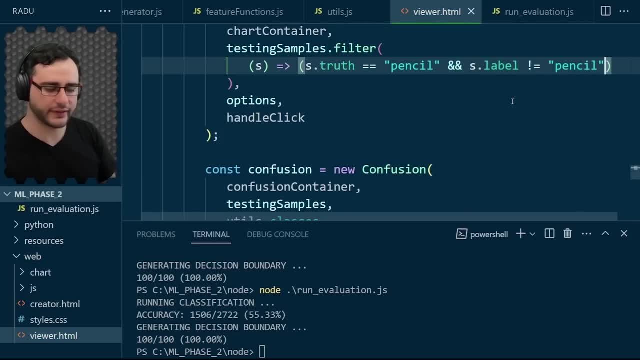 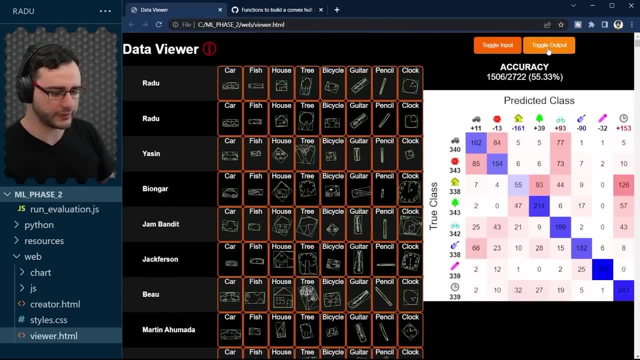 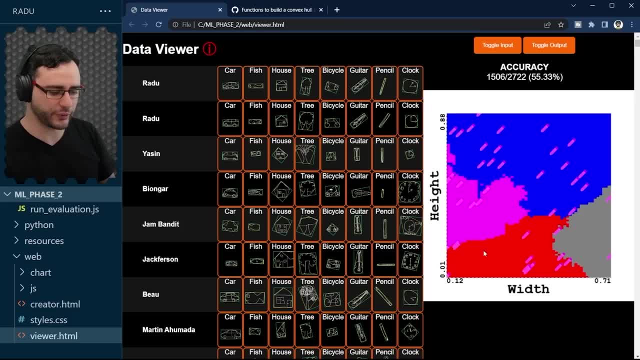 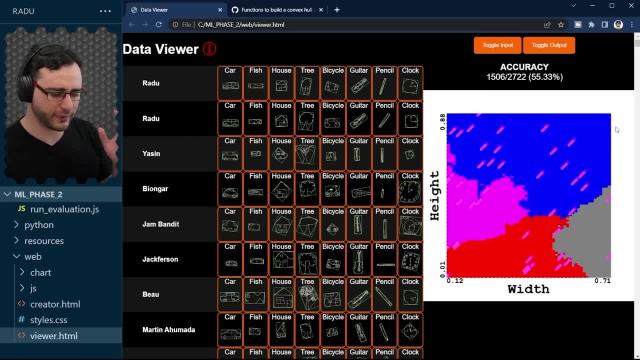 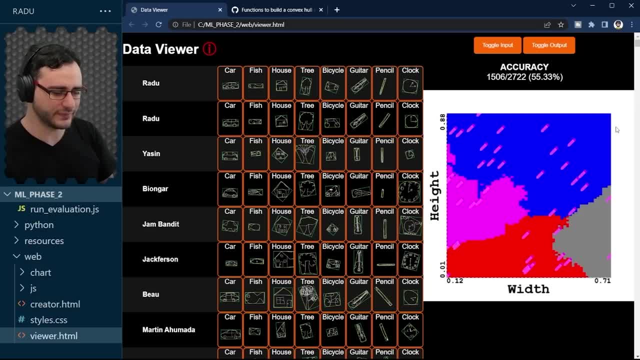 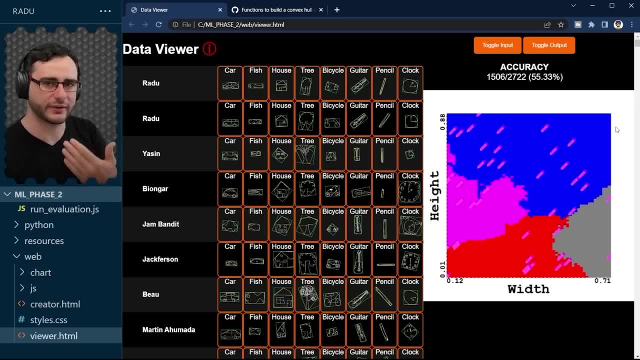 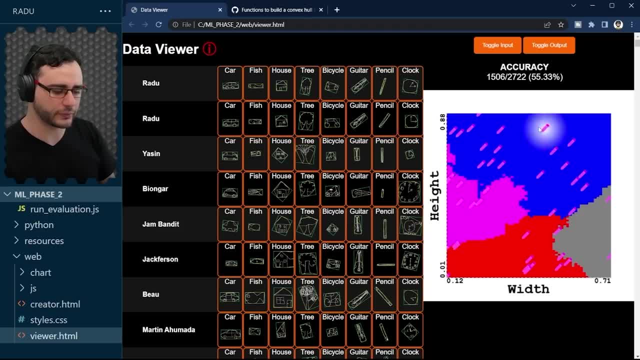 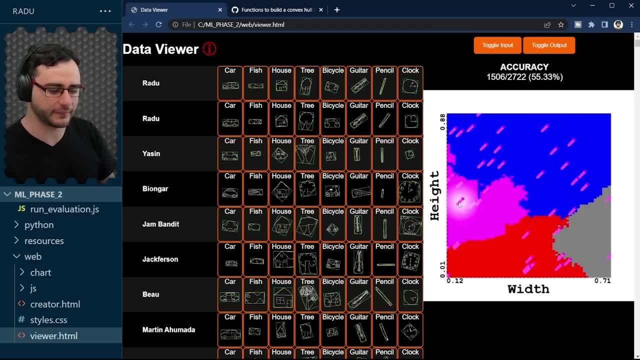 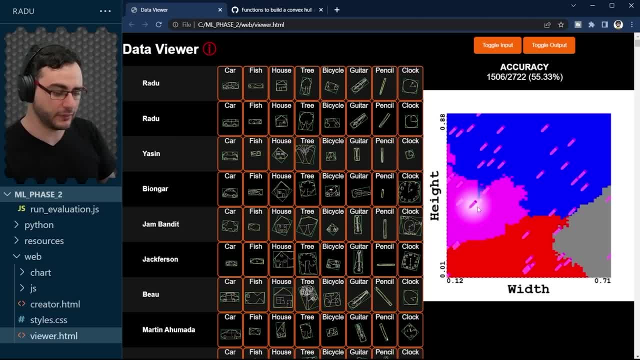 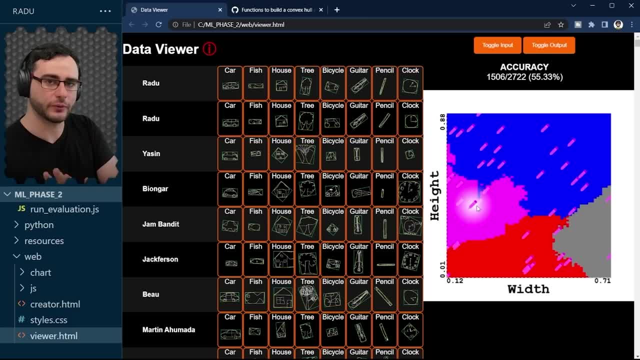 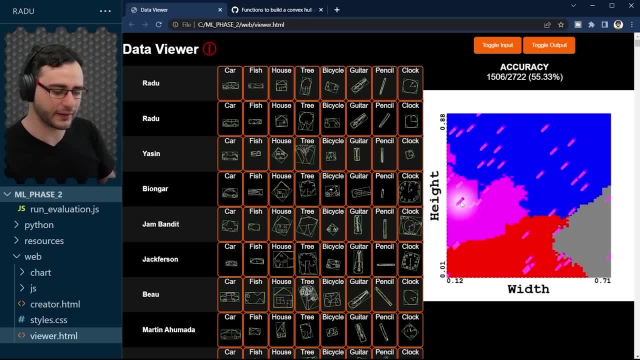 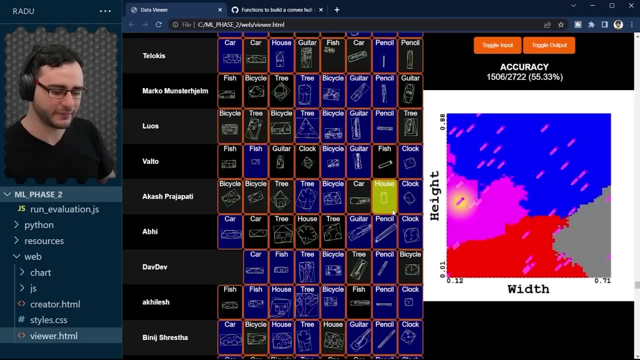 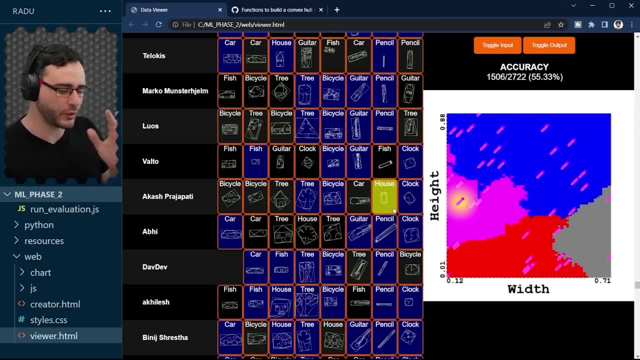 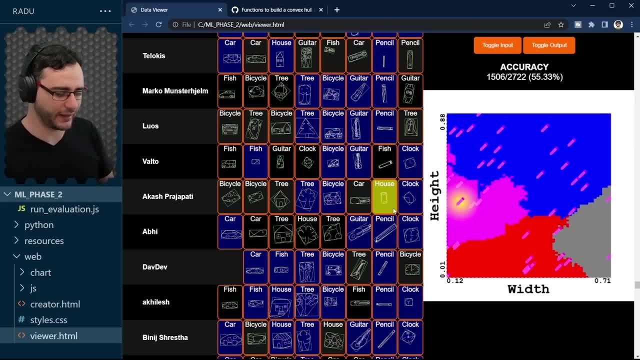 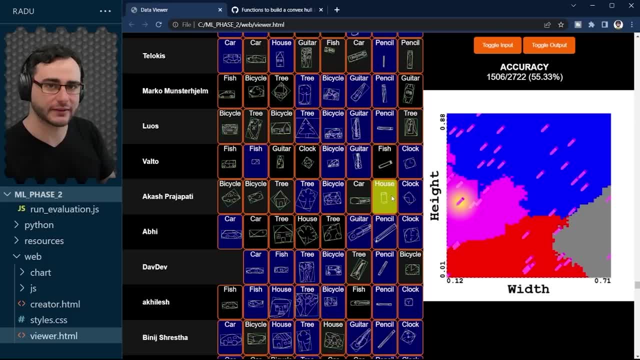 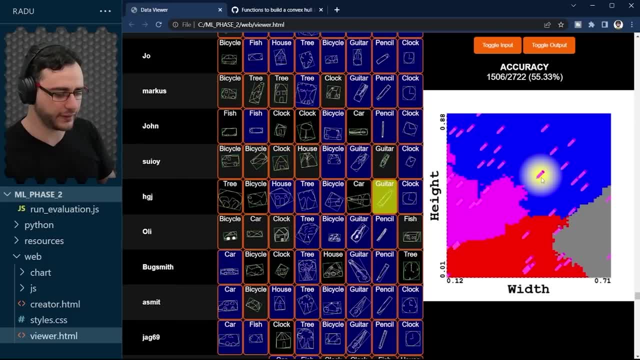 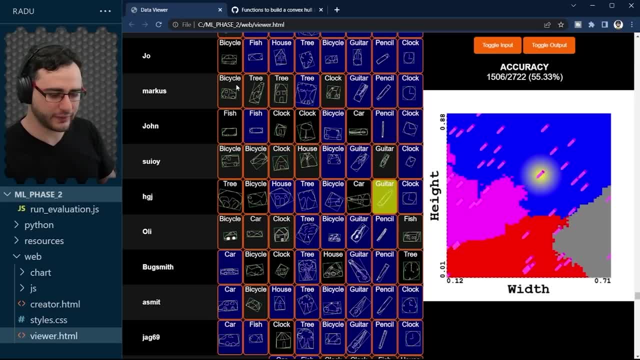 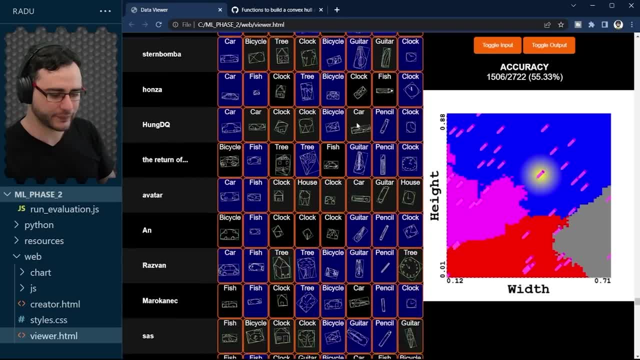 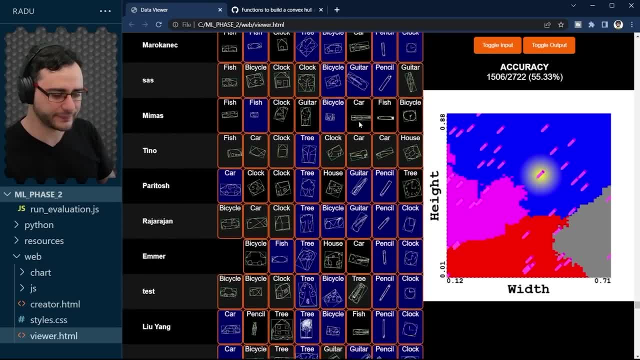 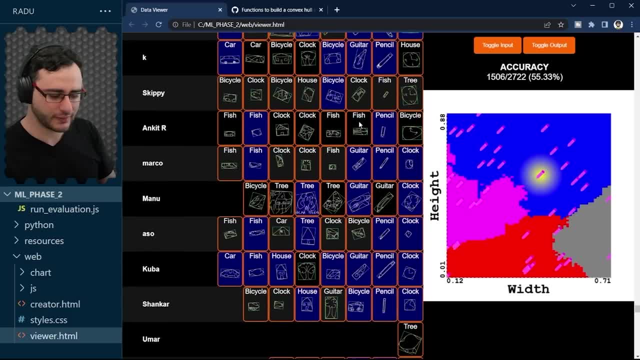 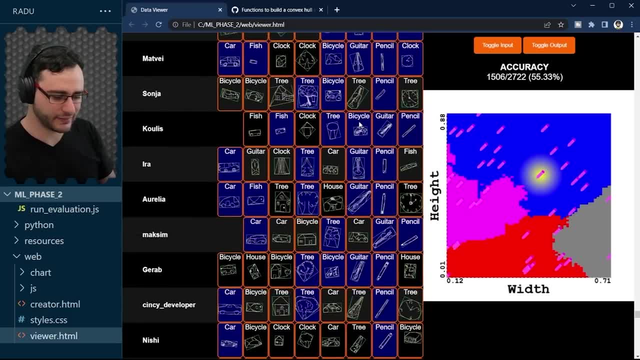 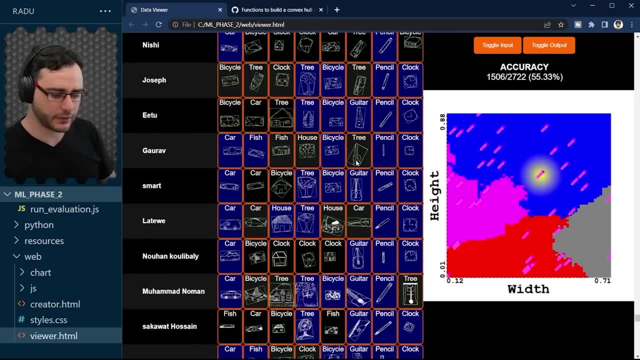 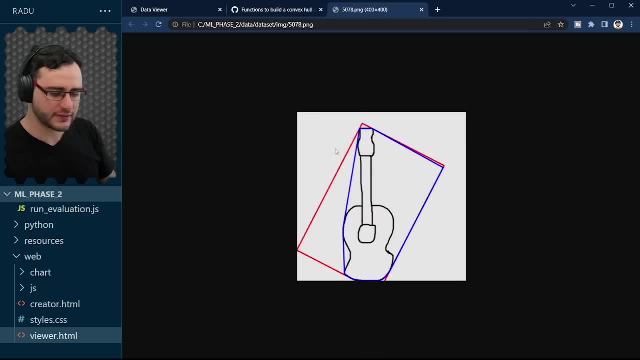 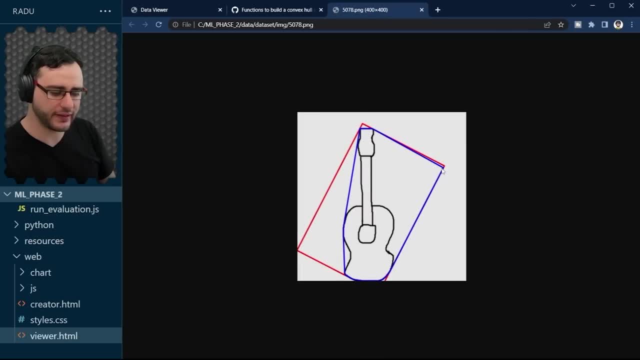 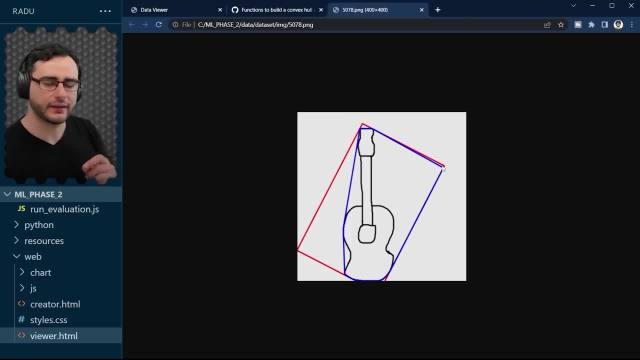 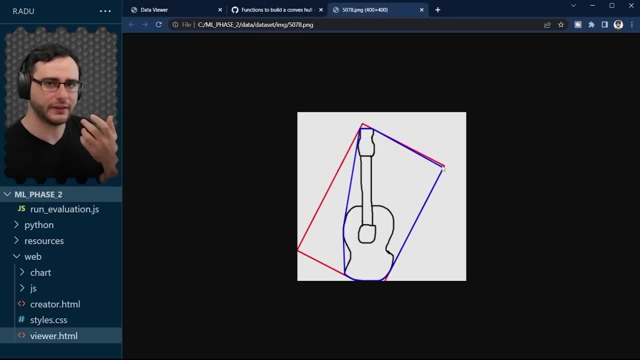 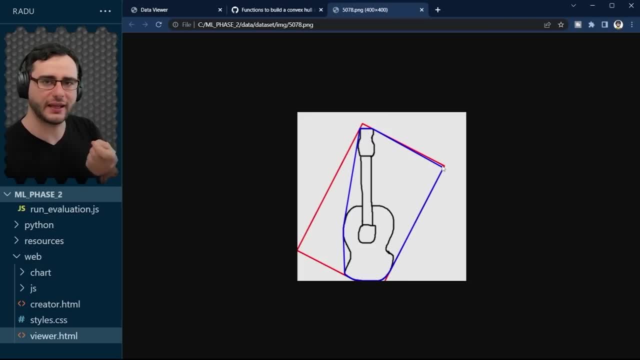 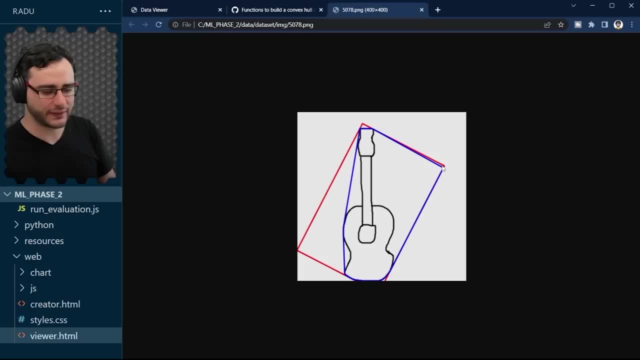 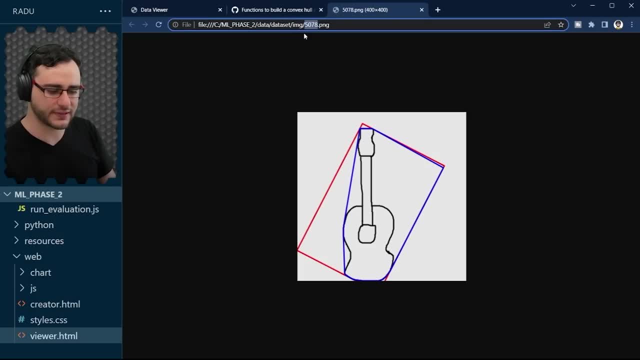 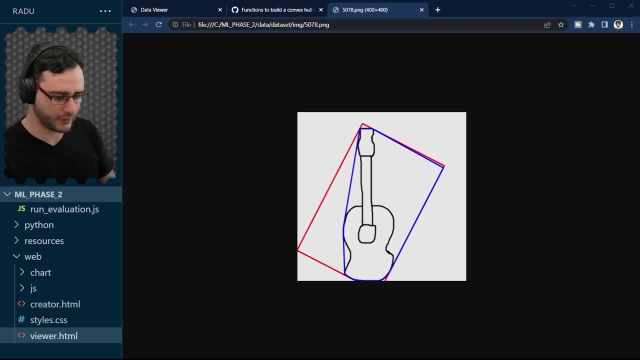 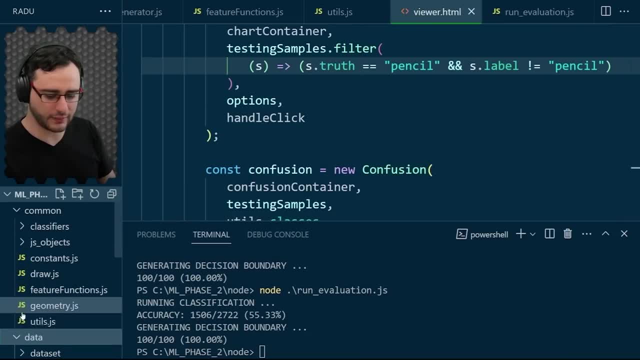 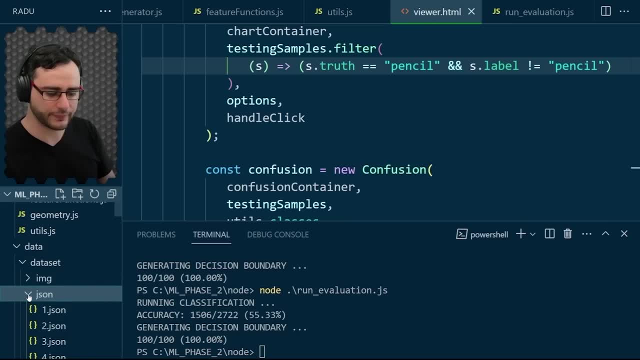 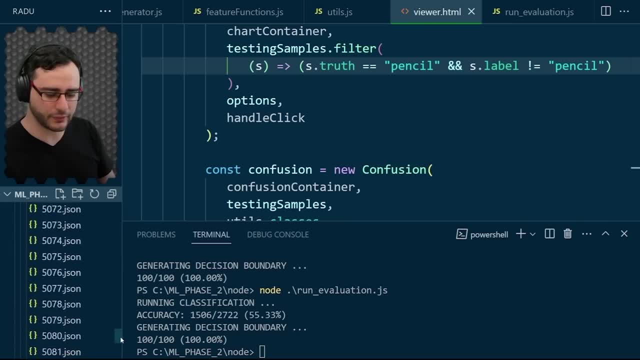 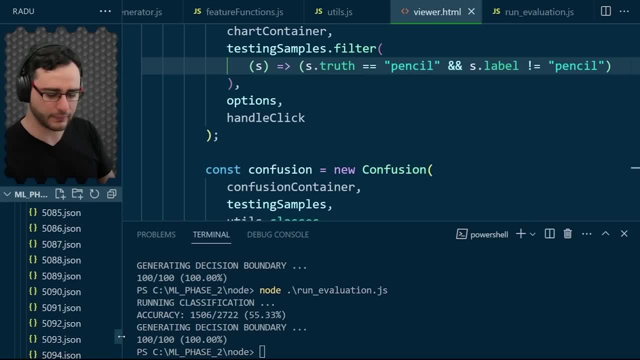 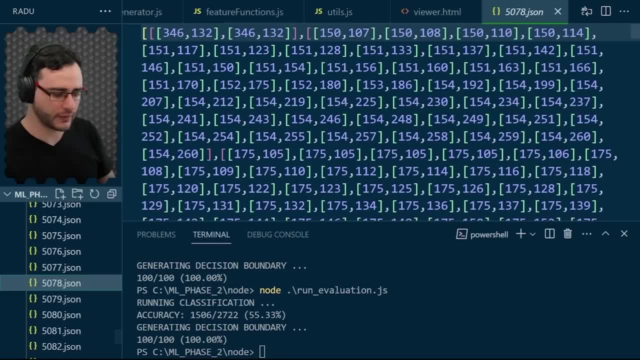 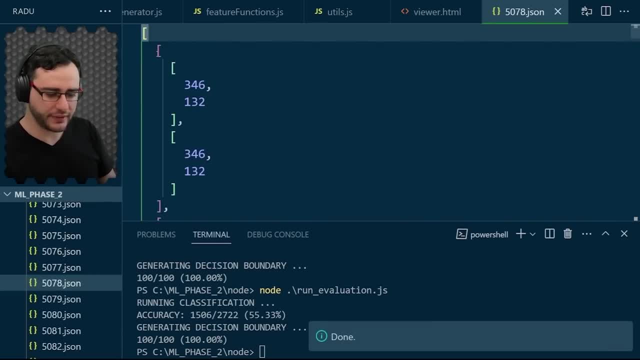 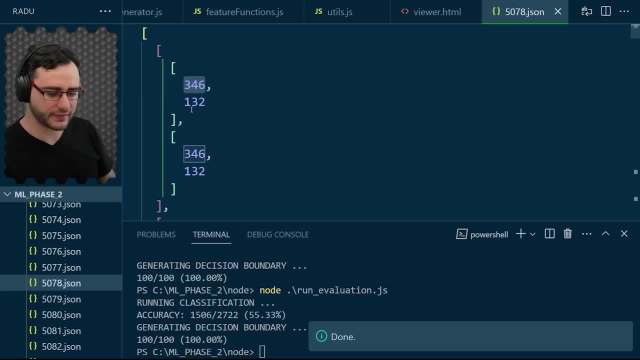 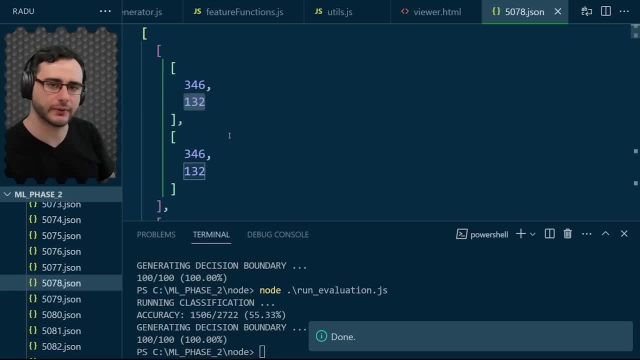 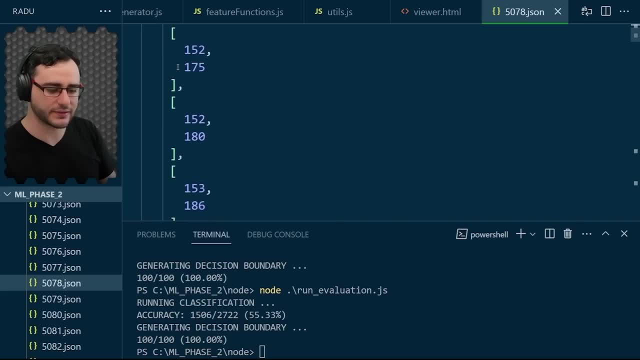 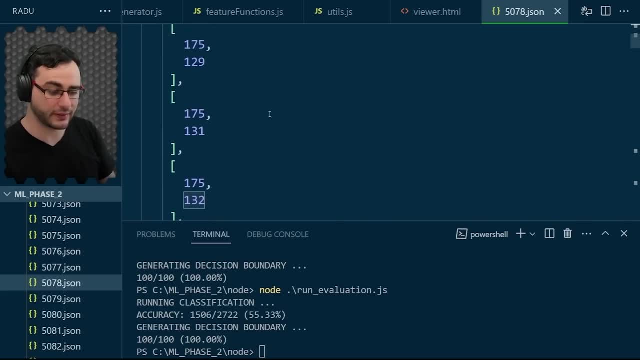 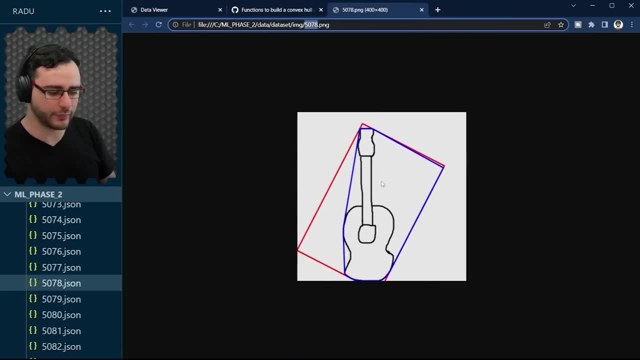 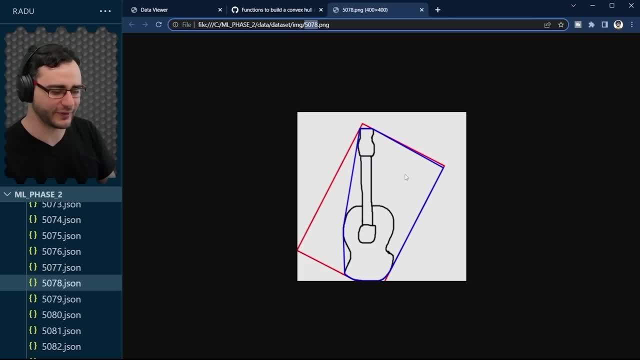 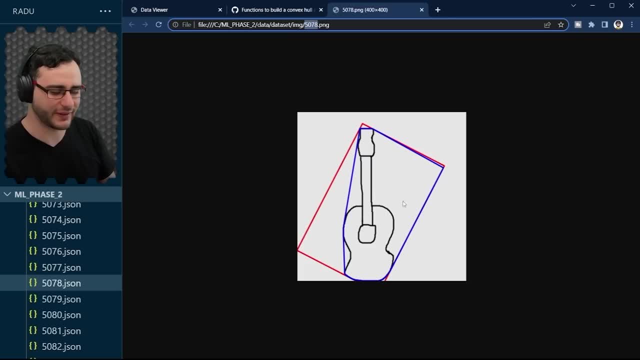 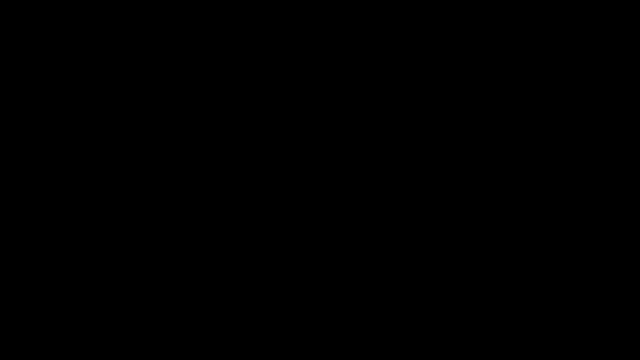 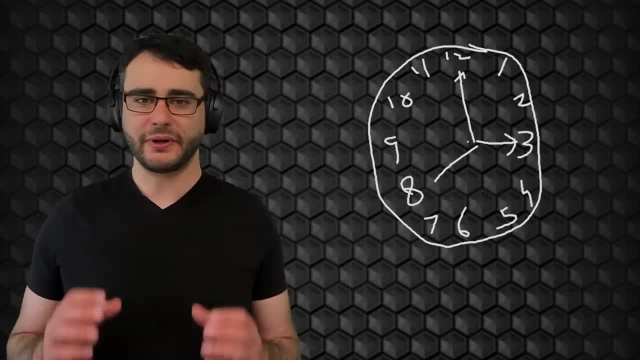 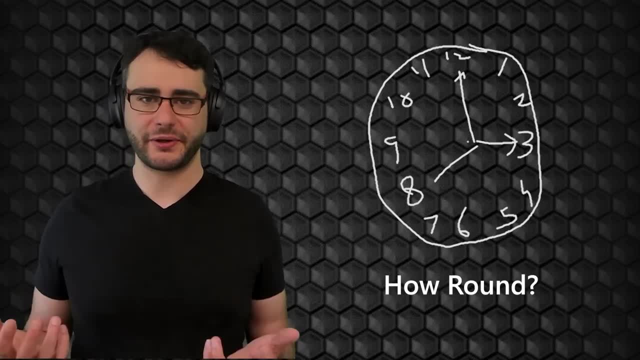 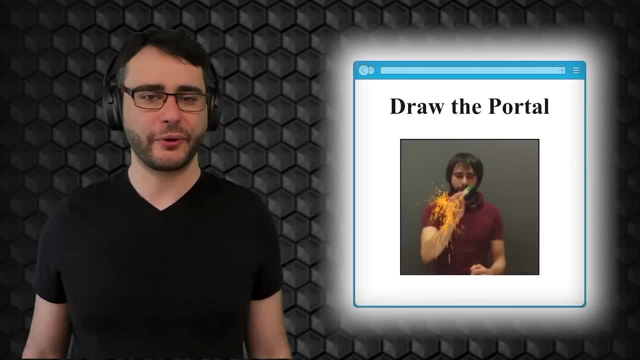 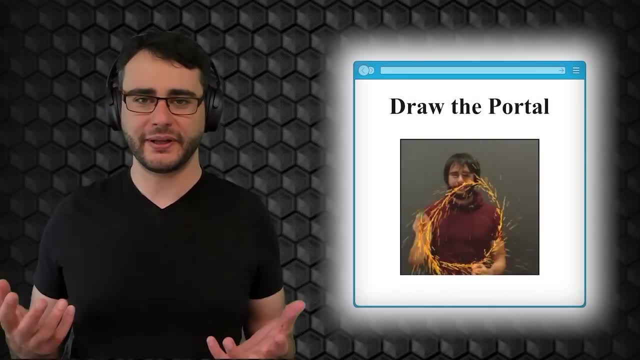 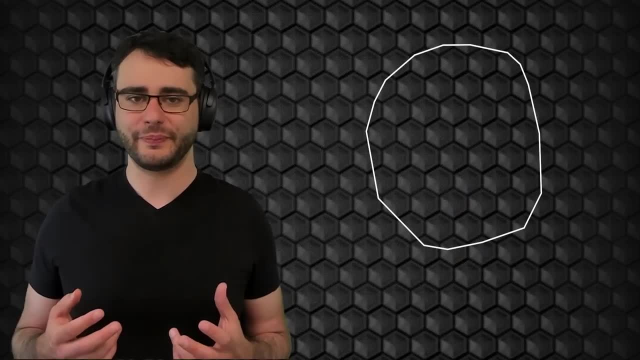 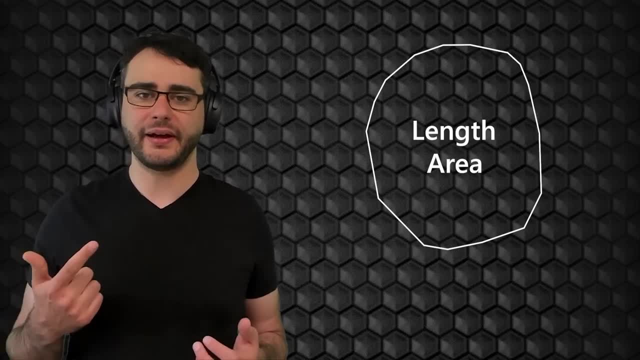 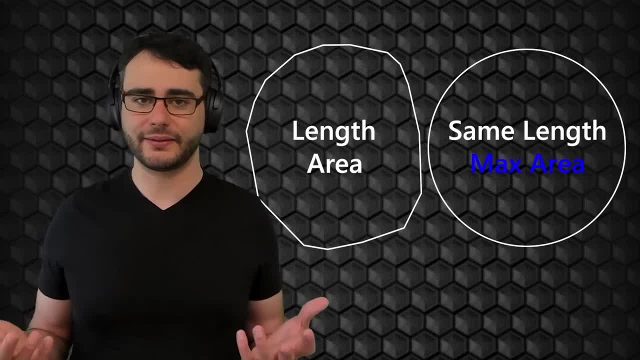 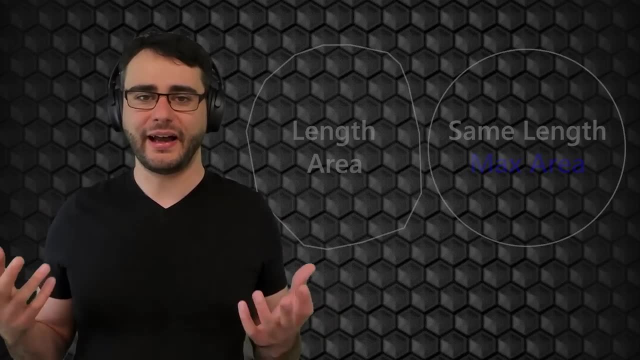 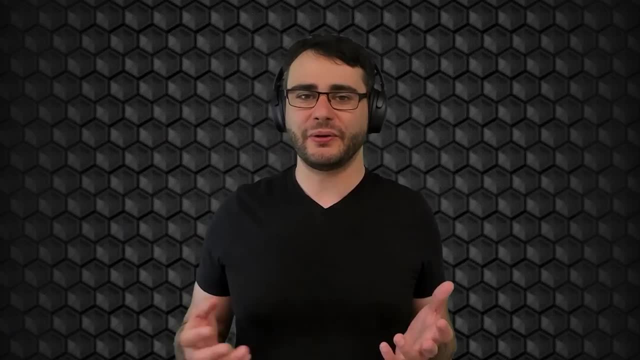 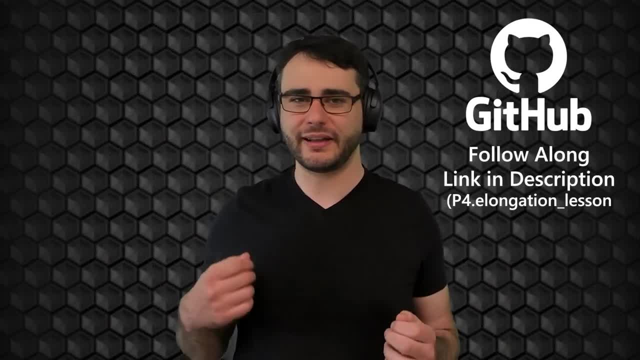 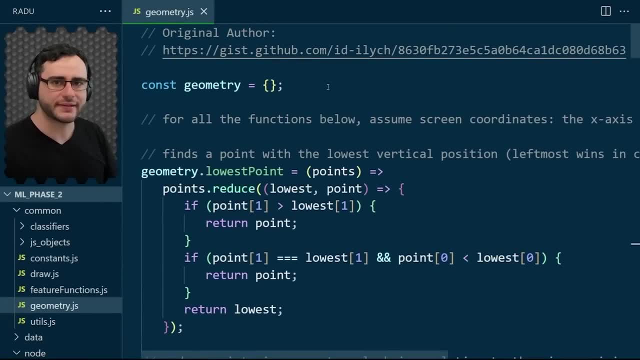 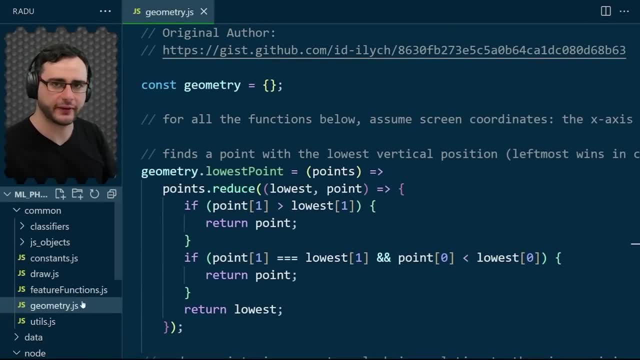 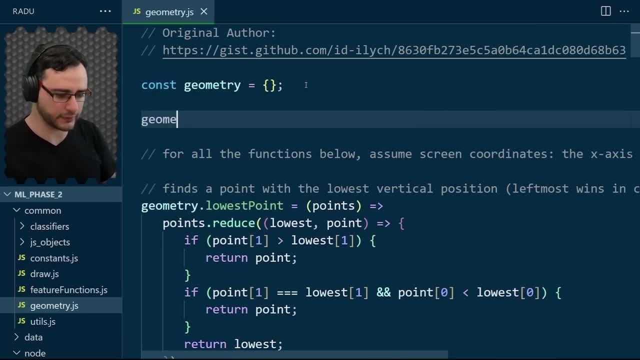 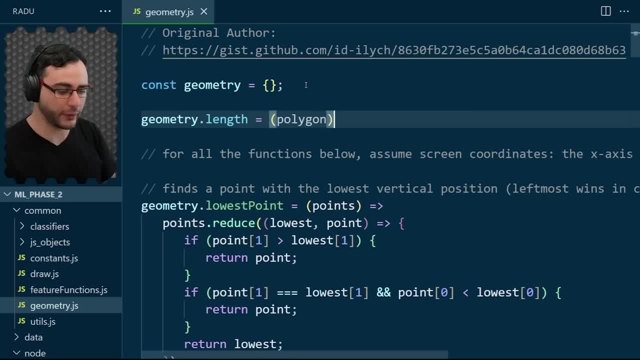 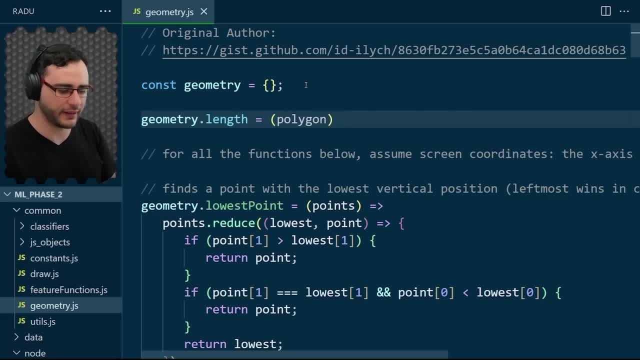 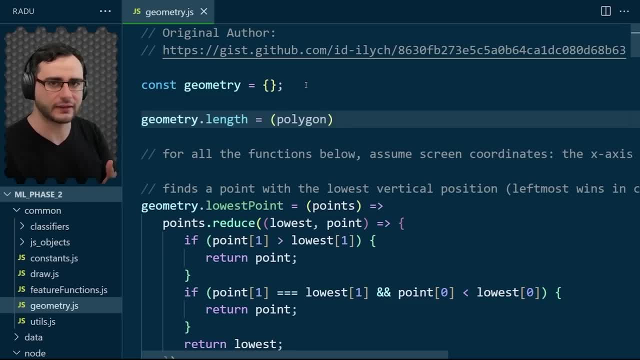 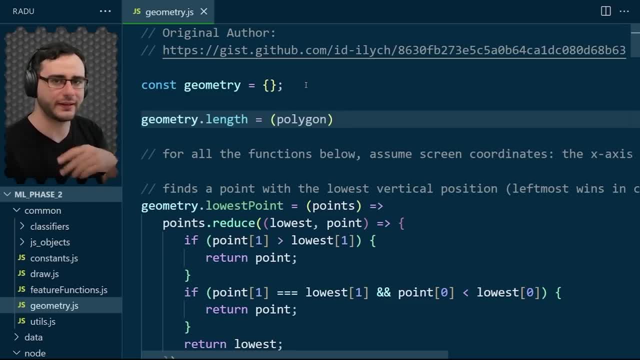 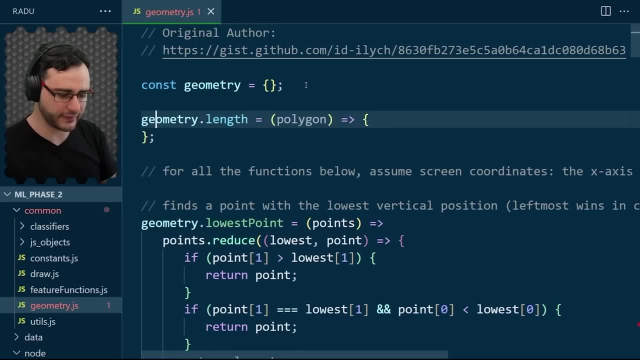 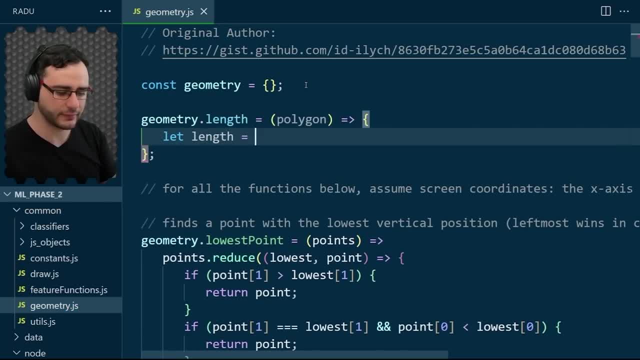 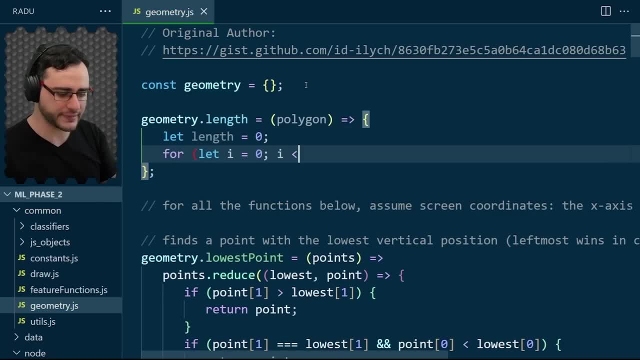 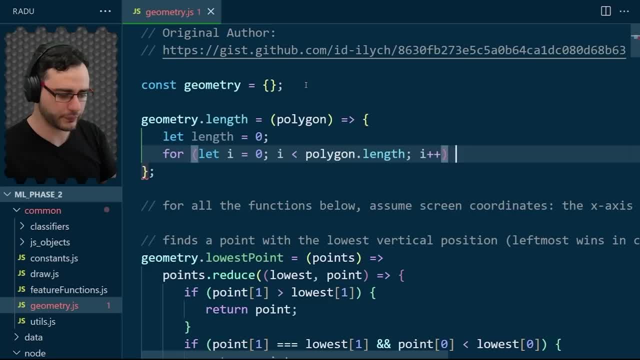 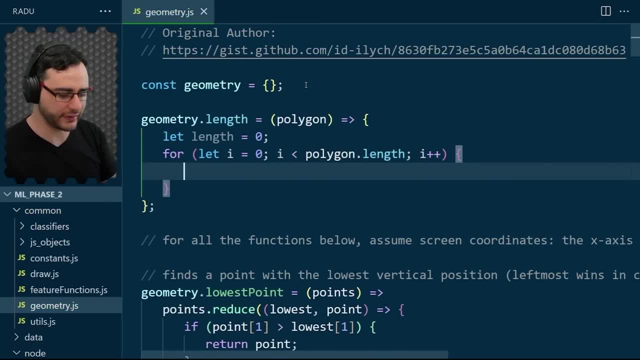 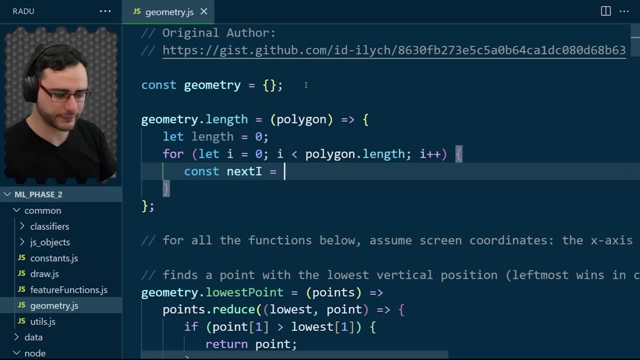 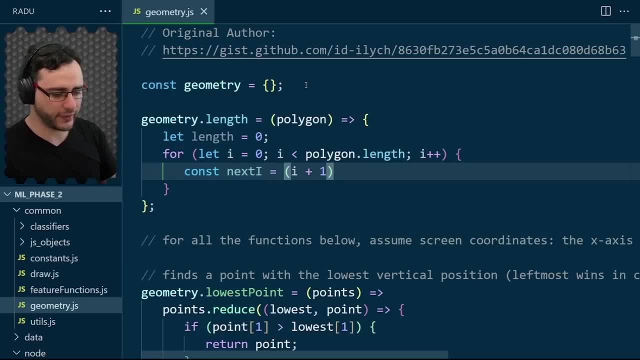 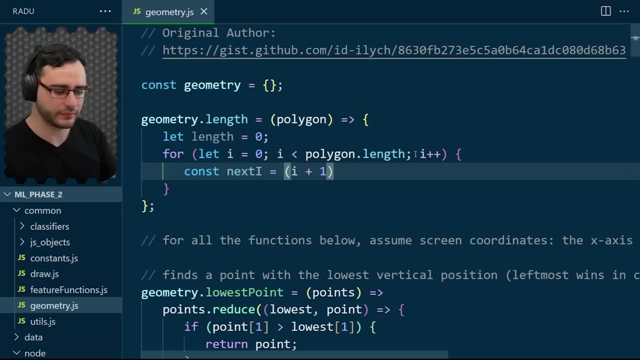 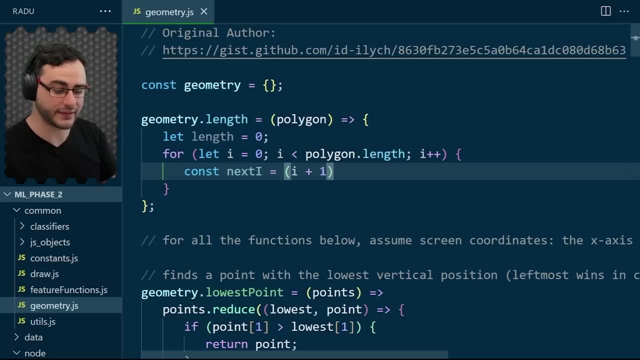 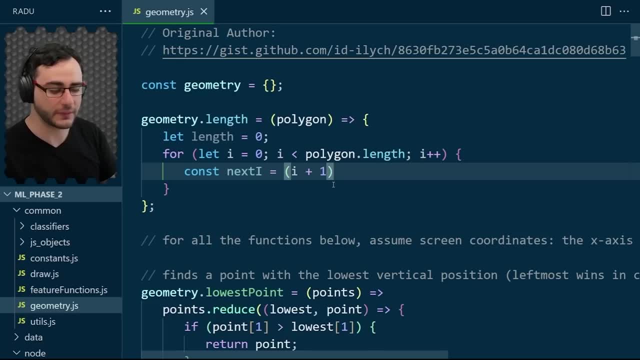 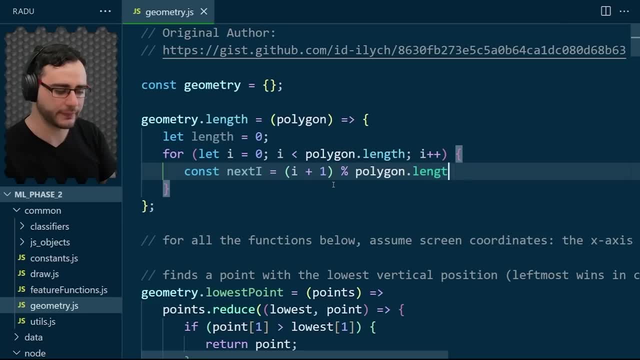 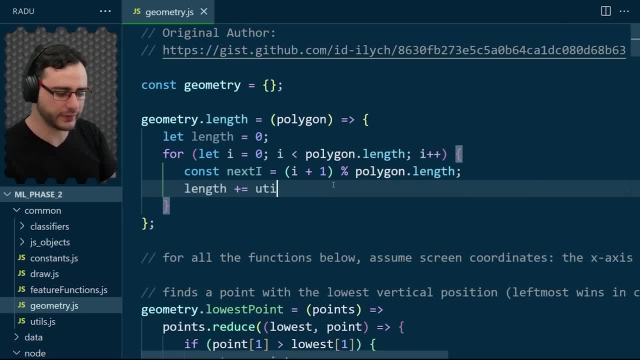 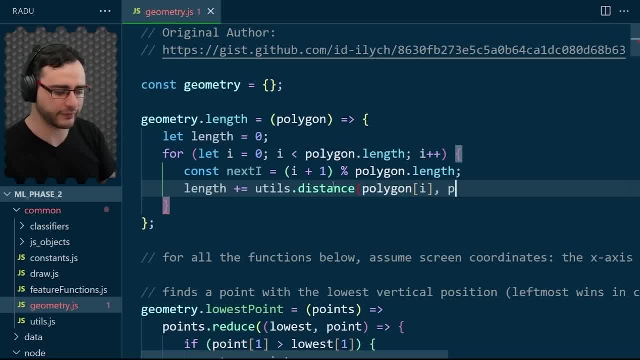 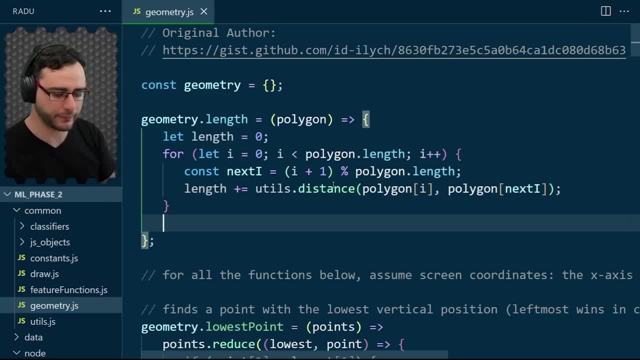 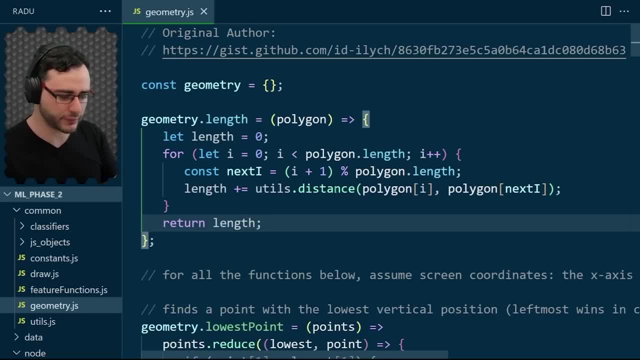 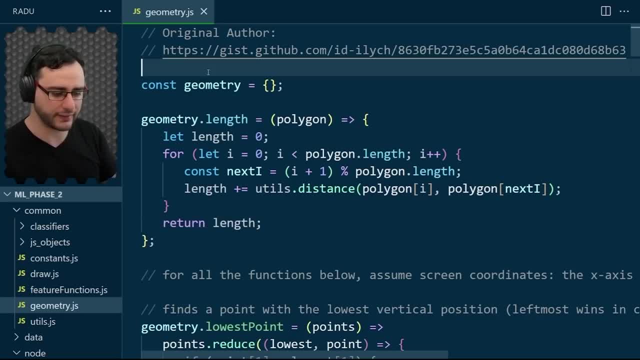 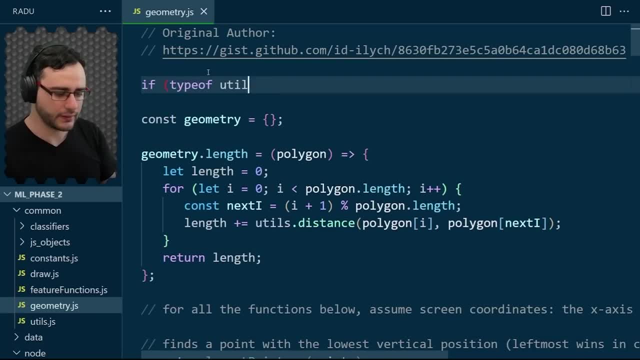 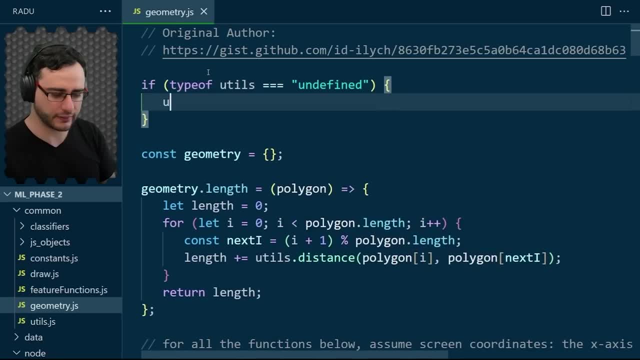 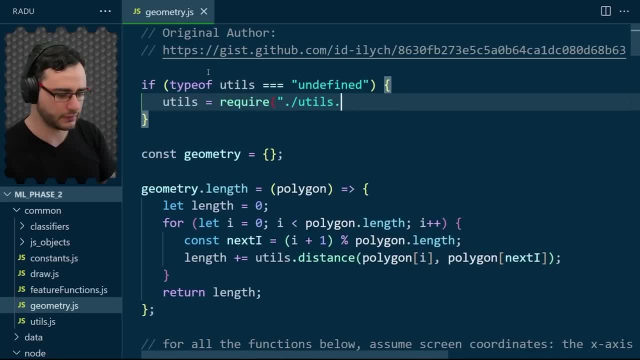 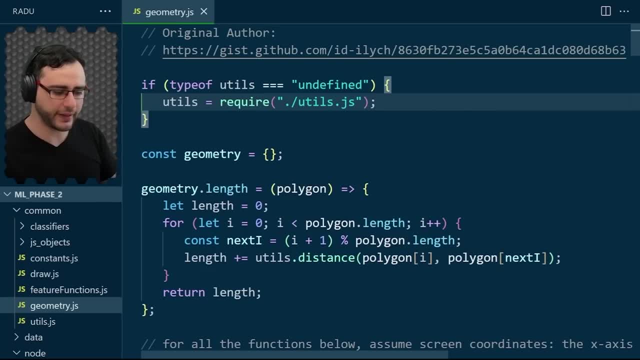 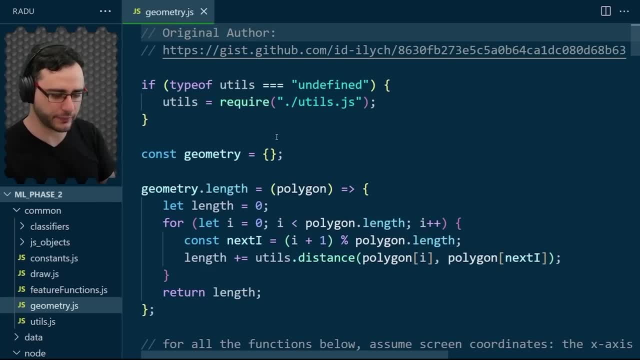 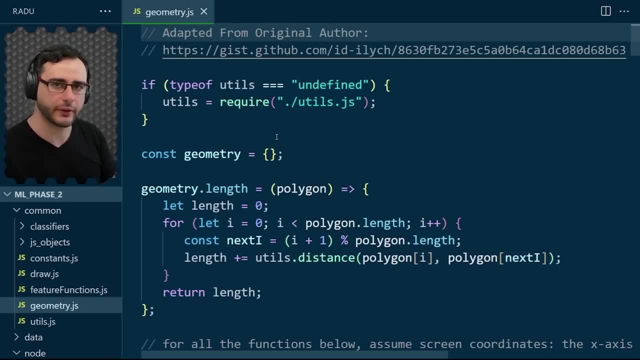 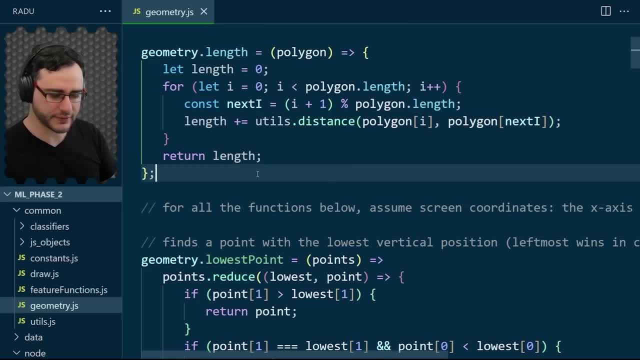 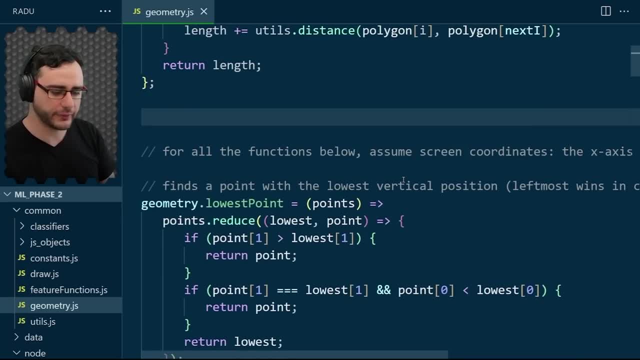 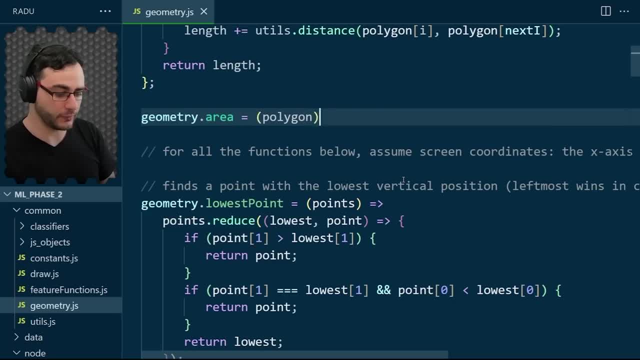 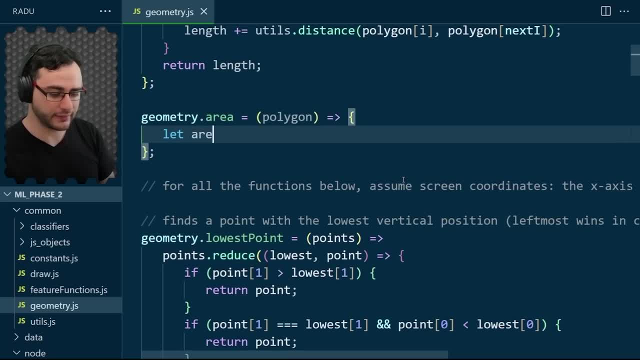 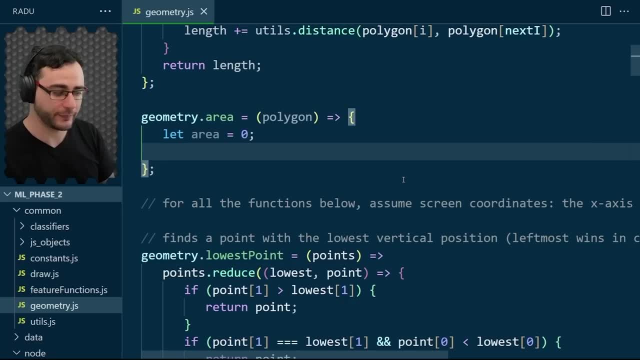 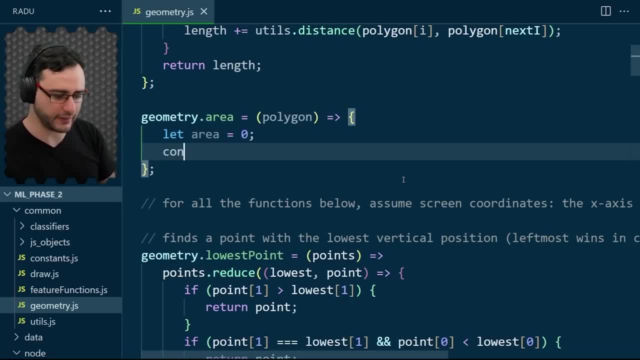 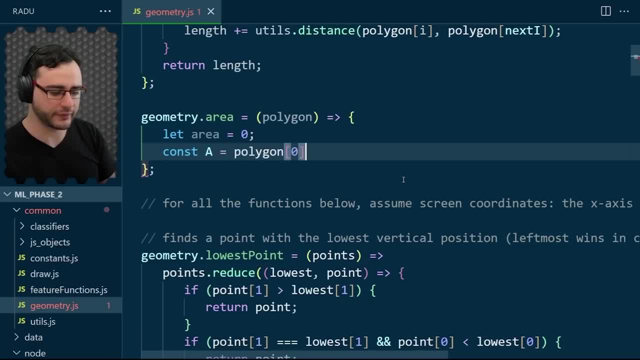 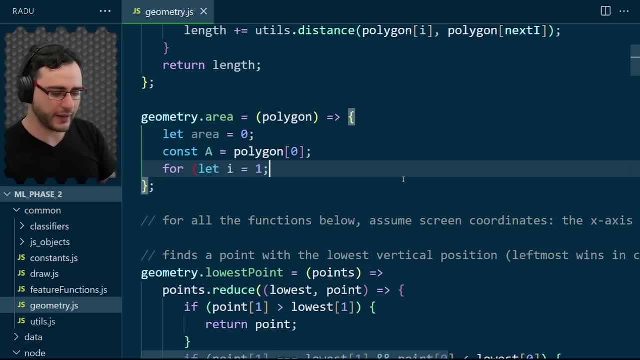 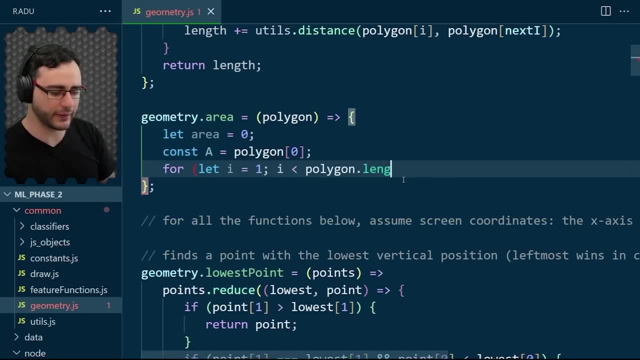 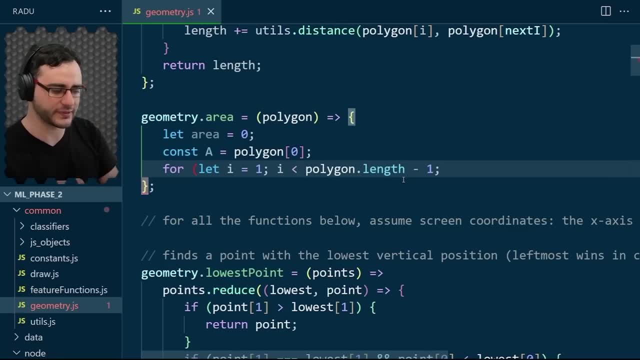 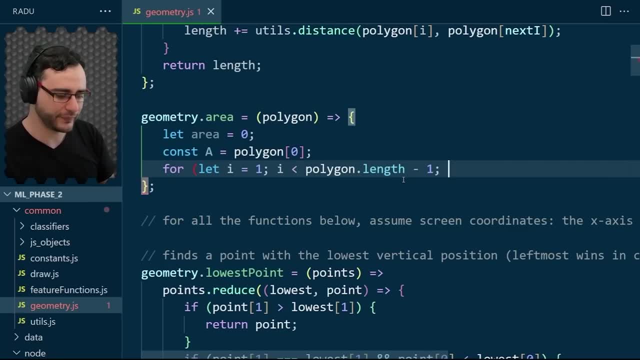 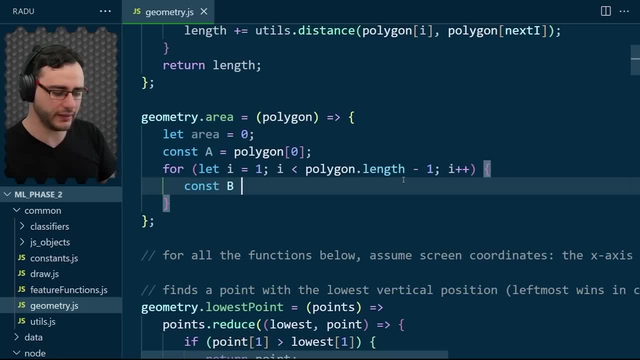 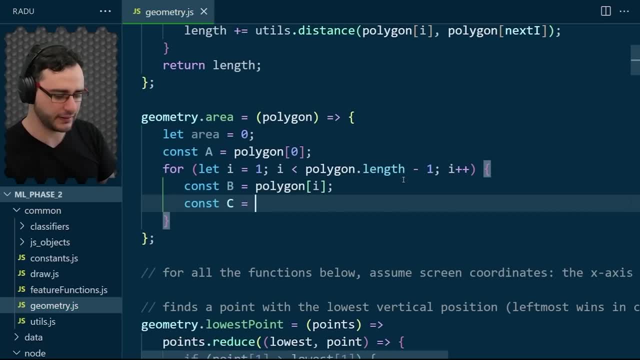 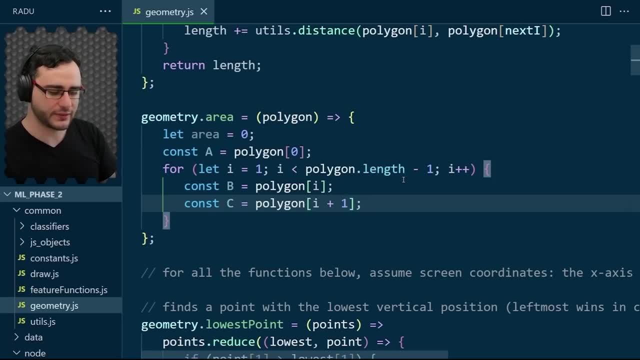 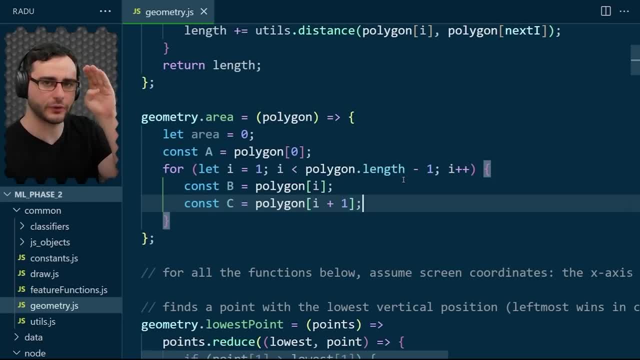 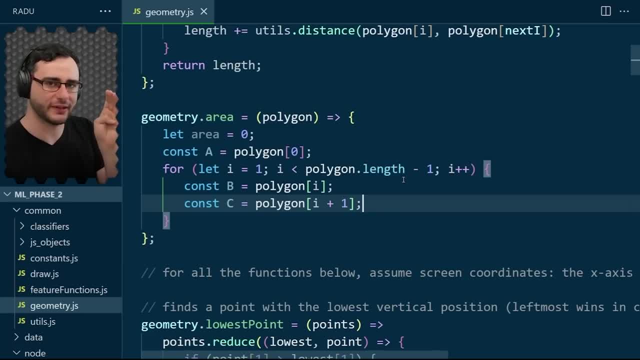 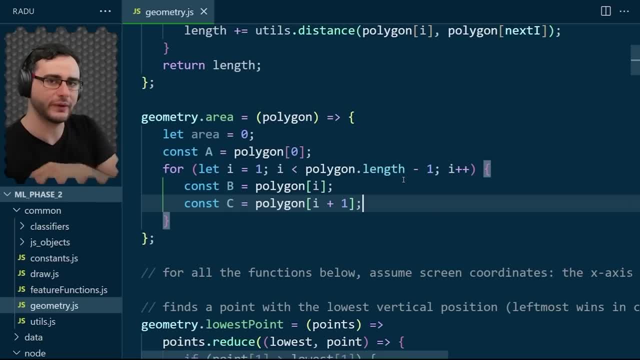 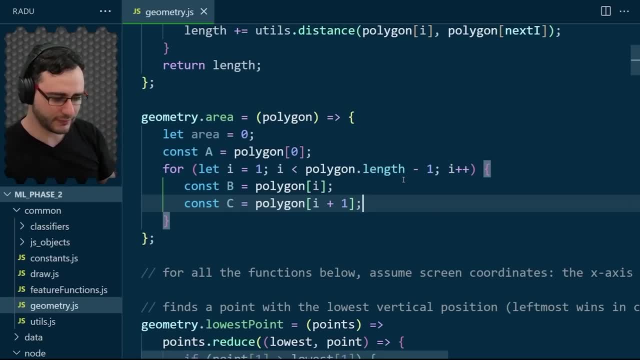 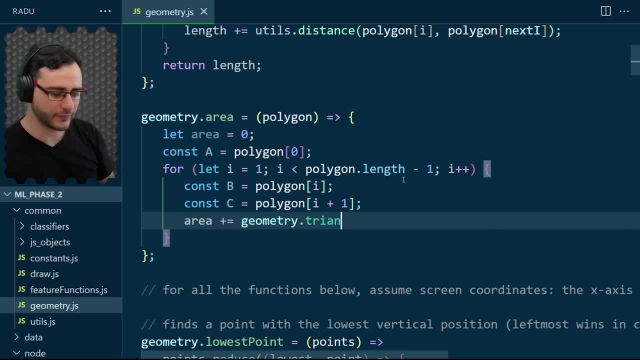 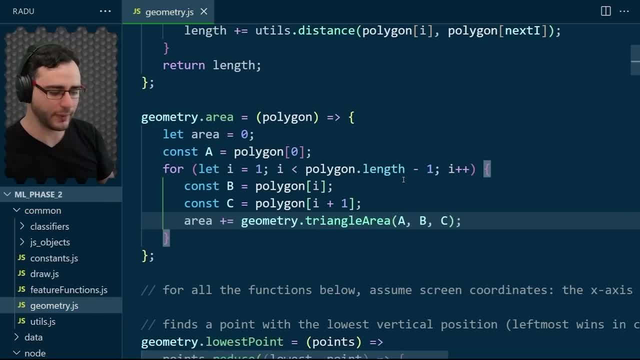 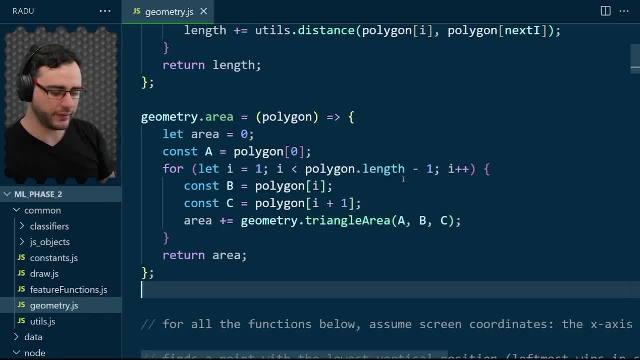 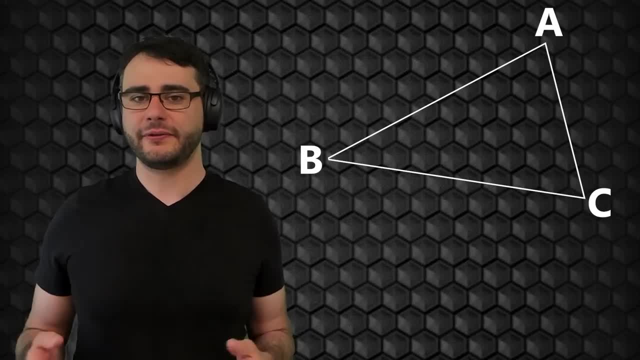 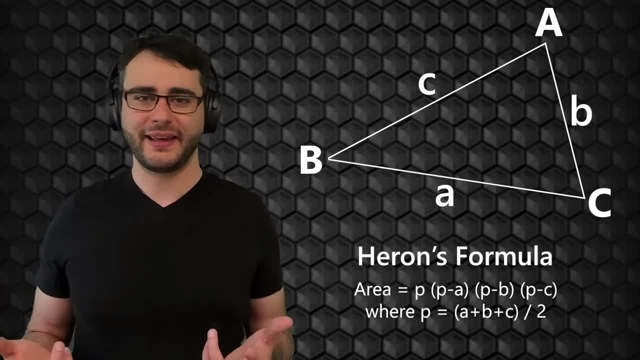 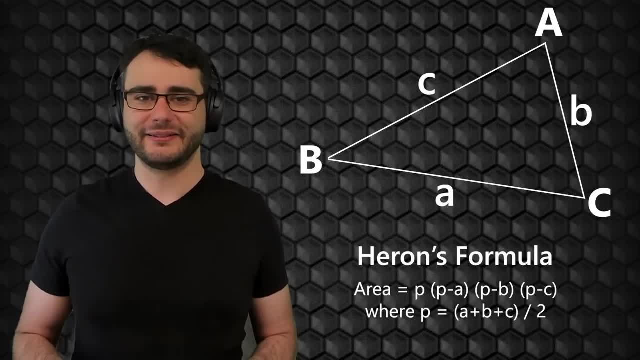 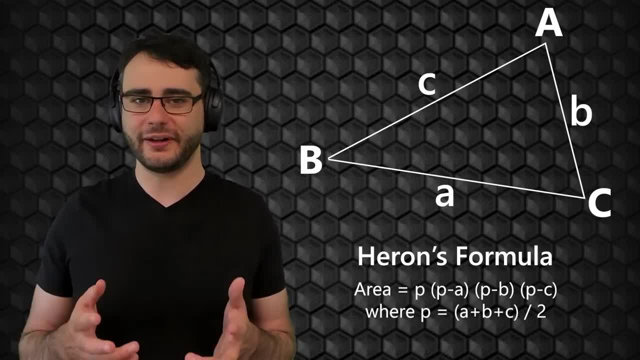 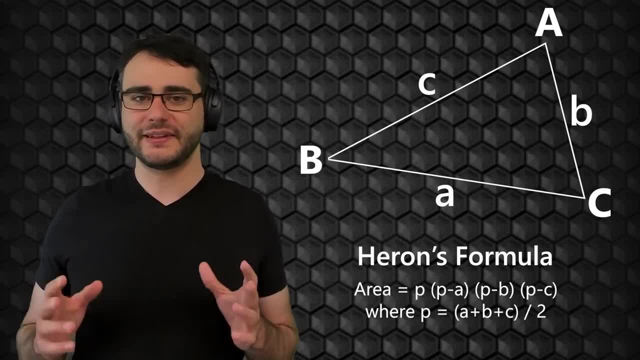 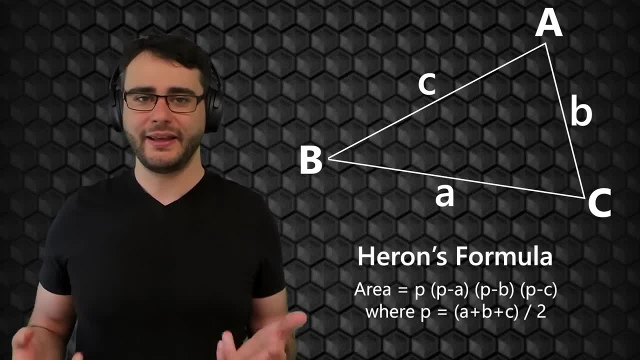 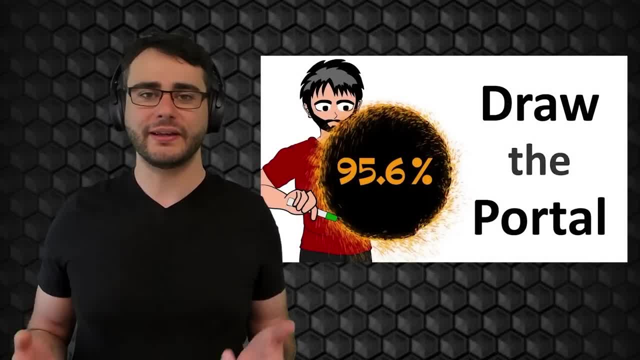 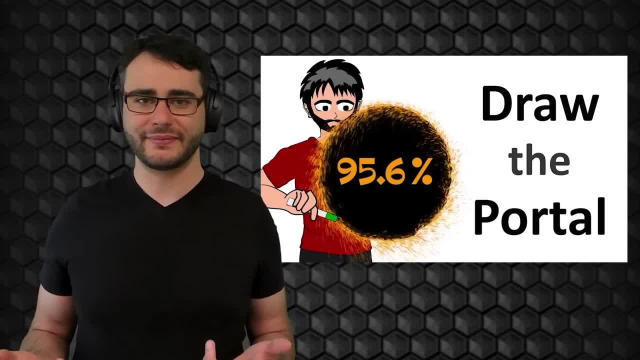 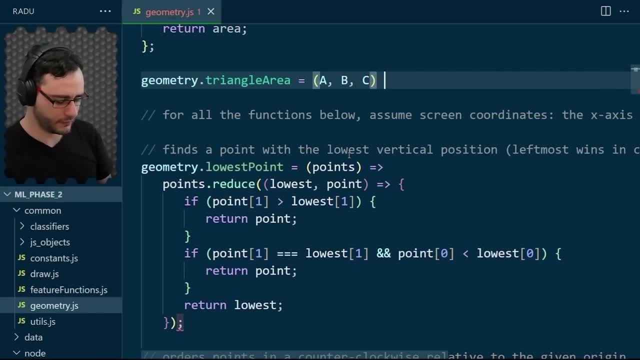 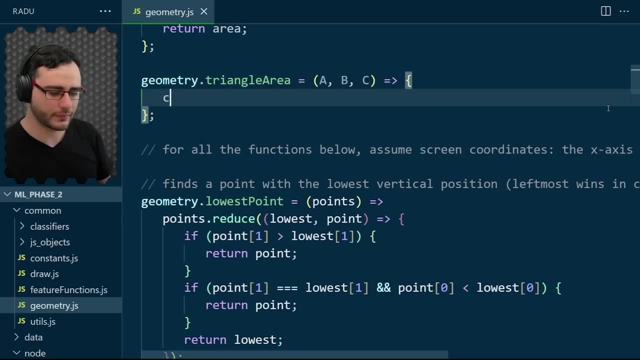 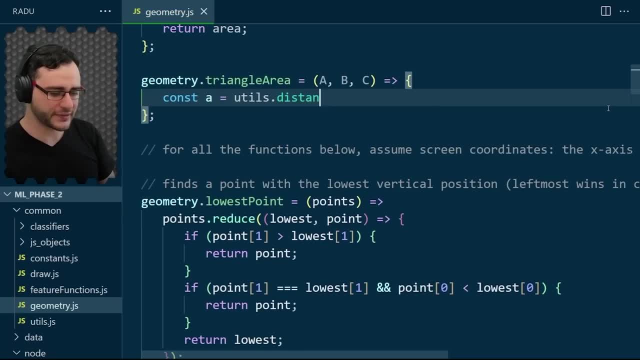 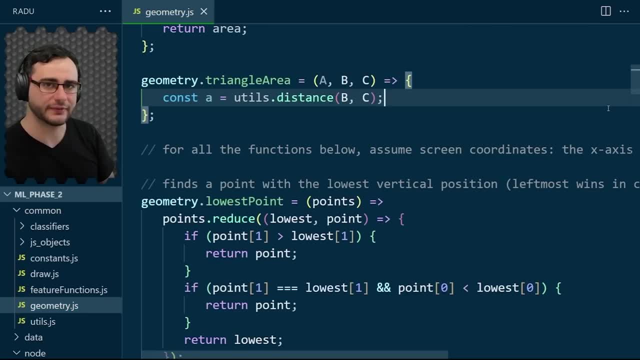 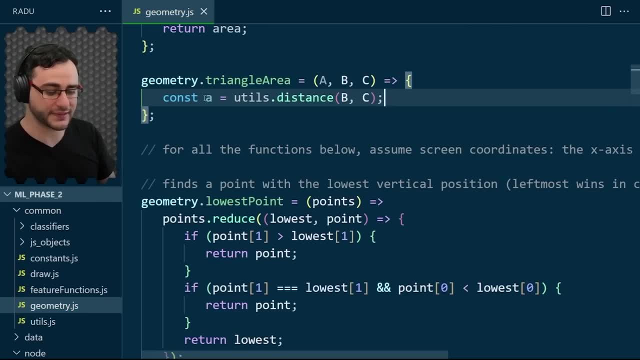 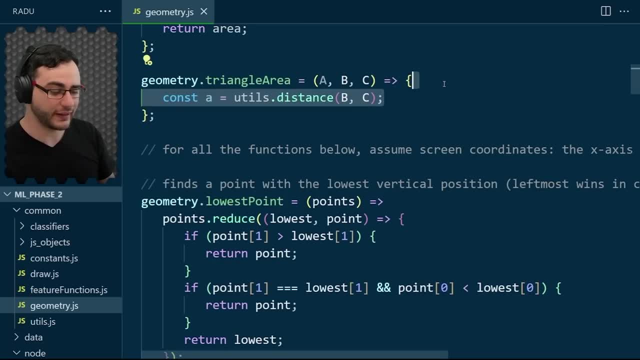 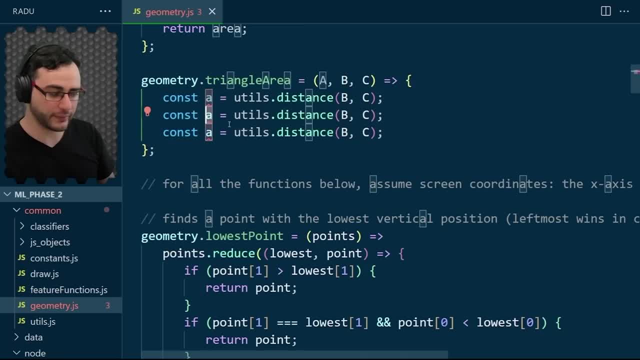 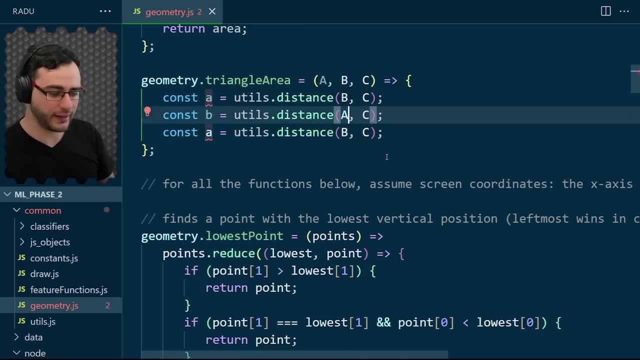 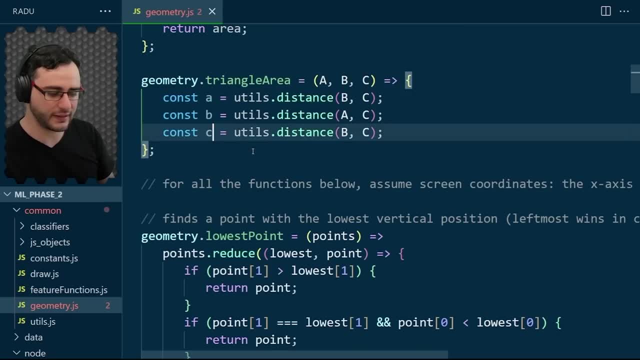 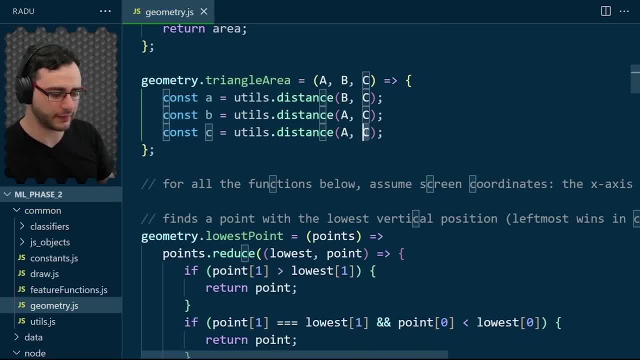 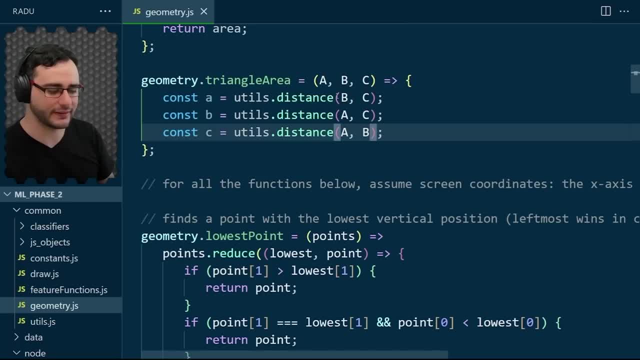 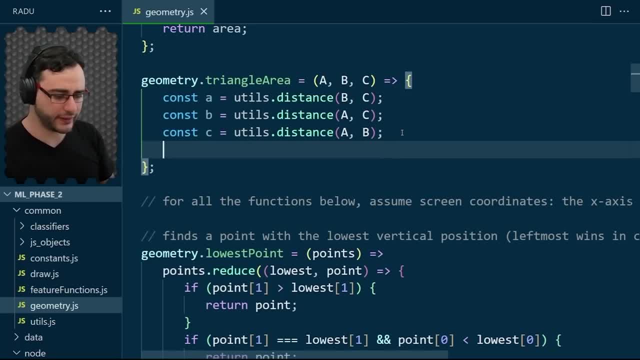 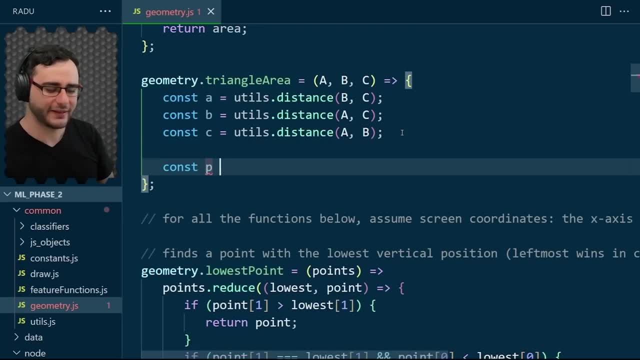 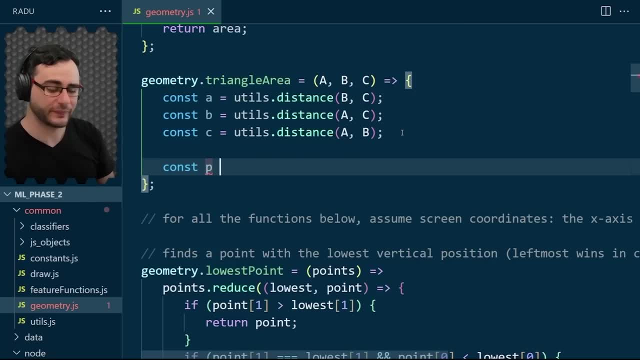 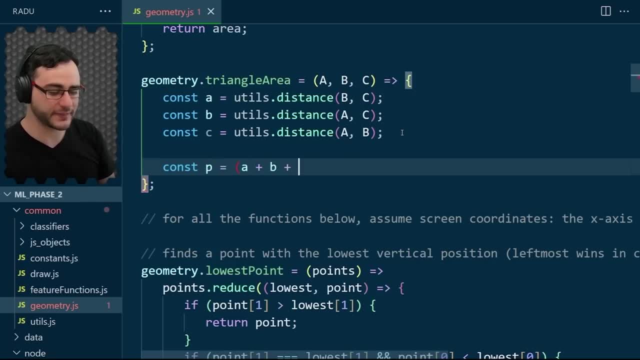 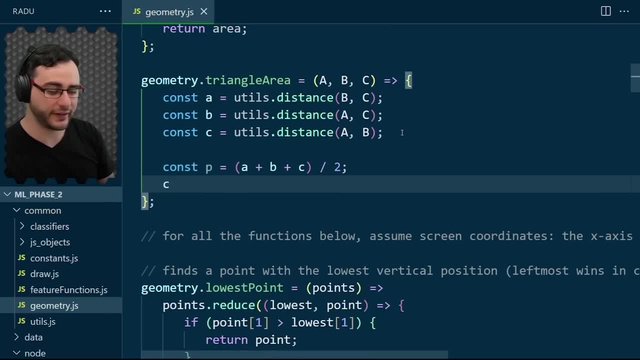 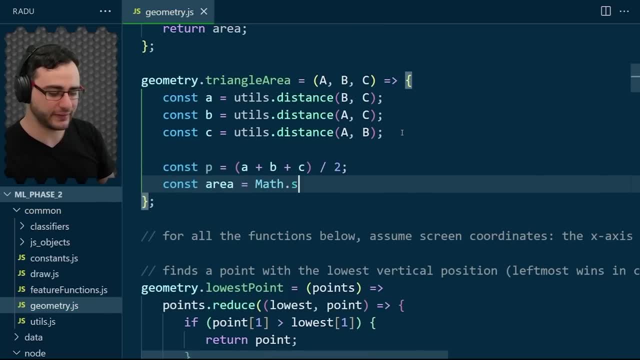 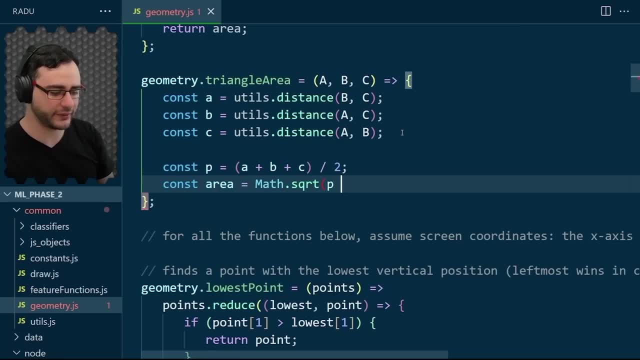 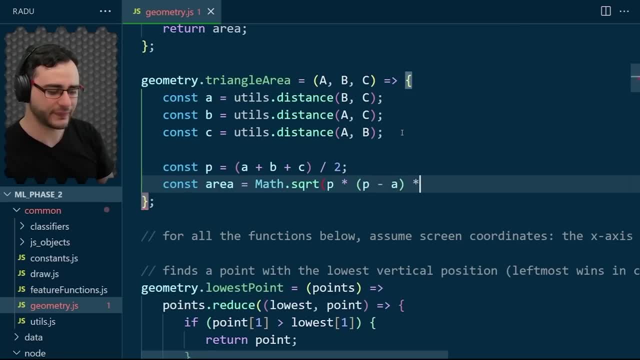 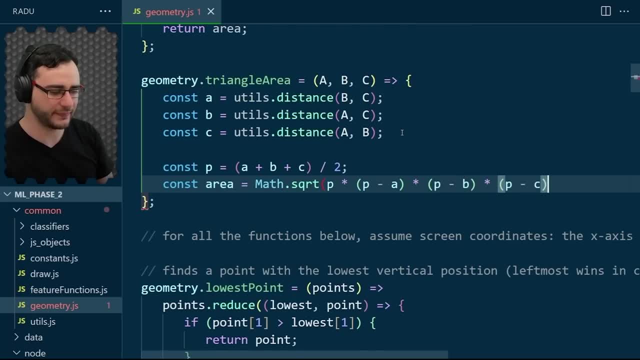 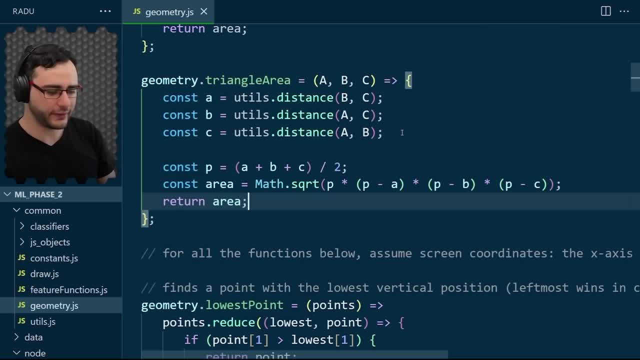 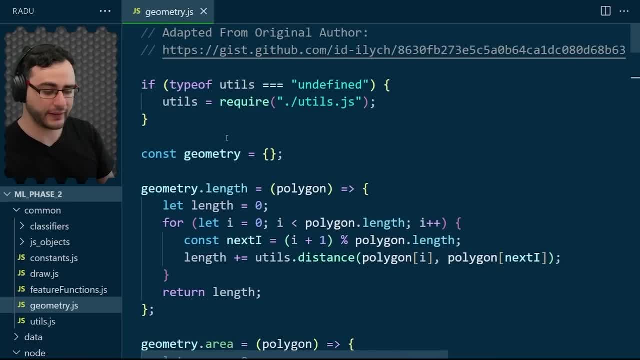 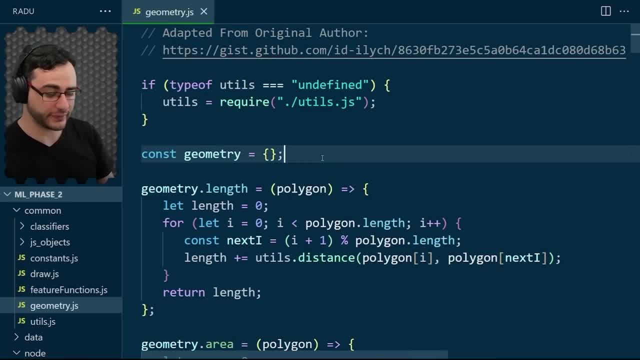 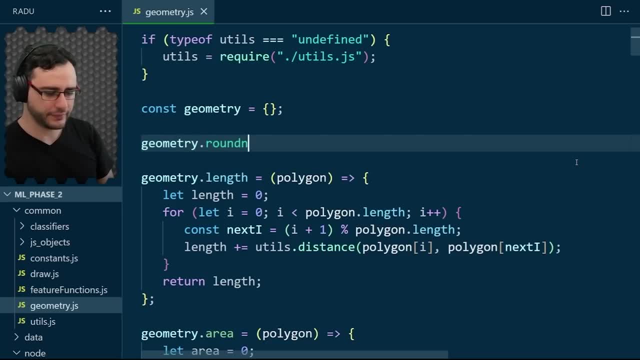 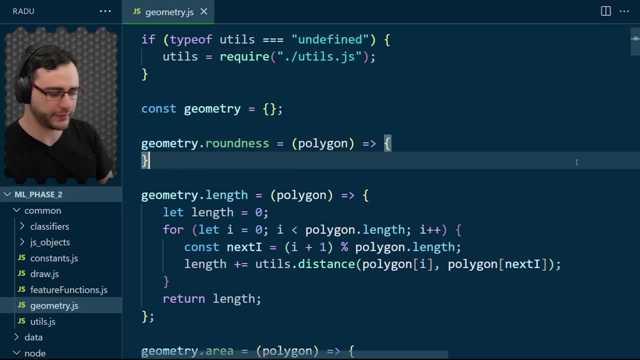 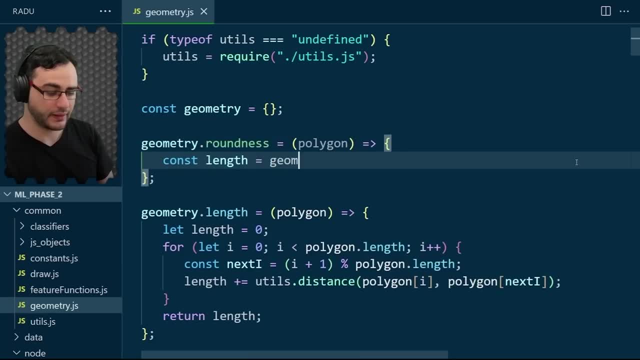 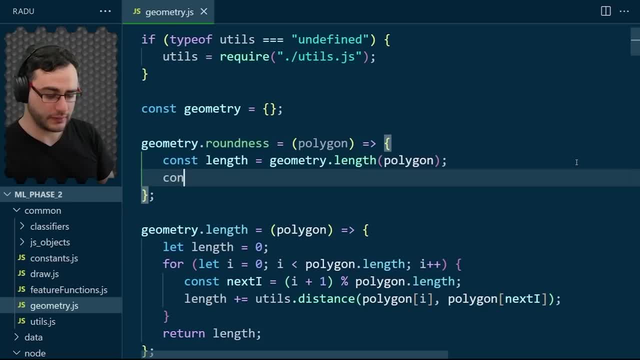 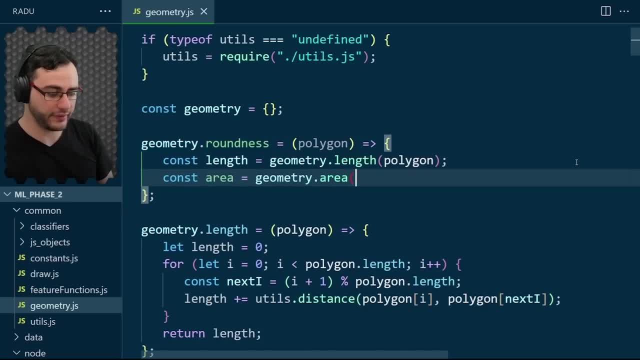 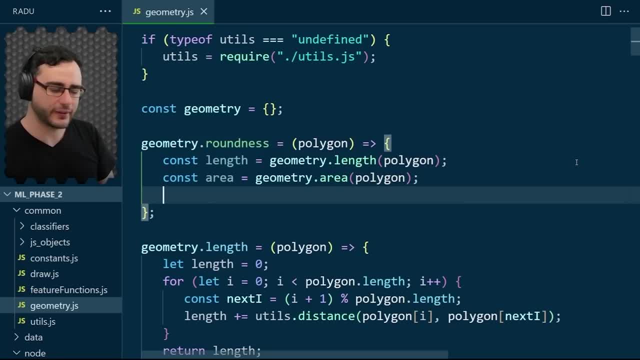 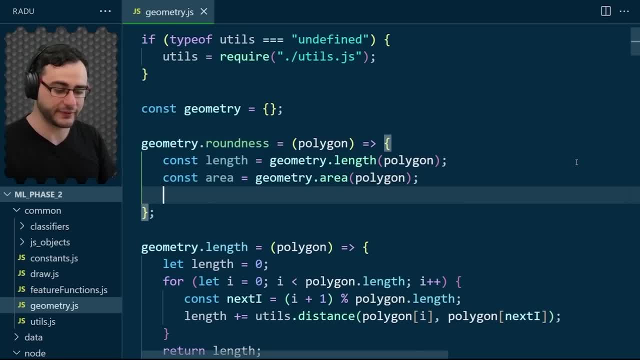 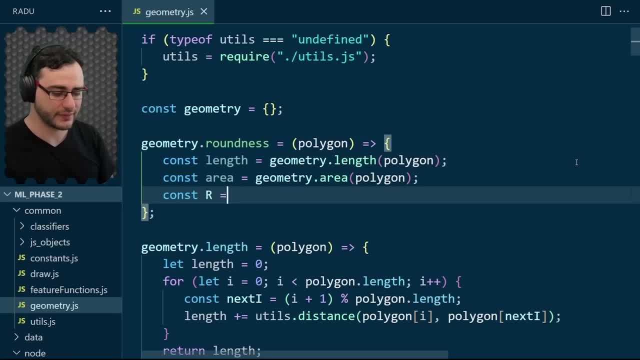 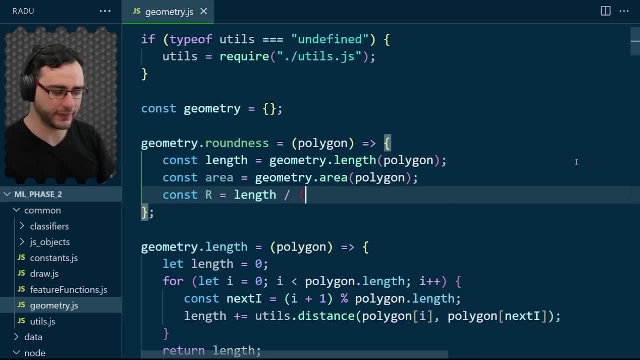 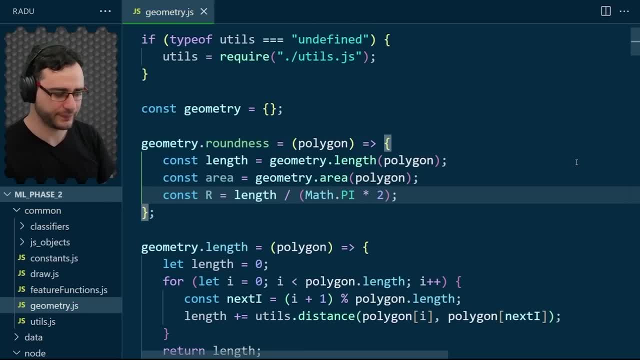 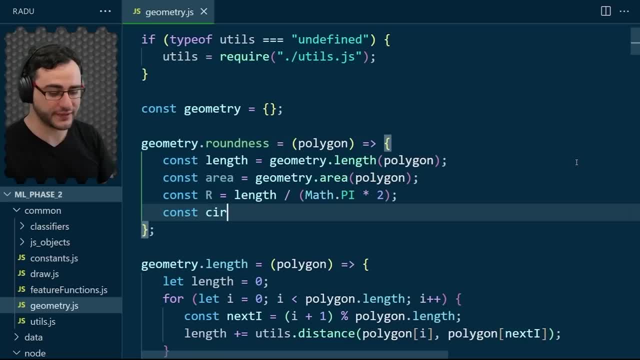 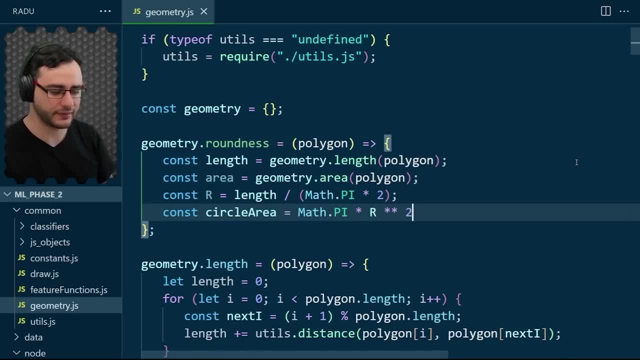 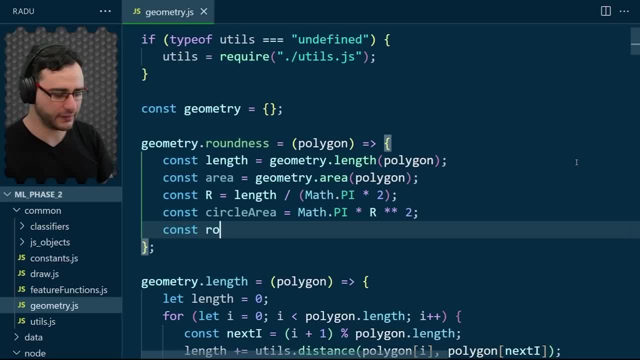 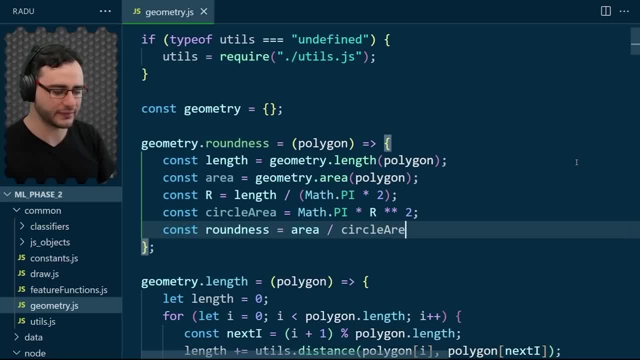 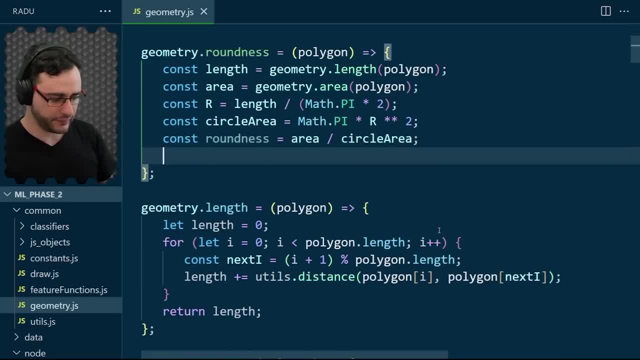 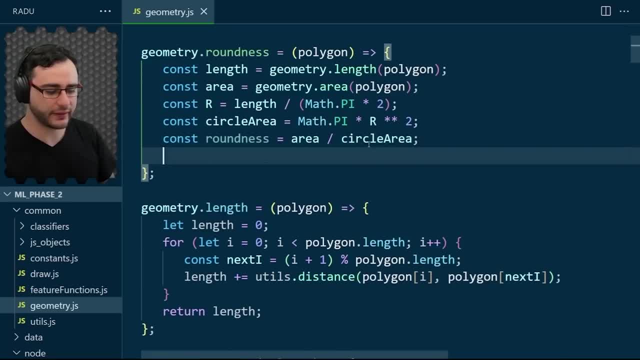 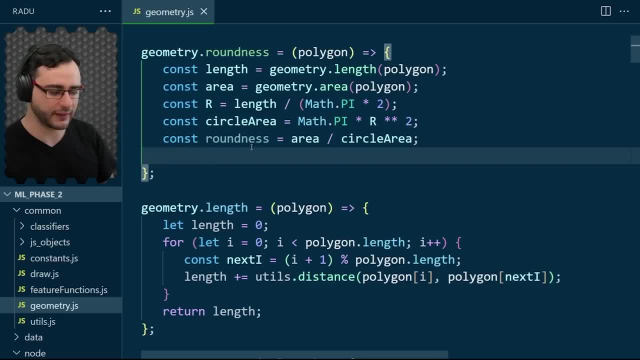 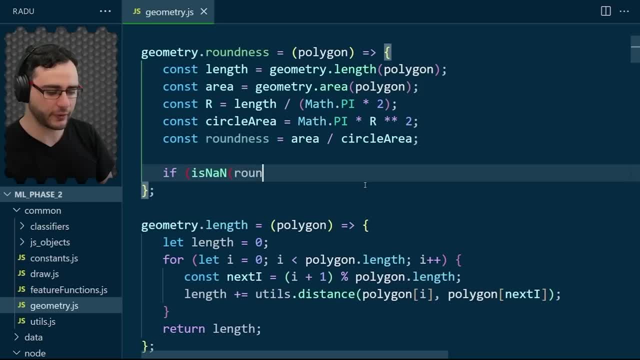 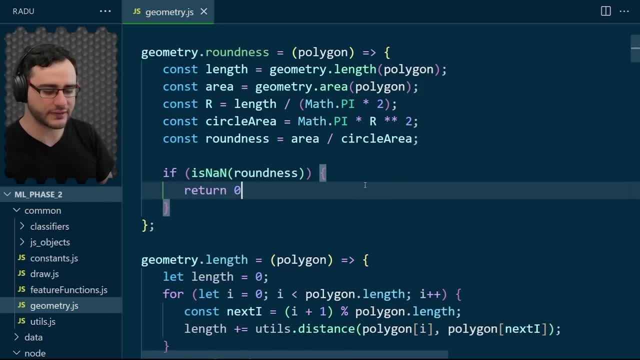 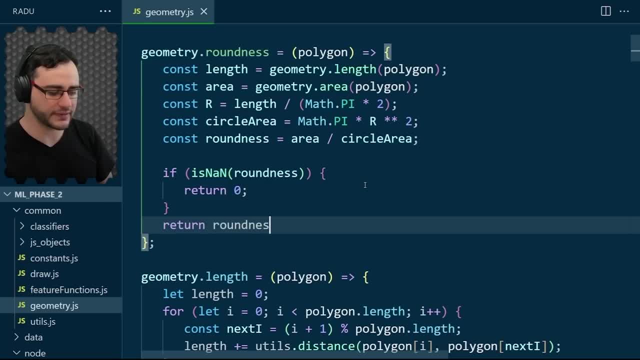 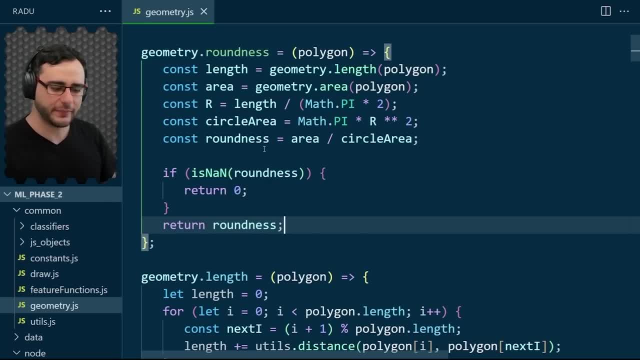 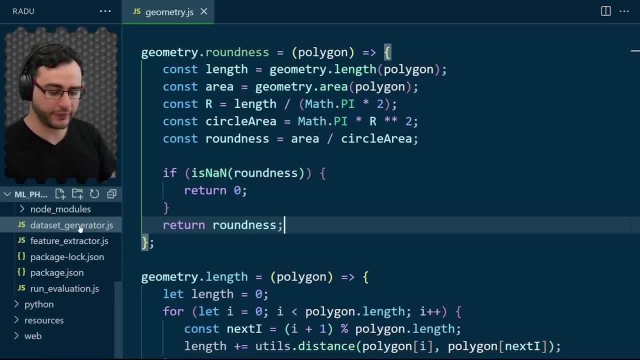 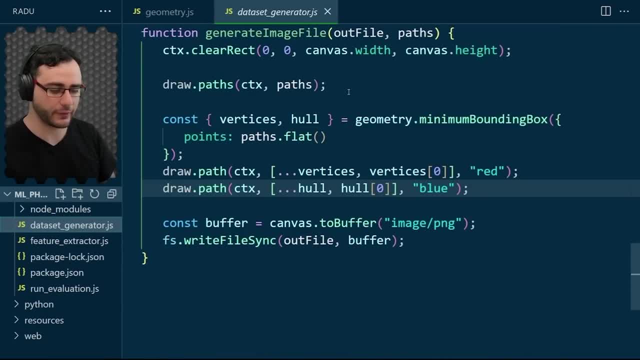 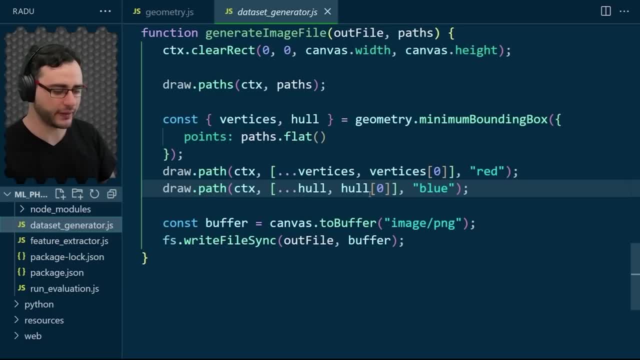 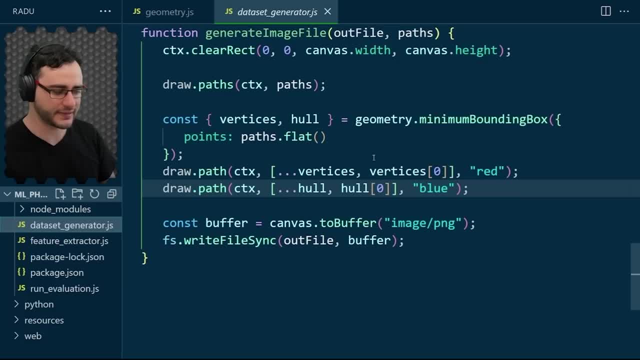 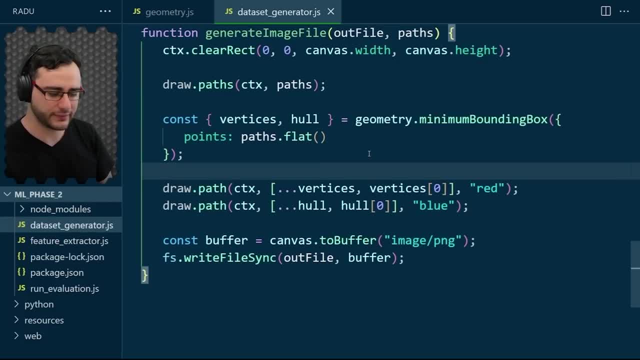 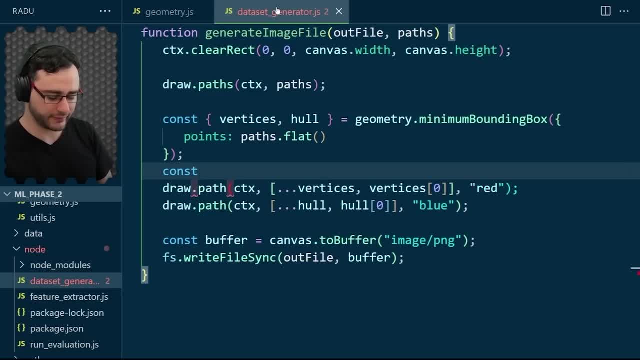 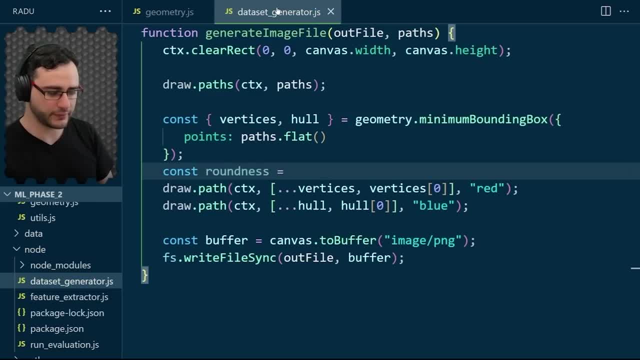 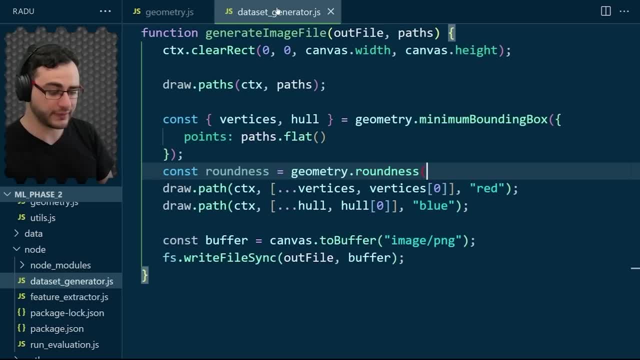 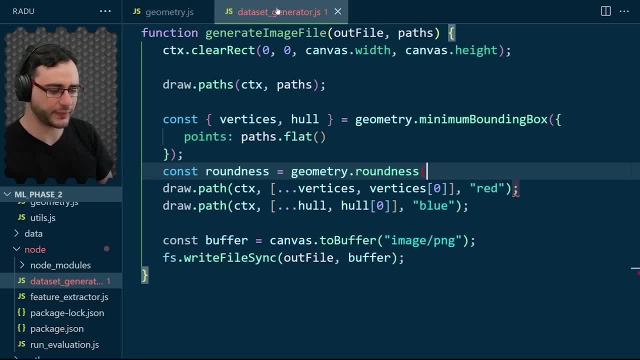 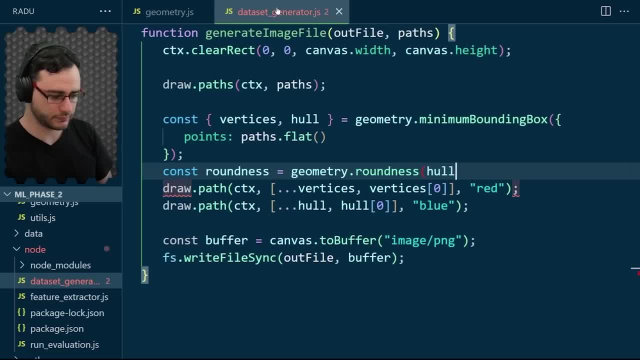 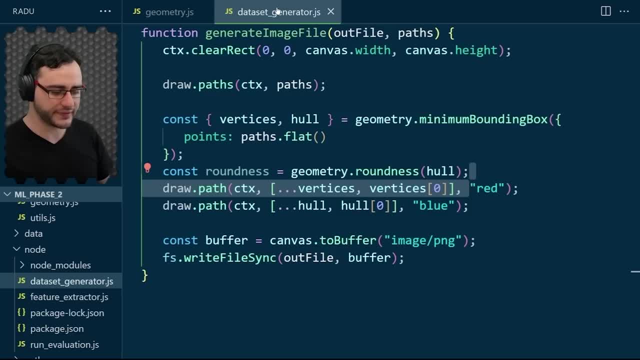 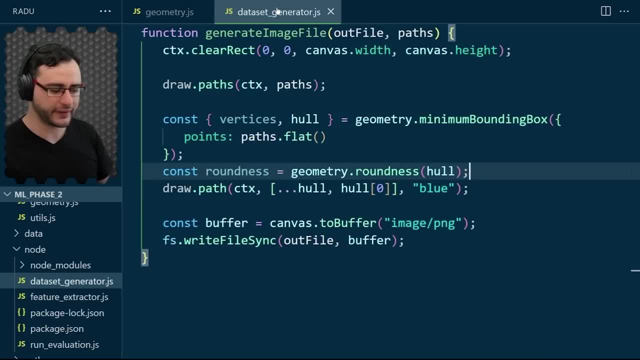 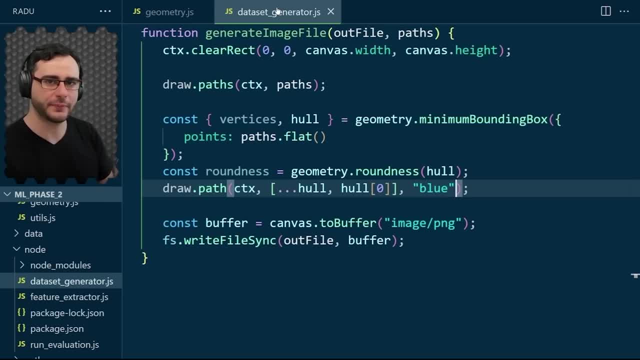 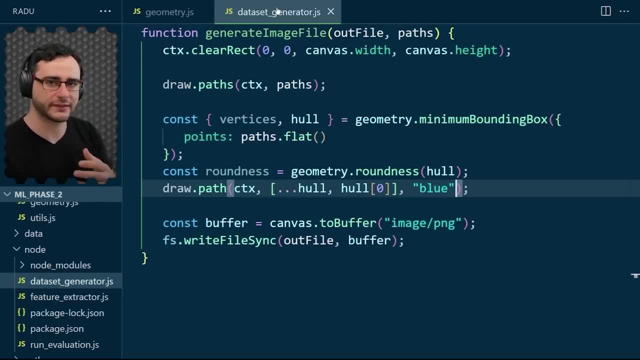 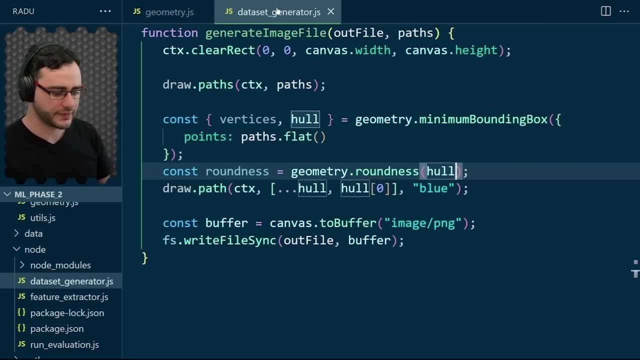 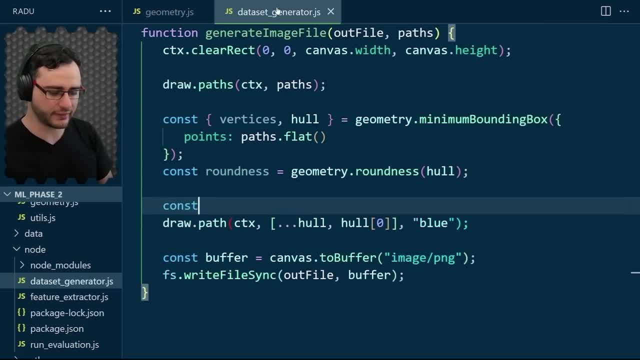 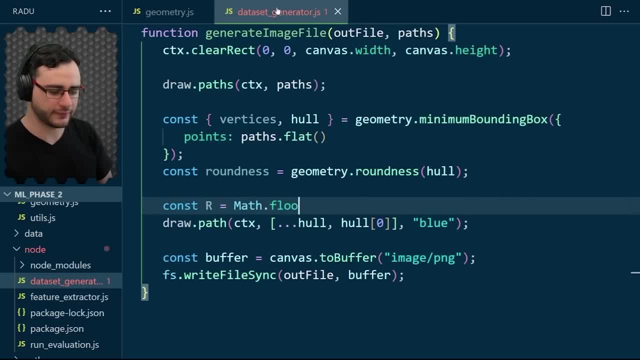 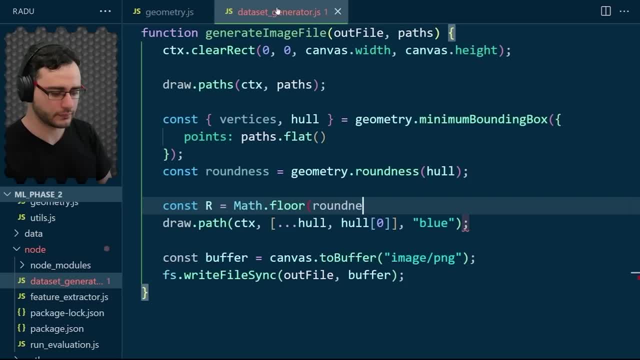 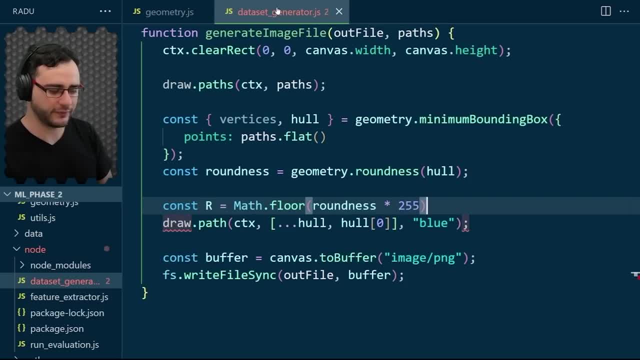 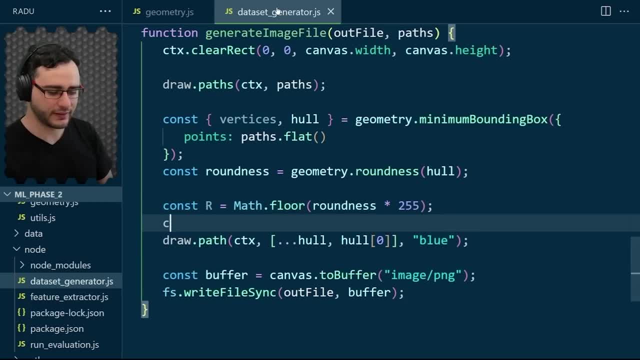 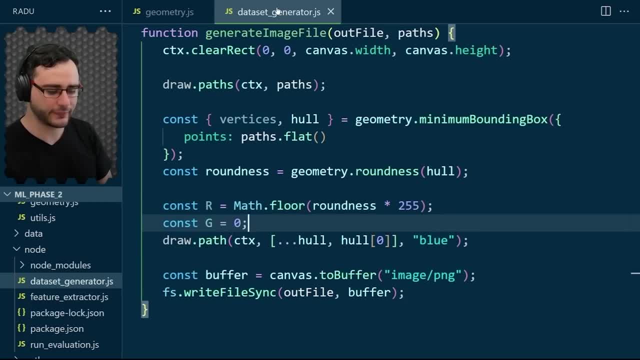 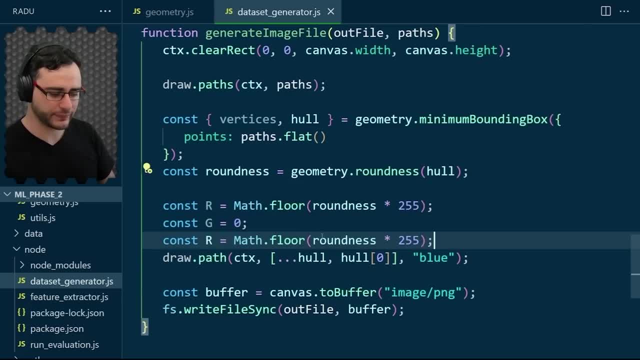 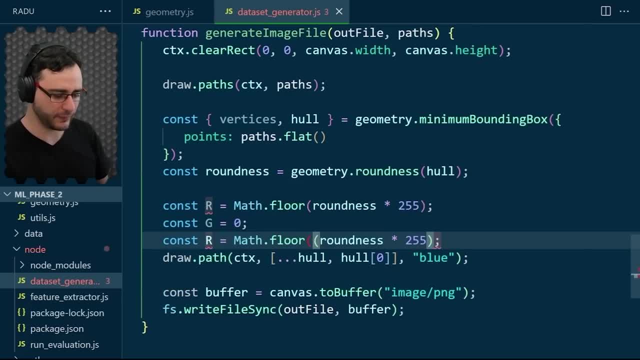 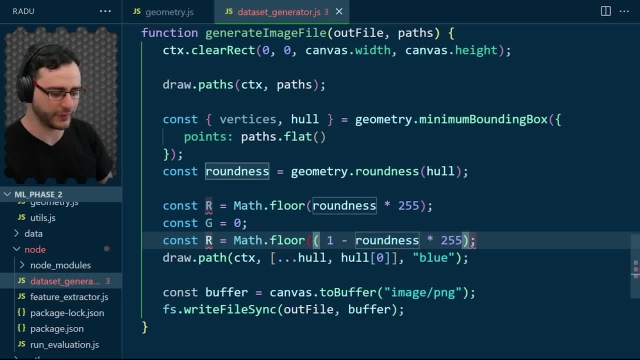 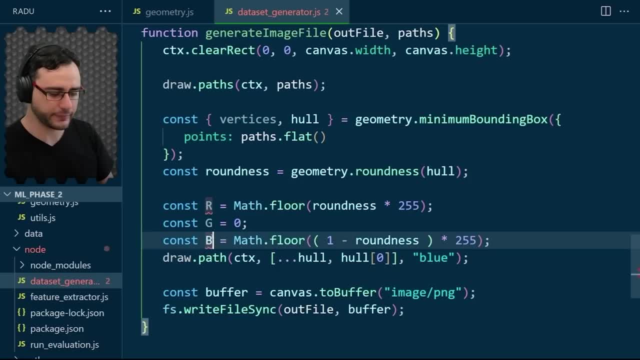 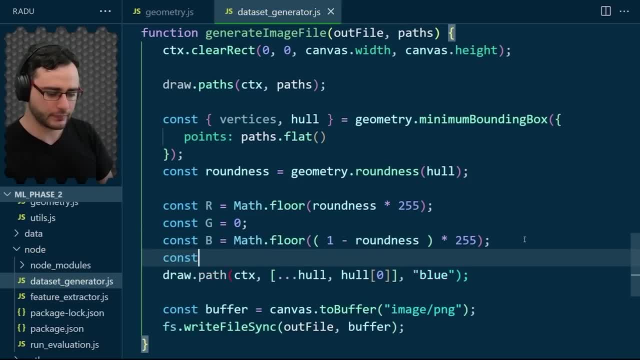 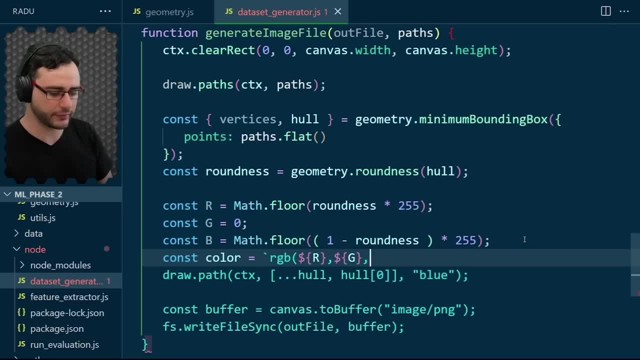 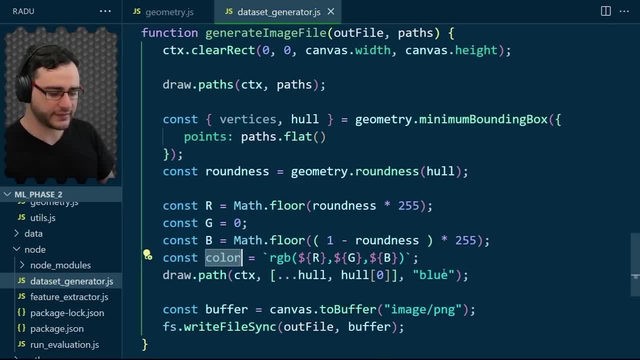 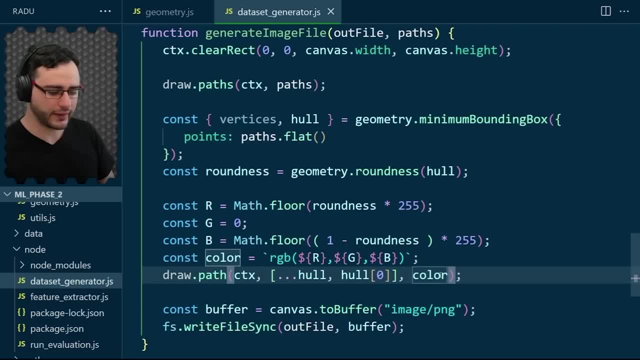 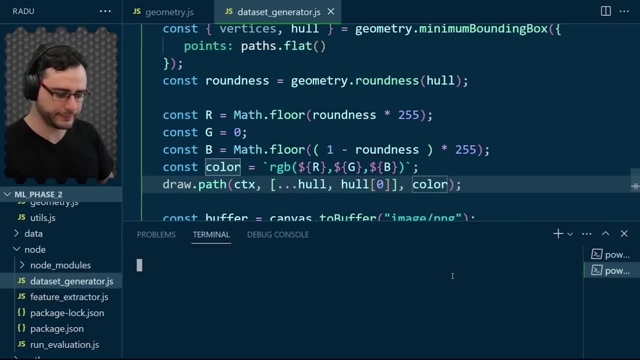 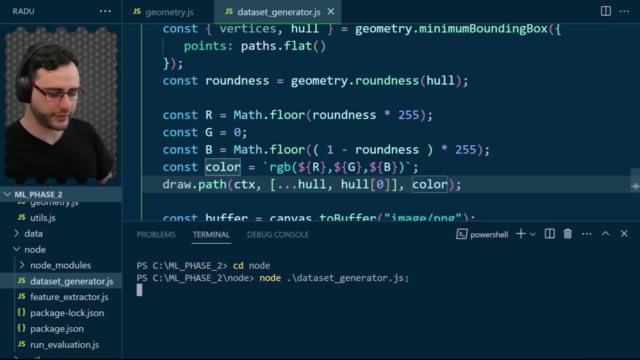 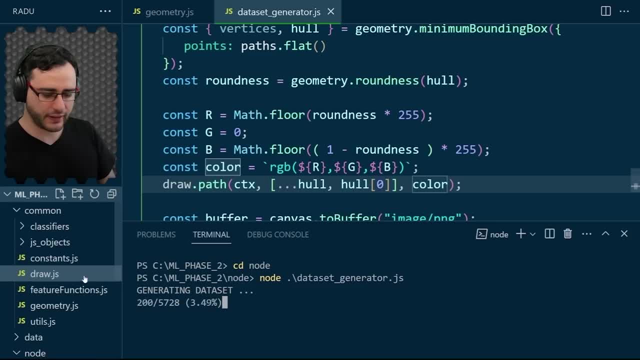 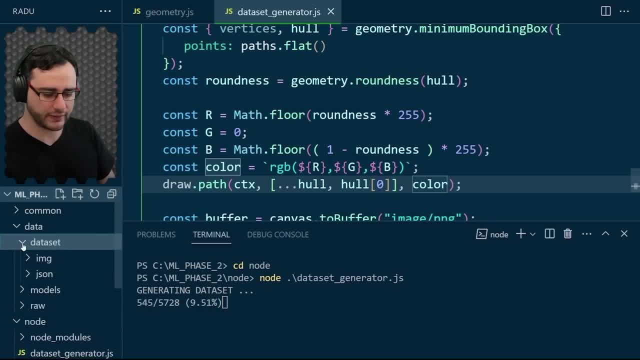 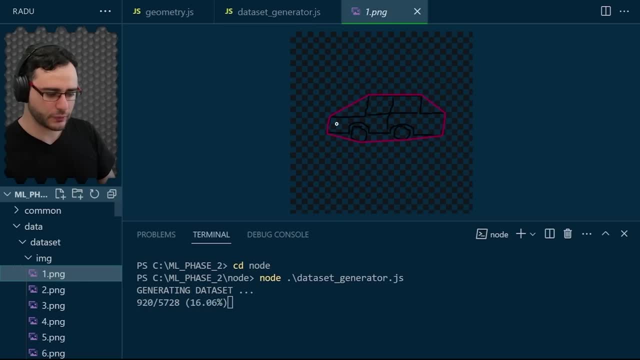 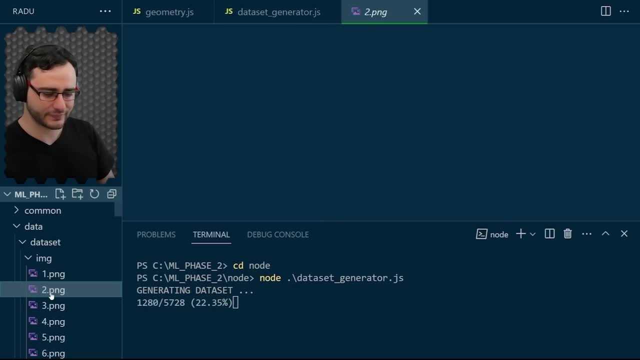 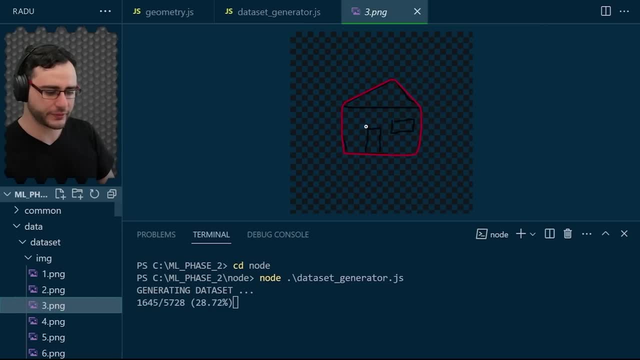 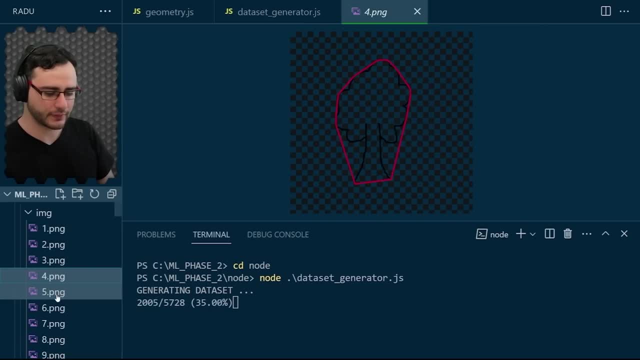 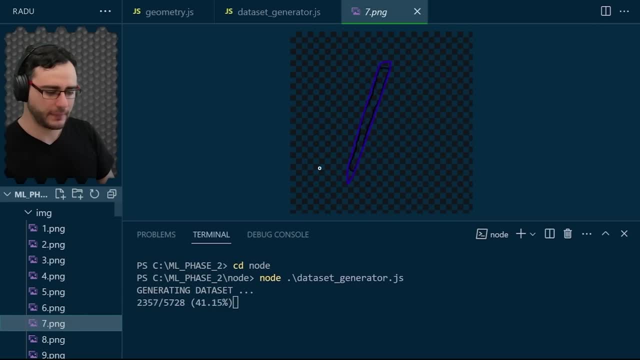 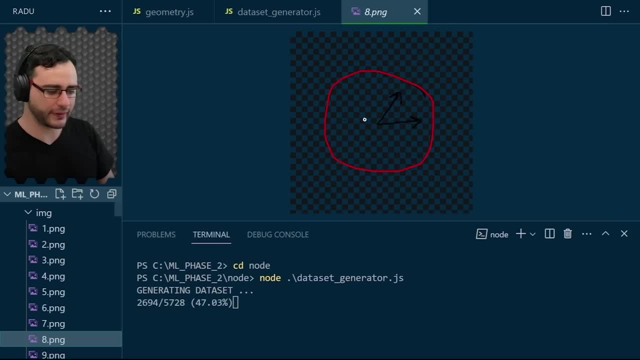 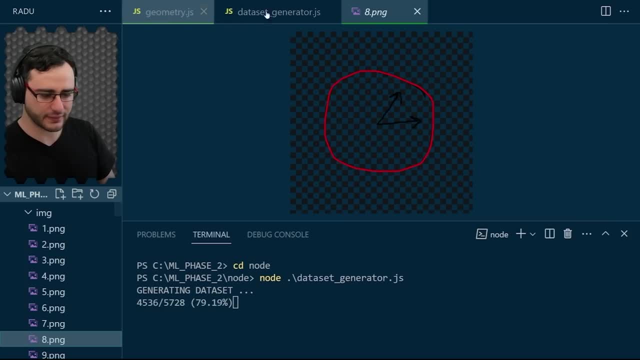 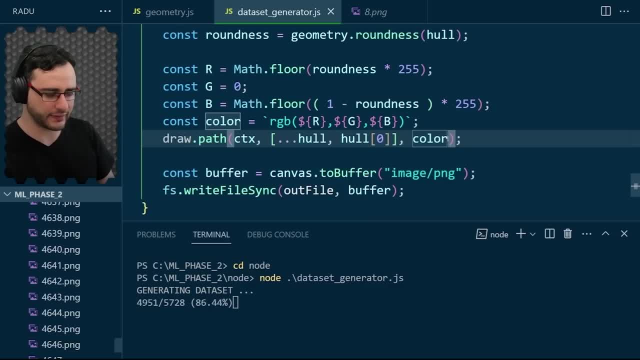 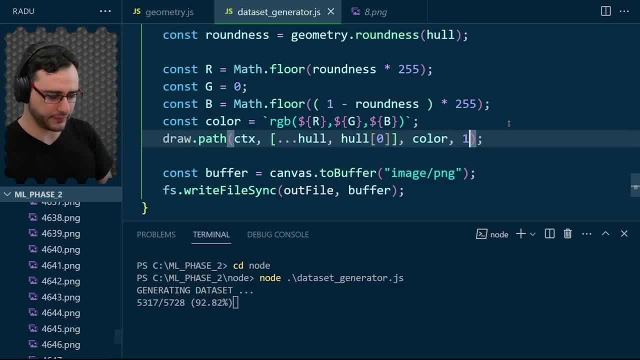 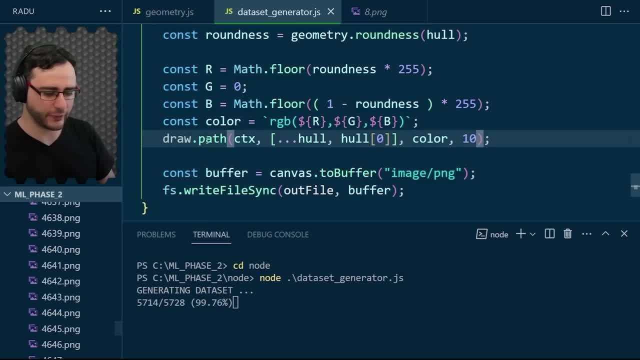 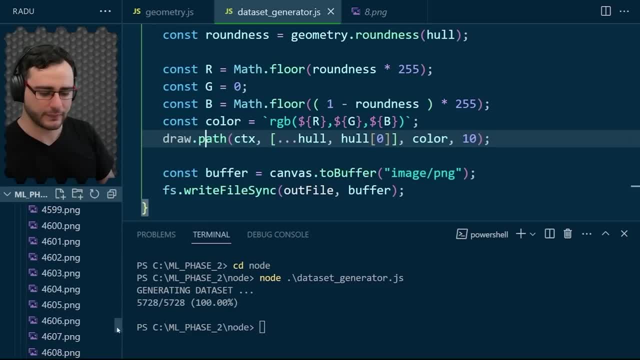 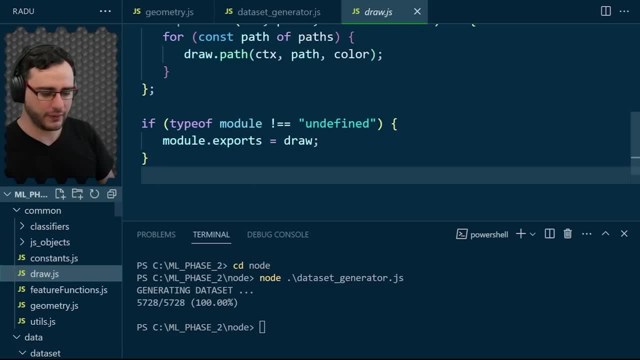 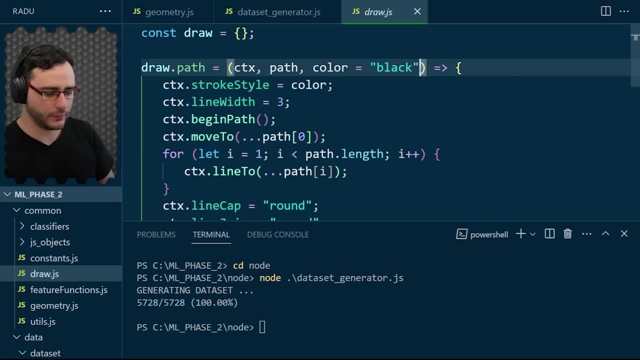 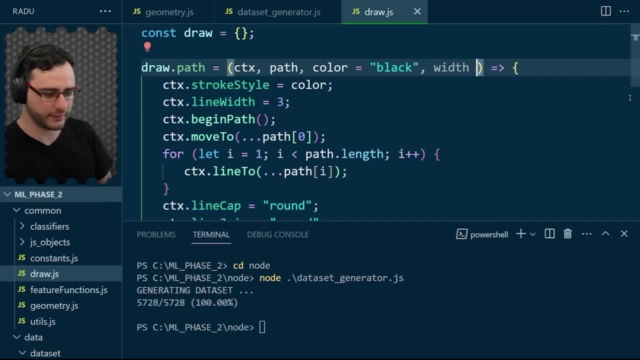 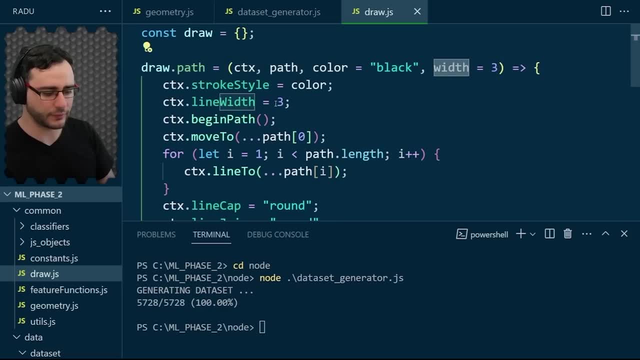 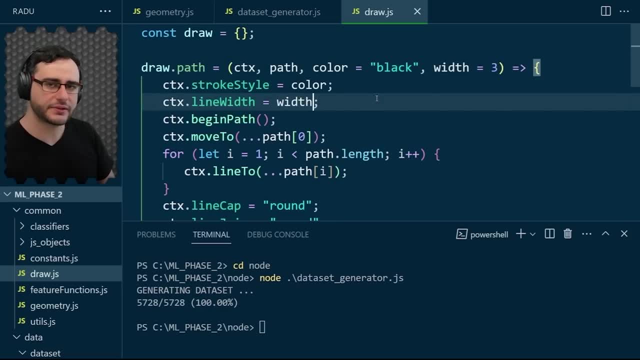 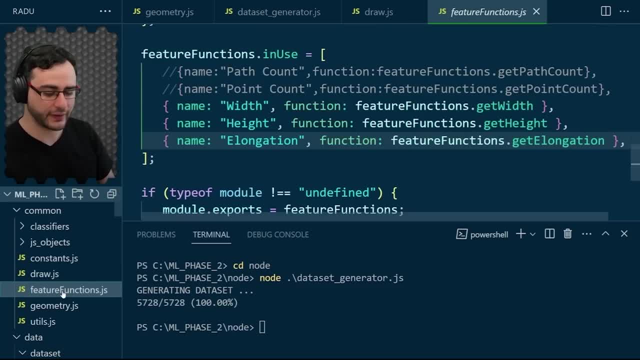 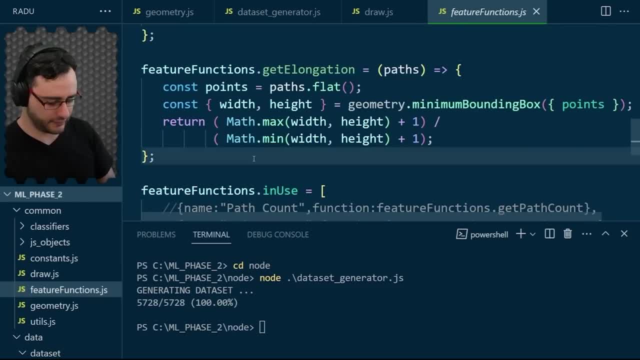 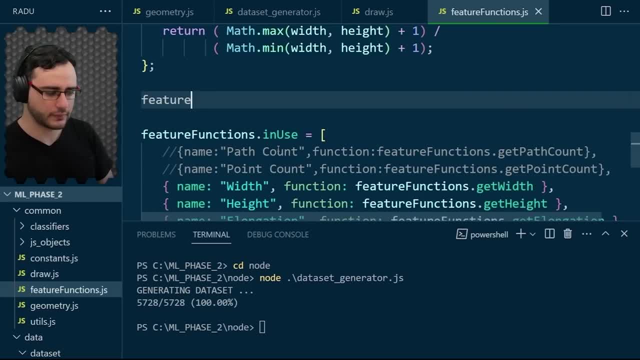 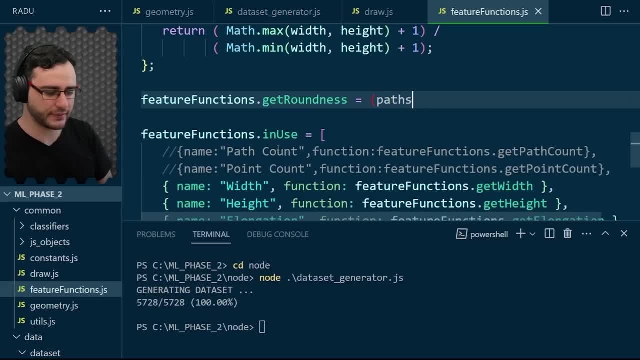 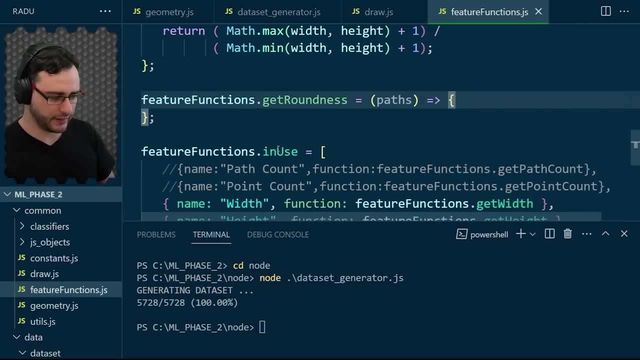 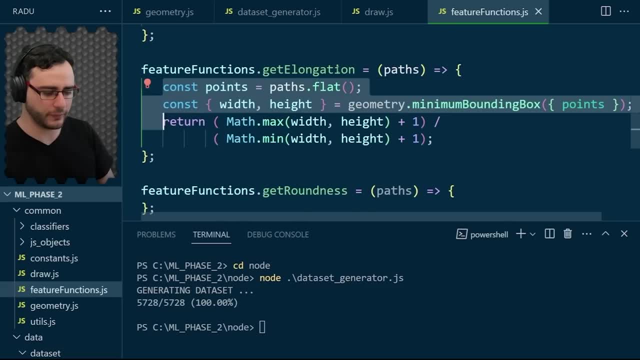 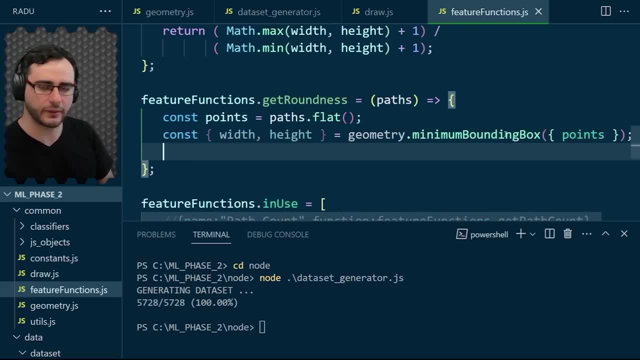 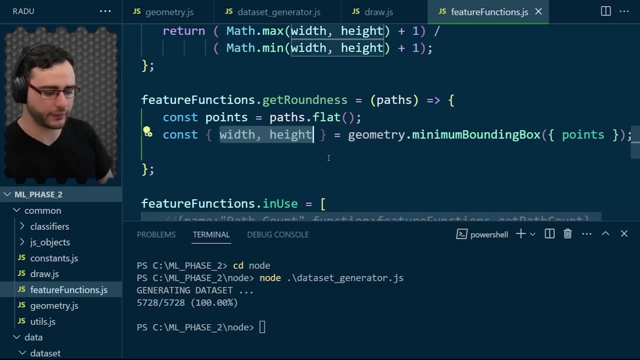 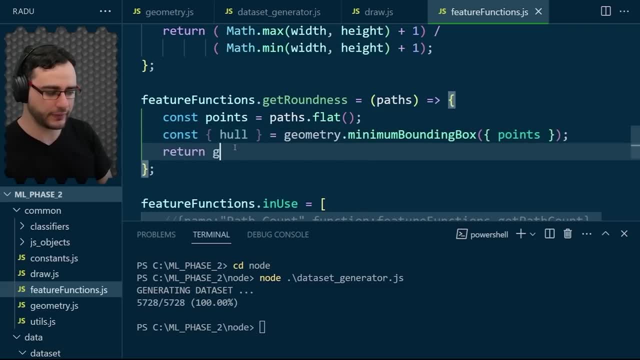 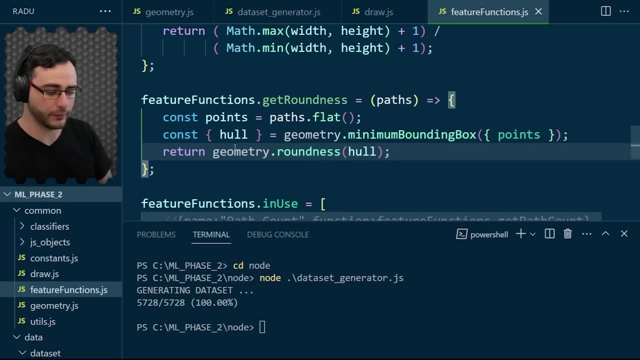 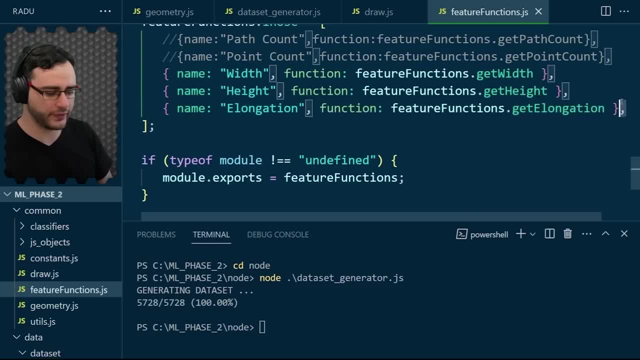 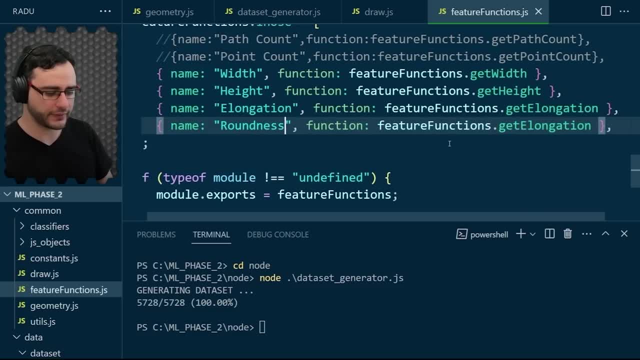 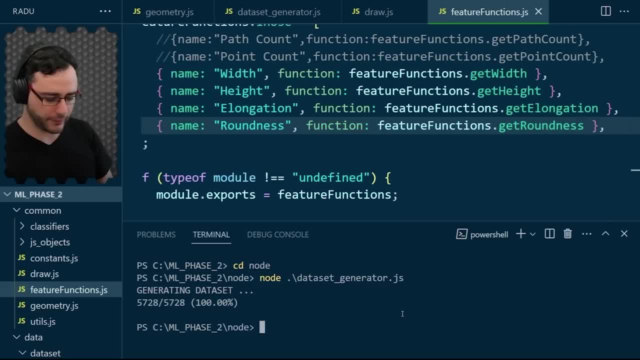 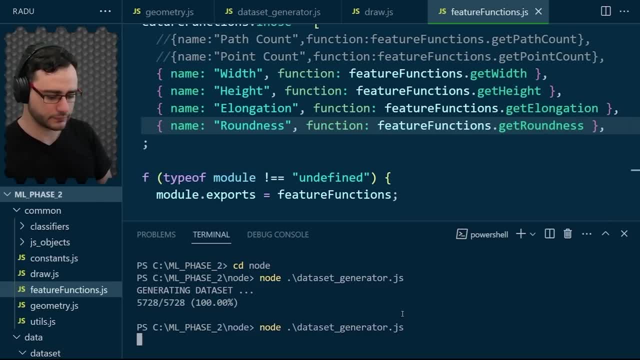 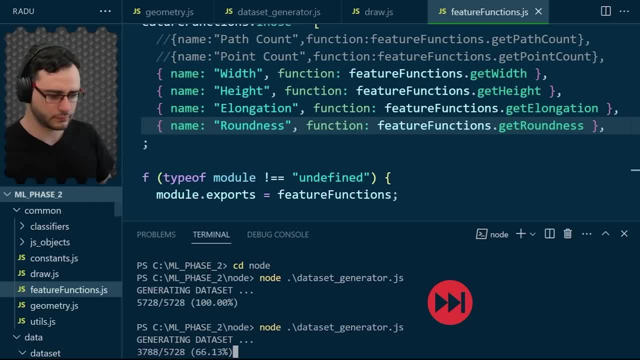 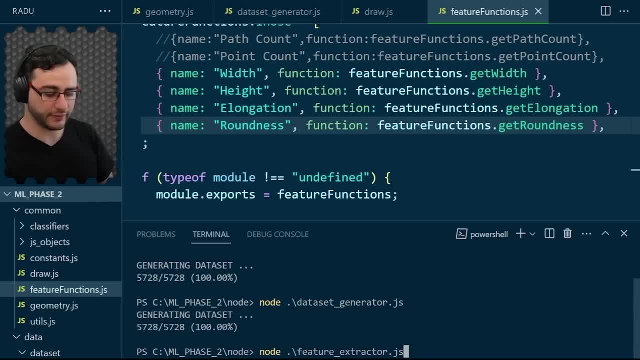 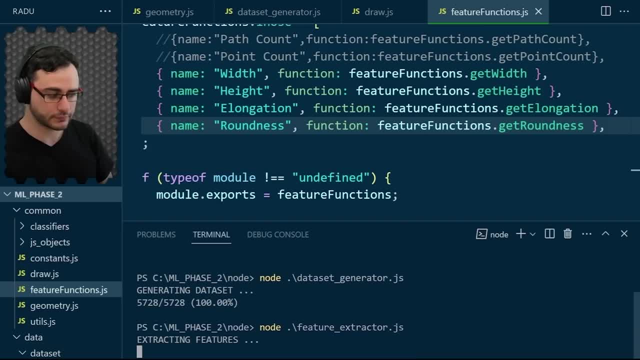 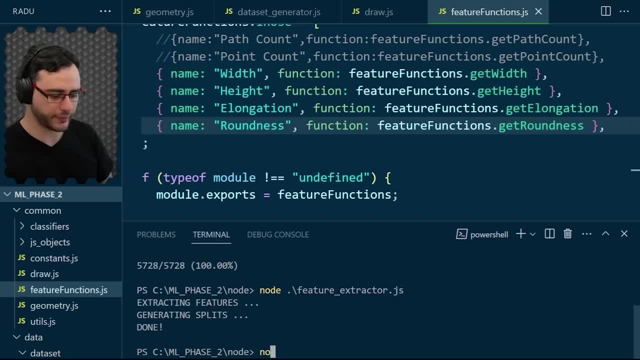 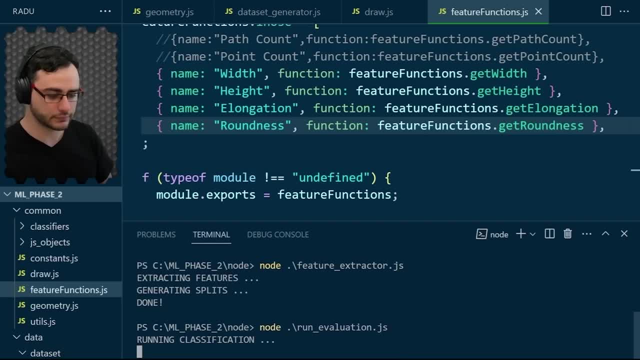 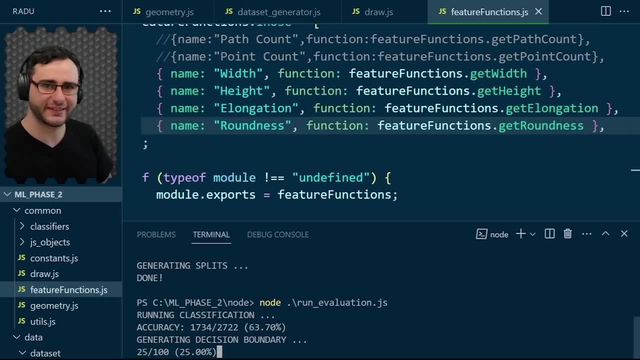 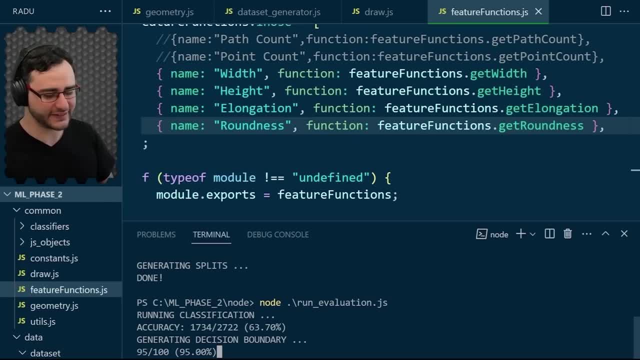 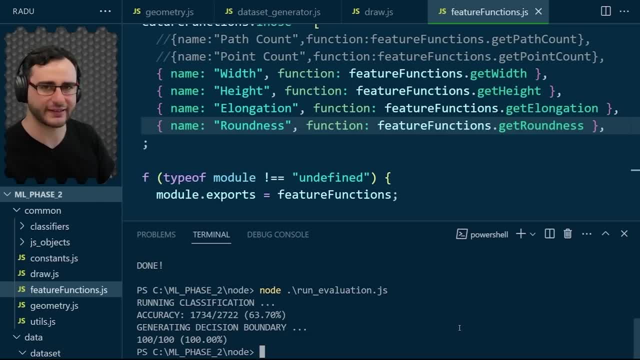 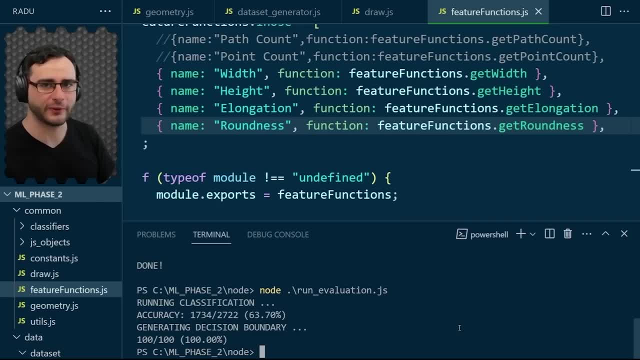 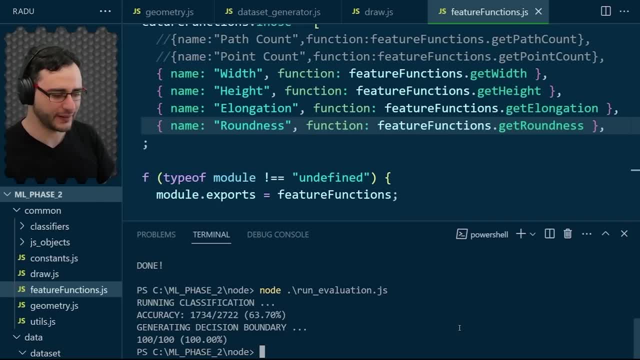 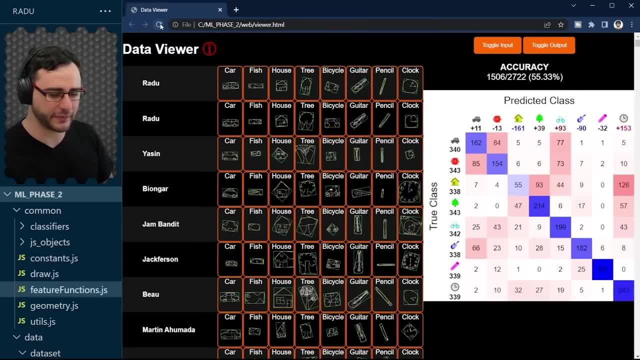 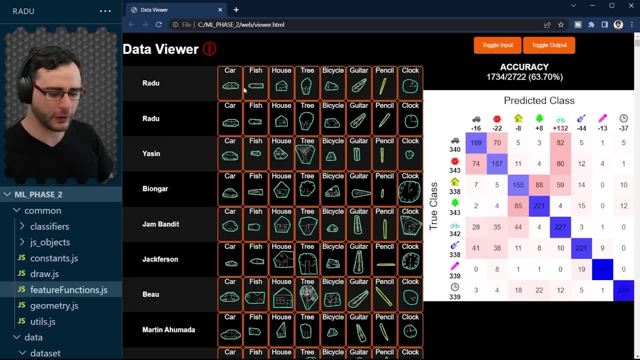 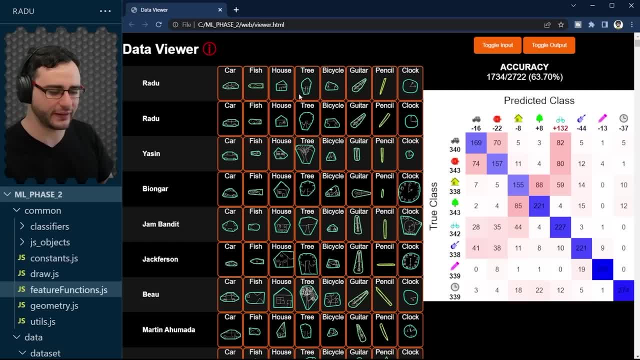 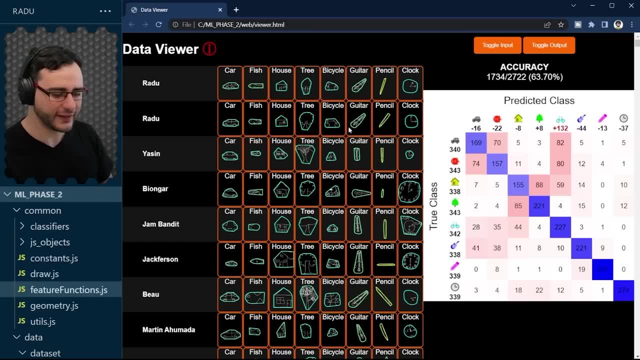 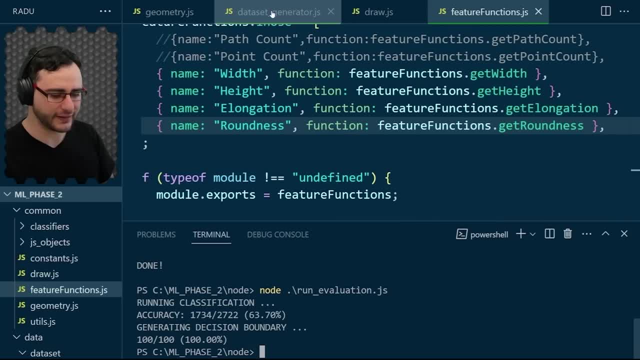 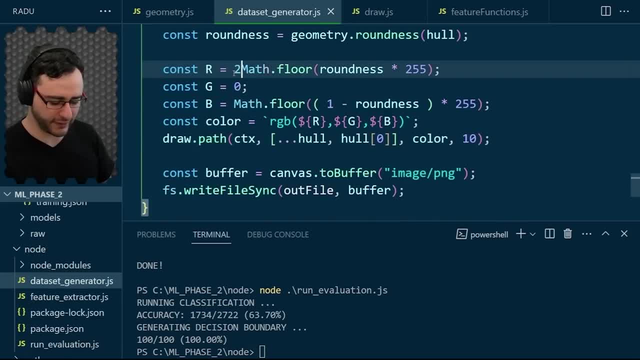 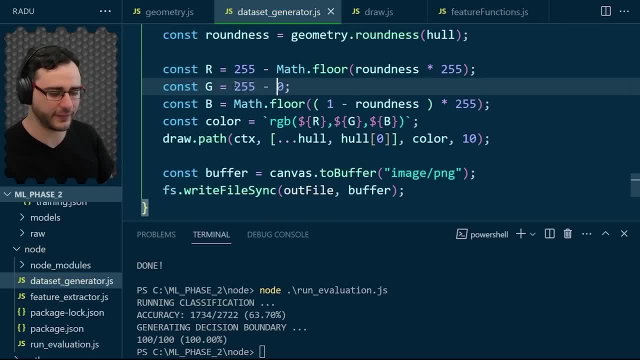 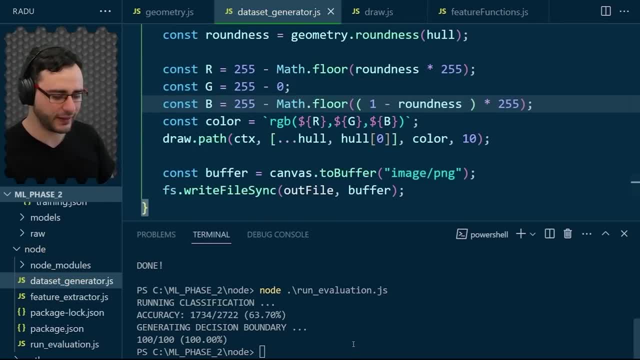 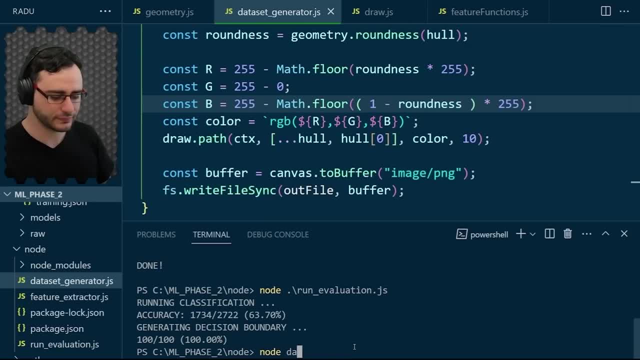 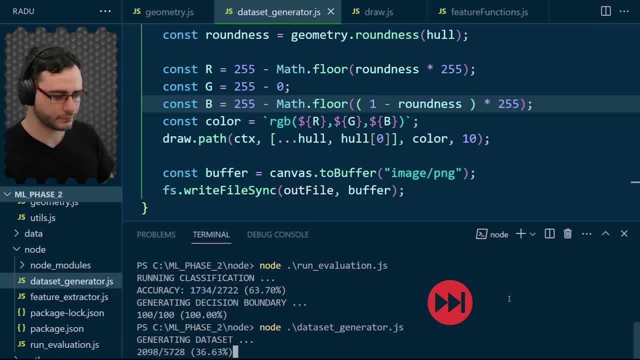 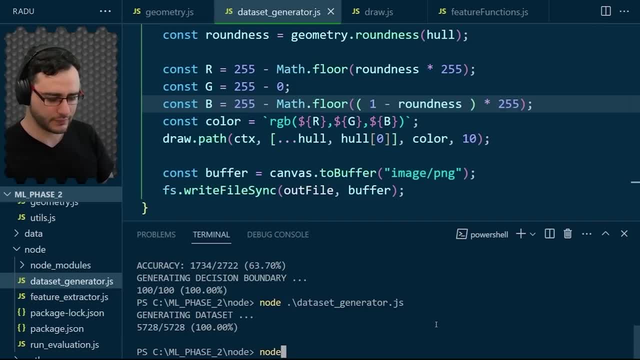 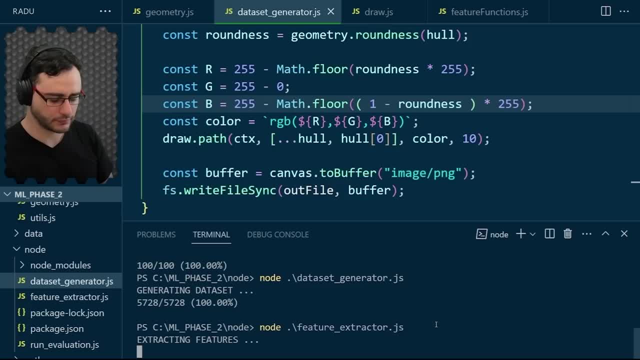 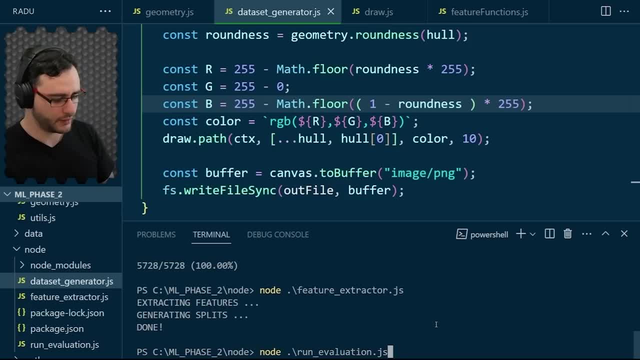 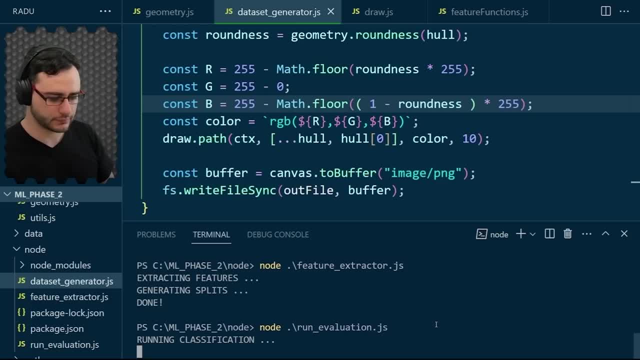 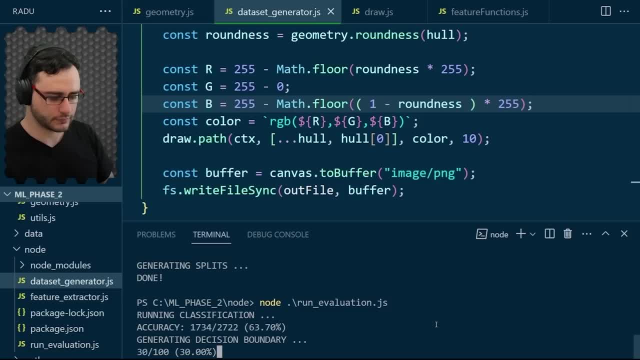 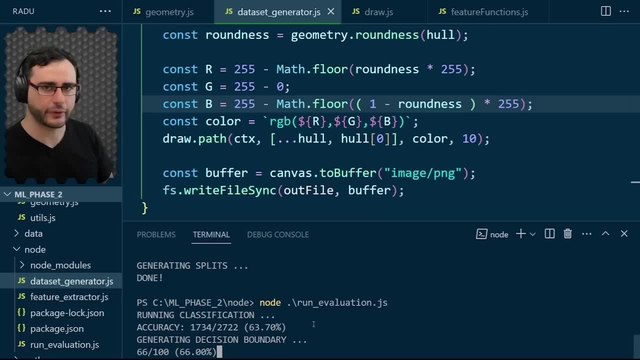 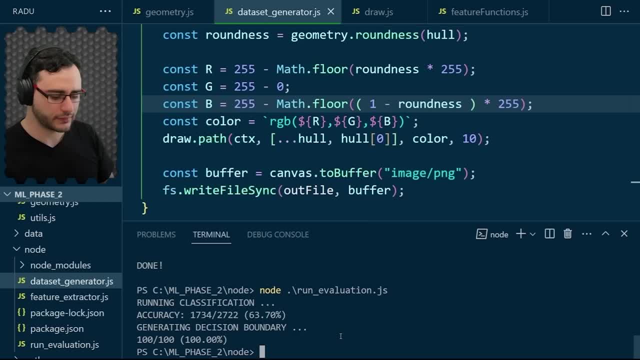 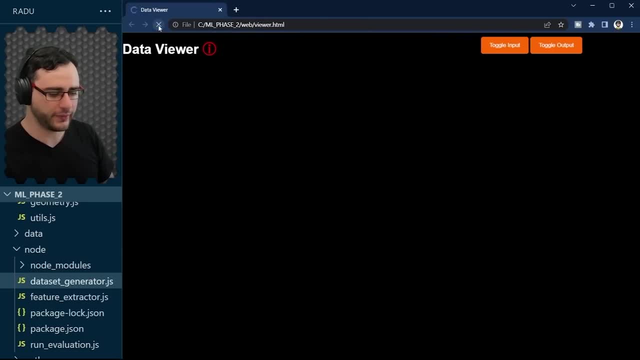 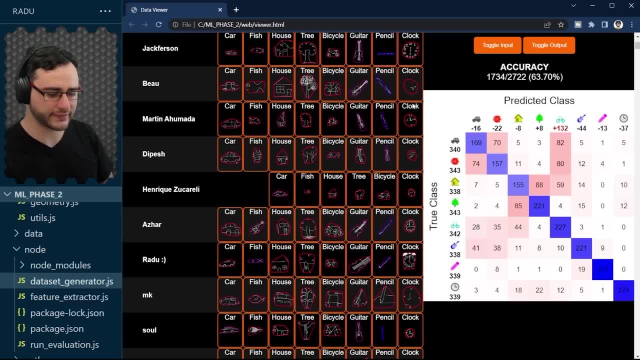 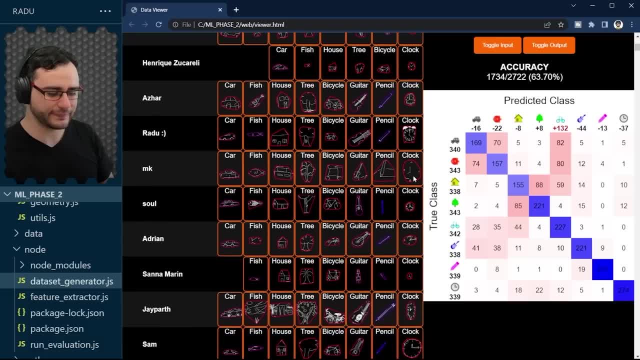 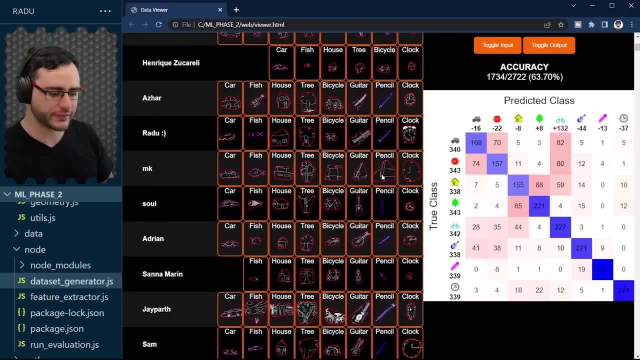 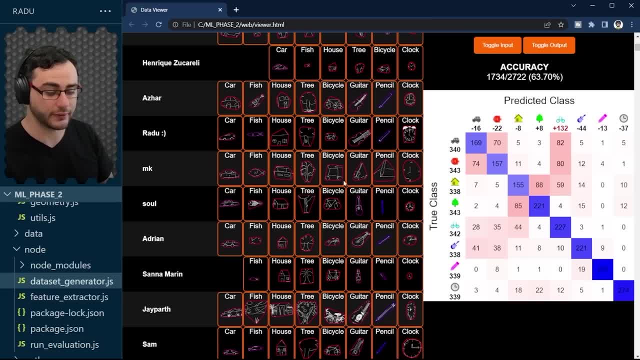 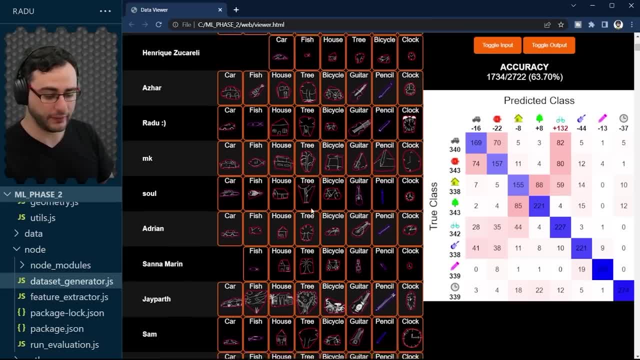 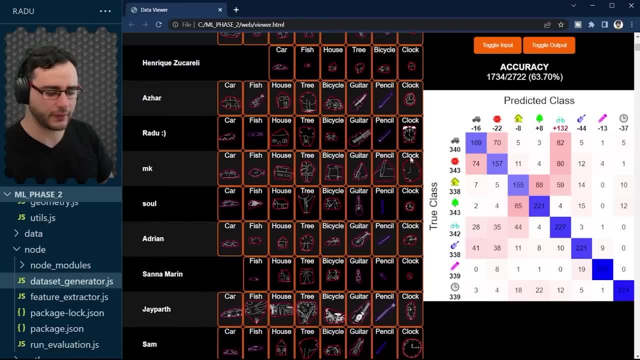 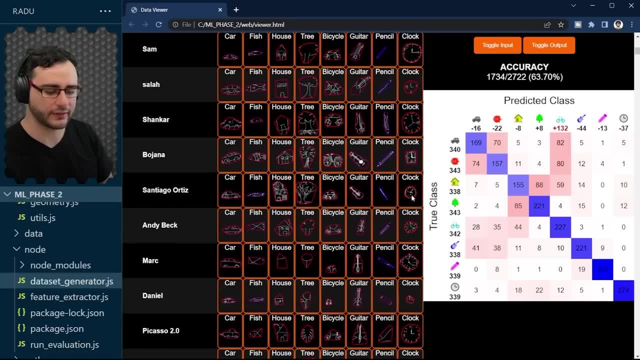 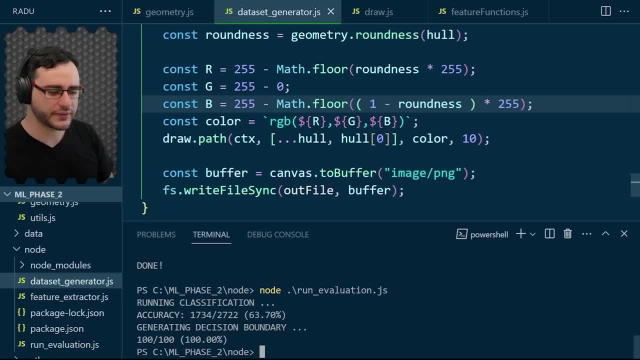 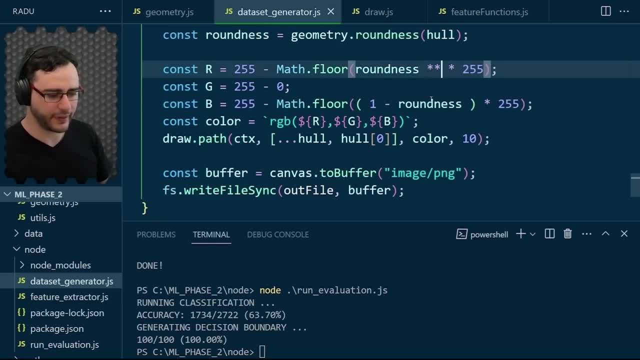 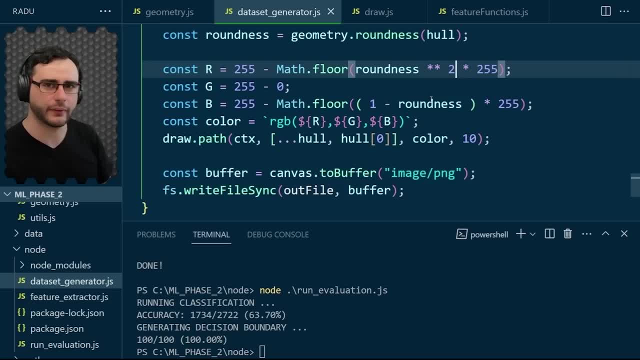 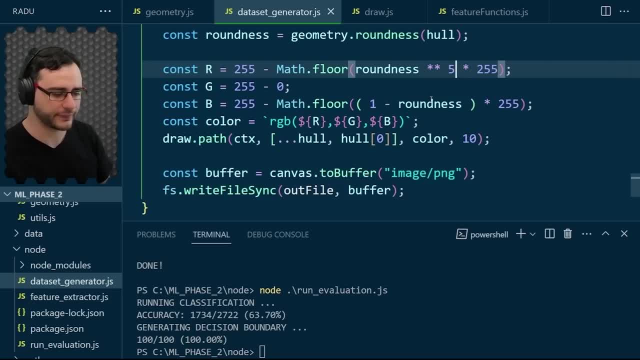 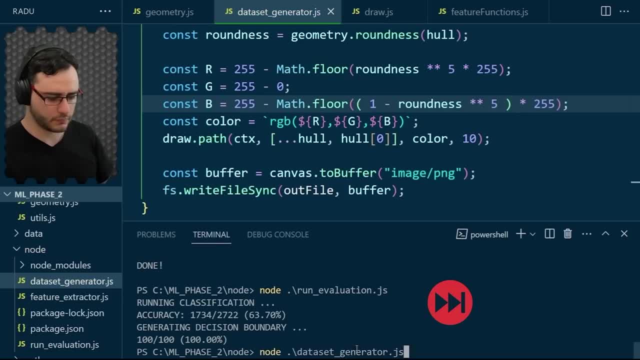 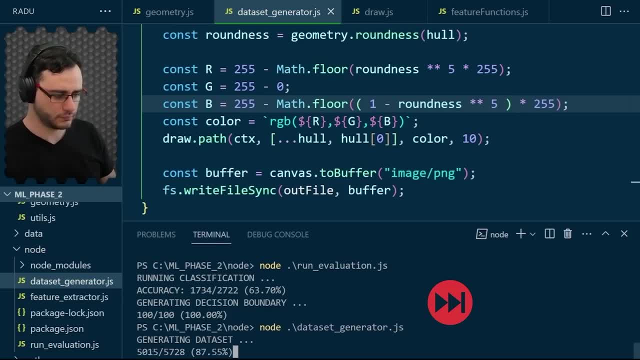 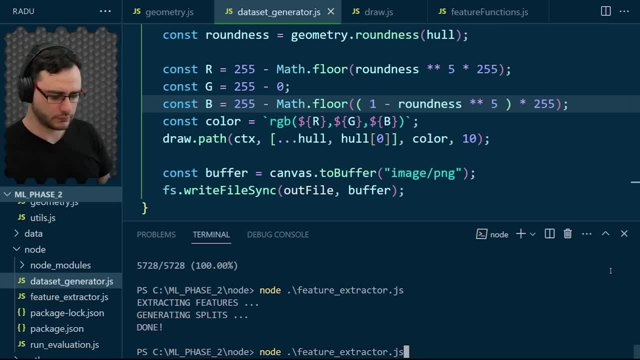 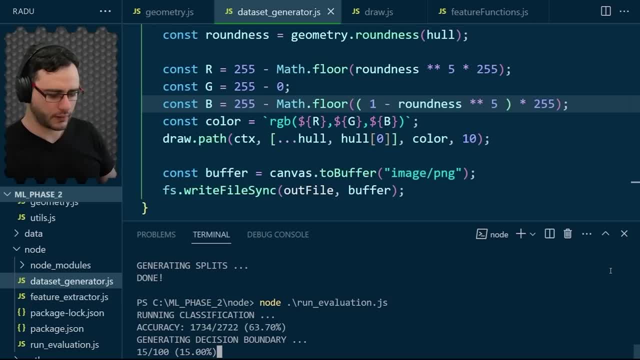 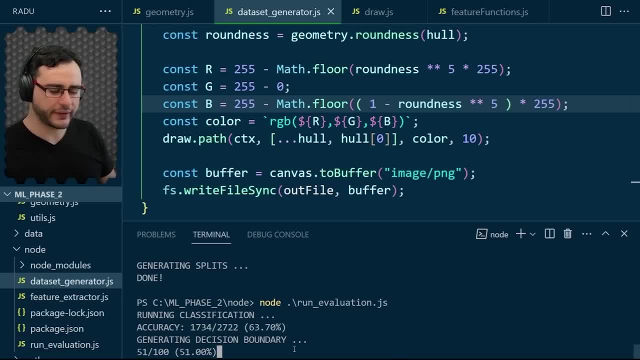 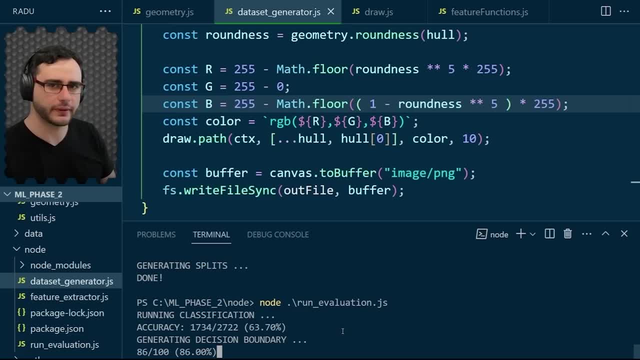 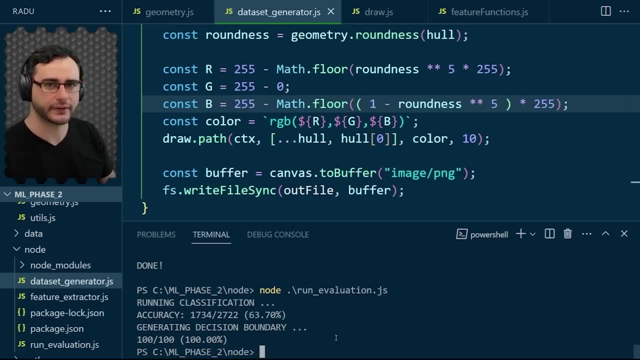 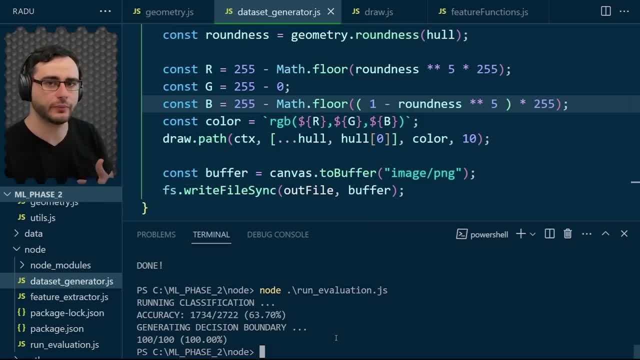 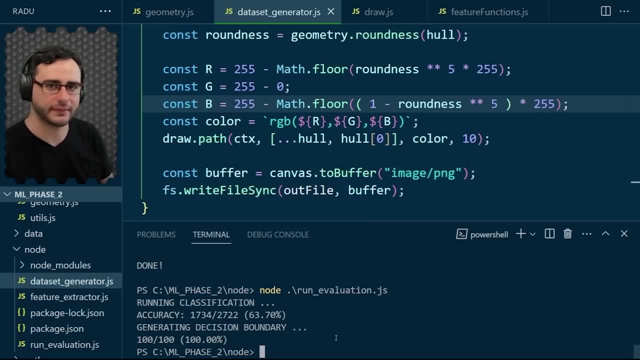 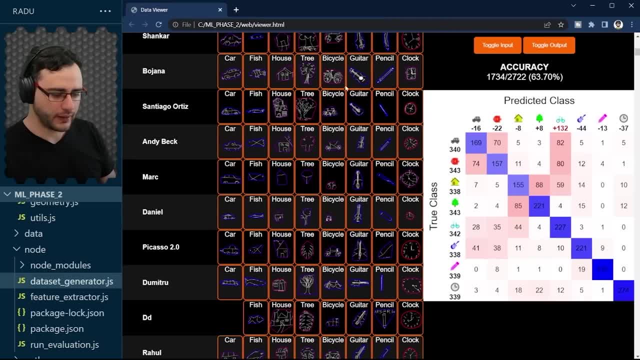 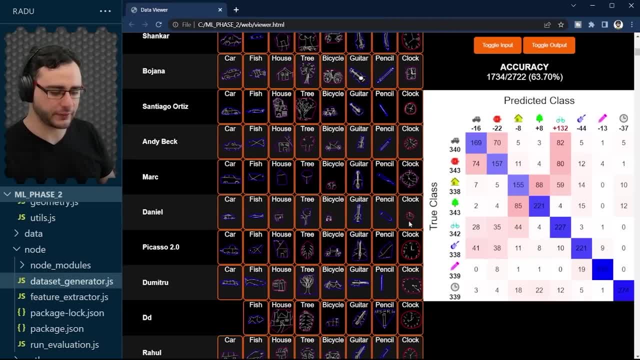 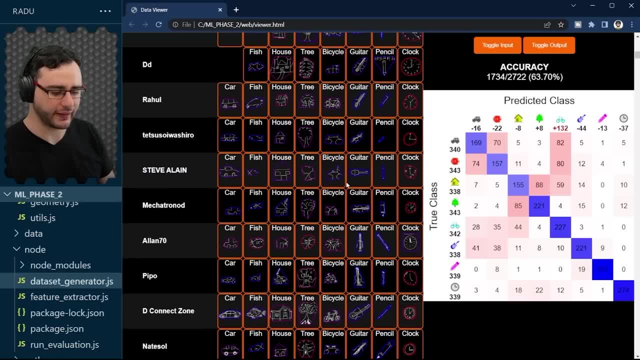 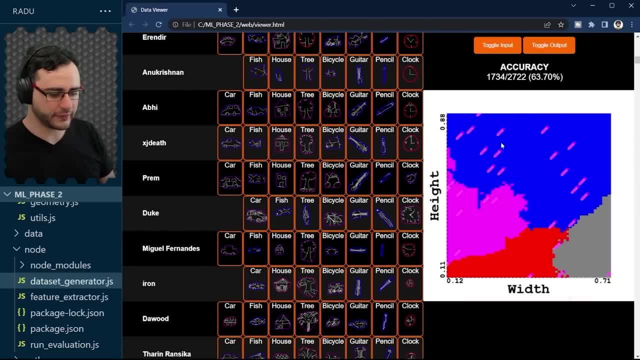 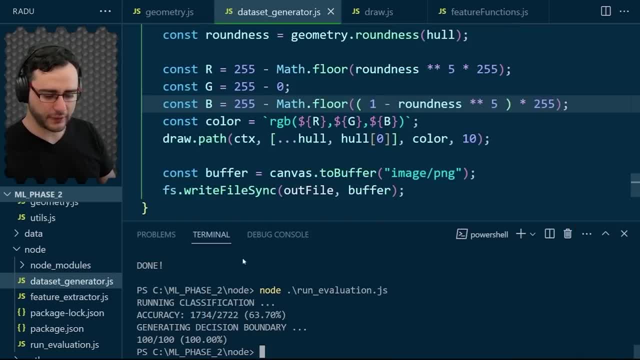 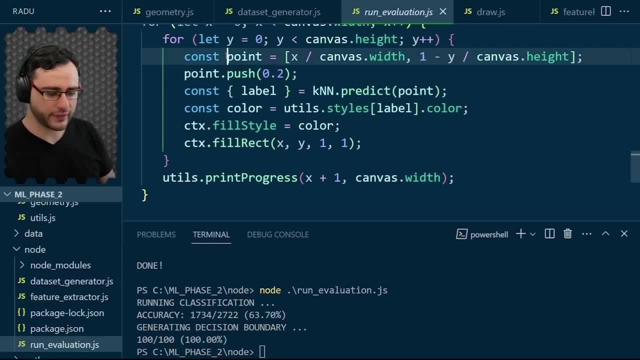 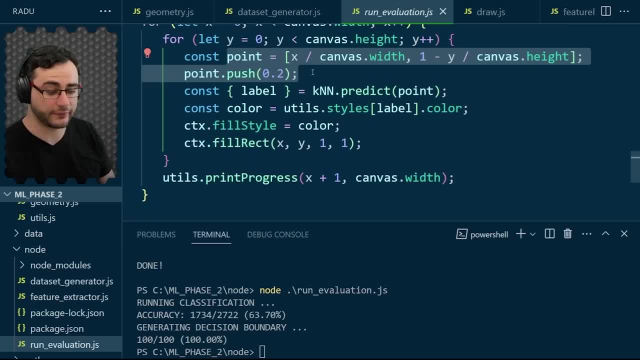 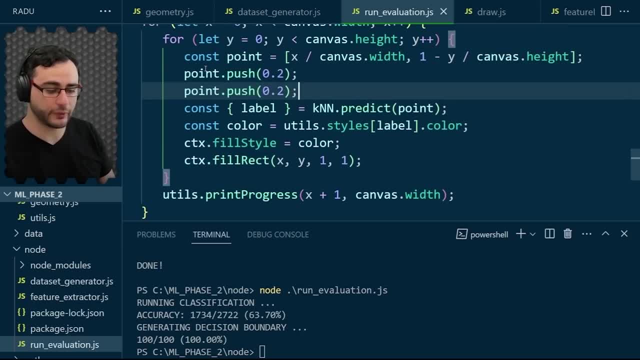 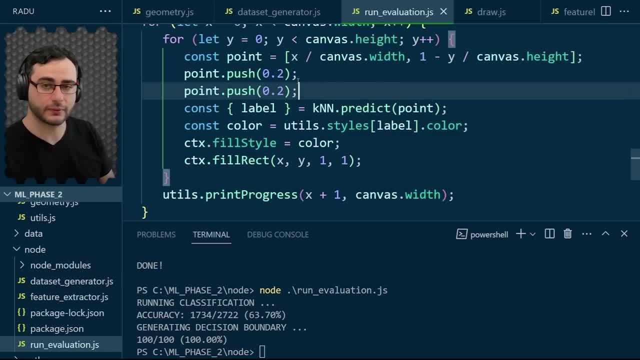 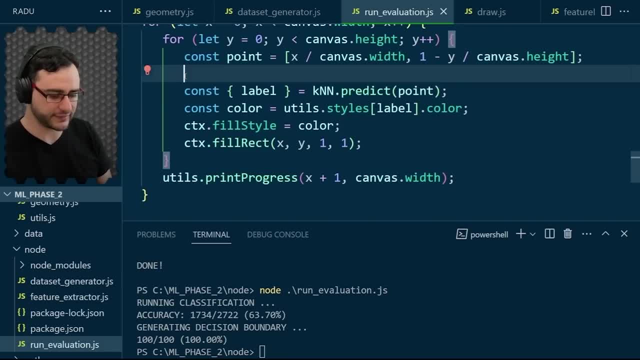 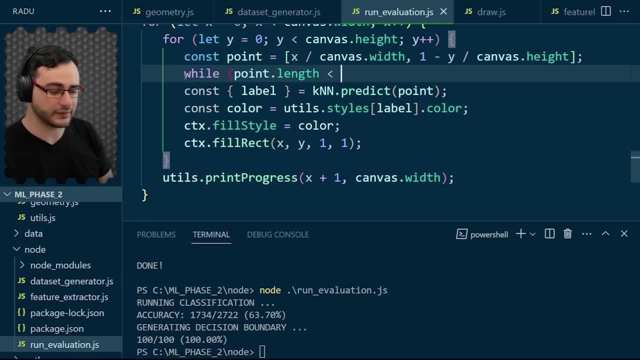 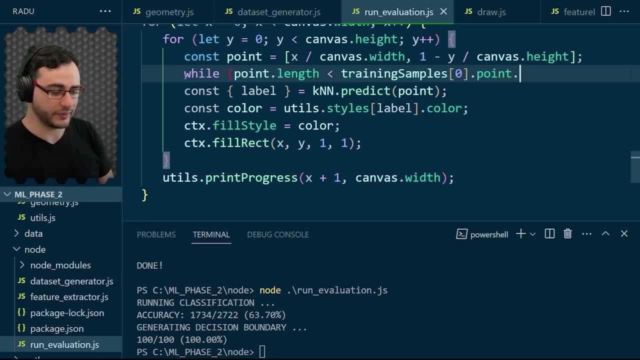 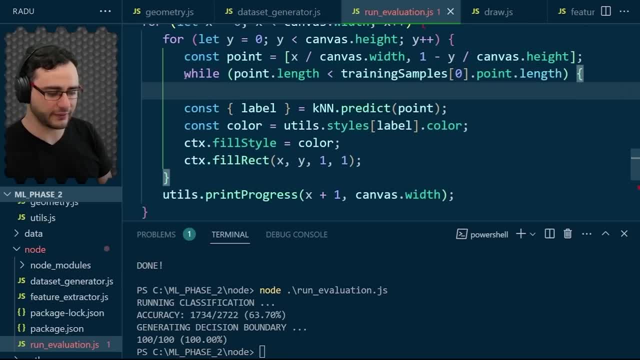 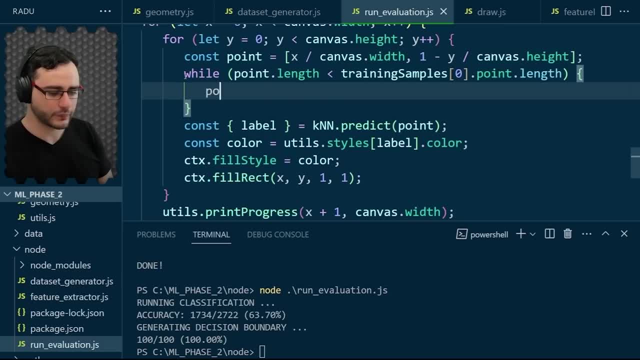 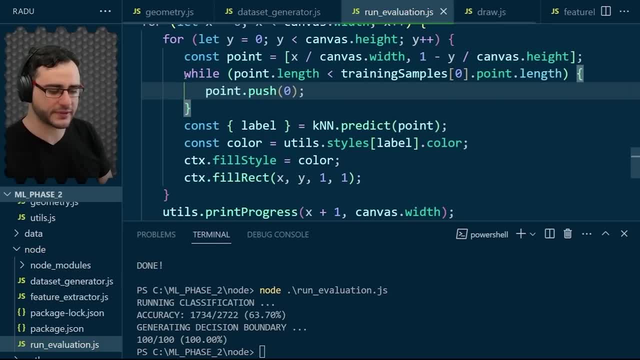 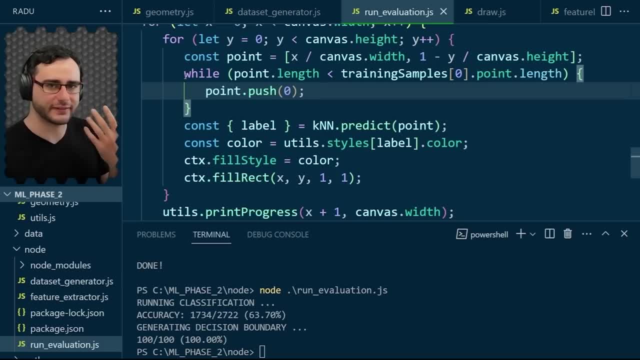 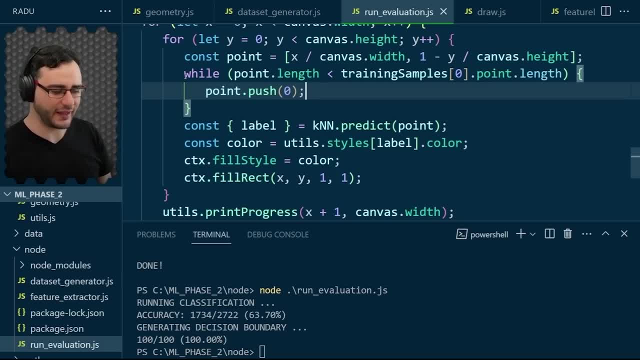 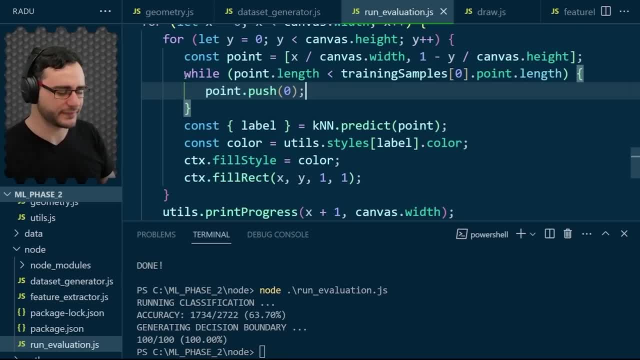 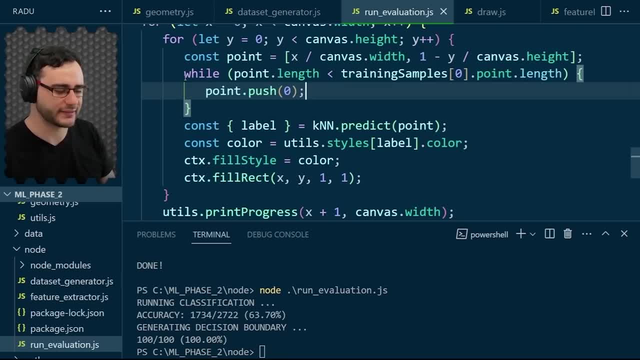 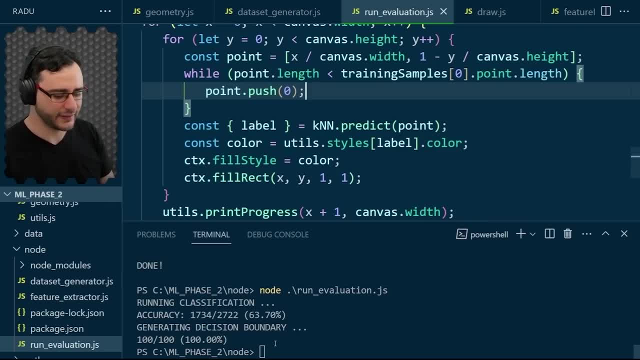 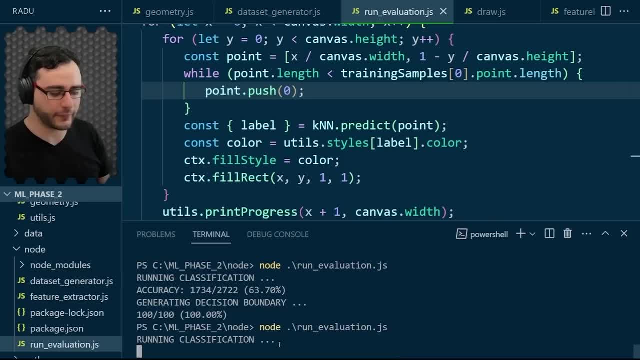 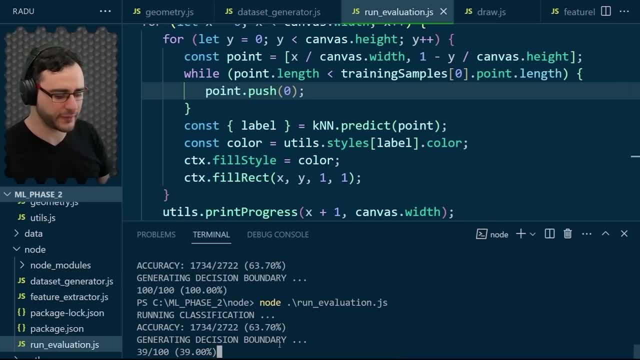 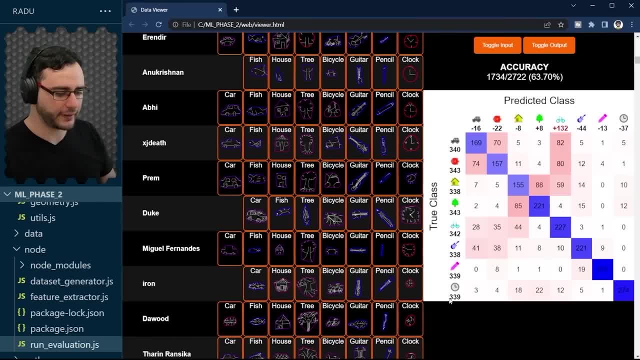 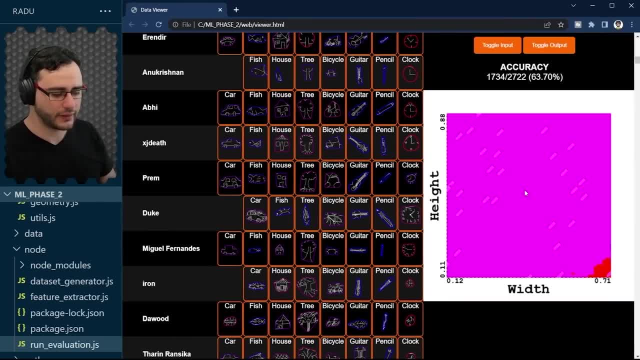 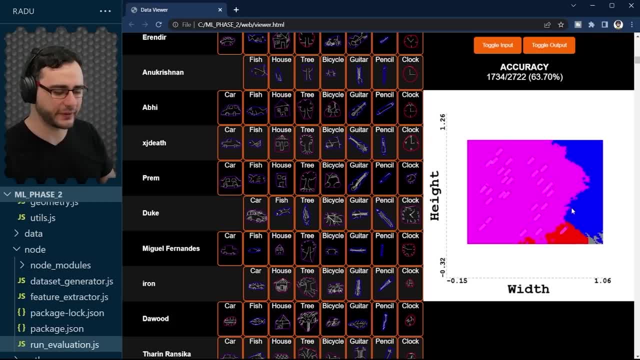 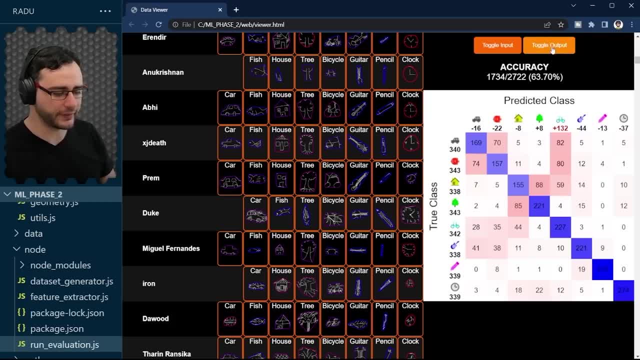 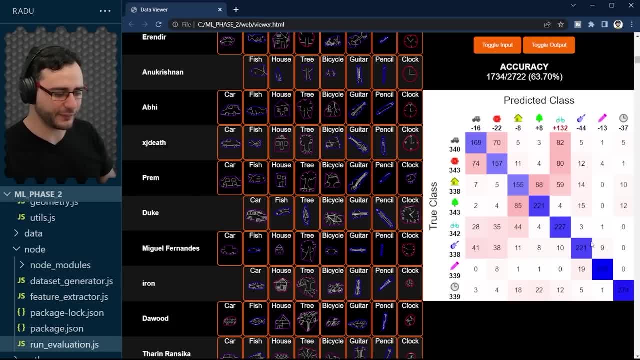 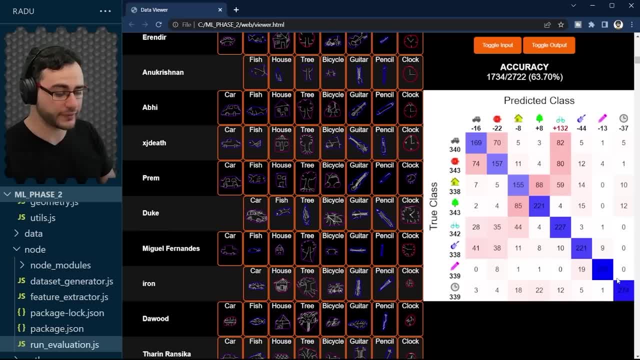 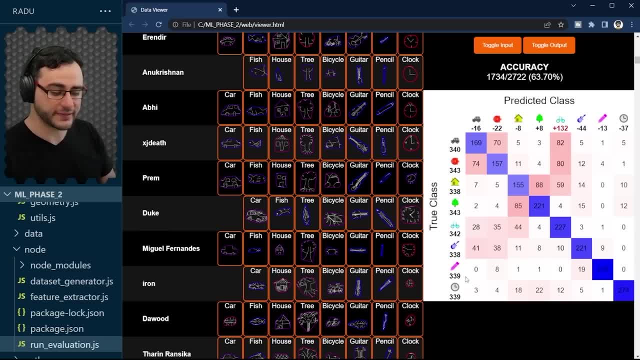 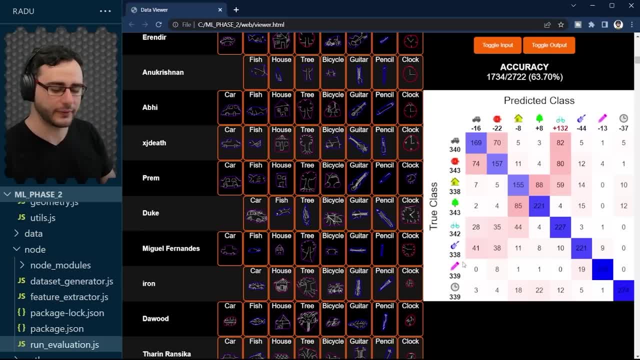 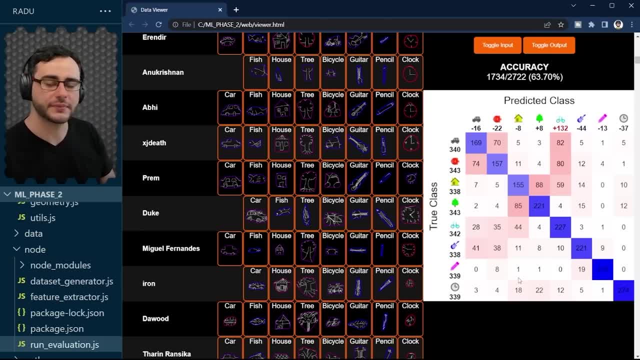 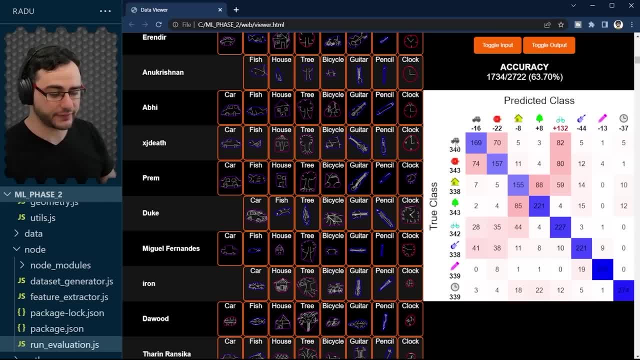 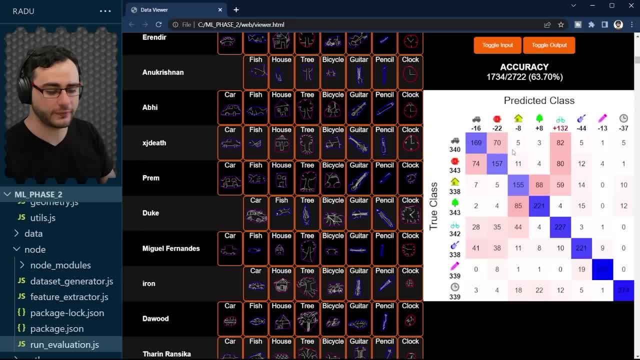 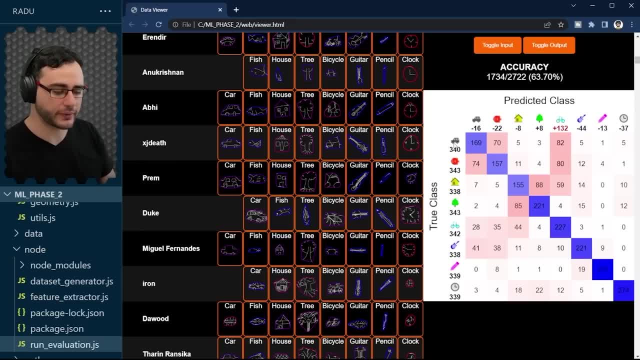 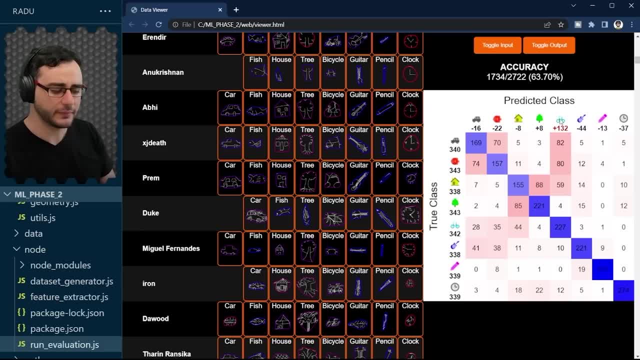 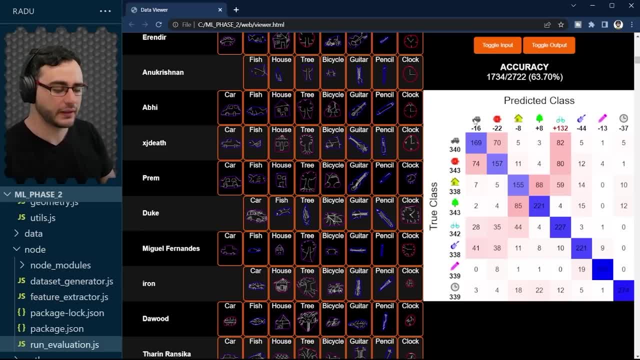 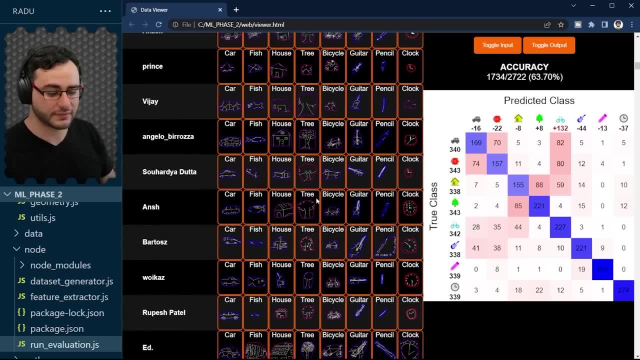 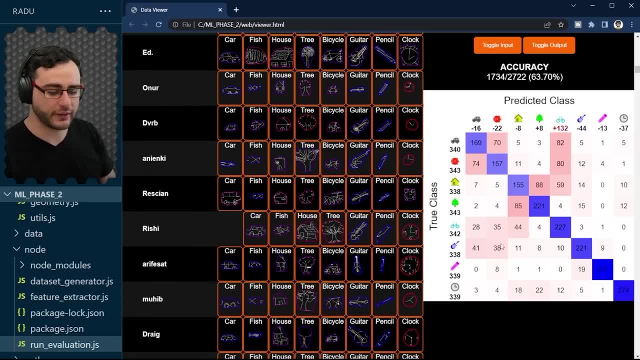 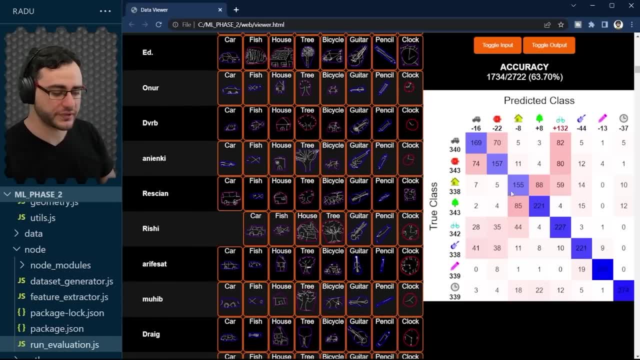 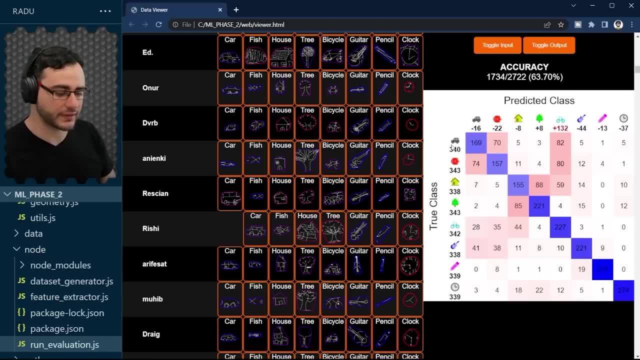 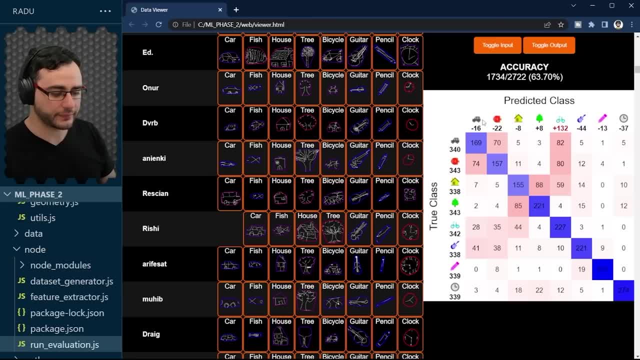 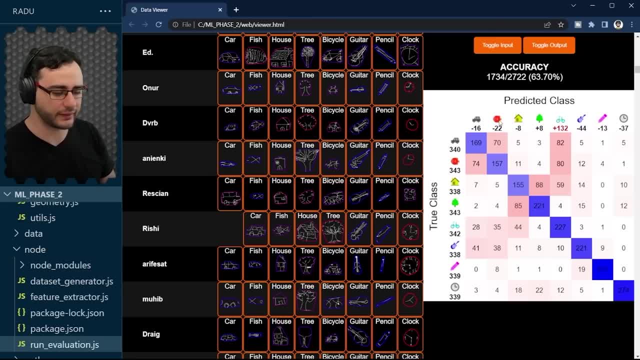 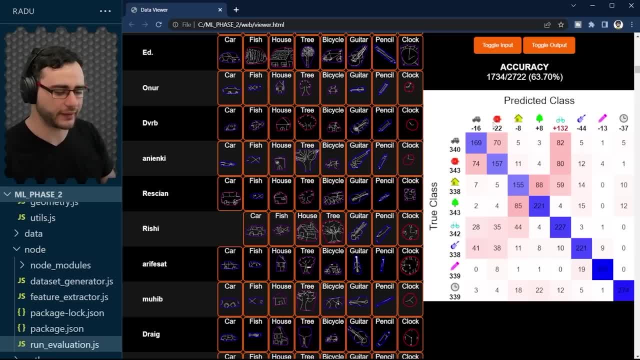 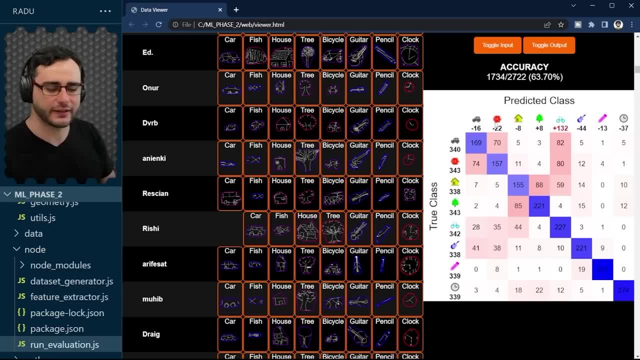 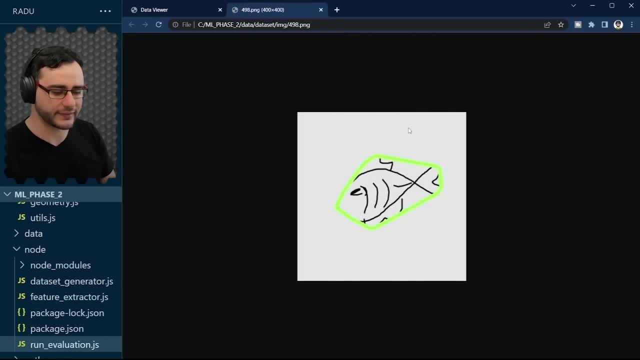 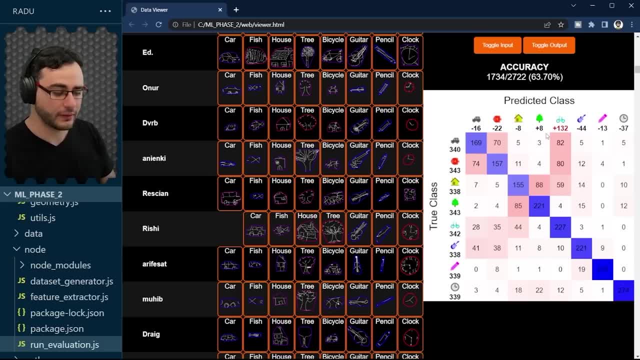 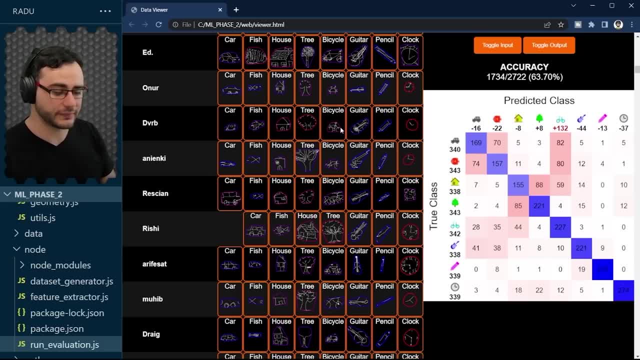 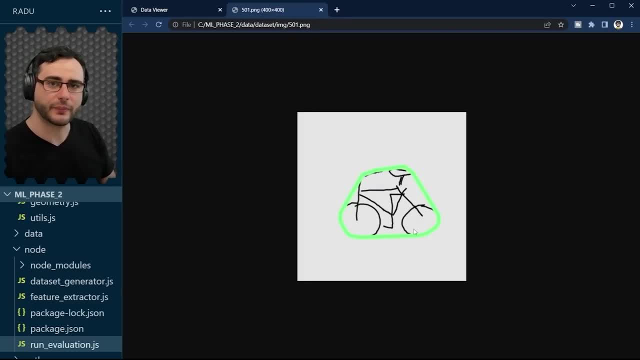 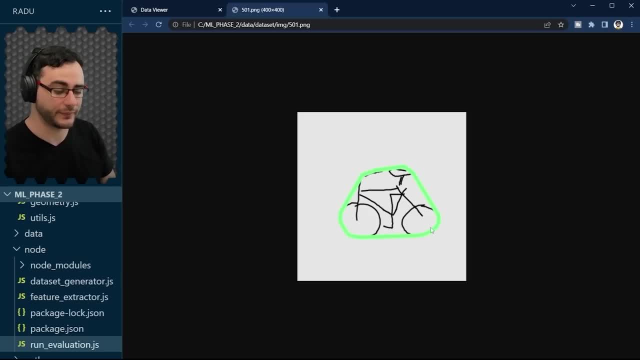 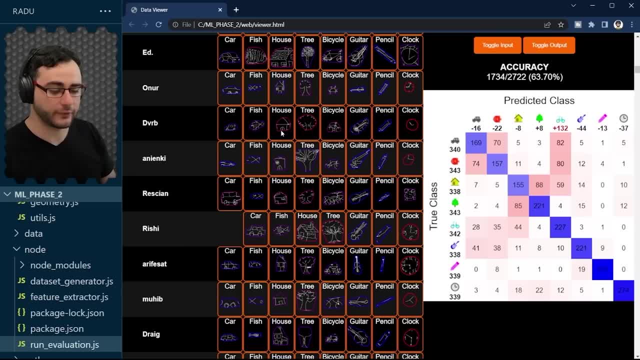 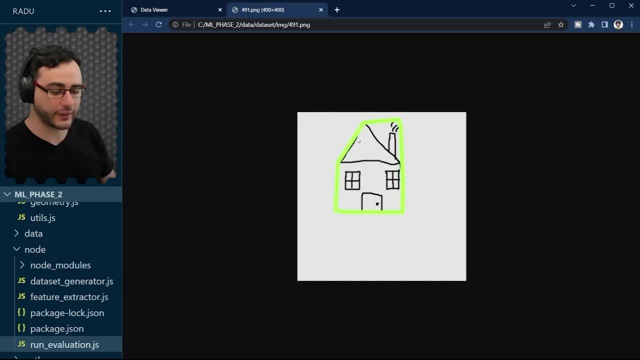 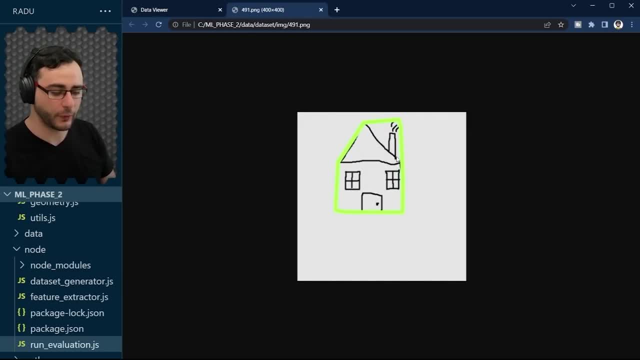 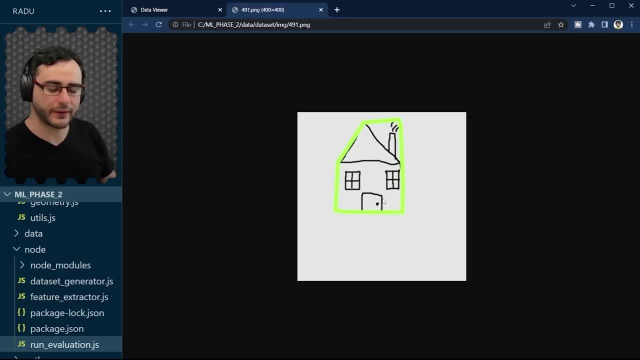 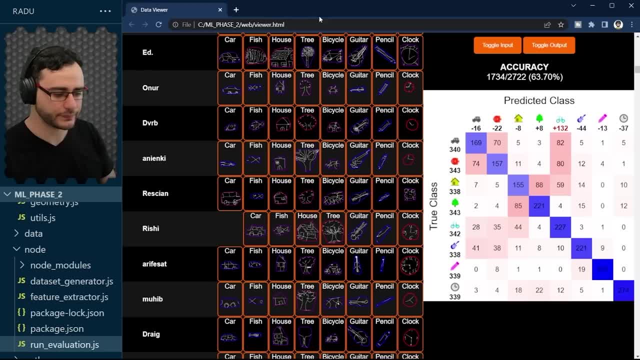 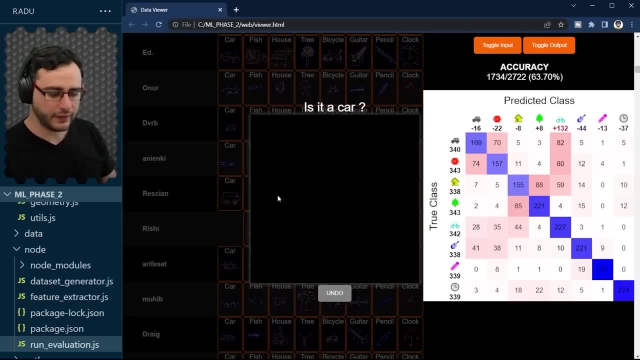 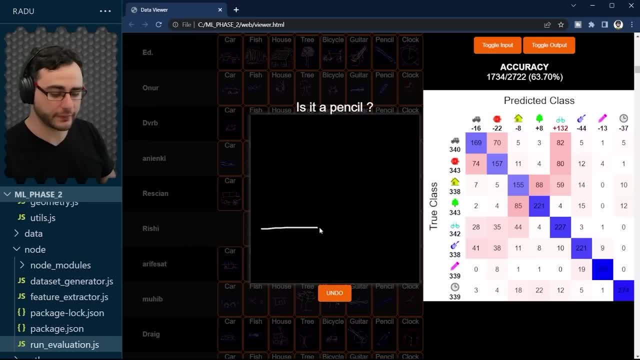 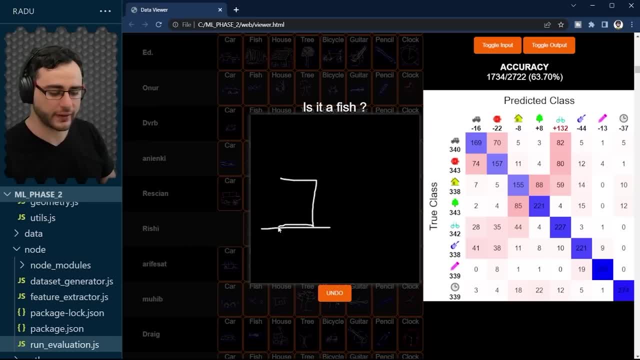 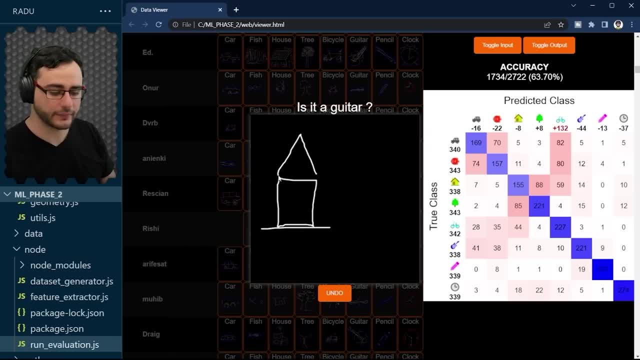 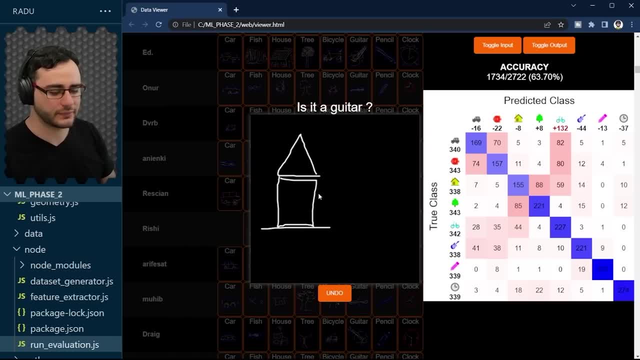 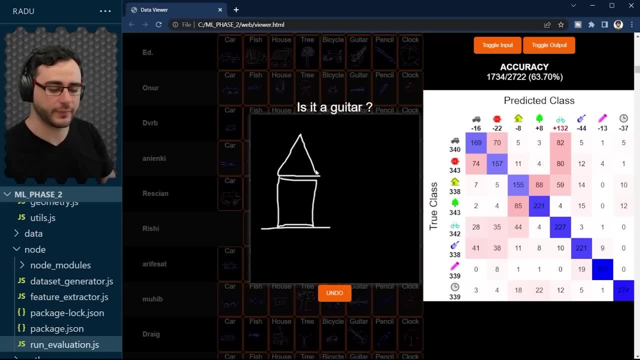 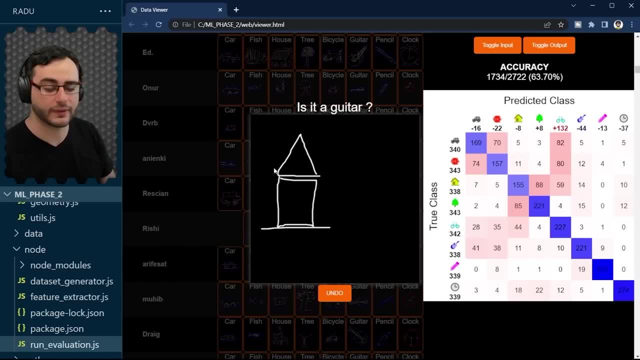 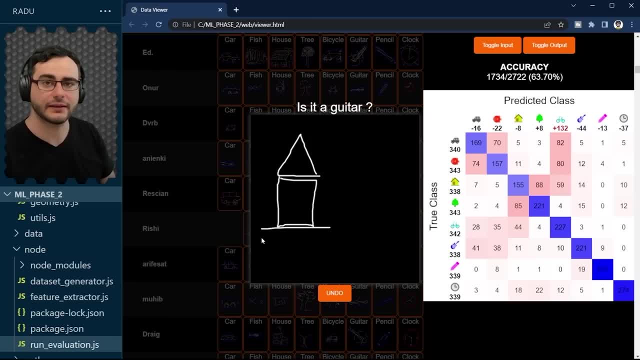 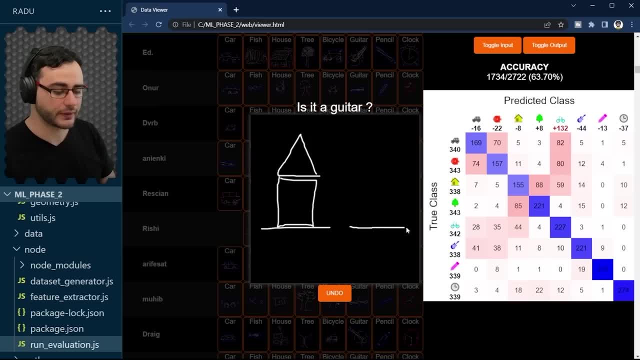 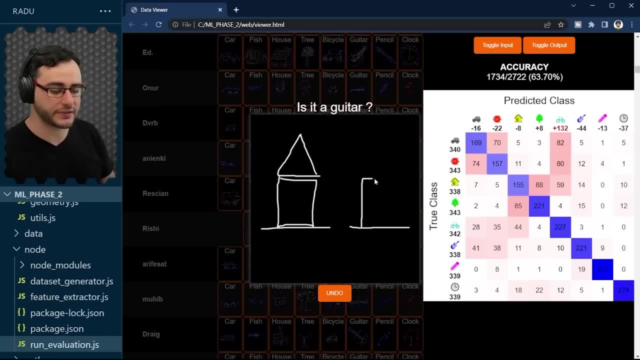 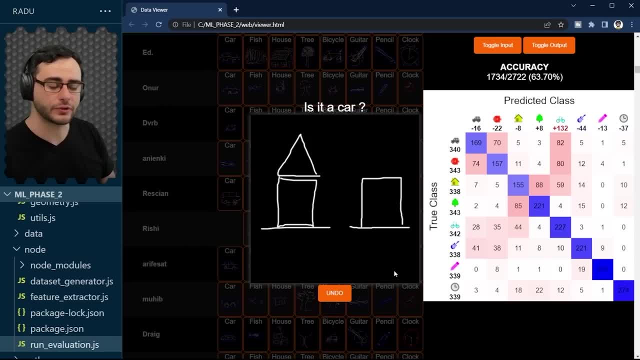 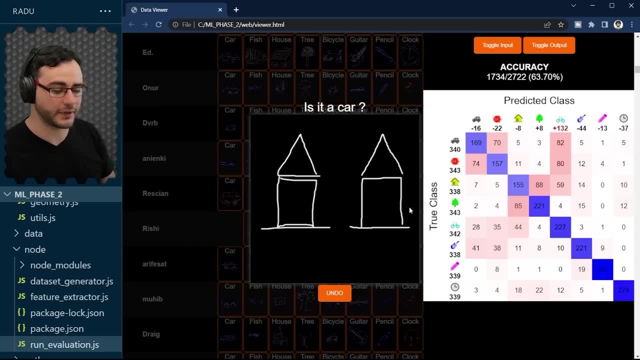 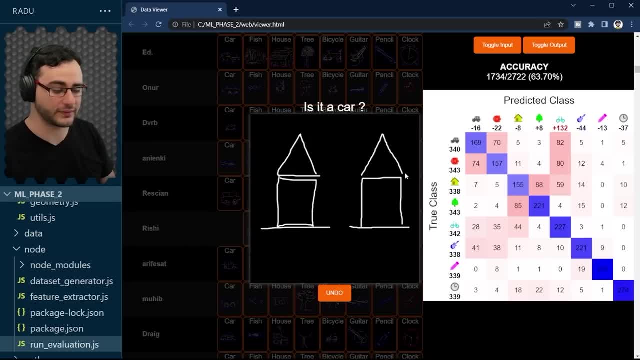 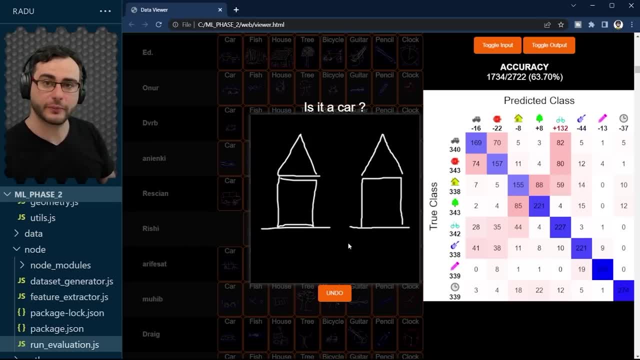 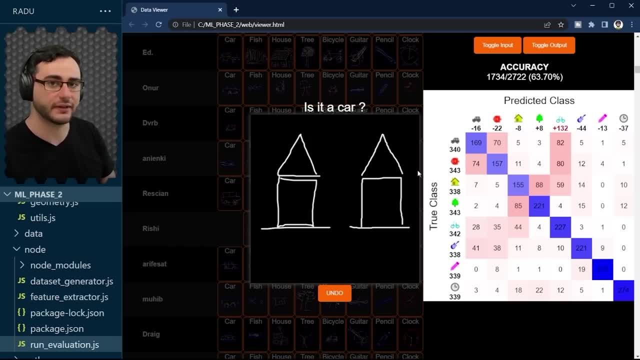 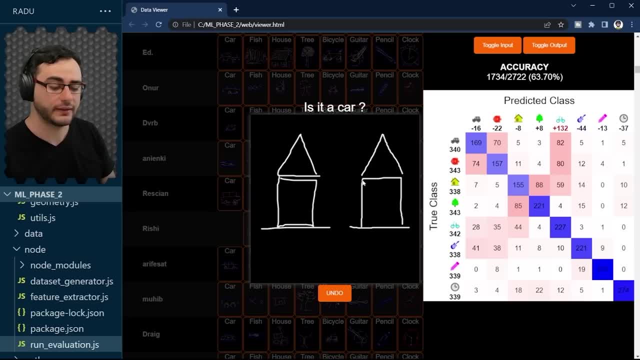 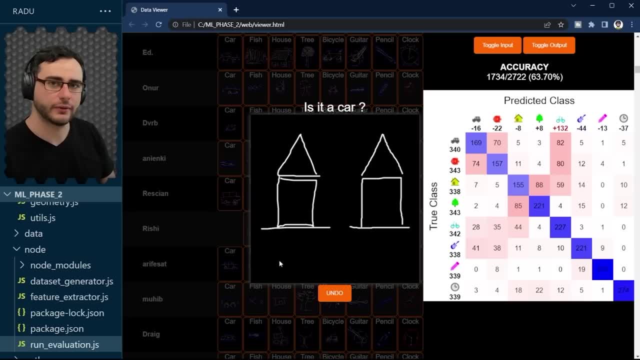 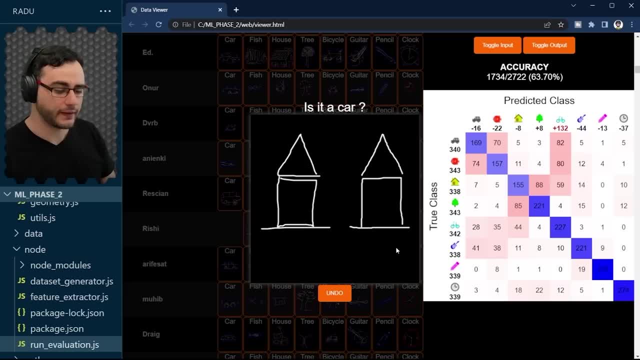 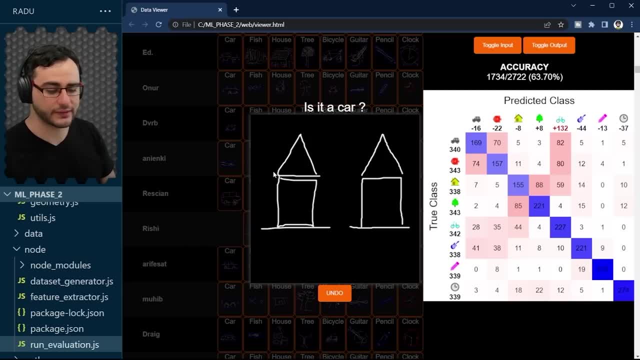 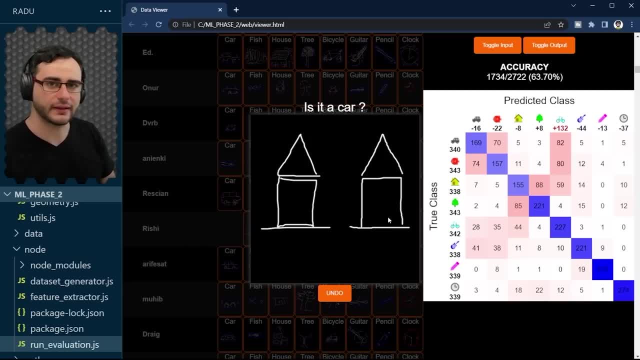 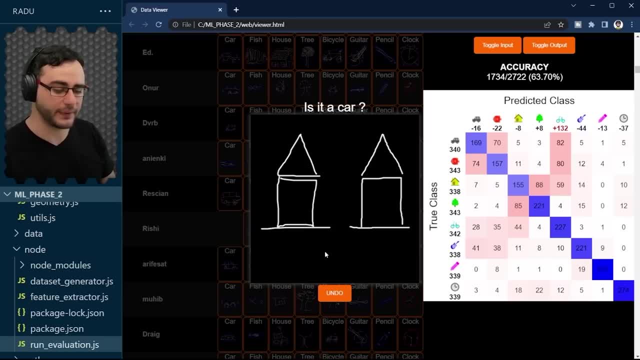 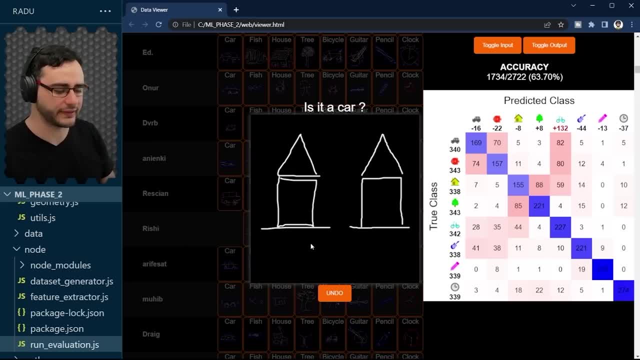 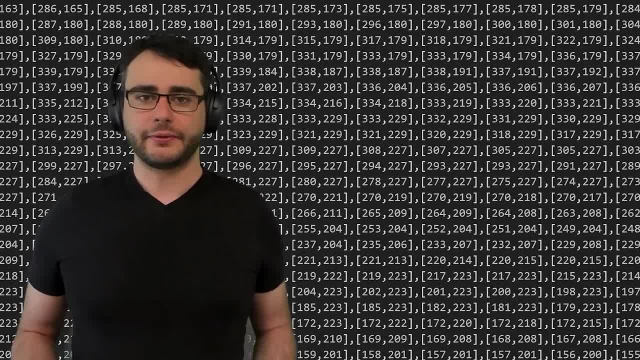 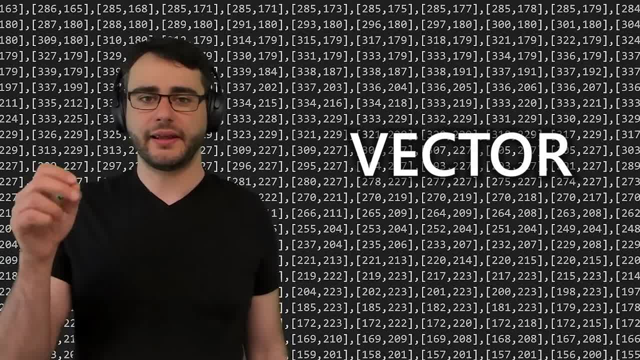 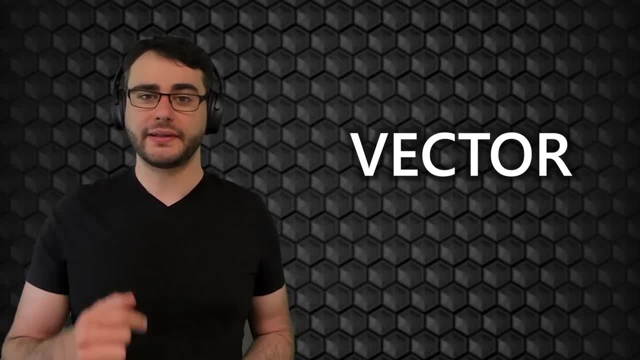 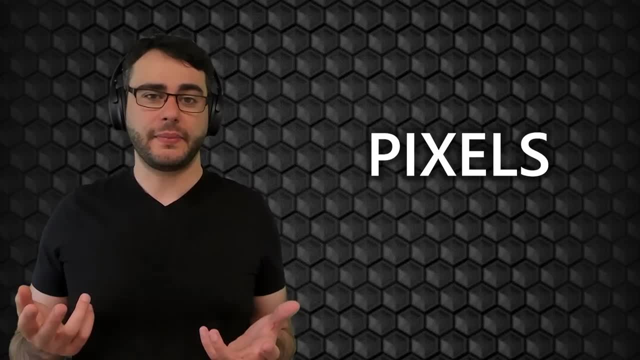 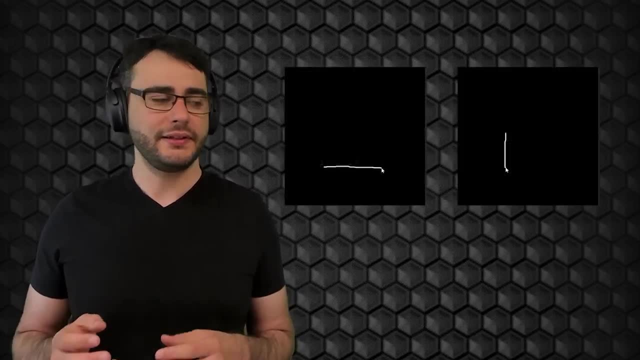 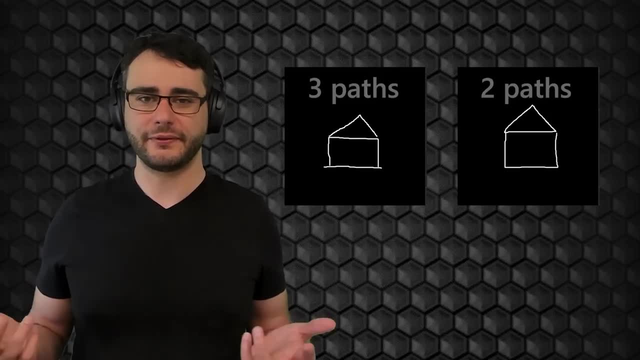 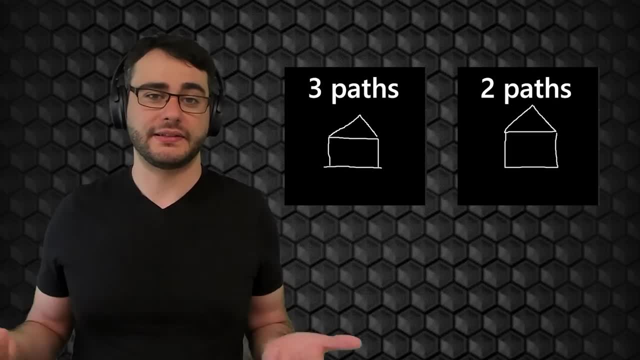 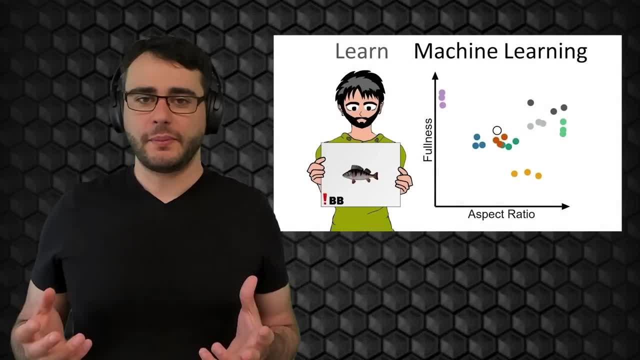 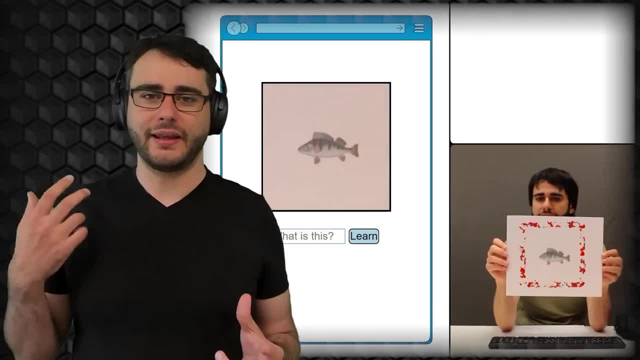 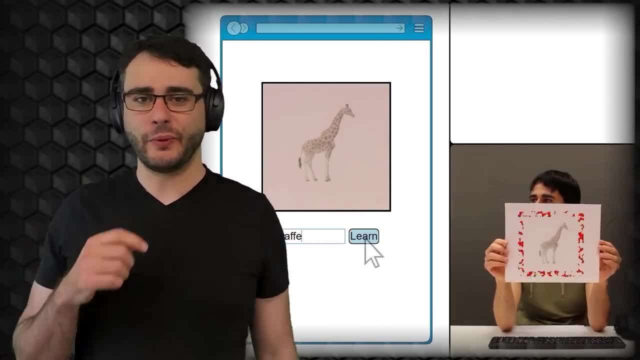 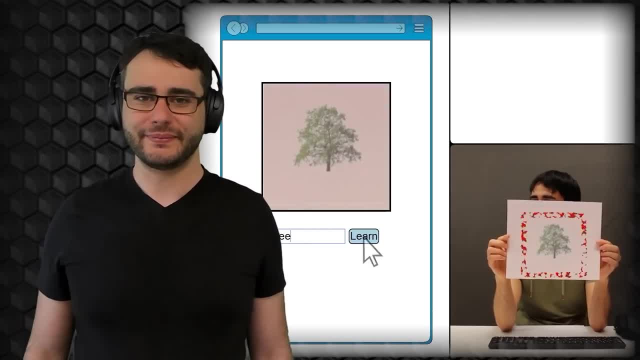 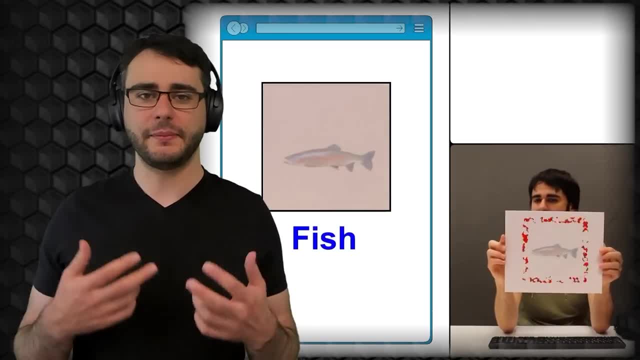 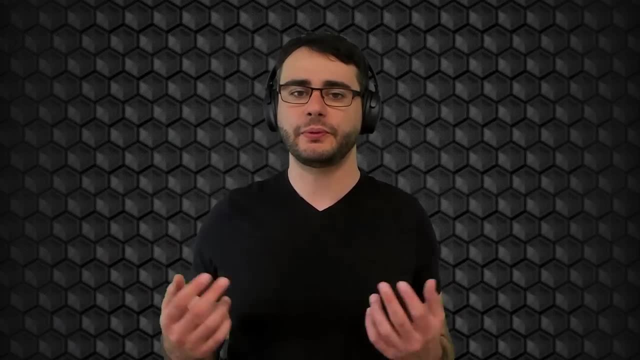 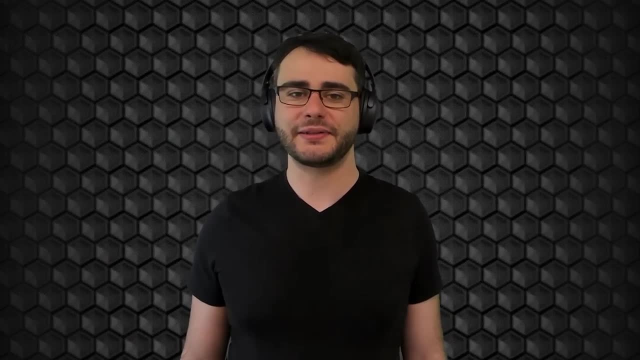 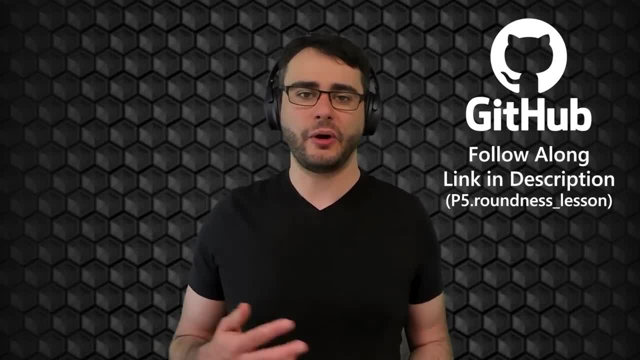 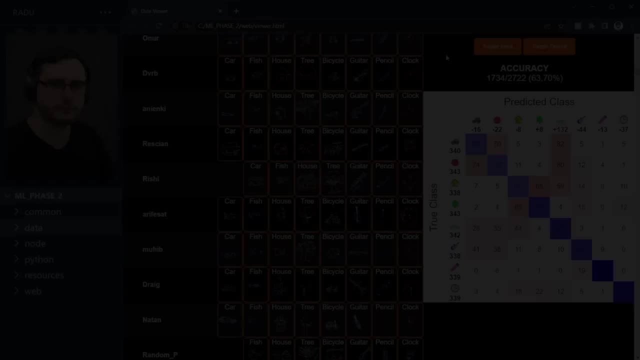 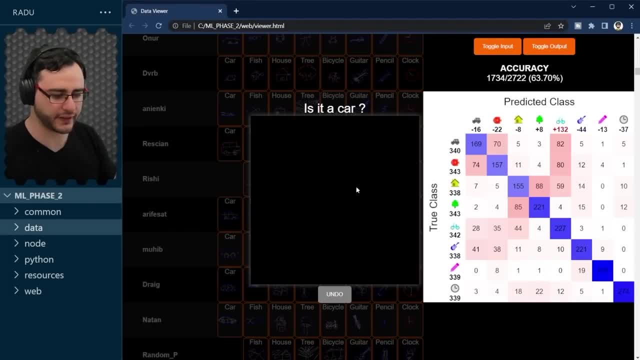 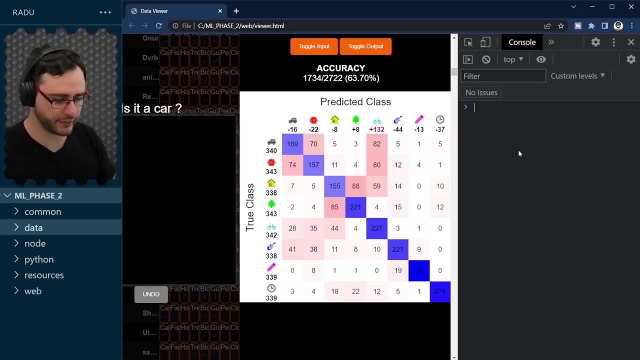 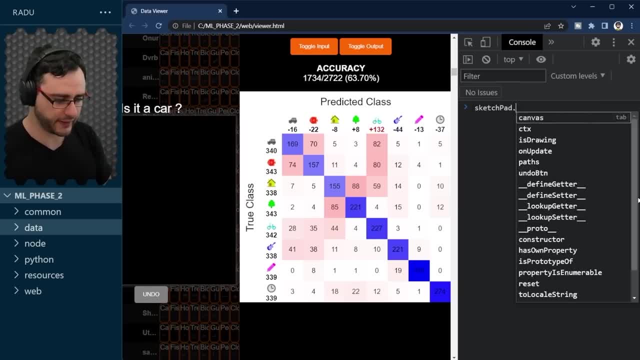 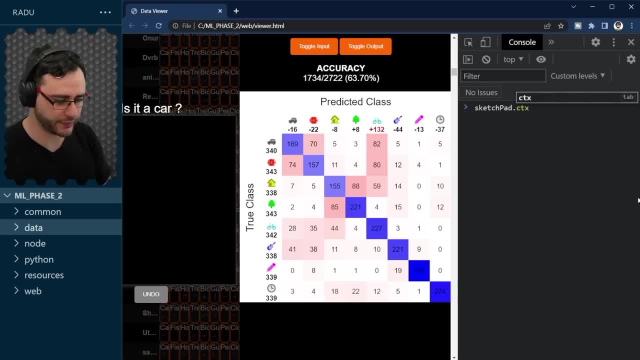 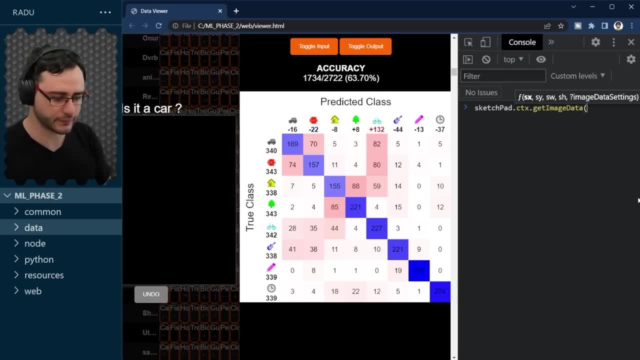 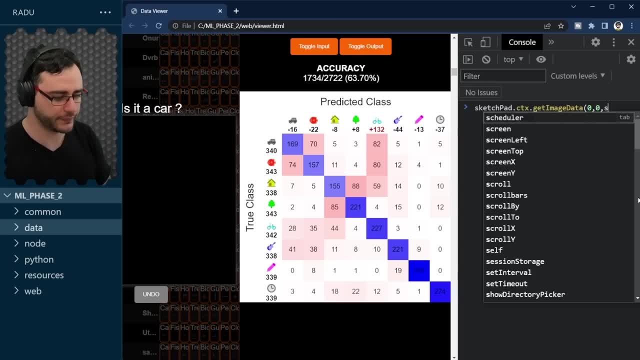 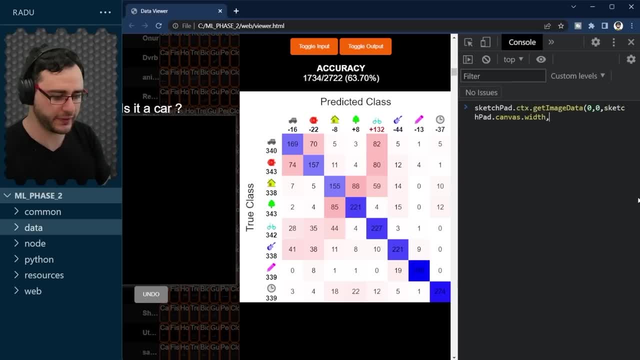 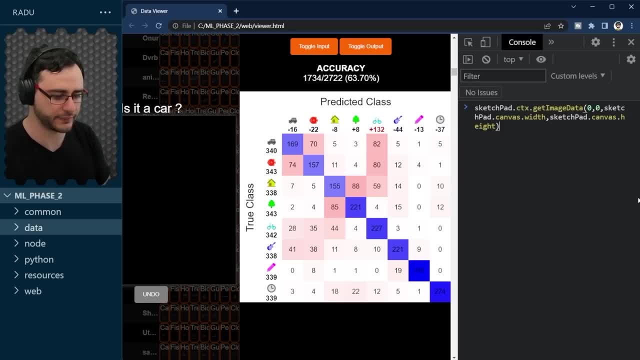 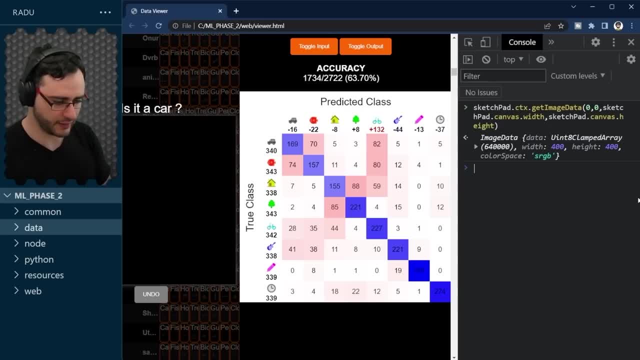 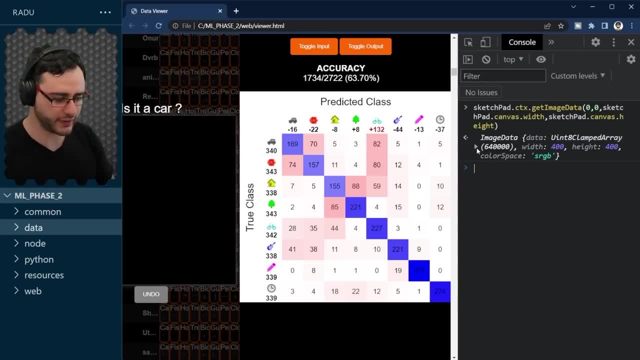 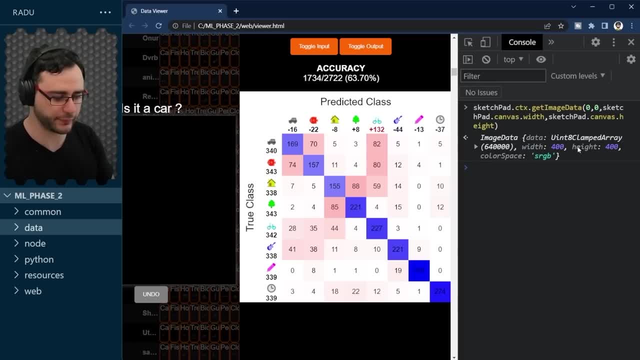 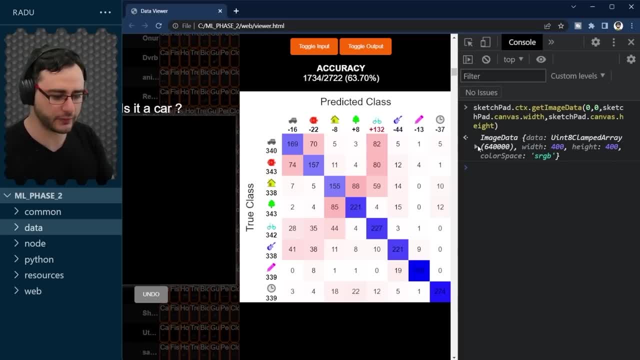 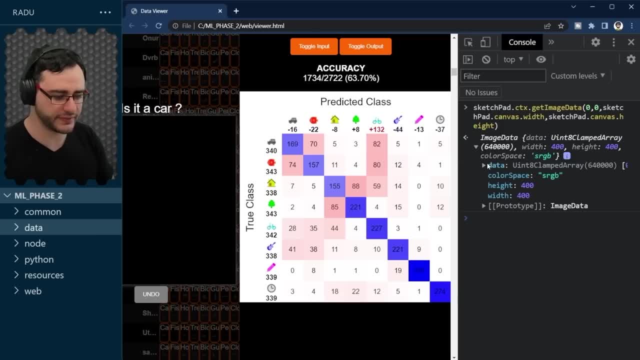 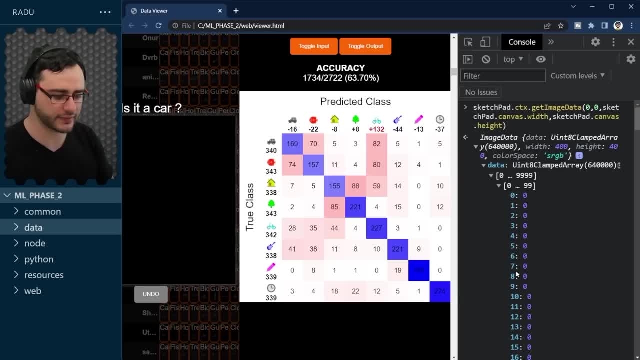 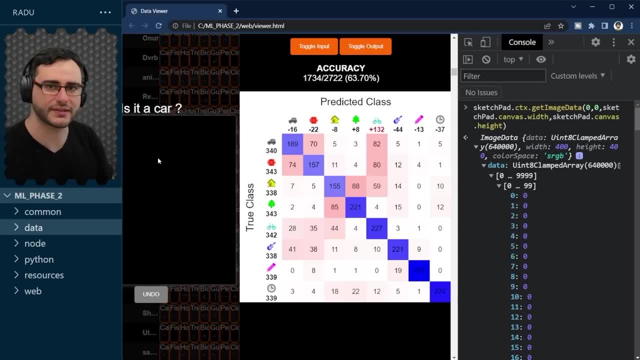 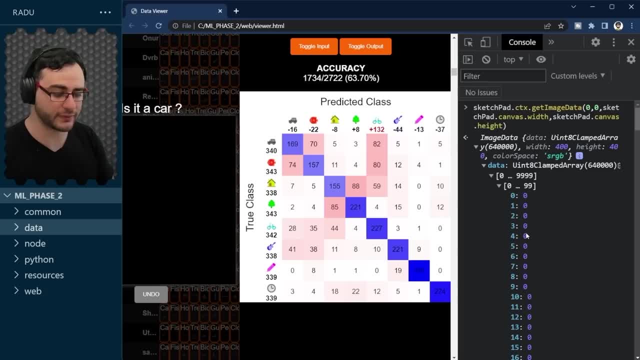 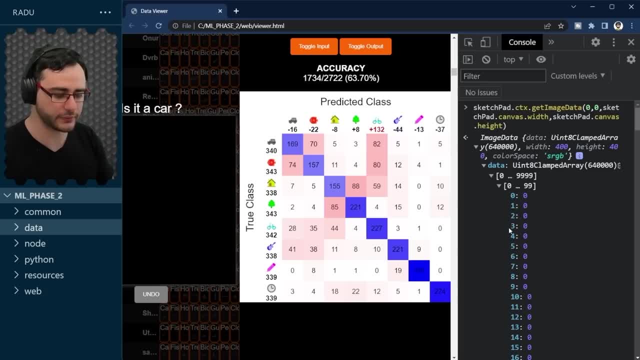 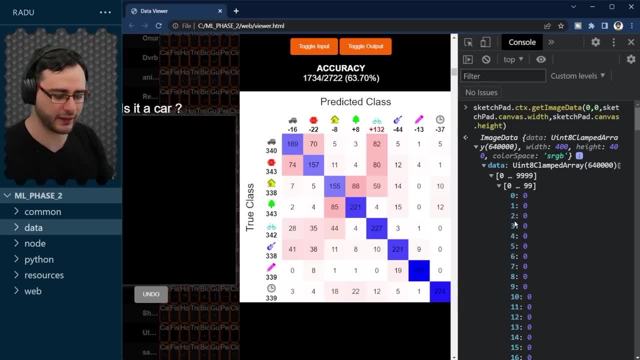 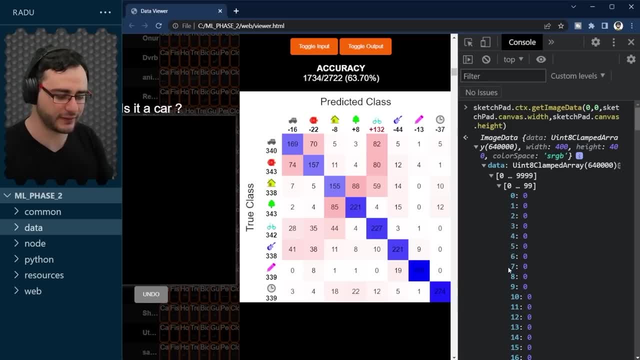 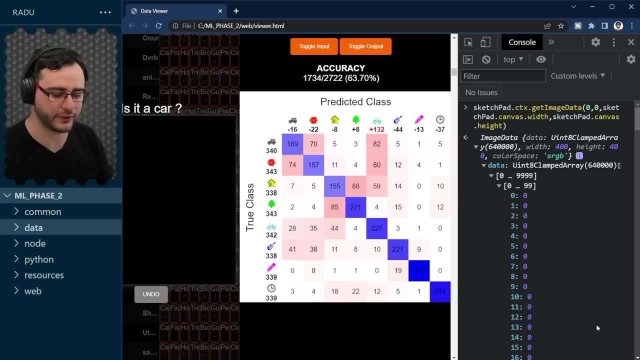 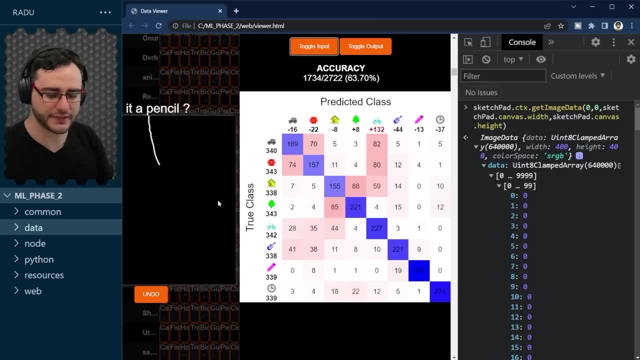 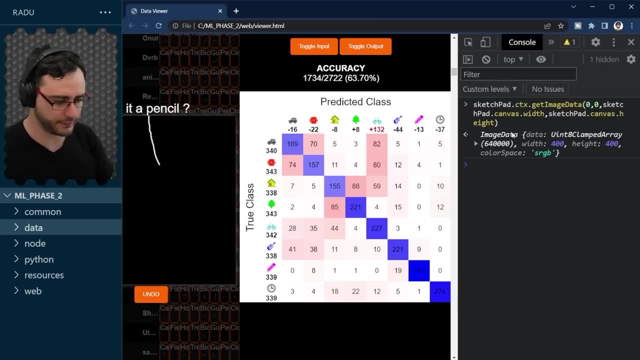 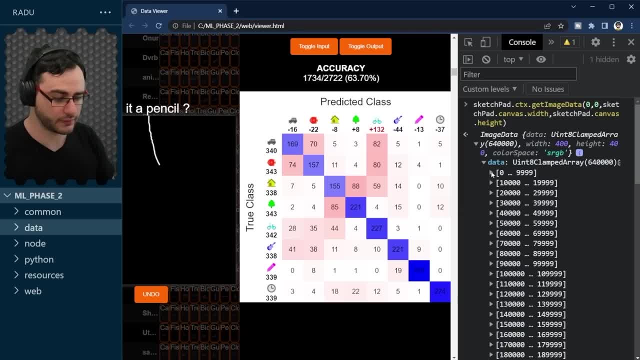 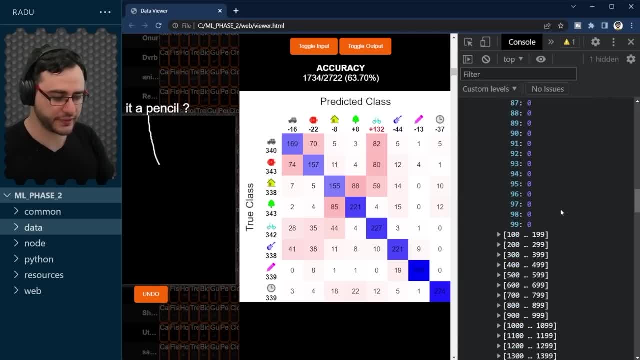 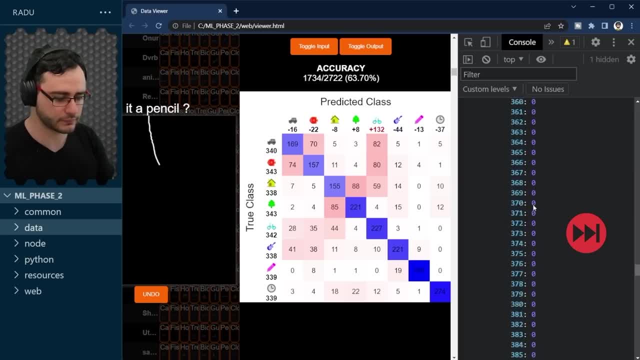 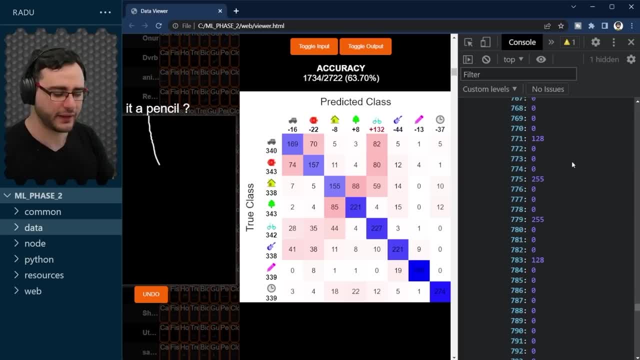 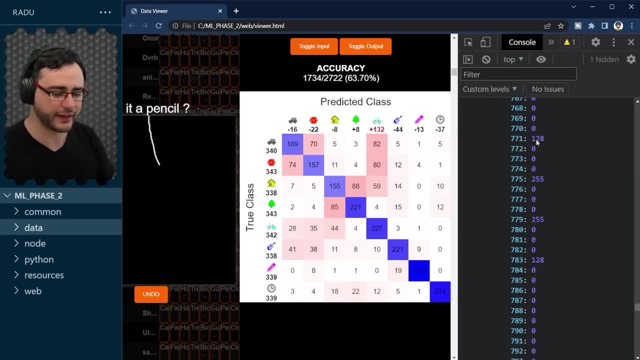 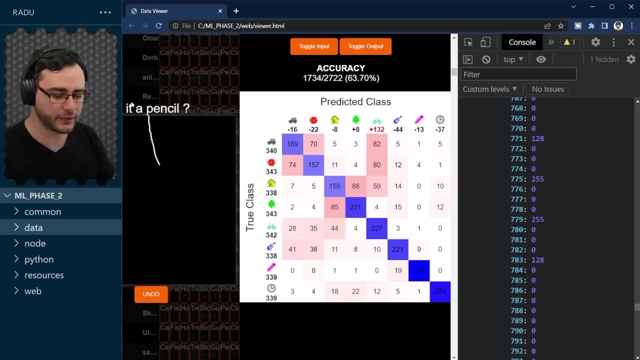 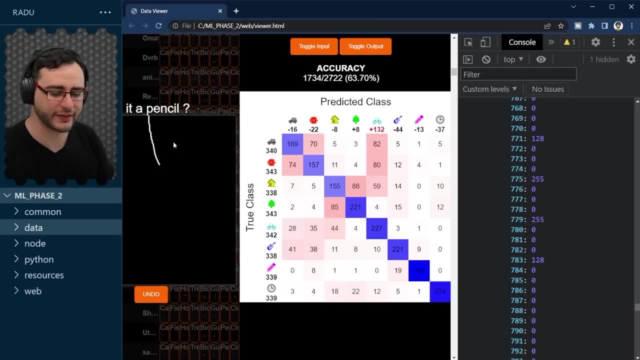 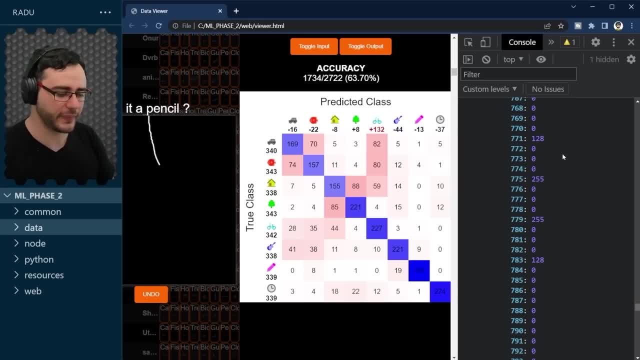 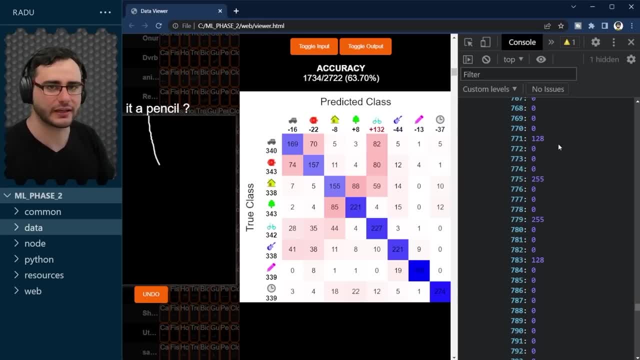 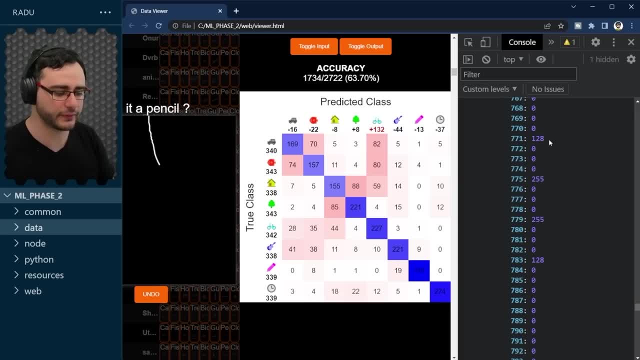 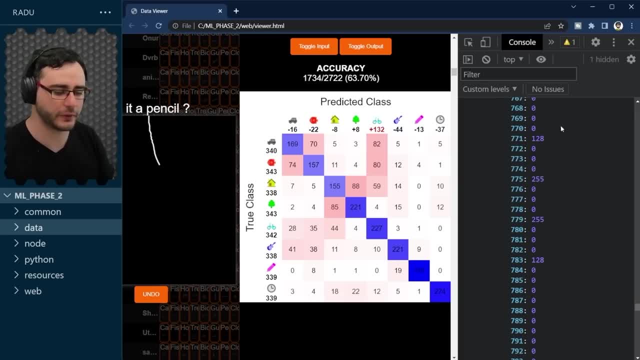 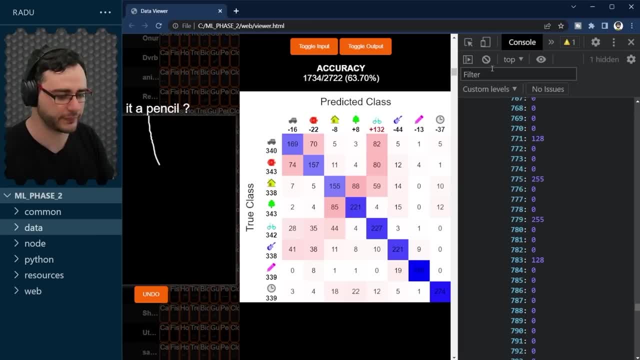 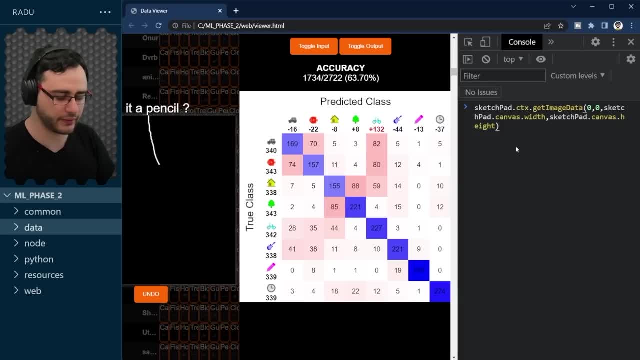 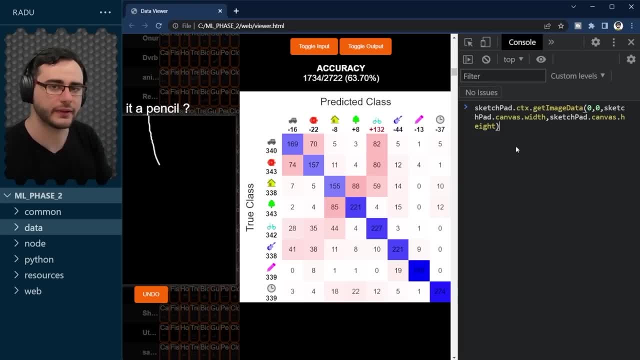 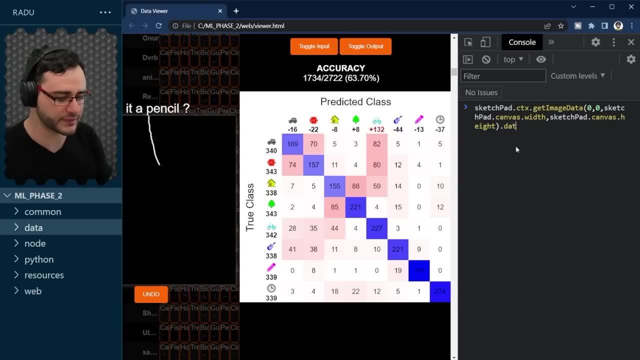 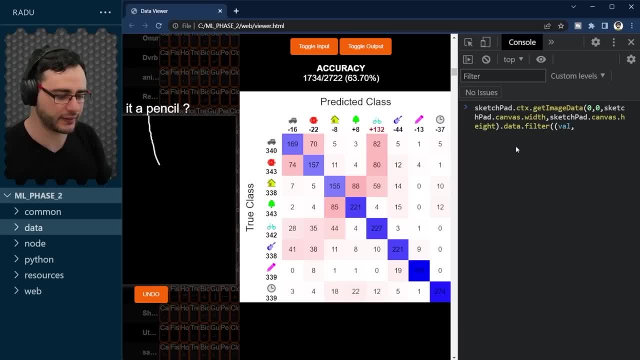 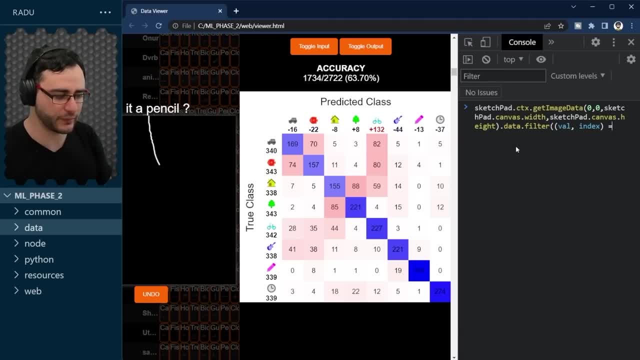 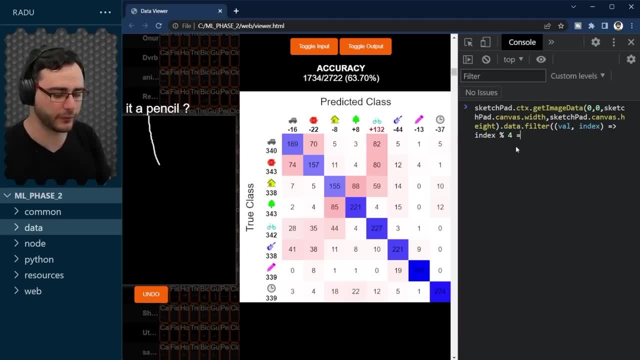 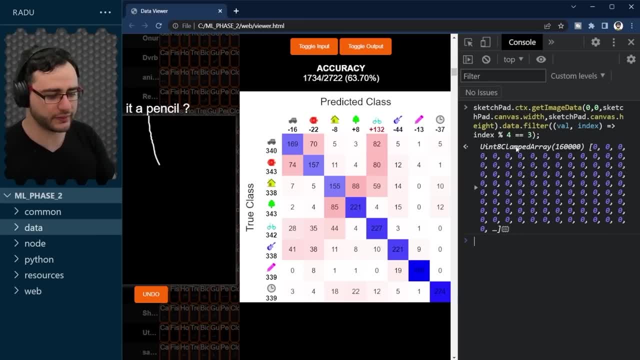 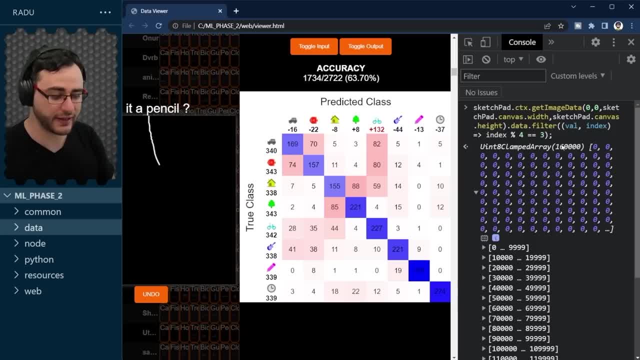 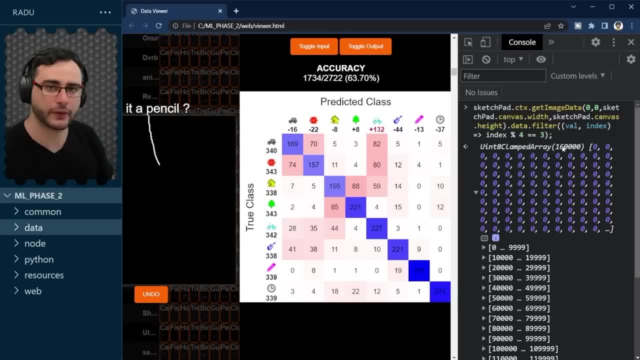 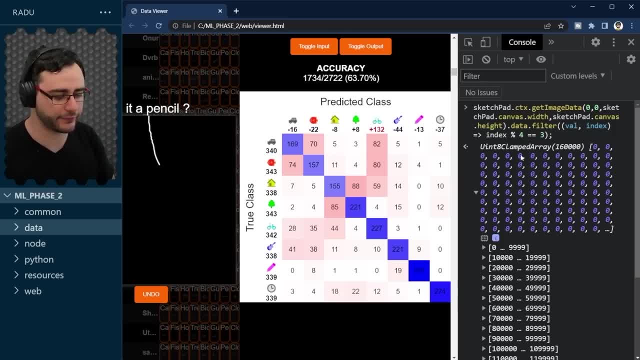 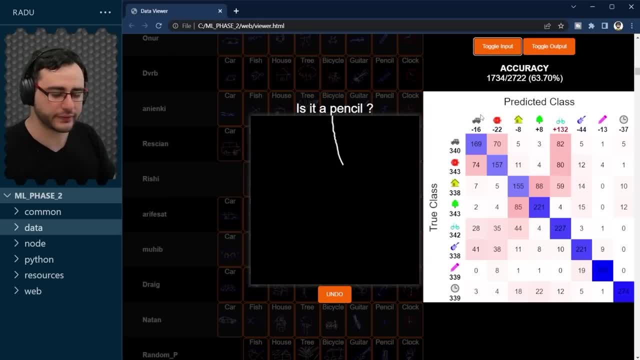 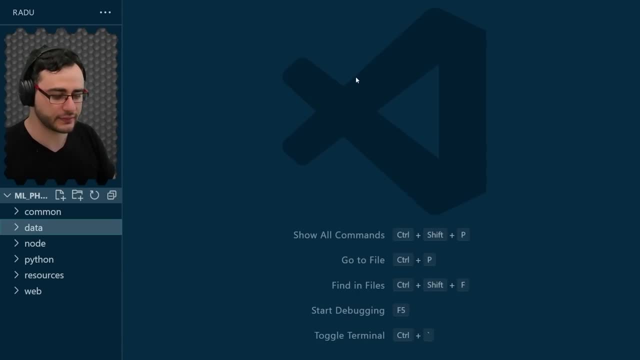 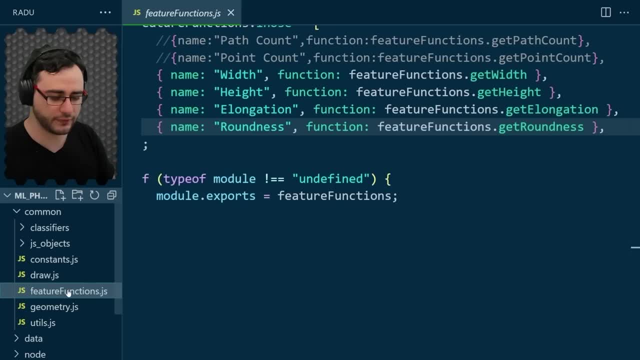 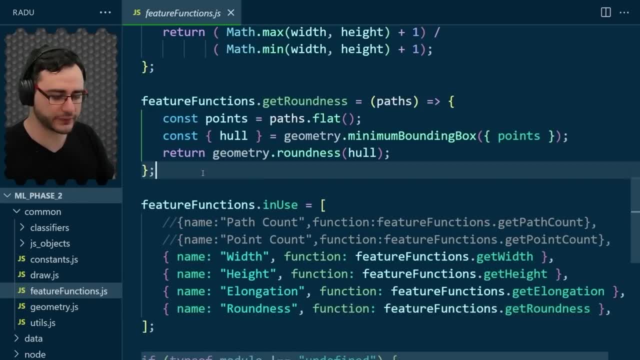 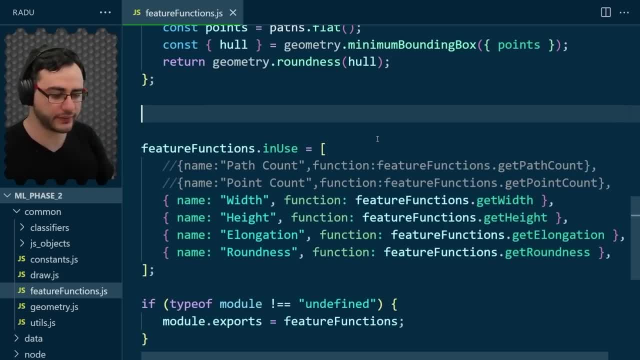 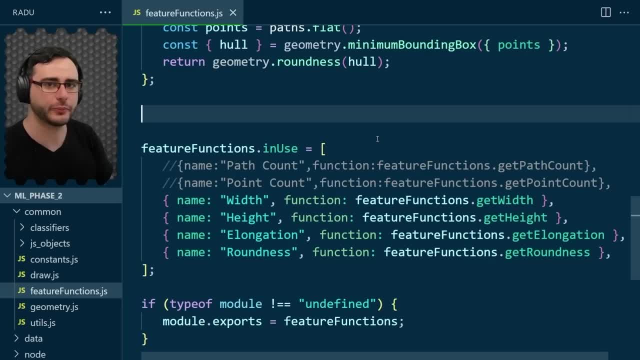 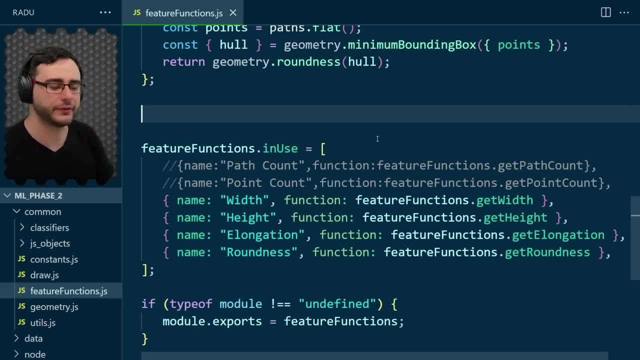 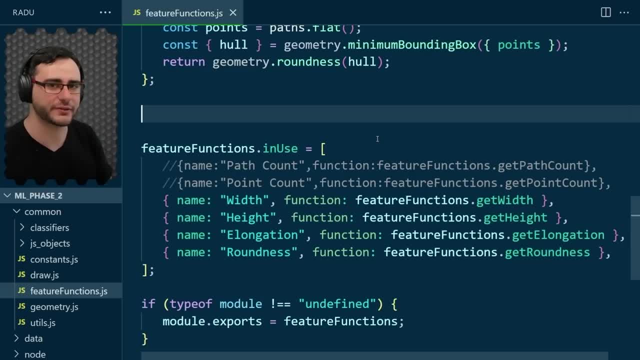 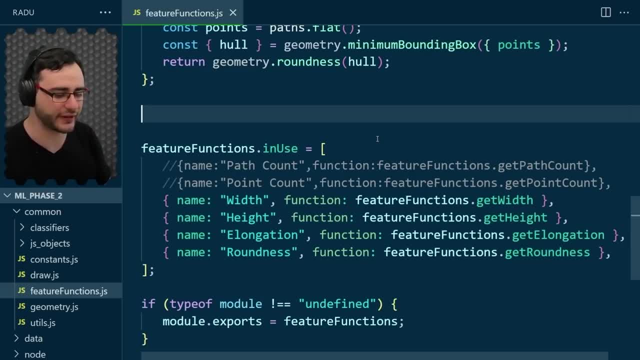 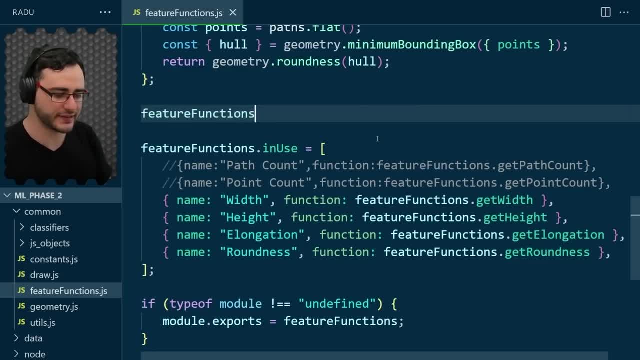 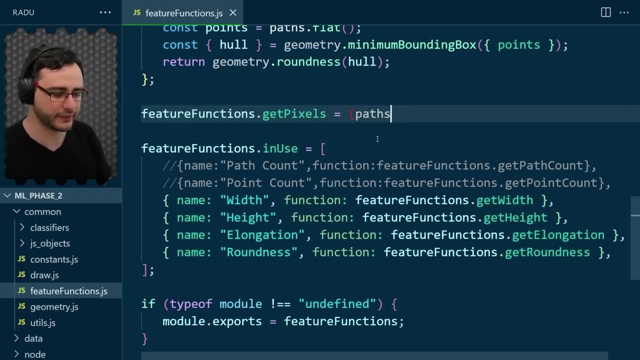 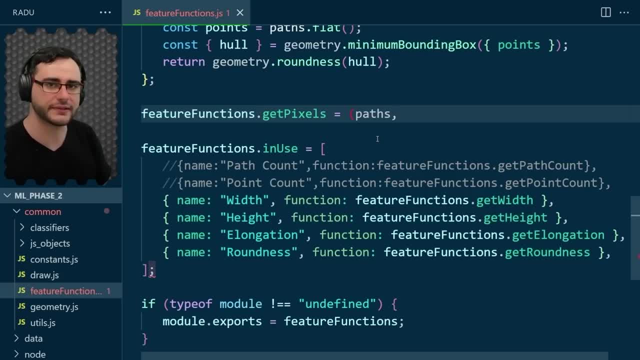 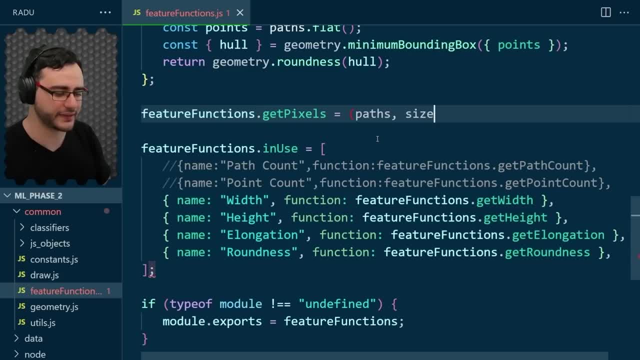 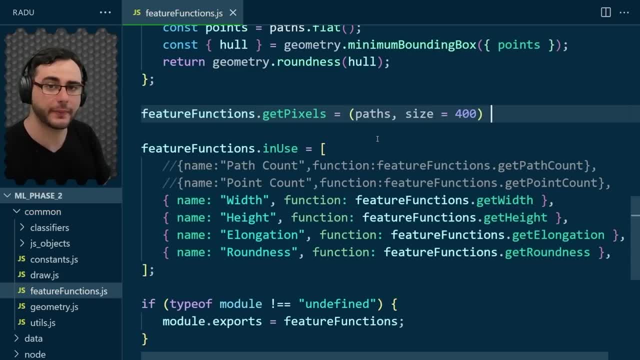 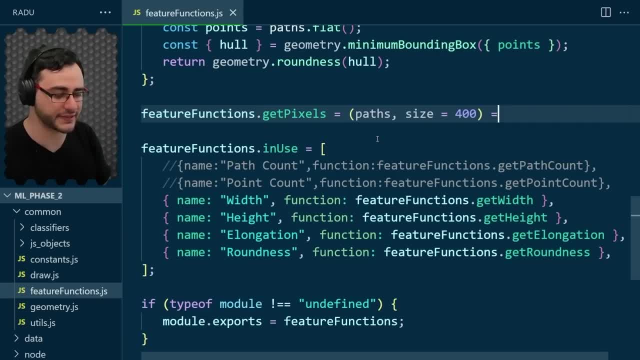 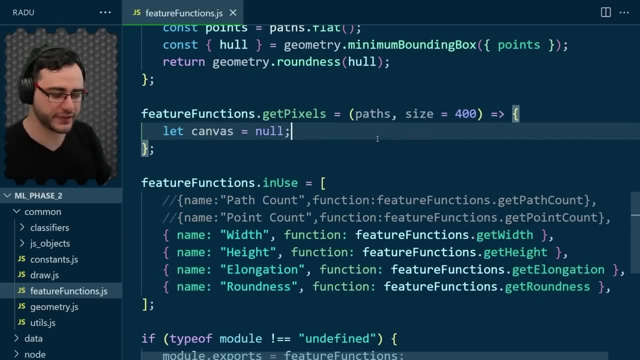 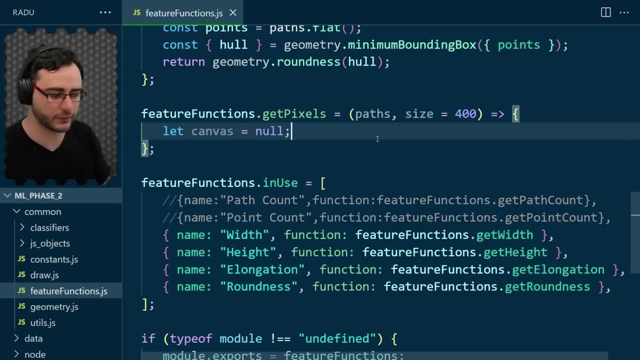 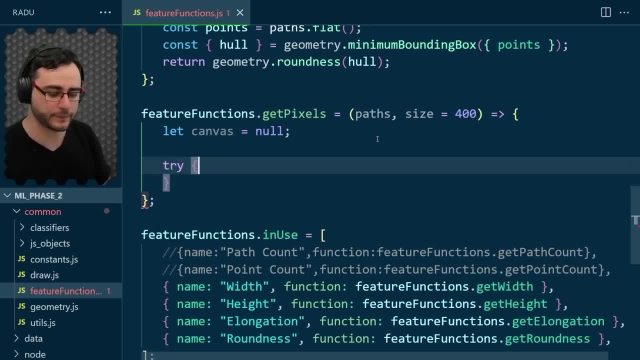 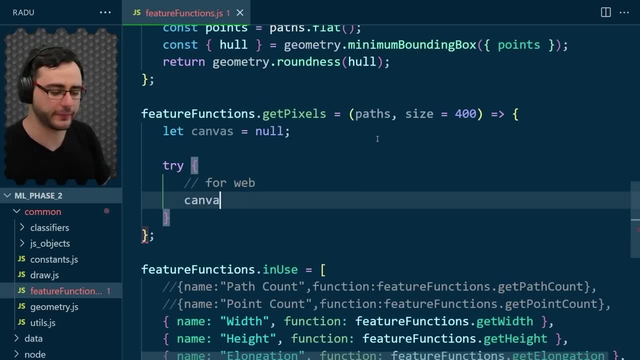 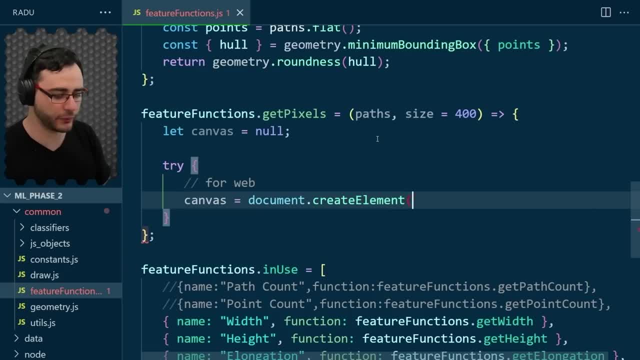 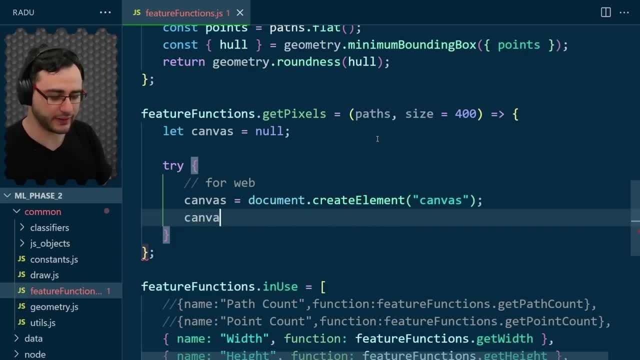 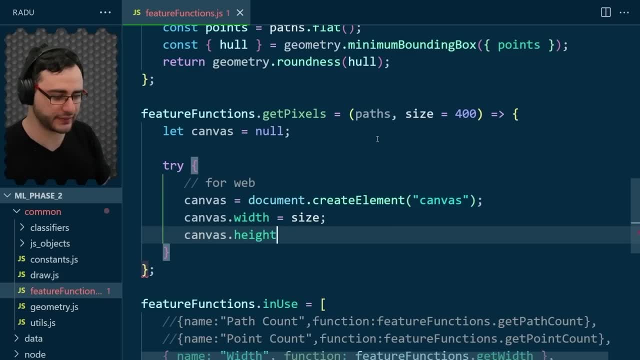 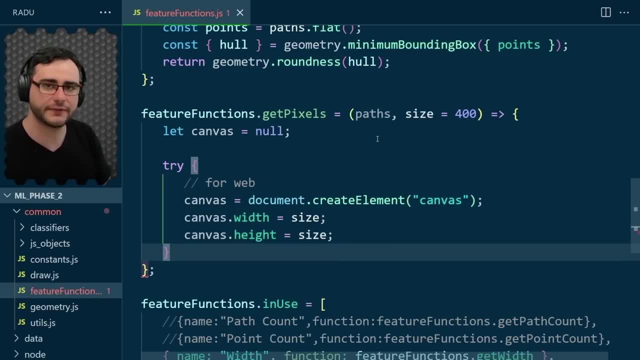 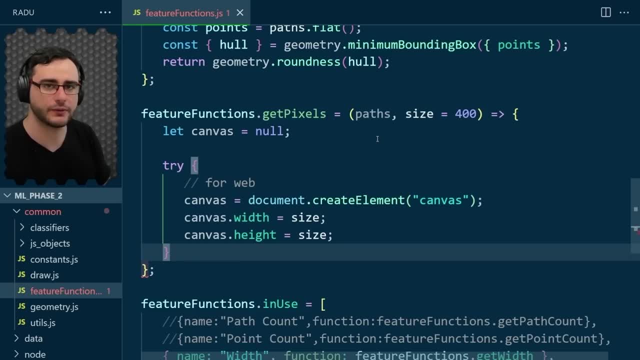 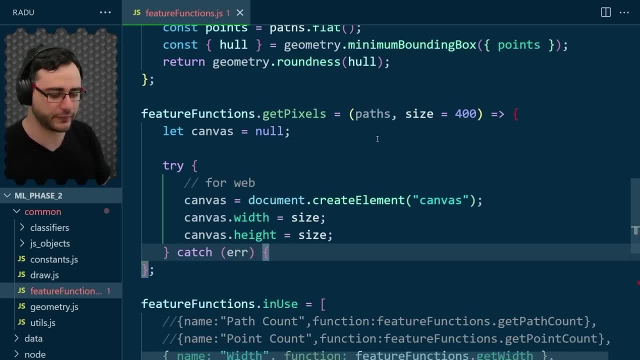 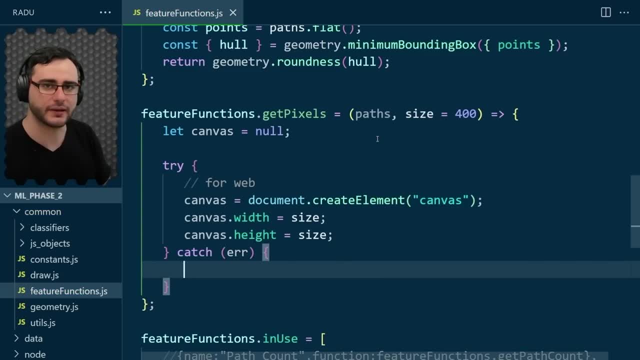 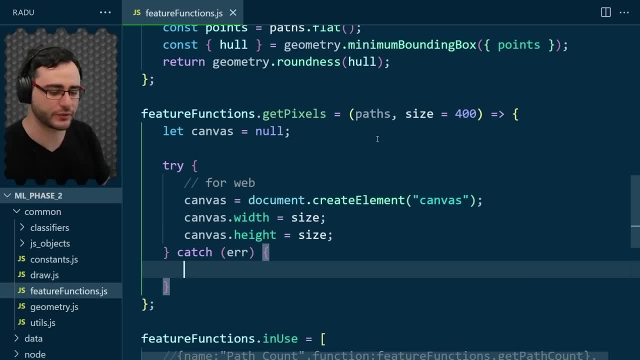 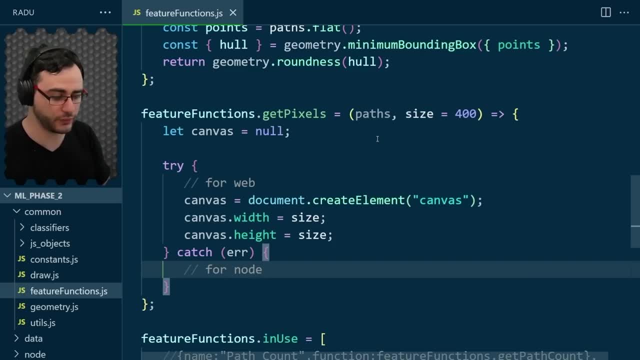 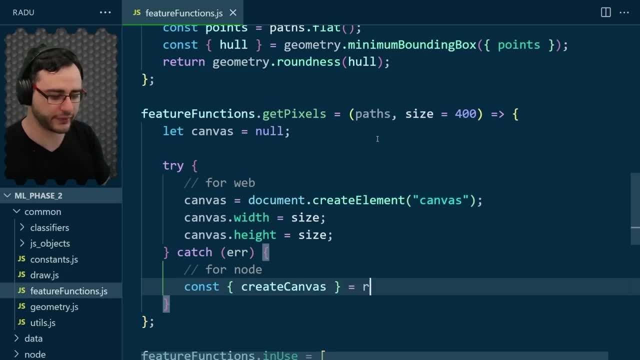 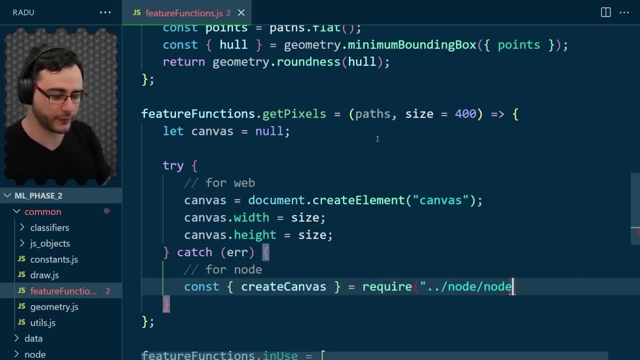 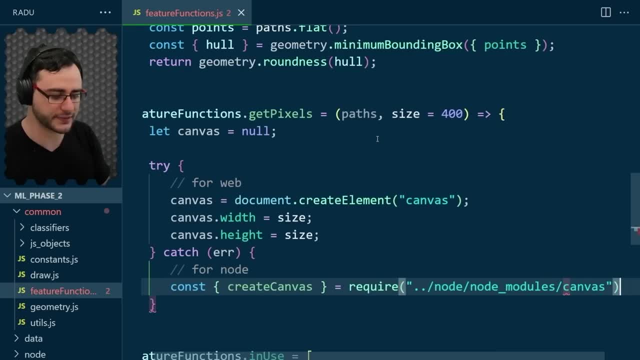 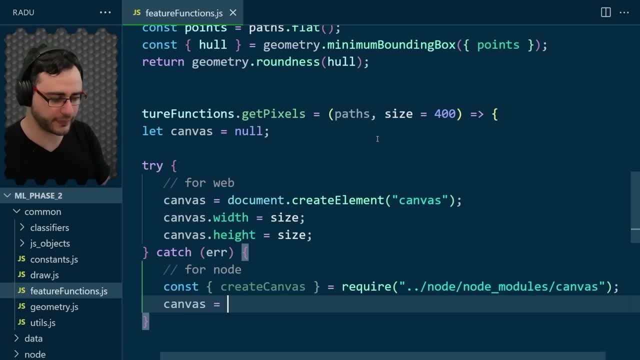 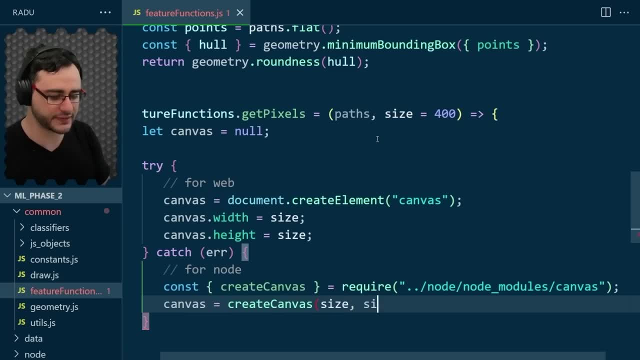 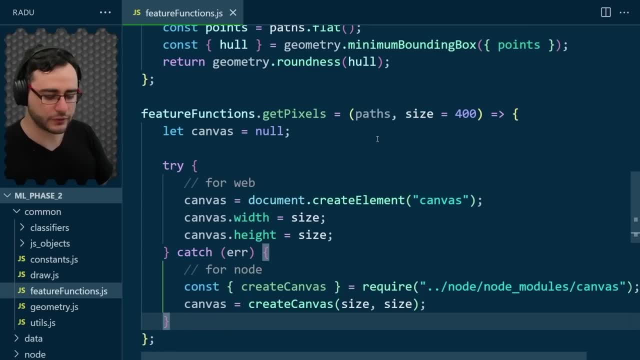 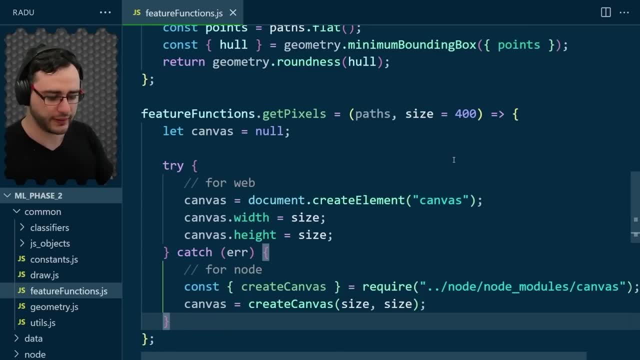 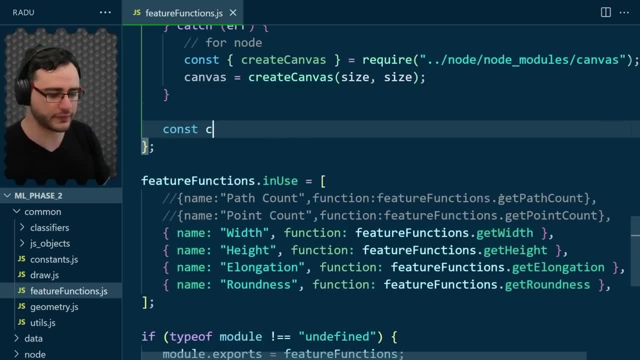 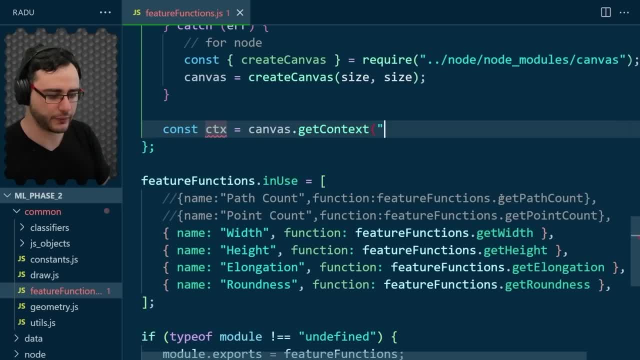 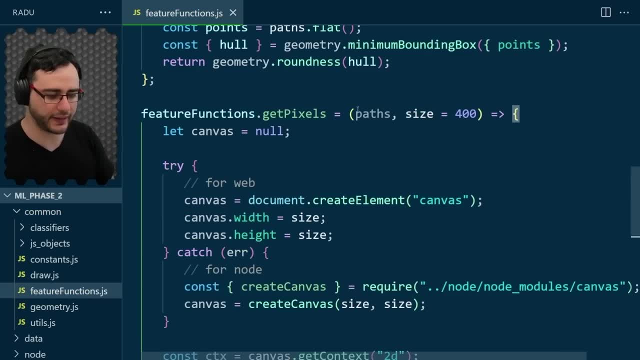 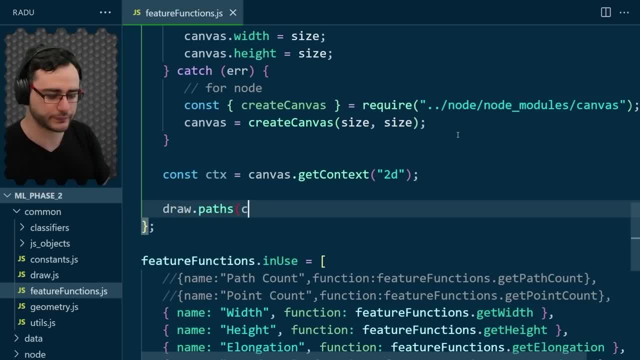 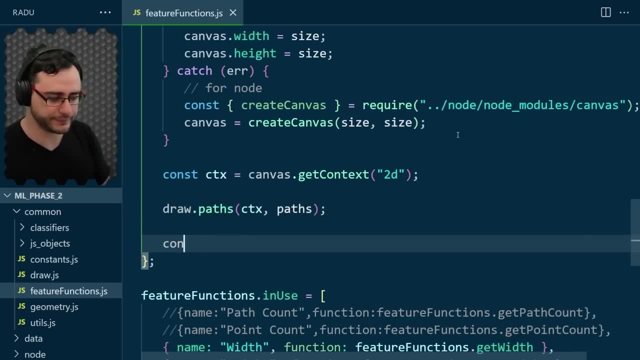 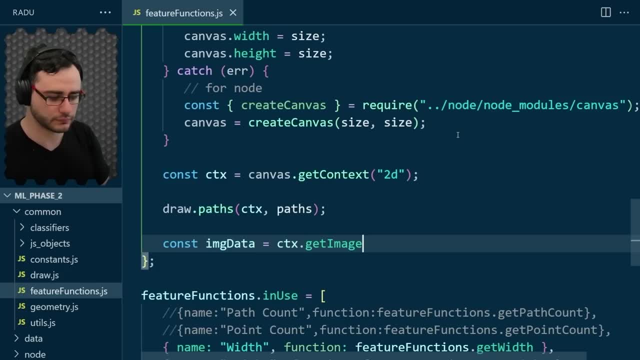 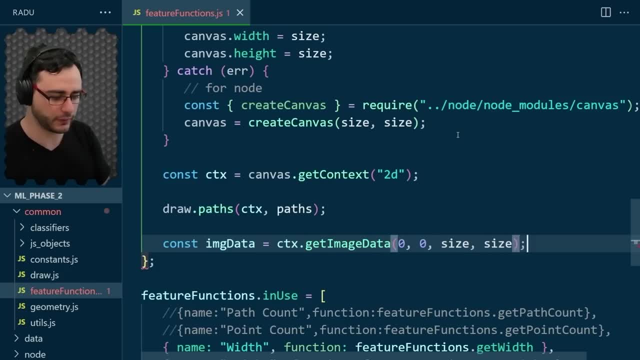 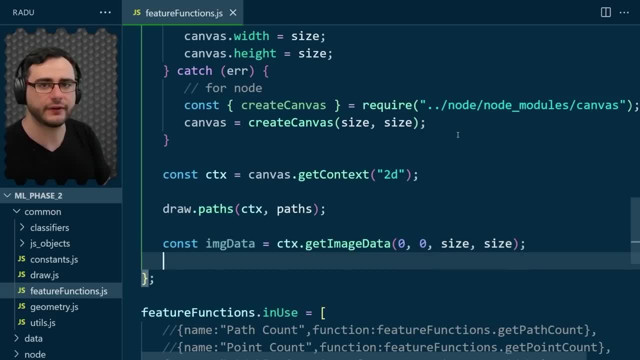 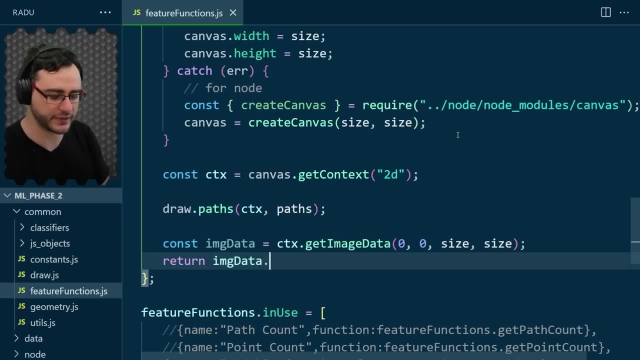 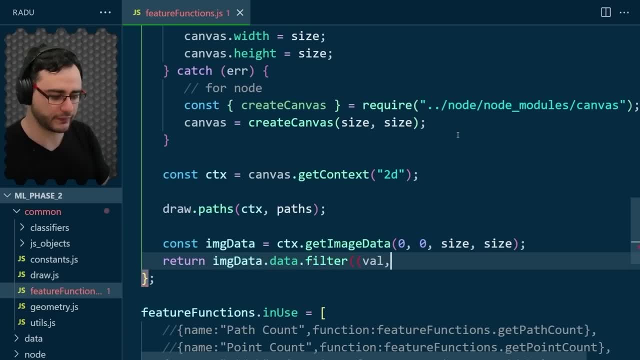 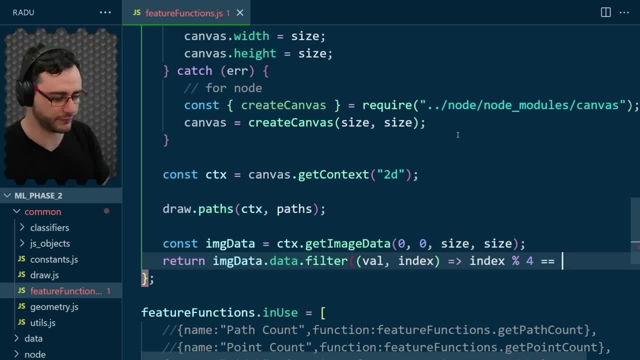 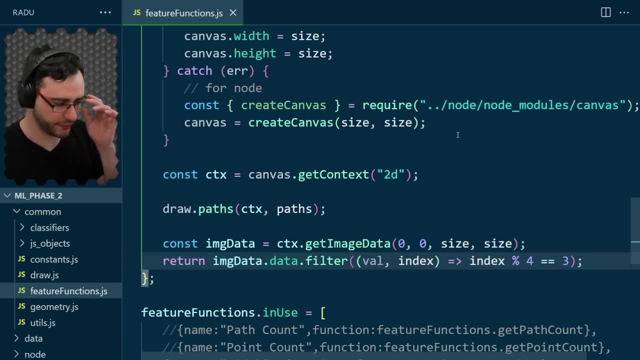 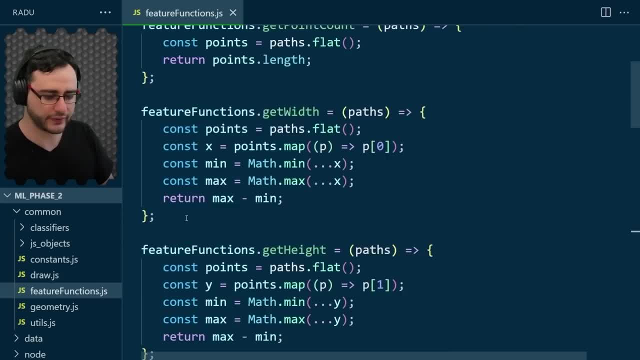 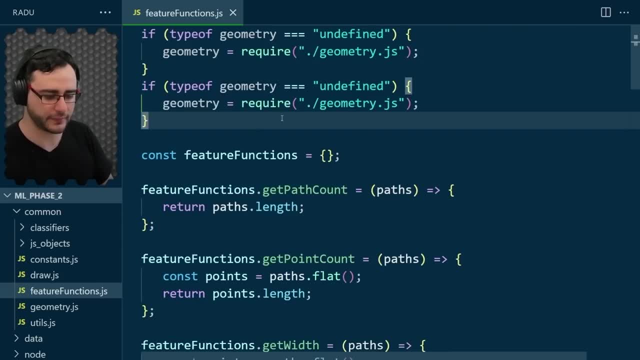 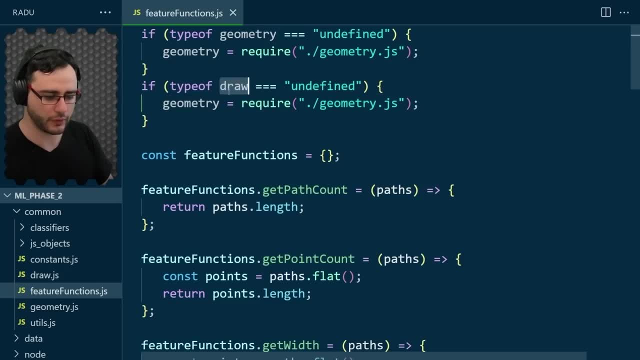 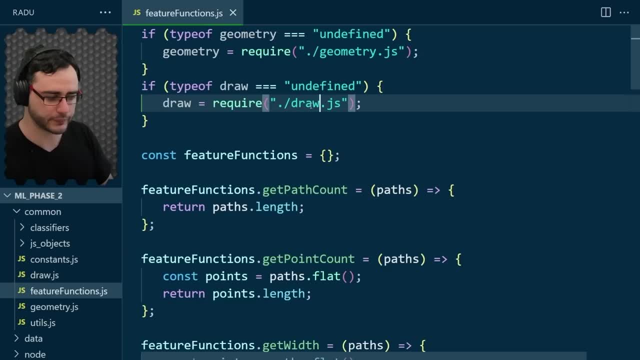 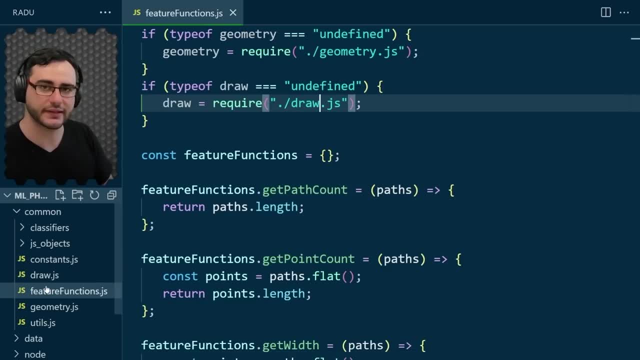 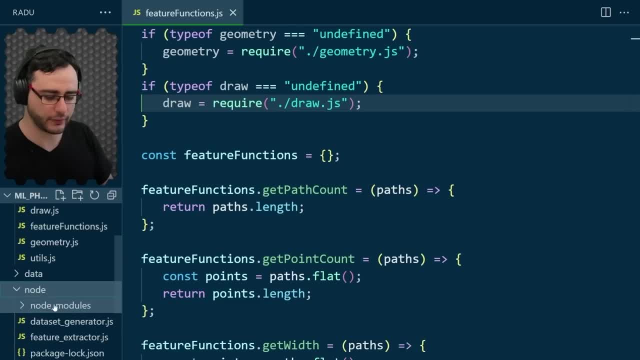 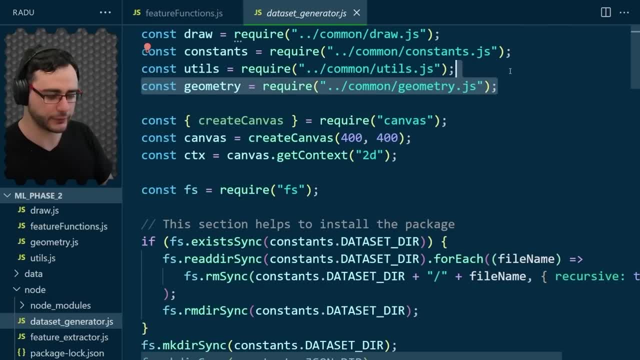 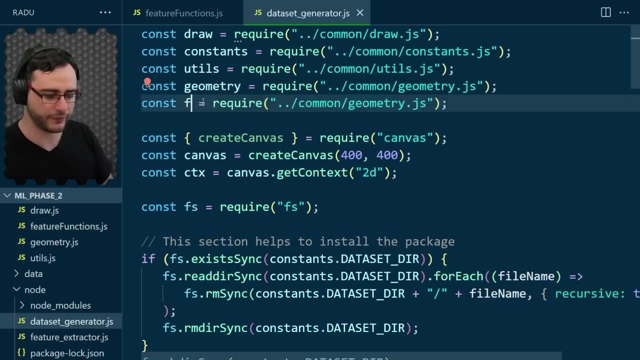 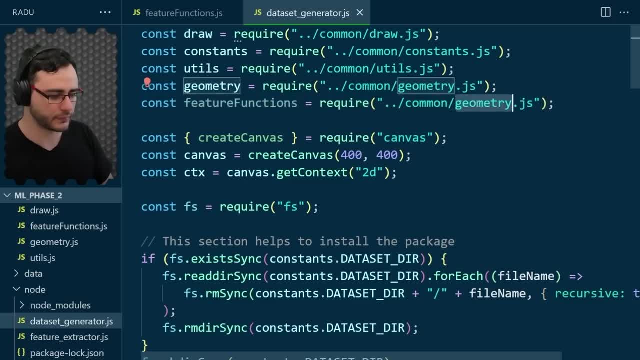 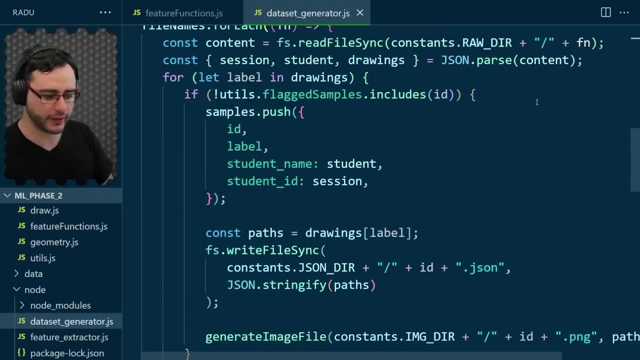 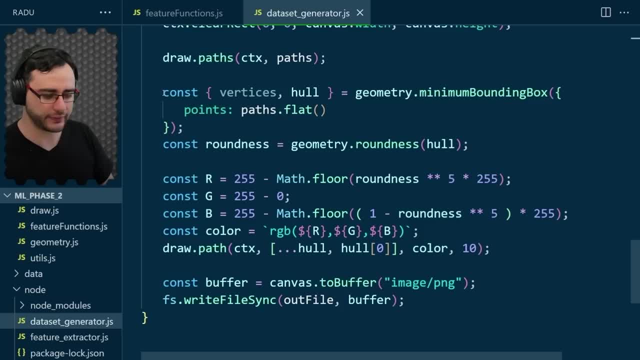 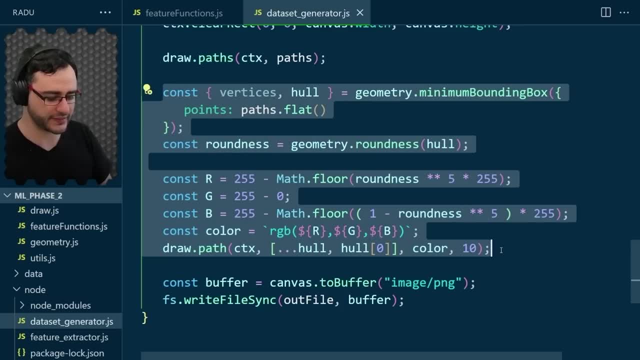 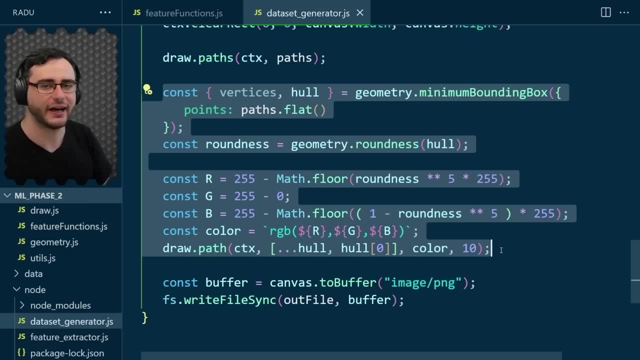 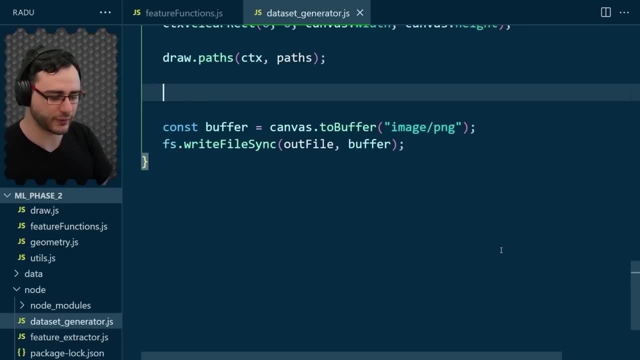 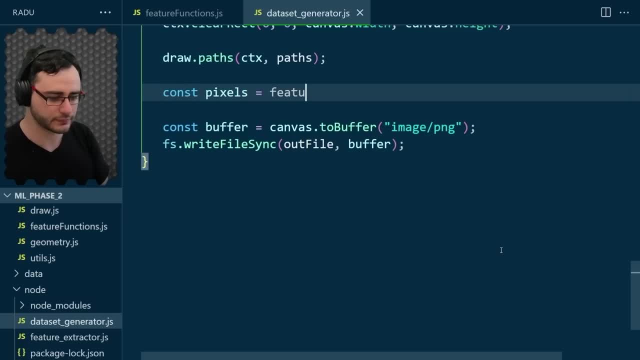 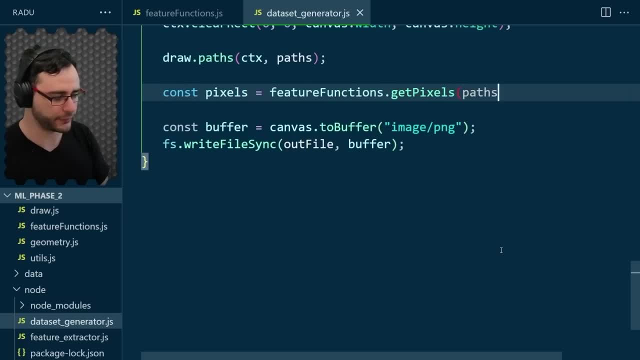 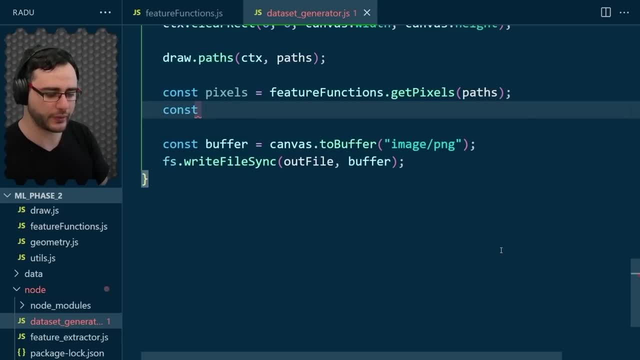 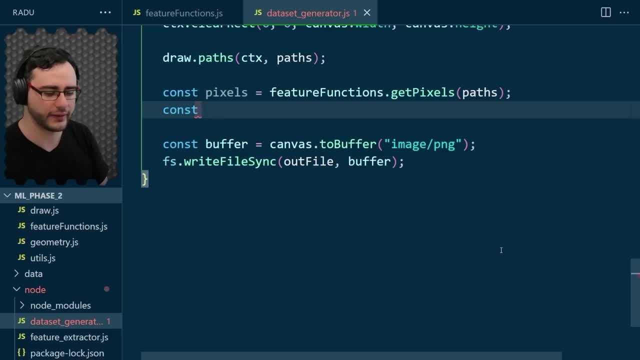 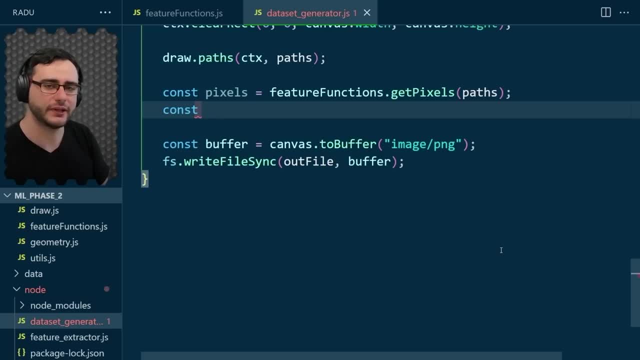 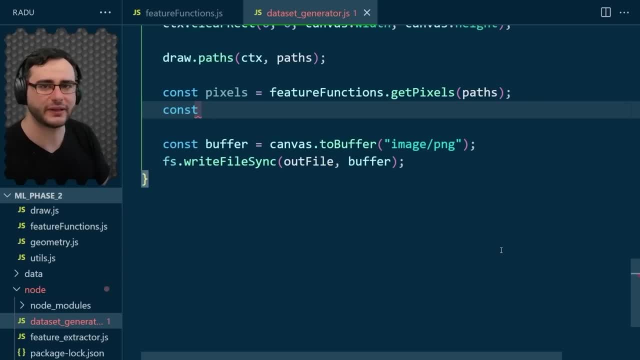 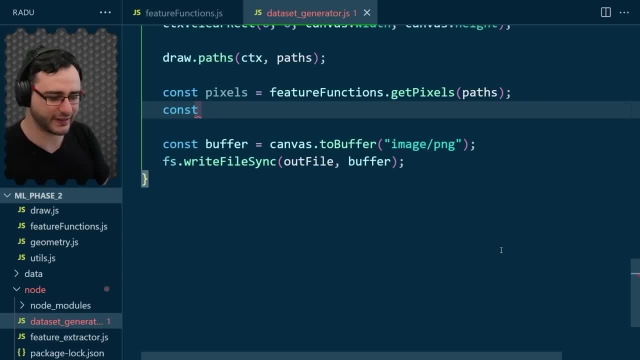 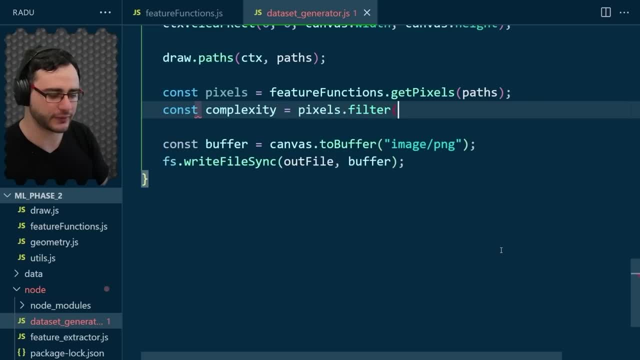 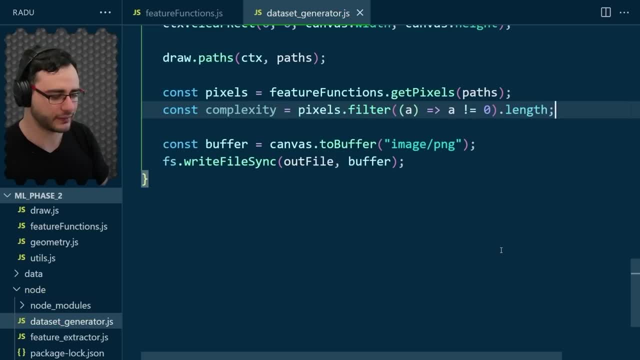 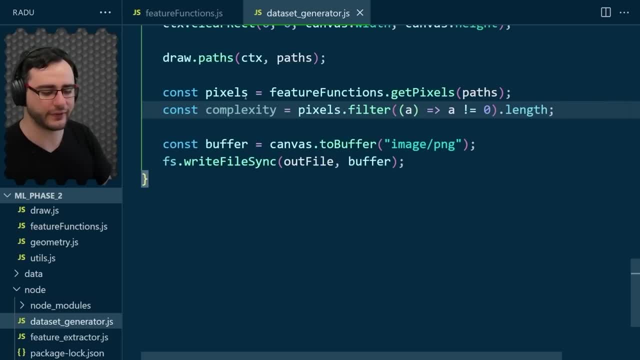 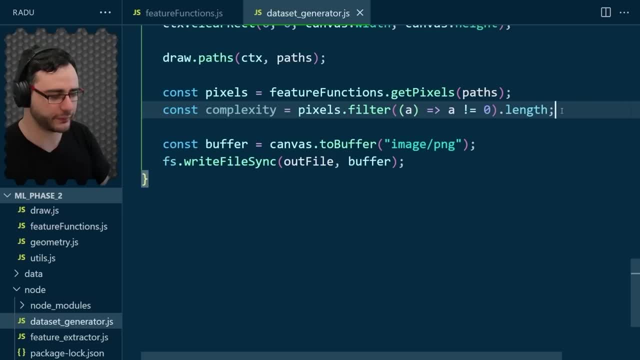 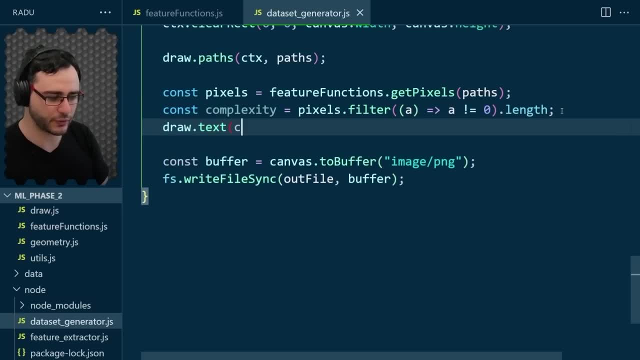 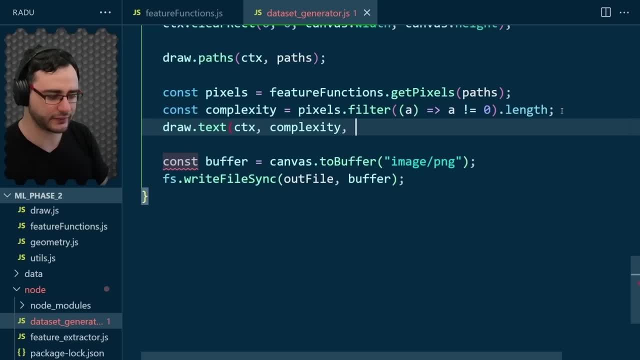 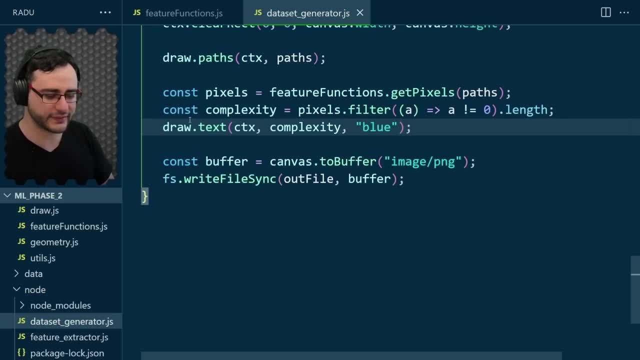 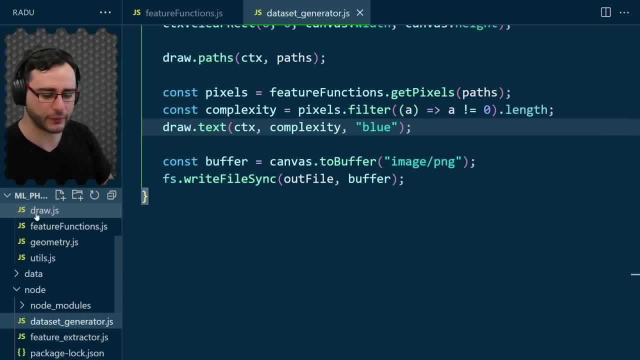 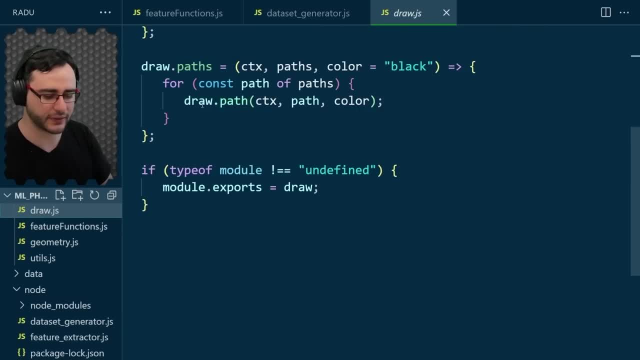 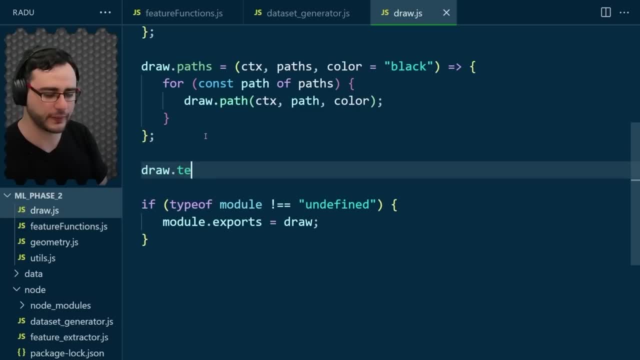 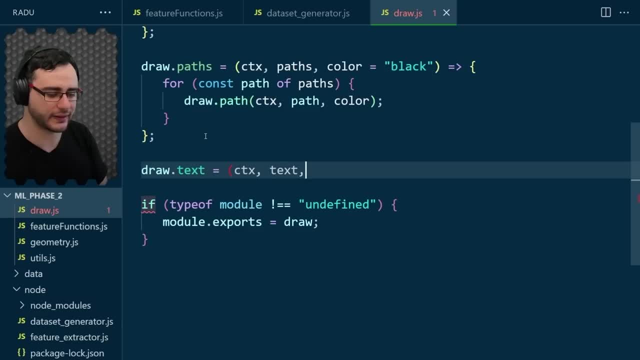 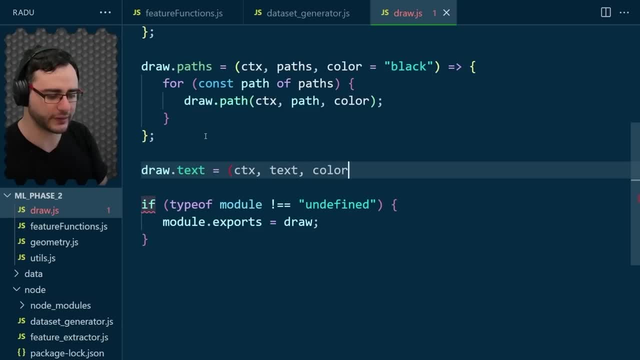 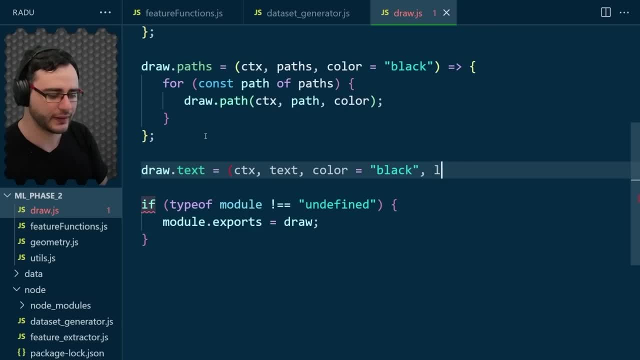 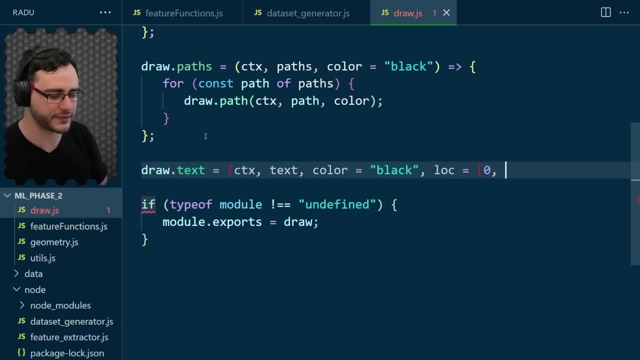 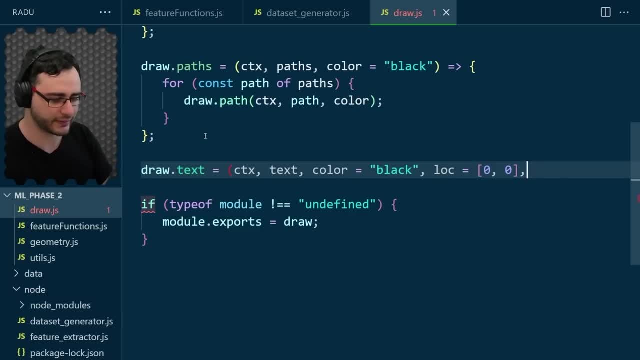 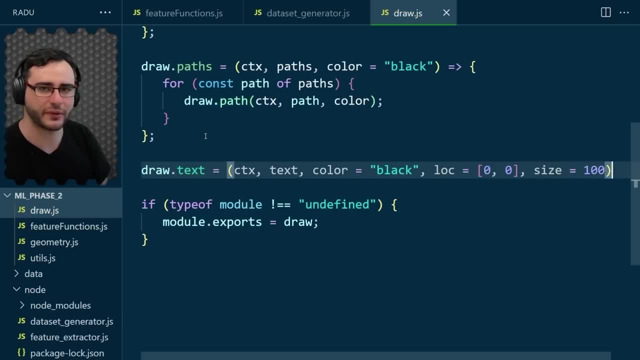 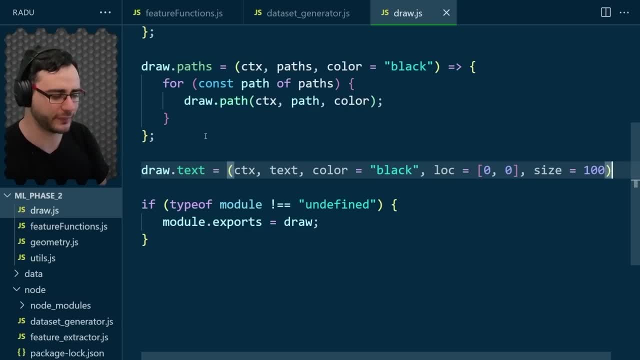 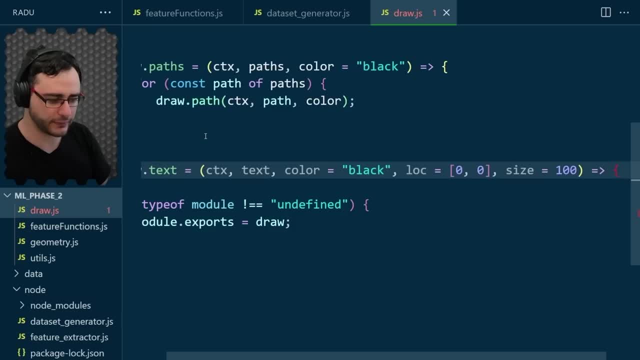 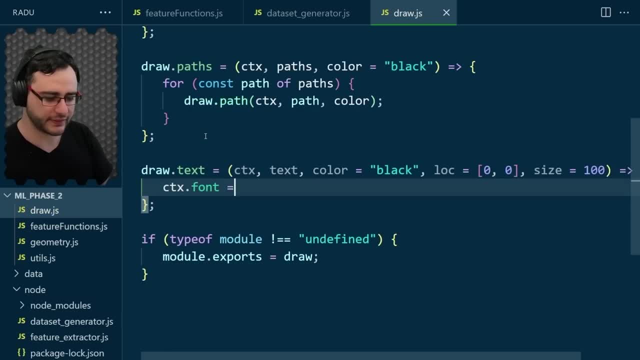 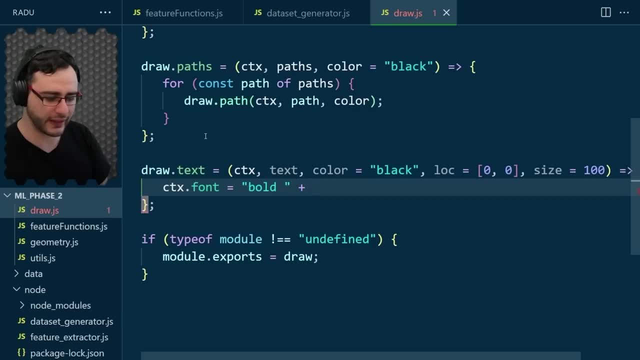 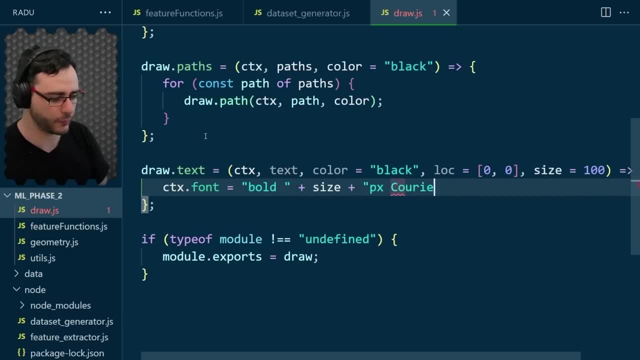 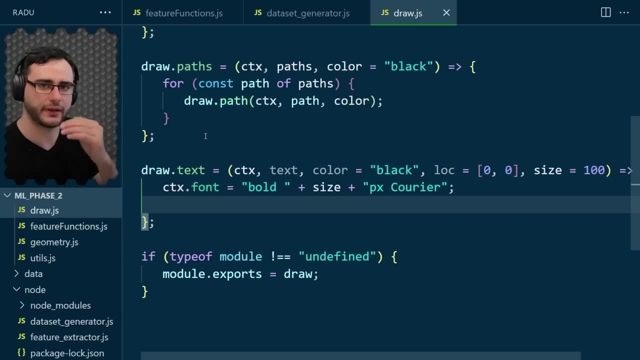 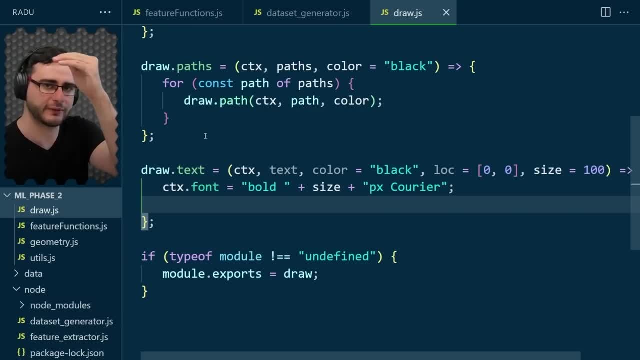 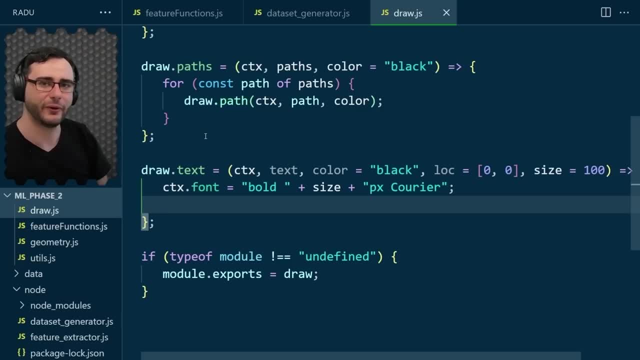 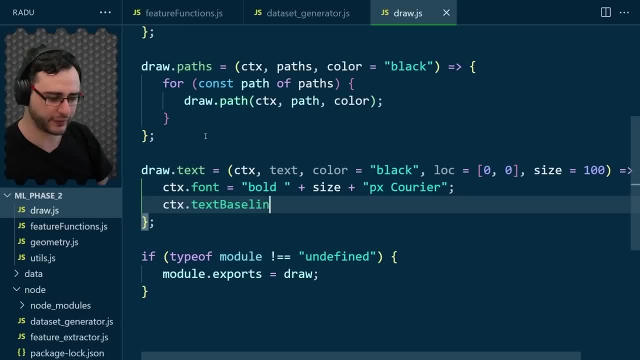 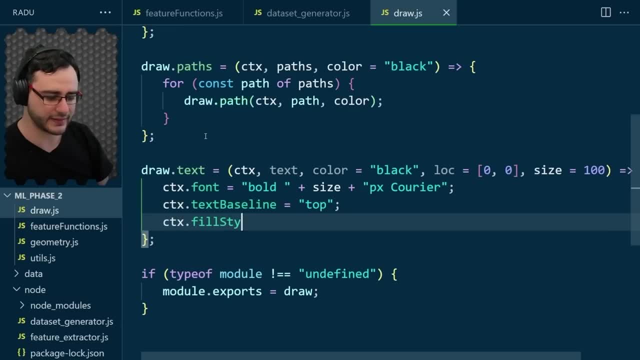 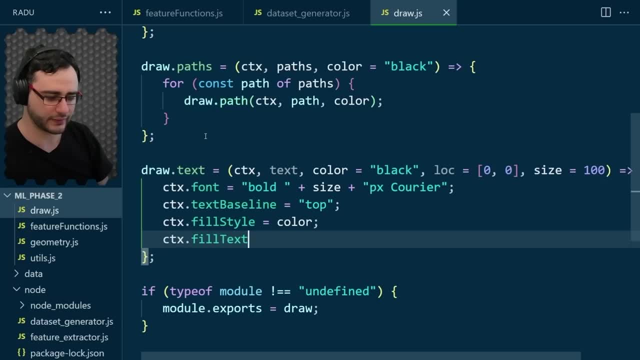 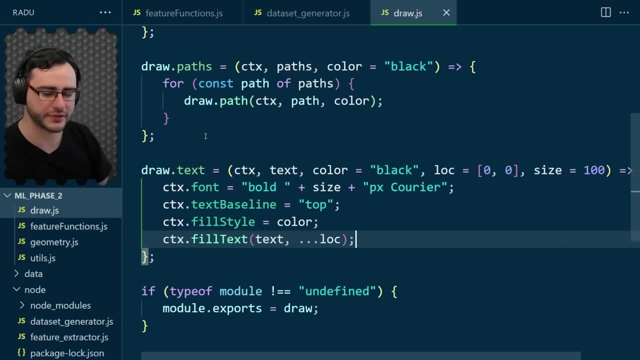 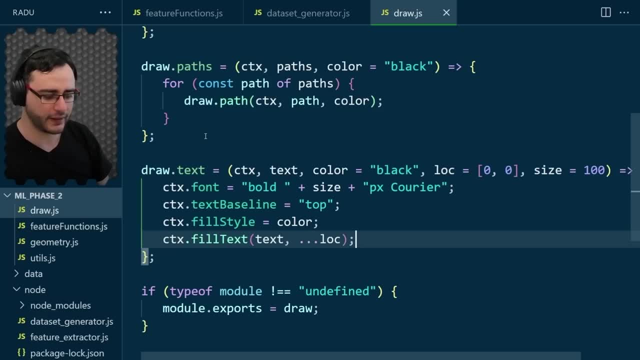 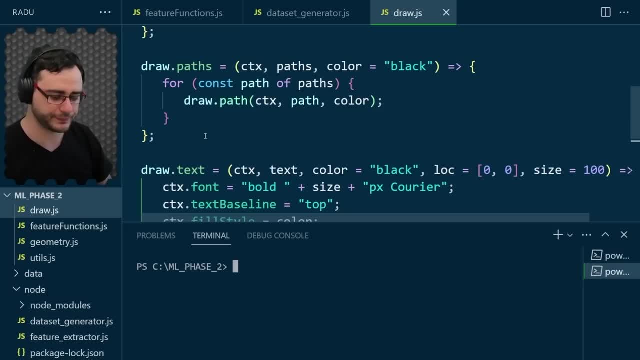 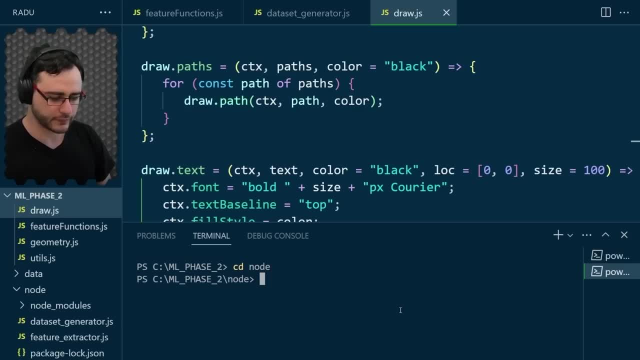 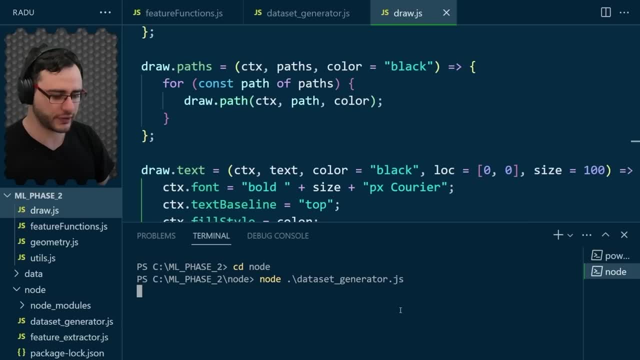 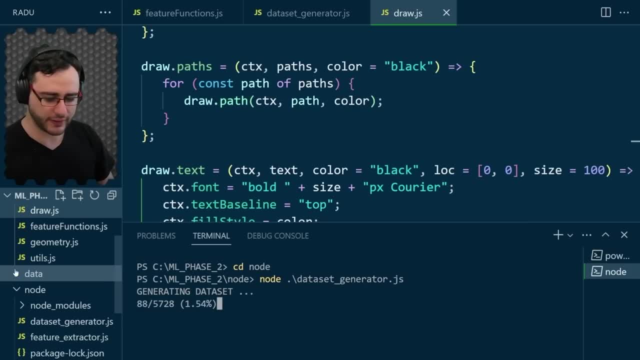 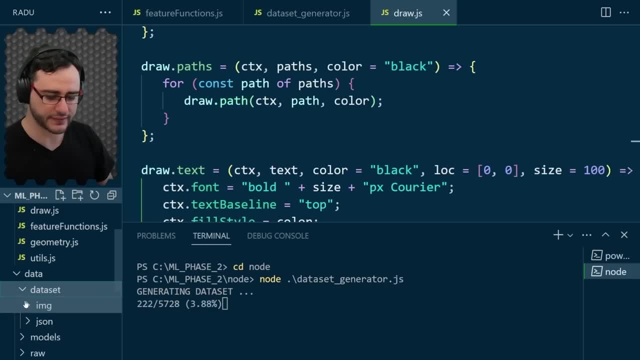 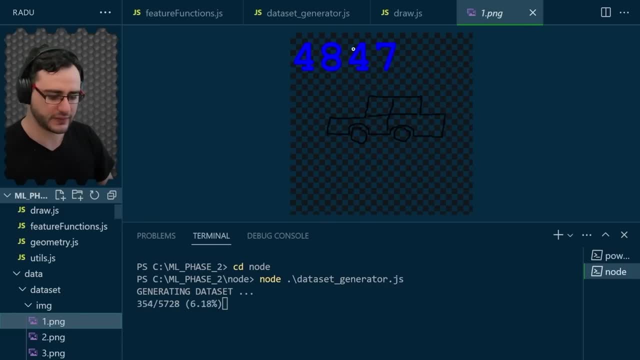 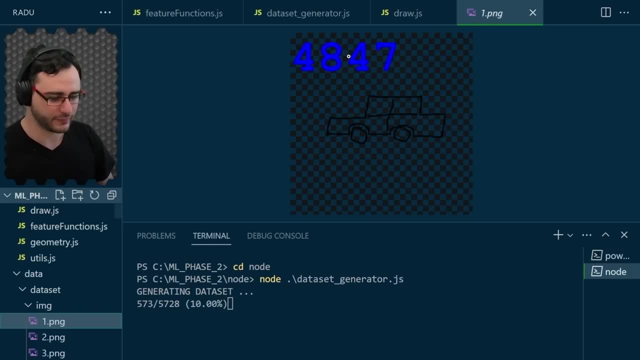 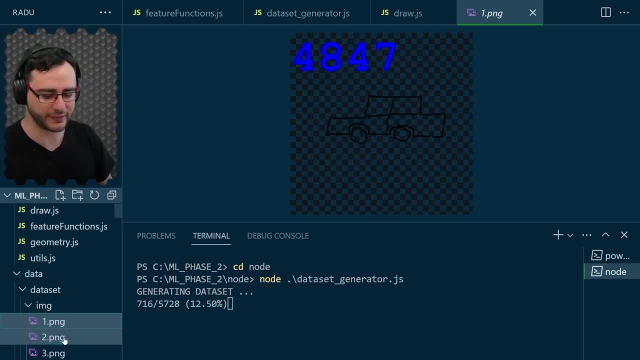 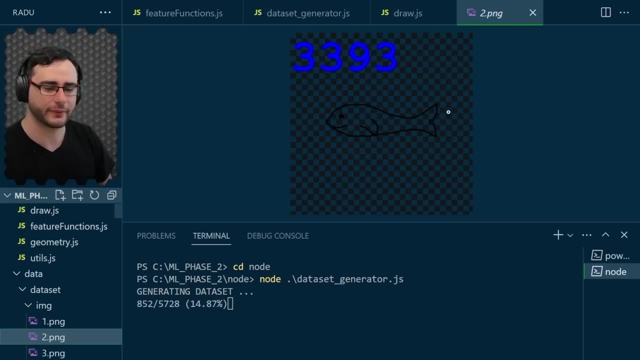 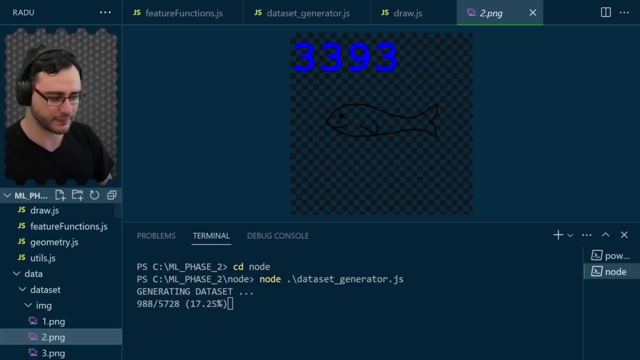 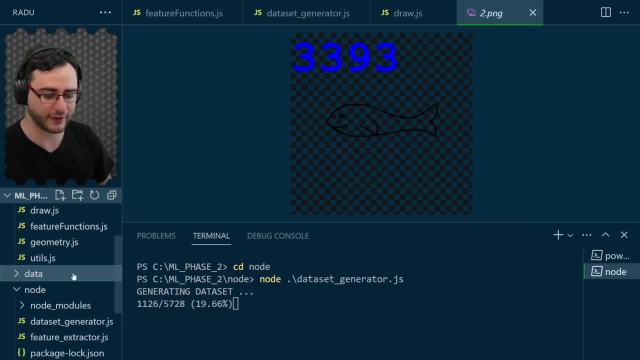 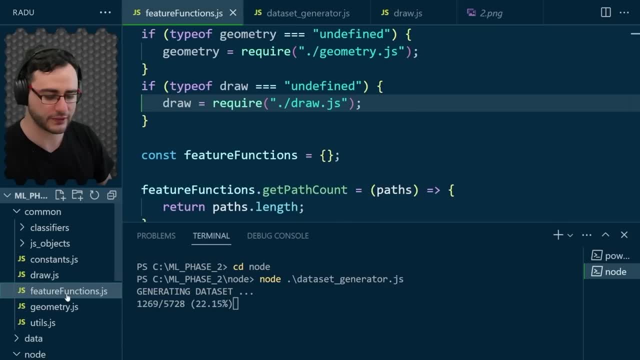 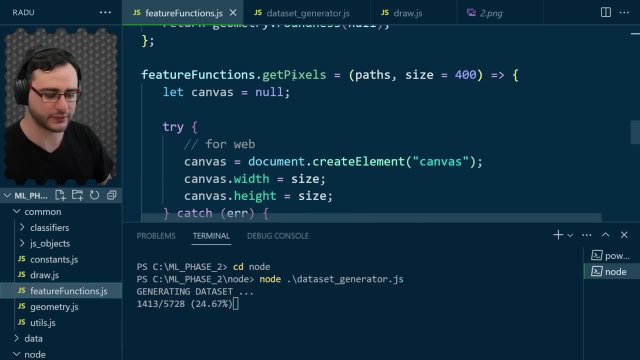 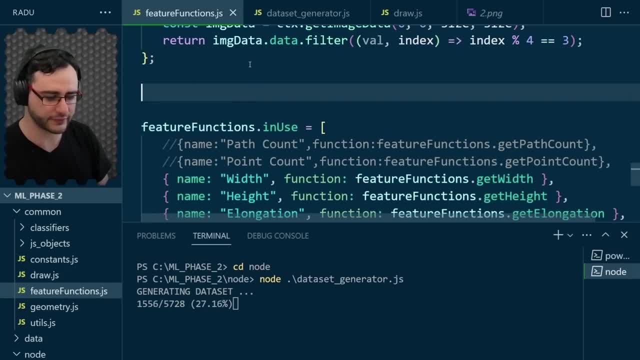 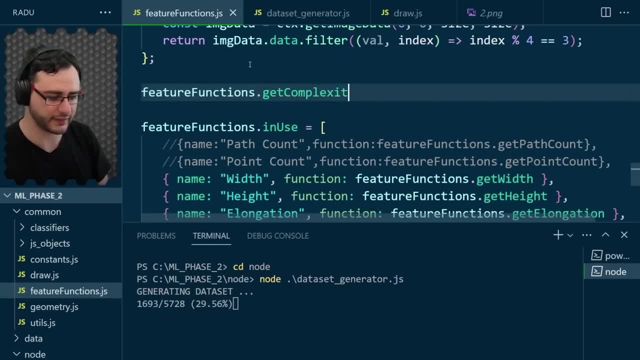 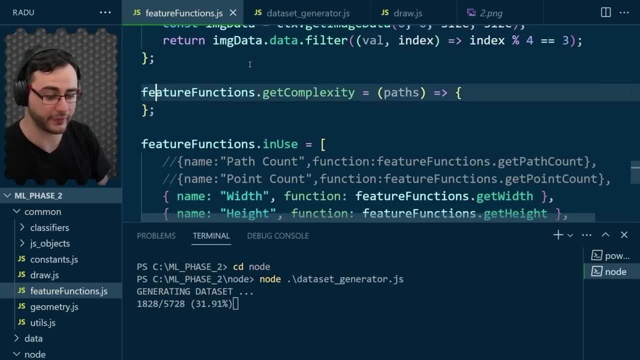 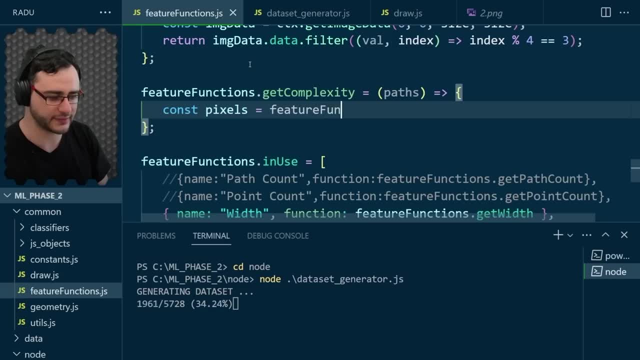 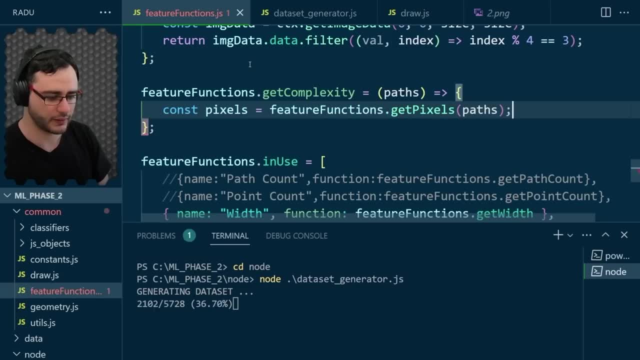 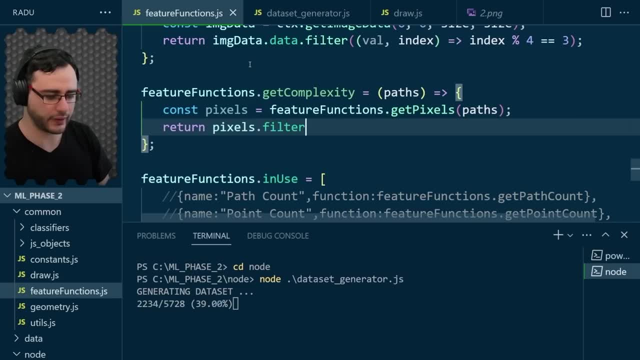 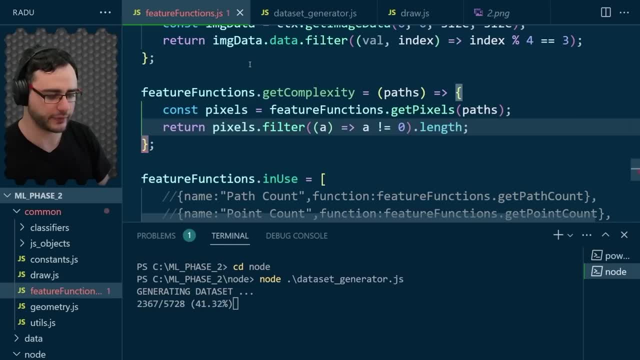 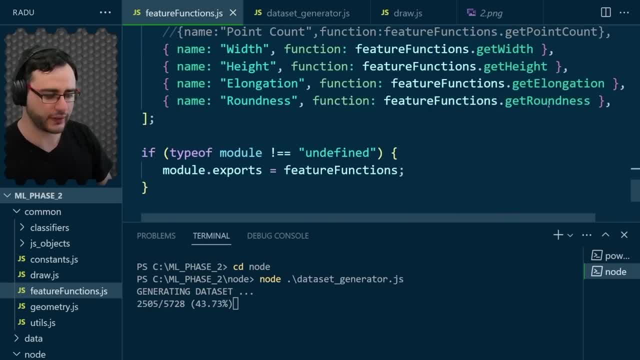 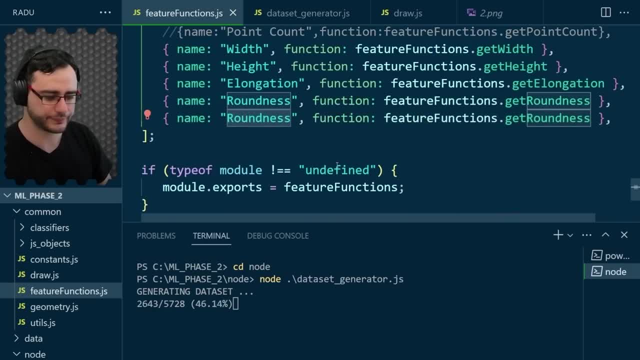 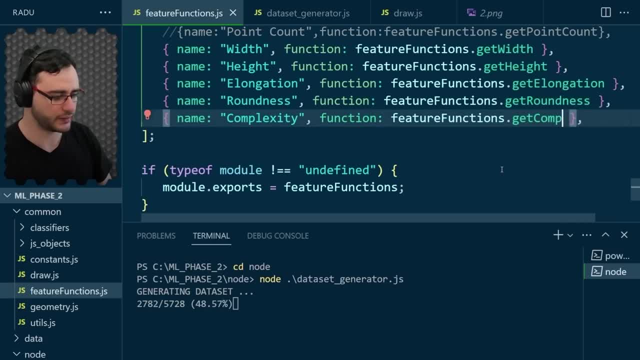 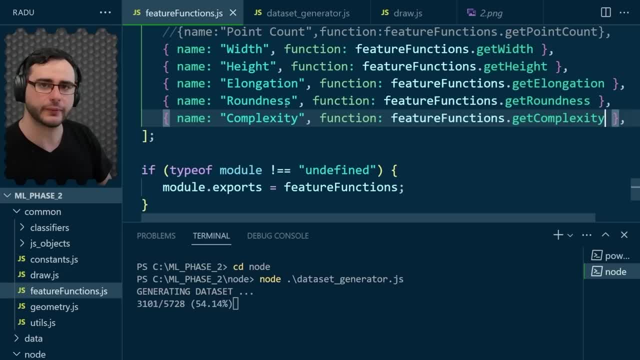 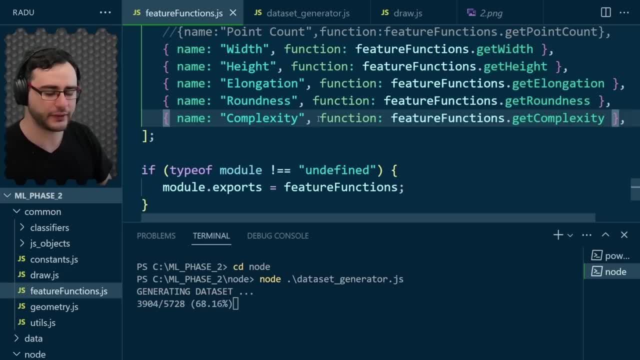 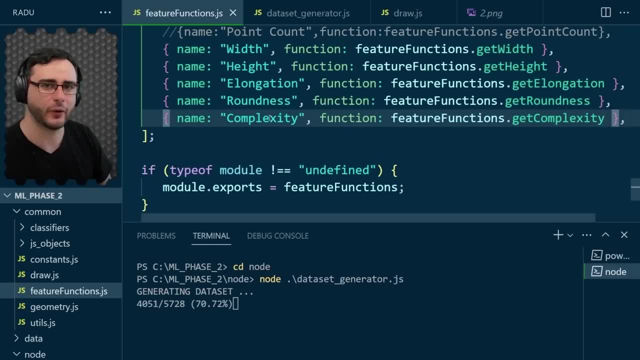 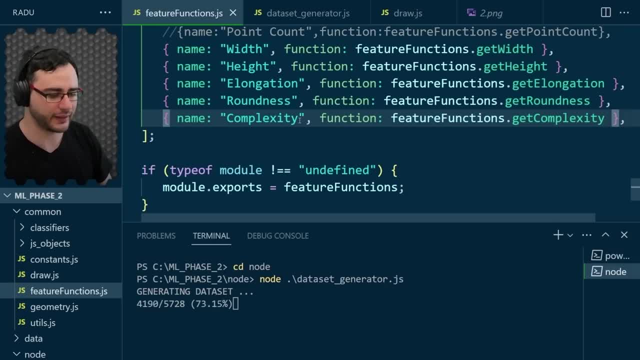 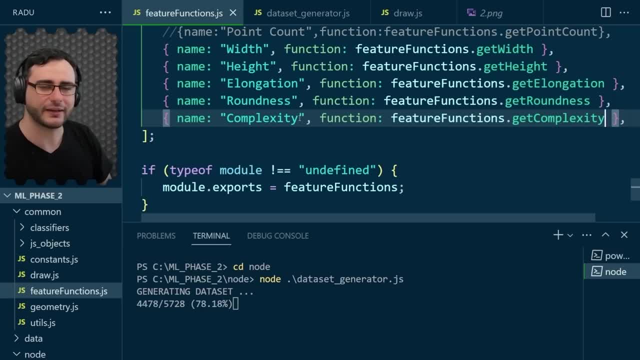 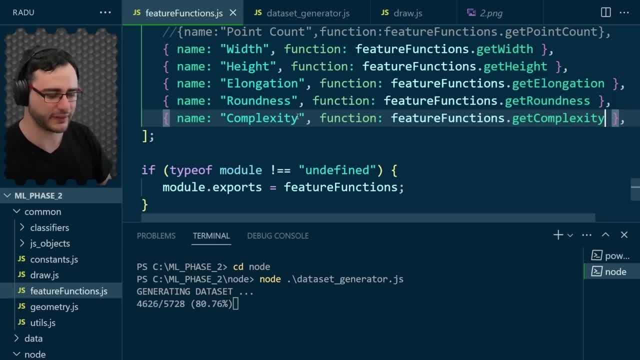 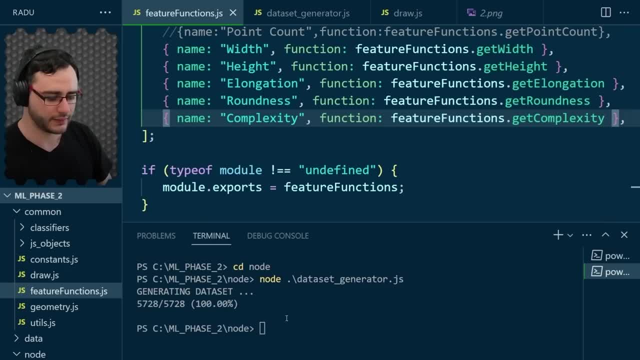 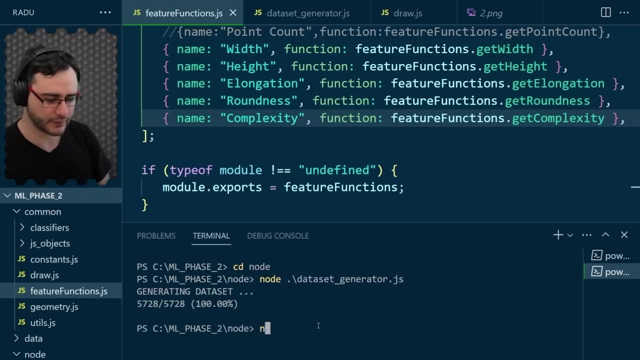 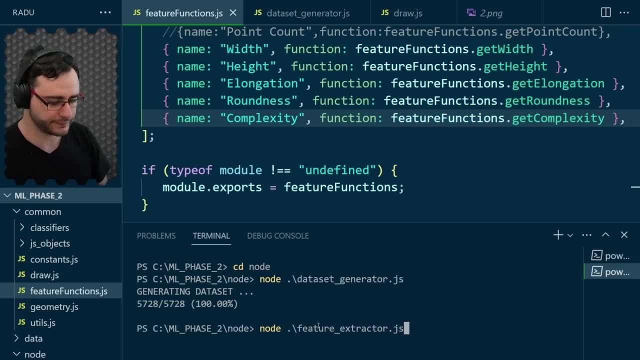 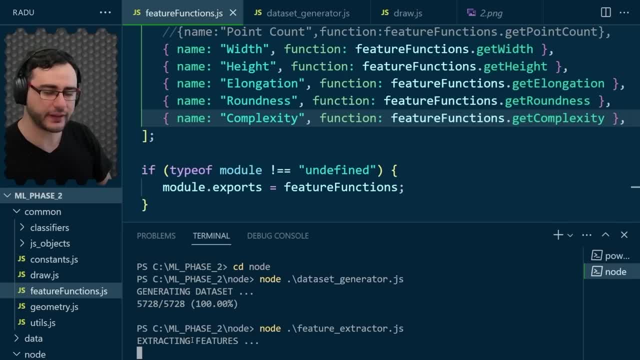 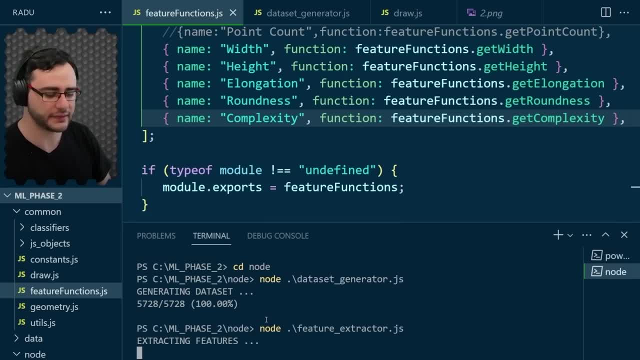 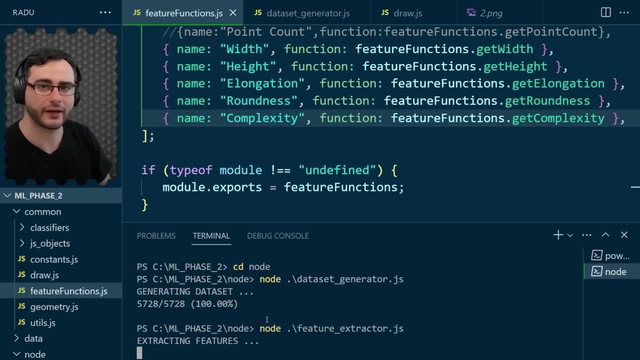 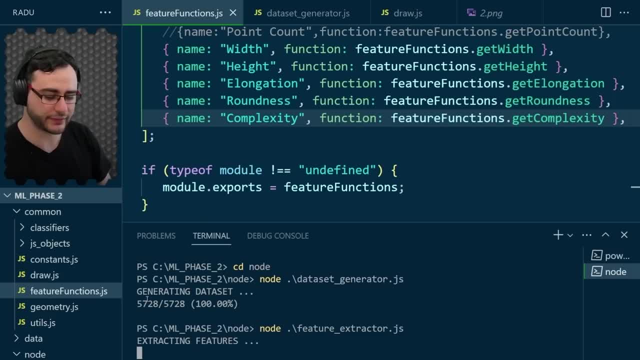 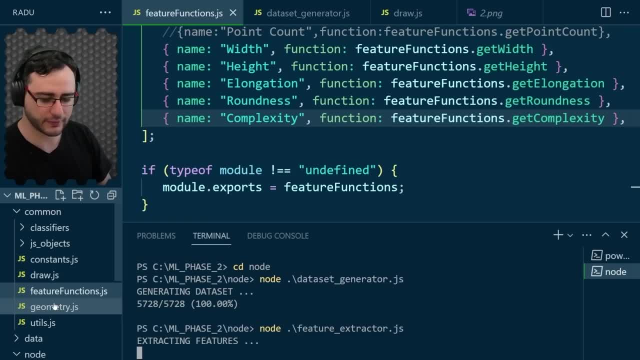 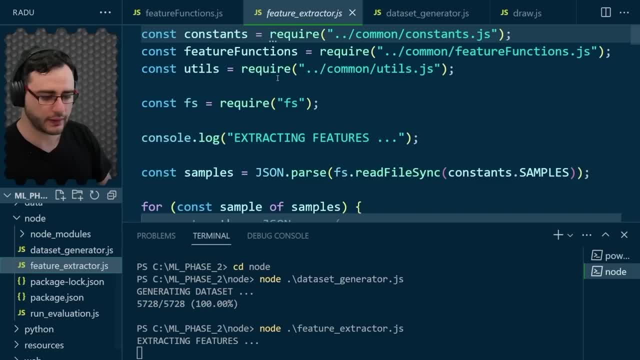 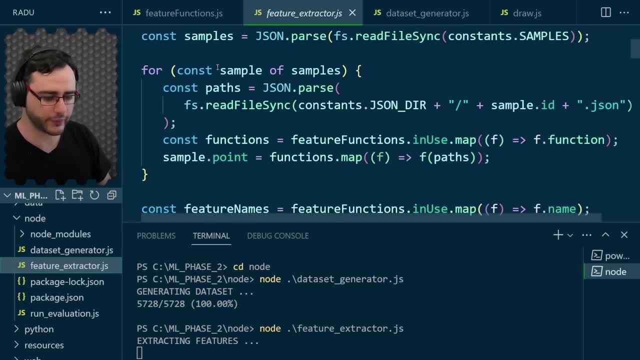 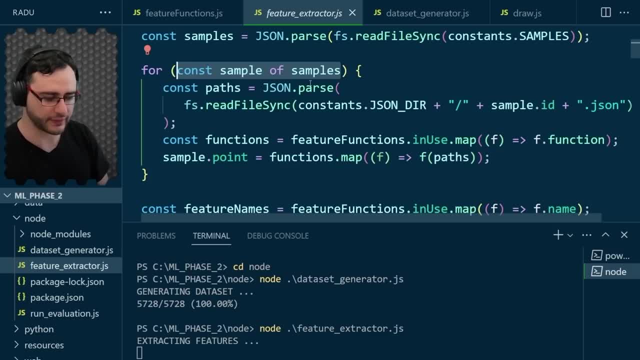 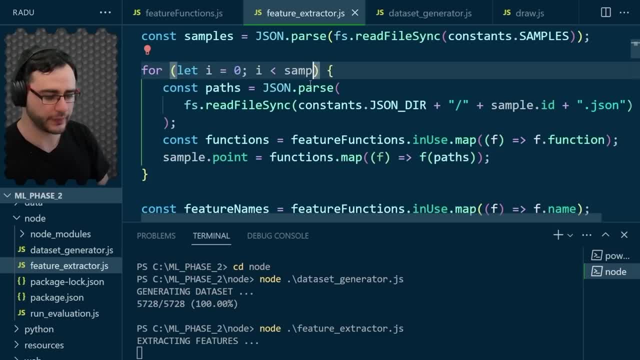 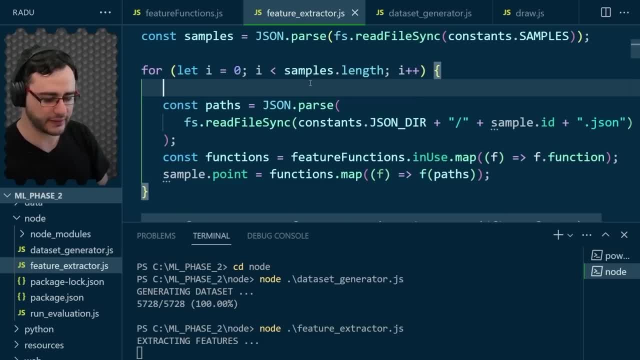 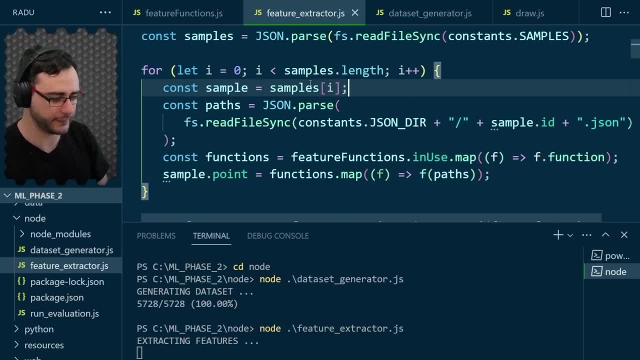 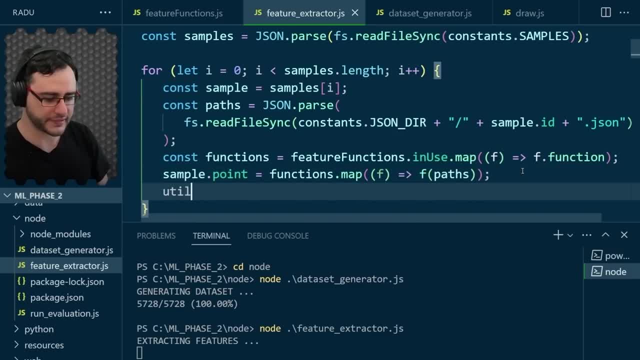 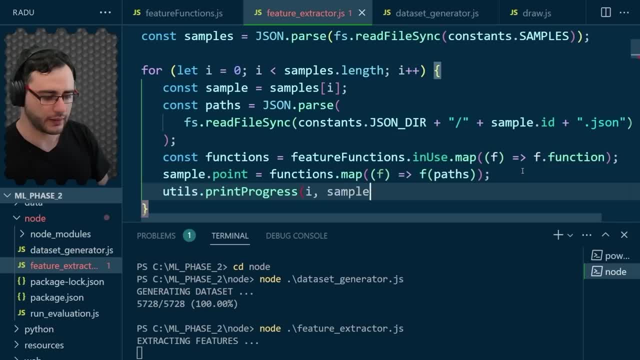 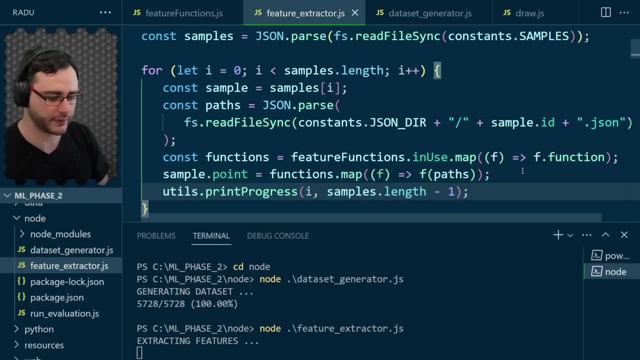 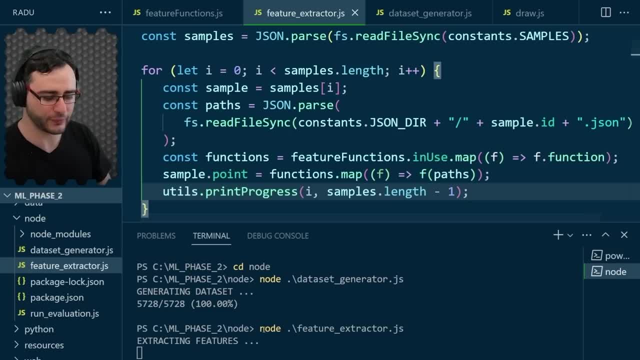 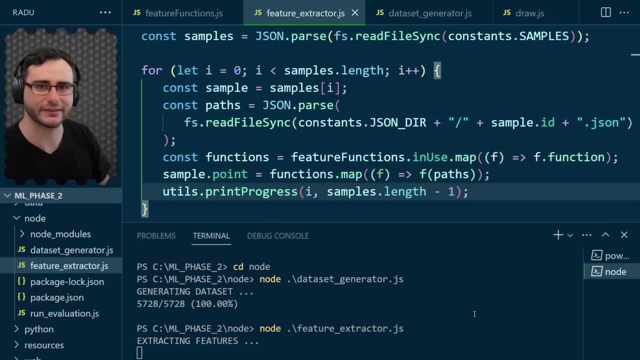 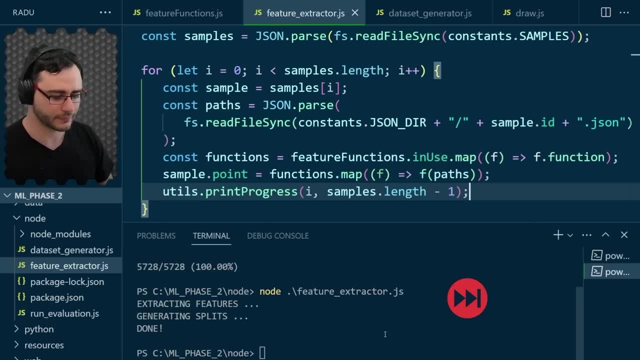 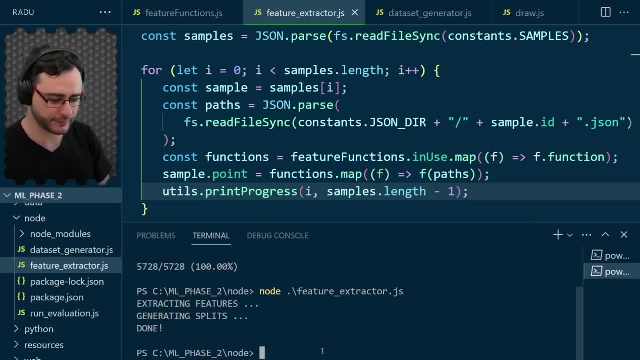 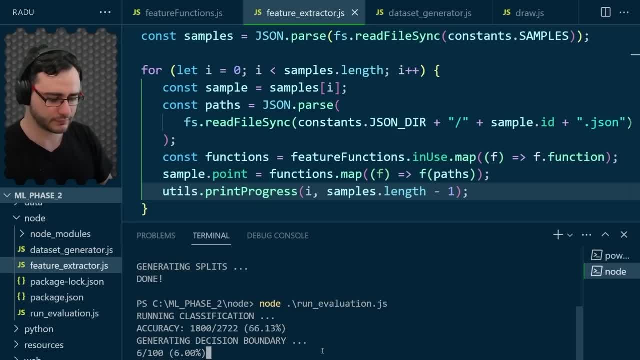 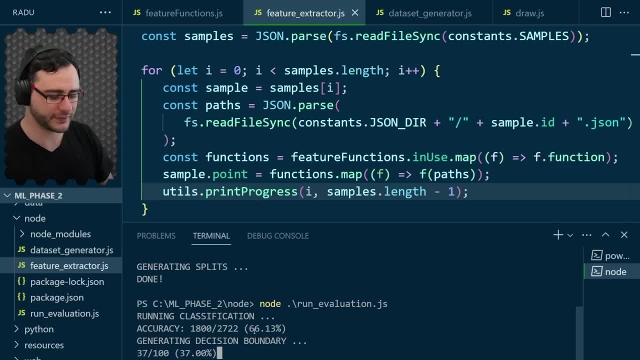 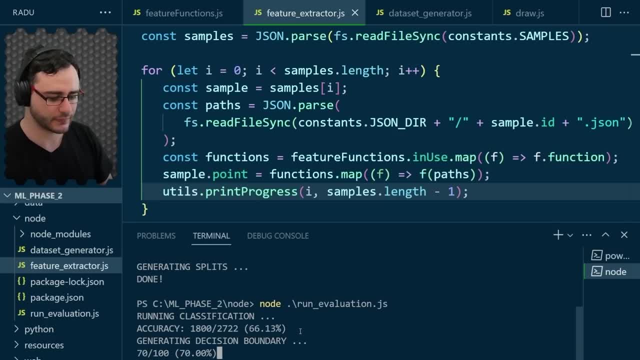 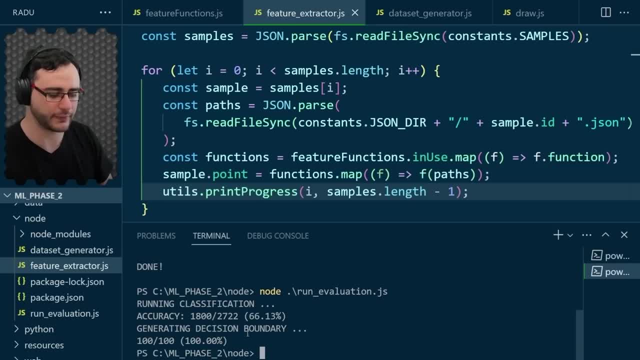 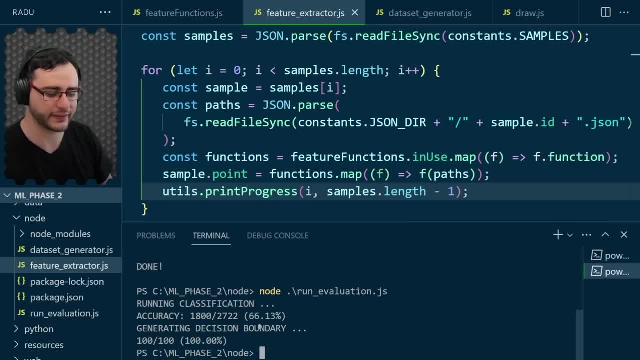 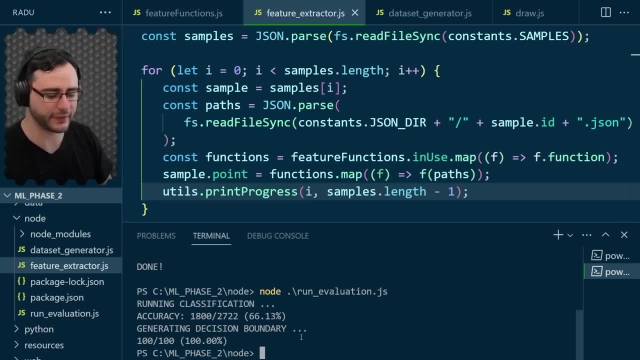 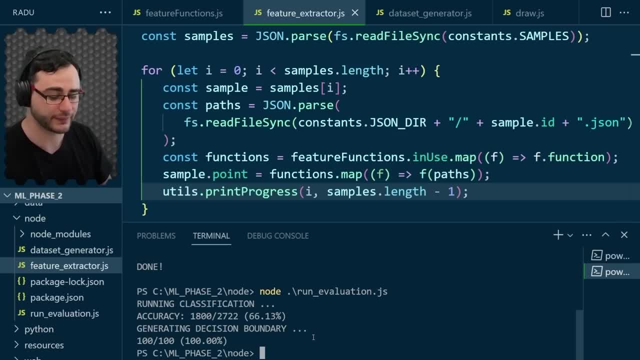 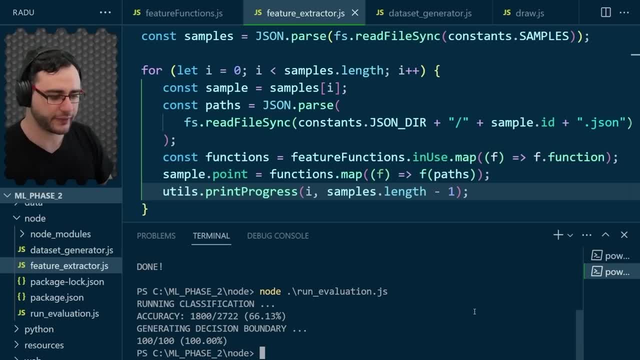 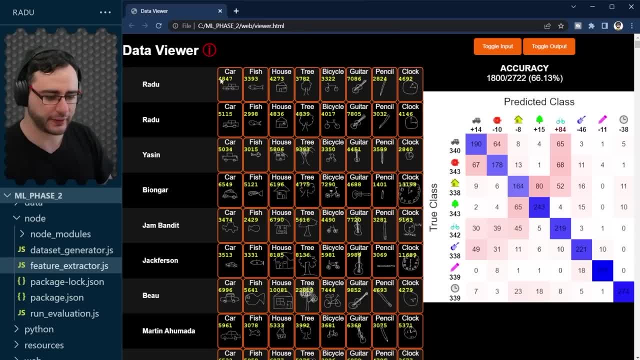 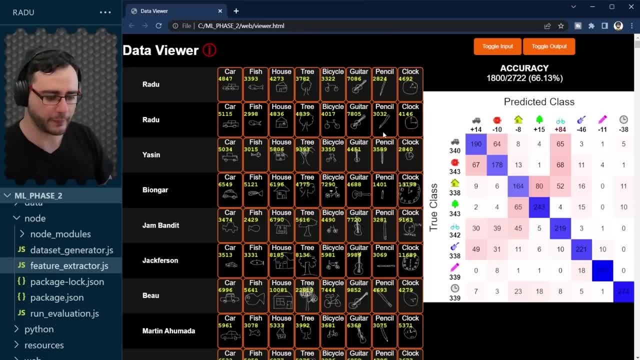 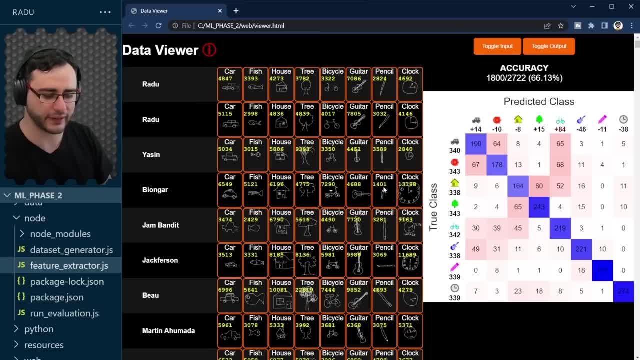 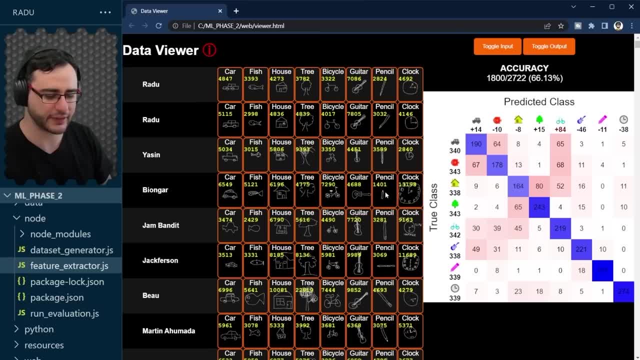 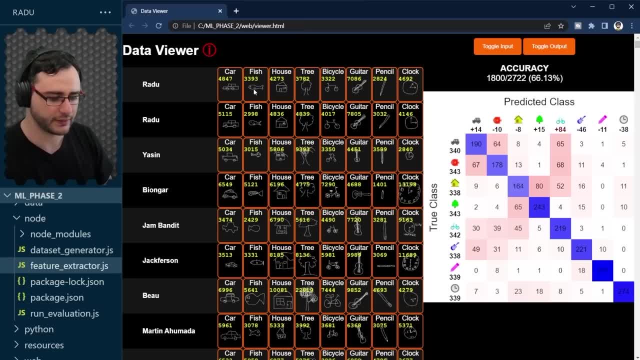 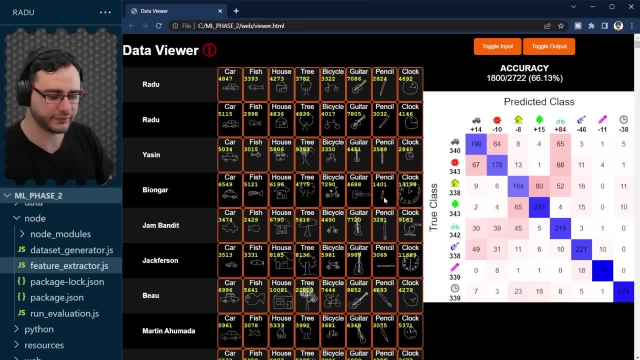 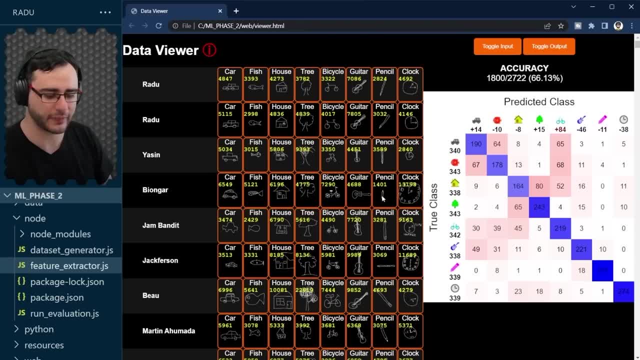 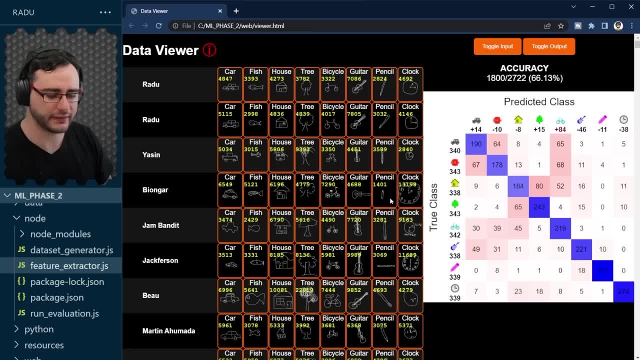 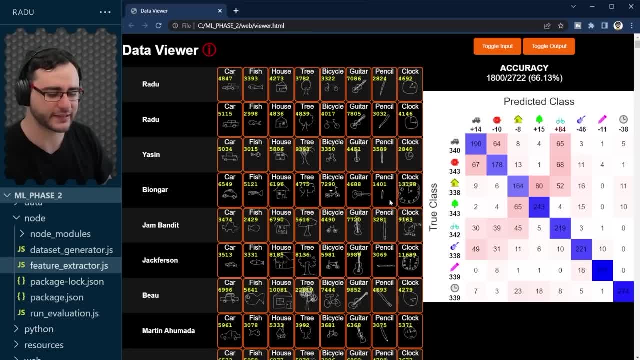 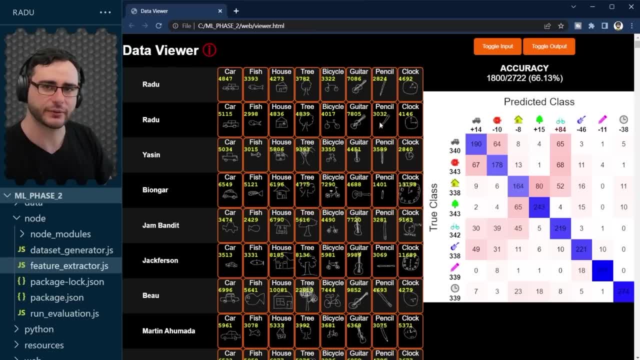 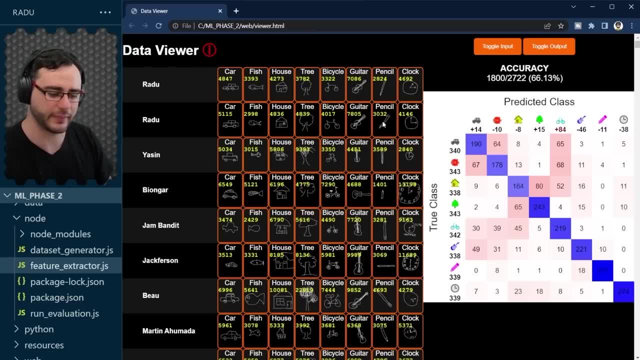 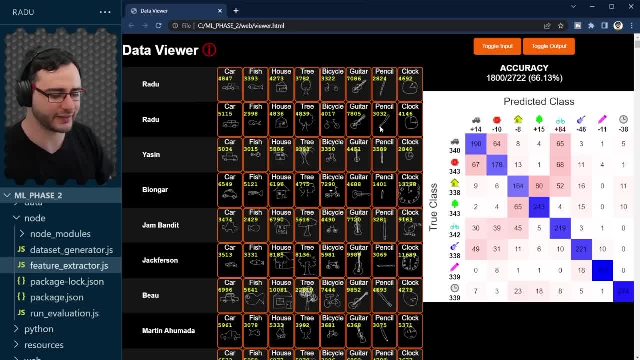 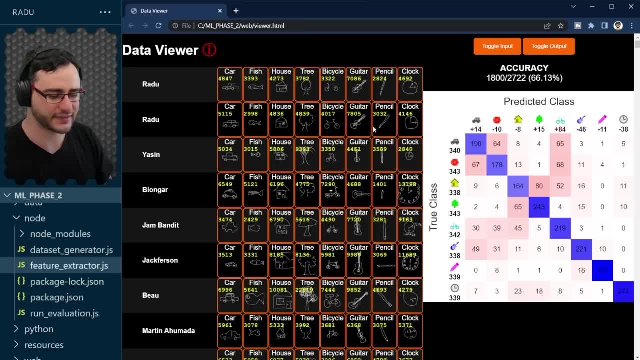 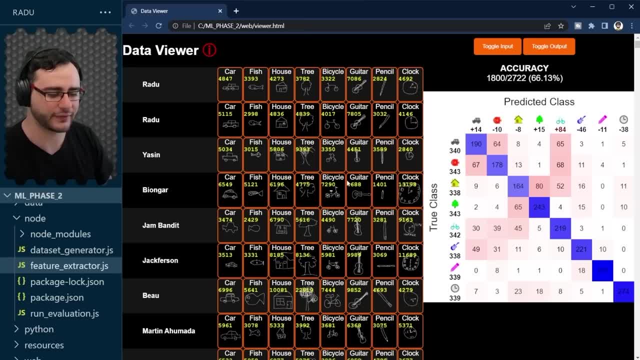 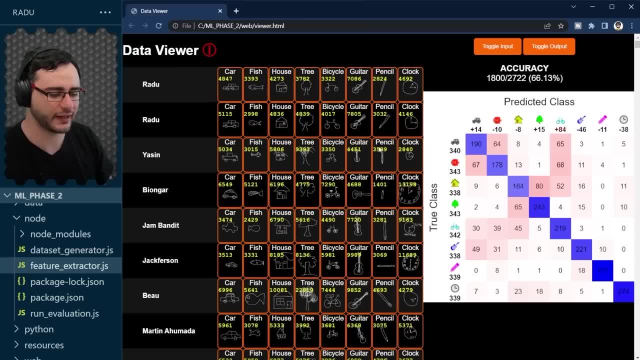 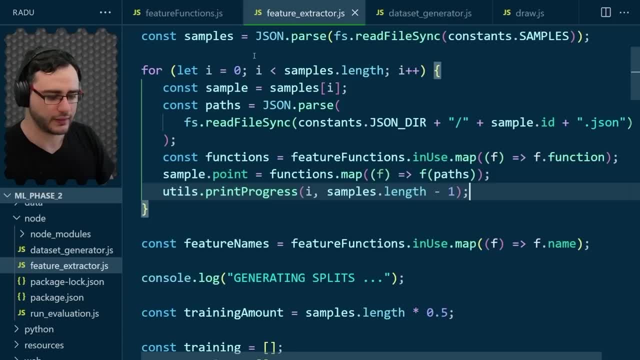 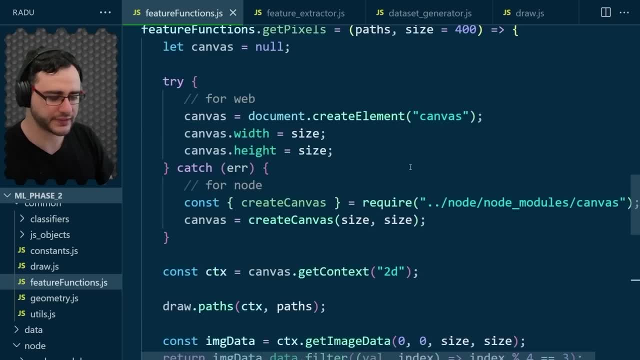 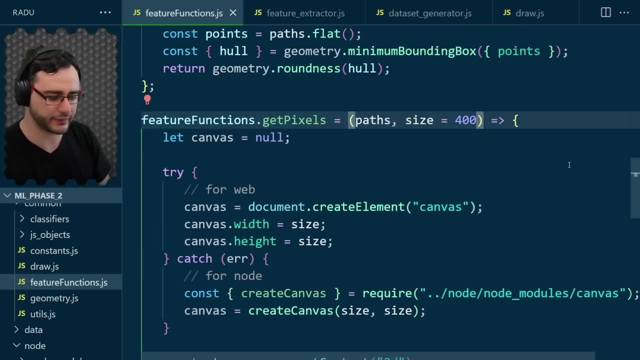 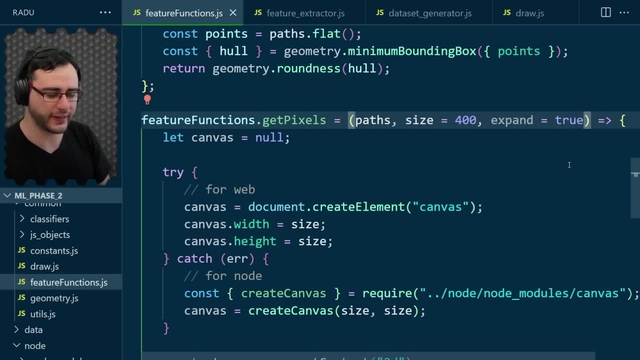 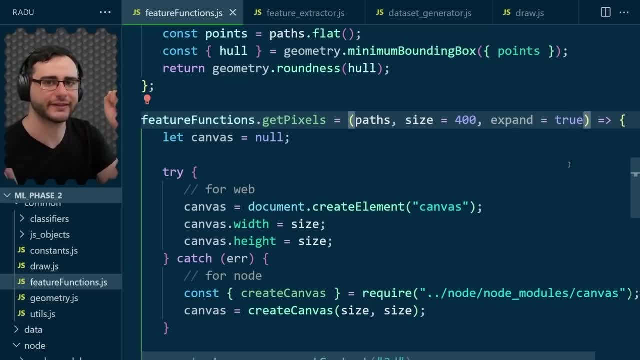 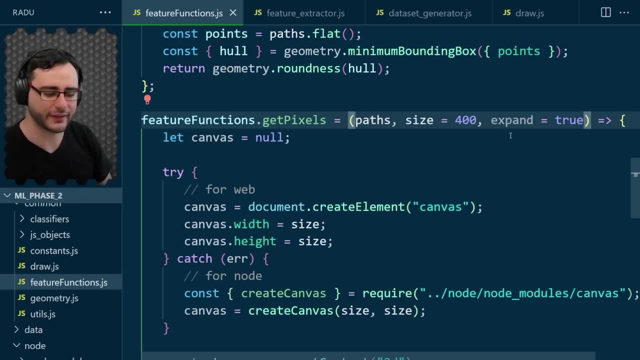 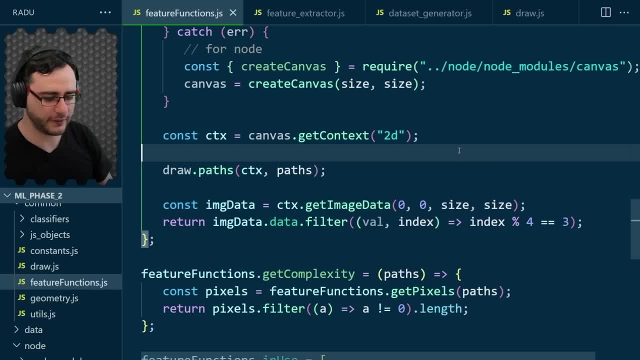 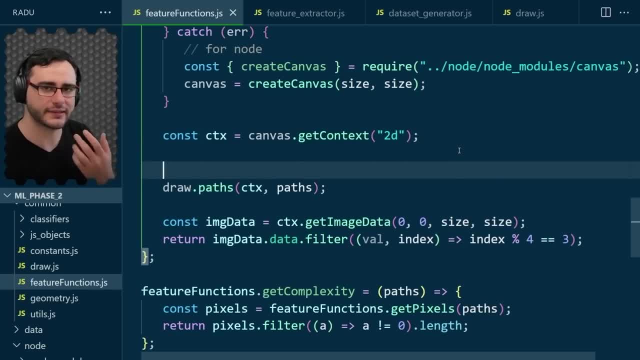 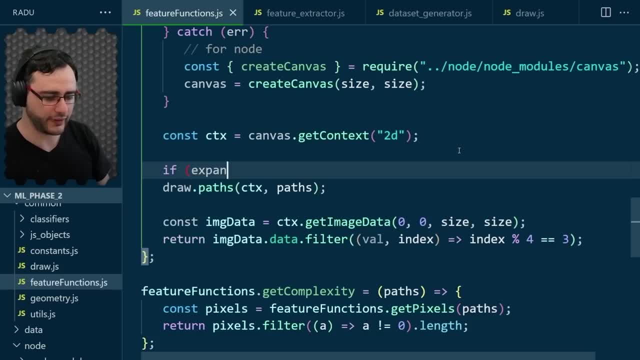 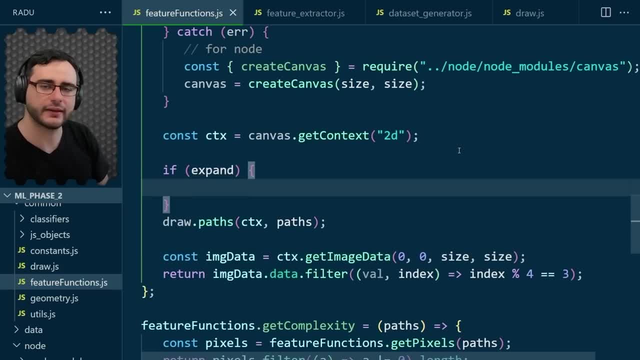 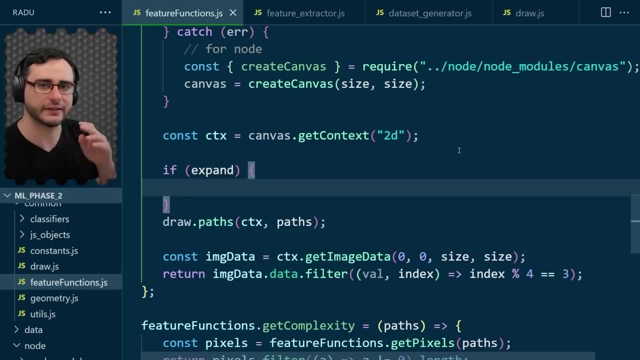 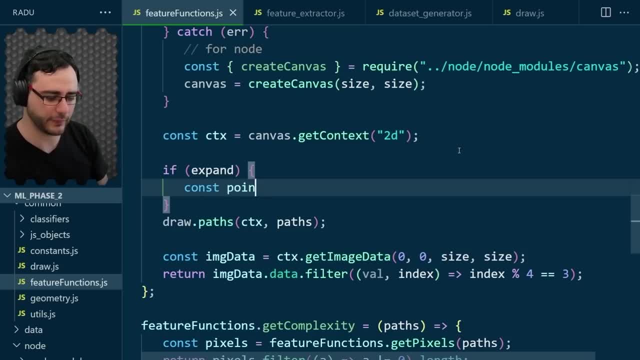 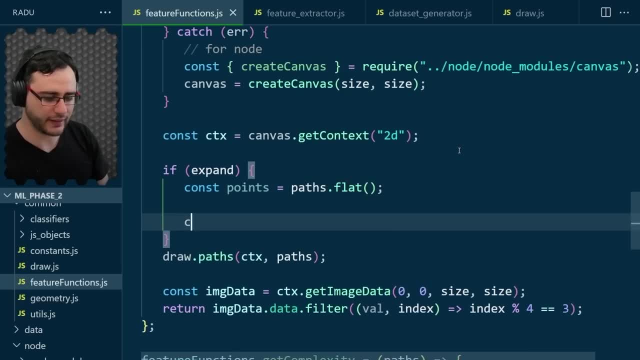 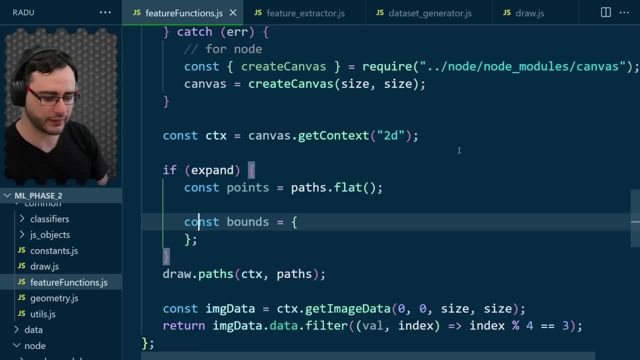 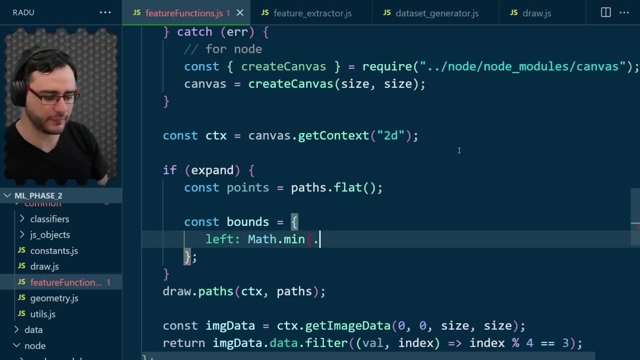 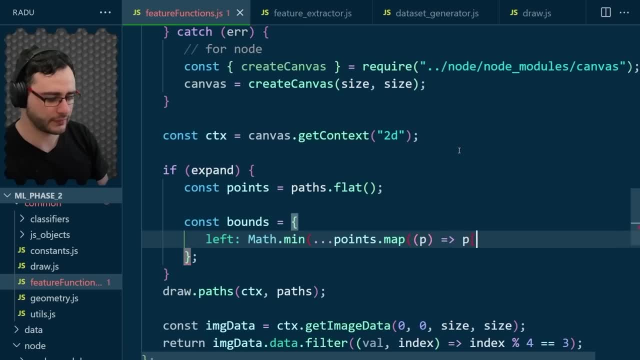 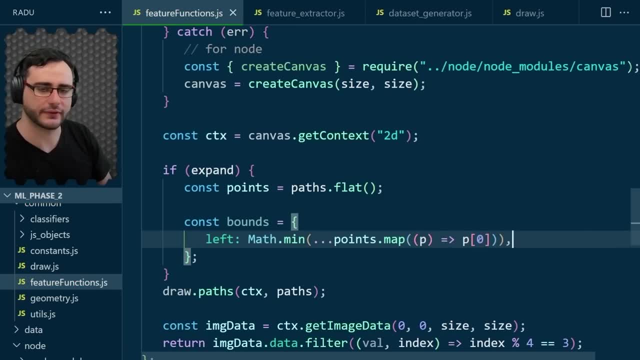 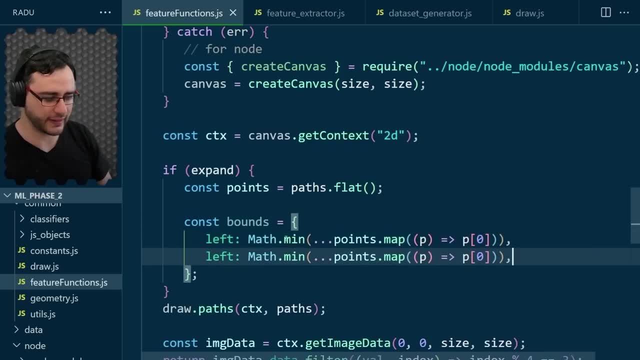 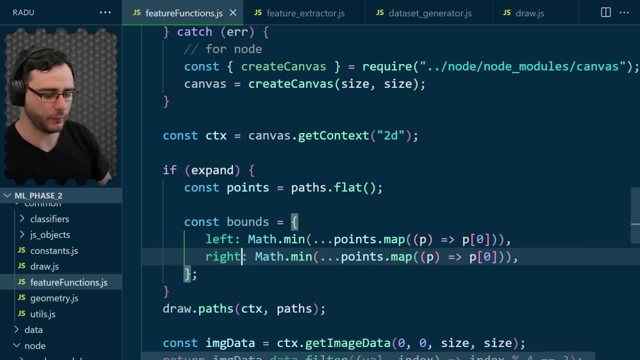 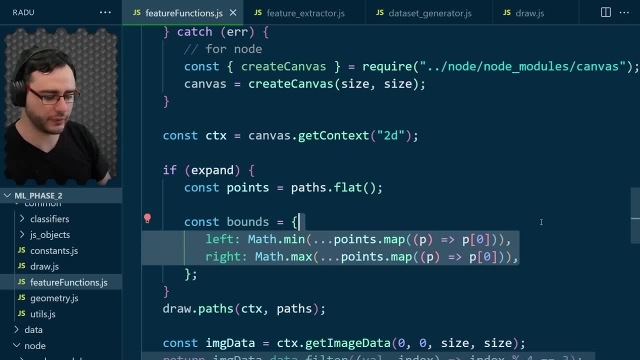 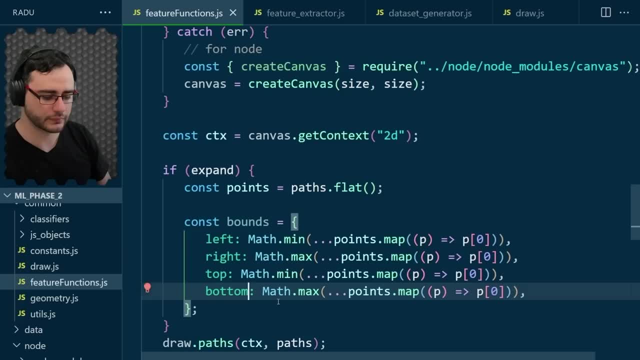 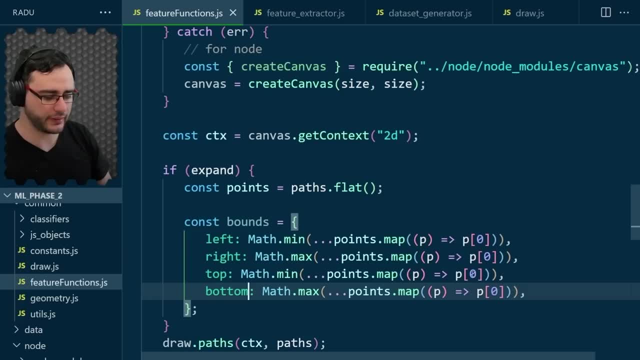 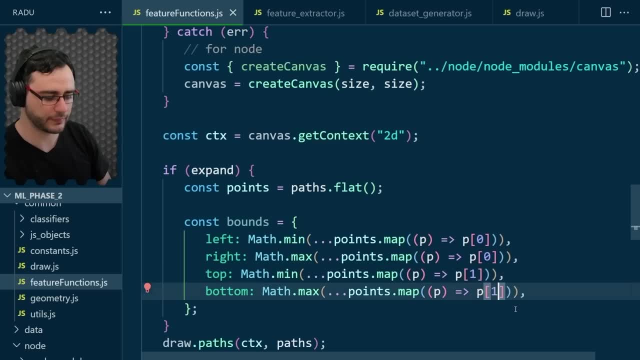 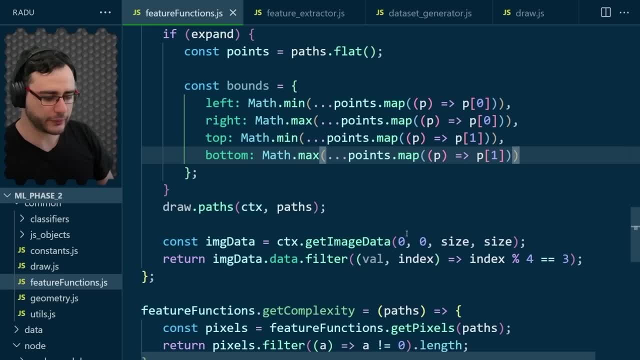 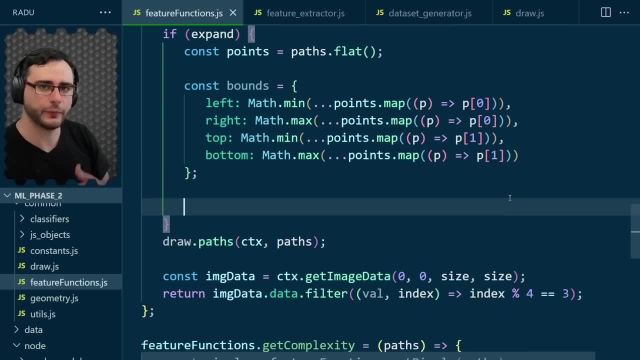 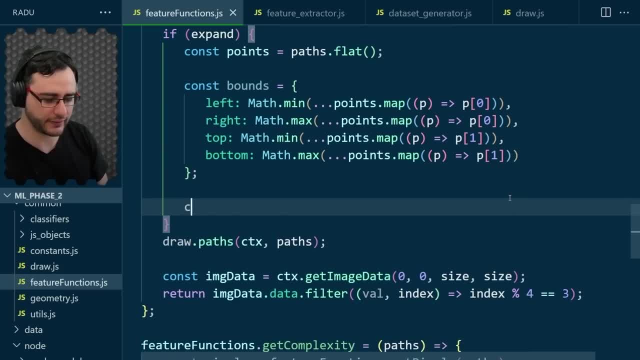 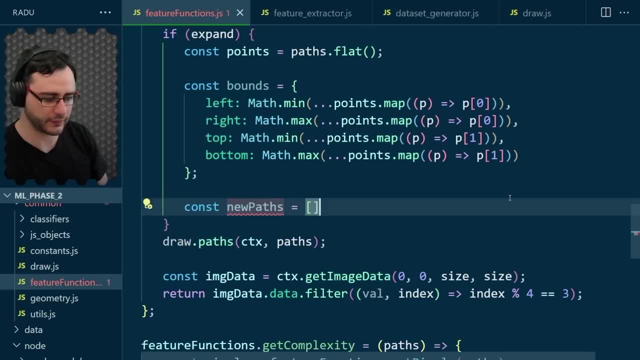 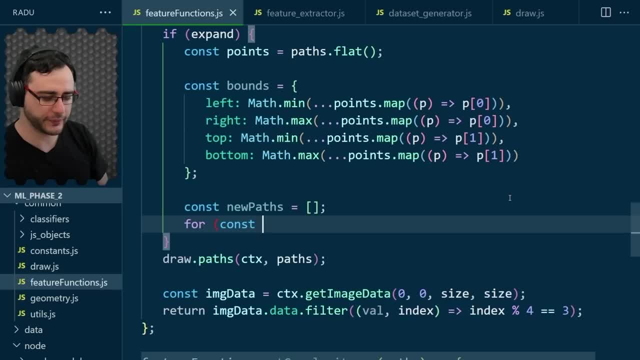 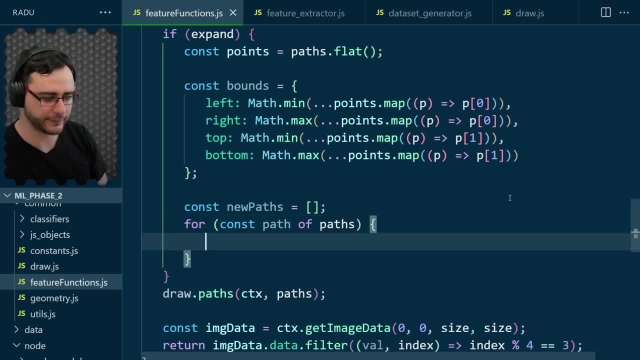 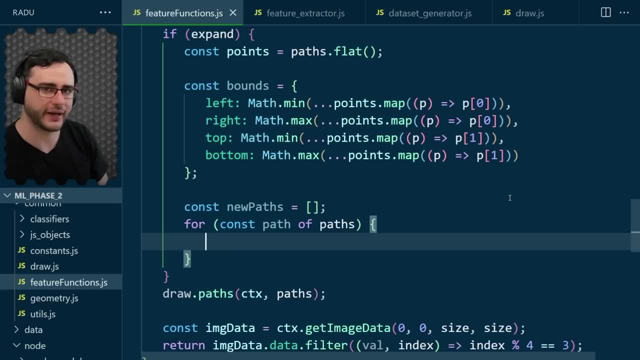 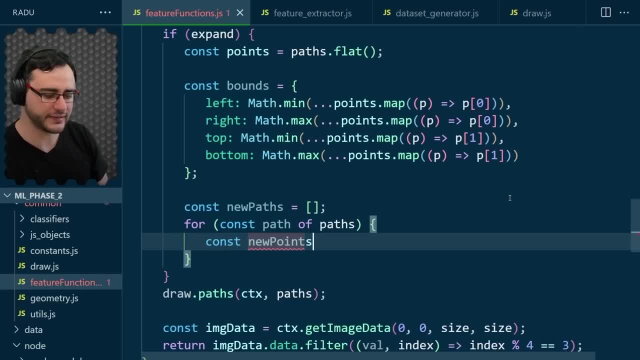 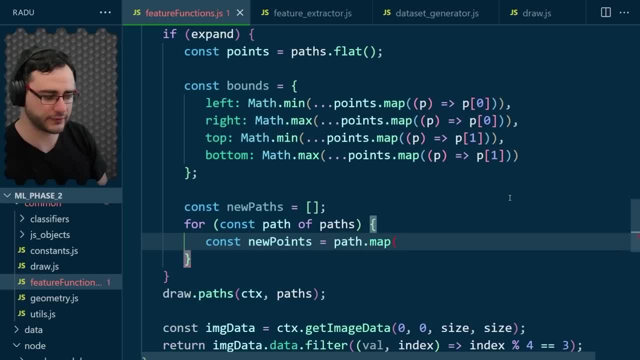 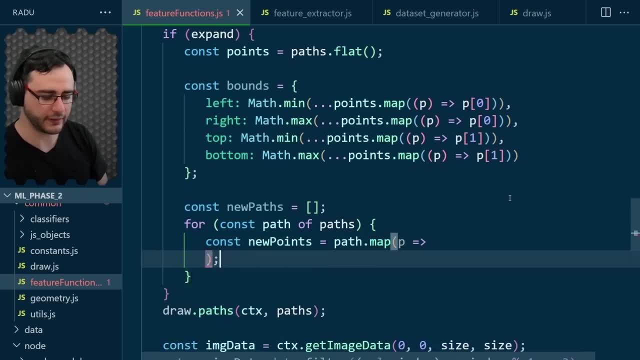 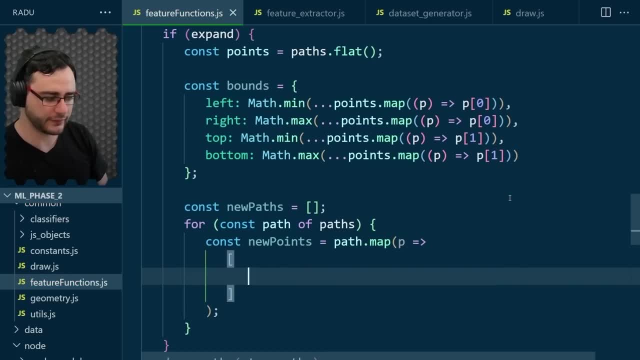 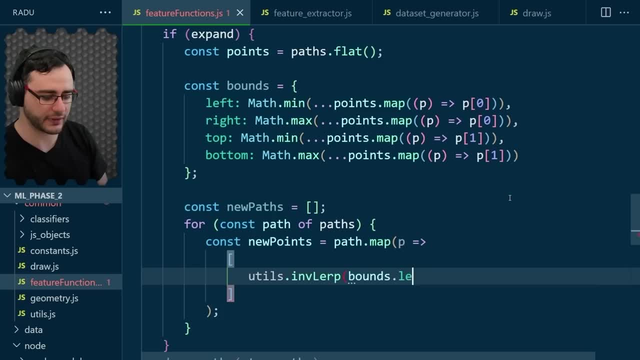 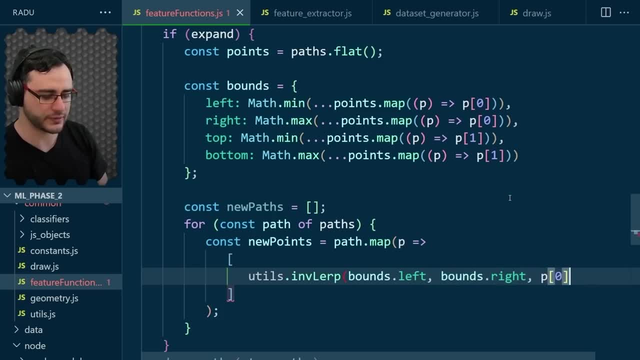 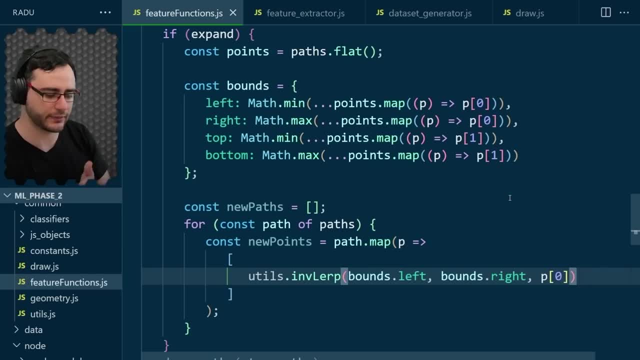 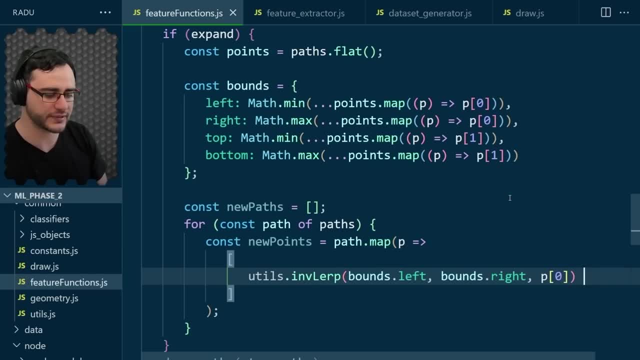 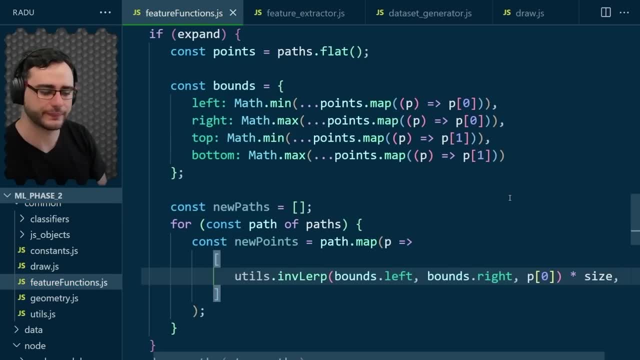 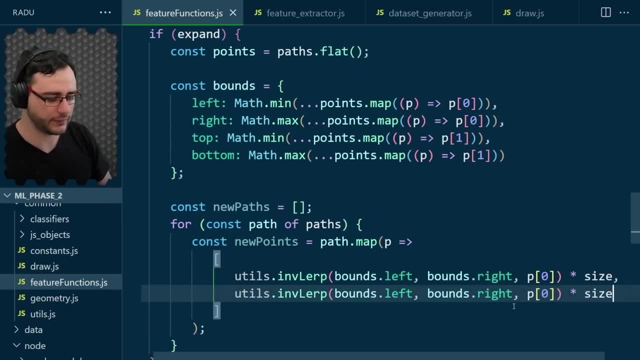 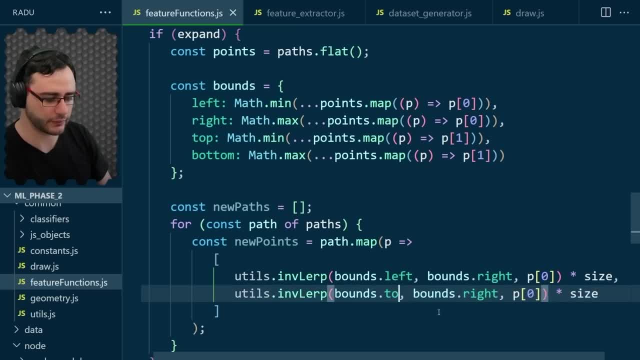 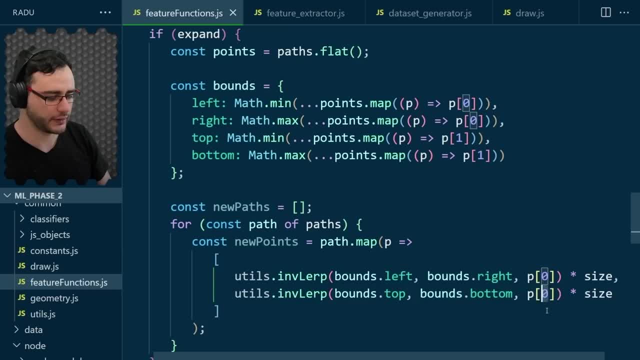 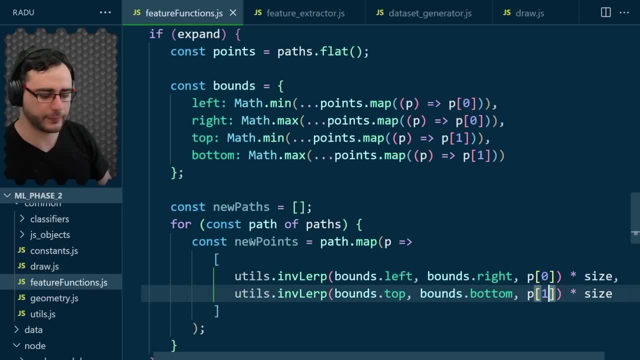 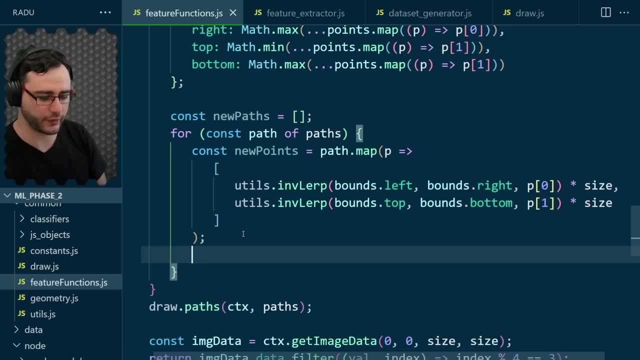 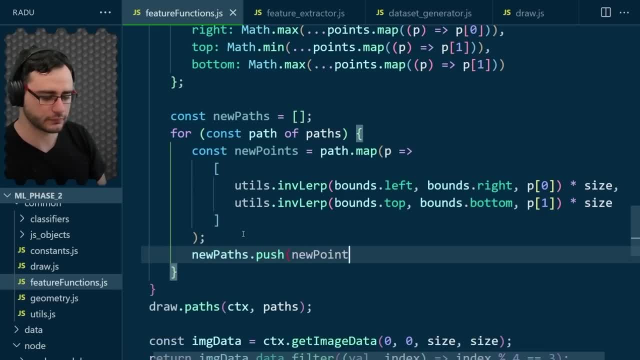 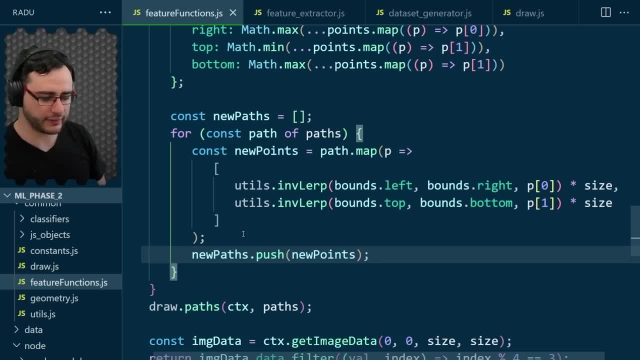 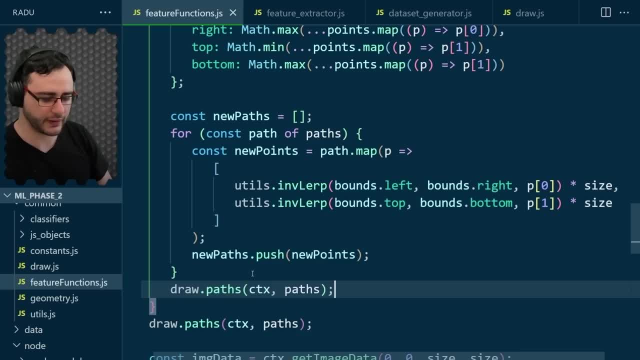 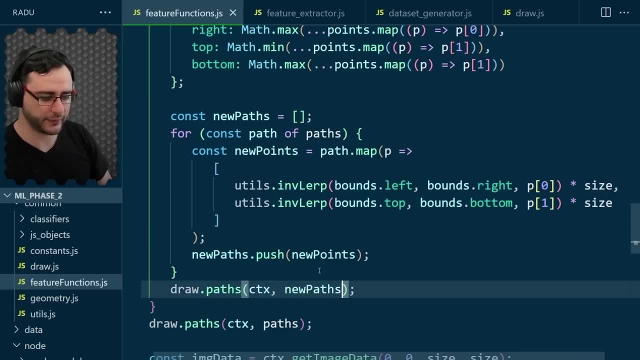 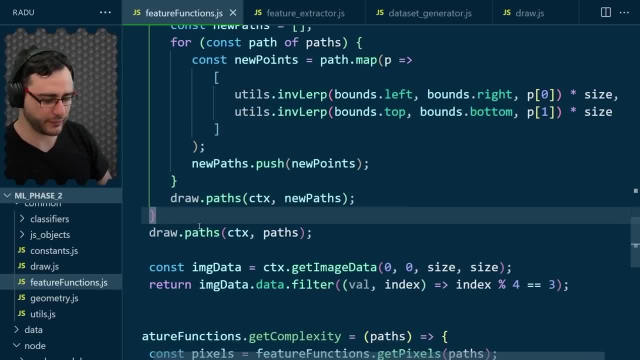 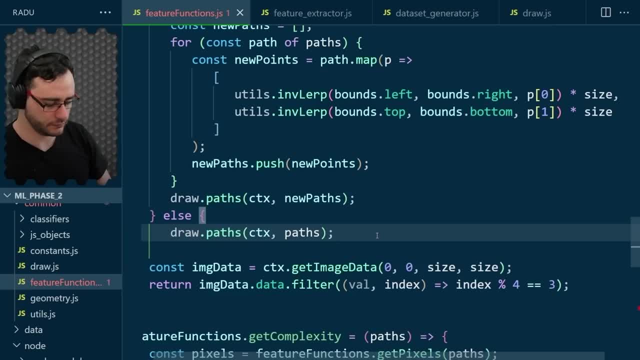 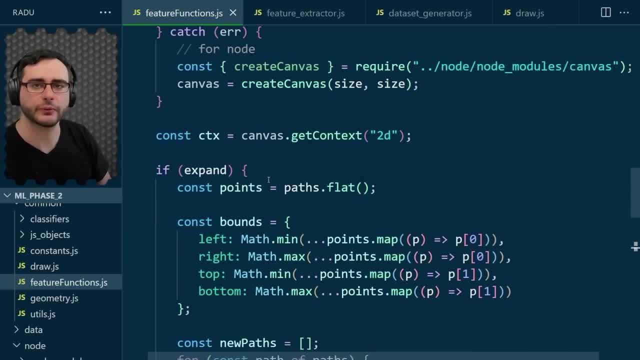 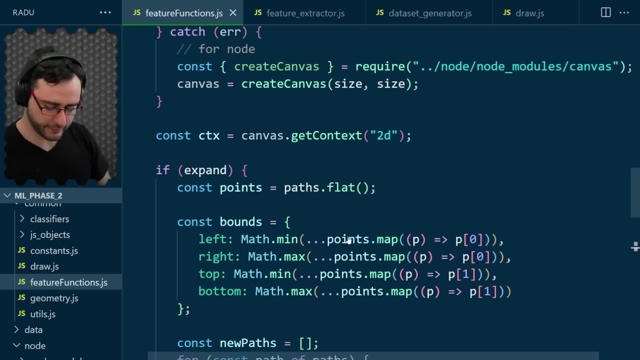 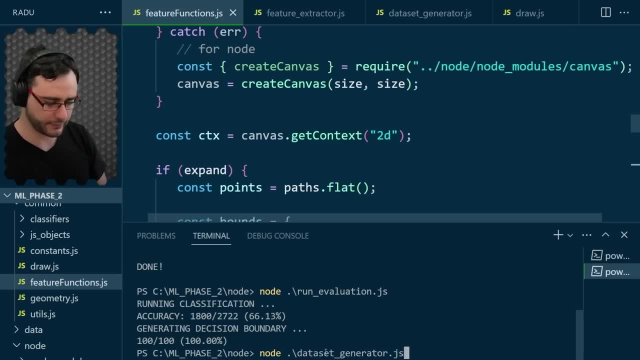 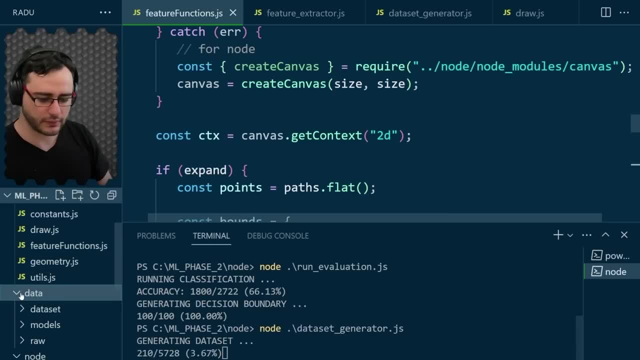 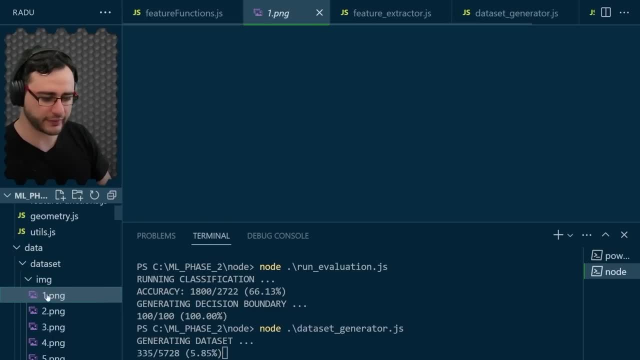 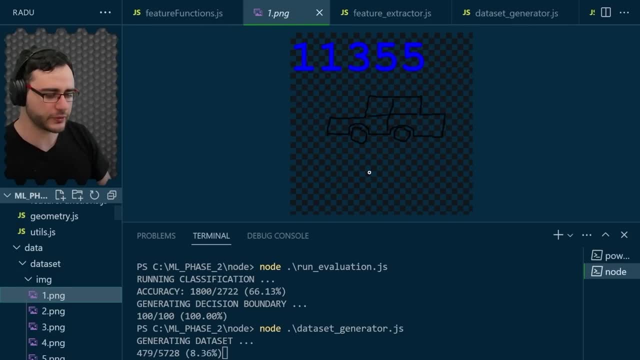 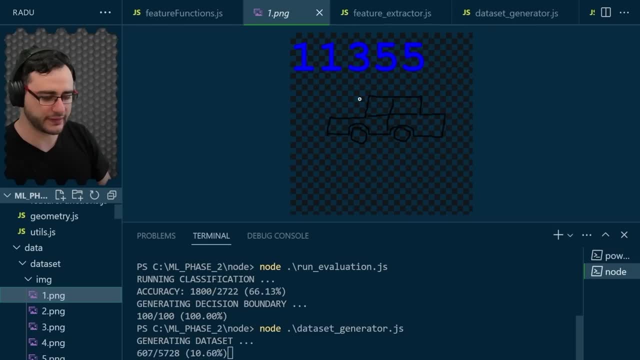 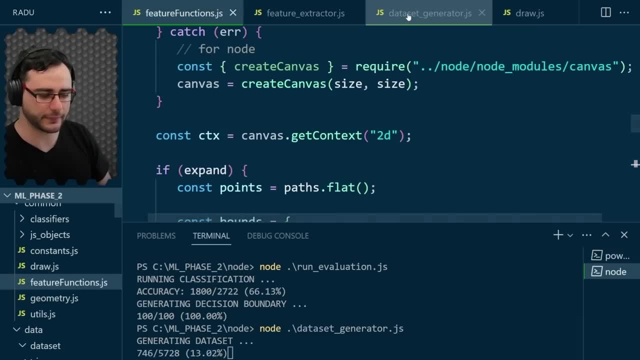 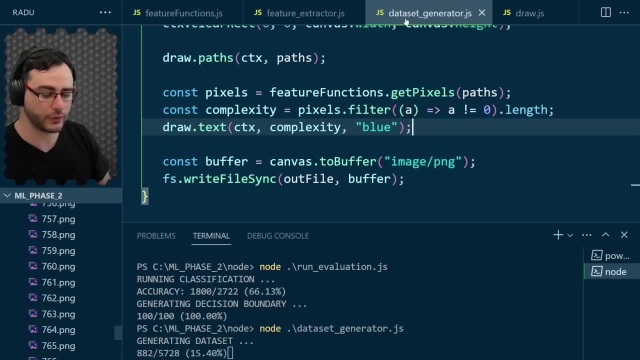 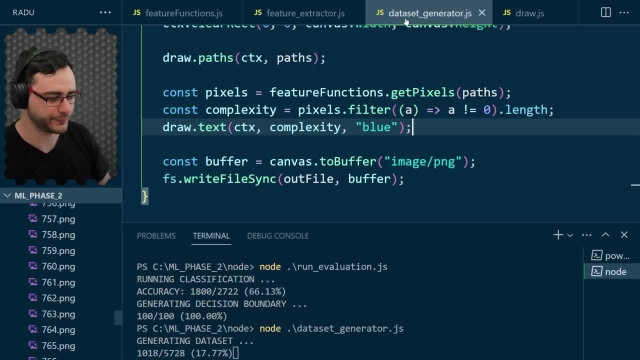 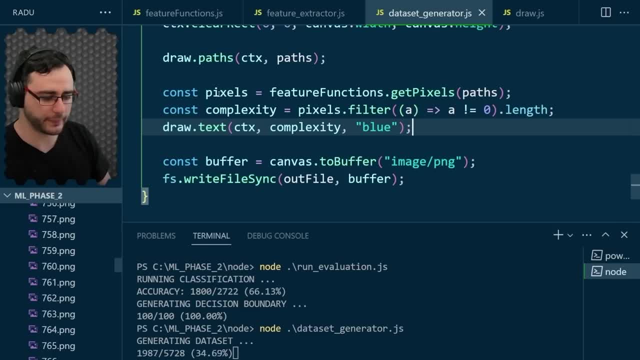 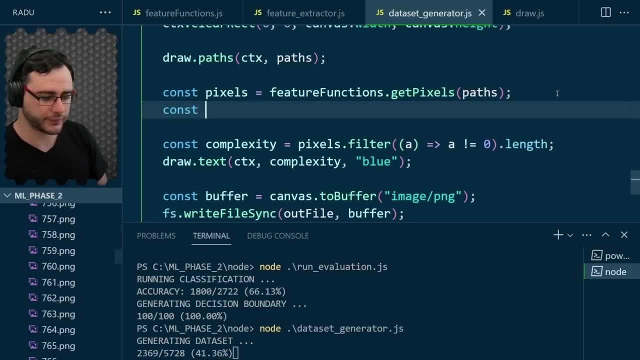 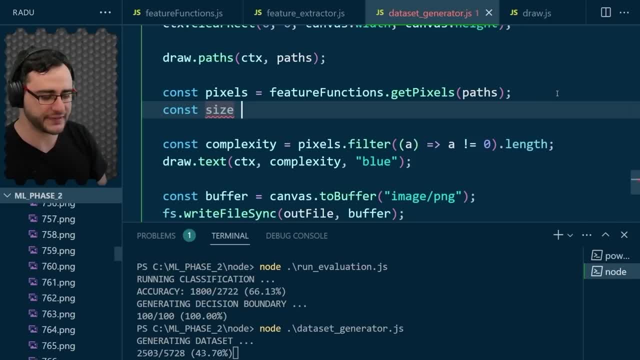 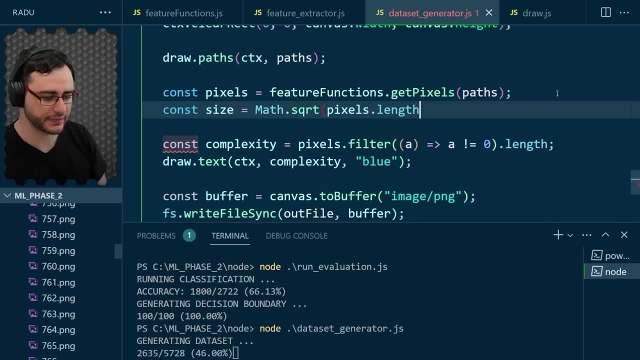 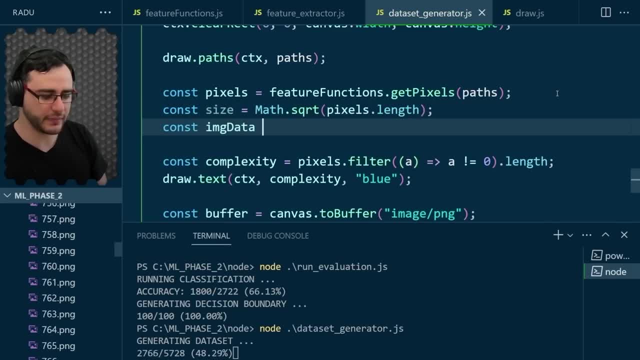 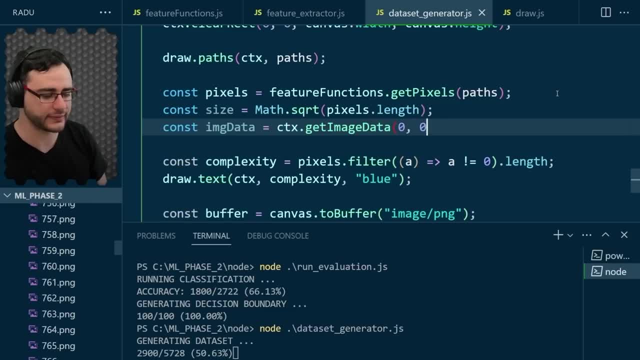 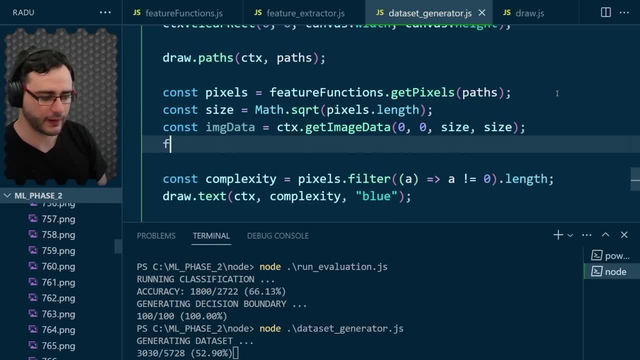 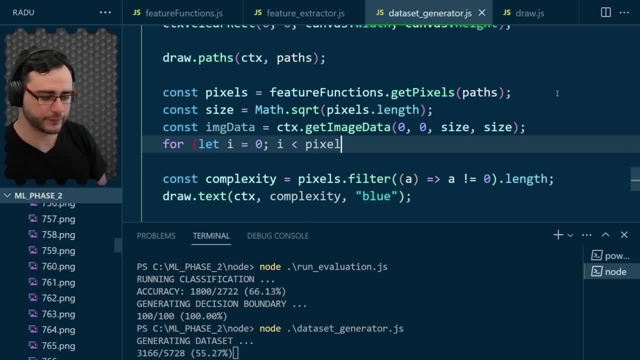 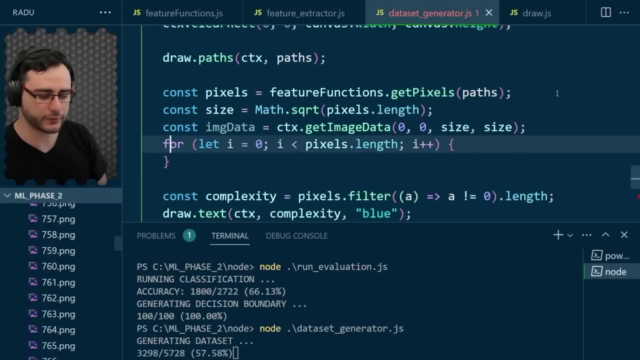 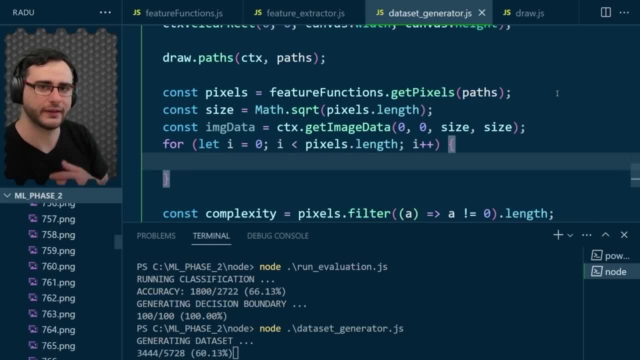 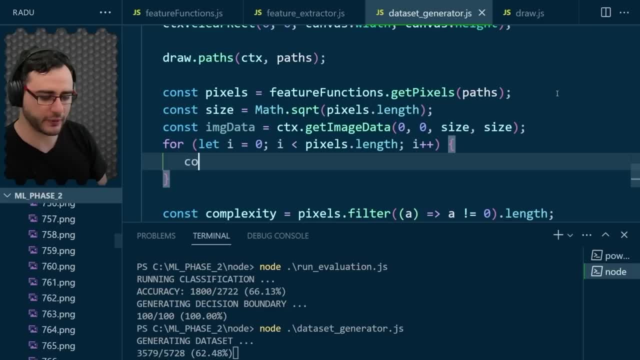 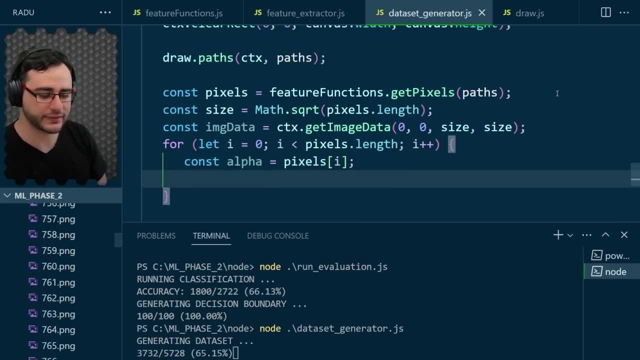 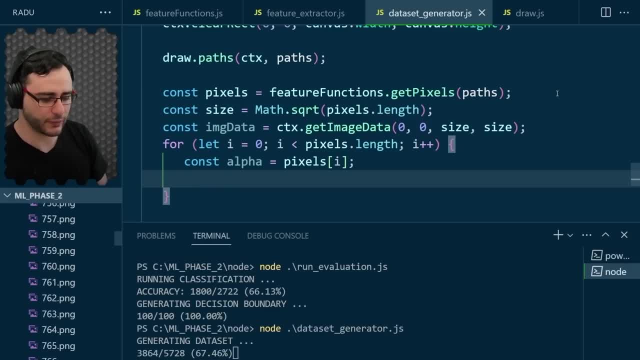 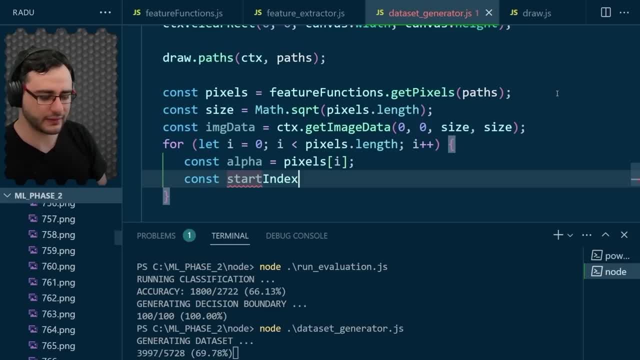 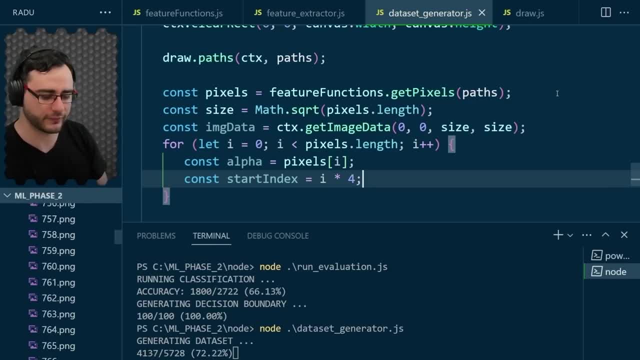 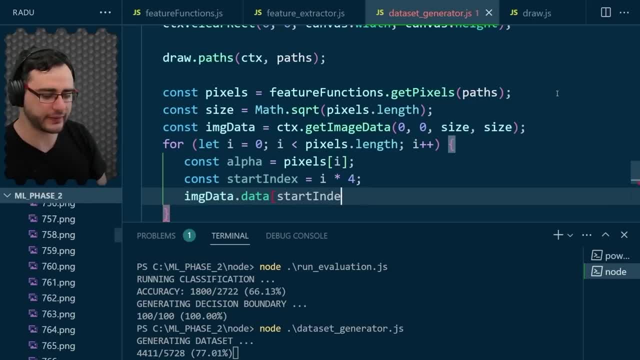 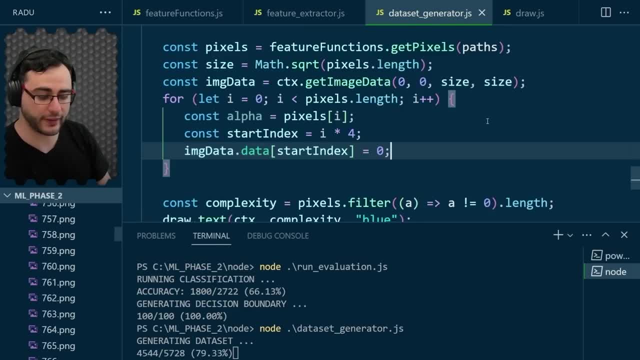 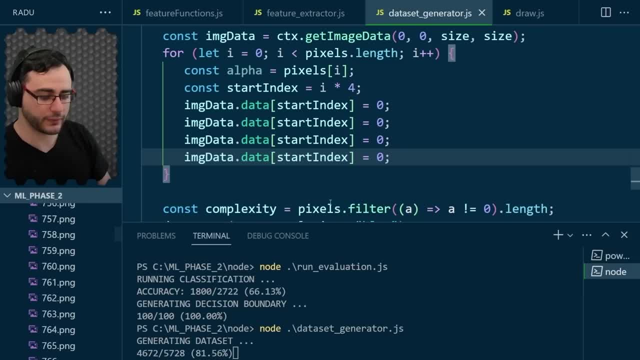 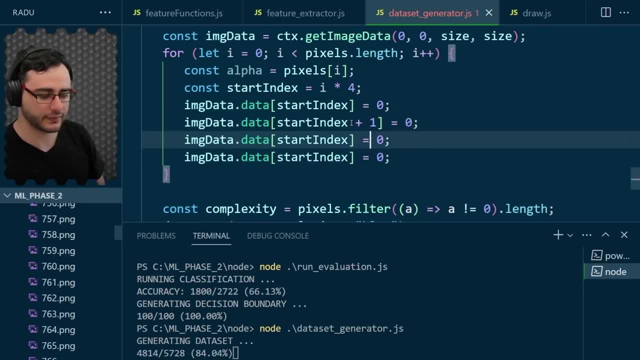 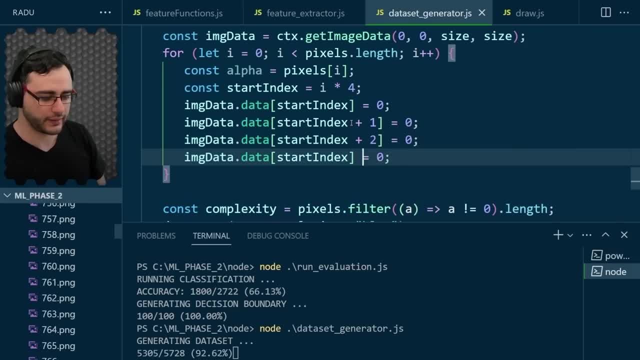 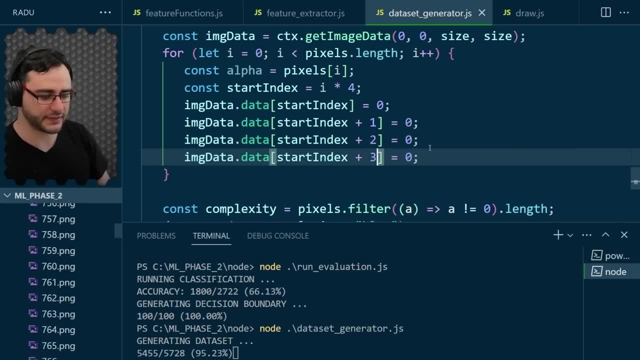 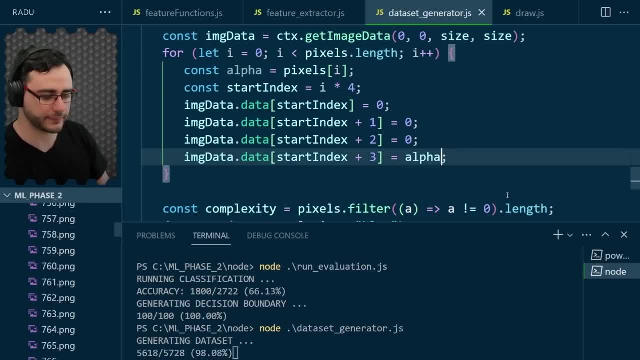 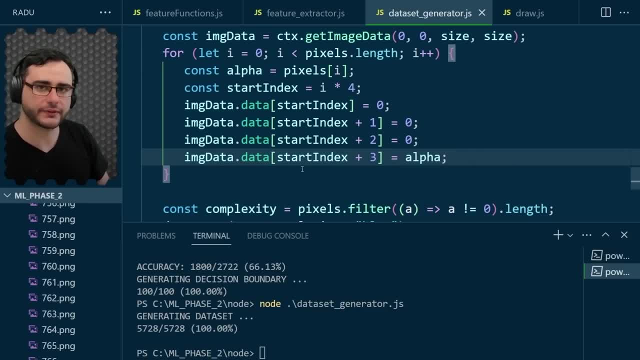 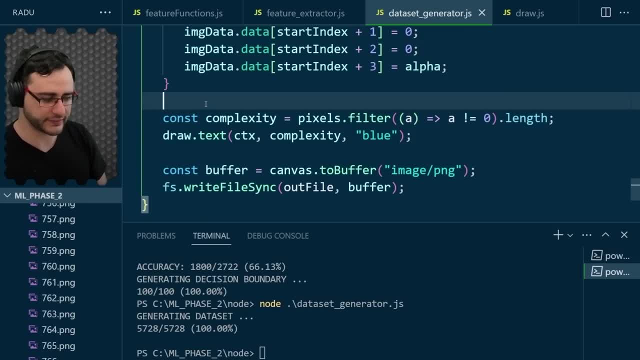 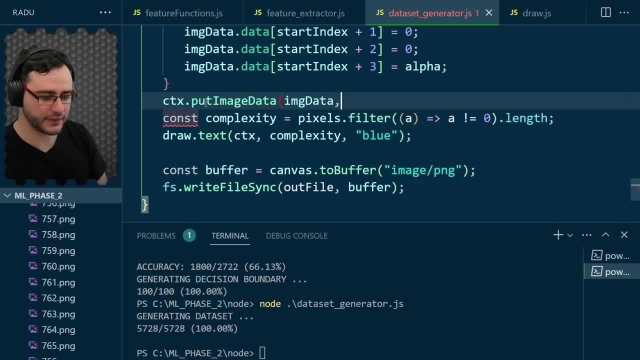 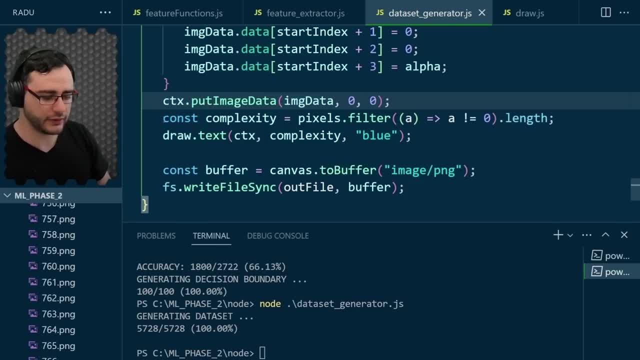 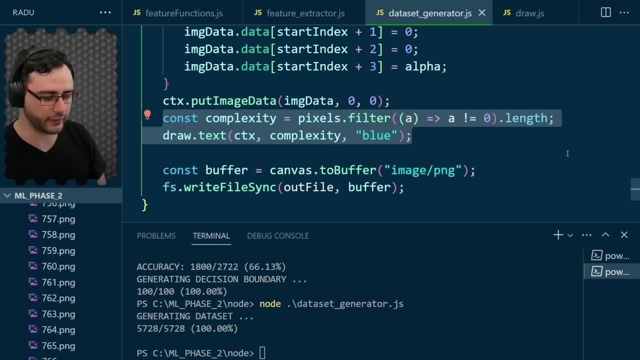 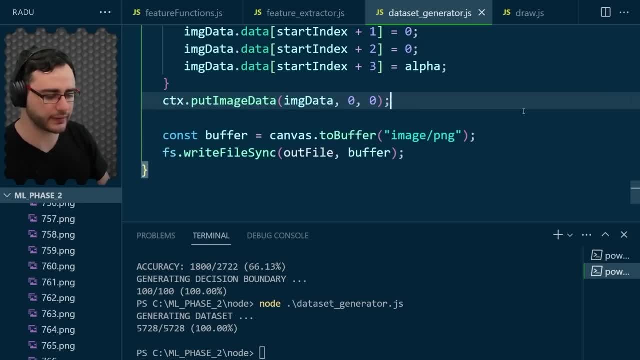 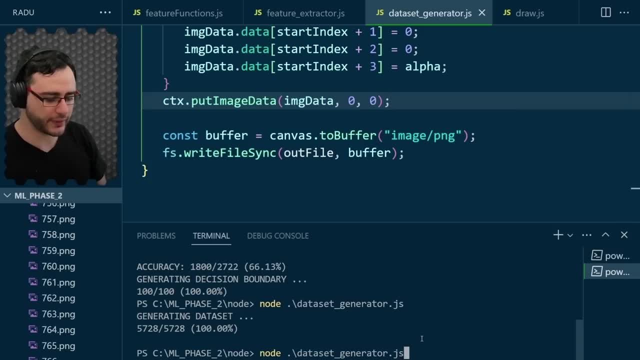 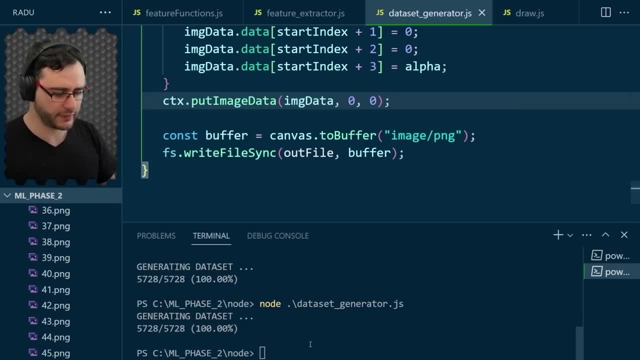 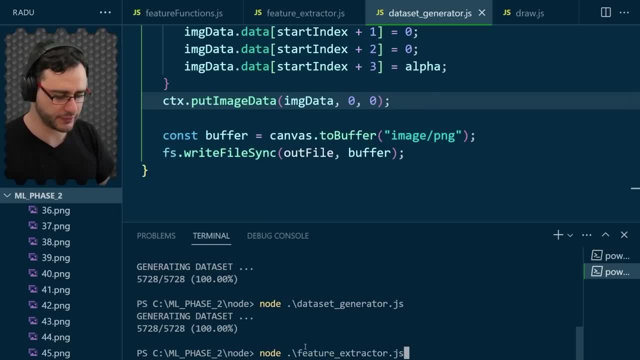 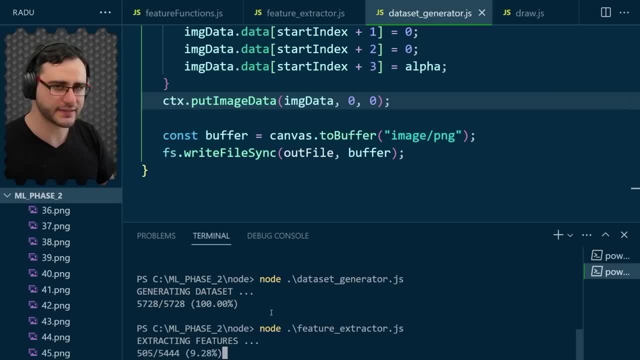 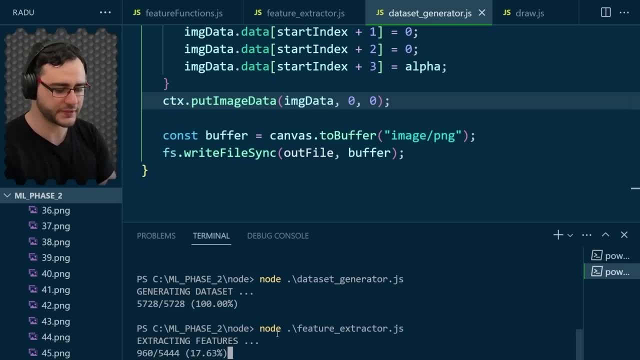 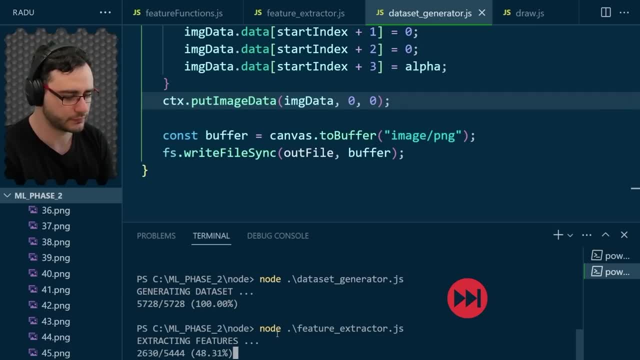 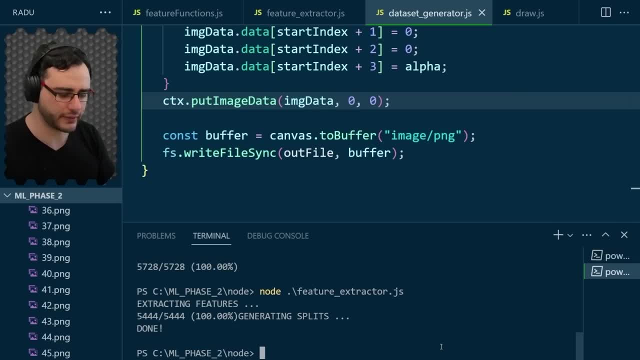 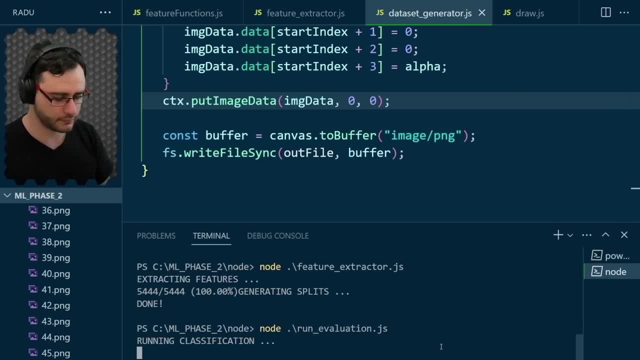 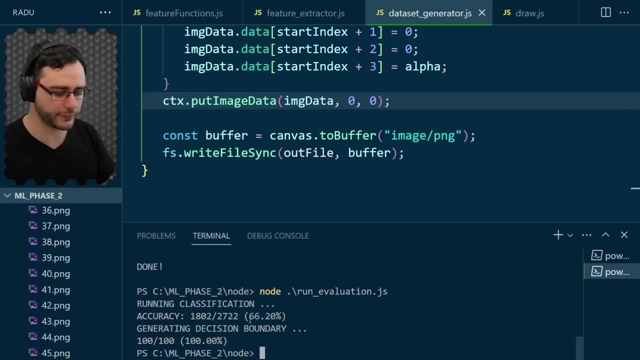 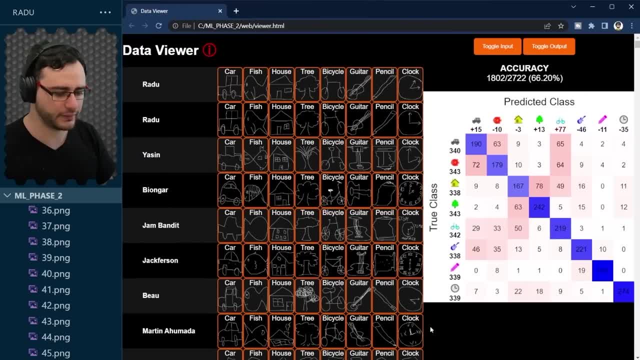 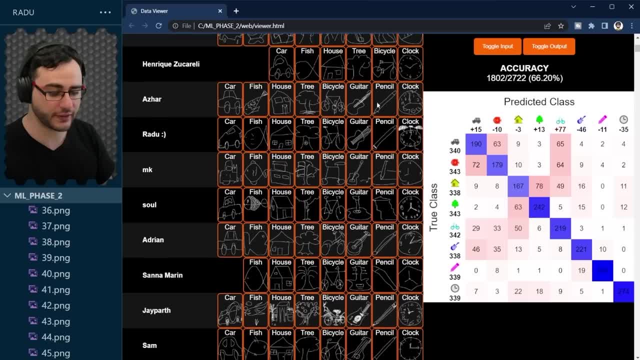 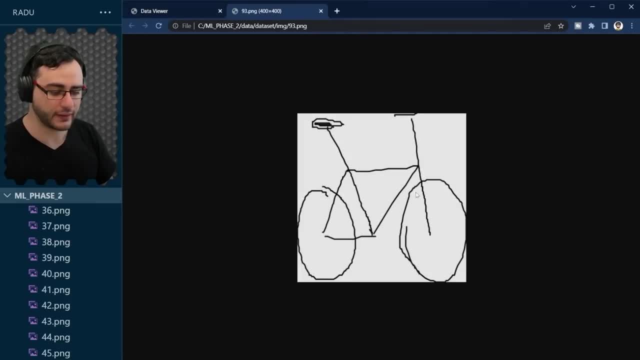 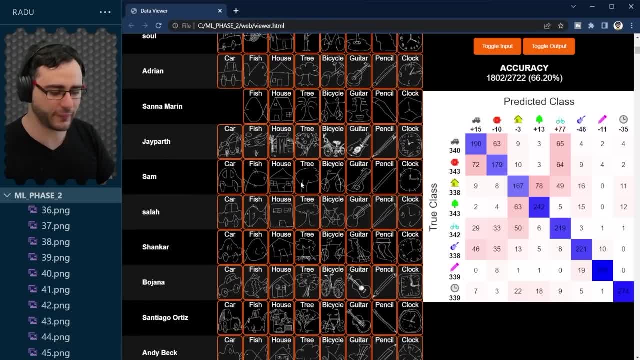 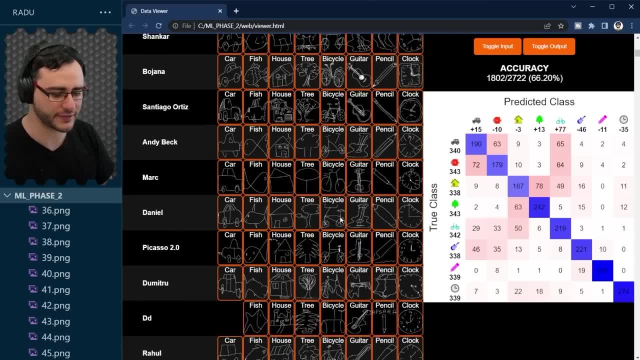 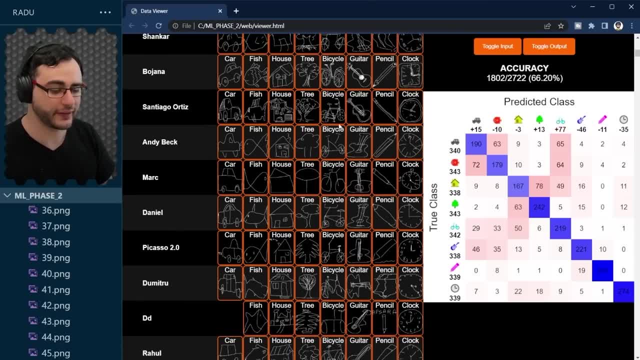 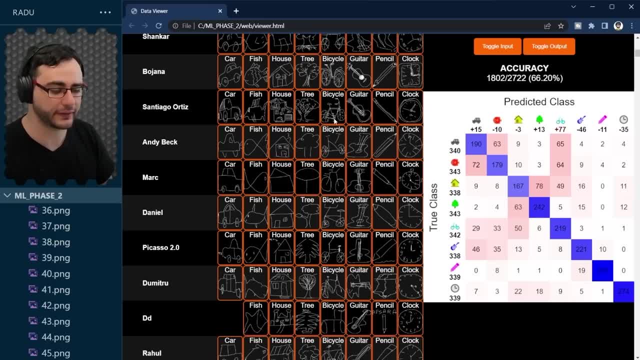 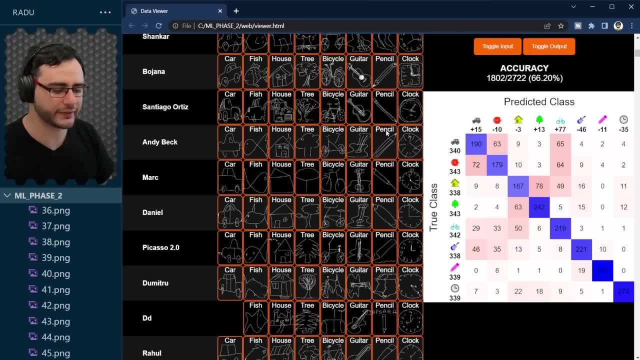 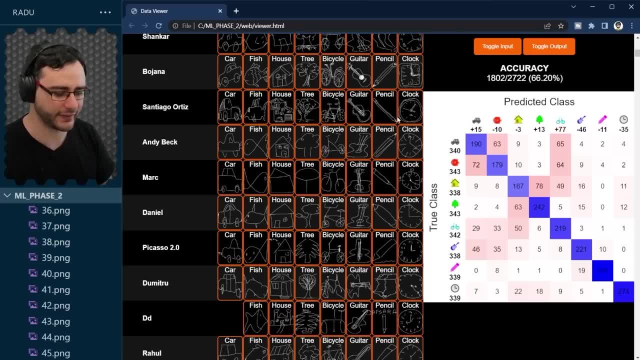 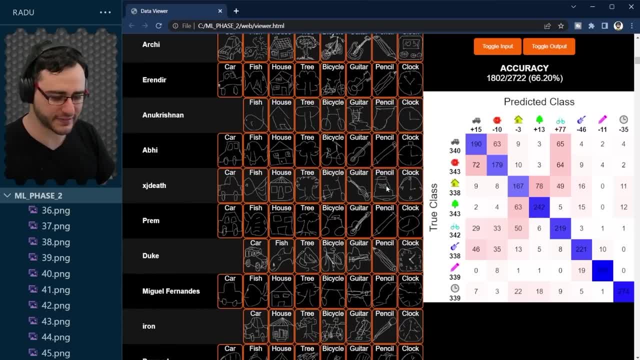 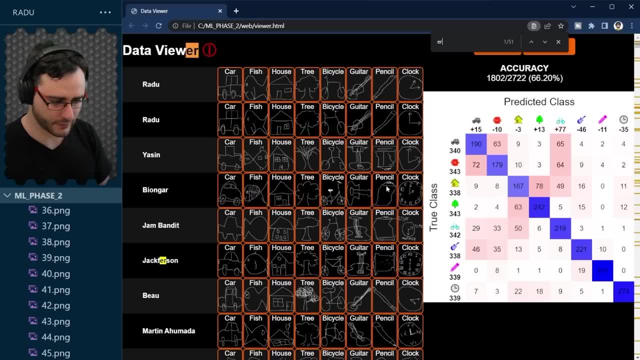 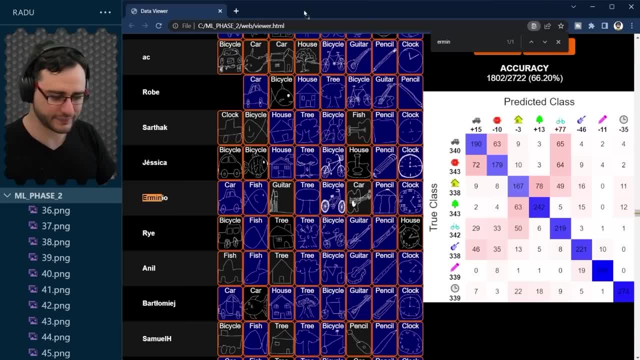 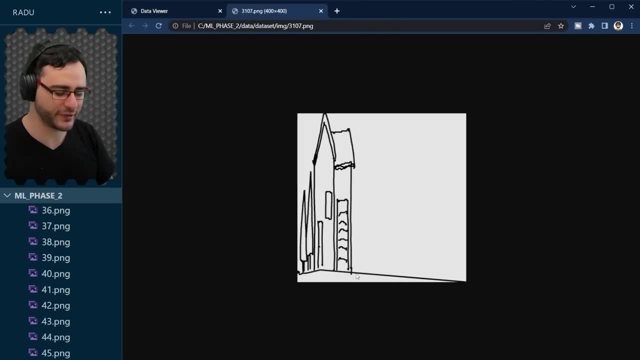 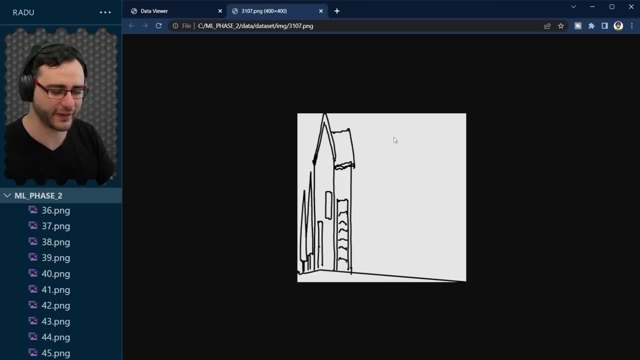 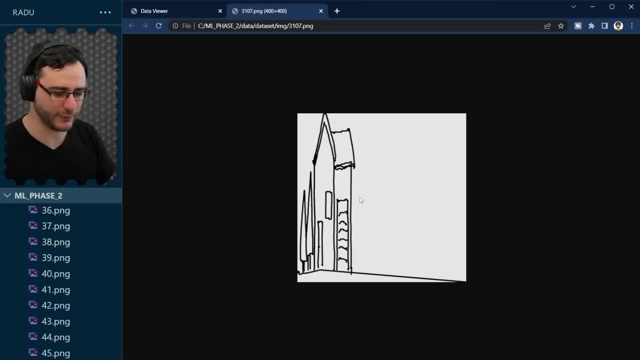 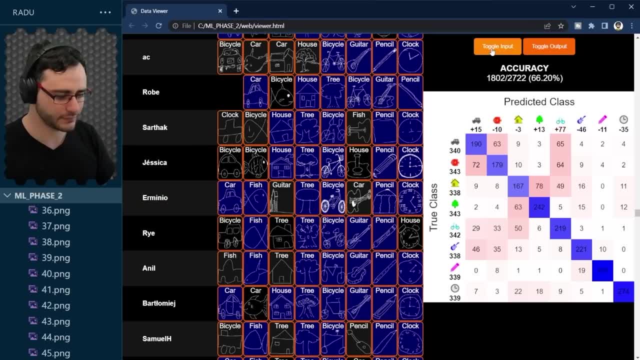 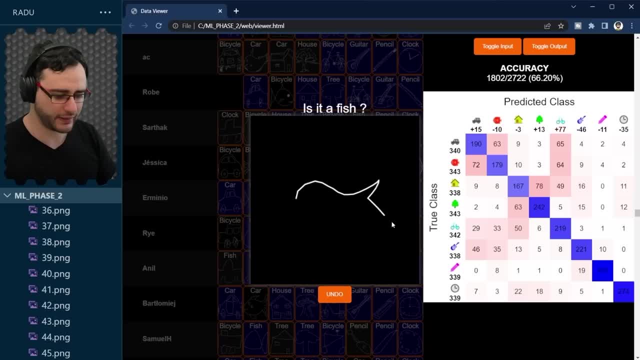 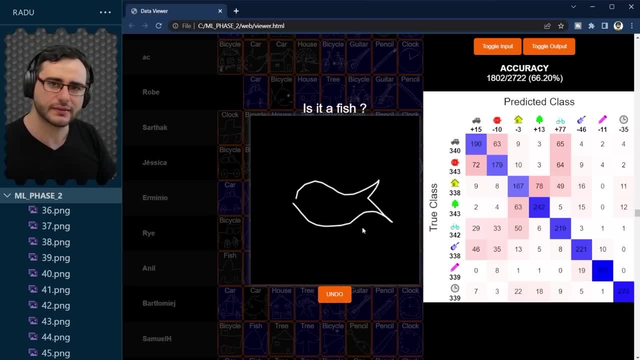 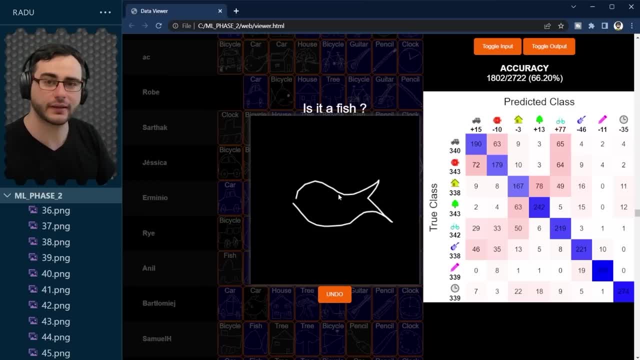 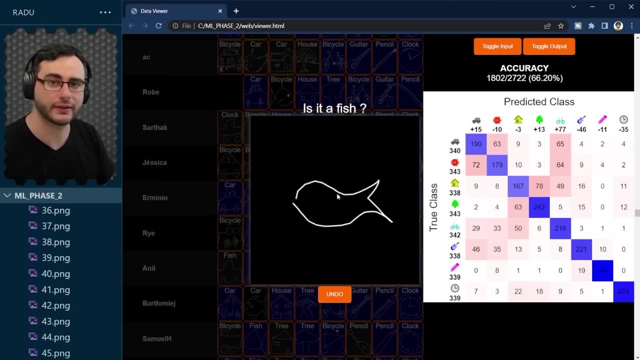 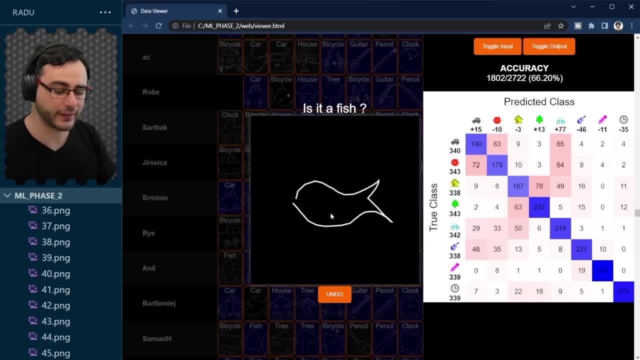 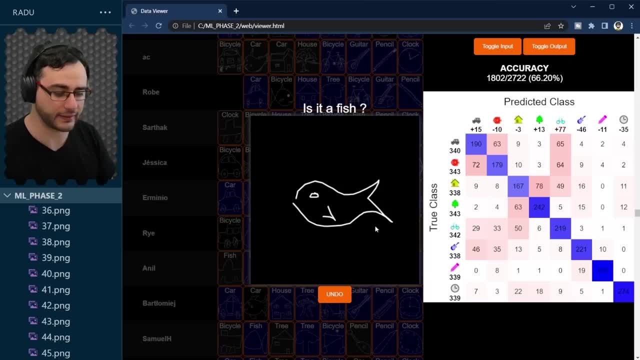 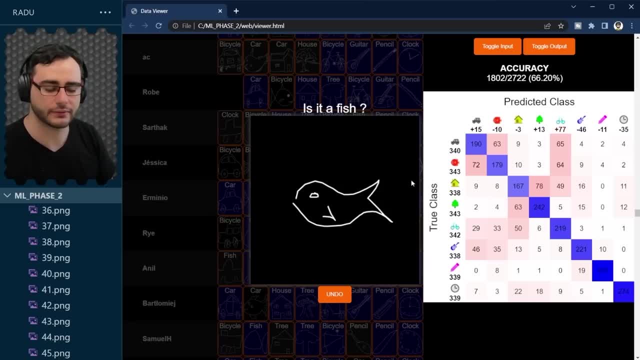 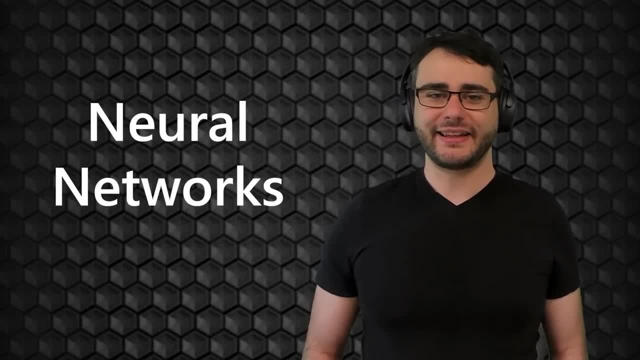 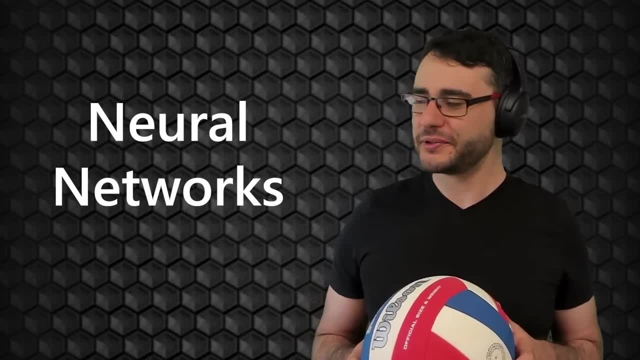 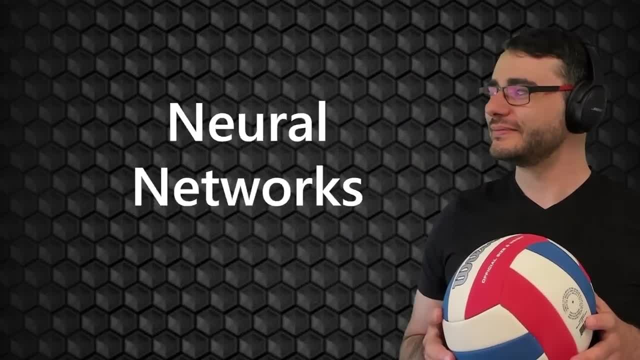 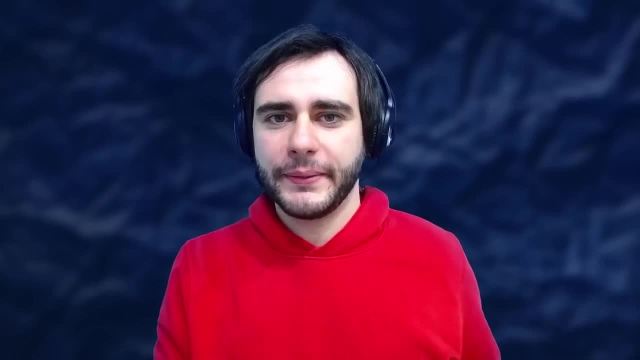 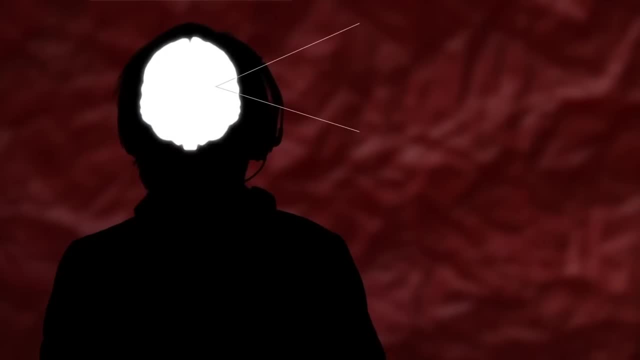 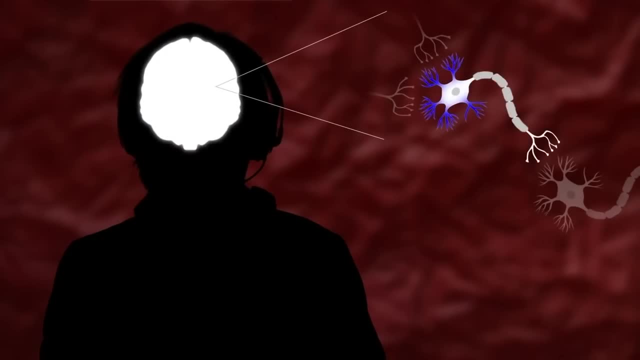 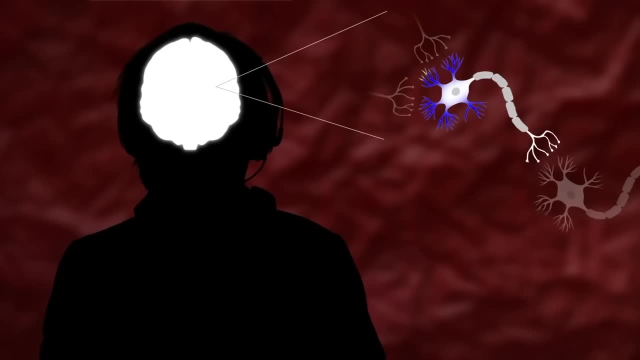 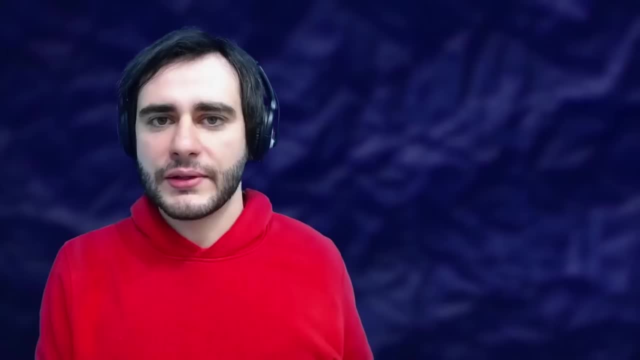 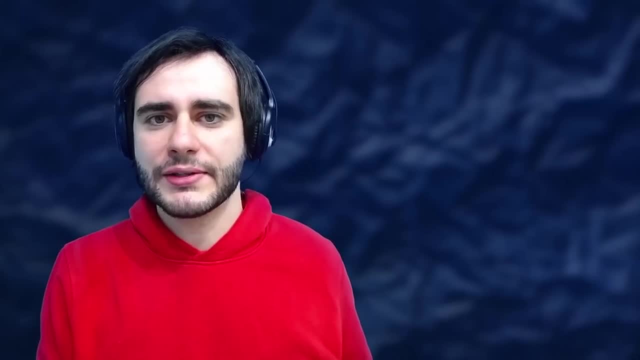 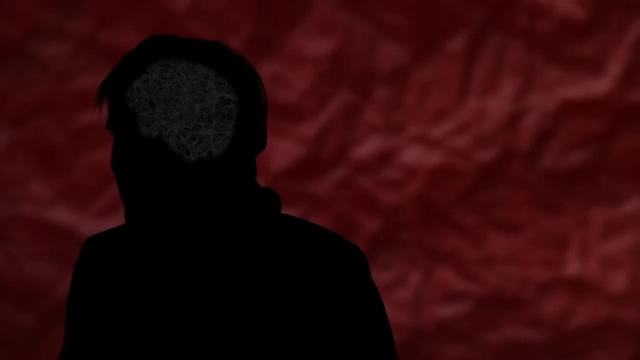 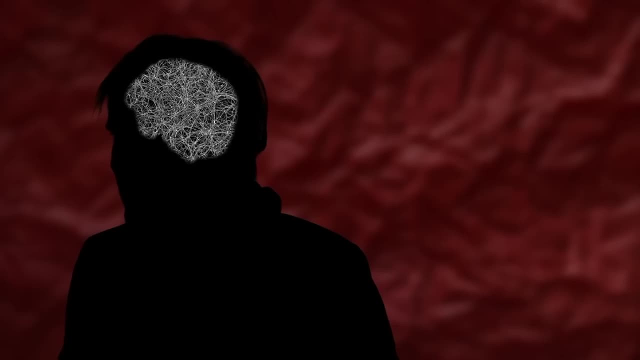 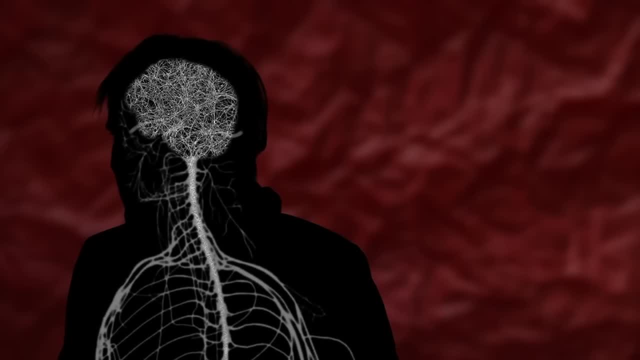 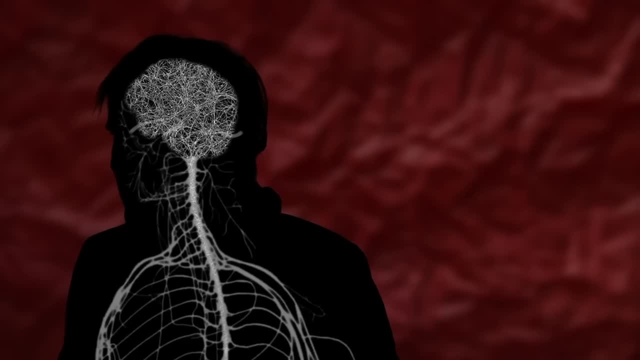 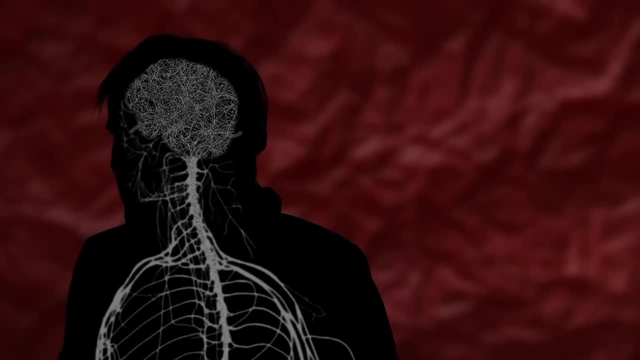 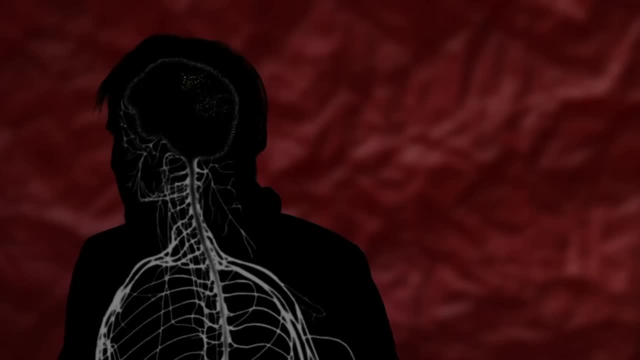 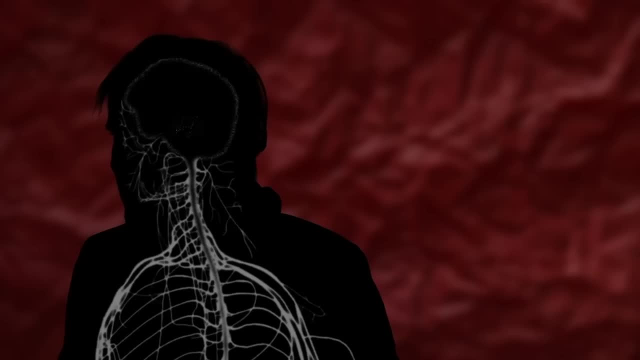 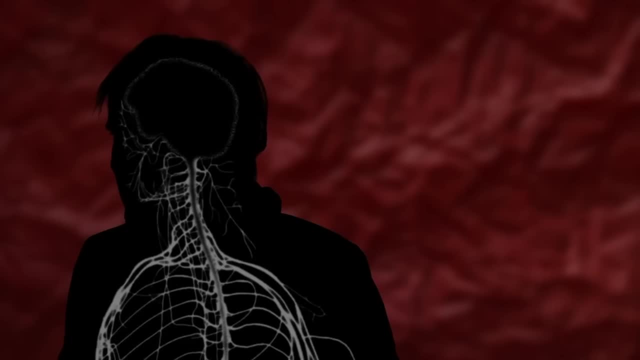 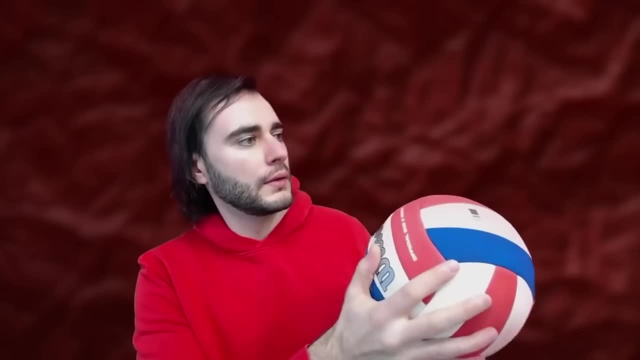 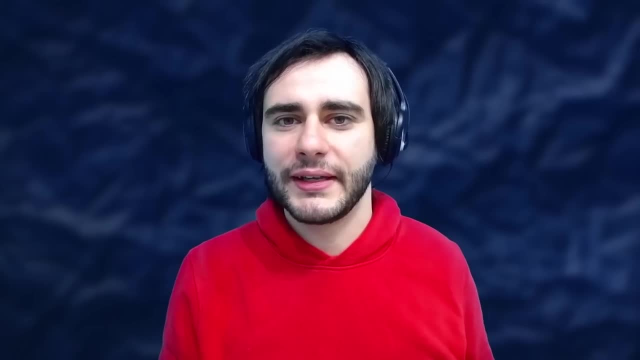 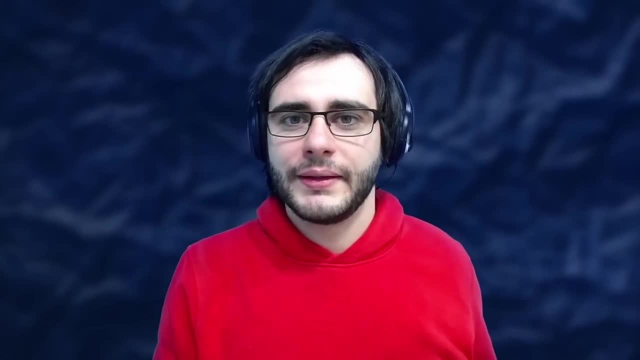 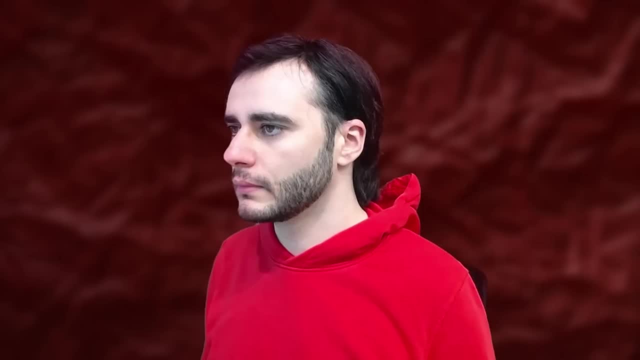 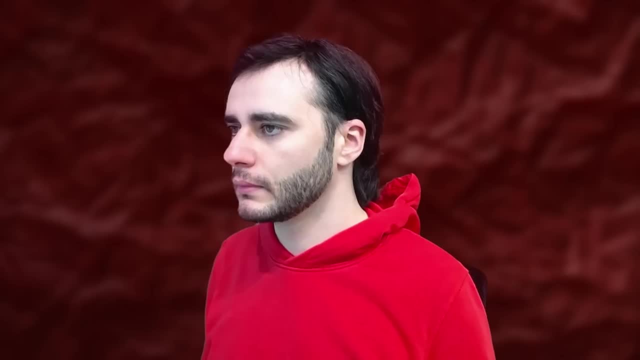 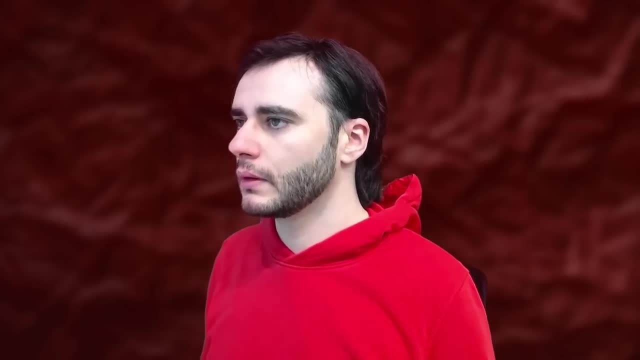 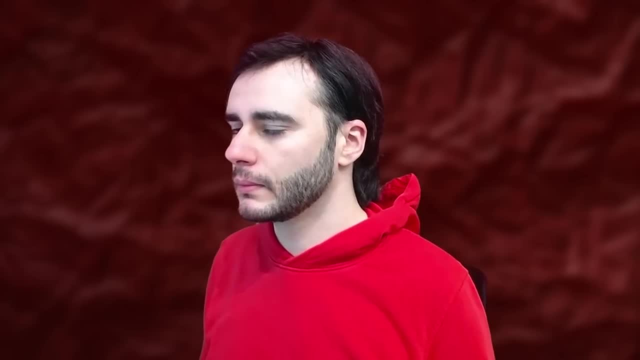 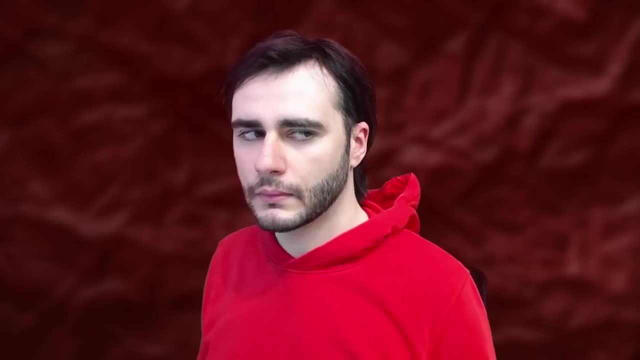 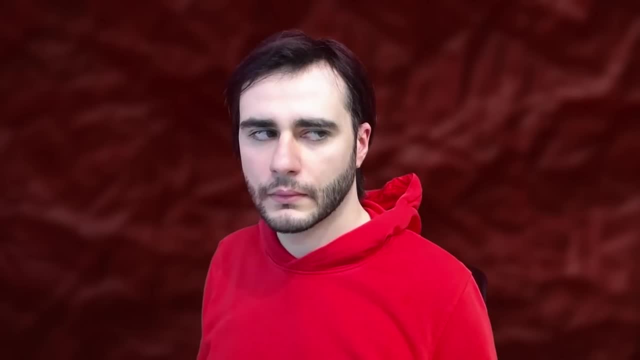 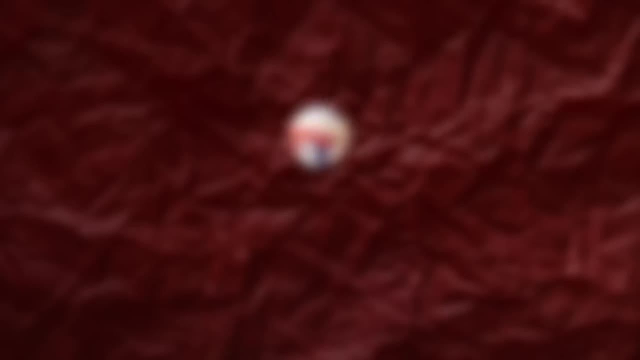 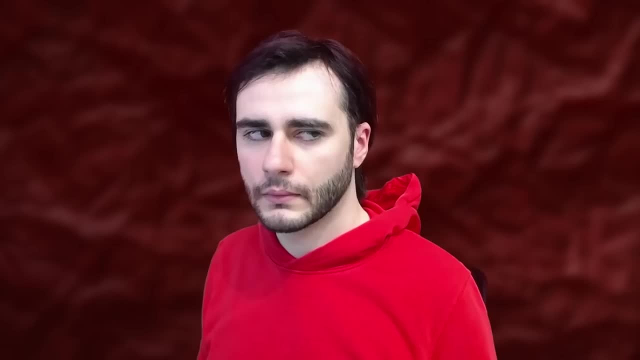 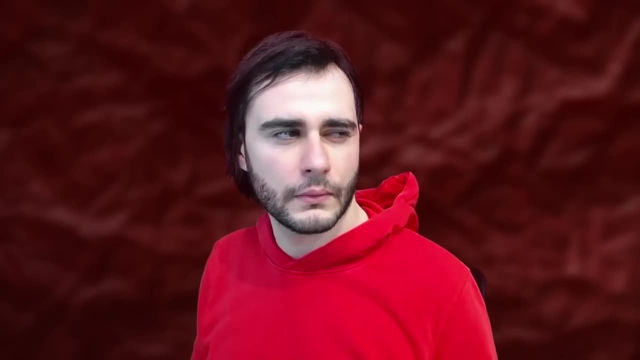 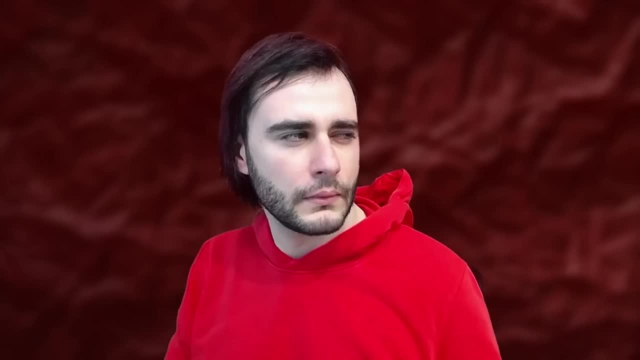 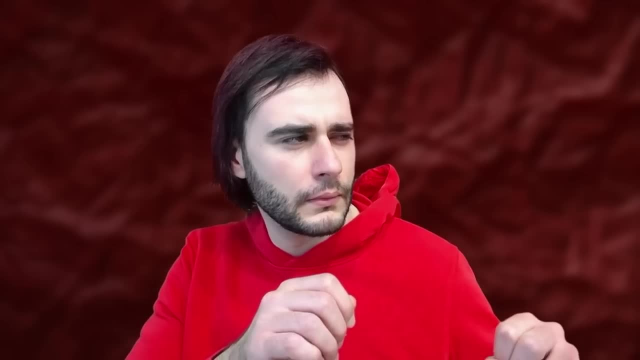 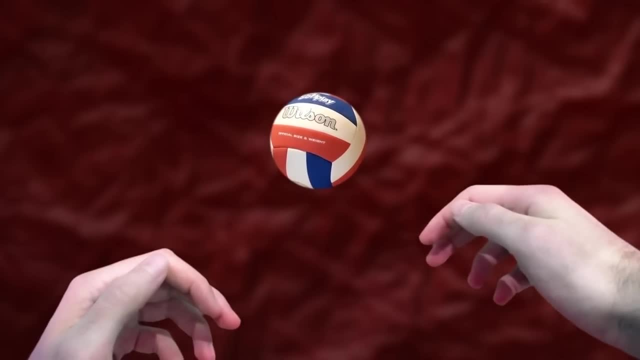 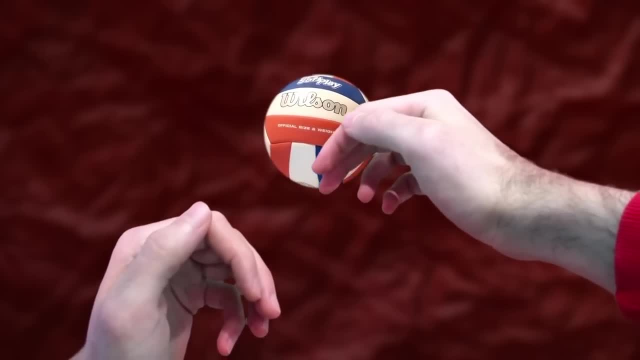 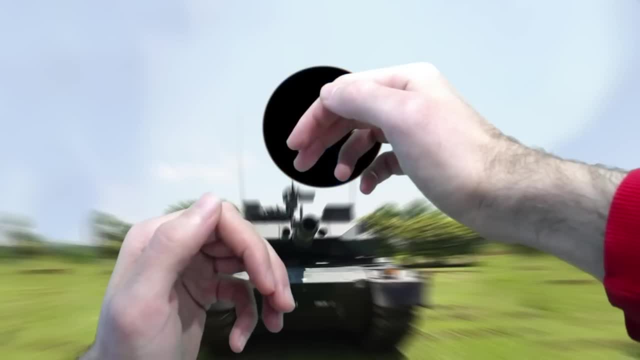 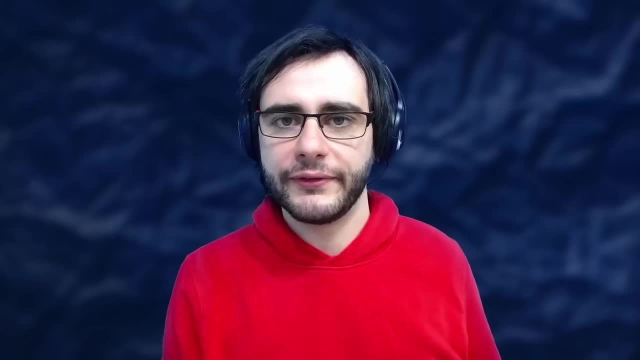 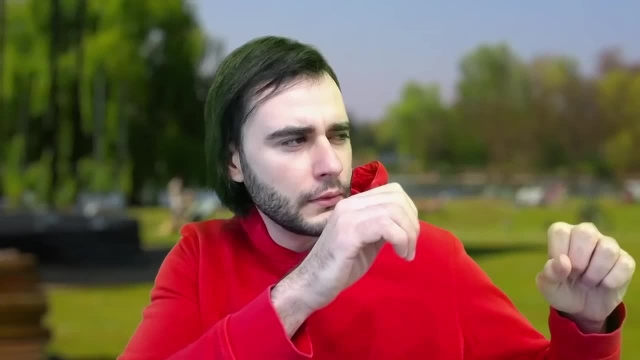 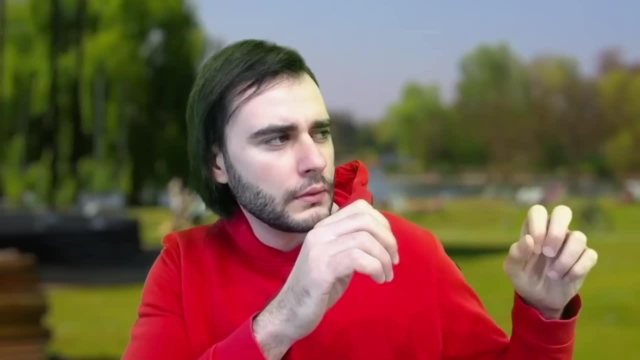 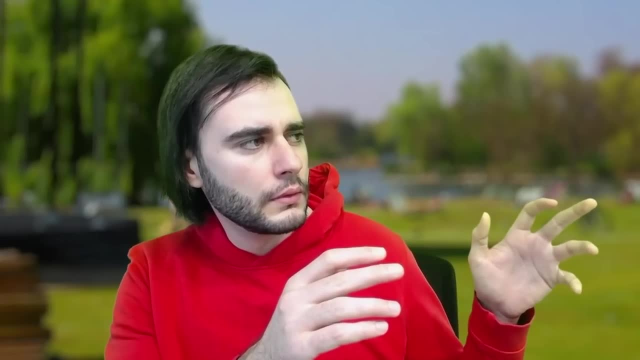 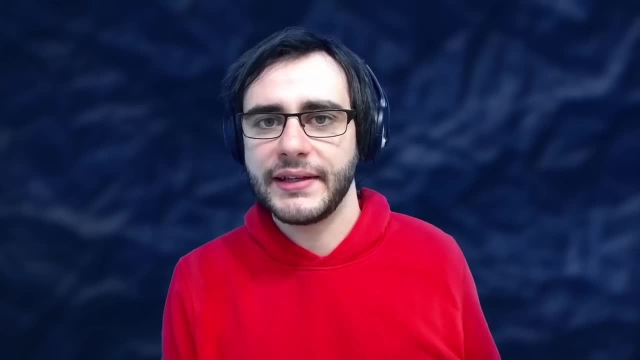 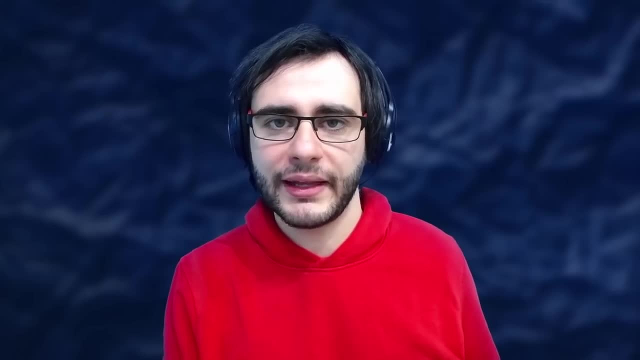 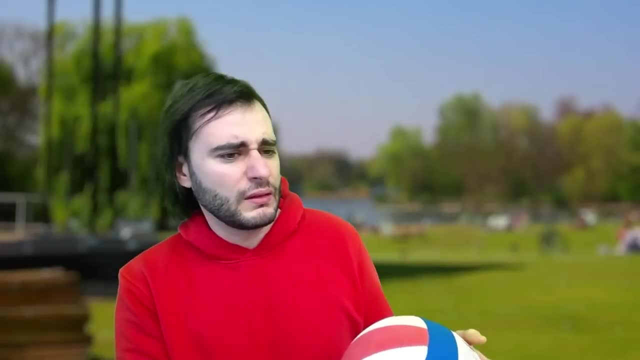 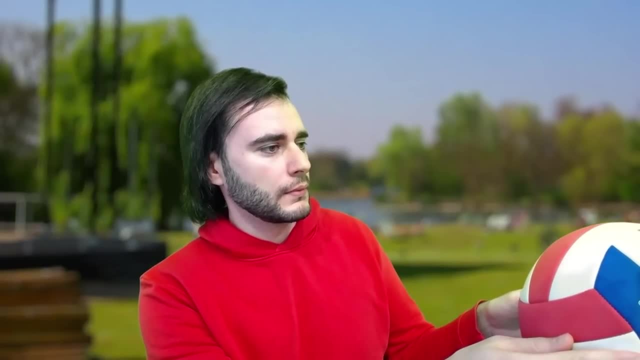 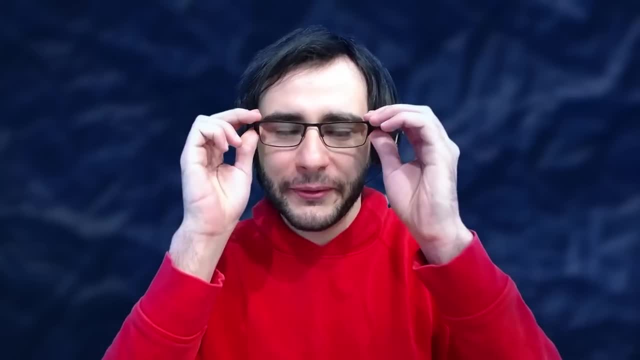 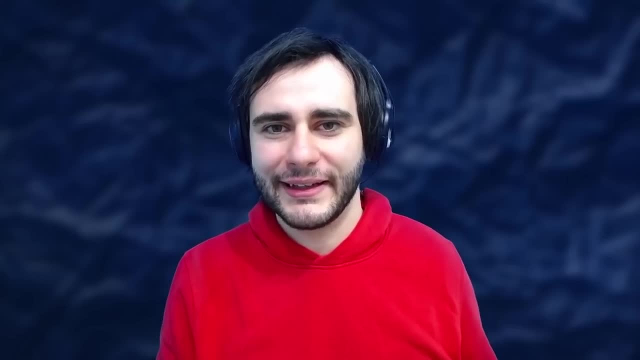 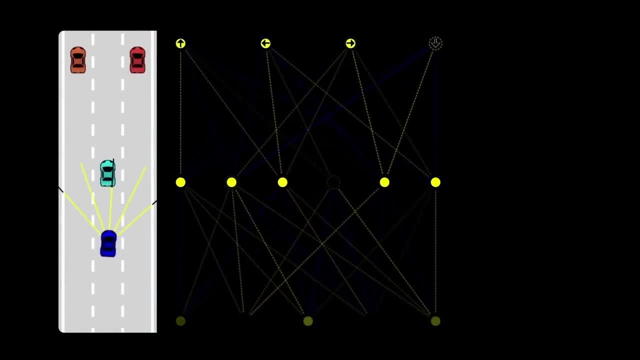 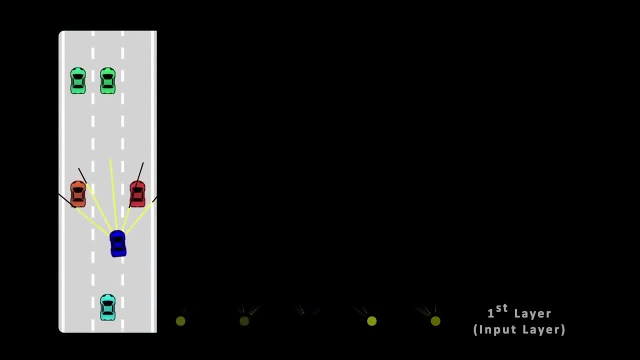 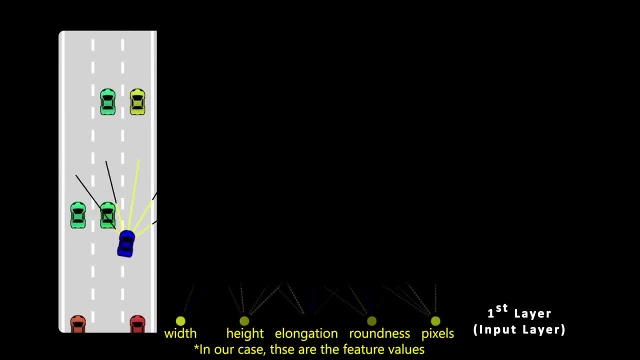 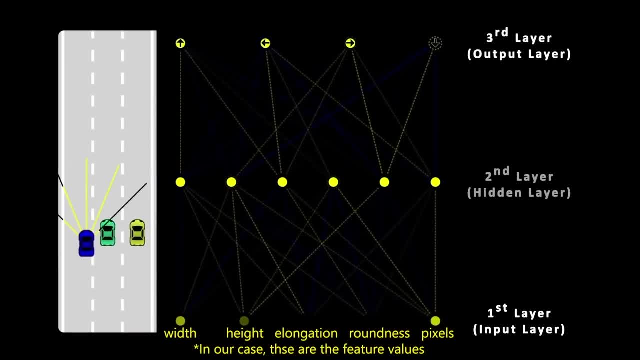 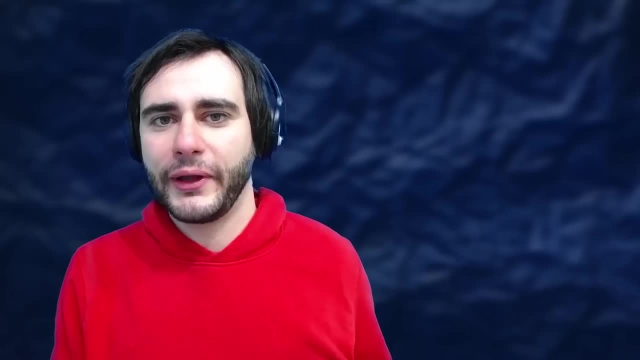 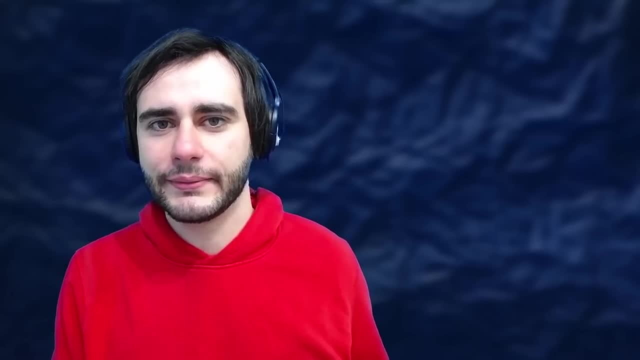 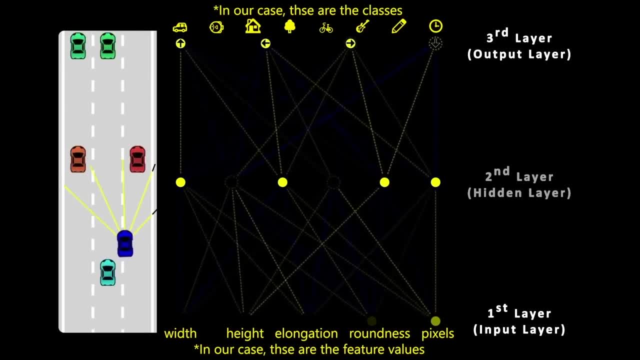 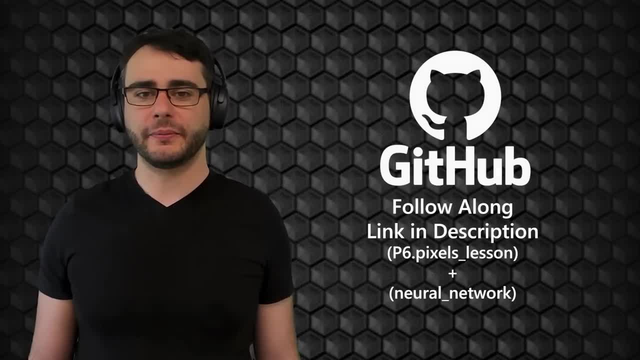 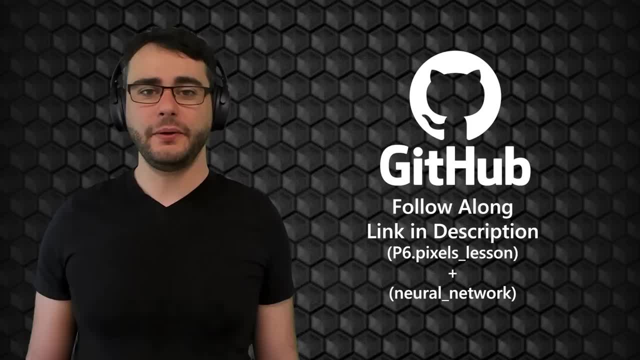 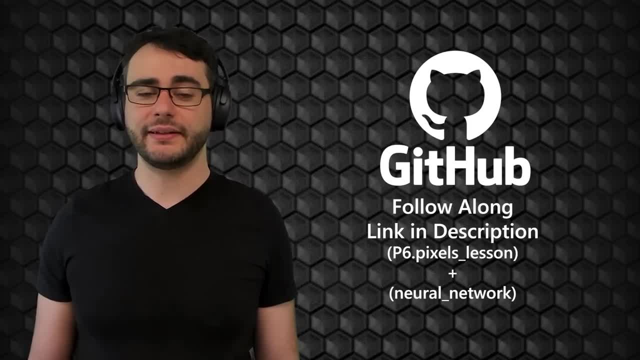 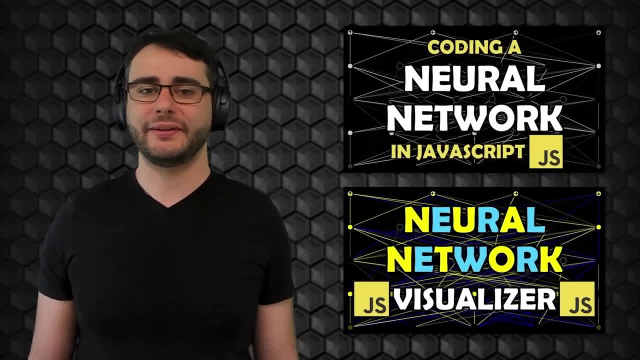 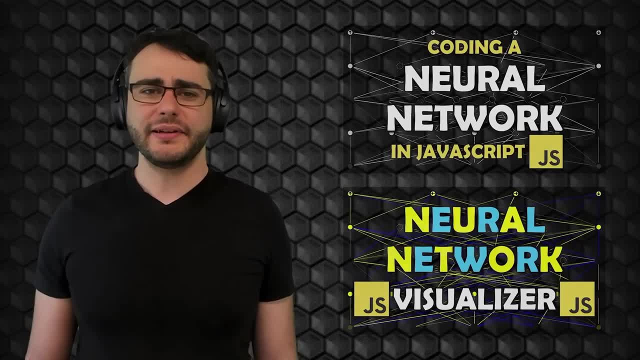 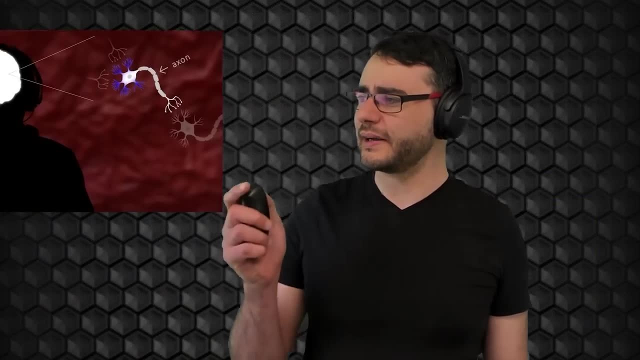 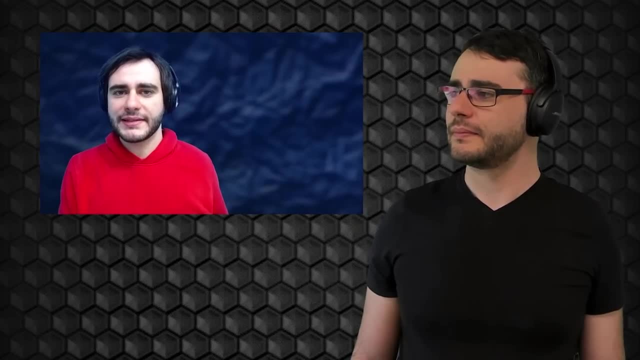 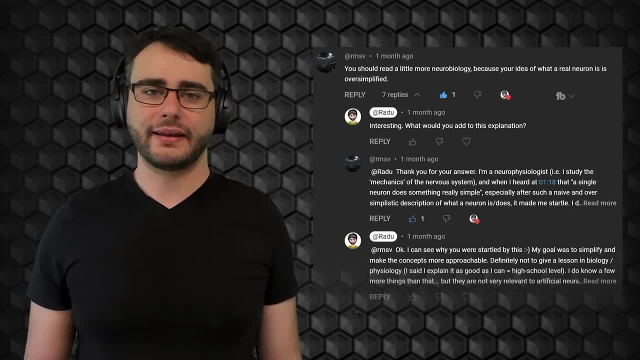 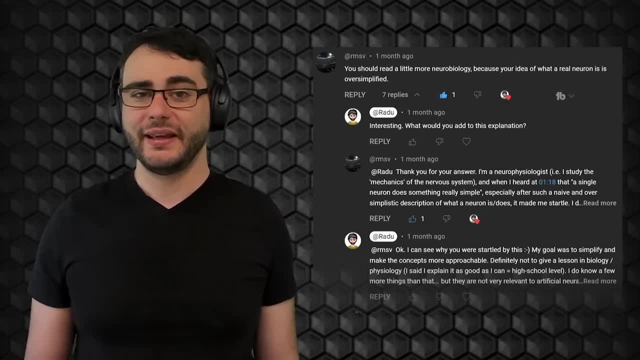 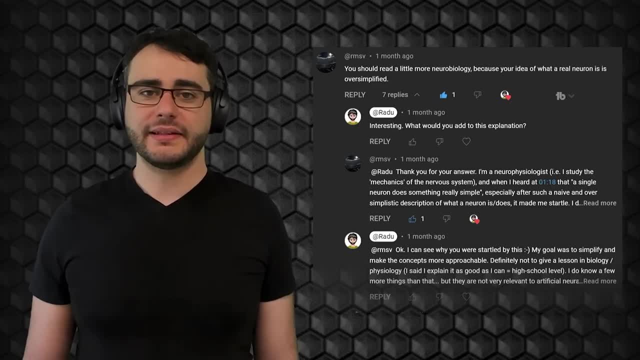 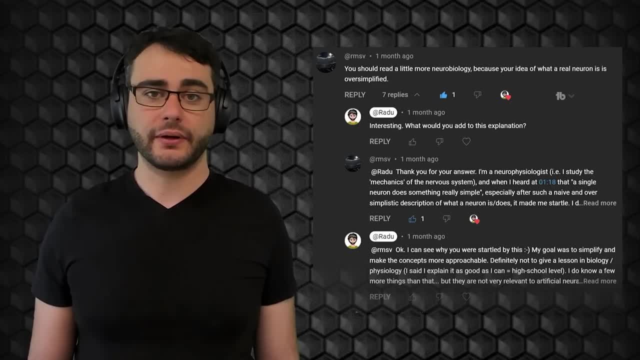 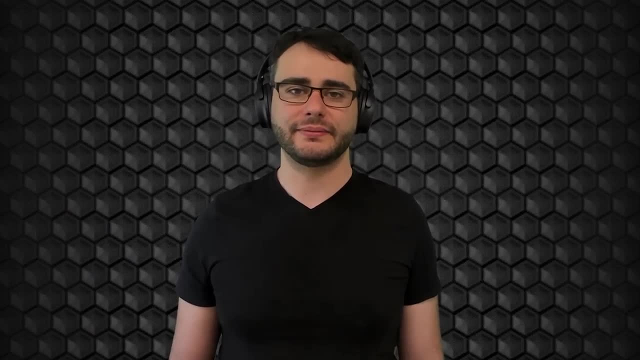 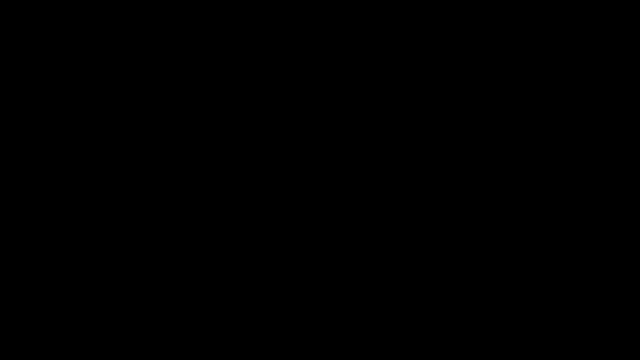 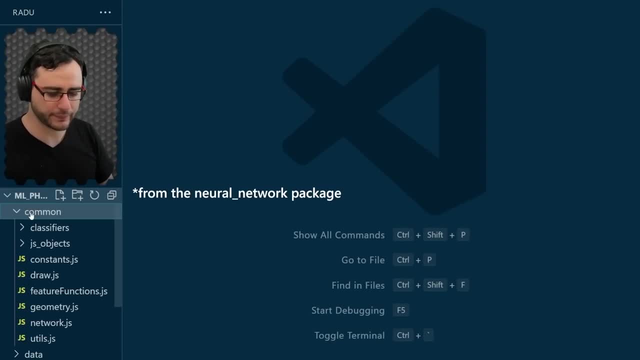 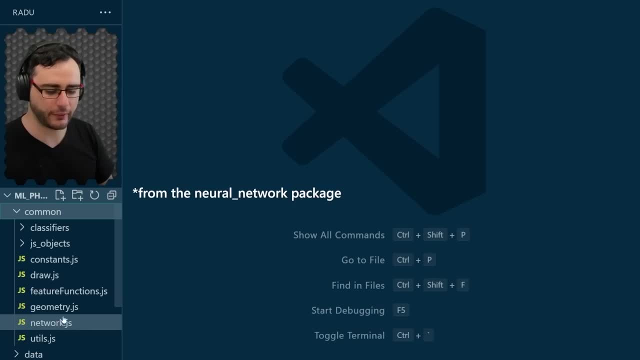 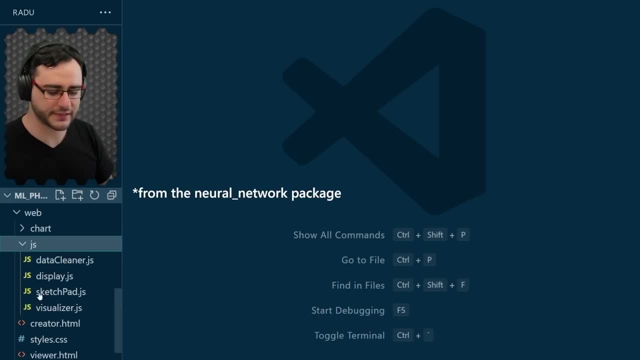 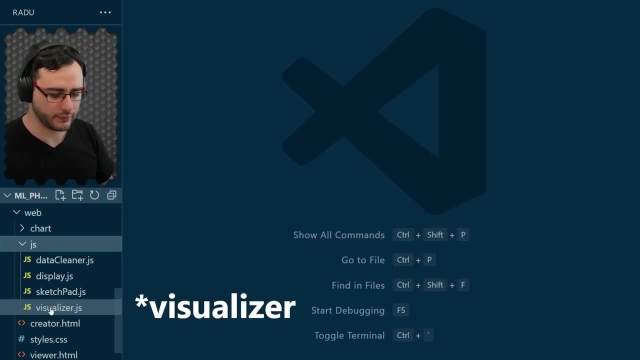 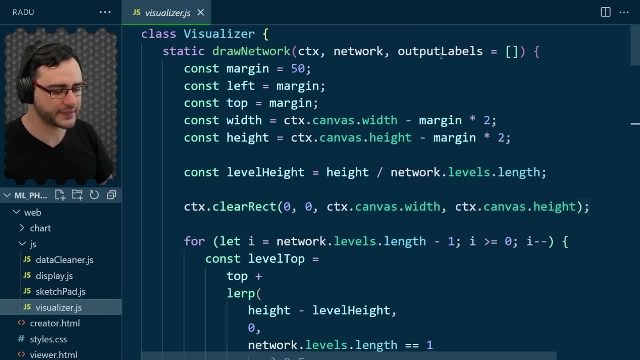 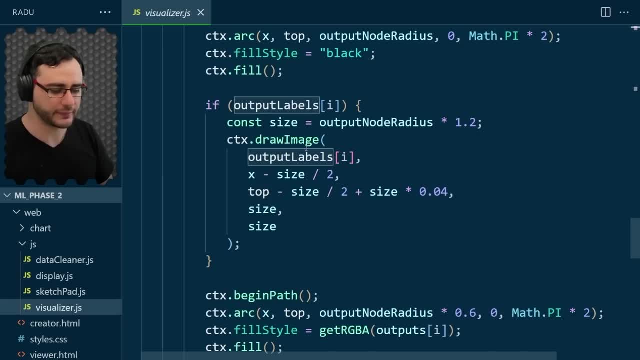 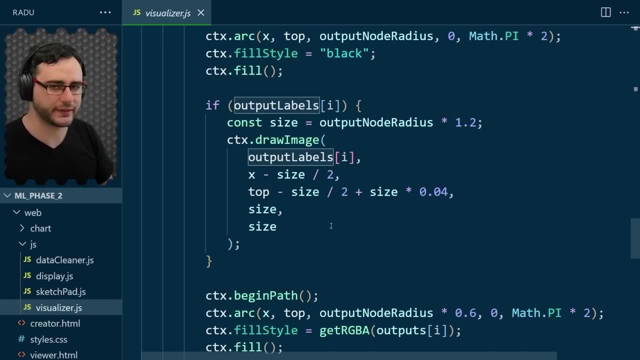 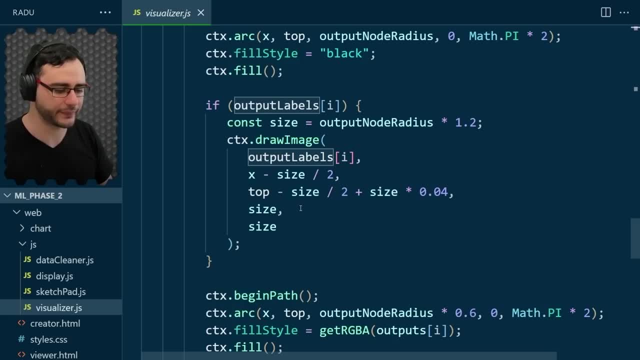 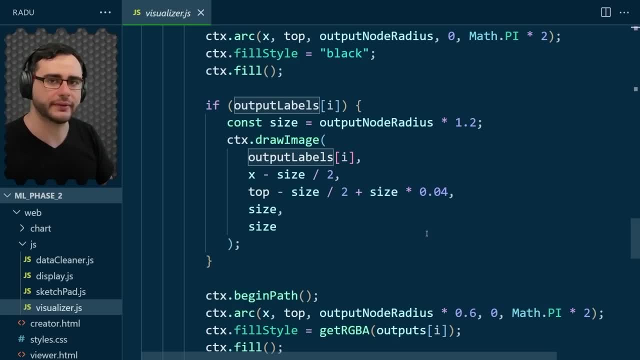 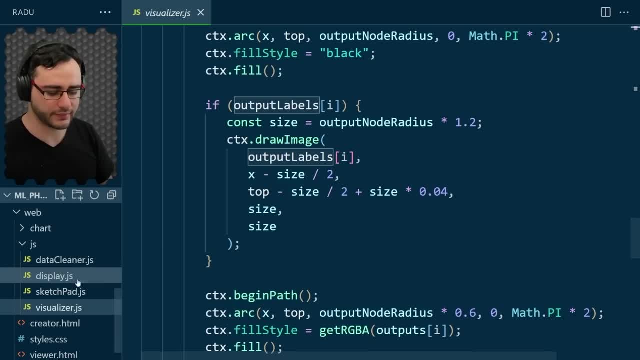 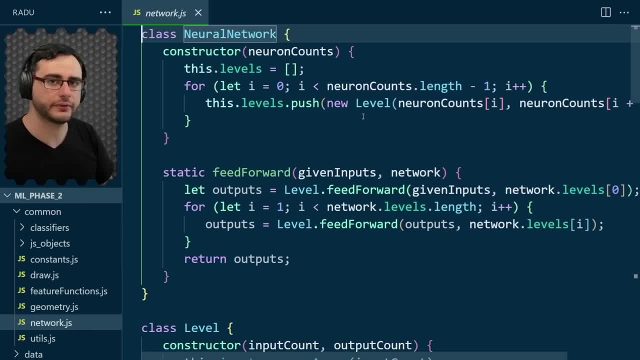 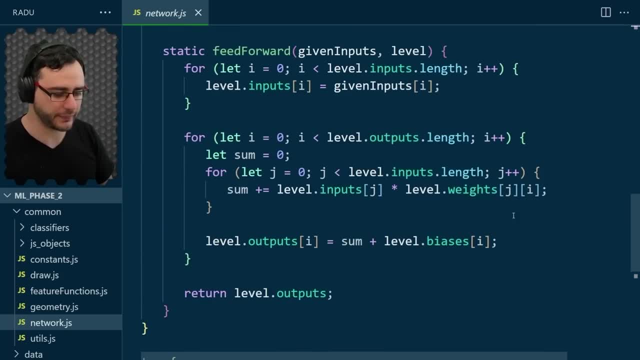 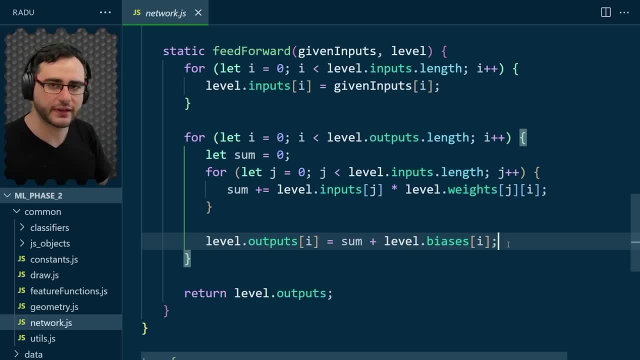 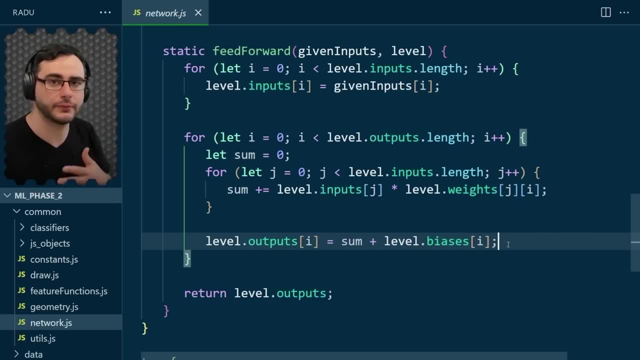 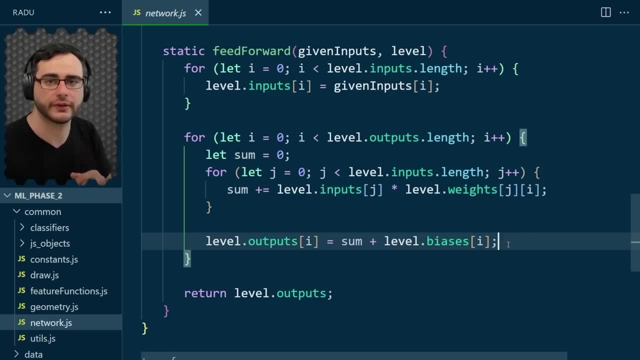 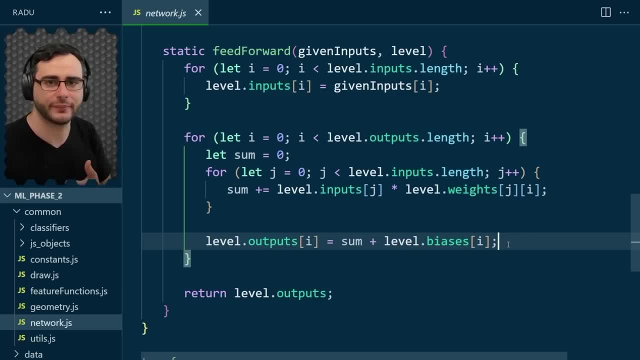 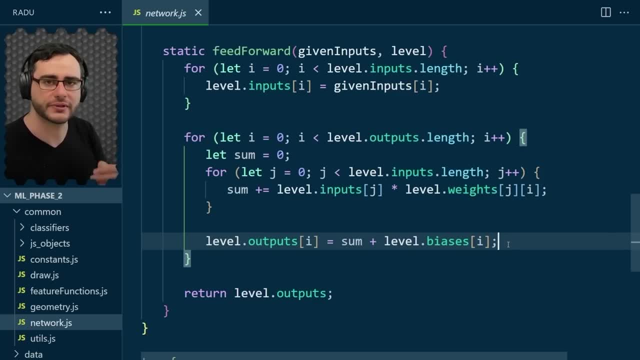 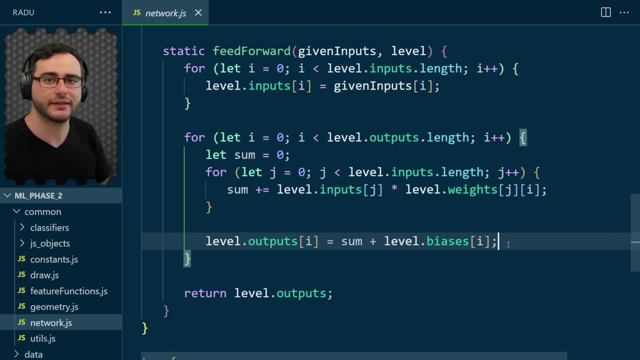 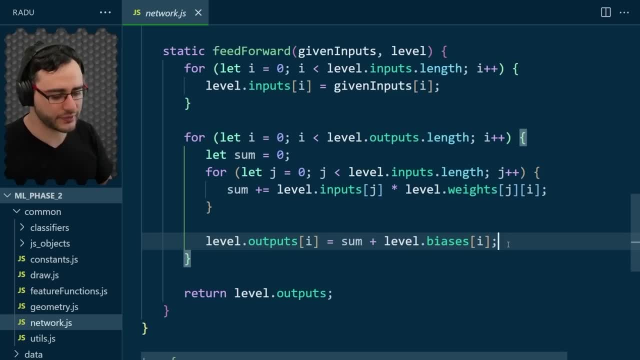 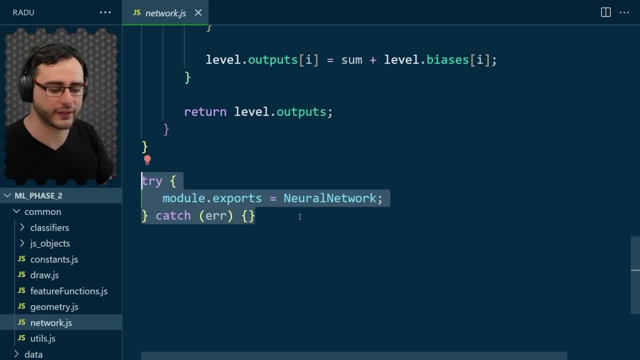 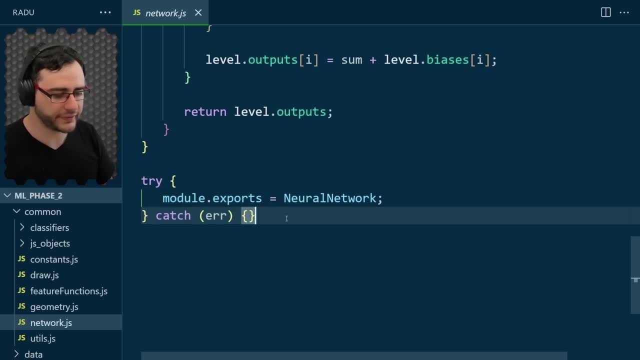 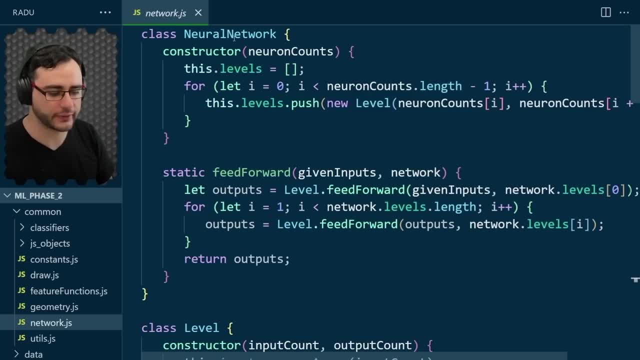 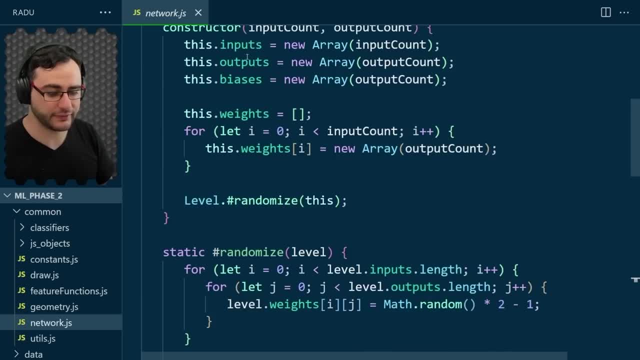 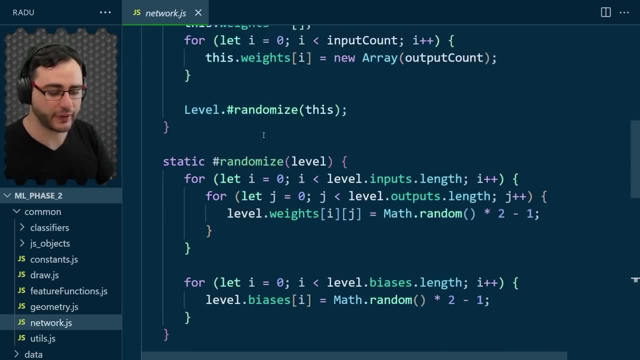 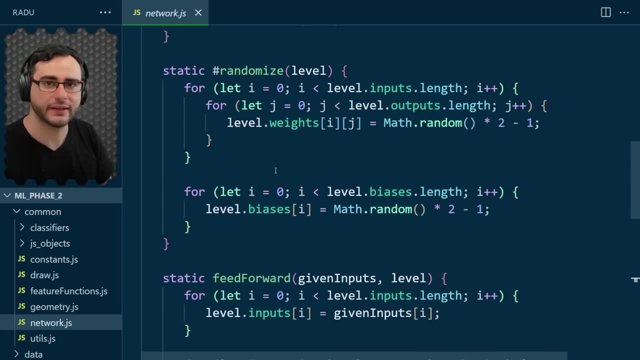 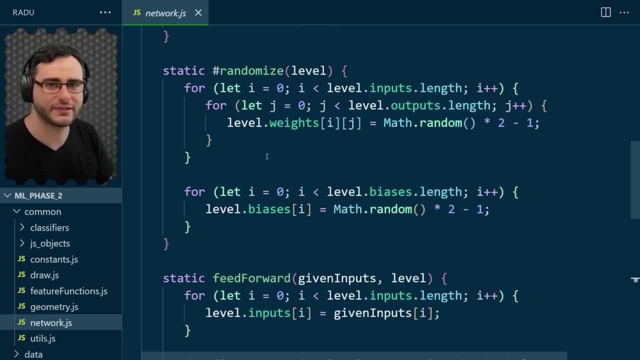 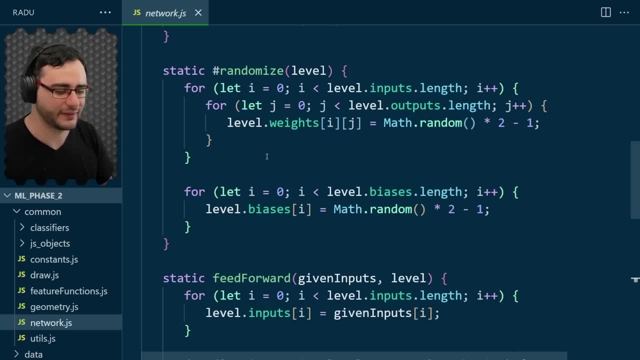 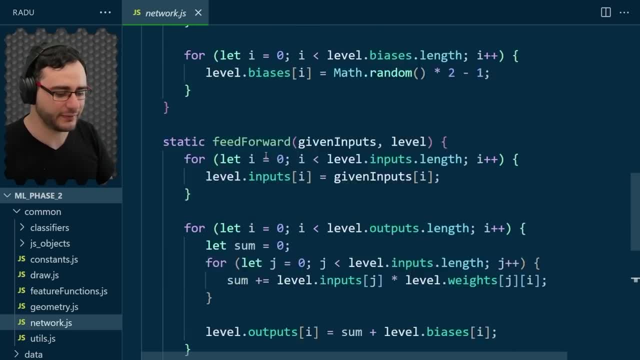 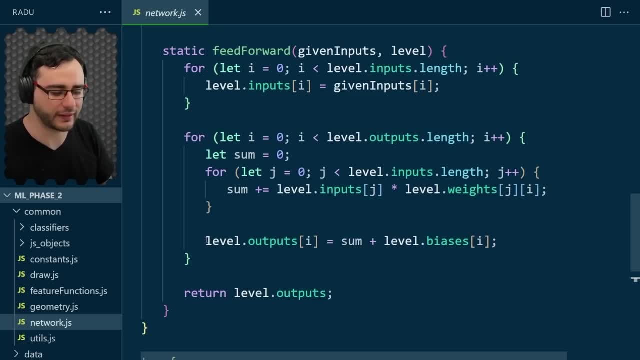 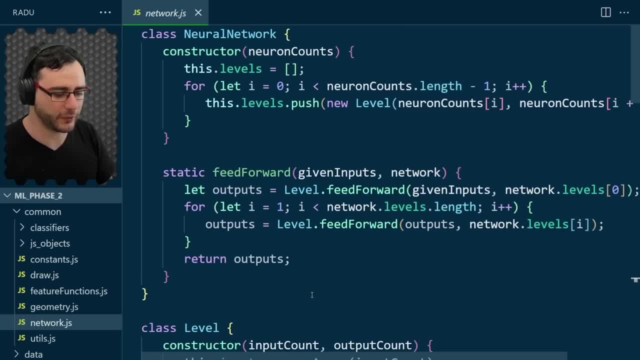 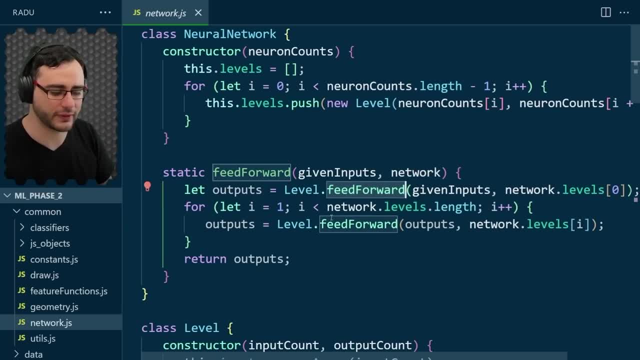 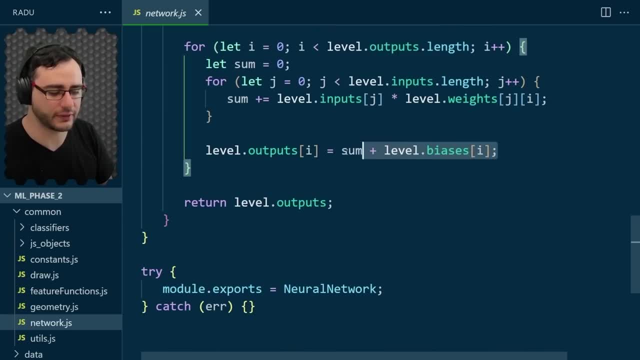 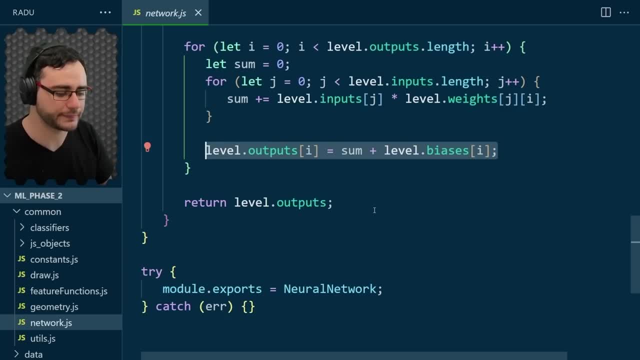 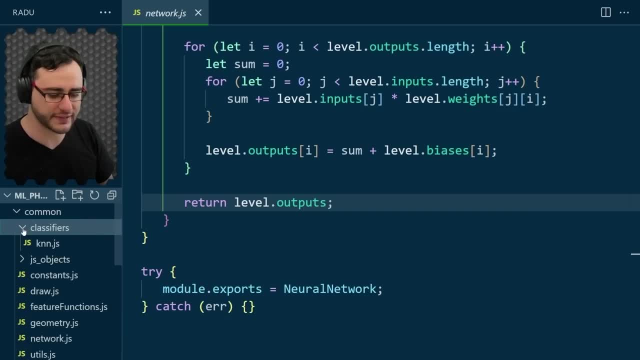 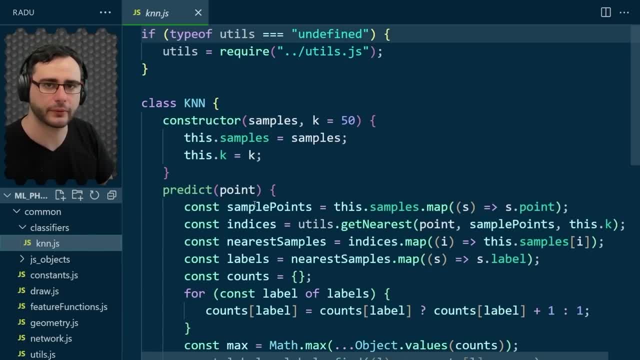 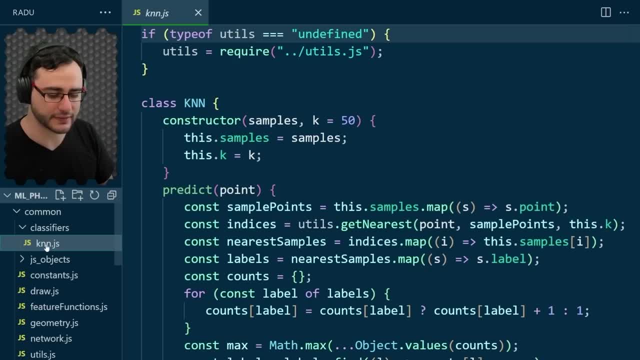 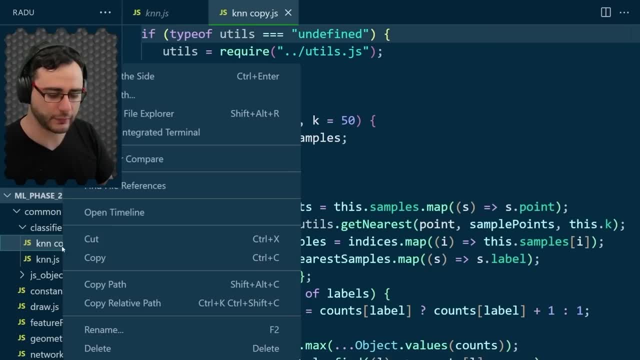 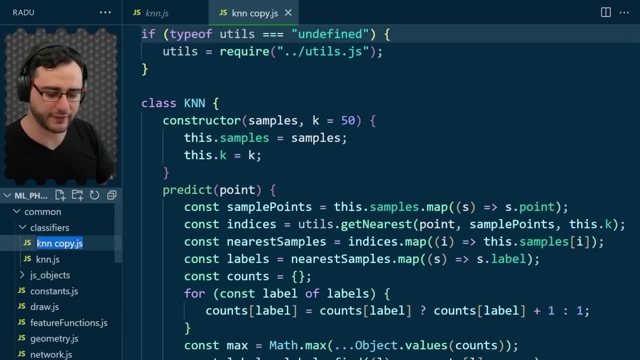 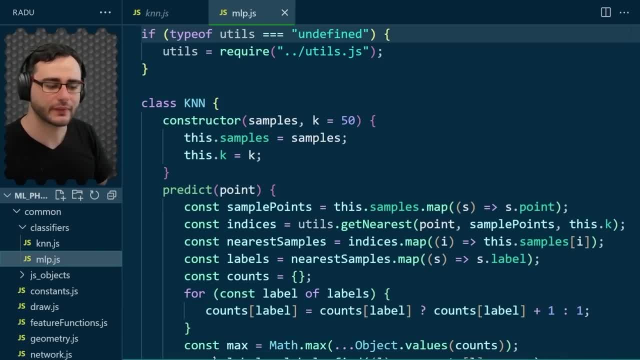 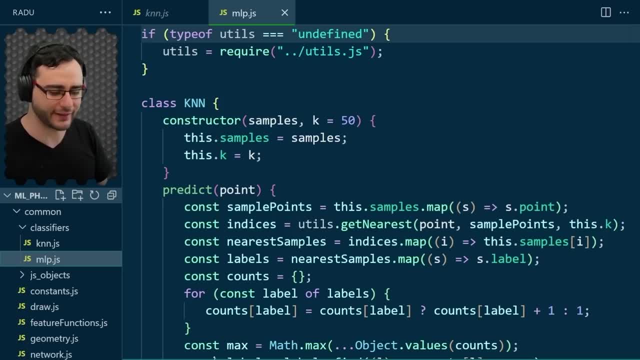 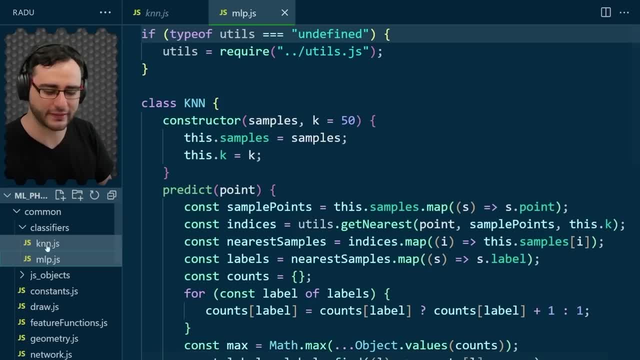 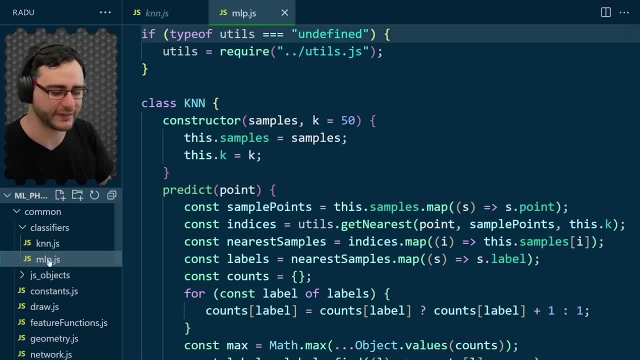 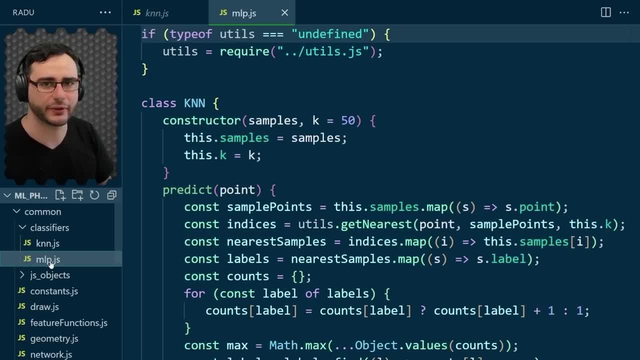 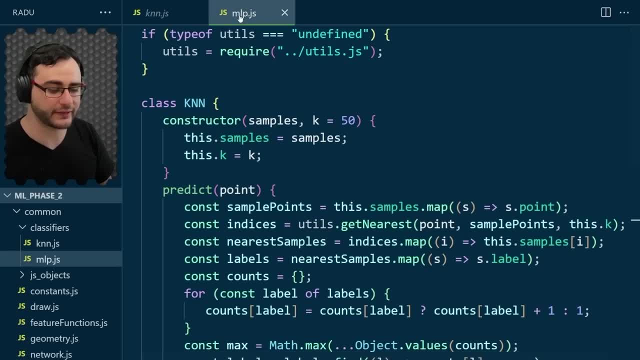 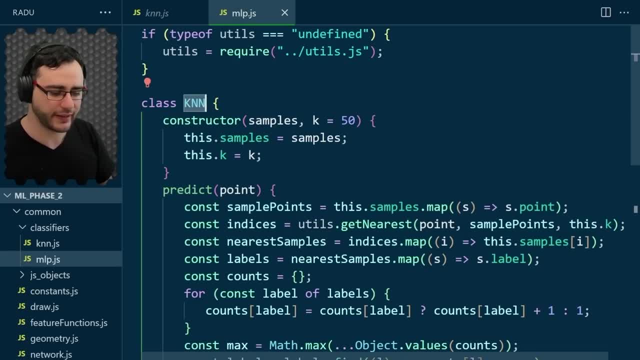 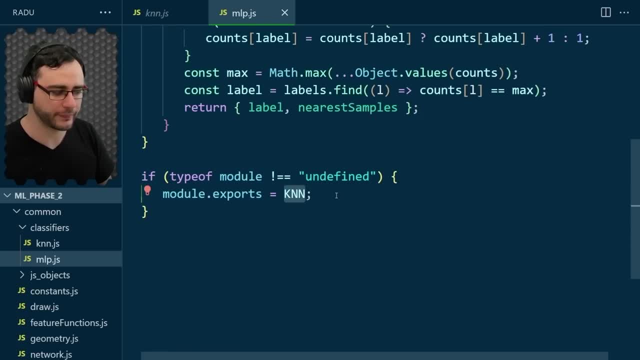 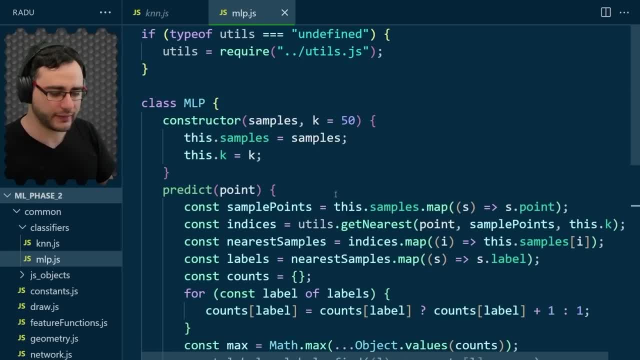 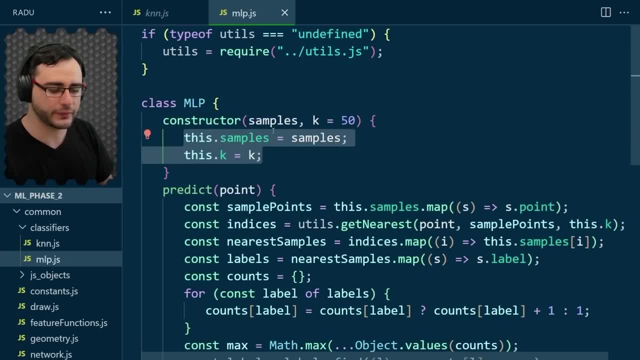 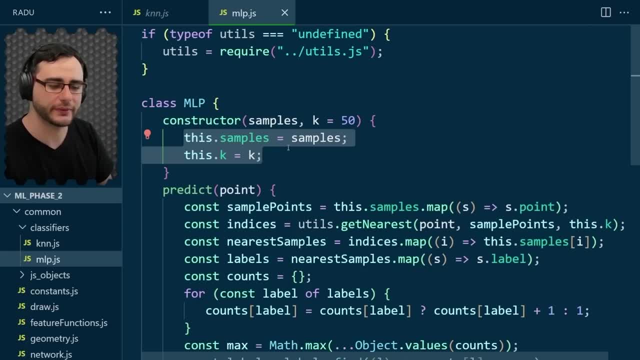 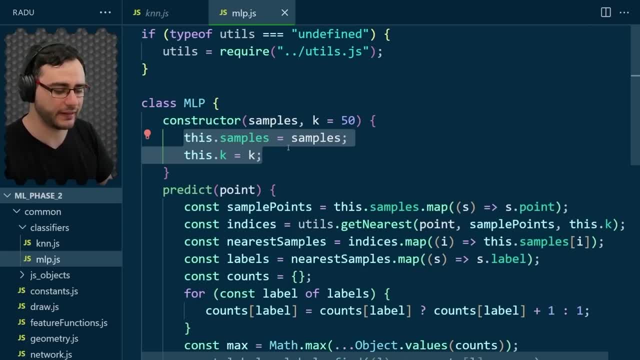 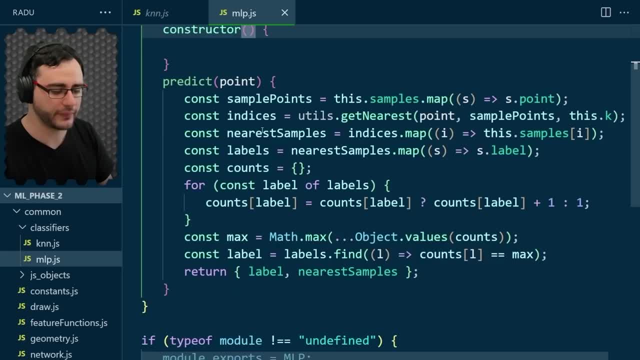 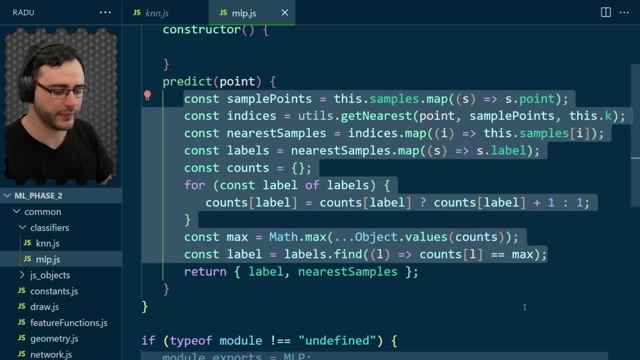 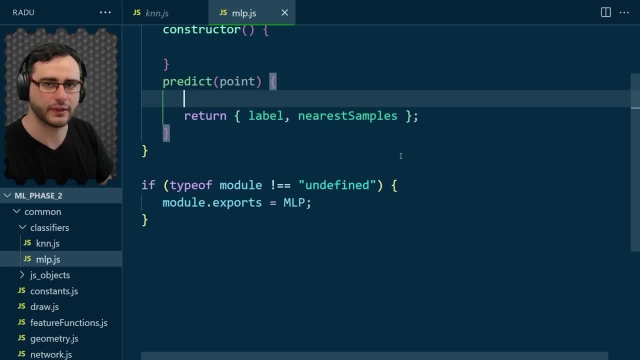 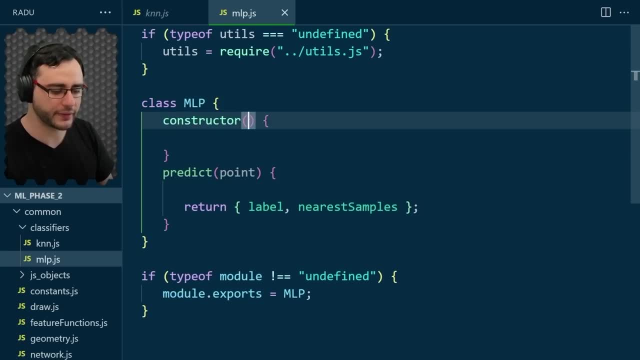 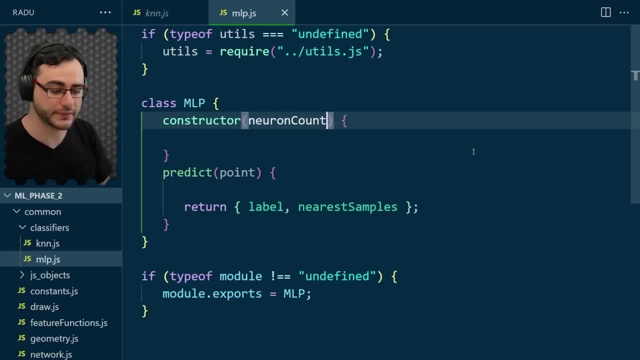 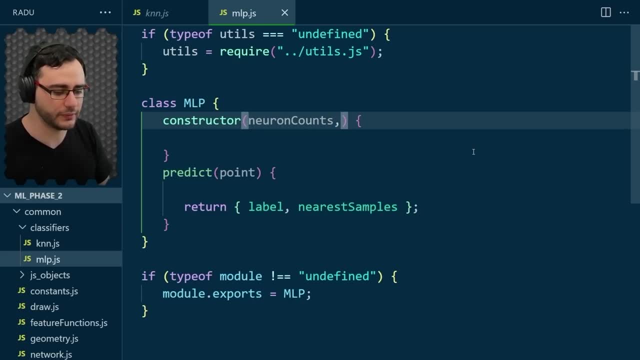 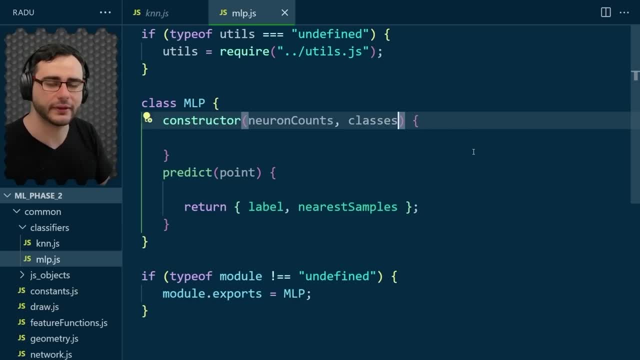 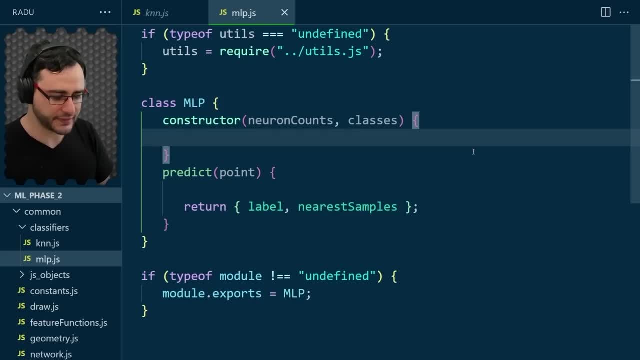 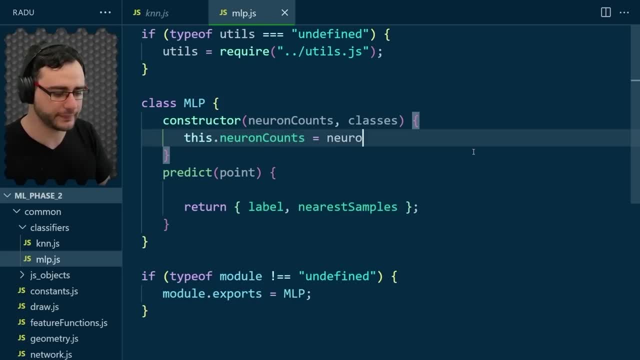 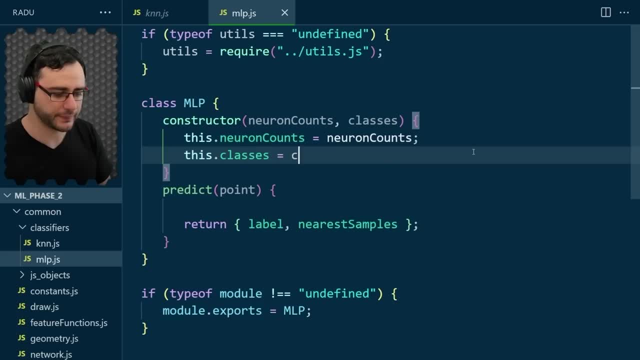 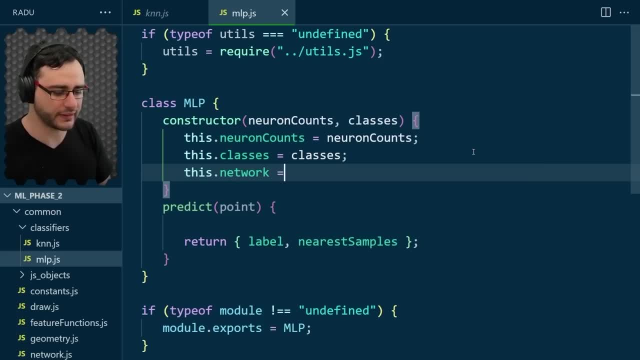 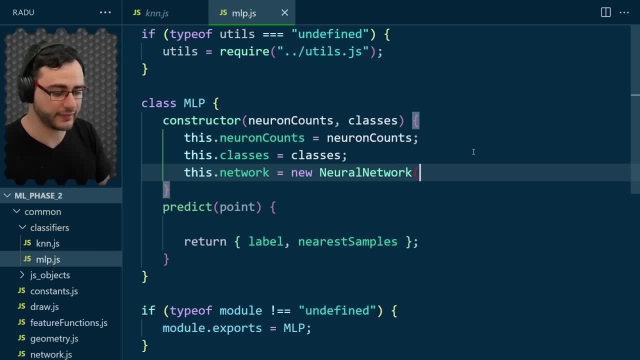 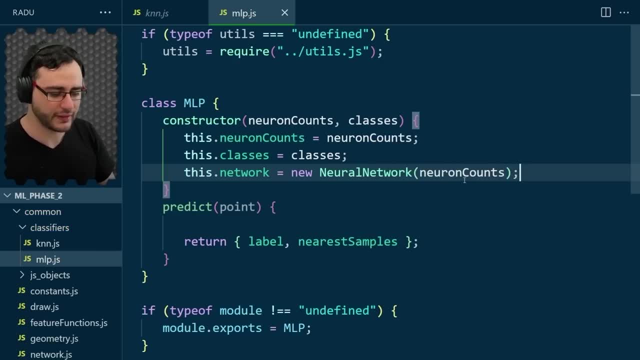 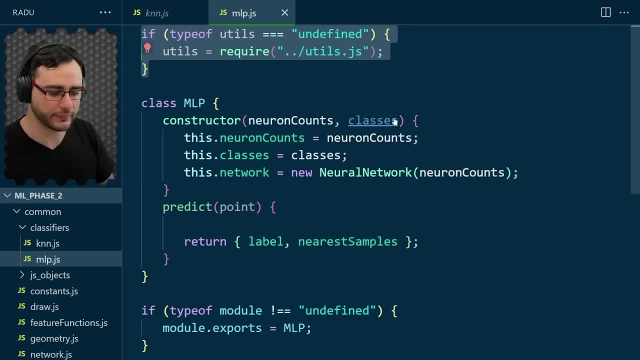 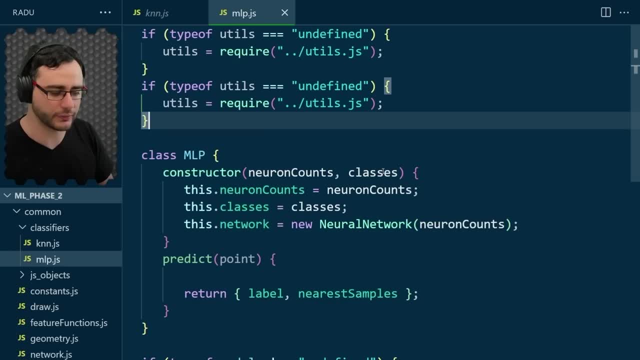 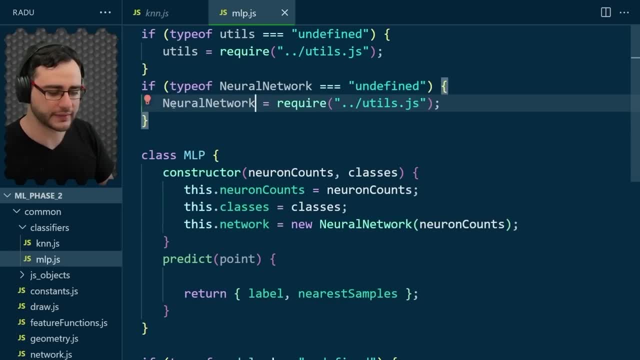 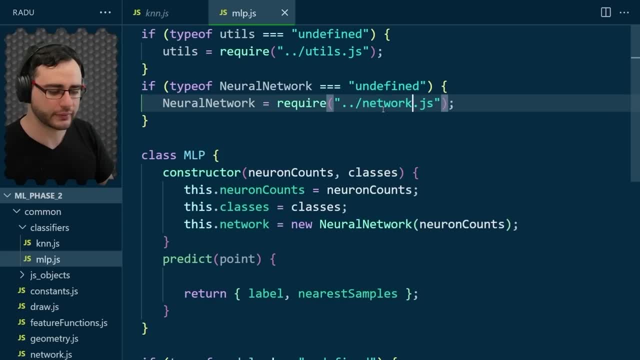 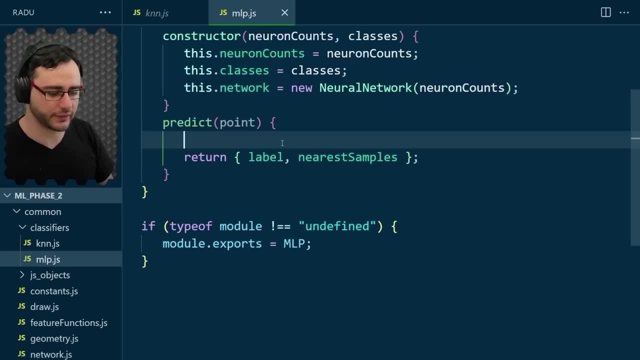 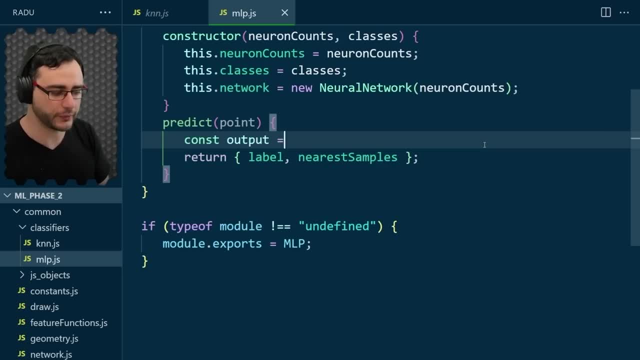 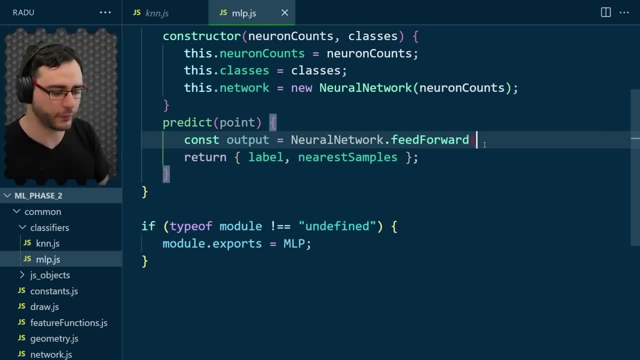 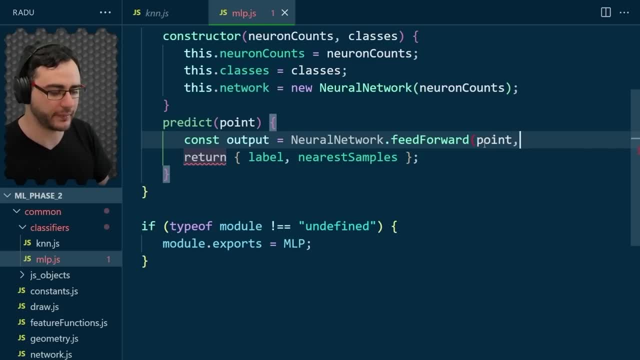 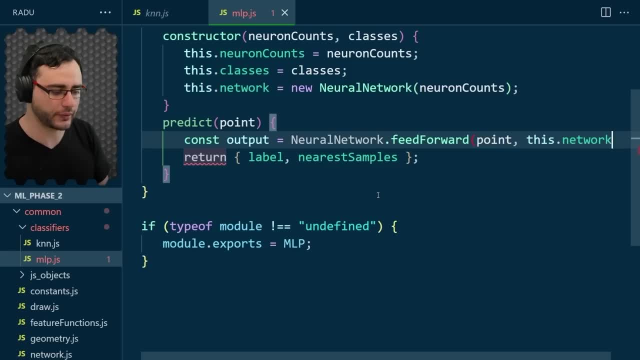 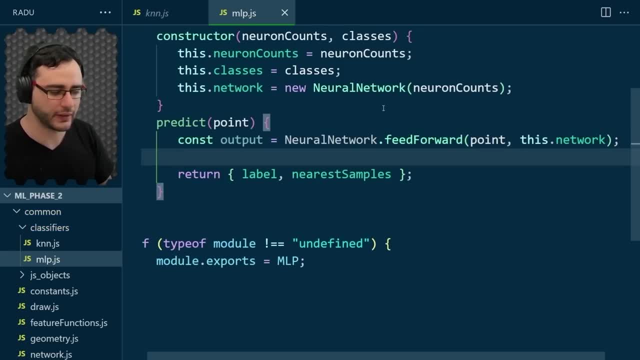 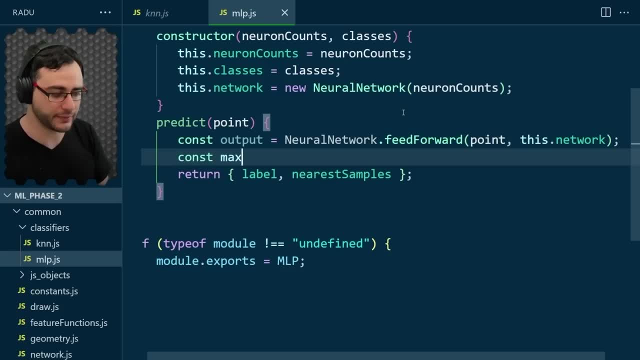 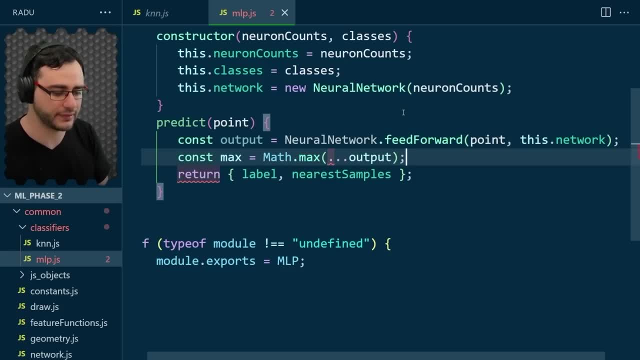 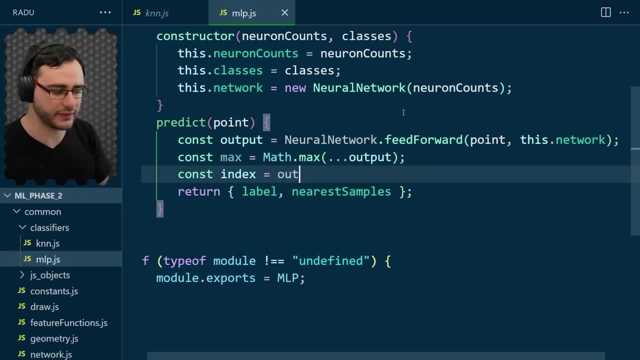 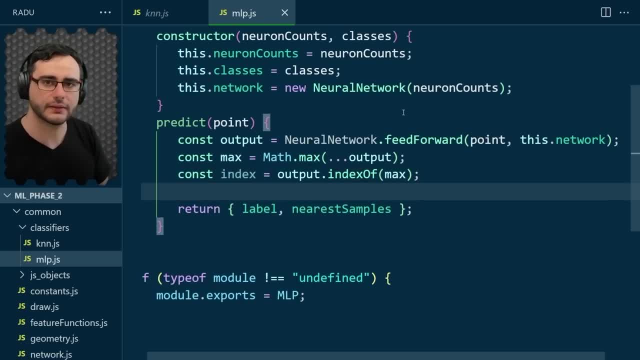 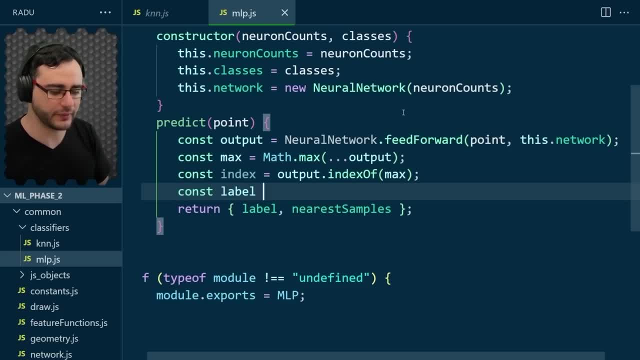 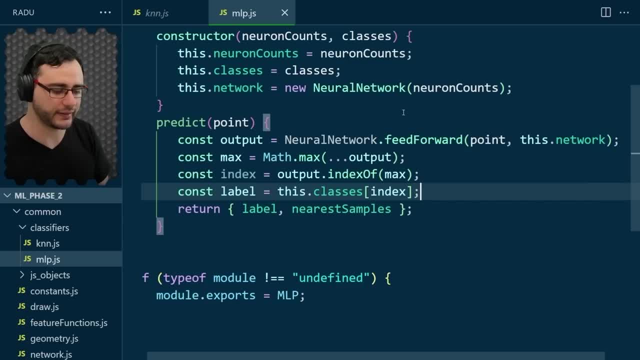 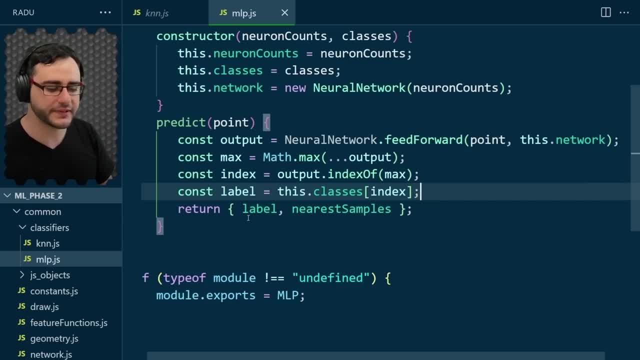 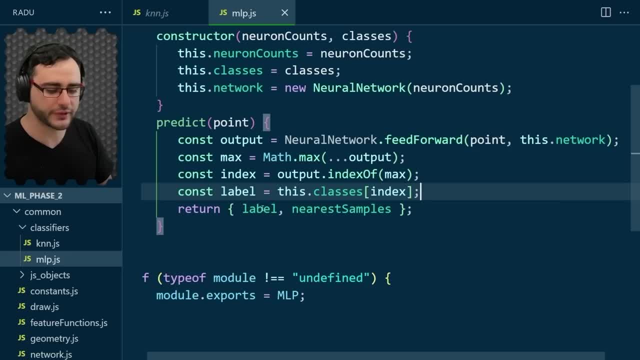 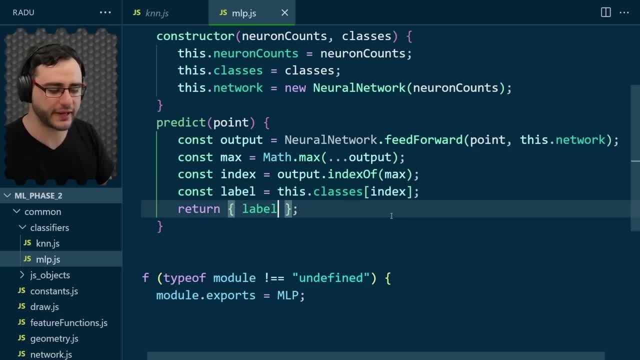 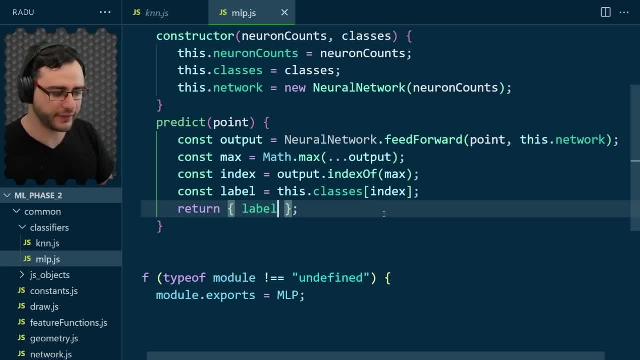 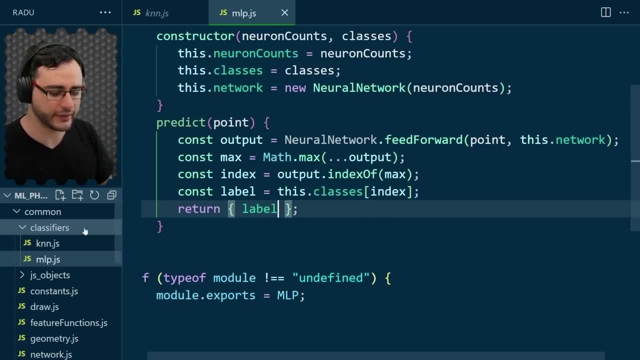 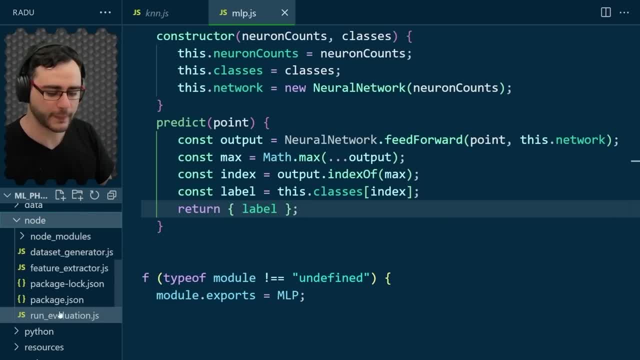 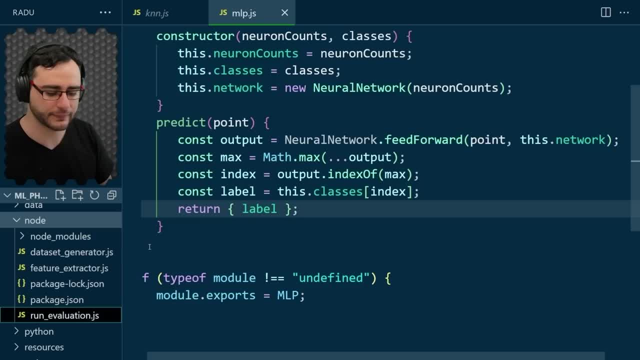 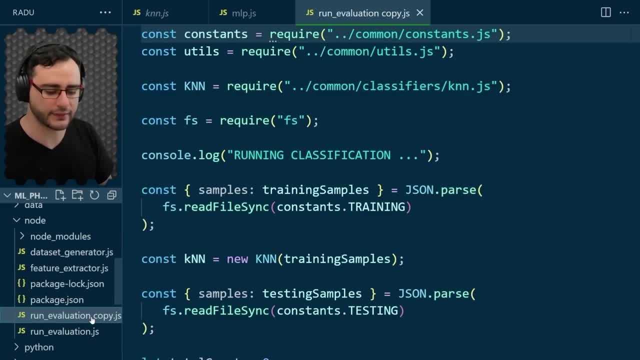 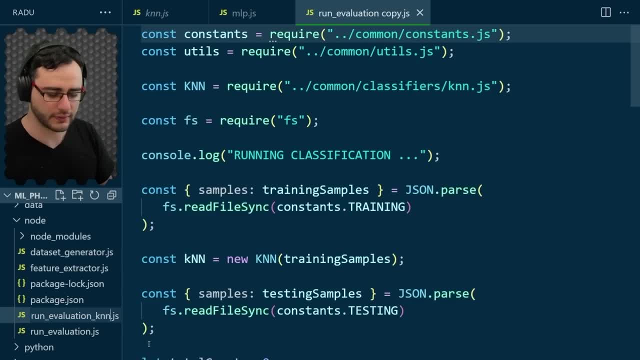 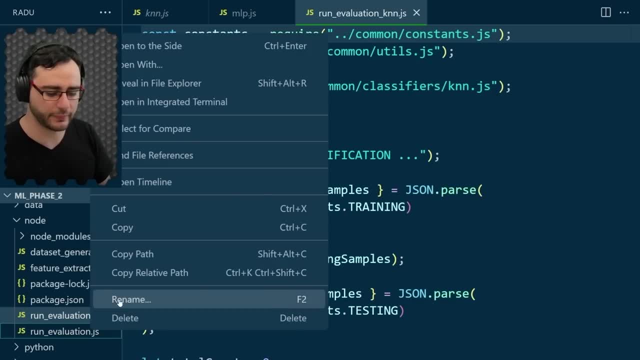 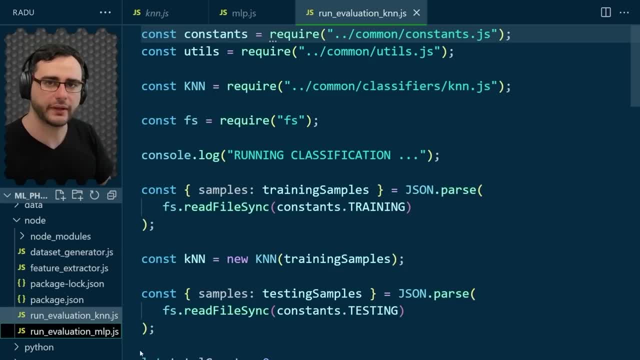 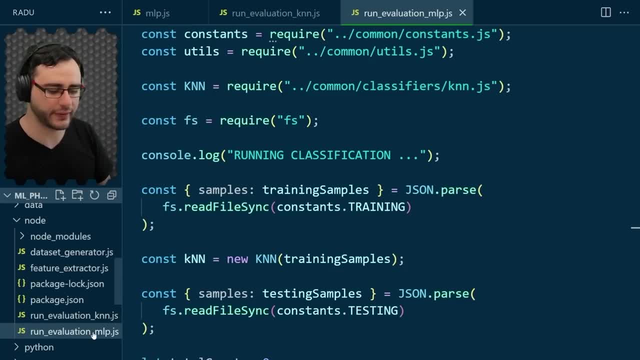 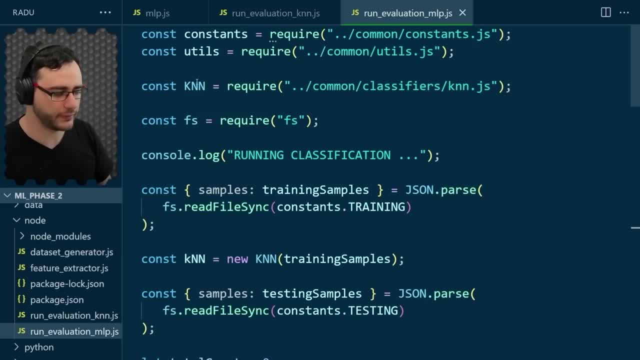 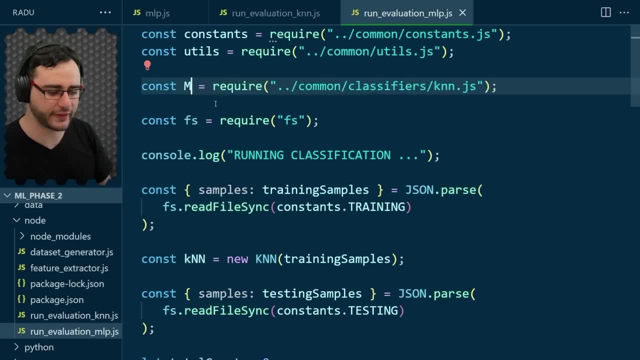 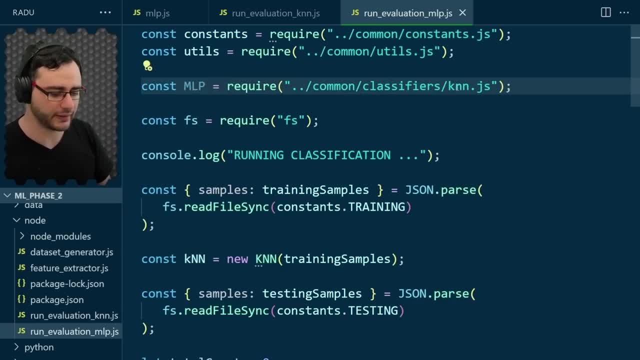 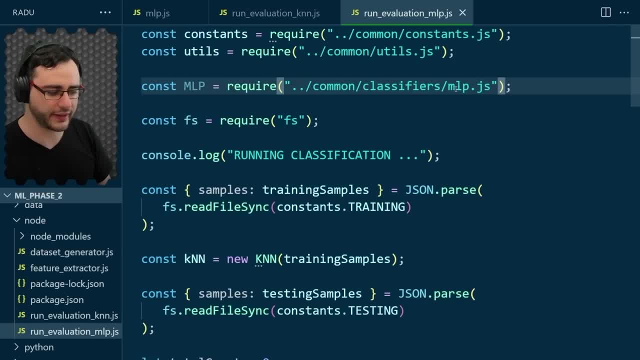 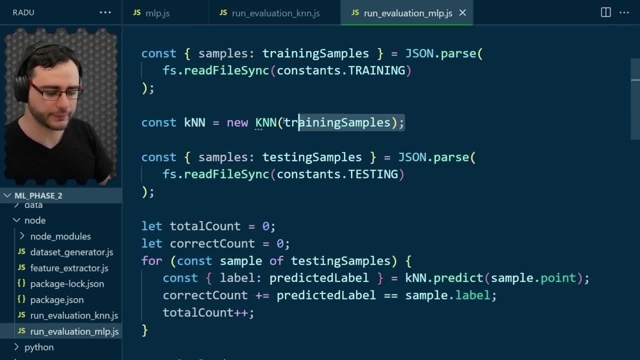 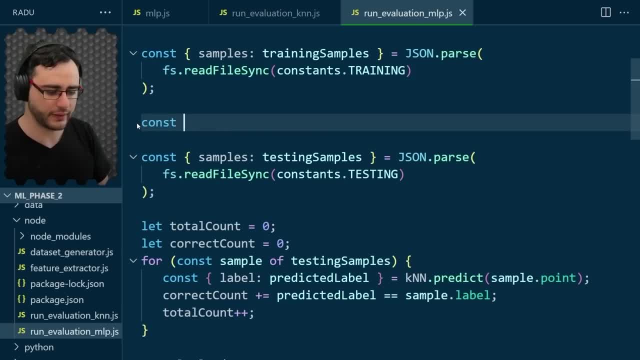 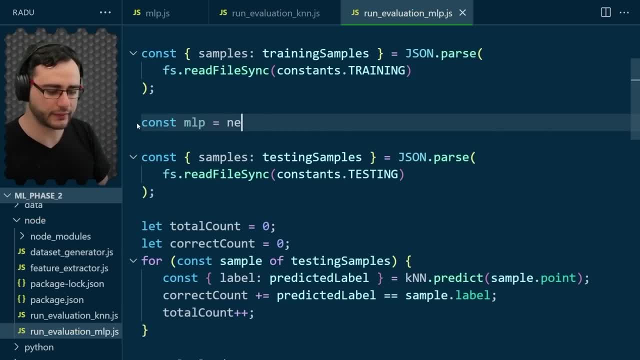 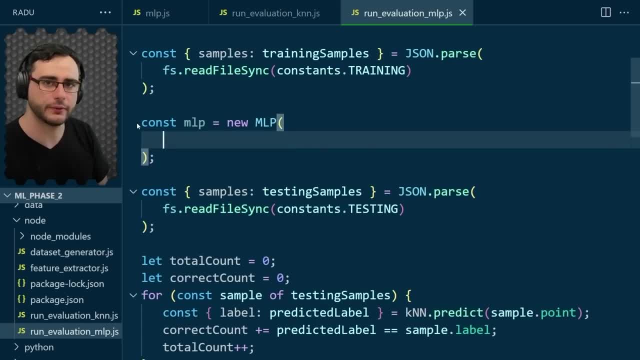 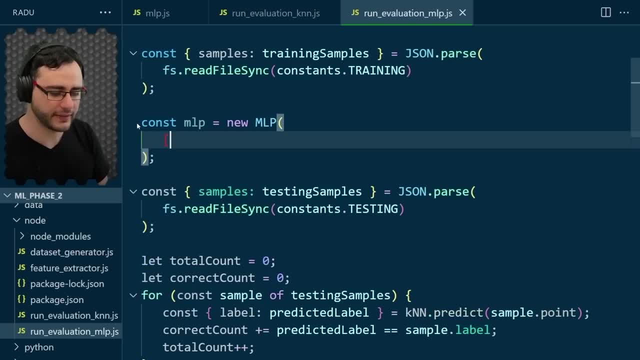 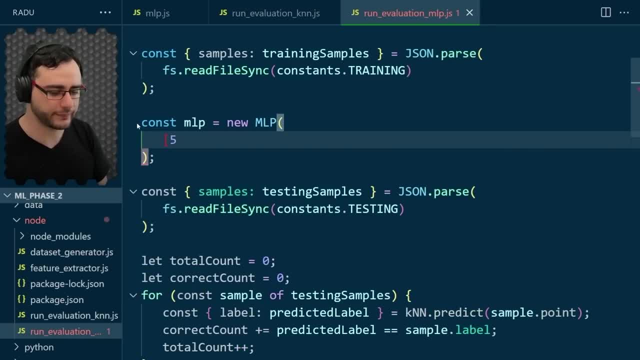 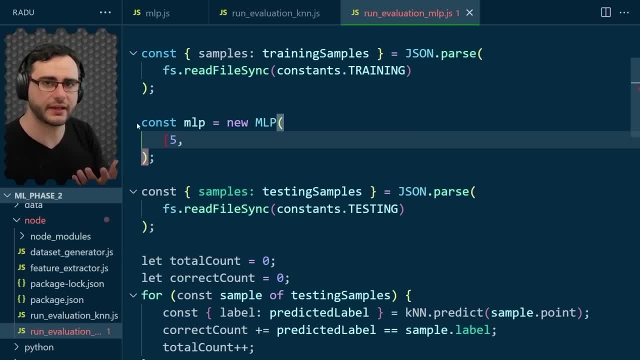 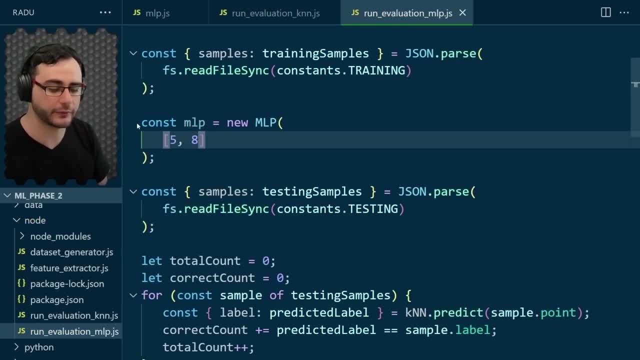 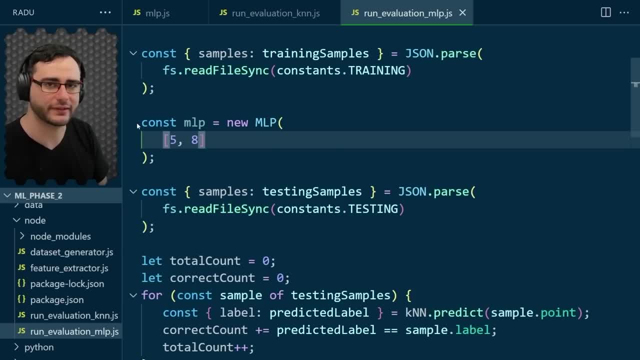 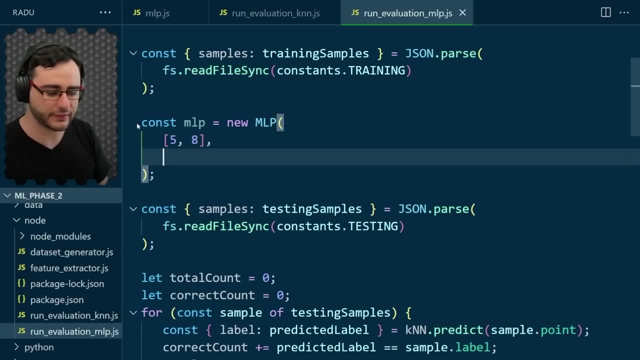 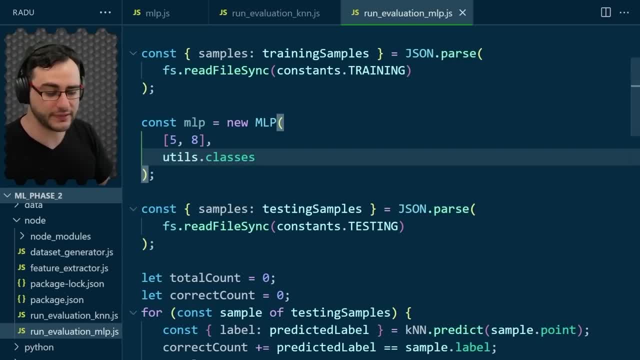 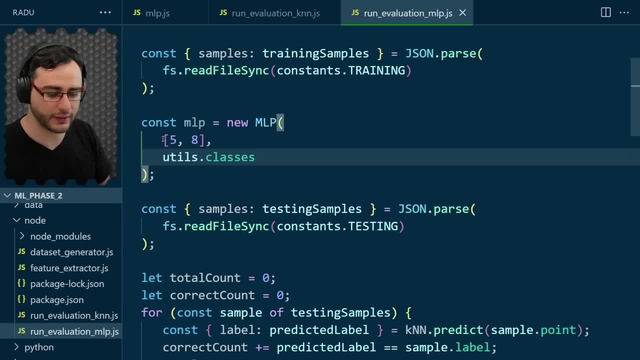 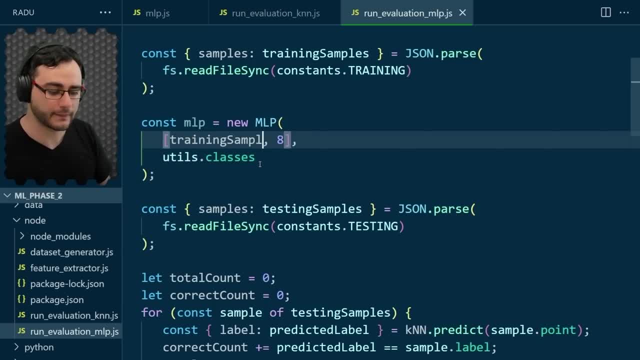 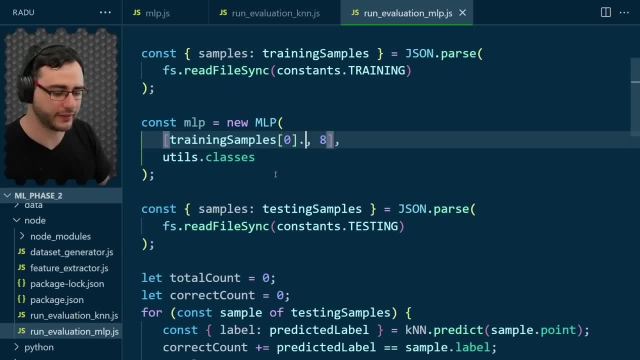 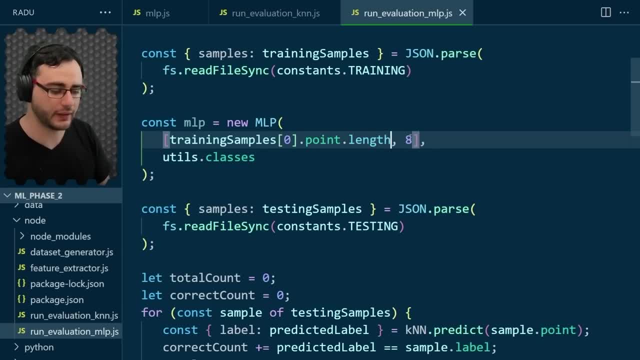 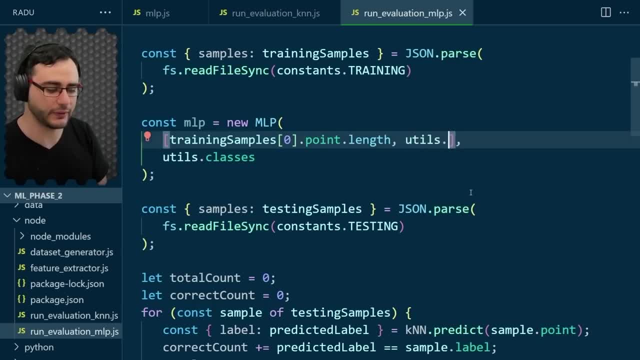 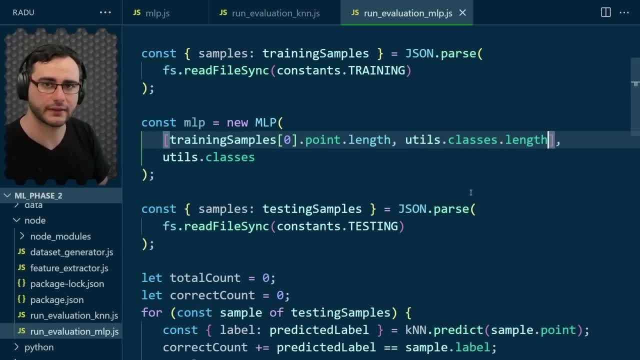 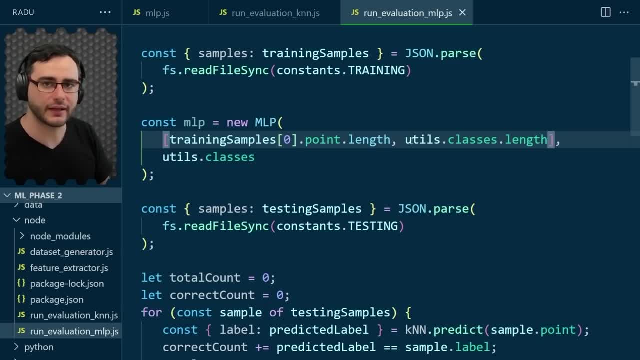 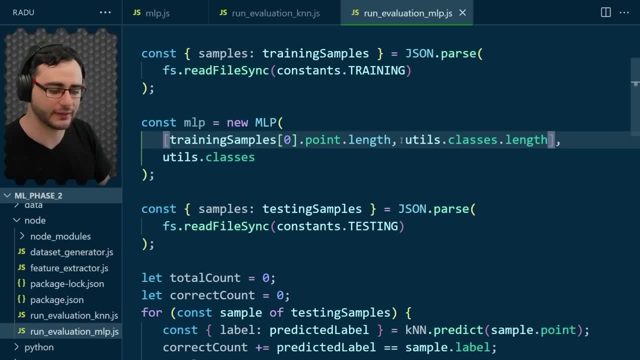 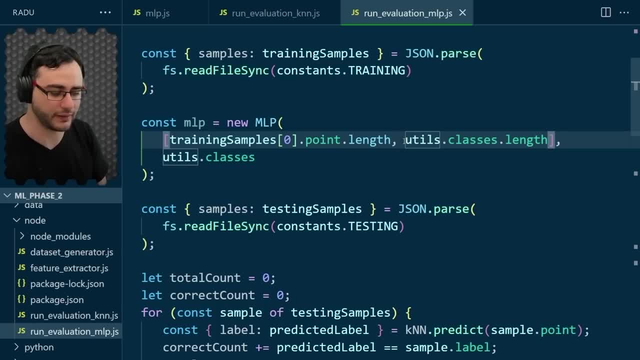 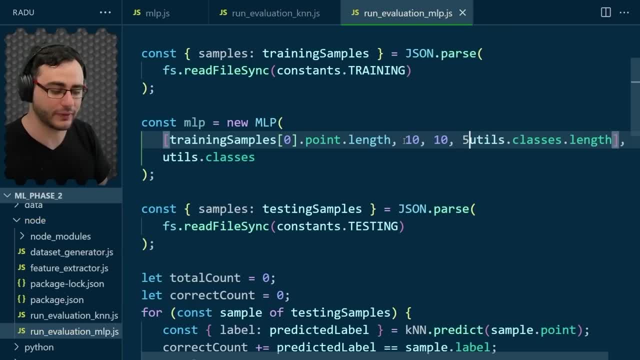 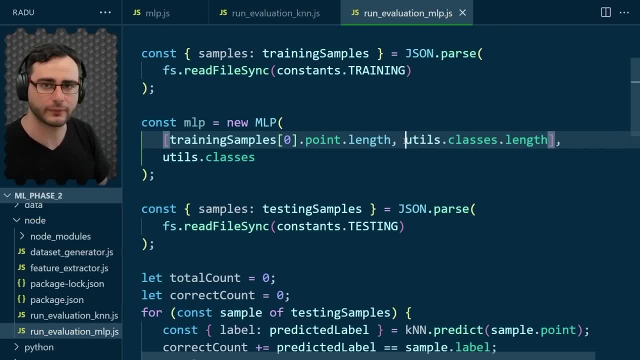 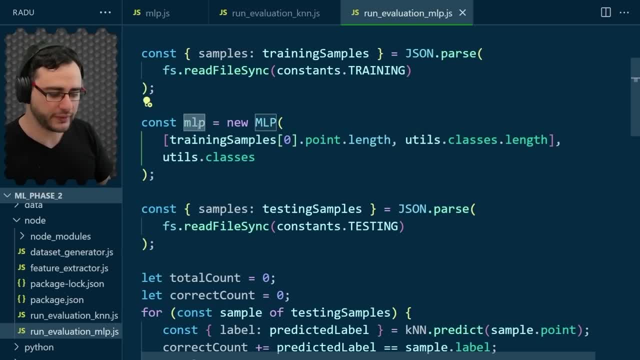 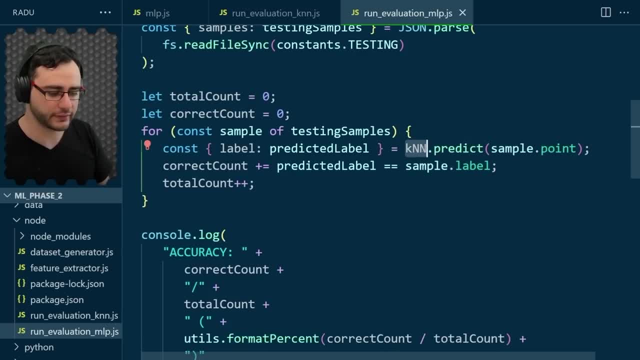 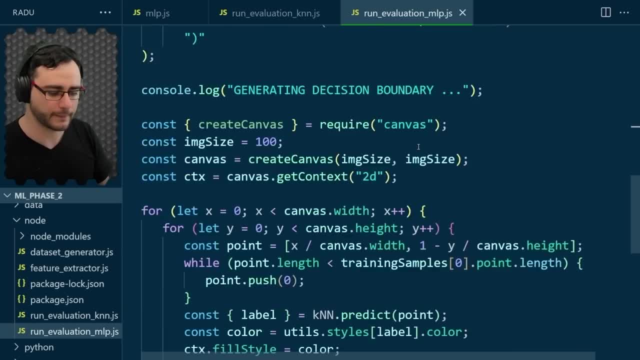 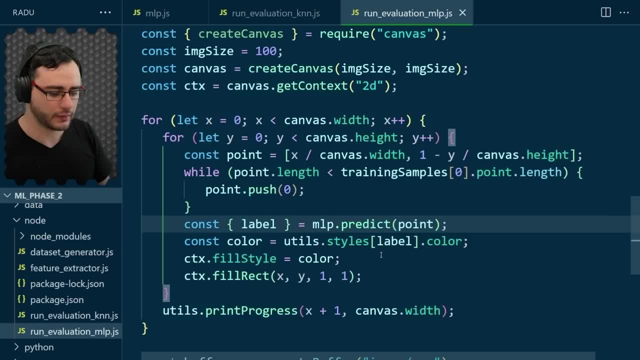 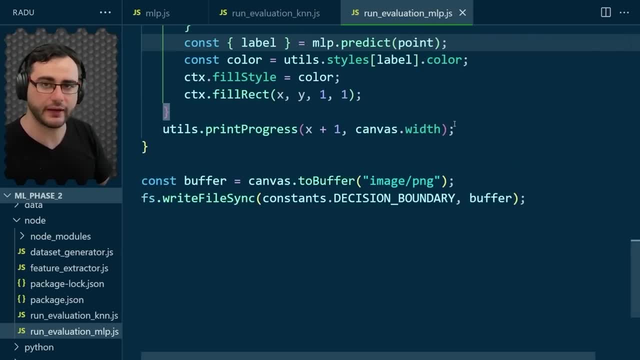 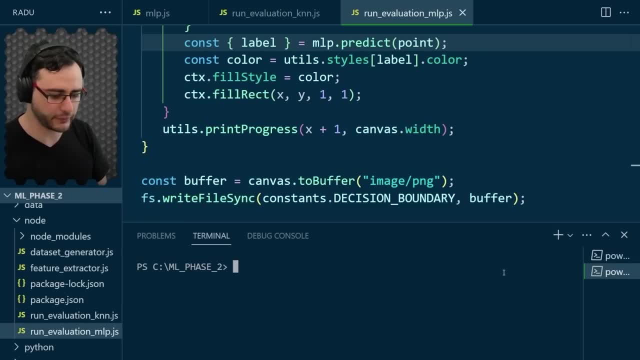 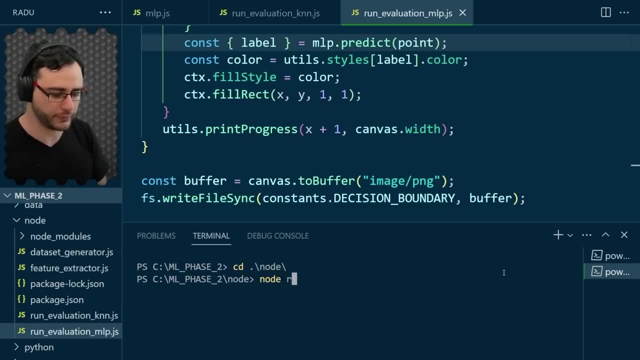 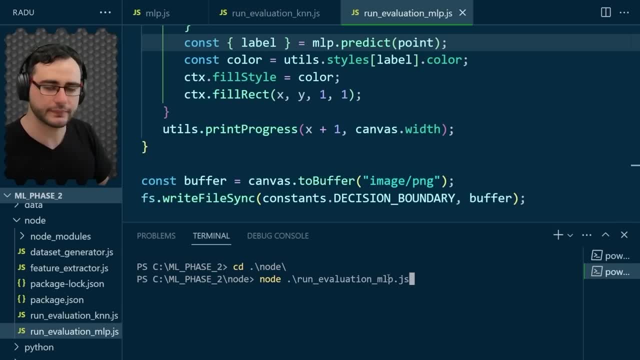 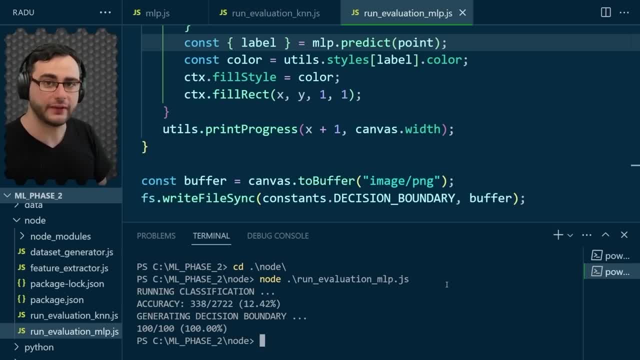 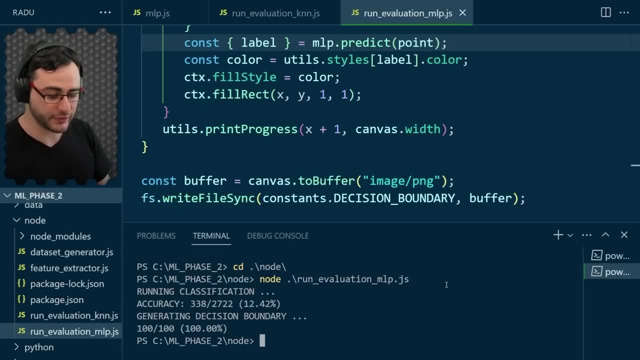 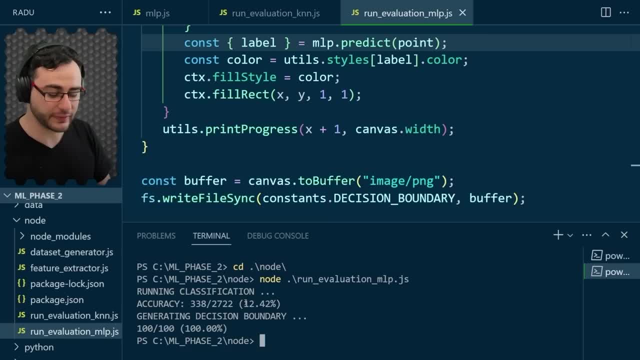 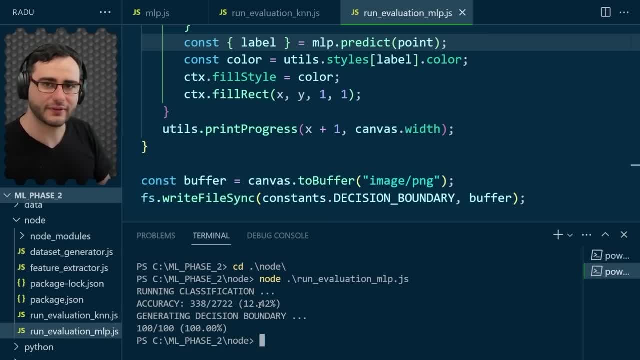 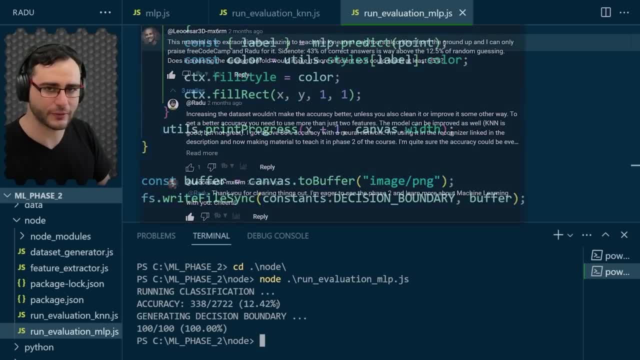 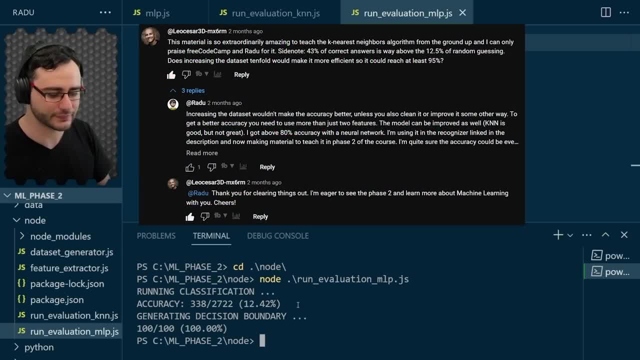 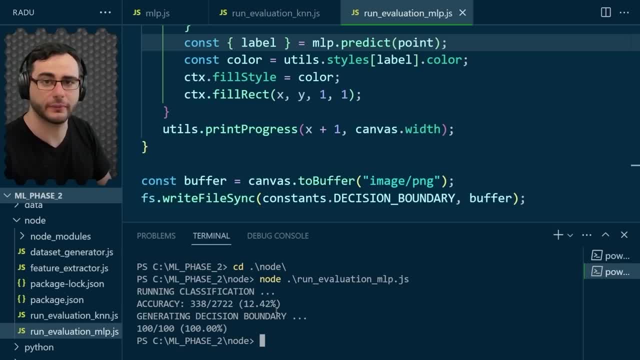 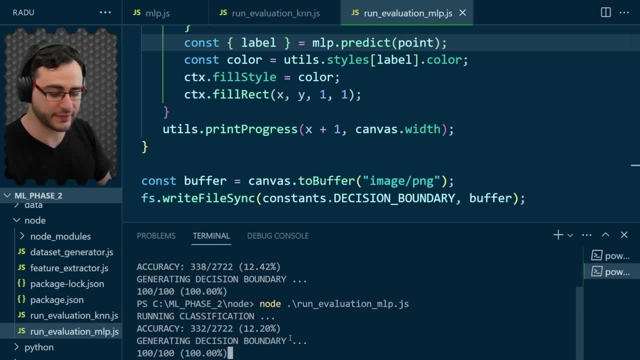 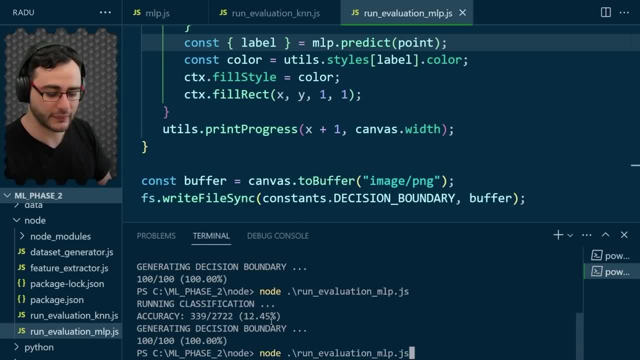 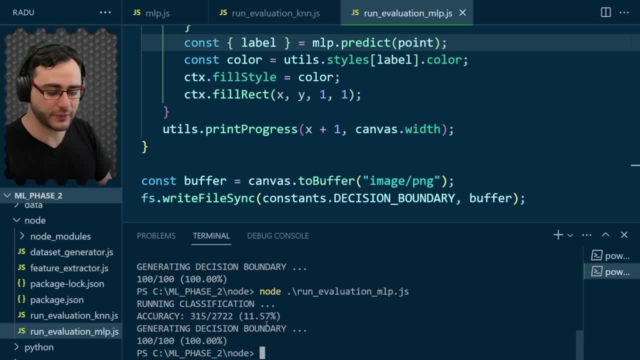 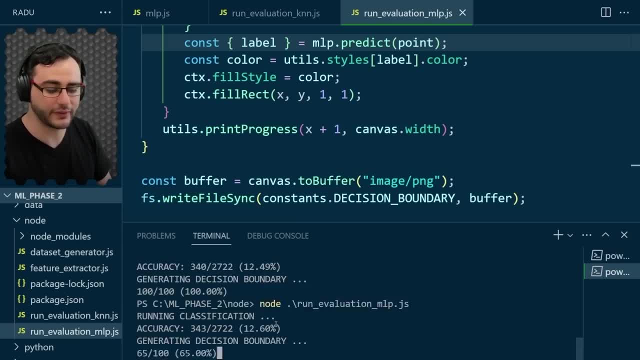 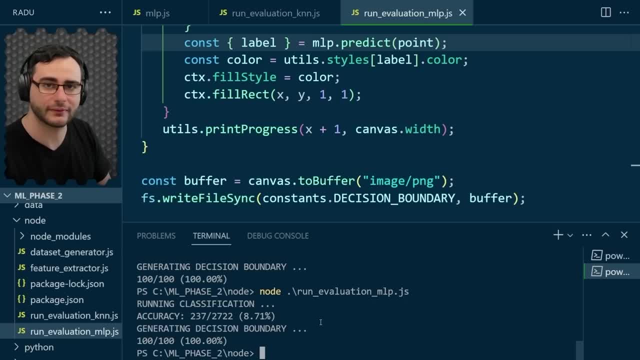 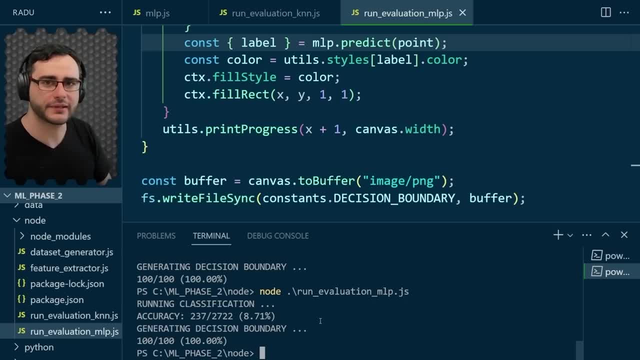 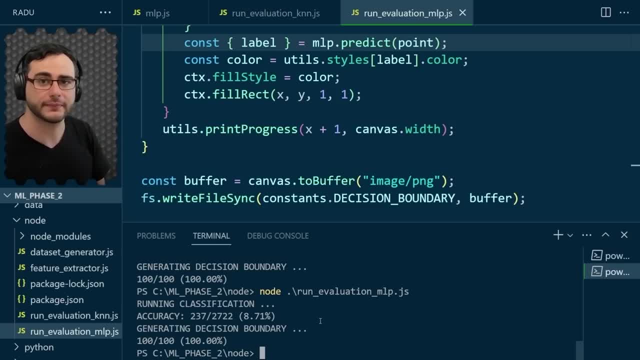 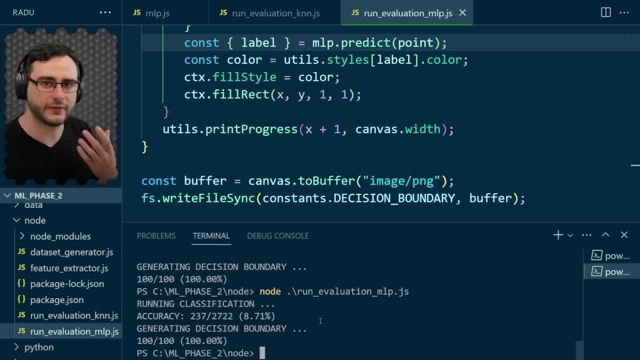 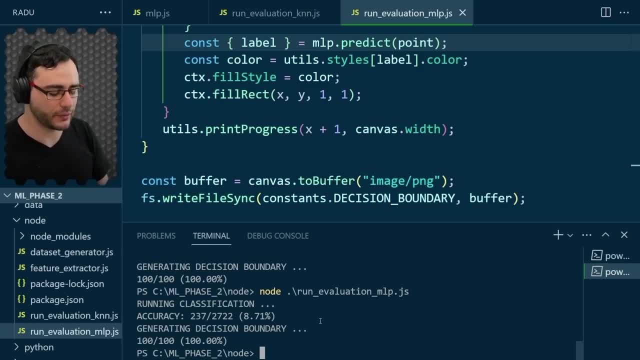 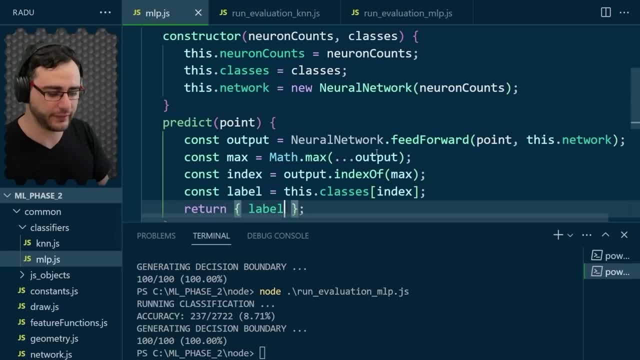 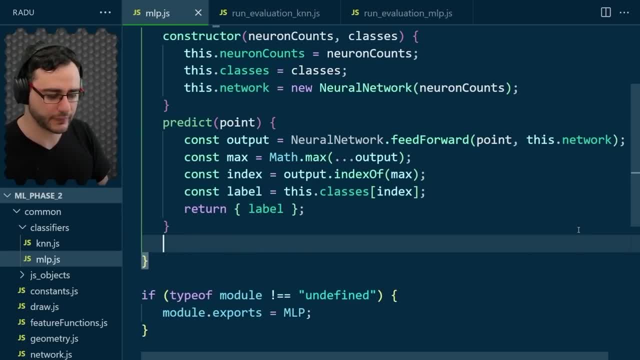 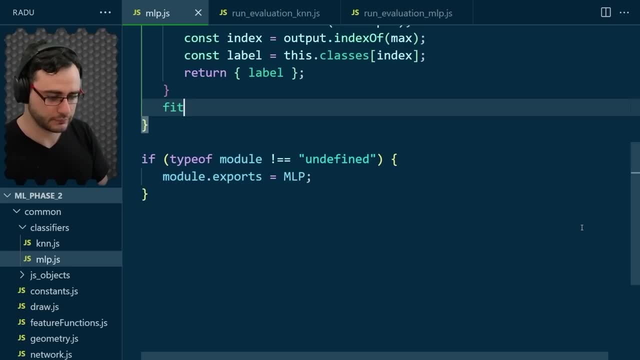 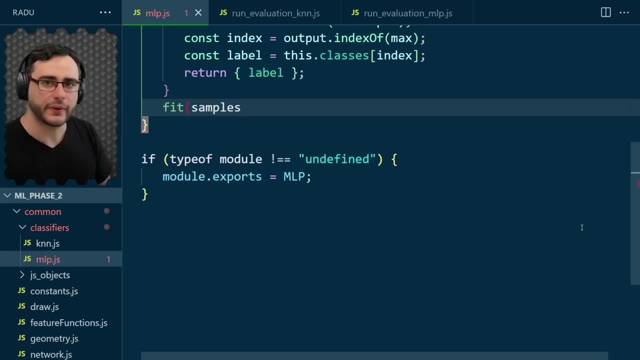 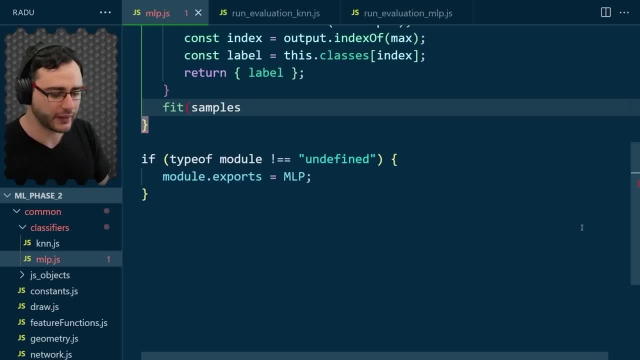 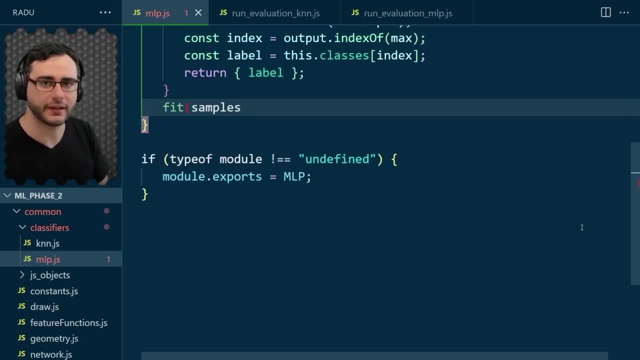 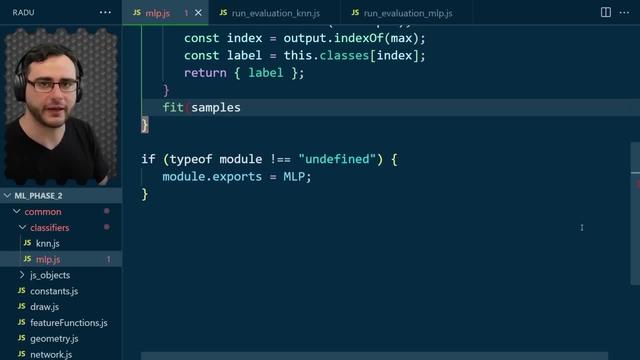 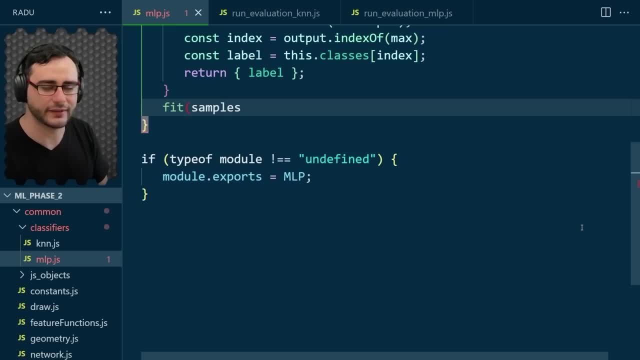 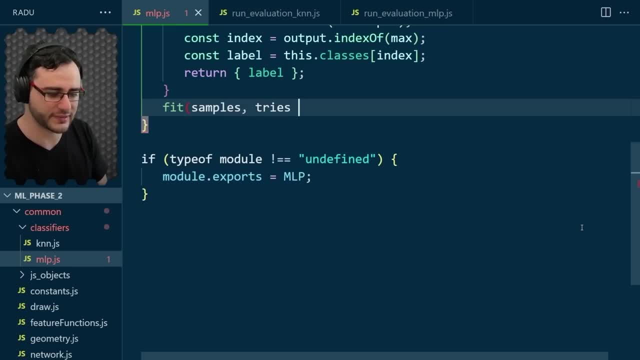 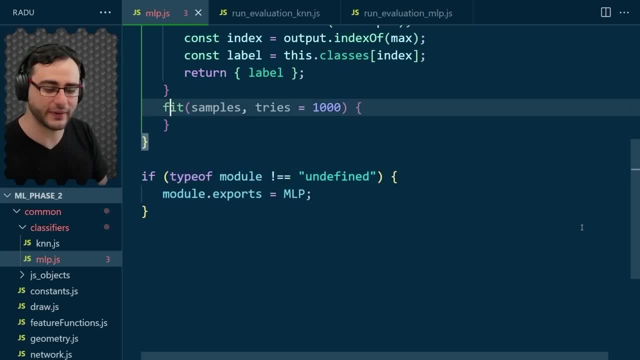 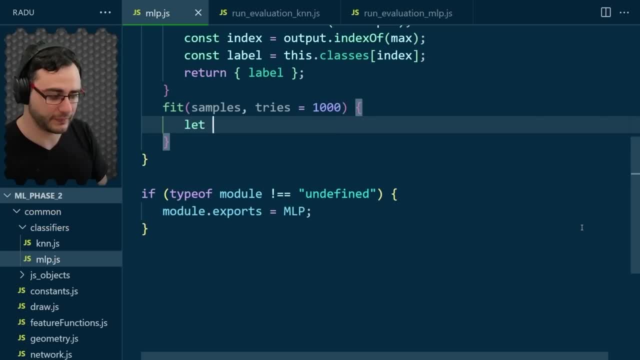 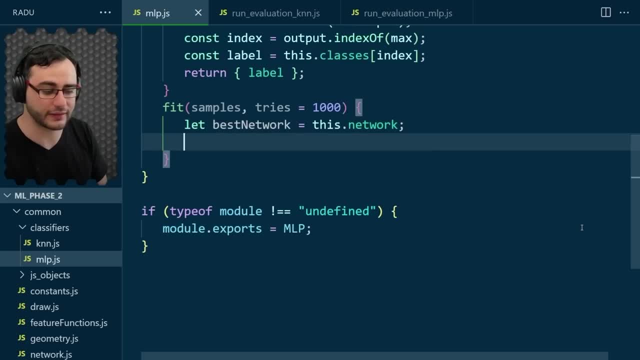 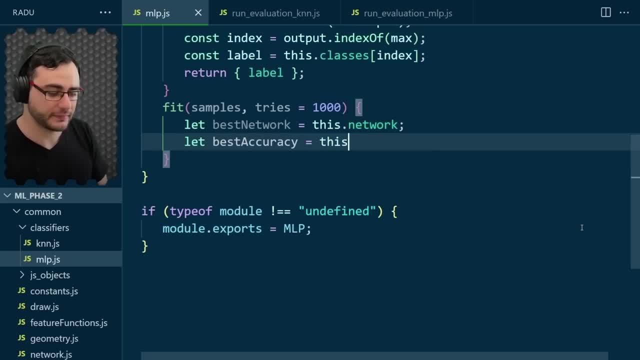 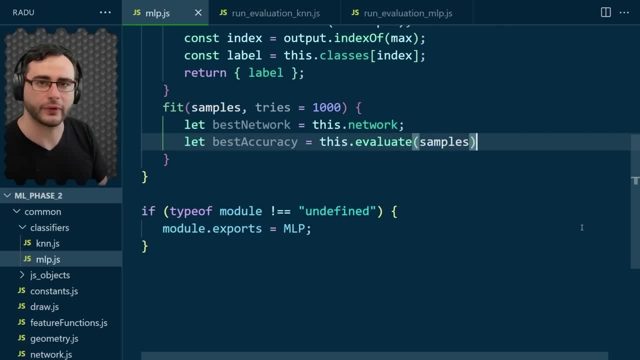 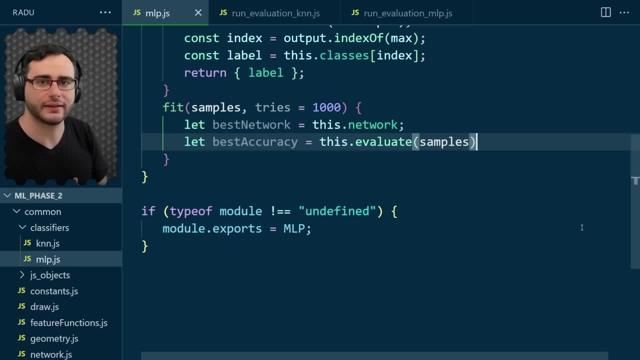 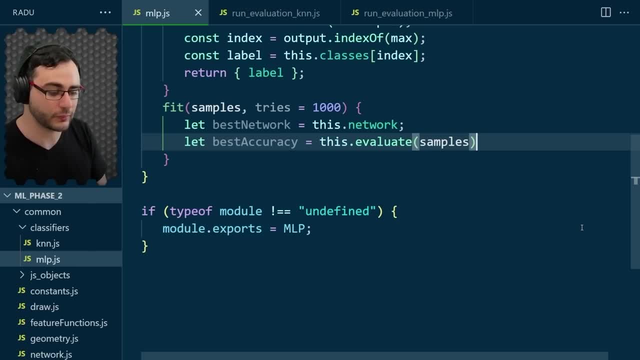 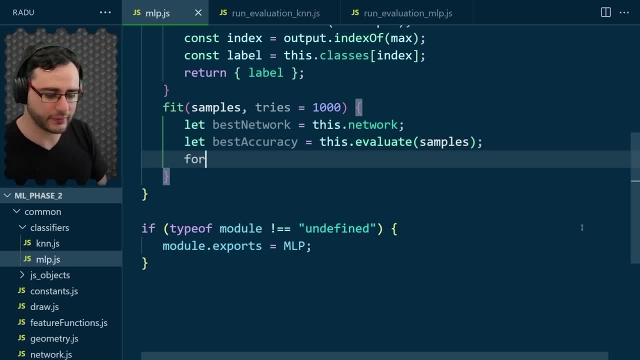 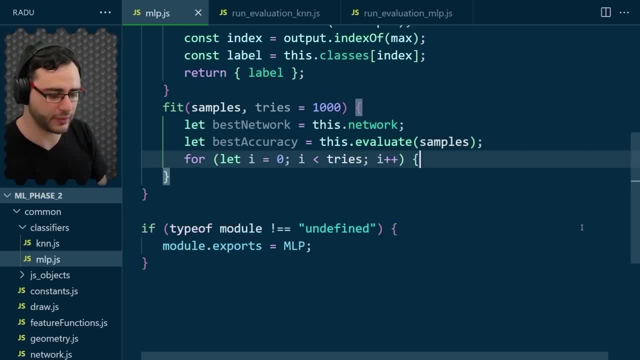 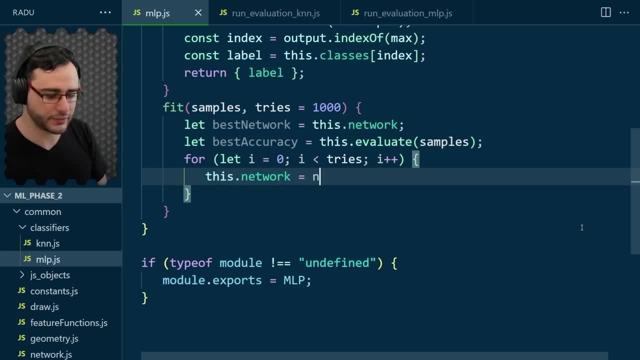 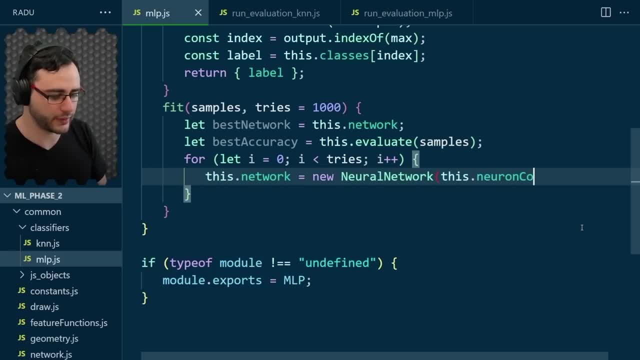 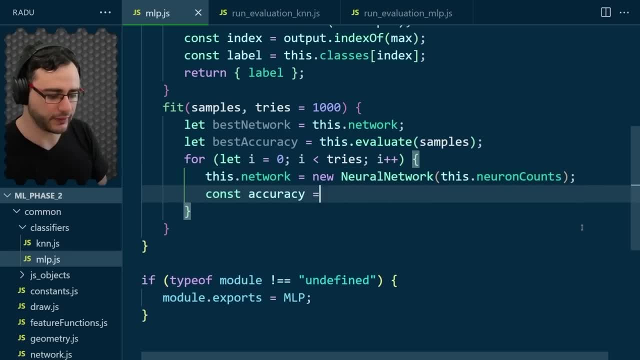 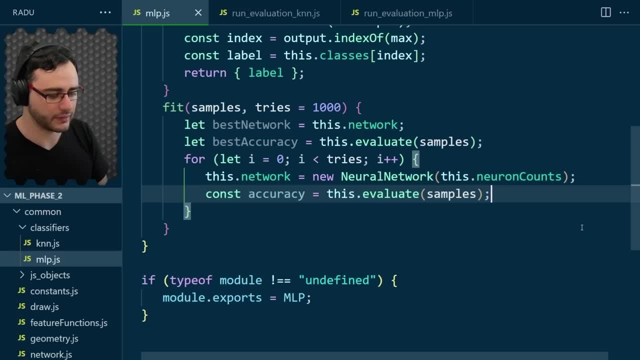 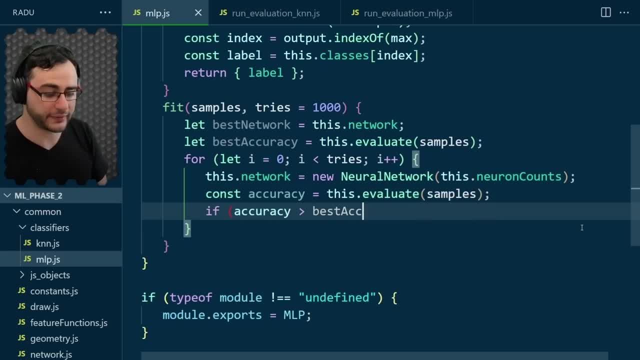 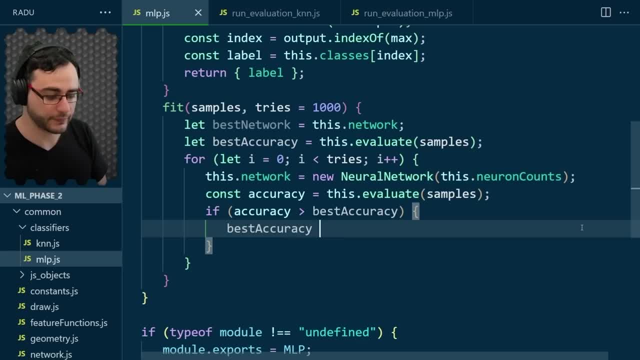 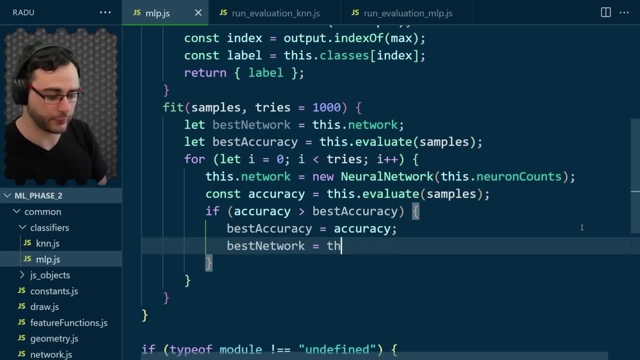 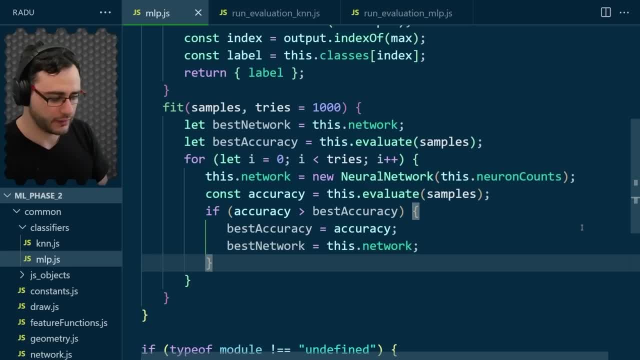 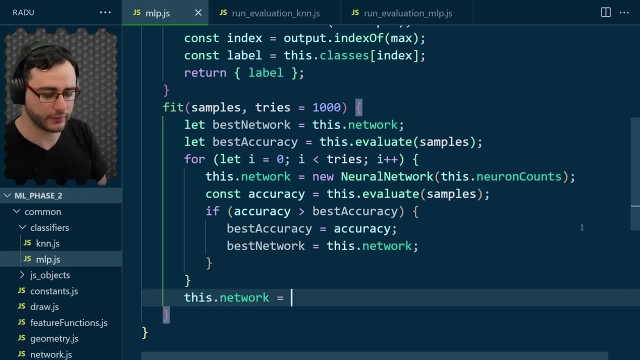 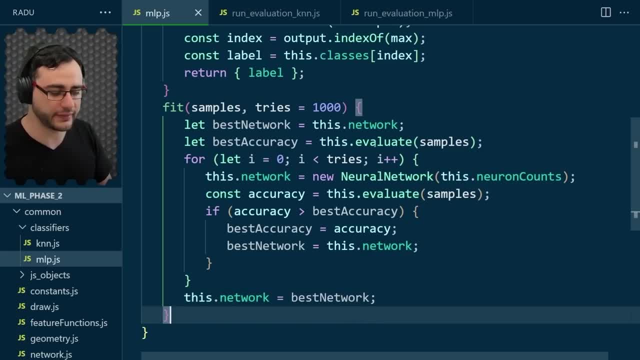 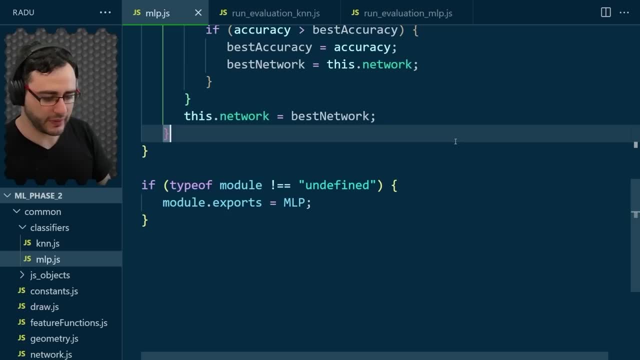 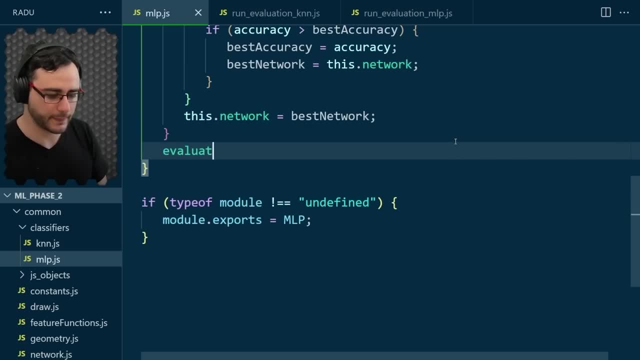 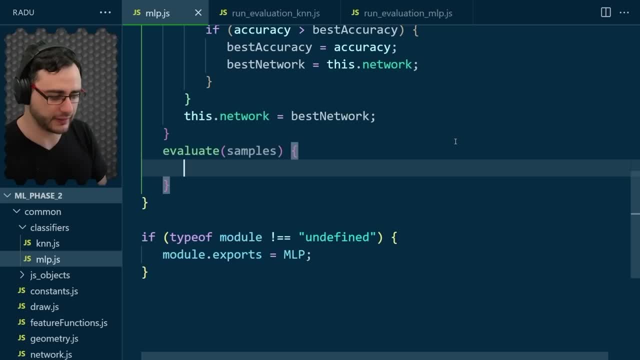 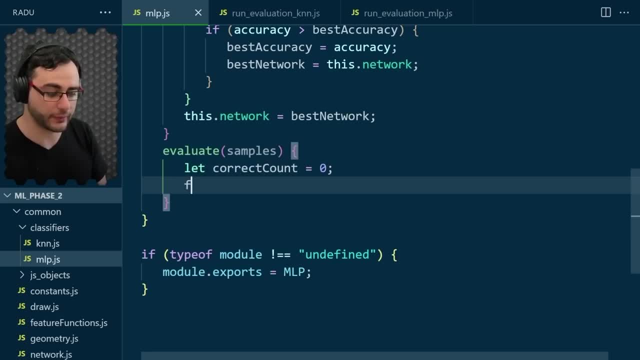 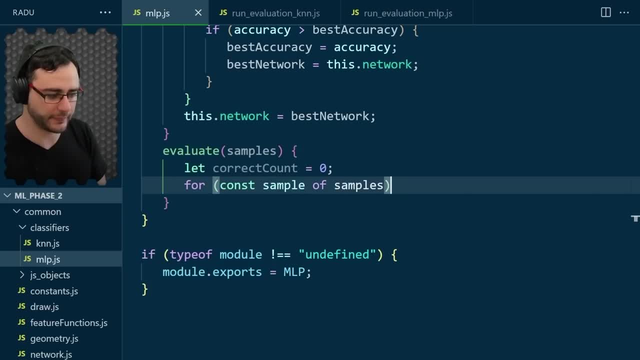 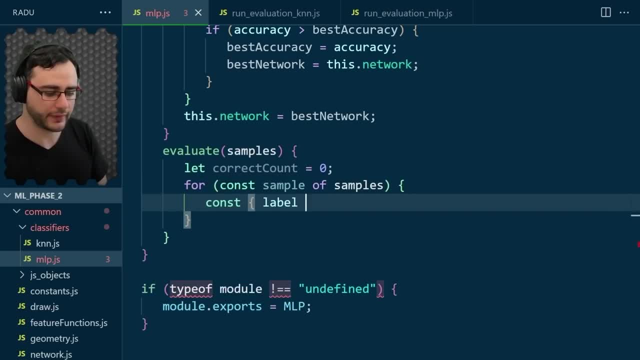 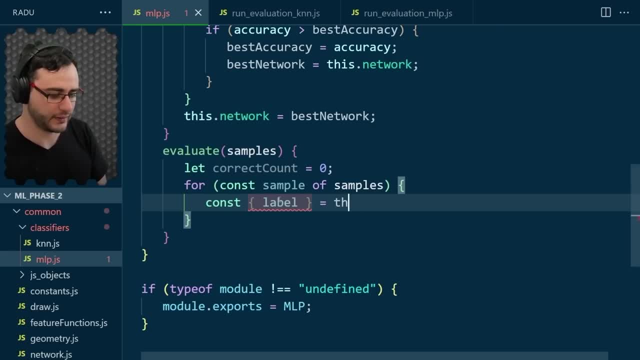 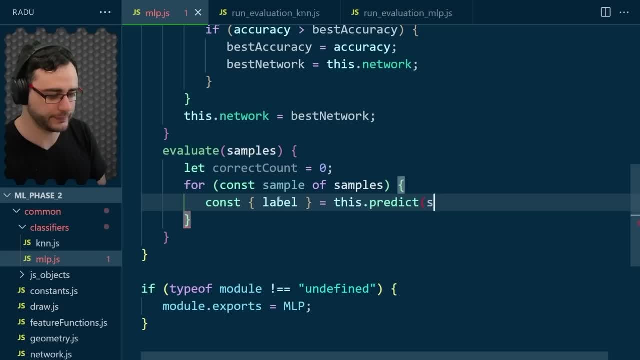 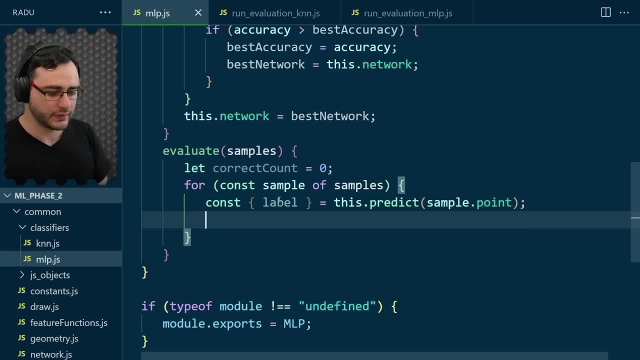 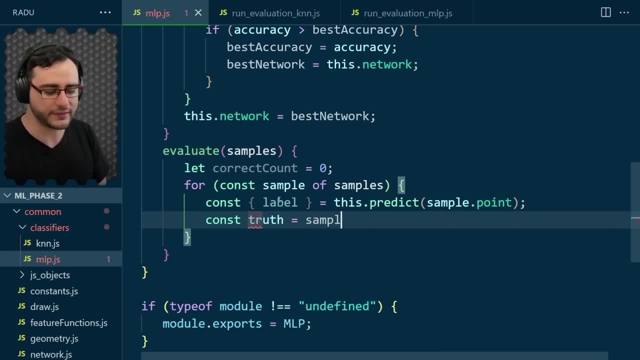 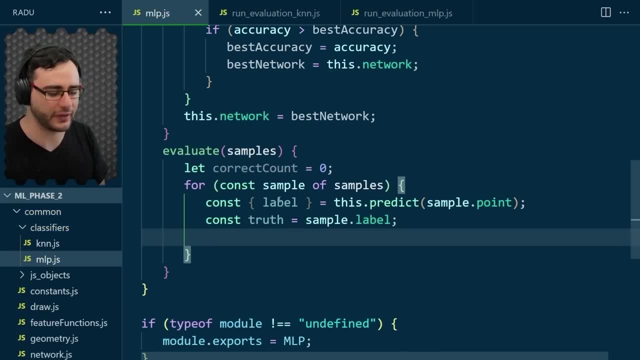 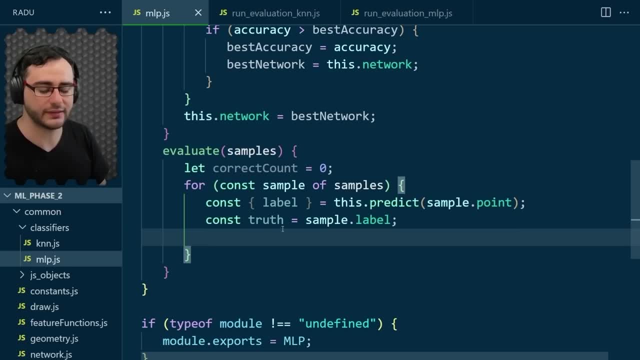 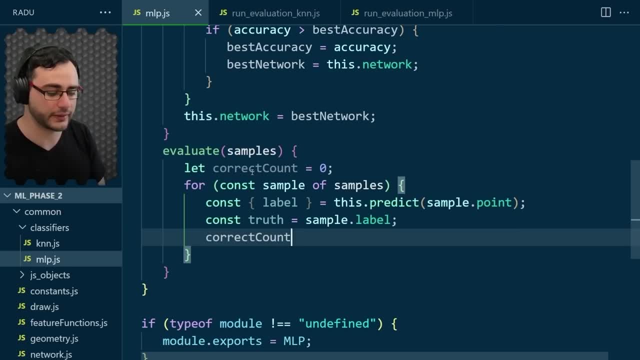 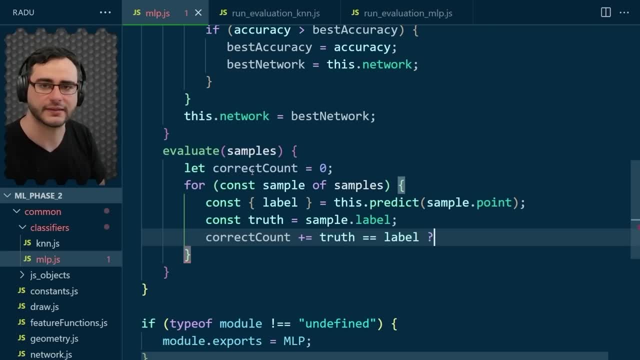 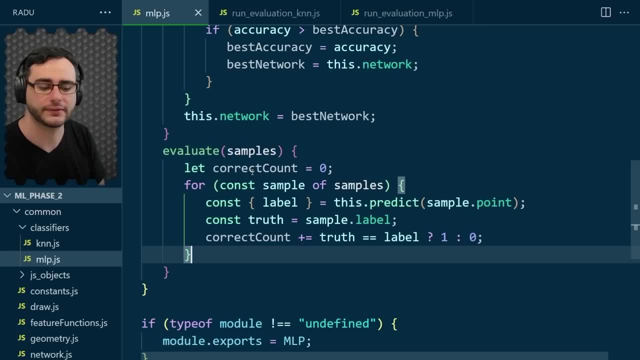 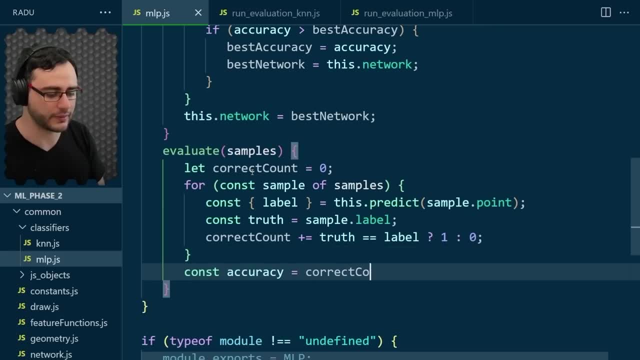 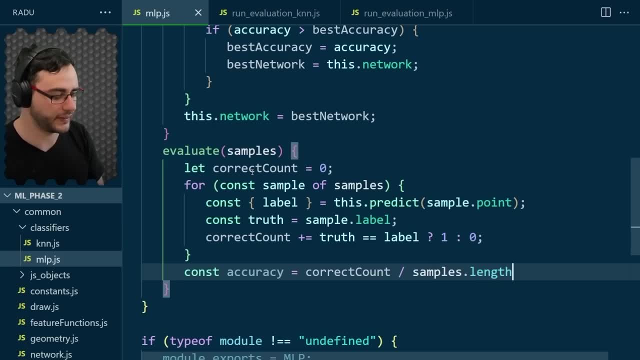 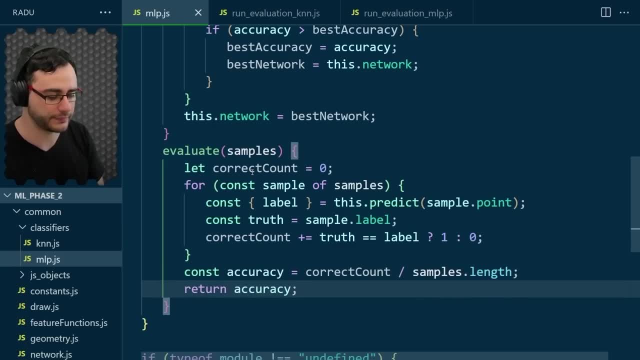 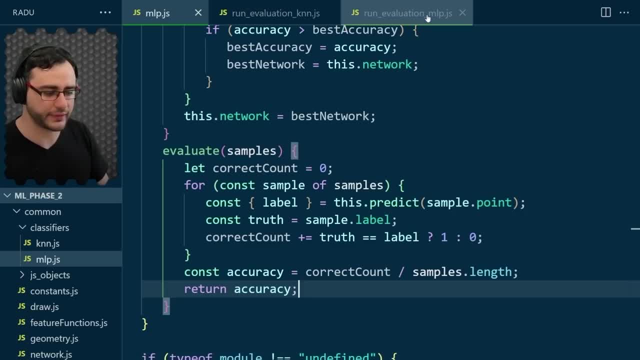 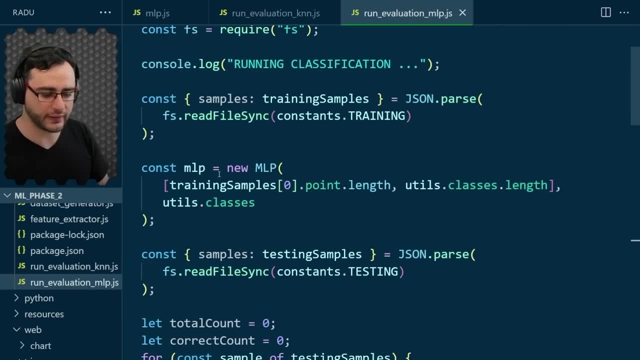 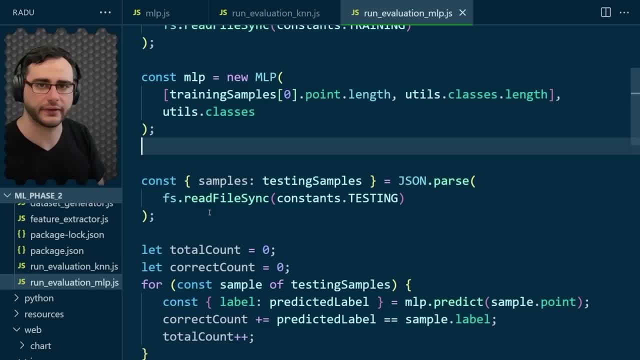 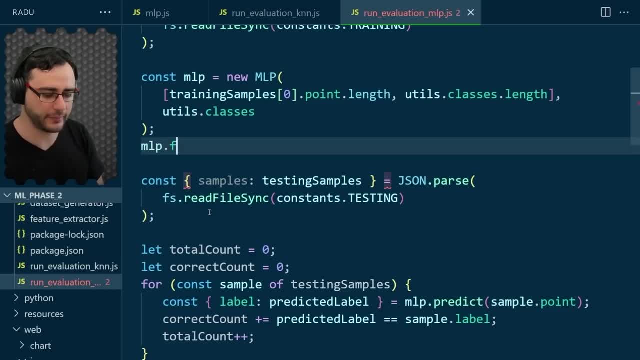 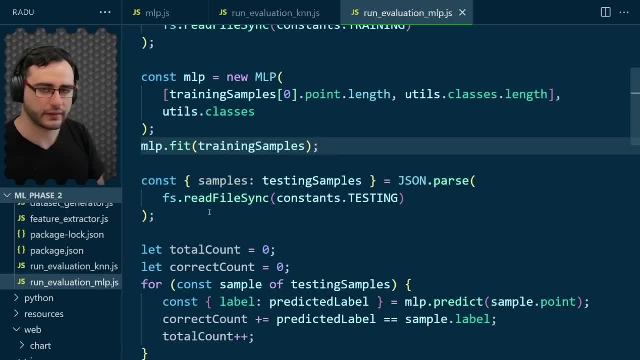 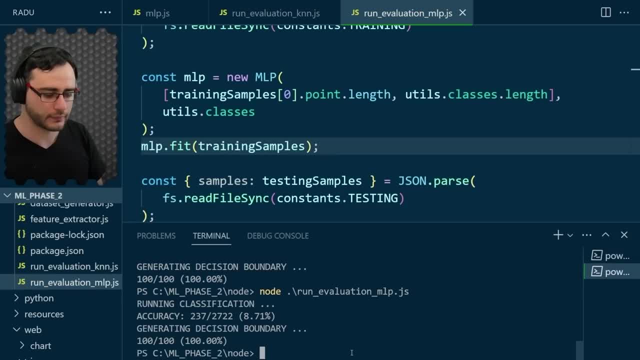 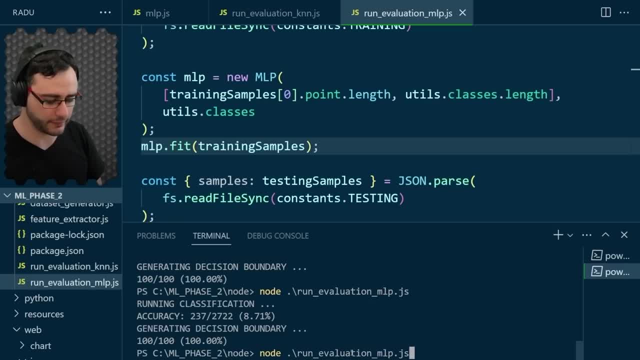 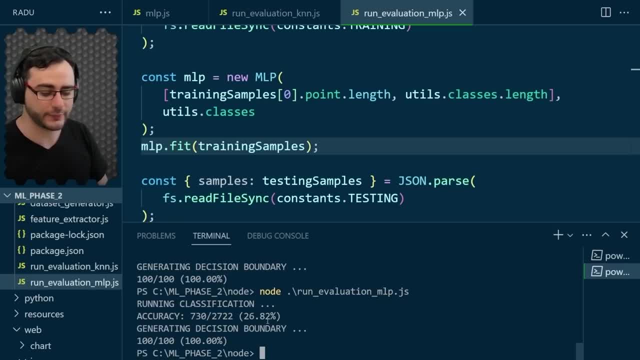 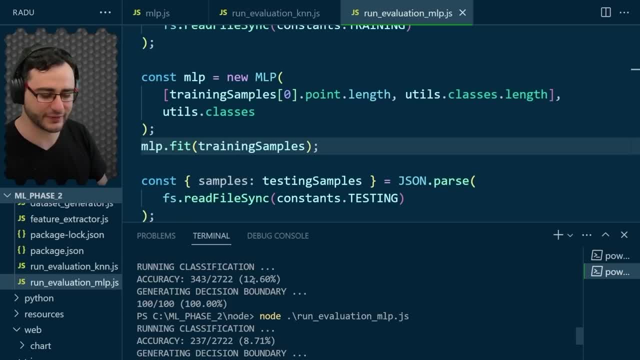 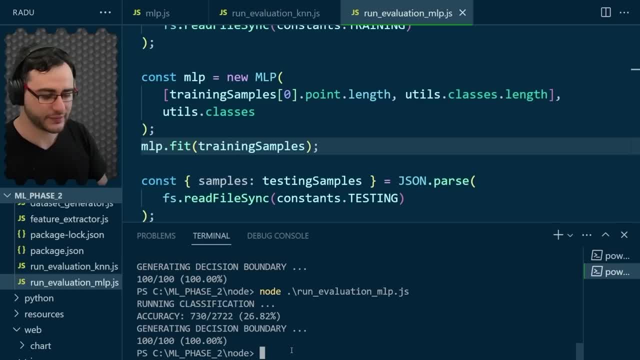 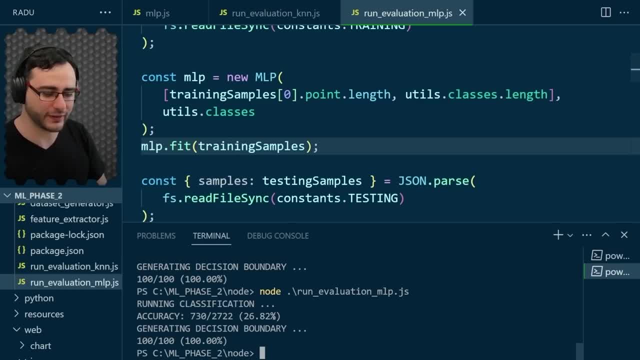 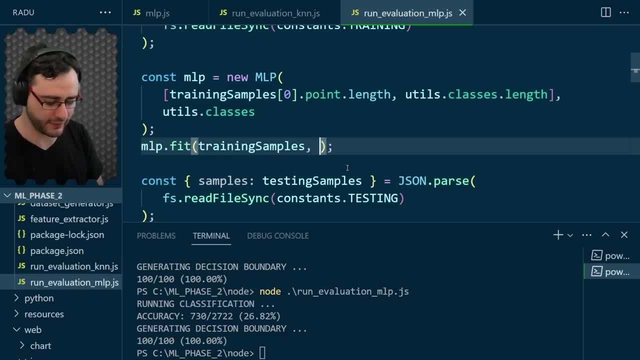 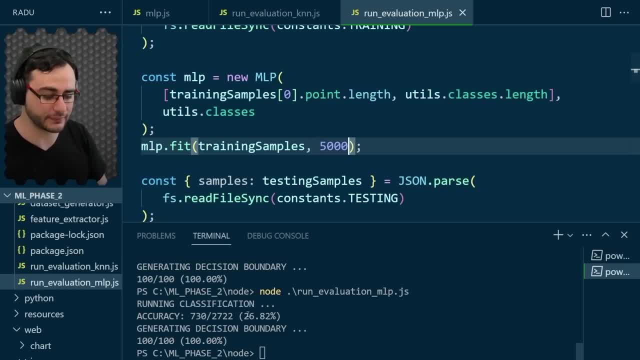 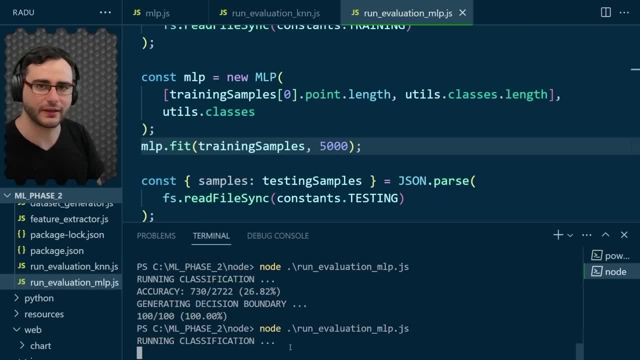 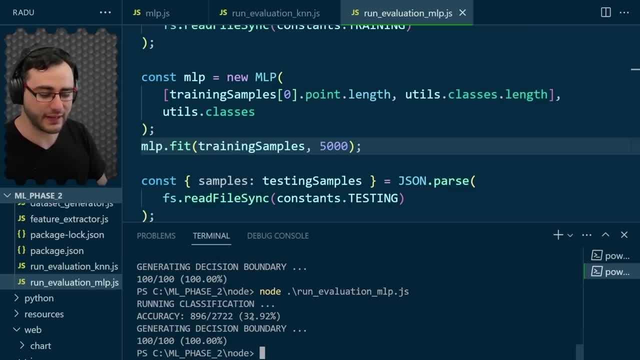 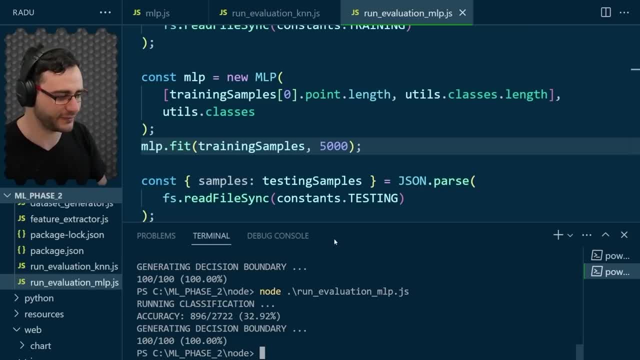 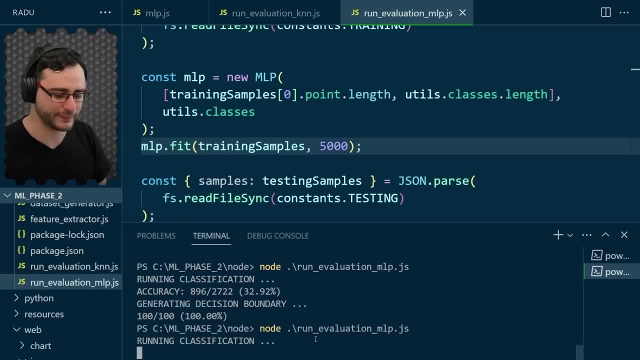 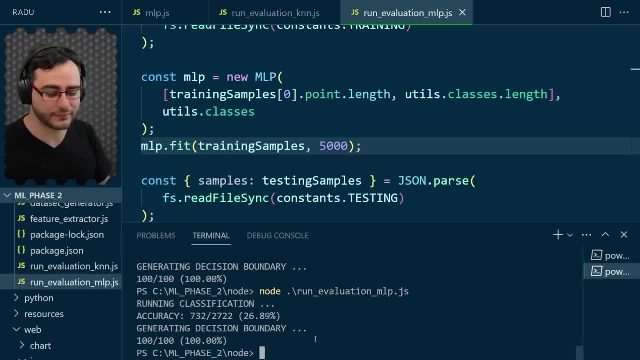 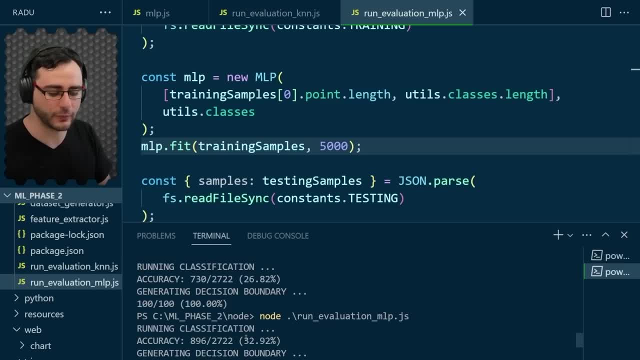 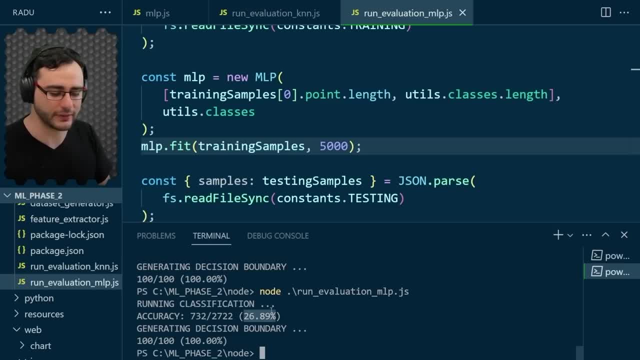 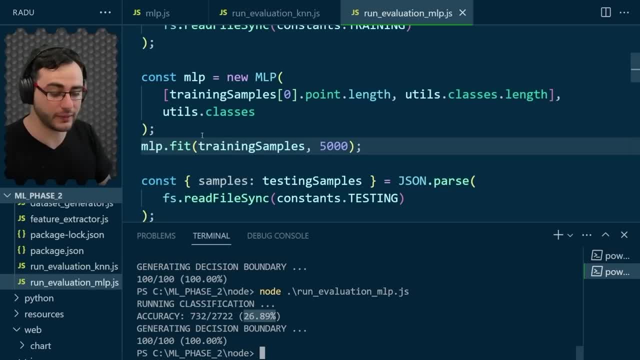 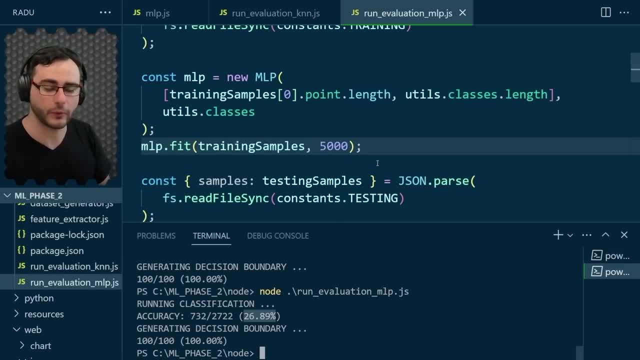 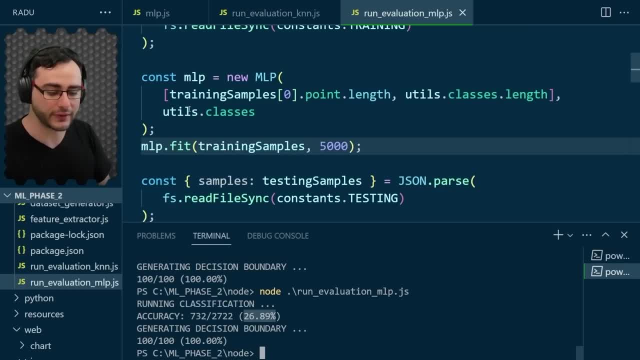 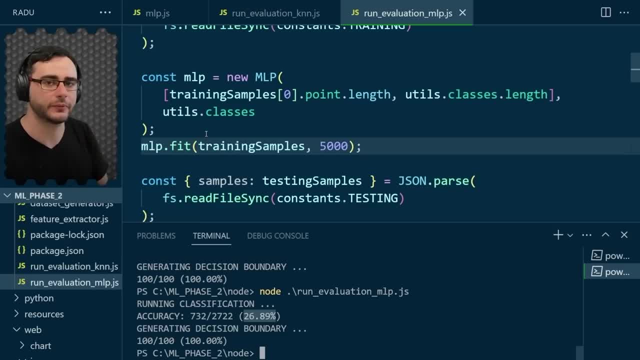 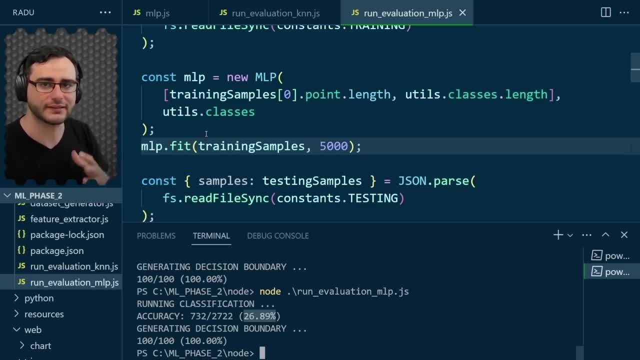 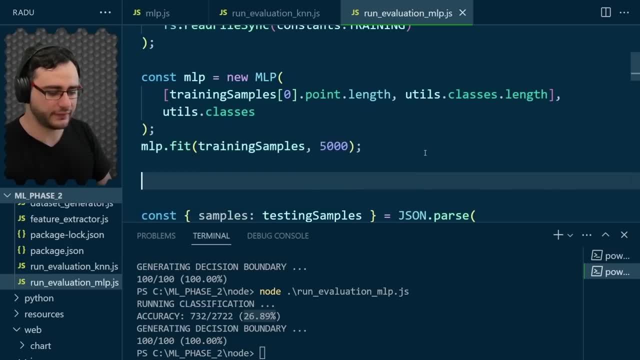 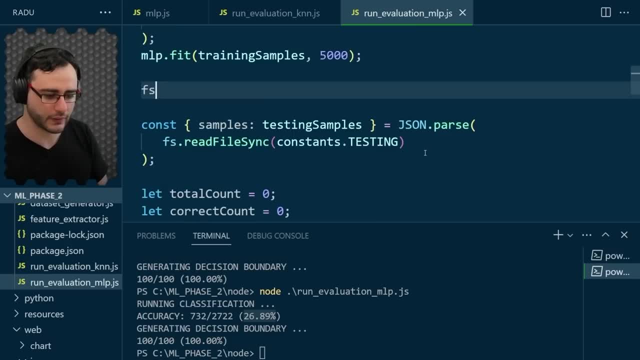 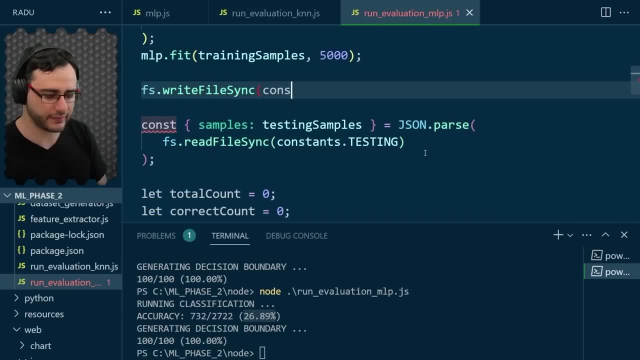 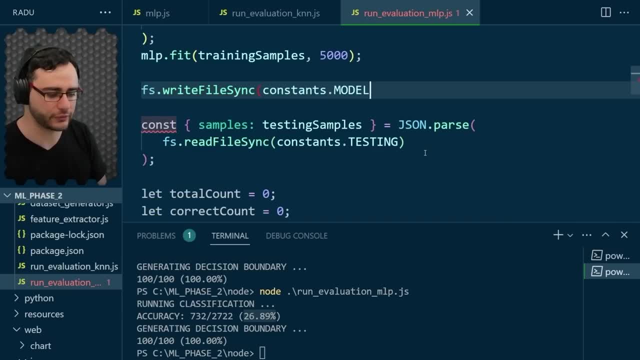 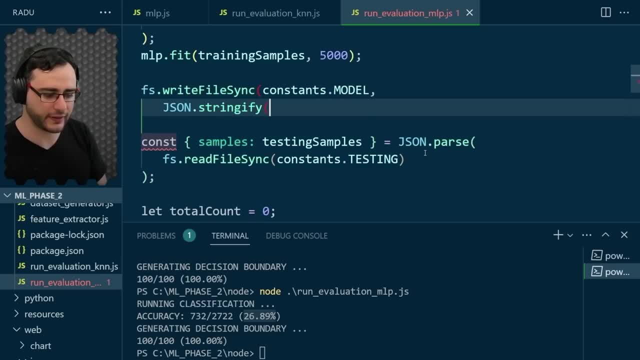 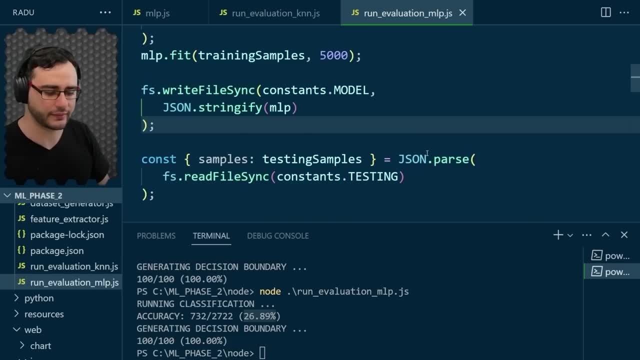 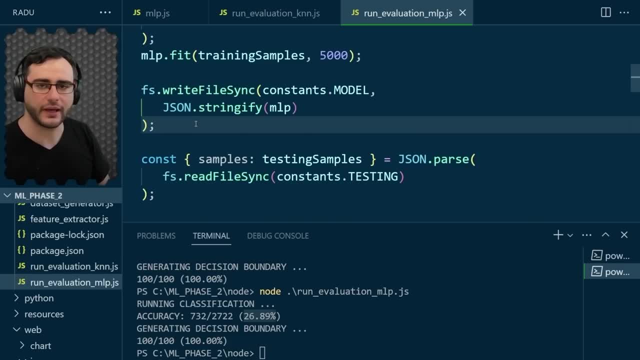 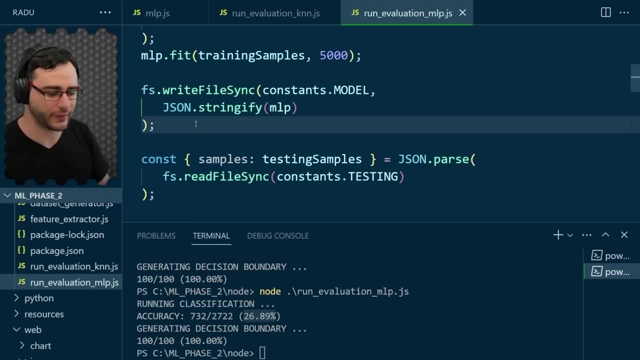 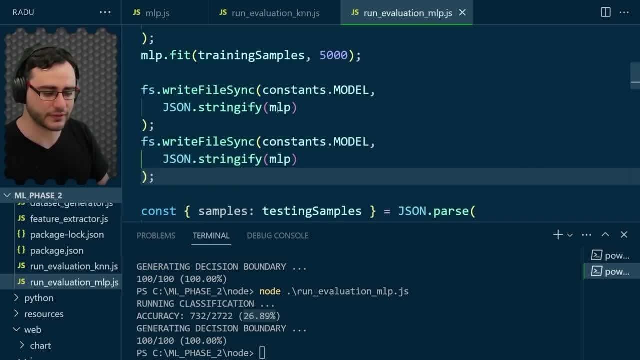 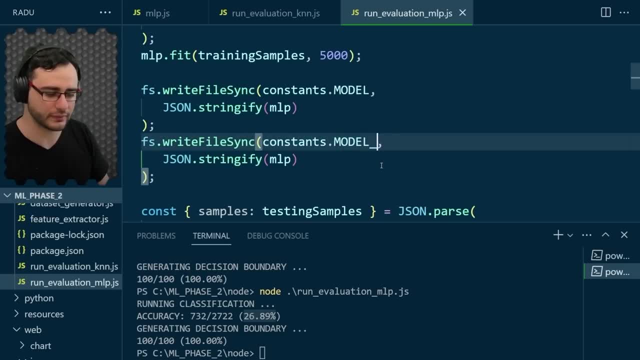 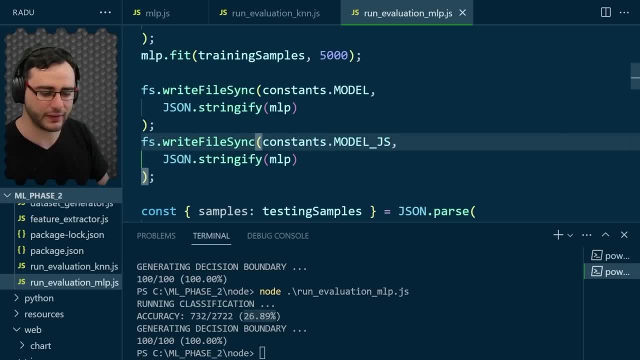 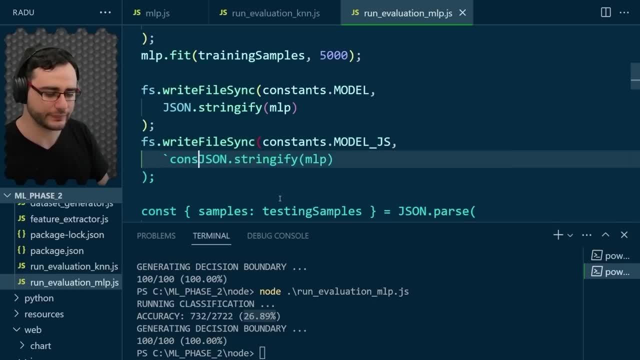 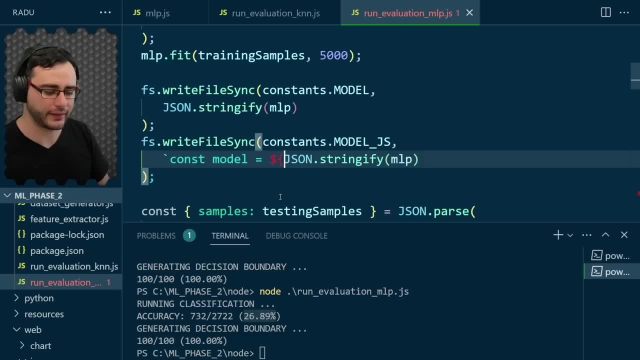 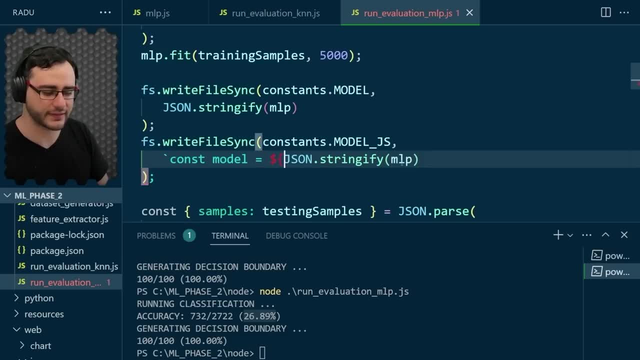 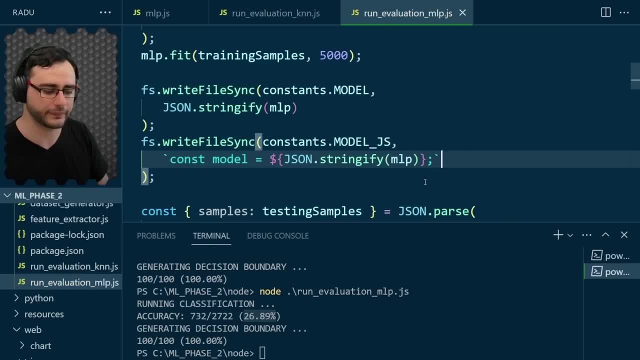 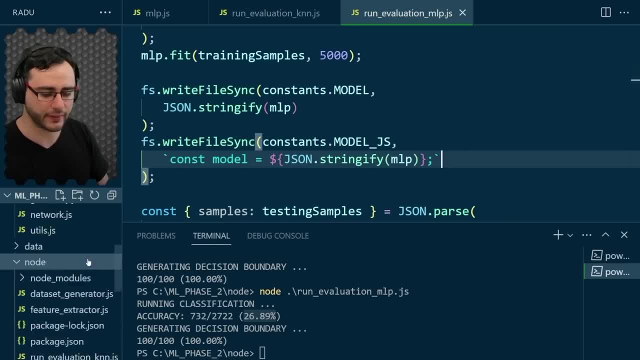 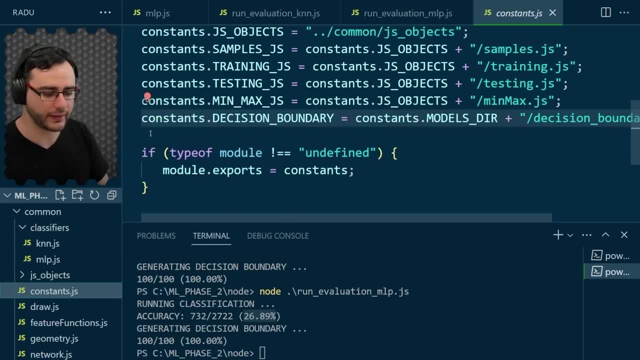 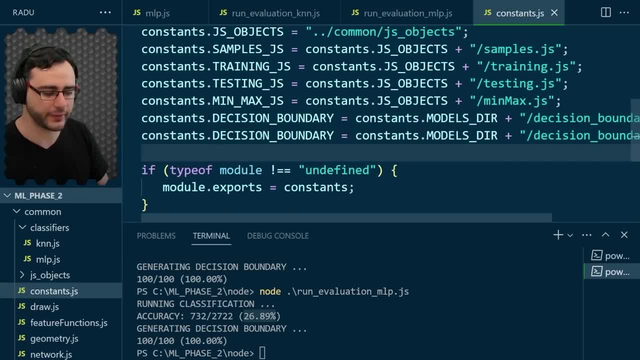 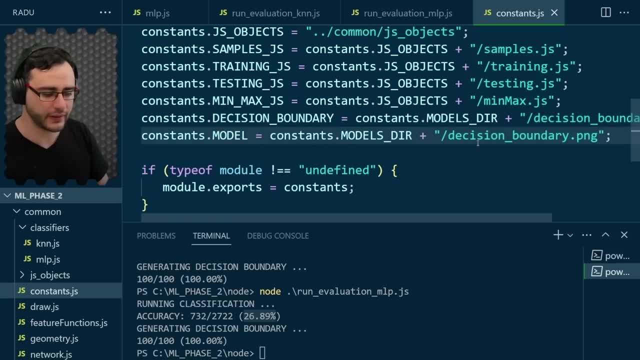 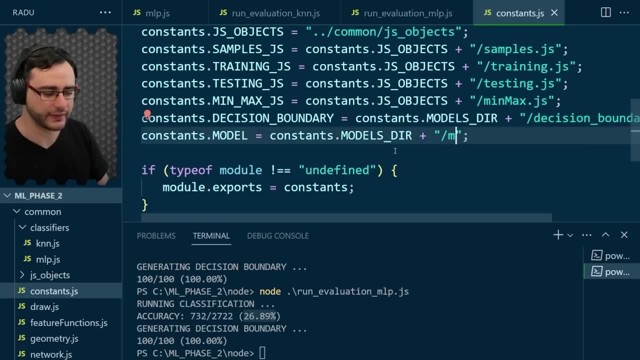 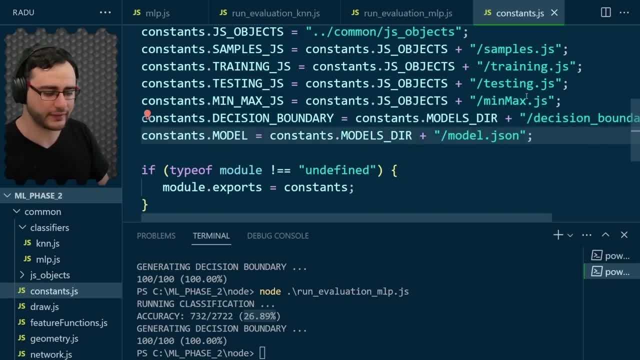 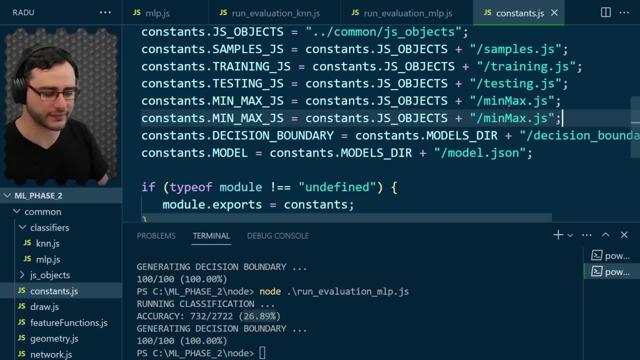 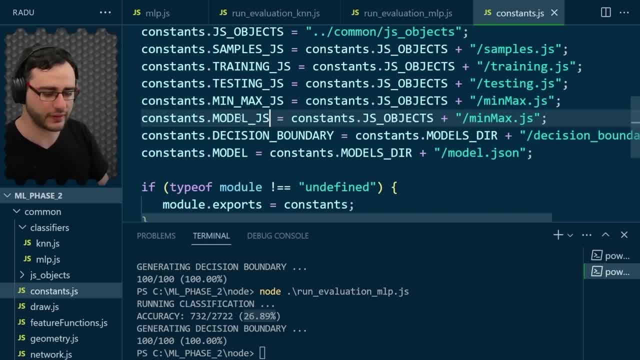 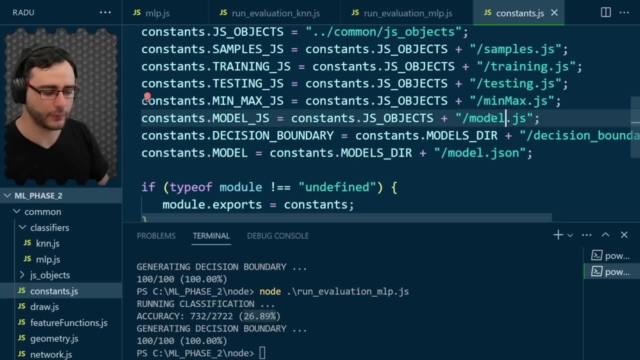 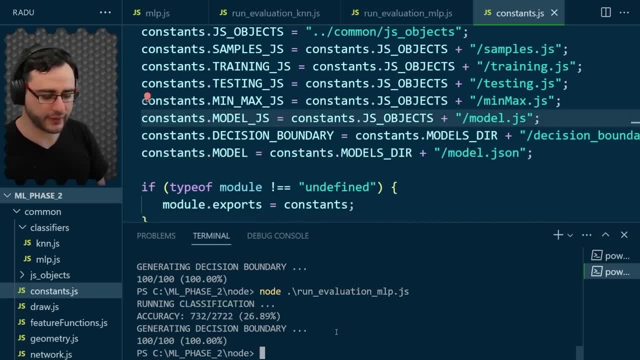 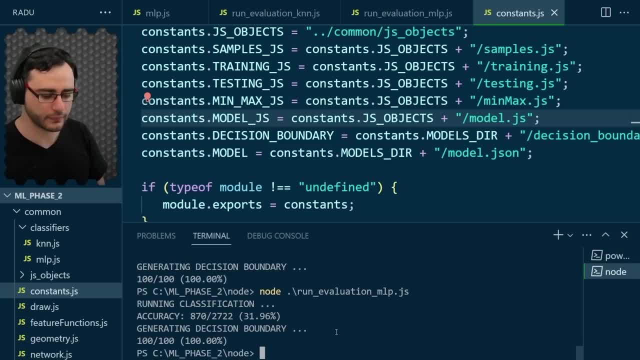 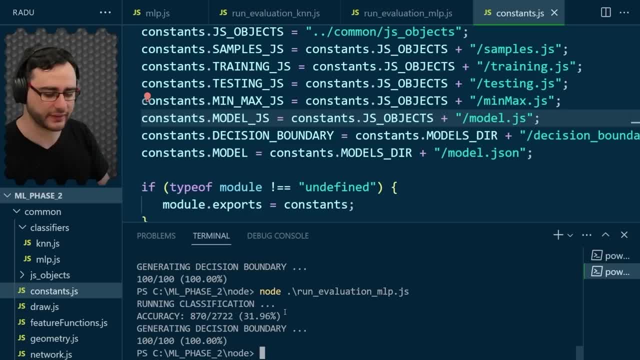 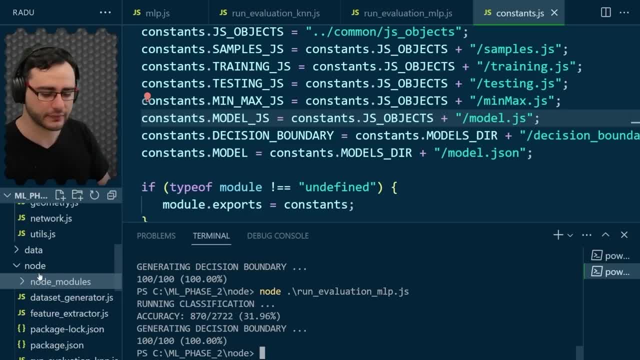 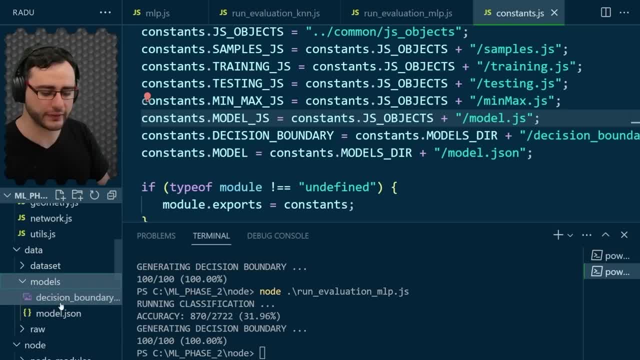 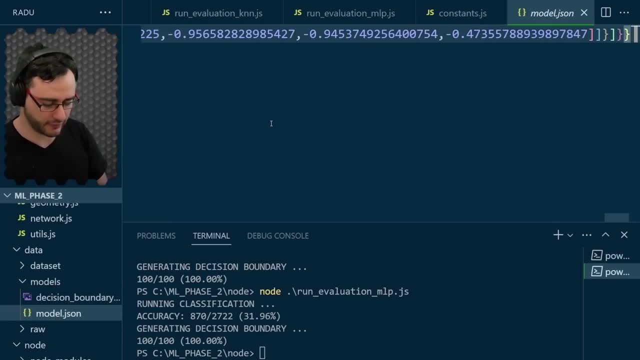 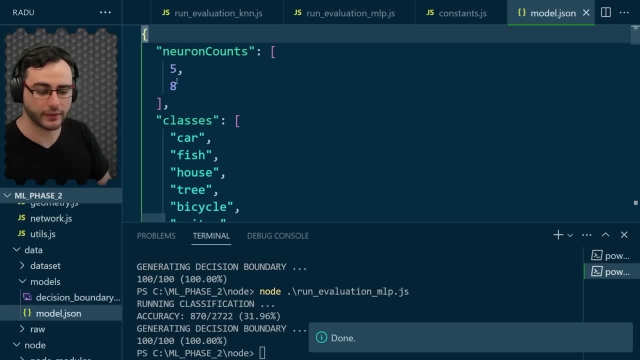 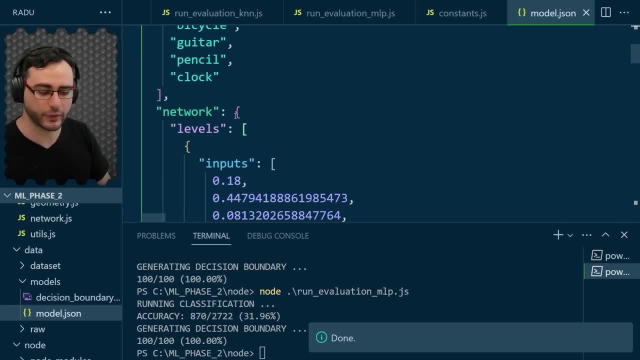 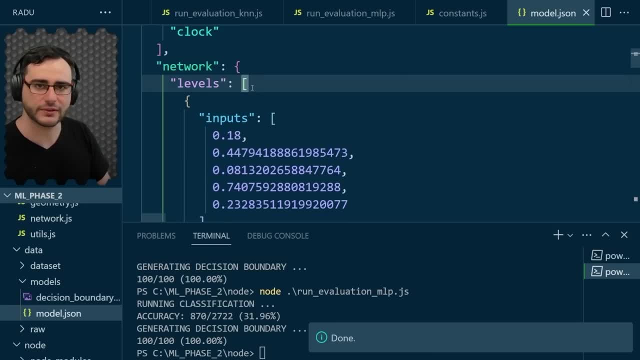 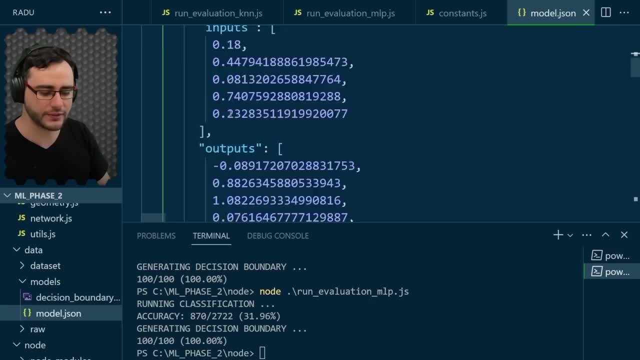 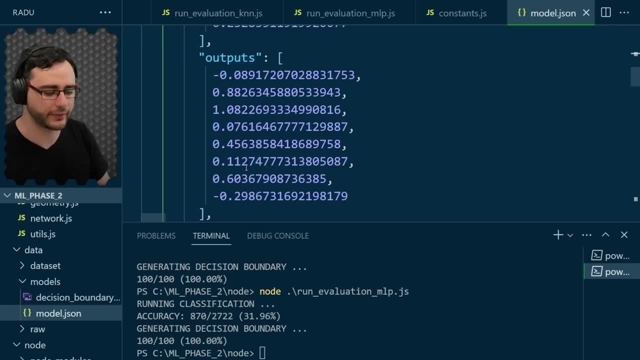 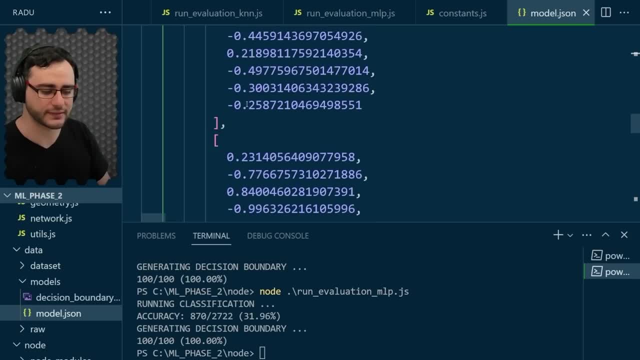 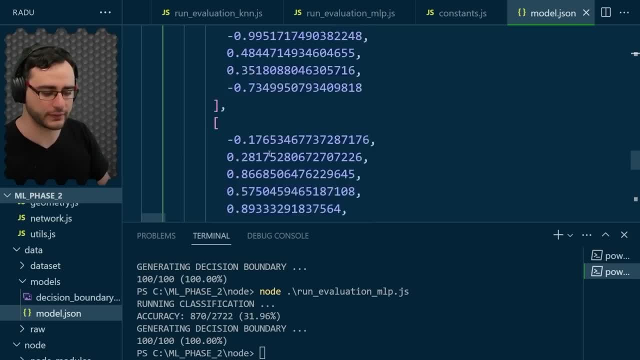 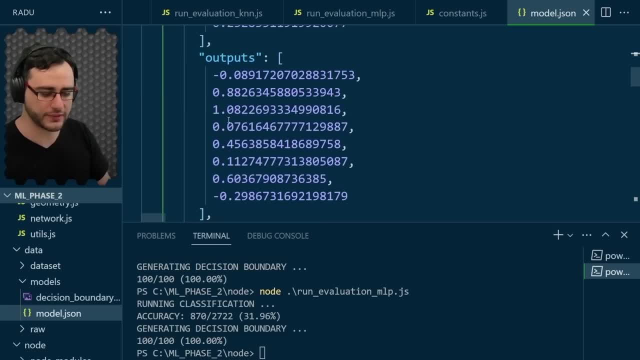 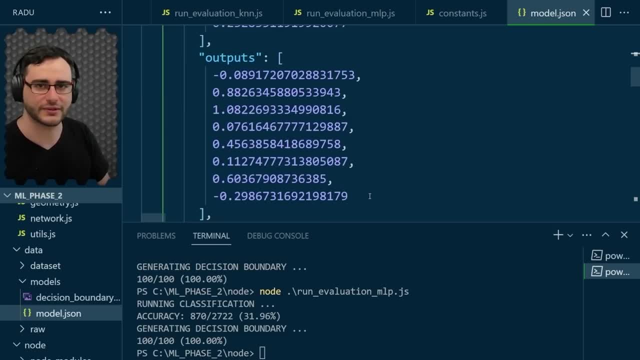 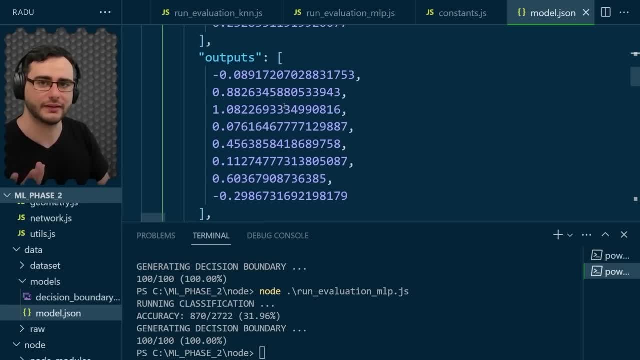 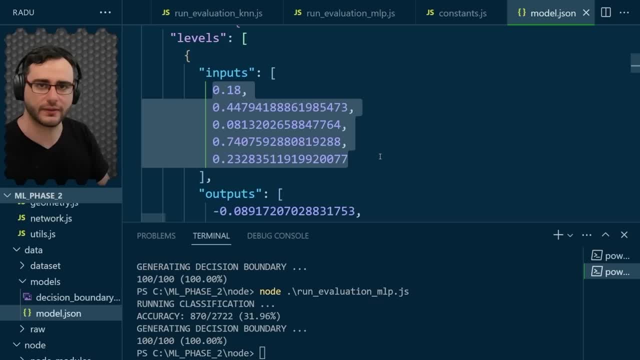 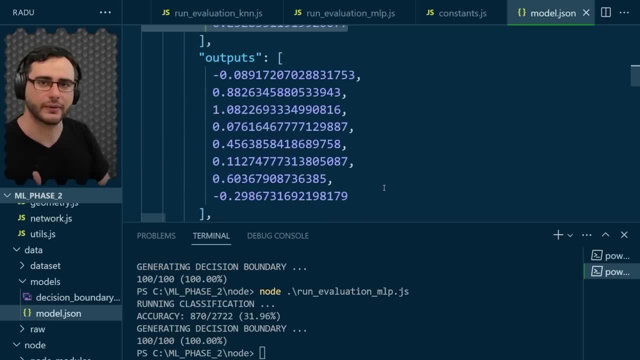 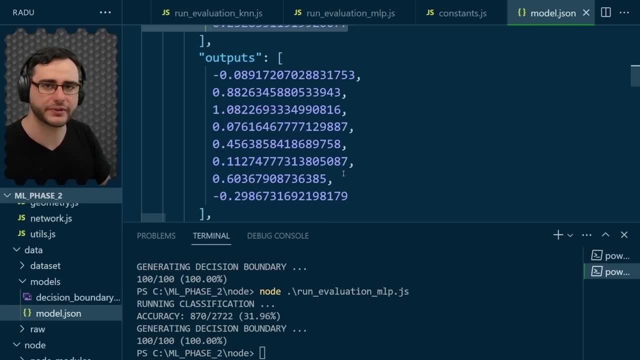 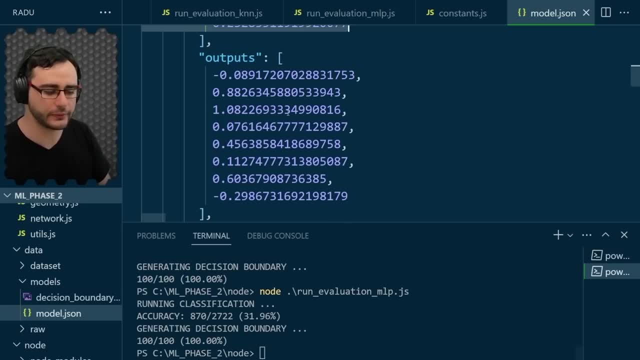 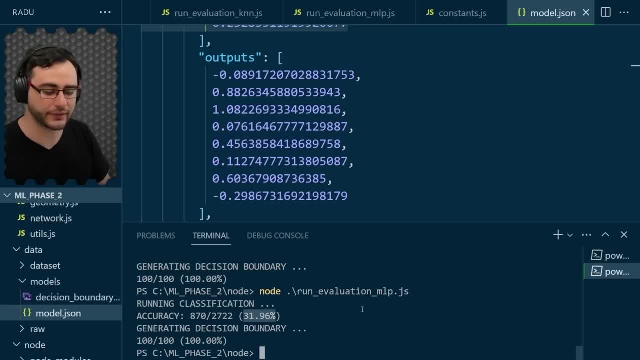 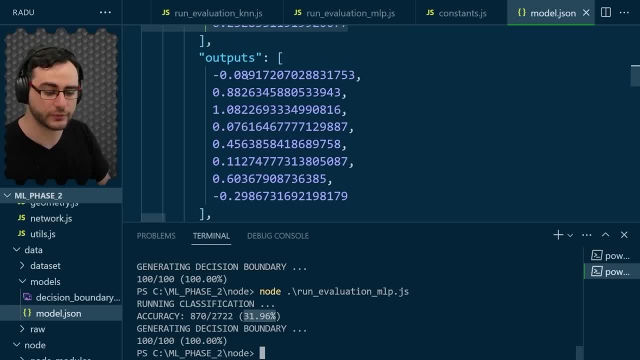 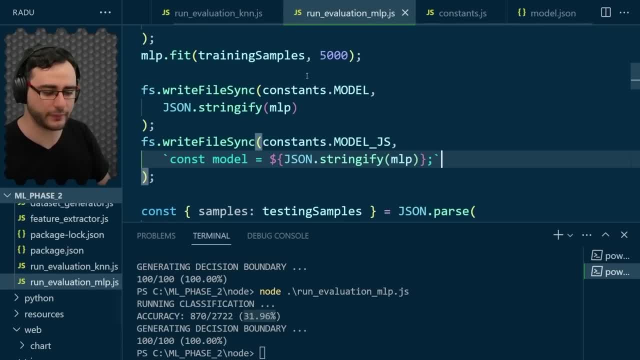 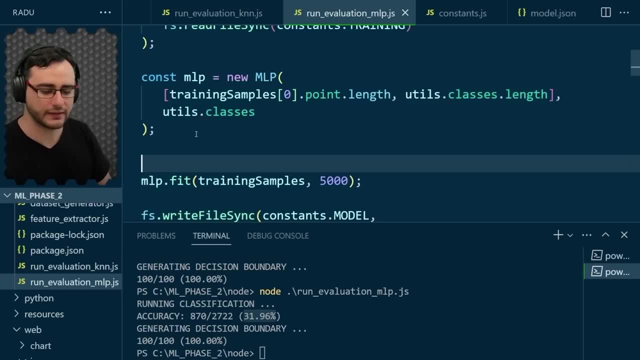 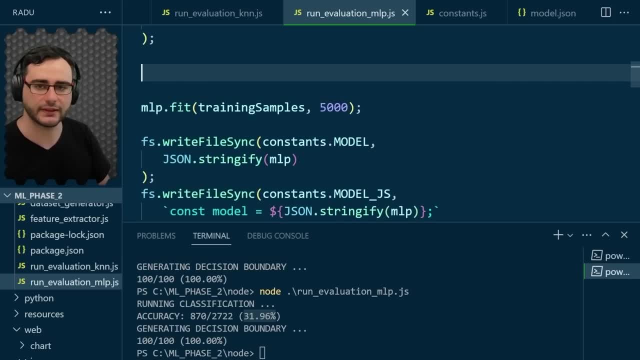 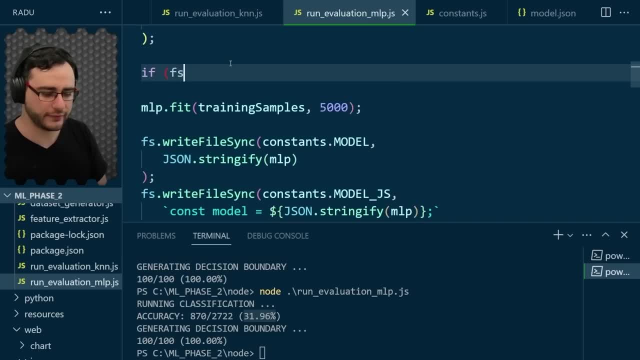 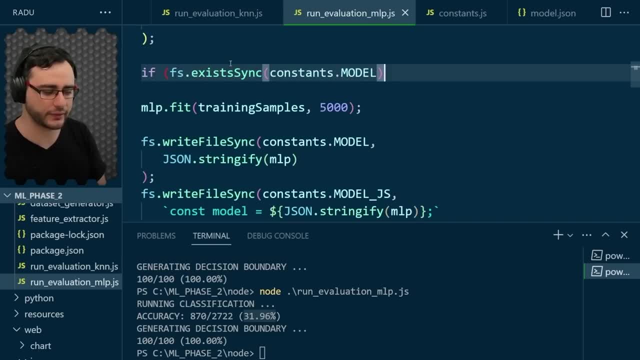 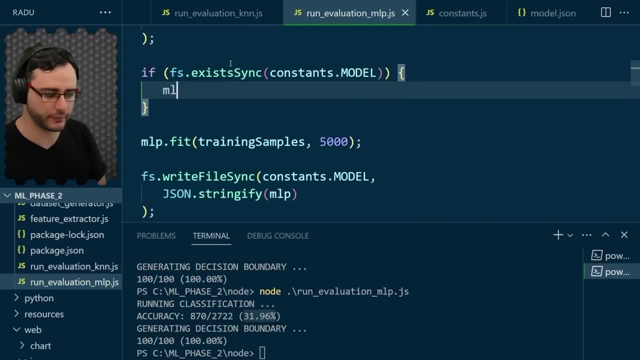 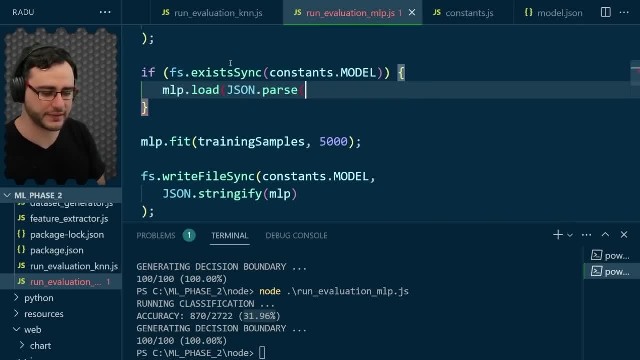 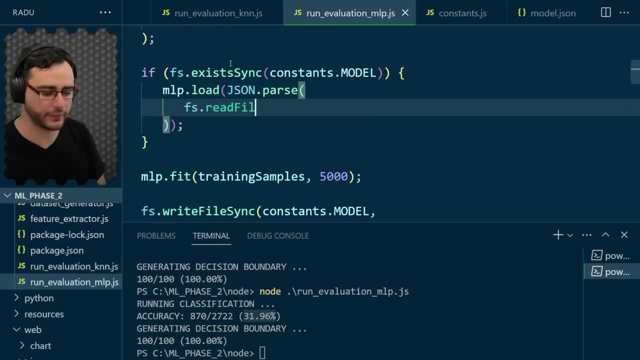 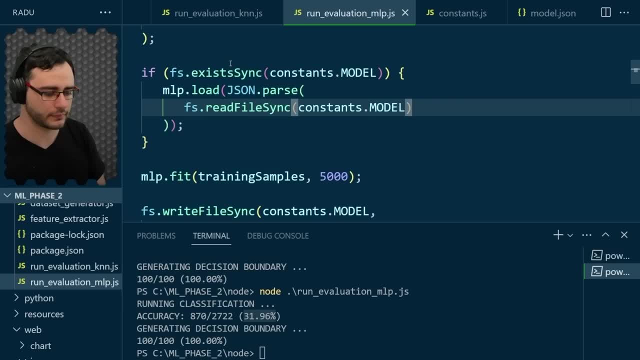 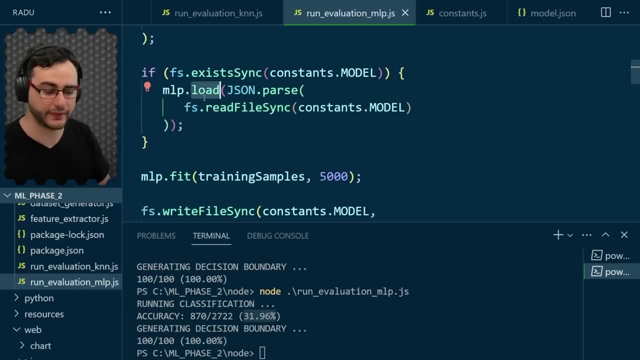 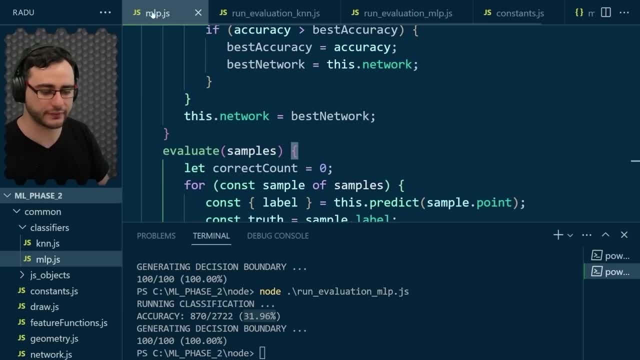 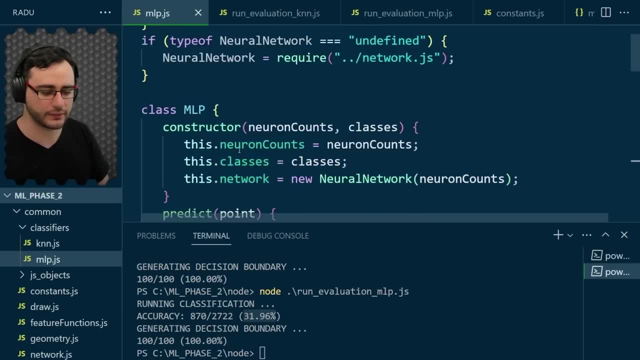 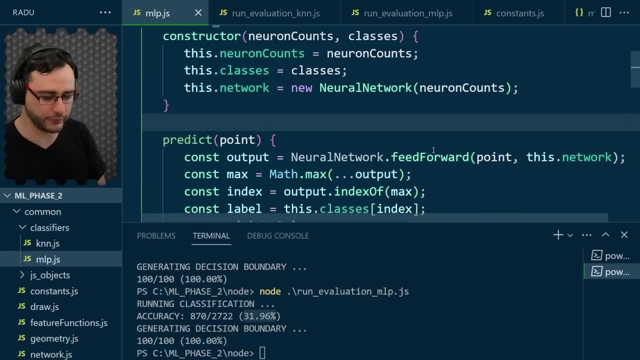 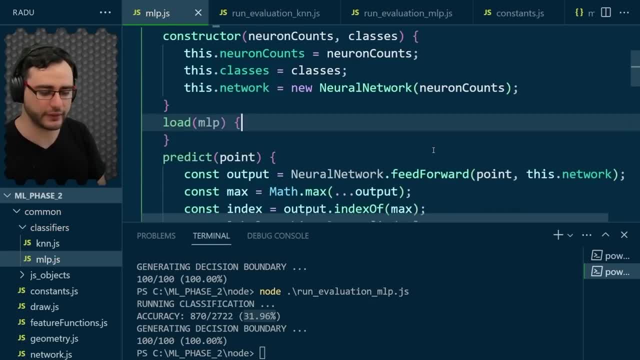 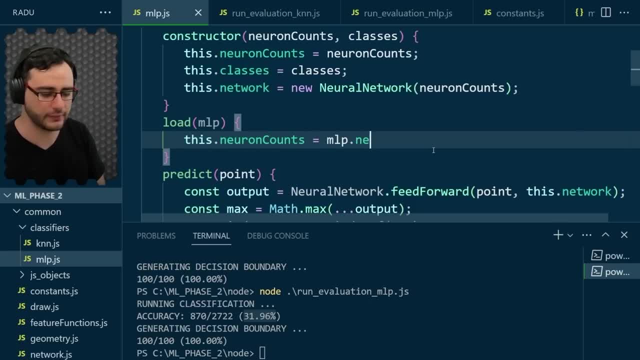 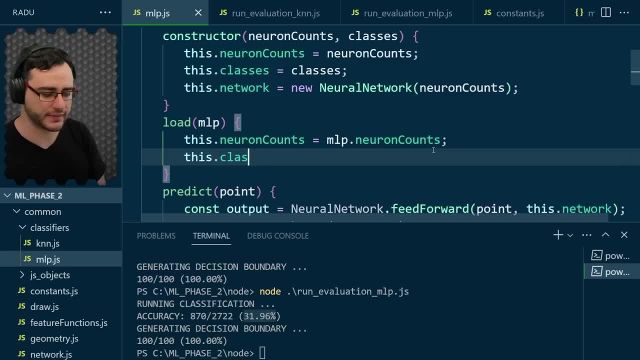 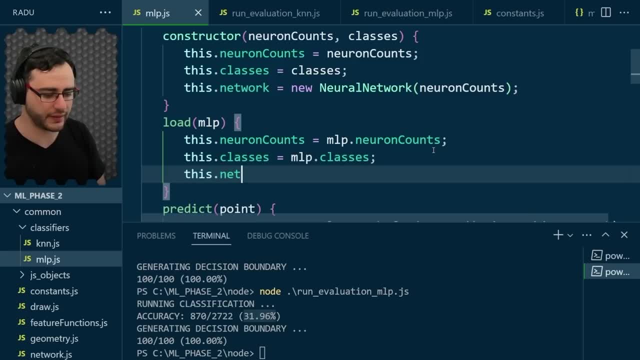 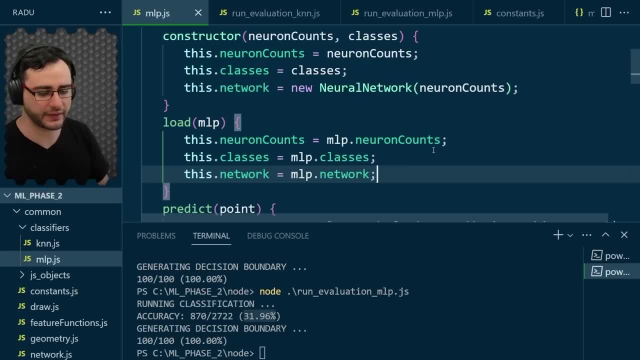 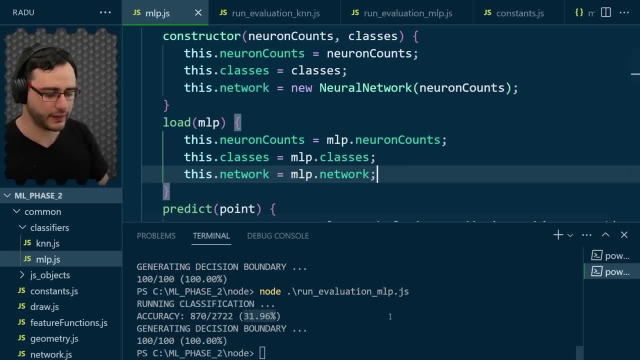 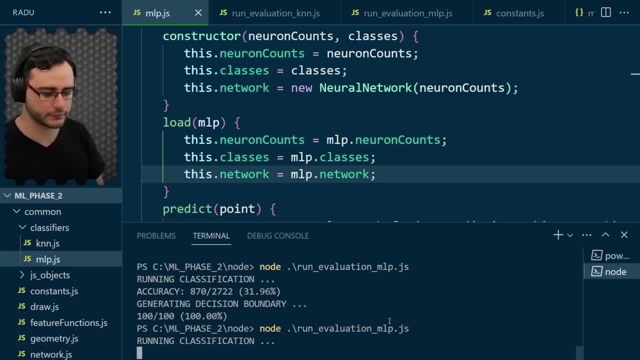 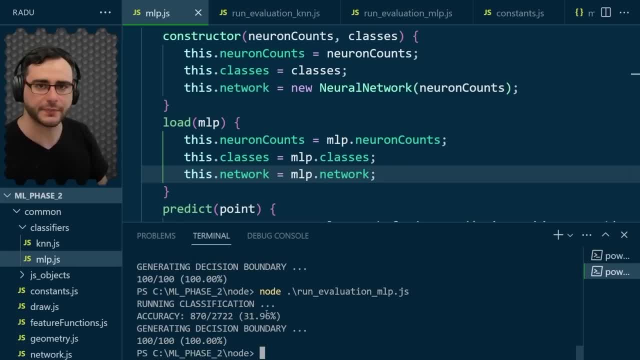 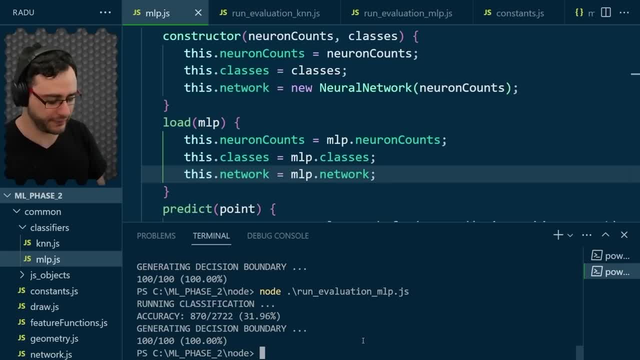 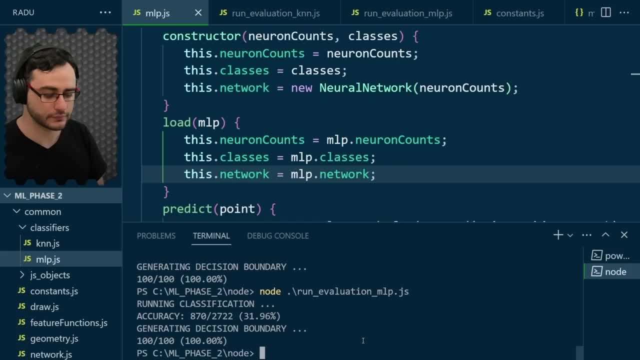 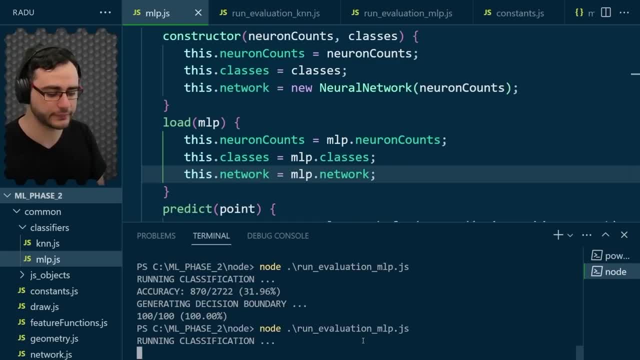 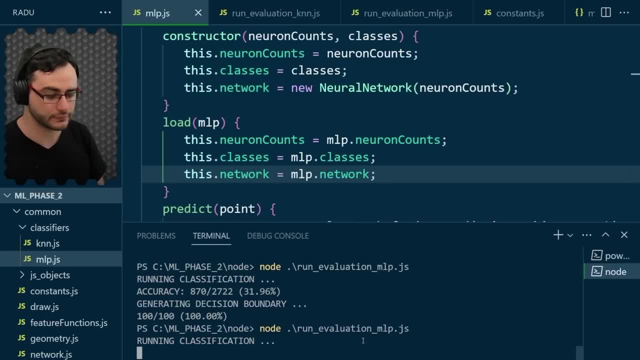 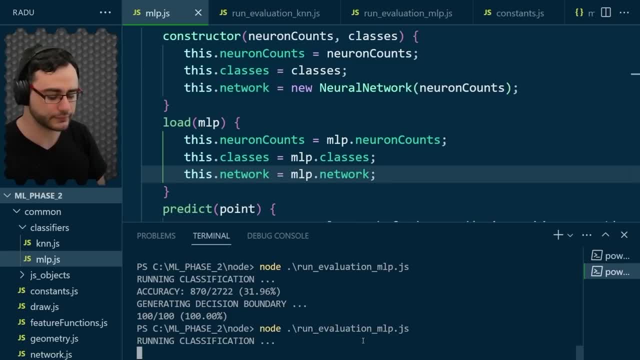 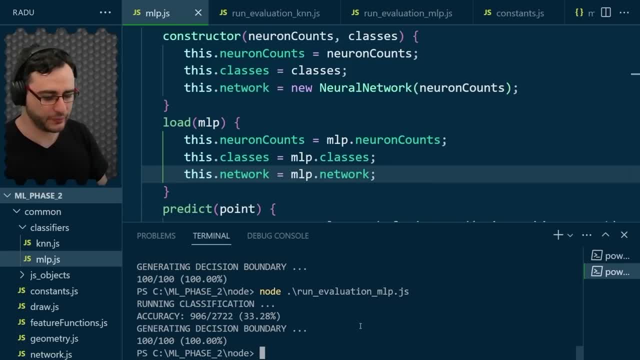 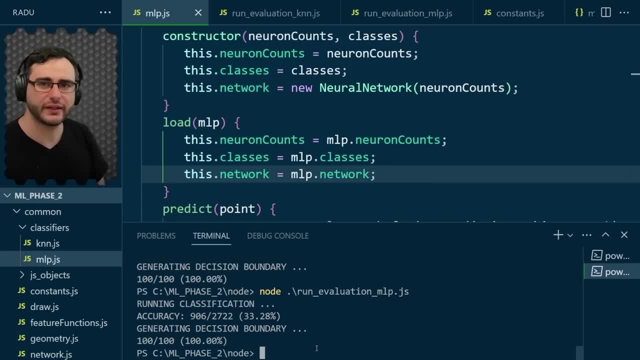 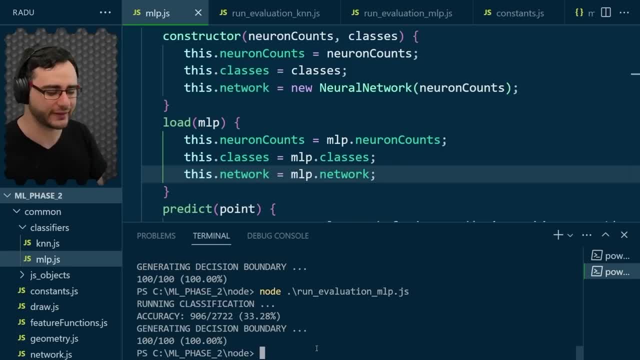 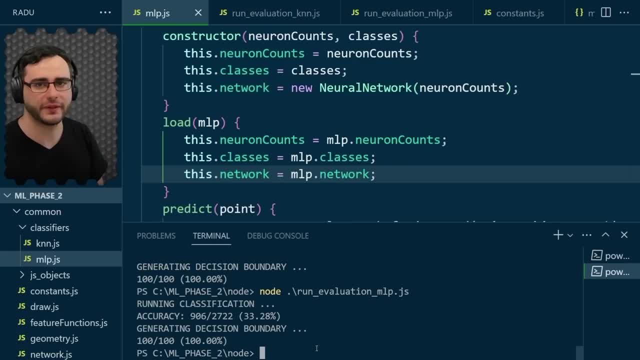 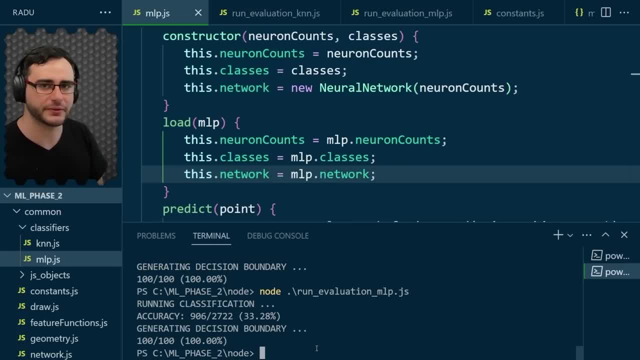 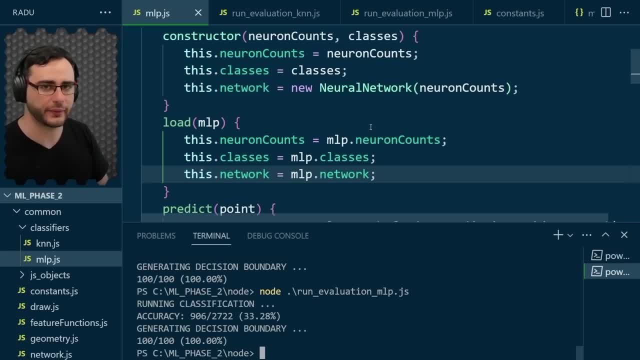 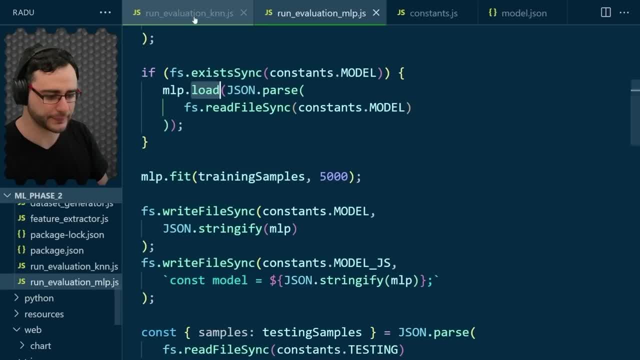 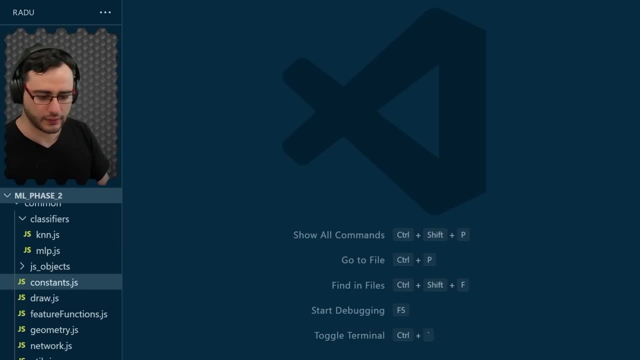 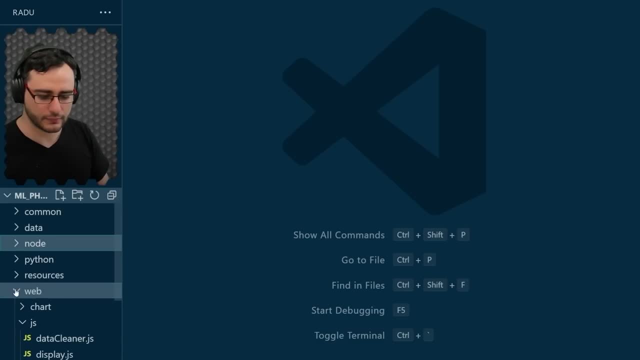 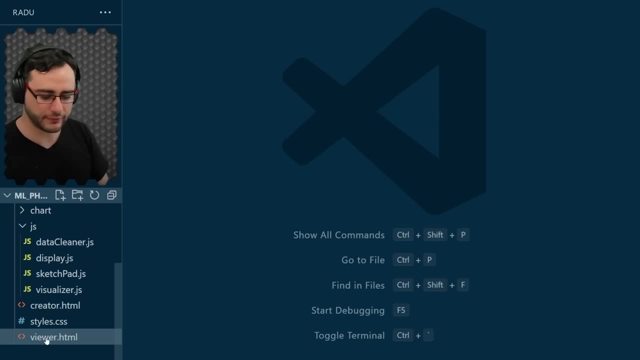 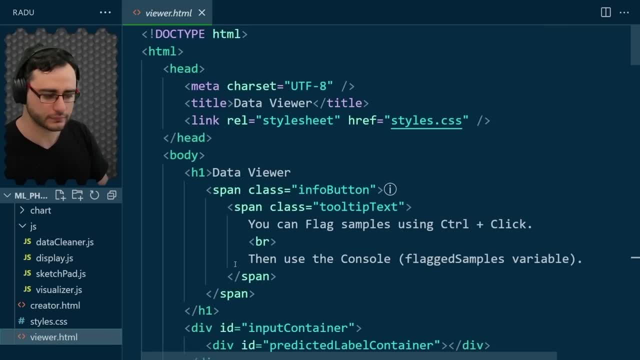 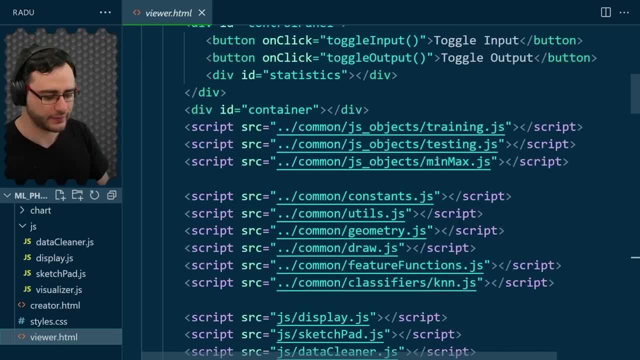 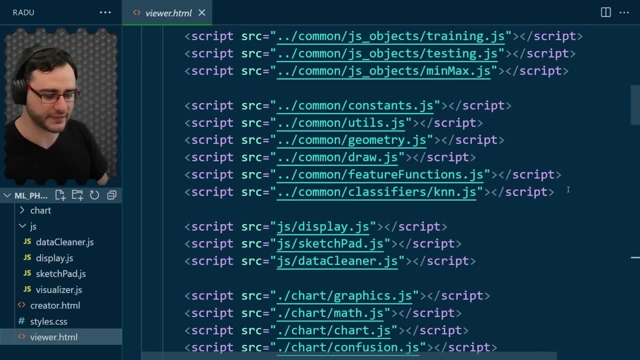 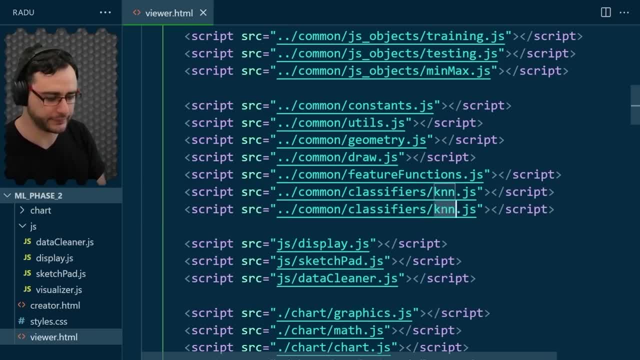 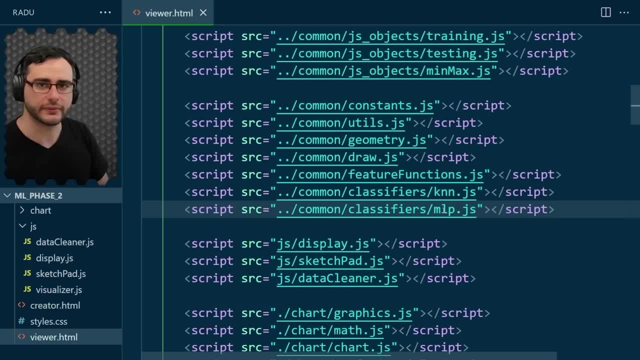 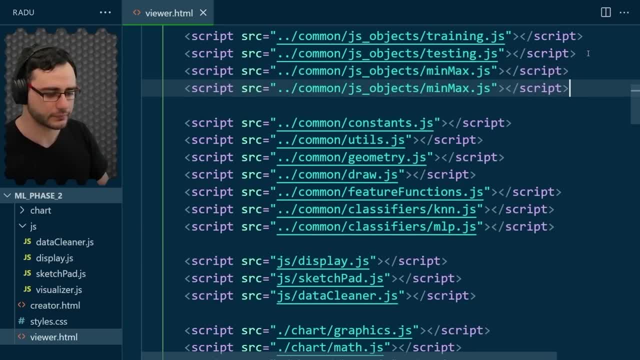 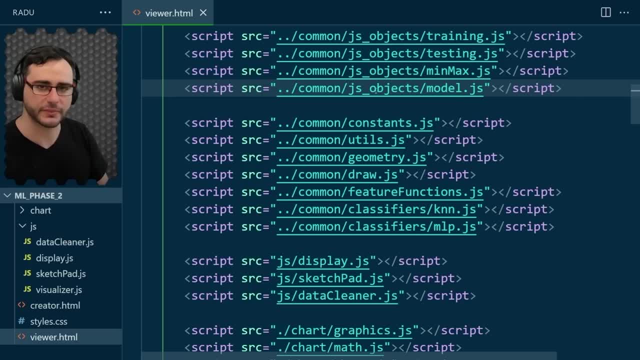 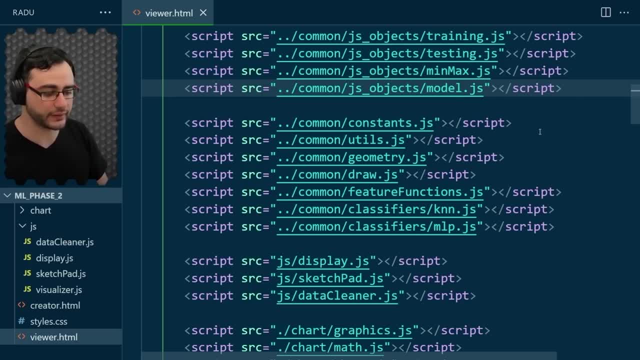 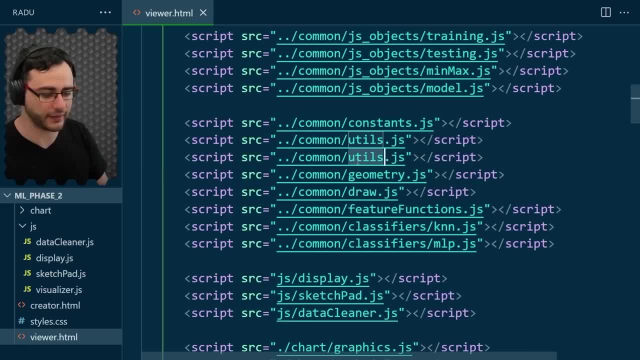 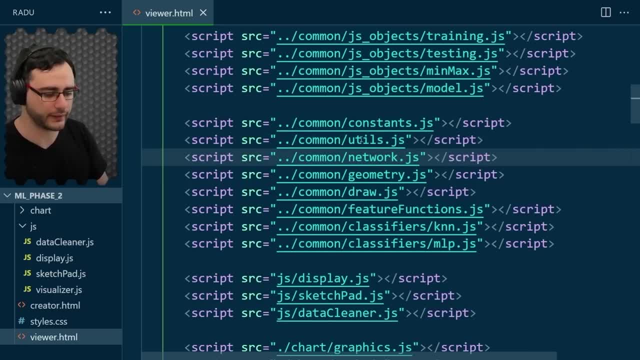 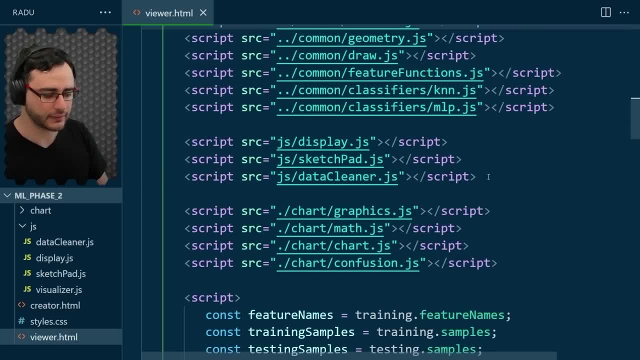 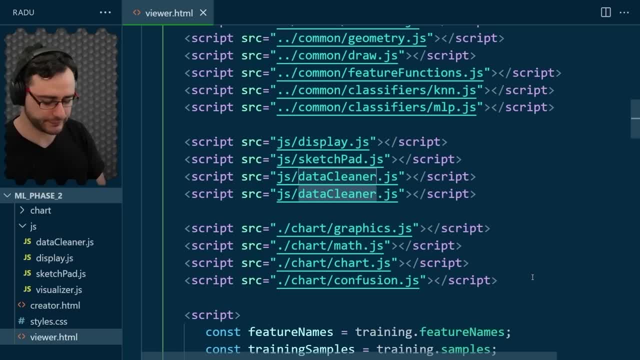 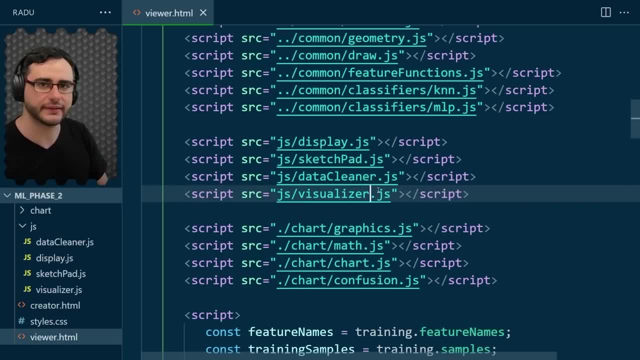 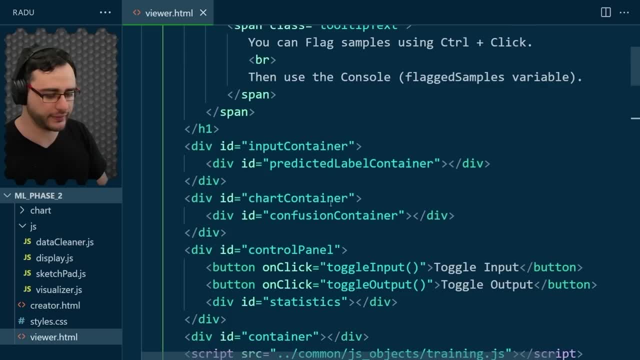 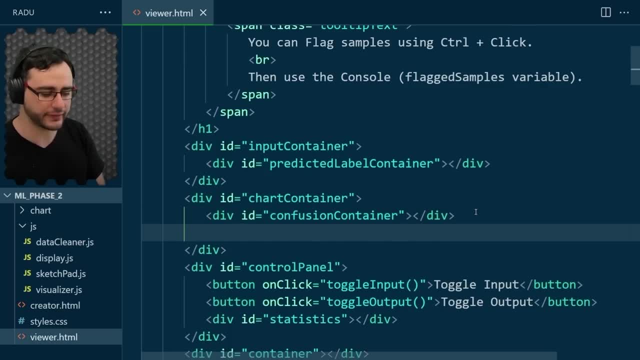 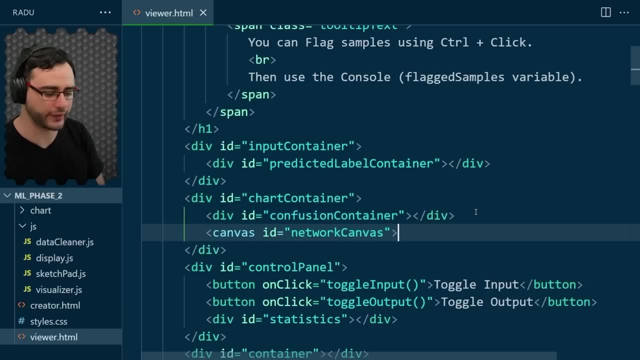 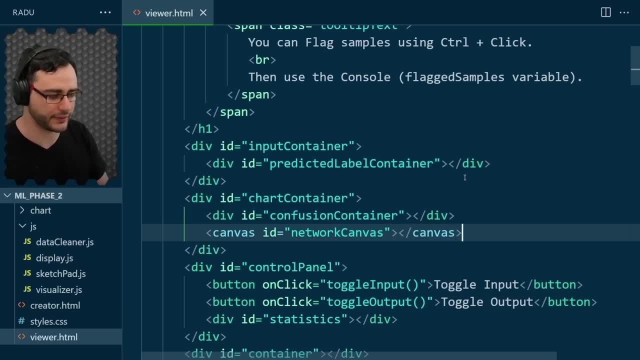 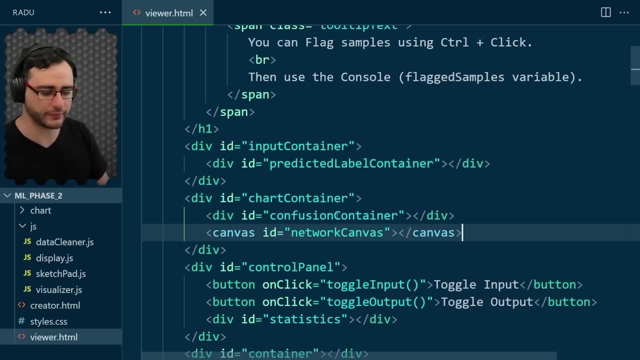 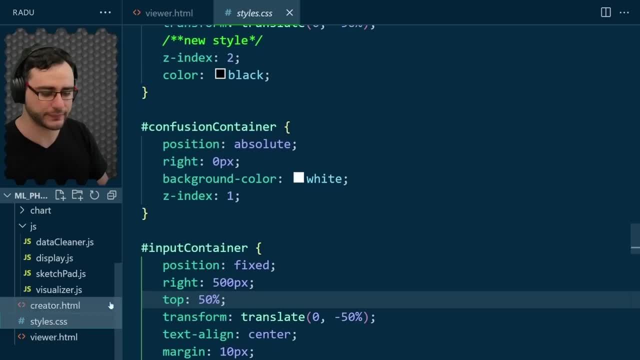 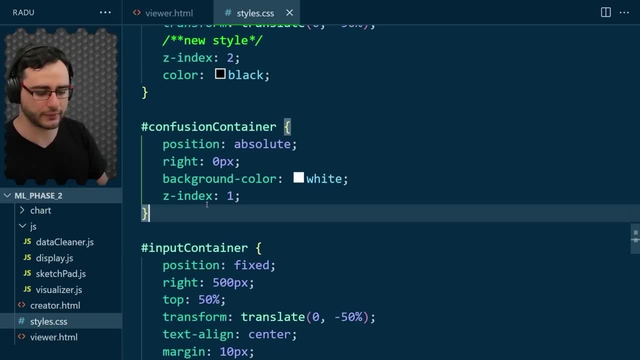 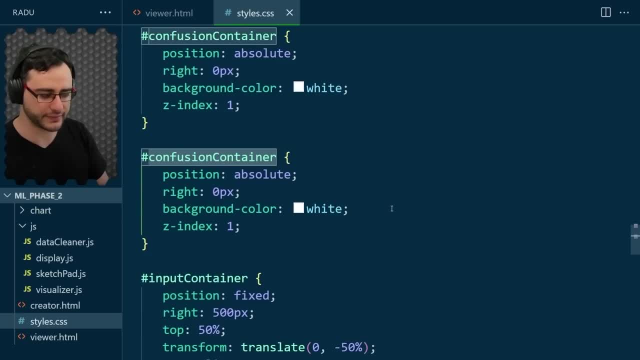 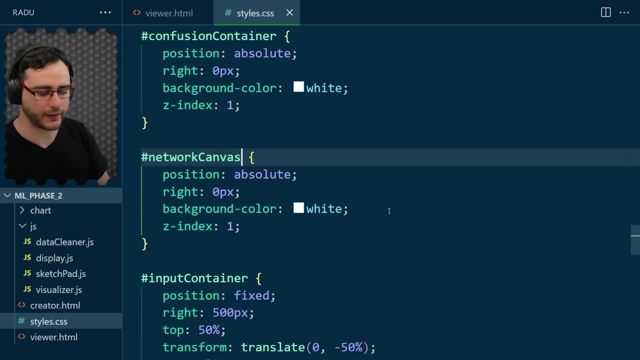 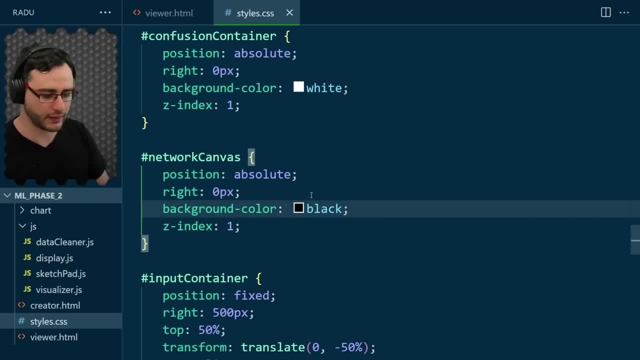 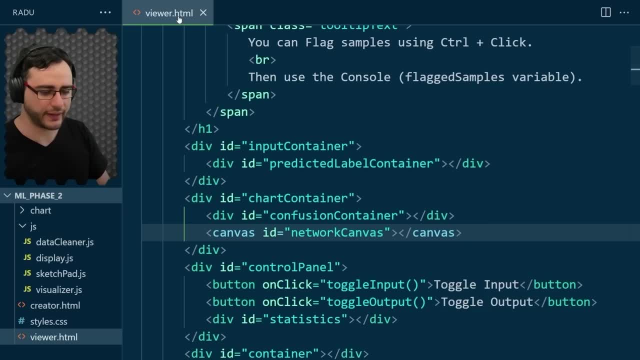 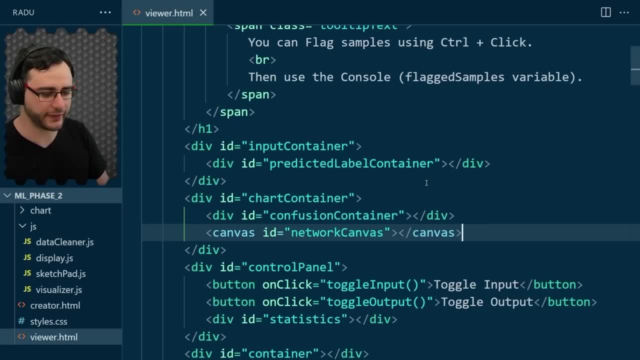 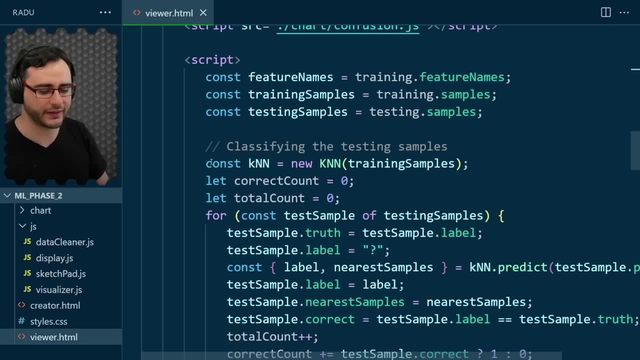 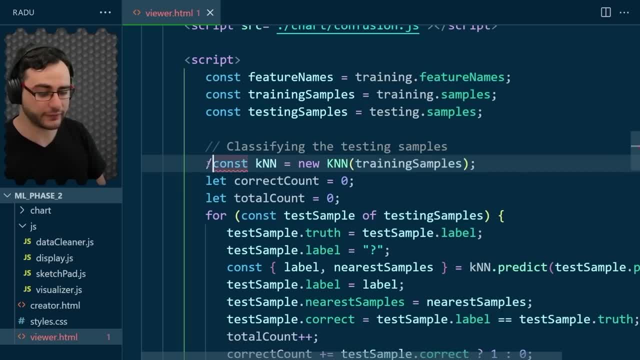 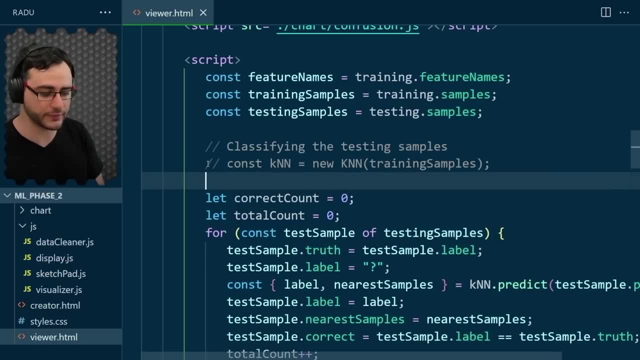 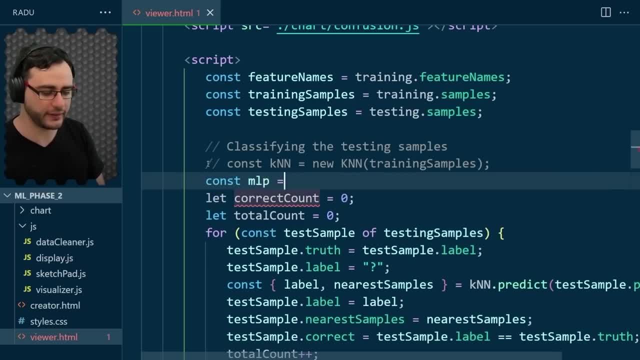 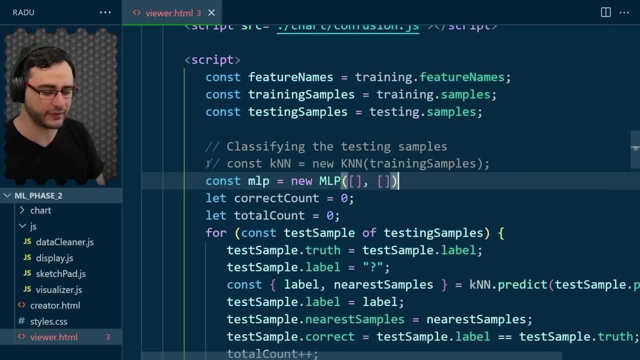 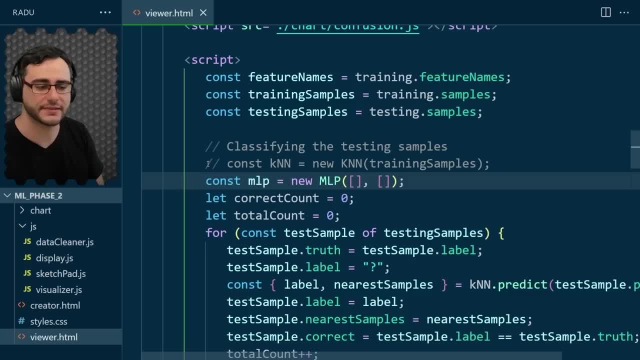 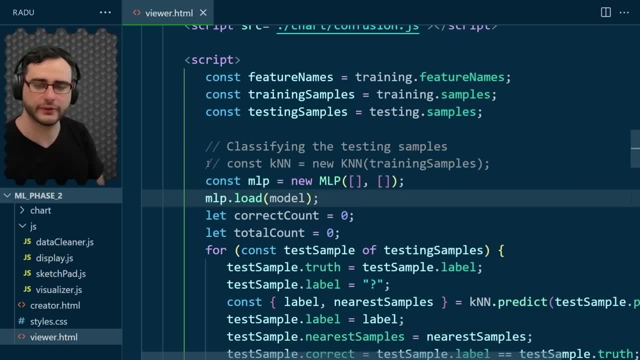 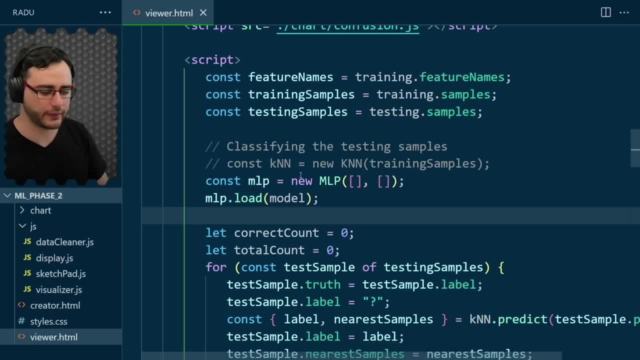 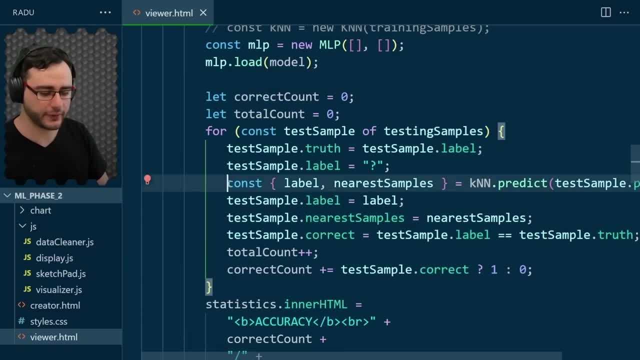 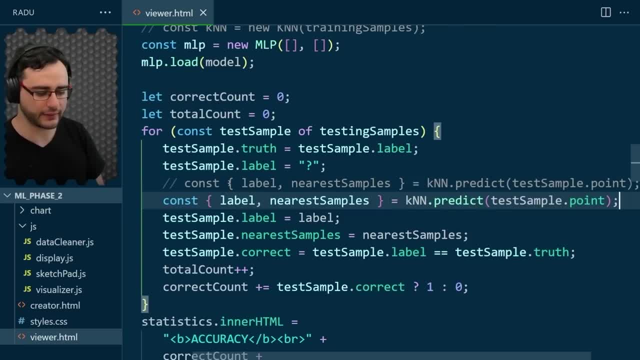 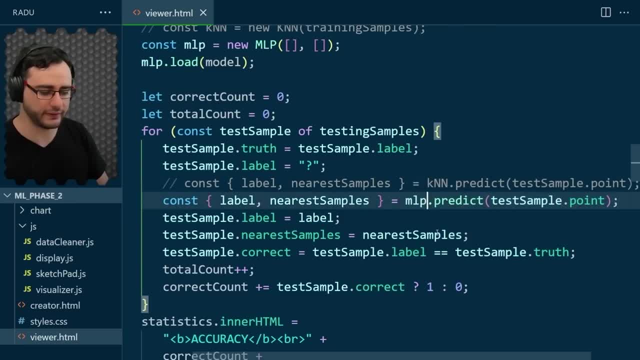 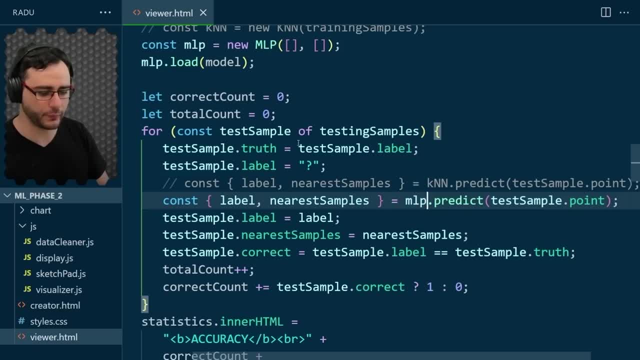 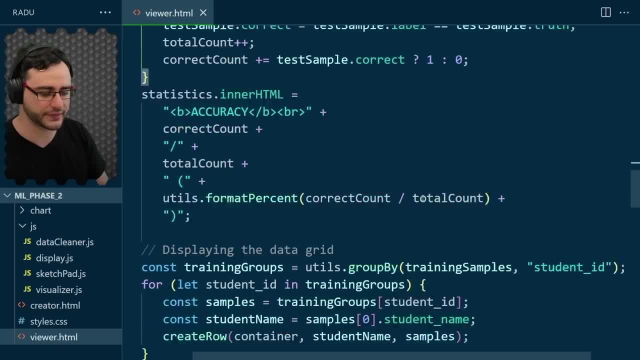 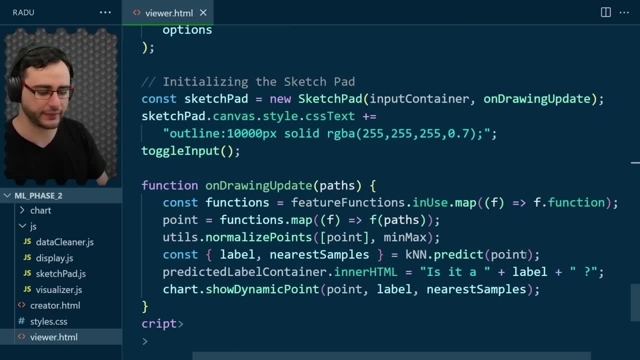 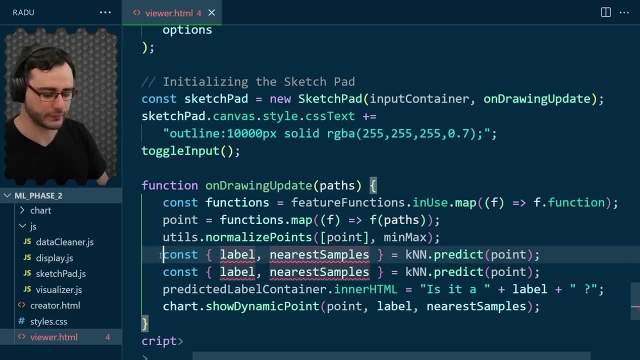 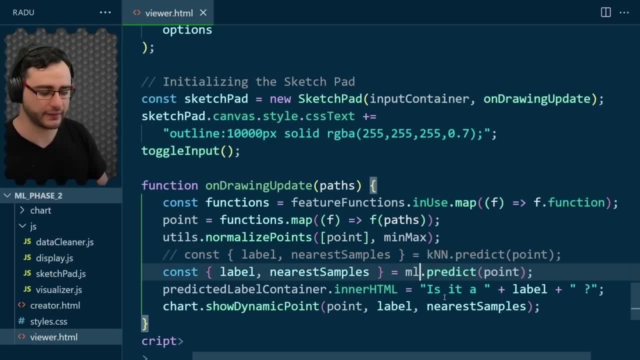 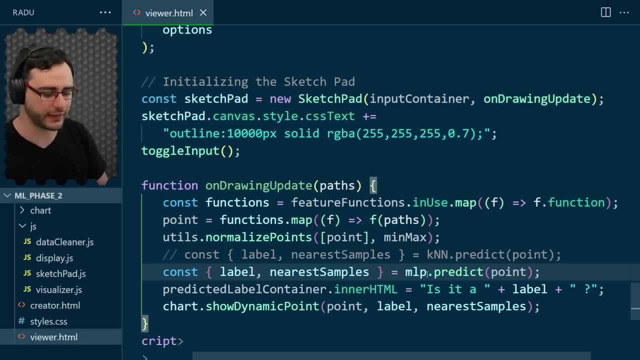 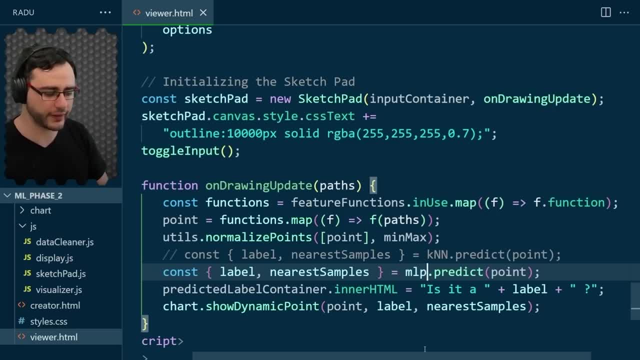 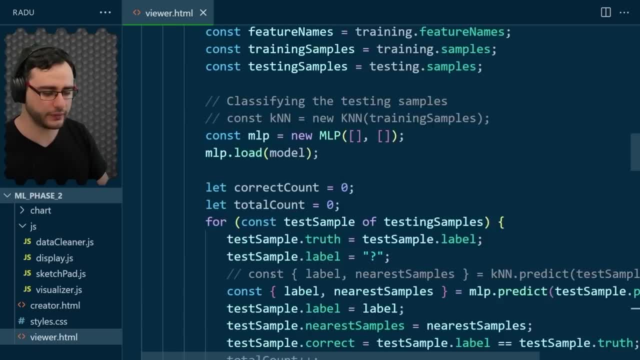 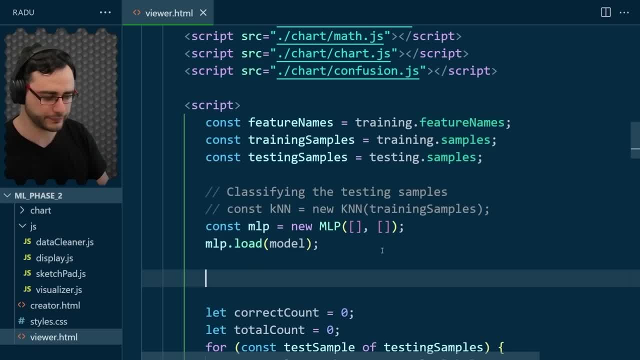 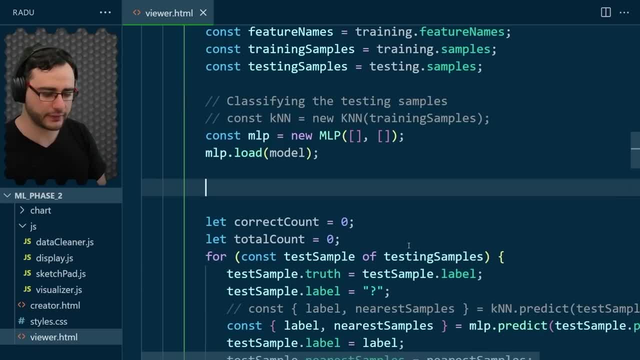 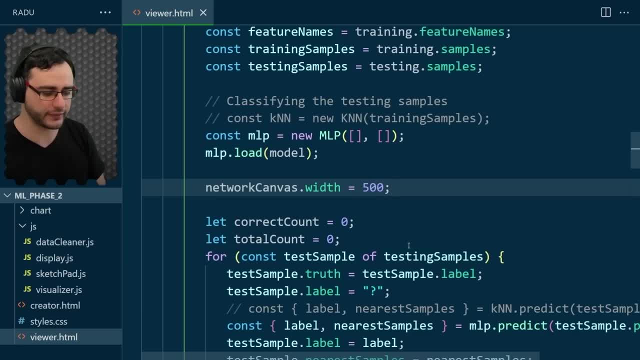 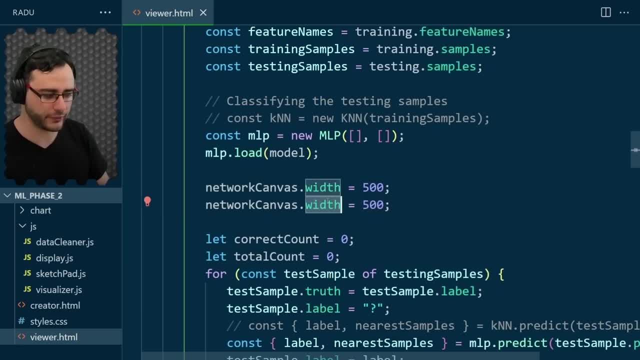 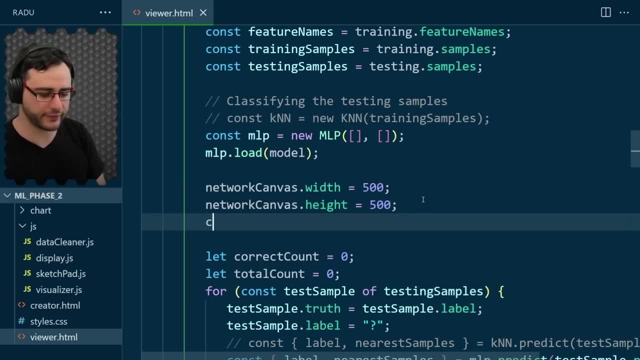 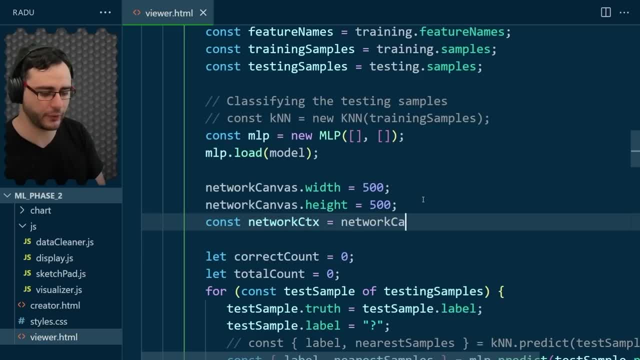 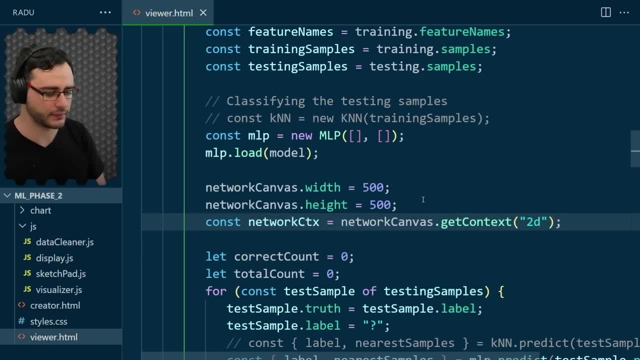 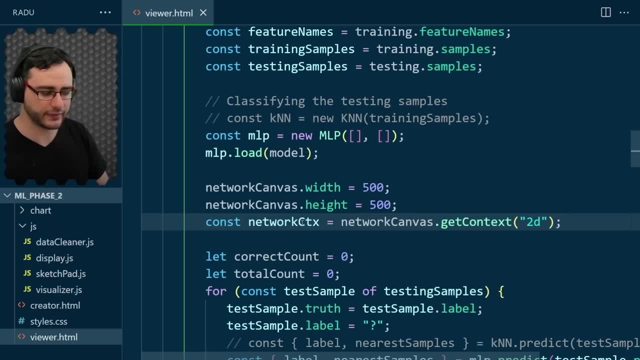 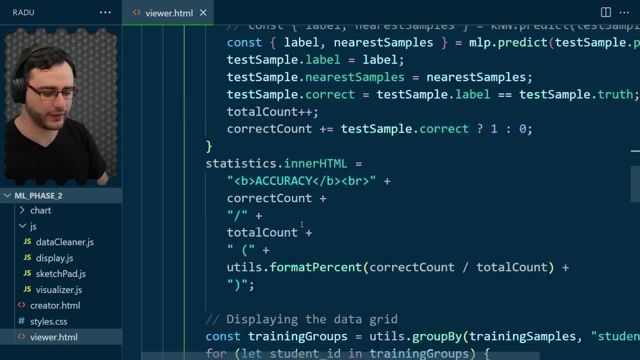 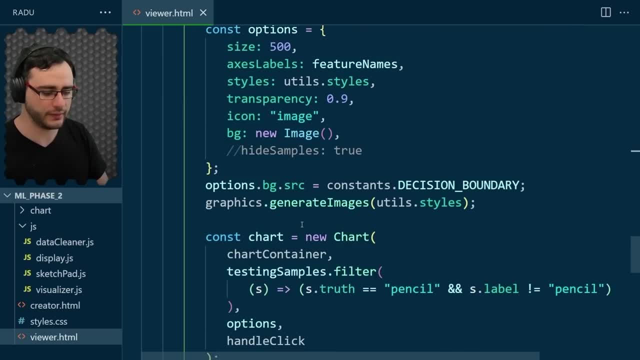 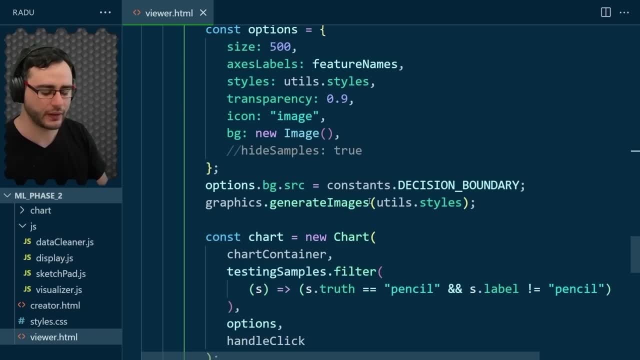 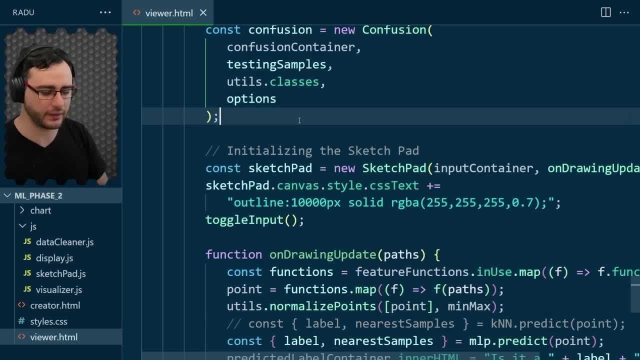 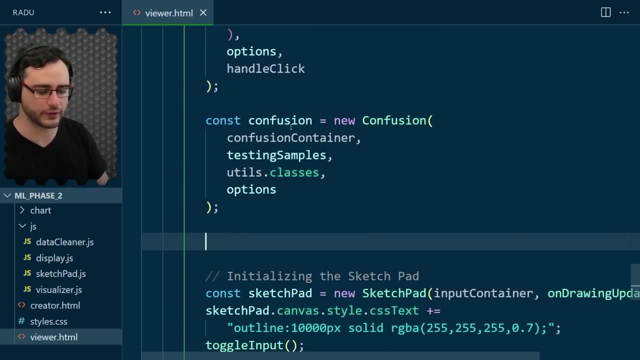 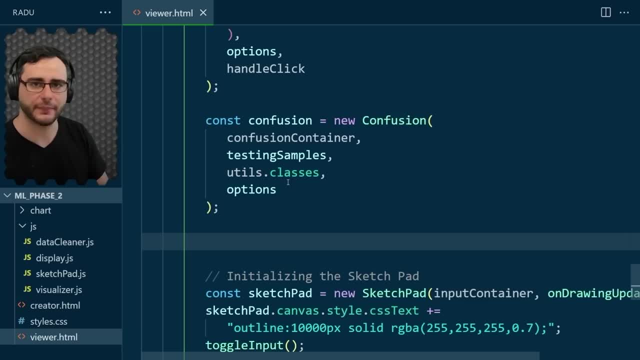 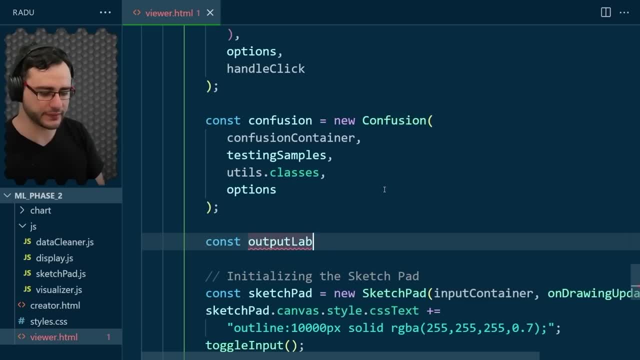 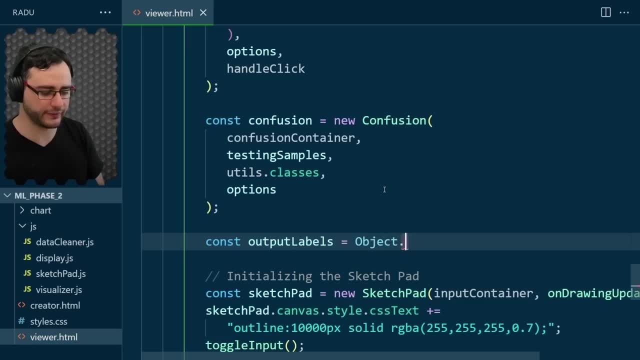 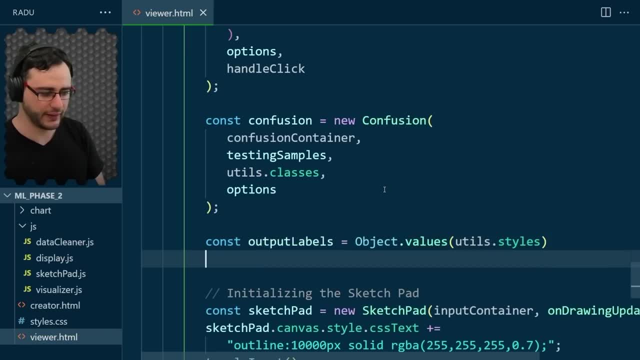 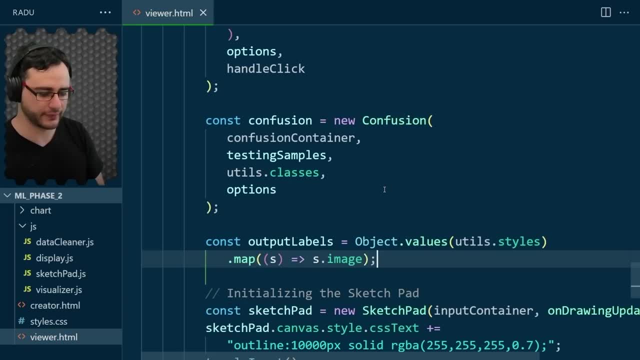 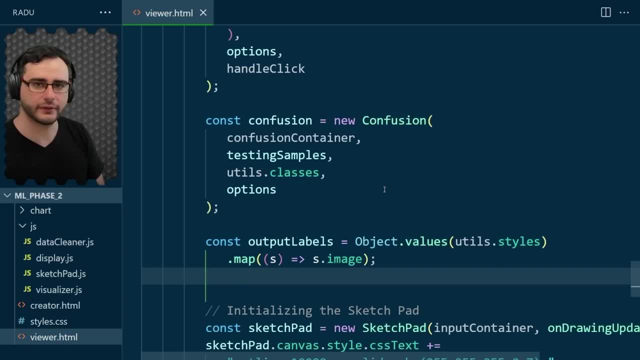 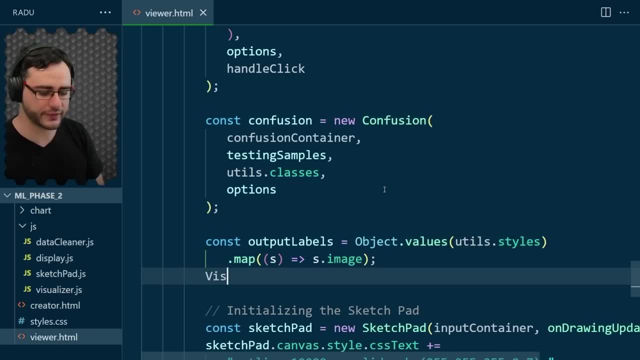 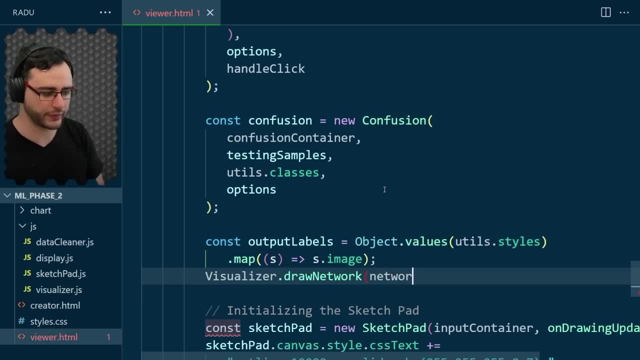 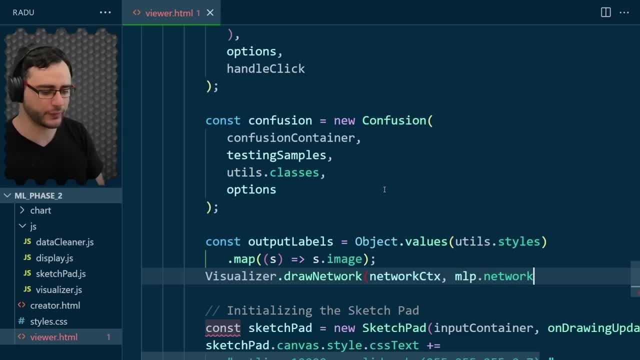 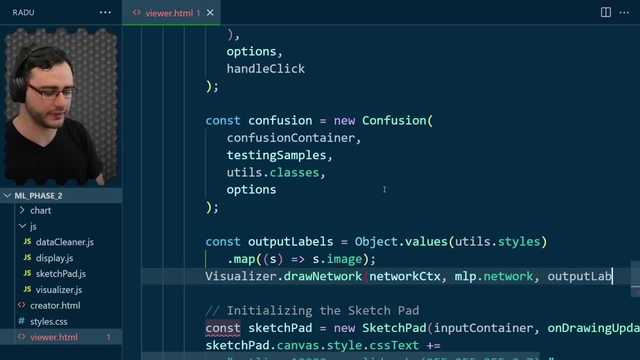 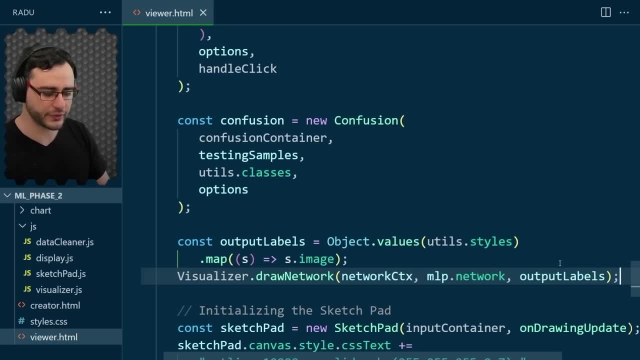 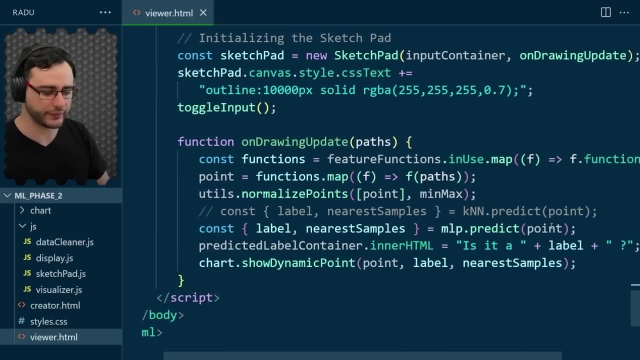 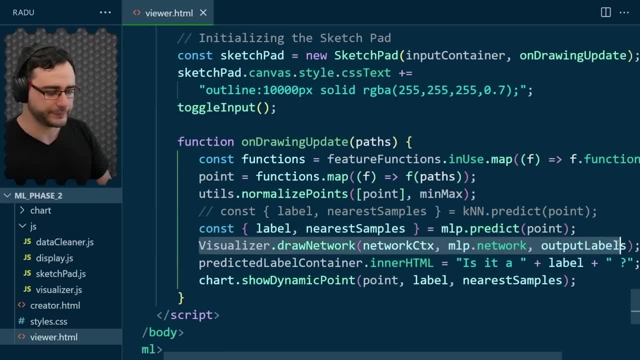 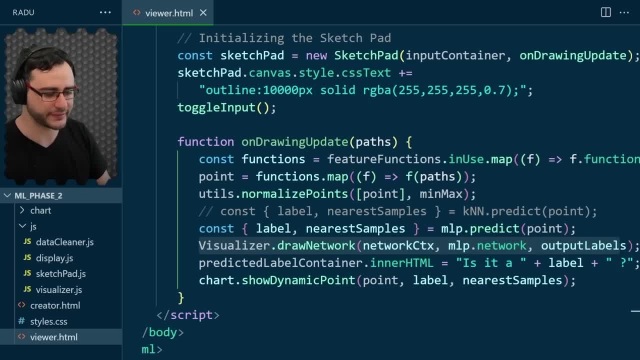 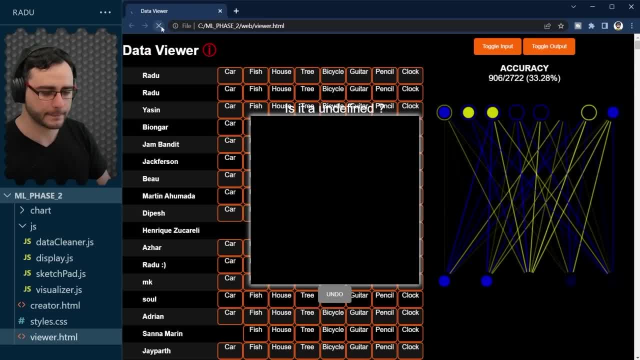 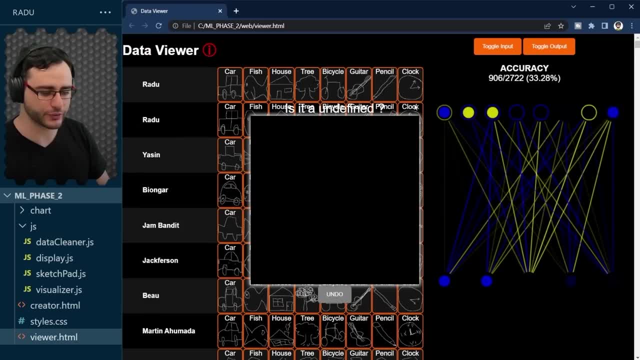 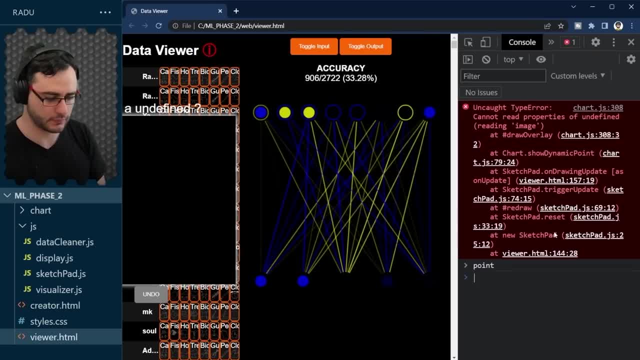 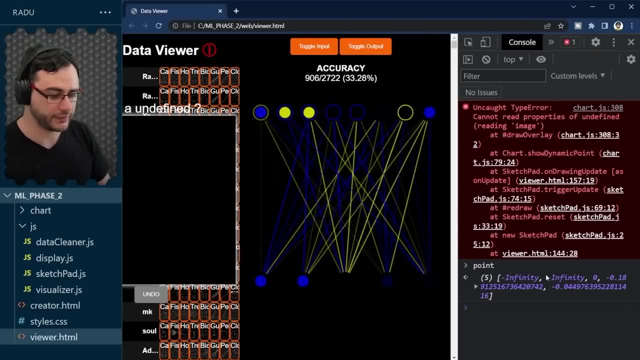 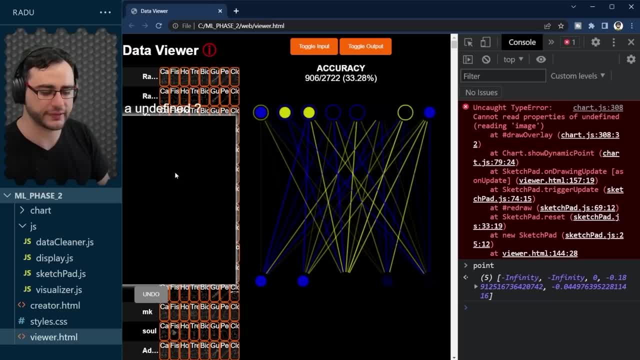 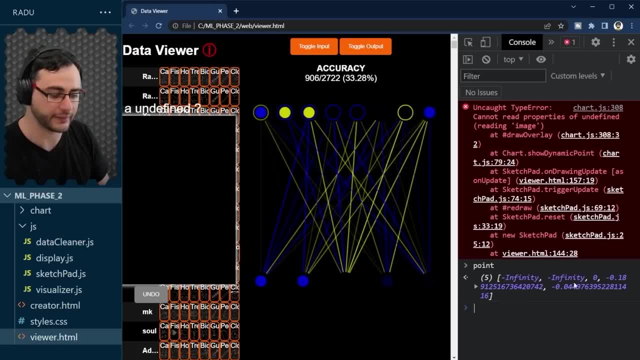 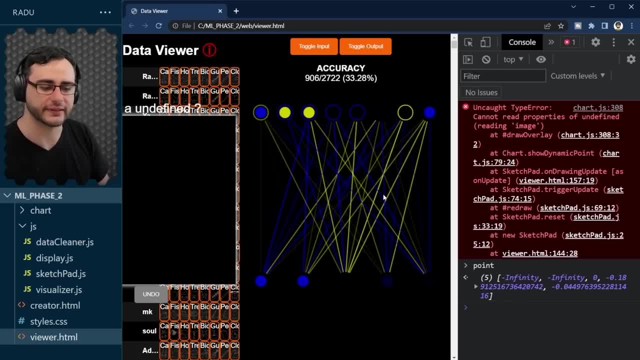 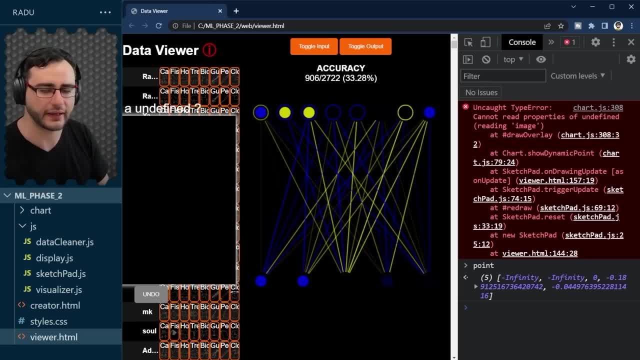 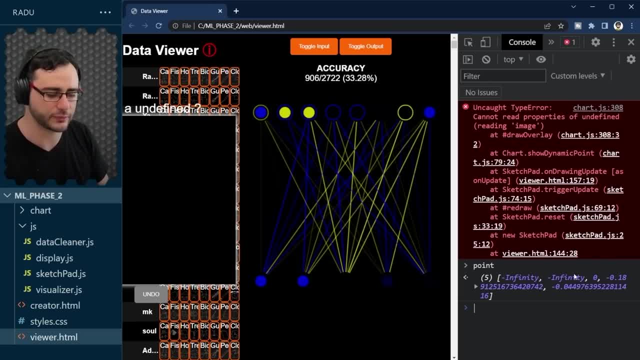 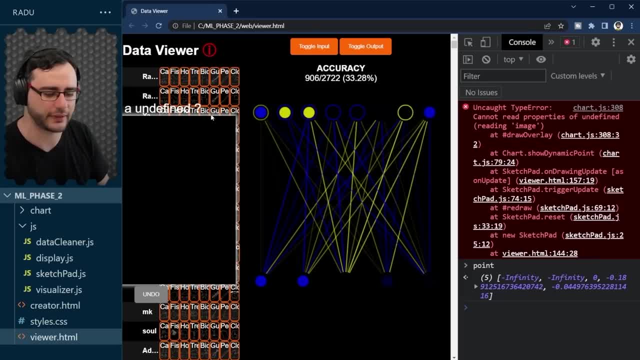 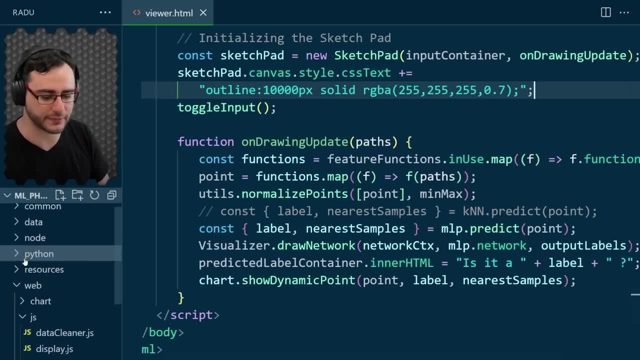 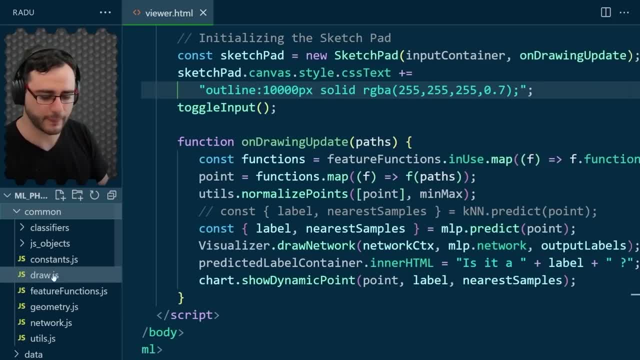 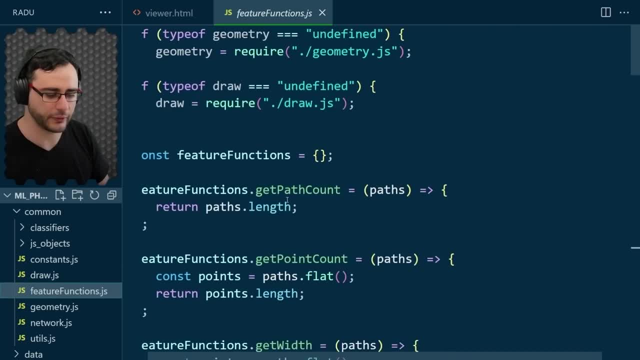 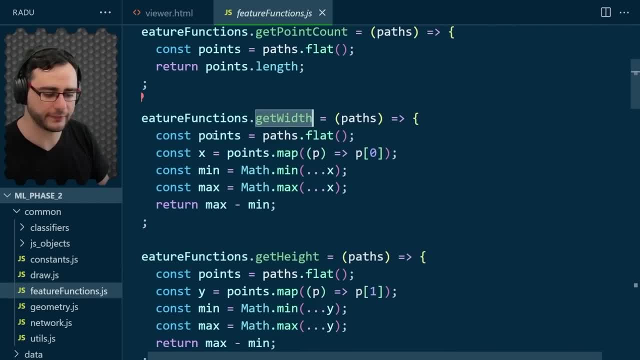 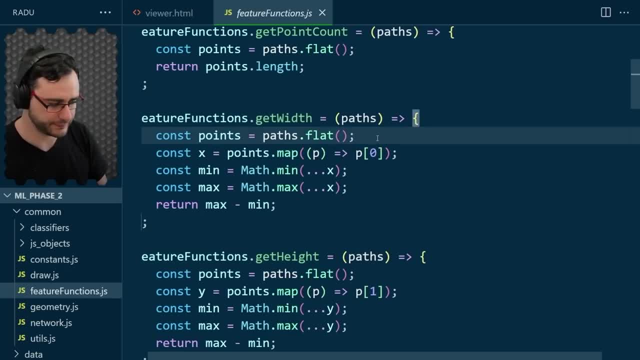 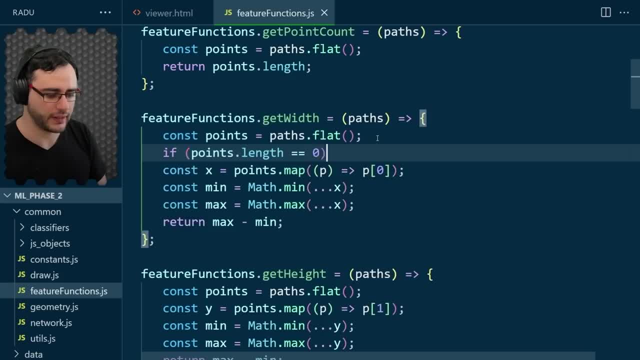 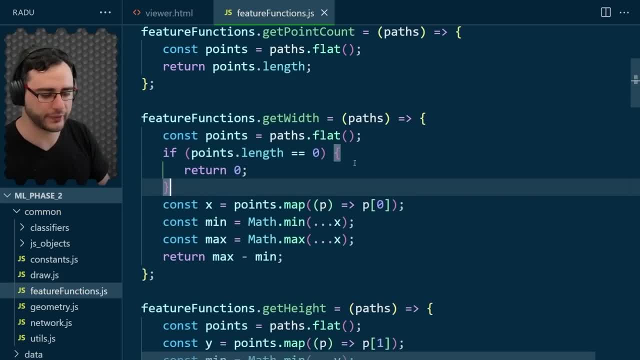 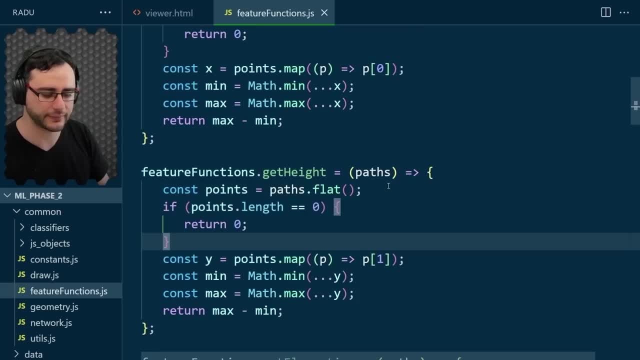 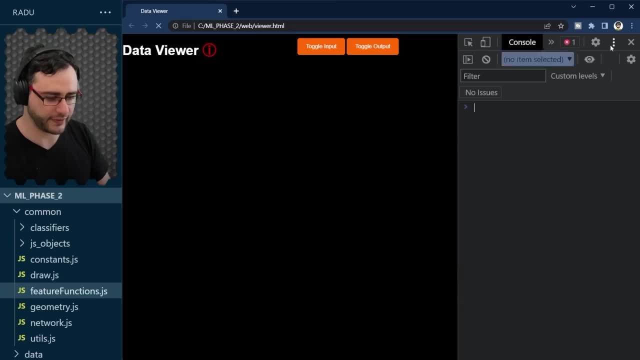 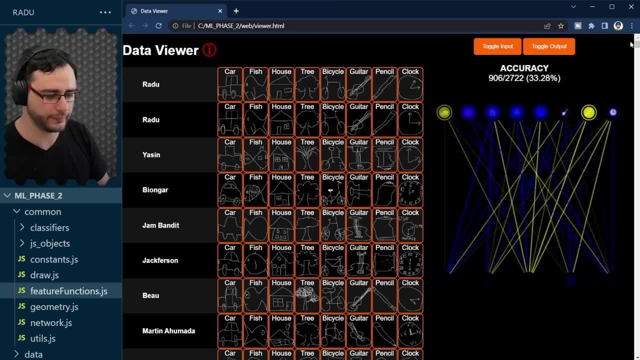 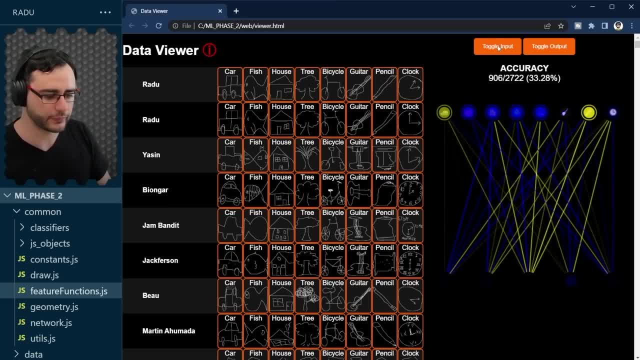 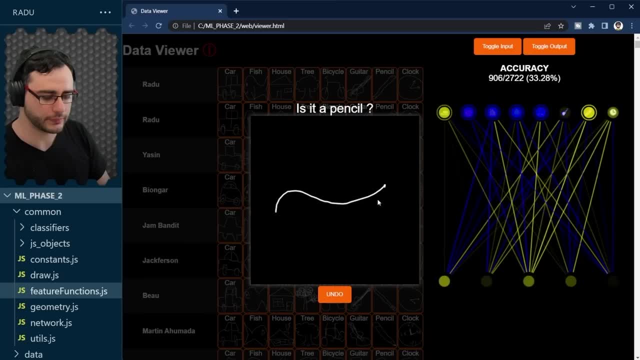 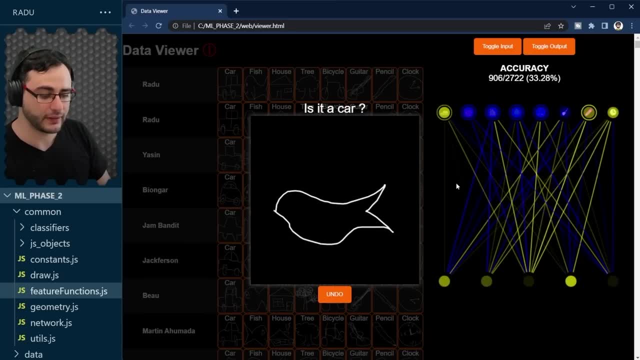 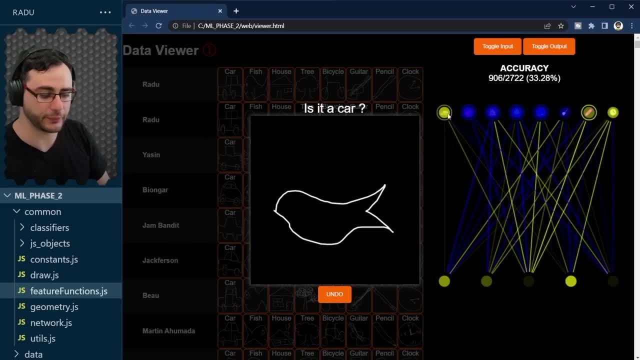 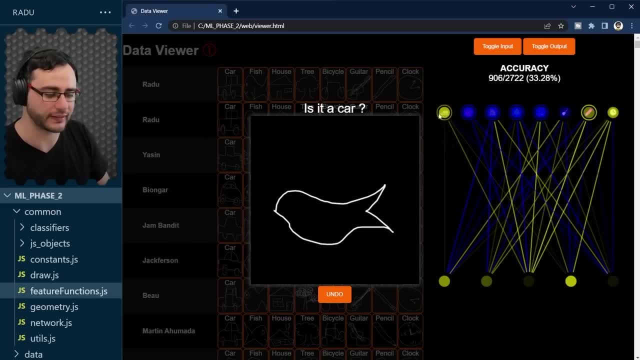 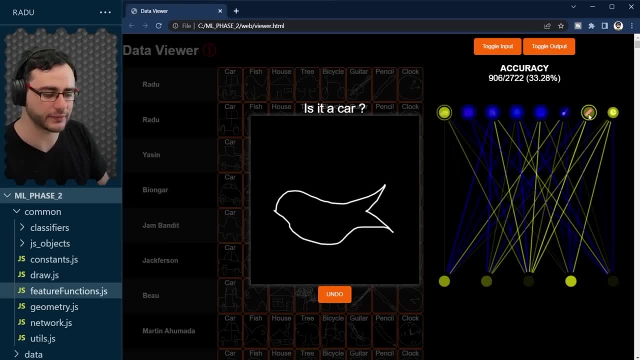 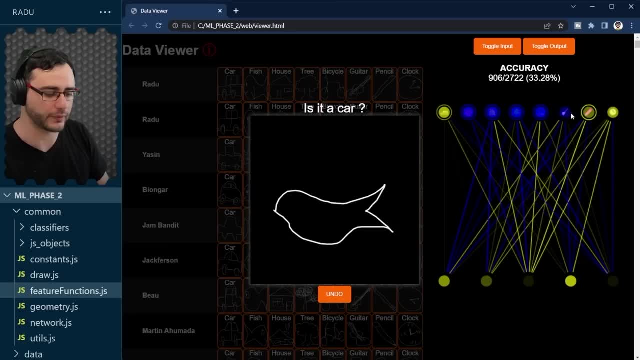 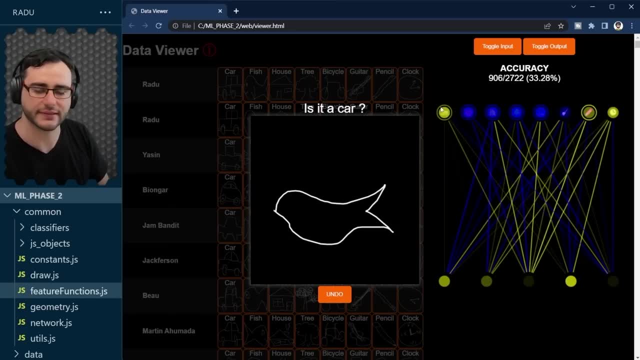 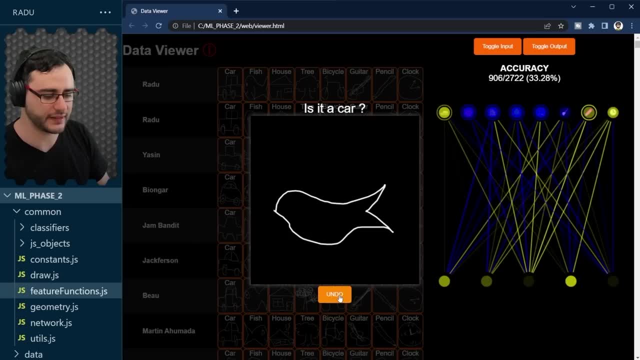 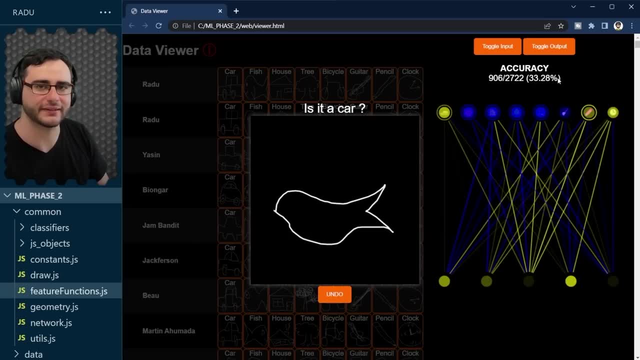 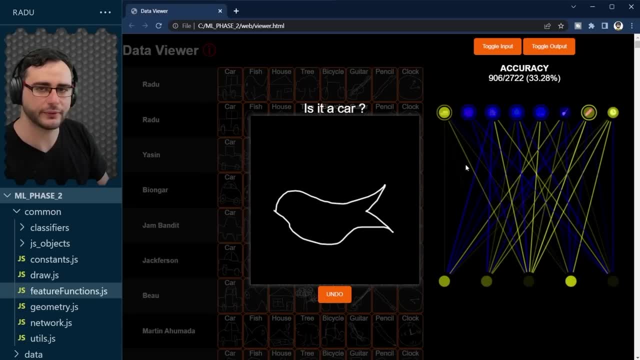 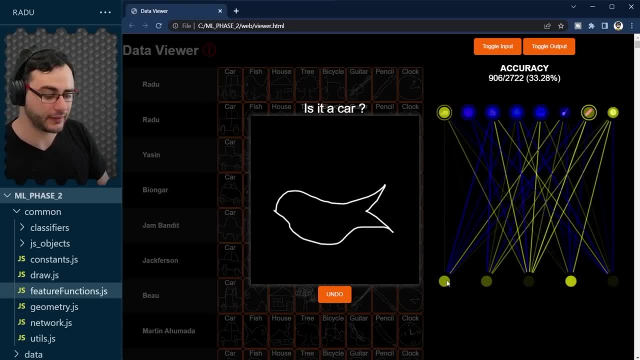 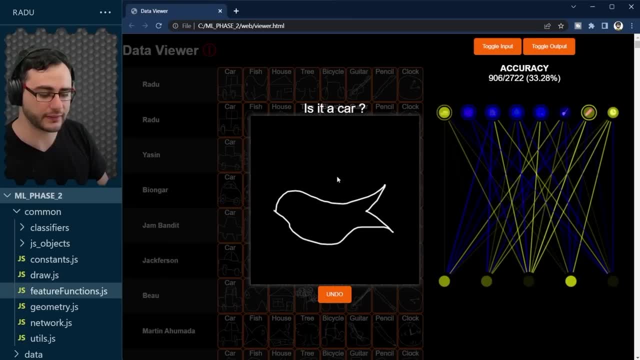 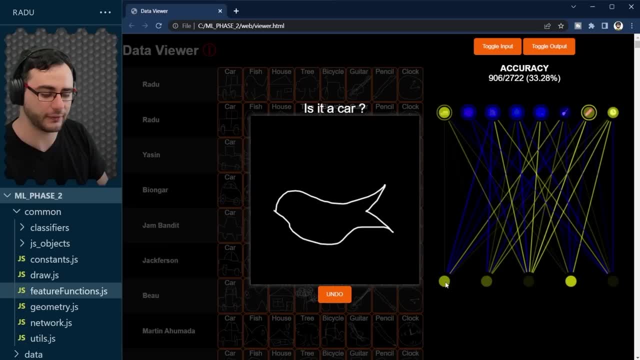 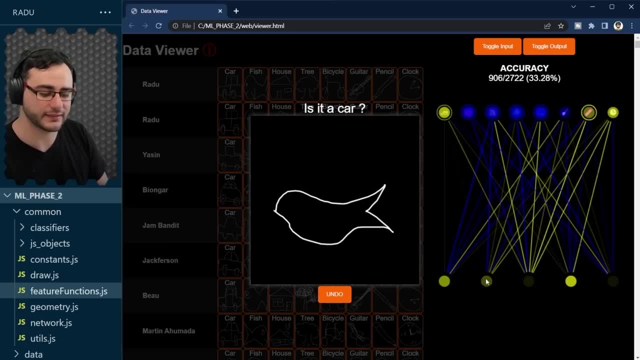 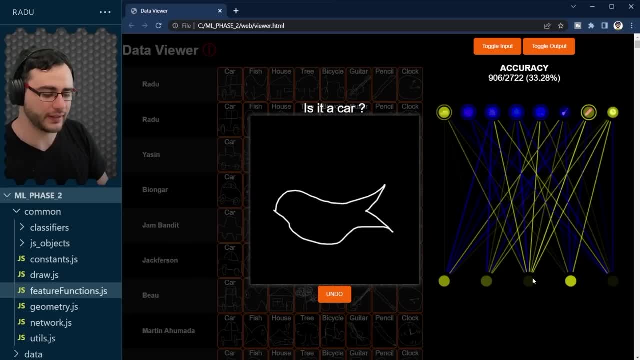 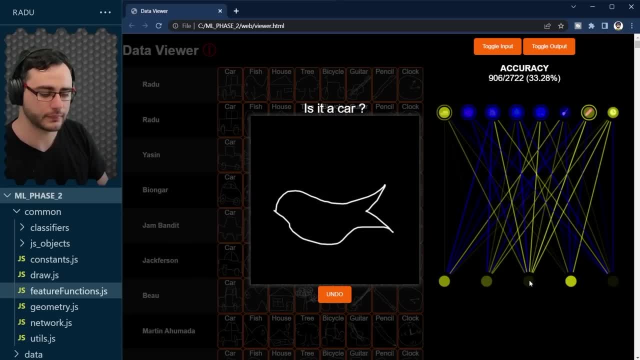 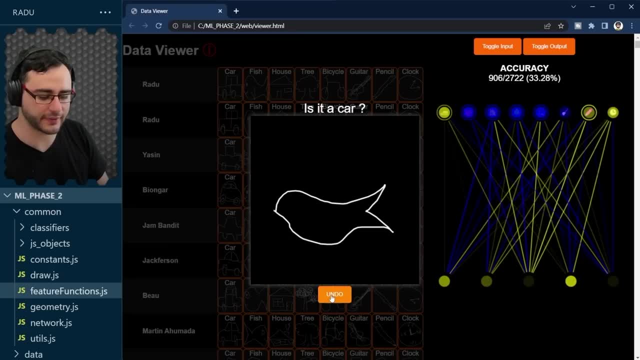 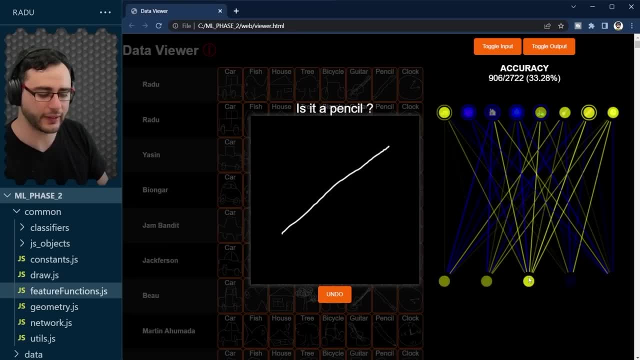 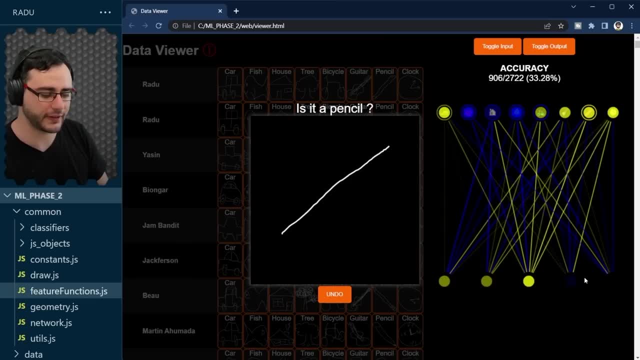 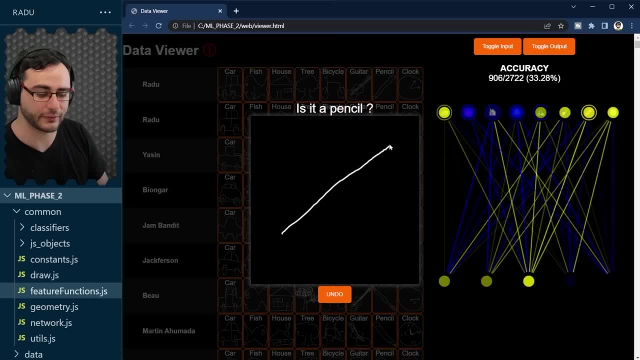 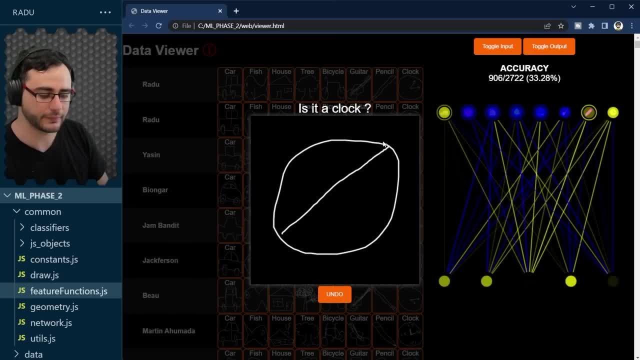 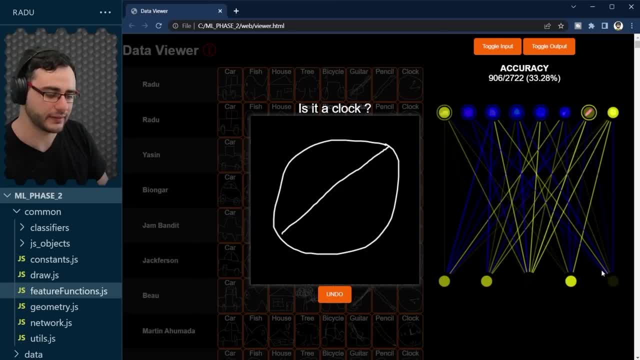 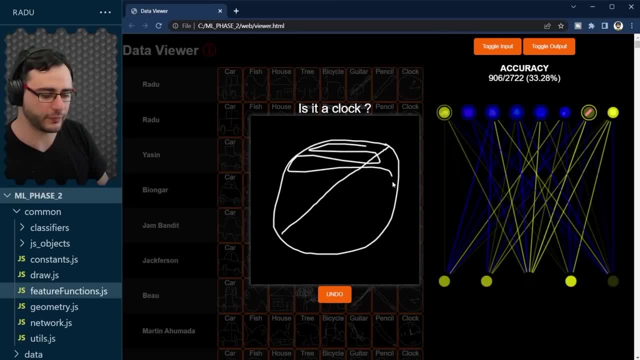 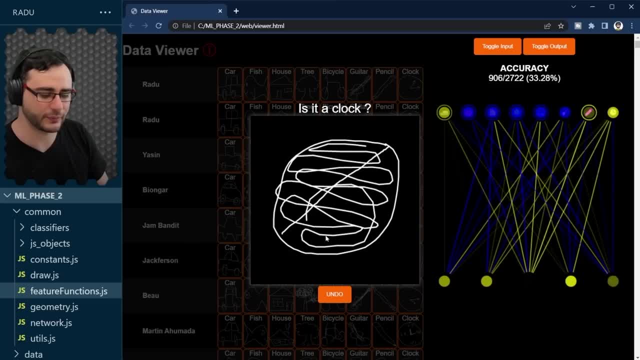 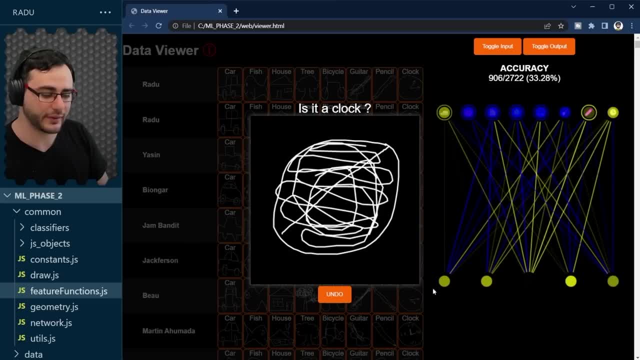 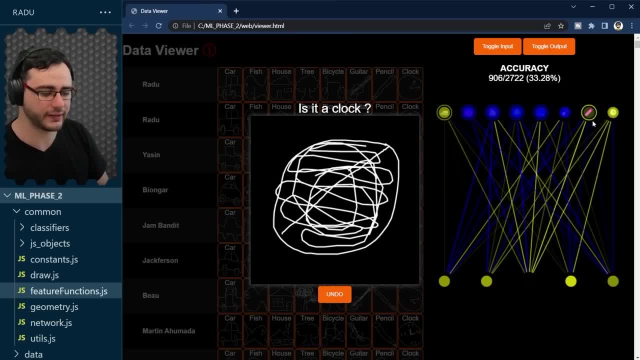 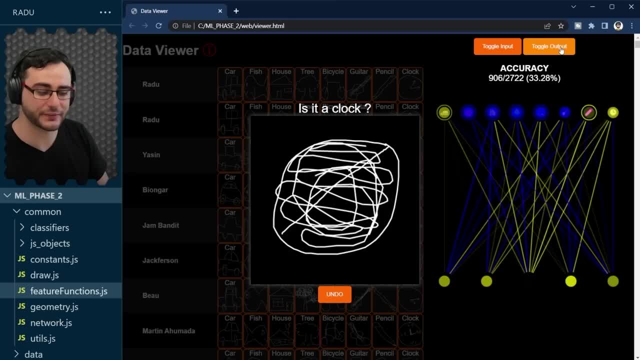 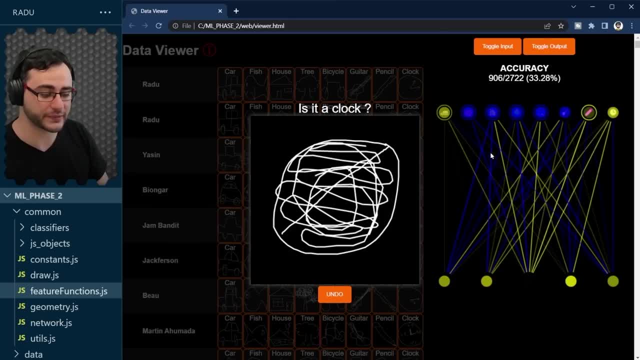 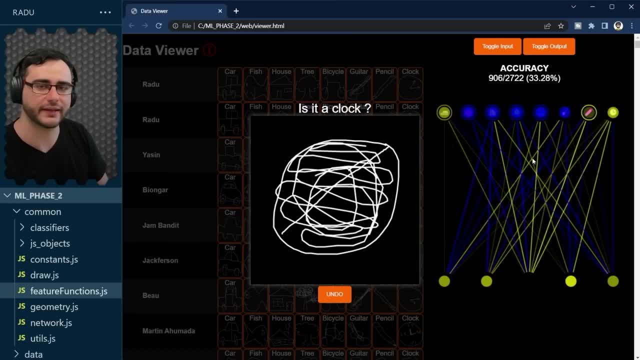 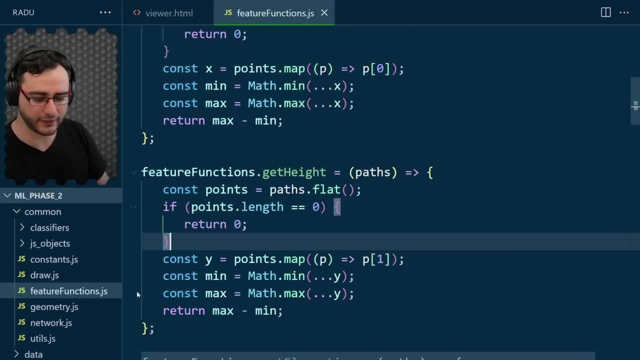 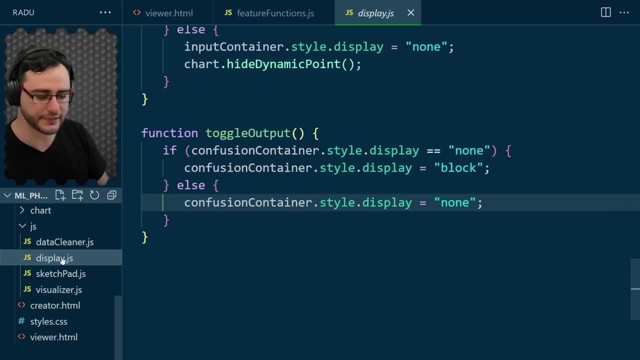 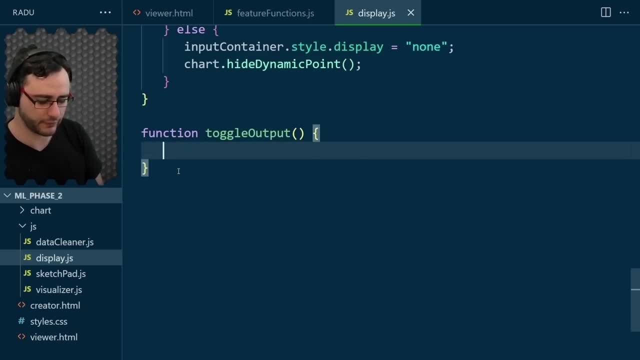 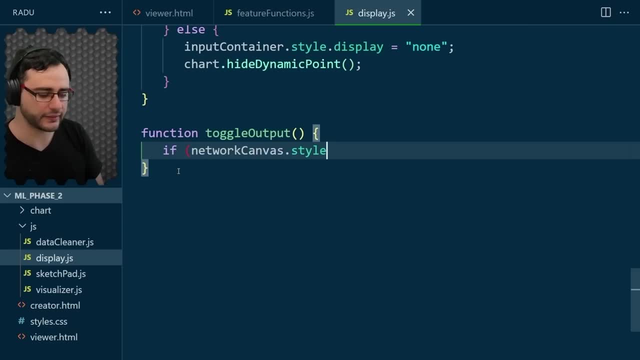 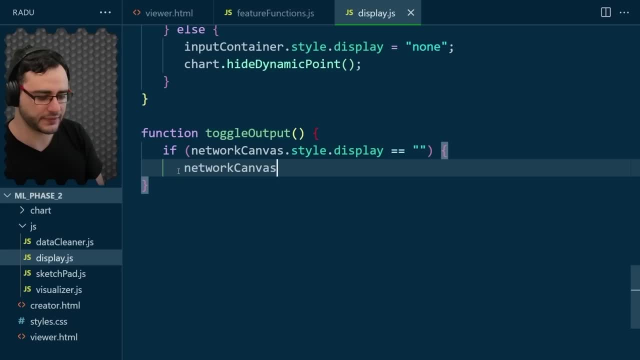 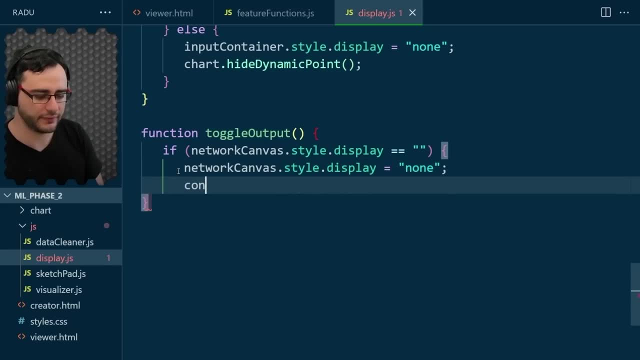 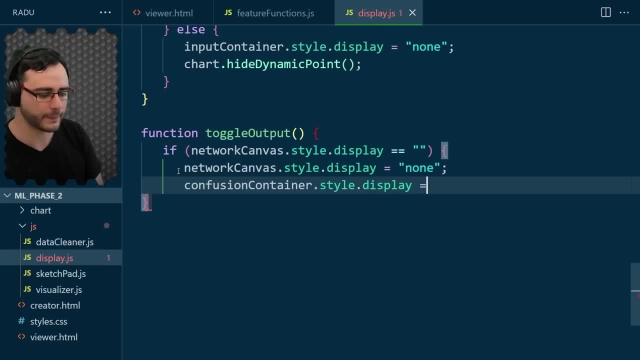 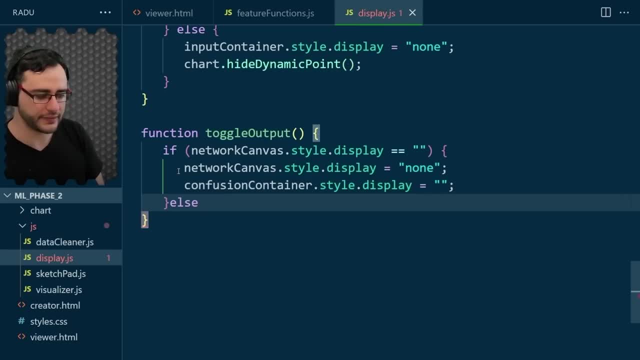 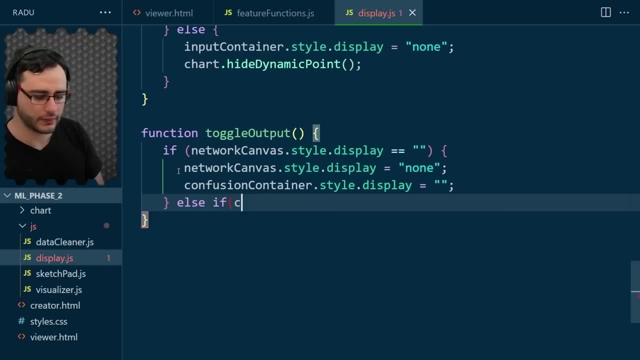 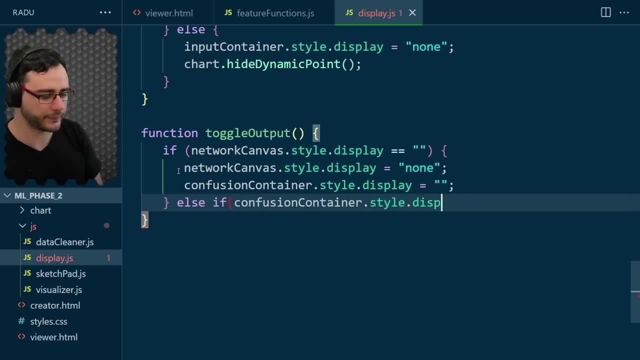 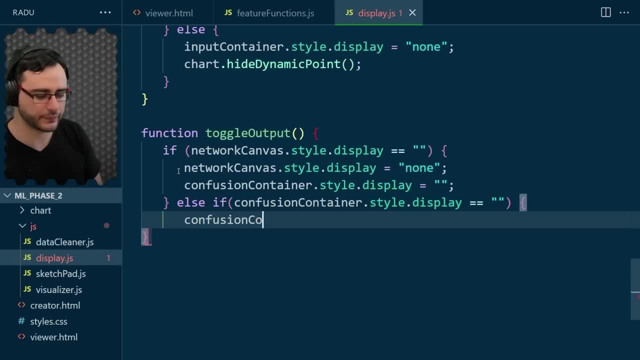 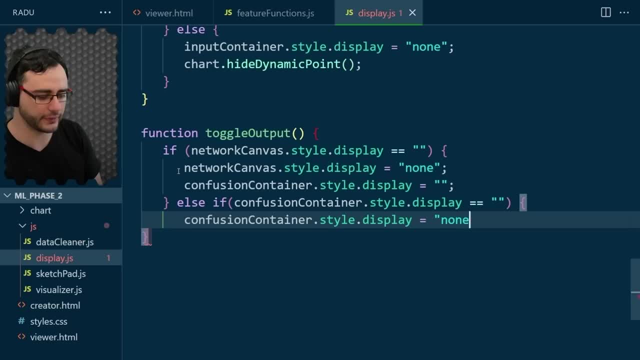 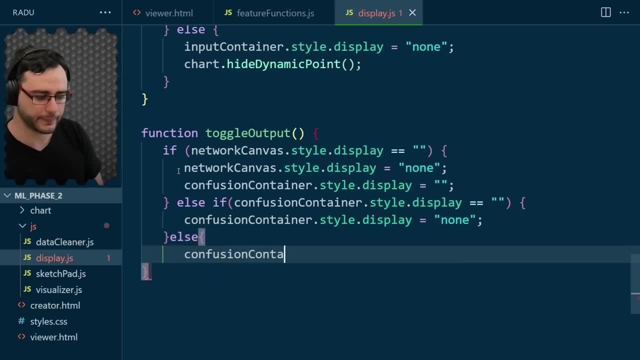 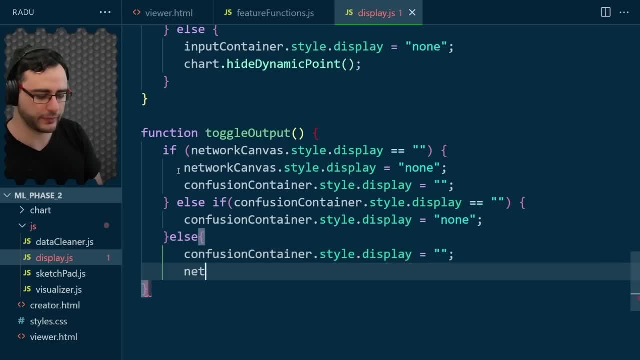 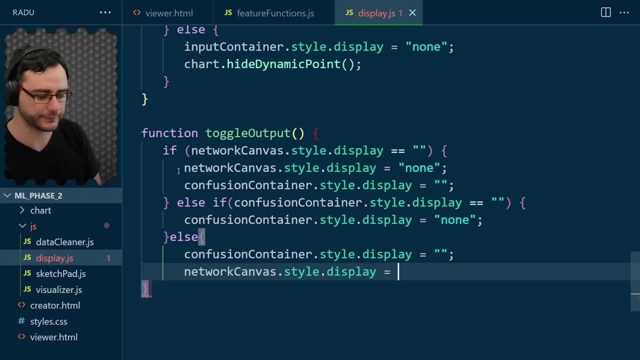 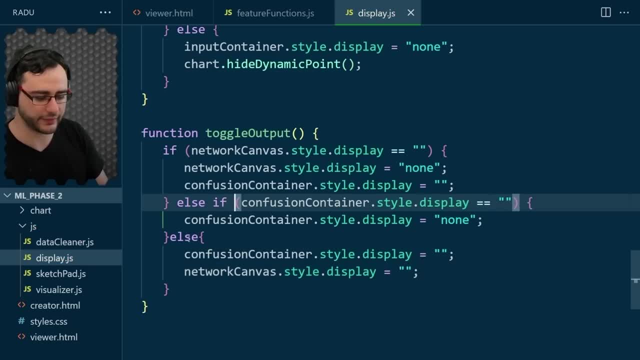 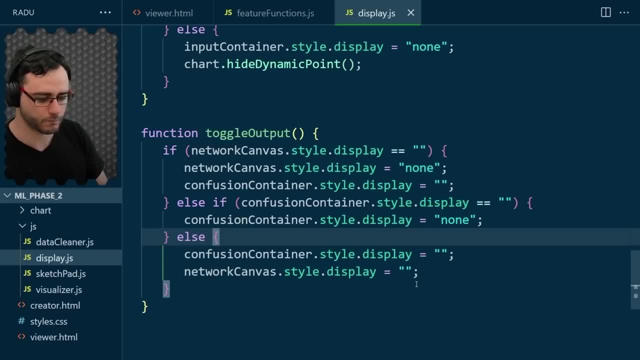 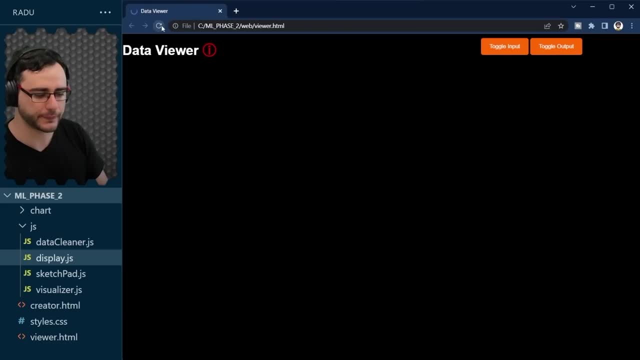 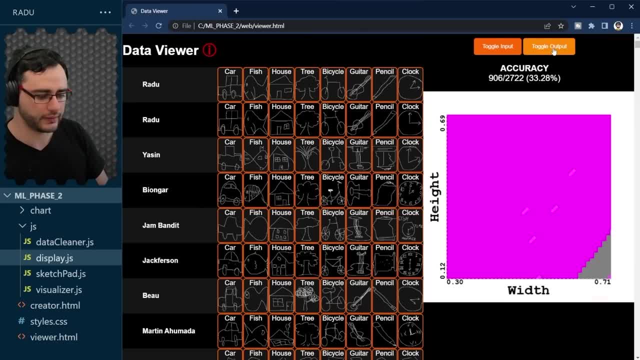 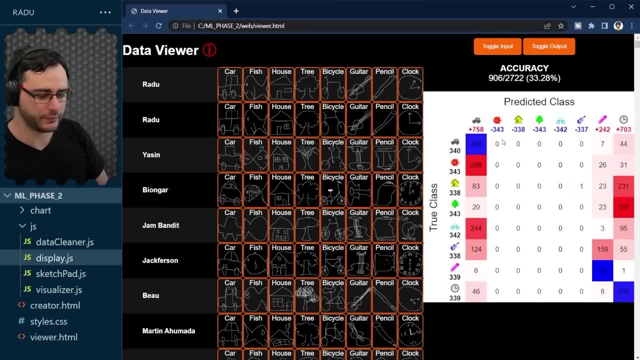 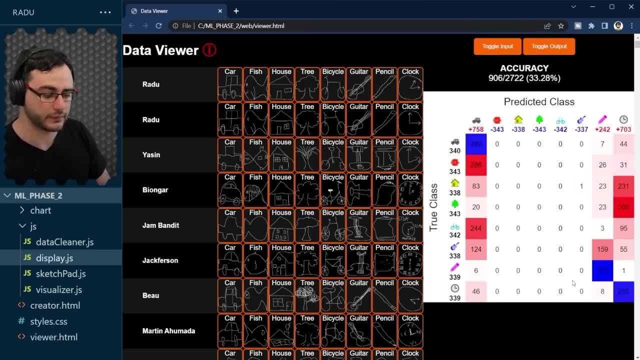 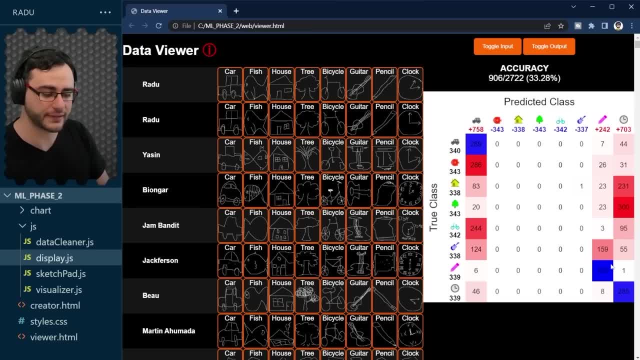 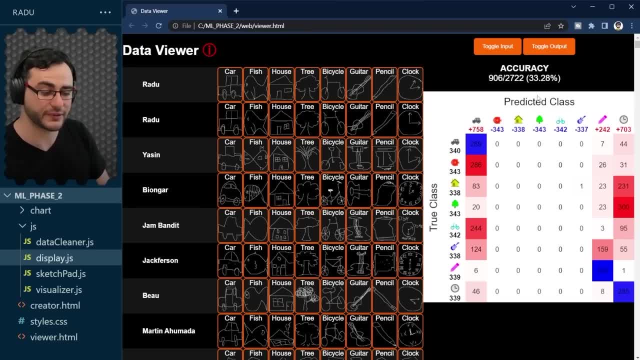 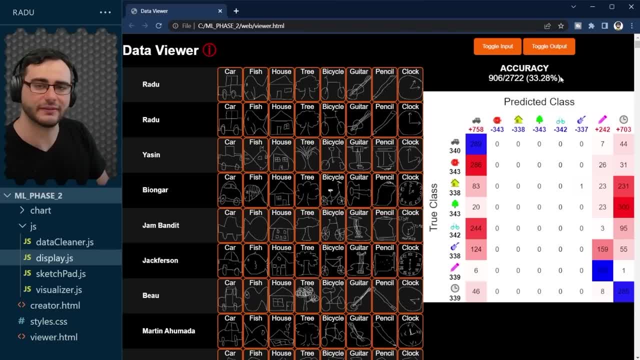 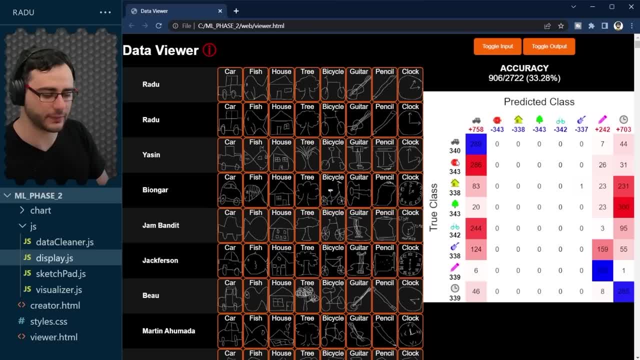 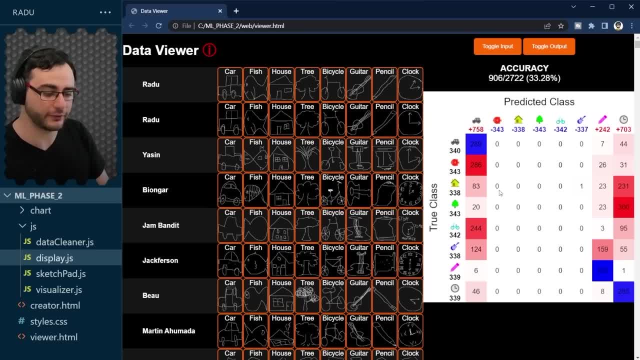 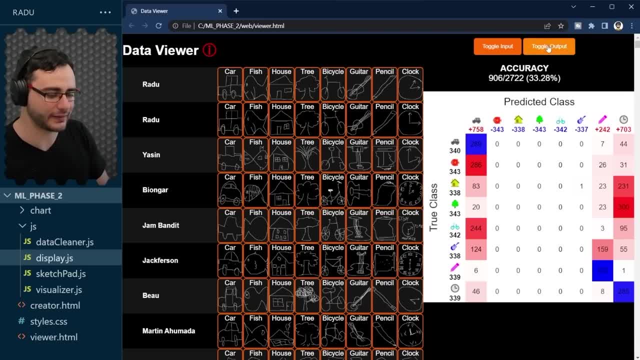 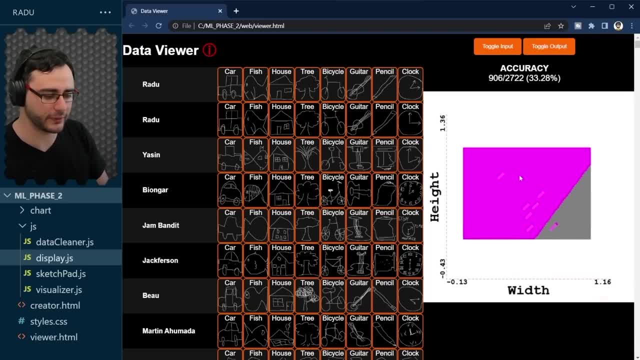 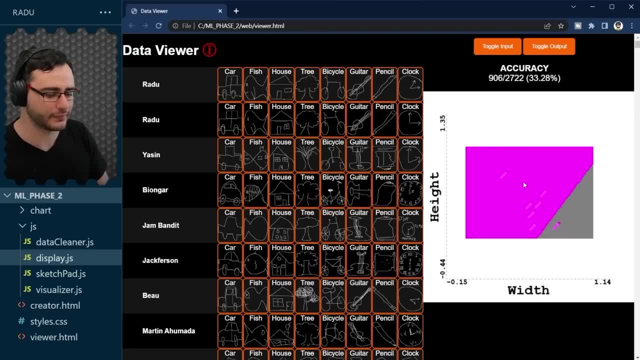 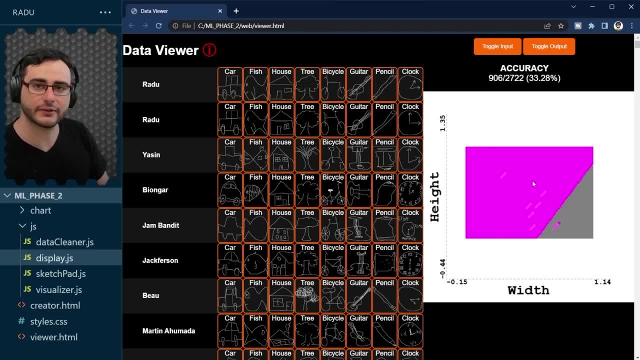 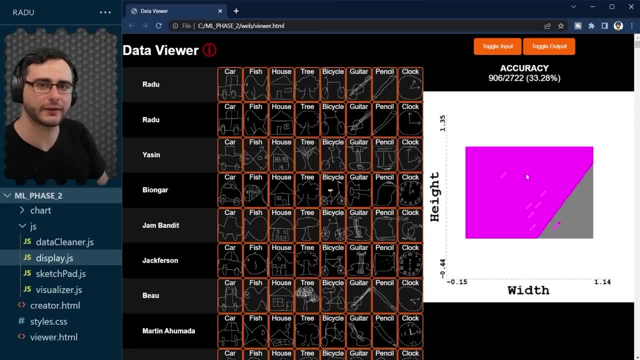 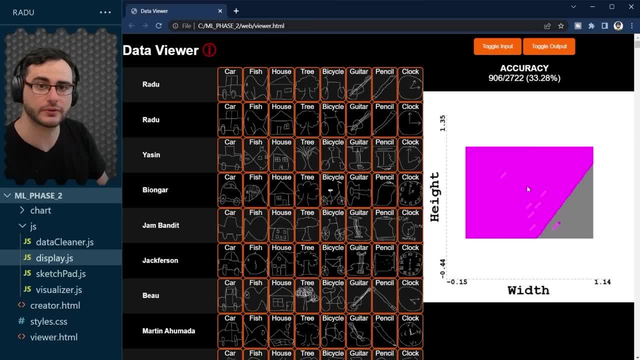 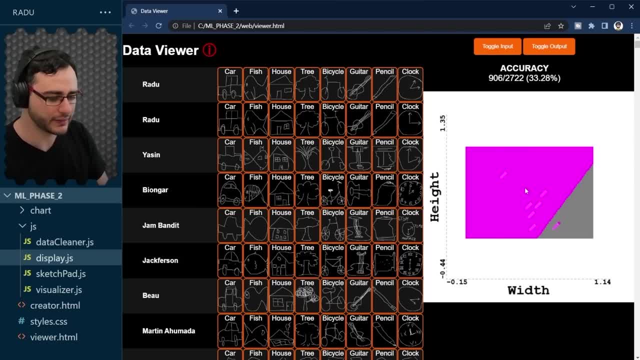 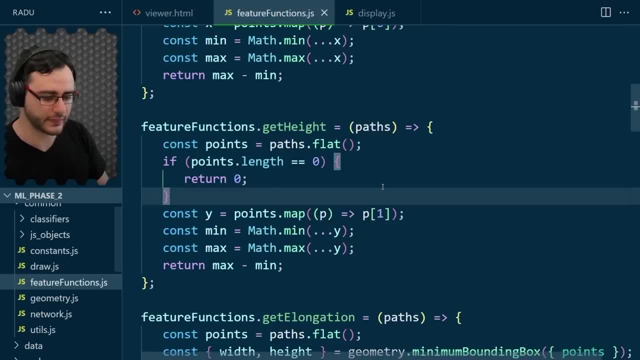 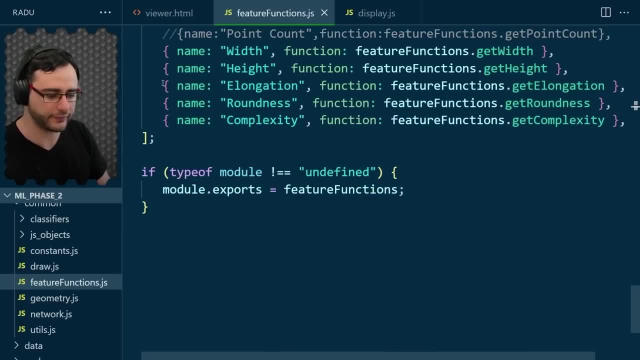 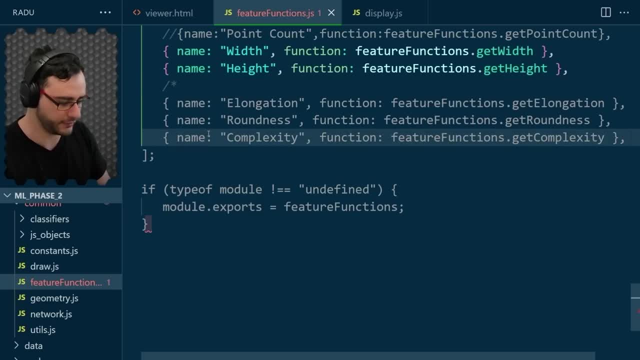 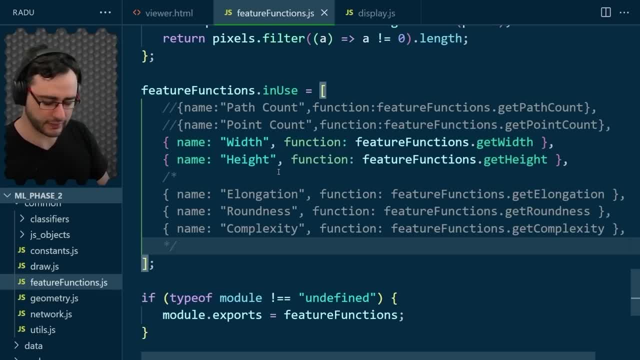 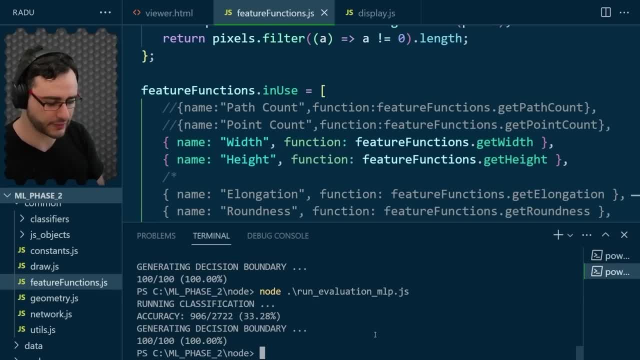 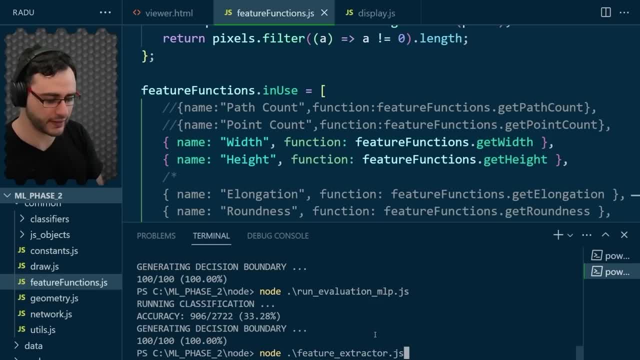 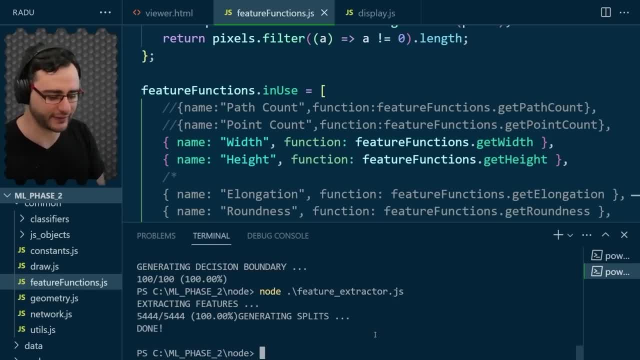 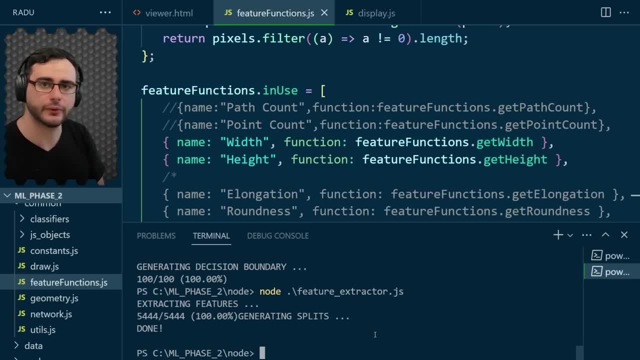 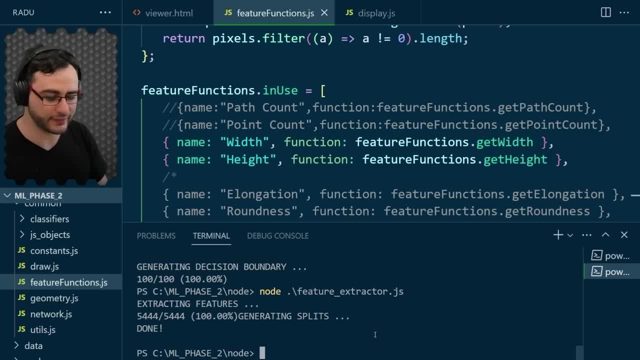 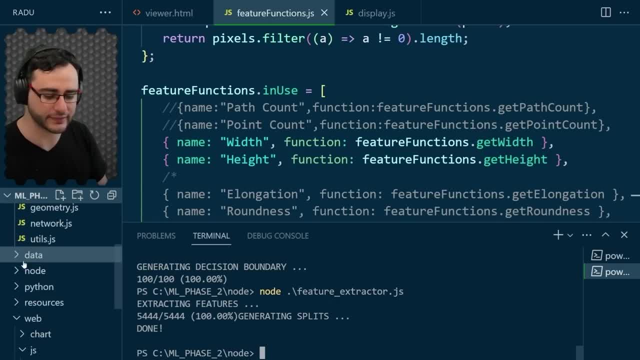 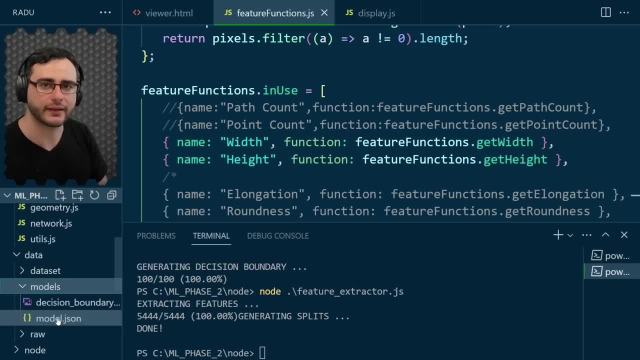 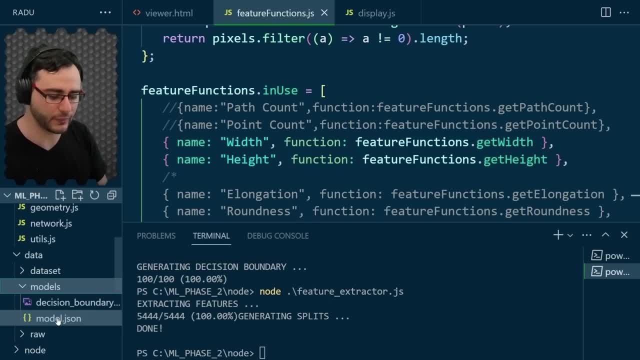 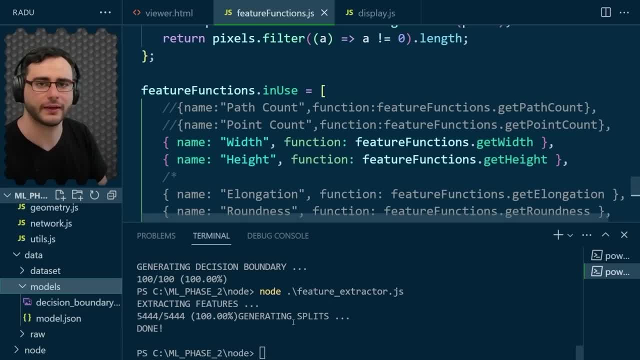 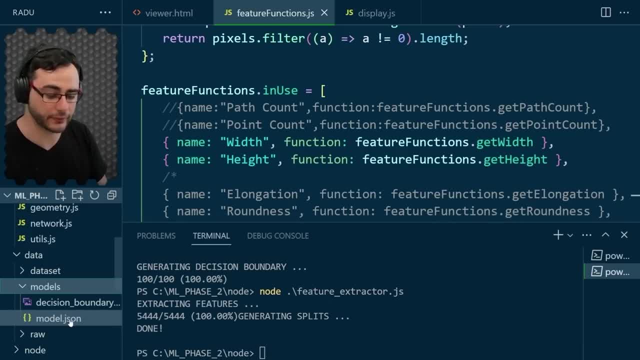 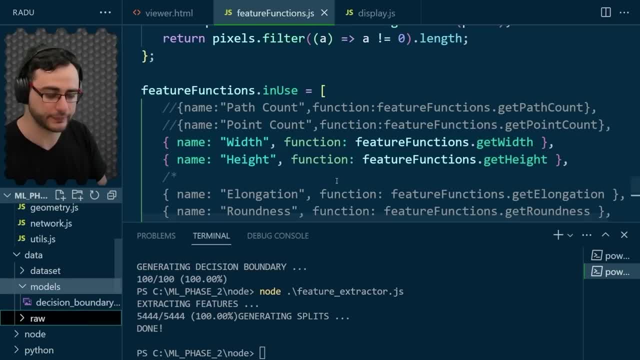 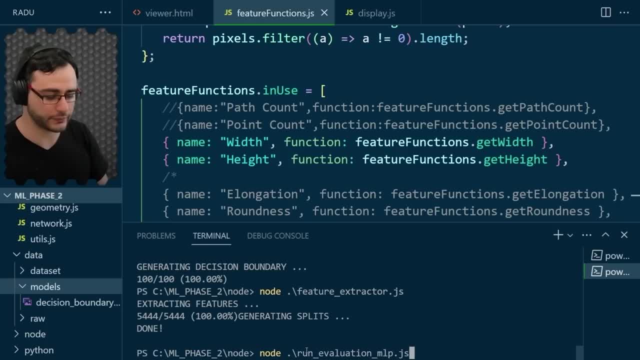 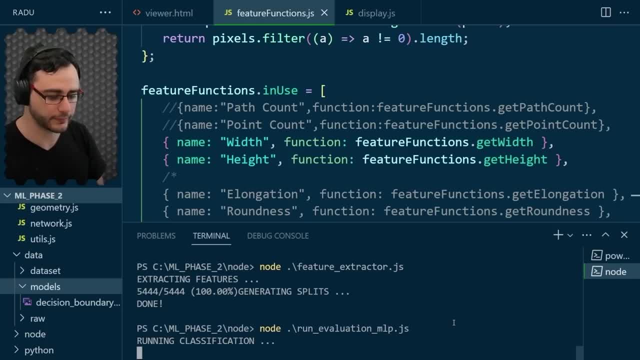 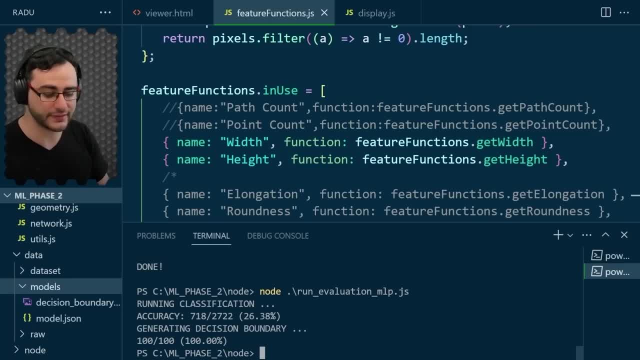 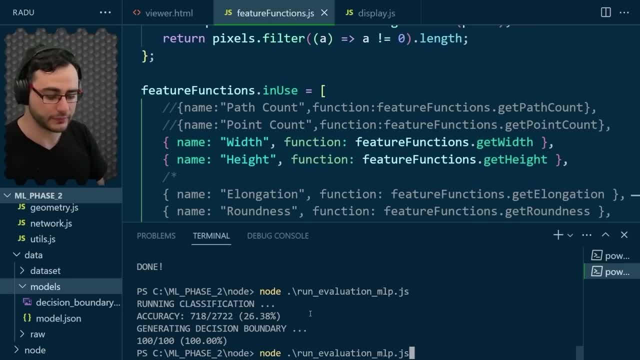 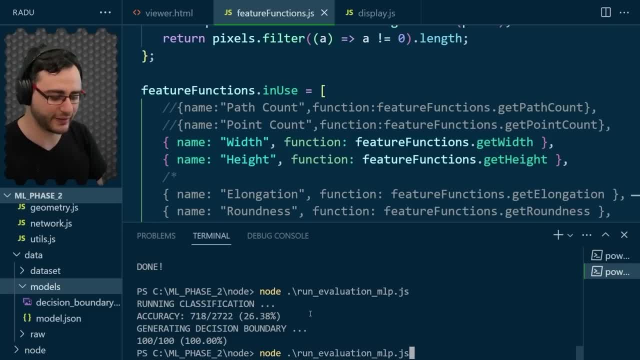 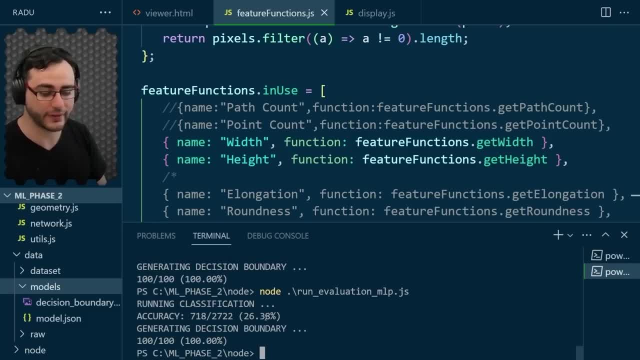 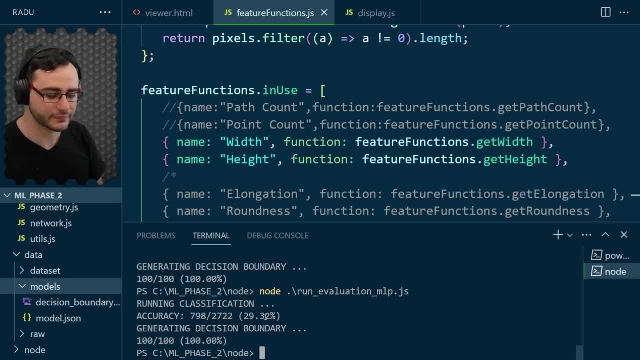 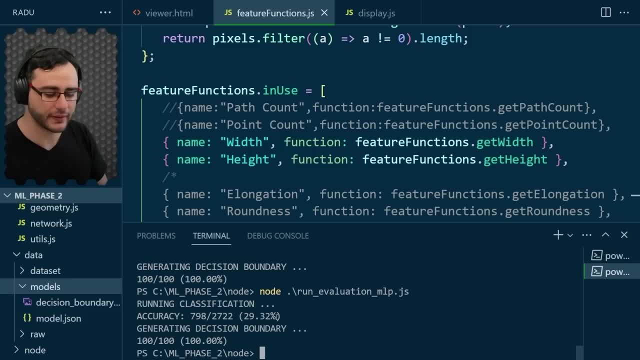 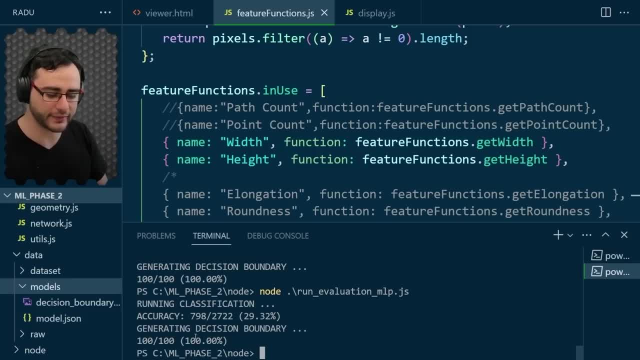 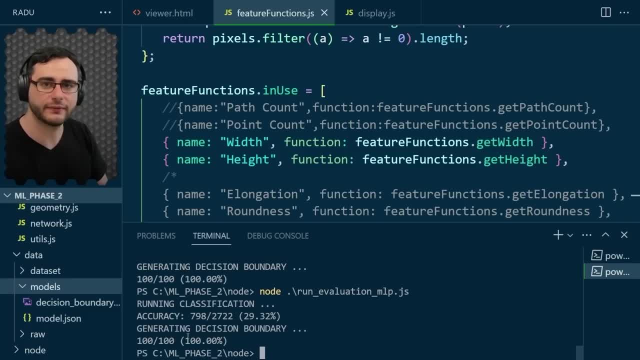 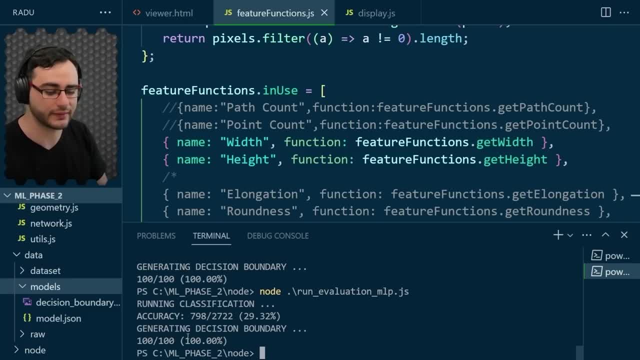 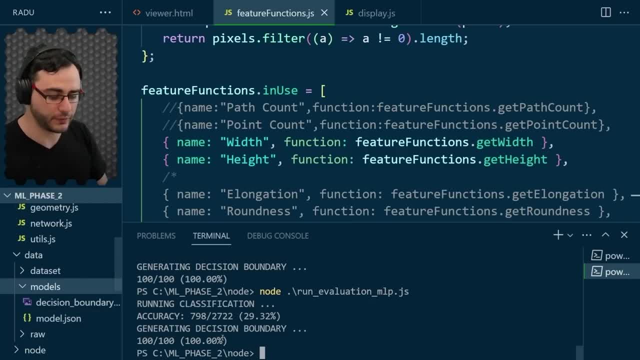 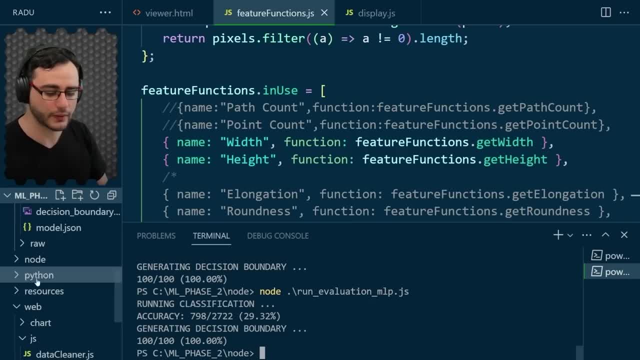 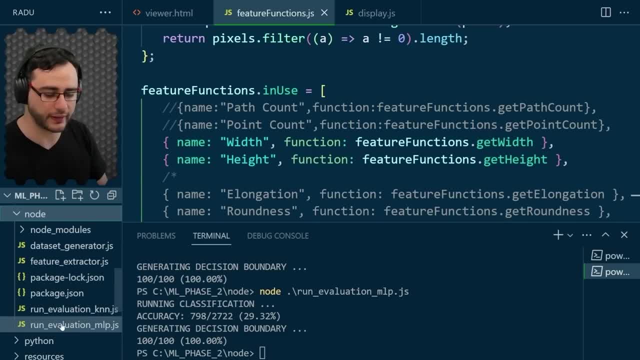 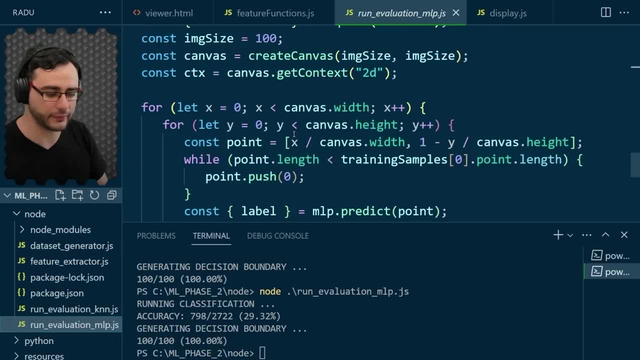 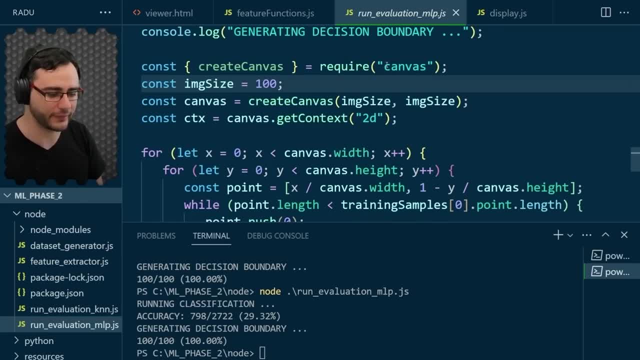 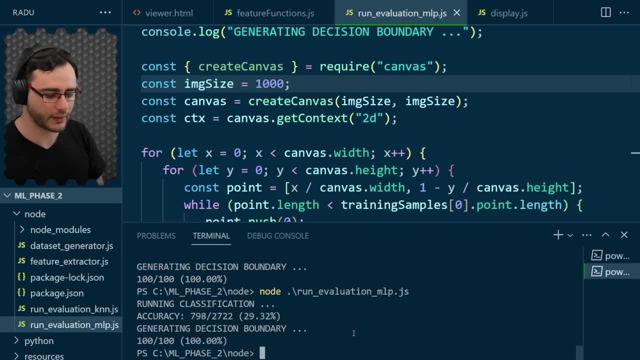 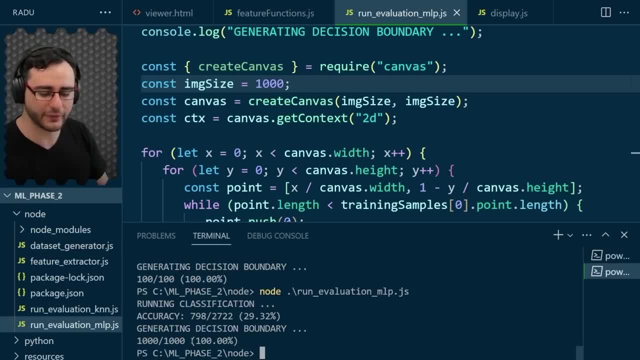 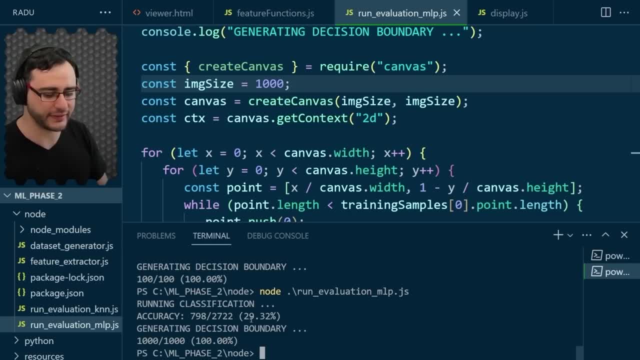 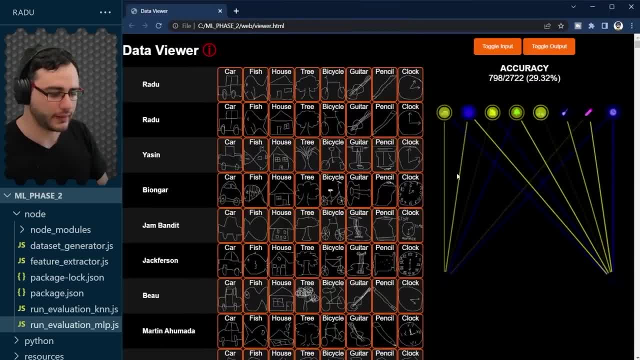 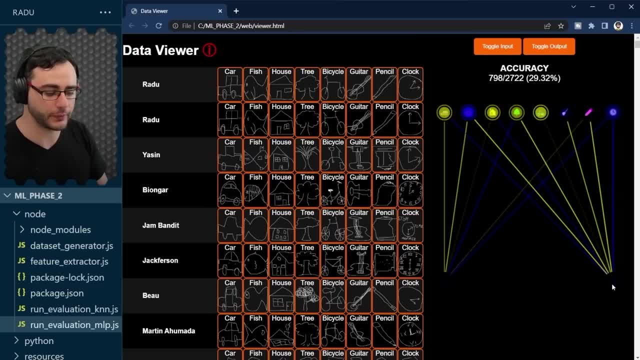 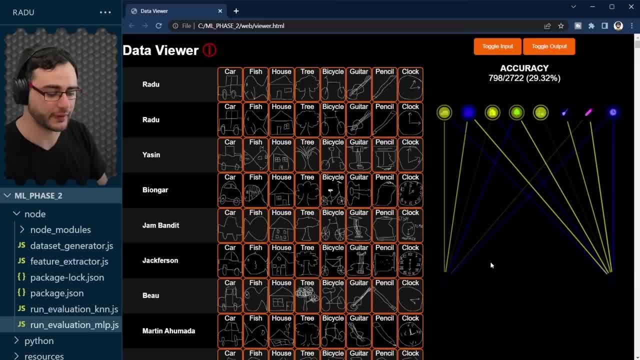 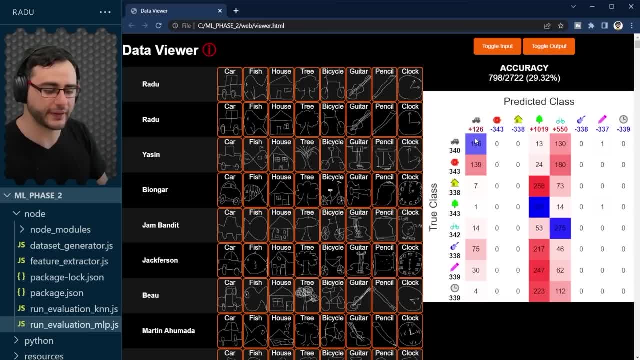 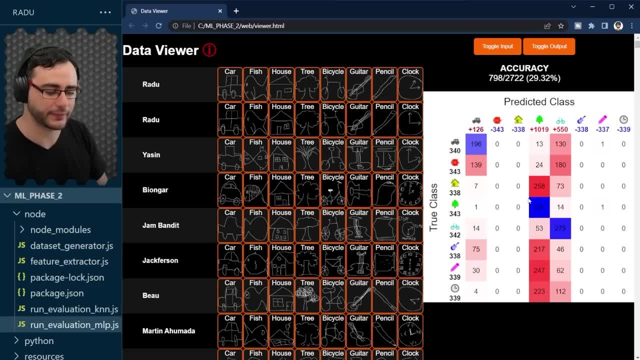 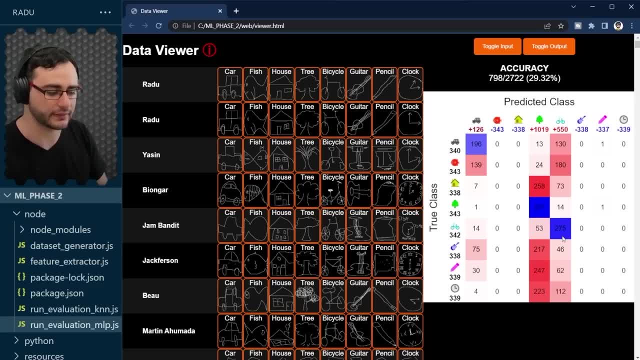 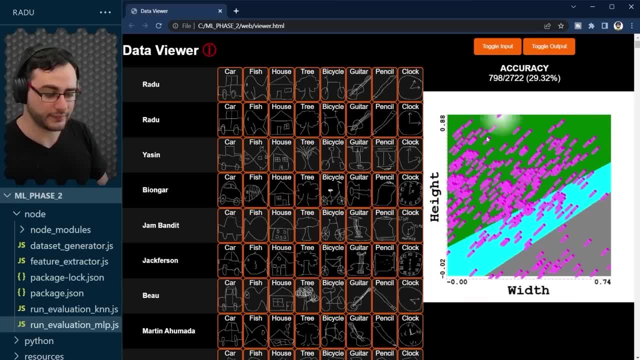 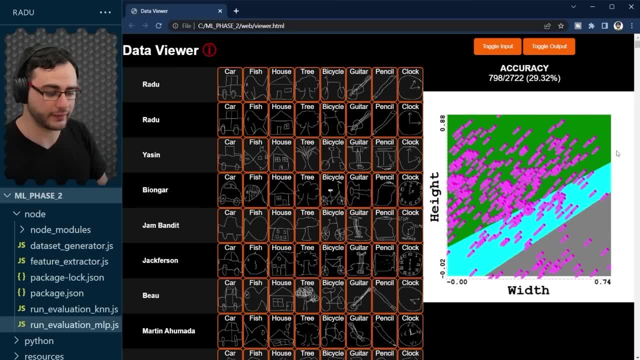 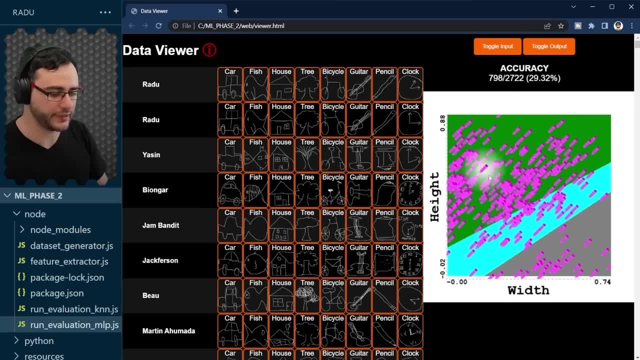 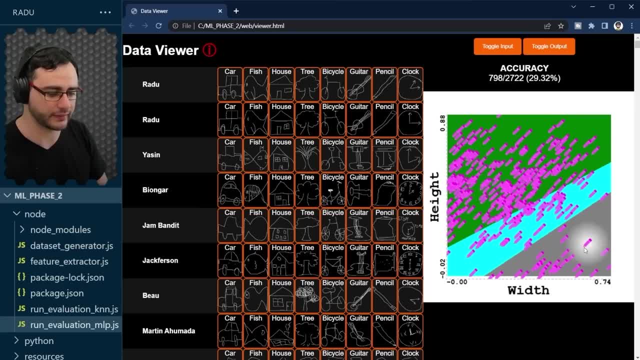 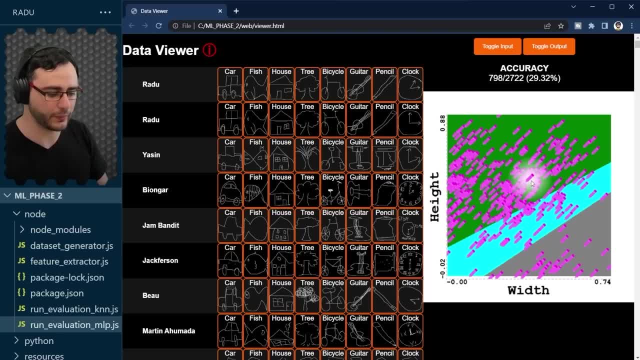 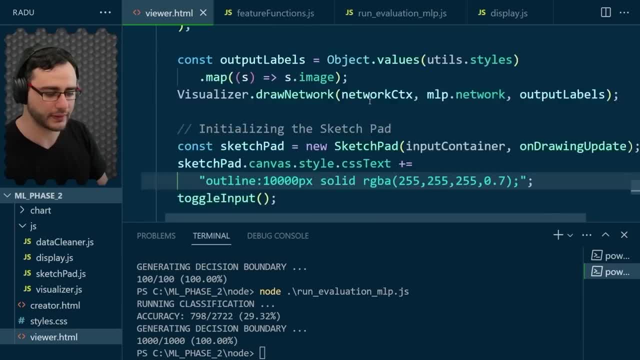 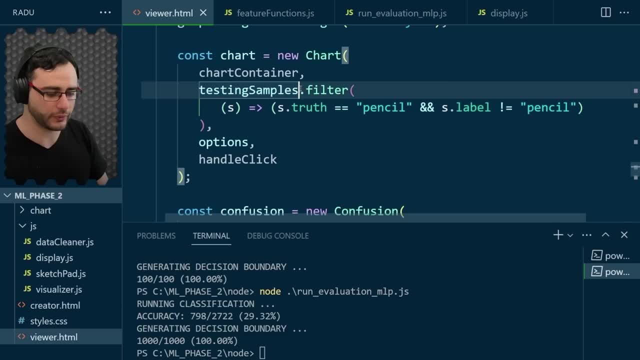 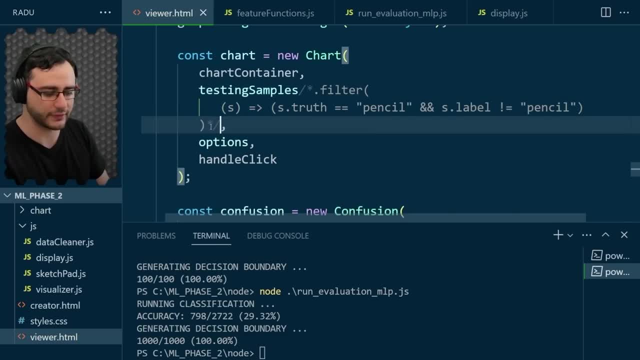 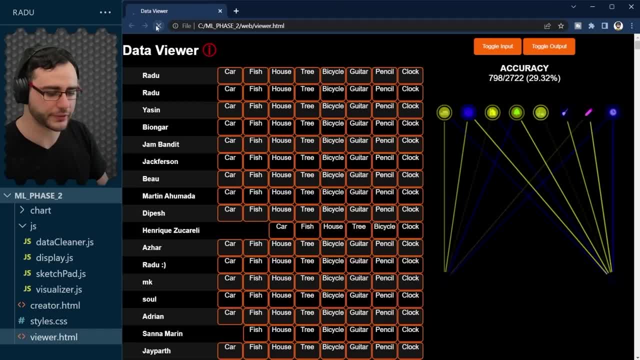 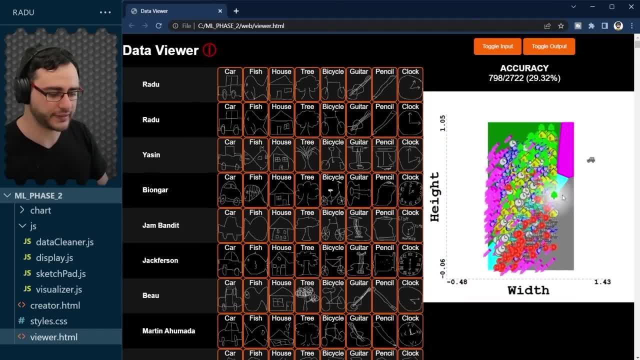 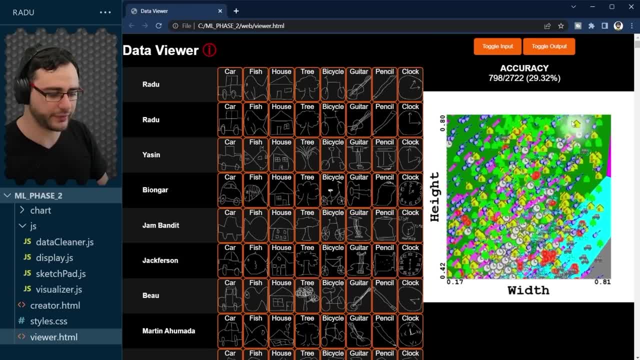 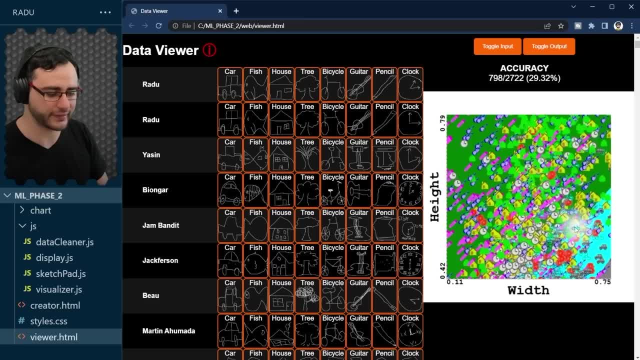 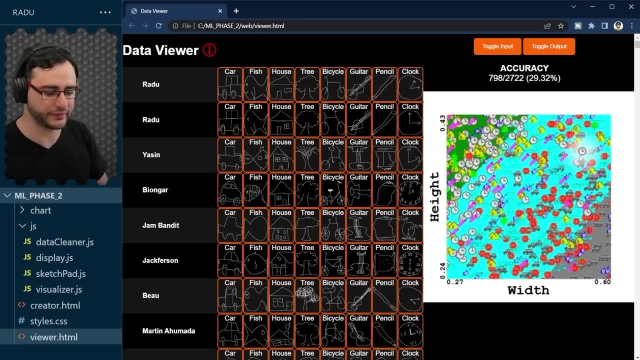 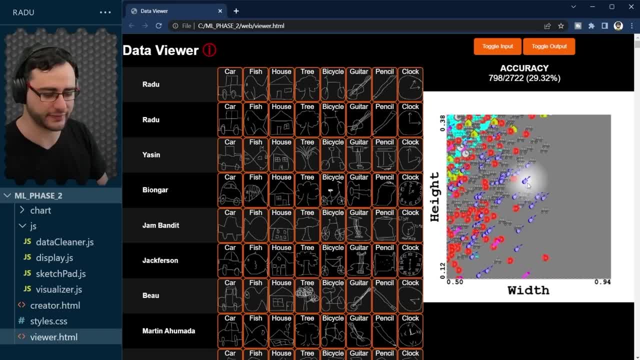 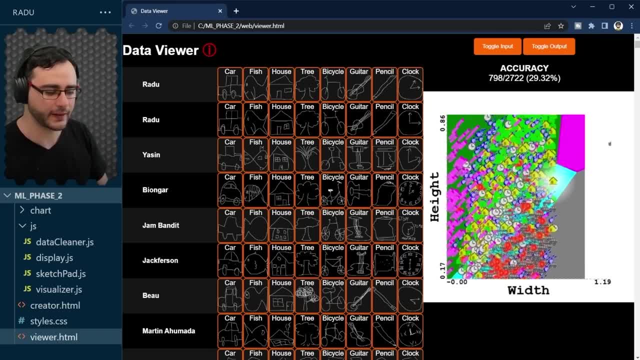 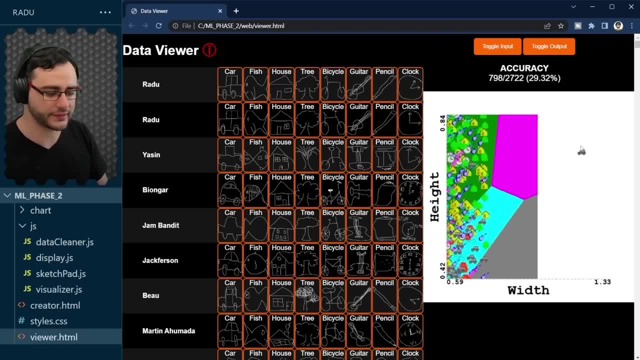 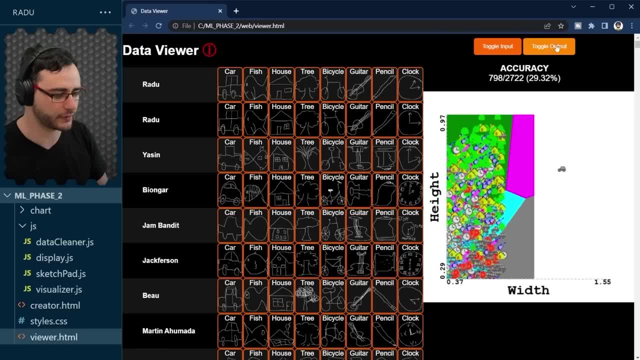 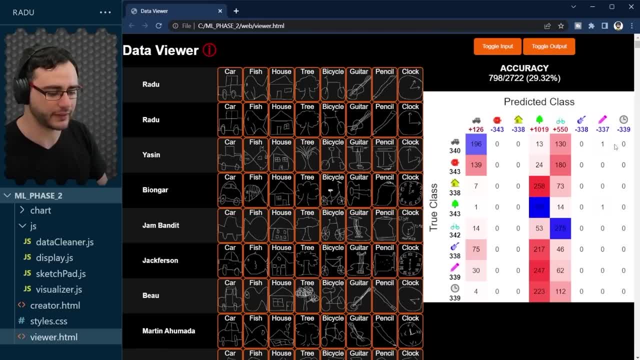 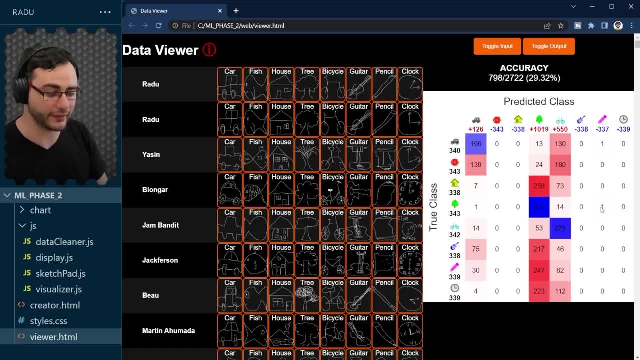 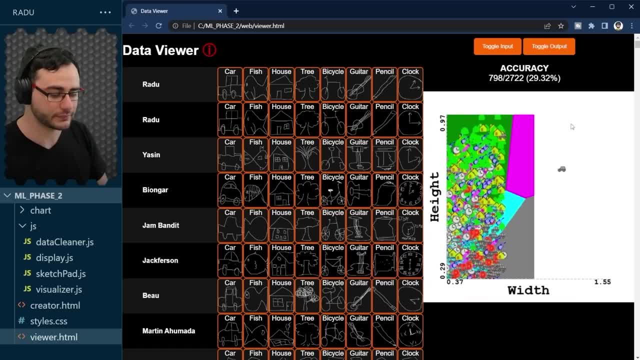 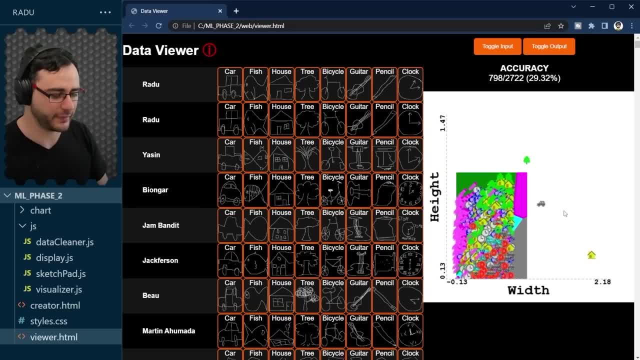 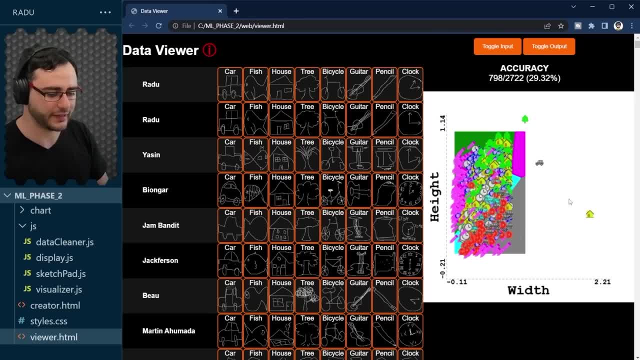 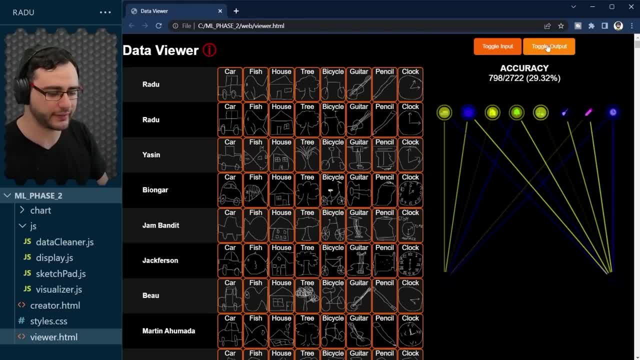 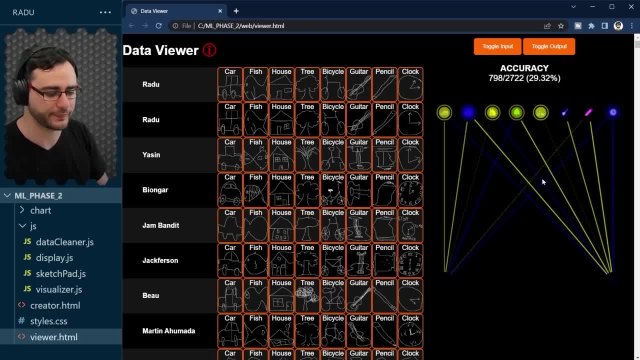 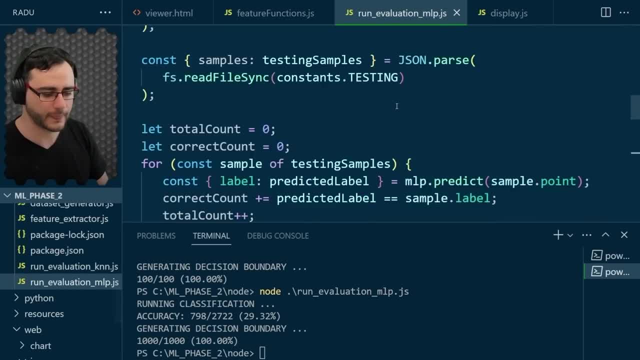 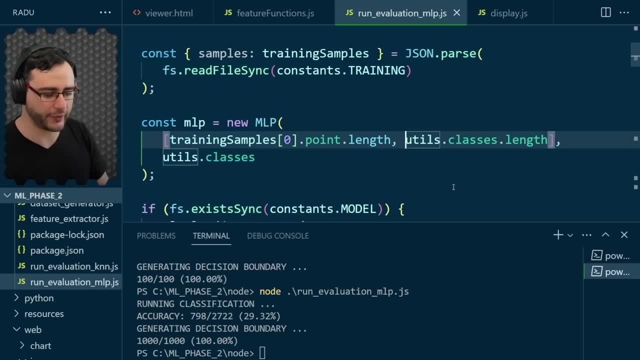 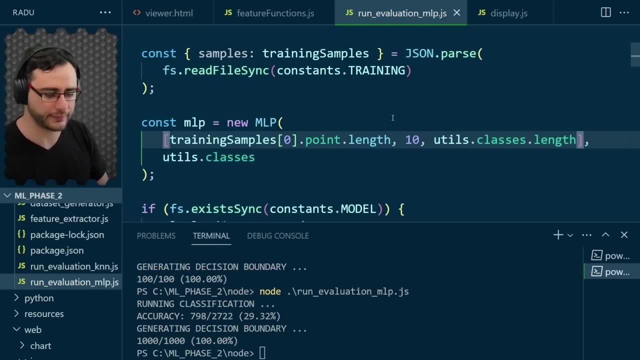 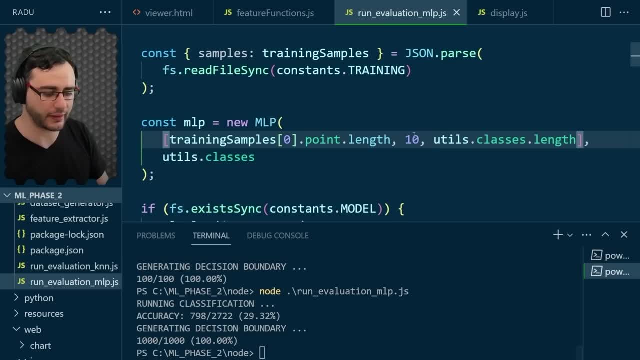 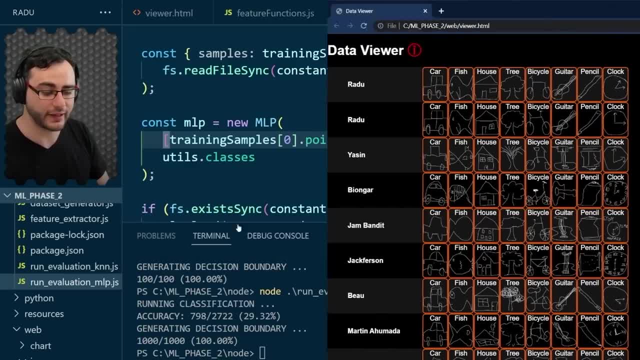 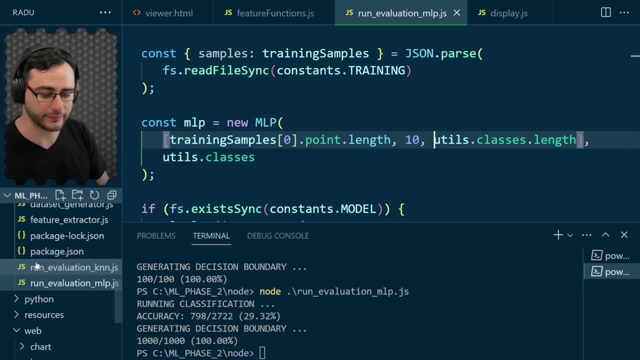 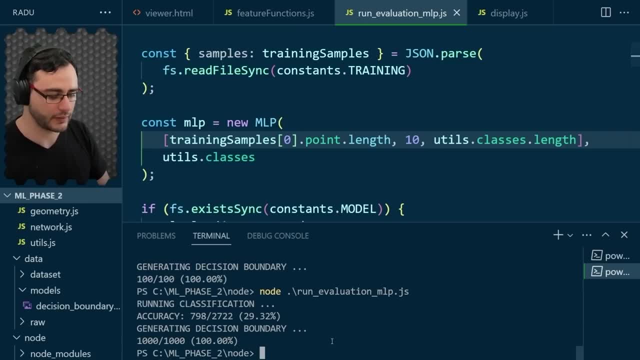 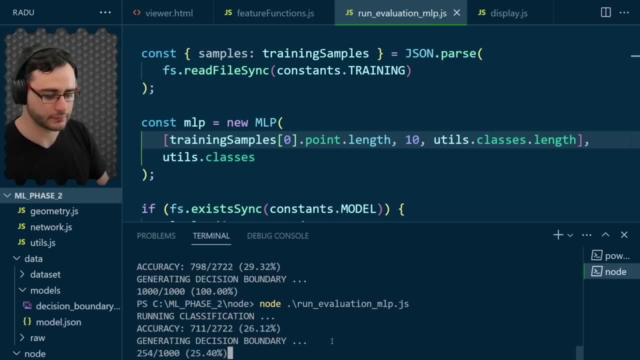 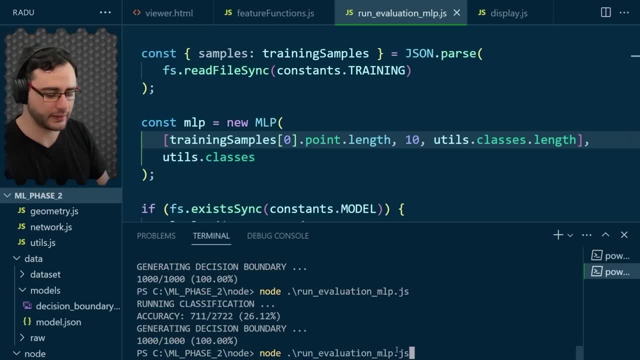 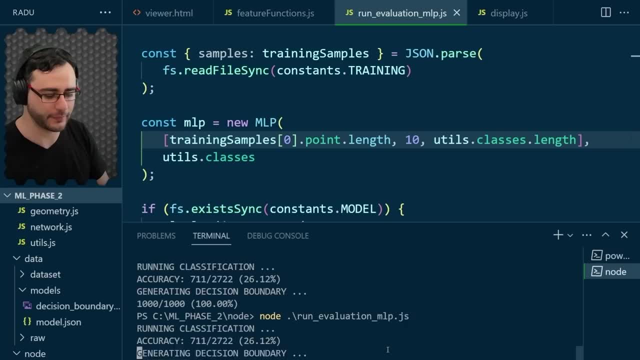 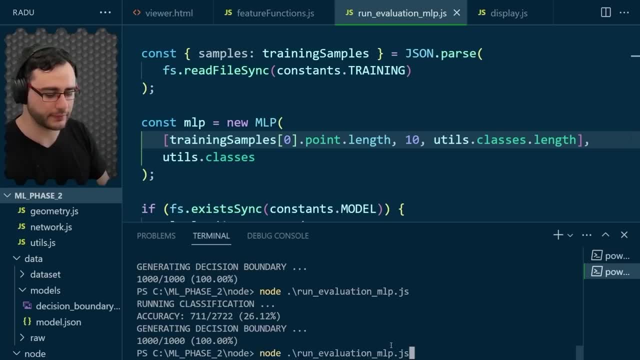 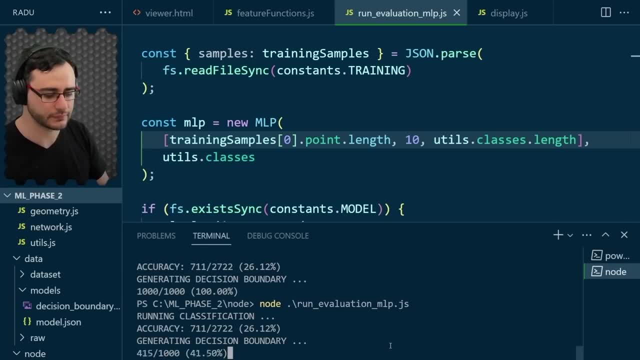 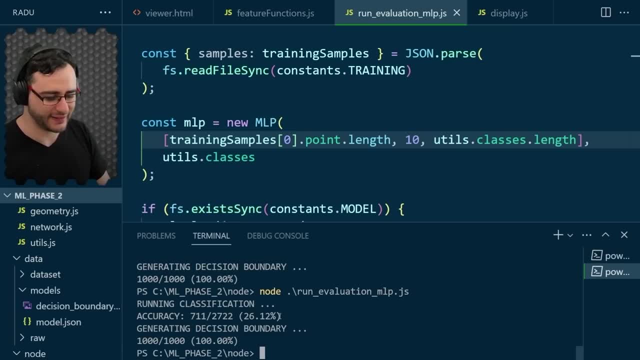 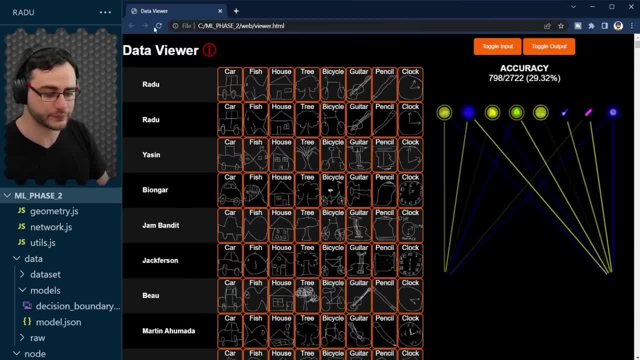 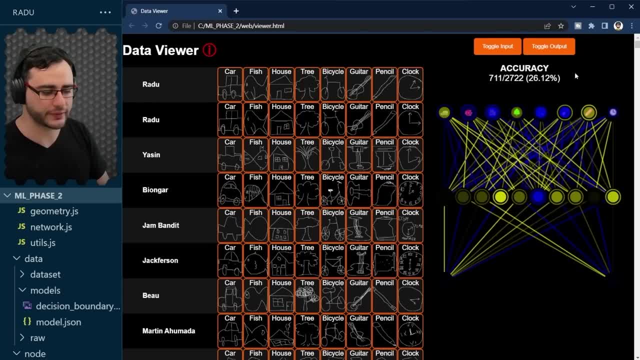 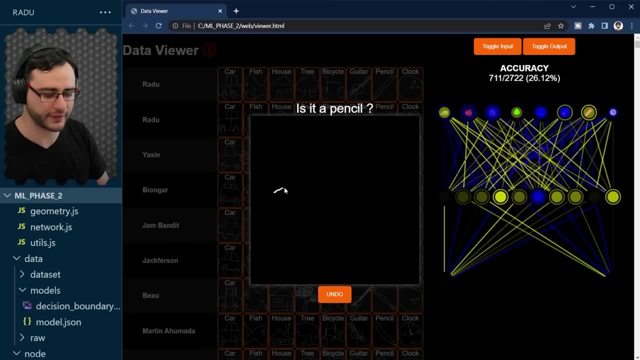 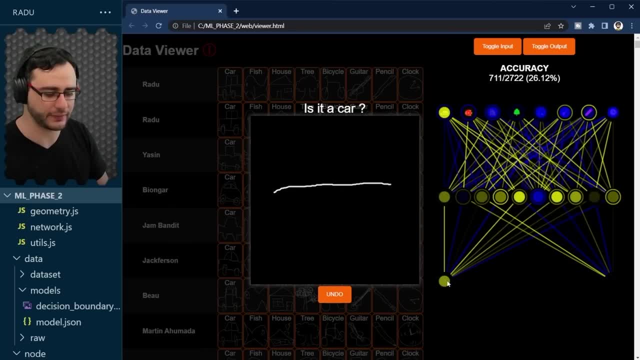 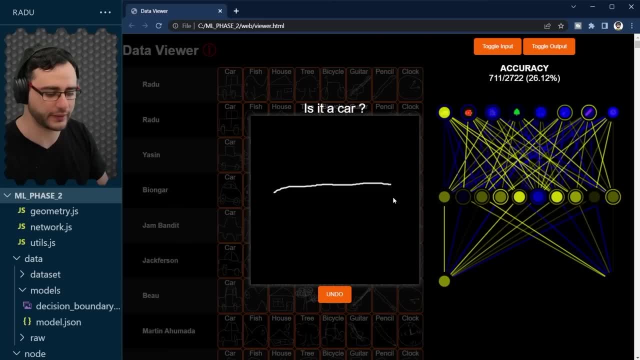 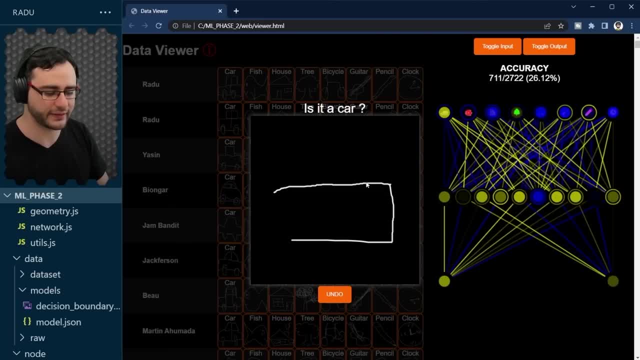 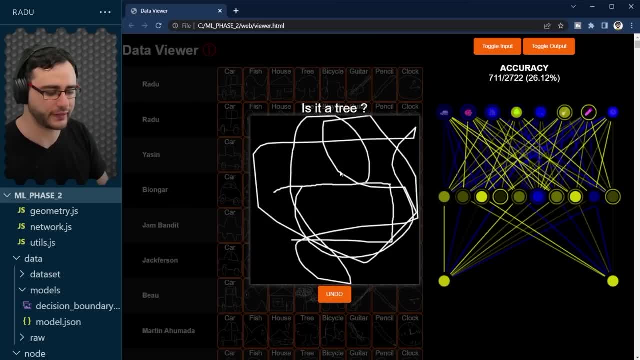 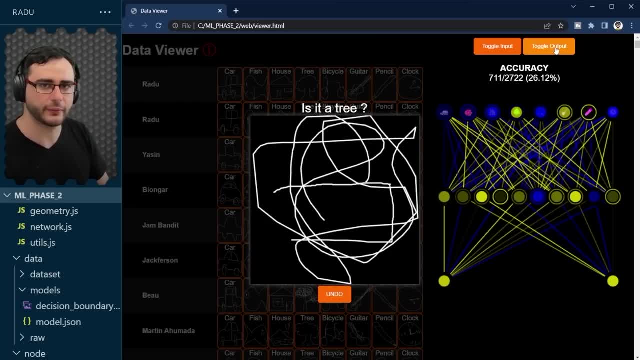 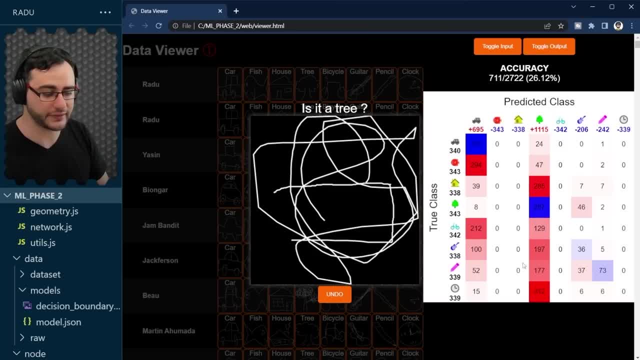 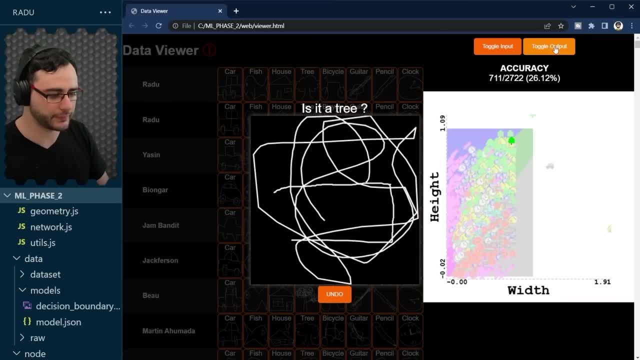 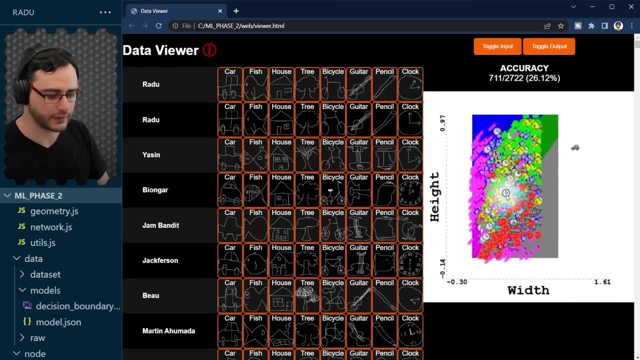 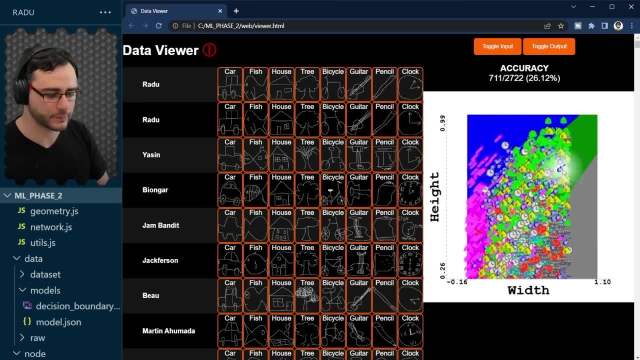 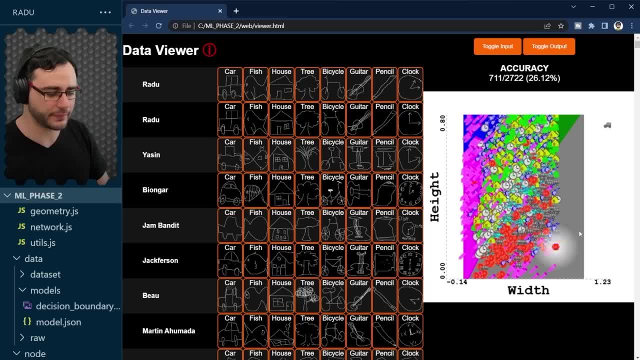 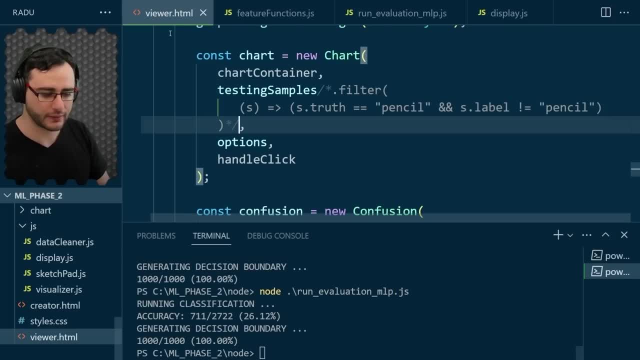 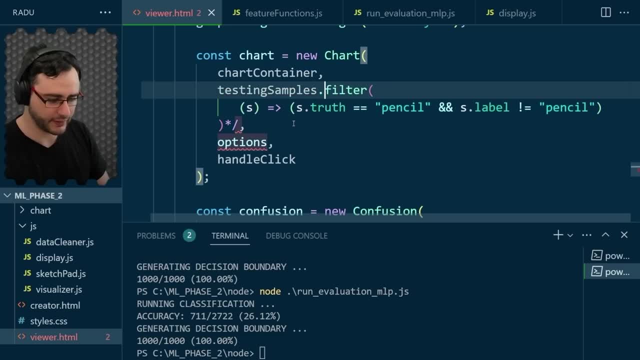 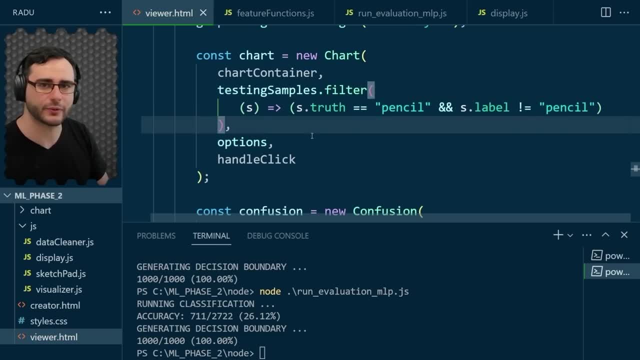 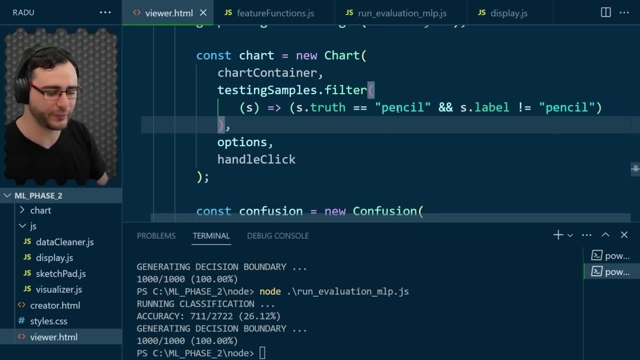 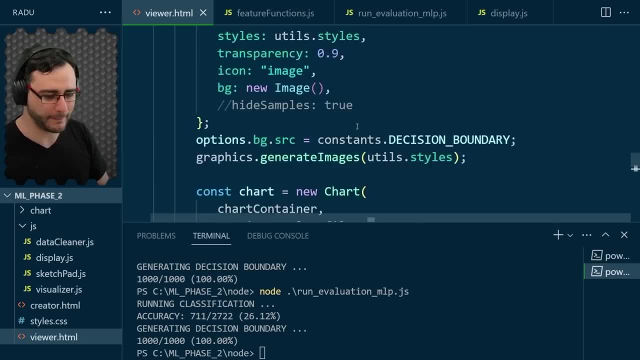 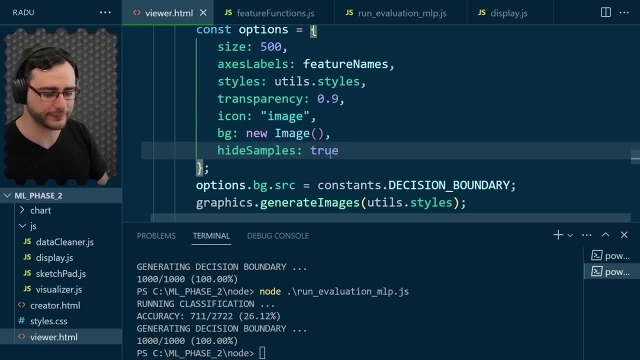 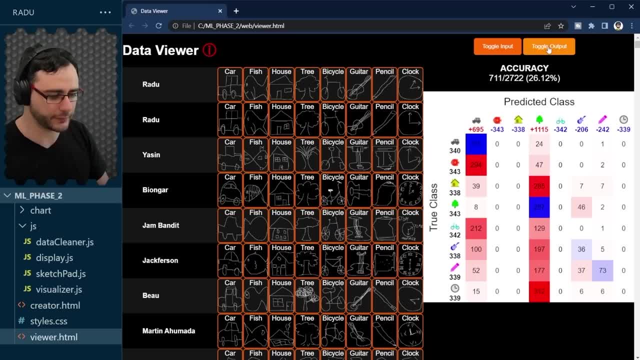 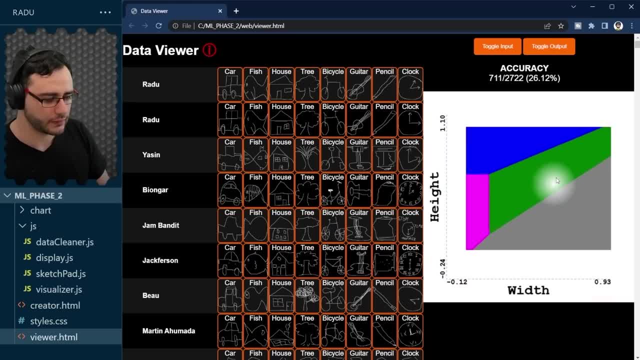 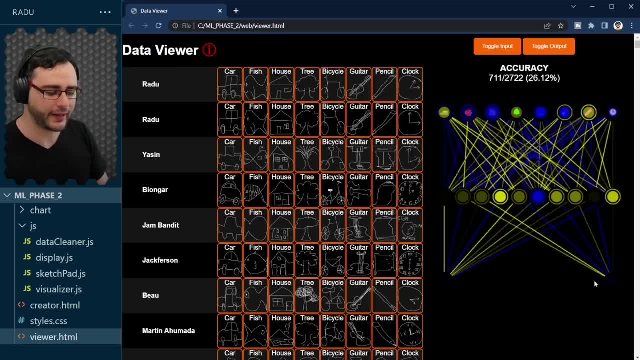 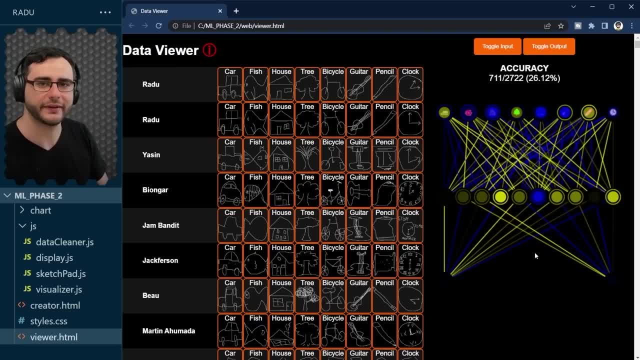 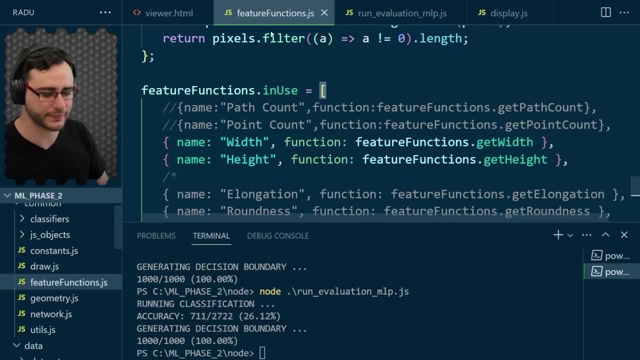 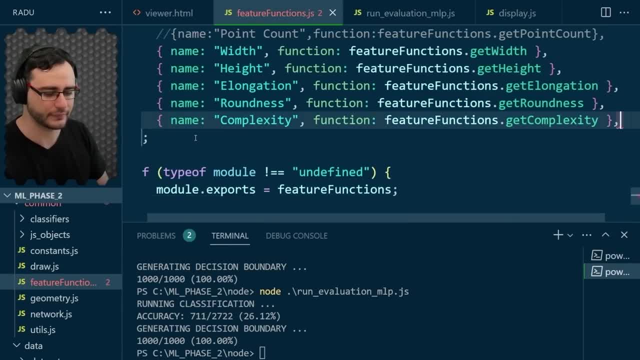 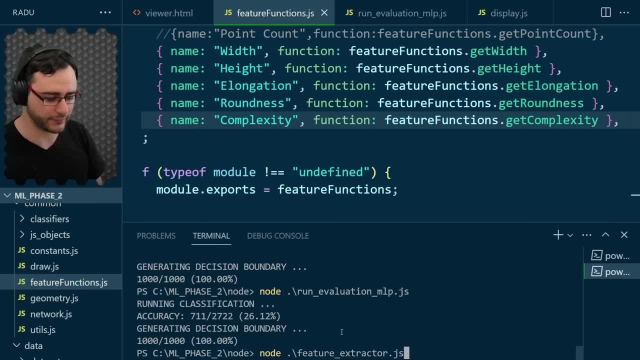 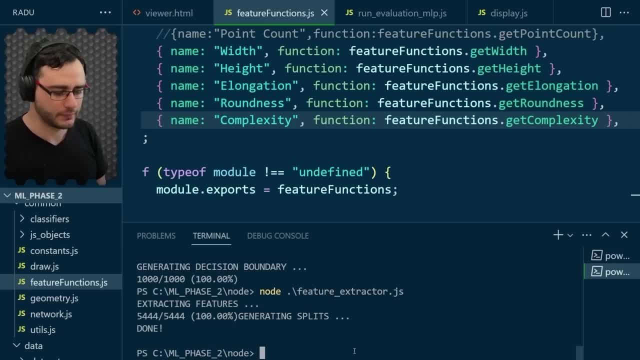 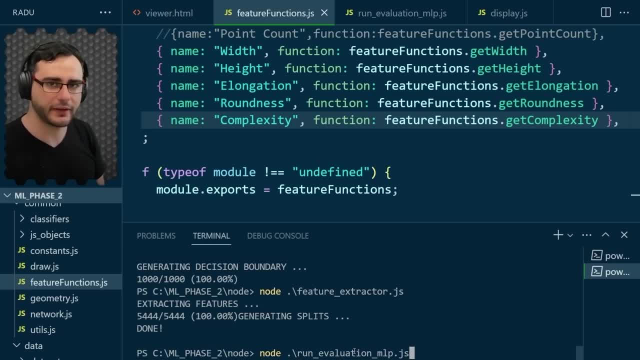 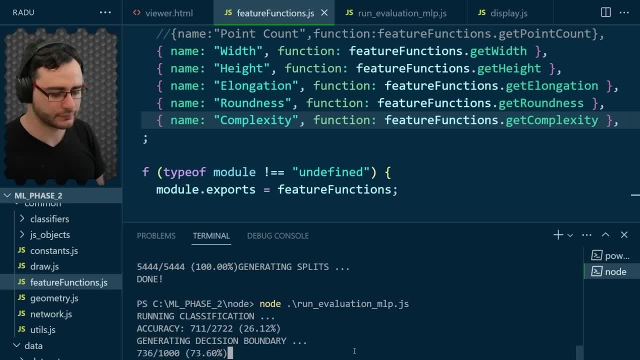 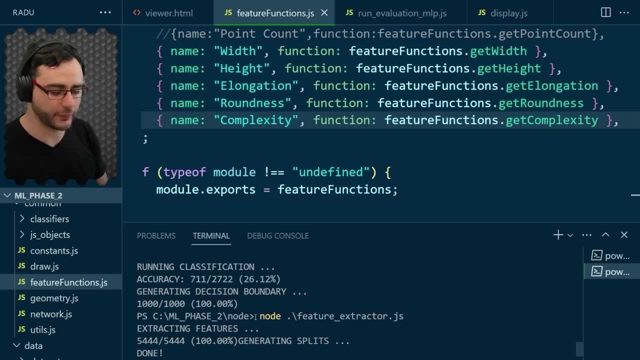 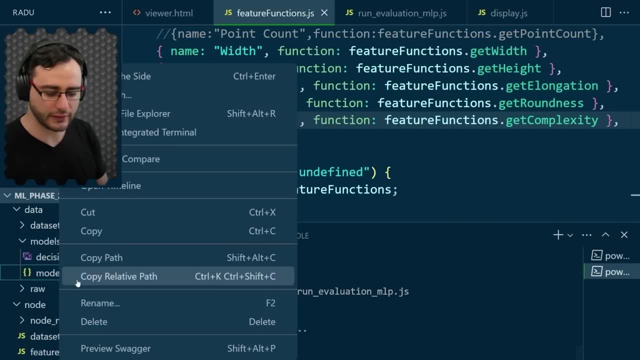 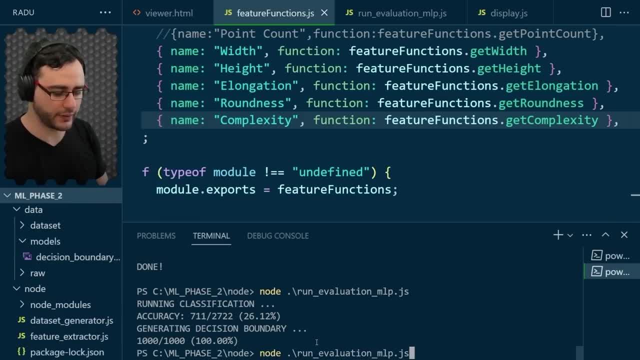 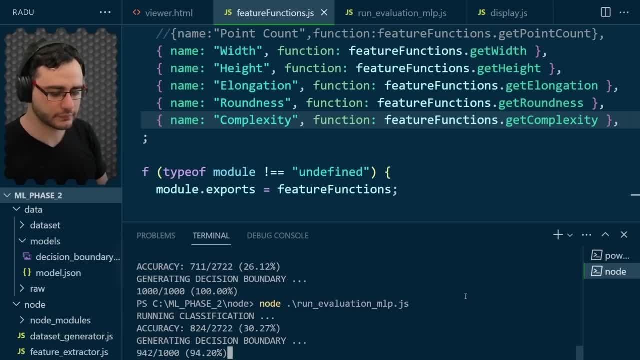 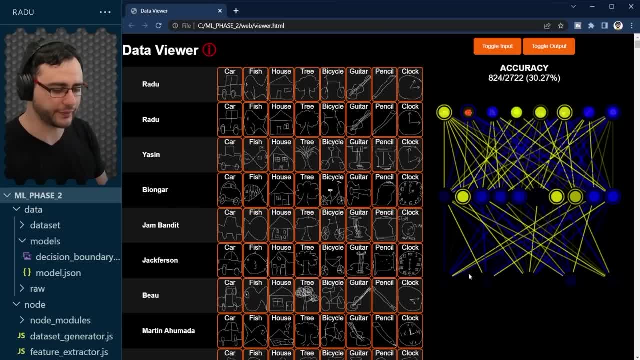 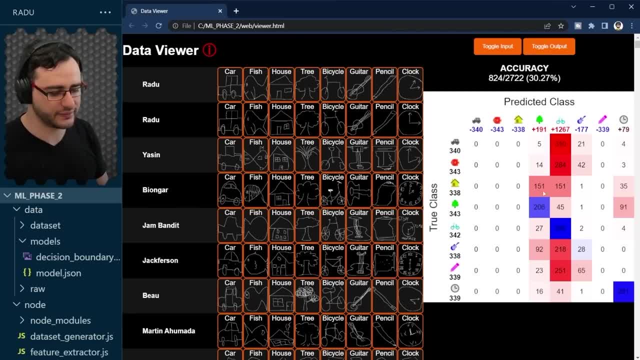 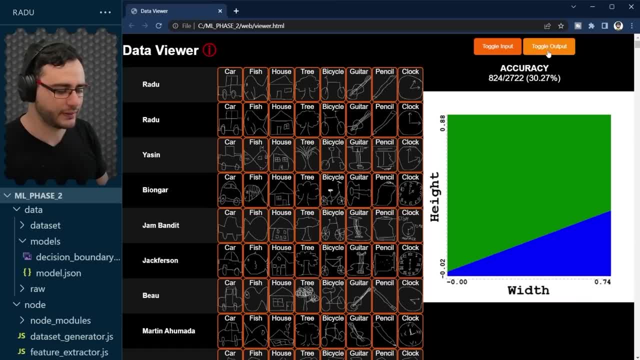 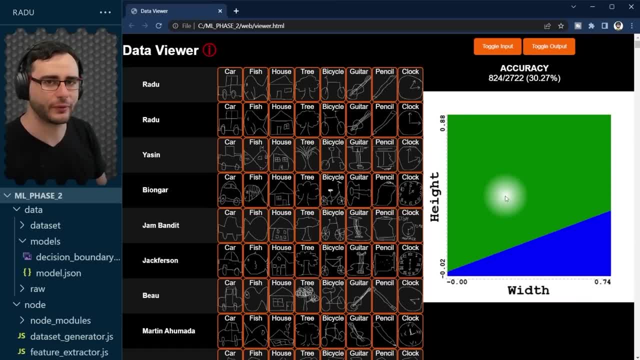 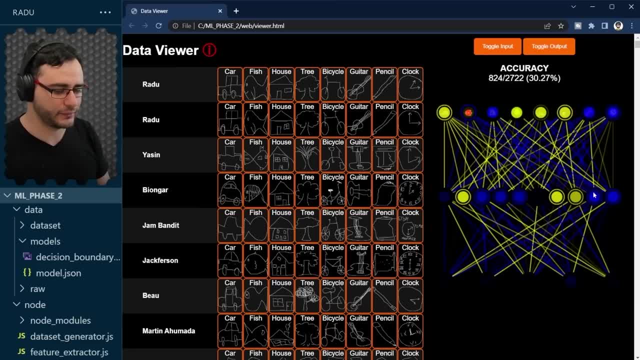 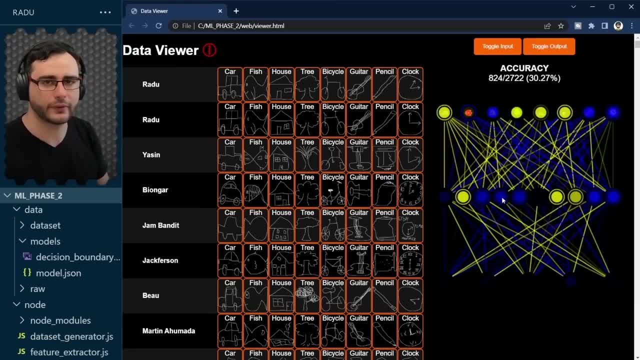 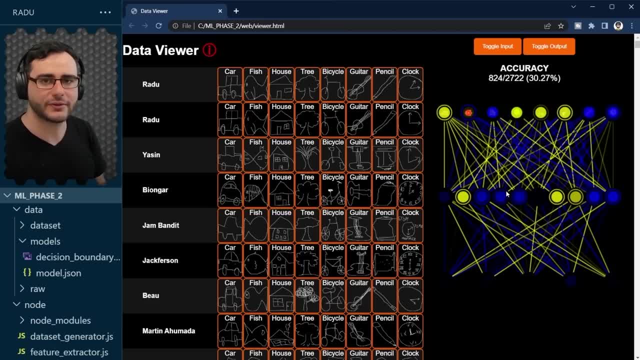 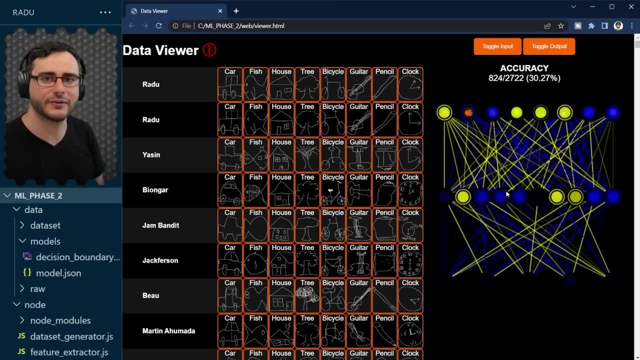 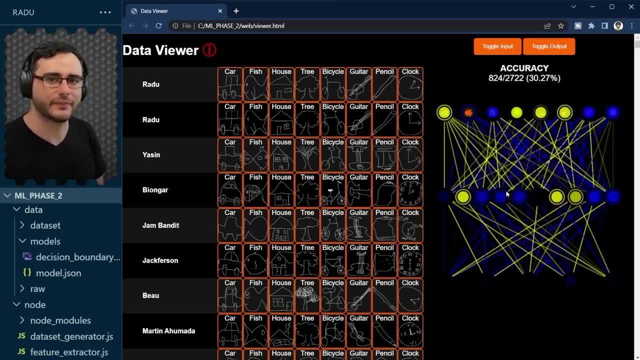 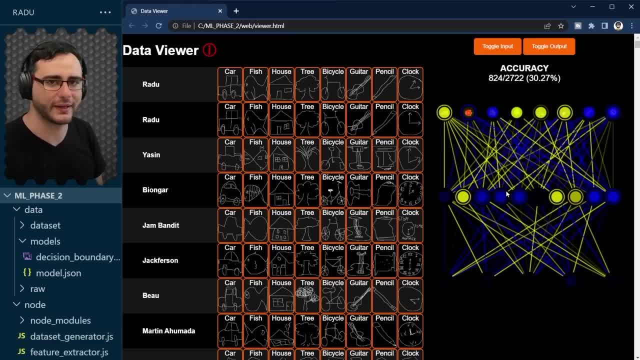 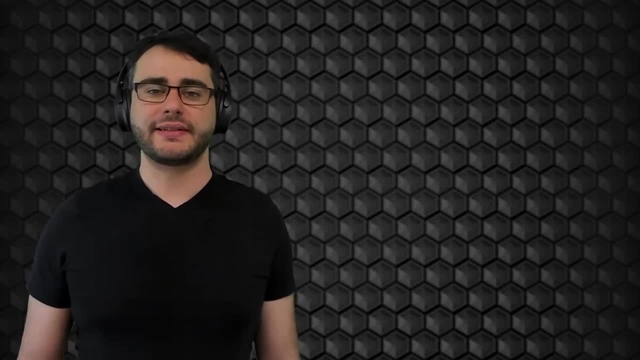 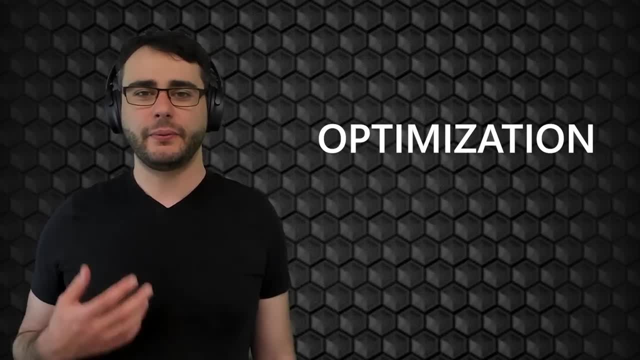 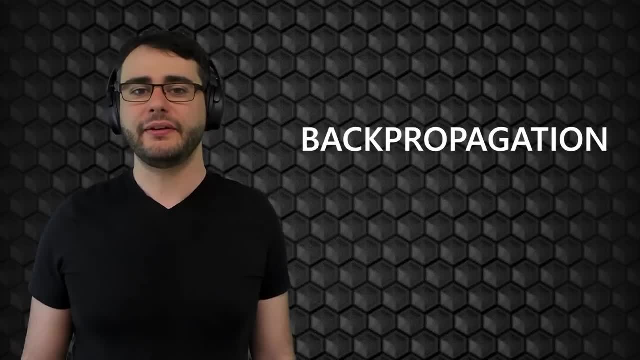 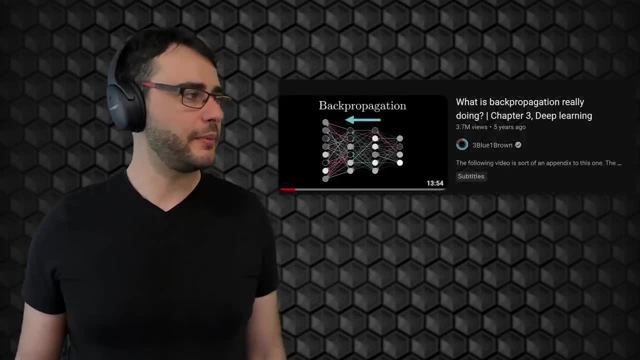 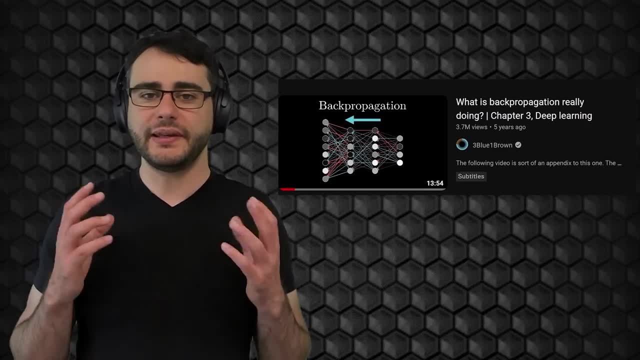 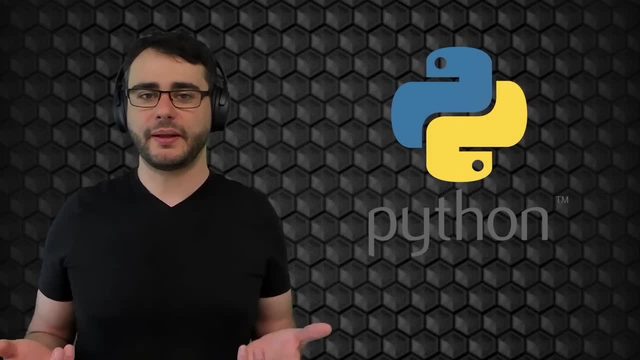 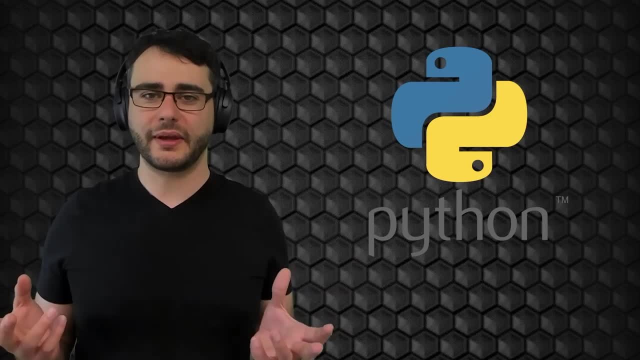 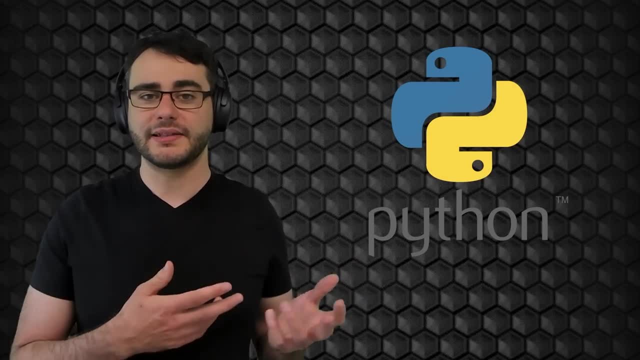 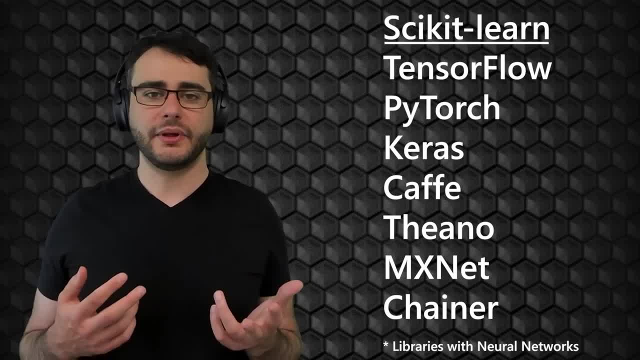 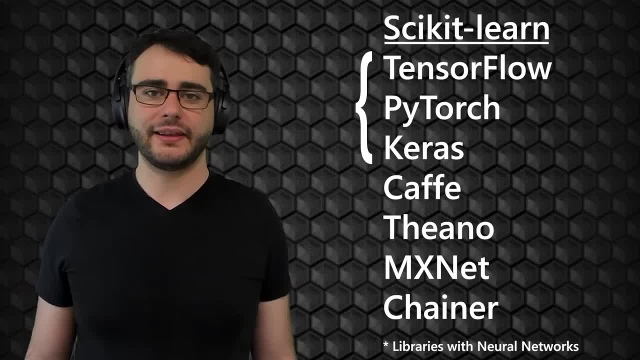 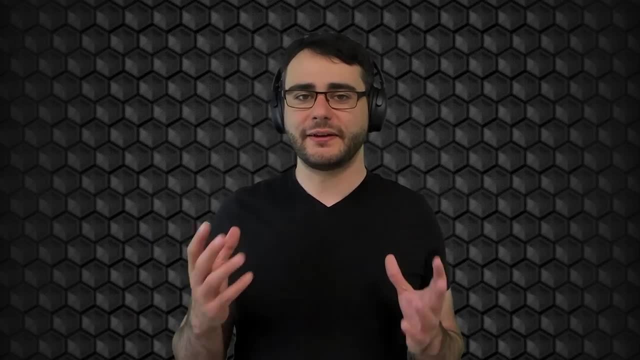 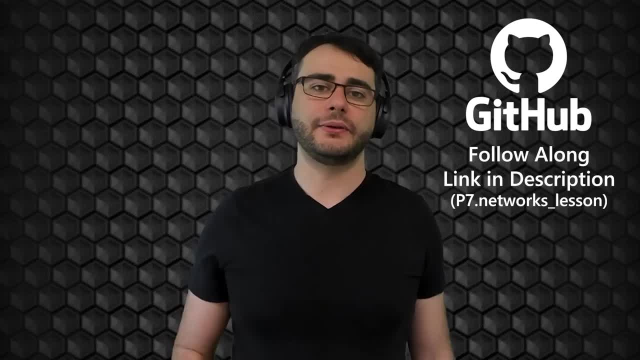 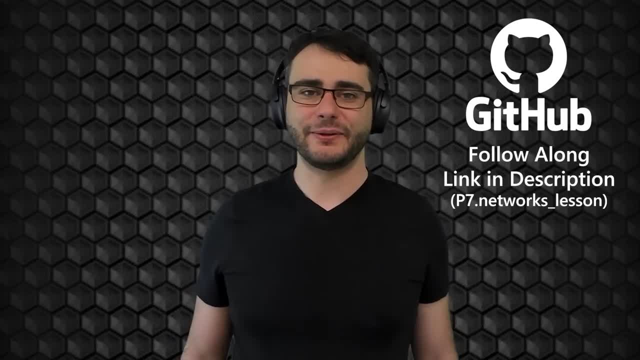 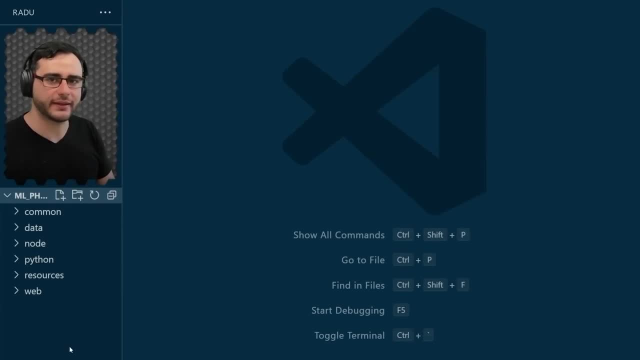 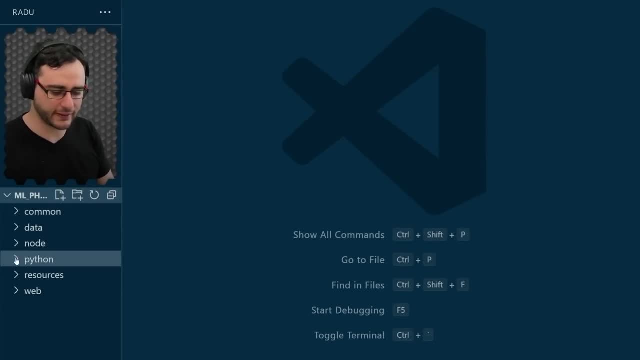 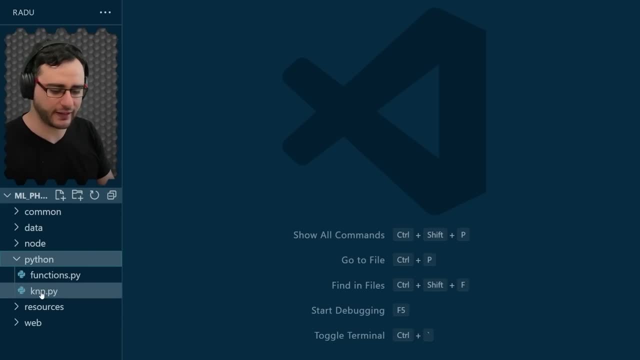 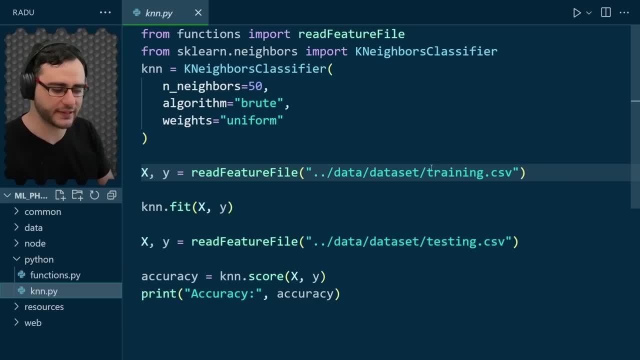 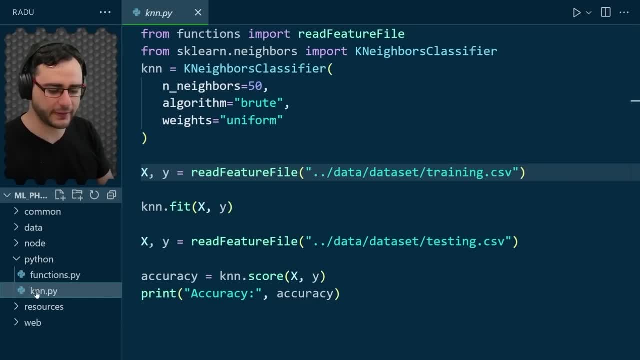 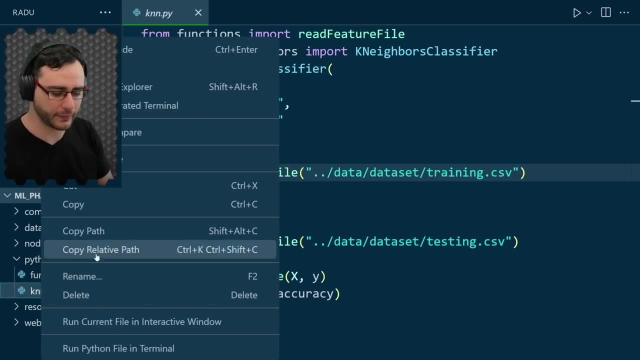 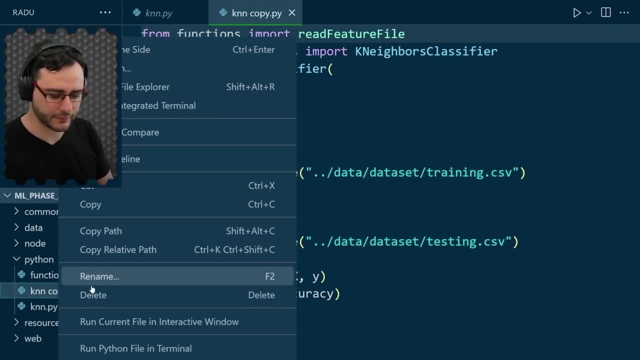 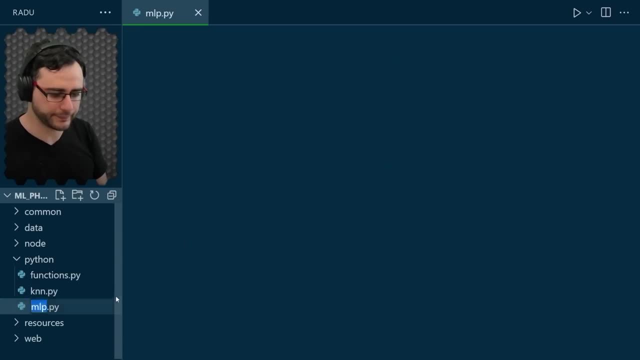 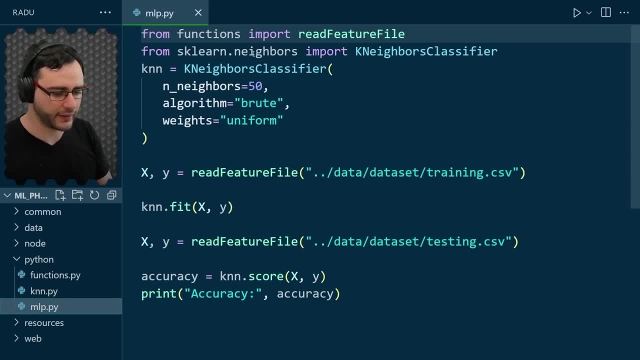 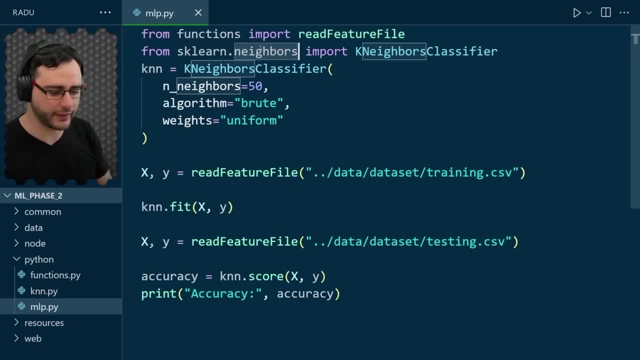 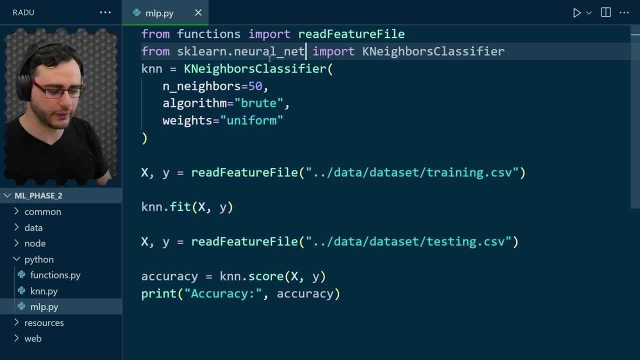 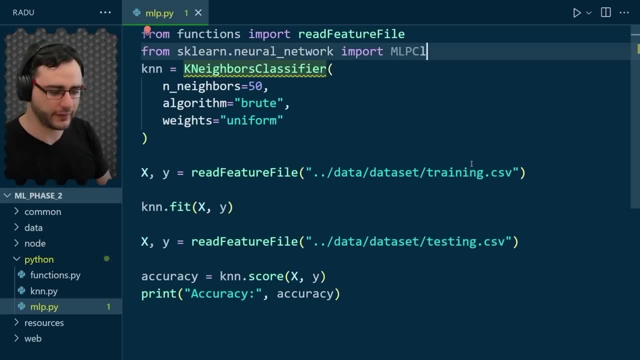 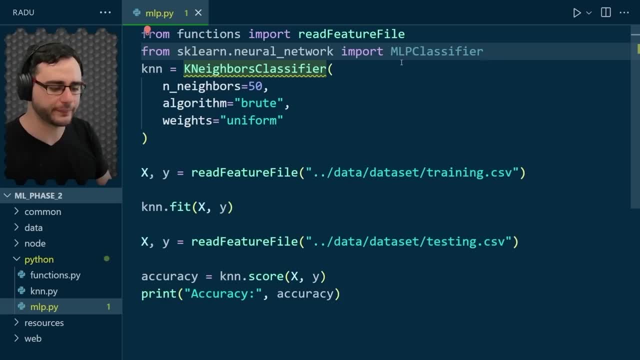 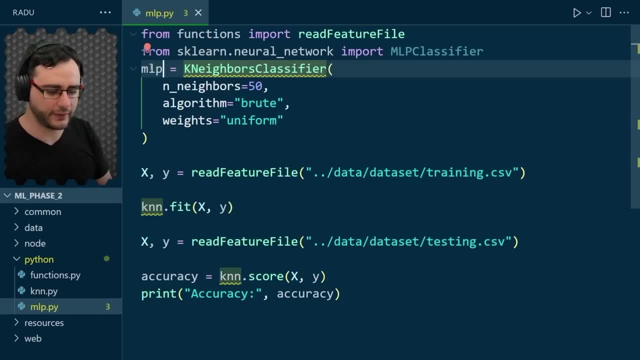 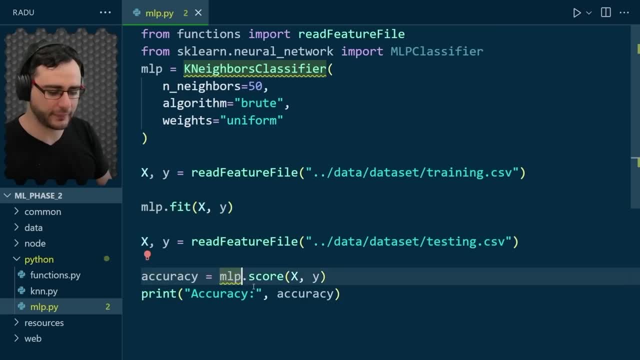 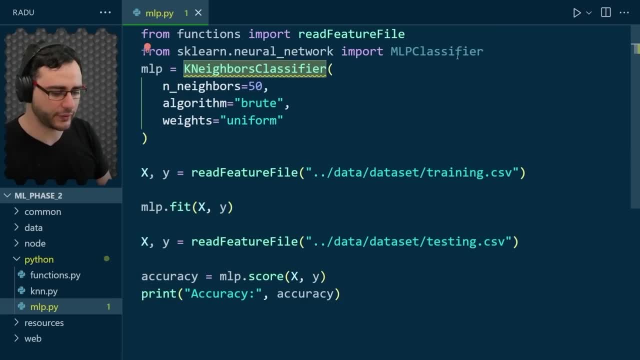 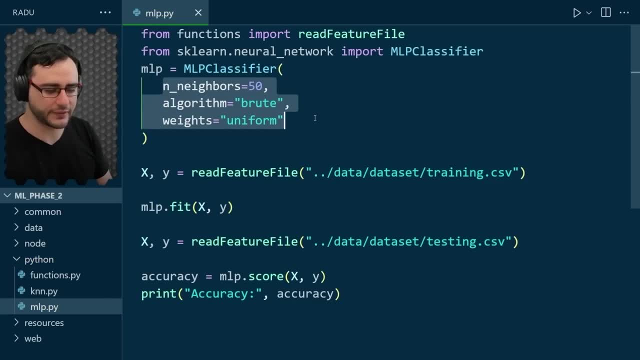 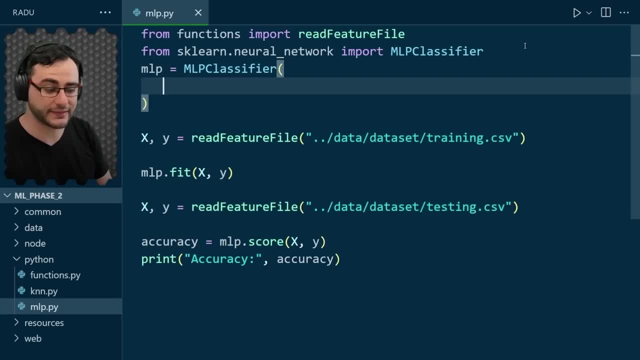 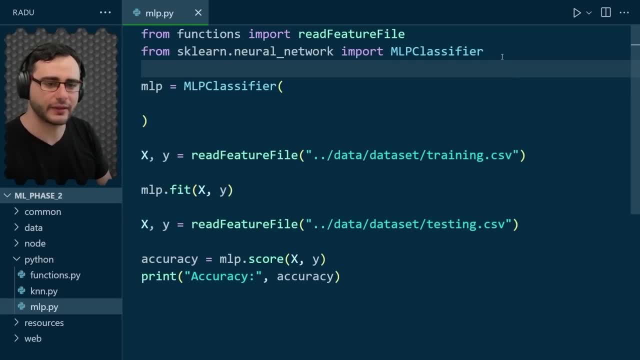 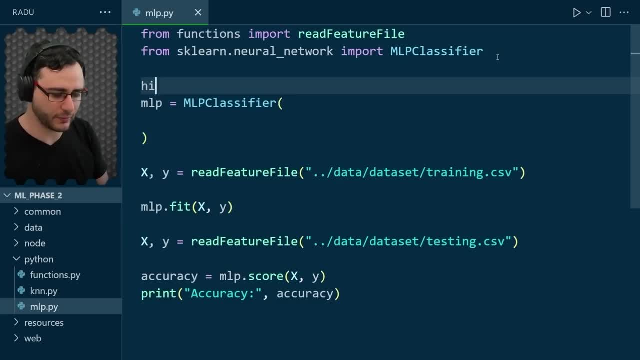 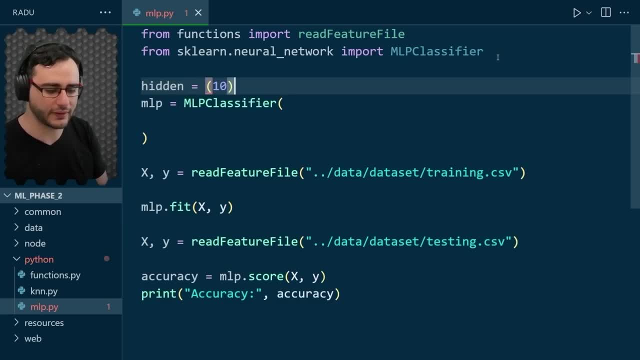 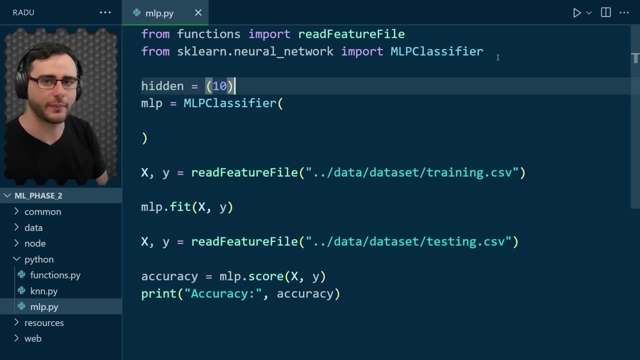 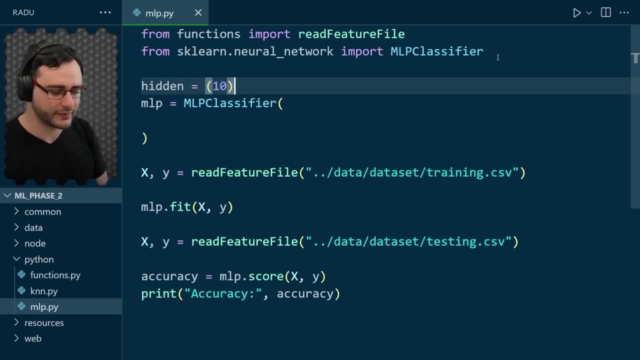 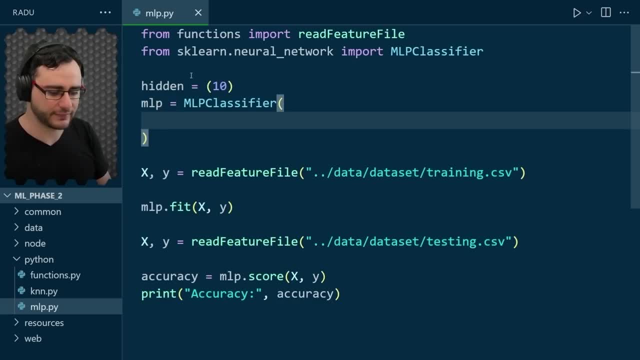 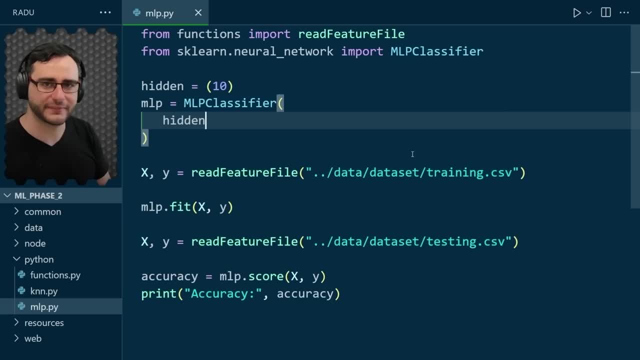 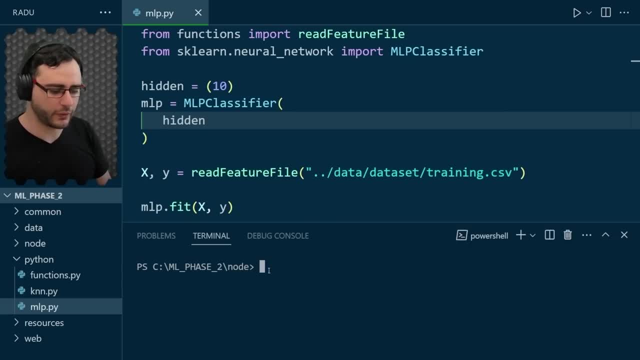 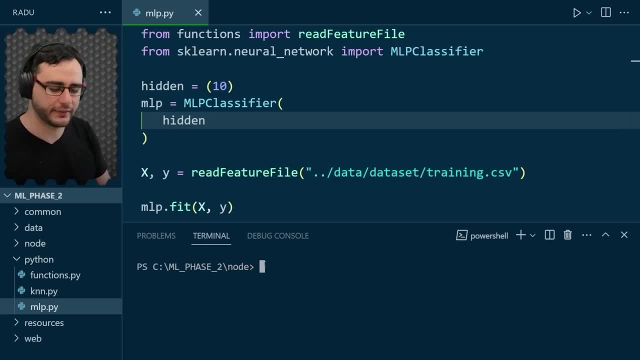 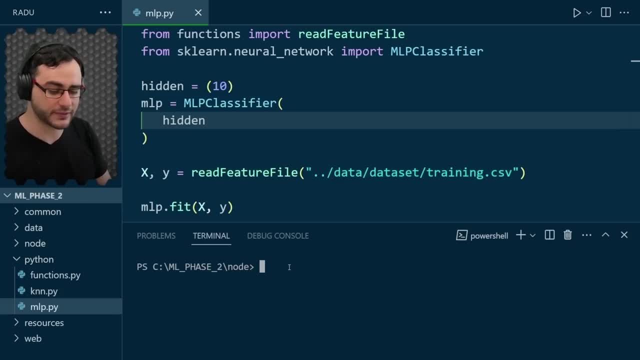 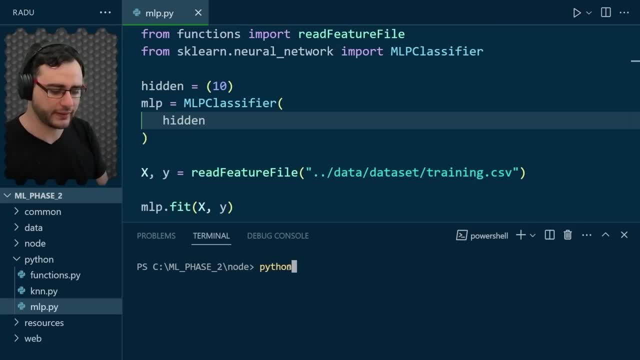 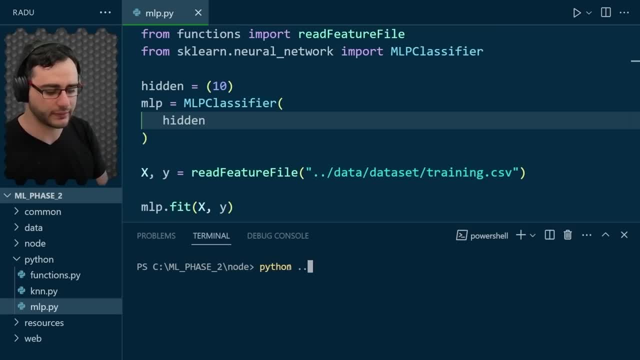 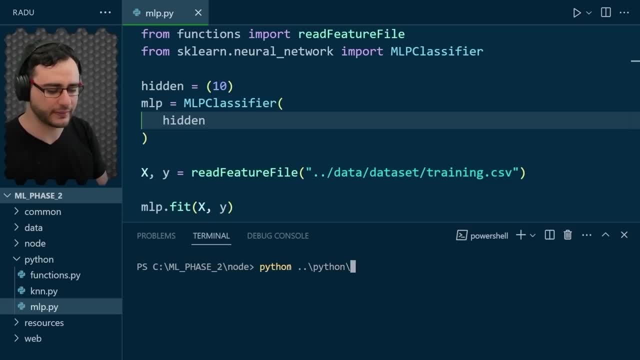 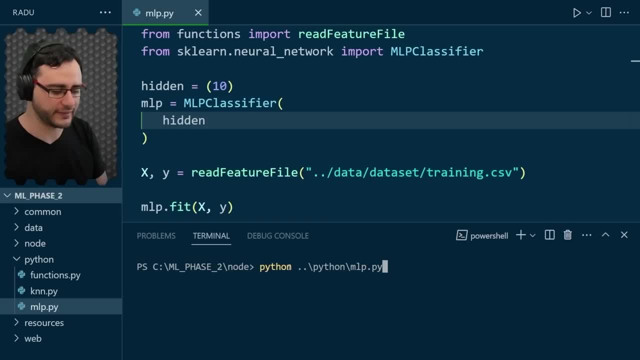 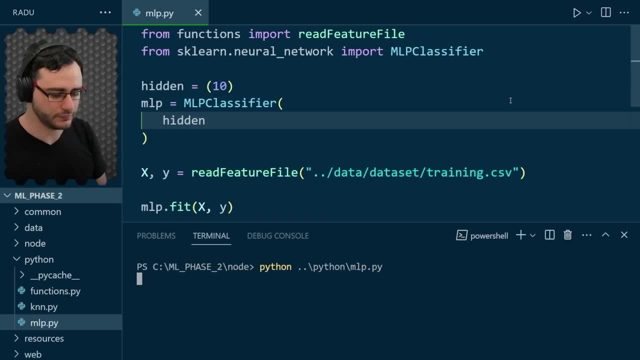 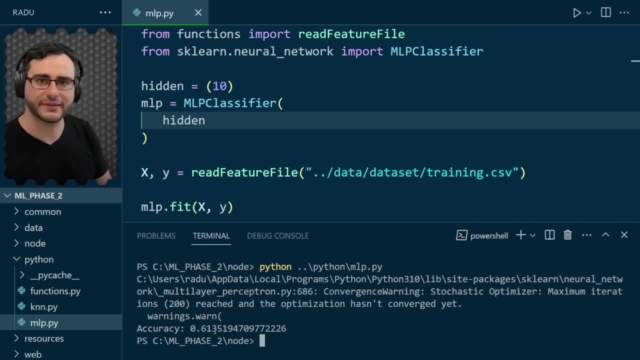 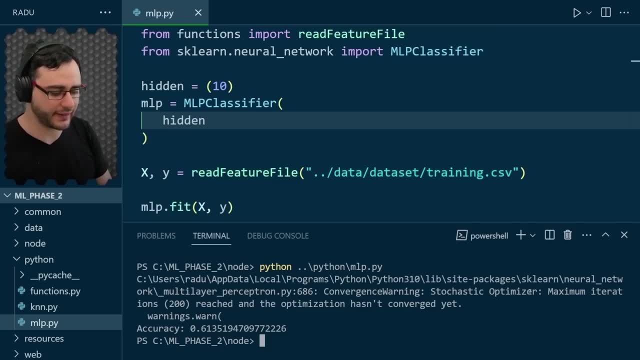 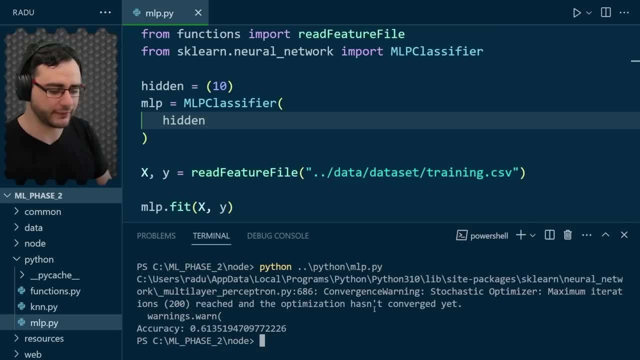 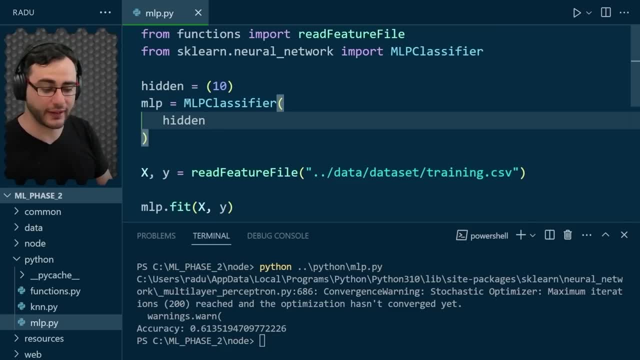 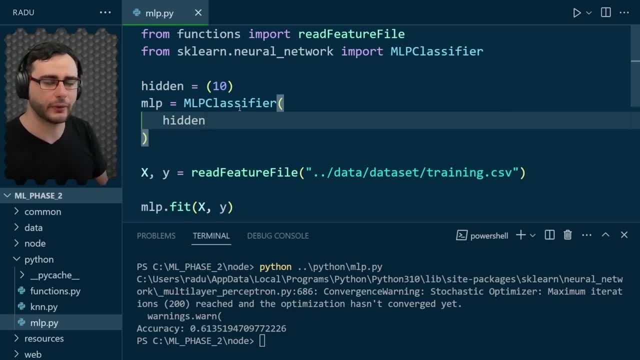 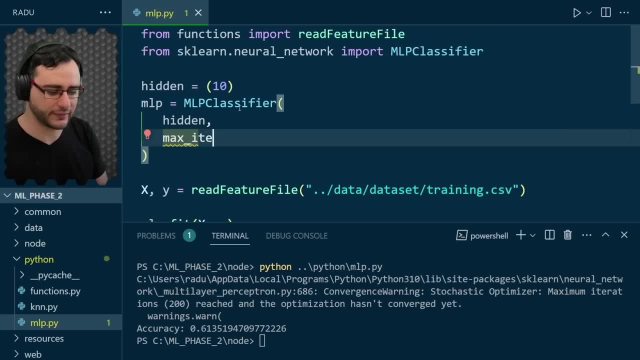 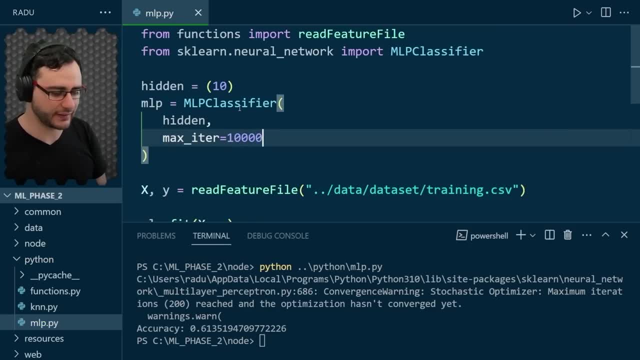 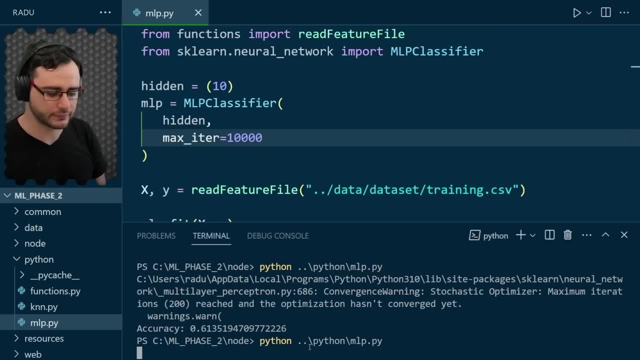 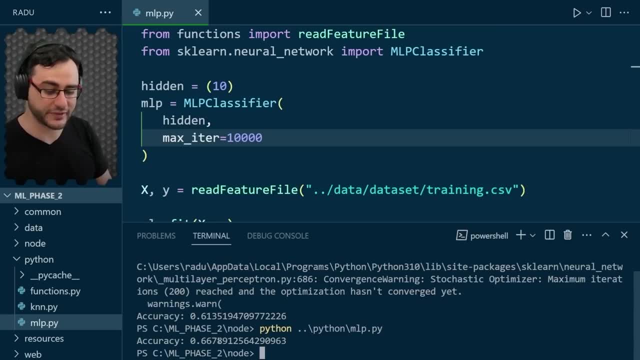 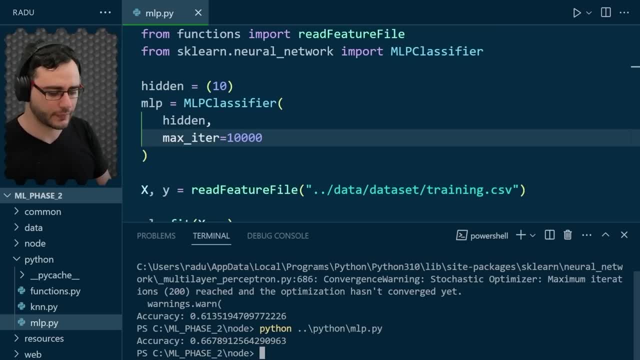 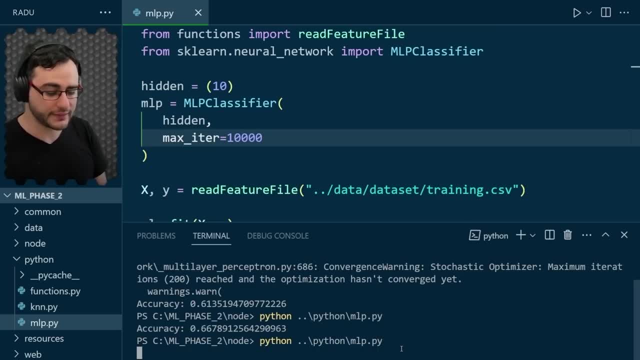 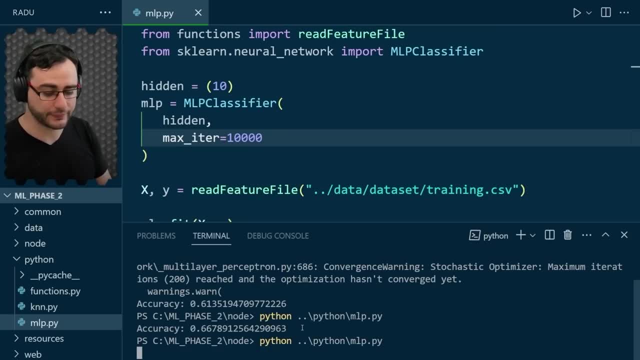 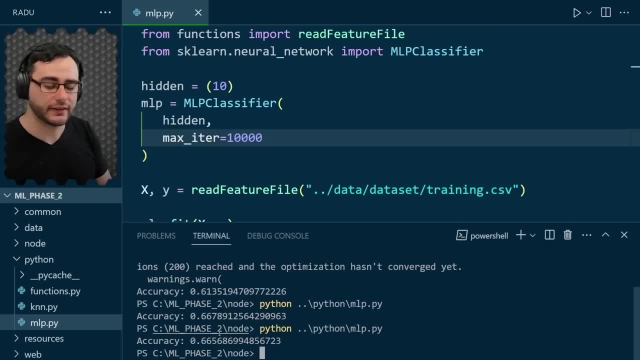 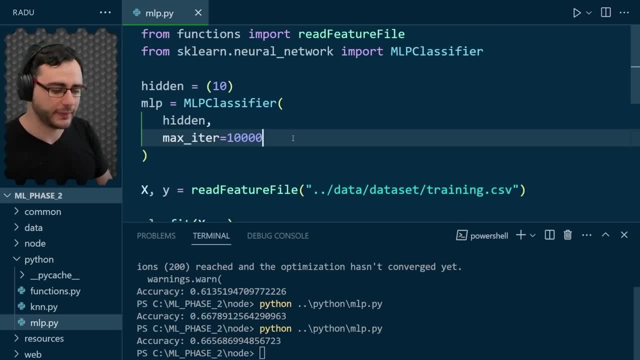 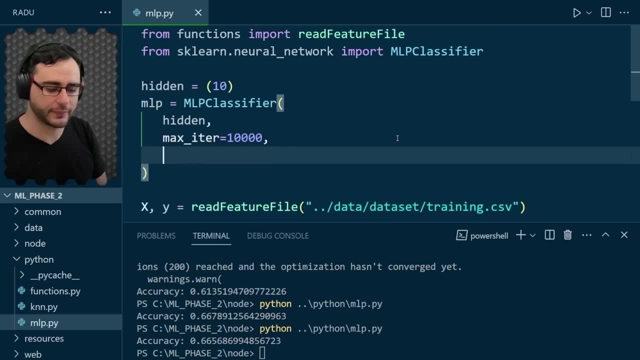 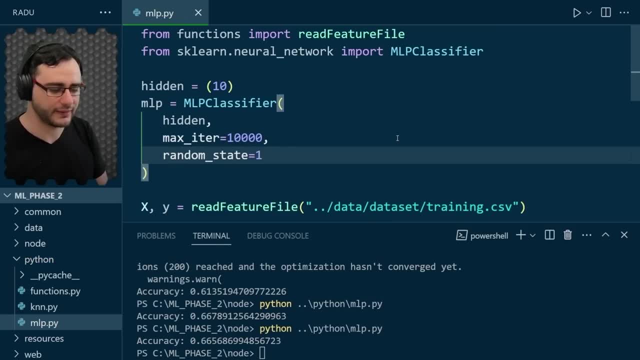 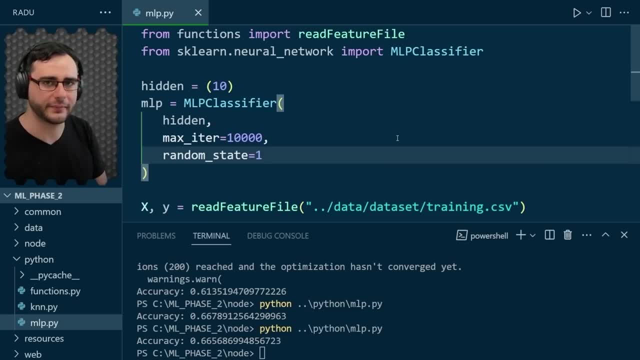 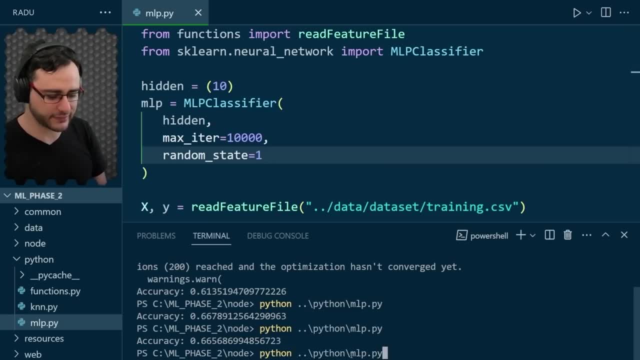 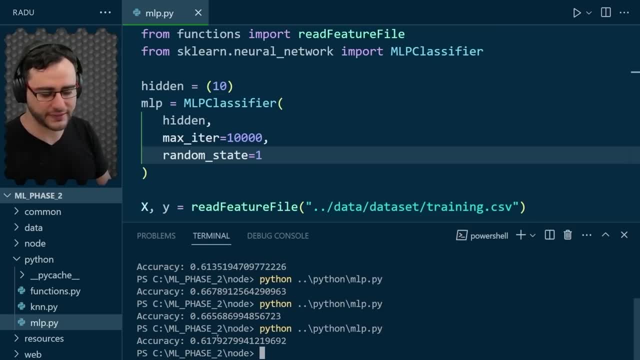 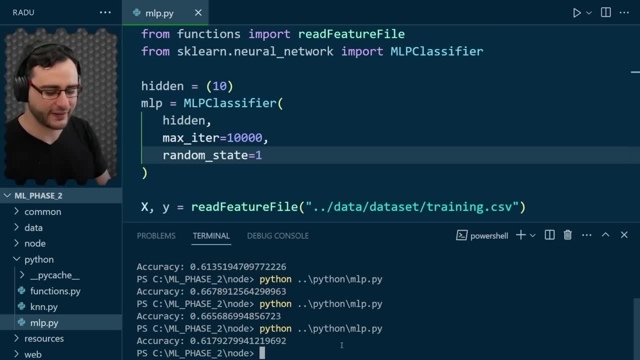 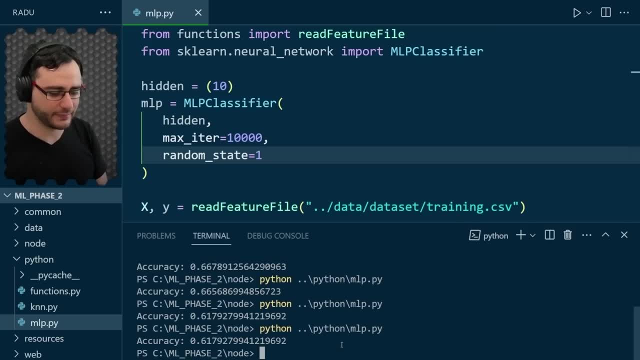 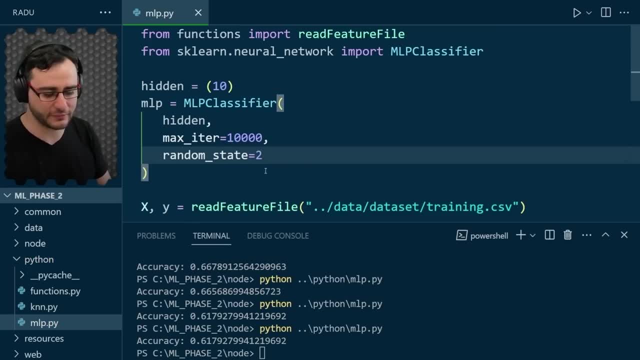 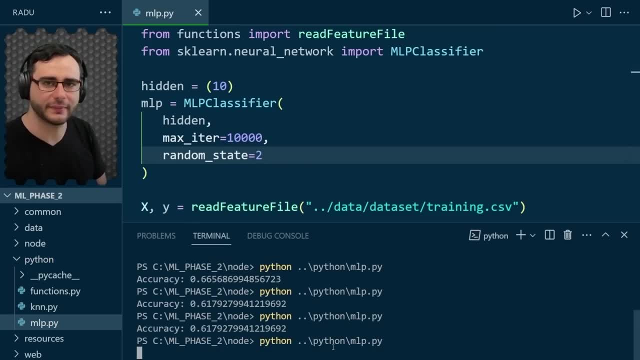 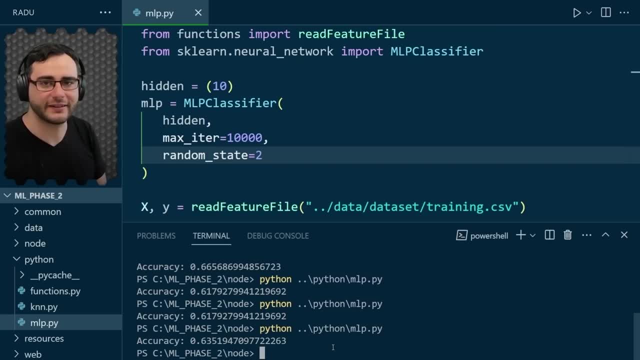 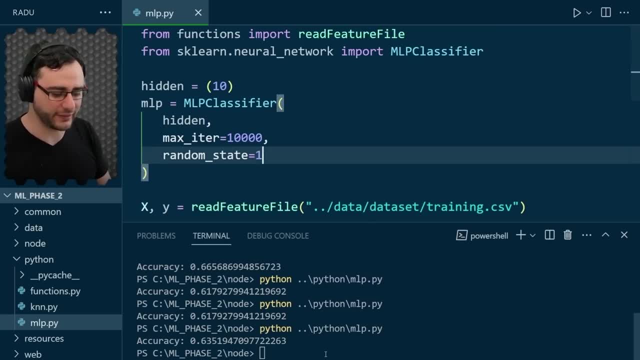 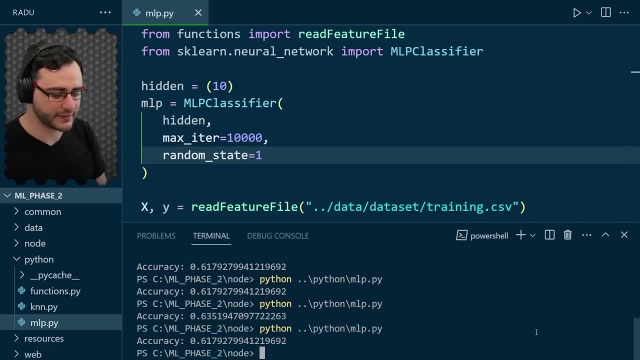 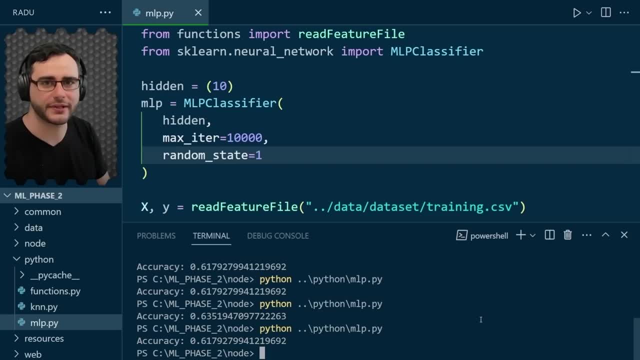 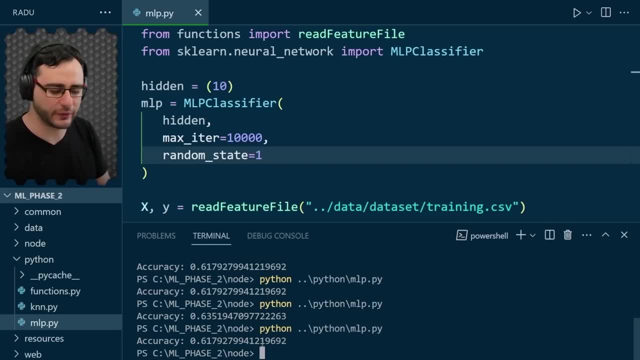 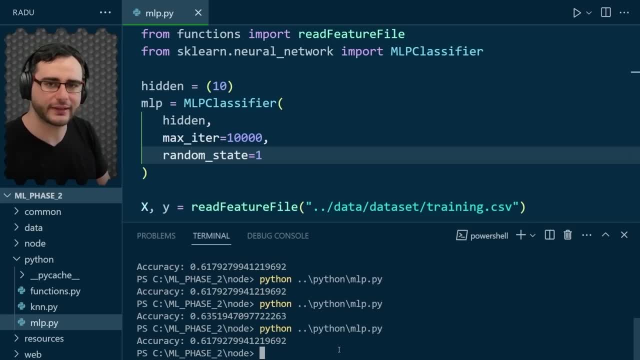 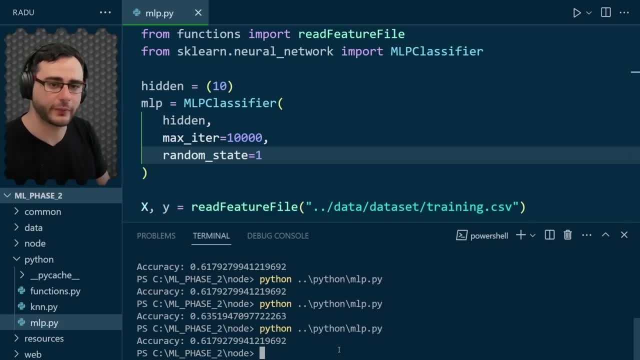 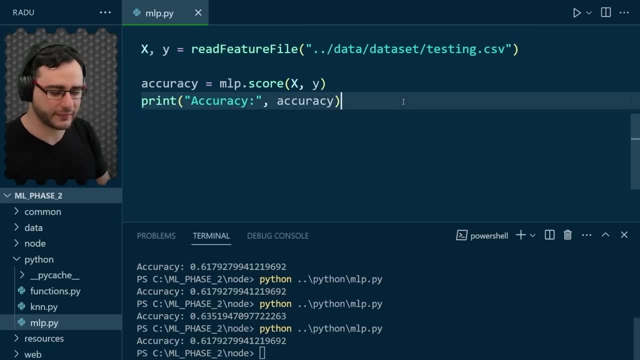 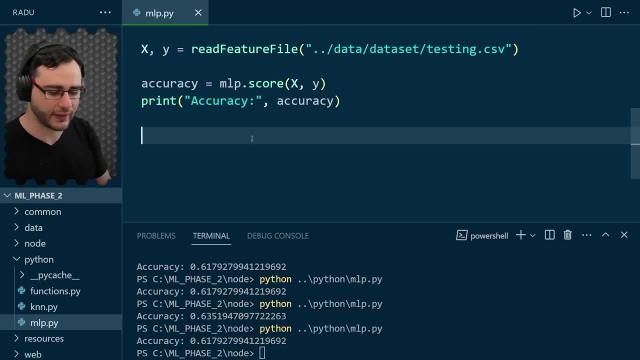 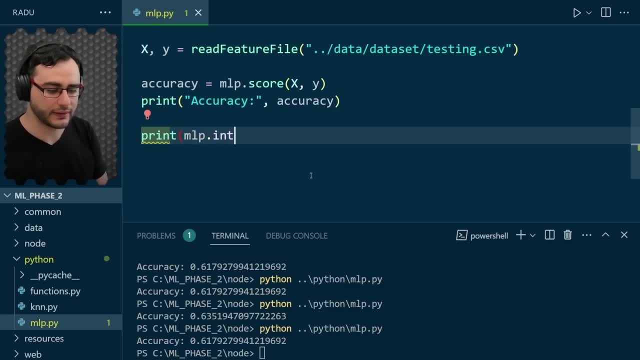 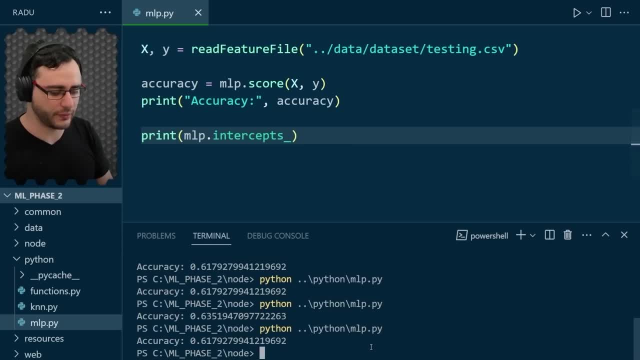 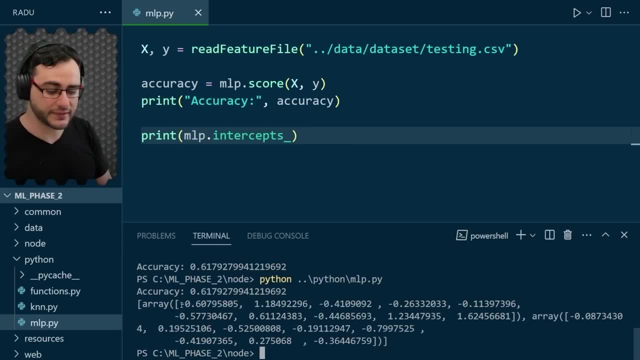 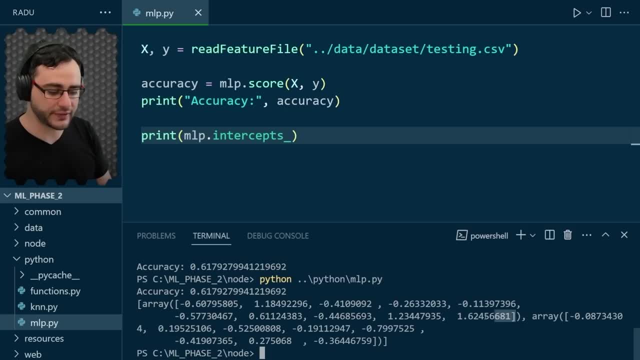 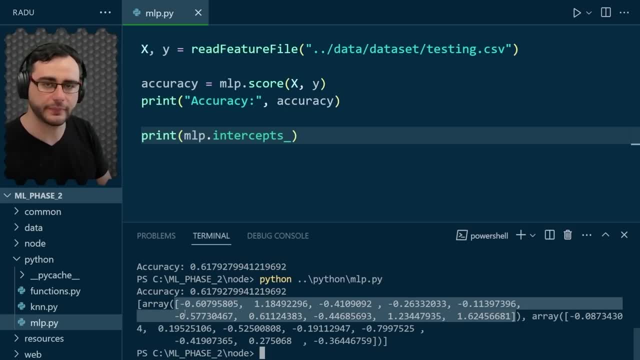 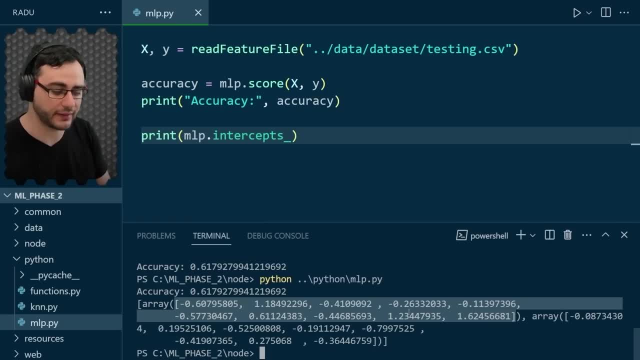 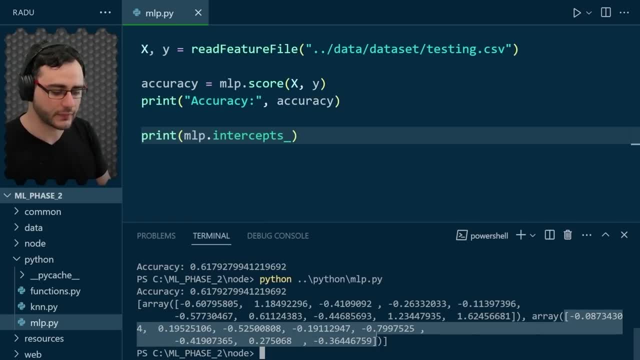 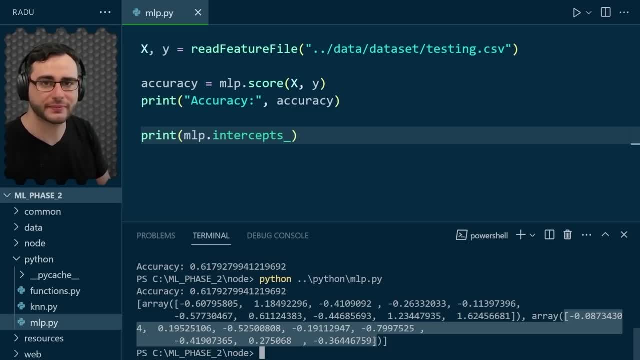 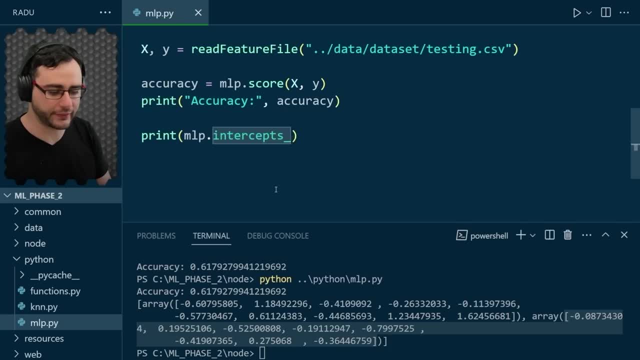 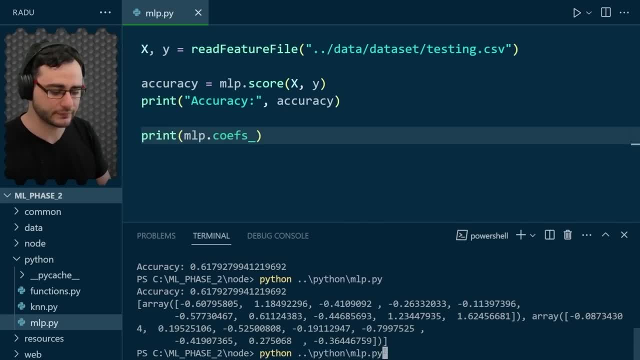 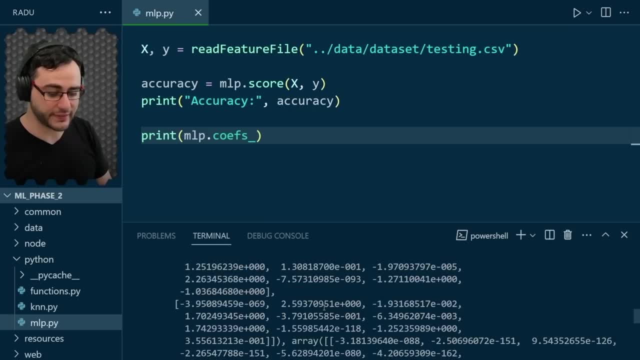 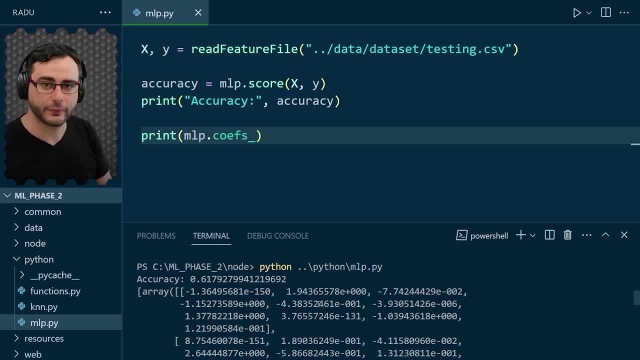 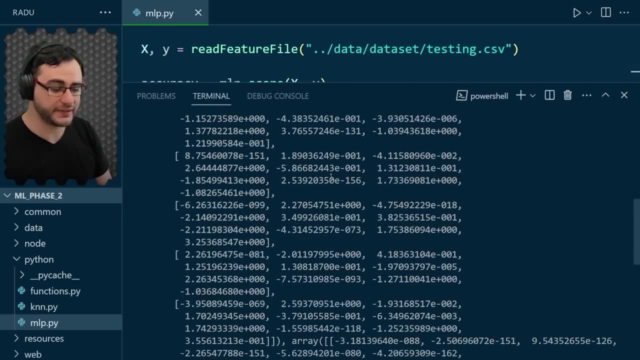 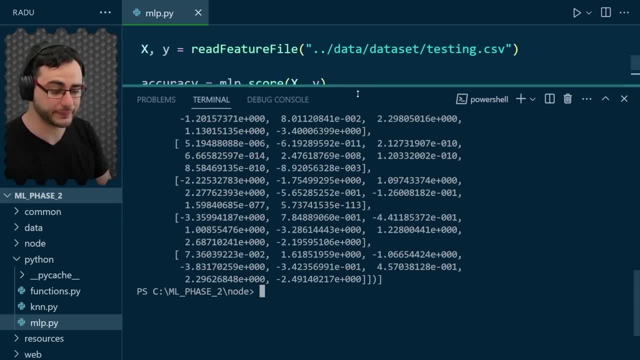 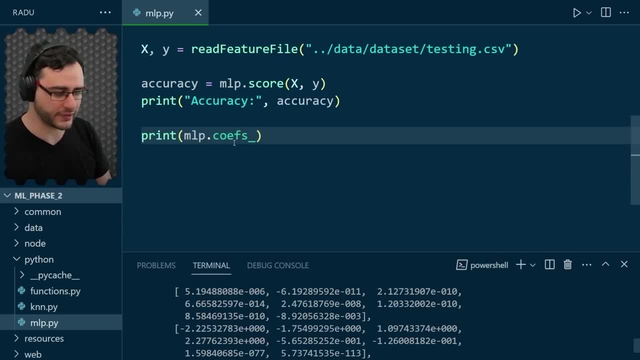 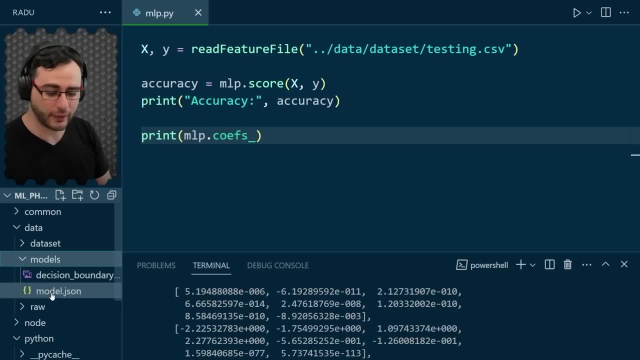 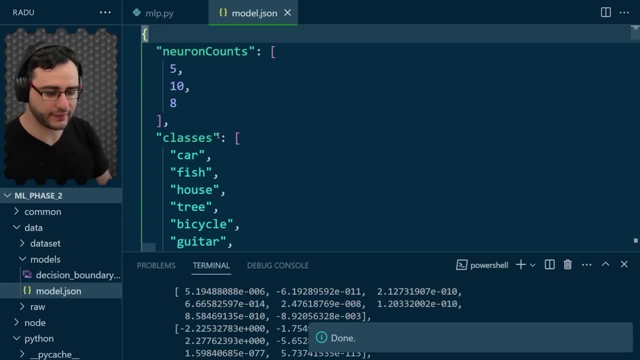 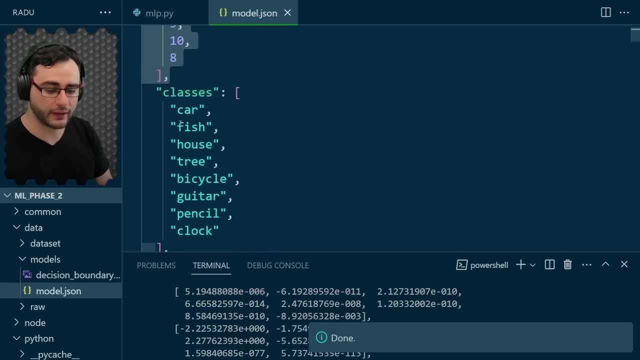 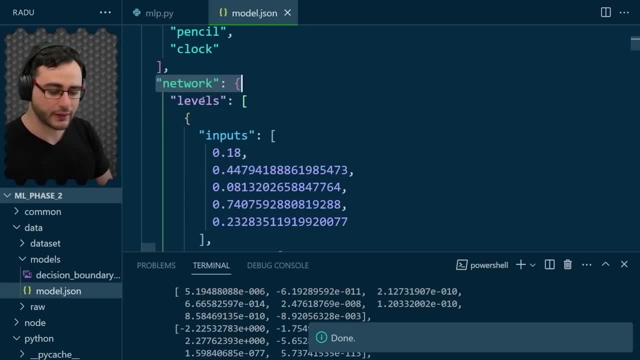 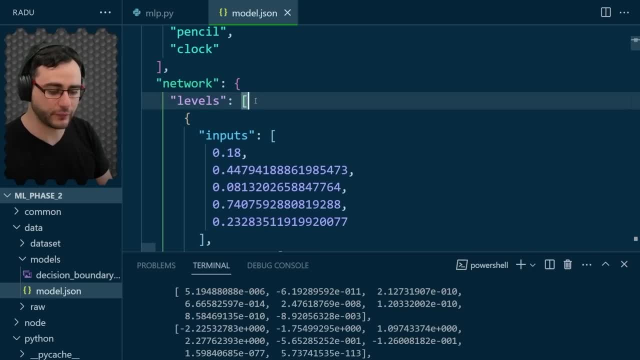 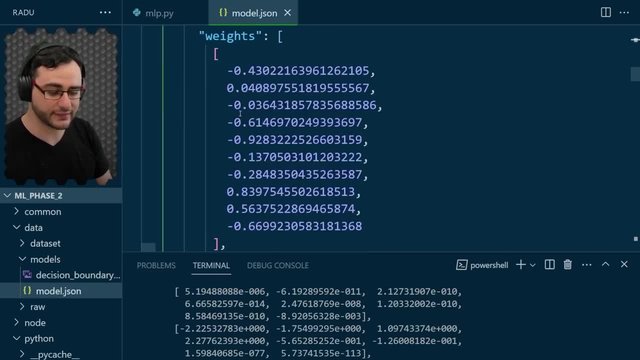 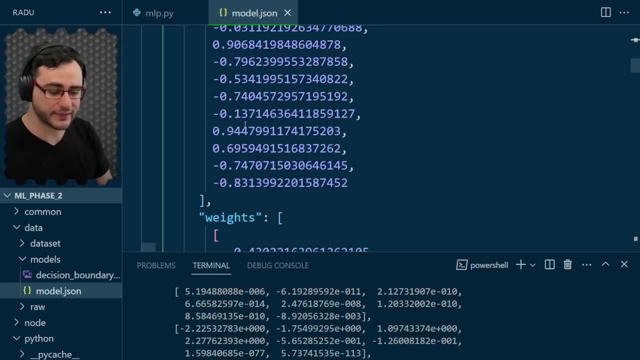 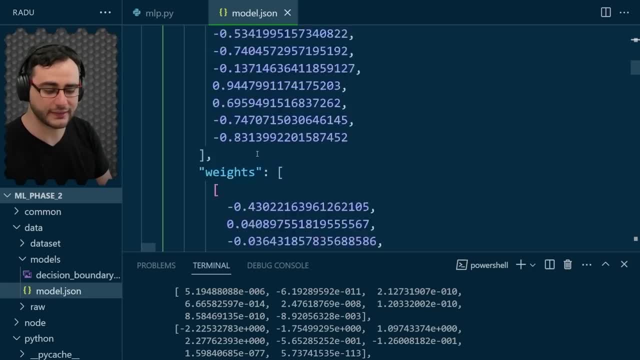 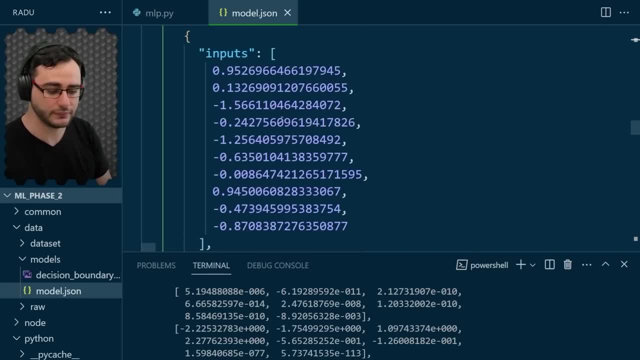 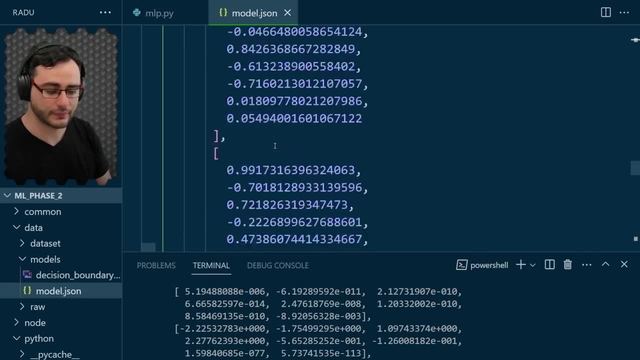 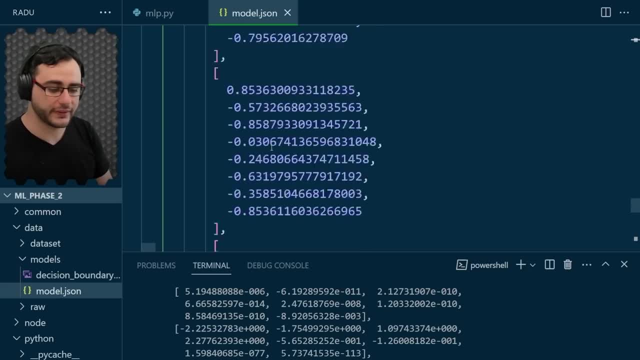 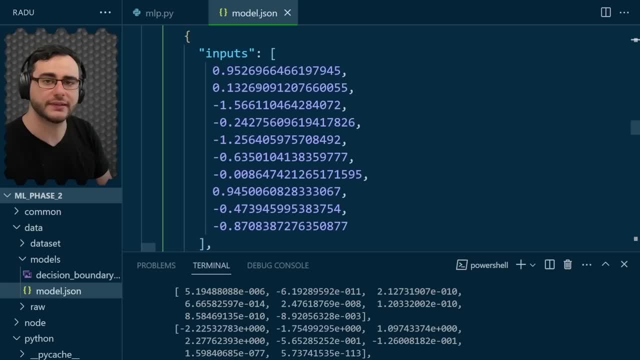 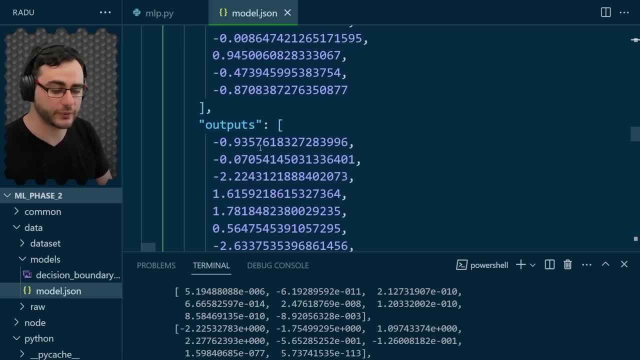 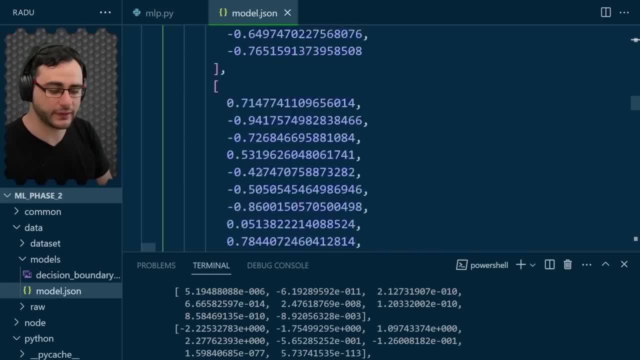 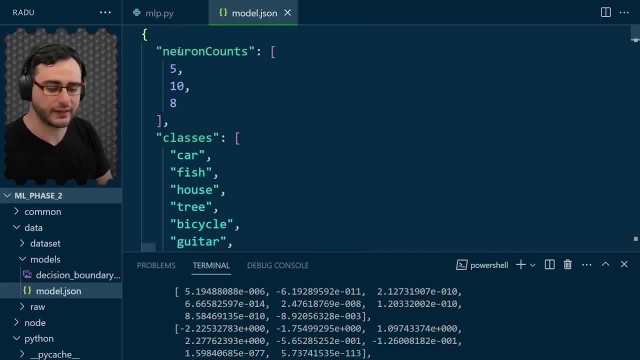 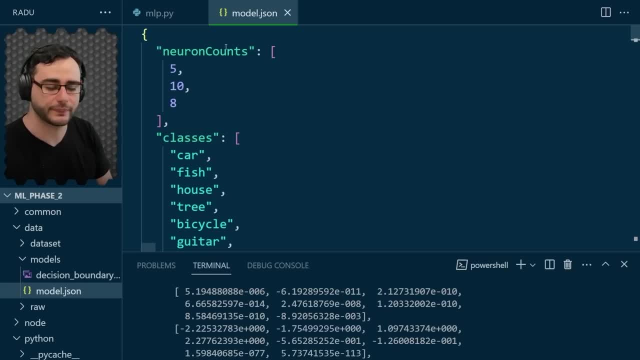 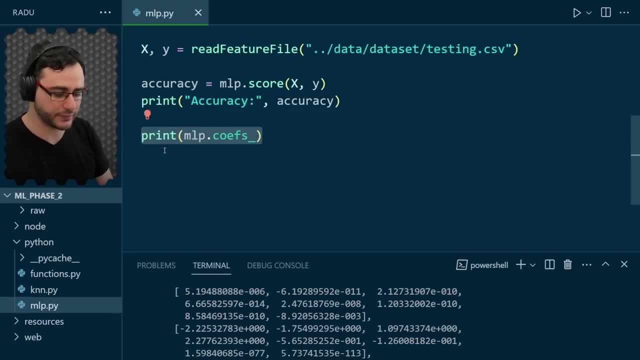 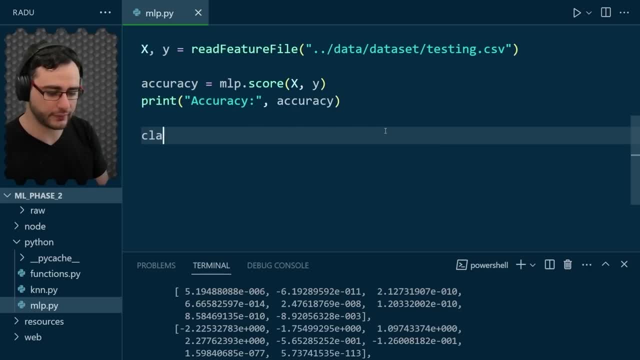 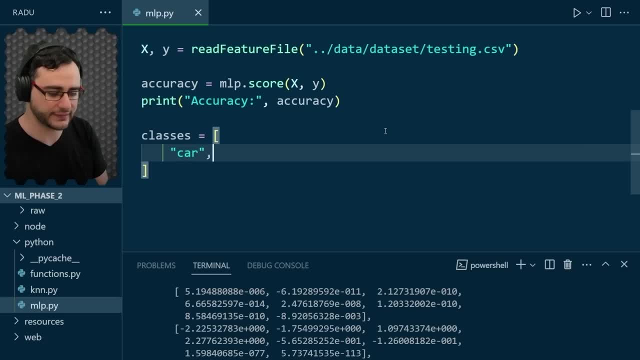 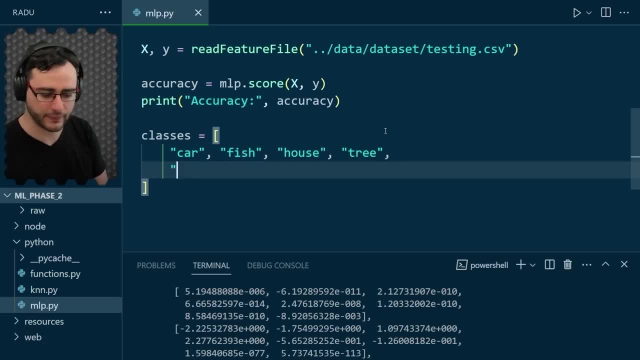 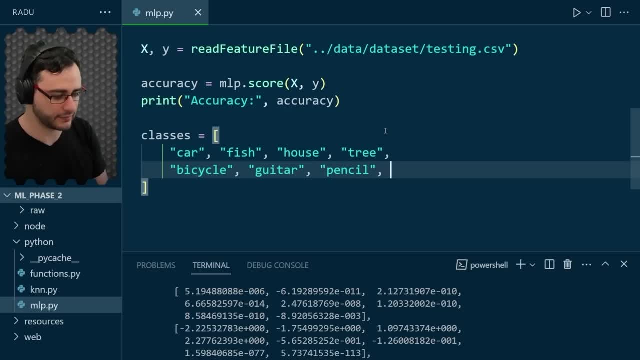 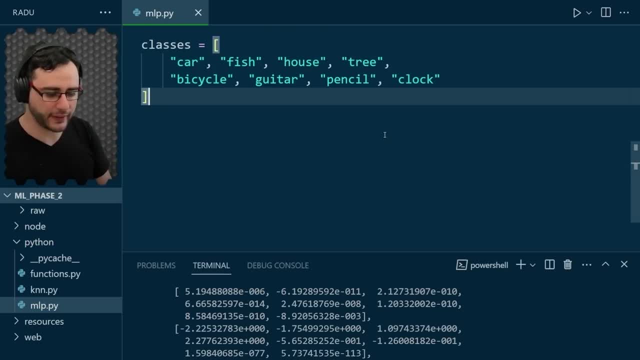 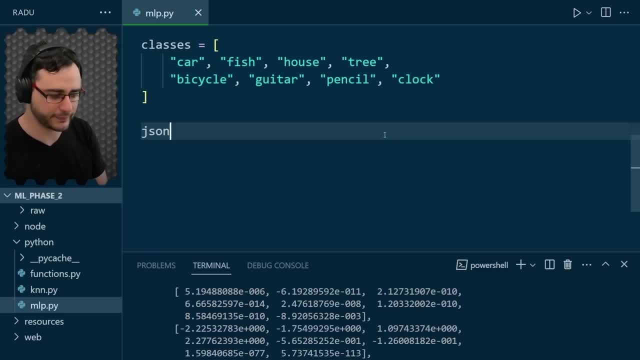 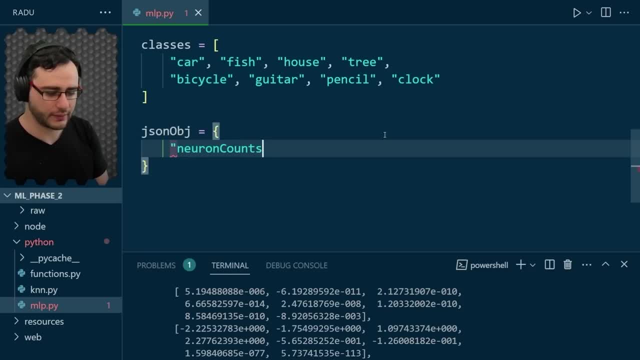 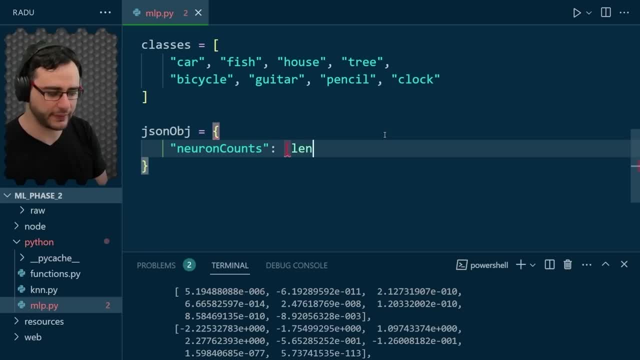 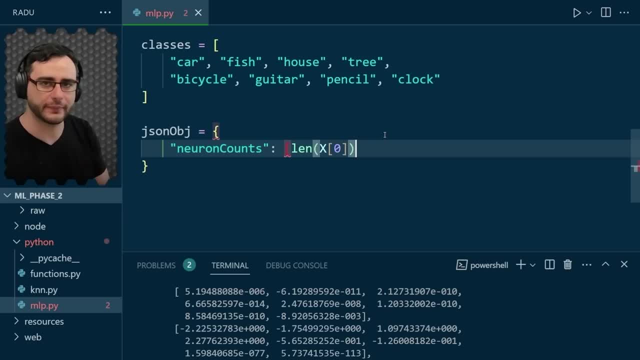 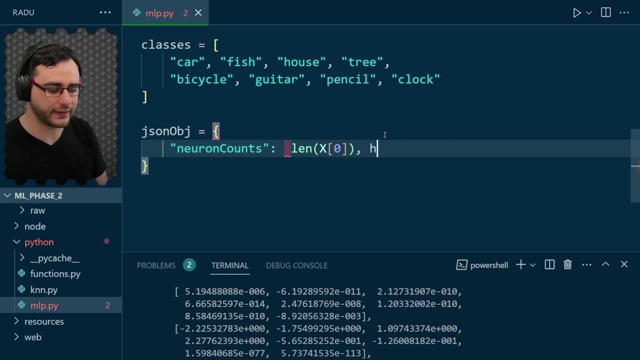 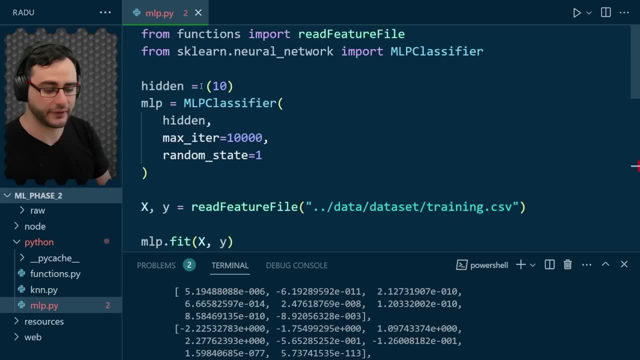 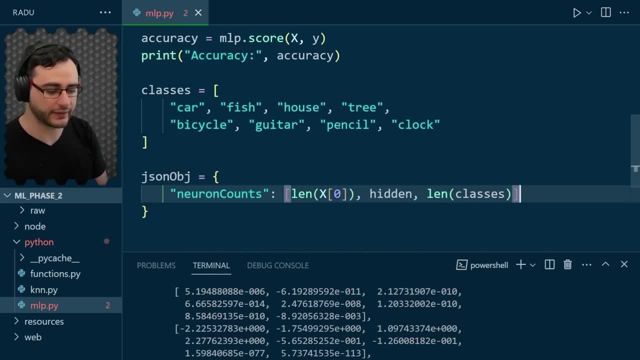 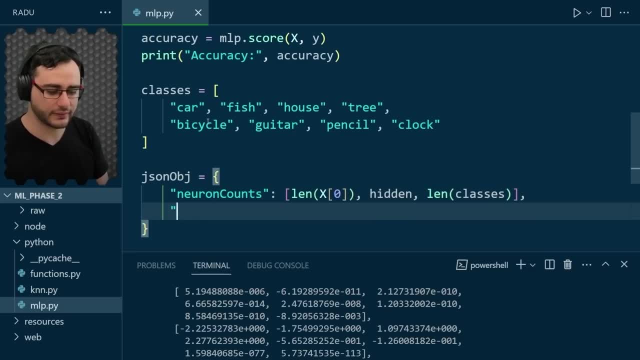 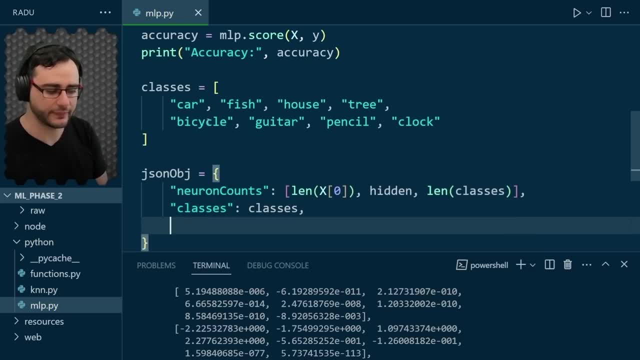 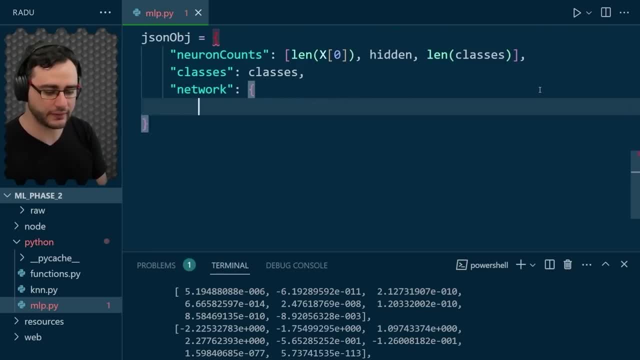 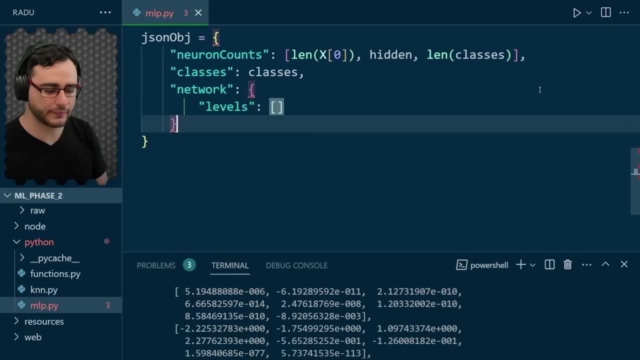 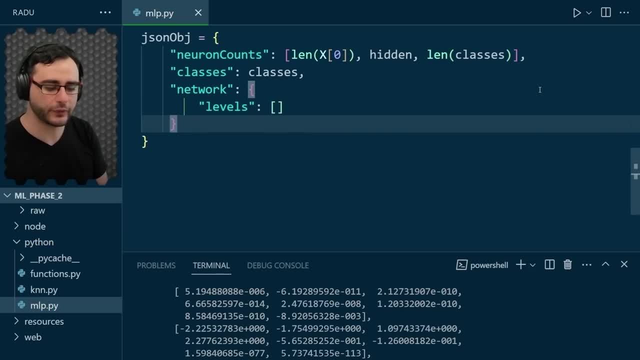 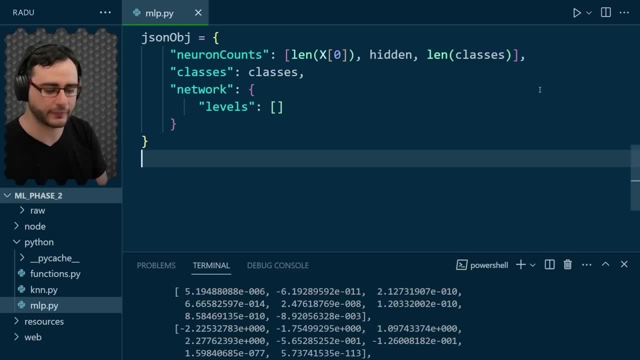 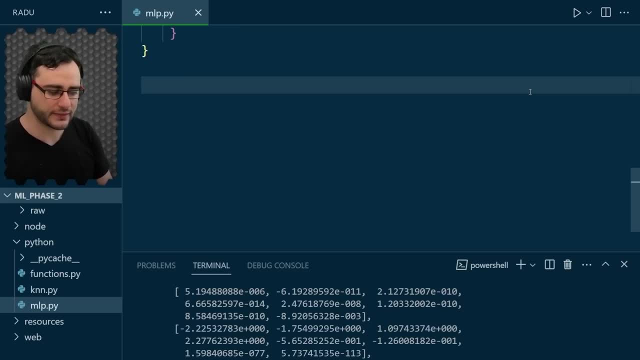 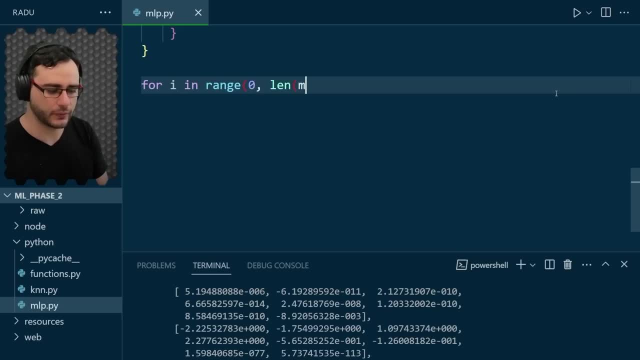 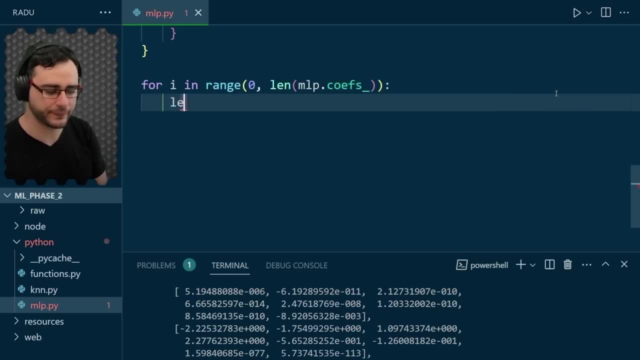 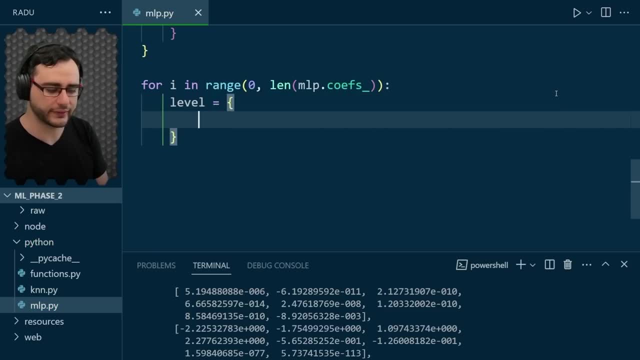 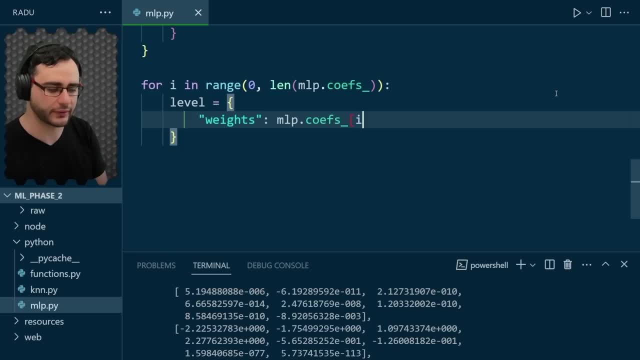 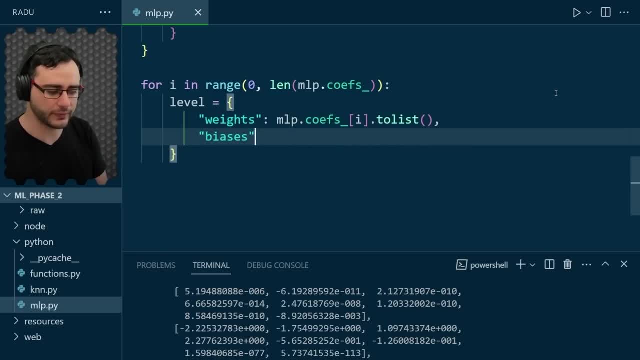 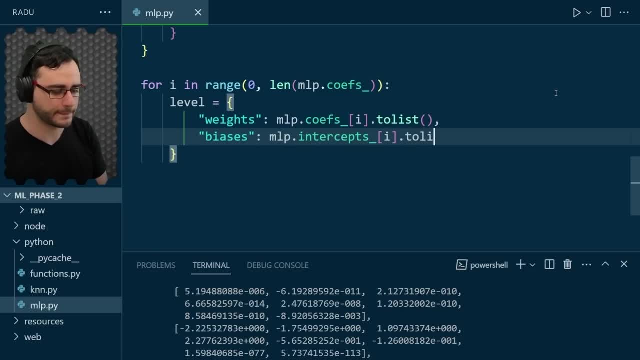 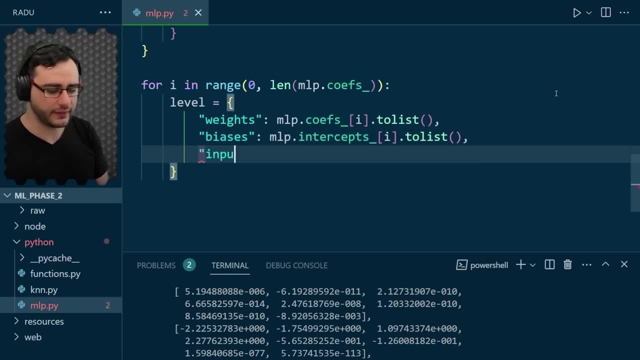 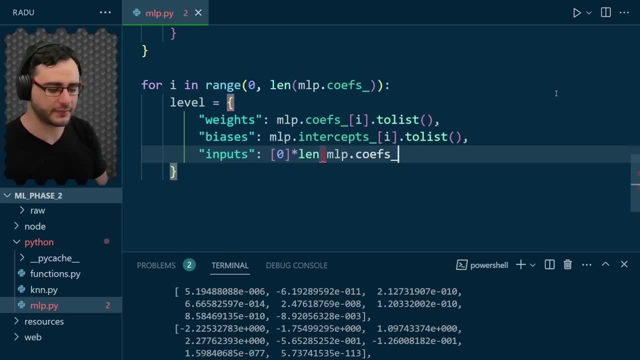 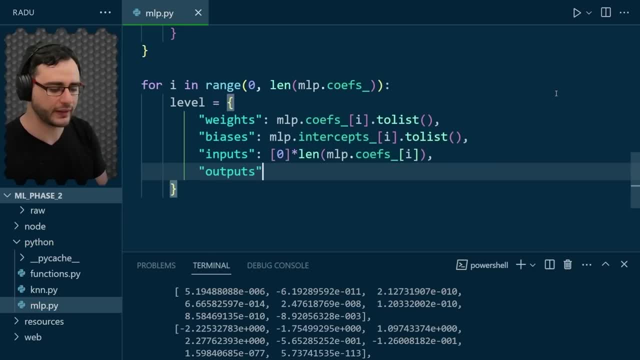 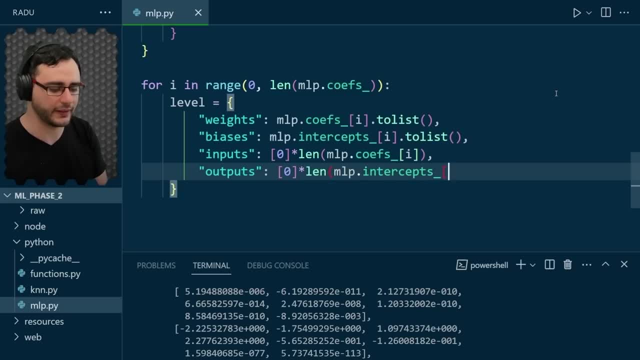 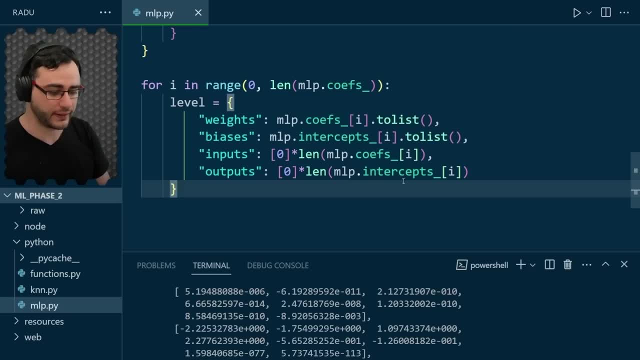 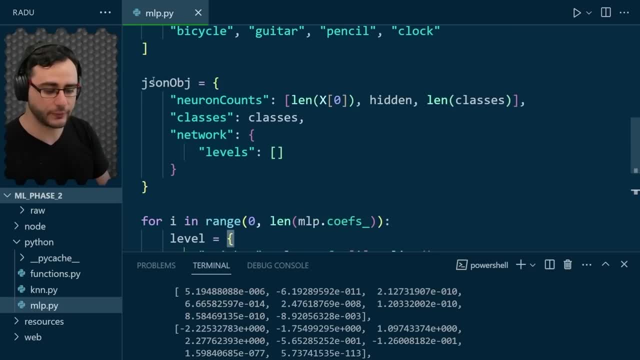 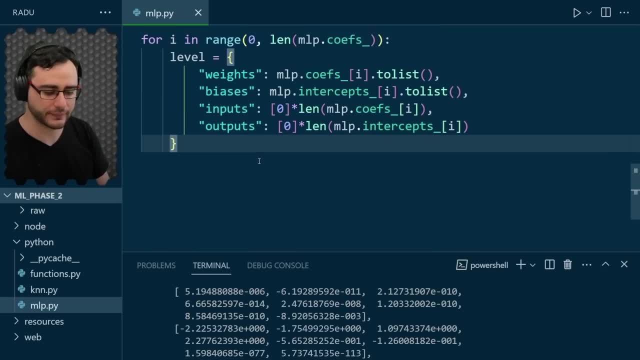 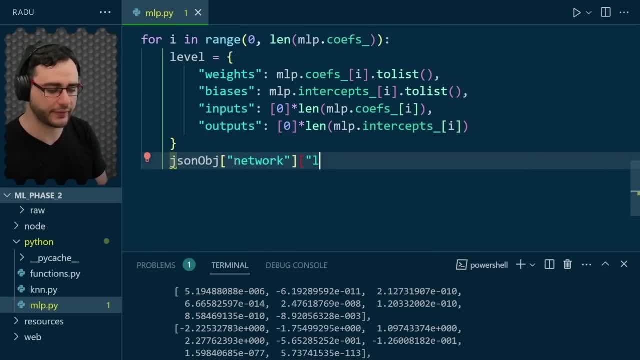 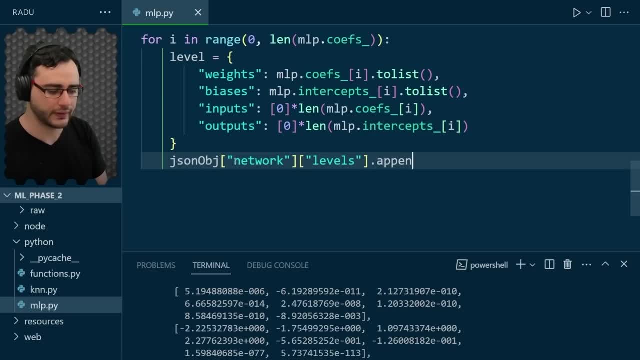 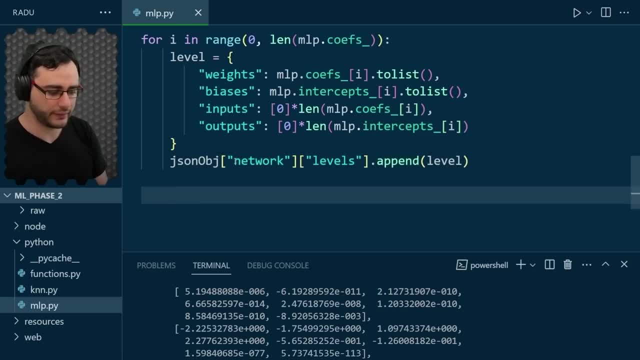 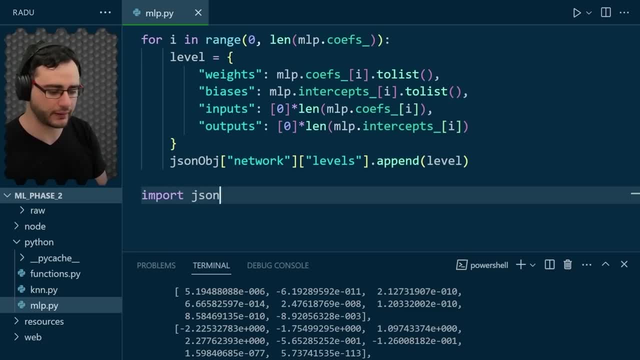 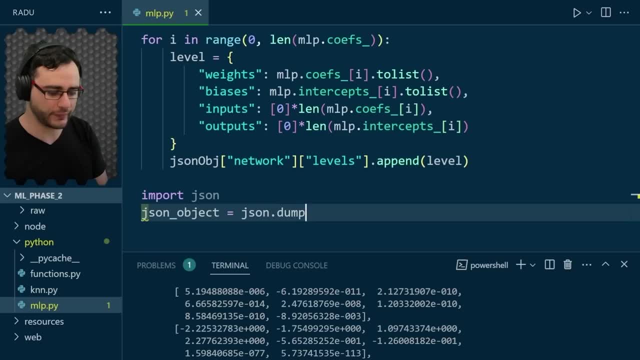 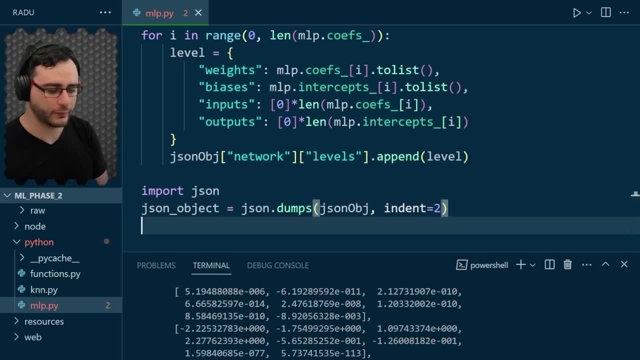 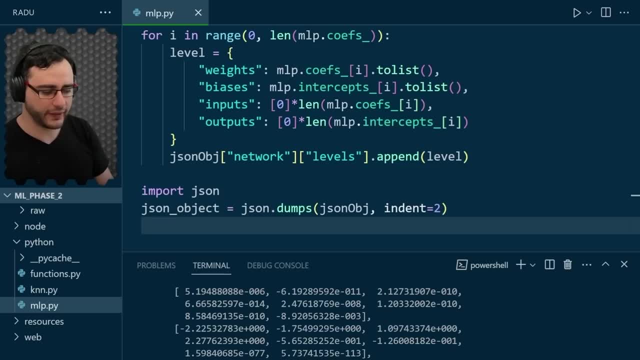 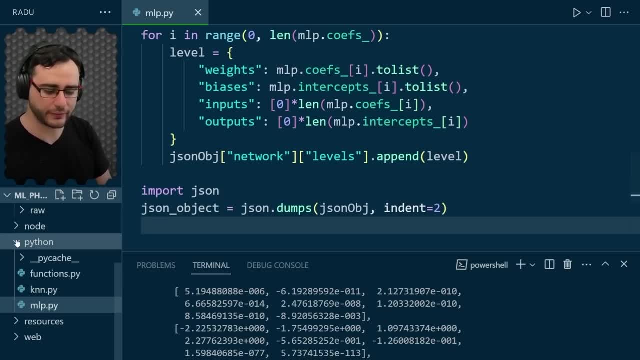 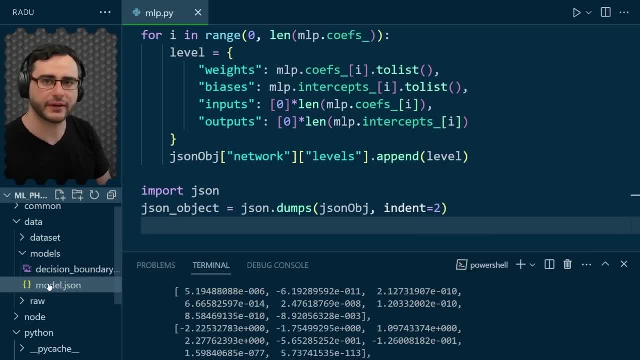 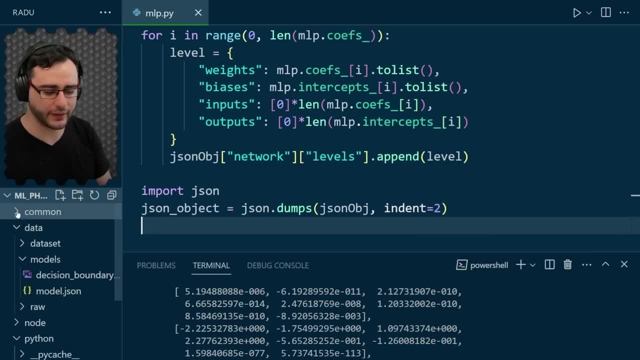 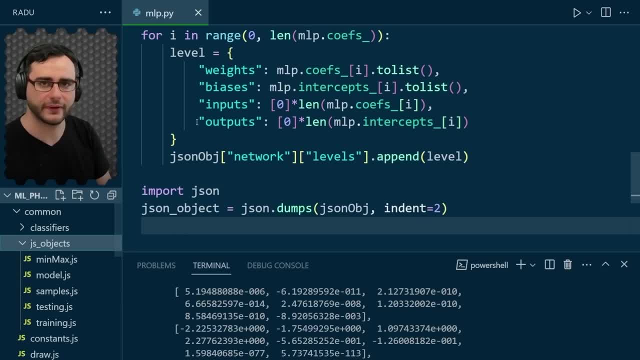 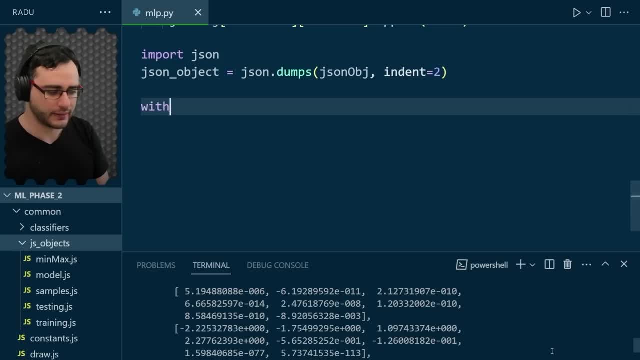 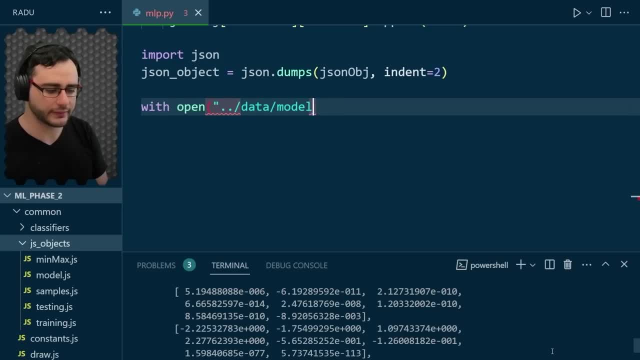 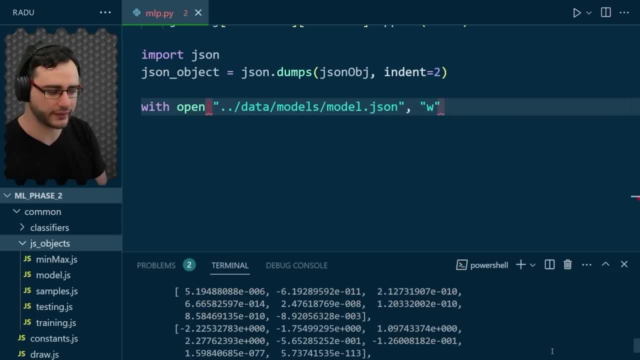 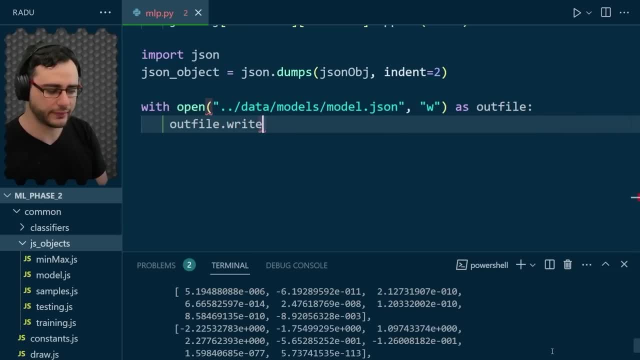 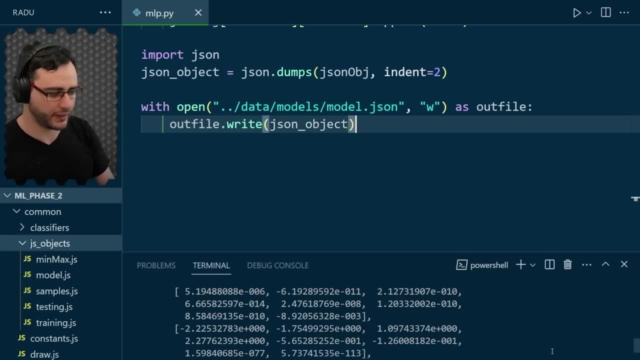 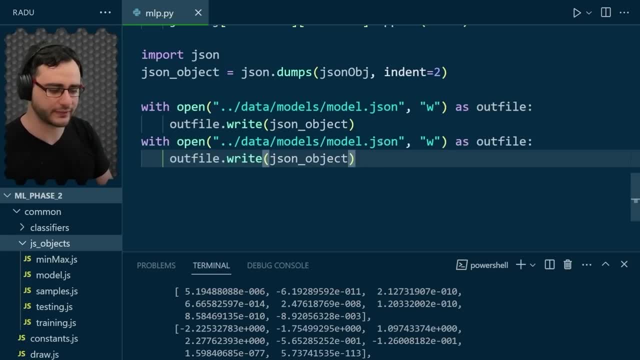 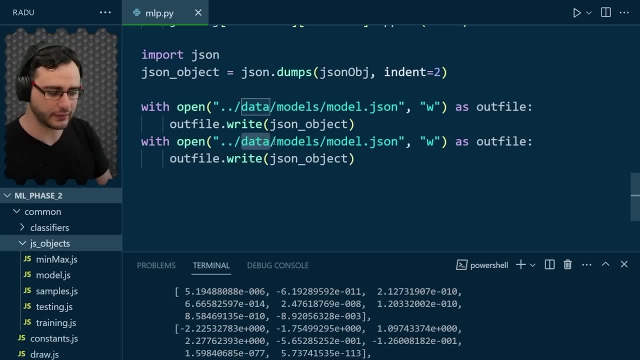 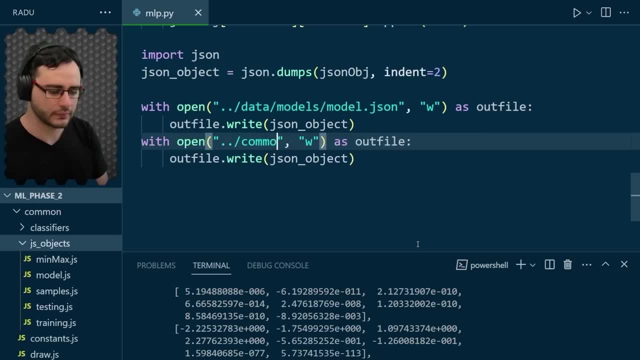 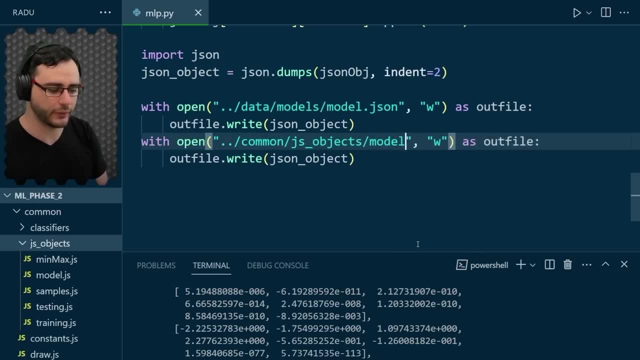 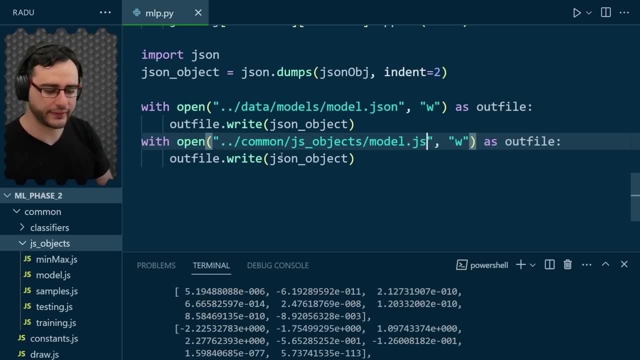 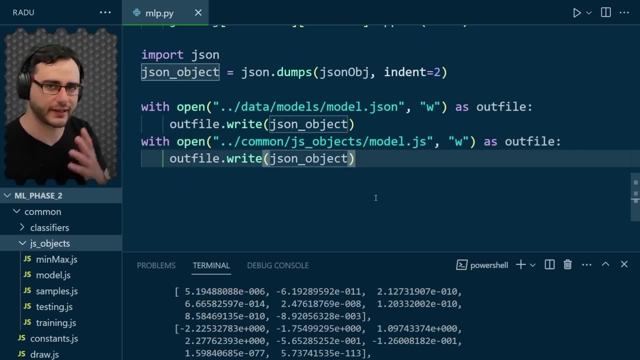 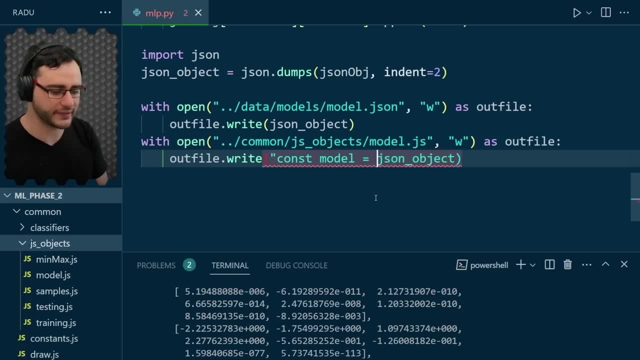 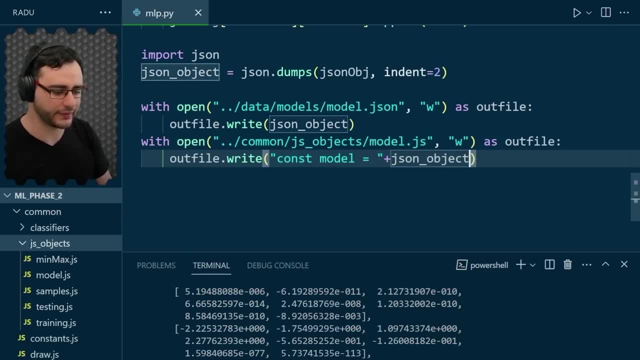 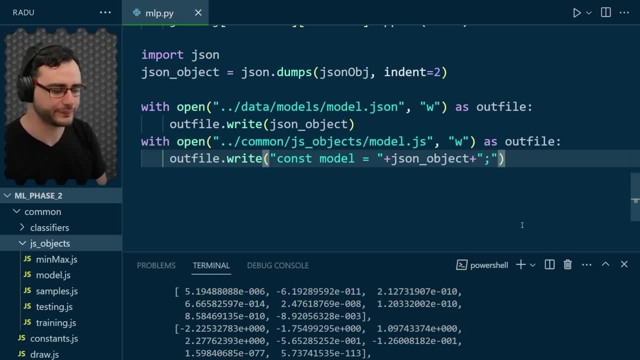 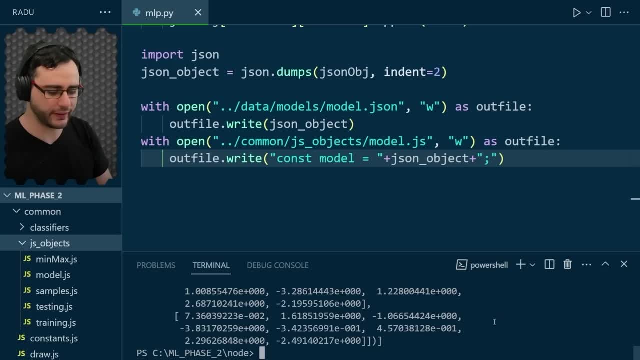 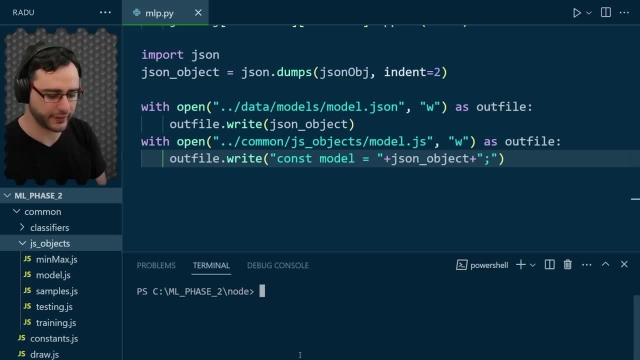 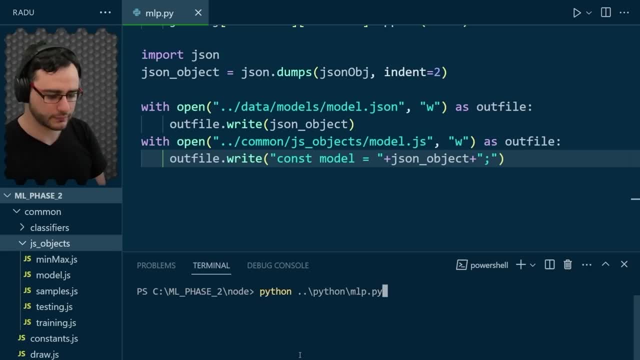 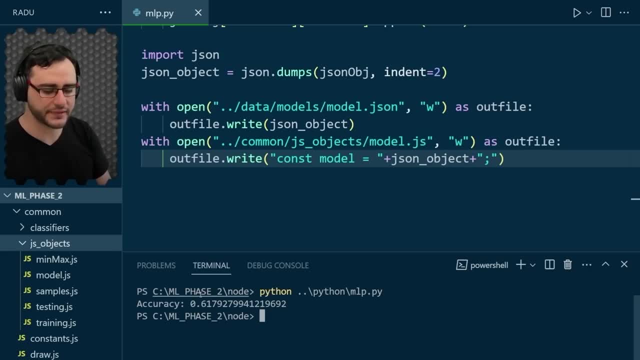 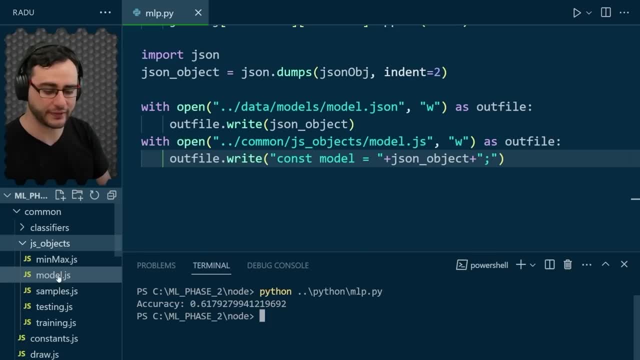 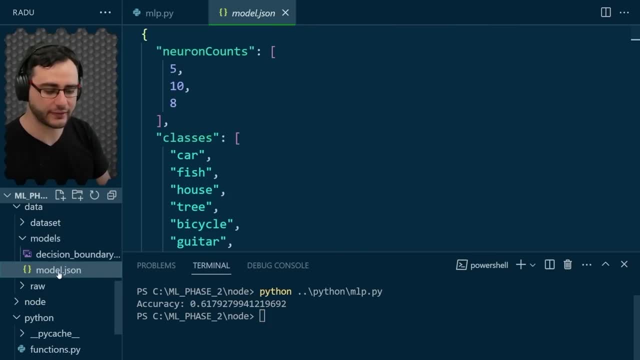 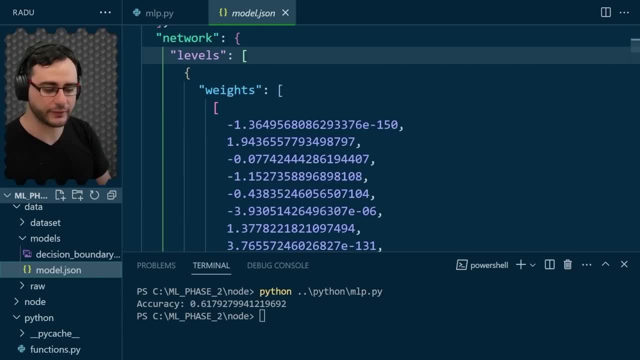 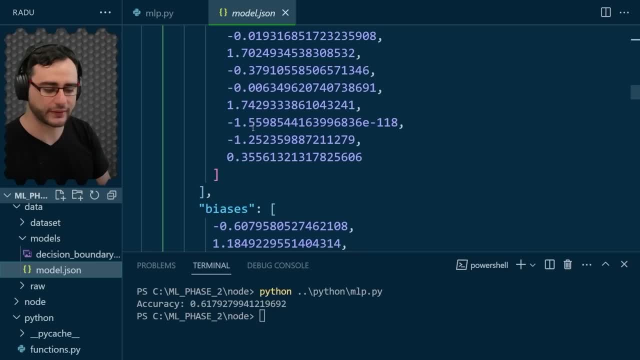 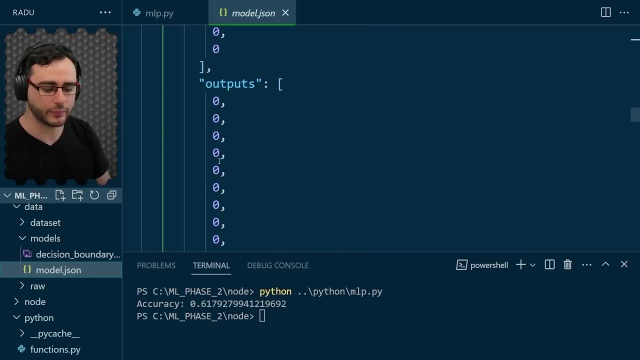 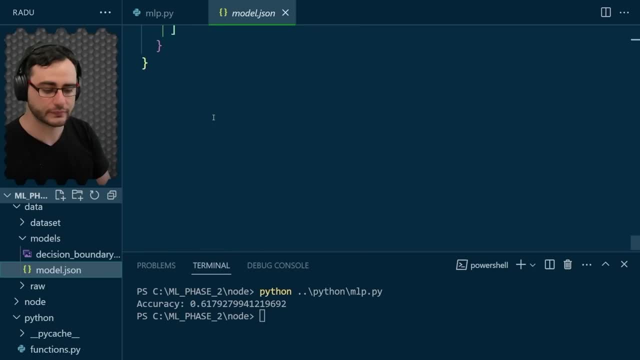 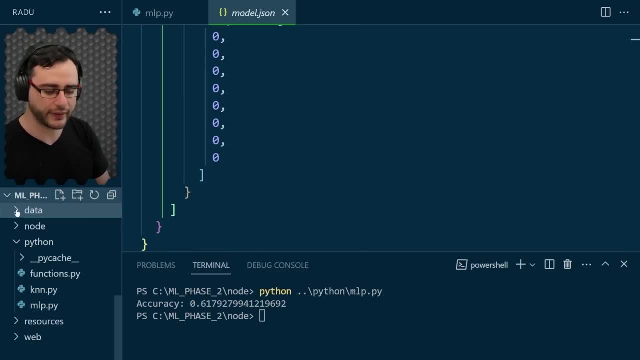 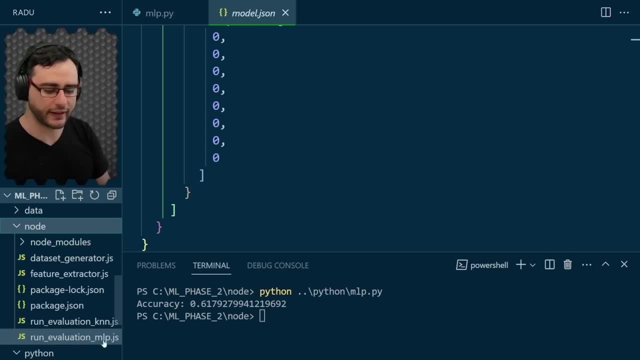 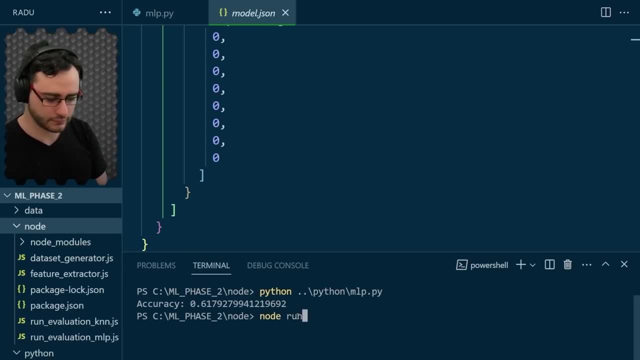 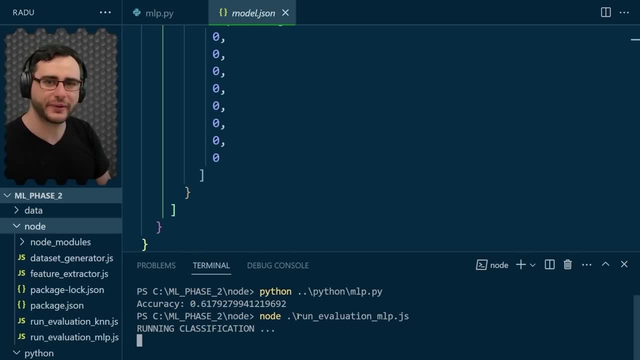 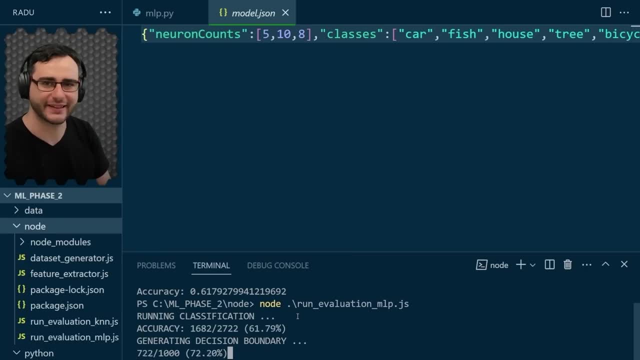 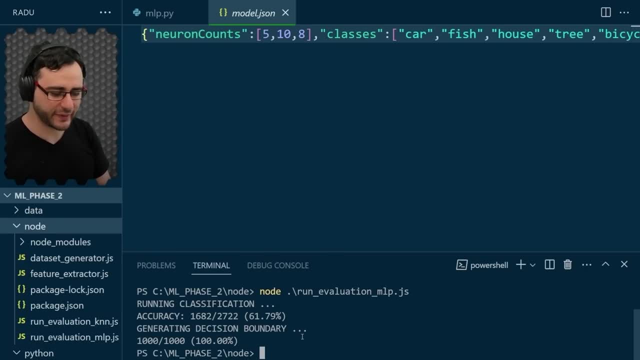 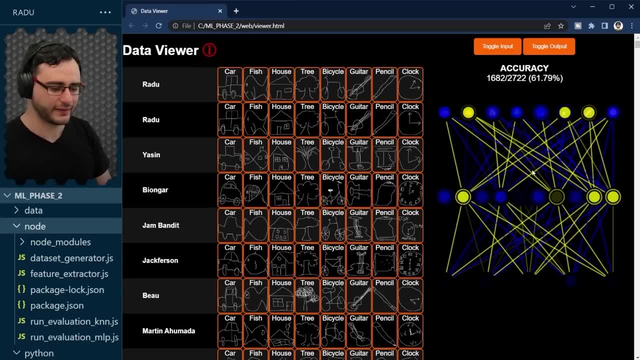 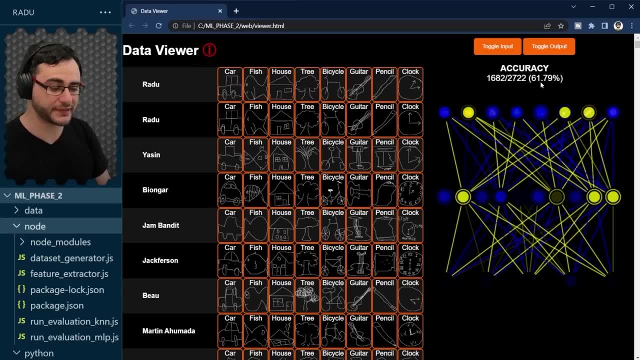 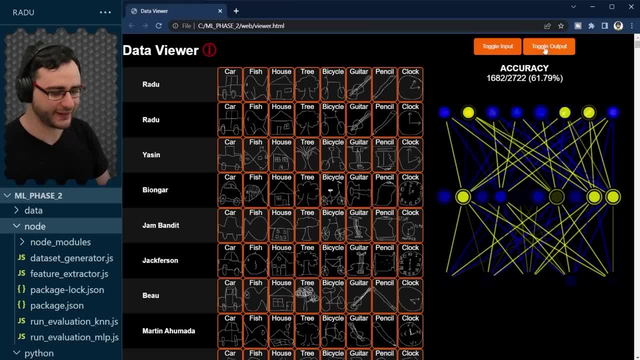 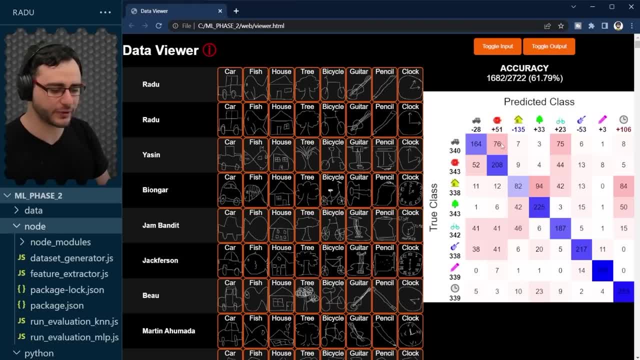 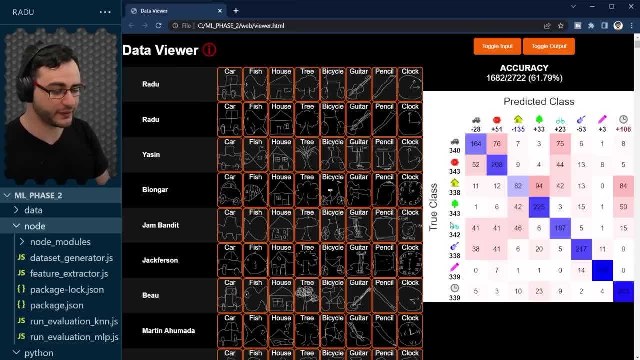 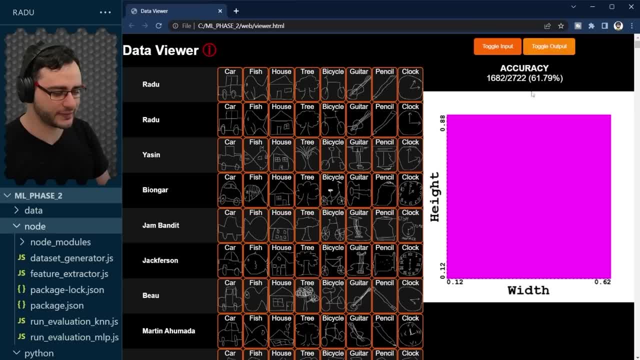 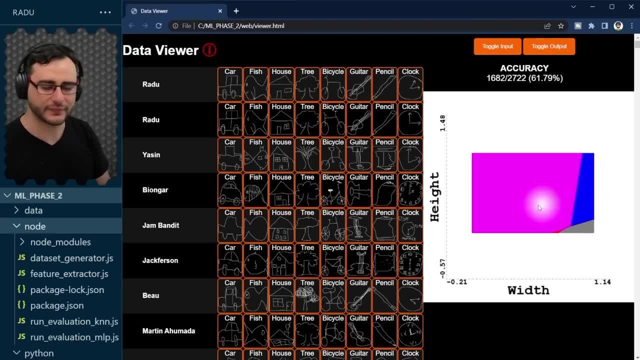 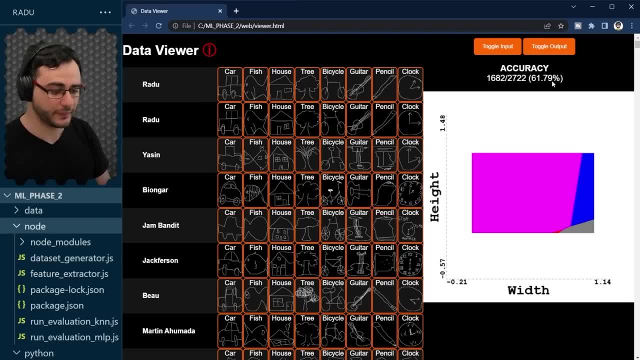 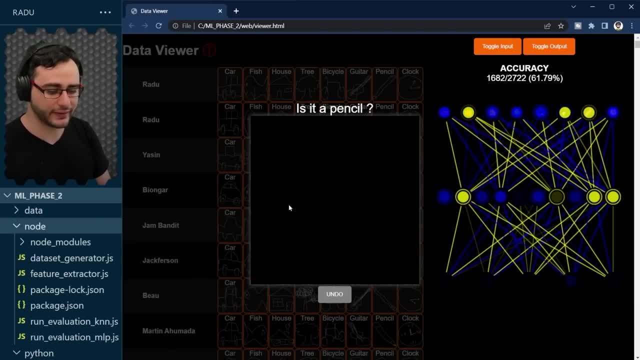 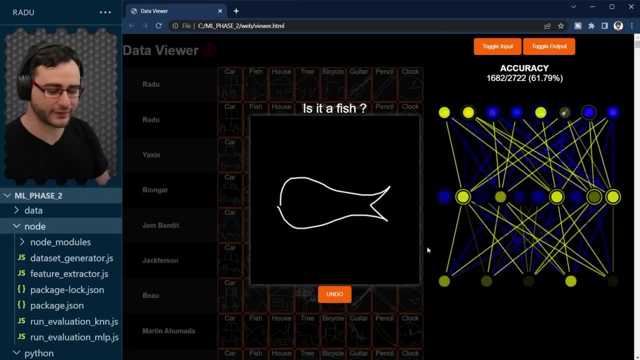 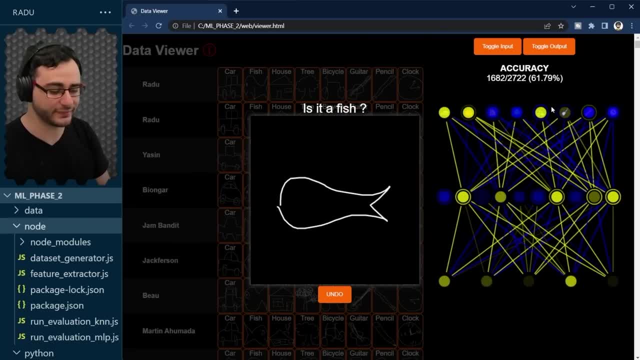 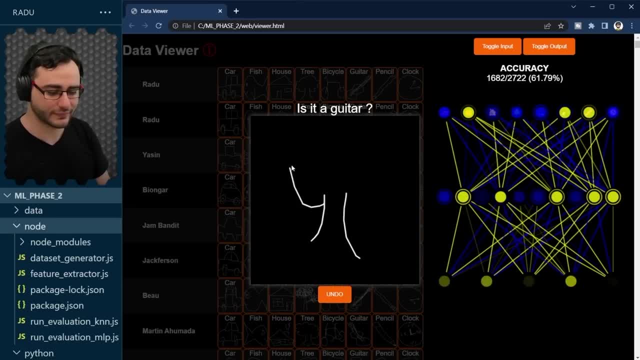 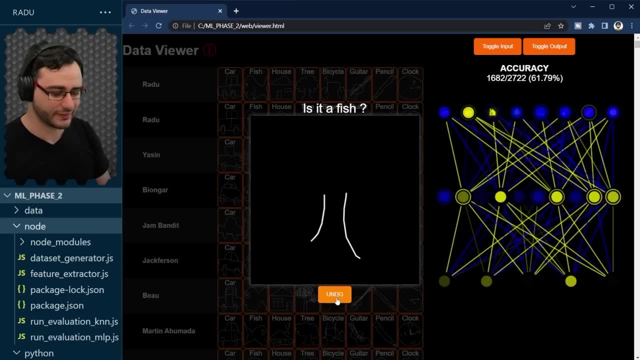 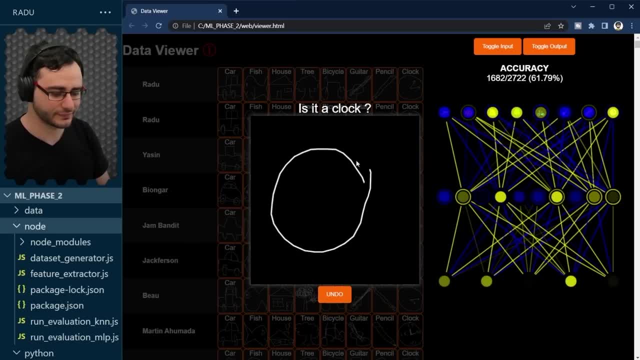 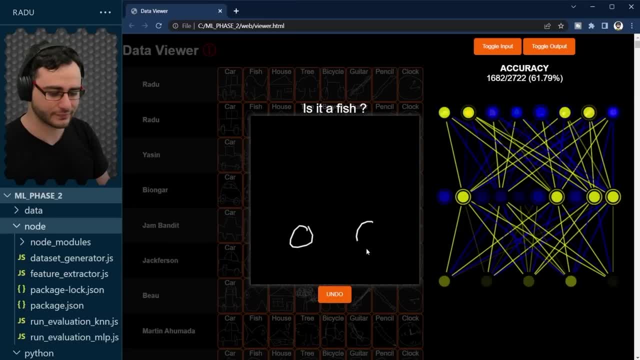 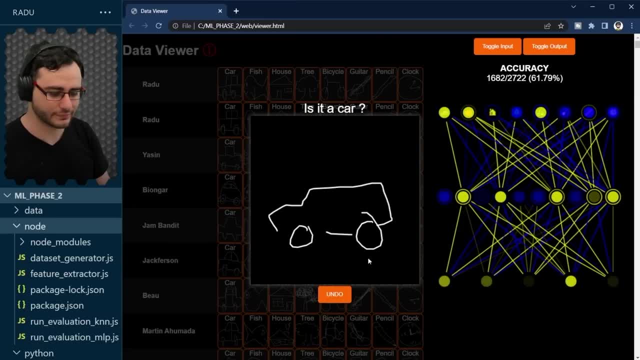 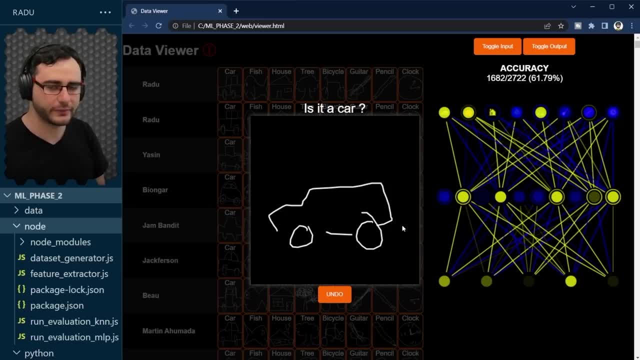 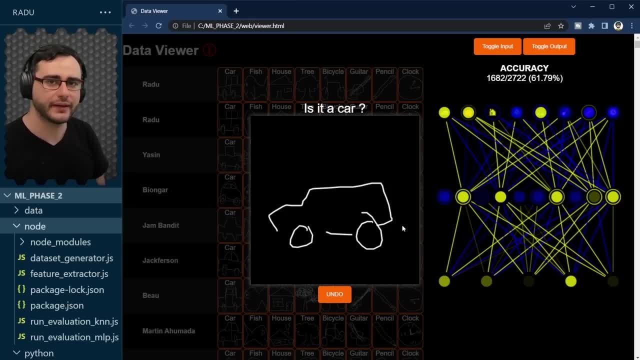 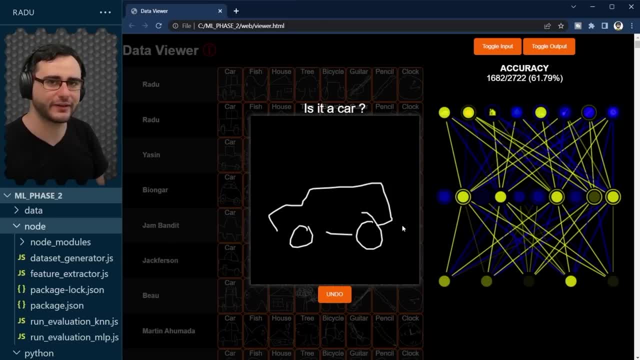 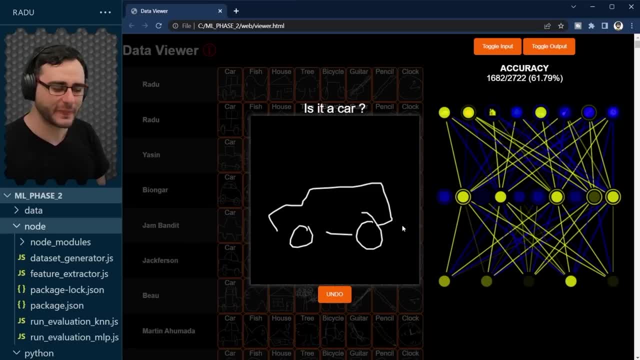 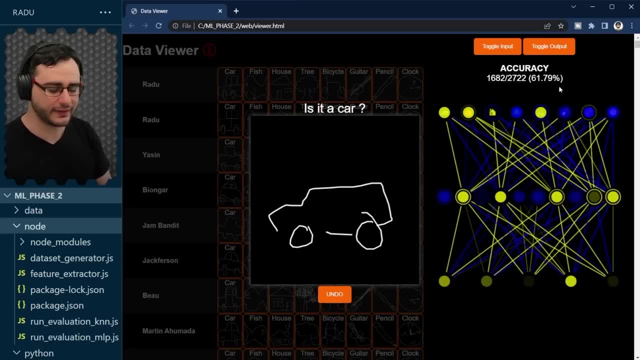 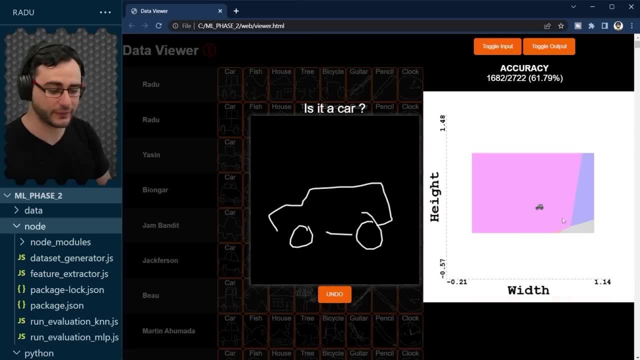 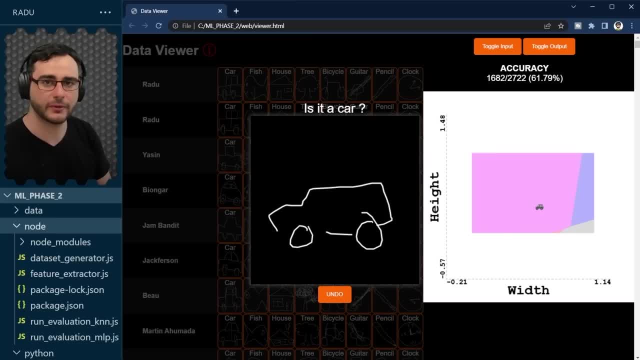 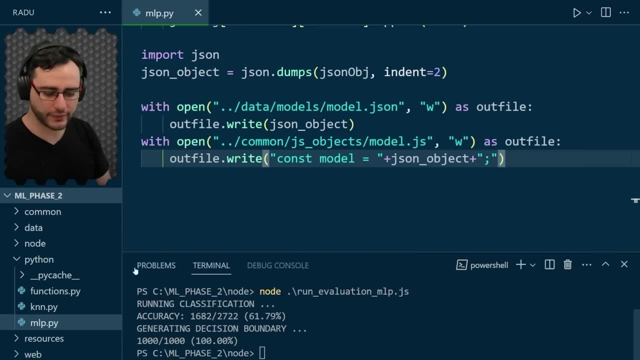 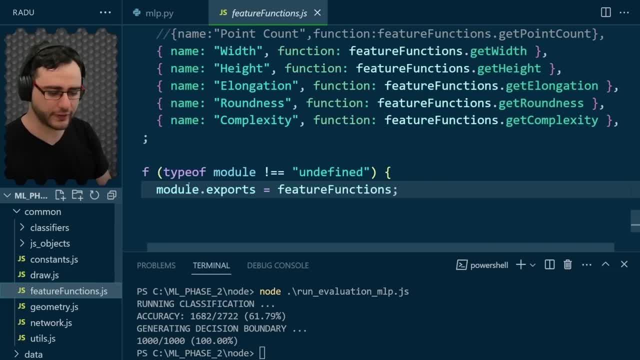 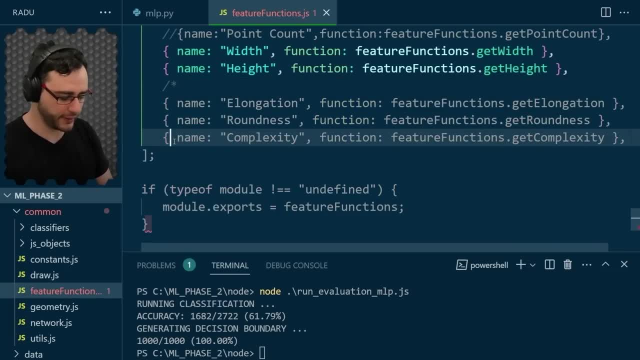 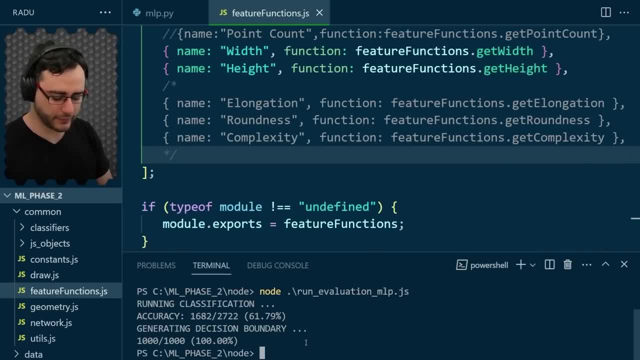 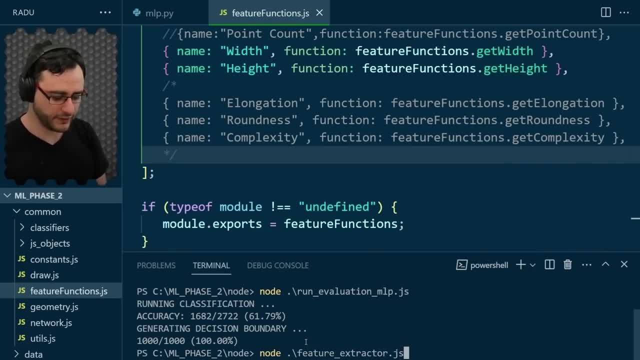 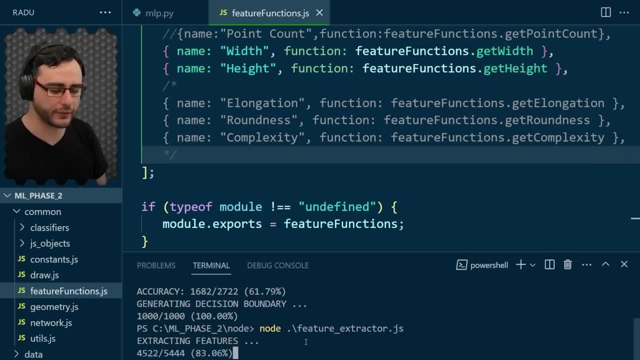 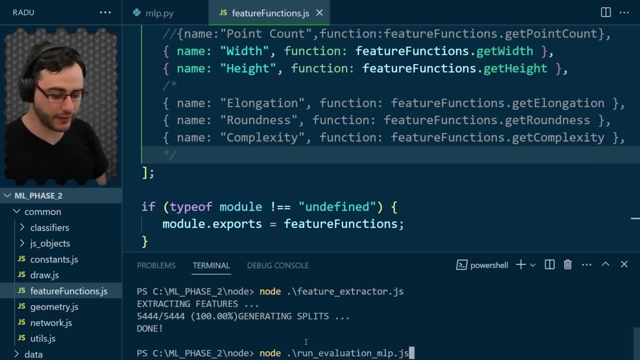 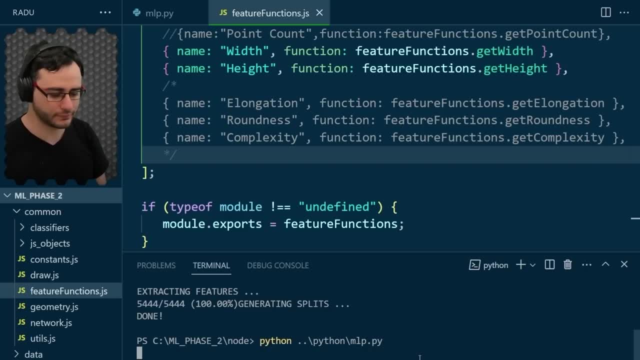 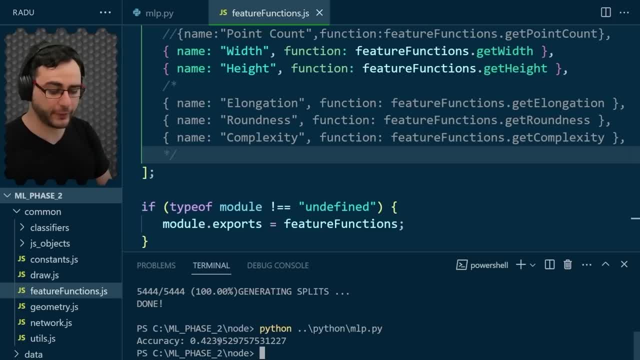 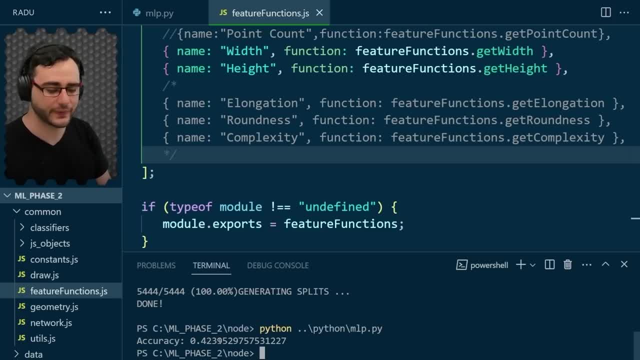 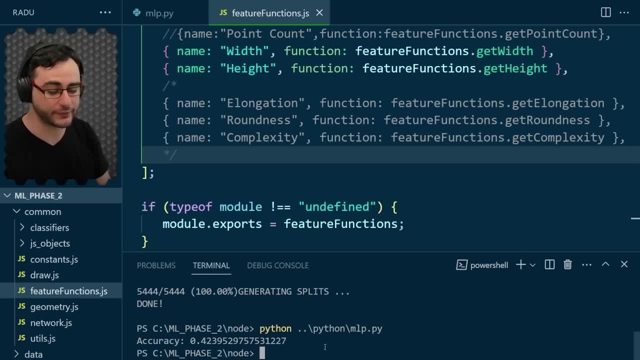 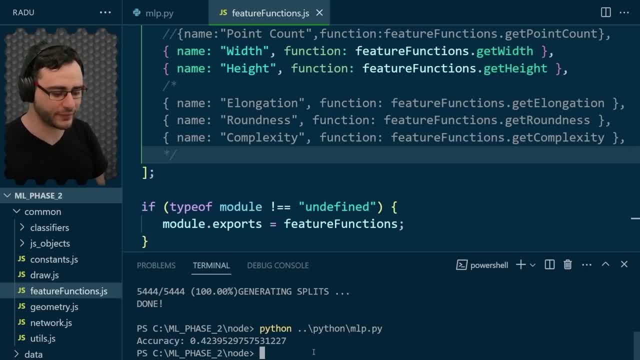 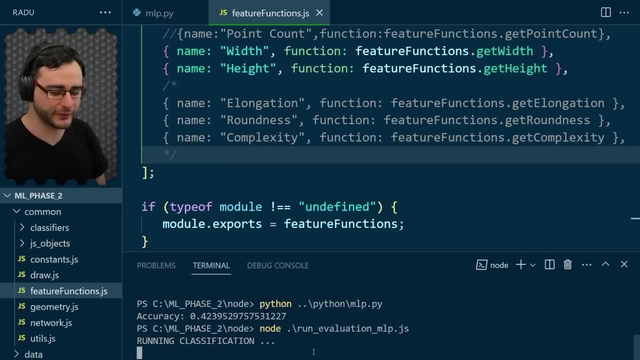 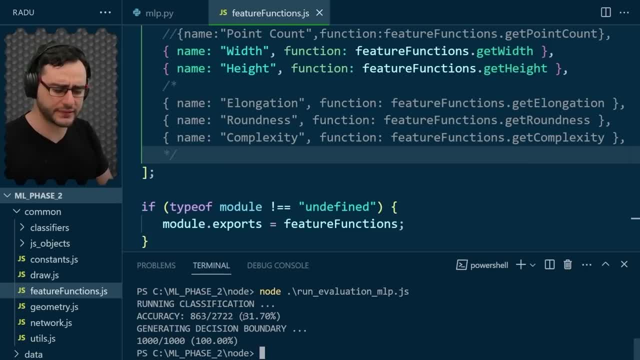 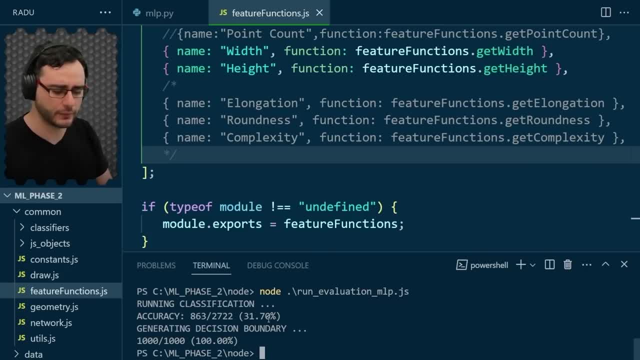 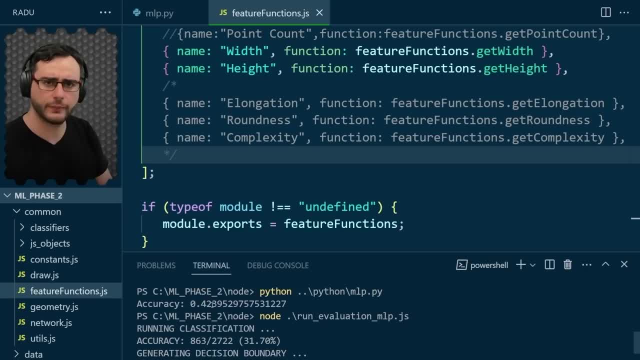 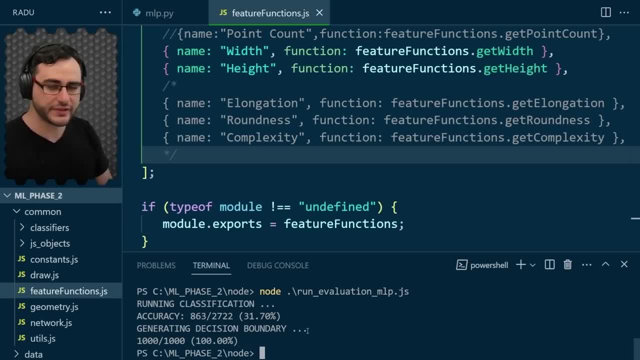 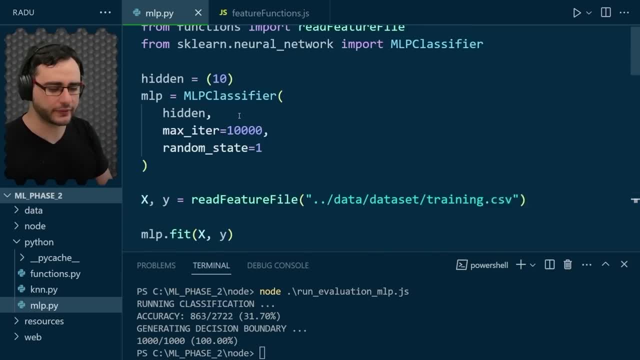 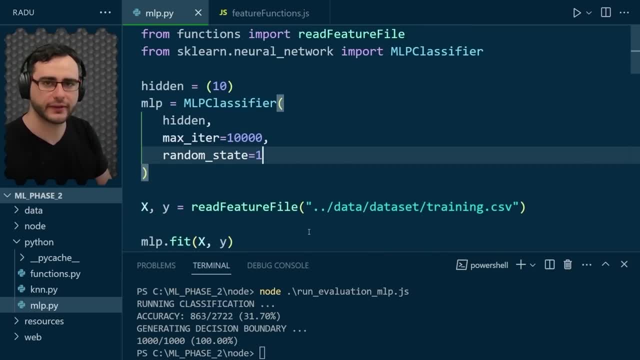 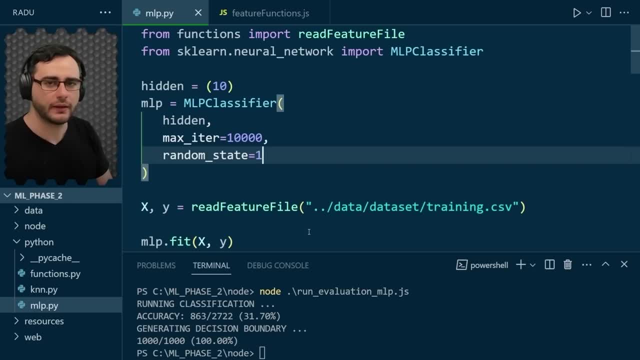 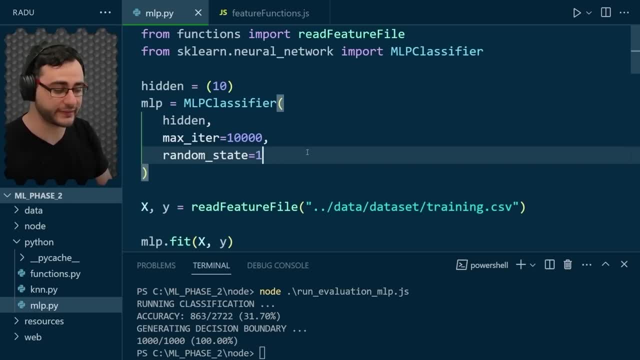 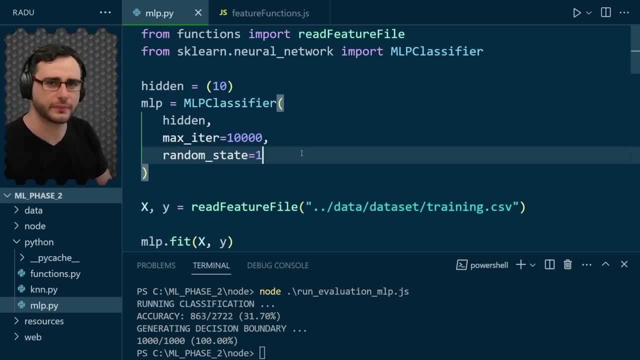 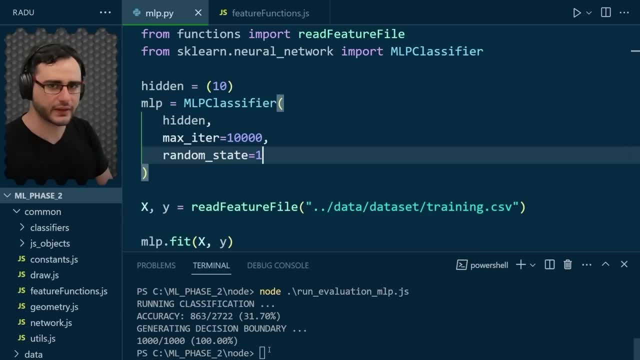 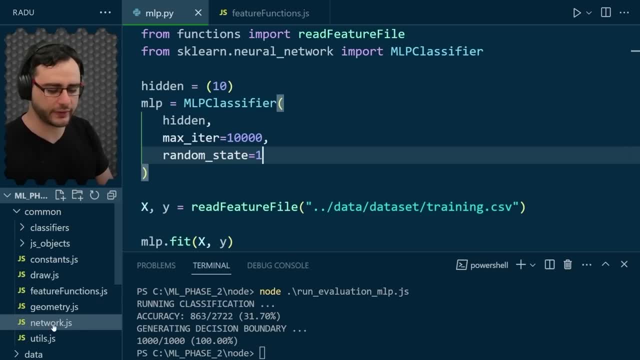 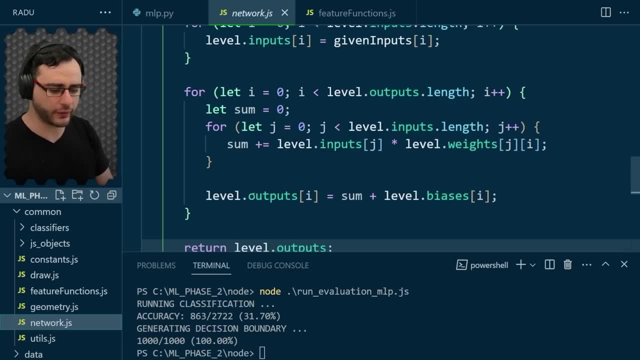 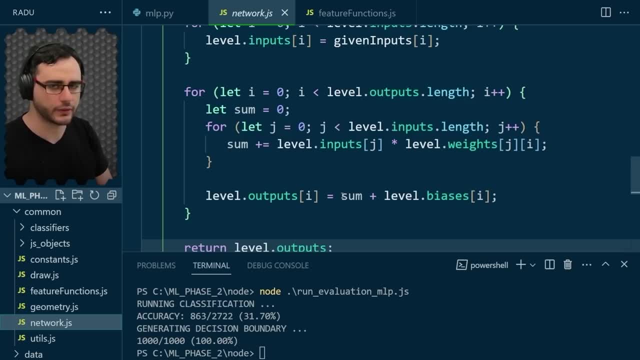 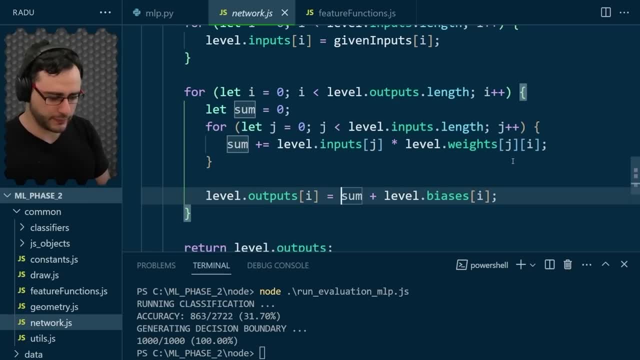 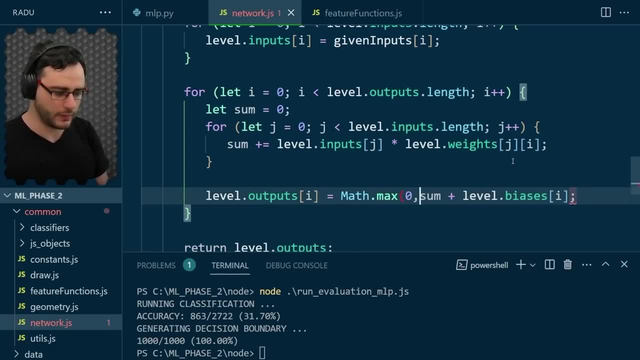 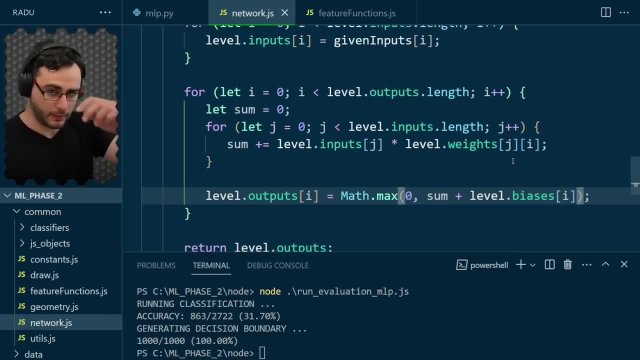 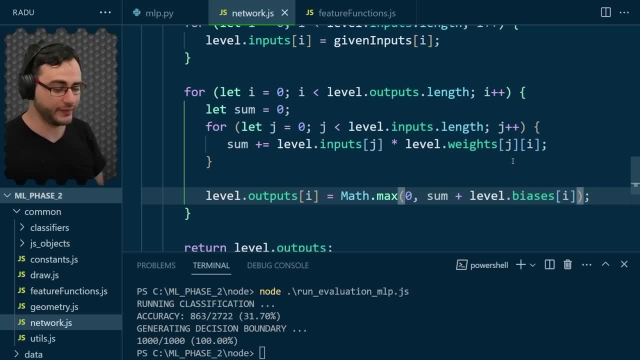 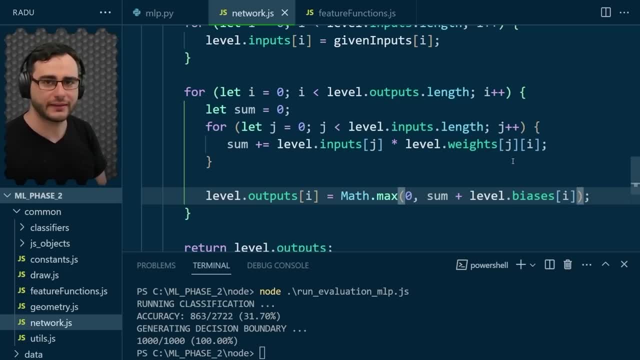 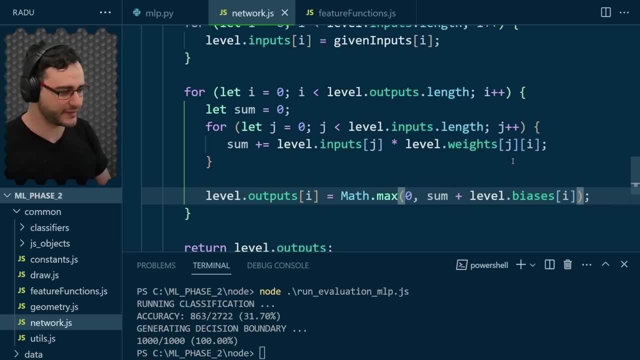 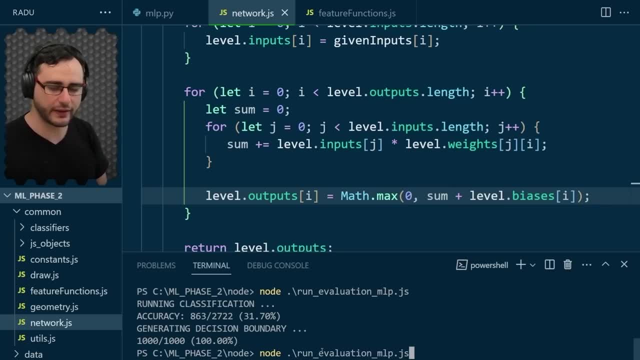 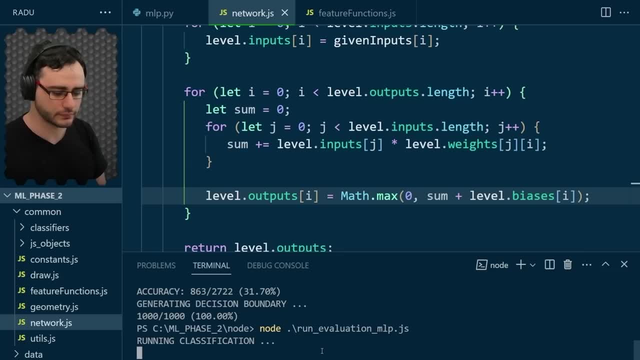 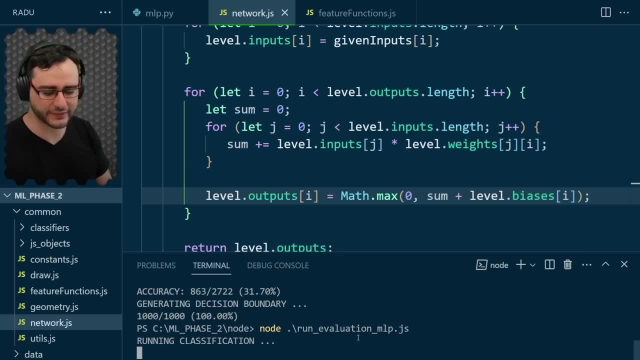 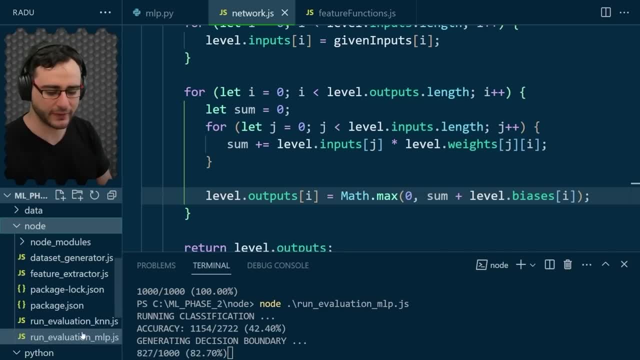 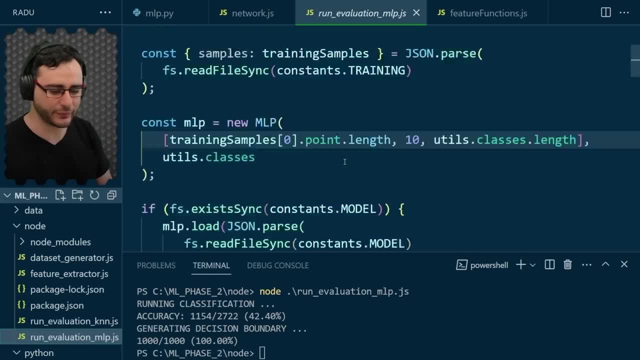 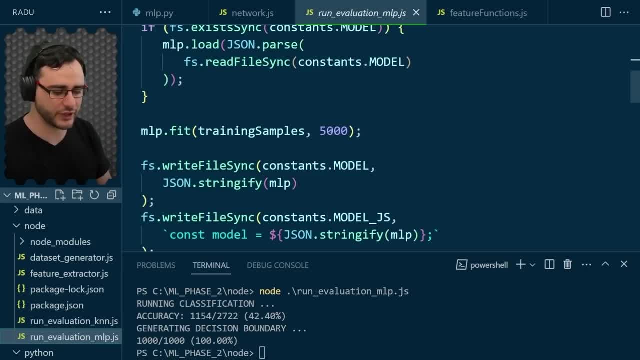 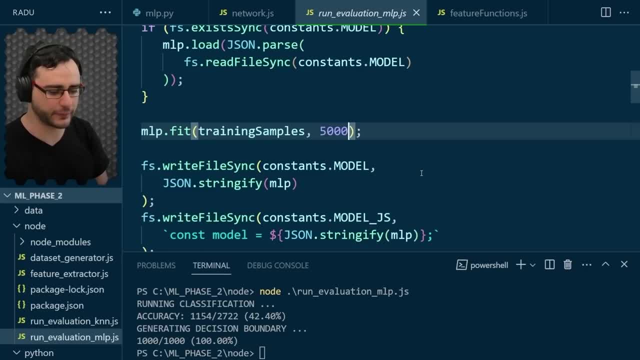 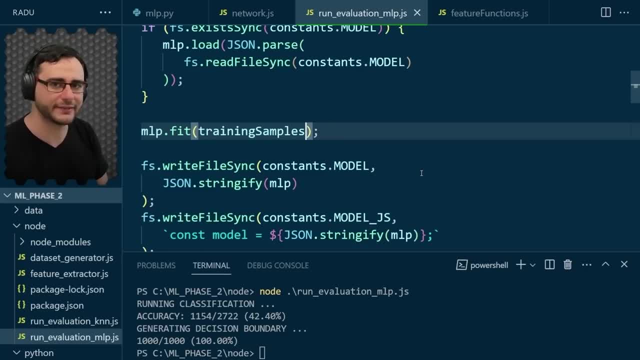 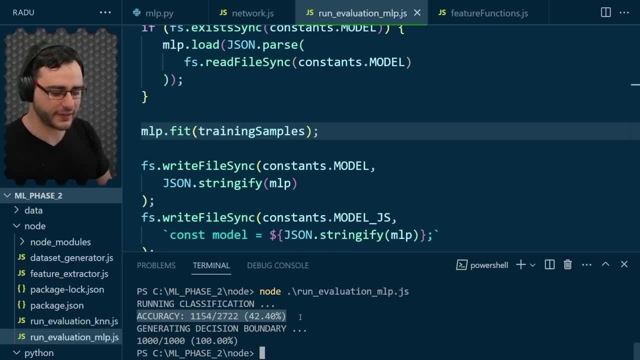 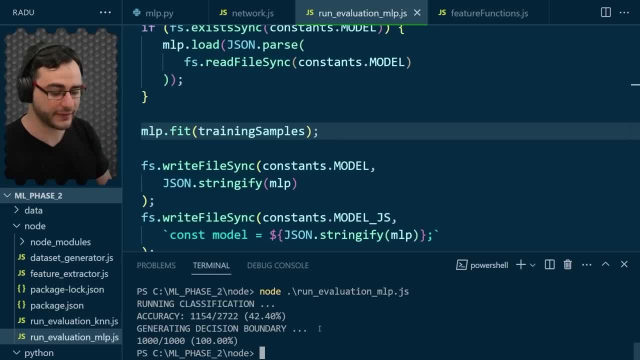 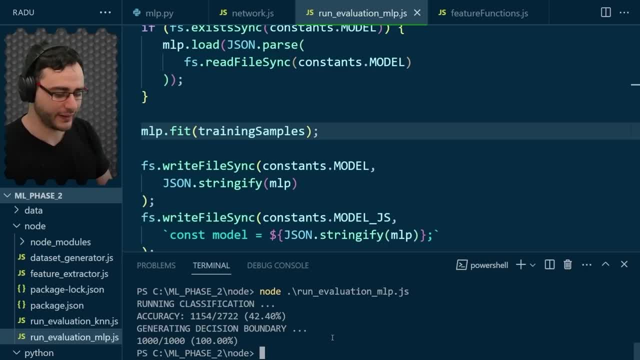 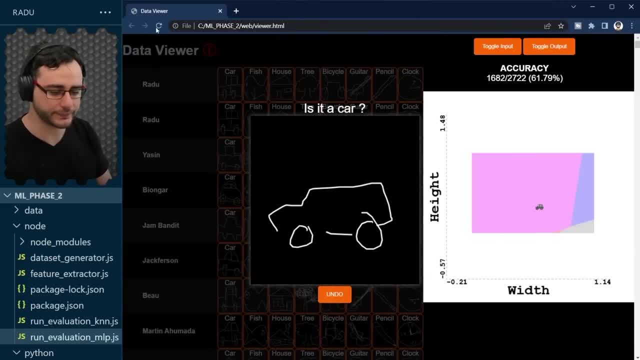 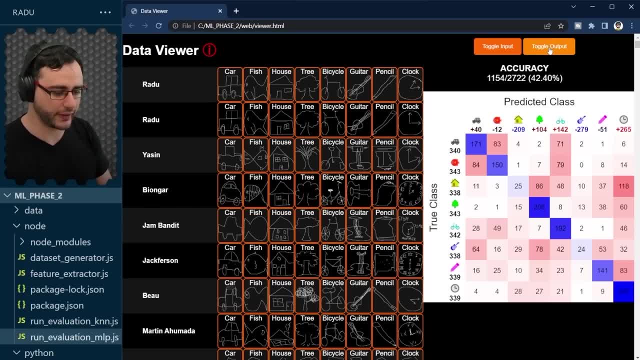 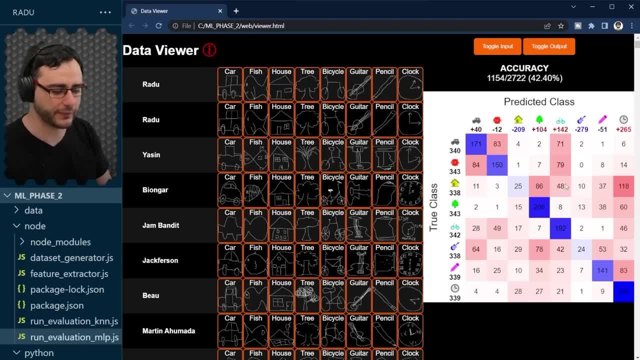 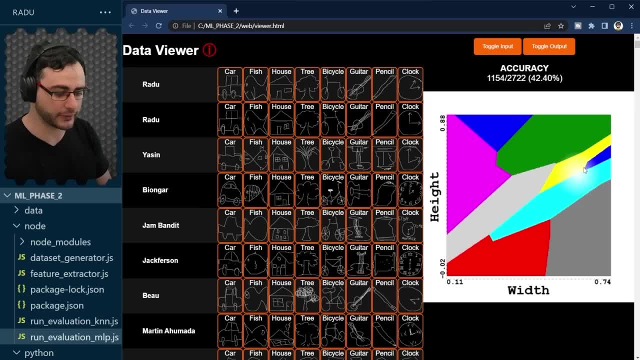 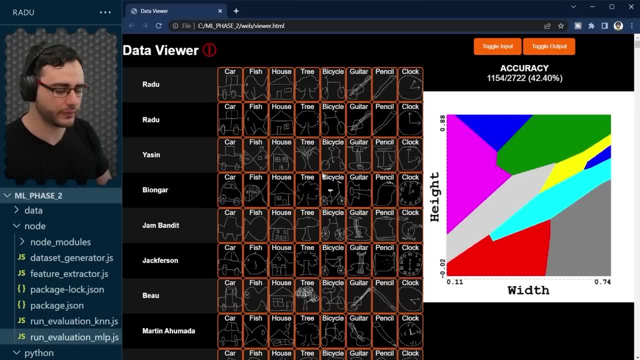 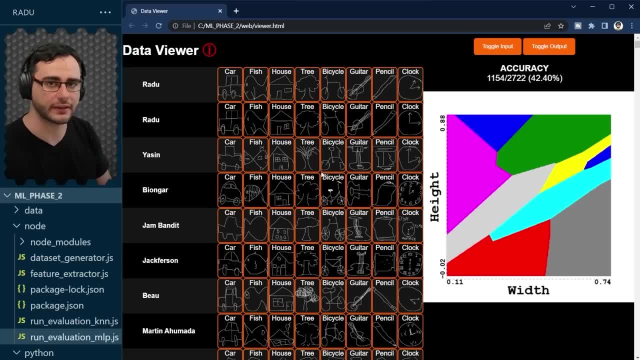 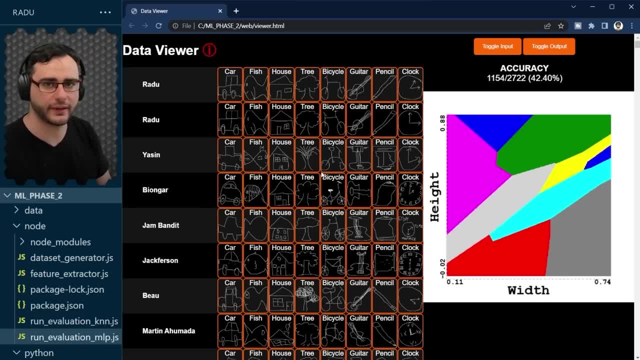 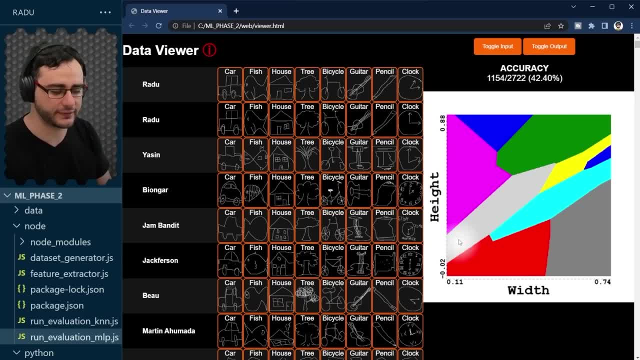 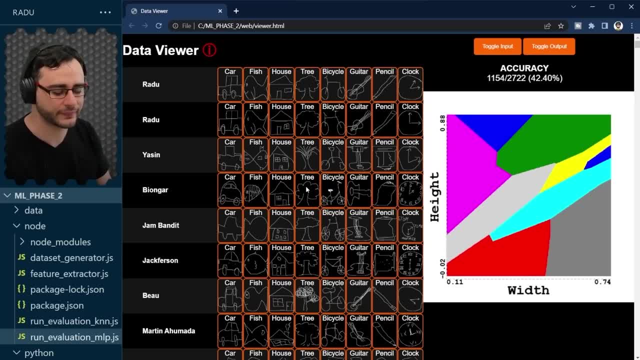 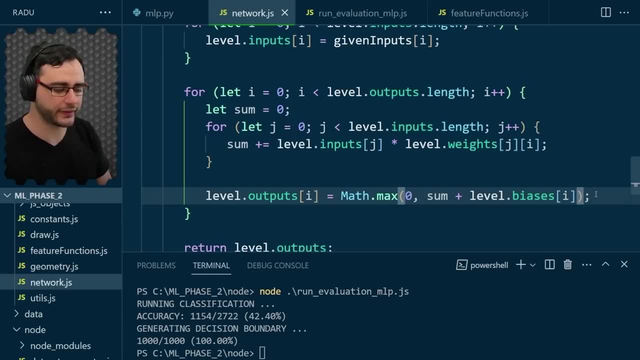 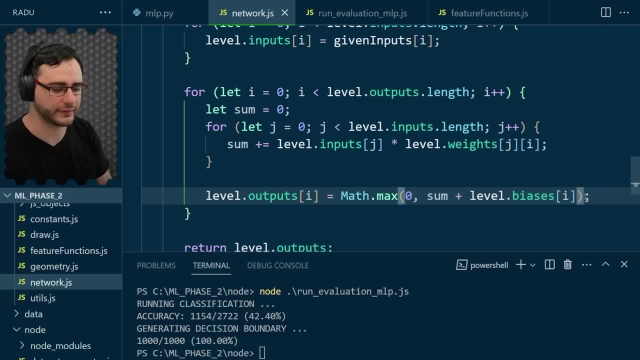 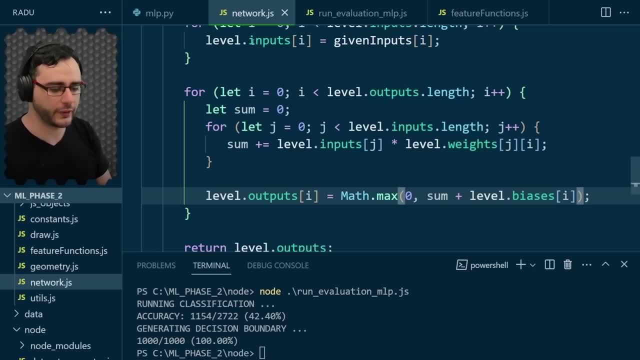 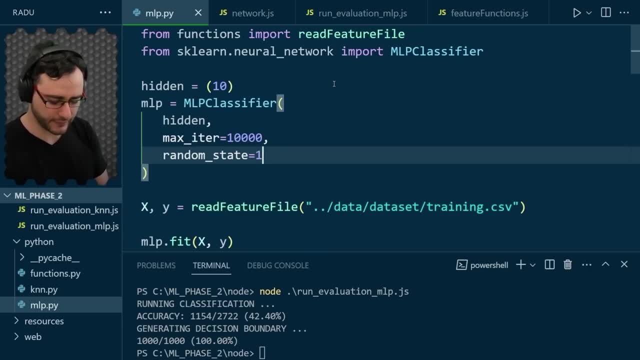 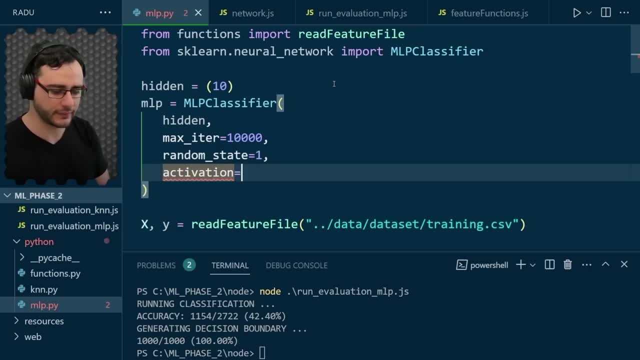 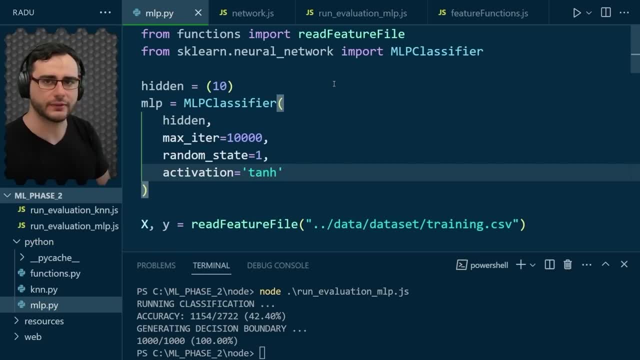 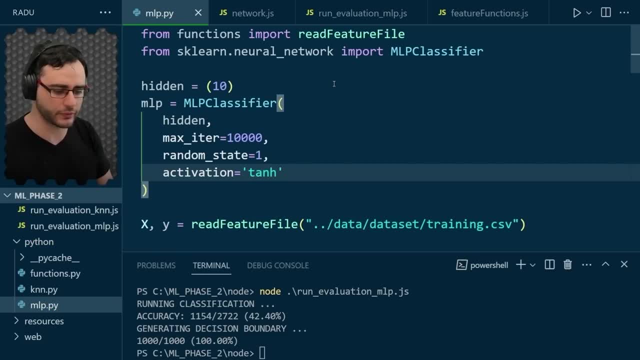 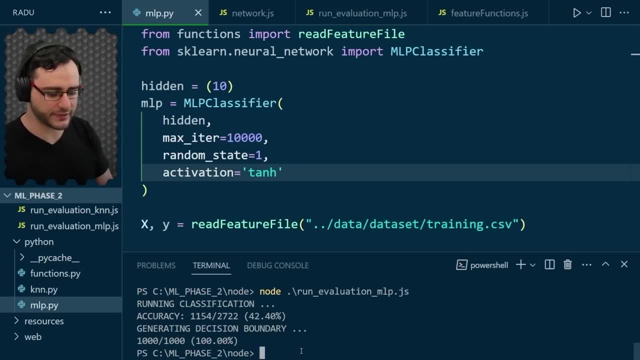 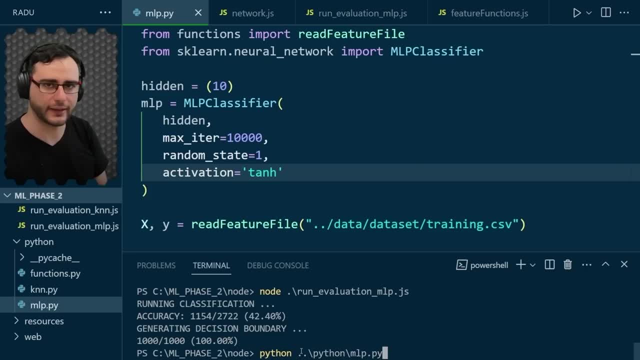 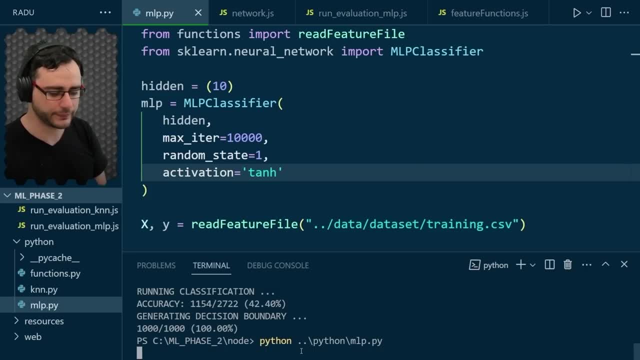 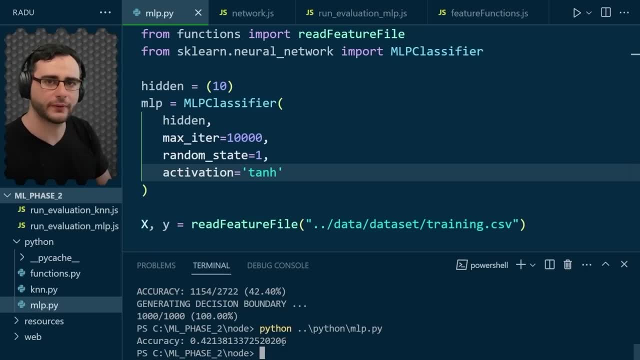 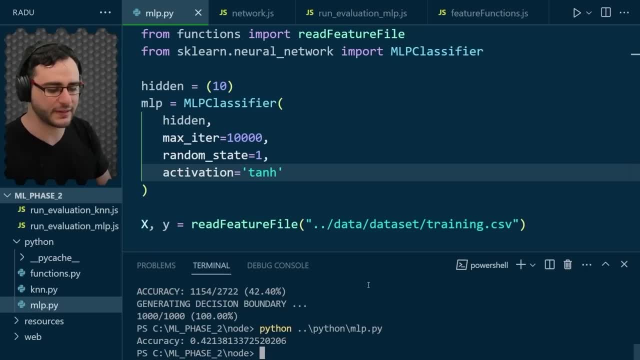 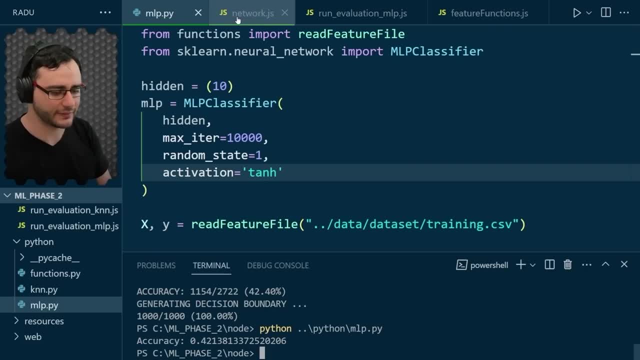 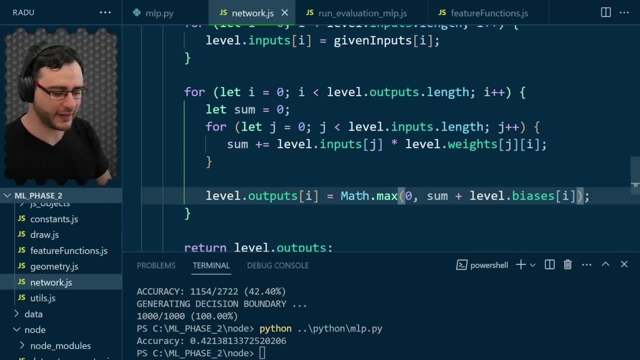 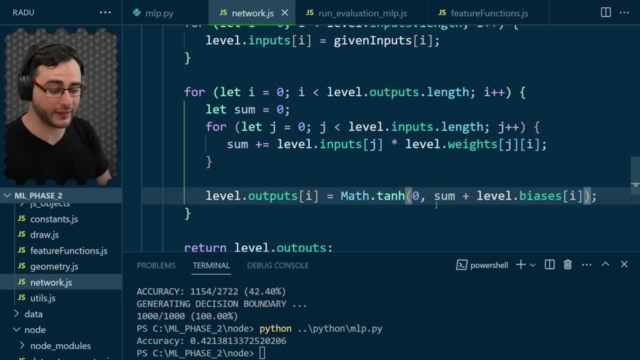 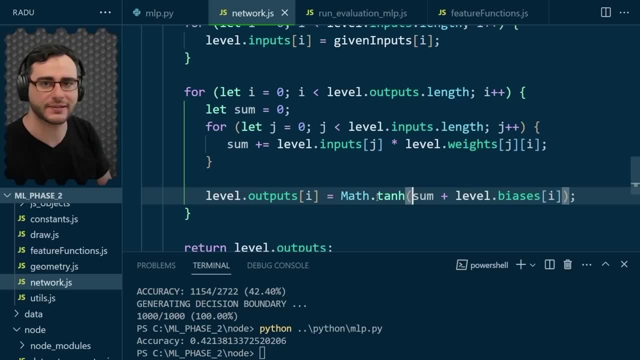 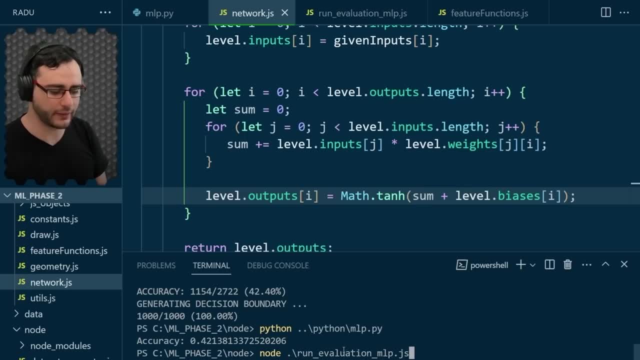 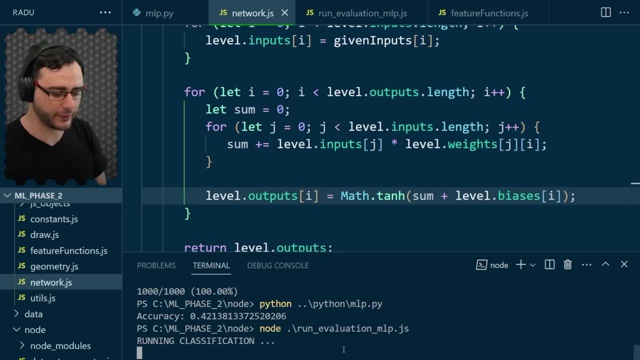 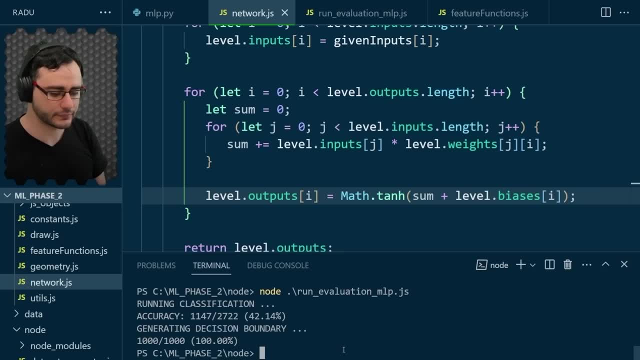 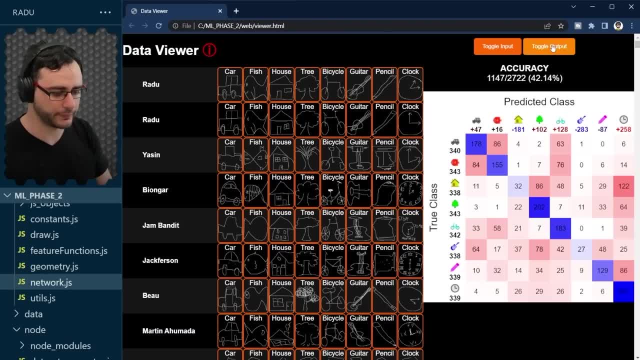 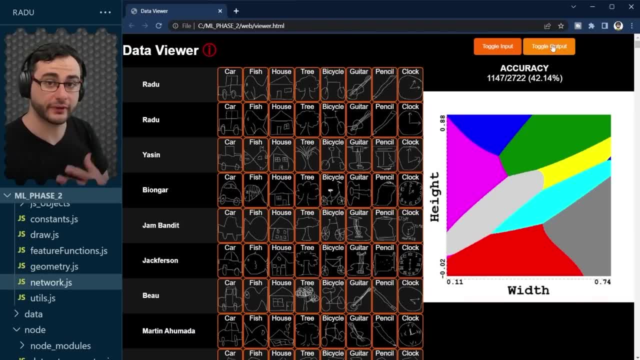 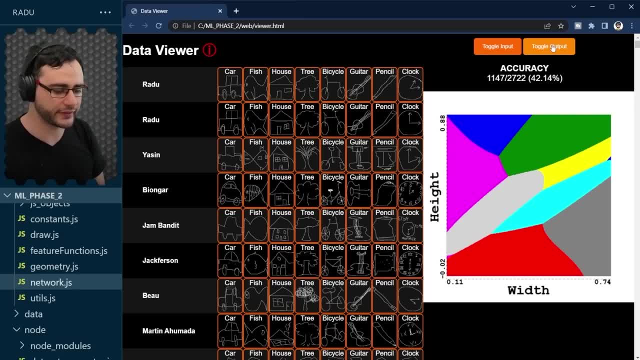 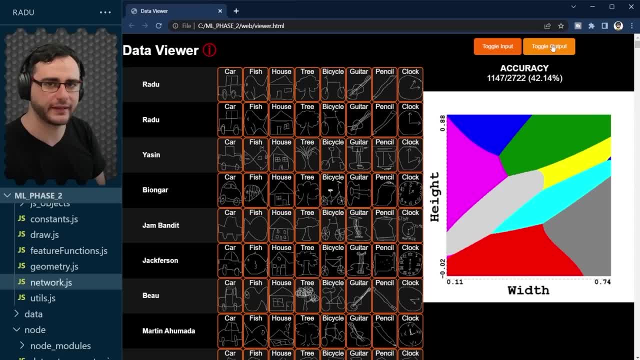 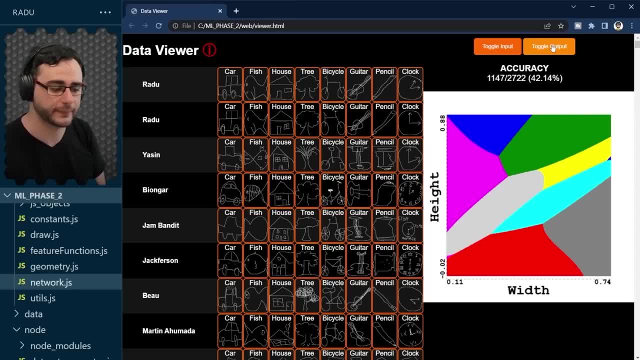 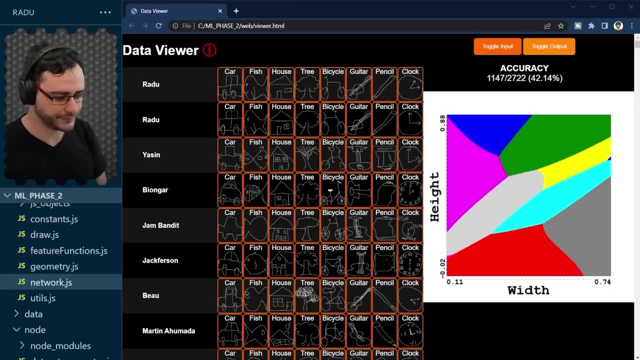 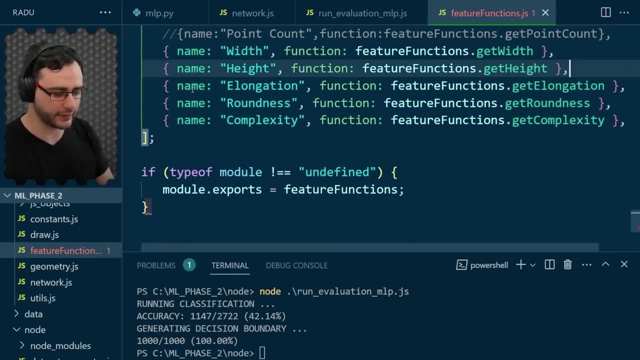 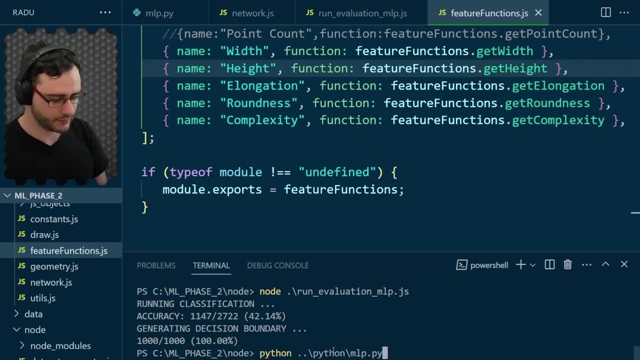 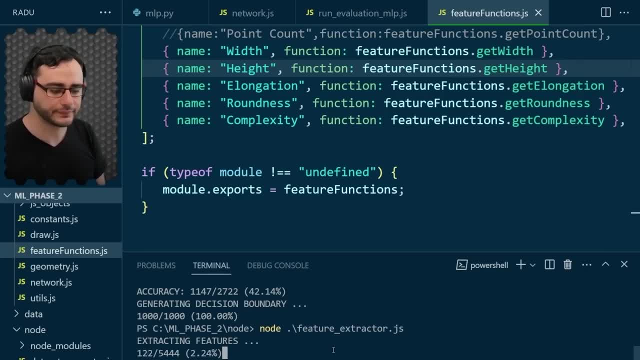 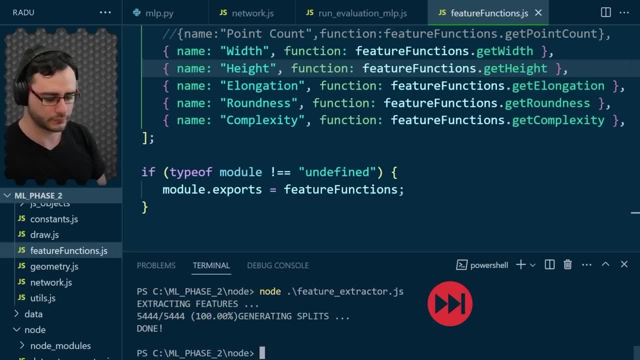 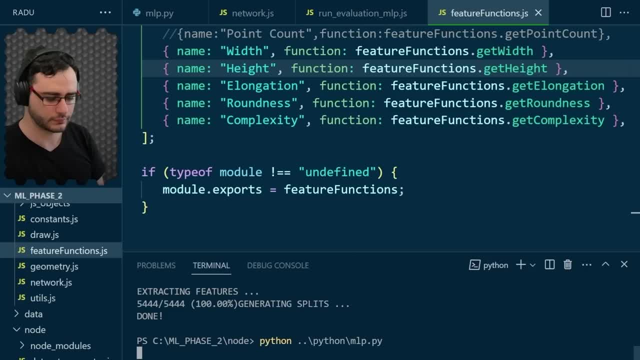 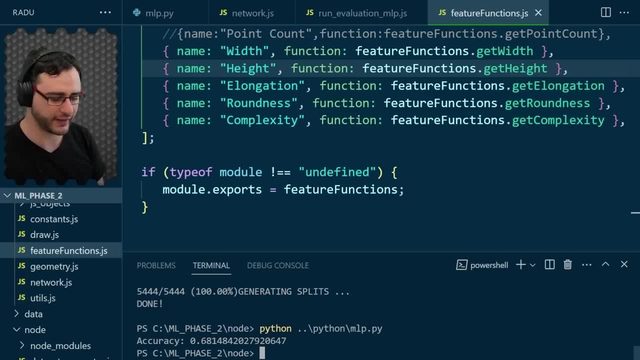 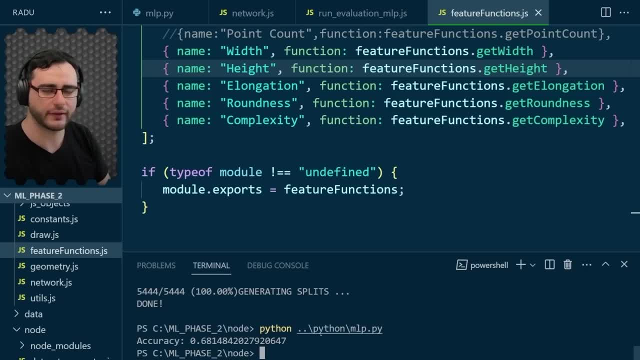 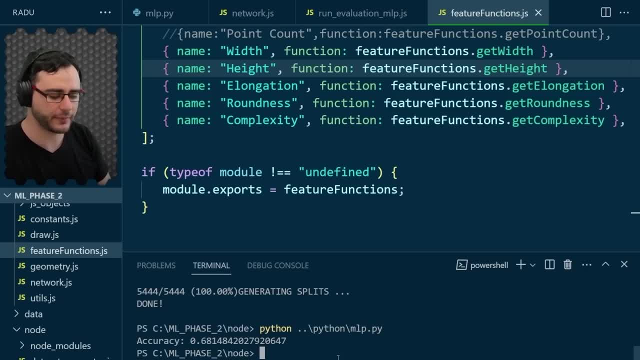 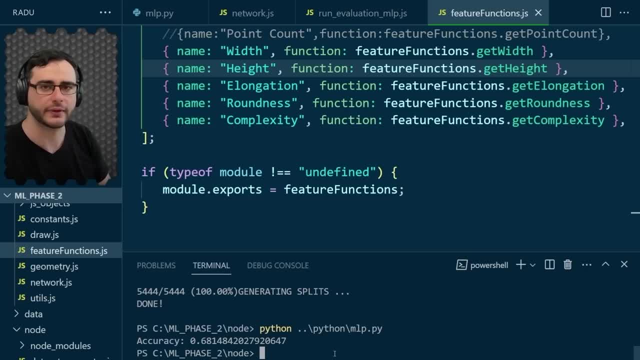 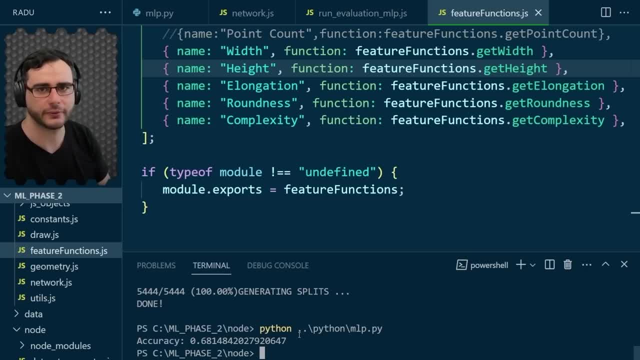 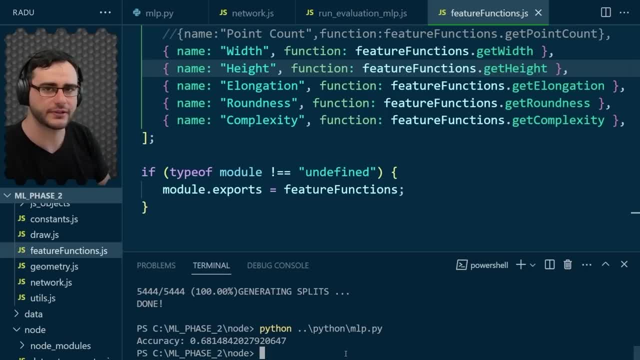 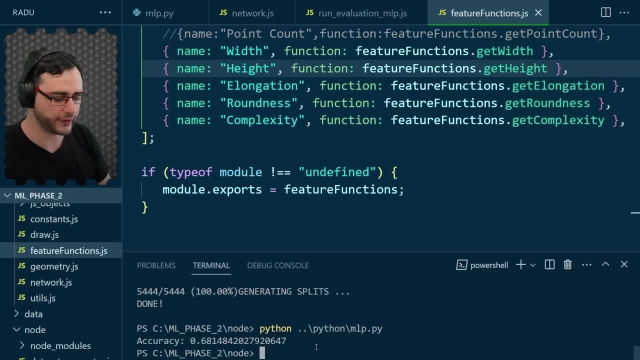 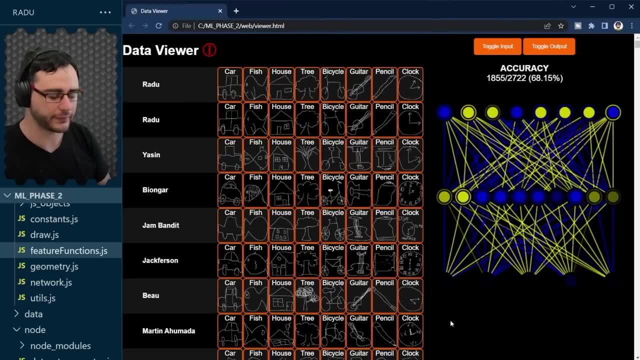 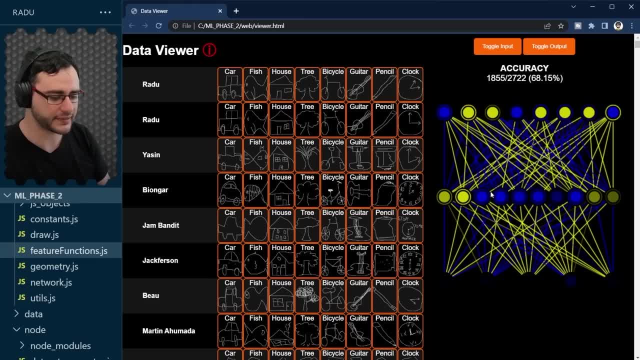 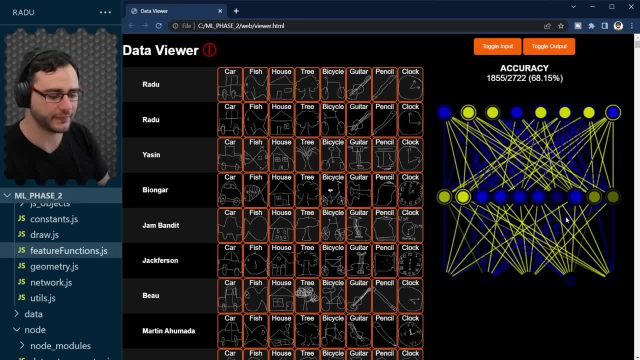 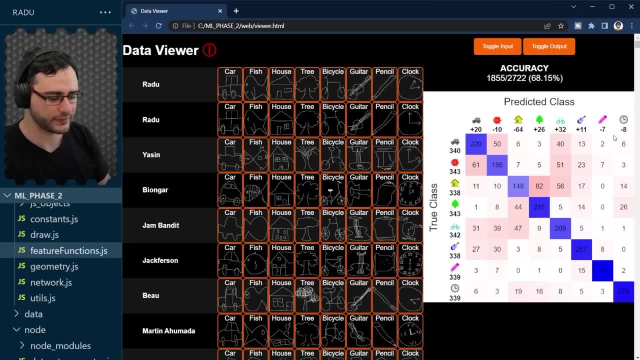 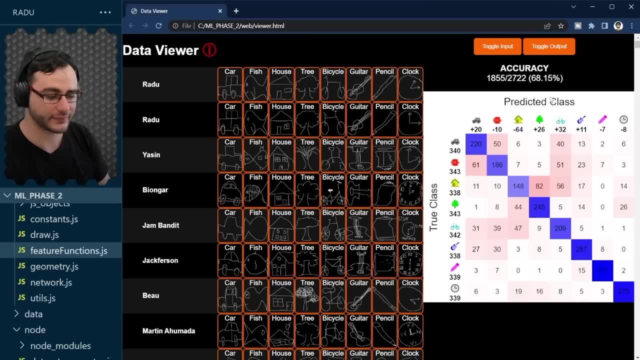 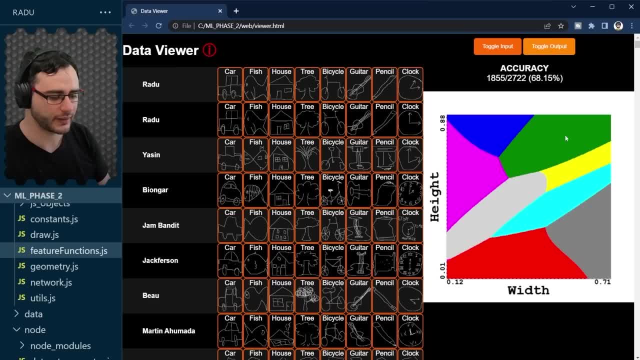 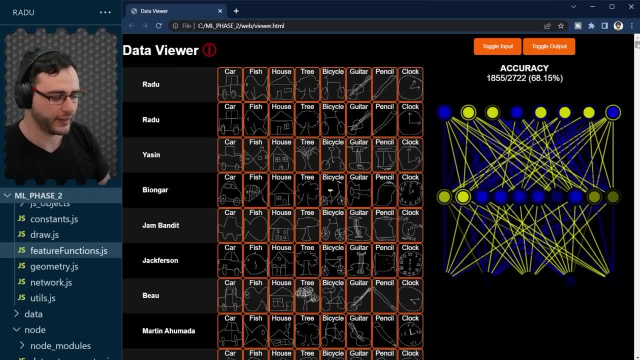 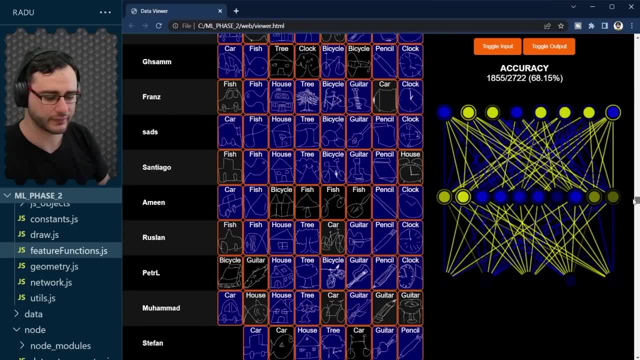 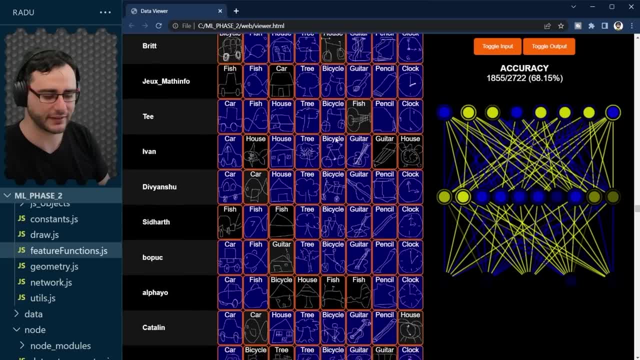 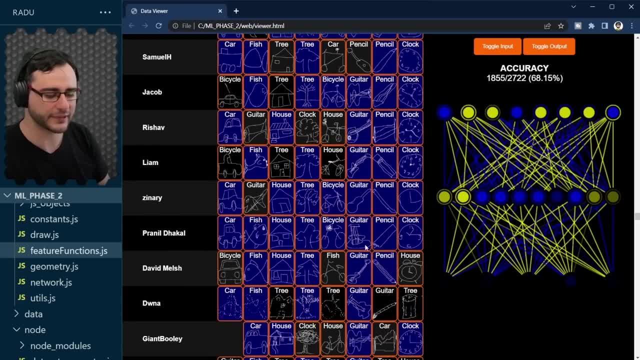 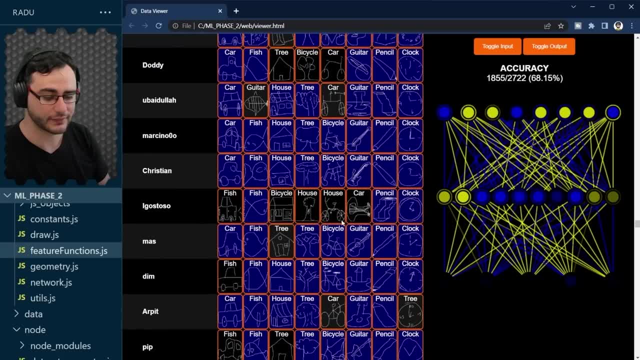 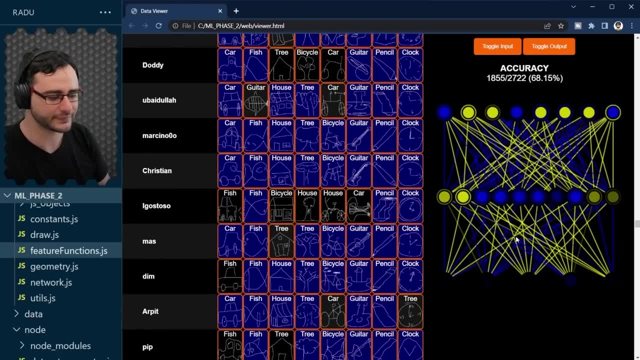 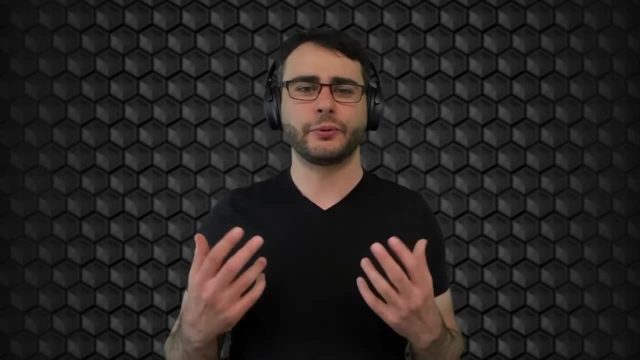 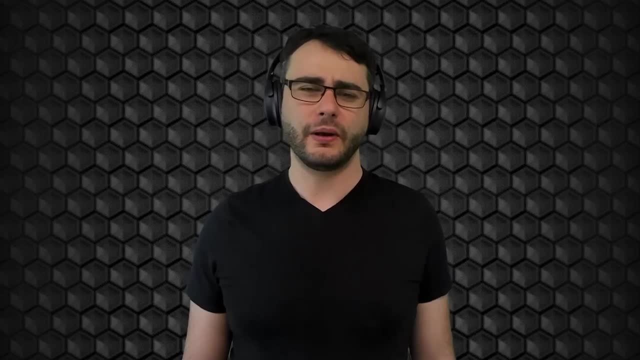 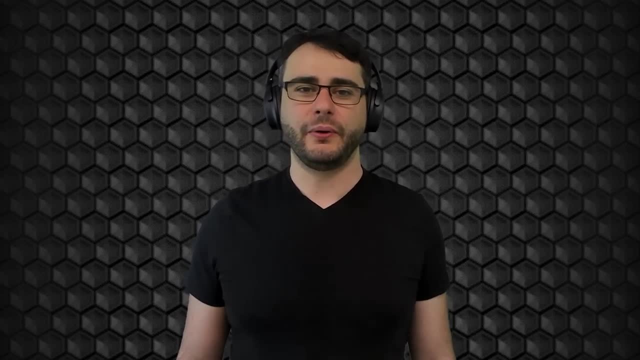 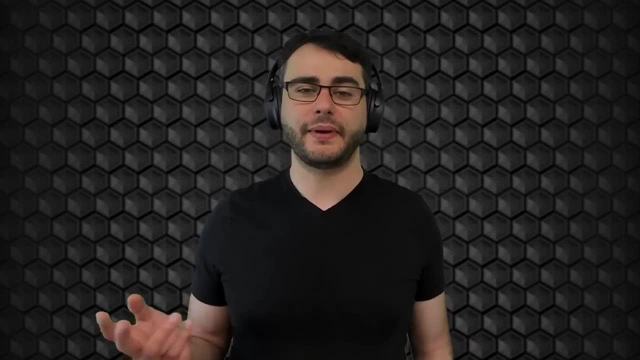 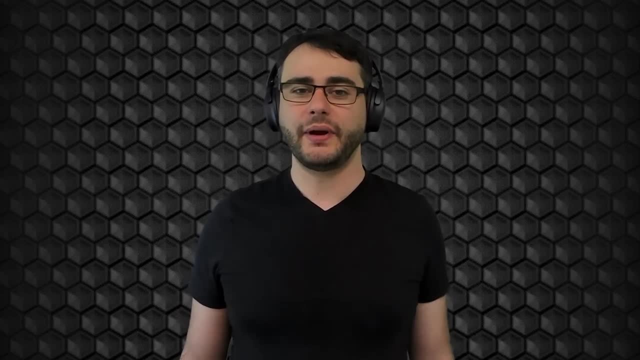 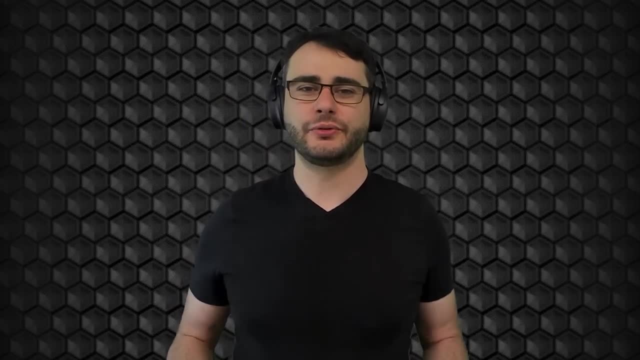 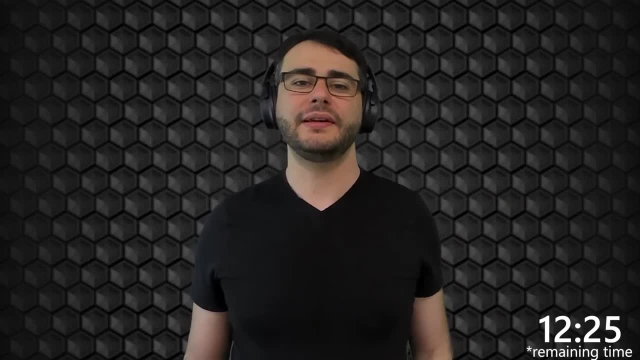 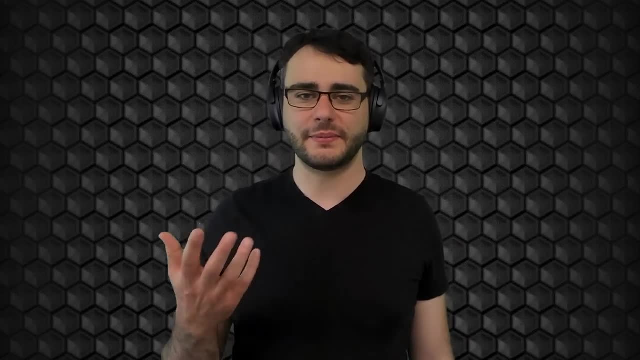 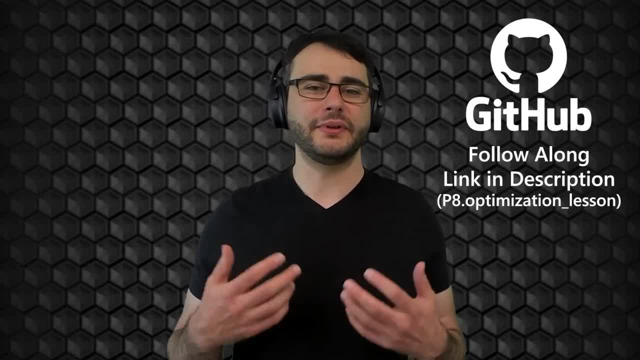 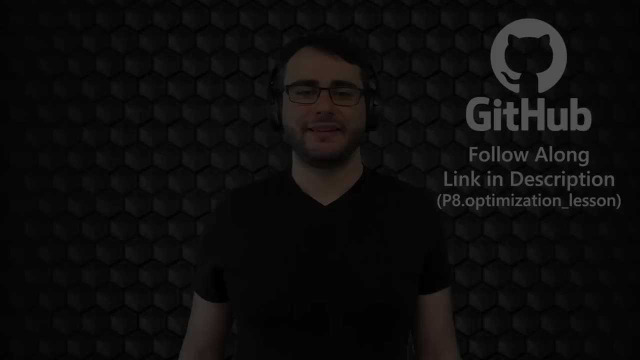 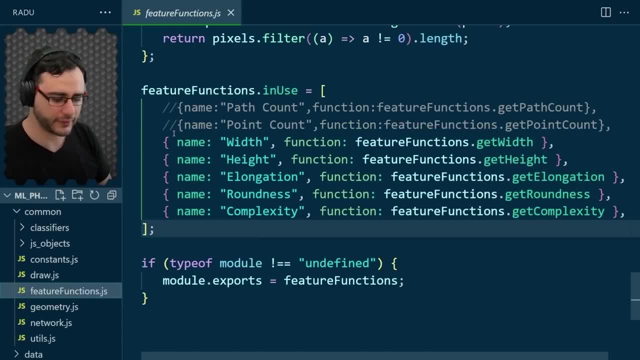 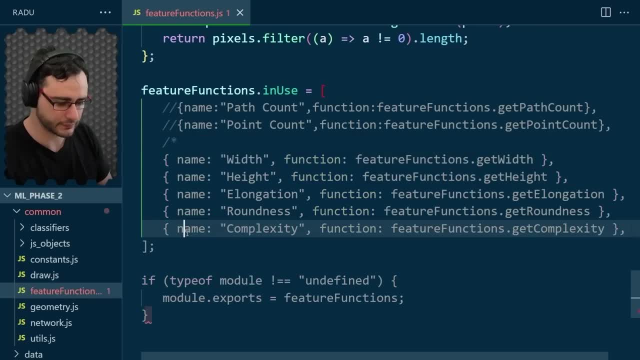 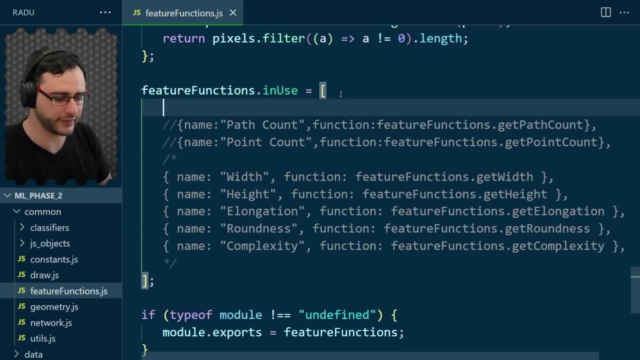 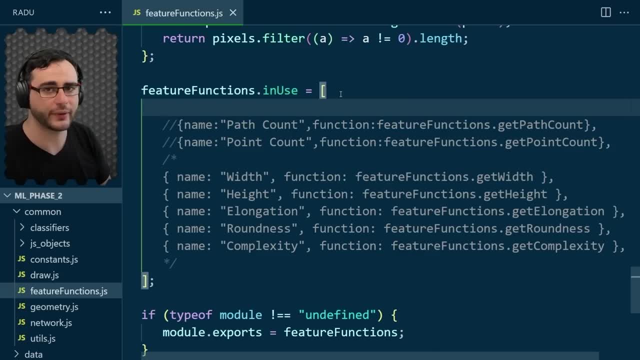 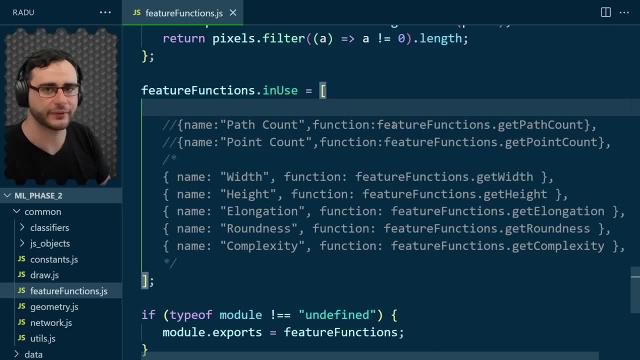 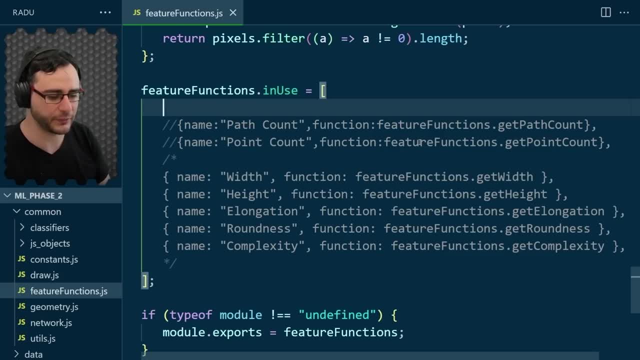 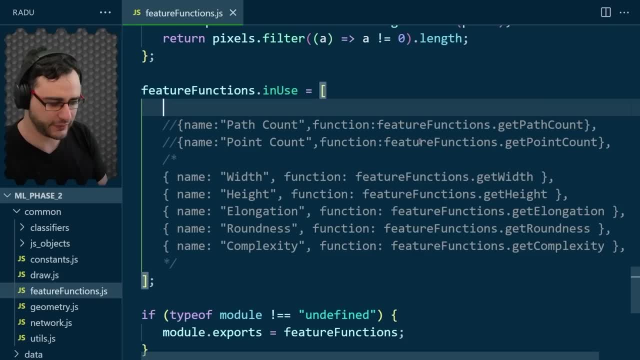 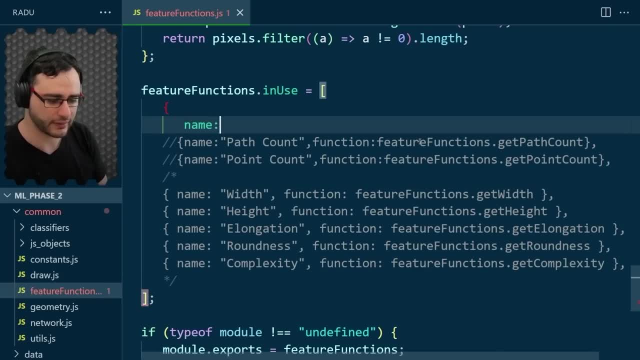 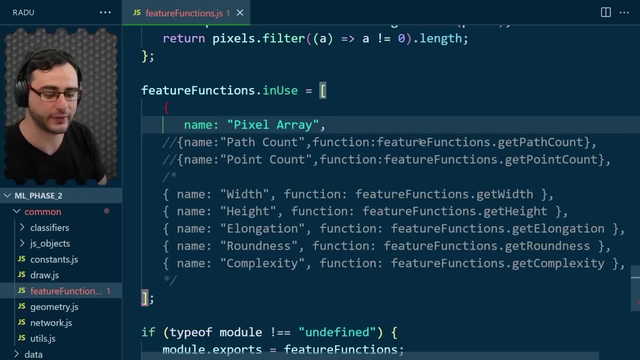 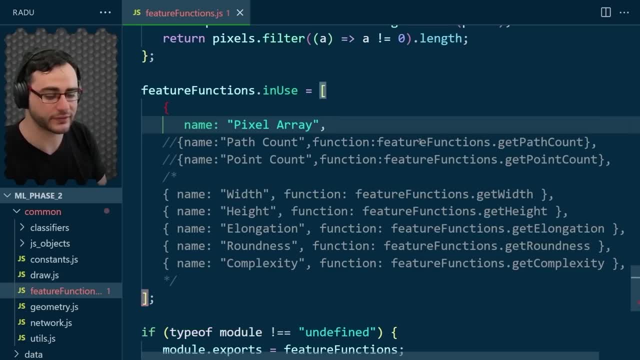 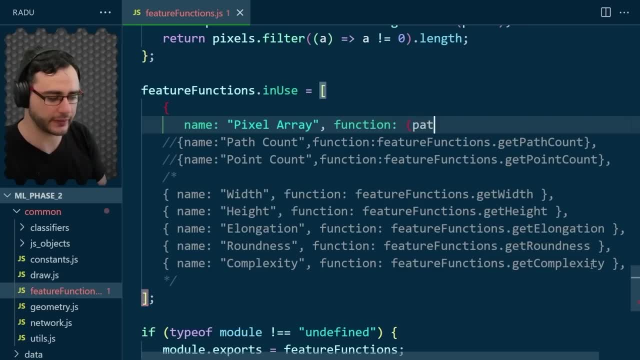 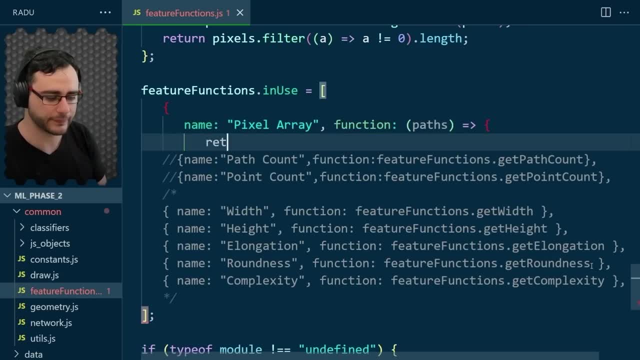 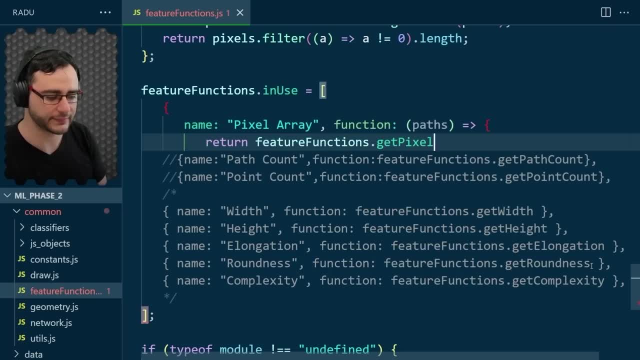 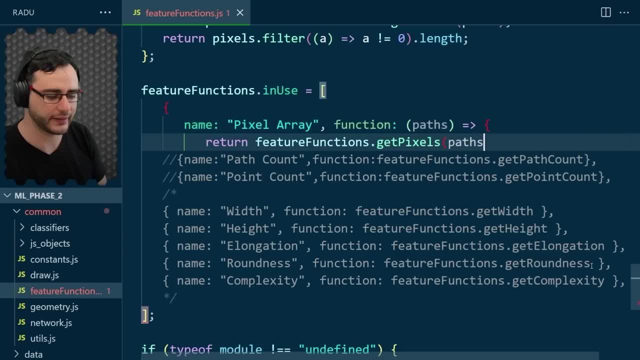 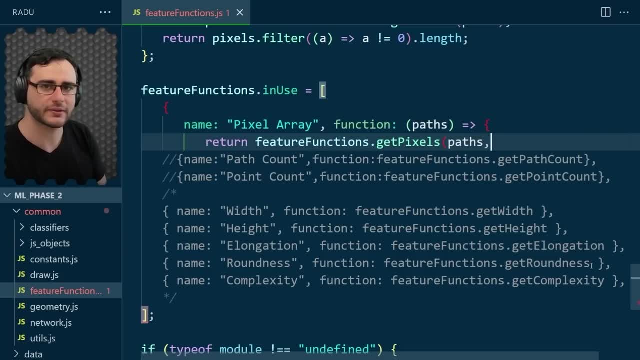 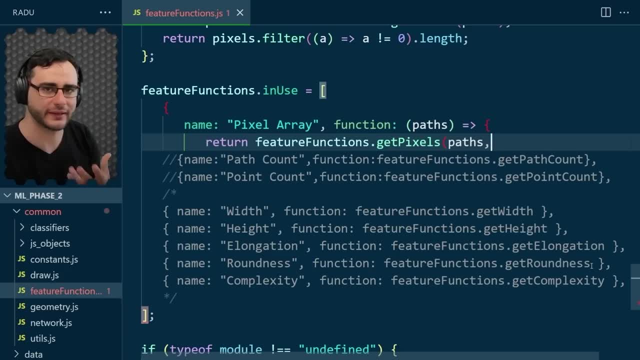 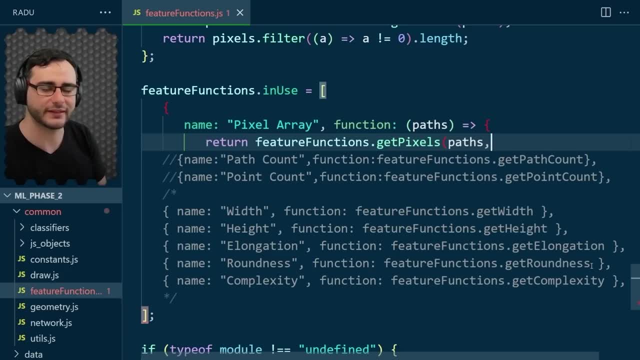 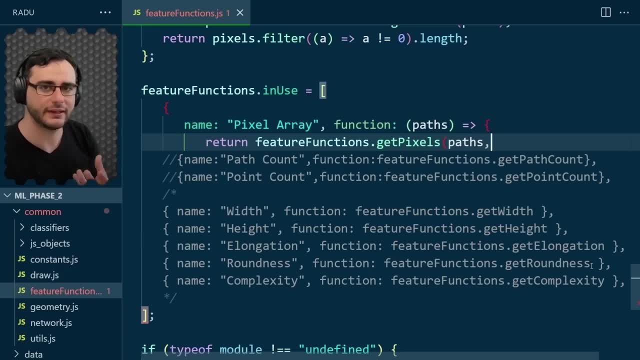 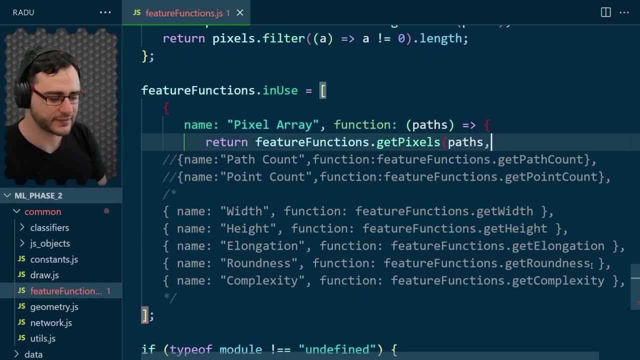 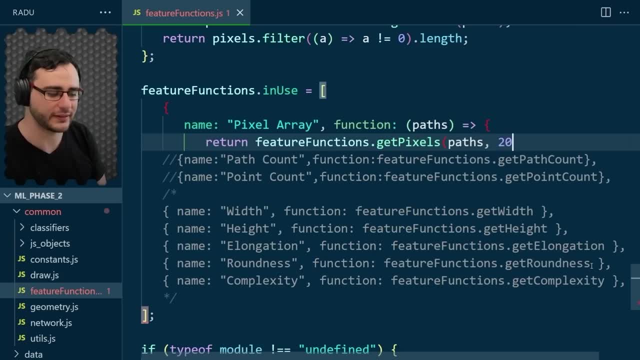 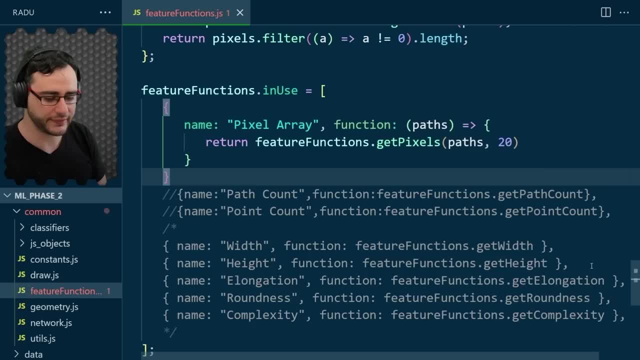 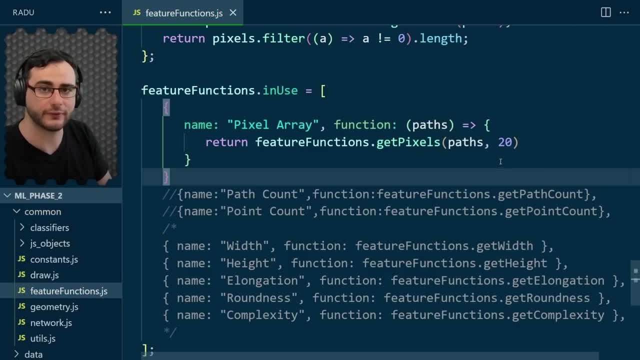 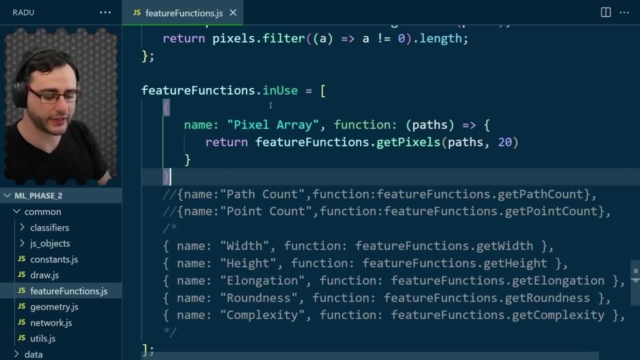 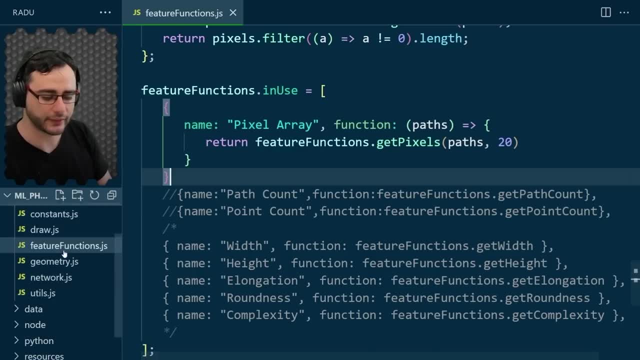 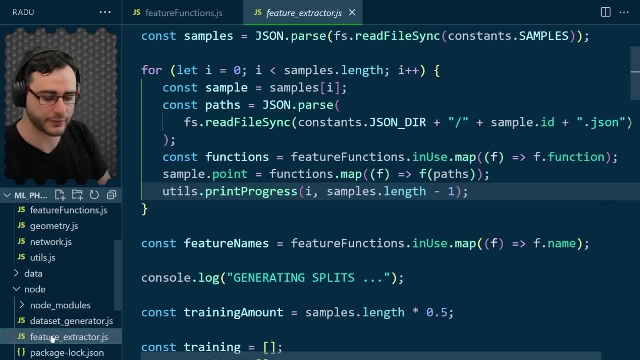 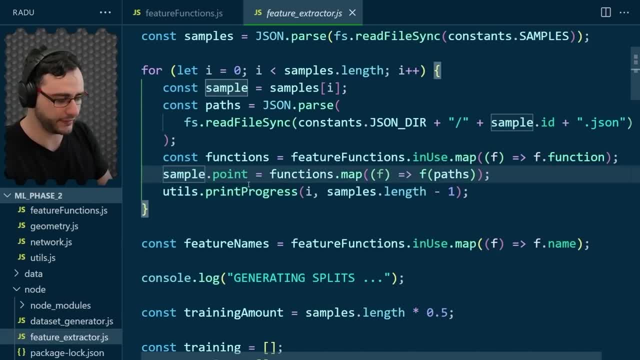 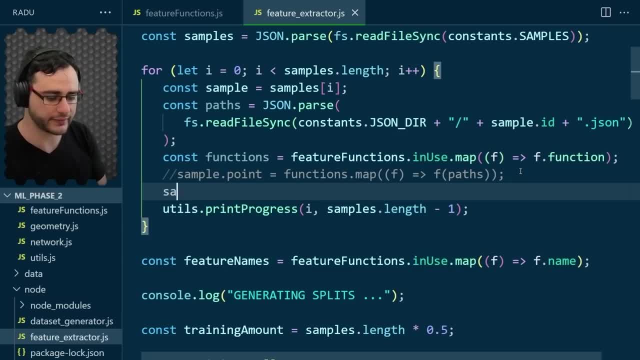 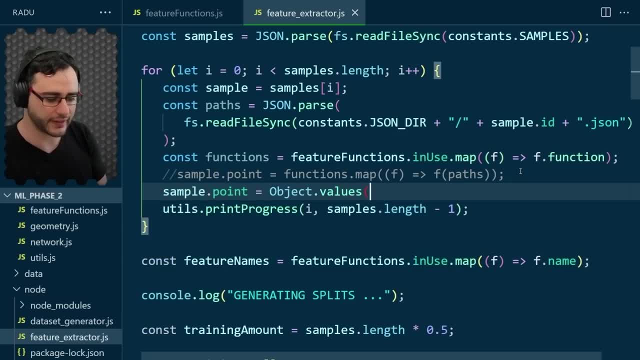 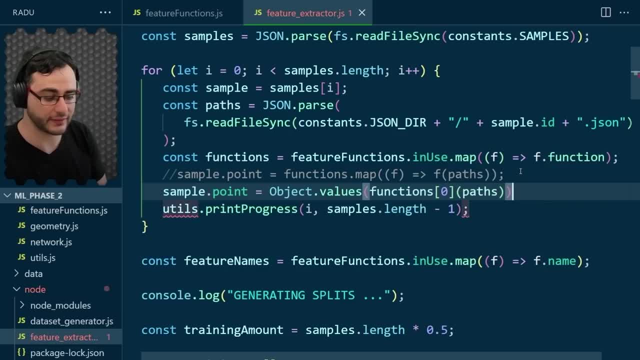 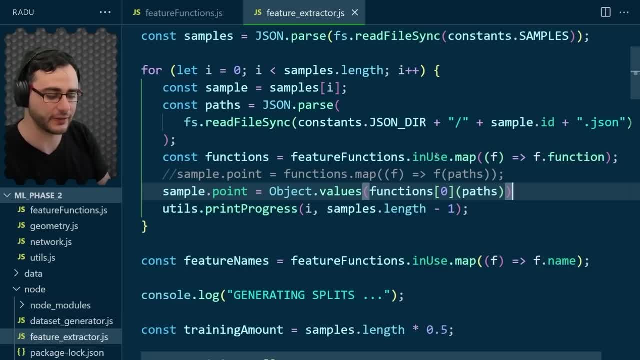 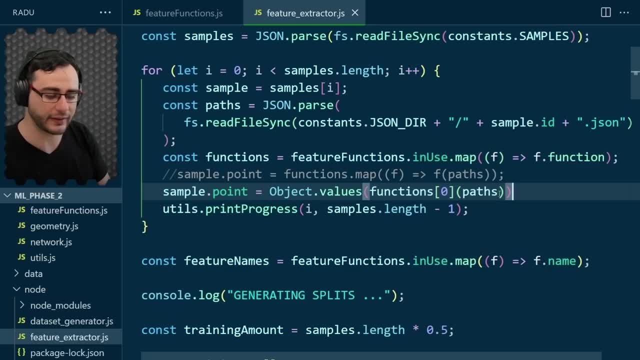 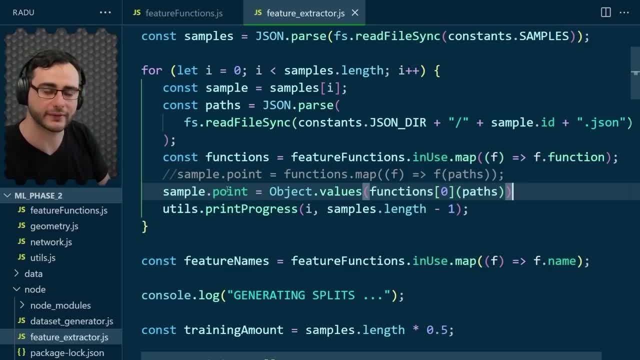 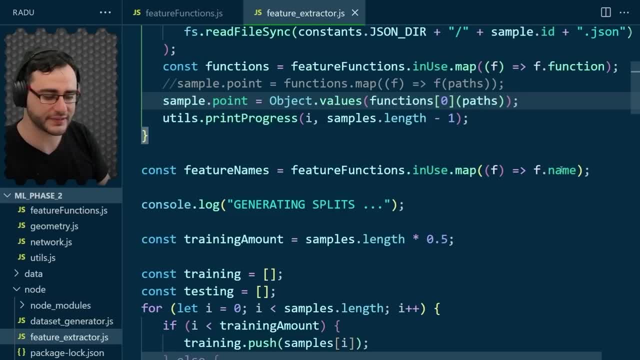 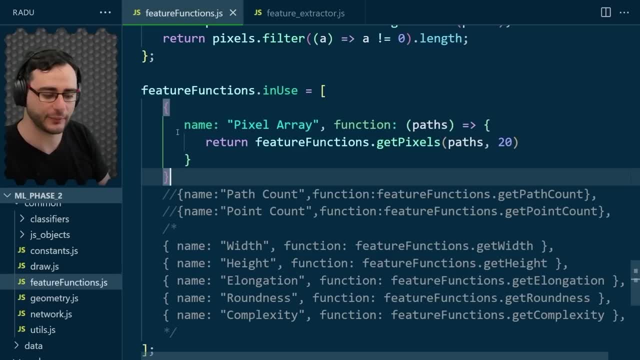 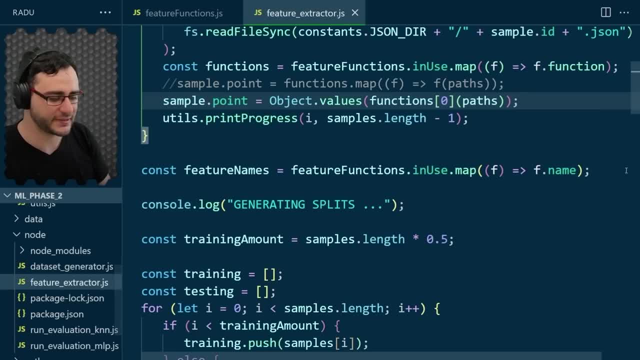 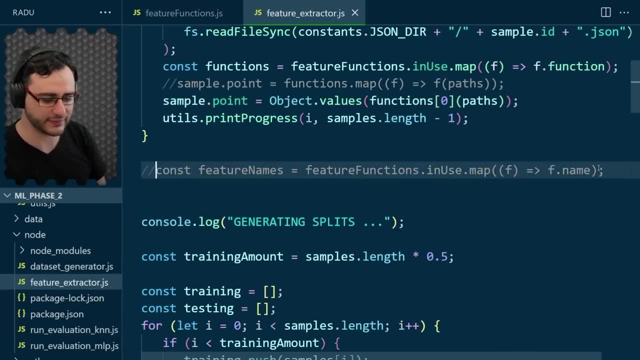 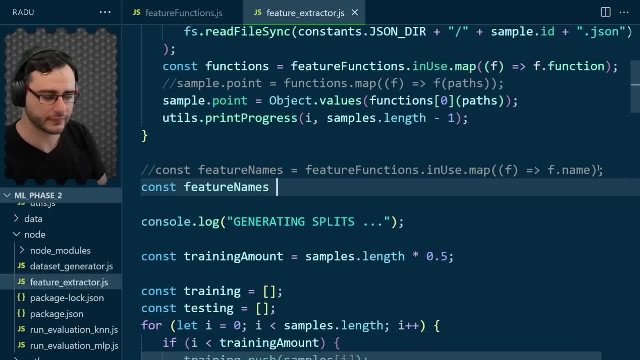 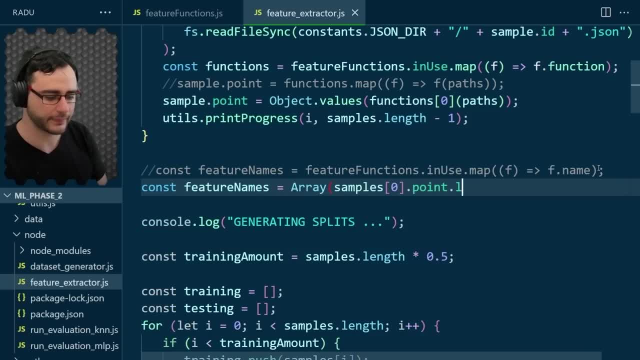 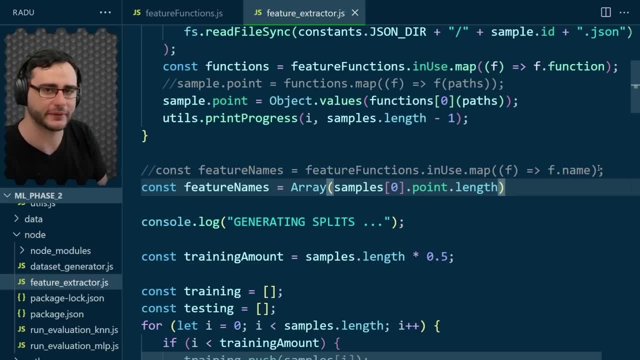 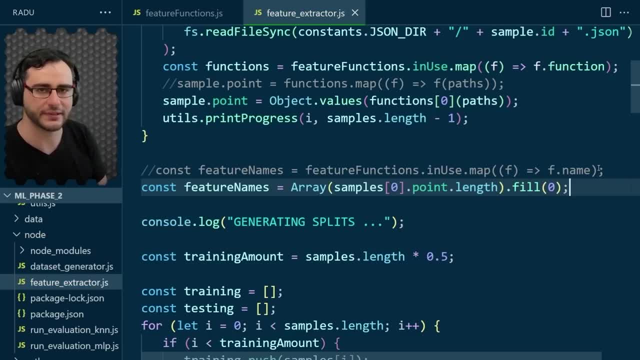 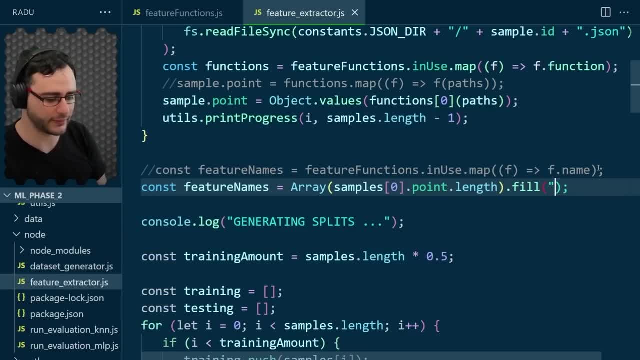 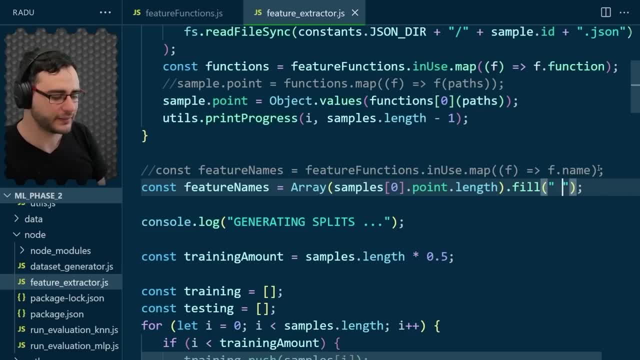 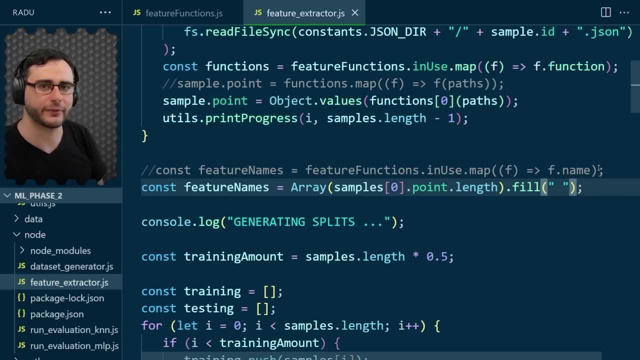 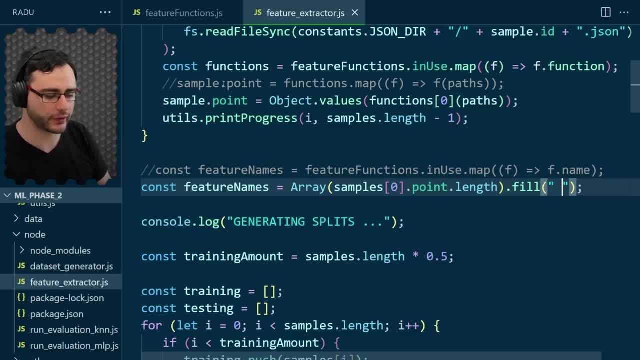 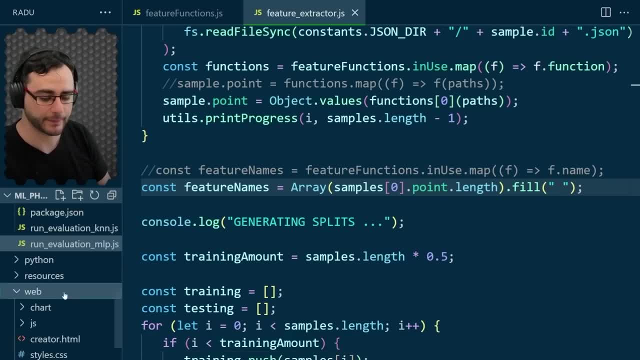 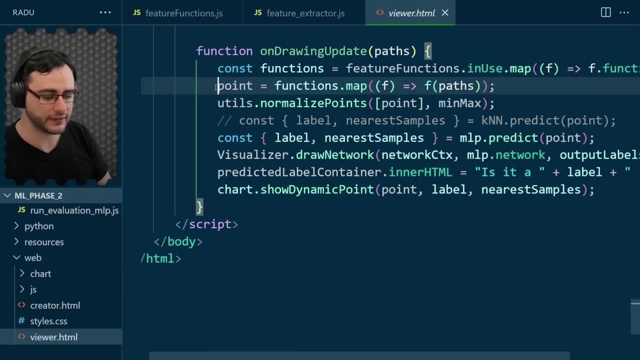 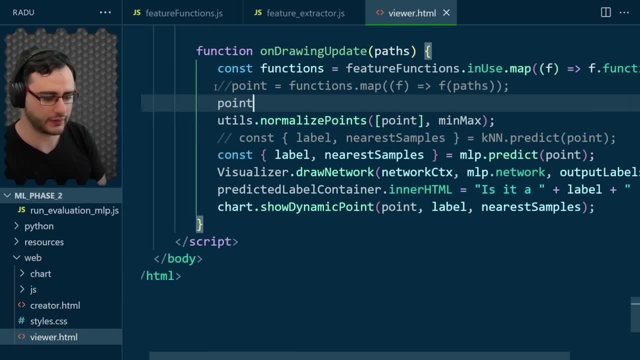 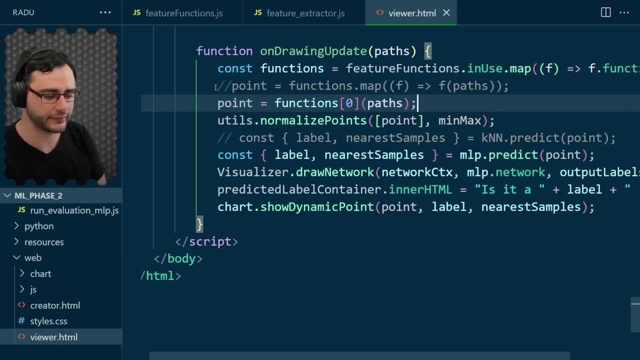 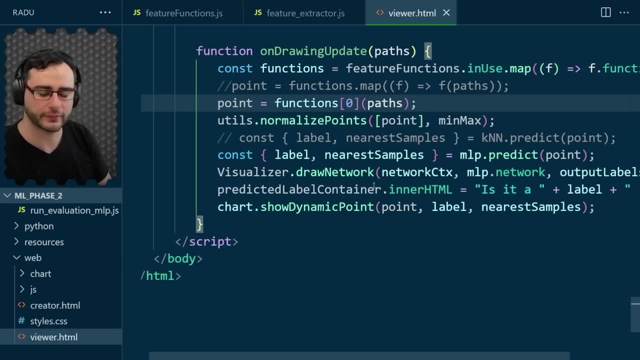 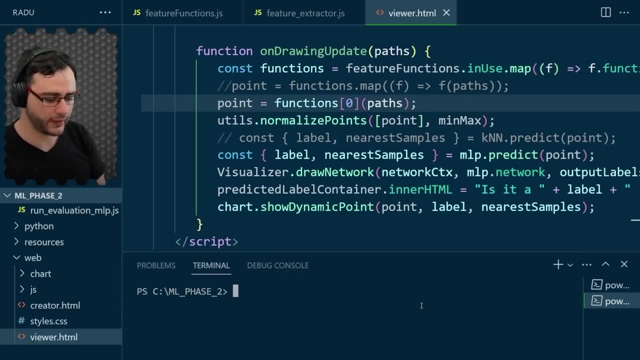 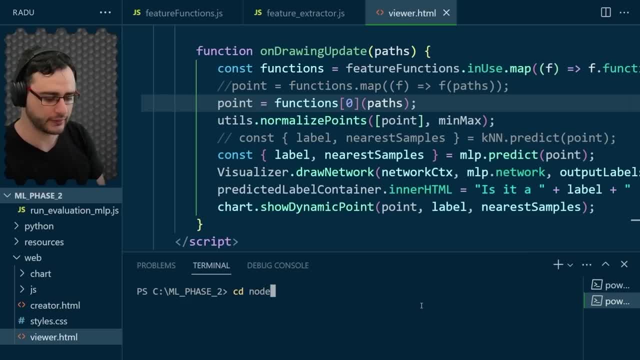 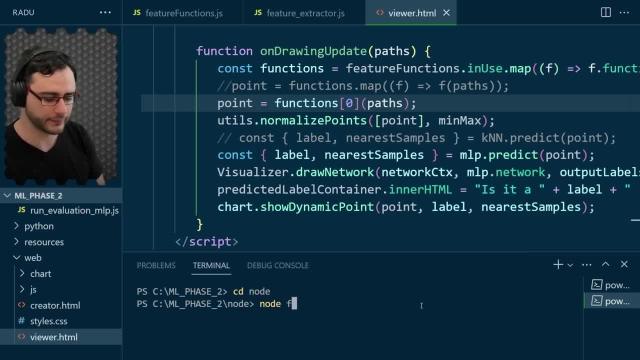 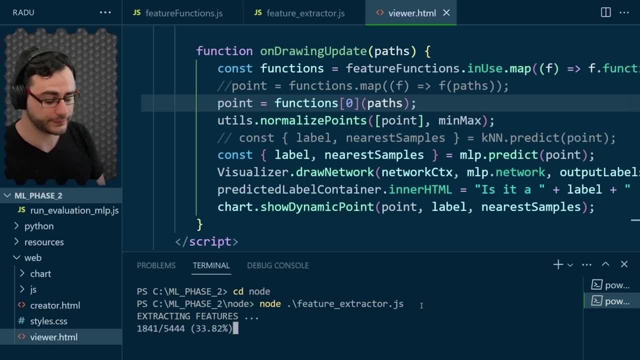 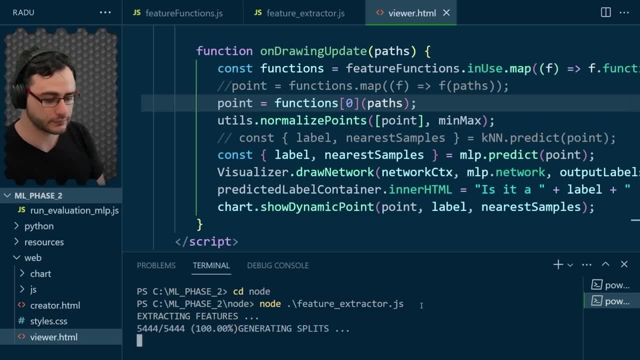 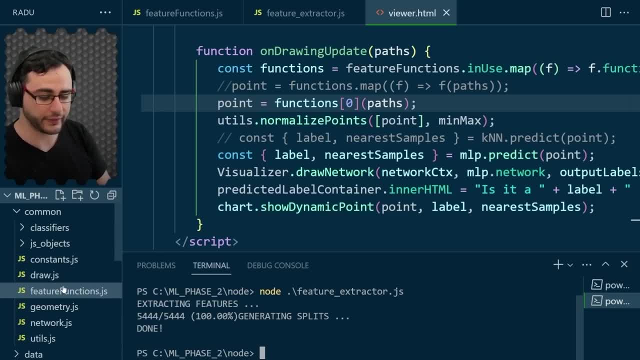 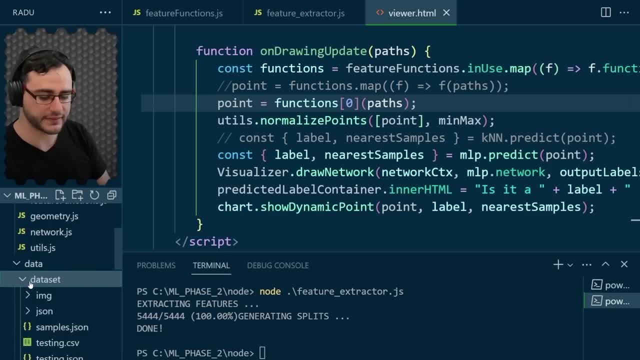 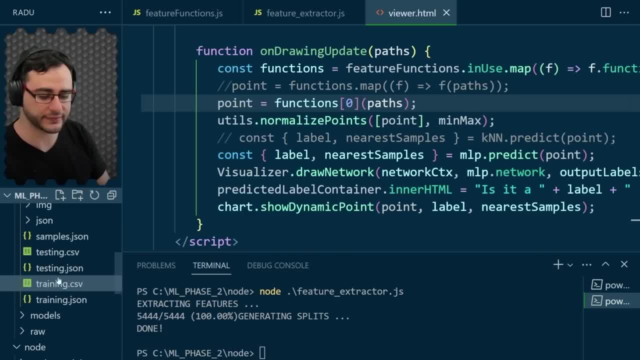 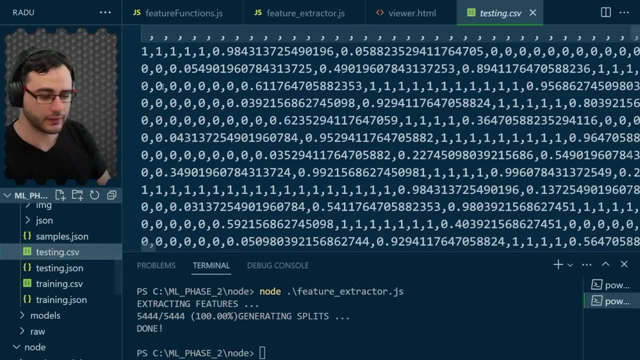 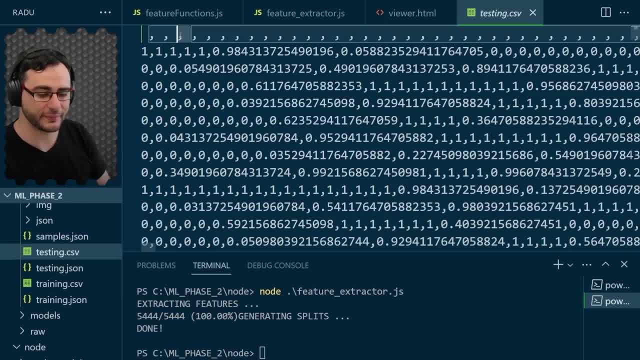 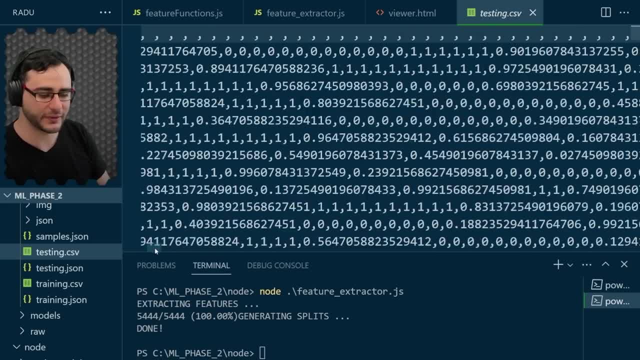 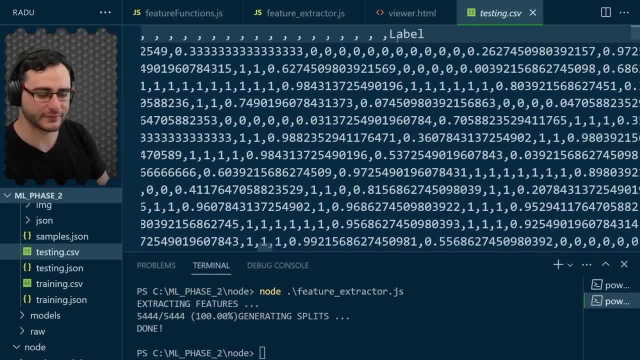 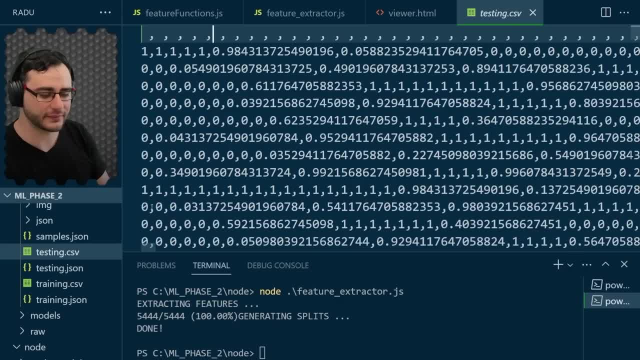 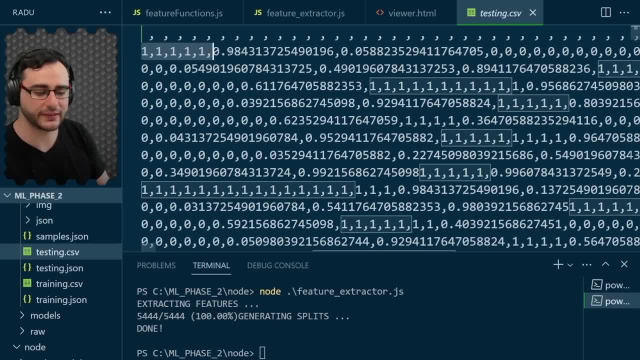 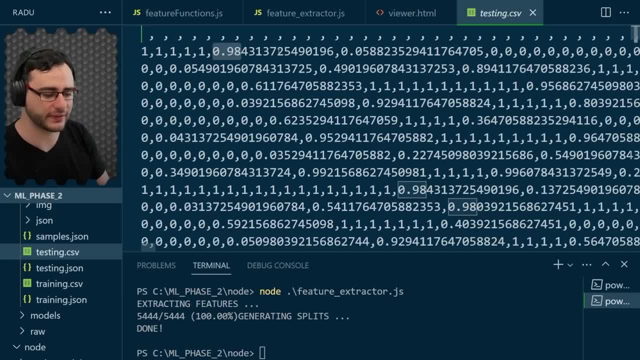 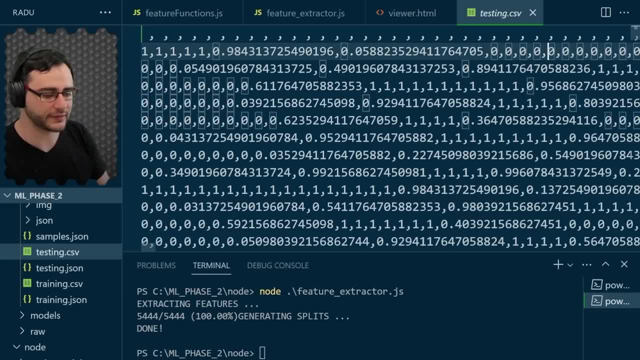 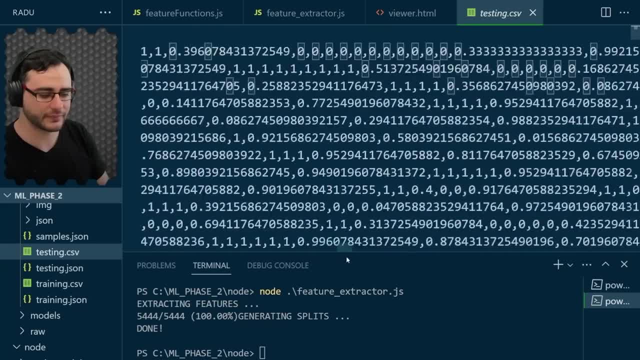 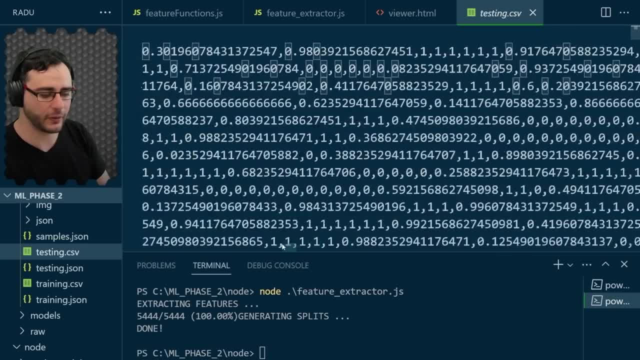 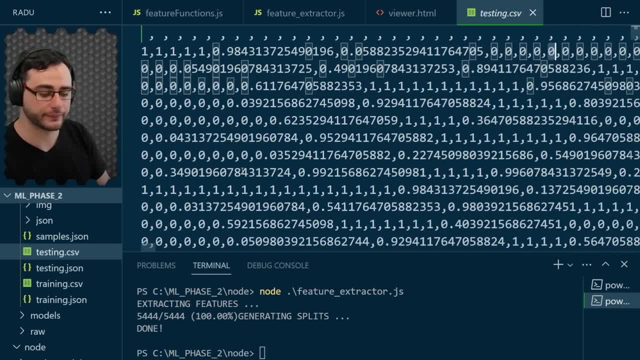 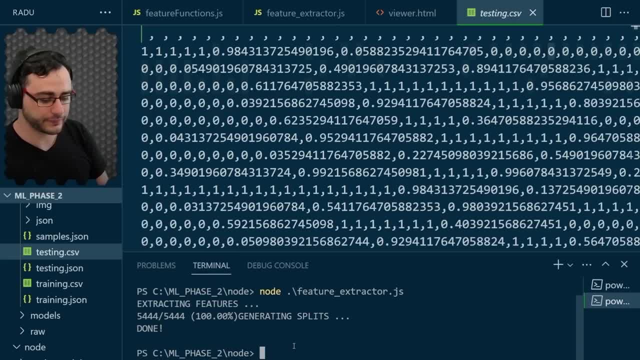 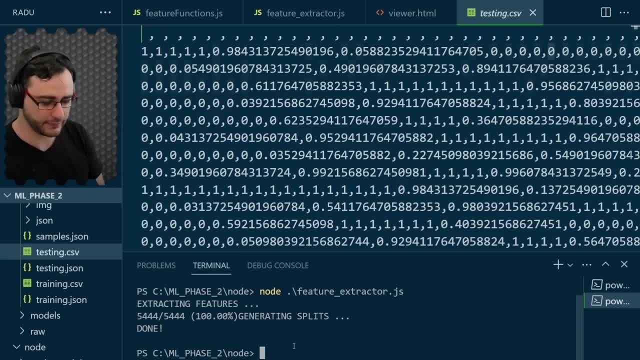 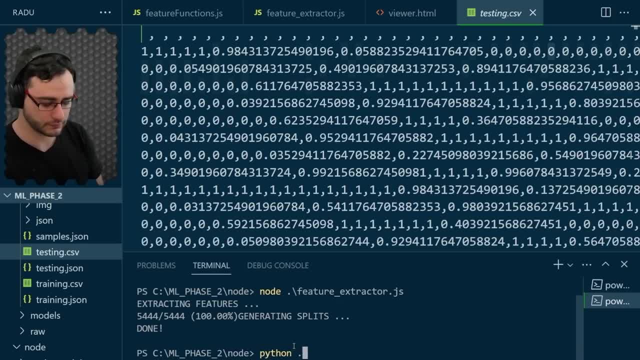 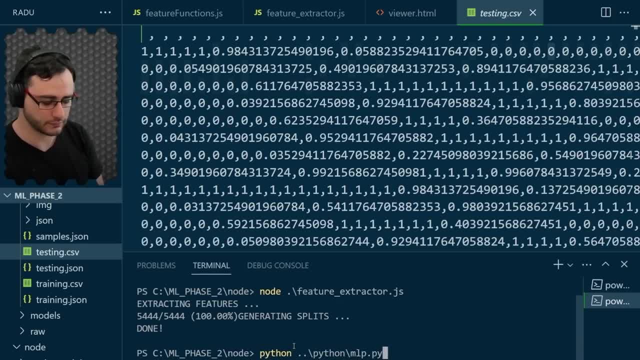 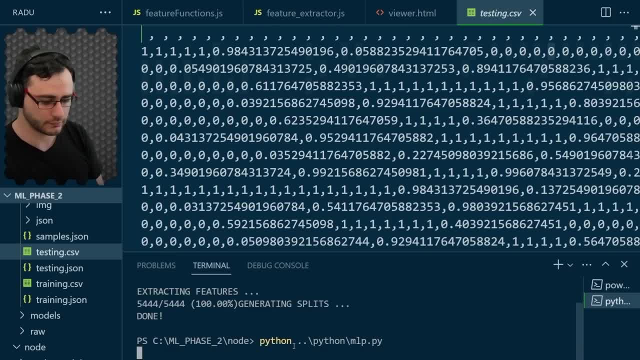 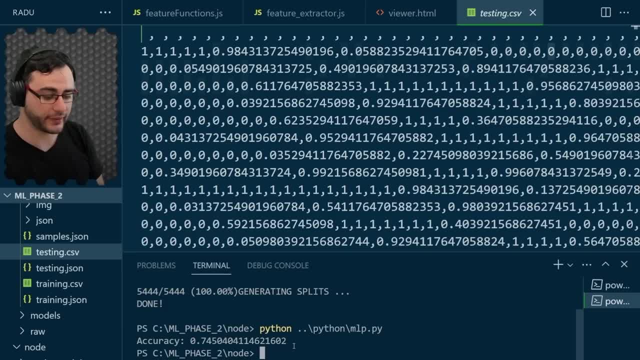 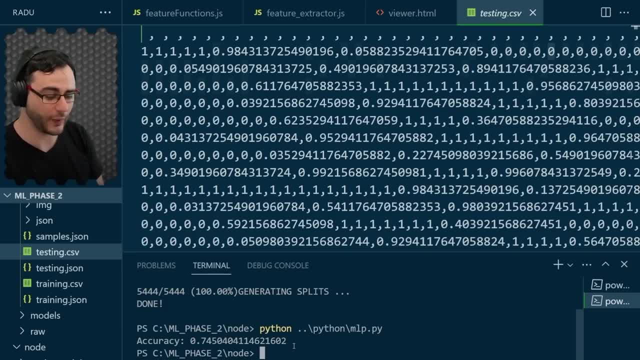 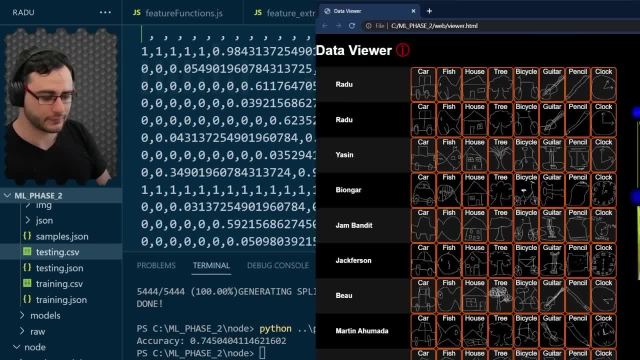 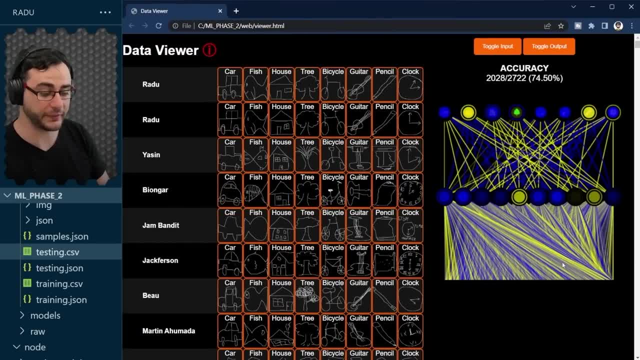 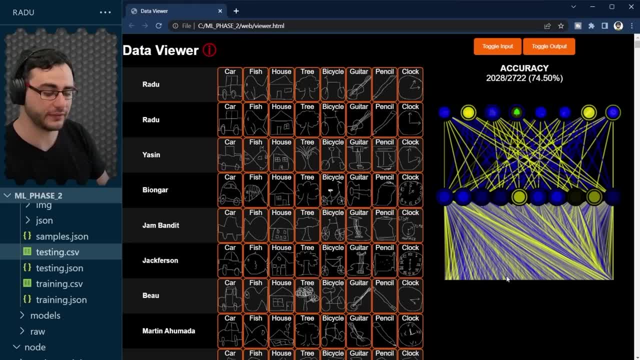 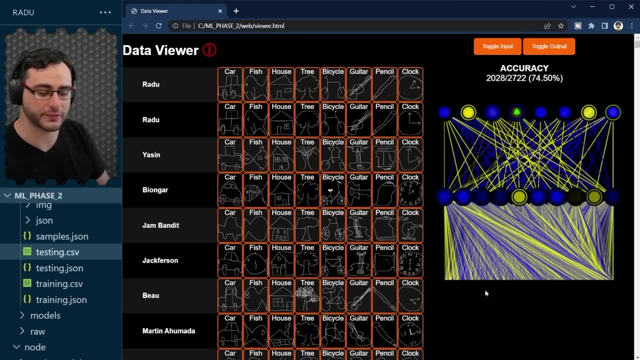 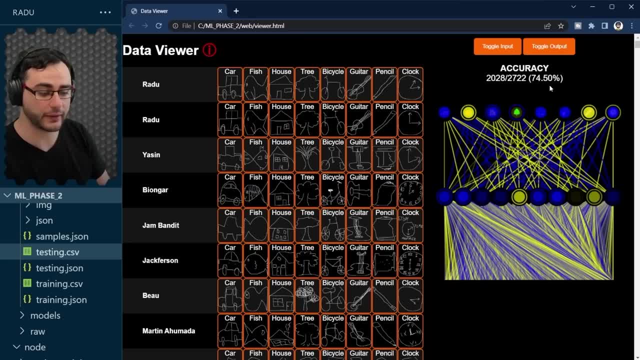 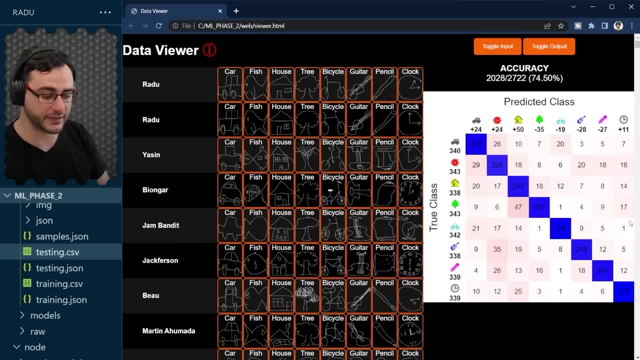 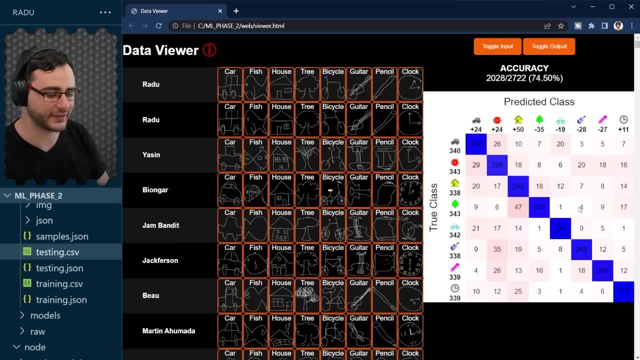 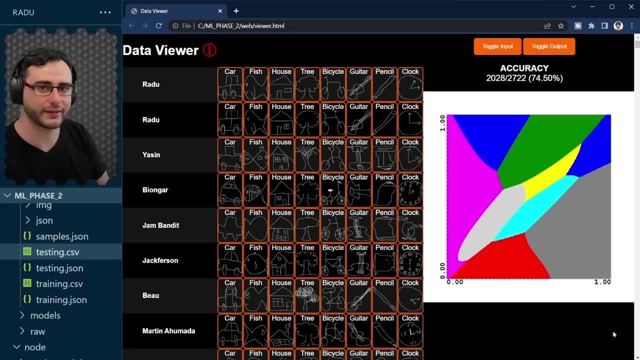 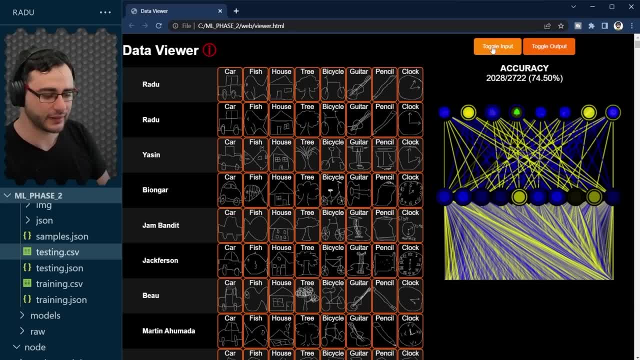 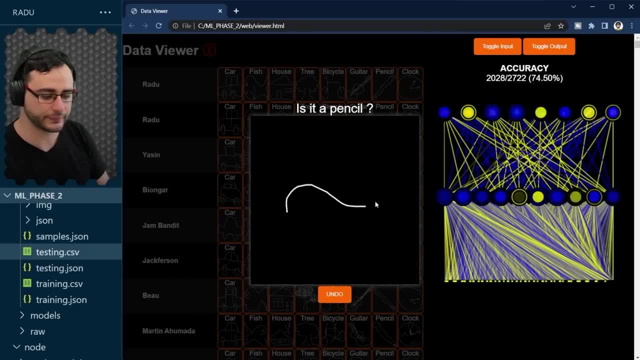 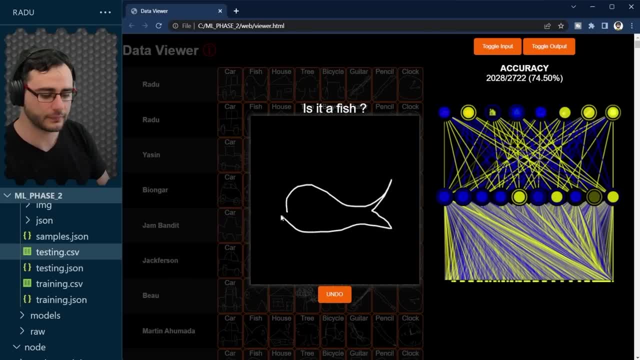 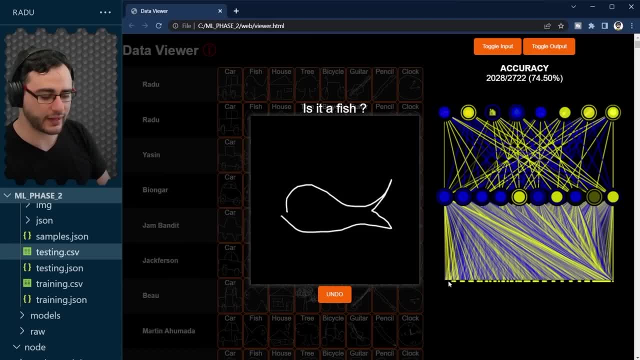 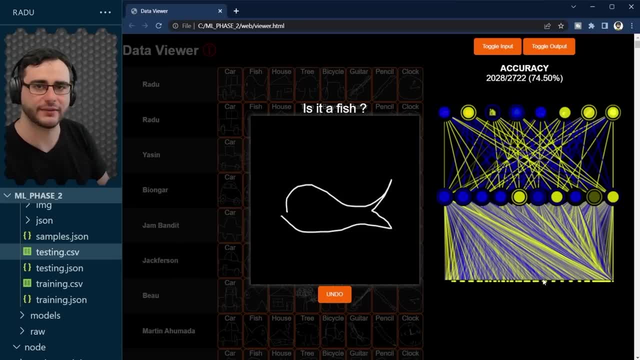 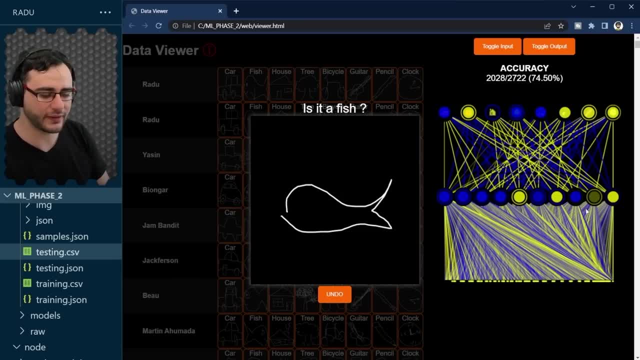 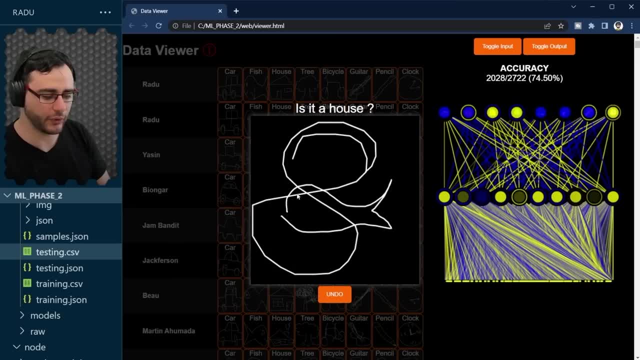 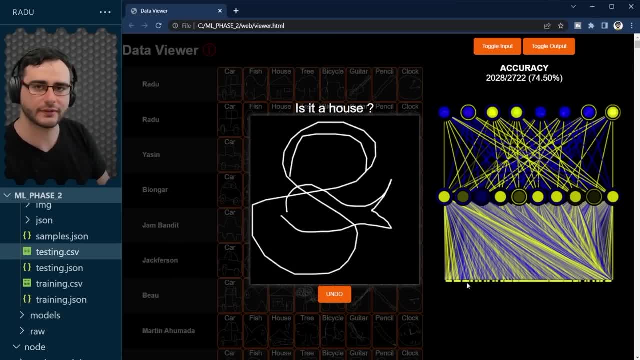 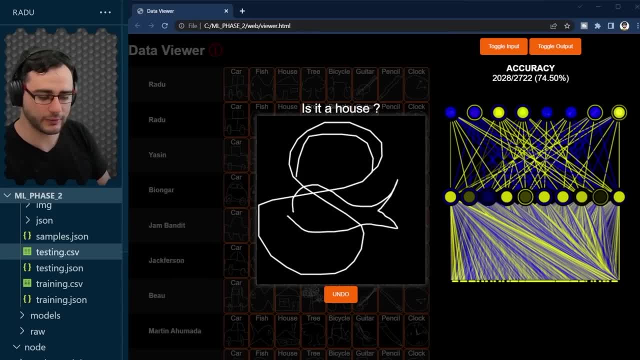 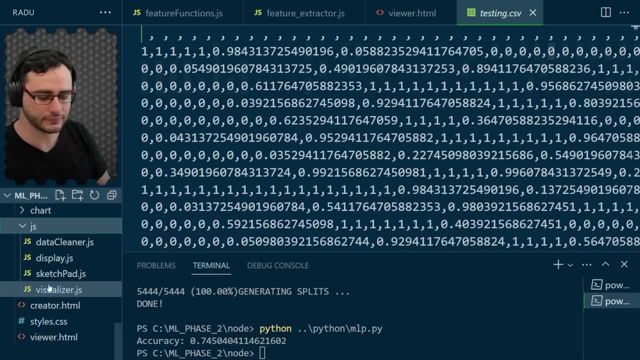 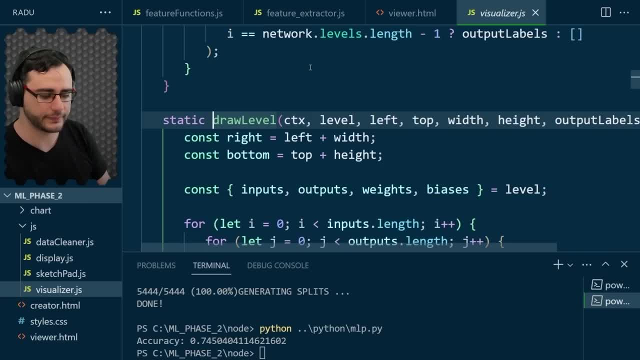 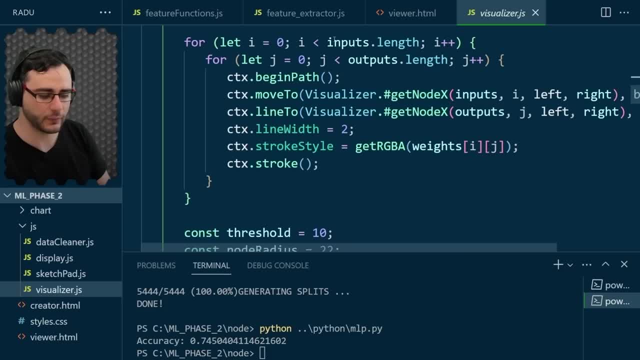 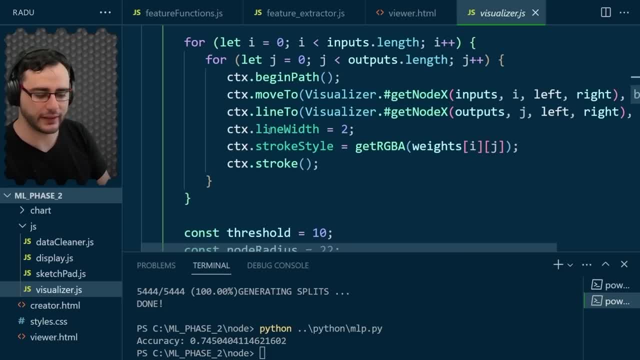 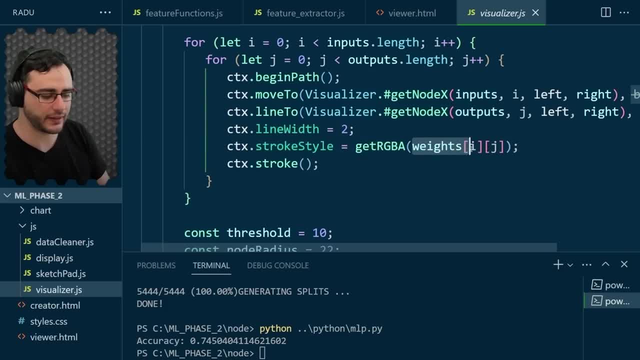 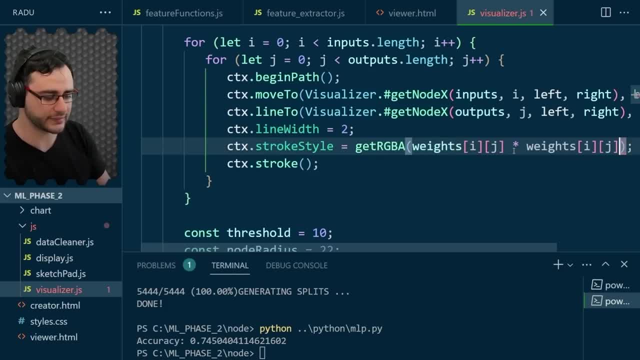 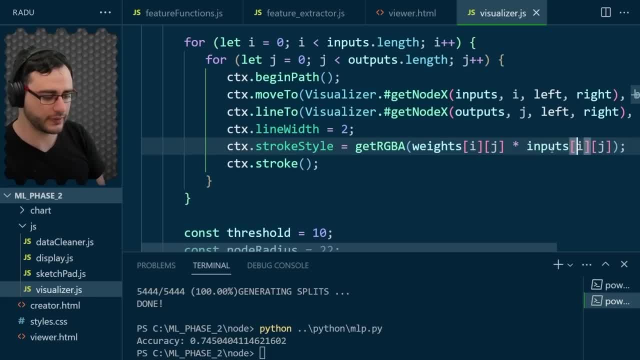 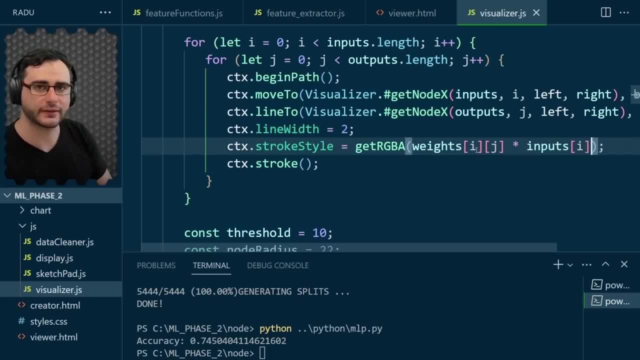 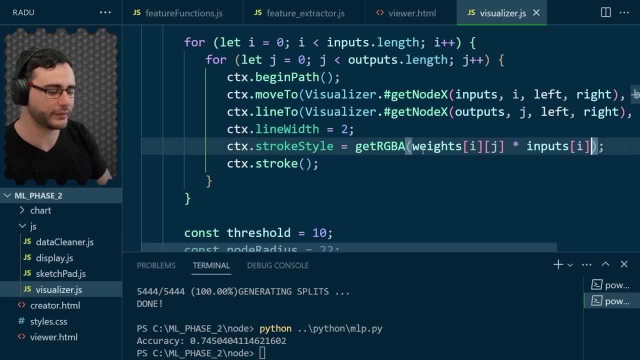 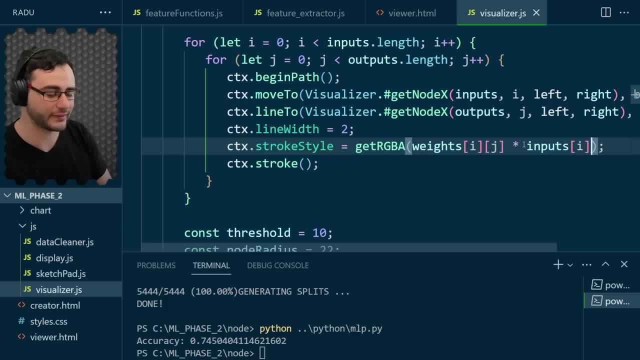 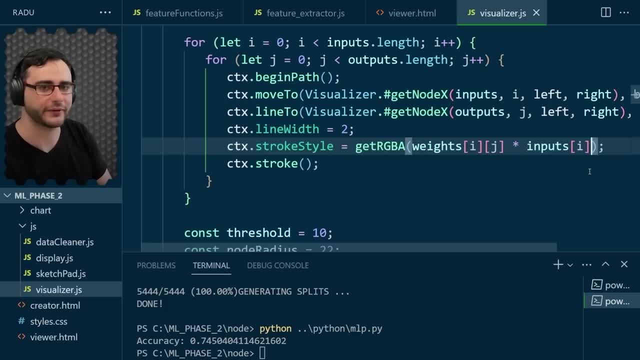 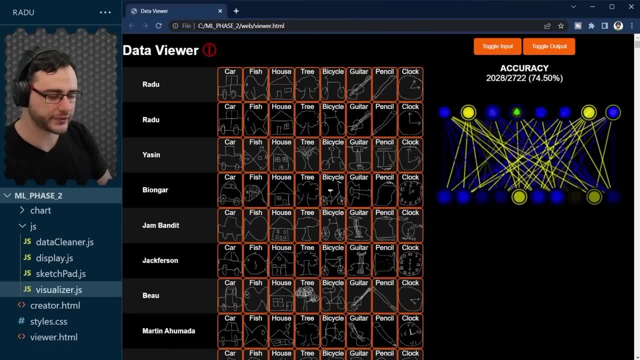 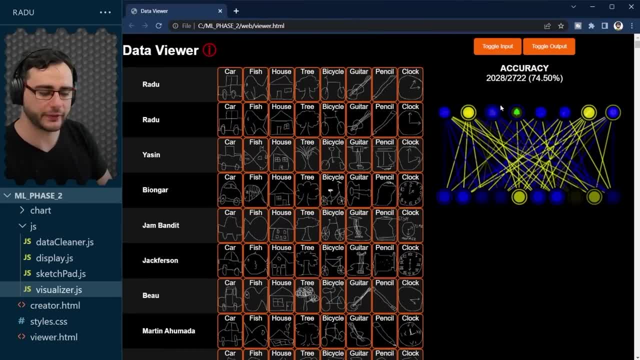 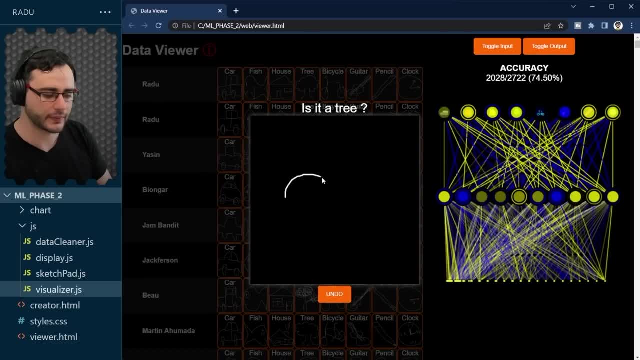 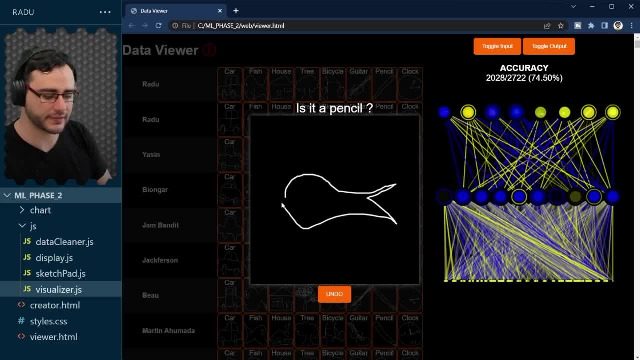 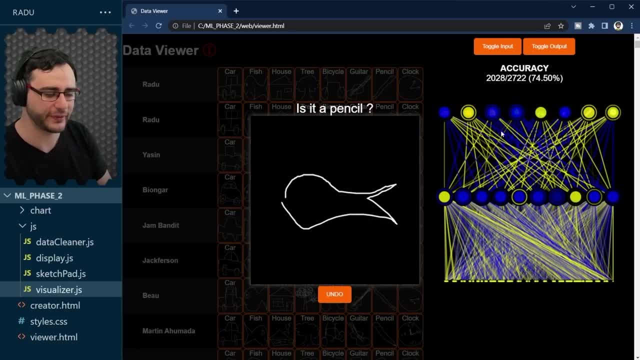 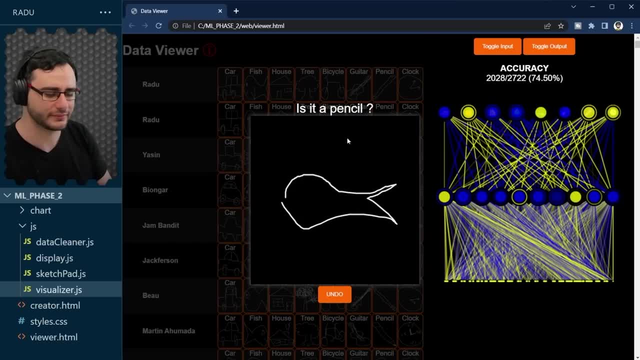 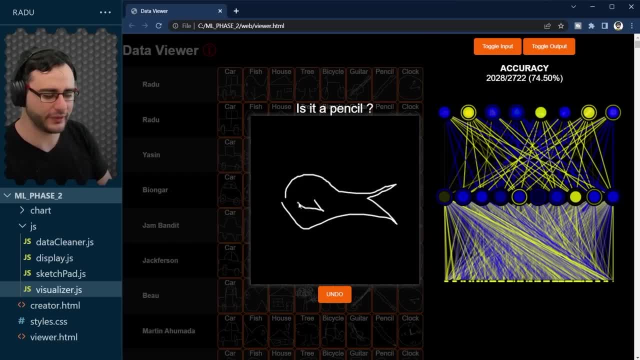 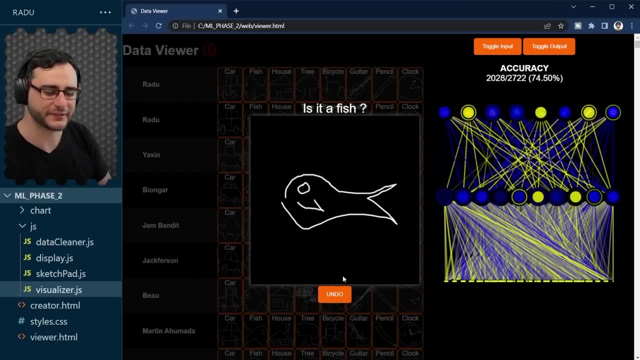 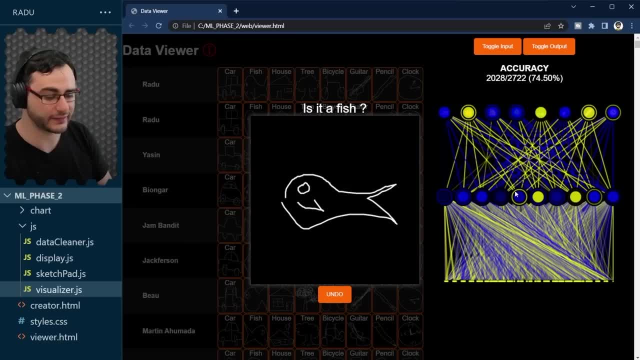 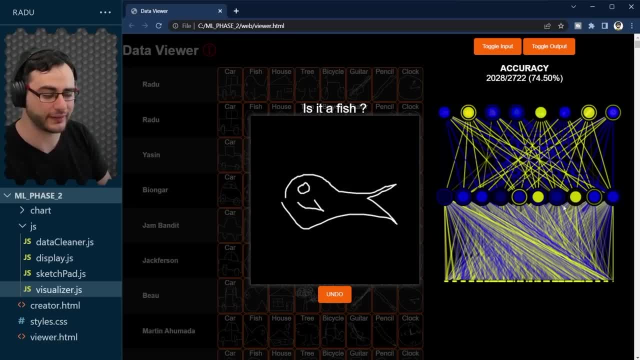 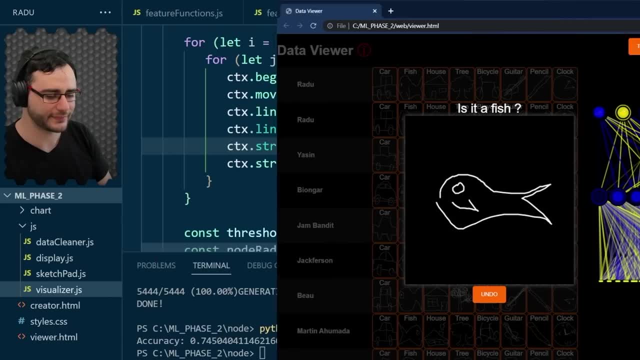 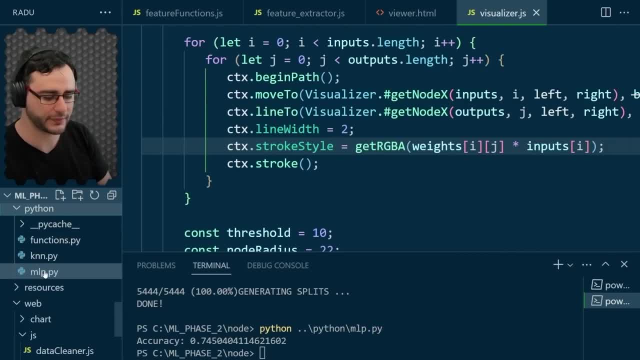 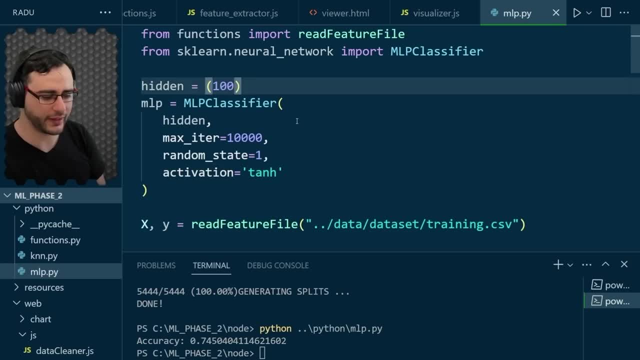 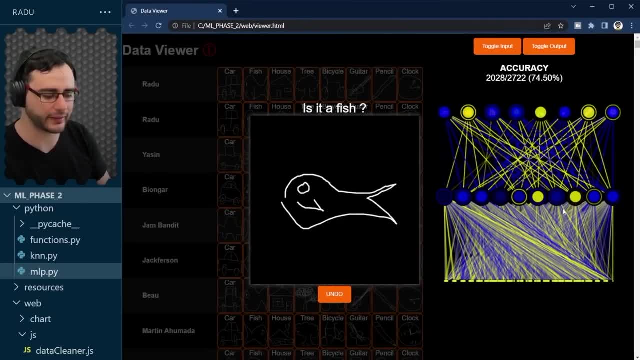 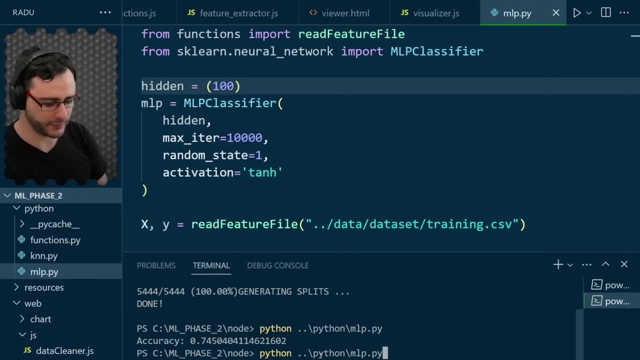 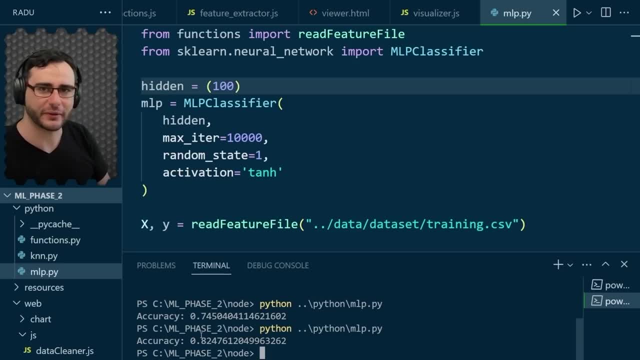 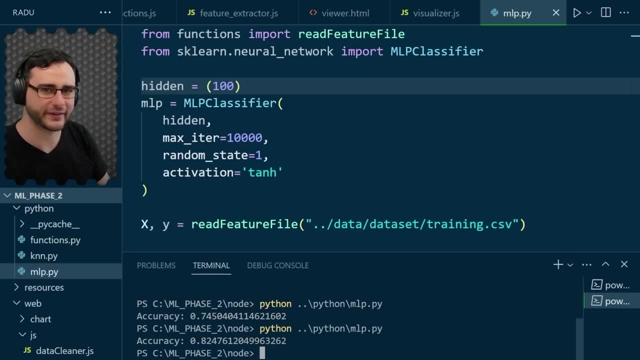 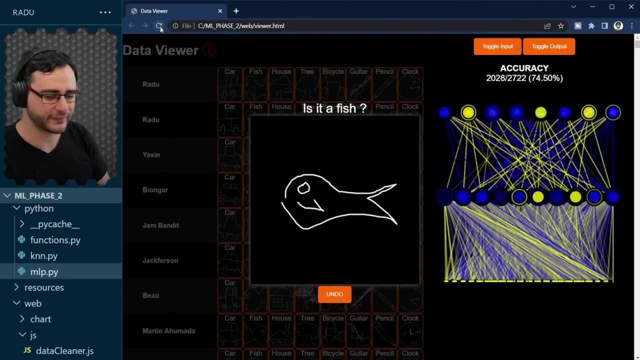 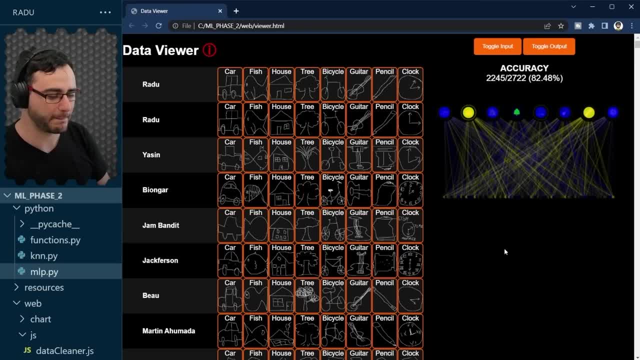 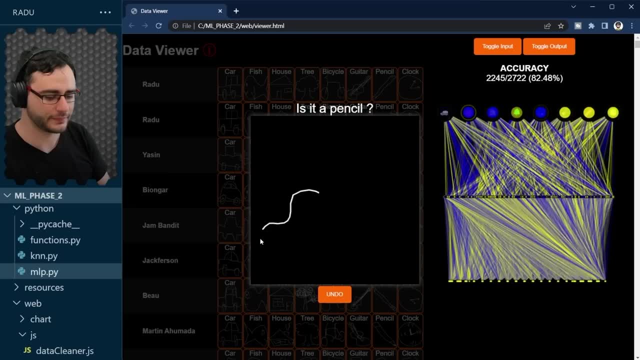 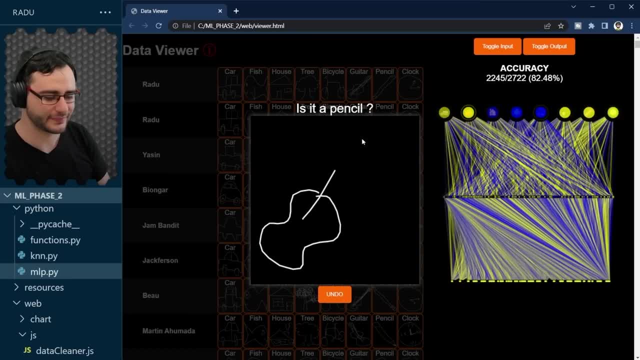 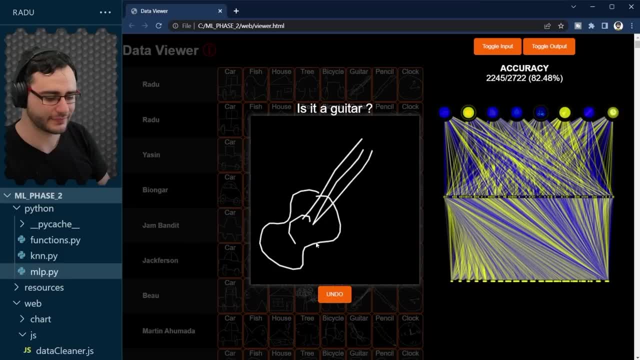 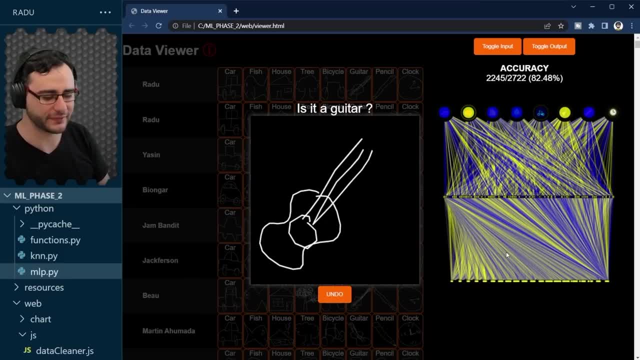 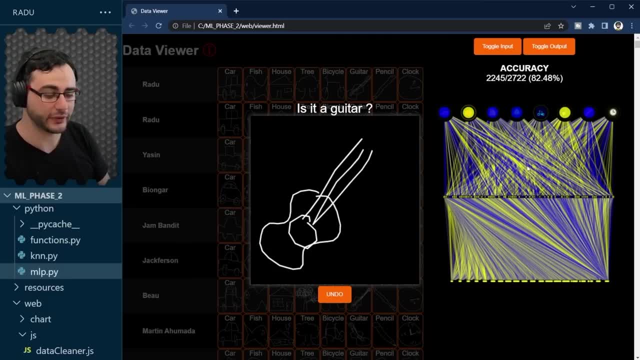 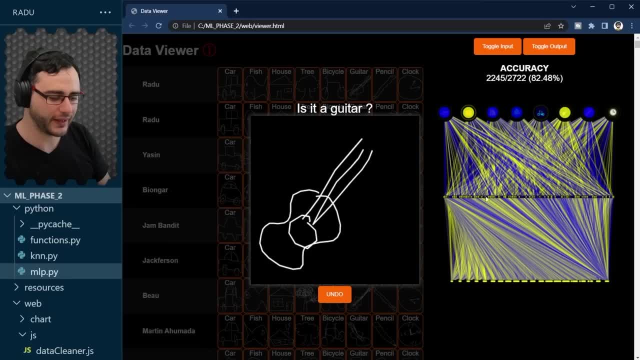 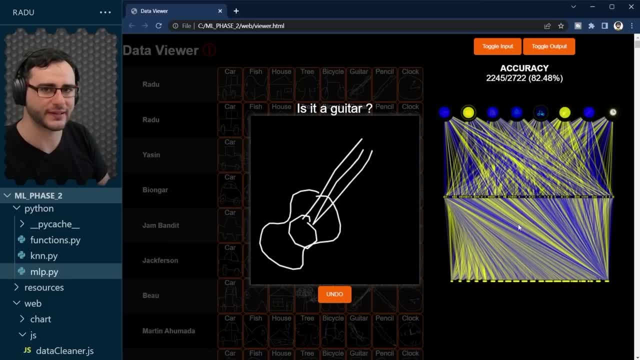 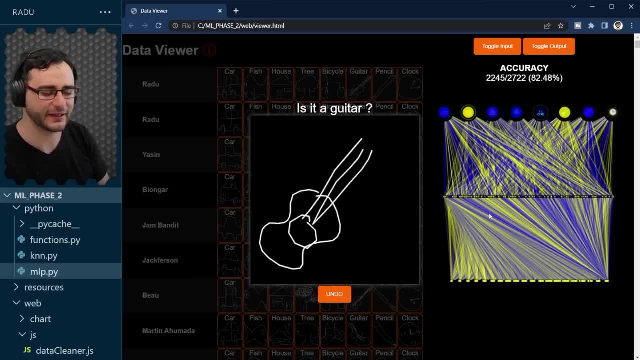 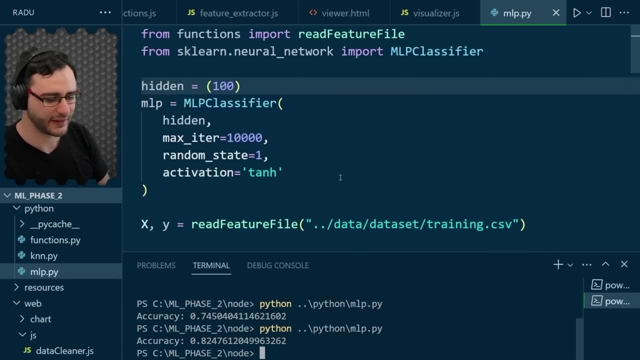 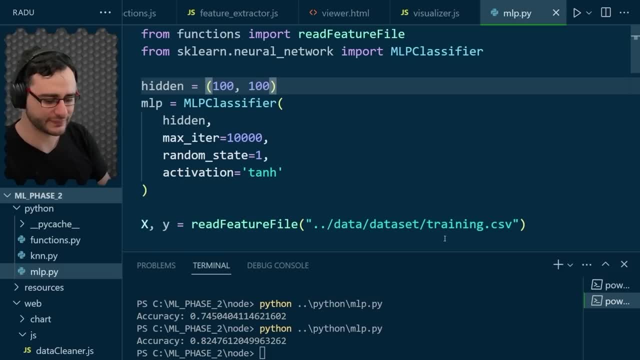 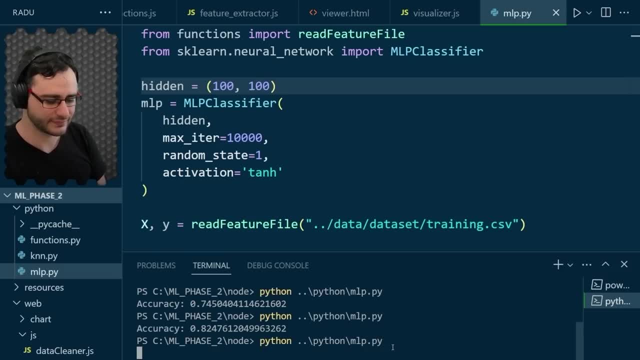 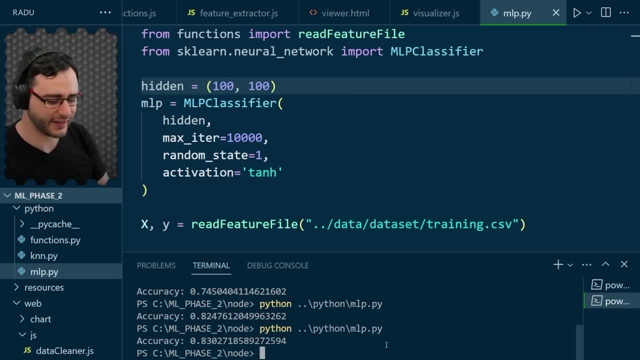 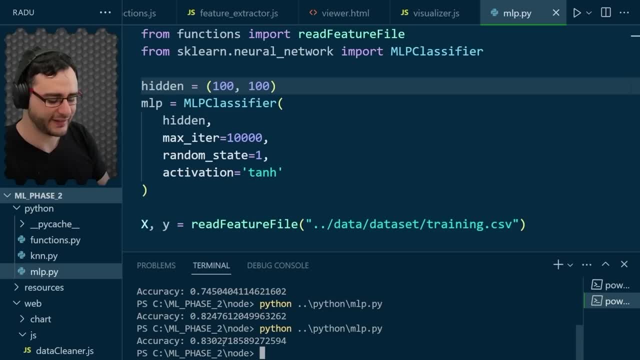 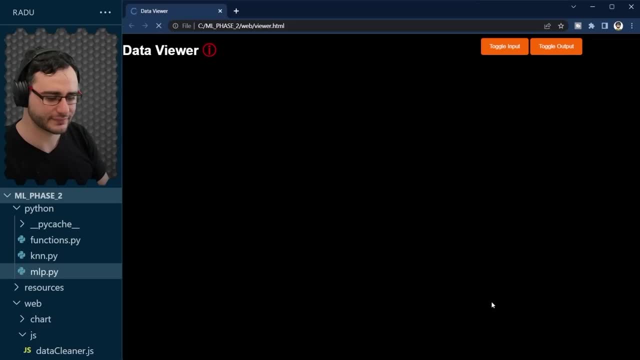 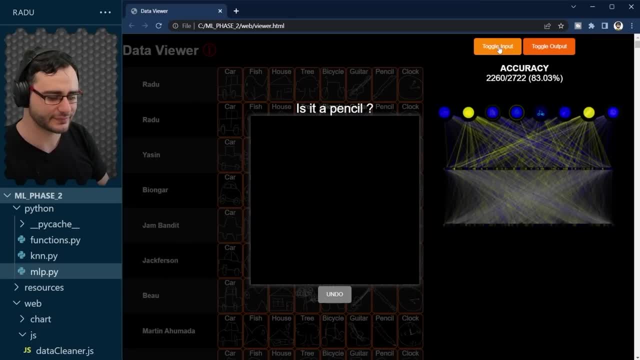 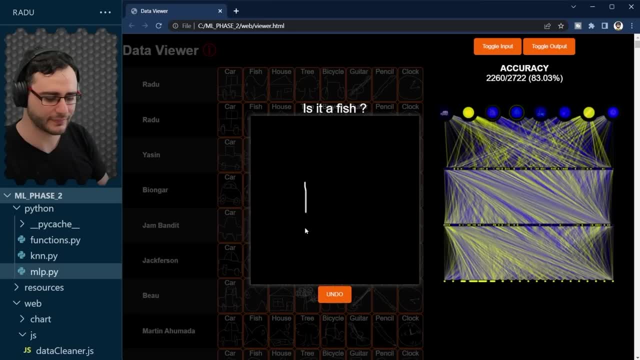 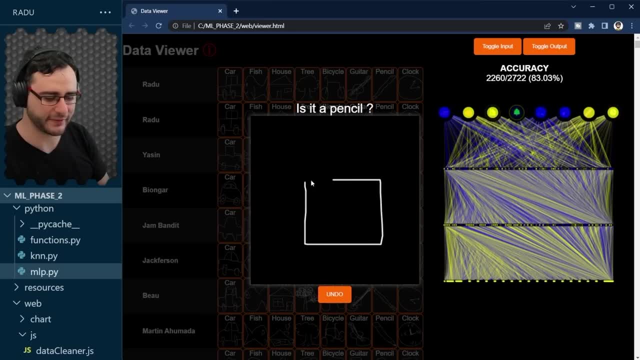 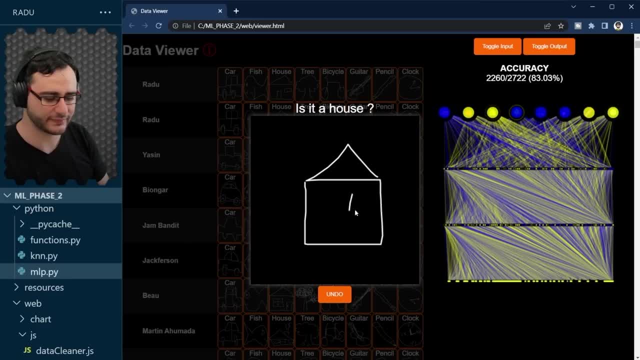 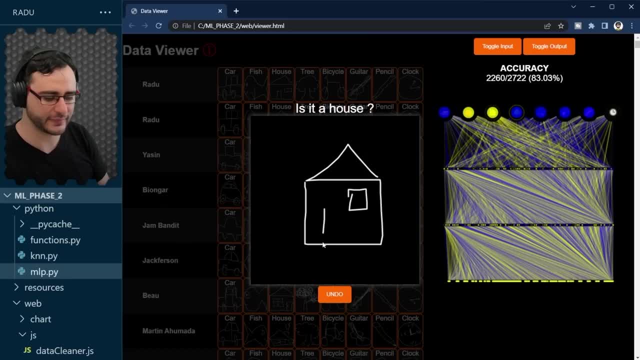 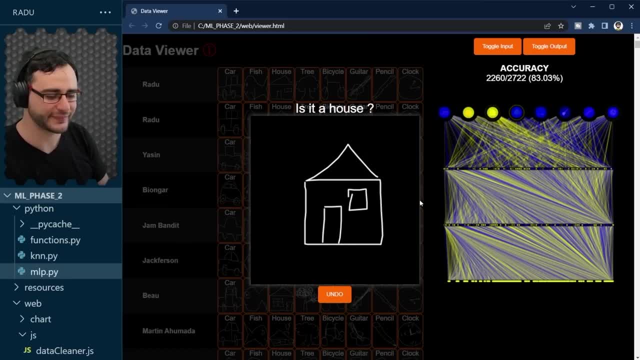 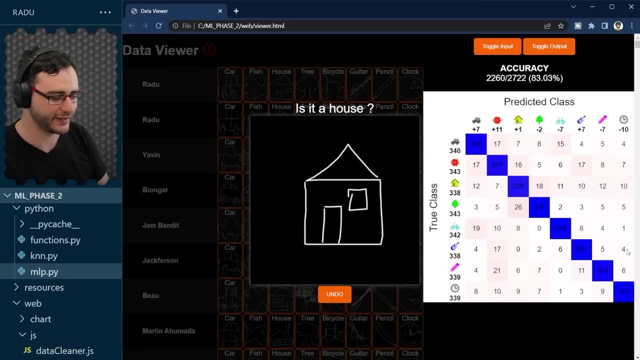 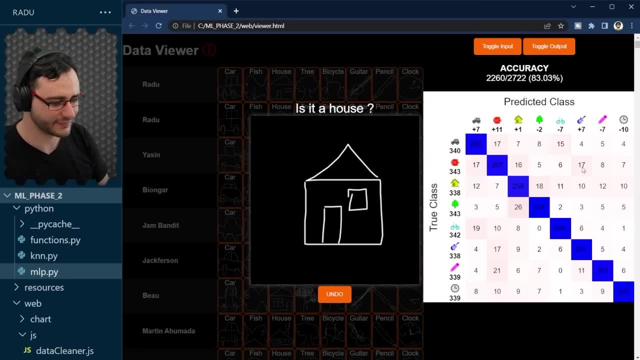 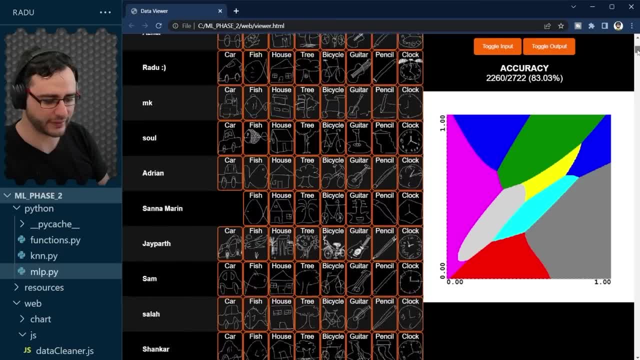 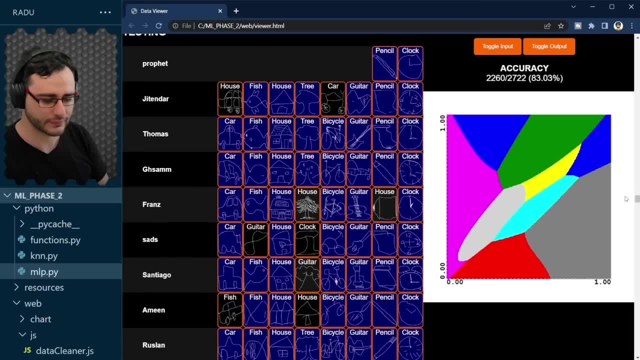 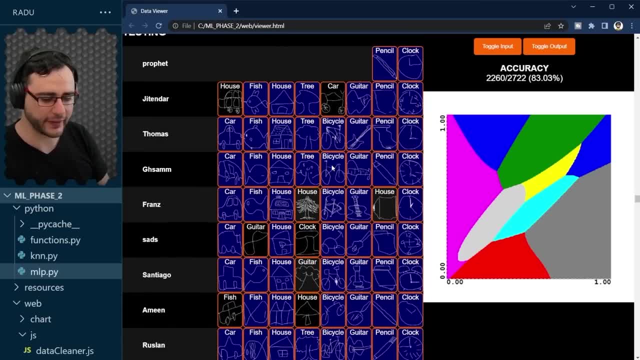 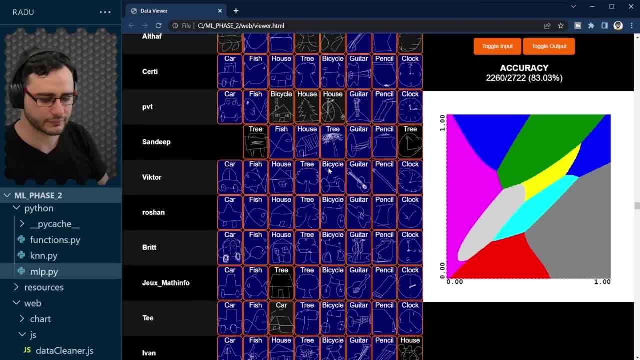 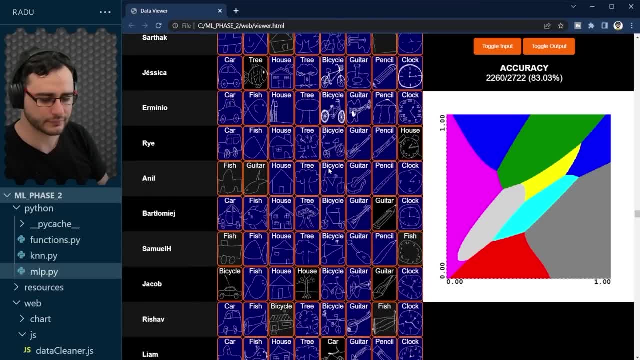 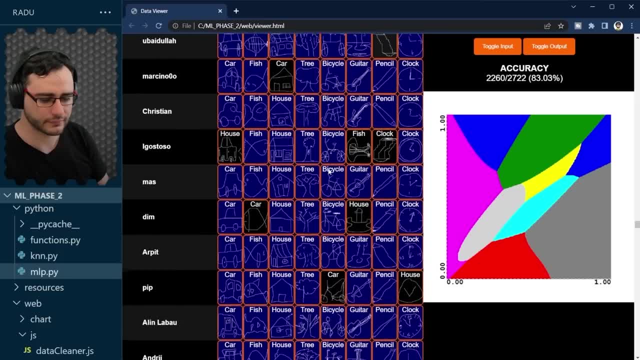 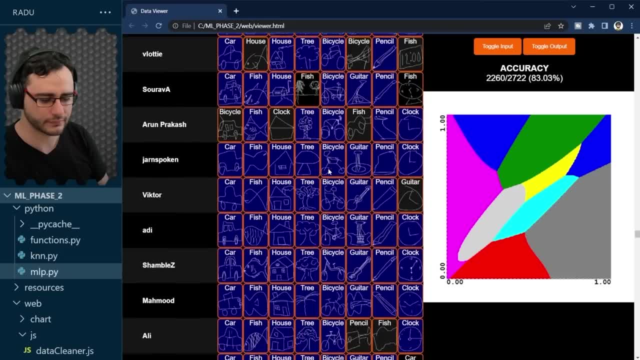 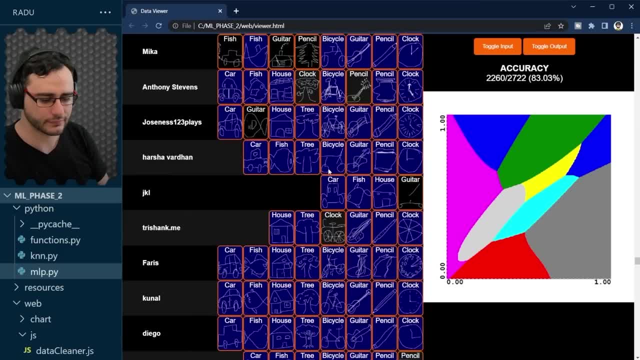 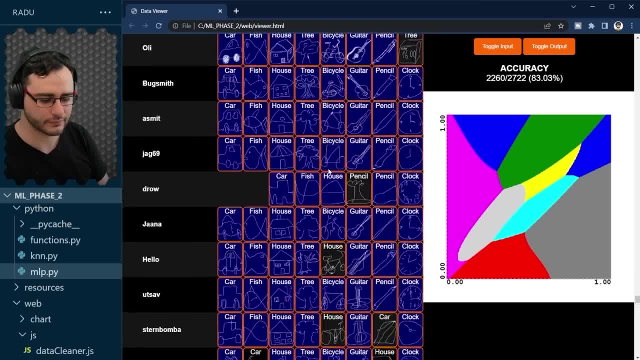 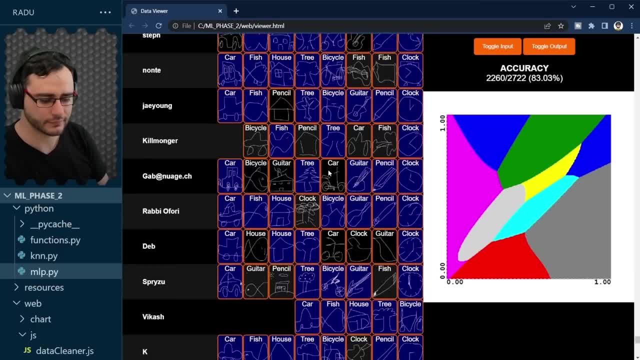 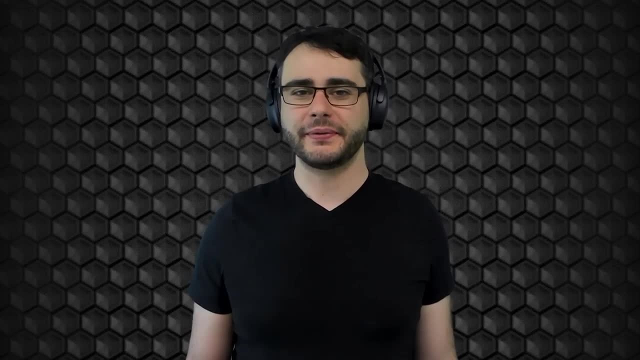 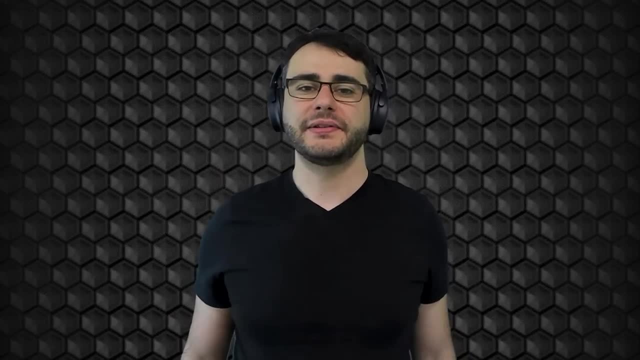 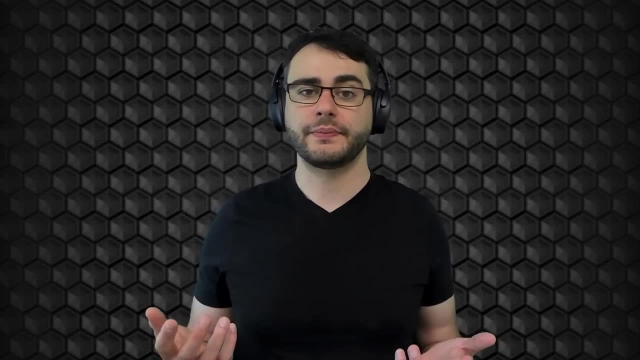 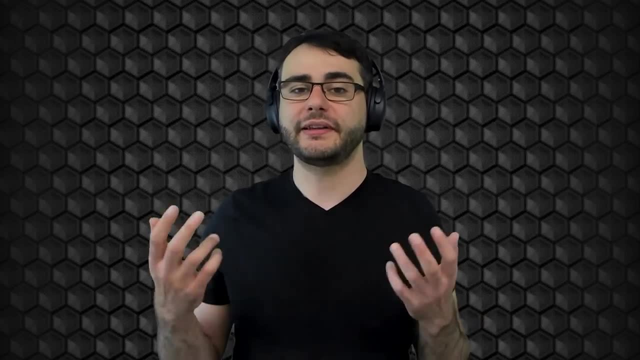 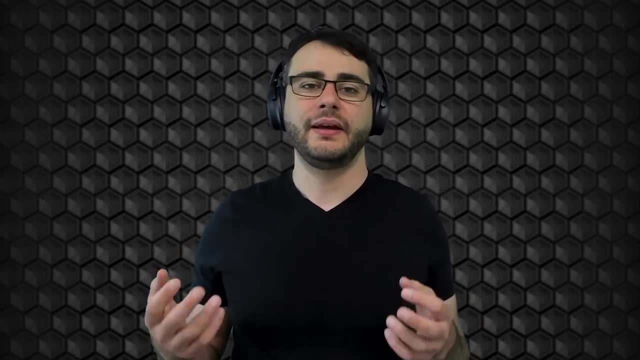 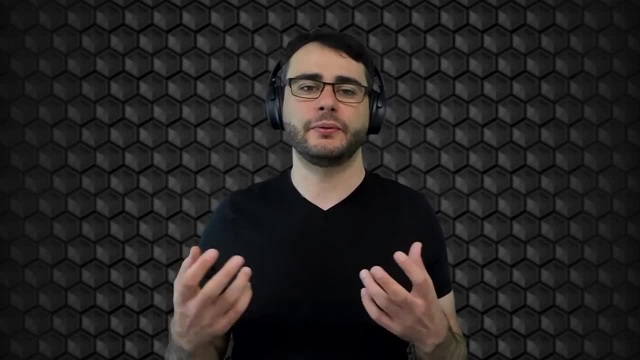 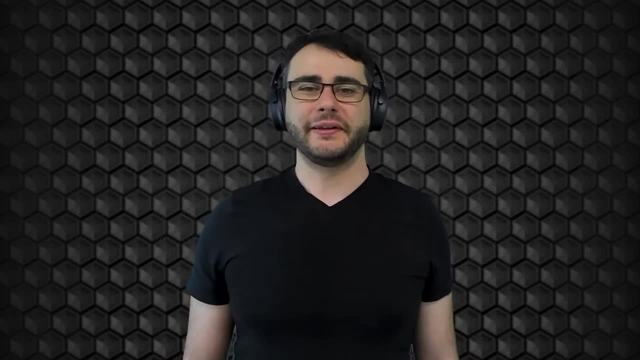 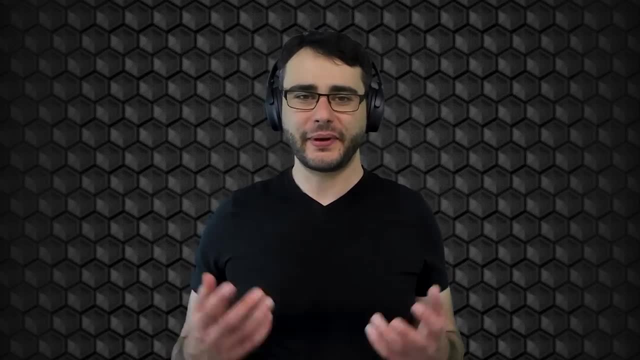 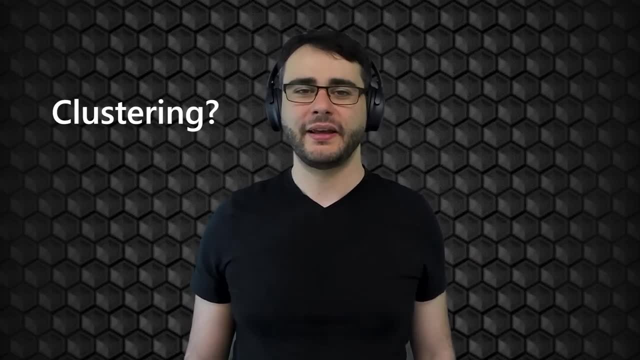 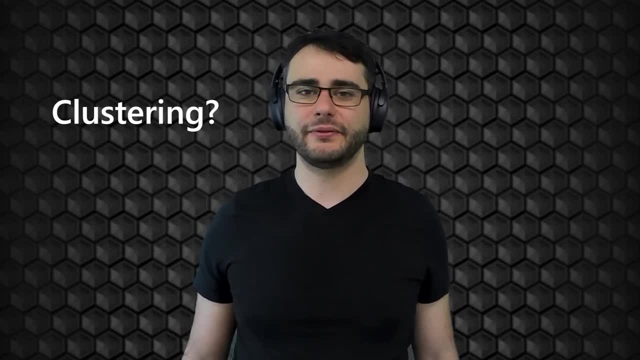 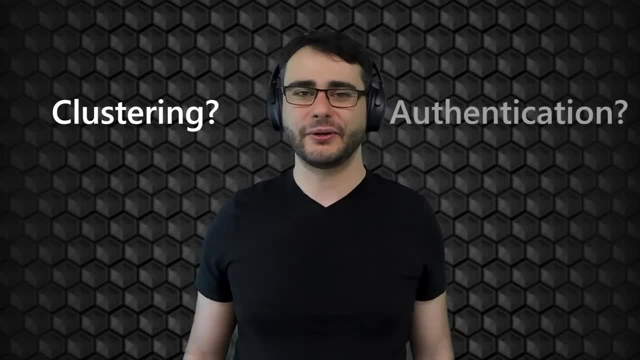 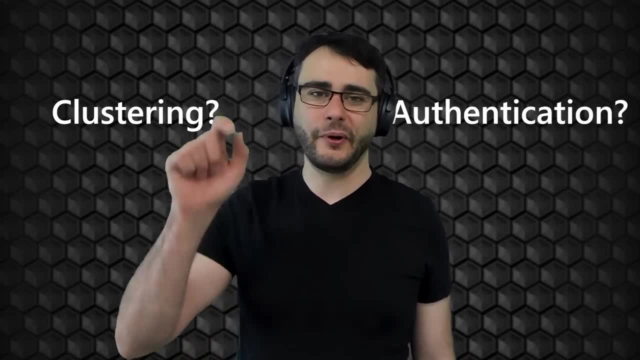 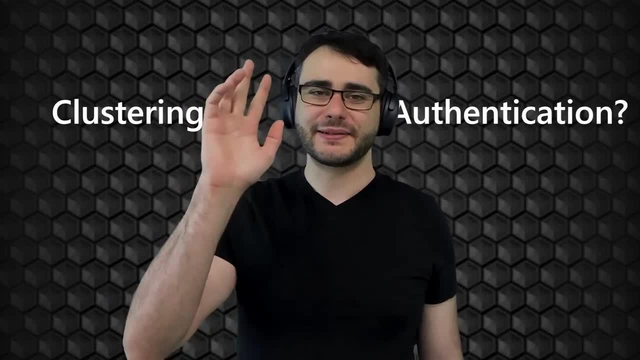 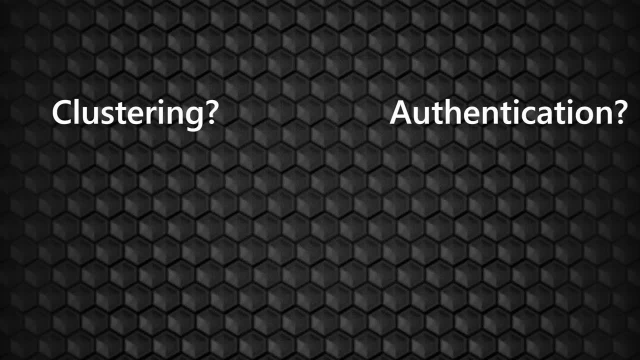